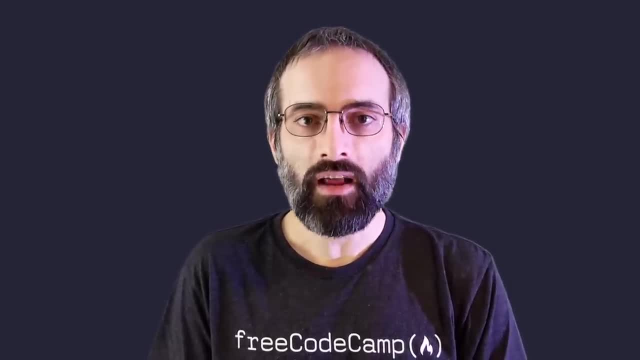 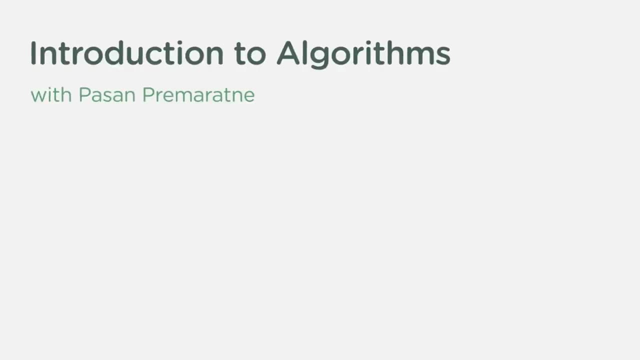 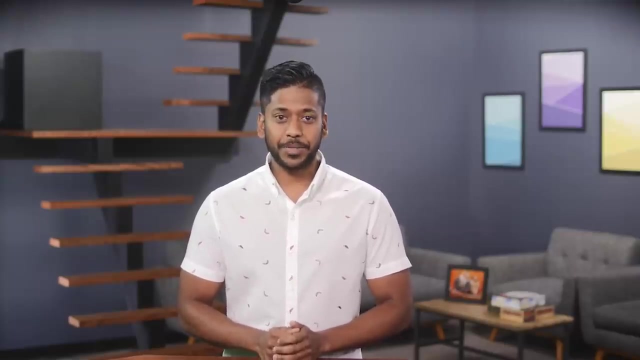 The link is in the description, along with time codes to the different sections in this course. Hi, my name is Pasan, I'm an instructor here at Treehouse and welcome to Introduction to Algorithms, Whether you are a high school or college student, a developer in the industry. 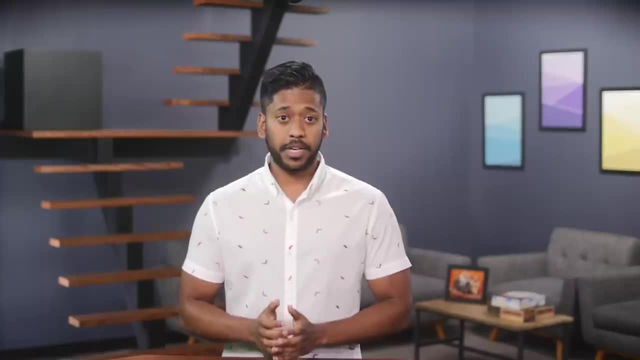 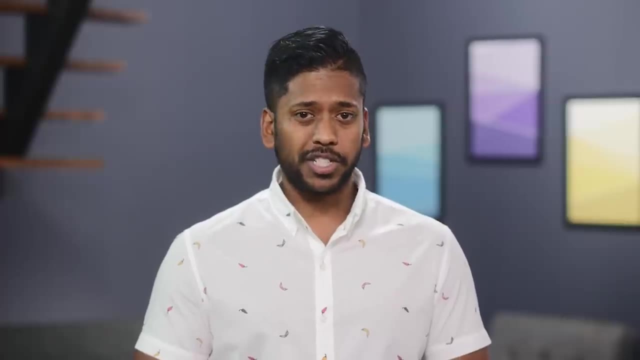 or someone who is learning to code. you have undoubtedly run into the term algorithm. For many people, this word is kind of scary. It represents this body of knowledge that you are learning to code. You have undoubtedly run into the term algorithm. For many people, this word is kind of scary. It represents this body of knowledge that 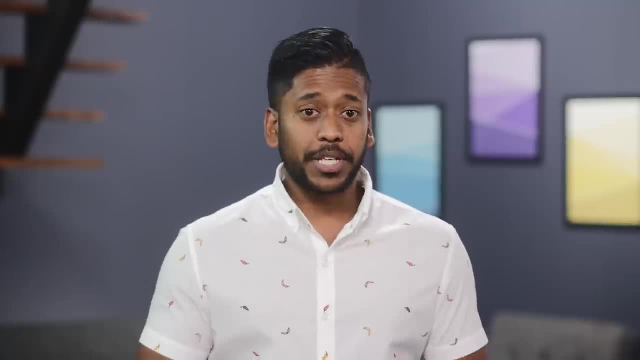 seems just out of reach. Only people with computer science degrees know about algorithms. To others this brings up feelings of imposter syndrome. You might already know how to code, but you're not a real developer because you don't know anything about algorithms. 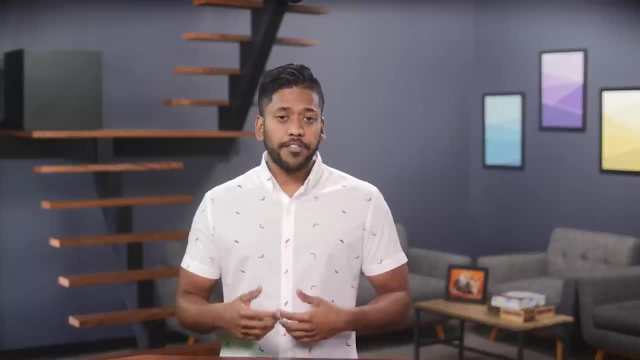 Personally, it made me frame certain jobs as above my skill level because the interview contained algorithm questions. Well, whatever your reasons are, in this course our goal is to dispel all those feelings and get you comfortable with the basics of algorithms, Like any other subject. I like to start my courses. 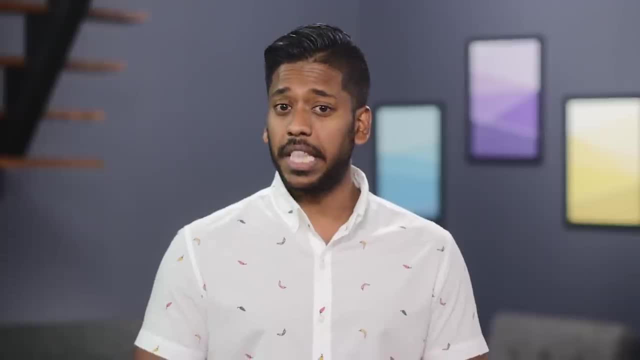 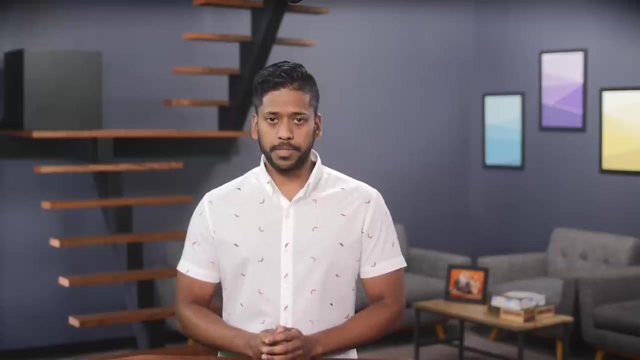 with what the course is and is not. In this course, we're going to cover the very basic set of knowledge that you need as a foundation for learning about algorithms. This course is less about specific algorithms and more about the tools you will need to evaluate algorithms. 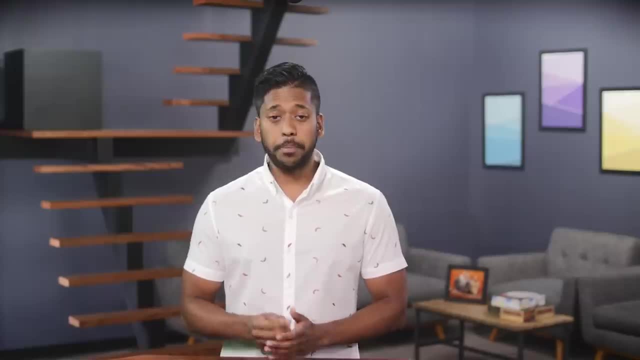 understand how they perform, compare them to each other and make a statement about the utility of an algorithm in a given context. Now, don't worry, none of this will be theoretical, and we will learn these concepts by using well-known algorithms. In this course, we will also be writing code, so I do. 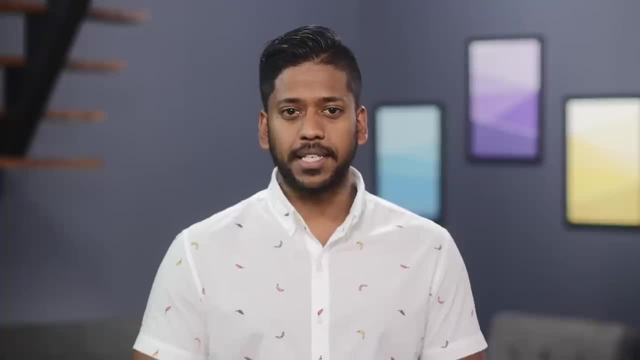 expect you to have some programming experience if you intend to continue with this topic. You can definitely stick around even if you don't know how to code, but you might want to learn the basics of programming in the meantime. In this course, we will be using the Python programming language. Python reads a lot like: 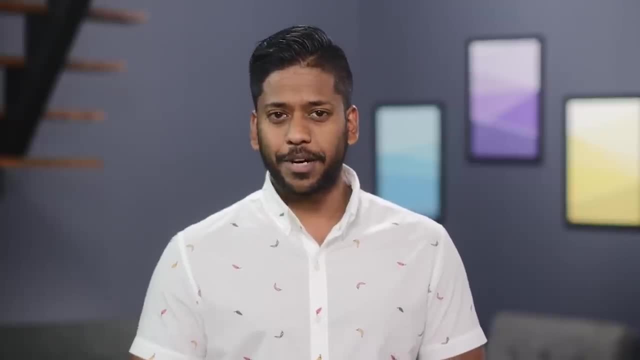 regular English And is the language you will most likely encounter when learning about algorithms these days. If you don't know how to code, or if you know how to code in a different language, check out the notes section of this video for links to other content that might be useful to you. 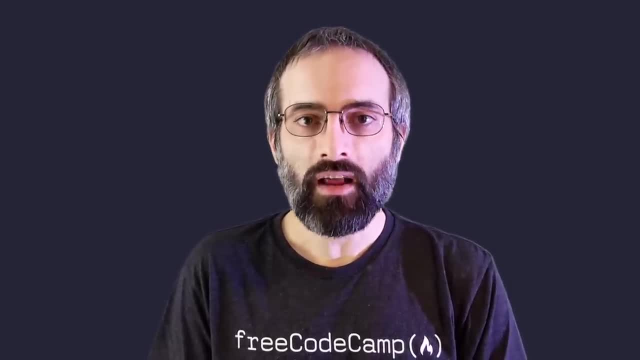 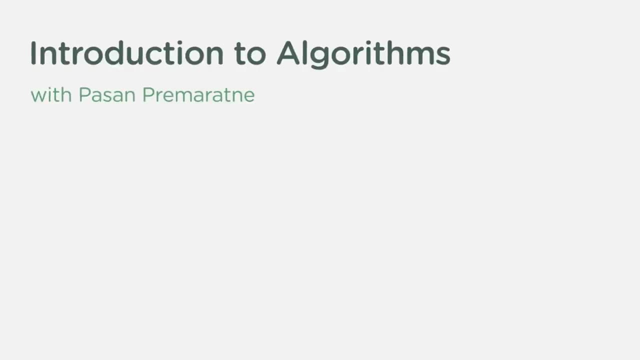 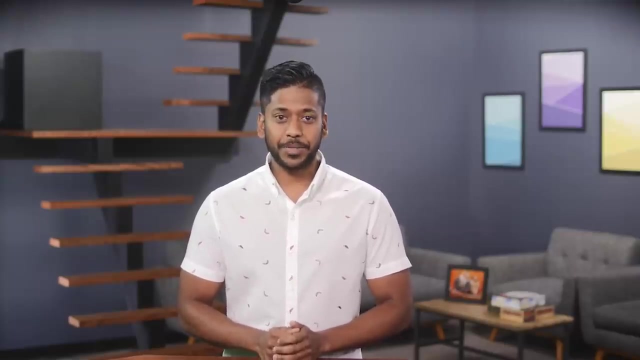 The link is in the description, along with time codes to the different sections in this course. Hi, my name is Pasan, I'm an instructor here at Treehouse and welcome to Introduction to Algorithms, Whether you are a high school or college student, a developer in the industry. 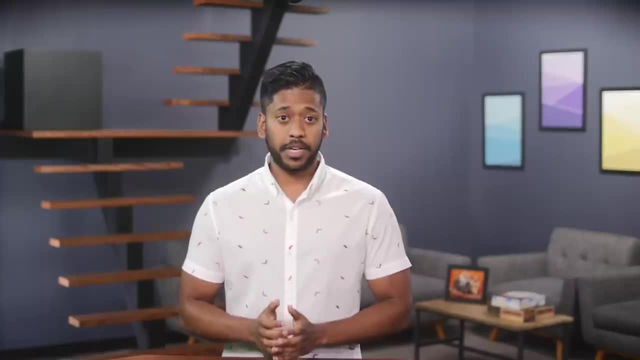 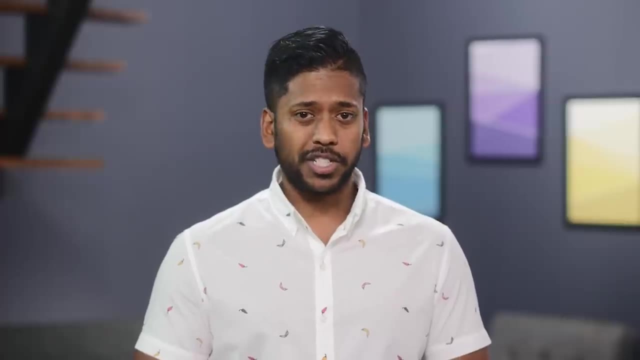 or someone who is learning to code. you have undoubtedly run into the term algorithm. For many people, this word is kind of scary. It represents this body of knowledge that you are learning to code. You have undoubtedly run into the term algorithm. For many people, this word is kind of scary. It represents this body of knowledge that 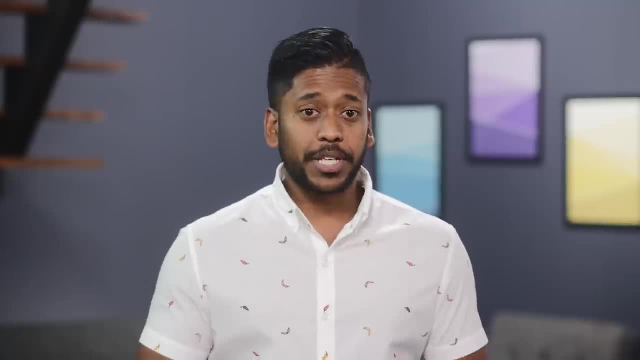 seems just out of reach. Only people with computer science degrees know about algorithms. To others this brings up feelings of imposter syndrome. You might already know how to code, but you're not a real developer because you don't know anything about algorithms. 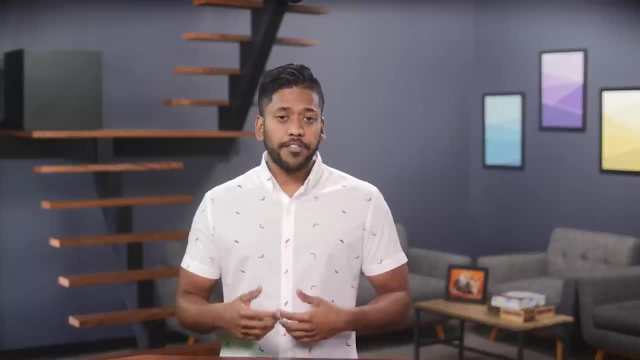 Personally, it made me frame certain jobs as above my skill level because the interview contained algorithm questions. Well, whatever your reasons are, in this course our goal is to dispel all those feelings and get you comfortable with the basics of algorithms, Like any other subject. I like to start my courses. 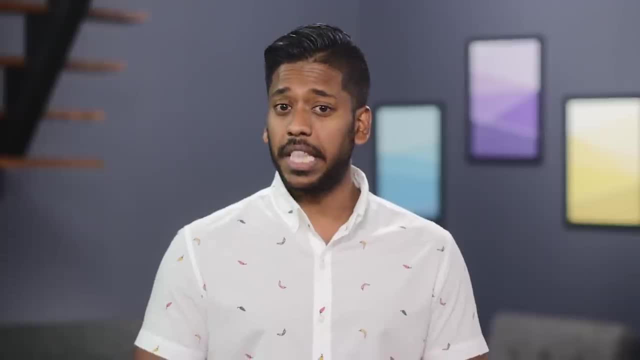 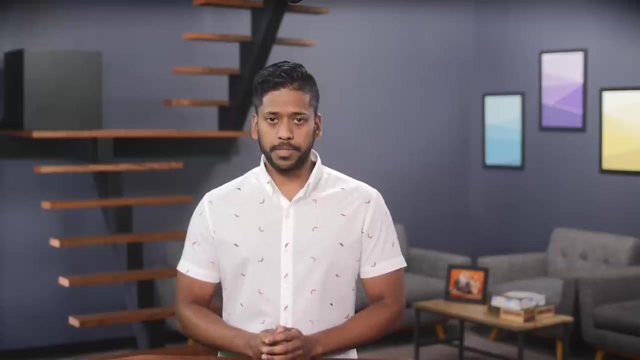 with what the course is and is not. In this course, we're going to cover the very basic set of knowledge that you need as a foundation for learning about algorithms. This course is less about specific algorithms and more about the tools you will need to evaluate algorithms. 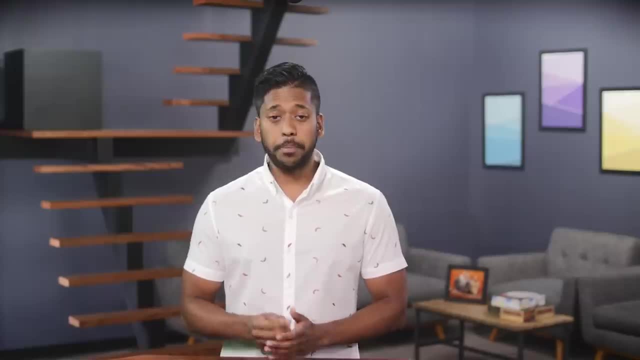 understand how they perform, compare them to each other and make a statement about the utility of an algorithm in a given context. Now, don't worry, none of this will be theoretical, and we will learn these concepts by using well-known algorithms. In this course, we will also be writing code, so I do. 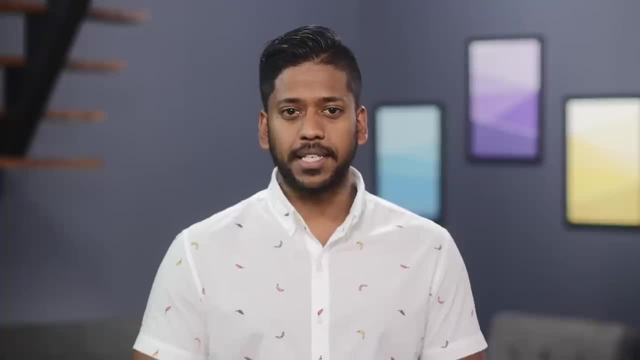 expect you to have some programming experience if you intend to continue with this topic. You can definitely stick around even if you don't know how to code, but you might want to learn the basics of programming in the meantime. In this course, we will be using the Python programming language. Python reads a lot like: 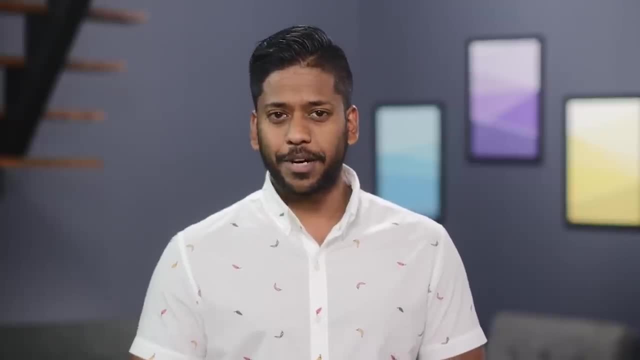 regular English And is the language you will most likely encounter when learning about algorithms these days. If you don't know how to code, or if you know how to code in a different language, check out the notes section of this video for links to other content that might be useful to you. 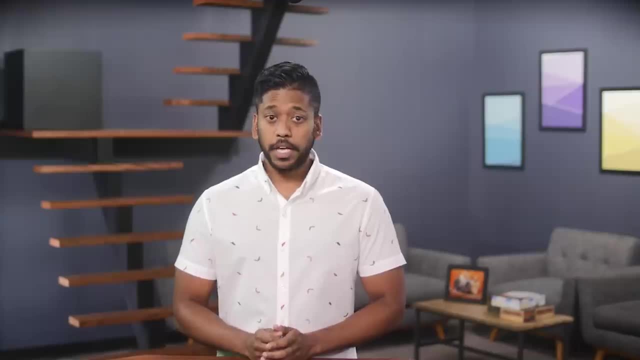 As long as you understand the fundamentals of programming, you should be able to follow along pretty well. If you're a JavaScript developer or a student who's learning JavaScript, for example, chances are good that you'll still be able to understand the code we write. 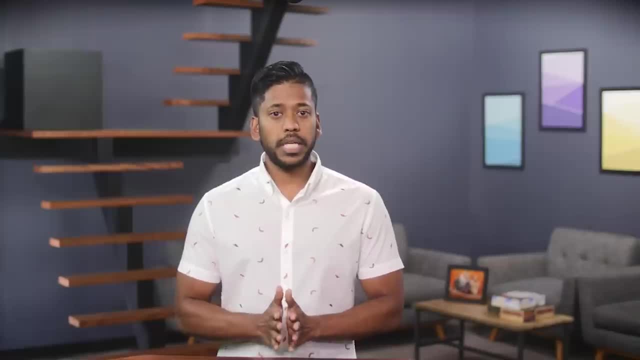 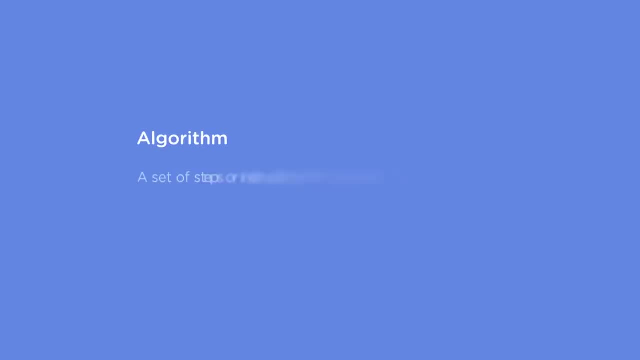 I'll be sure to provide links along the way if you need anything to follow up on. Let's start with something simple. What is an algorithm? An algorithm is a set of steps or instructions for completing a task. This might sound like an oversimplification, but really that's precisely what an algorithm is. 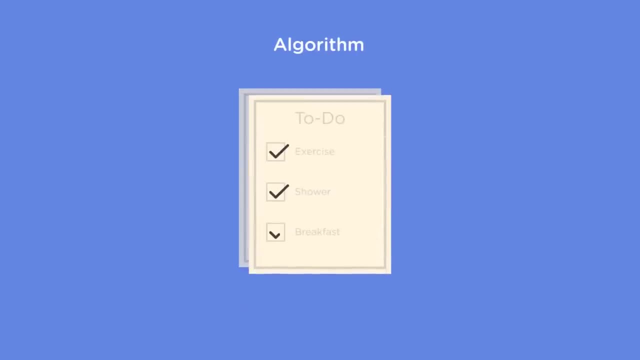 A recipe is an algorithm, your morning routine when you wake up is an algorithm and the driving directions you follow to get to a destination is also an algorithm. In computer science, the term algorithm more specifically means the set of steps a program takes to finishing a task. If you've written code before, any code really. 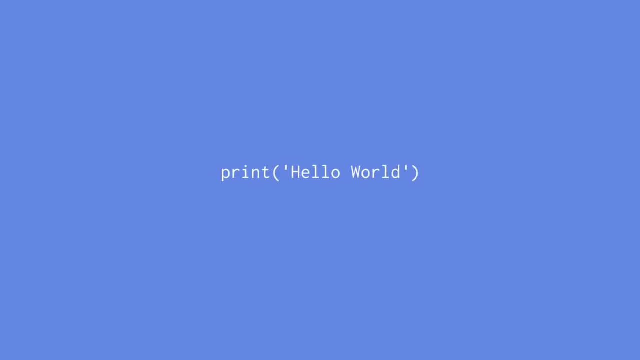 generally speaking, you have written an algorithm. Given that much of the code we write can be considered an algorithm, what do people mean when they say you should know about algorithms? Consider this. Let's say I'm a teacher in a classroom and I tell everyone I have an. 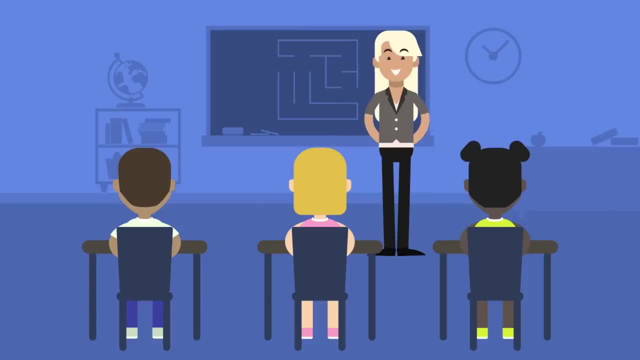 assignment for them. What do these algorithms actually mean On their desks? on their desks, They have a picture of a maze and their task is to come up with a way to find the quickest way out of the maze. Everyone does their thing and comes up with a solution. 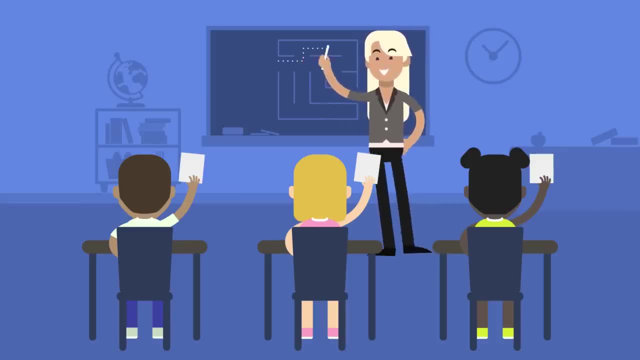 Every single one of these solutions is a viable solution and is a valid example of an algorithm, The steps one needs to take to get out of the maze. But from being in classrooms or any group of any sort, you know that some people will have better ideas than others. 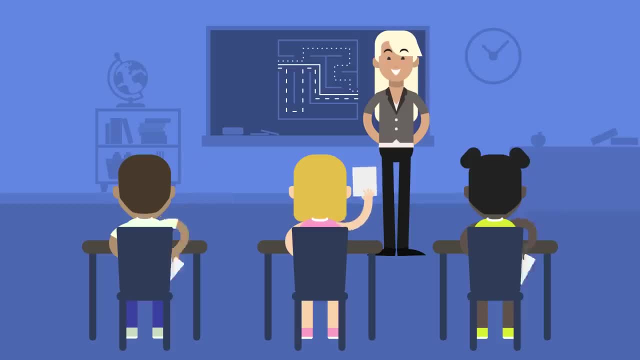 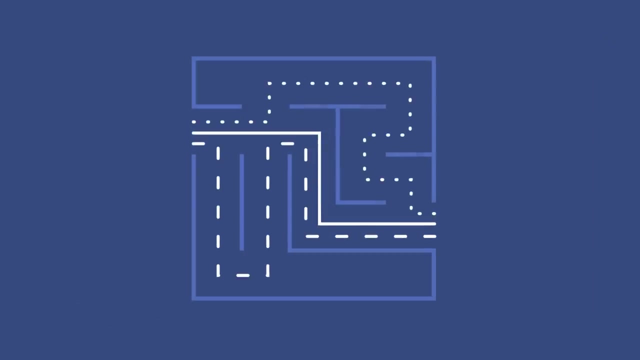 We all have a diverse array of skill sets. Over time, our class picks the best of these solutions and any time we want to solve a maze, we go with one of these solutions. This is what the field of algorithms is about. There are many problems in computer science, but some of them are pretty common, regardless of what project you're working on. 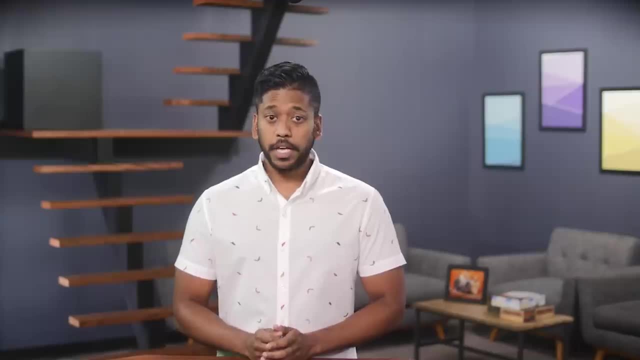 As long as you understand the fundamentals of programming, you should be able to follow along pretty well. If you're a JavaScript developer or a student who's learning JavaScript, for example, chances are good that you'll still be able to understand the code we write. 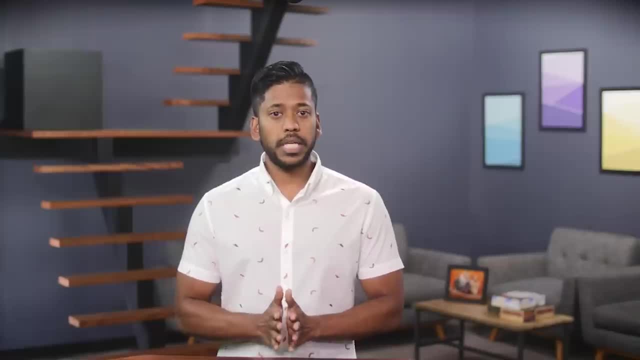 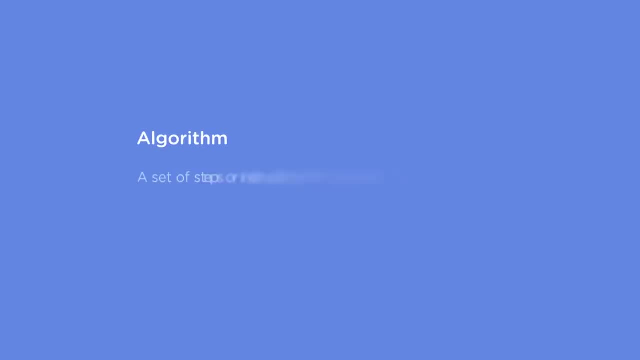 I'll be sure to provide links along the way if you need anything to follow up on. Let's start with something simple. What is an algorithm? An algorithm is a set of steps or instructions for completing a task. This might sound like an oversimplification, but really that's precisely what an algorithm is. 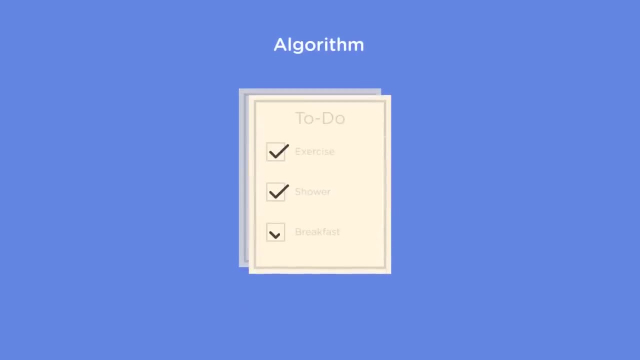 A recipe is an algorithm, your morning routine when you wake up is an algorithm and the driving directions you follow to get to a destination is also an algorithm. In computer science, the term algorithm more specifically means the set of steps a program takes to finish a task. If you've written code before, any code really. 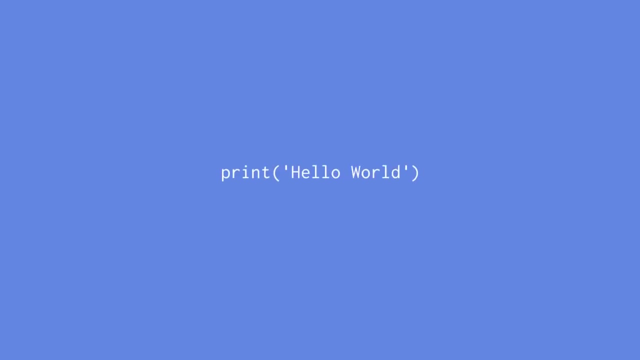 generally speaking, you have written an algorithm. Given that much of the code we write can be considered an algorithm, what do people mean when they say you should know about algorithms? Consider this. Let's say I'm a teacher in a classroom and I tell everyone I have 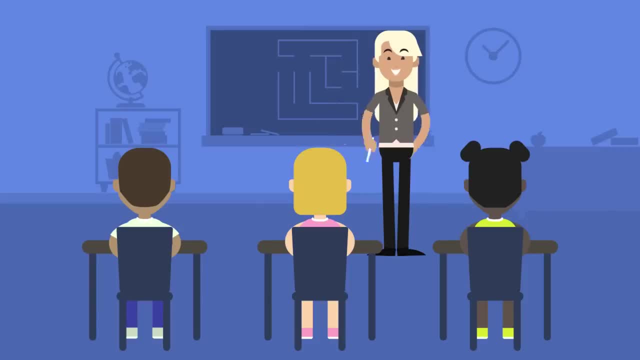 an assignment for them. Now, all I have to do to translate this is write an assignment for them. Then, when they're done, they'll need to figure out the correct word, And then I'll tell everyone. On their desks they have a picture of a maze. 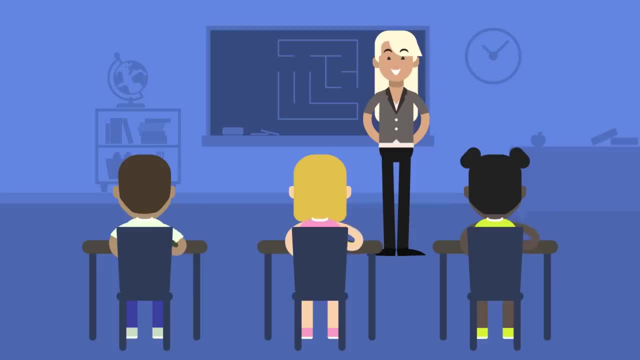 and their task is to come up with a way to find the quickest way out of the maze. Now everyone does their thing and comes up with a solution. Every single one of these solutions is a viable solution and is a valid example of an algorithm. 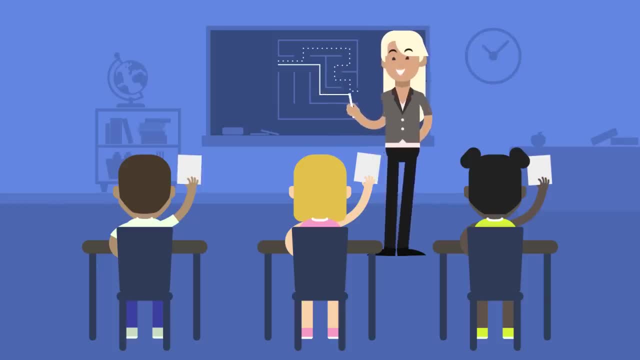 the steps one needs to take to get out of the maze. But from being in classrooms or any group of any sort, you know that some people will have better ideas than others. We all have a diverse array of skill sets. Over time our class picks the best of these solutions. 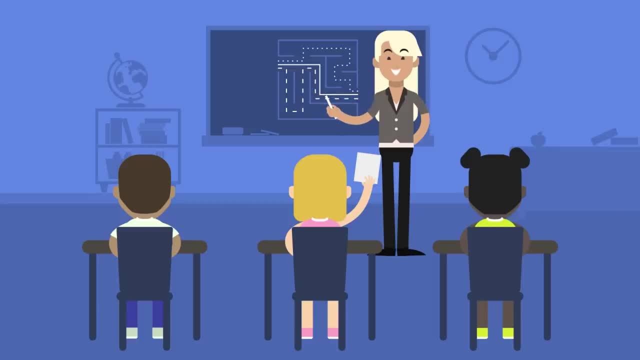 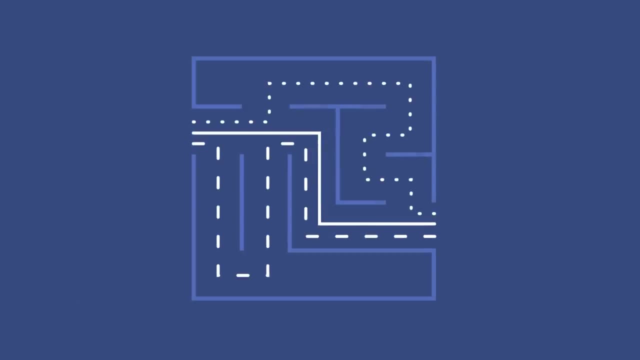 and any time we want to solve a maze, we go with one of these solutions. This is what the field of algorithms is about. There are many problems in computer science, but some of them are pretty common, regardless of what project you're working on. 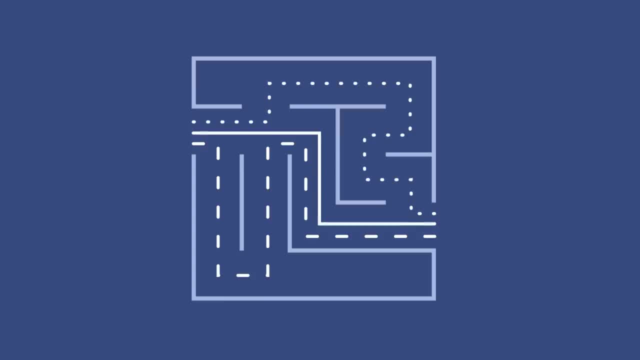 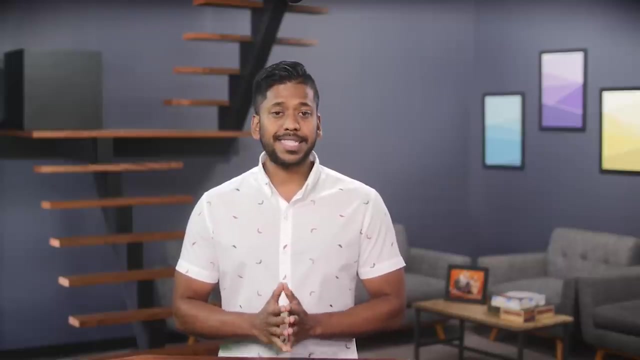 Different people have come up with different solutions to these common problems and over time the field of computer science has identified several that do the job well for a given task. When we talk of algorithms, we're referring to two points. We're primarily saying there's an established body of knowledge on how to solve particular problems well. 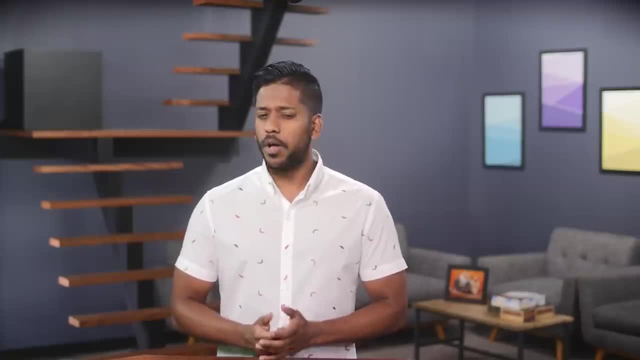 and it's important to know what these solutions are. Now, why is it important? If you're unaware that a solution exists, you might try to come up with one yourself, and there's a likelihood that your solution won't be as good or efficient, whatever that means. 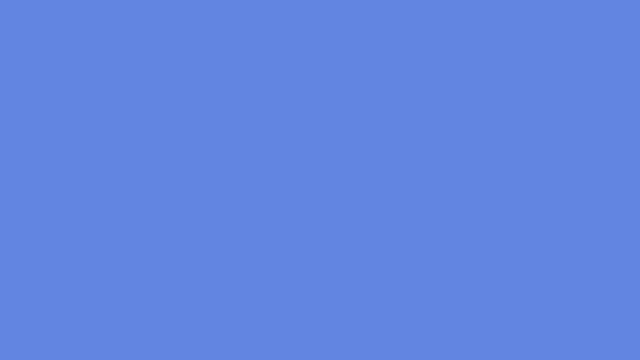 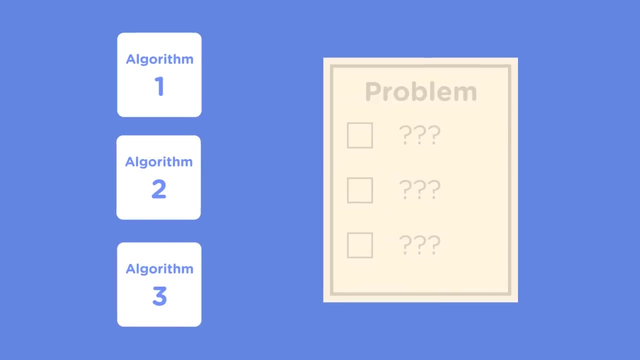 compared to those that have been thoroughly reviewed. But this isn't all. There's a second component to it as well. Part of understanding algorithms is not just knowing that an algorithm exists, but understanding when to apply it. Understanding when to apply an algorithm requires properly understanding the problem at hand. 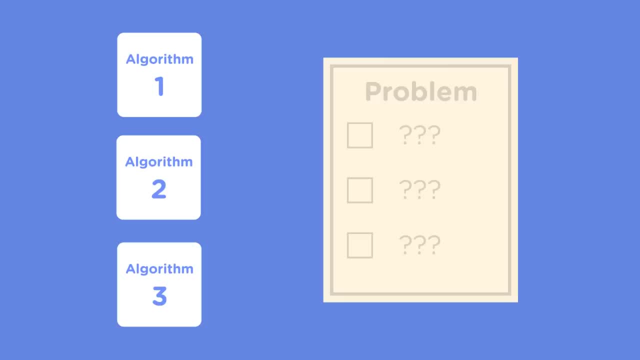 and this, arguably, is the most important part of learning about algorithms and data structures. As you progress through this content, you should be able to look at a problem and break it down into distinct steps. When you have a set of steps, you should then be able to identify which algorithm or data structure is best for the task at hand. 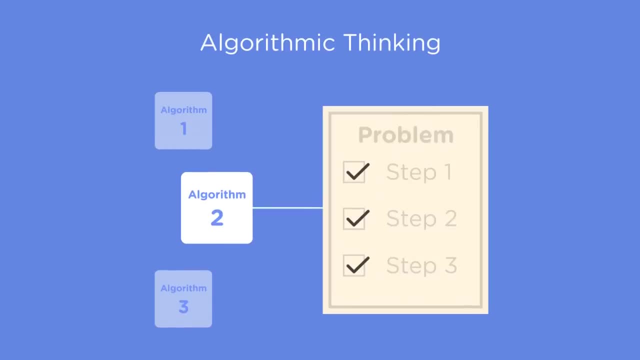 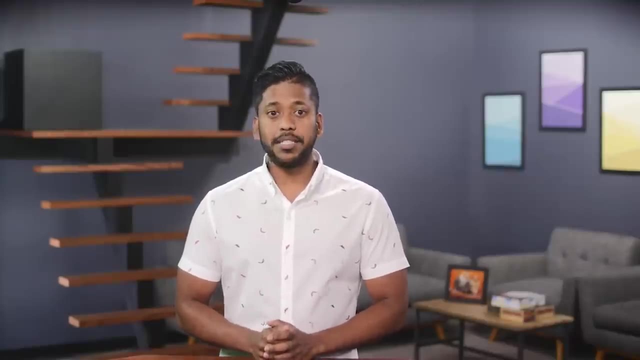 This concept is called algorithmic thinking, and it's something we're going to try and cultivate together as we work through our content. Lastly, learning about algorithms gives you a deeper understanding about complexity and efficiency in programming. Having a better sense of how your code will perform in different situations is something that you'll always want to develop and hone. 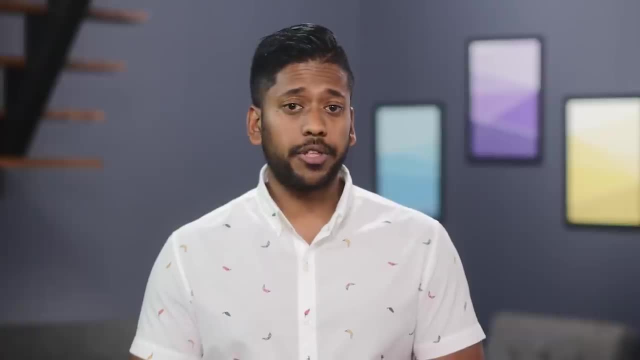 Algorithmic thinking is why algorithms also come up in big tech interviews. Interviewers don't care as much that you are able to write a specific algorithm in code, but more about the fact that you can break a seemingly insurmountable problem into distinct components. 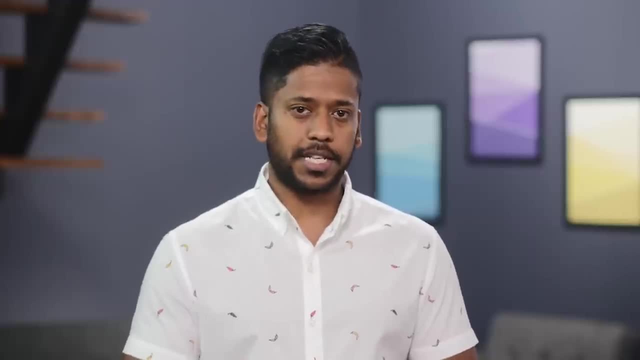 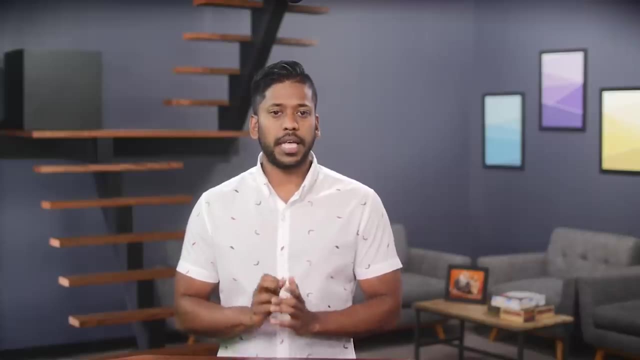 and identify the right tools to solve each distinct component, And that is what we plan on doing In this course, though, we're going to focus on some of the tools and concepts you'll need to be aware of before we can dive into the topic of algorithms. 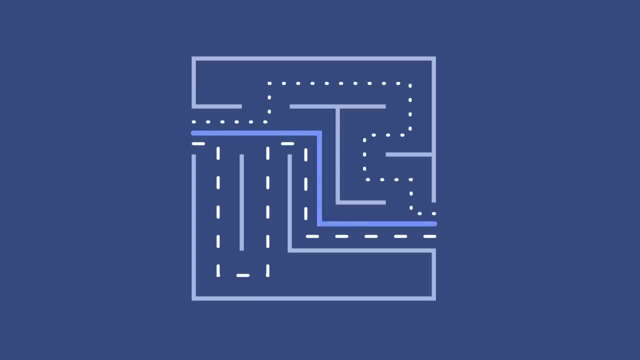 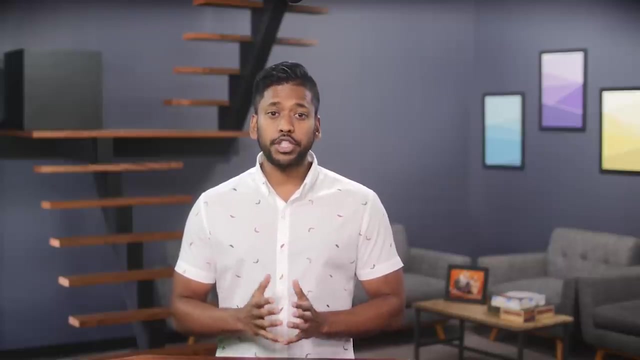 Different people have come up with different solutions to these common problems and over time the field of computer science has identified several that do the job well for a given task. When we talk of algorithms, we're referring to two points. We're primarily saying there's an established body of knowledge. 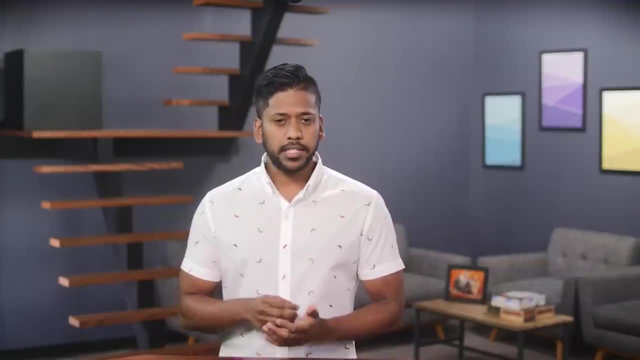 on how to solve particular problems well, and it's important to know what these solutions are. Now, why is it important? If you're unaware that a solution exists, you might try to come up with one yourself, and there's a likelihood that your solution 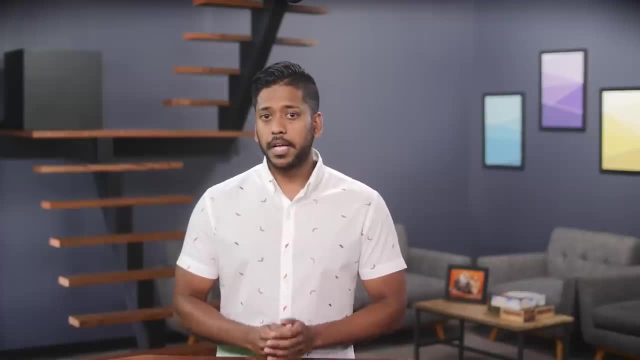 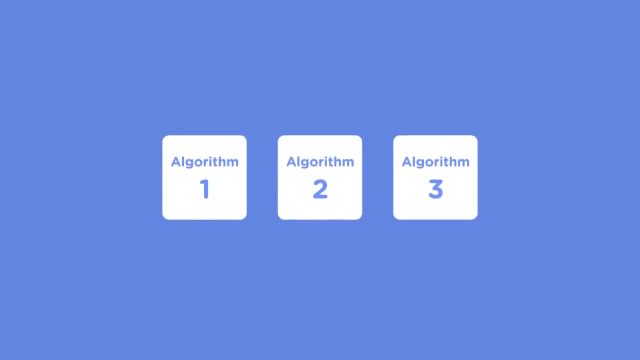 won't be as good or efficient, whatever that means, compared to those that have been thoroughly reviewed. But there's a possibility that your solution won't be as good or efficient, and there's a second component to it as well, Part of understanding algorithms. 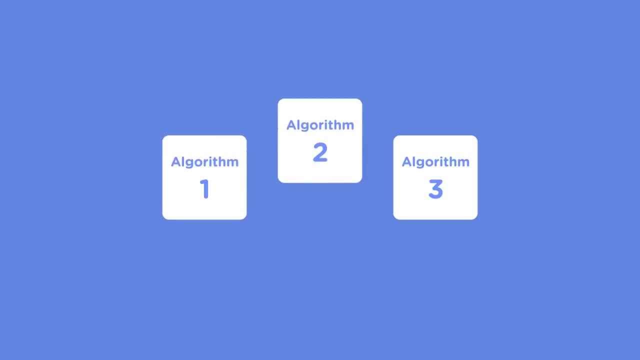 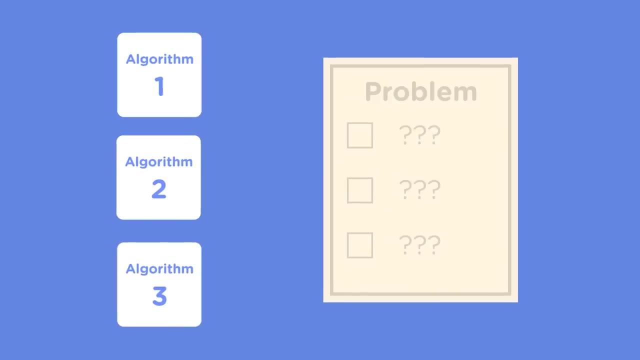 is not just knowing that an algorithm exists, but understanding when to apply it. Understanding when to apply an algorithm requires properly understanding the problem at hand, and this, arguably, is the most important part of learning about algorithms and data structures As you progress through this content. 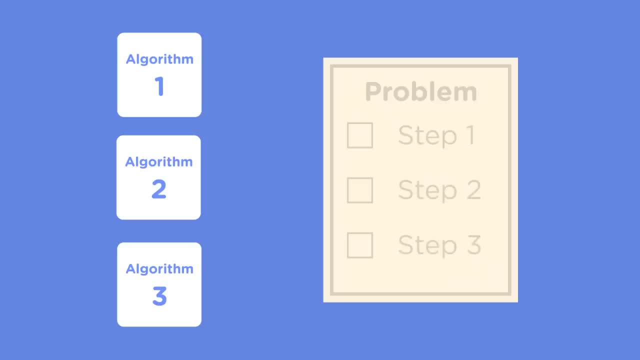 you should be able to look at a problem and break it down into distinct steps. When you have a set of steps, you should then be able to identify which algorithm or data structure is best for the task at hand. This concept is called algorithmic thinking. 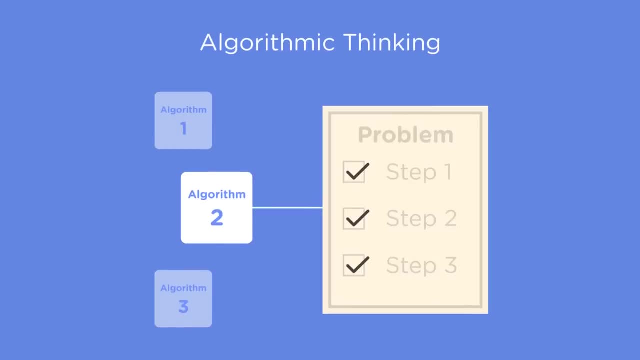 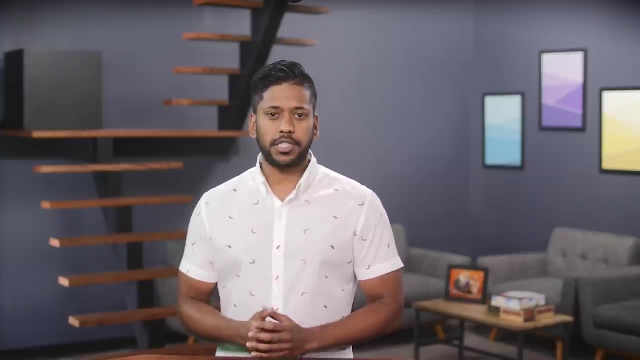 and it's something we're going to try and cultivate together as we work through our content. Lastly, learning about algorithms gives you a deeper understanding about complexity and efficiency in programming. Having a better sense of how your code will perform in different situations is something that you'll always want to develop and hone. 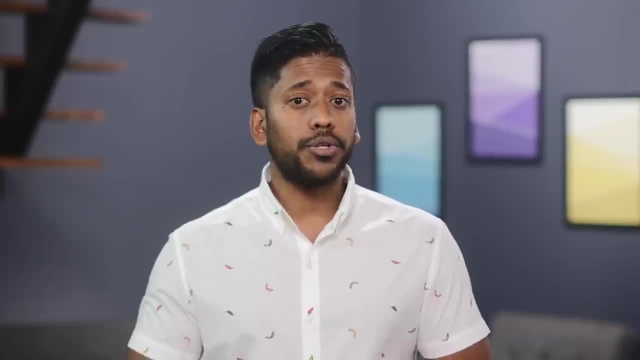 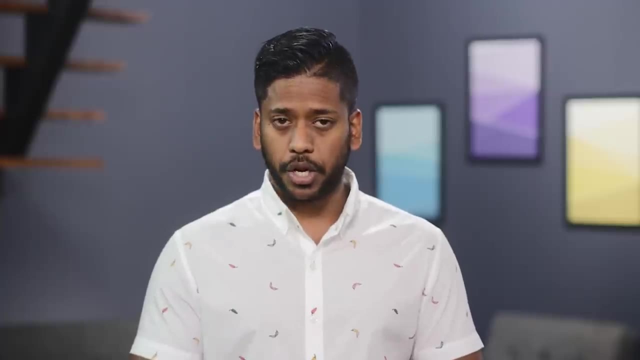 Algorithmic thinking is why algorithms also come up in big tech interviews. Interviewers don't care as much that you are able to write a specific algorithm in code, but more about the fact that you can break a seemingly insurmountable problem into distinct components. 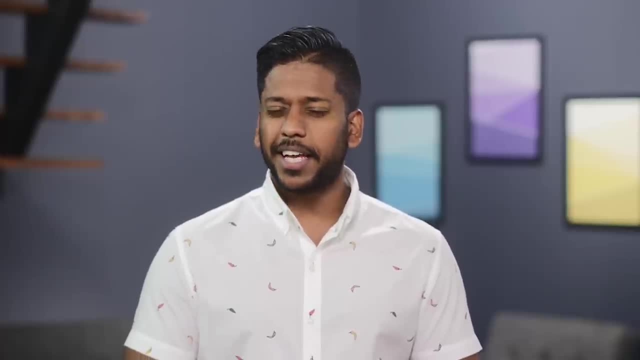 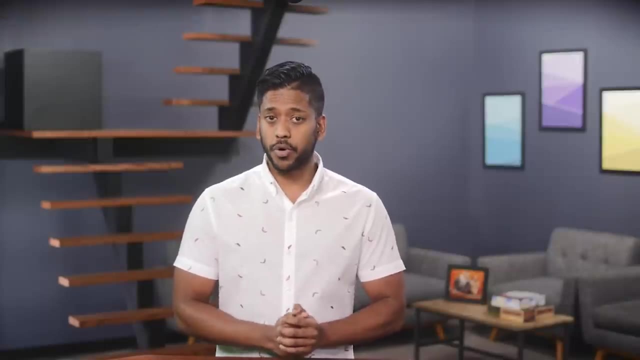 and identify the right tools to solve each distinct component, And that is what we plan on doing In this course, though, we're going to focus on some of the tools and concepts you'll need to be aware of before you start to think about. 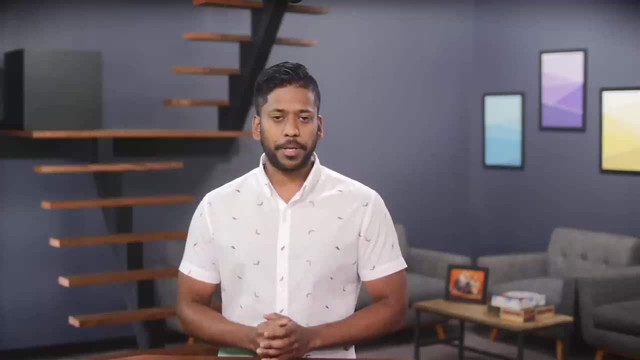 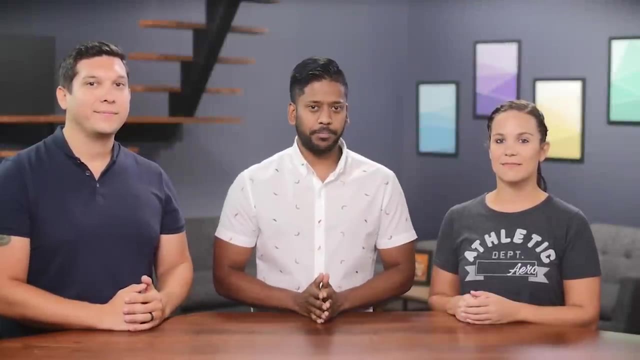 how you're going to solve a problem Before we can dive into the topic of algorithms. If you're ready, let's get started. Hey, again In this video we're going to do something unusual. We're going to play a game. 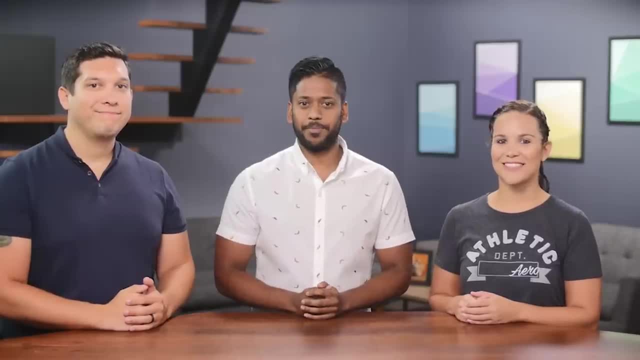 And by we I mean me and my two friends here, Brittany and John. This game is really simple, and you may have played it before. It goes something like this. I'm going to think of a number between 1 and 10,. 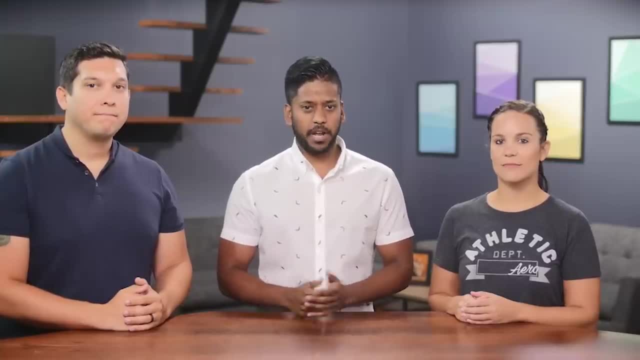 and they have to guess what. the number is. Easy, right. When they guess a number, I'll tell them if their guess is too high or too low. The winner is the one with the fewest points. All right, John, let's start with you. 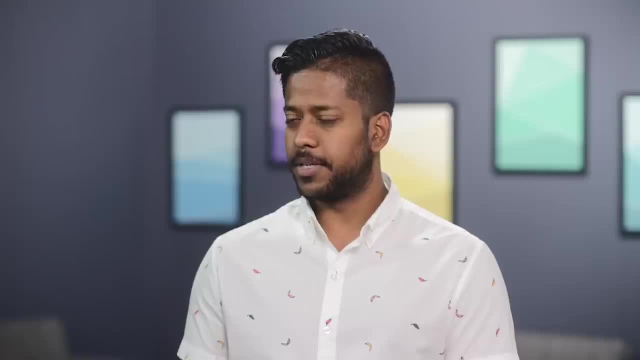 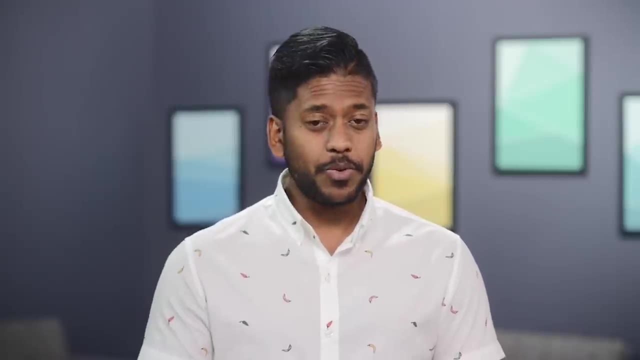 I'm thinking of a number between 1 and 10.. What is it Between you and me? the answer is 3.. Quick question: Does the range include 1 and 10?? That is a really good question. So what John did right there was to establish. 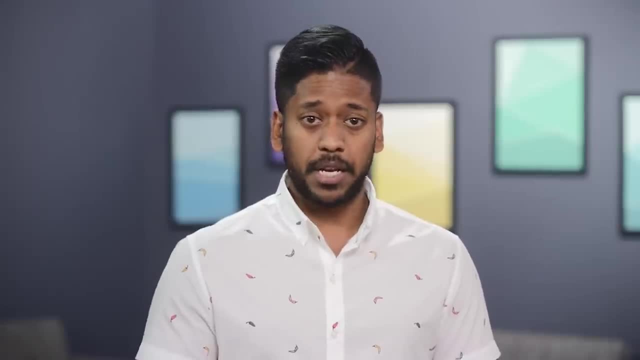 the bounds of our problem. No solution works on every problem And an important part of algorithmic thinking is to clearly define what the problem set is and clarify what values count as inputs. Yeah, 1 and 10 are both included. Is it 1 and 10?? 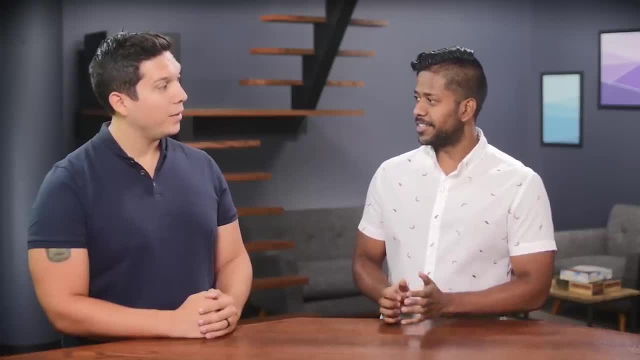 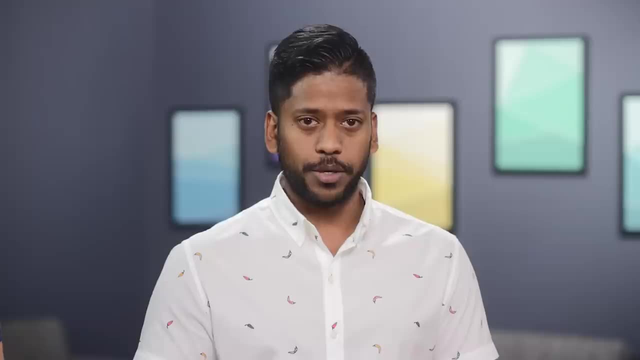 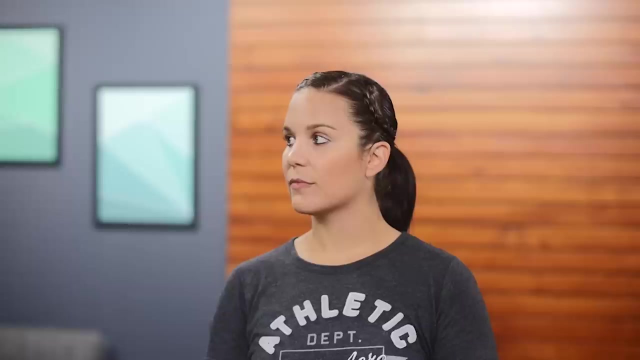 Too low, Is it 2?? Too low, Is it 3?? Correct, Okay, so that was an easy one. It took John three tries to get the answer. Let's switch over to Brittany and play another round using the same number as the answer. 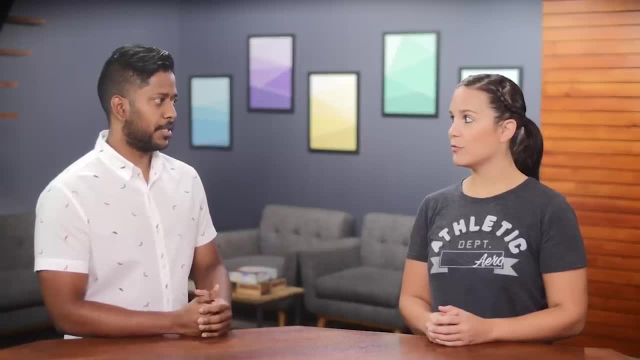 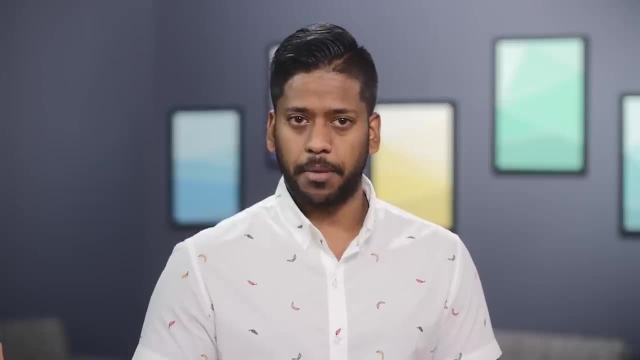 Okay, Brittany, I'm thinking of a number between 1 and 10 inclusive, so both 1 and 10 are in the range. What number am I thinking of? Is it 5? Too high, Even such a simple game. 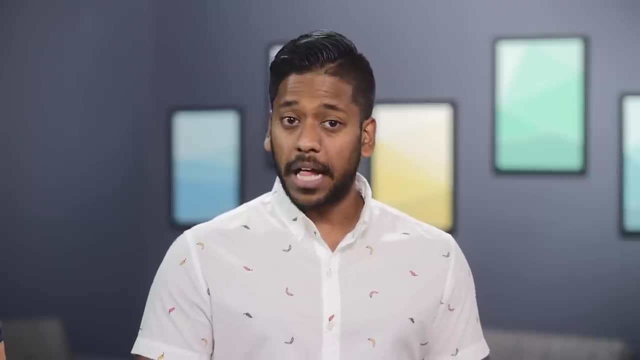 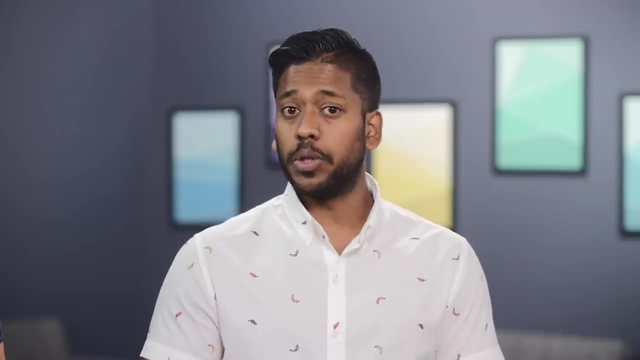 we saw different approaches to figuring out a solution. To go back to algorithmic thinking for a second, this means that with any given problem, there's no one best solution. Instead, what we should try and figure out is what solution works better for the current problem. 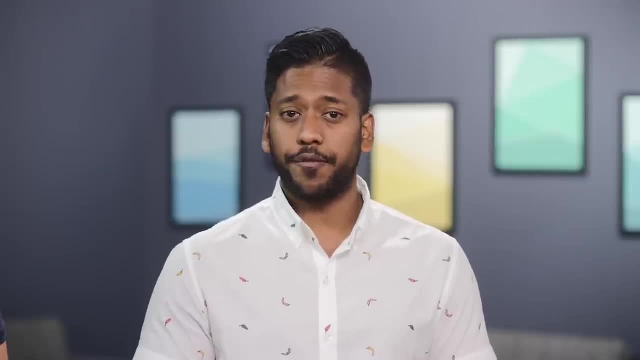 In this first pass at the game, they both took the same amount of turns to find the answer, So it's not obvious who has the better approach, And that's mostly because the game was easy. Let's try this one more time. This time the answer is 10.. 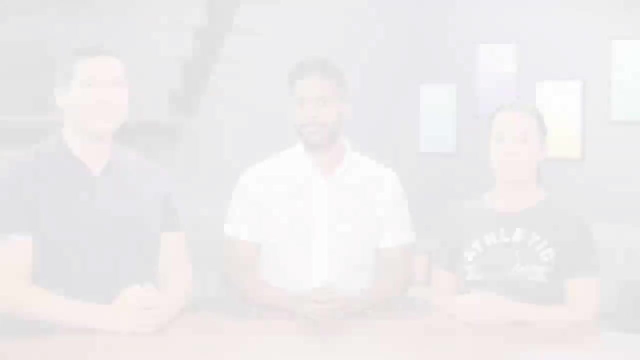 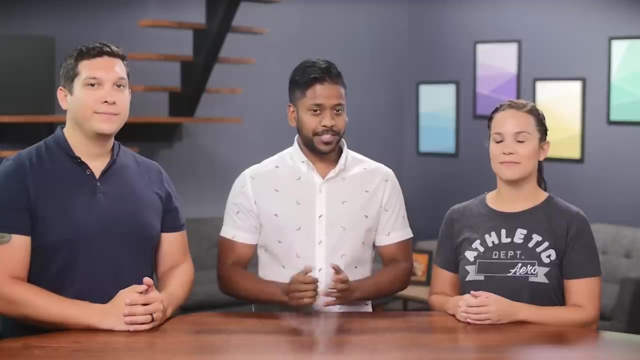 If you're ready, let's get started. Hey again, In this video, we're going to do something unusual. We're going to play a game, And by we I mean me and my two friends here, Brittany and John. This game is really simple and you may have played it before. 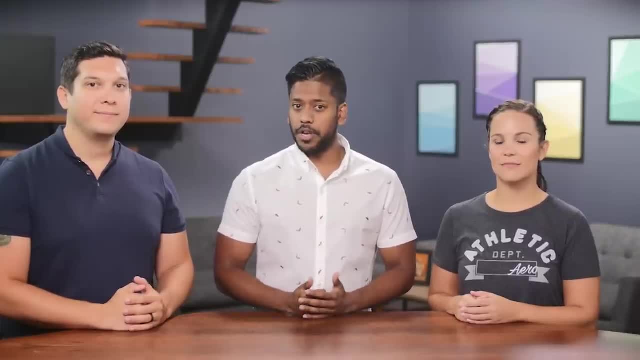 It goes something like this: I'm going to think of a number between 1 and 10, and they have to guess what the number is. Easy, right, When they guess a number, I'll tell them if their guess is too high or too low. 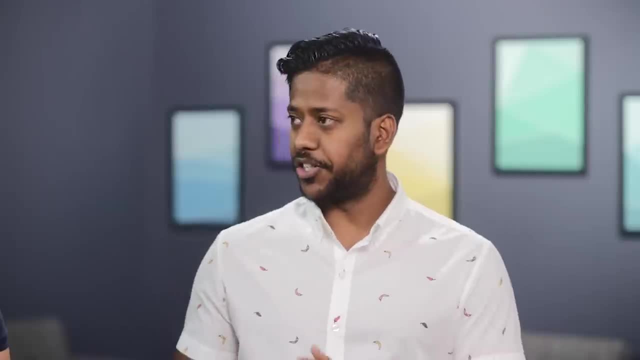 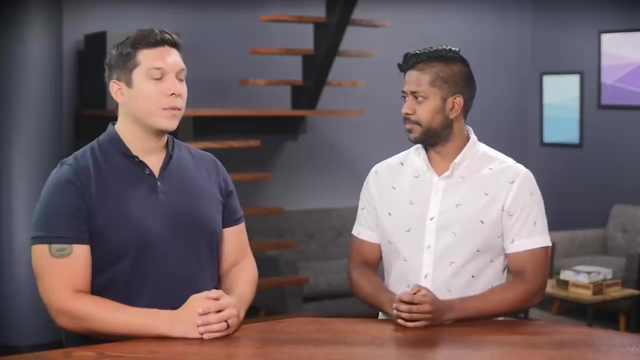 The winner is the winner. The winner is the one with the fewest tries. All right, John, Let's start with you. I'm thinking of a number between 1 and 10.. What is it Between you and me? the answer is 3.. 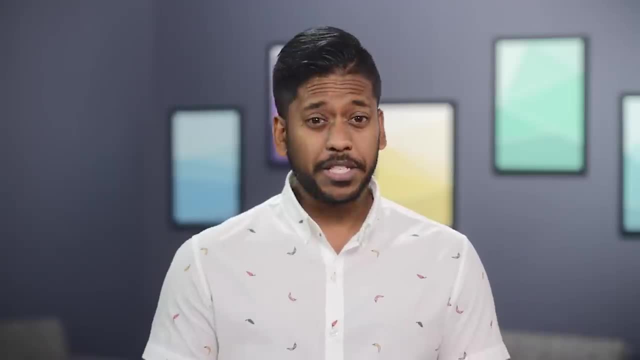 Quick question: Does the range include 1 and 10?? That is a really good question. So what John did right there was to establish the bounds of our problem. No solution works on every problem, And an important part of algorithmic thinking is to clearly define what the problem set is. 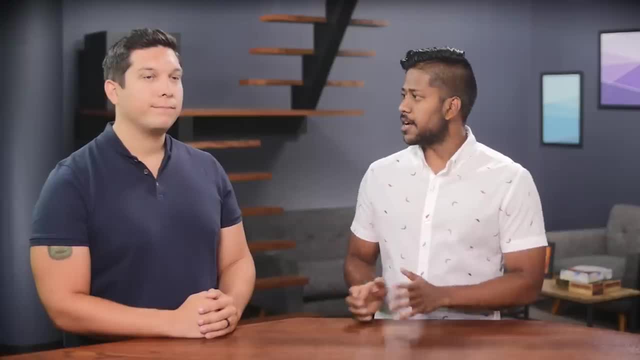 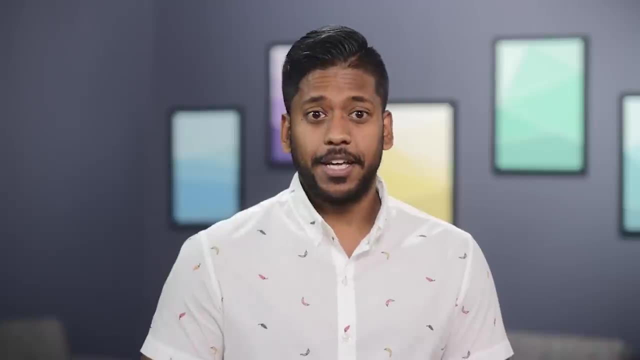 and clarify what values count as inputs. Yeah, So 1 and 10 are both included. Is it 1? Too low? Is it 2? Too low? Is it 3? Correct, OK, So that was an easy one. 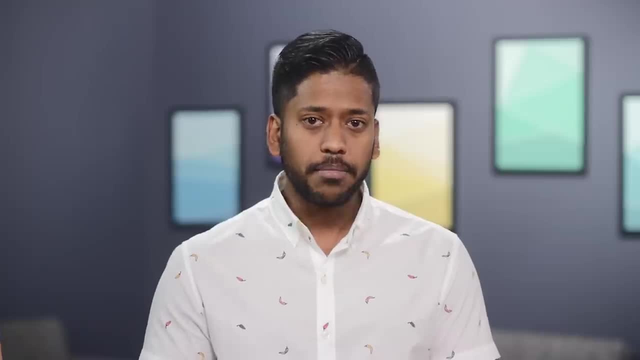 It took John three tries to get the answer. Let's switch over to Brittany and play another round using the same number as the answer. OK, Brittany, I'm thinking of a number between 1 and 10 inclusive. So both 1 and 10 are in the range. 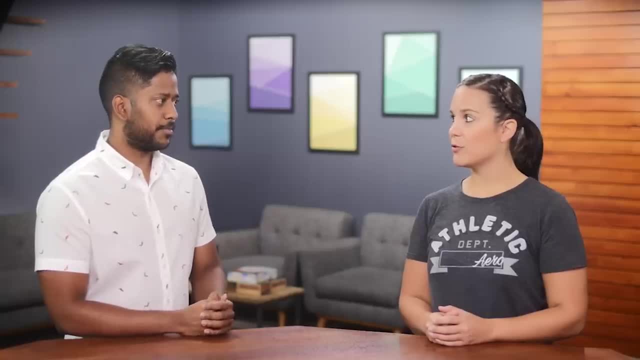 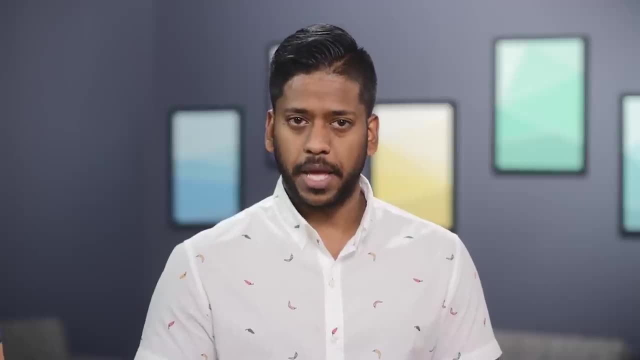 What number am I thinking of? Is it 5? Too high? 2? Too low? Is it 3? Correct, All right, So we have two different ways of playing the same game. Somehow, with even such a simple game, we saw different approaches to figuring out a solution. 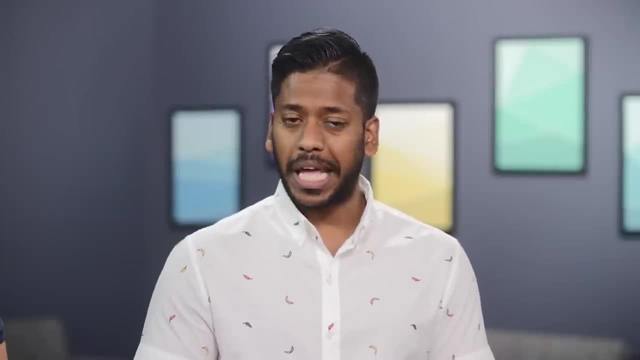 To go back to algorithmic thinking for a second. this means that with any given problem, there is no one best solution. Instead, what we should try and figure out is what solution works better for the current problem. In this first pass at the game, they both took the same amount of turns to find the answer. 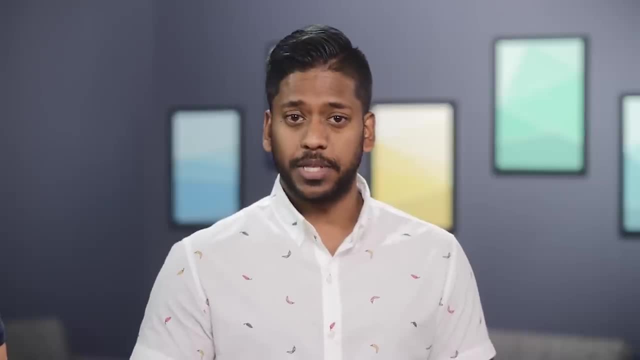 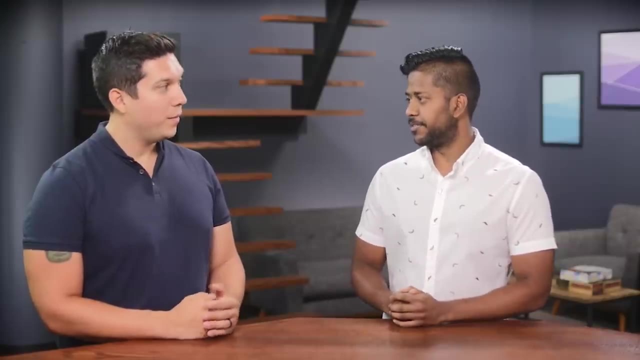 So it's not obvious who has the better approach, And that's mostly because the game was easy. Let's try this one more time Now. this time, the answer is 10.. All right, John, You first. Is it 1?? 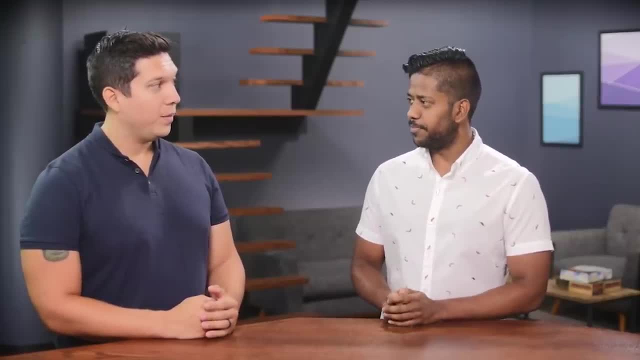 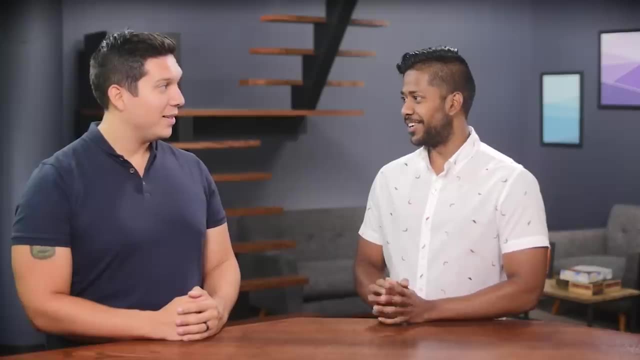 All right, John, you first. Is it 1? Too low? Is it 2? Still too low? Is it 3? Too low? Is it 4? Too low? Is it 5? Still too low? Is it 6? Too low? 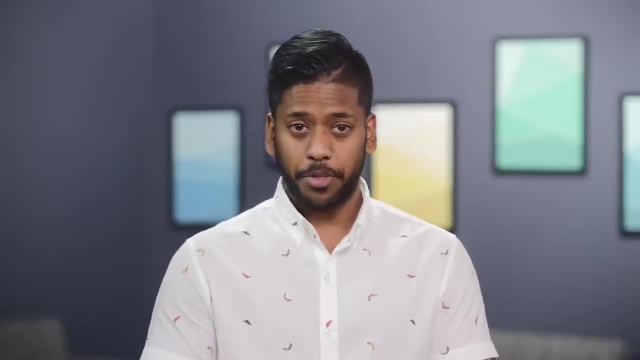 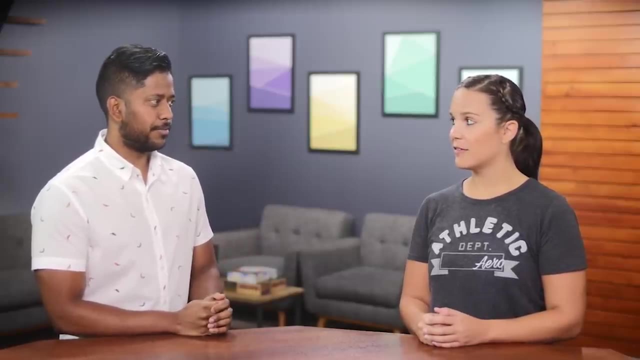 Is it 7? Too low? Is it 8? Too low? Is it 9? Too low? Is it 10?? Correct, You got it. Okay. so now same thing, but with Brittany this time. All right. so here we start to see a difference. 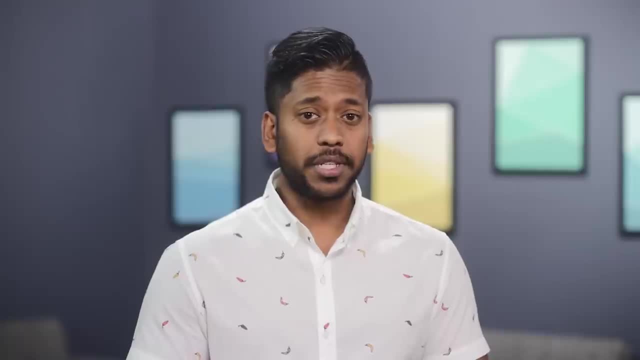 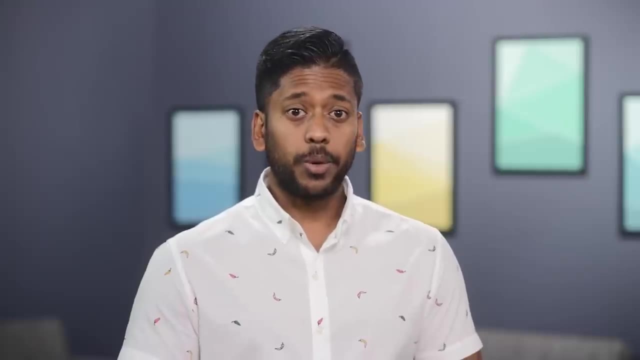 between their strategies. When the answer was 3, they both took the same number of turns. This is important When the number was larger, but not that much larger- 10. in this case, we start to see that Brittany's strategy did better. She took 4 tries. 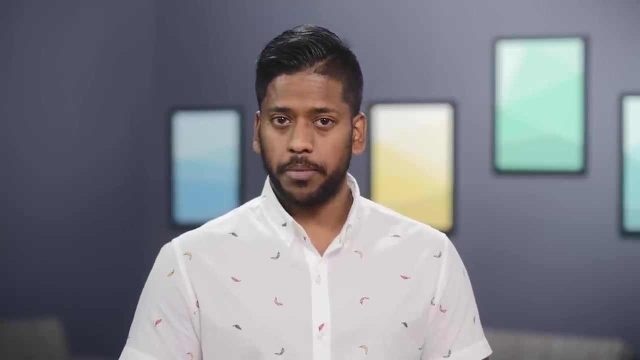 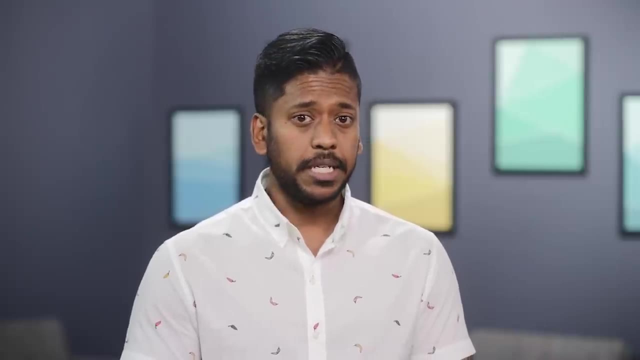 while John took 10.. We've played two rounds so far and we've seen a different set of results based on the number they were looking for. If you look at John's way of doing things, then the answer being 10, the round we just played. 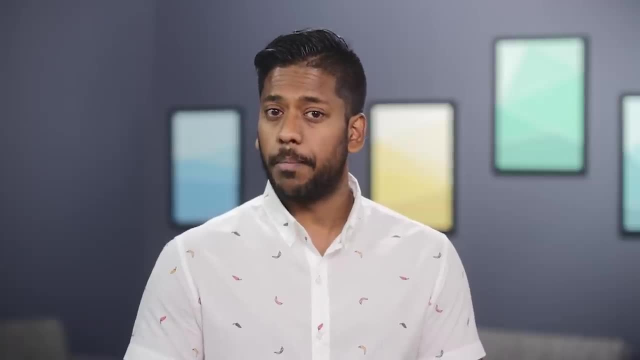 is his worst case scenario. He will take the maximum number of turns, 10, to guess it. When we picked a random number like 3, it was hard to differentiate which strategy was better because they both performed exactly the same. But in John's worst case, 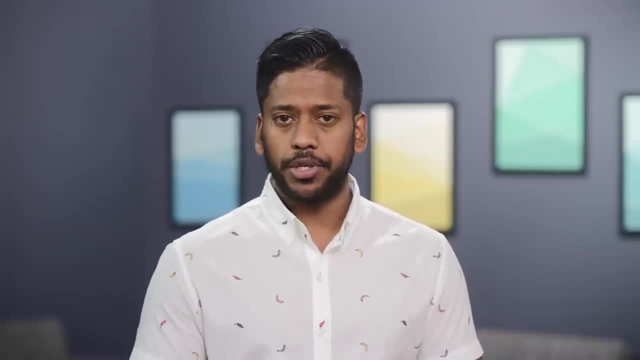 scenario, a clear winner in terms of strategy emerges. In terms of algorithmic thinking, we're starting to get a sense that the specific value they're searching for may not matter as much as where that value lies in the range that they have been given. 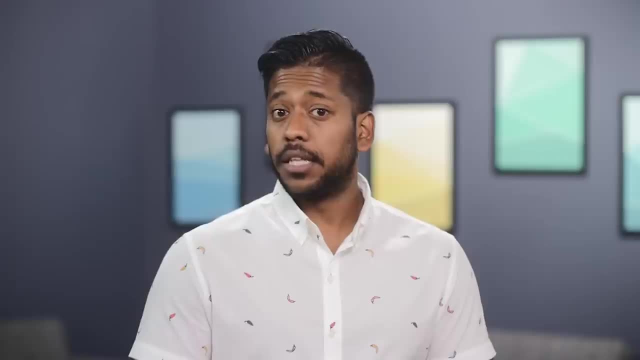 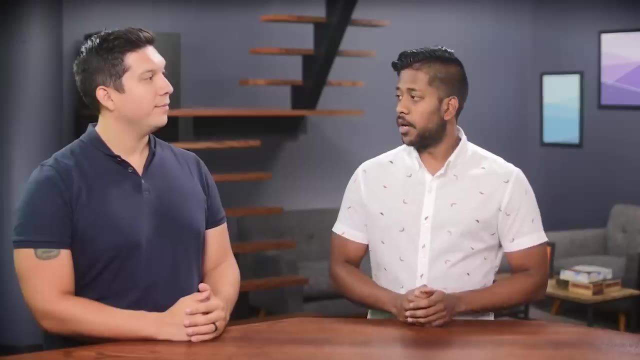 Identifying. this helps us understand our problem better. Let's do this again for a range of numbers from 1 to 100.. We'll start by picking 5 as an answer to trick them. Okay, so this time we're going to run through. 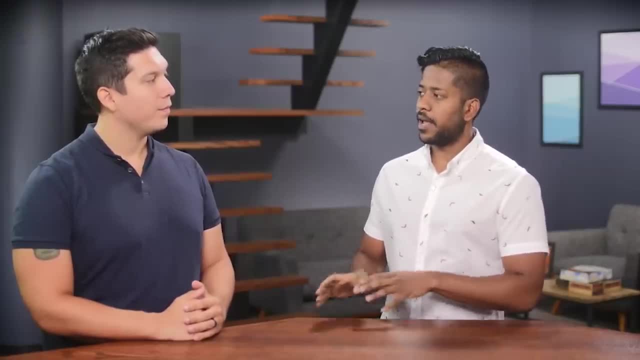 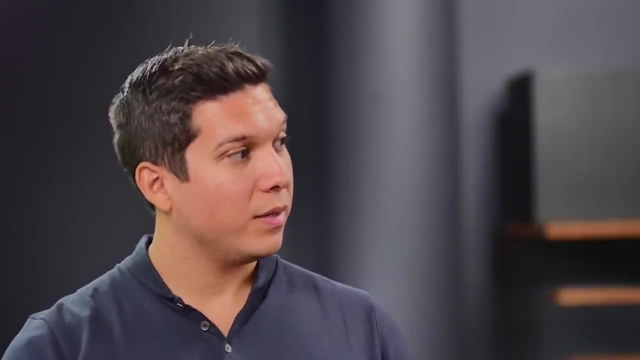 the exercise again, but this time from 1 to 100, and both 1 and 100 are included. At this point, without even having to run through it, we can guess how many tries John is going to take, Since he starts at 1 and keeps going. 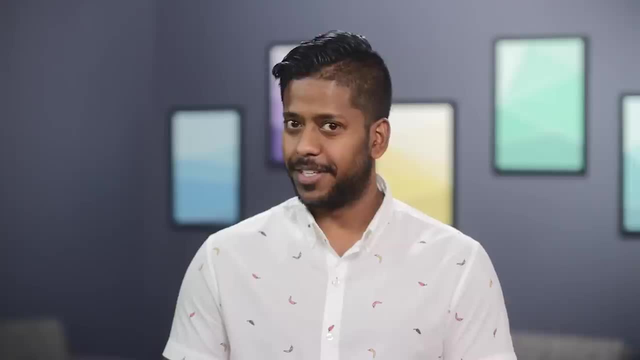 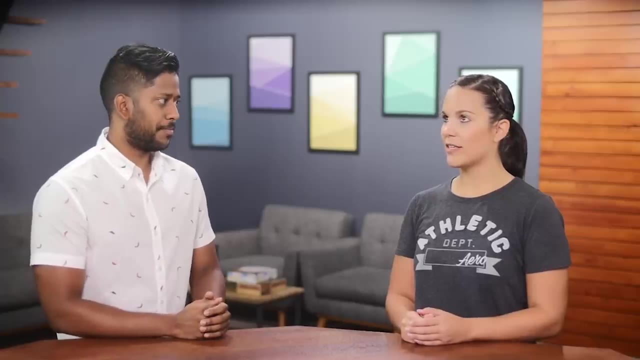 he's going to take 5 tries, as we're about to see. Cool correct. Okay, now for Brittany's turn. Is it 50? Too high? Is it 25? Still too high? Is it 13? Too high? 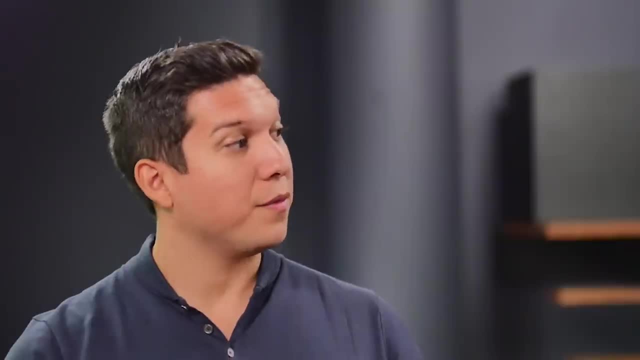 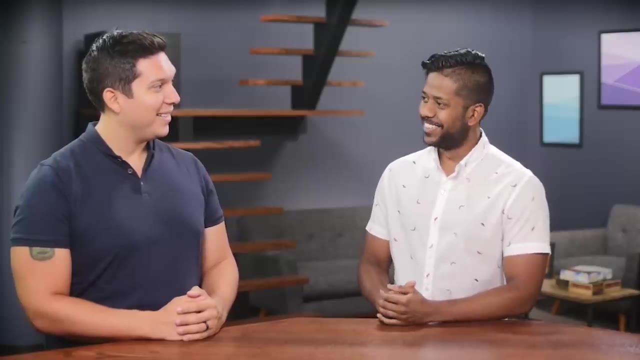 Too low. Is it 2? Still too low? Is it 3? Too low? Is it 4? Too low? Is it 5? Still too low? Is it 6? Too low? Is it 7? Too low? 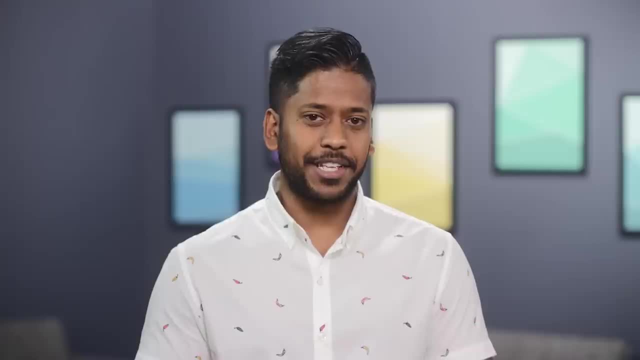 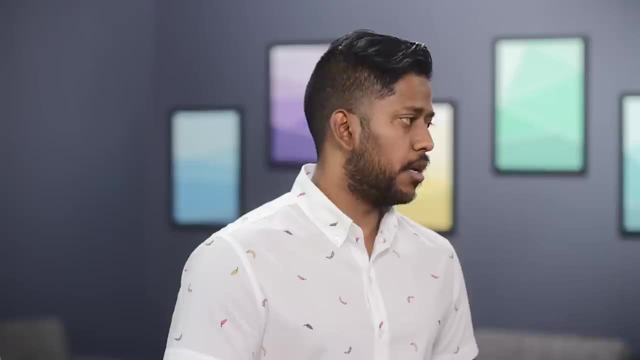 Is it 8? Too low. Is it 9? Too low, Is it 10?? Correct, You got it OK. So now same thing, but with Brittany. this time Still too low, It's 10.. All right, 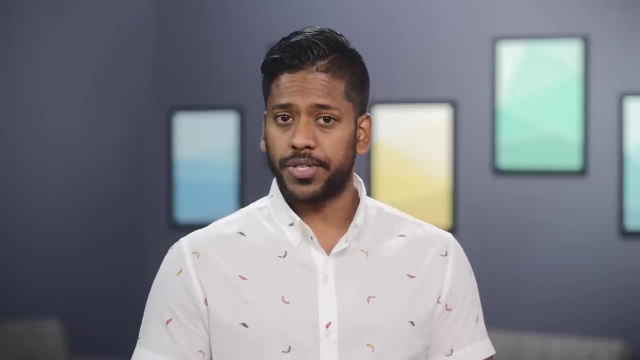 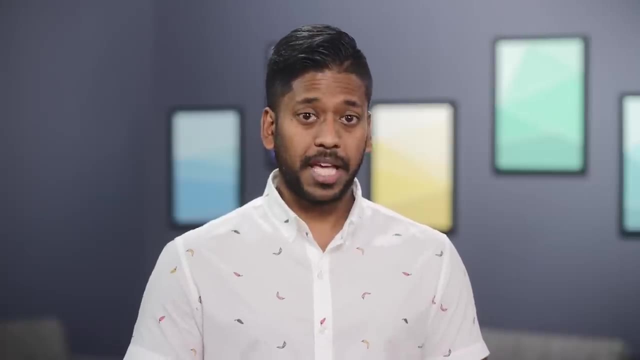 So here we start to see a difference between their strategies. When the answer was 3, they both took the same number of turns. This is important. When the number was larger, but not that much larger- 10 in this case, we start to see that 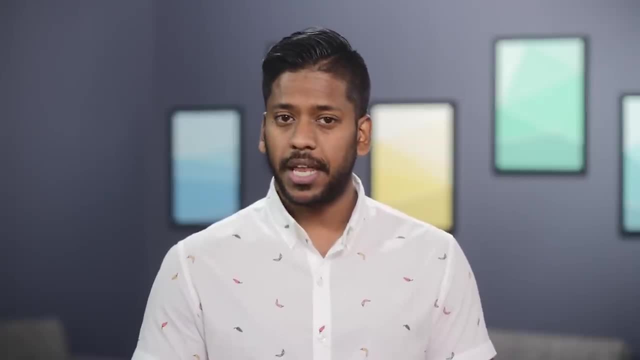 Brittany's strategy did better. She took 4 tries, while John took 10.. We've played two rounds so far and we've seen a different set of results based on the number they were looking for. If you look at John's way of doing things then the answer being 10, the round we just 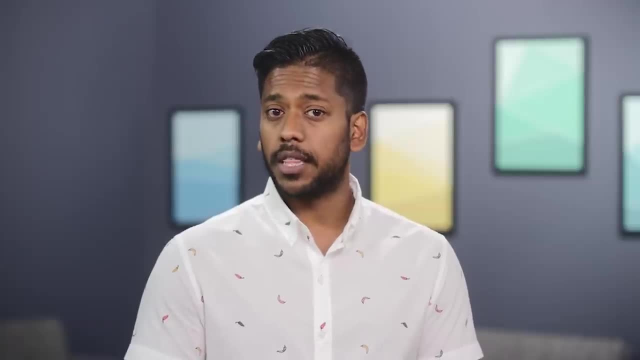 played is his worst-case scenario. He will take the maximum number of turns, 10,. to guess it, When we picked a random number like 3, it was hard to differentiate which strategy was better, because they both performed exactly the same. 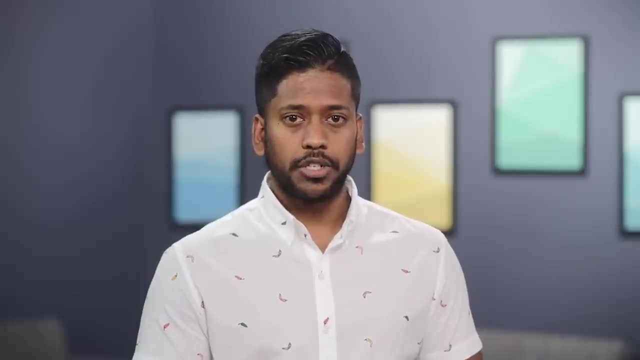 But in John's worst-case scenario, a clear winner in terms of strategy emerges. In terms of algorithmic thinking, we're starting to get a sense that the specific value they're searching for may not matter as much as where that value lies in the random number. 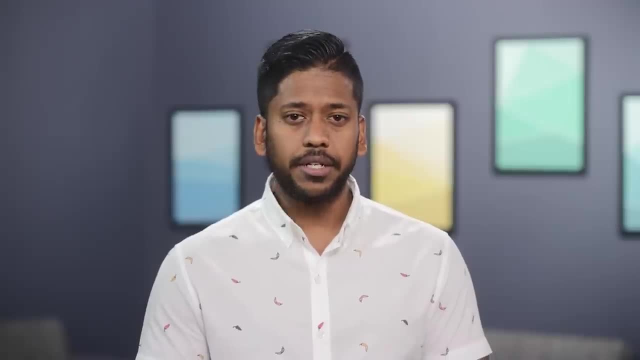 Identifying. this helps us understand our problem better. Let's do this again for a range of numbers from 1 to 100.. We'll start by picking 5 as an answer to trick them. Okay, so this time we're going to run through the exercise again, but this time from 1 to 100,. 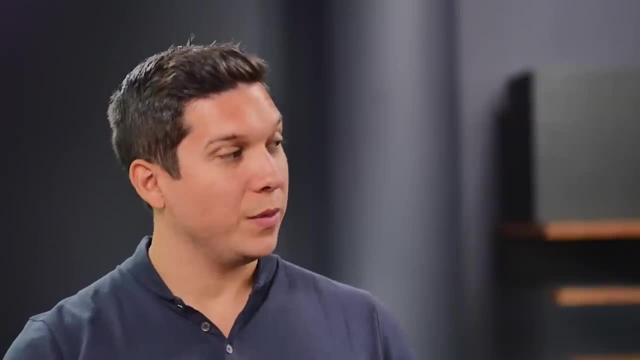 and both 1 and 100 are included. At this point, without even having to run through it, we can guess how many tries John is going to take, Since he starts at 1 and keeps going. he's going to take 5 tries, as we're about to see. 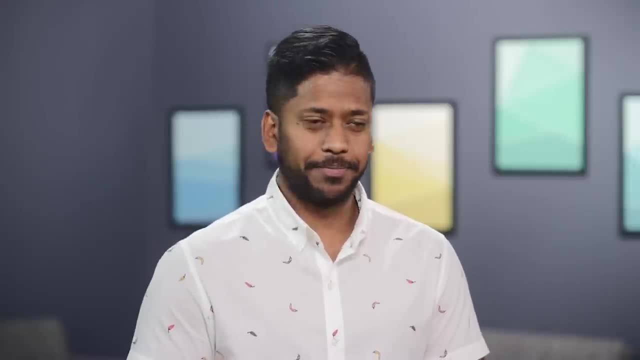 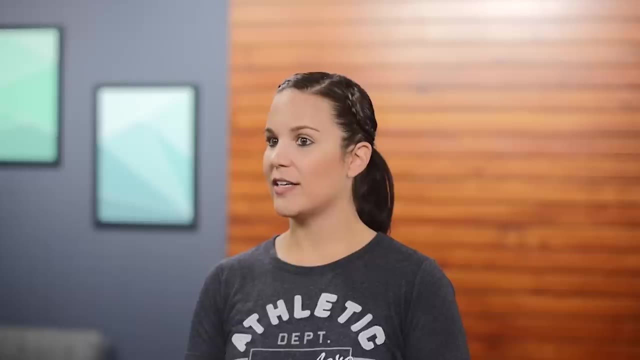 Cool, correct. Okay, now for Brittany's turn. Is it 50? Too high? Is it 25? Still too high? Is it 13? Too high? Is it 7? Too high? Is it 4? Too low? 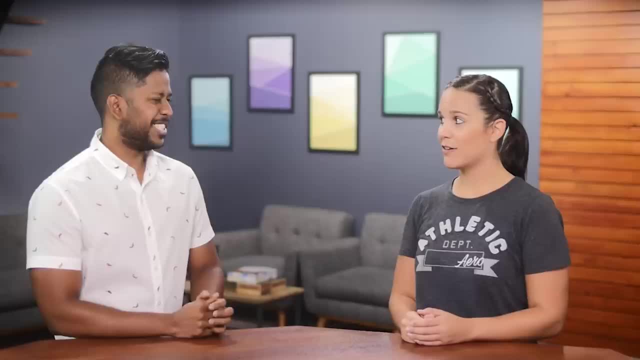 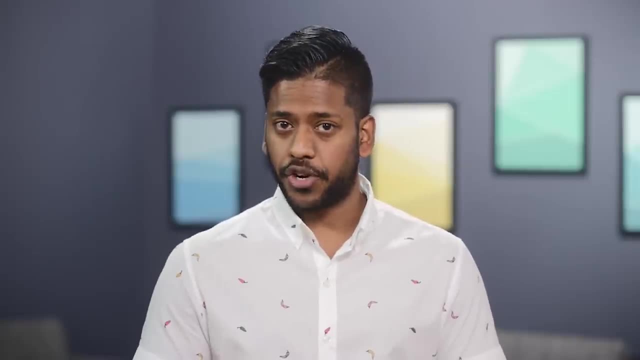 Is it 7? Too high? Is it 4? Too low? Is it 6? Too high? Is it 5? Correct, Let's evaluate. John took 5 tries. Brittany, on the other hand, took 7 tries. So John wins. 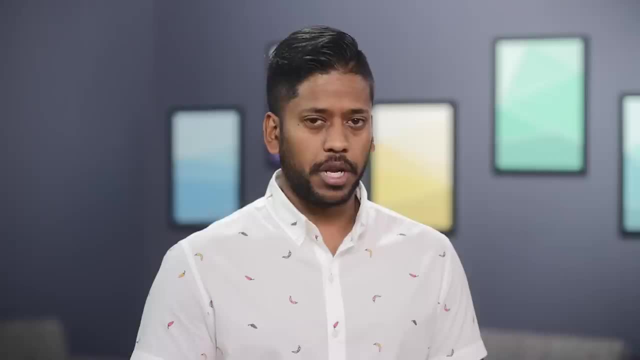 this round. but again, in determining whose strategy is preferred, there's no clear winner right now. What this tells us is that it's not particularly useful to look at the easy answers, where we arrive at the number fairly quickly because it's at the start of the range. 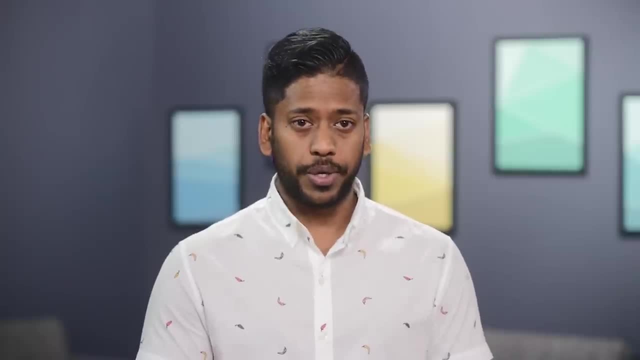 Instead, let's try one where we know John is going to do poorly. Let's look at his worst-case scenario, where the answer is 100, and see how Brittany performs in such a scenario. Okay, John, let's do this one more time. 1. 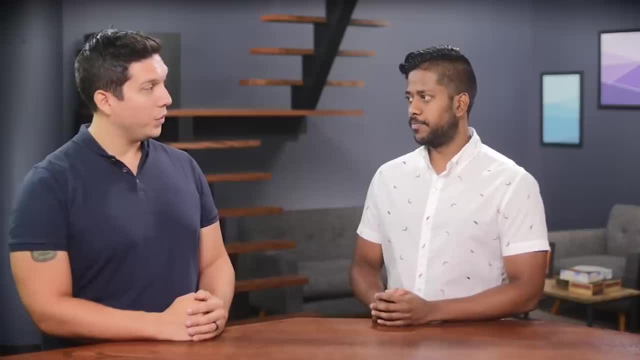 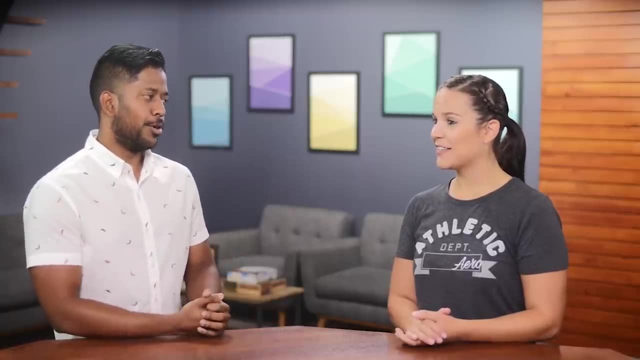 through 100 again. Is it 1?? We can fast-forward this scene because well, we know what happens: John takes 100 tries. Alright, Brittany, you're up. Is it 50? Too low? Is it 75?? 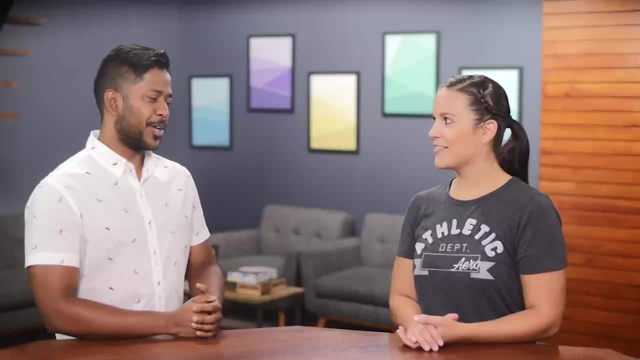 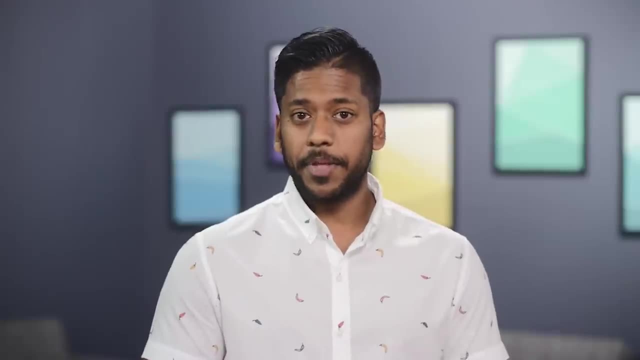 Too low. 88? Too low, 94? Too low, Is it 97?? Too low? 99? Too low, 100.. Okay, so that took Brittany 7 turns again, and this time she is the clear winner If you compare their individual. 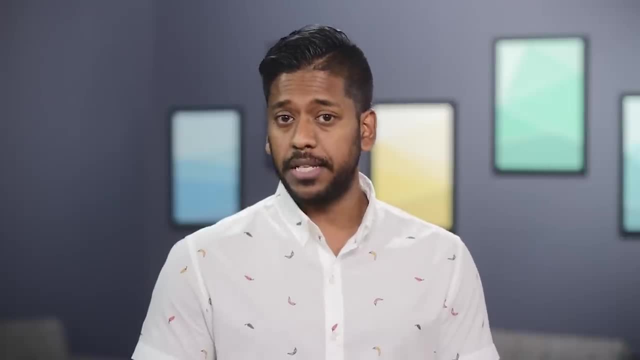 performances for the same number set, you'll see that Brittany's approach leaves John's in the dust. When the answer was 5, so right around the start of the range, John took 5 turns. But when the answer was 100, right at 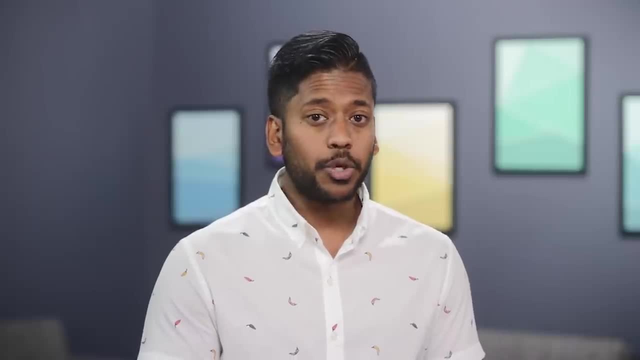 the end of the range he took 100 tries. It took him 20 times the amount of tries to get that answer, compared to Brittany. On the other hand, if you compare Brittany's efforts, when the number was 5, she took 7. 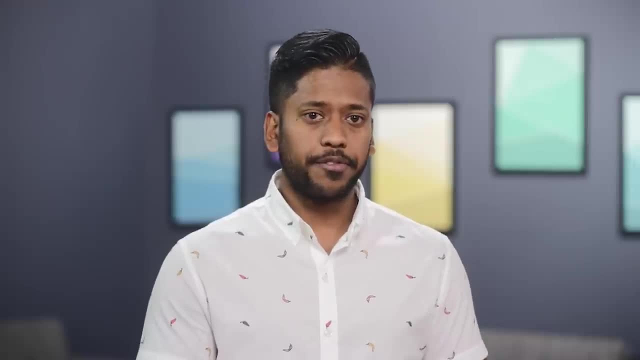 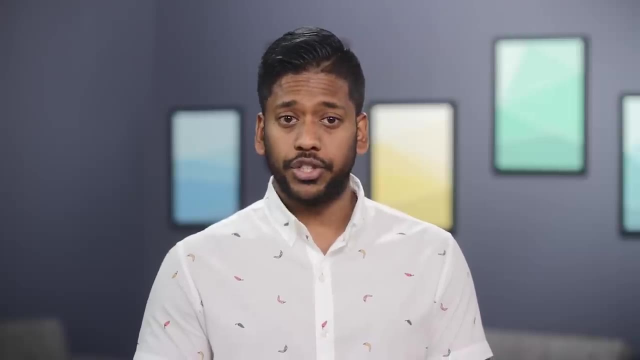 tries, But when the number was 100, she took the same amount of tries. This is pretty impressive. If we pretend that the number of tries is the number of seconds it takes Brittany and John to run through their attempts, this is a good estimate for how 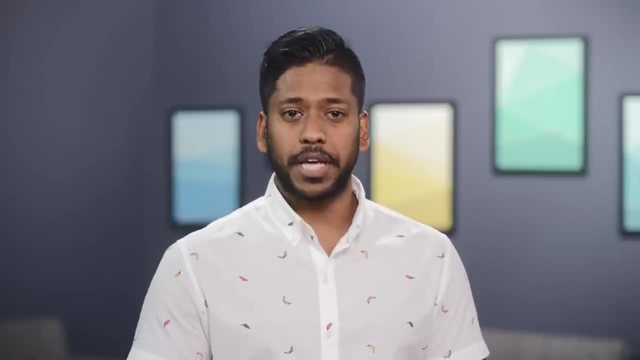 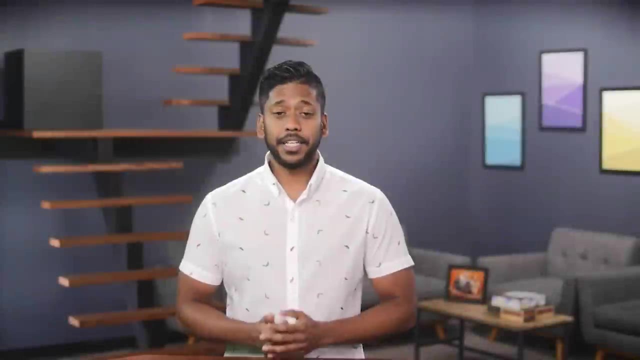 fast. their solutions are Okay. we've done this a couple times and Brittany and John are getting tired. Let's take a break. In the next video we'll talk about the point of this exercise. In the last video we ran through. 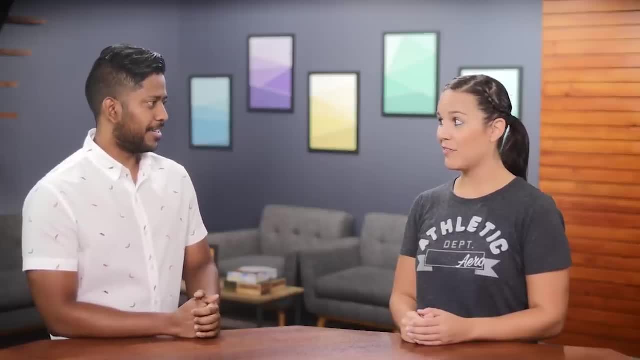 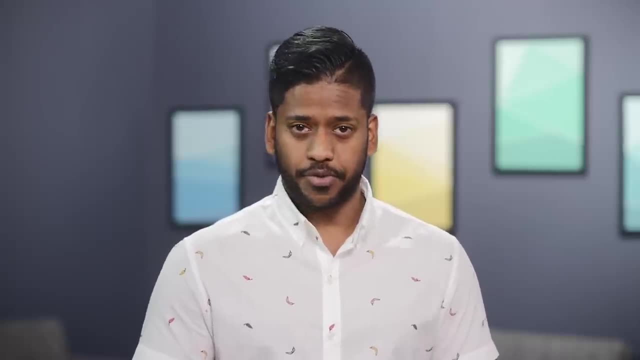 Is it 6? Too high? Is it 5? Correct? Let's evaluate. John took 5 tries. Brittany, on the other hand, took 7 tries. So John wins this round. but again, in determining whose strategy is preferred, there's no clear. 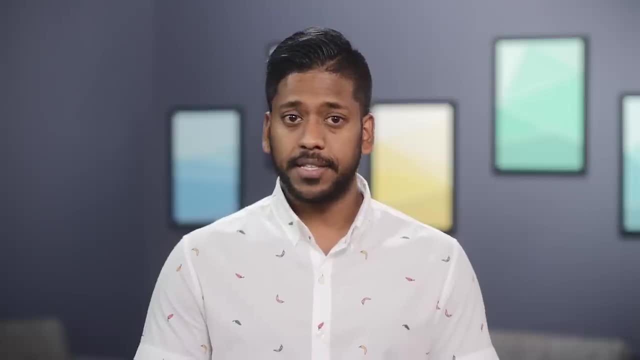 winner right now. What this tells us is that it's not particularly useful to look at the easy answers where we arrive at the number fairly quickly because it's at the start of the range. Instead, let's try one where we know John is going to do poorly. 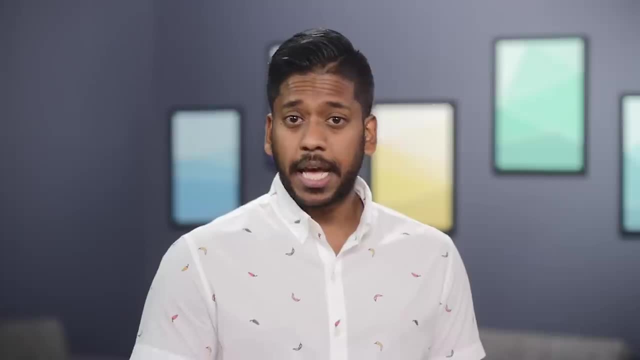 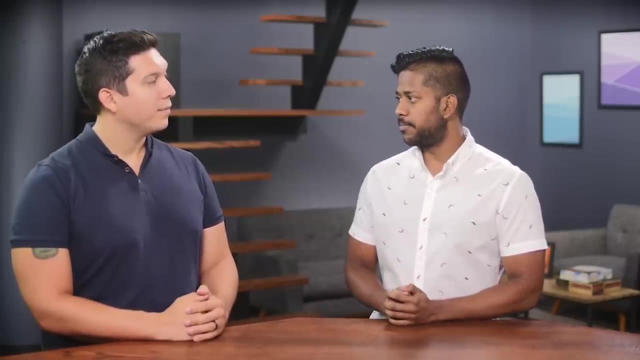 Let's look at his worst case scenario, where the answer is 100, and see how Brittany performs in such a scenario. Okay, John, let's do this one more time: 1 through 100 again. Is it 1?? We can fast forward this scene because, well, we know what happens. 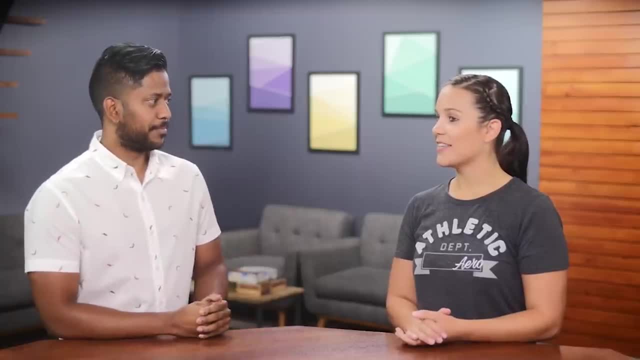 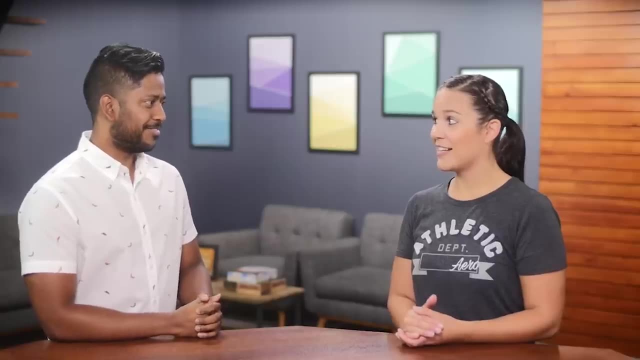 John takes 100 tries. Alright, Brittany, you're up. Is it 50? Too low? Is it 75? Too low? 88? Too low? 94? Too low? Is it 97? Too low? 99?? 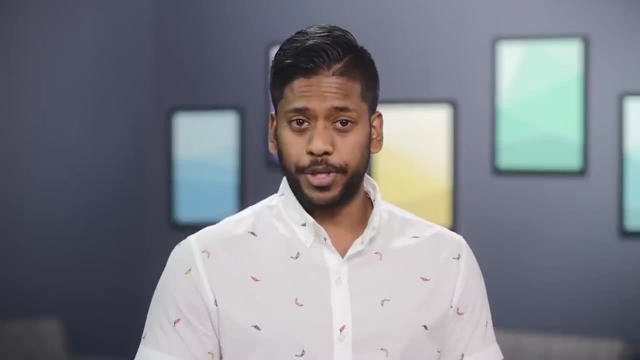 Too low: 100.. Okay, so that took Brittany 7 turns again, and this time she is the clear winner. If you compare their individual performances for the same number set, you'll see that Brittany's approach leaves John's in the dust. 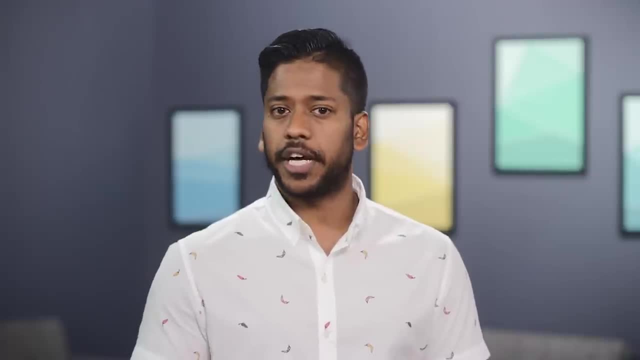 When the answer was 5, so right around the start of the range, John took 5 turns. But when the answer was 100, right at the end of the range, he took 100 tries. It took him 20 times the amount of tries to get that answer, compared to Brittany. 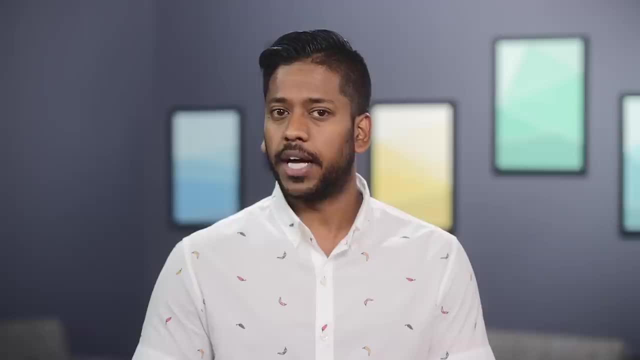 On the other hand, if you compare Brittany's efforts, when the number was 5, she took 7 tries, but when the number was 100, she took the same amount of tries. This is pretty impressive. If we pretend that the number of tries is the number of seconds it takes Brittany and 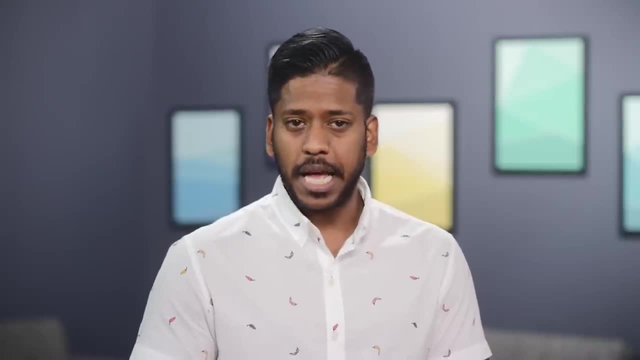 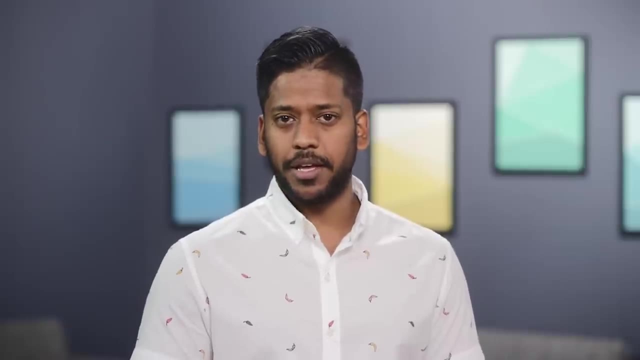 John to run through their attempts. this is a good estimate for how fast their solutions are. Okay, we've done this a couple times and Brittany and John are getting tired. Let's take a break. In the next video we'll talk about the point of this exercise. 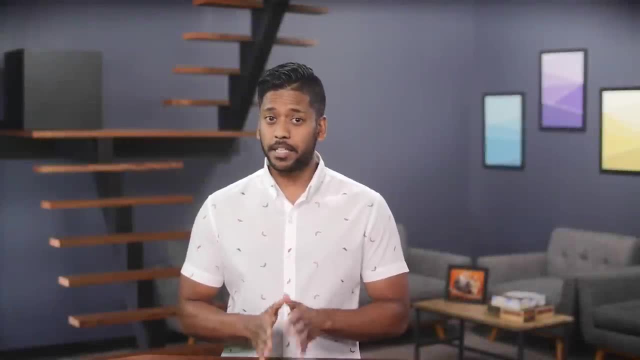 In the last video, we ran through an exercise where I had some of my coworkers- guess what number? I was thinking: So what was the point of that exercise? You might be thinking. hey, I thought I was here to learn about algorithms. The exercise we just did was an example of a real-life situation you will run into when 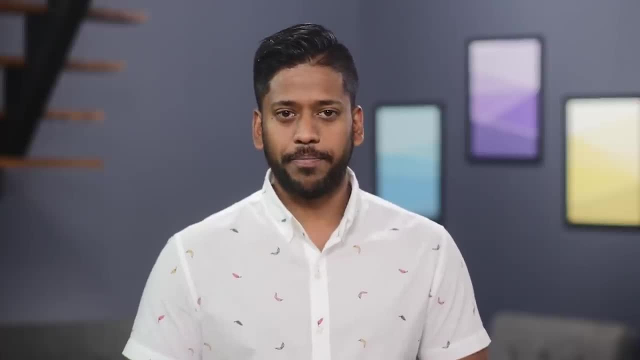 building websites, apps and writing code- Both approaches taken by John and Brittany to find the number I was thinking of- are examples of searching for a value. It might be weird to think that there's more than one way to search, but, as you saw in 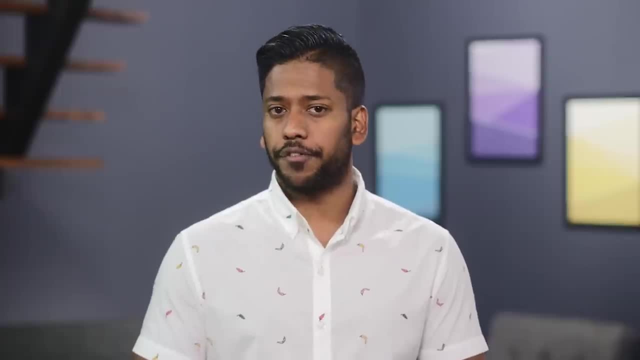 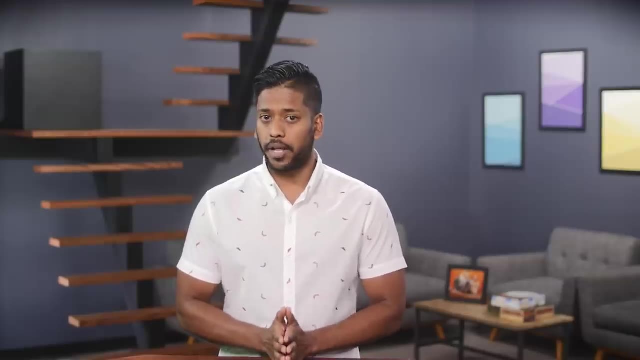 the game. the speed at which the result was obtained differed between John and Brittany. Think about this problem from the perspective of a company like Facebook. At the time of this recording, Facebook has 2.19 billion active users. Let's say you're traveling in a different country and meet someone you want to add on. 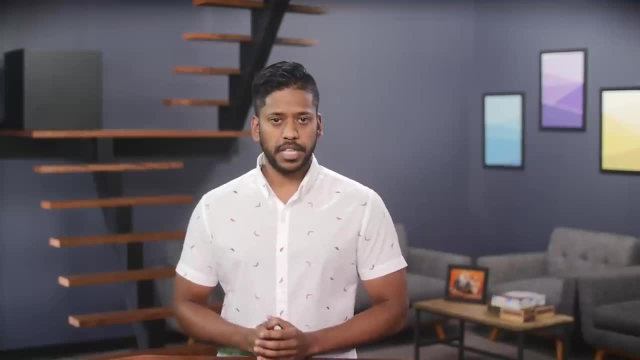 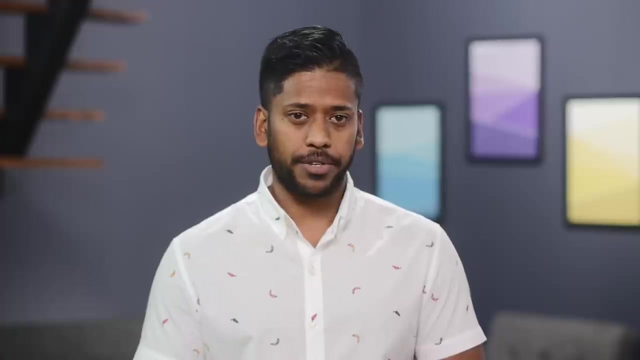 Facebook, You go into the search bar and type out this person's name. If we simplify how the Facebook app works, it has to search across these 2.19 billion records and find the person you are looking for. The speed at which you find this person really matters. 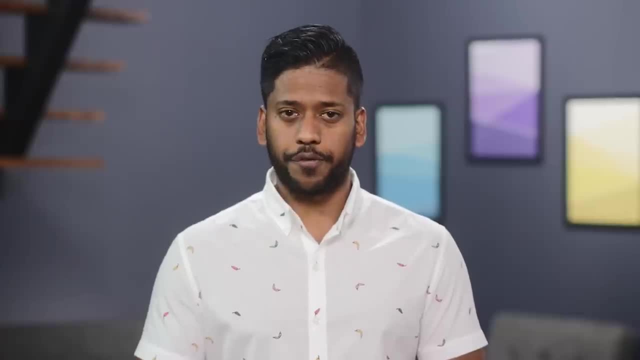 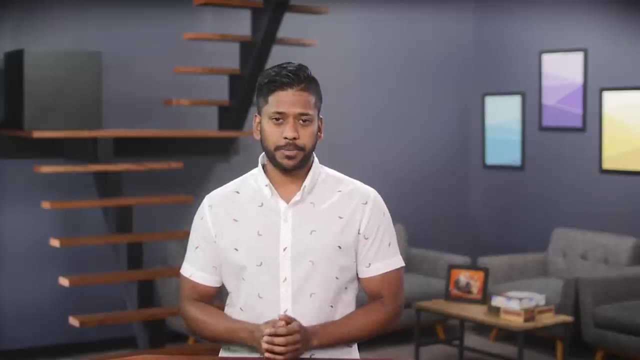 Imagine what kind of experience it would be if, when you search for a friend, Facebook put up a spinning activity indicator and said: come back in a couple hours. I don't think we'd use Facebook as much if that was the case From the company's perspective, working on making search as fast as possible using different 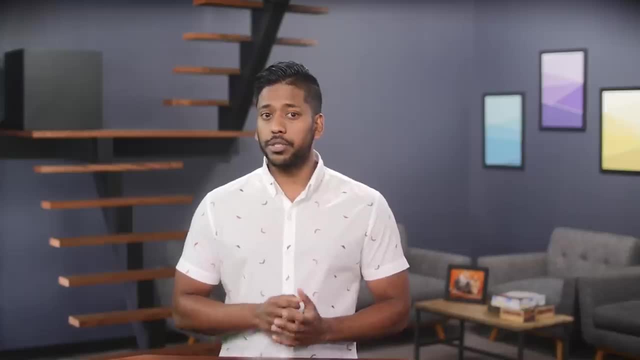 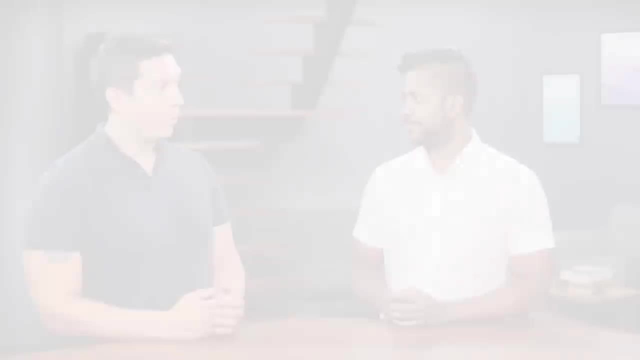 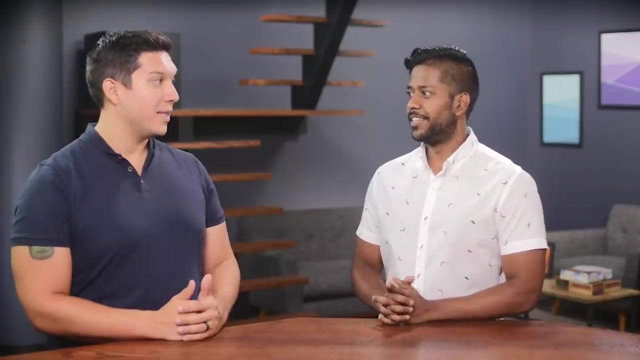 strategies really matters Now. I said that the two strategies Brittany and John used were examples of search. More specifically, these are search algorithms. The strategy John took, where he started at the beginning of the range and just counted one number after the other, is a type of search called linear search. 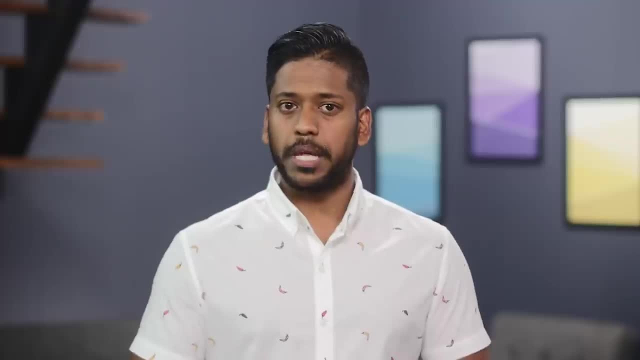 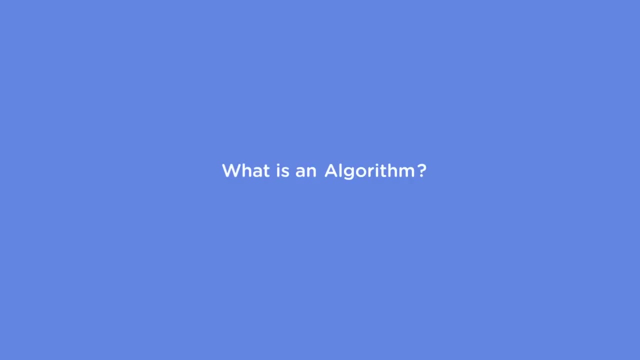 It is also called sequential search, which is a better description, Or even simple search, since it really is quite simple. But what makes his approach an algorithm as opposed to just looking for something? Remember we said that an algorithm is a set of steps or instructions to complete a task. 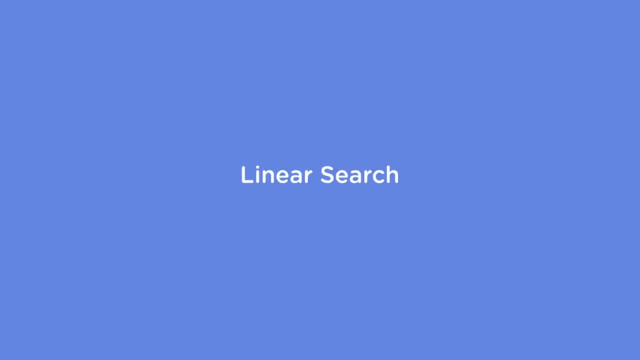 Linear search is a search algorithm and we can define it like this: We start at the beginning of the list or the range of values, Then we compare the current value to the target. If the current value is the target- the target value that we're looking for- we're done. 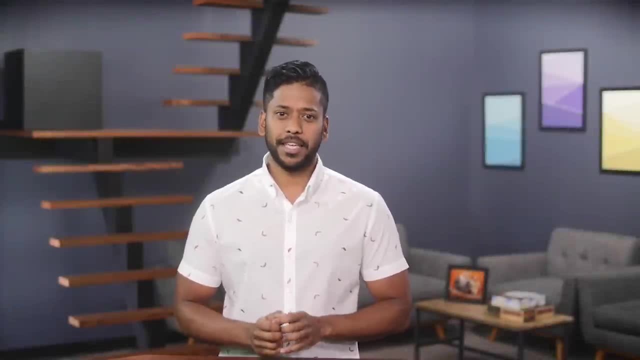 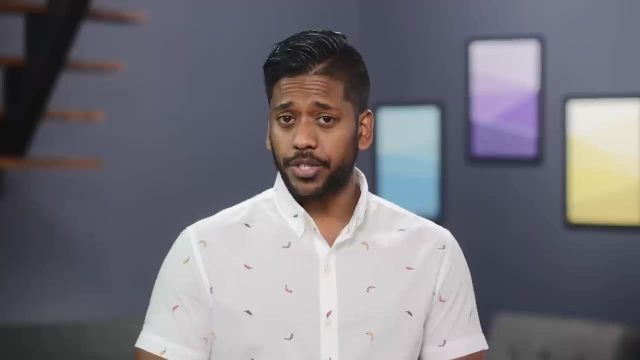 an exercise where I had some of my co-workers. guess what number. I was thinking. So what was the point of that exercise? You might be thinking: hey, I thought I was here to learn about algorithms. The exercise we just did was an example of a real-life situation. 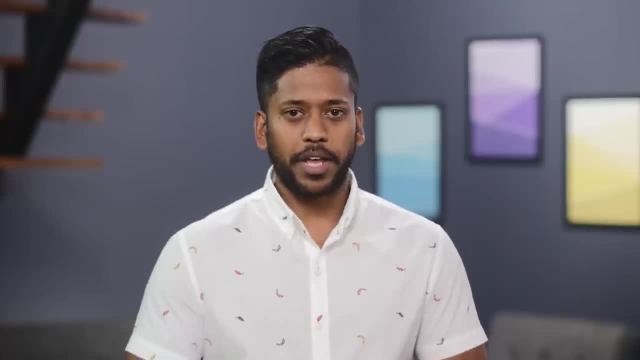 you will run into when building websites, apps and writing code. Both approaches taken by John and Brittany define the number I was thinking of are examples of searching for a value. It might be weird to think that there's more than one way to search, but, as you 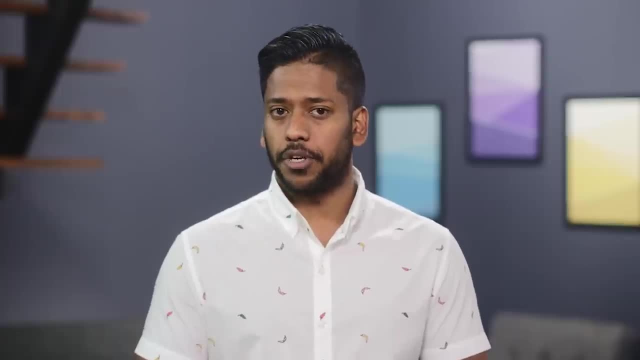 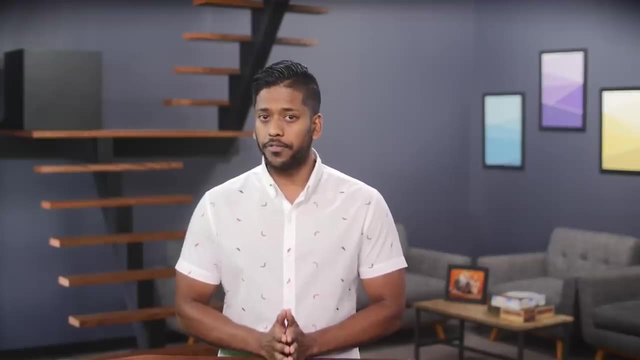 saw in the game, the speed at which the result was obtained differed between John and Brittany. Think about this problem from the perspective of a company like Facebook. At the time of this recording, Facebook has 2.19 billion active users. Let's say you're traveling in a different country. 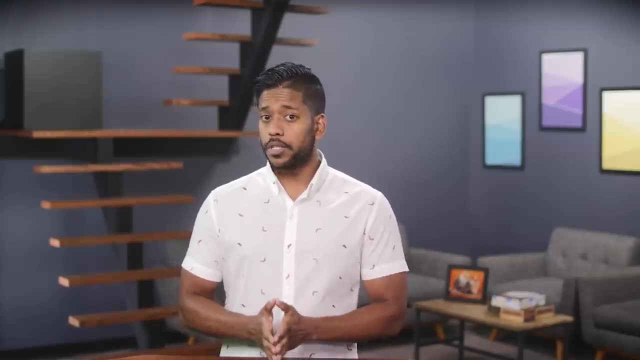 and meet someone you want to add on Facebook. You go into the search bar and type out this person's name. If we simplify how the Facebook app works, it has to search across these 2.19 billion records and find the person you are looking for. 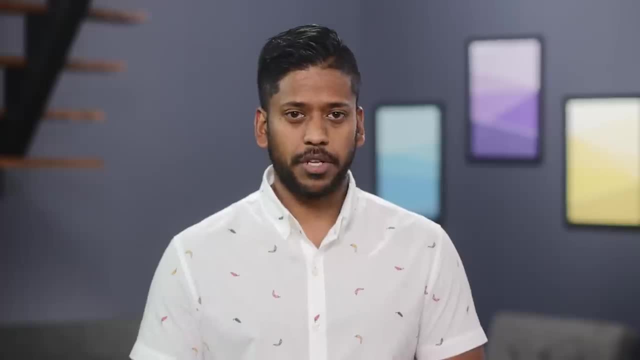 The speed at which you find this person really matters. Imagine what kind of experience it would be if, when you search for a friend, Facebook put up a spinning activity indicator and said: come back in a couple hours. I don't think we'd use. 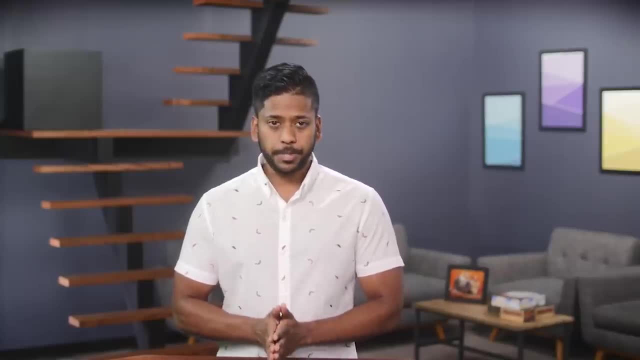 Facebook as much if that was the case. From the company's perspective, working on making search as fast as possible using different strategies, really matters. Now. I said that the 2 strategies Brittany and John used were examples of search. More specifically, these are search algorithms. 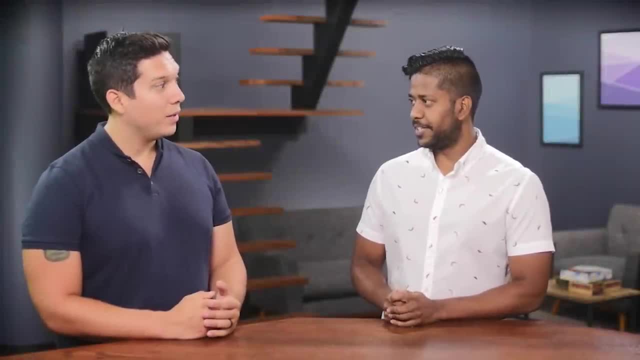 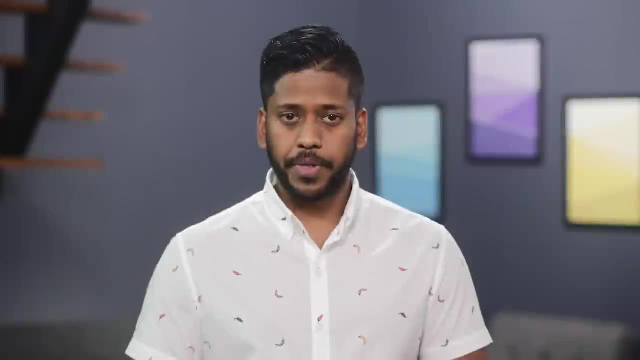 The strategy John took, where he started at the beginning of the range and just counted one number after the other, is a type of search called linear search. It is also called sequential search, which is a better description of how it works, or even simple. 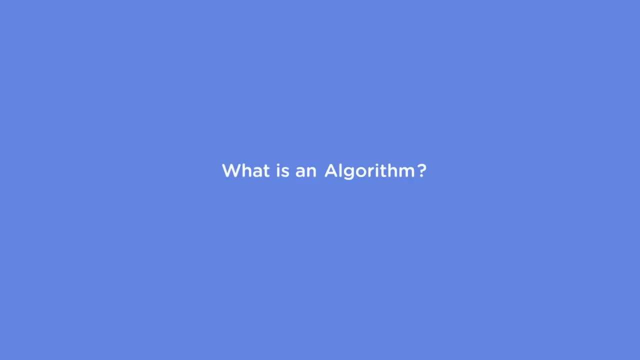 search, since it really is quite simple. But what makes his approach an algorithm as opposed to just looking for something? Remember we said that an algorithm is a set of steps or instructions to complete a task. Linear search is a search algorithm and we can define it like this. 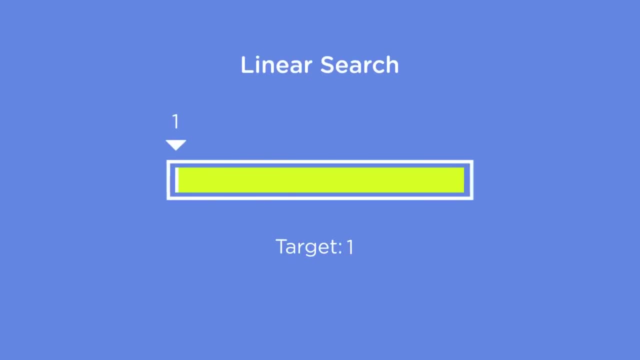 We start at the beginning of the list or the range of values. Then we compare the current value to the target. If the current value is the target value that we're looking for, we're done. If it's not, we'll move on sequentially to. 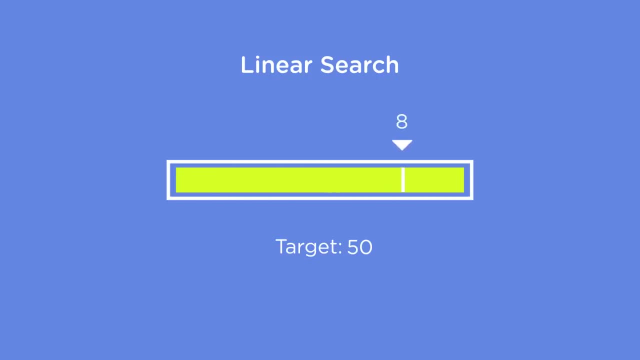 the next value in the list and then repeat step two. If we reach the end of the list, then the target value is not in the list. This definition has nothing to do with programming and in fact, you can use it in the real world. 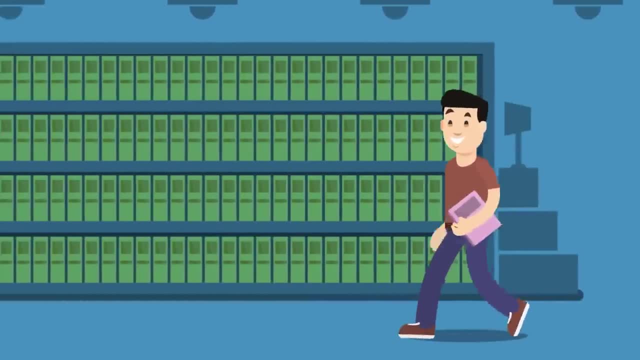 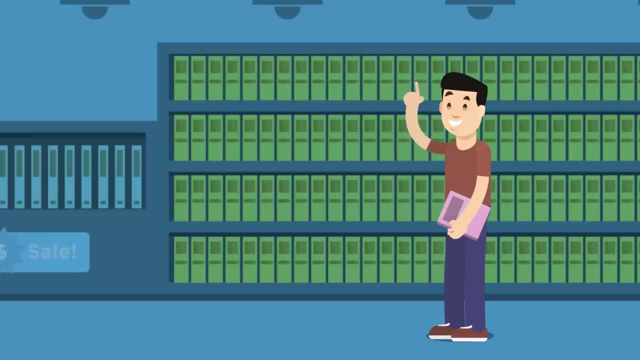 For example, I could tell you to walk into a bookstore and find me a particular book, And one of the ways you could do it is using the linear search algorithm. You could start at the front of the bookstore and read the cover or the spine of every book. 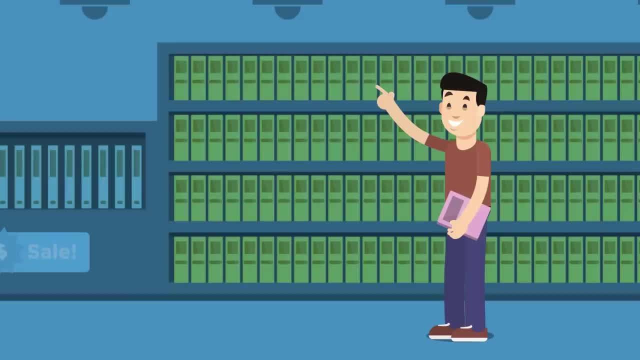 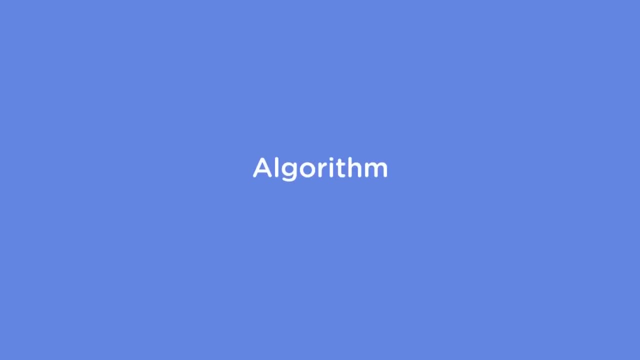 to check that it matches the book that you're looking for. If it doesn't, you go to the next book and repeat until you find it or run out of books. What makes this an algorithm is the specificity of how it is defined, In contrast to just jumping into a problem. 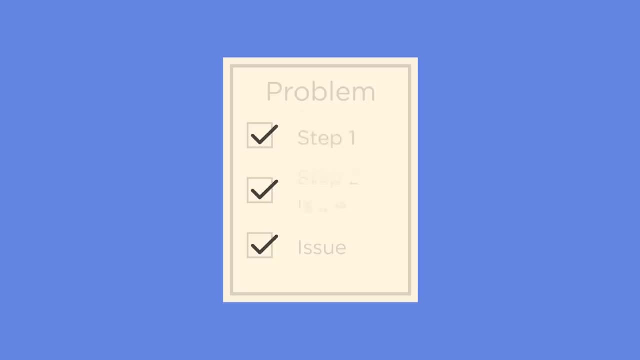 and solving it as we go along. an algorithm follows a certain set of guidelines and we use the same steps to solve the problem each time we face it. An important first step to defining the algorithm isn't the algorithm itself, but the problem we're trying to solve. 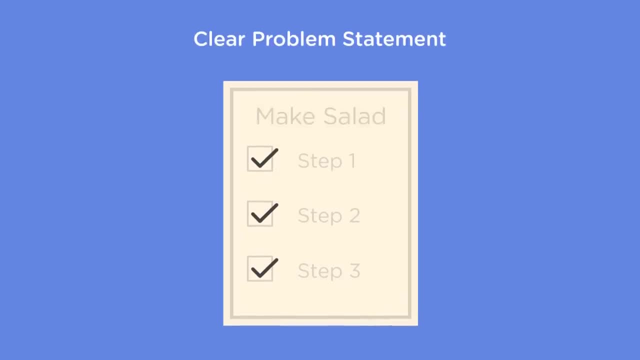 Our first guideline is that an algorithm must have a clear problem statement. It's pretty hard to define an instruction set when you don't have a clear idea of what problem you're trying to solve. In defining the problem, we need to specify how the input 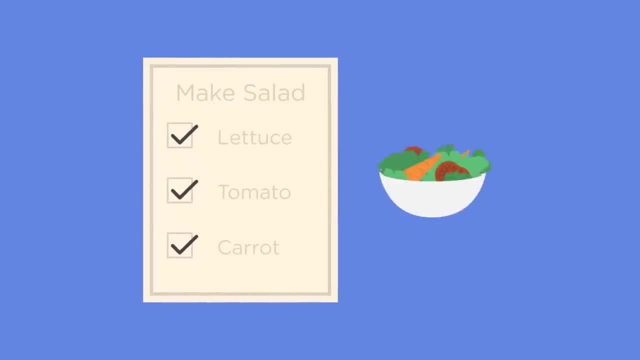 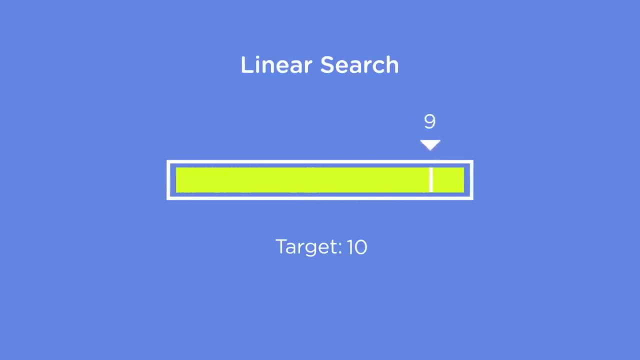 is defined and what the output looks like when the algorithm has done its job. For linear search, the input can be generally described as a series of values and the output is a value matching the one we're looking for Right now. we're trying to stay away from anything code-. 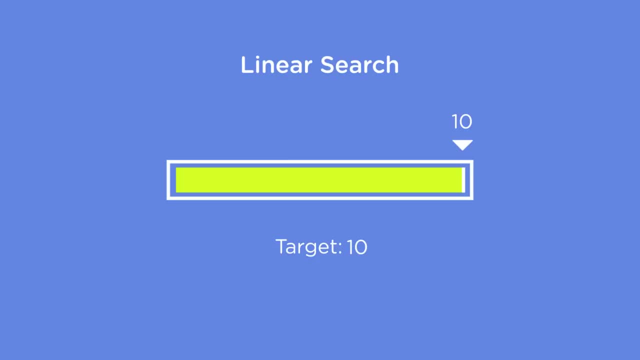 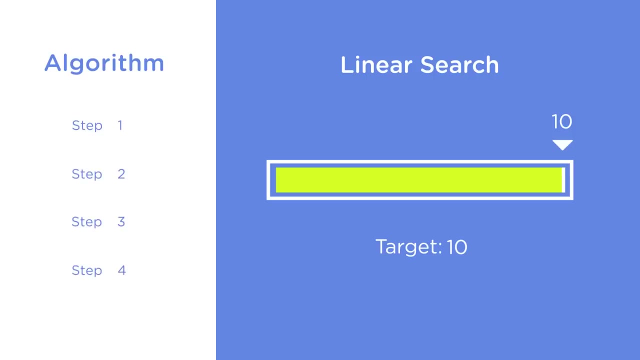 related. so this problem statement definition is pretty generic, but once we get to code we can actually tighten this up. Once we have a problem, an algorithm is a set of steps that solves this problem. Given that the next guideline is that an algorithm, 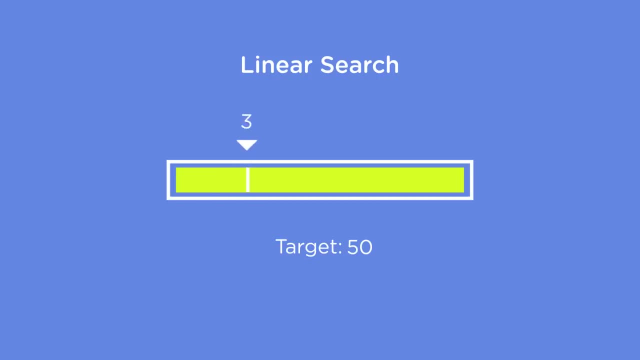 If it's not, we'll move on sequentially to the next value in the list and then repeat step two. If we reach the end of the list, then the target value is not in the list. This definition has nothing to do with programming. 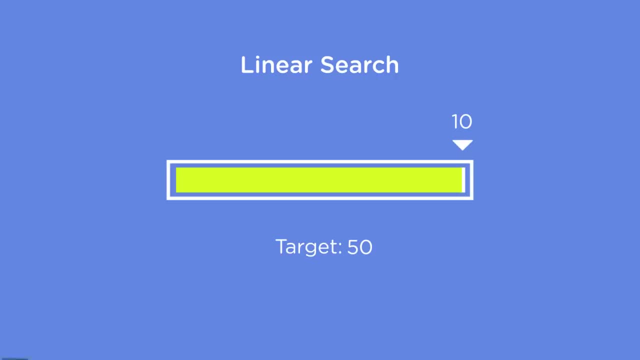 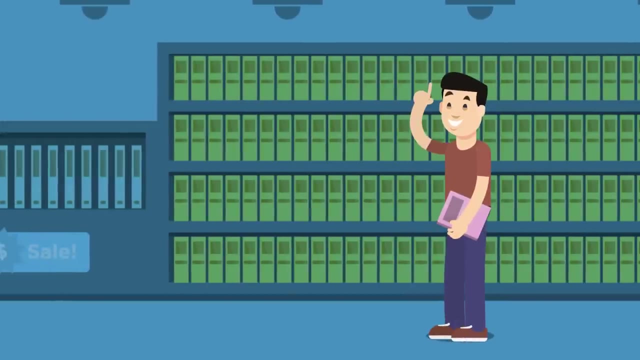 and in fact, you can use it in the real world. For example, I could tell you to walk into a bookstore and find me a particular book, And one of the ways you could do it is using the linear search algorithm. You could start at the front of the book. 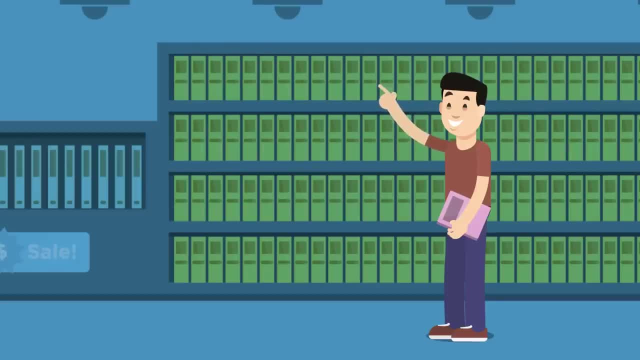 go to the bookstore and read the cover or the spine of every book to check that it matches the book that you're looking for. If it doesn't, you go to the next book and repeat until you find it or run out of books. 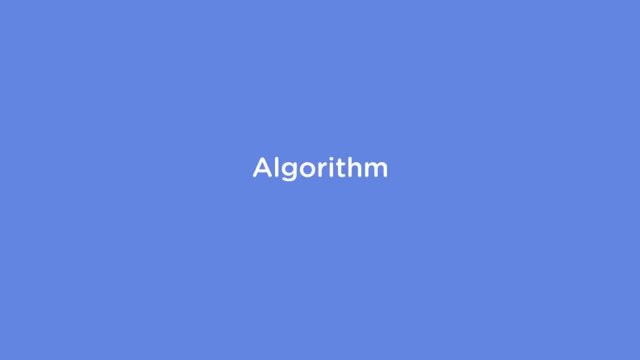 What makes this an algorithm is the specificity of how it is defined. In contrast to just jumping into a problem and solving it as we go along, an algorithm follows a certain set of guidelines and we use the same steps to solve the problem each time we face it. 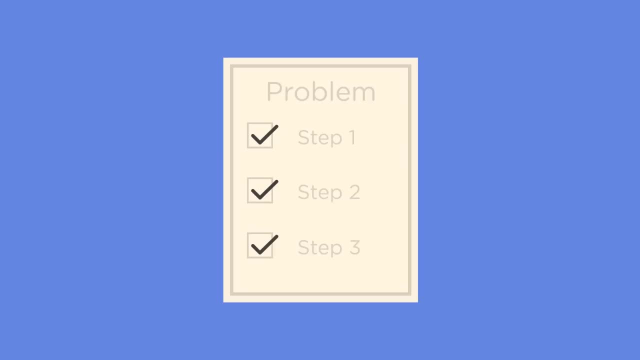 An important first step to defining the algorithm isn't the algorithm itself, but the problem we're trying to solve. Our first guideline is that an algorithm must have a clear problem statement. It's pretty hard to define an instruction set when you don't have a clear idea of what problem you're trying to solve. 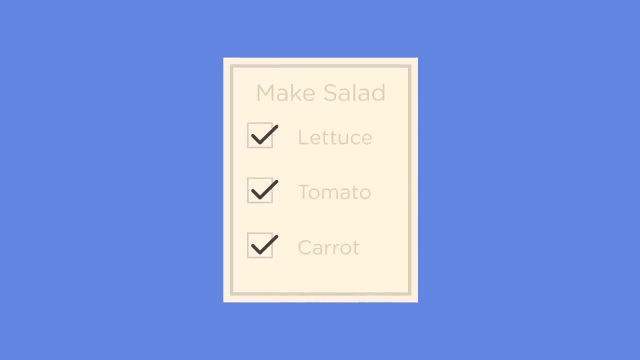 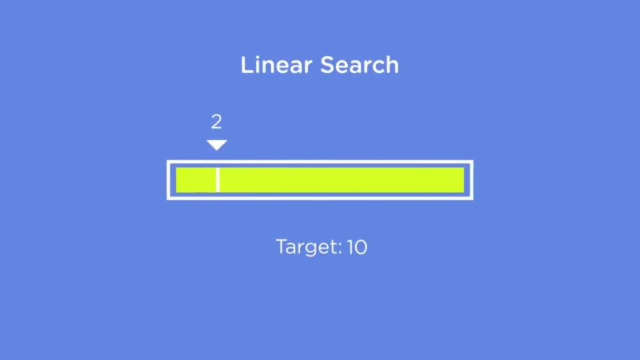 In defining the problem, we need to specify how the input is defined and what the output looks like when the algorithm has done its job. For linear search, the input can be generally described as a series of values and the output is a value matching the one we're looking for. 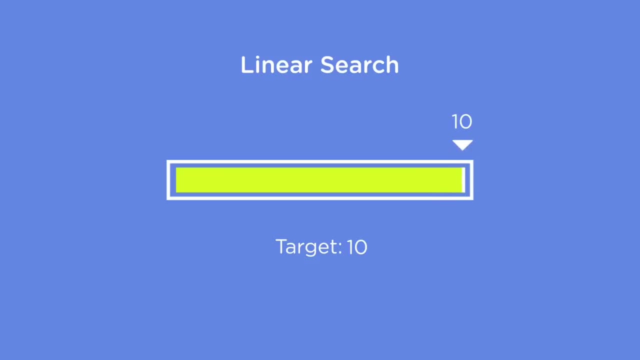 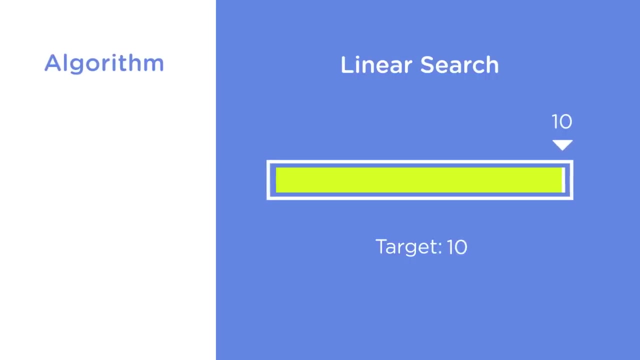 Right now we're trying to stay away from anything code-related, so this problem statement definition is pretty generic, but once we get to code we can actually tighten this up. Once we have a problem, an algorithm is a set of steps that solves this problem. 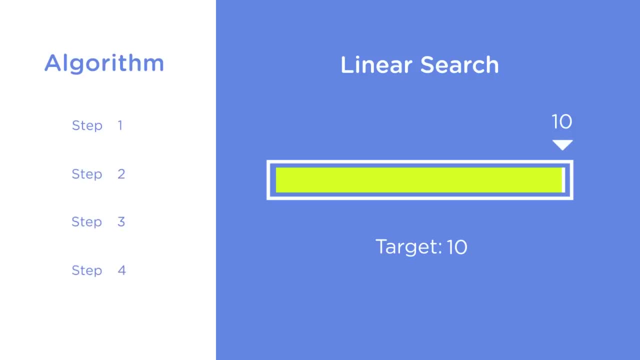 Given that the next guideline is that an algorithm definition must contain a specific set of instructions in a particular order, We really need to be clear about the order in which these instructions are executed. Taking our simple definition of linear search, if I switched up the order, 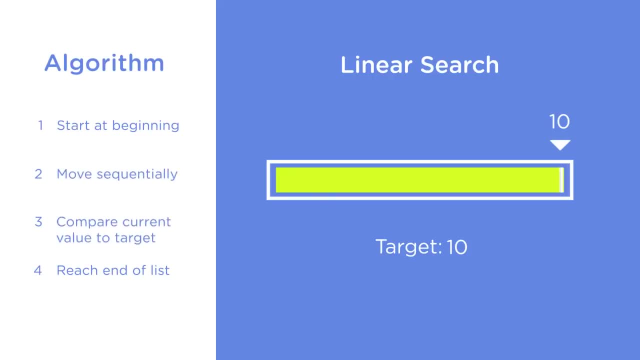 and said: move sequentially to the next value, before specifying that first comparison step. if the first value were the target one, our algorithm wouldn't find it because we moved to the second value before comparing. Now you might think, okay, that's just an avoidable mistake. 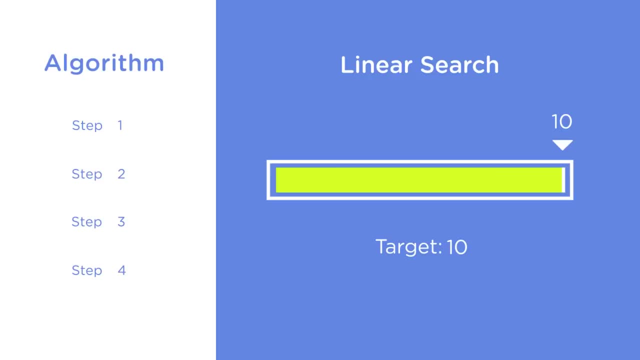 definition must contain a specific set of instructions in a particular order. We really need to be clear about the order in which these instructions are executed. Taking our simple definition of linear search, if I switched up the order and said move sequentially to the next value before specifying, 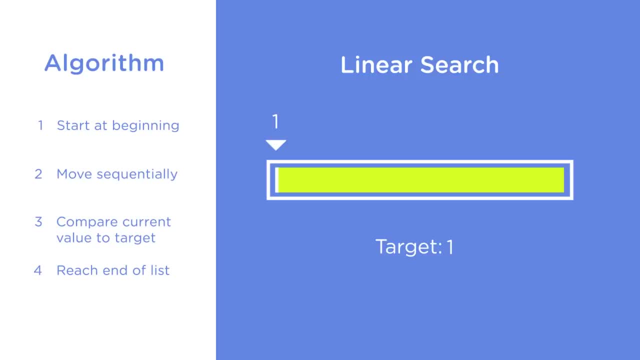 that first comparison step. if the first value were the target one, our algorithm wouldn't find it, because we moved to the second value before comparing. Now you might think, okay, that's just an avoidable mistake and kind of common sense. The thing is, computers don't know any of that. 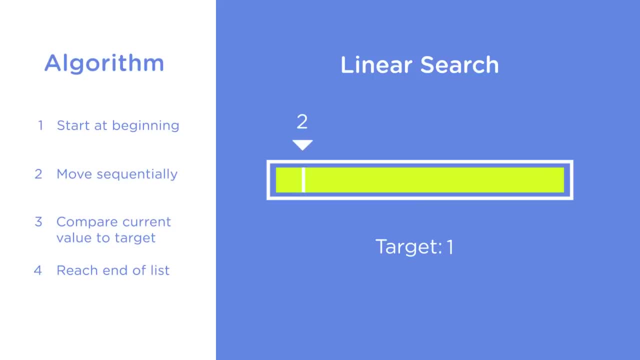 and just do exactly as we tell them. So specific order is really important. The third guideline is that each step in our algorithm definition must not be a complex one. It needs to be explicitly clear. What I mean by that is that you shouldn't be able to break down any of the 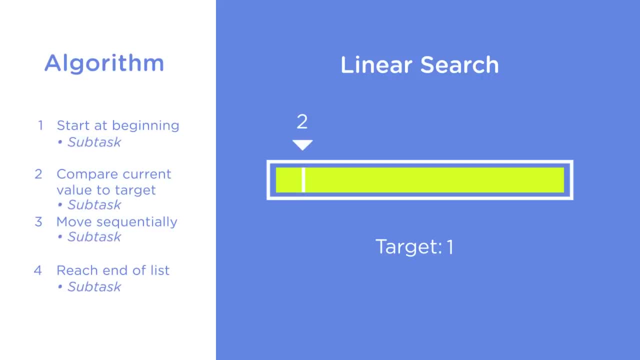 steps further into additional subtasks. Each step needs to be a distinct one. We can't define linear search as search until you find this value, because that can be interpreted in many ways and further broken down into many more steps. It's not clear. 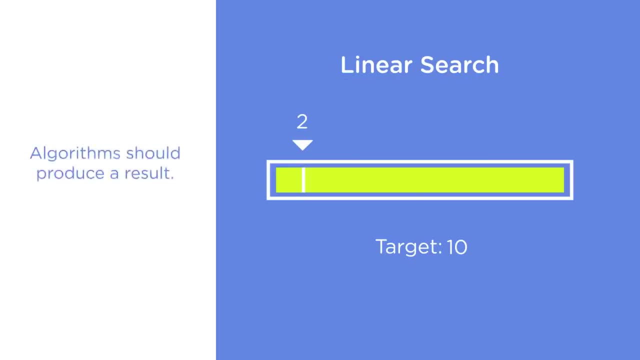 Next, and this one might seem obvious, but algorithms should produce a result. If it didn't, how would we know whether the algorithm works or not? To be able to verify that our algorithm works correctly, we need a result Now when using a search algorithm. 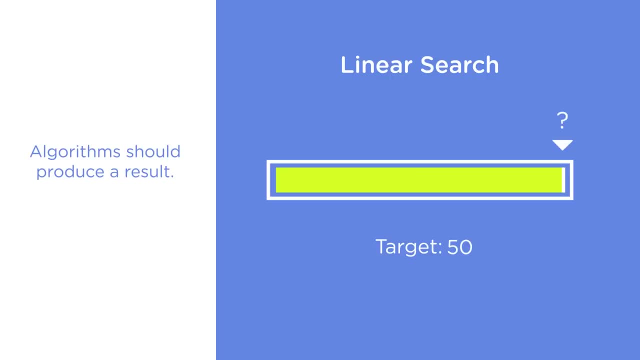 the end result can actually be nothing, which indicates that the value wasn't found, But that's perfectly fine. There are several ways to represent nothing in code, and as long as the algorithm can produce some result, we can understand its behavior. The last guideline is that the 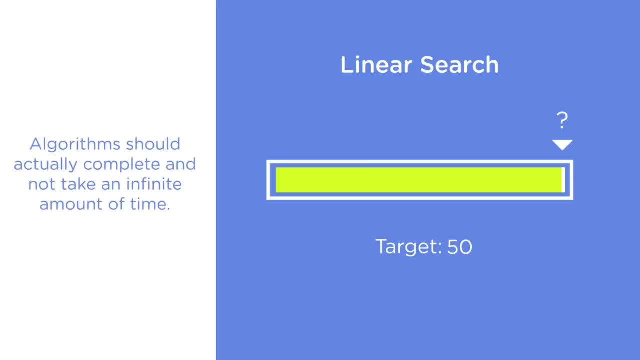 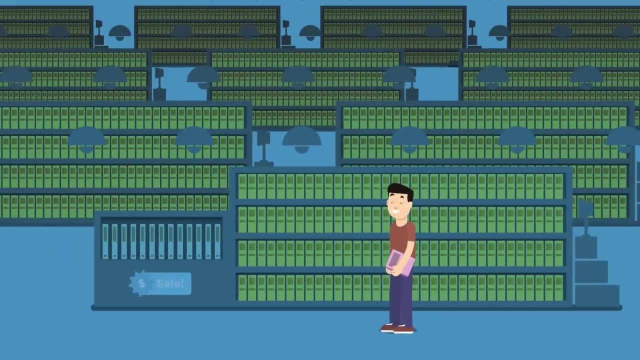 algorithm should actually complete and cannot take an infinite amount of time. If we let John loose in the world's largest library and asked him to find a novel, we have no way of knowing whether he succeeded or not, unless he came back to us with a. 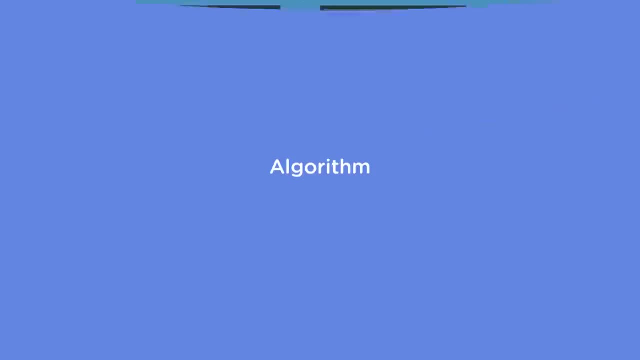 result. Okay, so quick recap What makes an algorithm an algorithm and not just something you do One. it needs to have a clearly defined problem statement, input and output. When using linear search, the input needs to be just a series of values. 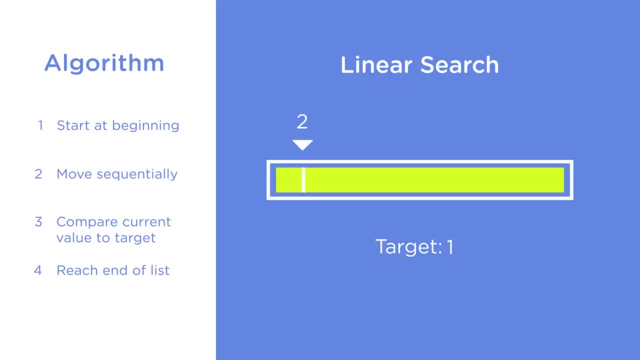 and kind of common sense. The thing is, computers don't know any of that and just do exactly as we tell them, so specific order is really important. The third guideline is that each step in our algorithm definition must not be a complex one and needs to be explicitly clear. 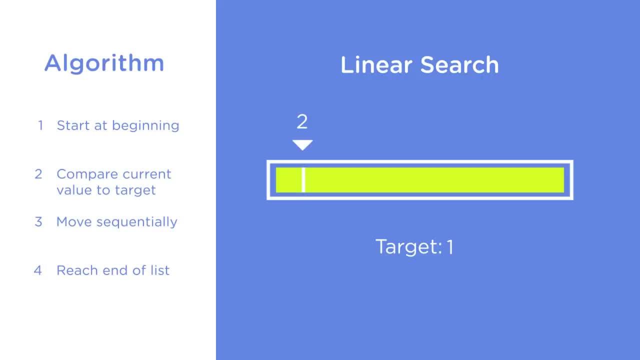 What I mean by that is that you shouldn't be able to break down any of the steps further into additional subtasks. Each step needs to be a distinct one. We can't define linear search as search until you find this value, because that can be interpreted in many ways. 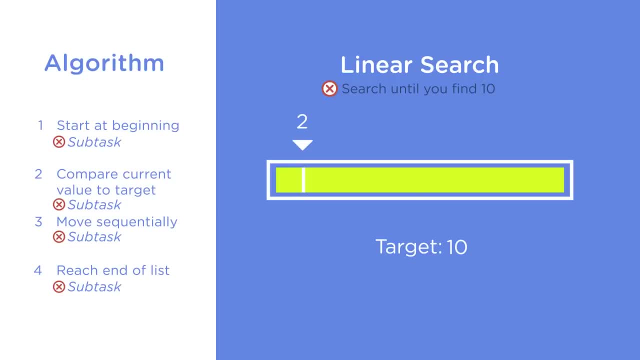 and further broken down. It's not clear. Next, and this one might seem obvious, but algorithms should produce a result. If it didn't, how would we know whether the algorithm works or not? To be able to verify that our algorithm works correctly? 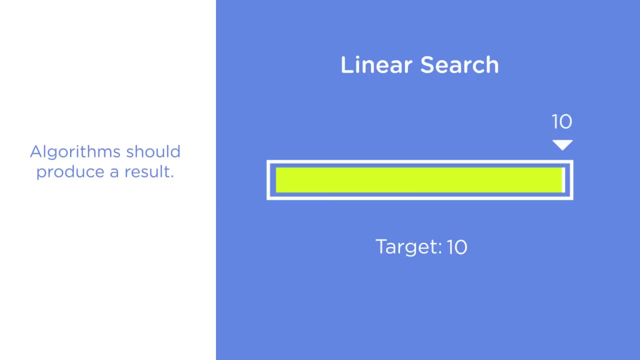 we need a result Now. when using a search algorithm, the end result can actually be nothing, which indicates that the value wasn't found, but that's perfectly fine. There are several ways to represent nothing in code and as long as the algorithm can produce some result, 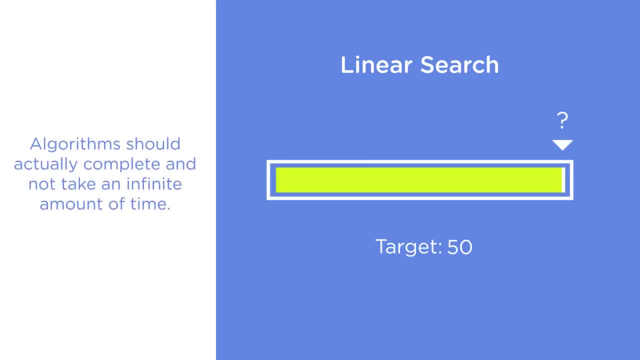 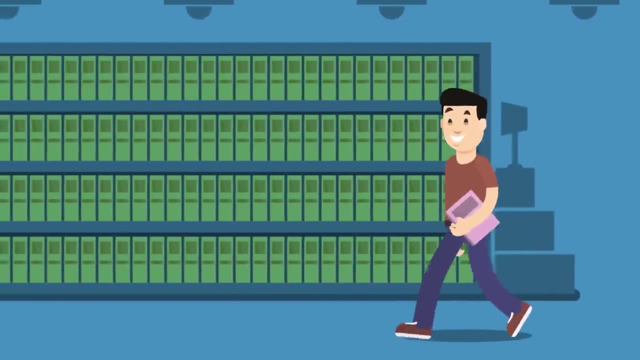 we can understand its behavior. The last guideline is that the algorithm should actually complete and cannot take an infinite amount of time. If we let John loose in the world's largest library and asked him to find a novel, we have no way of knowing whether he succeeded or not. 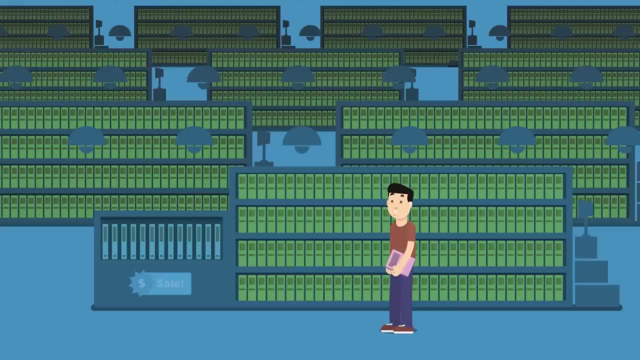 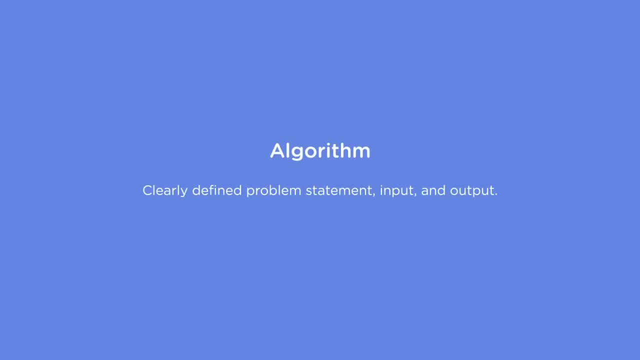 unless he came back to us with a result. Okay, so quick recap What makes an algorithm an algorithm and not just something you do One. it needs to have a clearly defined problem statement, input and output When using linear search. 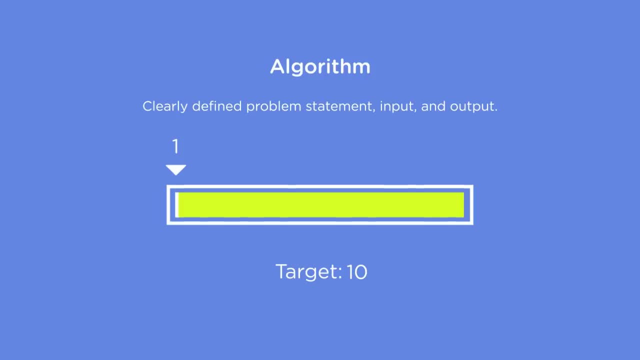 the input needs to be just a series of values. But to actually use Brittany's strategy, there's one additional precondition, so to speak. If you think about her strategy, it required that the numbers be sorted in ascending order. This means that where the input for John 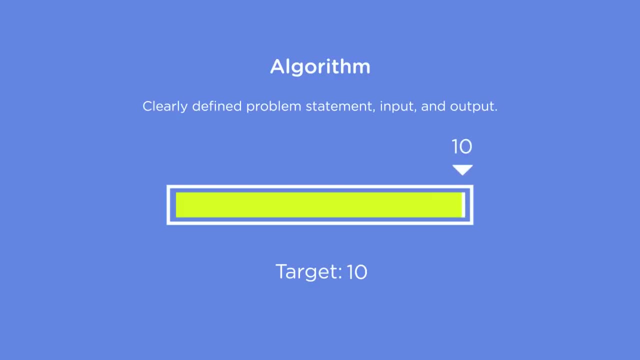 is just a series of values to solve the problem. the input to Brittany's algorithm needs to be a sorted series of values, So clearly defined problem statement, clearly defined input and clearly defined output. Second, the steps in the algorithm need to be in a very specific order. 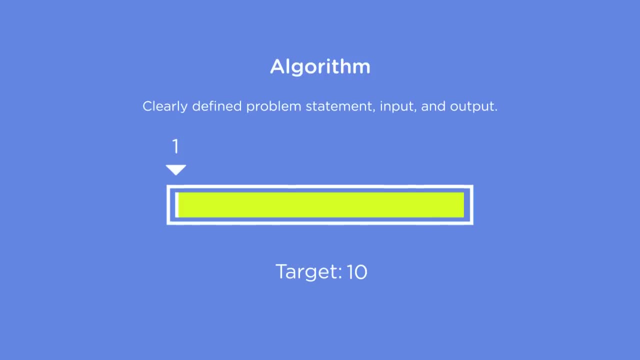 But to actually use Brittany's strategy, there's one additional precondition, so to speak. If you think about her strategy, it required that the numbers be sorted in ascending order. This means that where the input for John is just a series of values to solve, 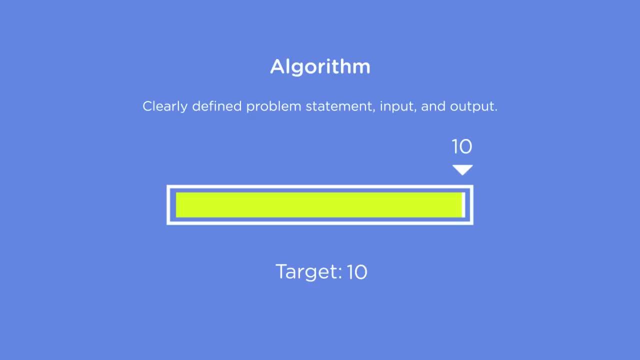 the problem. the input to Brittany's algorithm needs to be a sorted series of values, So clearly defined problem statement, clearly defined input and clearly defined output. Second, the steps in the algorithm need to be in a very specific order. The steps also need to be distinct. 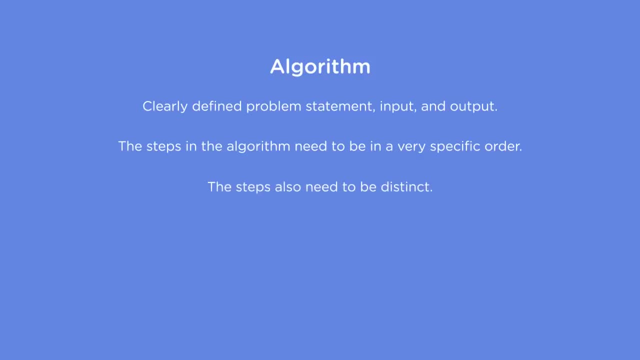 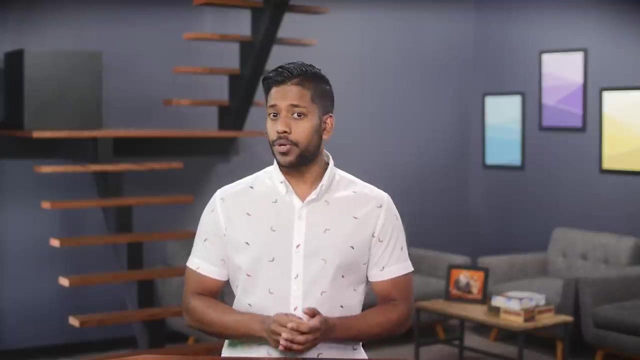 You should not be able to break it down into further subtasks. Next, the algorithm should produce a result And finally, the algorithm should complete in a finite amount of time. These guidelines not only help us define what an algorithm is, but also helps us. 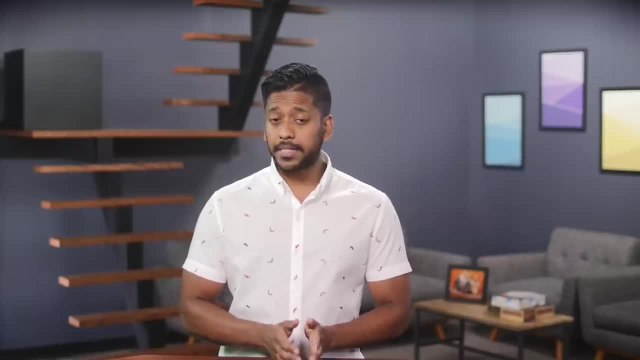 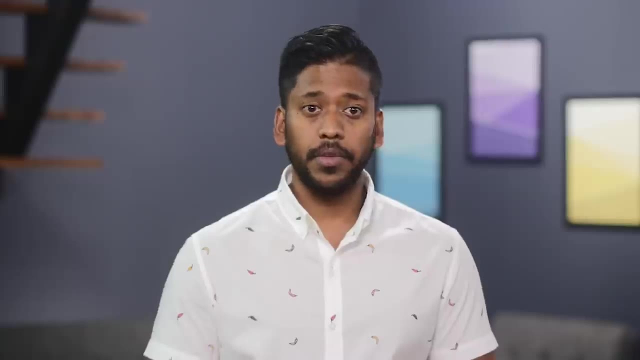 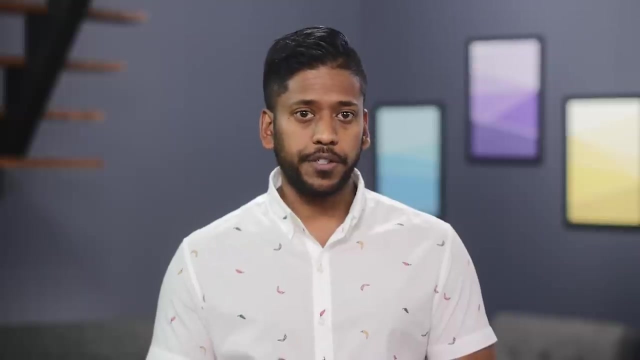 verify that the algorithm is correct. Executing the steps in an algorithm for a given input must result in the same output every time. If, in the game I play, the answer was 50 every time, then every single time John must take 50 turns. 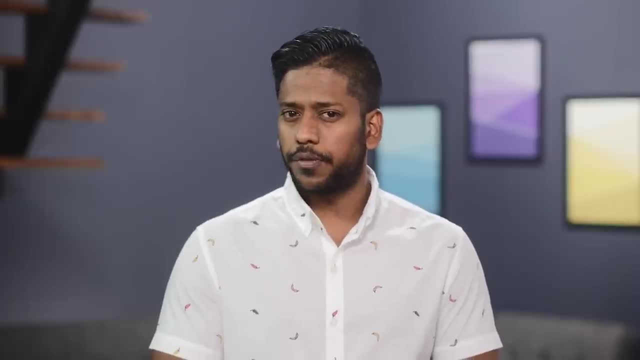 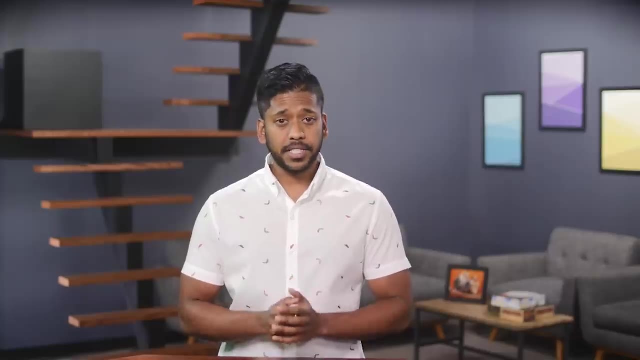 to find out that the answer is 50. If somehow he takes 50 turns in one round, then 30 the next, then we technically don't have a correct algorithm. Consistent results for the same set of values is how we know that the algorithm. 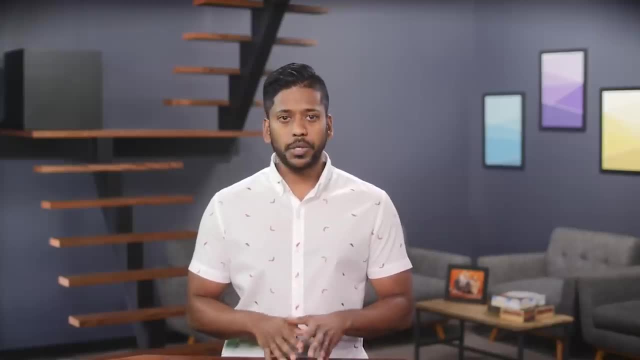 is correct. I should stress that we're not going to be designing any algorithms on our own, and we'll start off and spend most of our time learning the tried and true algorithms that are known to efficiently solve problems. The reason for talking about what makes for a good. 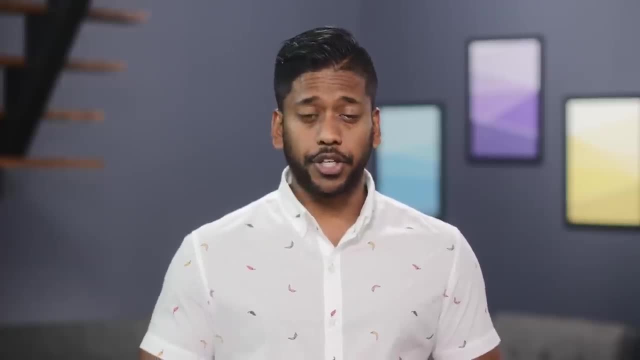 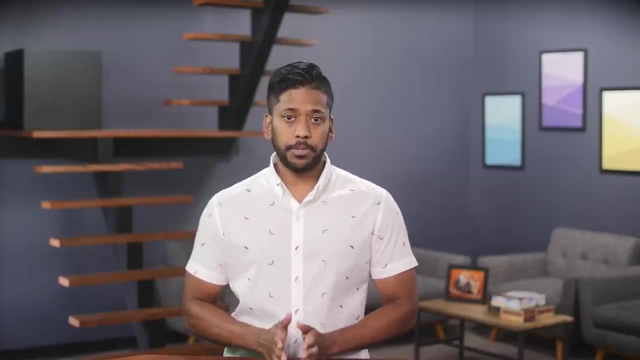 algorithm, though, is that the same set of guidelines makes for good algorithmic thinking, which is one of the most important skills we want to cultivate. When we encounter a problem, before rushing in and thinking about solutions, what we want to do is work through the guidelines. 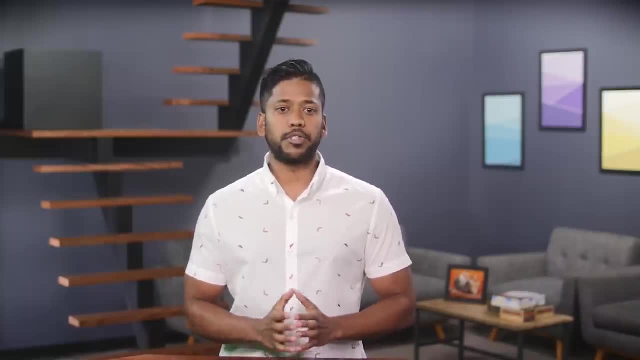 First, we break down the problem into any possible number of smaller problems, where each problem can be clearly defined in terms of an input and an output. Now that we know how to generally define an algorithm, let's talk about what it means to have a good algorithm. 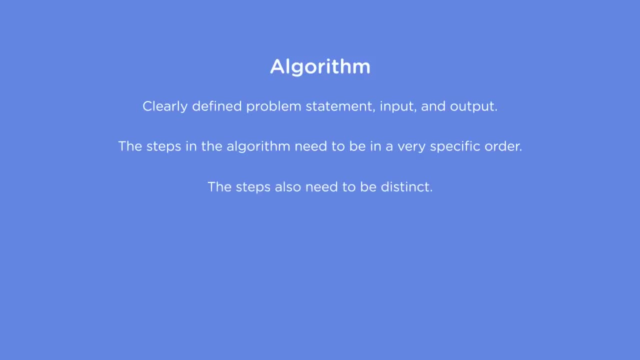 The steps also need to be distinct. You should not be able to break it down into further subtasks. Next, the algorithm should produce a result And finally, the algorithm should complete in a finite amount of time. These guidelines not only help us define. 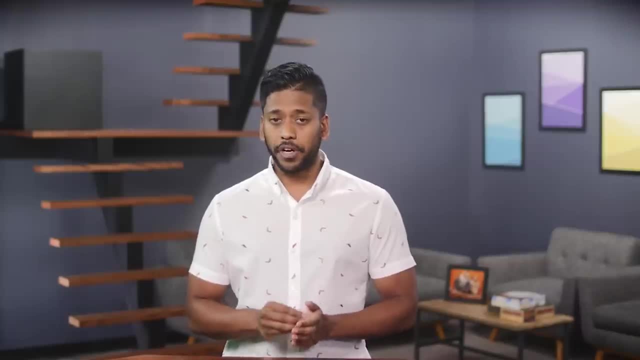 what an algorithm is, but also helps us verify that the algorithm is correct. Executing the steps in an algorithm for a given input must result in the same output every time. If, in the game I played, the answer was 50 every time. 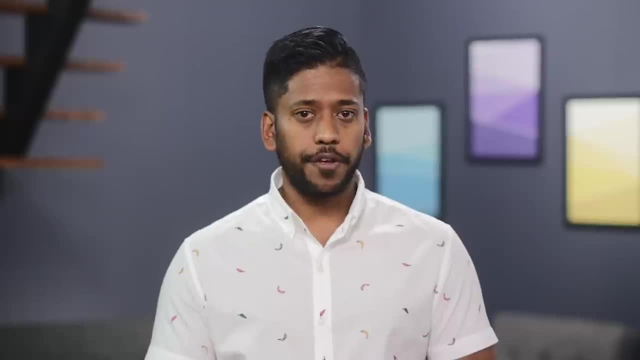 then every single time John must take 50 turns to find out that the answer is 50. If somehow he takes 50 turns in one round, then 30 the next, then we technically don't have a correct algorithm: Consistent results for the same set of values. 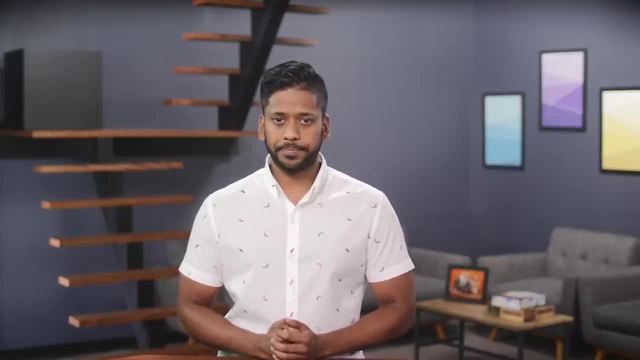 is how we know that the algorithm is correct. I should stress that we're not going to be designing any algorithms on our own, and we'll start off and spend most of our time learning the tried and true algorithms that are known to efficiently solve problems. 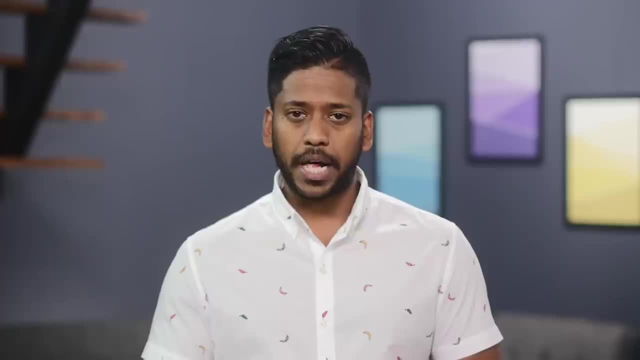 The reason for talking about what makes for a good algorithm, though, is that the same set of guidelines makes for good algorithmic thinking, which is one of the most important skills we want to cultivate When we encounter a problem, before rushing in and thinking about it. 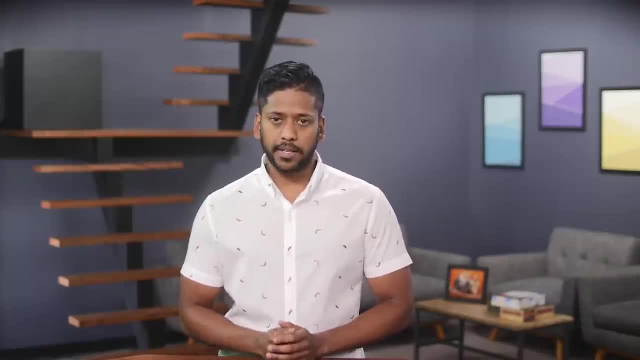 or thinking about solutions. what we want to do is work through the guidelines. First, we break down the problem into any possible number of smaller problems, where each problem can be clearly defined in terms of an input and an output. Now that we know how to generally define an algorithm, 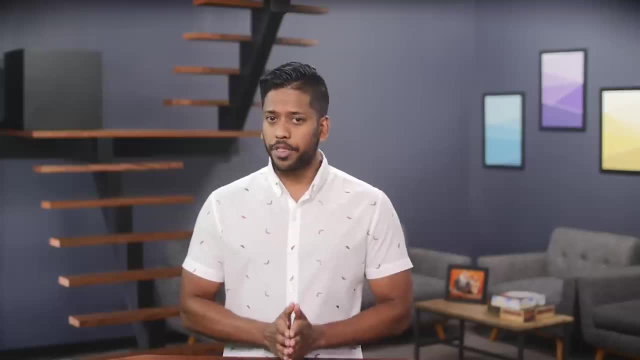 let's talk about what it means to have a good algorithm. An important thing to keep in mind is that there's no one single way to measure whether an algorithm is the right solution, because it is all about context. Earlier, we touched on two concepts. 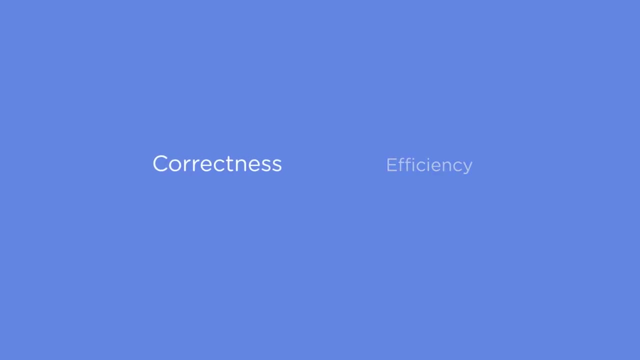 correctness and efficiency. Let's define correctness more clearly, because before we can evaluate an algorithm on efficiency, we need to ensure its correctness. Before we define our algorithms, we start by defining our problem. In the definition of that problem, we have a clearly defined input. 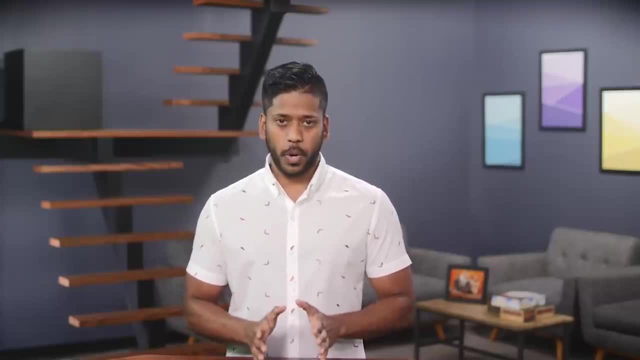 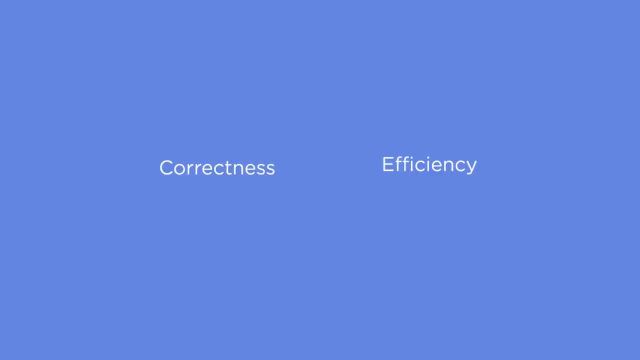 An important thing to keep in mind is that there's no one single way to measure whether an algorithm is the right solution, because it is all about context. Earlier we touched on two concepts: correctness and efficiency. Let's define correctness more clearly, because before we can evaluate an 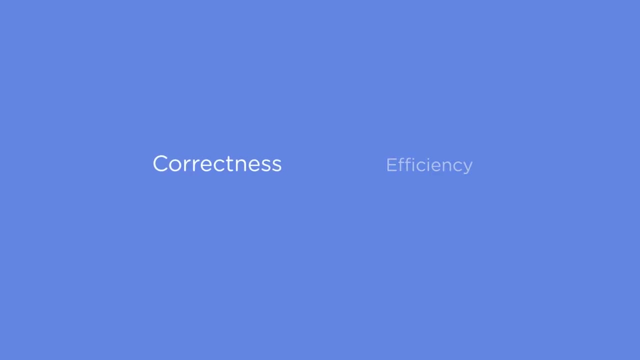 algorithm on efficiency, we need to ensure its correctness. Before we define our algorithms, we start by defining our problem. In the definition of that problem, we have a clearly defined input, satisfying any preconditions, and a clearly defined output. An algorithm is deemed correct if on. 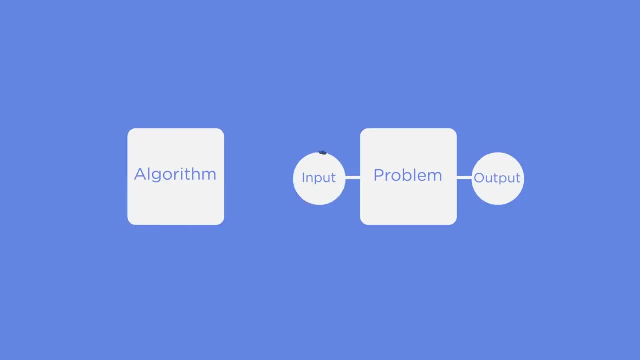 every run of the algorithm against all possible values in the input data, we always get the output we expect. Part of correctness means that for any possible input the algorithm should always terminate or end. If these two are not true, then our algorithm isn't correct. If you. 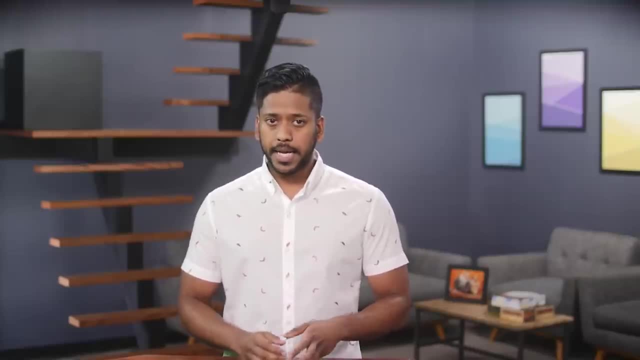 were to pick up an algorithm's textbook and look up correctness, you will run into a bunch of mathematical theory. This is because, traditionally, algorithm correctness is proved by mathematical induction, which is a form of reasoning used in mathematics to verify that a statement is correct. 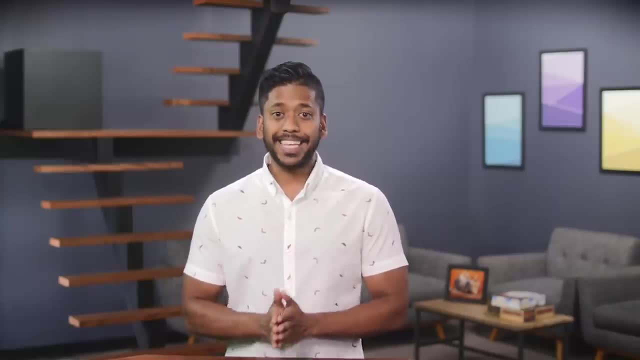 This approach involves writing what is called a specification and a correctness proof. We won't be going into that in this course. Proof through induction is an important part of designing algorithms, but we're confident that you can understand algorithms, both in terms of how. 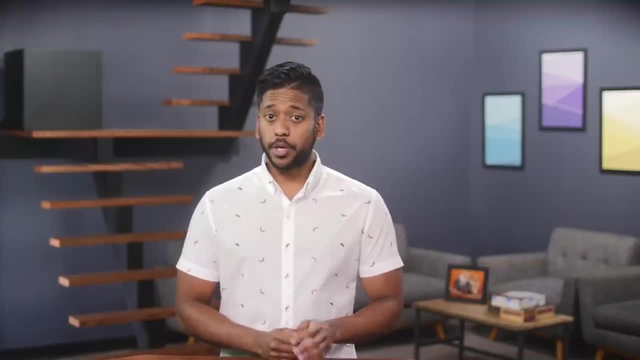 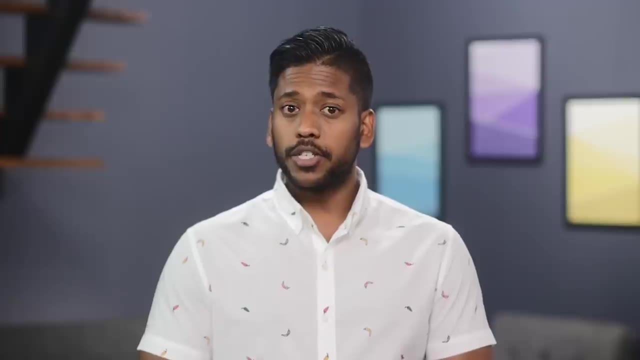 and when to use them, without getting into the math. So if you pick up a textbook and feel daunted, don't worry, I do too, but we can still figure things out without it. Alright, so once we have a correct algorithm, we can start to talk about how efficient an algorithm is. Remember that this efficiency, ultimately, can be achieved by combining that value with the range of values from 1 to n. again Doing it this way, for each value in the range of 1 to n, we create: an n number of values and we end up with 16 points, which is also n times n or n squared. This is an algorithm with a quadratic runtime, because for any given value of n, we carry out n squared number of operations. Now I picked a. relatively easy, so to speak, example here, because in English at least, we often denote map sizes by height, times, width. so we would call this a 4 by 4 grid, which is just another way of saying 4 squared or n squared. In big O notation, we would write this as big O of n squared, or say that this is an algorithm with a quadratic runtime. Many search algorithms have a worst case, quadratic runtime, which you'll learn about soon. Now, in addition to quadratic, runtimes. you may also run into cubic runtimes as you encounter different algorithms. In such an algorithm, for a given value of n, the algorithm executes n raised to the third power number of operations. These aren't as common as quadratic algorithms, though, so we won't. look at any examples, but I think it's worth mentioning Thrown up on our graph. quadratic and cubic runtimes look like this: So this is starting to look pretty expensive computationally, as they say. We can see here that for small changes in n. there's a pretty significant change in the number of operations that we need to carry out. The next worst case runtime we're going to look at is one that's called quasi-linear and is sort of easier to understand, for lack of a better word. by starting with the big O notation. Quasi-linear runtimes are written out as big O of n times, log n. We learned what log n was right: A logarithmic runtime. whereas n grew, the number of operations only increased by a small. factor With a quasi-linear runtime. what we're saying is that for every value of n we're going to execute a log n number of operations, hence the runtime of n times log n. So you saw earlier with the quadratic runtime that for each value of n, we conducted n operations. It's sort of the same in that as we go through the range of values in n, we're executing log n operations. In comparison to other runtimes, a quasi-linear algorithm has a runtime that lies. somewhere between a linear runtime and a quadratic runtime. So where would we expect to see this kind of runtime in practical use? Well, sorting algorithms is one place. you will definitely see it. Mergesort, for example, is a sorting algorithm that has a worst. 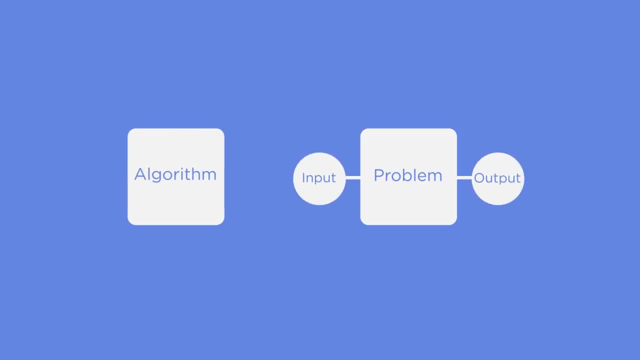 satisfying any preconditions and a clearly defined output. An algorithm is deemed correct if on every run of the algorithm against all possible values in the input data, we always get the output we expect. Part of correctness means that for any possible input the algorithm should always terminate or end. 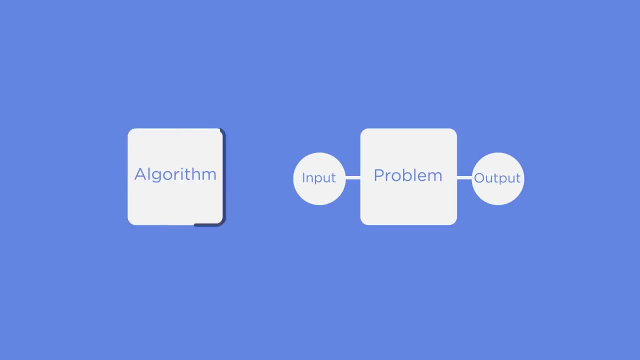 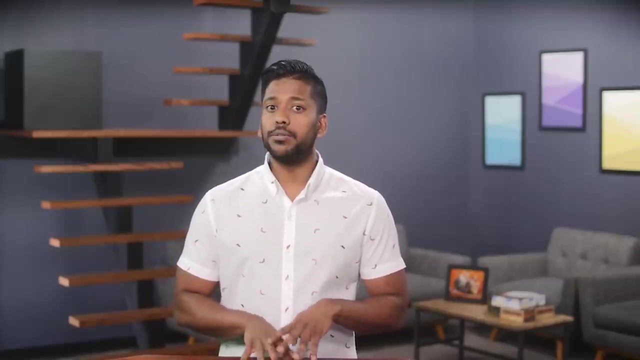 If these two are not true, then our algorithm isn't correct. If you were to pick up an algorithm's textbook and look up correctness, you will run into a bunch of mathematical theory. This is because, traditionally, algorithm correctness is proved by mathematical induction. 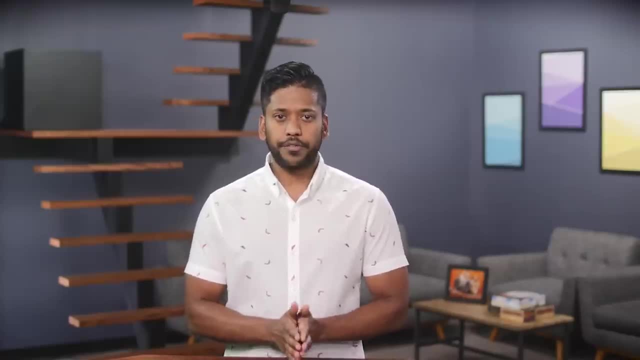 which is a form of reasoning used in mathematics to verify that a statement is correct. This approach involves writing what is called a specification and a correctness proof. We won't be going into that in this course. Proof through induction is an important part of designing algorithms. 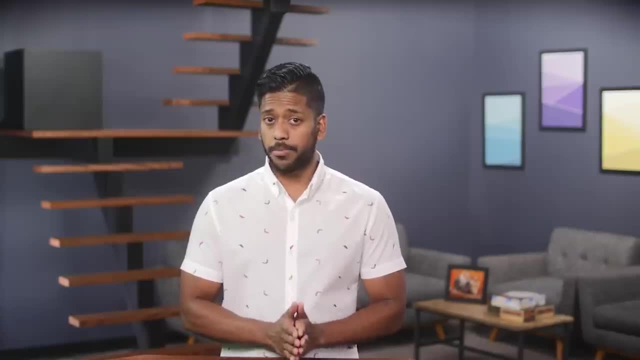 but we're confident that you can understand algorithms, both in terms of how and when to use them, without getting into the math. So if you pick up a textbook and feel daunted, don't worry, I do too, but we can still figure things out without it. 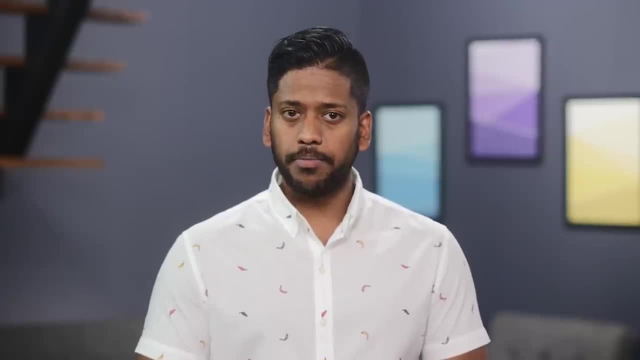 Alright. so once we have a correct algorithm, we can start to talk about how efficient an algorithm is. Remember that this efficiency ultimately matters because they help us solve problems faster and deliver a better end-user experience in a variety of fields. For example, algorithms are used in the sequencing of DNA. 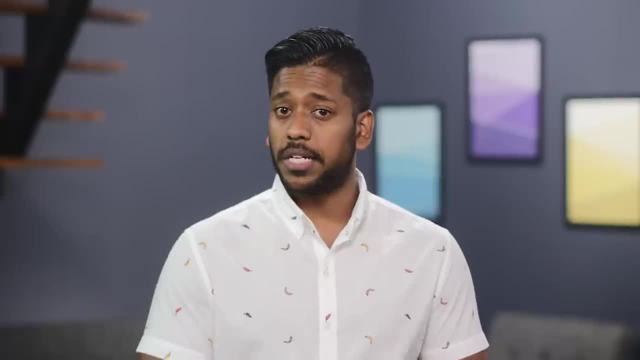 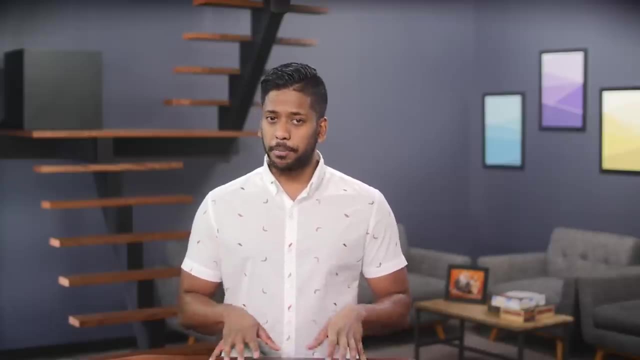 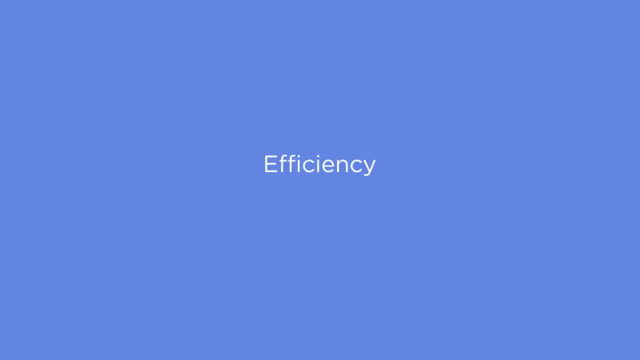 and more efficient sequencing algorithms allow us to research and understand diseases better and faster. But let's not get ahead of ourselves. We'll start simple, by evaluating John's linear search algorithm in terms of its efficiency. First, what do we mean by efficiency? 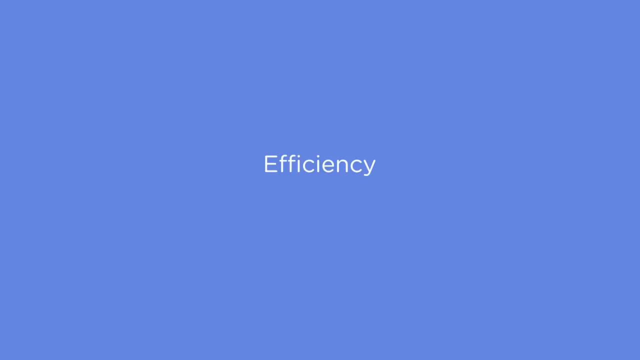 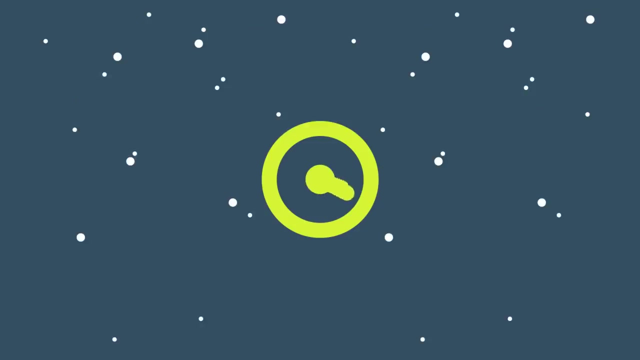 There are two measures of efficiency when it comes to algorithms: time and space. Sounds really cool and very sci-fi, huh. Efficiency measured by time- something you'll hear called time complexity- is a measure of how long it takes the algorithm to run. 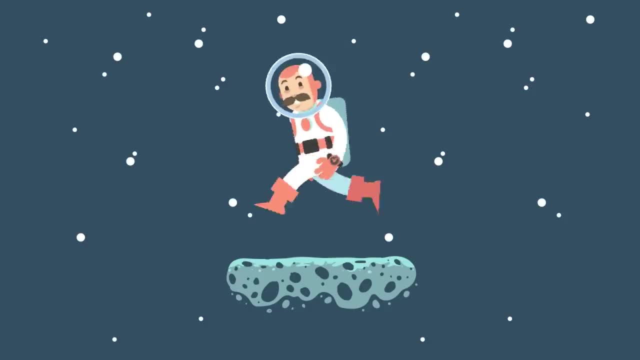 Time complexity can be understood generally, outside the context of code and computers, because how long it takes to complete a job is a universal measure of efficiency. The less time you take, the more efficient you are. The second measure of efficiency is called space complexity. 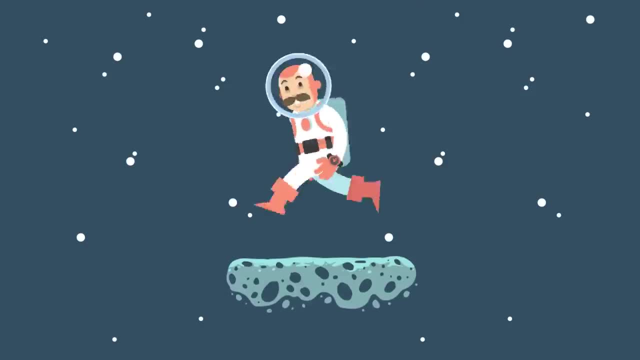 and this is pretty computer-specific. It deals with the amount of memory taken up on the computer. Good algorithms need to balance between these two measures to be useful. For example, you can have a blazingly fast algorithm, but it might not matter if the algorithm 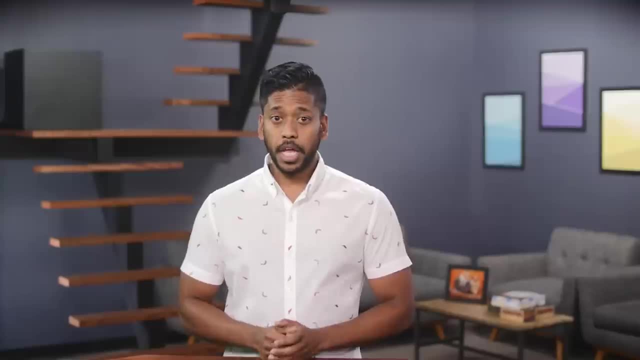 consumes more memory than you have available. Both of these concepts- time and space complexity- are measured using the same metric, But it is a very technical-sounding metric, so let's build up to it slowly and start simple. A few videos ago, I played a game. 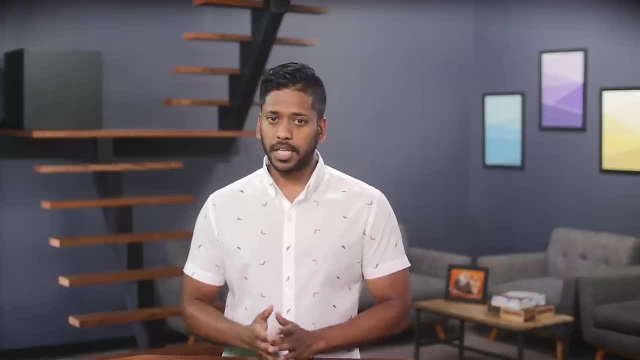 with Brittany and John, where they tried to guess the number I was thinking of. Effectively, they were searching for a value. So how do we figure out how efficient each algorithm is and which algorithm was more suited to our purposes, If we consider the number of tries they took? 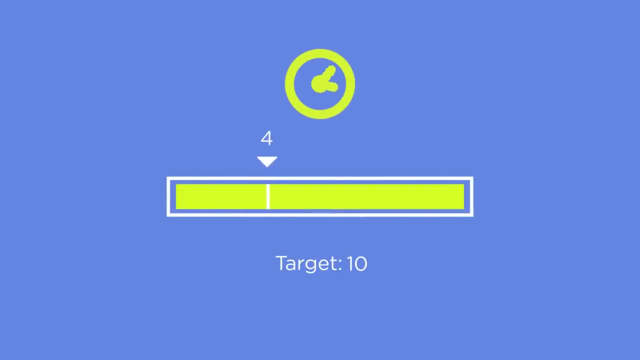 to guess or search for the value as an indicator of the time they take to run through the exercise. this is a good indicator of how long the algorithm runs for a given set of values. This measurement is called the running time of an algorithm and we'll use it to define time complexity. 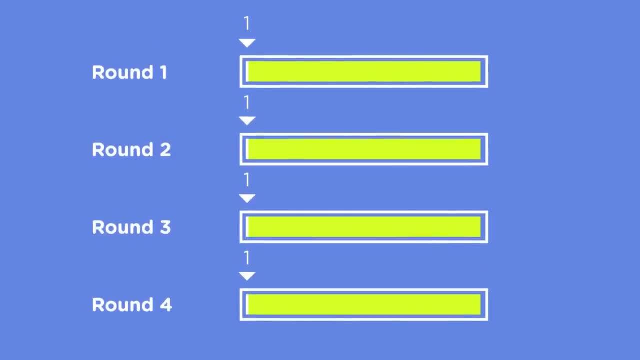 In the game we played four rounds. Let's recap those here, focusing on John's performance. In round 1, we had 10 values, the target was 3, and John took 3 turns. In round 2, we had 10 values. 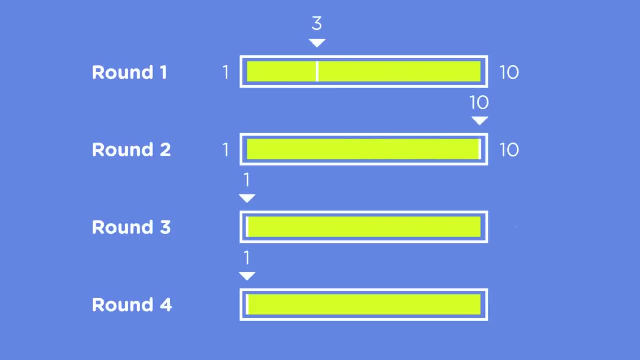 the target was 10, and John took 10 turns. In round 3, we had 100 values, the target was 5,, John took 5 tries And finally, in round 4, when the target was 100,. 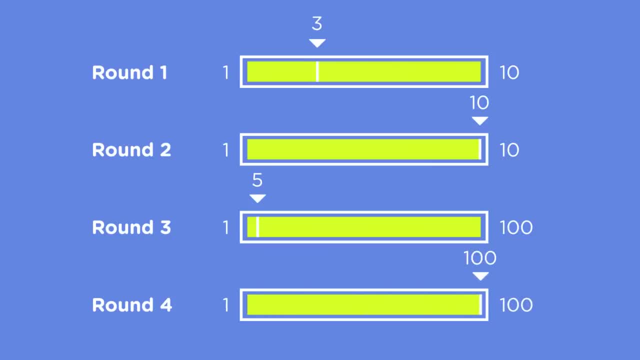 given 100 values. John took 100 tries On paper. it's hard to gauge anything about this performance. When it comes to anything with numbers, though, I like to put it up on a graph so we can compare visually On the vertical or y-axis. 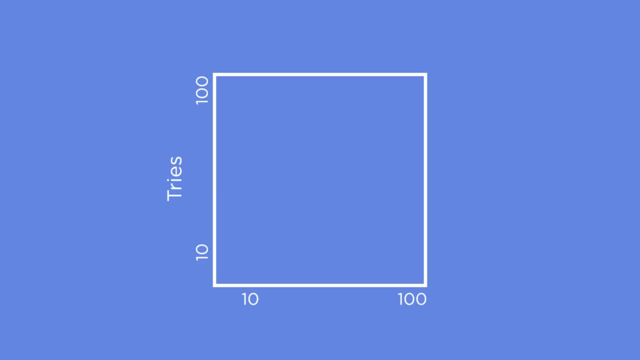 let's measure the number of tries it took John to guess the answer, or the running time of the algorithm On the horizontal or x-axis. what do we put For each turn? we have a number of values, as well as a target value. 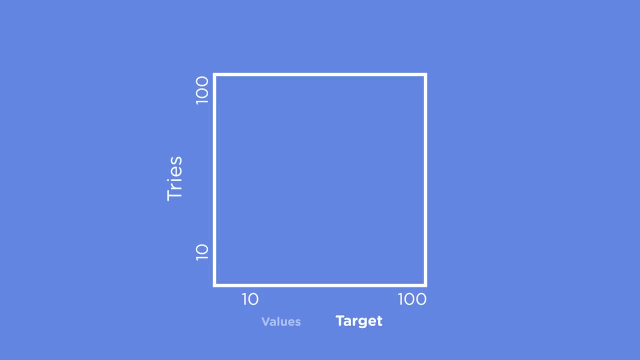 We could plot the target value on the horizontal axis, but that leaves some context and meaning behind. It's far more impressive that John took 5 tries when the range went up to 100 than when he took 3 tries for a maximum of 10 values. 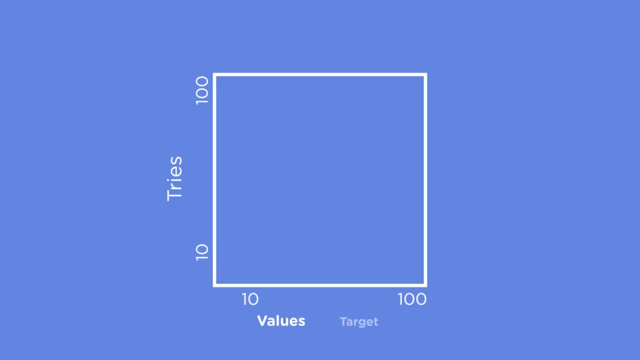 We could plot the maximum range of values, but then we're leaving out the other half of the picture. There are data points, however, that satisfy both requirements If we only plot the values where the target, the number John was looking for. 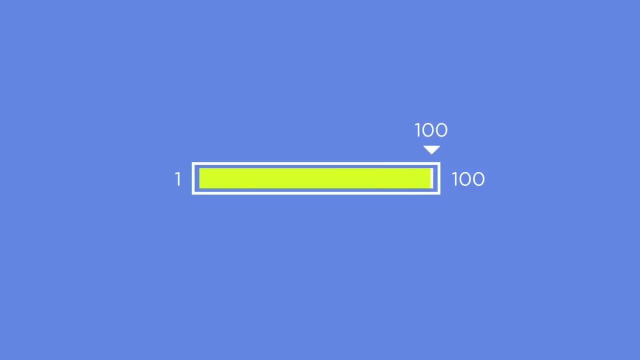 was the same as the maximum range of values. we have a data point that includes both the size of the data set as well as his effort. There's an additional benefit to this approach as well. There are three ways we can measure how well John does. 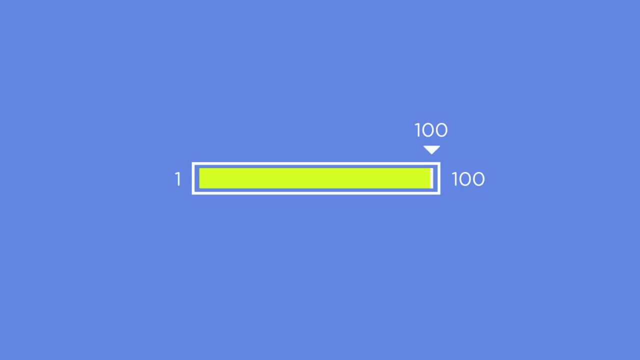 or, in general, how well any algorithm does. First we can check how well John does in the best case or good scenarios, from the perspective of his strategy, In the range of 100 values, the answer being a low number like 3 at the start of the range. 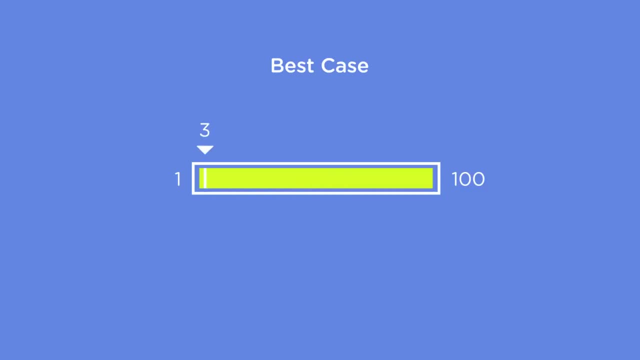 is a good scenario. He can guess it fairly quickly. 1 is his best case scenario, Or we could check how well he does on average. We could run this game a bunch of times and average out the running time. This would give us a much better picture. 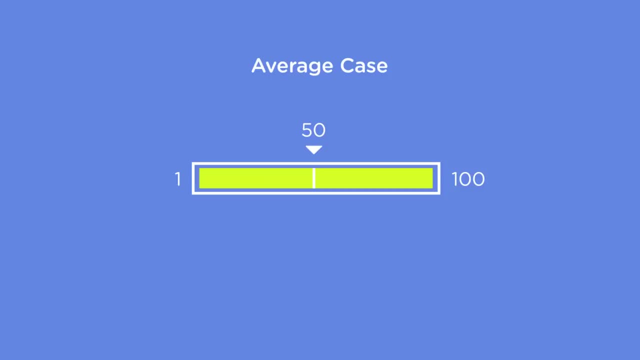 of John's performance over time, but our estimates would be too high if the value he was searching for was at the start of the range, or far too low if it was at the end of the range. Let's imagine a scenario where Facebook naively implements: 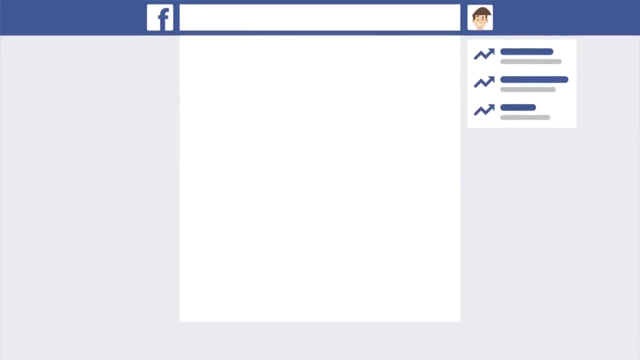 linear search when finding friends. They looked at the latest US census, saw that 50% of names start with the letters A through J, which is the first 40% of the alphabet, And thought, OK, on average, linear search serves us well. 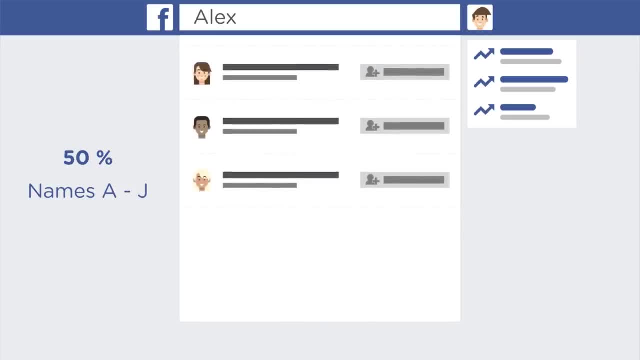 But what about the rest of those whose names start with the letter after J in the alphabet? Searching for my name would take longer than the average, and much longer for someone whose name starts with the letter Z. So, while measuring the run time of an algorithm on average, 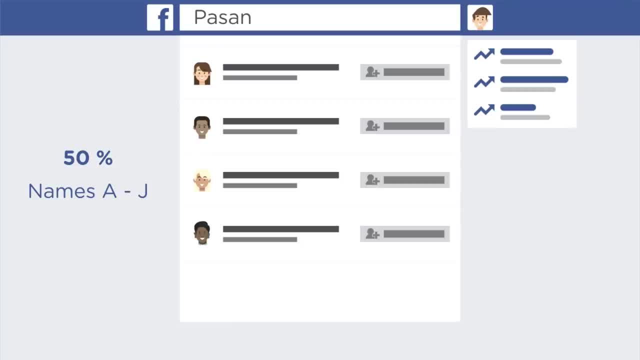 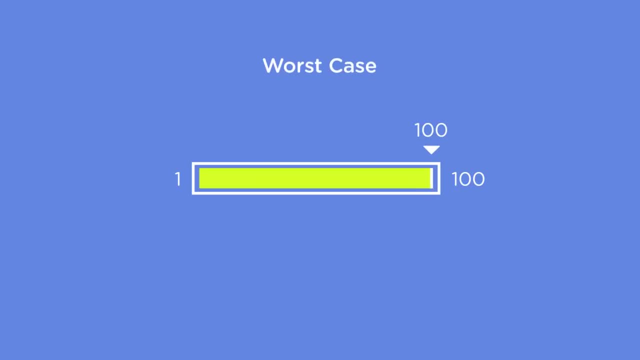 might seem like a good strategy, it won't necessarily provide an accurate picture. By picking the maximum in the range, we're measuring how our algorithm does in the worst case scenario. Analyzing the worst case scenario is quite useful because it indicates that the algorithm 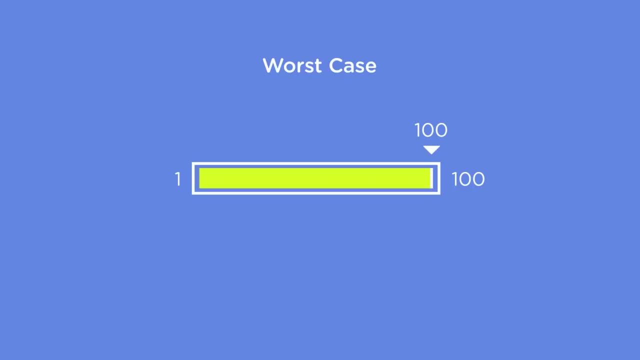 will never perform worse than we expect. There's no room for surprises. Back to our graph. we're going to plot the number of tries, a proxy for running time of the algorithm, against the number of values in the range which will shorten to n. 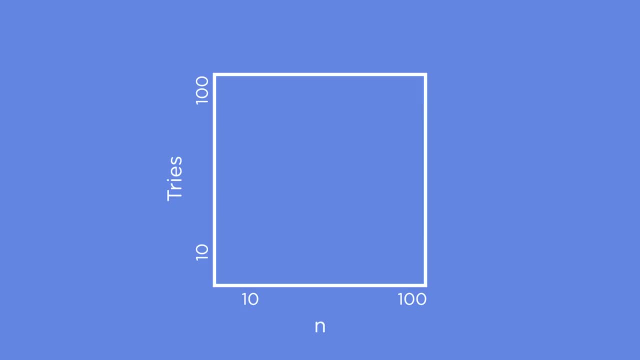 n here also represents John's worst case scenario: When n is 10, he takes 10 turns. When n is 100, he takes 100 turns. But these two values alone are insufficient to really get any sort of visual understanding. Moreover, it's not realistic. 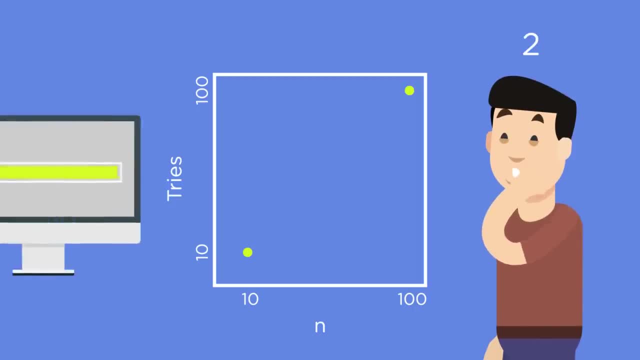 John may take a long time to work through 100 numbers, but a computer can do that in no time. To evaluate the performance of linear search in the context of a computer, we should probably throw some harder and larger ranges of values at it. 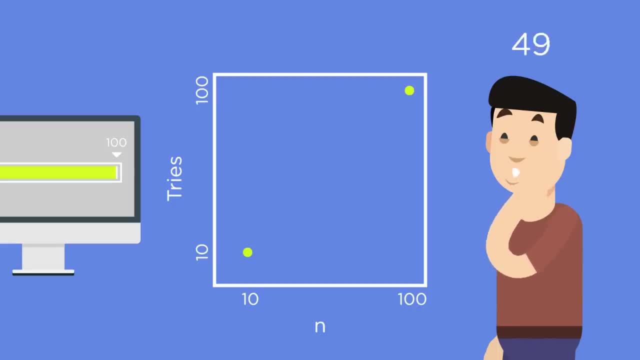 The nice thing is, by evaluating a worst case scenario, we don't actually have to do that work. We know what the result will be For a given value of n. using linear search, it will take n tries to find the value in the worst case scenario. 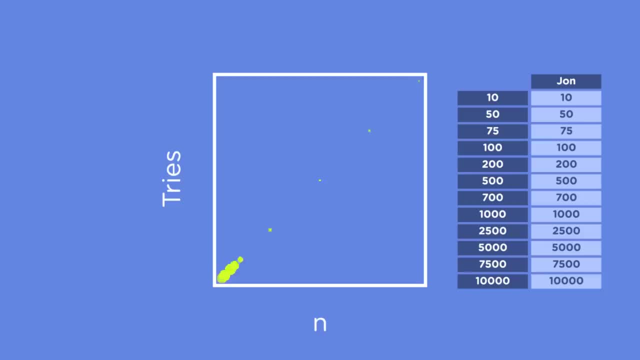 So let's add a few values in here to build out this graph. Okay, so we have a good picture of what this is starting to look like. As the values get really large, the running time of the algorithm gets large as well. 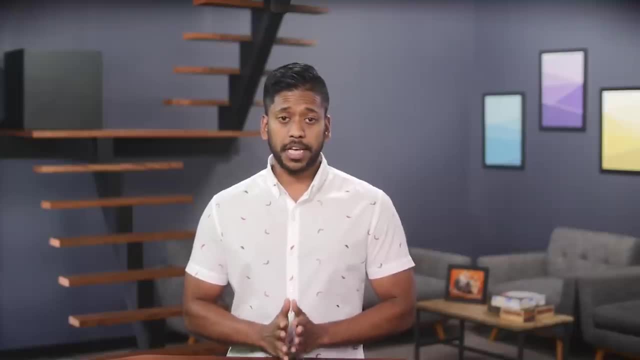 Well, we sort of already knew that. Before we dig into this run time any deeper, let's switch tracks and evaluate Brittany's work. By having something to compare against, it should become easier to build a mental model around time complexity. The algorithm John used. 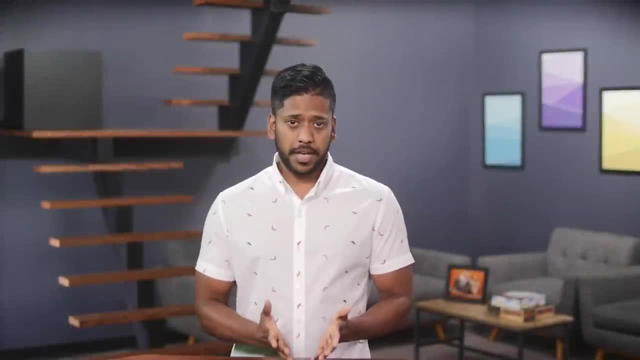 linear search seemed familiar to us, And you could understand it, because it's how most of us search for things in real life anyway. Brittany's approach, on the other hand, got results quickly, but it was a bit harder to understand, So let's break it down. 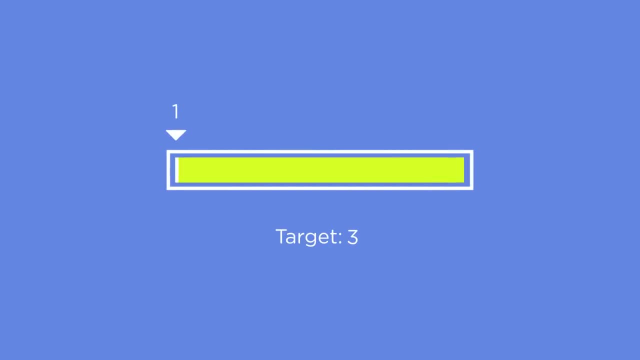 Just like John's approach, Brittany started with a series of values or a list of numbers as her input, Where John just started at the beginning of the list and searched sequentially. Brittany's strategy is to always start in the middle of the range. From there she asks: 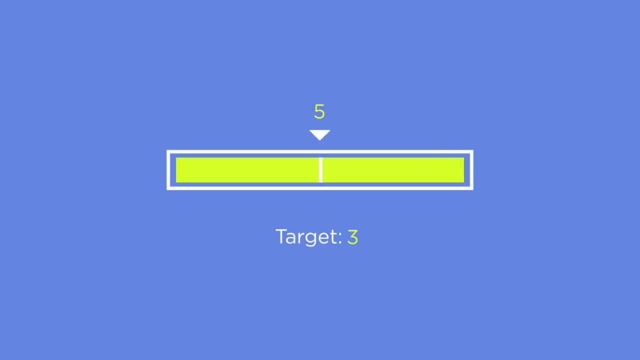 a comparison question. Is the number in the middle of the range equal to the answer she's looking for? And if it's not, is it greater than or less than the answer? If it's greater than, she can eliminate all the values less than the one. 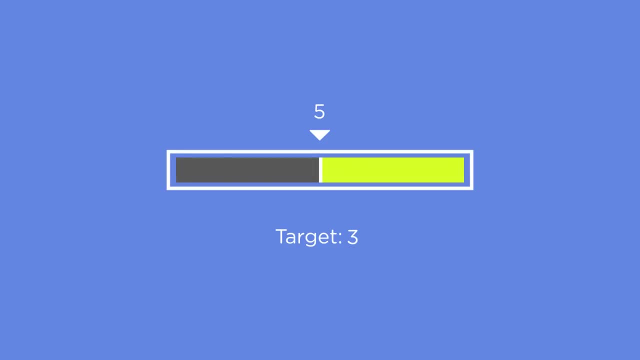 she's currently evaluating. If it's lesser than the answer, she can eliminate all the values greater than the one she's currently evaluating With the range of values that she's left over with. she repeats this process until she arrives at the answer. 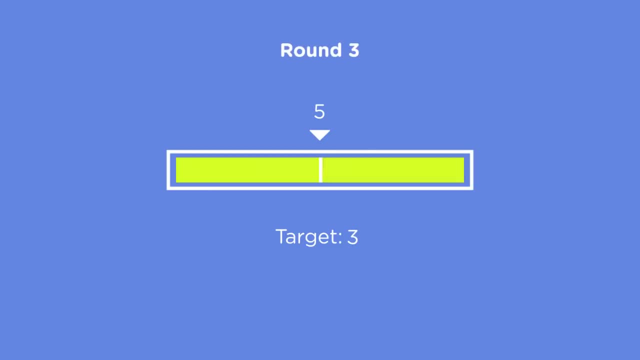 Let's visualize how she did this by looking at round 3.. In round 3, the number of values in the range was 100.. The answer was 5.. The bar here represents the range of values: One at the left, 100 at the right. 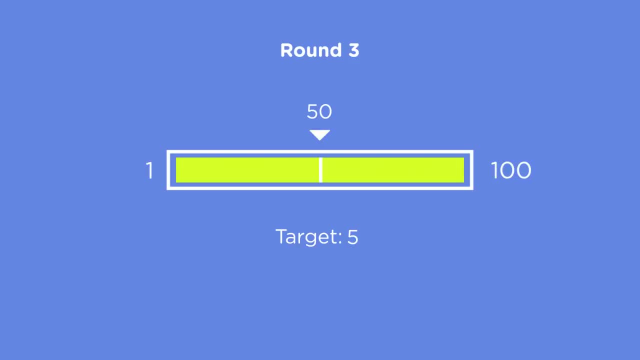 And this pointer represents the value Brittany chooses to evaluate. So she starts in the middle, at 50. She asks: is it equal to the answer? I say it's too high. So this tells her that the value she is evaluating is greater than our target value. 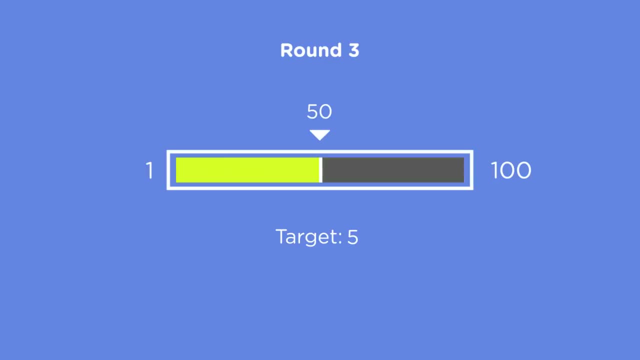 which means there's no point in searching any of the values to the right of 50. That is, values greater than 50 in this range. So she can discard those values altogether. She only has to consider values from 1 to 50 now. 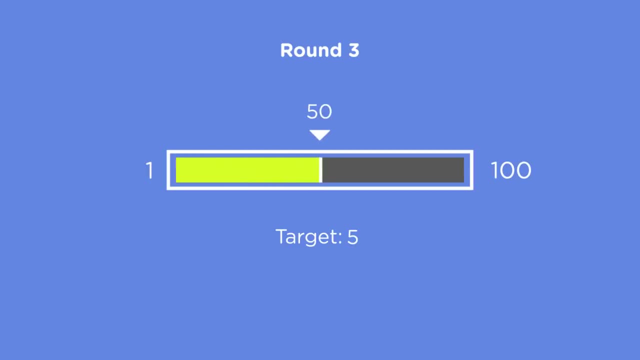 The beauty of this strategy, and the reason why Brittany was able to find the answer in such few turns, is that with every value she evaluates, she can discard half of the current range. On her second turn, she picks the value in the middle of the current range. 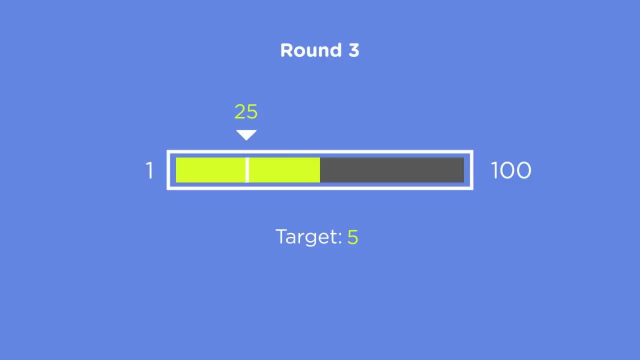 which is 25.. She asks the same question. I say that the value is too high again, and this tells her that she can discard everything greater than 25, and the range of values drops from 1 to 25.. Again, she evaluates. 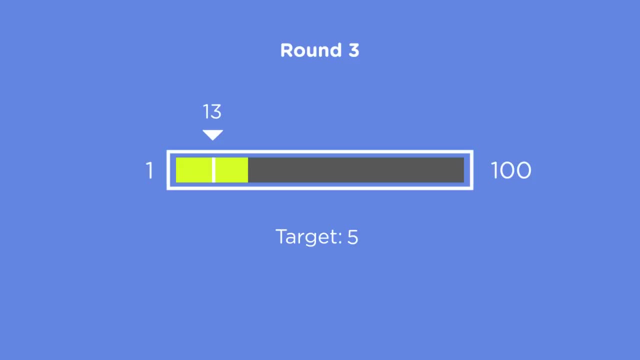 the number in the middle roughly. so that'd be 13 here. I tell her this is still too high. She discards the values greater, moves to value at 7,, which is still too high. Then she moves to 4,. 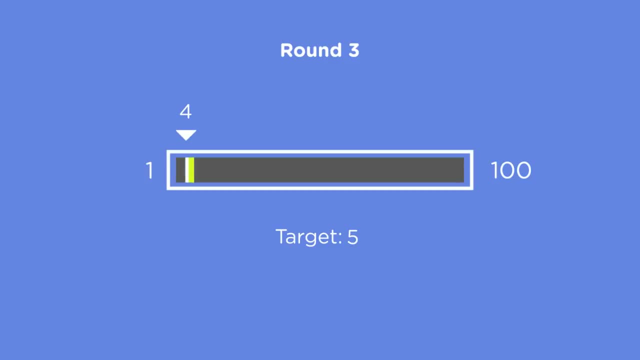 which is now 2.. This is still too low. She can discard everything less than 4,, which leaves the numbers 4 through 7.. Here she picked 6,, which was too high, which only leaves one value: 5.. 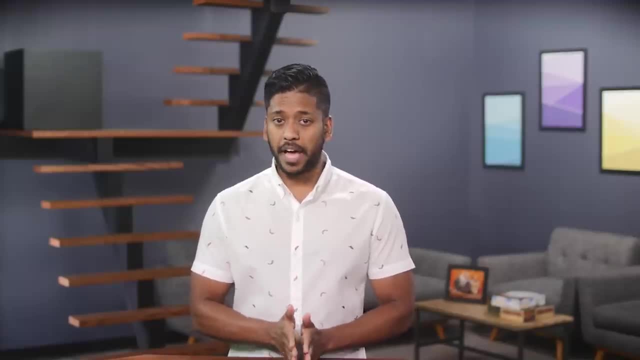 This seems like a lot of work, but being able to get rid of half the values with each turn is what makes this algorithm much more efficient. Now there's one subtlety to using binary search, and you might have caught on to this. 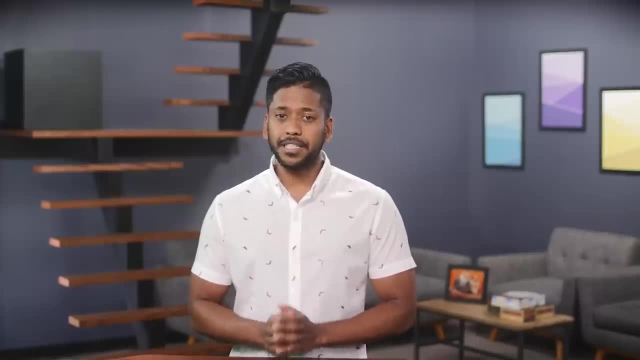 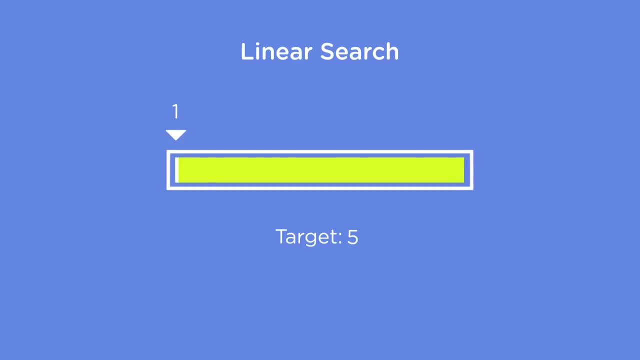 For this search method to work, as we've mentioned, the values need to be sorted. With linear search, it doesn't matter if the values are sorted, Since a linear search algorithm just progresses sequentially, checking every element in the list if the target value exists. 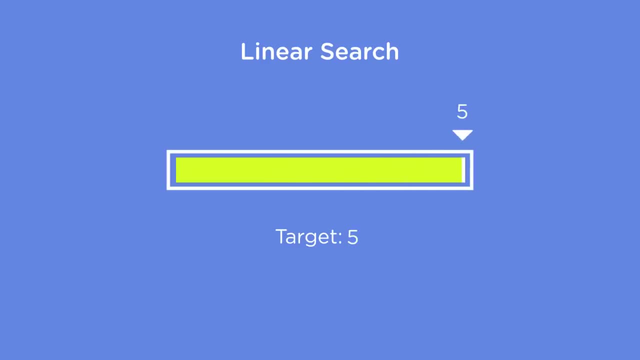 in the list it will be found. But let's say this range of values, 1 to 100, was unsorted. Brittany would start at the middle with something like 14 and ask if this value was too low or too high. I say it's too high. 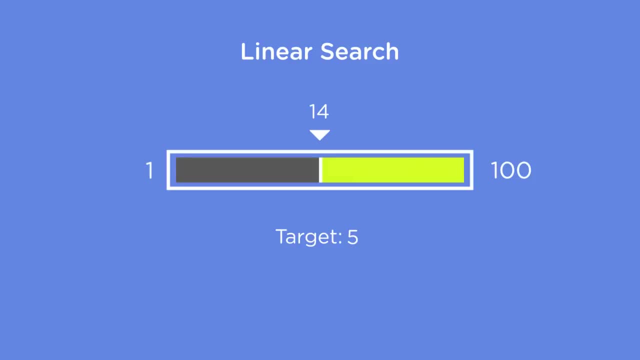 so she discards everything less than 14.. Now this example starts to fall apart here, because while Brittany knows what numbers are less than 14 and greater than 1, she doesn't need an actual range of values to solve this. A computer, however. 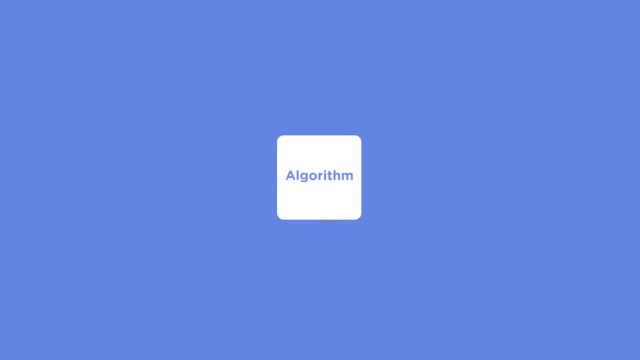 does need that Remember. search algorithms are run against lists containing all sorts of data. It's not always just a range of values containing numbers. In a real use case of binary search, which we're going to implement in a bit, the algorithm wouldn't return. 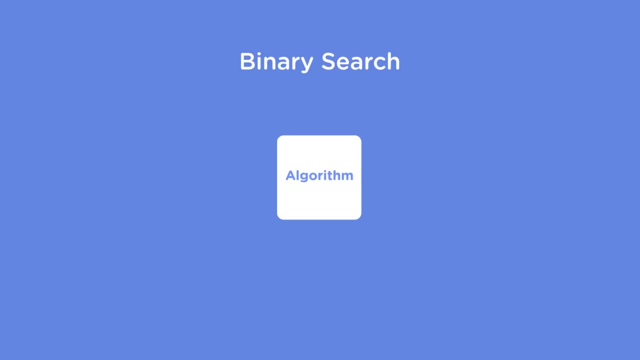 the target value because we already know that It's a search algorithm, so we're providing something to search for. Instead, what it returns is the position in the list that the target occupies, Without the list being sorted. a binary search algorithm would discard all the values. 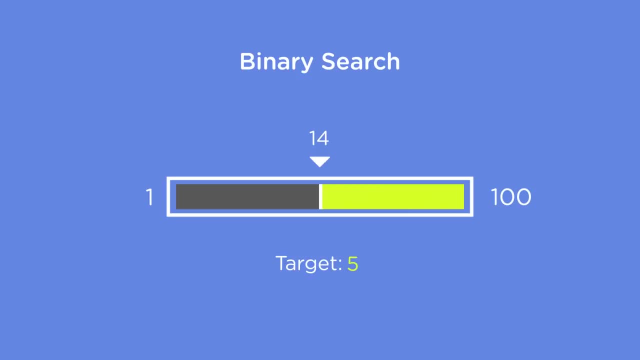 to the left of 14, which over here could include the position where our target value is. Eventually, we'd get a result back saying the target value doesn't exist in the list, which is inaccurate. Earlier when defining linear simple search. 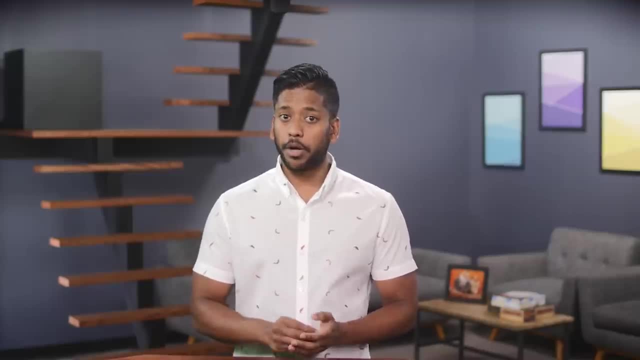 I said that the input was a list of values and the output was the target value or, more specifically, the position of the target value in the list. So with binary search there's also that precondition. The input list must be sorted. So let's formally define. 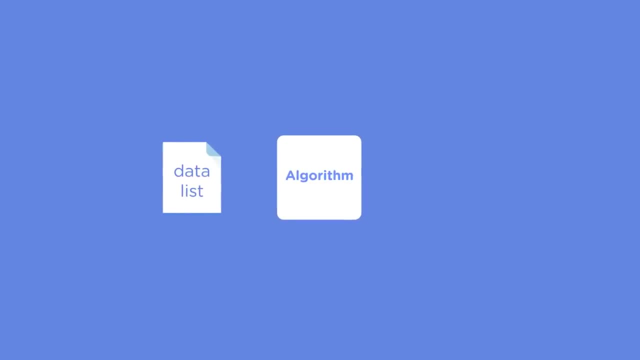 binary search. First, the input: a sorted list of values. The output: the position in the list of the target value we're searching for, or some sort of values indicate that the target does not exist in the list. Remember our guidelines for defining an algorithm. 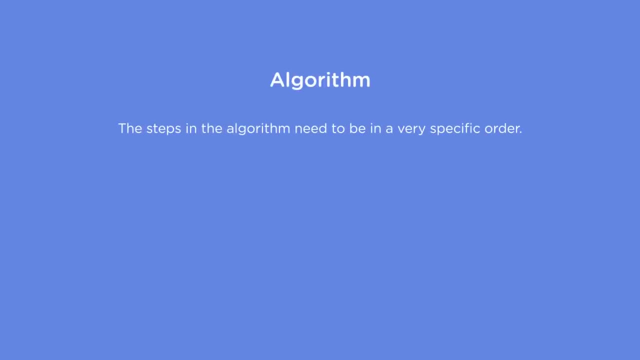 Let me put those up again really quick. The steps in the algorithm need to be in a specific order. The steps also need to be very distinct. The algorithms should produce a result And finally, the algorithm should complete in a finite amount of time. 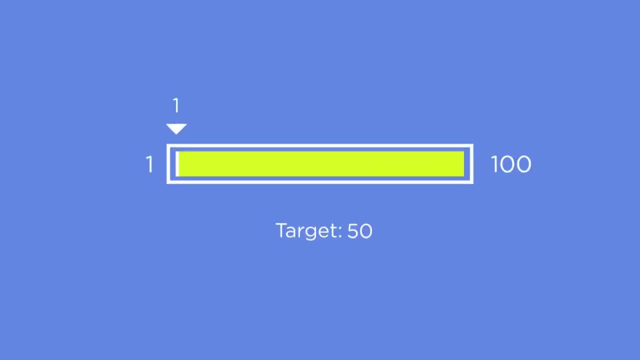 Let's use those to define this algorithm. Step one: we determine the middle position of the sorted list. Step two: we compare the element in the middle position to the target element. Step three: if the elements match, we return the middle position. 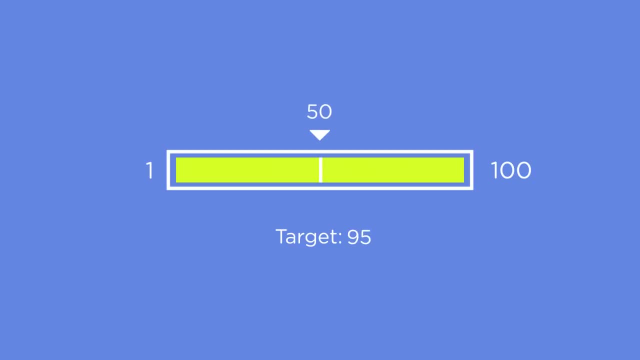 and end If they don't match. in step four we check whether the element in the middle position is smaller than the target element. If it is, then we go back to step two with a new list that goes from the middle position of the current list. 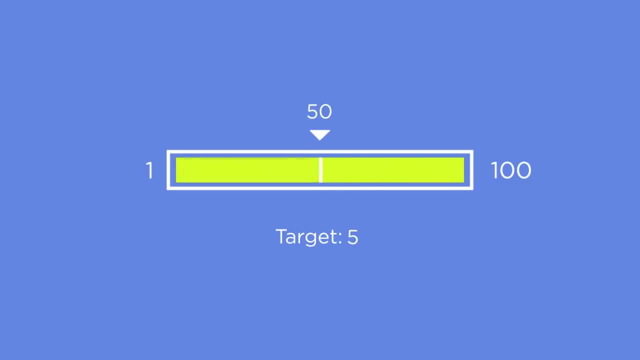 to the end of the current list In step five. if the element in the middle position is greater than the target element, then again we go back to step two with a new list that goes from the start of the current list to the middle position. 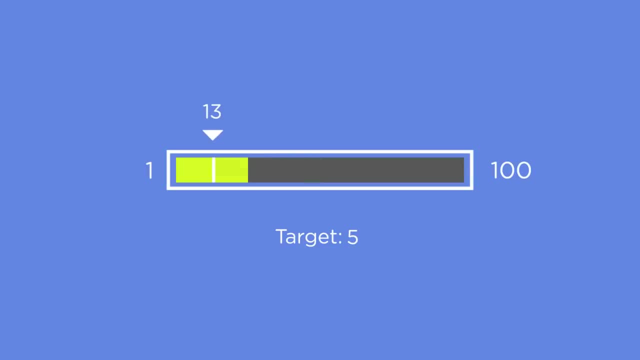 of the current list. We repeat this process until the target element is found, or until a sub-list contains only one element. If that single element sub-list does not match the target element, then we end the algorithm indicating that the element does not exist in the list. 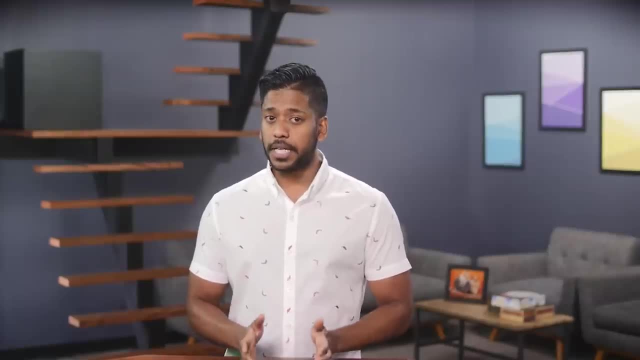 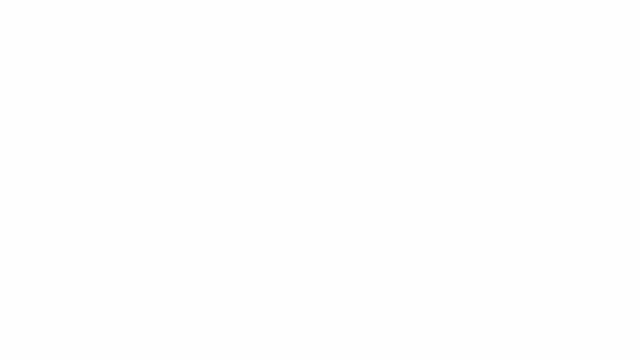 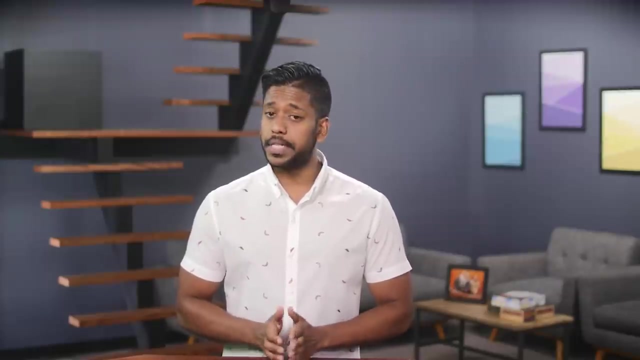 Okay, so that is the magic behind how Brittany managed to solve the round much faster. In the next video, let's talk about the efficiency of binary search. We have a vague understanding that Brittany's approach is better in most cases. But just like with linear search, 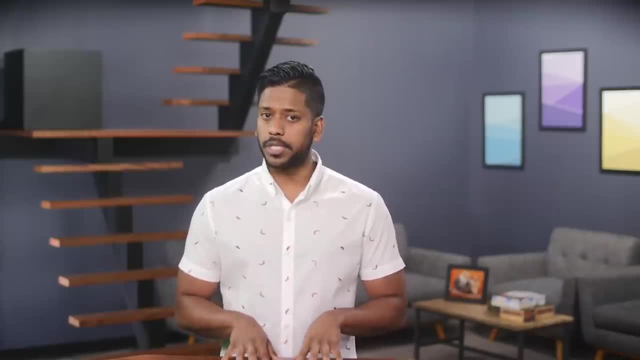 it helps to visualize this, Much like we did with linear search. when determining the efficiency of an algorithm- and remember, we're still only looking at efficiency in terms of time- time complexity, as it's called- we always want to evaluate how the algorithm performs. 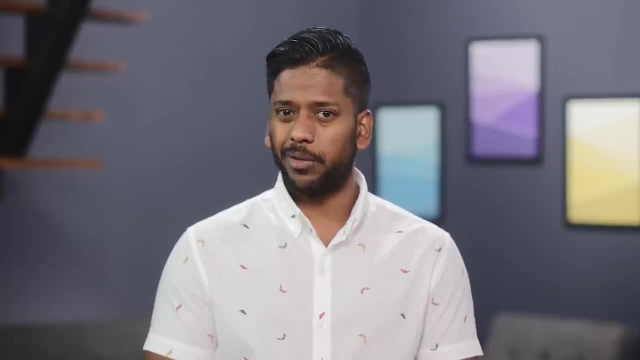 in the worst case scenario. Now you might be thinking: well, that doesn't seem fair because, given a series of data, if the target value we're searching for is somewhere near the front of the list, then linear search may perform just as well. 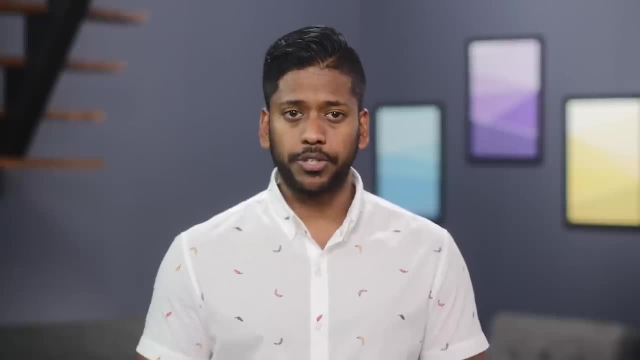 if not slightly better than binary search, And that is totally true. Remember, a crucial part of learning algorithms is understanding what works better in a given context. When measuring efficiency, though, we always use the worst case scenarios as a benchmark, because, remember- 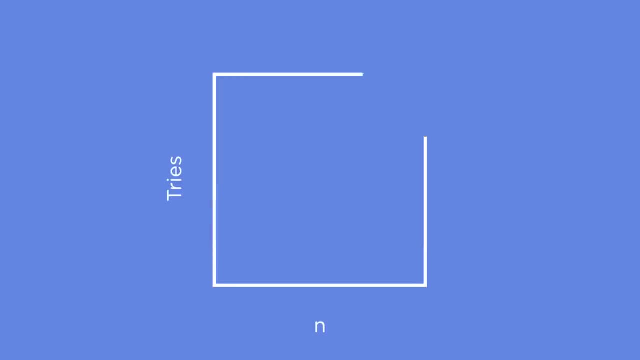 it can never perform worse than the worst case. Let's plot these values on the graph. we started earlier With the number of tries or the runtime of the algorithm on the y-axis and the maximum number of values in the series, or n. 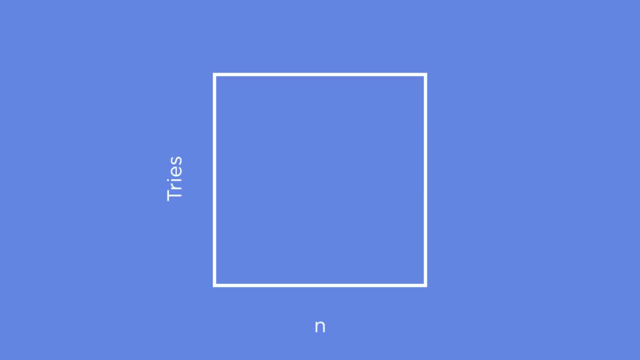 on the horizontal axis to represent the worst case scenario. We have two data points: When n equals 10, Brittany took 4 tries using binary search. And when n equals 100, it took 7 tries, But even side by side. 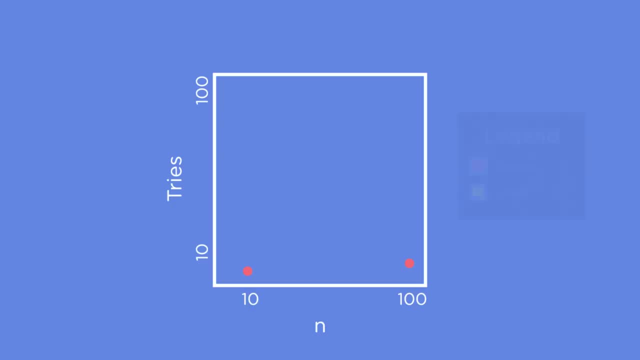 these data points are sort of meaningless. Remember that, while there is quite a difference between the runtime of linear search and binary search, at an n value of 100, for a computer that shouldn't matter. What we should do is check out how the algorithm performs. 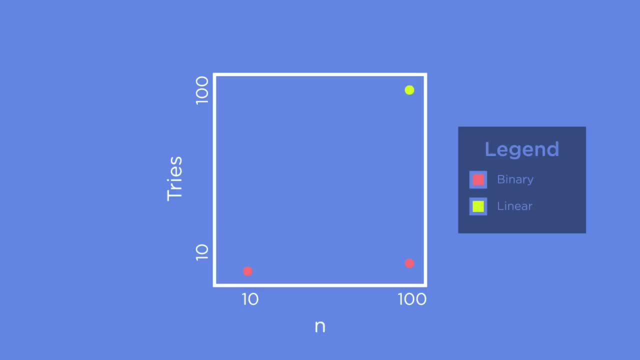 at levels of n that might actually slow a computer down As n grows larger and larger. how do these algorithms compare to one another? Let's add that to the graph. Okay, now a picture starts to emerge As n gets really large. 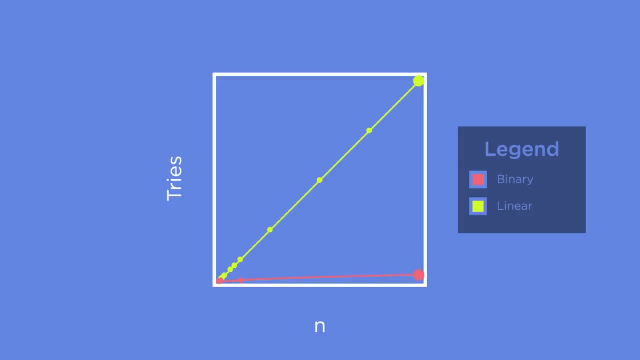 the performance of these two algorithms differs significantly. The difference is kind of staggering, actually. Even with a simple game we saw that binary search was better, but now we have a much more complete idea of how much better, For example, when n is 1000,. 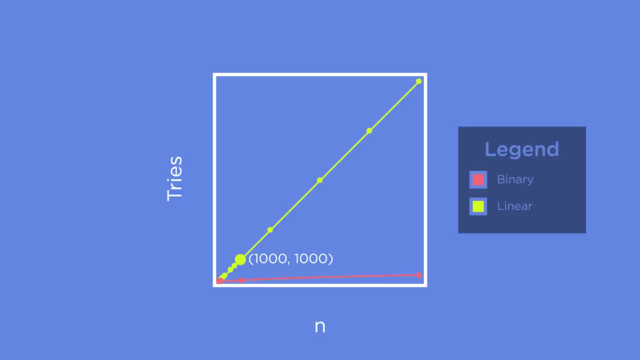 the runtime of linear search, measured by the number of operations or turns, is also 1000.. For binary search it takes just 10 operations. Now let's look at what happens when we increase n by a factor of 10. At 10,000,. 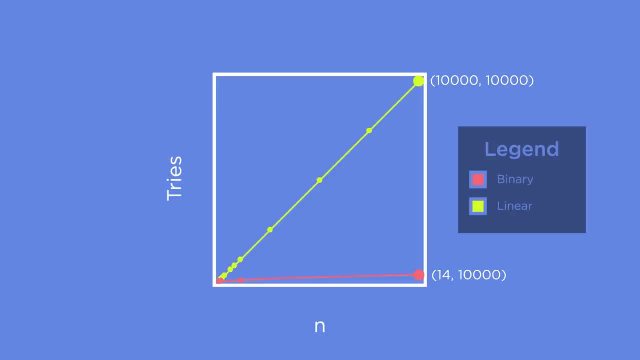 linear search takes 10,000 operations, while binary search takes 14 operations. An increase by a factor of 10 in binary search only needs 4 more operations to find a value If we increase it again by a factor of 10 once more. to an n value of 100,000, binary search takes only 17 operations. It is blazing fast. What we've done here is plotted on a graph how the algorithm performs as the input set. it is working on increases, In other words. 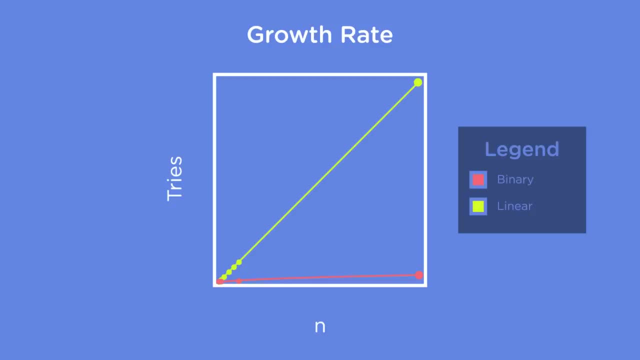 we've plotted the growth rate of the algorithm, also known as the order of growth. Different algorithms grow at different rates, and by evaluating their growth rates we get a much better picture of their performance, because we know how the algorithm will hold up as n grows larger. 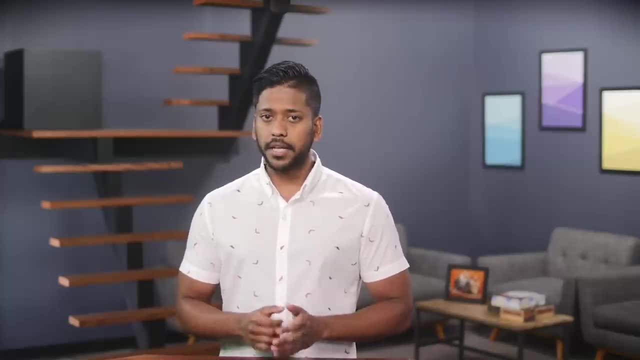 This is so important. In fact, it is the standard way of evaluating an algorithm and brings us to a concept called Big O. You might have heard this word thrown about and if you found it confusing, don't worry, We've already built up. 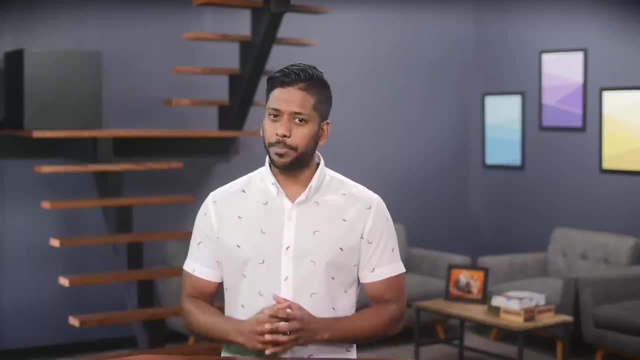 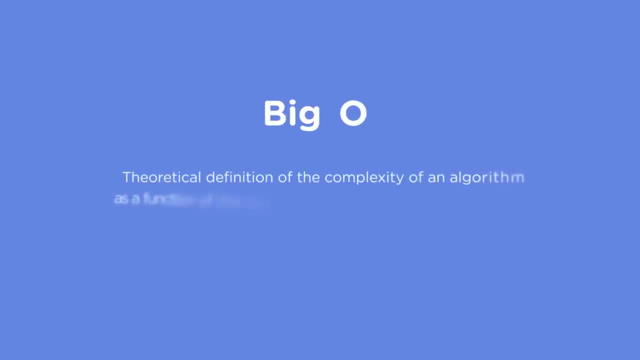 a definition in the past few videos. We just need to bring it all together. Let's start with a common statement. you'll see in studies on algorithms, Big O is a theoretical definition of the complexity of an algorithm as a function of the size. 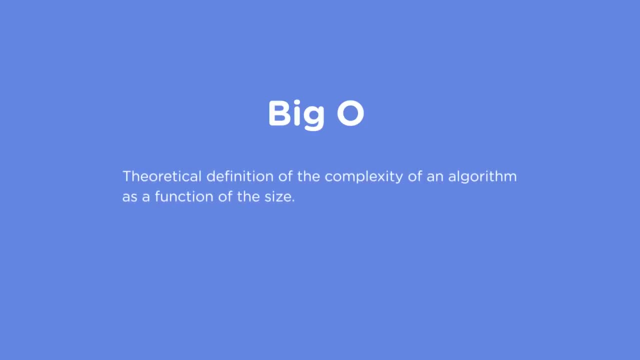 Wow, what a mouthful. This sounds really intimidating, but it's really not. Let's break it down. Big O is a notation used to describe complexity, And what I mean by notation is that it simplifies everything we've talked about down into a single variable. 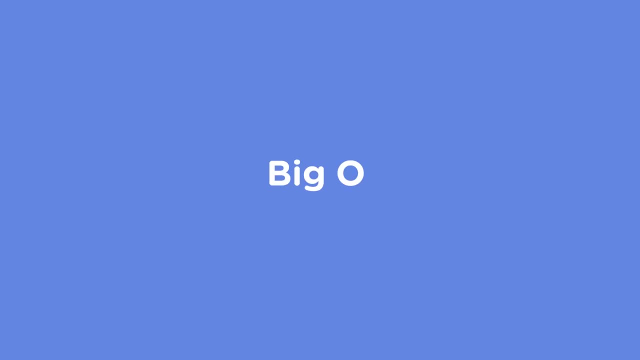 An example of complexity, written in terms of Big O looks like this: As you can see, it starts with an uppercase letter O. That's why we call it Big O. It's literally a Big O. The O comes from order of magnitude of complexity. 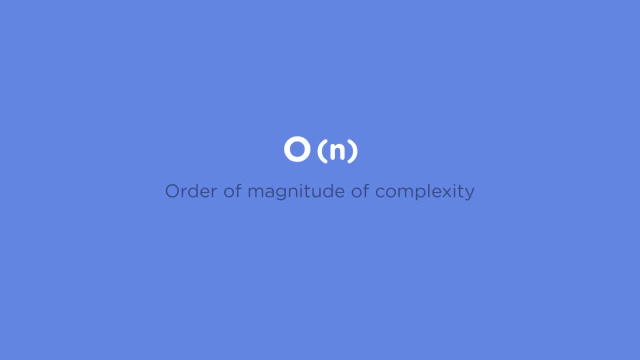 So that's where we get the Big O from Now. complexity here refers to the exercise we've been carrying out in measuring efficiency. If it takes Brittany four tries when n is 10, how long does the algorithm take when n is 10 million? 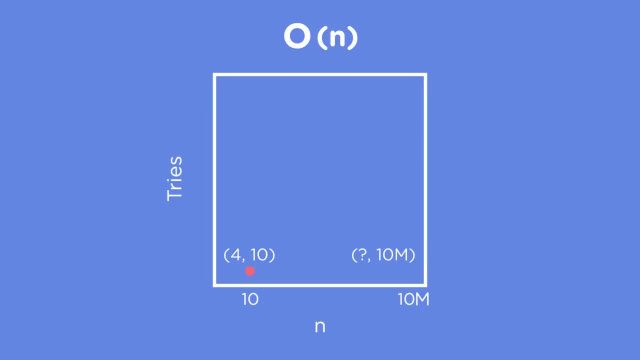 When we use Big O for this, the variable used, which we'll get to, distills that information down so that by reading the variable, you get a big picture view without having to run through data points and graphs just like we did. It's important to remember. 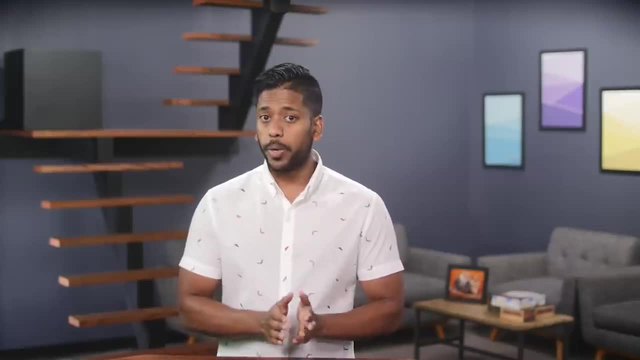 that complexity is relative. When we evaluate the complexity of the binary search algorithm, we're doing it relative to other search algorithms, not all algorithms. Big O is a useful notation for understanding both time and space complexity, but only when comparing amongst algorithms. 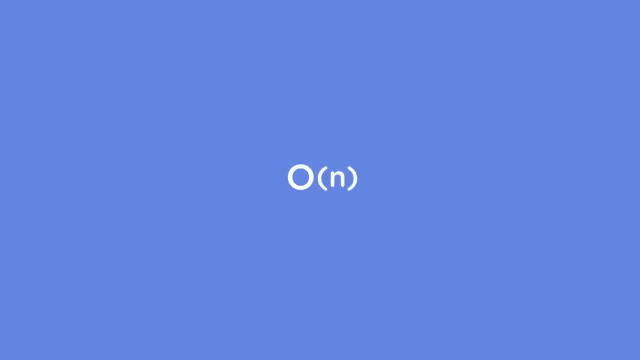 that solve the same problem. The last bit in that definition of Big O is a function of the size, And all this means is that Big O measures complexity as the input size grows, Because it's not important to understand how an algorithm performs in a single data set. 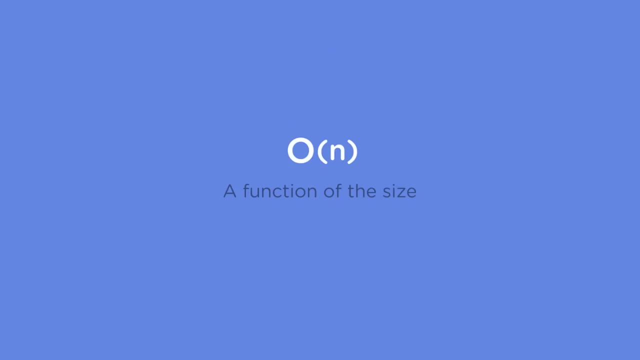 but in all possible data sets You will also see Big O referred to as the upper bound of the algorithm, And what that means is that Big O measures how the algorithm performs in the worst case scenario. So that's all. Big O is Nothing special. 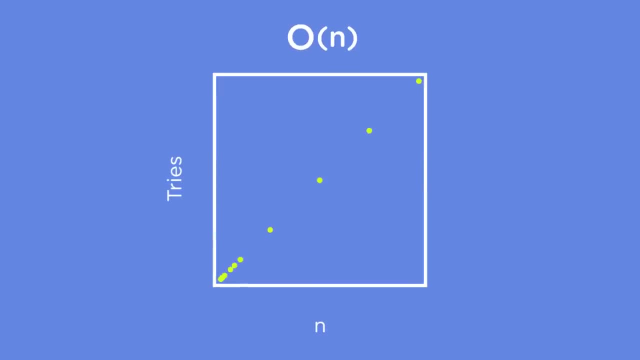 It's just a notation that condenses the data points and graphs that we've built up down to one variable. Okay, so what do these variables look like? For John's strategy, linear search, we say that it has a time complexity of Big O and then N. 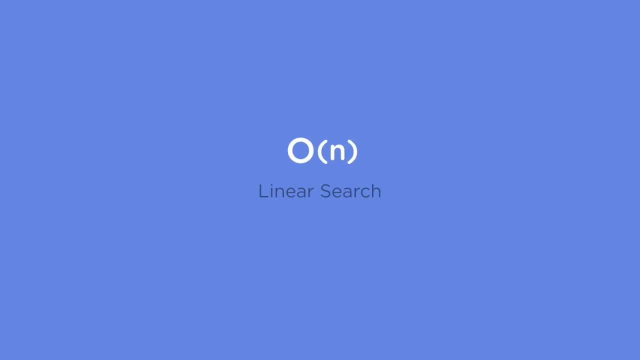 So that's again Big O with an N inside parentheses. For Brittany's strategy, binary search, we say that it has a time complexity of Big O, of log N. That's Big O with something called a log and an N inside parentheses. Now don't worry if you don't understand that. 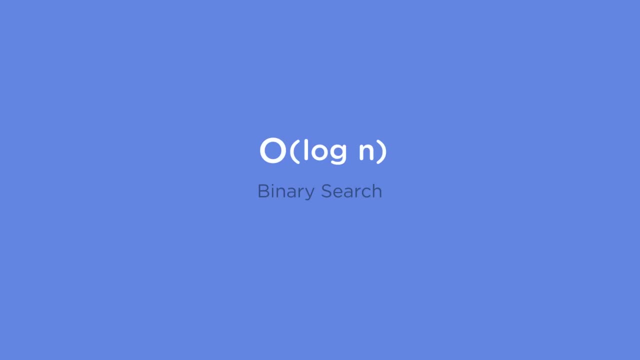 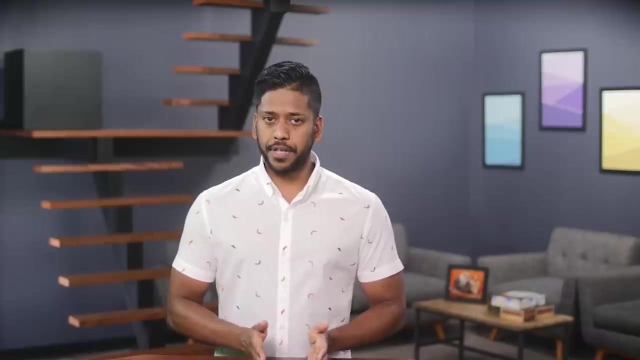 We'll go into that in more detail later on in the course. Each of these has a special meaning, but it helps to work through all of them to get a big picture view. So over the next few videos let's examine what are called. 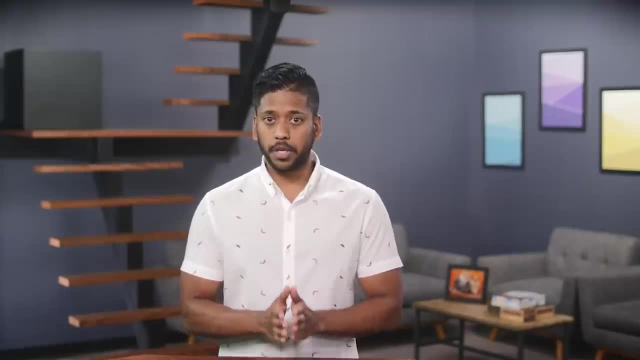 common complexities or common values of Big O that you will run into and should internalize. In our discussions of complexity, we made one assumption: that the algorithm as a whole had a single measure of complexity. That isn't true and we'll get at how we arrive. 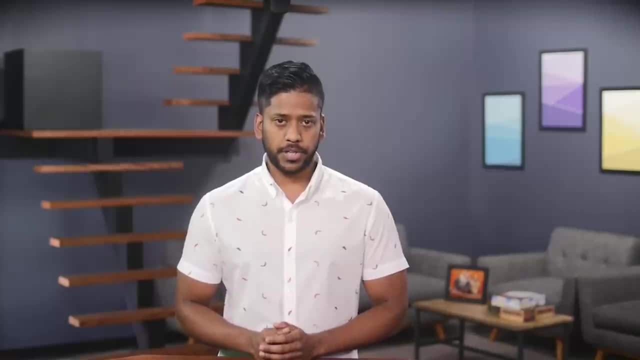 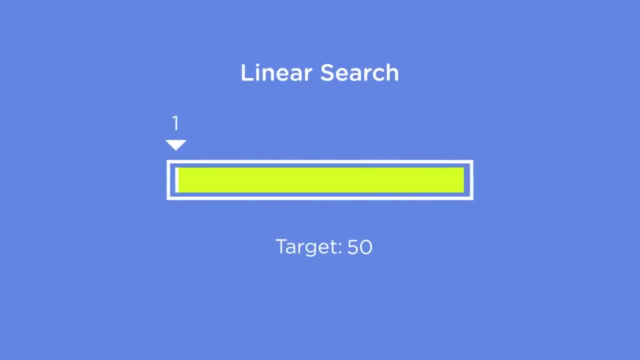 at these measures for the entire algorithm at the end of this exercise. But each step in the algorithm has its own space and time complexity. In linear search, for example, there are multiple steps and the algorithm goes like this: Start at the beginning of the list. 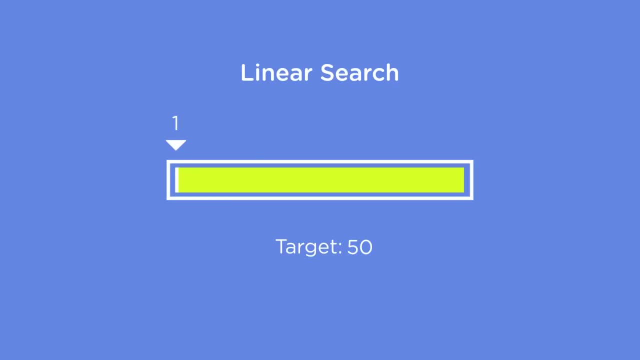 or range of values. Compare the current value to the target. If the current value is the target that we're looking for, we're done. If it's not, we'll move on sequentially to the next value in the list and repeat step two. 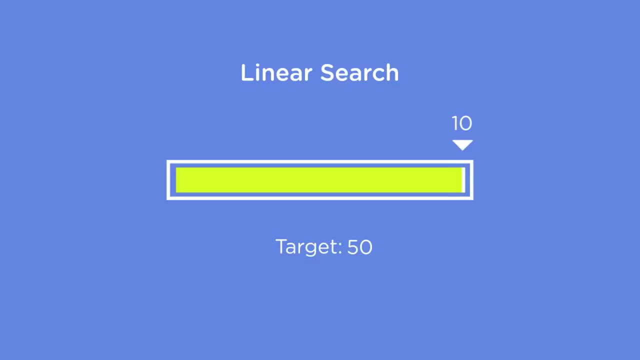 If we reach the end of the list, then the target value is not in the list. Let's go back to step two for a second comparing the current value to the target. Does the size of the data set matter for this step? When we're at step two, 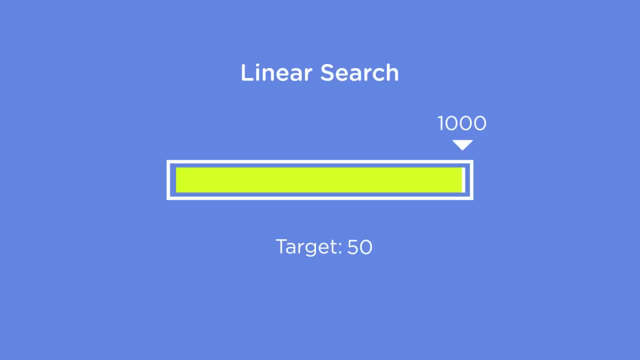 we're already at that position in the list and all we're doing is reading the value to make a comparison. Reading the value is a single operation And if we were to plot it on a graph of runtime per operations against n, it looks like this: 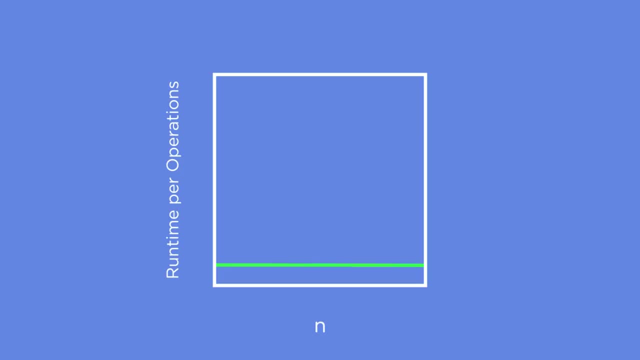 A straight line that takes constant time, regardless of the size of n. Since this takes the same amount of time in any given case, we say that the runtime is constant time. It doesn't change. In Big O notation we represent this as Big O. 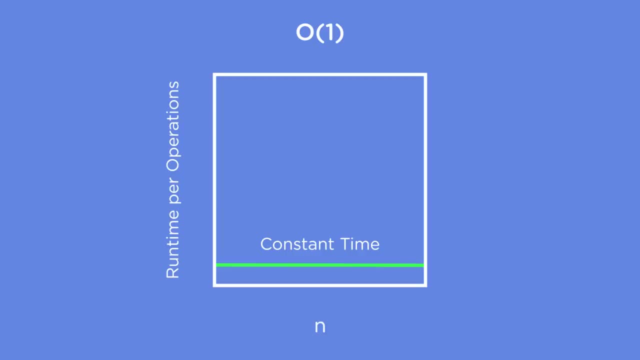 with a one inside parentheses. Now, when I first started learning all this, I was really confused as to how to read this, even if it was in my own head. Should I say Big O of one. When you see this written, you're going to read this as constant time. 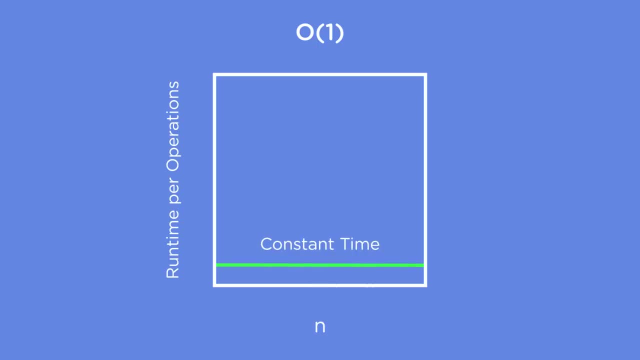 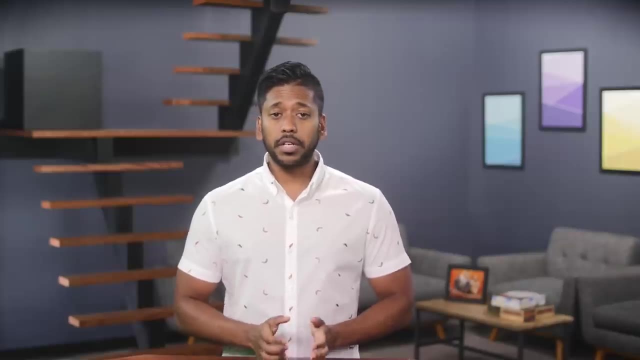 So reading a value in a list is a constant time operation. This is the most ideal case when it comes to runtimes, because input size does not matter and we know that, regardless of the size of n, the algorithm runtime will remain the same. 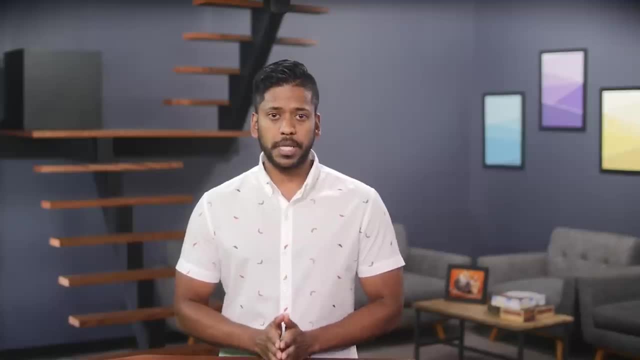 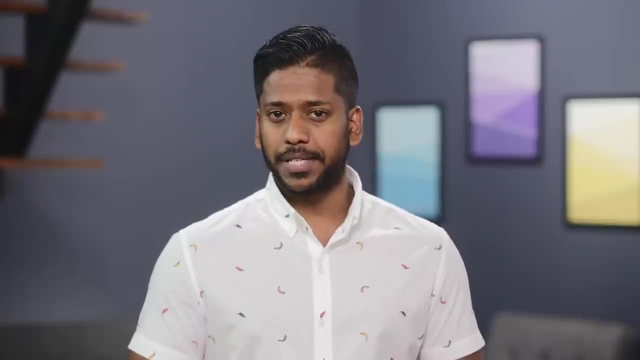 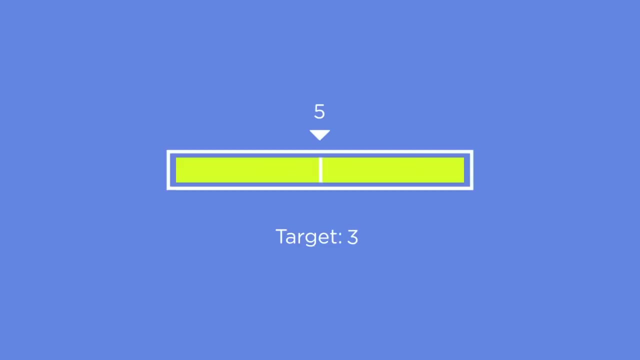 The next step up in complexity, so to speak, is the situation we encountered with the binary search algorithm. Traditionally, explaining the time complexity of binary search involves math, and I'm going to try to do it both with and without. When we played the game using binary search? 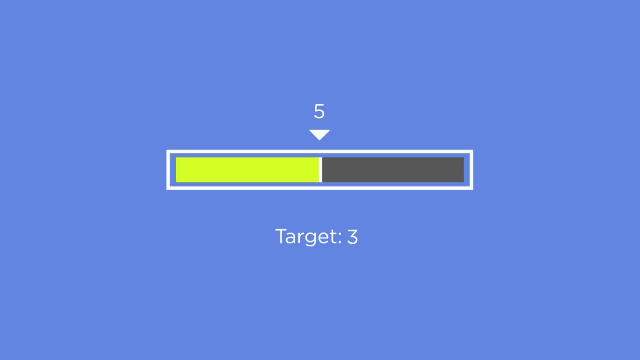 we noticed that with every turn we were able to discard half of the data. But there's another pattern that emerges that we didn't explore. Let's say n equals 10.. How long does it take to find an item at the 10th position of the list? 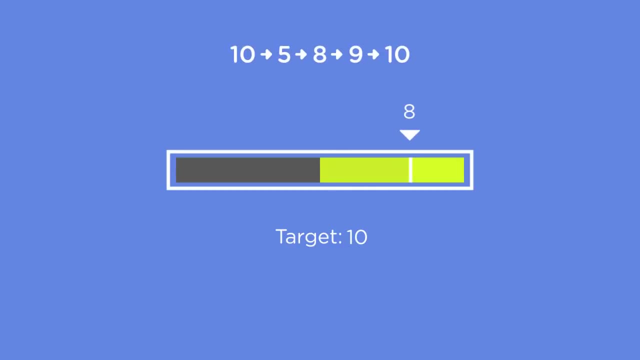 We can write this out. So we go from 10 to 5 to 8 to 9 and then down to 10.. Here it takes us four tries to cut down the list to just one element and find the value we're looking for. 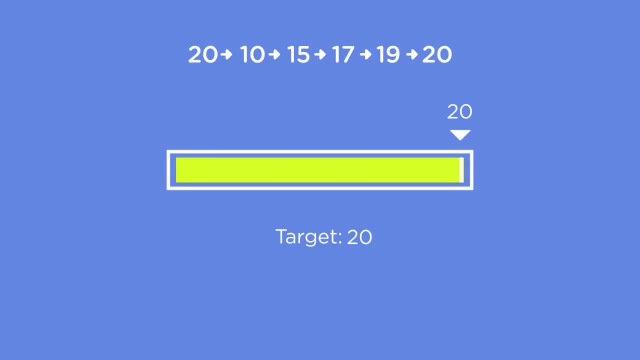 Let's double the value of n to 20 and see how long it takes for us to find an item at the 20th position. So we start at 20 and then we pick 10.. From there we go to 15,, 17,, 19, and finally 20.. 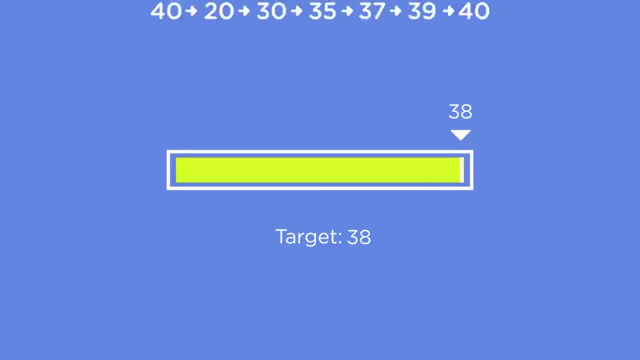 So here it takes us five tries. Okay, let's double it again so that n is 40, and we try to find the item in the 40th position. So when we start at 40, the first midpoint we're going to pick is 20.. 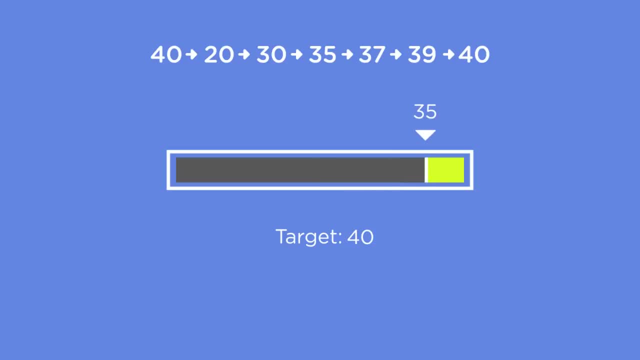 From there we go to 30,, then 35,, 37,, 39, and then 40.. Notice that every time we double the value of n, the number of operations it takes to reduce the list down to a single element only increases by one. 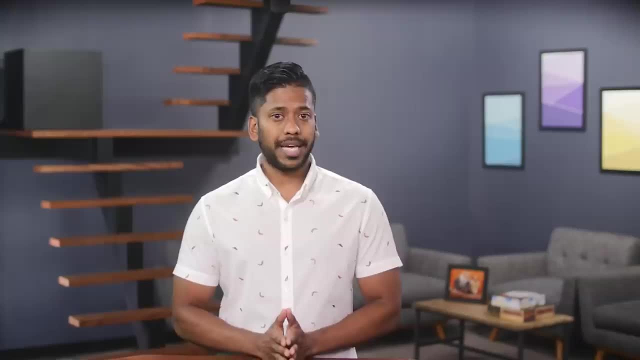 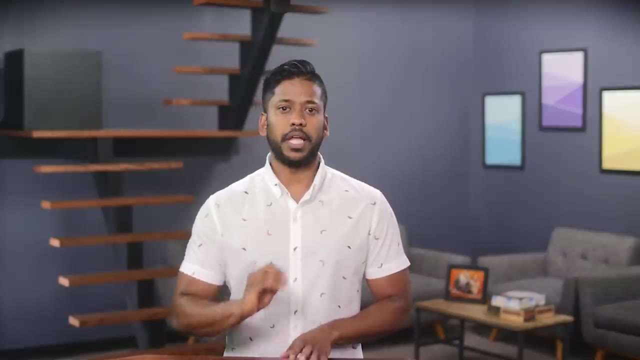 There's a mathematical relationship to this pattern and it's called a logarithm of n. You don't really have to know what logarithms truly are, but I know that some of you like underlying explainers, so I'll give you a quick one. 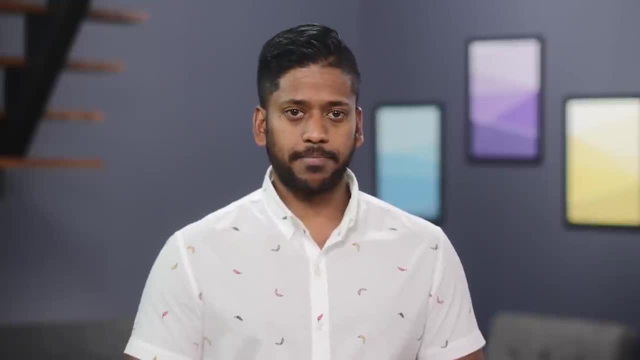 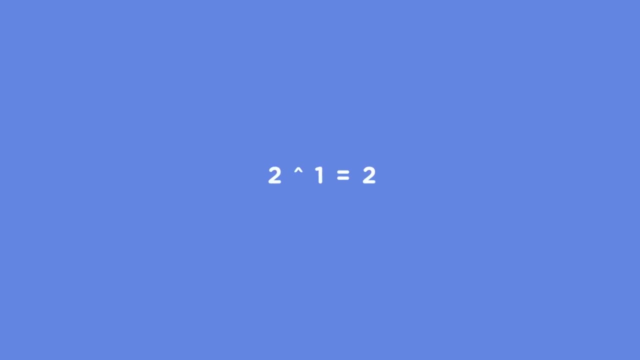 If you've taken algebra classes, you may have learned about exponents. Here's a quick refresher: 2 times 1 equals 2.. Now this can be written as 2 raised to the first power, because it is our base case. 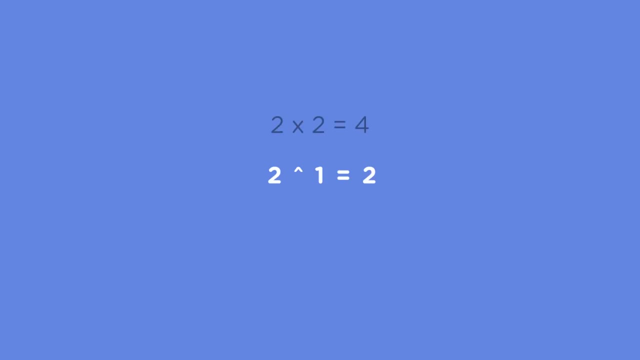 2 times 1 is 2.. Now 2 times 2 is 4.. This can be written as 2 raised to the second power, because we're multiplying 2 twice. First we multiply 2 times 1, then the result of that times 2.. 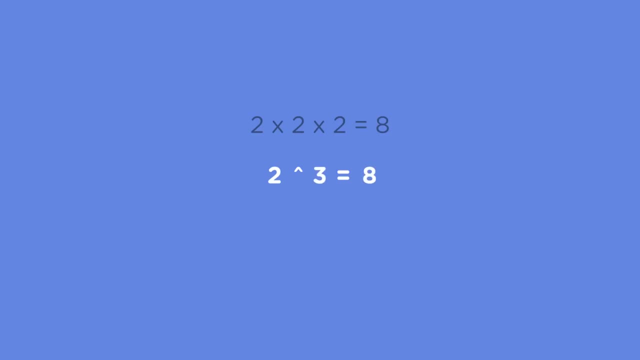 2 times 2 times 2 is 8, and we can write this as 2 raised to the third power, because we're multiplying 2 three times In: 2 raised to 2 and 2 raised to 3, the 2 and 3 there are called exponents. but as long as you take things slow, there's no reason for it to be impossible. Remember that not any block of code counts as an algorithm. To be a proper implementation of linear search, this block of code must return a value, must complete execution in a. finite amount of time and must output the same result every time for a given input set. So let's verify this with a small test. Let's write a function called verify that accepts an index value. If the value is not none, it prints the index position. If it is none, it informs us that the target was not found in the list. So def verify and this is going to take an index value and we'll say: if index is not none, then we'll print target found at index. oops, that's a colon here. index, else that needs to go back there we go, else will say: target not found in list. Okay, using this function, let's define a range of numbers now. so this will be a list numbers and we'll just go from one to, let's say, ten. Now, if you've written Python code before, you know that I can use a list comprehension to make this easier, but we'll keep things simple. We can now use our linear search function to search for the position of a target value in this list. So we can say: result equal: linear underscore search and we're going to pass in the numbers list. that's the one we're searching through and we want to look for the position where the value 12 exists and then we'll verify this result If our algorithm worked correctly, the verify function should inform us that the target did not exist, So make sure you save the file, which you can do by going up to file and save or hitting command s and then below in the terminal you're going to type out Python. linear search or you can hit tab and it should auto complete linear search. dot pi. As you can see, correct the target was not found in the list, so the output of our script is what we expect For our second test. let's search for the value 6 in the list So you can copy this command c to copy and then paste it again, and we'll just change 12 here to 6.. And then come back down to the terminal. hit the up arrow to execute the same command. again and hit enter, You'll notice that I forgot to hit save, so it did not account for that new change. we'll try that out again And there you'll see that if it works correctly- which it did- the index should be number 5.. Run the. program on your end and make sure everything works as expected. Our algorithm returned a result in each case. it executed in a finite time and the results were the ones we expect. In the next video, let's tackle binary search. In the last video, we left off with an. implementation of linear search. Let's do the same for binary search so that we get an understanding of how the process is represented in code. So we'll do this in a new file. back to a file, new file and we'll name this one binary. search dot py. Like before, we're going to start with a function named binary search. so we'll say def binary underscore search that takes a list and a target. If you remember, binary search works by breaking the array or list down into: smaller sets until we find the value we're looking for. We need a way to keep track of the position of the list that we're working with, so let's create two variables, First and last, to point to the beginning and end of the array. So first equal zero. Now, if you're new to programming, list positions are represented by index values that start at zero instead of one. So here we're setting first to zero to point to the first element in the list. Last is going to point to the last. element in the list. So we'll say: last equal len list minus one. Now this may be confusing to you, so a quick sidebar to explain what's going on. Let's say we have a list containing five elements. If we called len on that list, we should get five back because there are five elements. But remember that because the position numbers start at zero, the last value is not at position five but at four In nearly all programming languages. getting the position of the last element in the list. is obtained by determining the length of the list and deducting one, which is what we're doing. Okay, so we know what the first and last positions are. when we start the algorithm For our next line of code, we're going to create a while loop. A while loop takes a condition and keeps executing the code inside the loop until the condition evaluates to false. For our condition we're going to say to keep executing this loop until the value of first is less than or equal to the value of last. So, while first less than or equal to last- Well why, you ask. Why is this our condition? Well, let's work through this implementation and then a visualization should help. Inside the while loop, we're going to calculate the midpoint of our list, since that's the first step. of binary search Midpoint equal. so we'll say first plus last, and then we'll use the floor division double slash here, divided by two. Now the two forward slashes here are what Python calls a floor division operator. What it does is it rounds down to the nearest whole. number. So if we have an eight element array, first is zero, last is seven. if we divided zero plus seven, which is seven by two, we would get 3.5.. Now, 3.5 is not a valid index position, so we round that down to three. using the floor division operator. Okay, so now we have a midpoint. The next step of binary search is to evaluate whether the value at this midpoint is the same as the target we're looking for. So we'll say if list value at midpoint equals. 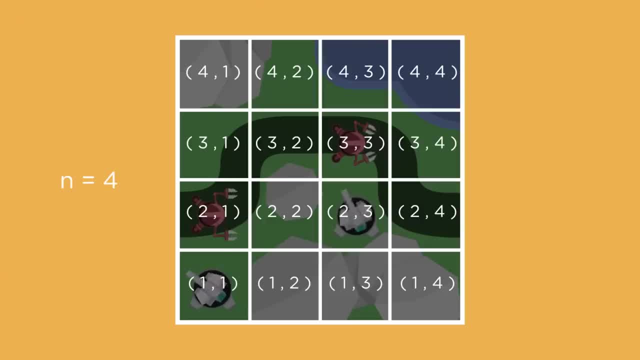 the target. well, if it is, then we'll go ahead and return the midpoint. So we'll say: return midpoint. The return statement terminates our algorithm. and over here we're done. This is our best case scenario. Next, we'll say else if list at midpoint. 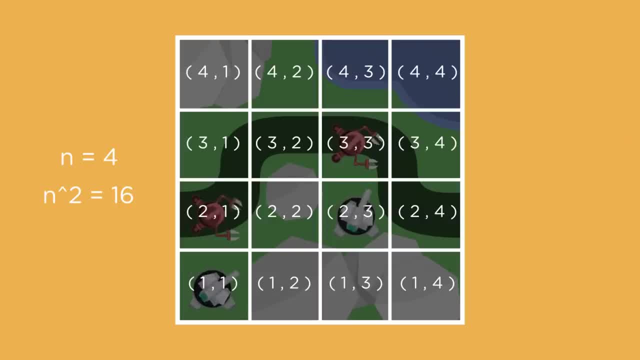 or value at midpoint is less than the target. Now here, if the value is less, the value at midpoint is less than the target, then we don't care about any of the values lower than the midpoint. So we redefine first to point to the value. 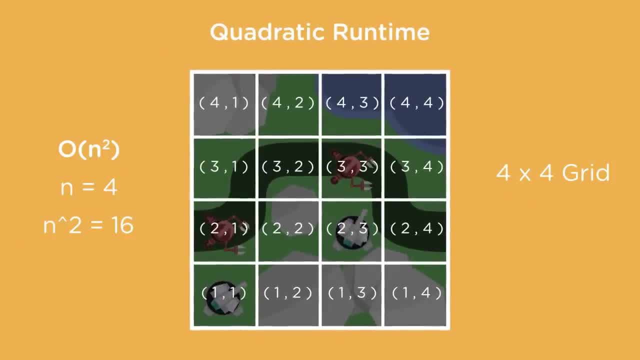 after the midpoint, So we'll say midpoint plus one. Now, if the value at the midpoint is greater than the target, then we can discard the values after the midpoint and redefine last to point to the value prior to the midpoint, So we'll say else. 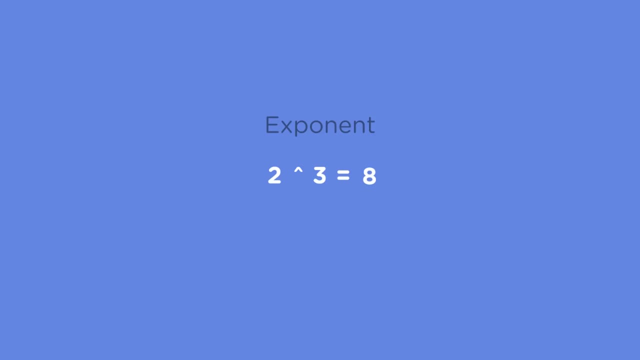 and they define how the number grows. With 2 raised to 3, we start with the base value and multiply itself three times. The inverse of an exponent is called a logarithm. So if I say log to the base, 2 of 8 equals 3,. 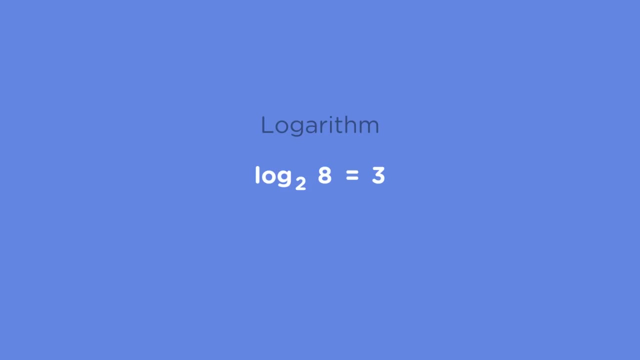 I'm basically saying the opposite of an exponent. Instead of saying how many times you have to multiply this value, I'm asking: how many times do I have to divide 8 by 2 to get the value 1.. This takes three operations. 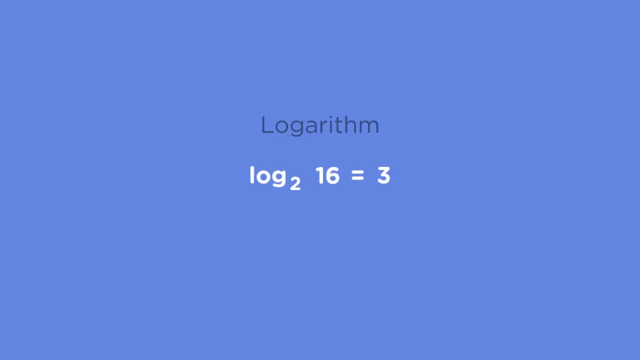 What about the result of log to the base 2 of 16?? That evaluates to 4.. So why does any of this matter? Notice that this is sort of how binary search works. Log to the base 2 of 16 is 4.. 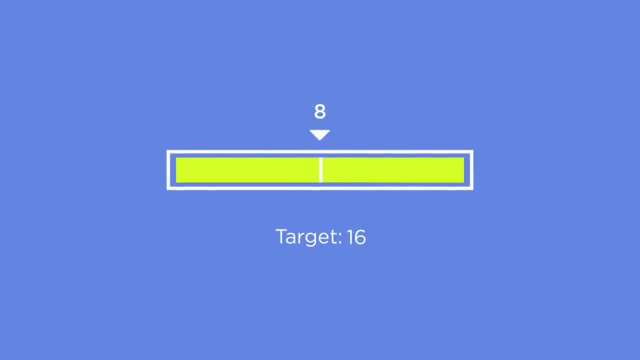 If n was 16,? how many tries does it take to get to that last element? Well, we start in the middle, at 8. That's too low, so we move to 12.. Then we move to 14,, then to 15, and then to 16,. 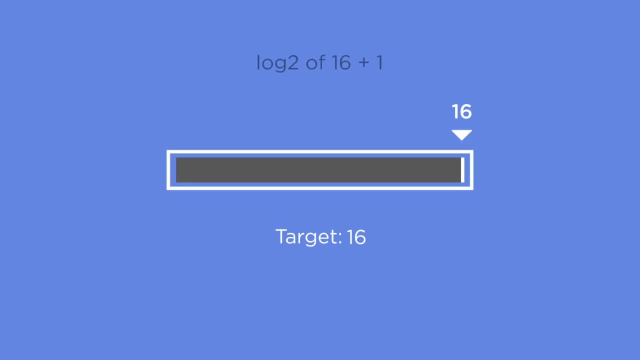 which is 5 tries, or log to the base 2 of 16 plus 1.. In general, for a given value of n, the number of tries it takes to find the worst-case scenario is log of n plus 1.. And because this pattern is, overall, a logarithmic pattern, 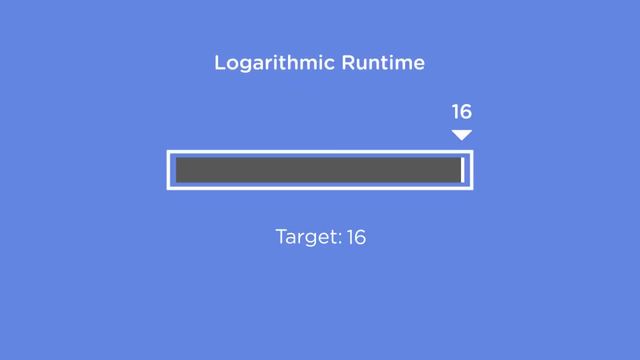 we say that the runtime of such algorithms is logarithmic. If we plot these data points on our graph, a logarithmic runtime looks like this In big-O notation: we represent a logarithmic runtime as big-O of log n, which is written as big-O with log n inside parentheses. 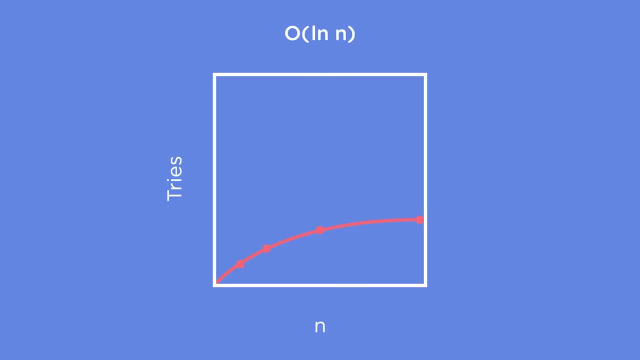 or even sometimes as ln n inside parentheses. When you see this, read it as logarithmic time. As you can see on the graph, as n grows really large, the number of operations grows very slowly and eventually flattens out, Since this line is below the line for a linear runtime. 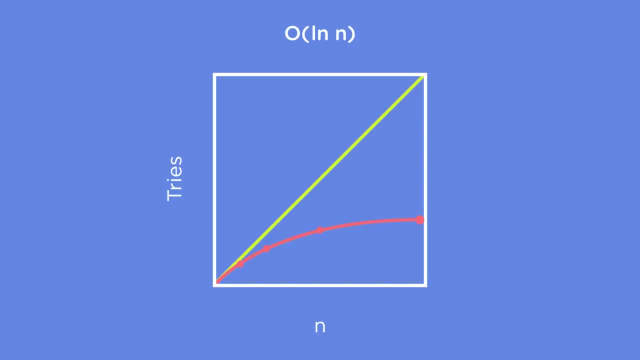 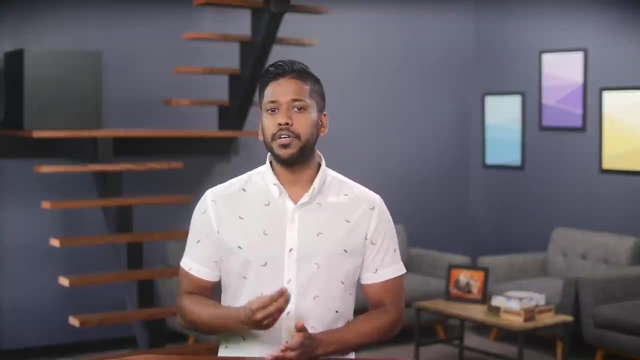 which we'll look at in a second. you might often hear algorithms with logarithmic runtimes being called sublinear. Logarithmic or sublinear runtimes are preferred to linear Because they're more efficient, But in practice, linear search has its own set of advantages. 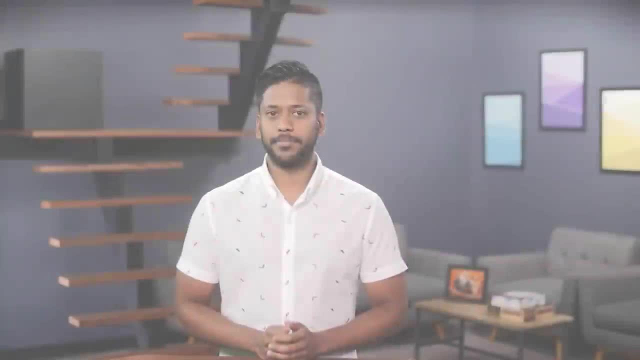 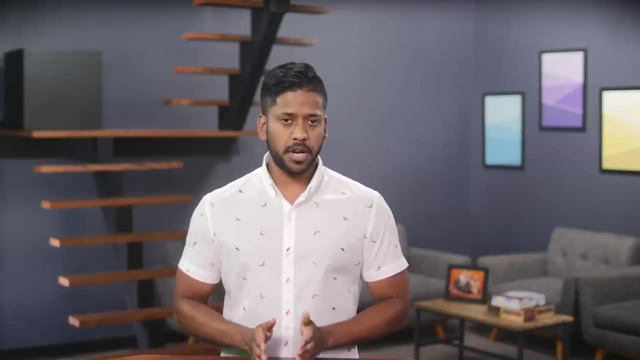 which we'll take a look at in the next video. Next up, let's look at the situation we encountered with the linear search algorithm. We saw that in the worst-case scenario, whatever the value of n was, John took exactly that many tries to find the answer. 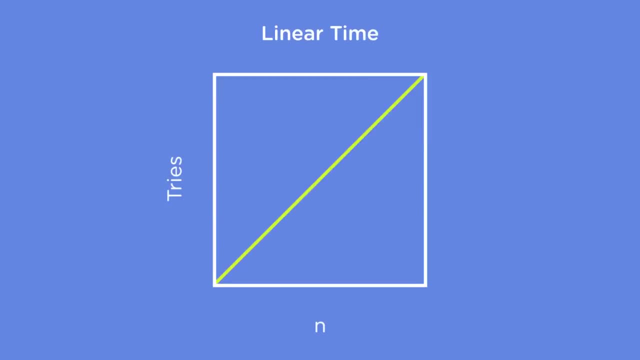 As in linear search, when the number of operations to determine the result in the worst-case scenario is at most the same as n, we say that the algorithm runs in linear time. We represent this as O. Now you can read that as O. 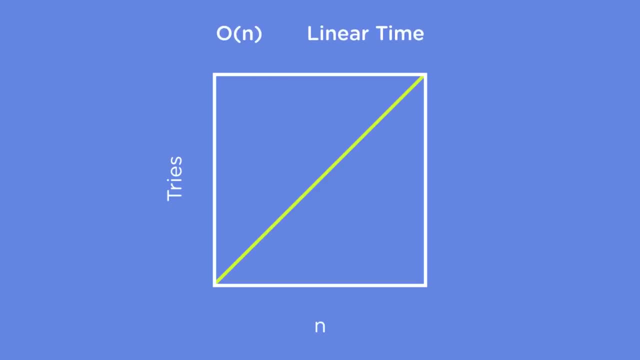 like I just said, or you can say linear time, which is more common. When we put that up on a graph against constant time and logarithmic time, we get a line that looks like this: Any algorithm that sequentially reads the input will have linear time. 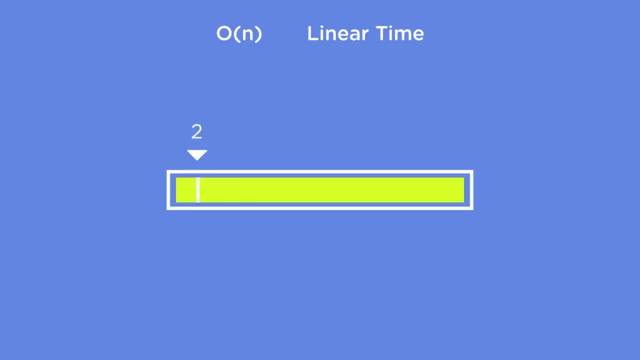 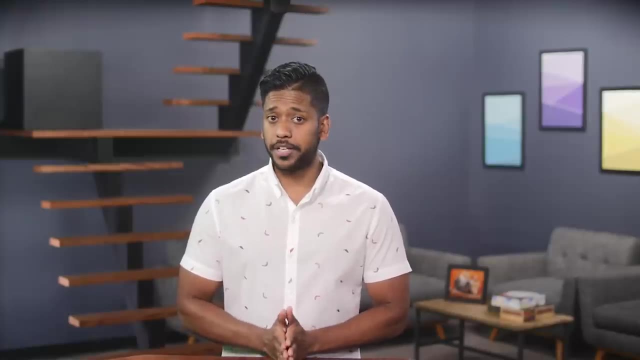 So remember any time you know. a problem involves reading every item in a list. that means a linear runtime. As you saw from the game we played, Brittany's strategy using binary search was clearly better and we can see that on the graph. 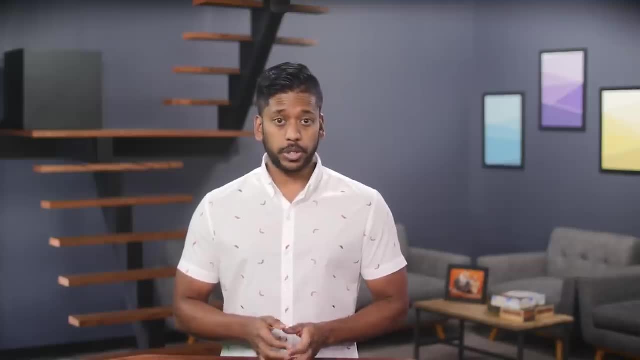 So if we had the option, why would we use linear search, which runs in linear time? Remember that binary search had a precondition: The input set had to be sorted. While we won't be looking at sorting algorithms in this course, as you learn more about algorithms, 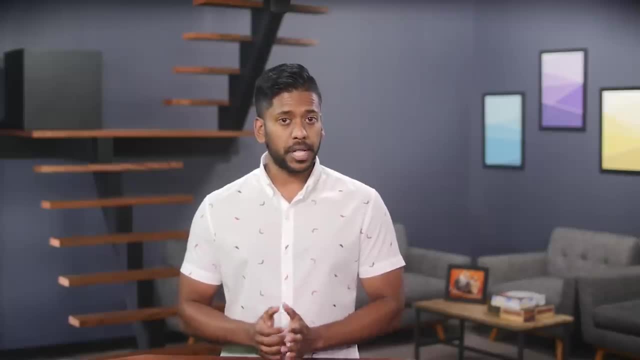 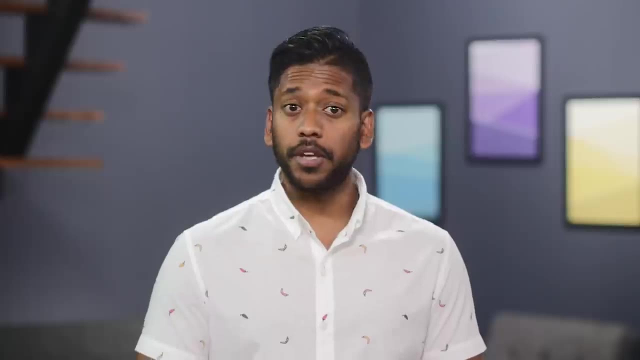 you'll find that sorting algorithms have varying complexities themselves, just like sorting. That's what search does, So we have to do additional work prior to using binary search. For this reason, in practice, linear search ends up being more performant up to a certain value of n. 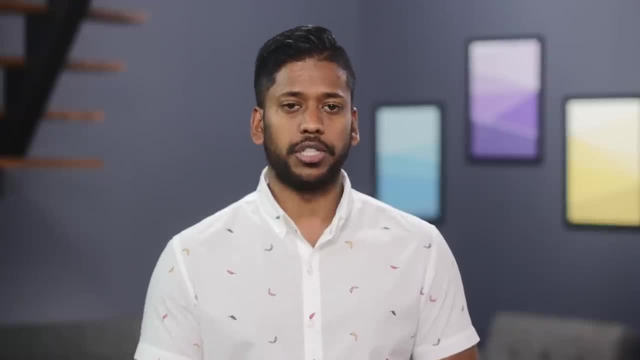 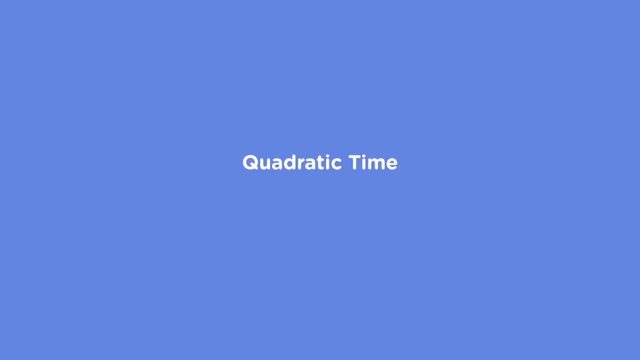 because the combination of sorting first and then searching using binary search adds up. The next common complexity you will hear about is when an algorithm runs in quadratic time. If the word quadratic sounds familiar to you, it's because you might have heard about it in math class. 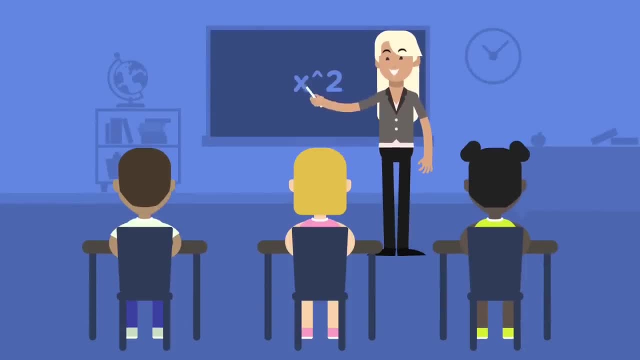 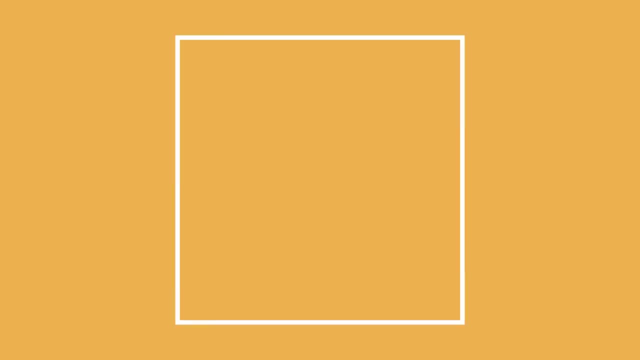 Quadratic is a word that means an operation raised to the second power or when something is squared. Let's say you and your friends are playing a tower defense game and to start it off, you're going to draw a map of the terrain. 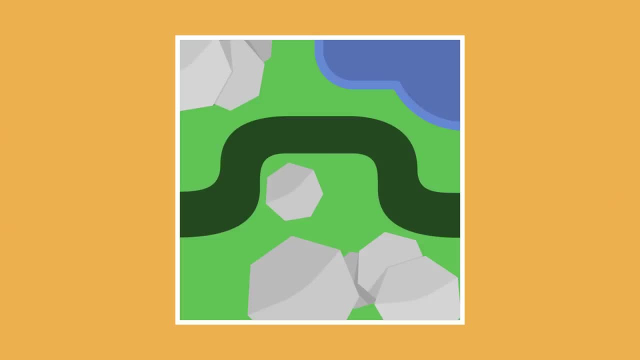 This map is going to be a grid and you pick a random number to determine how large this grid is. Let's set n, the size of the grid to 4.. Next, you need to come up with a list of coordinates so you can place towers and enemies. 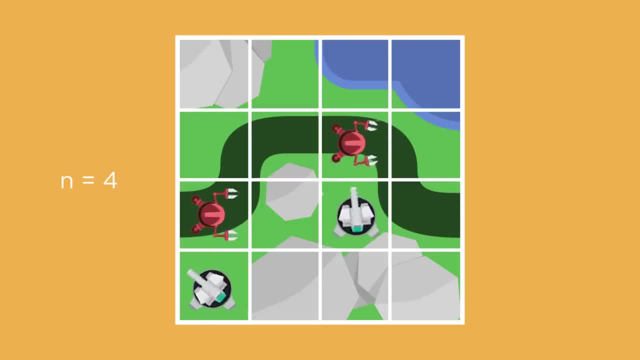 and stuff on this map. So how would we do this? If we start out horizontally, we'd have coordinate points that go 1, 1, 1, 2, 1, 3, and 1, 4.. 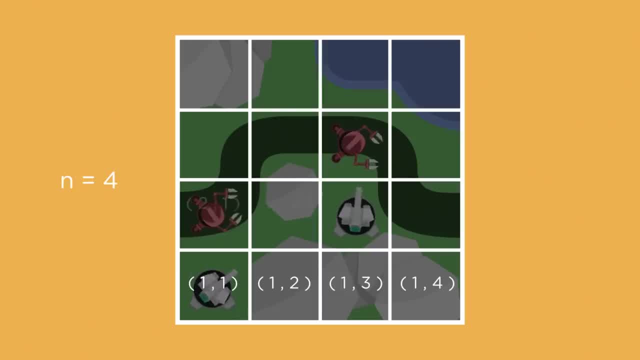 Then you go up one level vertically and we have points 2, 1,, 2,, 2,, 2,, 3, and 2, 4.. Go up one more and you have the points 3, 1, 3,, 2,, 3,, 3, and 3, 4.. 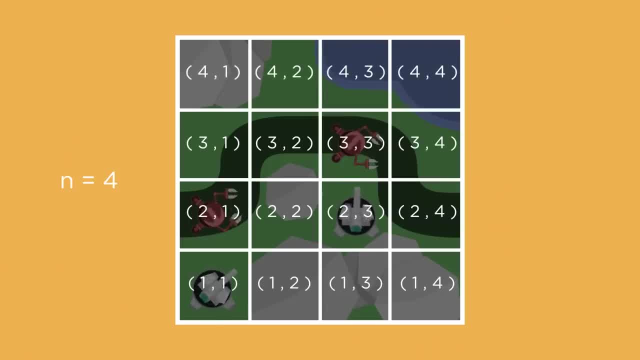 And on that last row you have the points 4, 1,, 4, 2,, 4, 3, and 4, 4.. Notice that we have a pattern here. For each row, we take the value. 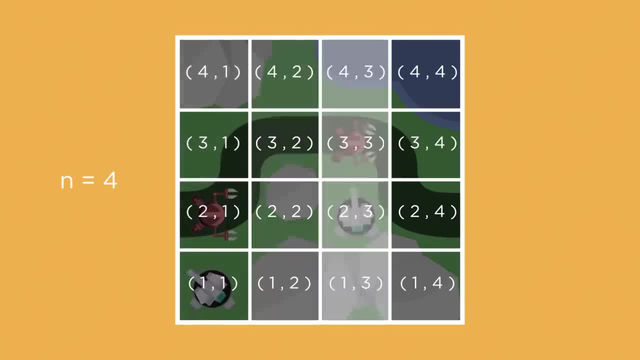 and then create a point. by adding to that every column value, The range of values go from 1 to the value of n. so we can generally think of it this way For the range of values from 1 to n, for each value in that range. 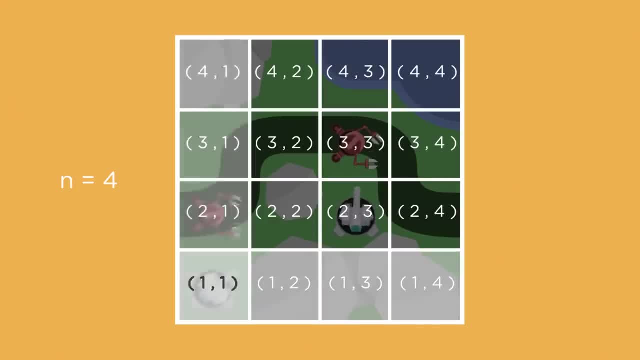 we create a point by combining that value with the range of values from 1 to n. again Doing it this way, for each value in the range of 1 to n, we create an n number of values and we end up with 16 points. 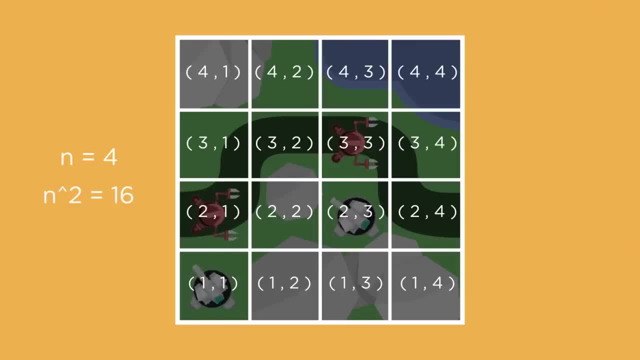 which is also n times n or n squared. This is an algorithm with a quadratic runtime, because for any given value of n, we carry out n squared number of operations. Now I picked a relatively easy, so to speak, example here. 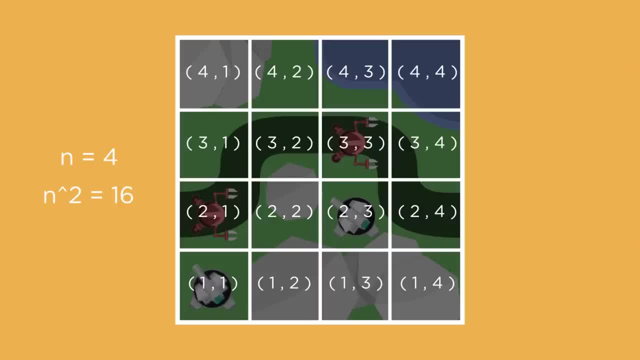 because in English at least, we often denote map sizes by height, times width, so we would call this a 4 by 4 grid, which is just another way of saying 4 squared or n squared. In big O notation we would write this as: 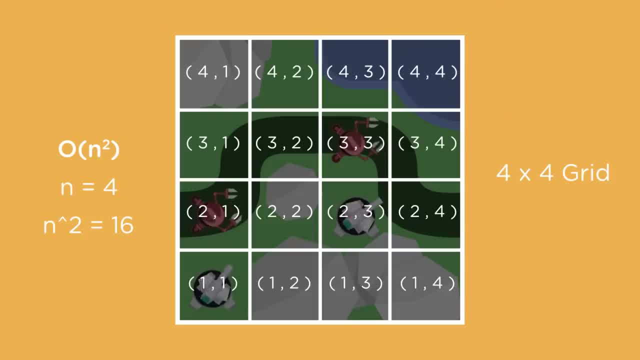 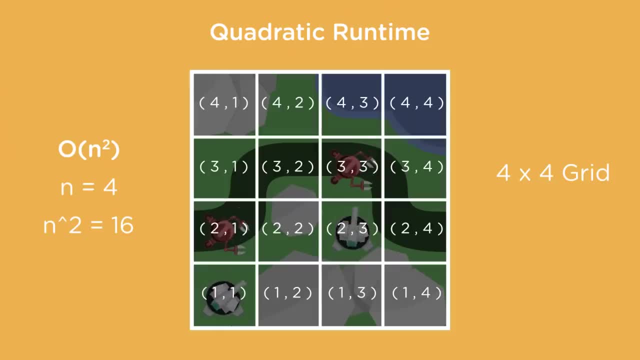 big O of n squared, or say that this is an algorithm with a quadratic runtime. Many search algorithms have a worst case, quadratic runtime, which you'll learn about soon. Now, in addition to quadratic runtimes, you may also run into cubic runtimes. 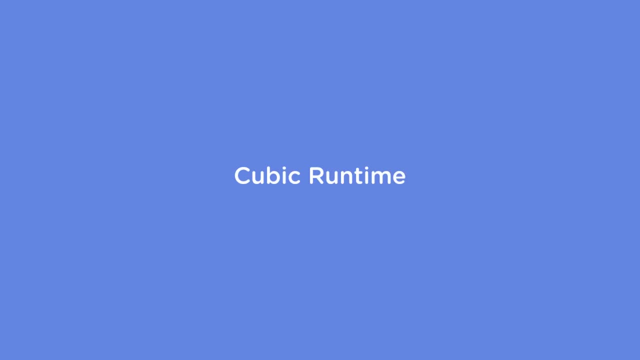 as you encounter different algorithms. In such an algorithm, for a given value of n, the algorithm executes n raised to the third power number of operations. These aren't as common as quadratic algorithms, though, so we won't look at any examples, but I think it's worth mentioning. 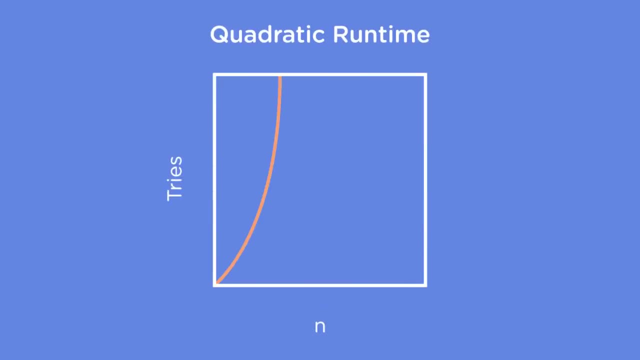 Thrown up on our graph. quadratic and cubic runtimes look like this. So this is starting to look pretty expensive computationally, as they say. We can see here that for small changes in n there's a pretty significant change in the number of operations. 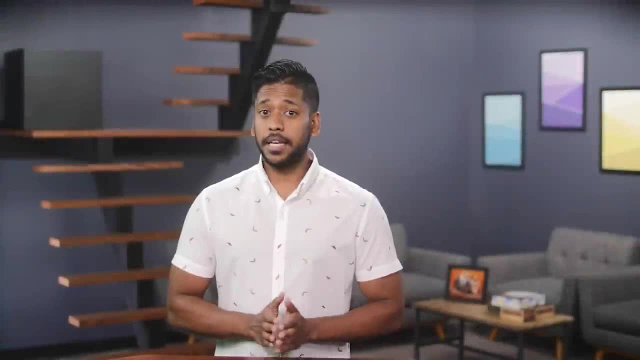 that we need to carry out. The next worst case runtime we're going to look at is one that's called quasi-linear and is sort of easier to understand- for lack of a better word- by starting with the big O notation: Quasi-linear runtimes. 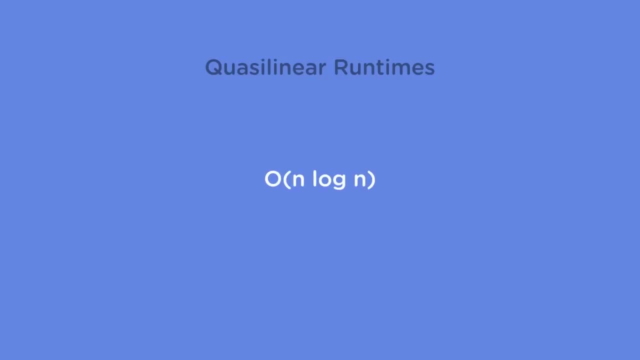 are written out as big O of n times: log n. We learned what log n was right: A logarithmic runtime. whereas n grew, the number of operations only increased by a small factor With a quasi-linear runtime. what we're saying? 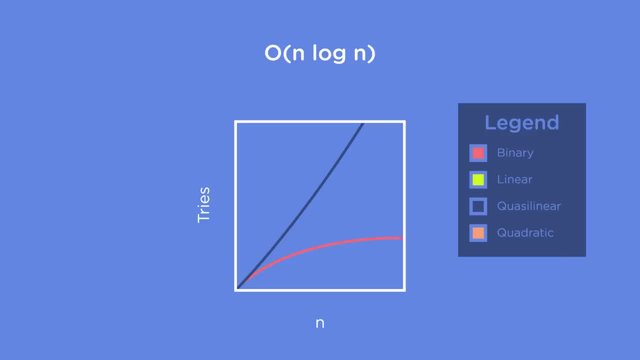 is that for every value of n we're going to execute a log n number of operations. hence the runtime of n times log n. So you saw earlier with the quadratic runtime that for each value of n we conducted n operations. It's sort of the same. 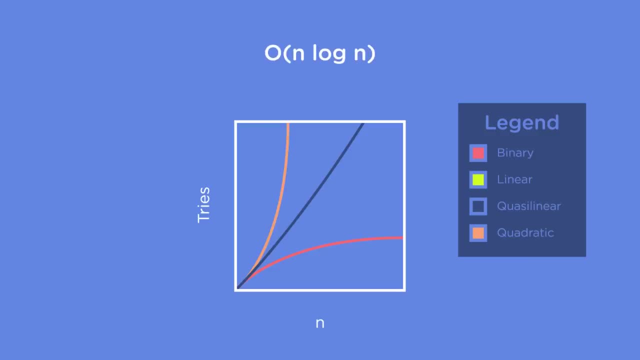 in that, as we go through the range of values in n, we're executing log n operations. In comparison to other runtimes, a quasi-linear algorithm has a runtime that lies somewhere between a linear runtime and a quadratic runtime, So where would we expect? 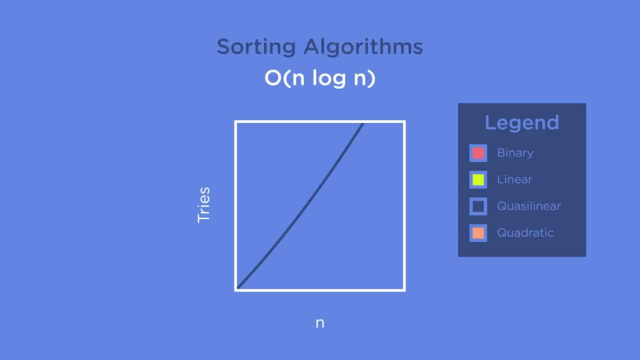 to see this kind of runtime in practical use. Well, sorting algorithms is one place you will definitely see it. Mergesort, for example, is a sorting algorithm that has a worst-case runtime of O. Let's take a look at a quick example. 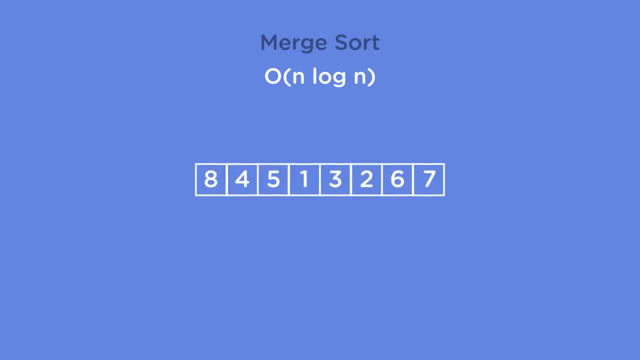 Let's say we start off with a list of numbers that looks like this and we need to sort it. Mergesort starts by splitting this list into two lists down the middle. It then takes each sublist and splits that in half down the middle again. 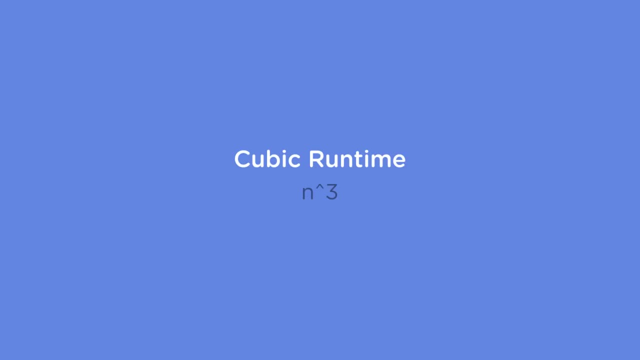 last, equal midpoint minus one. Let's visualize this. We're going to start with a list of nine integers. To make this easier to understand, let's specify these integers to be of the same value as its index position. So we have a range of values from zero to eight. 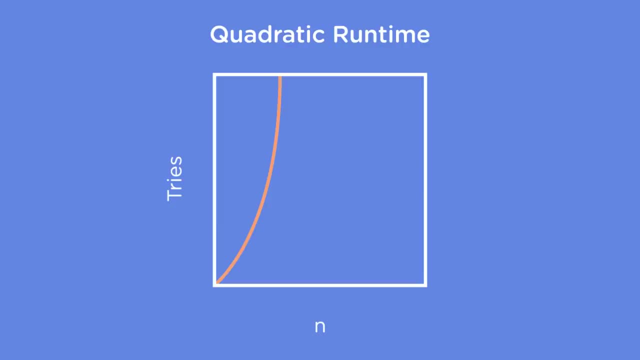 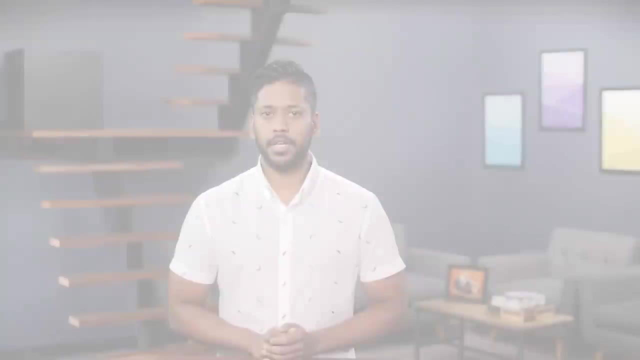 Our target is the worst case scenario. We're looking for the position of the value eight. At the start, our algorithm sets first to point to the index zero and last to point to the length of the list minus one, which is eight. Next we hit. 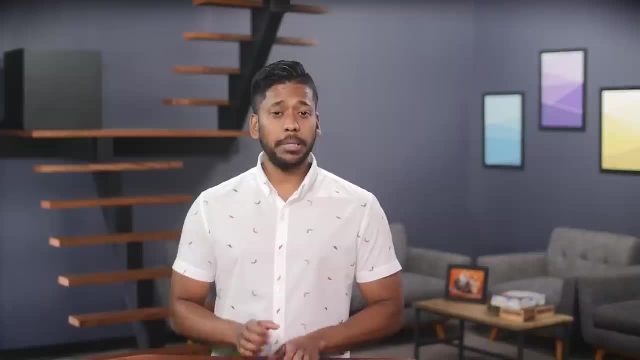 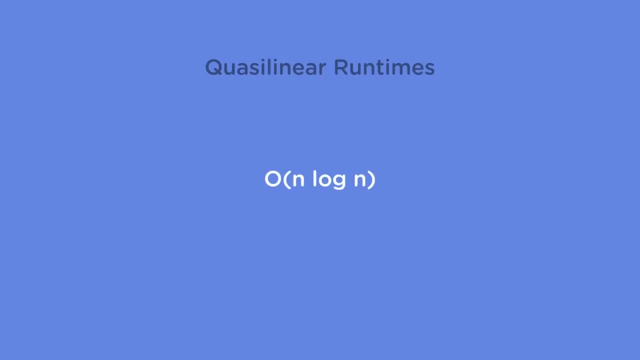 our while loop. The logic of this loop is going to be executed as long as the value of first is not greater than the value of last. Or, as we've defined it, we're going to keep executing the contents of the loop as long as first is less. 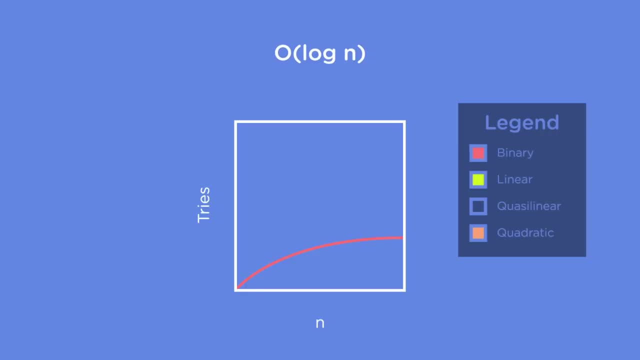 than or equal to last. On the first pass this is true. so we enter the body of the loop. The midpoint is first plus last, divided by two and rounded down, so we get a nice even four. The value at this position is four. Now, this is not equal to. 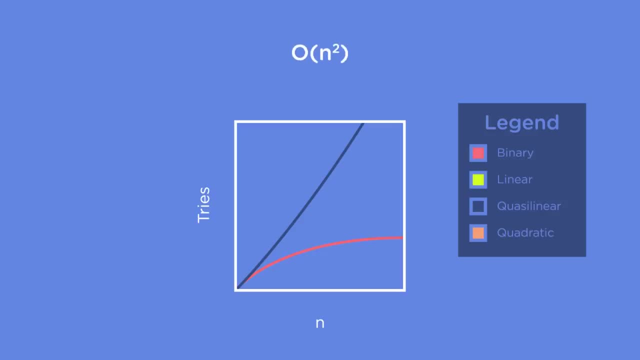 the target. so we move to the first, else if Four is less than eight. so now we redefine first to point to midpoint plus one, which is five. First is still less than last, so we run through the body of the loop again. The midpoint is now six. 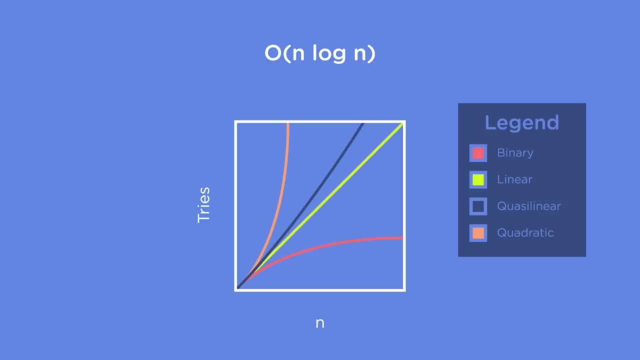 Six is less than eight, so we move first to point to seven. Seven is still less than or equal to eight, so we go for another iteration of the loop. The midpoint is seven, oddly enough, and seven is still less than the target, so we move. 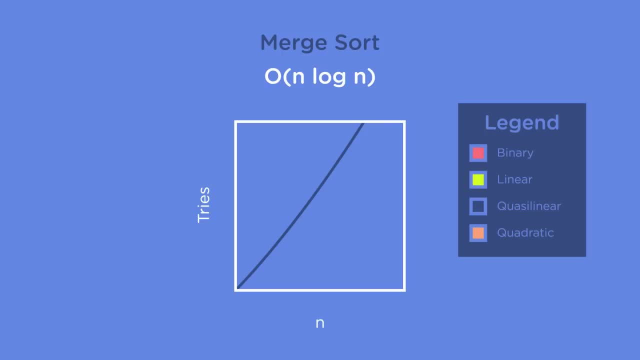 first to point to eight. First is equal to last. now, but our condition says: keep the loop going as long as first is less than or equal to last. So this is our final time through the loop. The midpoint is now eight, which makes the value at the midpoint 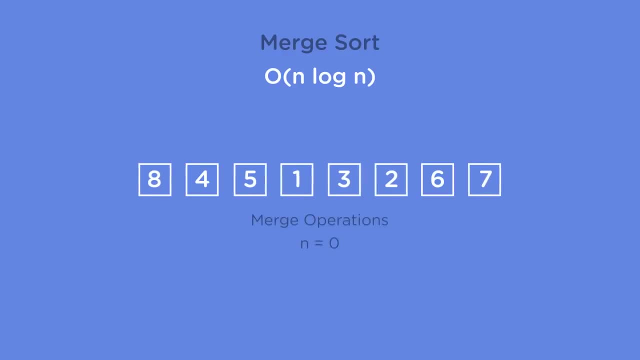 equal to the target and we finally exit our algorithm and return the position of the target. Now, what if we had executed all this code and never hit a case where midpoint equal the target? Well, that would mean the list did not contain the target value. so after the while, 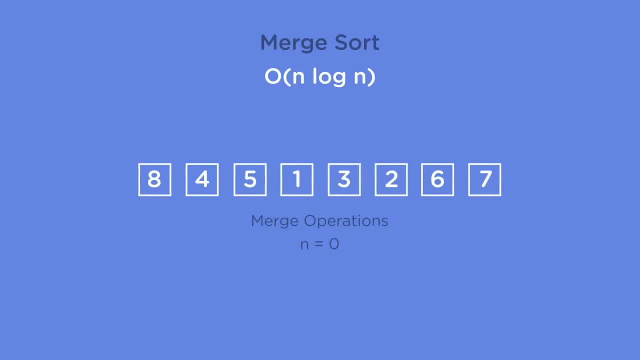 It keeps doing this until we end up with a list of just a single number. When we're down to single numbers, we can do one sort operation and merge these sublists back in the opposite direction. The first part of mergesort cuts those lists. 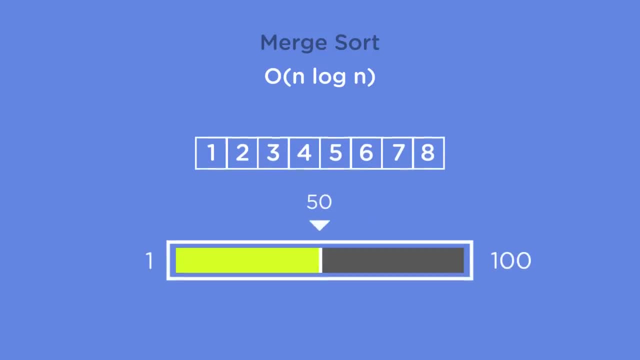 into sublists with half the numbers. This is similar to binary search, where each comparison operation cuts down the range to half the values. You know, the worst-case runtime in binary search is log n, so these splitting operations have the same runtime: O or logarithmic. 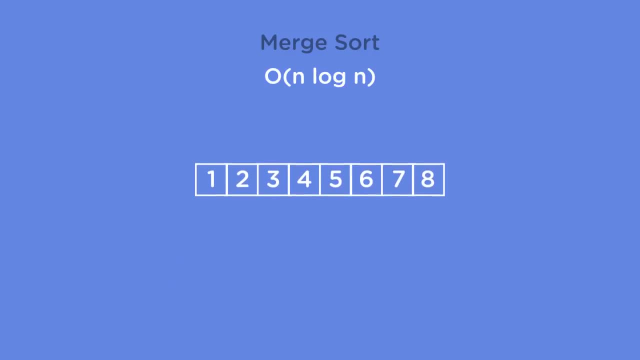 But splitting into half isn't the only thing we need to do with mergesort. We also need to carry out comparison operations so we can sort those values. And if you look at each step of this algorithm, we carry out an n number of comparison operations. 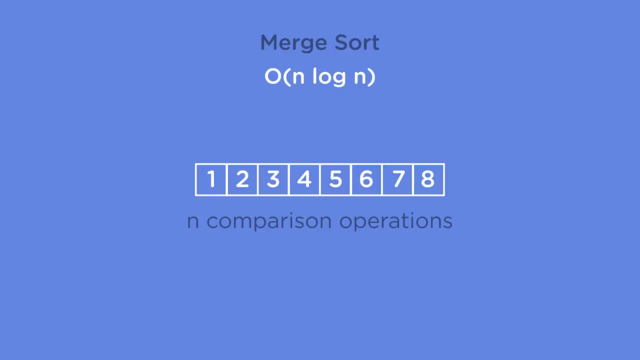 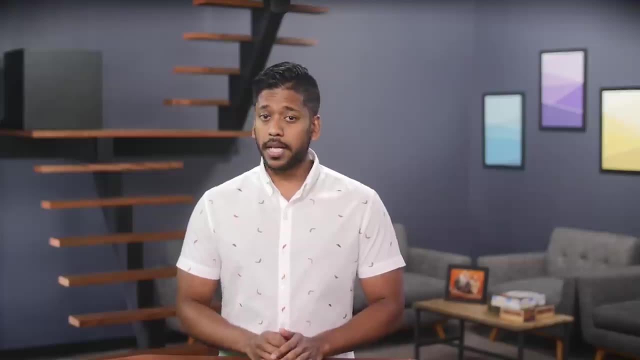 And that brings the worst-case runtime of this algorithm to n times log n, also known as quasi-linear. Don't worry if you didn't understand how mergesort works. That wasn't the point of this demonstration. We will be covering mergesort soon. 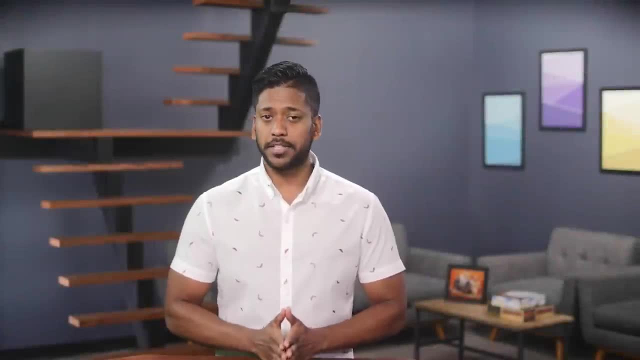 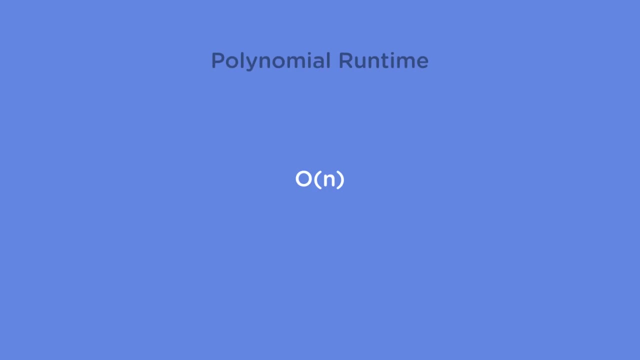 in a future course. The runtimes we've looked at so far are all called polynomial runtimes. An algorithm is considered to have a polynomial runtime if, for a given value of n, its worst-case runtime is in the form of n raised to the k power. 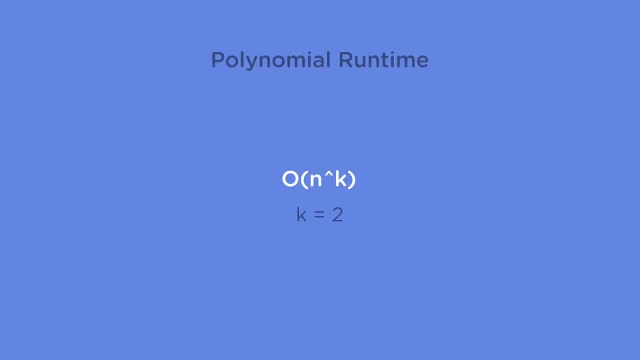 where k just means some value. So it could be n squared where k equals 2 for a quadratic runtime, n cubed for a cubic runtime, and so on. All of those are in the form of n raised to some power, Anything that is bounded by this. 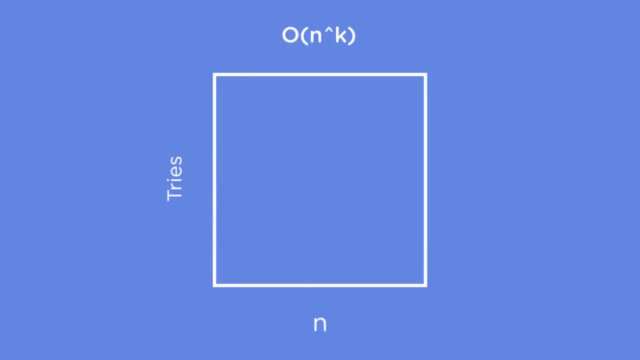 and what I mean by that is if we had a hypothetical line on our graph of n raised to the k power. anything that falls under this graph is considered to have a polynomial runtime, Algorithms with an upper bound or a runtime with a big O value. 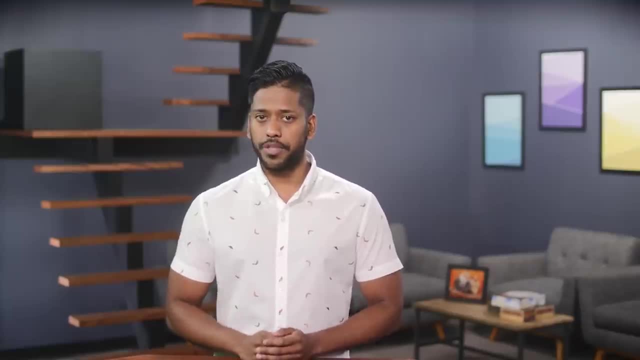 that is, polynomial, are considered efficient algorithms and are likely to be used in practice. Now, the next class of runtimes that we're going to look at are runtimes that we don't consider efficient, and these are called exponential runtimes. With these runtimes, 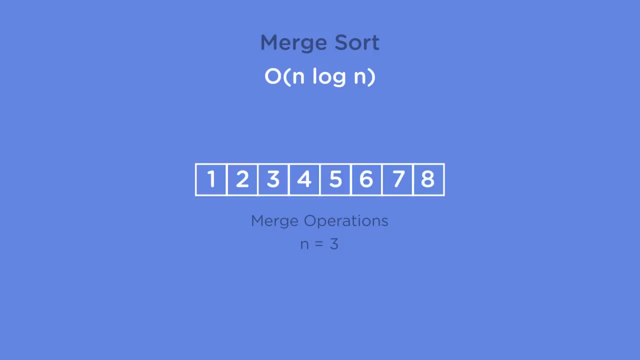 loop at the bottom, we'll return none. We have several operations that make up our binary search algorithm, so let's look at the runtime of each step. We start by assigning values to first and last. The value assigned to last involves a call to the len function to get the size. 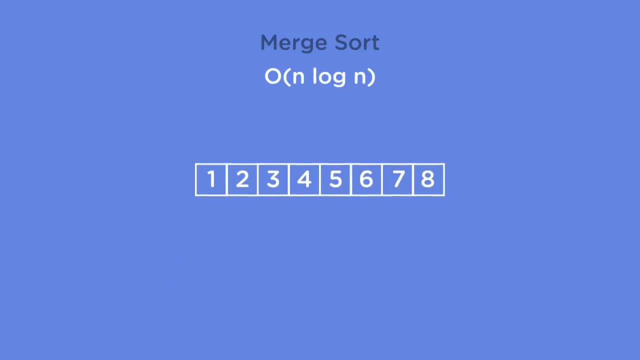 of the list. but we already know this is a constant time operation in Python, so both of these operations run in constant time. Inside the loop we have another value assignment and this is a simple division operation. so again, the runtime is constant. In the next line of code, 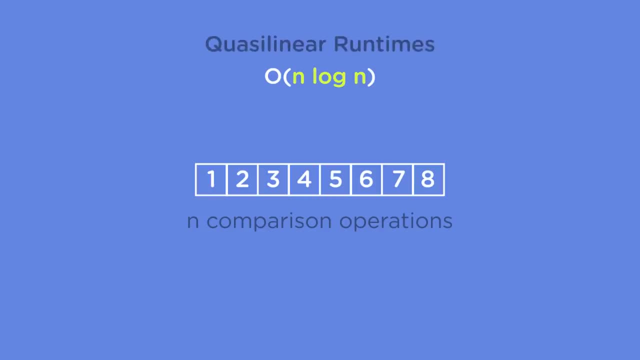 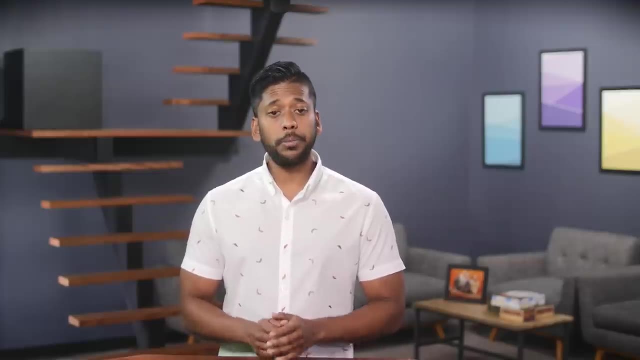 we're reading a value from the list and comparing the midpoint to the target. Both of these, again, are constant time operations. The remainder of the code is just a series of comparisons and value assignments, and we know that these are all constant time operations as well. So if all we have 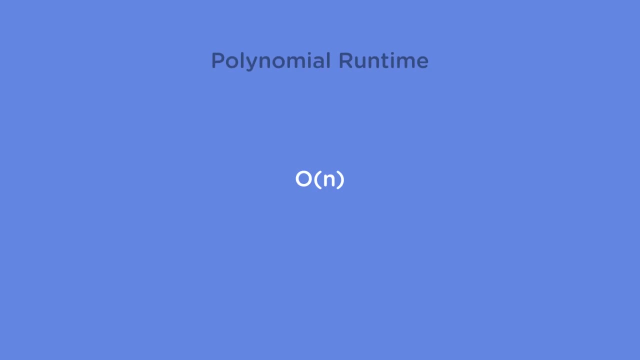 are a series of constant time operations. why does this algorithm have, in the worst case, a logarithmic runtime? It's hard to evaluate by just looking at the code, but the while loop is what calls the runtime to grow, Even though all we're doing is a. 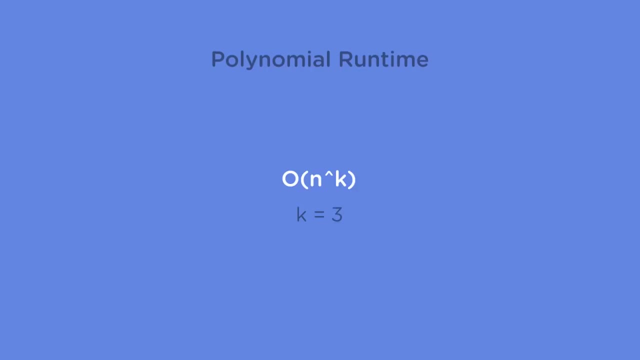 comparison operation by redefining first and last. over here, or rather in the last two steps over here, we're asking the algorithm to run as many times as it needs until first is equal or greater than last. Now, each time the loop does this the size. 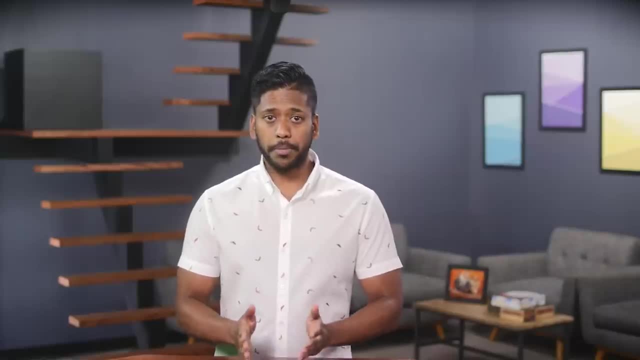 of the dataset. the size of the list grows smaller by a certain factor until it approaches a single element, which is what results in the logarithmic runtime. Okay, just like with linear search, let's test that our algorithm works. So we'll. 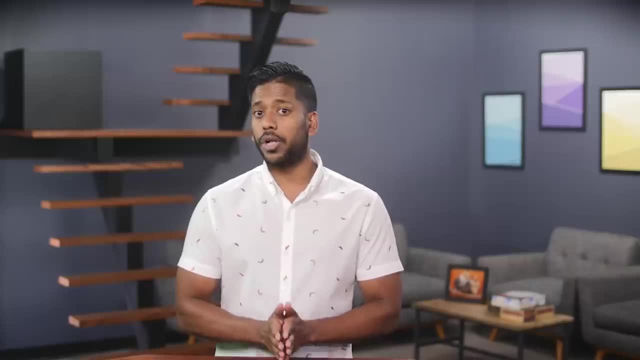 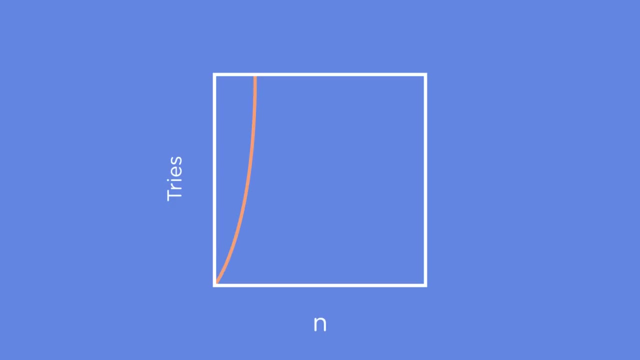 go back to LinearSearchpy and we're going to copy paste. so Command C to copy. if you're on a Mac, then go back to Binary Search and at the bottom, oops, we're going to paste in that verify function. Okay, we'll also go back. 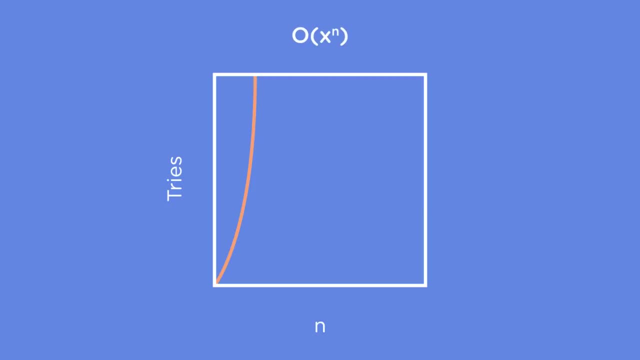 and grab this numbers. you know what? let's go ahead and copy all all of these things. so numbers and the two verify cases. we'll paste that in as well, and the only thing we need to change here is, instead of calling LinearSearch, this is going to call BinarySearch. 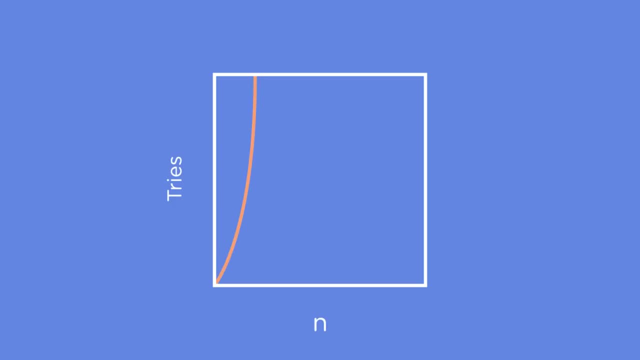 as n increases slightly, the number of operations increases exponentially And, as we'll see in a second, these algorithms are far too expensive to be used. An exponential runtime is an algorithm with a big O value of some number raised to the nth power. 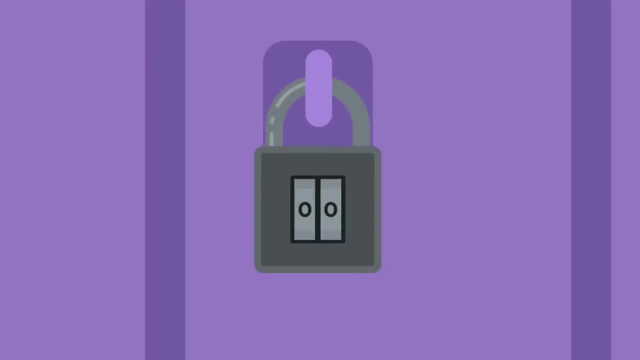 Imagine that you wanted to break into a locker that had a padlock on it. Let's assume you forgot your code. This lock takes a two-digit code and the digit for the code ranges from 0 to 9.. You start by setting the dials to 0,. 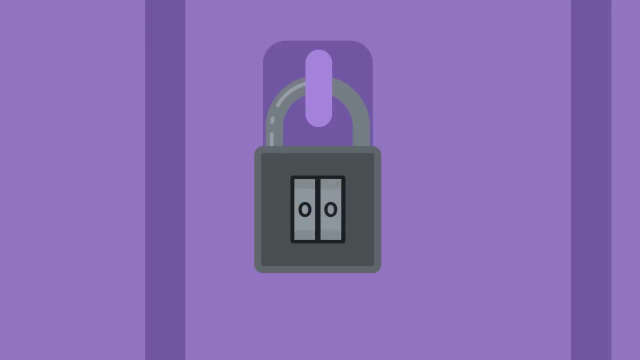 and then, with the first dial remaining on 0,, you change the second dial to 1 and try and open it. If it doesn't work, you set it to 2, then try again. You would keep doing this and if you still haven't succeeded, 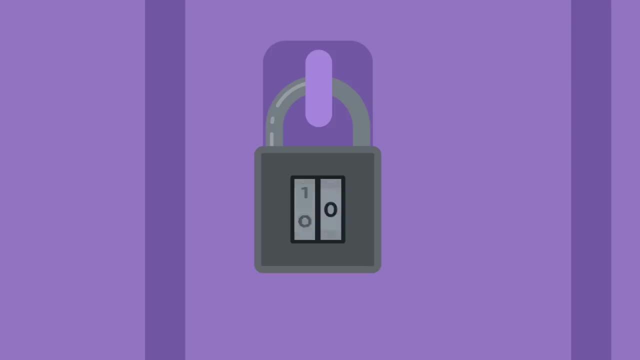 with the second dial set to 9,. then you go back to that first dial, set it to 1, and start the second dial over. The range of values you'd have to go through is 0, 0 to 9, 9,. 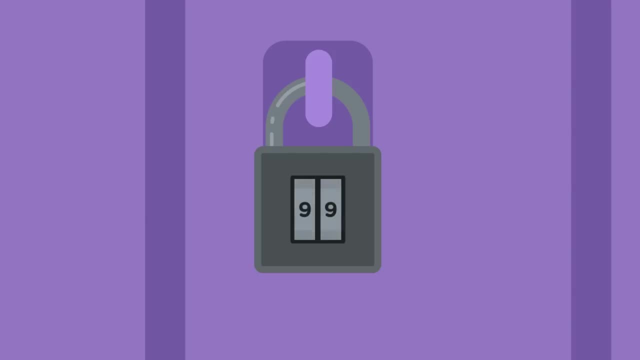 which is 100 values. This can be generalized as 10 to the second power, since there are 10 values on each dial raised to two dials. Searching through each individual value until you stumble on the right one is a strategy called brute force. 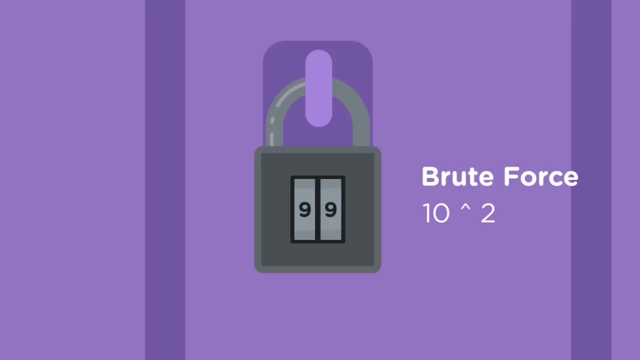 and brute force algorithms have exponential runtimes. Here there are two dials, so n is 2, and each dial has 10 values. so again we can generalize this algorithm as 10 raised to n, where n represents the number of dials. 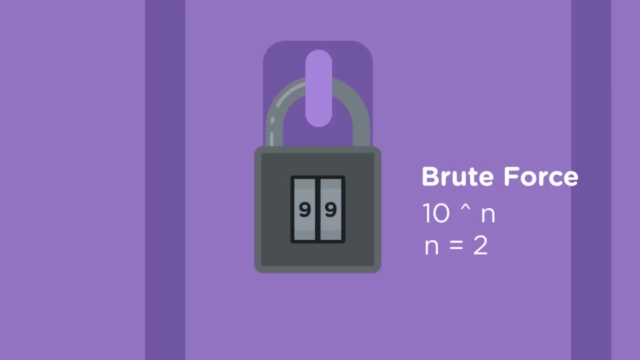 The reason that this algorithm is so inefficient is because with just one more dial on the lock, the number of operations increases significantly. With three dials, the number of combinations. in the worst-case scenario, where the correct code is the last digit in the range. 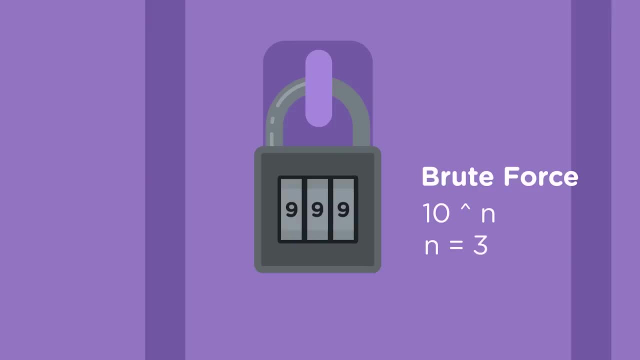 is 10 raised to 3, or 1,000 values. With an additional wheel it becomes 10, raised to 4, or 10,000 values. As n increases, the number of operations increases exponentially to a point where it's unsolvable in a realistic amount of time. 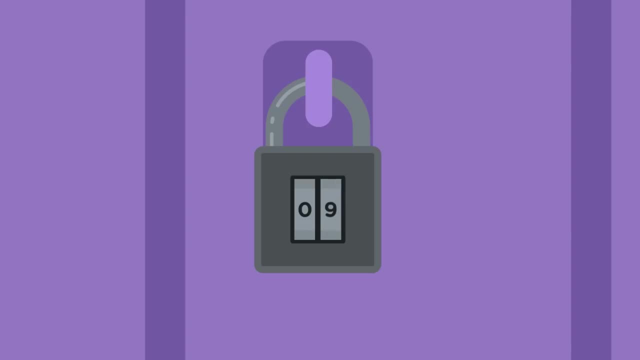 Okay, we'll hit Command S to save the file, and then I'm going to drag up my console and we'll run Python, BinarySearchpy, and hit enter And you'll see just like before. we get the same results back. Now, note that an extremely 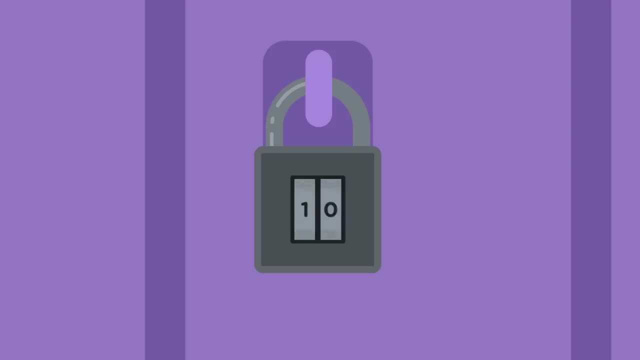 important distinction needs to be made here. The numbers list that we've defined for our test cases right here has to be sorted. The basic logic of BinarySearch relies on the fact that if the target is greater than the midpoint, then our potential values lie to the left or 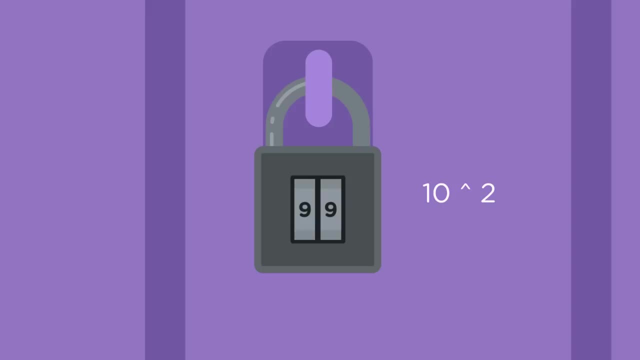 vice versa, since the values are sorted in ascending order. If the values are unsorted, our implementation of BinarySearch may return none, even if the value exists in the list. And just like that, you've written code to implement two search algorithms. How fun was that. 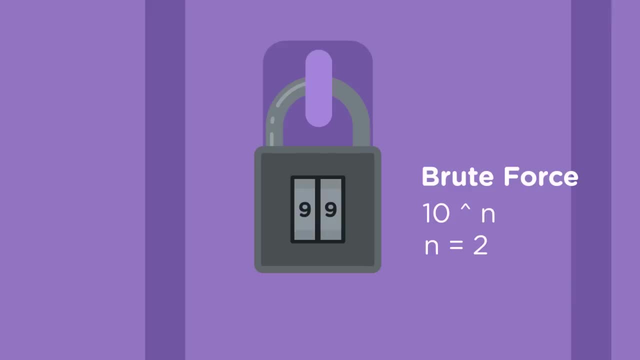 Hopefully this course has shown you that it isn't a topic to be afraid of and that algorithms, like any other topic with code, can be broken down and understood piece by piece. Now we have a working implementation of BinarySearch, But there's actually more than one way to write it. 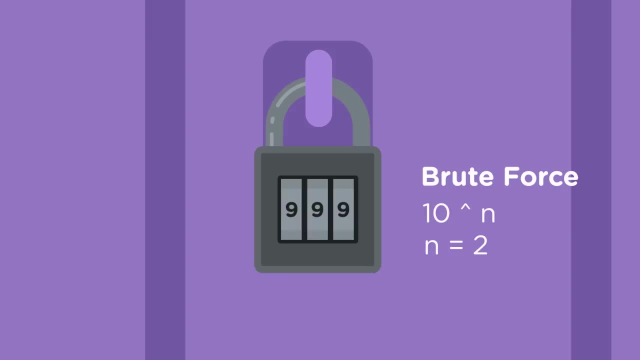 So in the next video, let's write a second version. I'm going to create a new file, as always, file, new file, And we'll name this recursive underscore, binary underscore, search dot py. Okay, so we're going to add our new implementation. 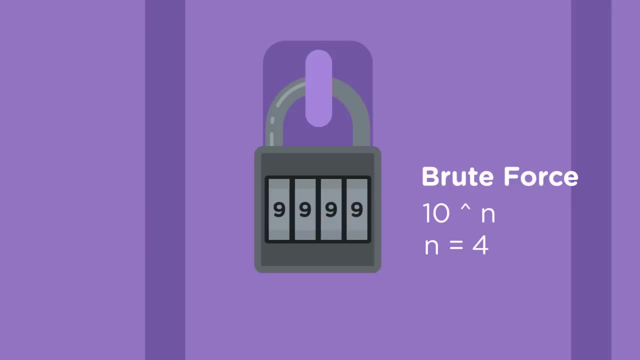 here so that we don't get rid of that first implementation. we wrote: Let's call this new function recursive binary search. Unlike our previous implementation, this version is going to behave slightly differently in that it won't return the index value of the target element. 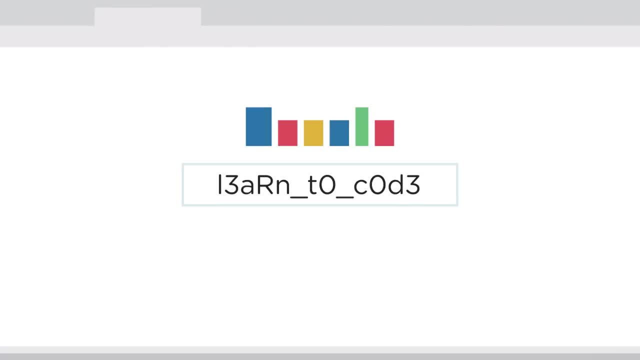 if it exists. Instead, it will just return a true value if it exists and a false if it doesn't. So recursive underscore, binary underscore search and, like before, this is going to take a list. it accepts a list and a target to look for. 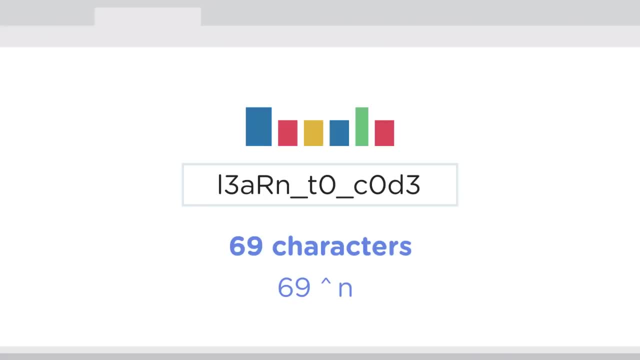 in that list. We'll start the body of the function by considering what happens if an empty list is passed in. In that case we would return false. So I would say if the length of the list, which is one way to figure out if it's empty. 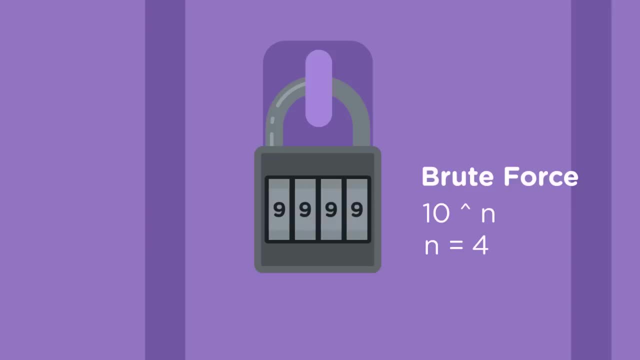 Now you might think: well, any computer can crack a four-digit numerical lock, and that's true because n here is sufficiently small. But this is the same principle that we use for passwords In a typical password field, implemented well. 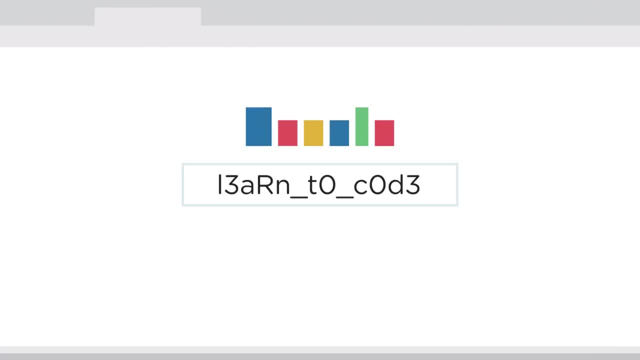 users are allowed to use letters of the English alphabet, so up to 26 characters, numbers from 0 to 9, and a set of special characters, of which there can be around 33.. So typically that means each character in a password. 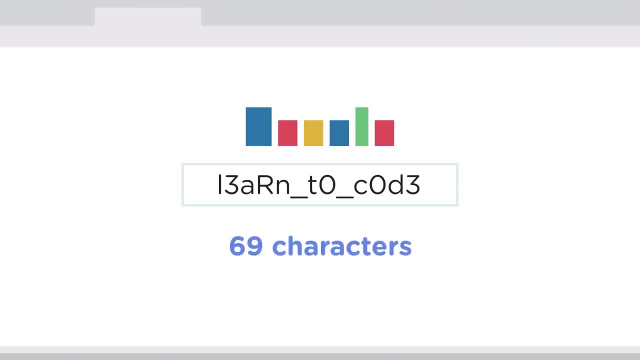 can be 1 out of 69 values. This means that for a one-character password it takes 69 to the nth power. so 1, which equals 69 operations in the worst-case scenario to figure out the password, Just increasing n to 2. increases the number of operations needed to guess the password to 69 squared or 4,761 operations. Now, usually on a secure website, there isn't really a limit, but in general, passwords are limited to around 20 characters in length. 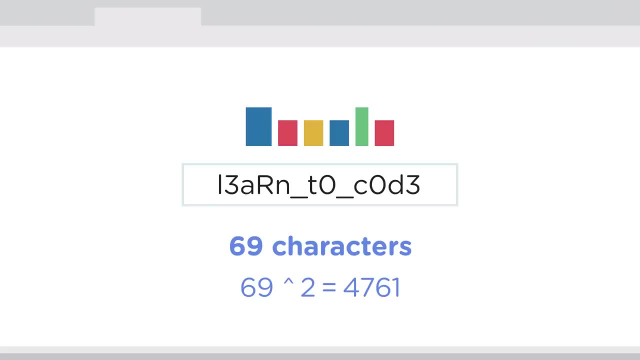 With each character being a possible 69 values and there being 20 characters, the number of operations needed to guess the password in the worst-case scenario is 69 raised to the 20th power, or approximately 6, followed by 36 zeros. 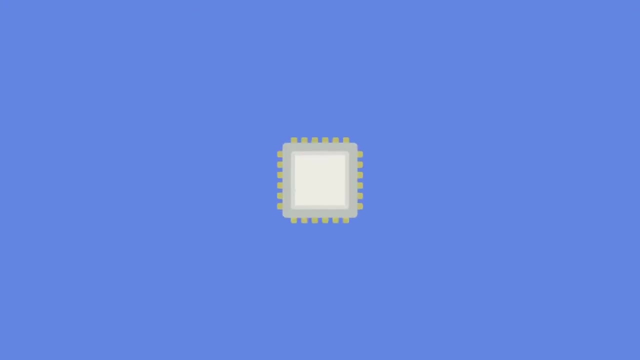 number of operations. An Intel CPU with five cores can carry out roughly about 65,000 million instructions per second. That's a funny number, I know. To crack our 20-digit passcode in this very simplistic model, it would take this Intel CPU. 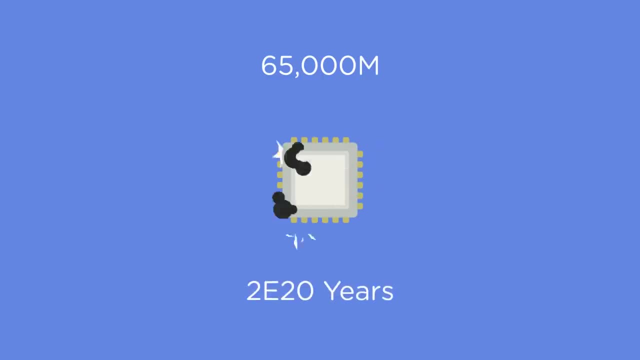 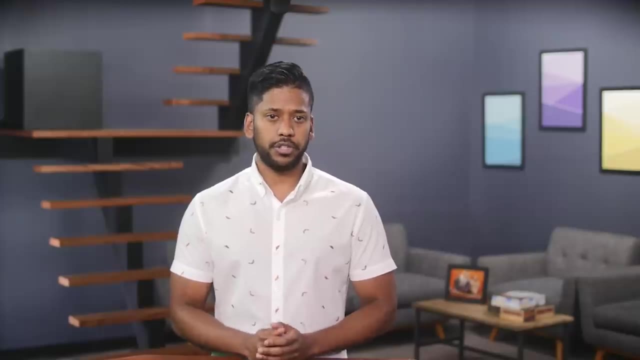 2 raised to the 20th power years to brute force the password. So, while this algorithm would eventually produce a result, it is so inefficient that it's pointless. This is one of the reasons why people recommend you have longer passwords, Since brute forcing is exponential. 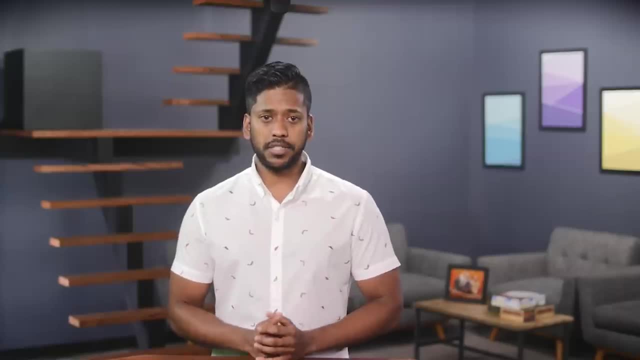 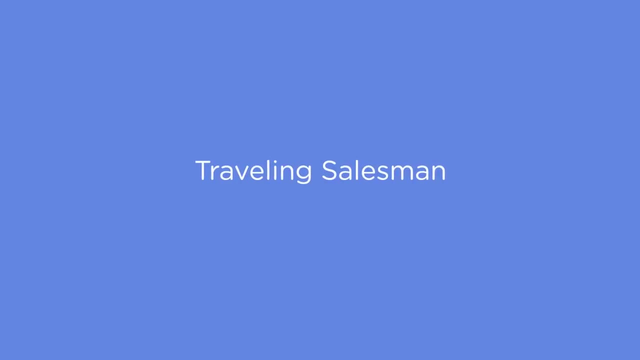 in the worst case, each character you add increases the number of combinations by an exponent. The next class of exponential algorithms is best highlighted by a popular problem known as the traveling salesman. The problem statement goes like this: Given a list of cities and the distance between, 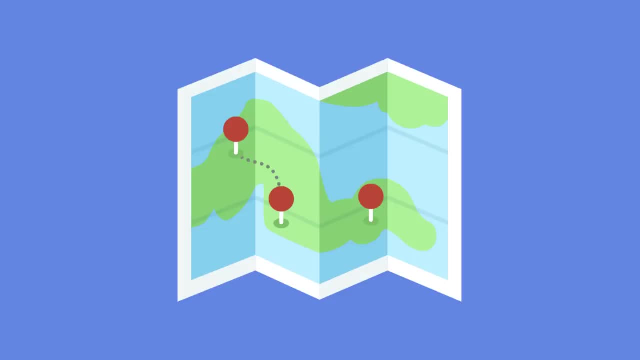 each pair of cities. what is the shortest possible route that visits each city and then returns to the origin city? This seems like a simple question, but let's start with a simple case- Three cities, A, B and C- To figure out what the shortest route is. 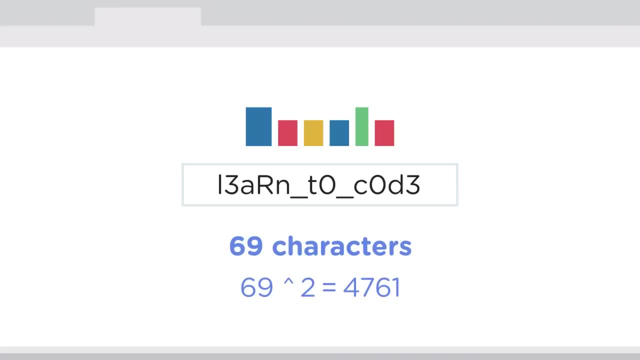 if it's equal to zero, then we'll return false. Now you might be thinking that in the previous version of binary search we didn't care if the list was empty. Well, we actually did, but in a roundabout sort of way. So in the previous version of binary search, 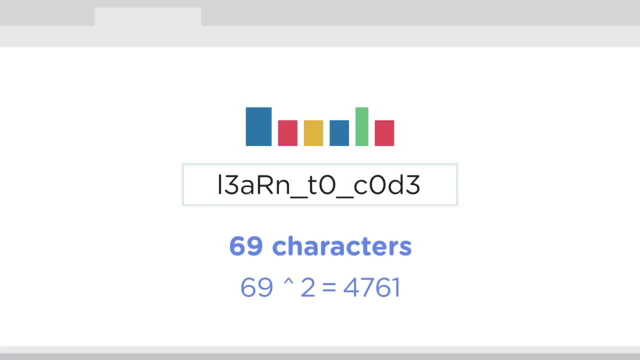 our function had a loop and that loop condition was true when first was less than or equal to last. So as long as it's less than or equal to last, we continue the loop. Now, if we have an empty list, then first is greater than last. 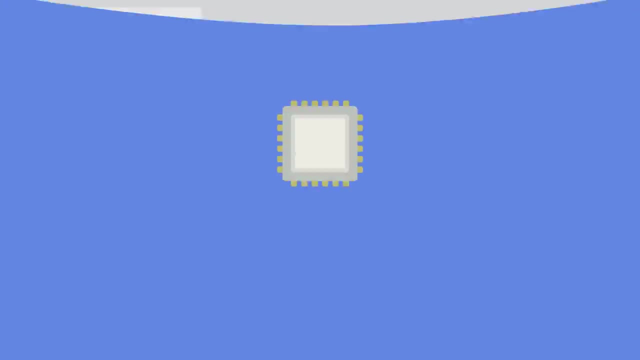 and the loop would never execute, and we return none at the bottom. So this is the same logic we're implementing here. we're just doing it in a slightly different way. If the list is not empty, we'll implement an else clause. Now, here we'll calculate the midpoint. 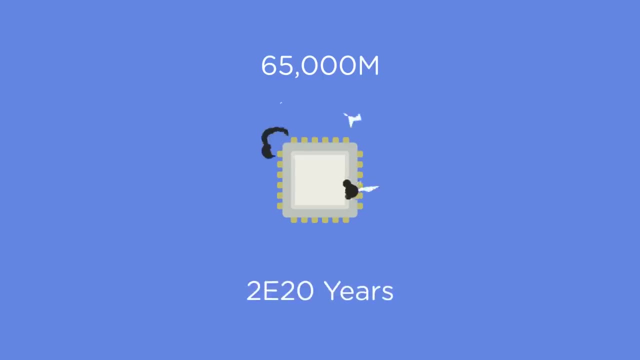 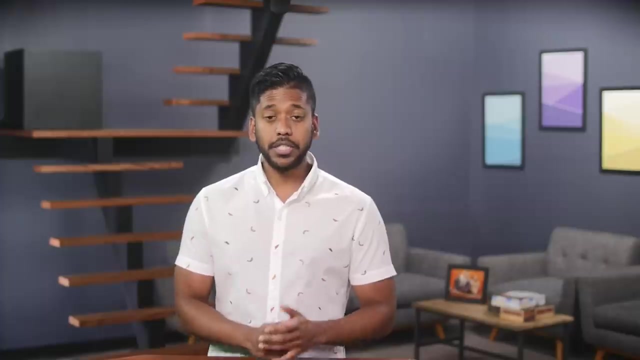 by dividing the length of the list by two and rounding down Again. there's no use of first and last here, So we'll say length of list and then, using the floor division operator, we'll divide that by two. If the value at the midpoint 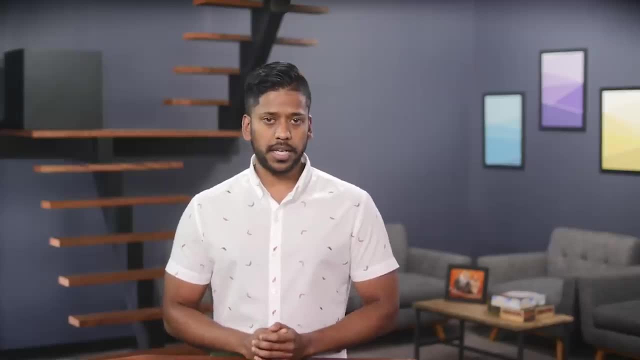 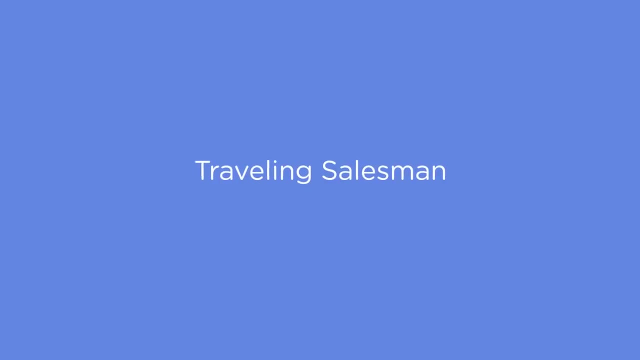 which we'll check by saying: if list using subscript notation, we'll say midpoint as the index. now if this value at the midpoint is the same as the target, then we'll go ahead and return true. So far, this is more or less the same, except for the value that we're returning. 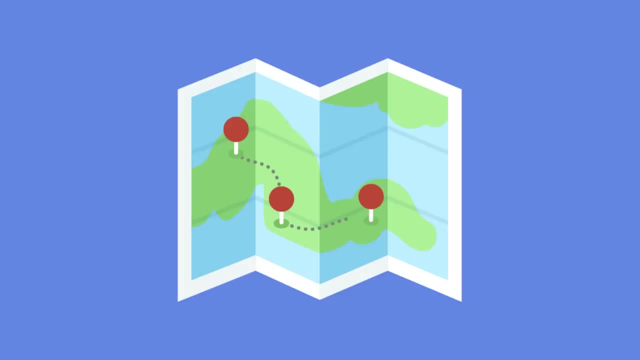 Let me actually get rid of all that. Okay, Alright. So if this is in the case, let's implement an else clause. Now here we have two situations. so first, if the value at the midpoint is less than the target. so if value at midpoint 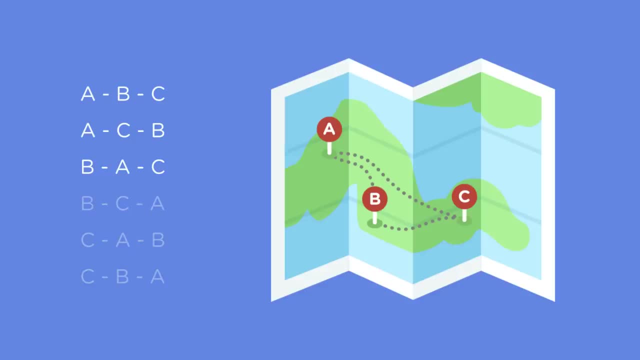 is less than the target, then we're going to do something new. then we're going to do something new. we're going to call this function again, This recursive binary search function that we're in the process of defining. we're going to call that again and we're going to give it the portion. 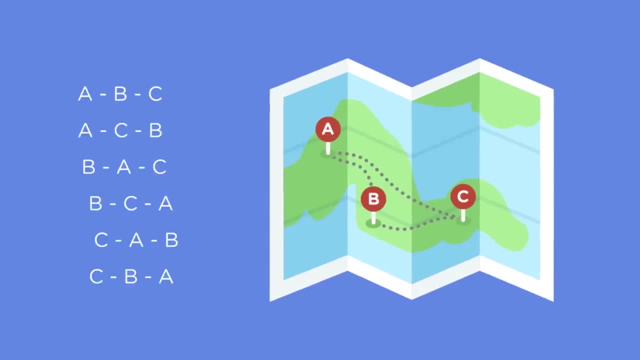 we need to come up with all the possible routes. With three cities we have six routes. In theory, at least Some of these routes can be discarded, because ABC is the same as CBA, but in the opposite direction. But as we do know, sometimes 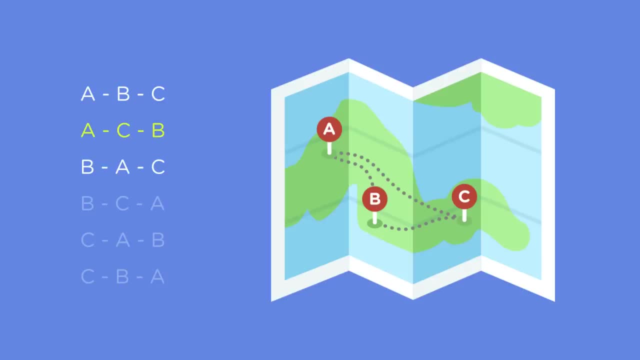 going from A to C through B may go through a different route than C to A through B, So we'll stick to the six routes and from there we could determine the shortest. No big deal Now if we increase this to four cities. 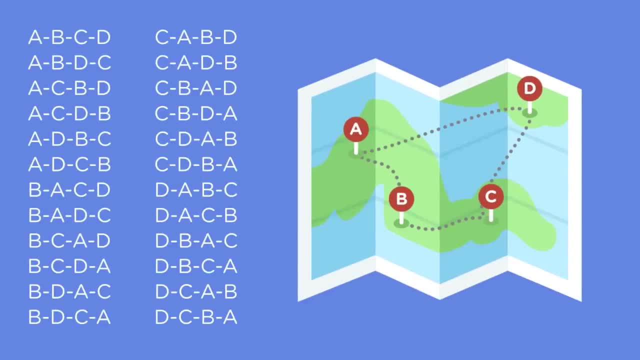 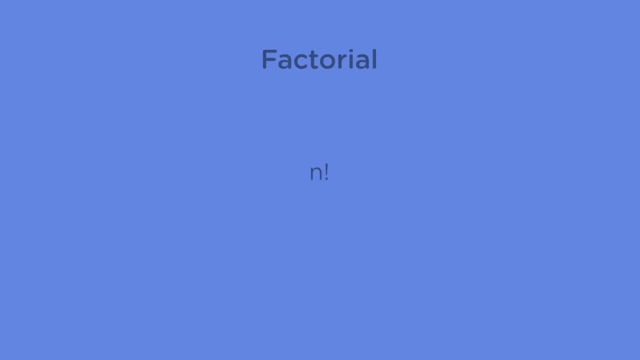 we jump to 24 combinations. The mathematical relationship that defines this is called a factorial and is written out as N, followed by an exclamation point. Factorials are basically N times N minus one, repeated until you reach the number one. So, for example: 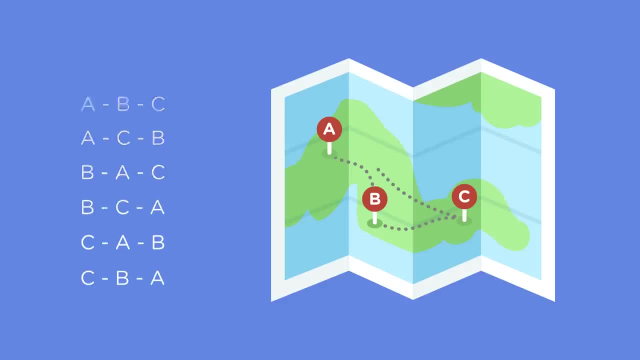 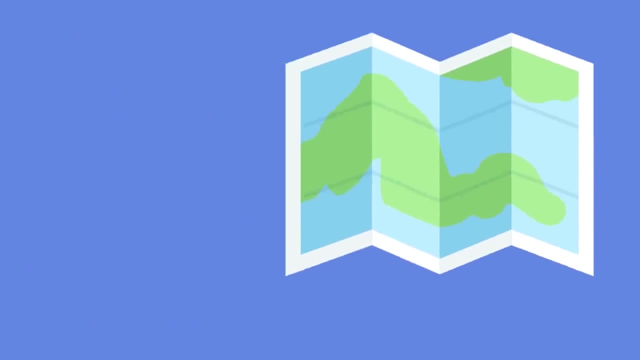 of the list that we want to focus on. In the previous version of binary search, we moved the first value to point to the value after the midpoint. Now, here we're going to create a new list using what is called a slice operation and create a sublist. 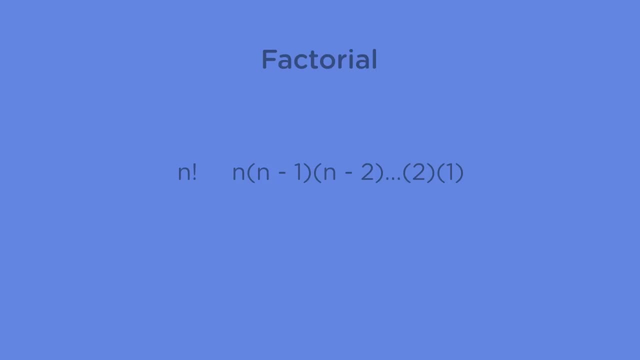 that starts at midpoint plus one and goes all the way to the end. We're going to specify the same target as our search target and when this function call is done we'll return the value. So we'll say return. the return is important, then we'll call this function again. 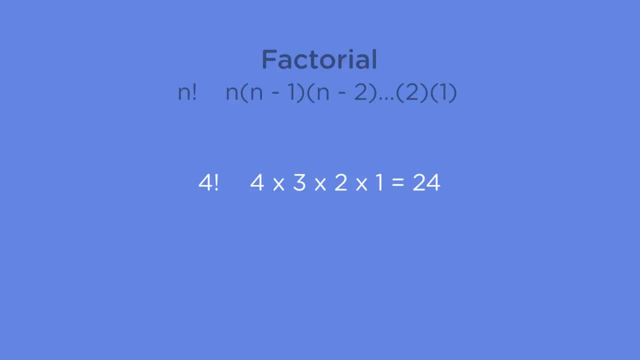 recursive binary search and this function takes a list and here we're going to use that subscript notation to perform a slice operation by using two indexes, a start and an end. So we'll say our new list that we're passing in, and then we'll go all the way. 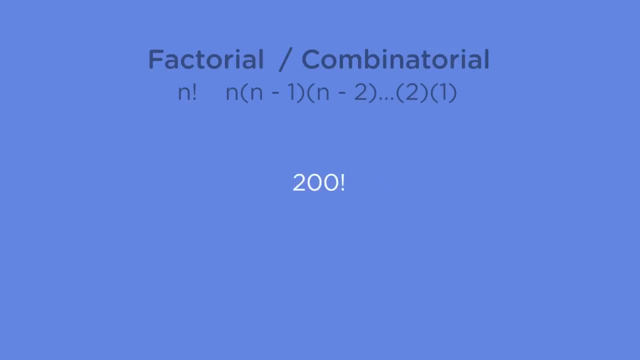 to the end, and this is a Python syntactic sugar, so to speak. If I don't specify an end index, Python knows to just go all the way to the end, Alright, so this is our new list that we're working with, and we need a target. 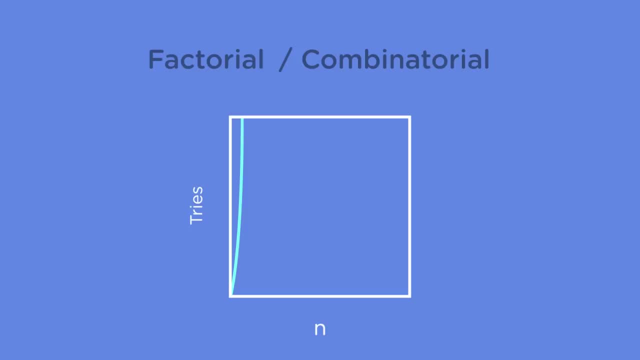 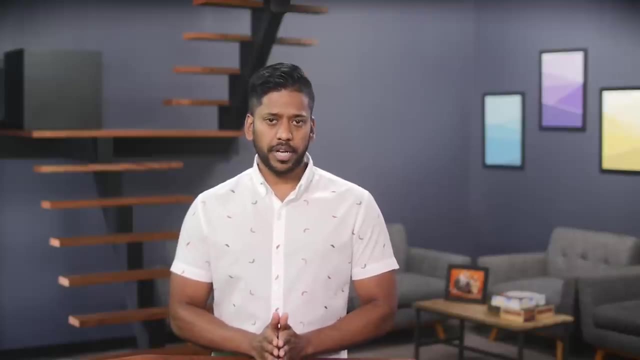 we'll just pass it through. If you're confused, bear with me just like before. we'll visualize this at the end. Okay, we have another else case here, and this is a scenario where the value at the midpoint is greater than the target. This means we only care about the values in the list. 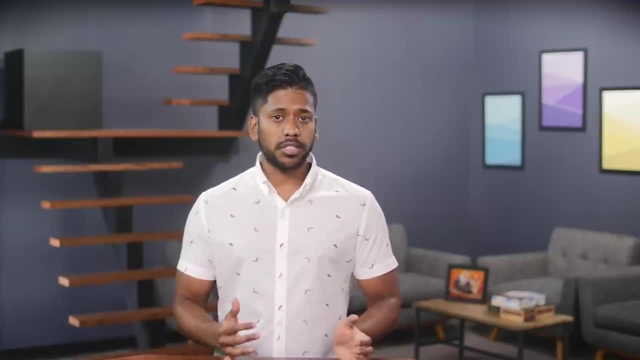 from the start, going up to the midpoint. Now, in this case as well, we're going to call the binary search function again and specify a new list to work with. This time, the list is going to start at the beginning and then go all the way up to the midpoint. 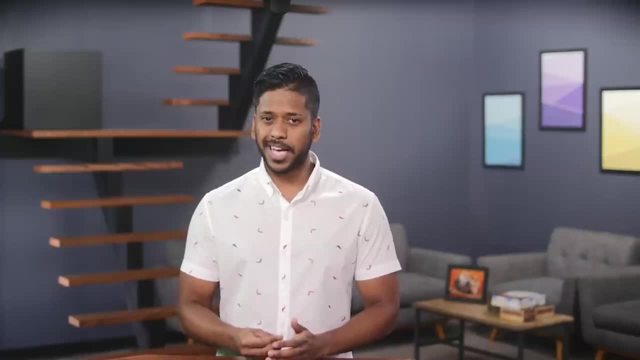 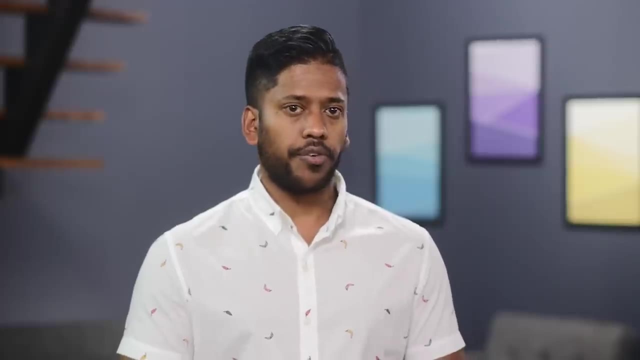 So it looks the same. we'll say: return recursive binary search. we're going to pass in a list here. so if we just put a colon here without a start index and we're going to go all the way up to the midpoint, the target here is the same. 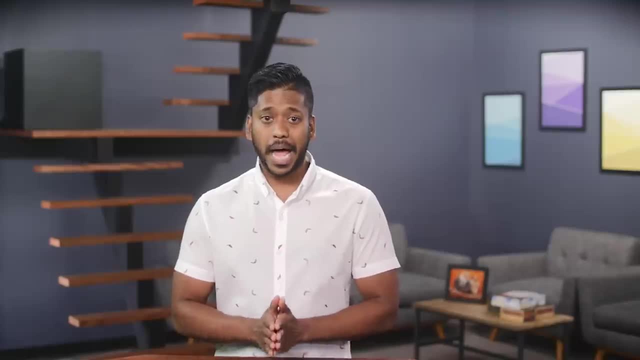 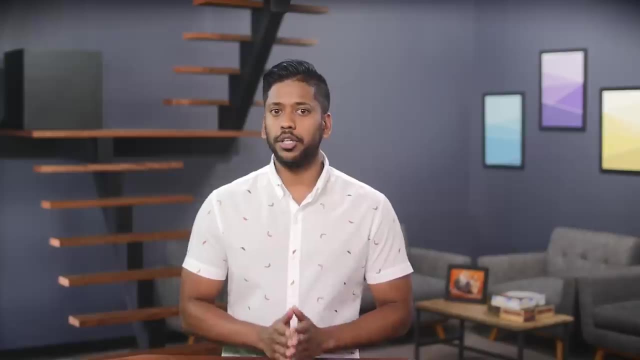 and this is our new binary search function. so let's see if this works actually. yes, down here we'll make some space and we'll define a verify function. we're not going to copy paste the previous one, because we're not returning none or an integer here. 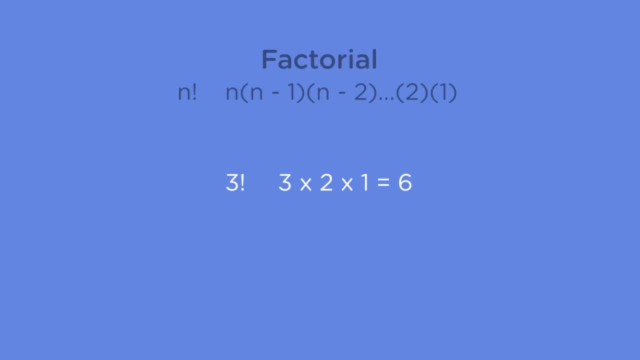 the factorial of three is three times two times one, which is six, which is the number of combinations we came up with for three cities. The factorial of four is four times three times two times one or 24,, which is the number of combinations. 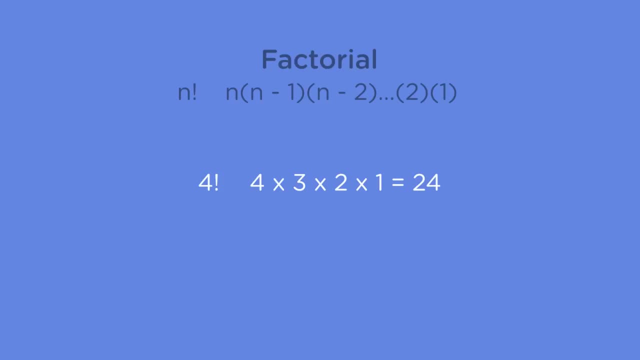 we arrived at with four cities. In solving the traveling salesman problem, the most efficient algorithm will have a factorial runtime, or a combinatorial runtime, as it's also called. At low values of N, algorithms with a factorial runtime may be used, but with an N value of, say, 200,. 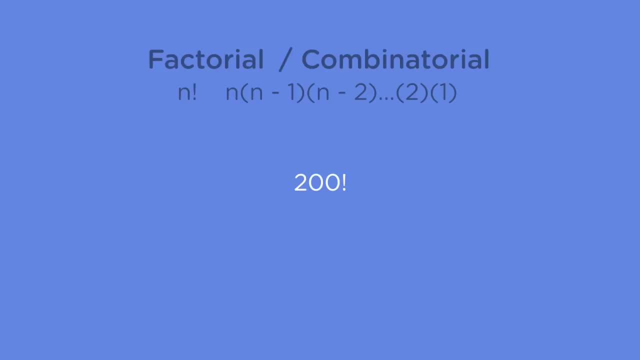 it would take longer than humans have been alive to solve the problem. For sake of completeness, let's plot a combinatorial runtime on our graph so that we can compare. An algorithm such as one that solves the traveling salesman problem has a worst-case runtime. 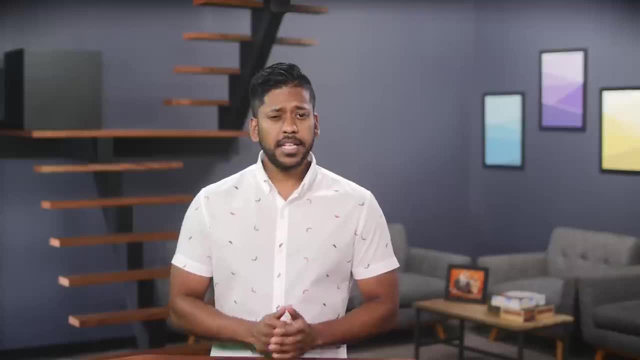 of O. Studying exponential runtimes like this are useful for two reasons. First, in studying how to make such algorithms efficient, we develop strategies that are useful across the board and can potentially be used to make existing algorithms even more efficient. Second, it's important to be aware of problems. 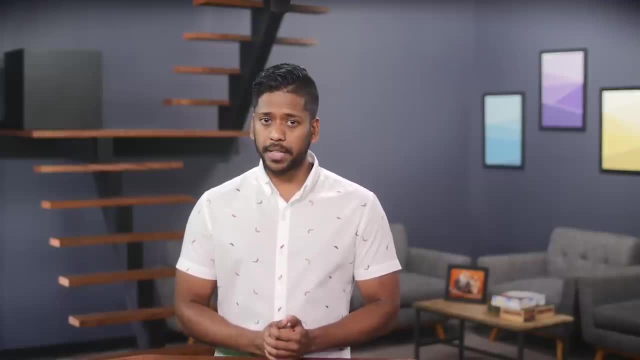 that take a long time to solve. Knowing right off the bat that a problem is somewhat unsolvable in a realistic time means you can focus your efforts on other aspects of the problem. As beginners, though, we're going to steer clear of all this. 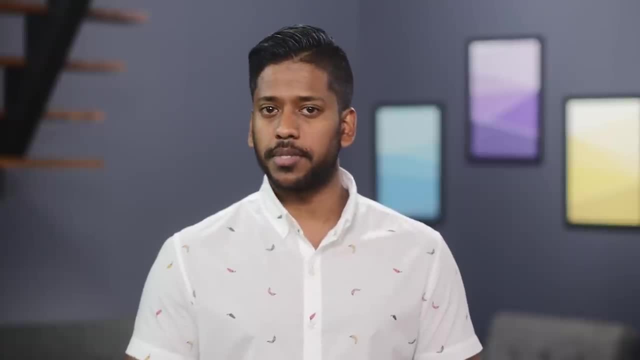 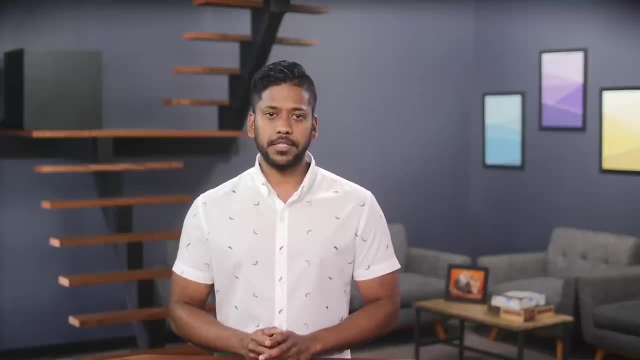 and focus our efforts on algorithms with polynomial runtimes, since we're much more likely to work with and learn about such algorithms Now that we know some of the common complexities. in the next video, let's talk about how we determine the complexity of an algorithm. 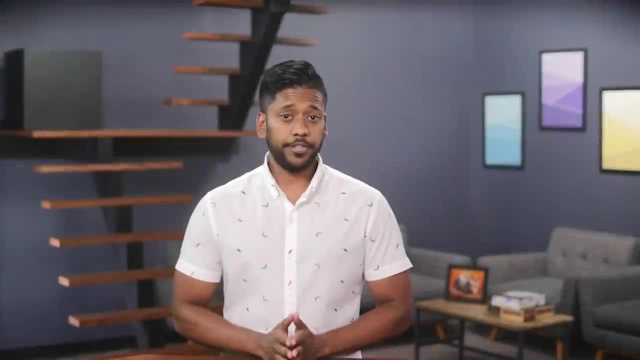 because there are some nuances. Over the last few videos we took a look at common complexities that we would encounter in studying algorithms, But the question remains: how do we determine what the worst-case complexity of an algorithm is? Earlier I mentioned that, even though we say 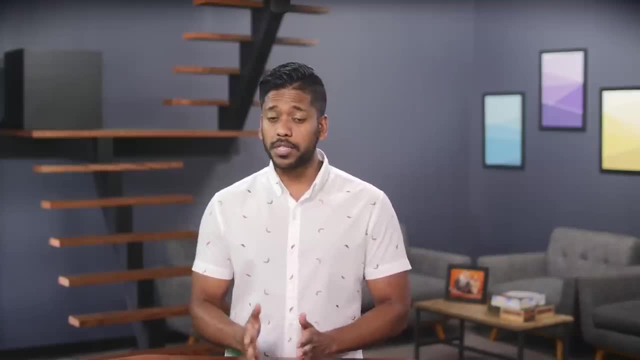 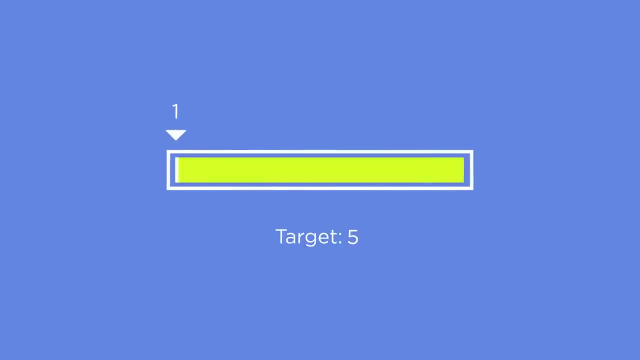 that an algorithm has a particular upper bound or worst-case runtime. each step in a given algorithm can have different runtimes. Let's bring up the steps for binary search again. Assuming the list is sorted, the first step is to determine the middle position of the list. 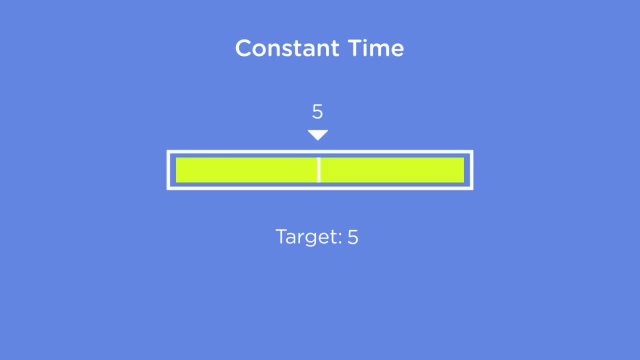 In general, this is going to be a constant-time operation. Many programming languages hold onto information about the size of the list, so we don't actually need to walk through the list to determine the size Now if we didn't have information about the size of the list. 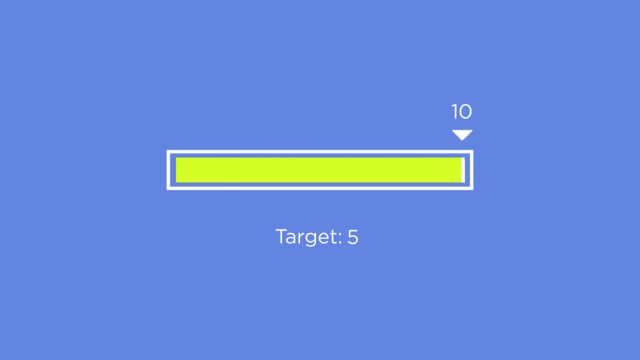 we would need to walk through counting each item one by one until we reach the end of the list, And this is a linear-time operation, But realistically this is a big O of 1, or constant time. Step 2 is to compare the element. 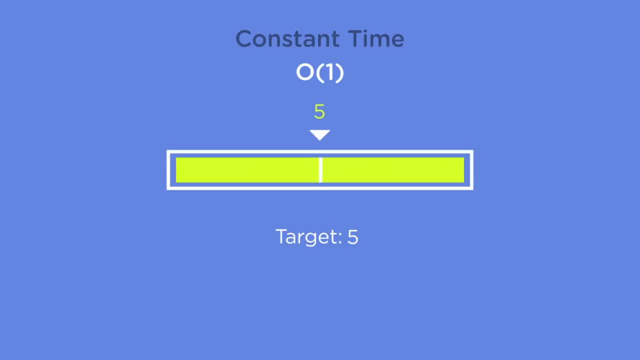 in the middle position to the target element. We can assume that in most modern programming languages this is also a constant-time operation, because the documentation for the language tells us it is. Step 3 is our success case and the algorithm ends. This is our best case. 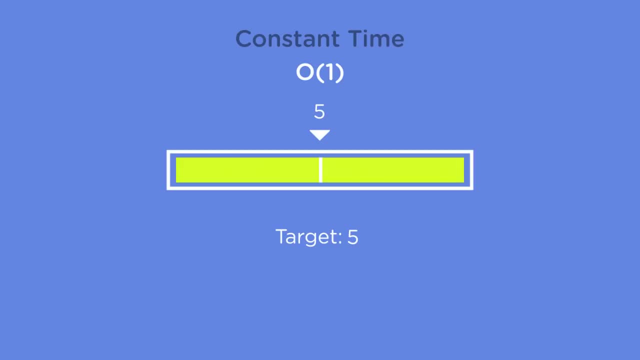 and so far we have only incurred two constant-time operations. So we would say that the best-case runtime of binary search is constant-time, which is actually true, But remember that best-case is not a useful metric. Step 4, if we don't match. 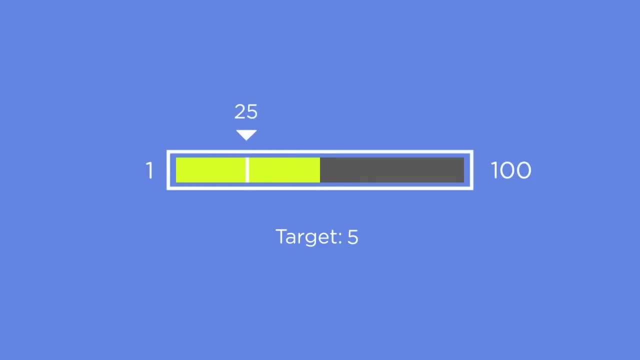 is splitting the list into sub-lists. Assuming the worst-case scenario, the algorithm would keep splitting into sub-lists until a single element list is reached with the value that we're searching for. The runtime for this step is logarithmic, since we discard half the values each time. 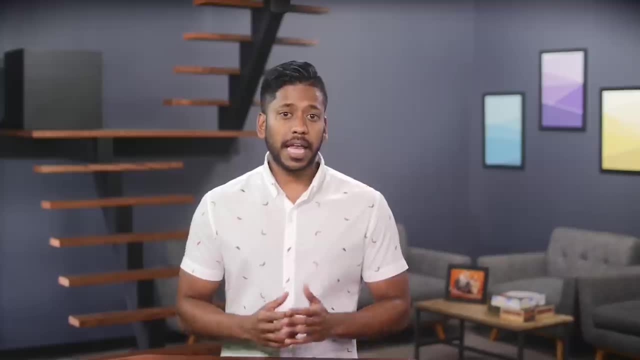 so we'll verify the result that we pass in and we'll say print found and this is just going to say true or false whether we found it. so, like before, we need a numbers list and we'll do something like 1, 2,, 3, 4, all the way up. 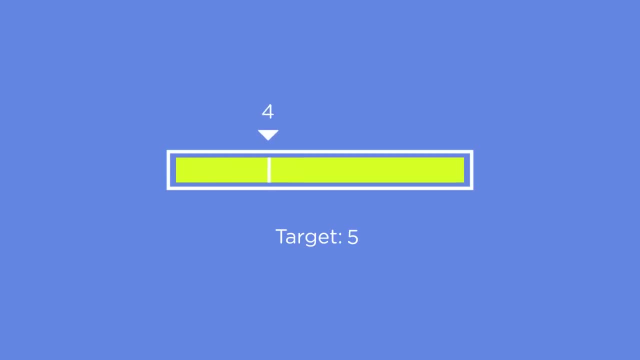 to 8. and now let's test this out. so we'll call our recursive binary search function and we'll pass in the numbers list and the target here is 12. we're going to verify this, verify the result, make sure it works and then we'll call it again. 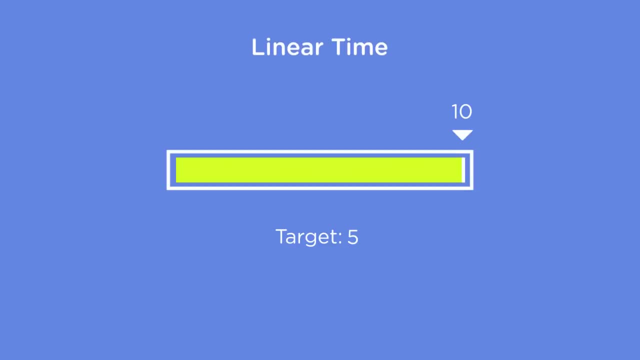 this time making sure that we give it a target that is actually in the list. so here we'll say 6 and we'll verify this again. make sure you hit command s to save and then in the console below we're going to type out: python: recursive binary search dot pi. 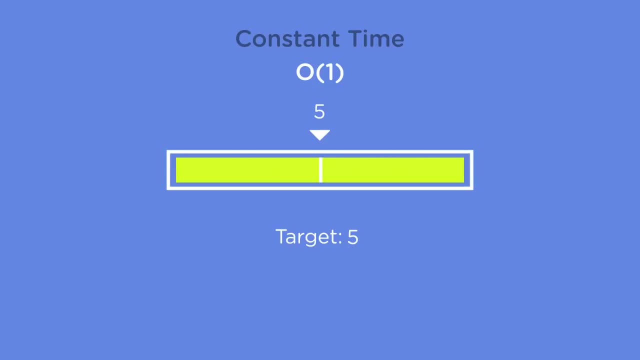 run it and you'll see that we verified that search works. while we can't verify the index position of the target value, which is a modification to how our algorithm works, we can guarantee, by running across all valid inputs, that search works as intended, so why write a different? 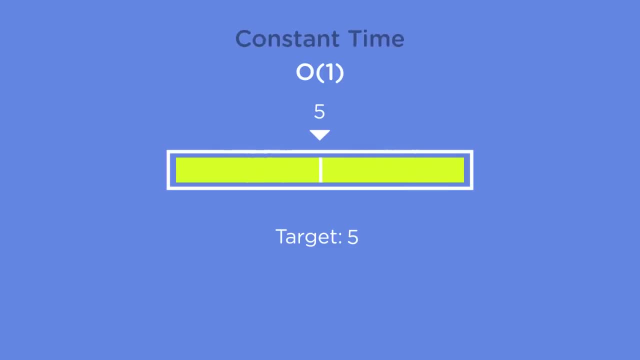 search algorithm here a different binary search algorithm, and what's the difference between these two implementations? anyway, the difference lies in these last four lines of code that you see here. we did something unusual here. now, before we get into this, a small word of advice. this is a confusing topic. 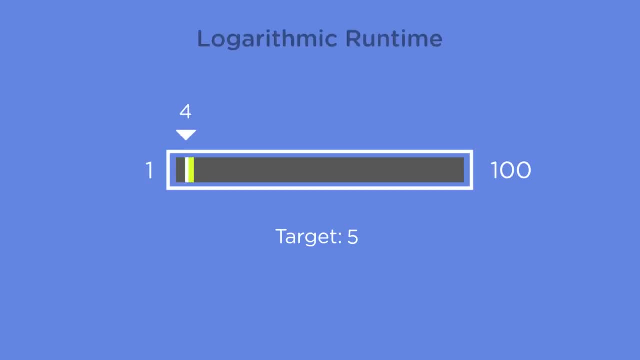 and people get confused by it all the time. don't worry, that doesn't make you any less of a programmer. in fact, I have trouble with it often and always look it up, including when I made this video. this version of binary search is a recursive binary search. 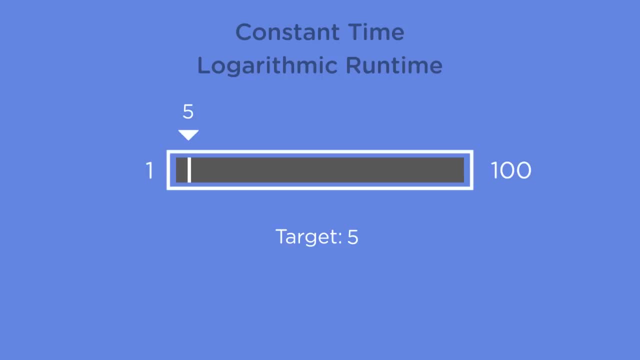 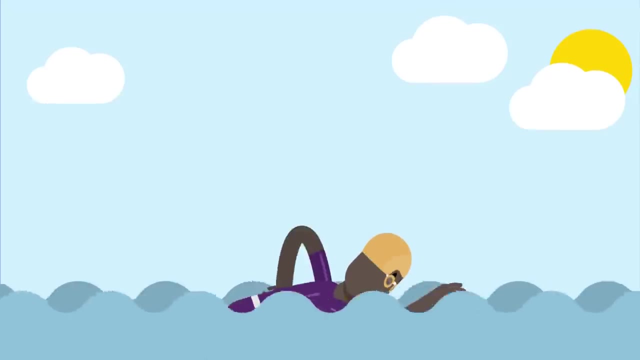 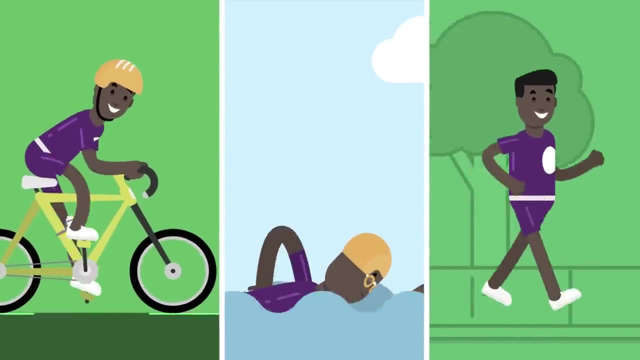 a recursive function is one that calls itself. this is hard for people to grasp sometimes because there's few easy analogies that make sense. so let's say you have this book that contains answers to multiplication problems. you're working on a problem and you look up an answer. 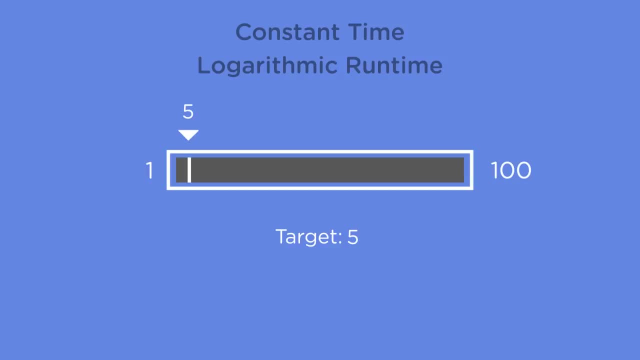 So in our algorithm we have a couple steps that are constant-time and one step that is logarithmic overall. When evaluating the runtime for an algorithm, we say that the algorithm has as its upper bound the same runtime as the least efficient step. 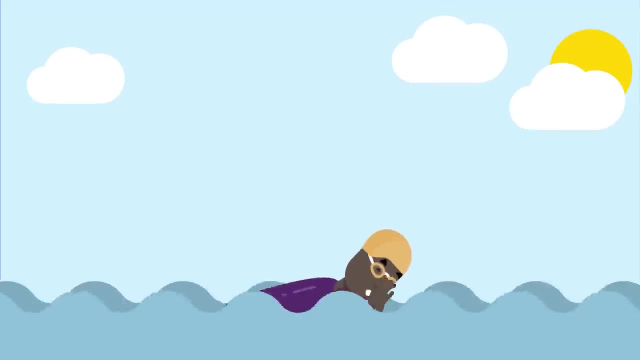 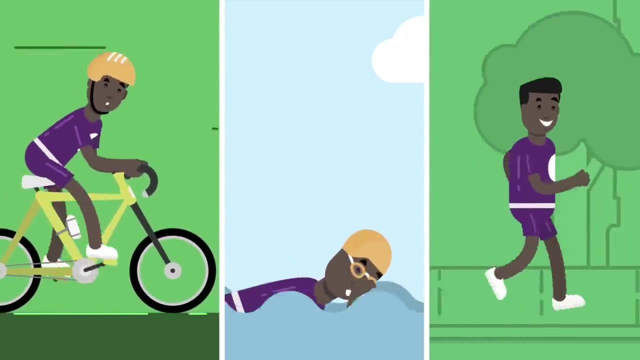 in the algorithm. Think of it this way: Let's say you're participating in a triathlon, which is a race that has a swimming, running and a cycling component. You could be a phenomenal swimmer and a really good cyclist, but you're a pretty terrible runner. 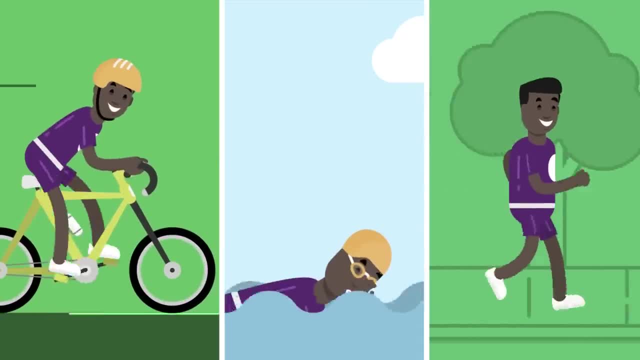 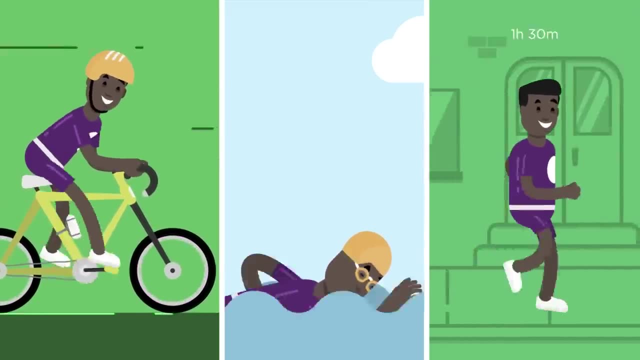 No matter how fast you are at swimming or cycling, your overall race time is going to be impacted the most by your running race time, because that's the part that takes you the longest If you take an hour thirty to finish the running component. 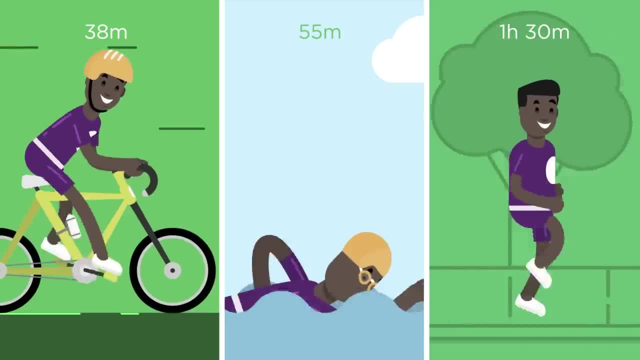 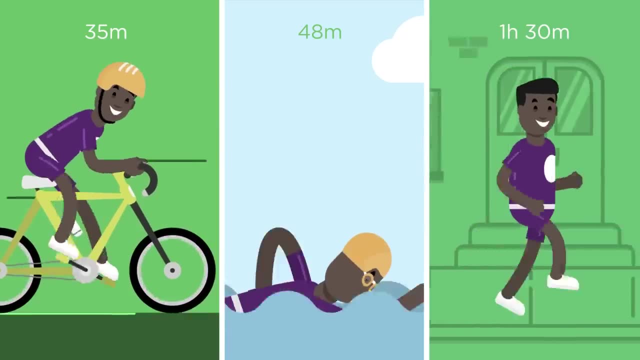 55 minutes to swim, 38 minutes to bike. it won't matter if you can fine-tune your swimming technique down to finish in 48 minutes and your cycle time to 35,, because you're still bounded at the top by your running time. 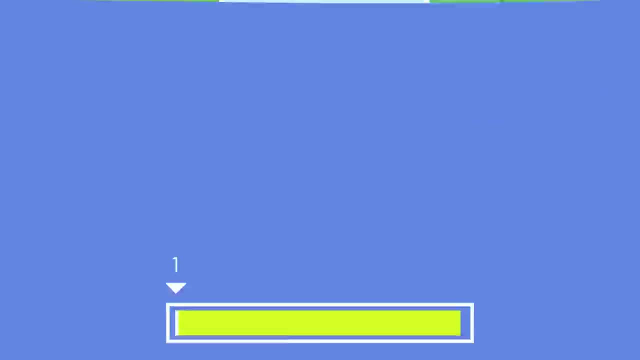 which is close to almost double your bike time. Similarly, with the binary search algorithm, it doesn't matter how fast we make the other steps. they're already as fast as they can be In the worst-case scenario: the splitting of the list down to a single element list. 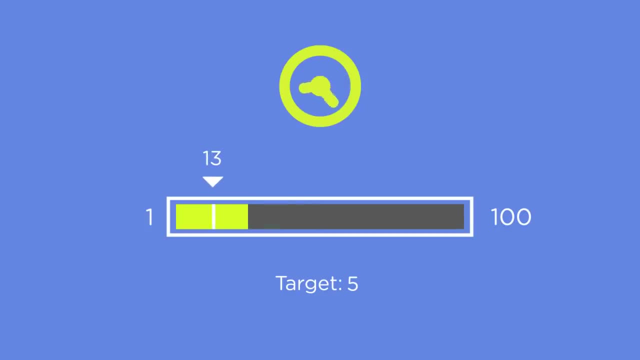 is what will impact the overall running time of your algorithm. This is why we say that the time complexity or run time of the algorithm, in the worst case, is O or logarithmic. As I alluded to, though your algorithm may hit a best-case run time, 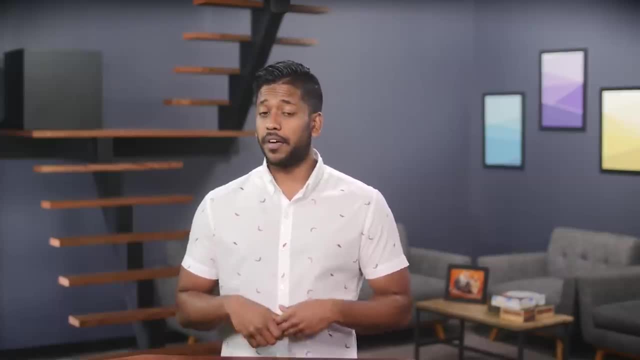 and in between the two best and worst case, have an average run time as well. This is important to understand, because algorithms don't always hit their worst case, But this is getting a bit too complex for us For now. we can safely ignore average case performances. 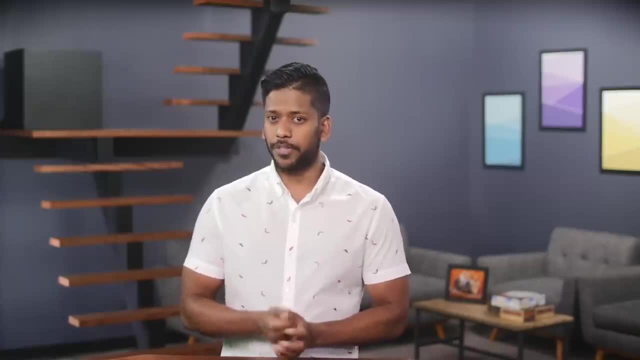 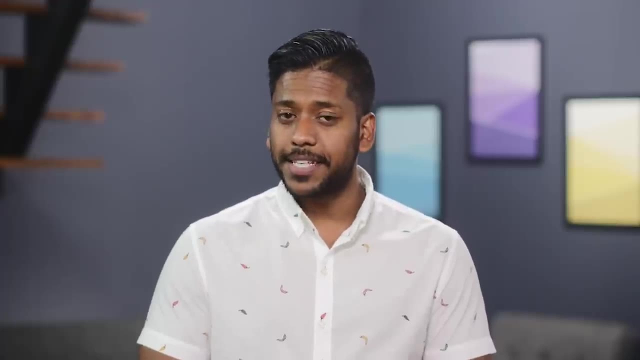 and focus only on the worst case. In the future, if you decide to stick around, we'll circle back and talk about this more. Now that you know about algorithms, complexities and Big O, let's take a break from all of that. 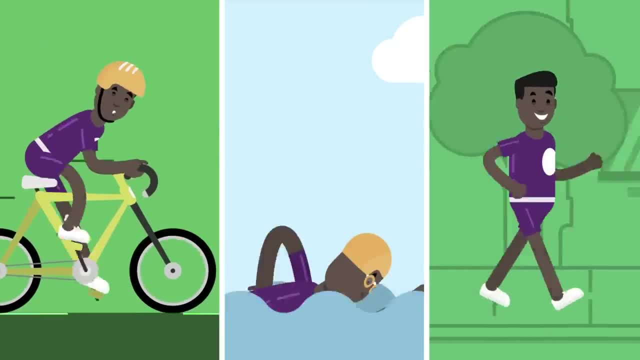 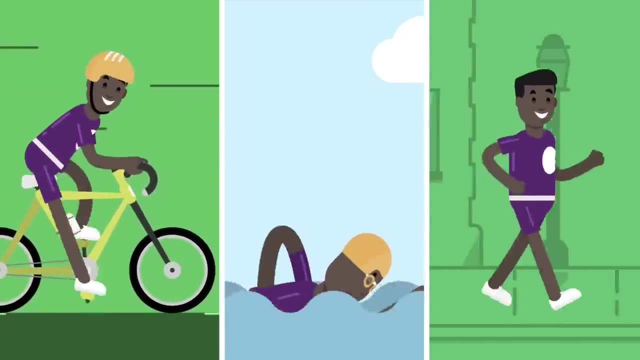 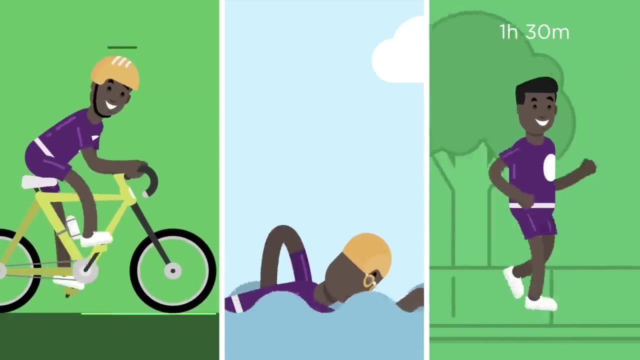 in the book, the answer for your problem says: add 10 to the answer for problem 52. ok, so you look up problem 52 and there it says: add 12 to the answer for problem 85. well then, you go and look up the answer to problem 85 and finally, 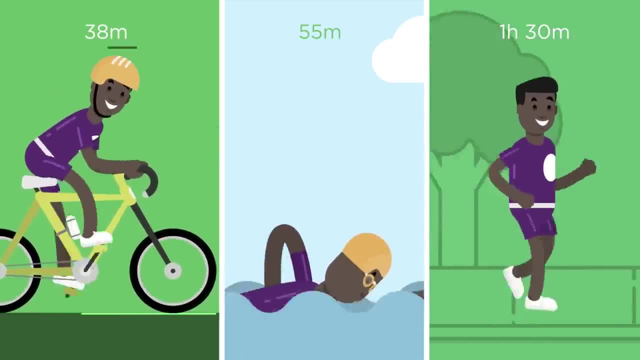 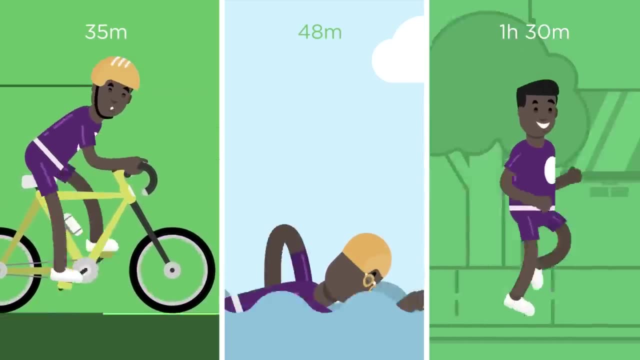 instead of redirecting you somewhere else. that answer says 10, so you take that 10 and then you go back to problem 52 because, remember, the answer for problem 52 was to add 12 to the answer for problem 85, so you take that 10. 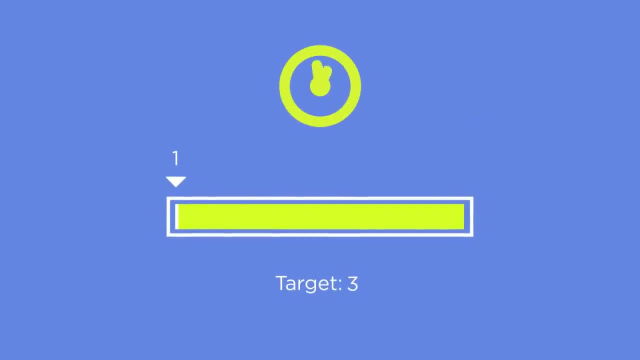 and then you now have the answer to problem 85. so you add 10 to 12 to get 22. then you go back to your original problem, where it said to add 10 to the answer for problem 52. so you add 10 to 22 and you get 32. 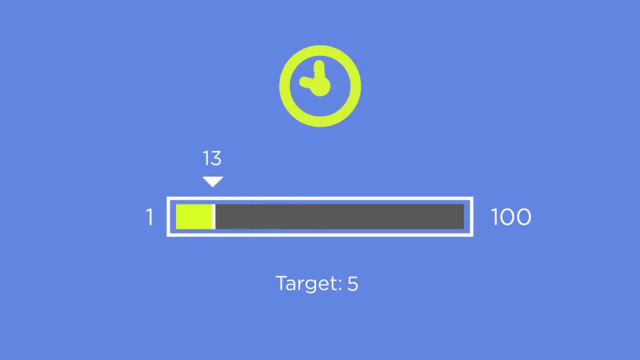 to end up with your final answer. so that's a weird way of doing it, but this is an example of recursion. the solution to your first lookup in the book was the value obtained by another lookup in the same book, which was followed by yet another lookup in the same book. 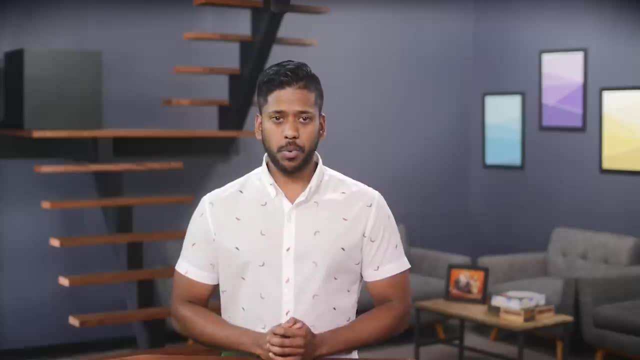 the book told you to check the book until you arrived at some base value. our function works in a similar manner, so let's visualize this with an example of a list. like before. we have a 9 element list here with values 0 through 8, the target we're searching for. 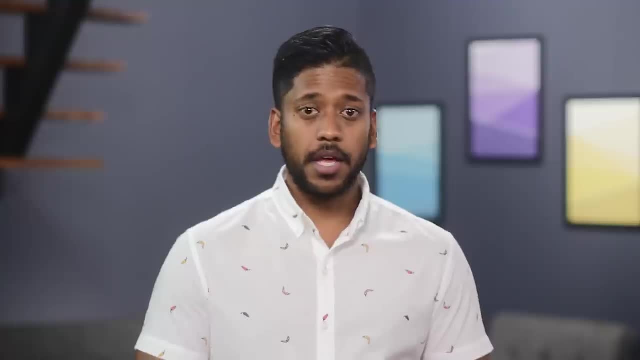 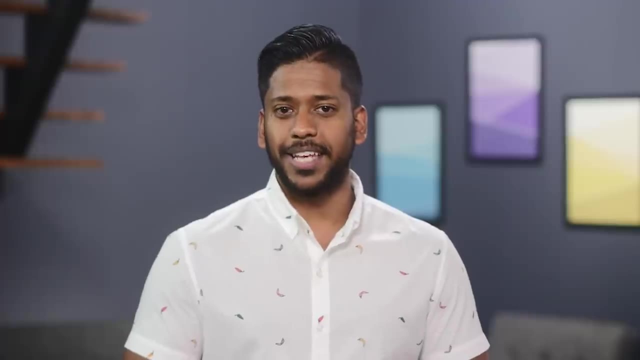 is the value 8. we'll check if the list is empty by calling len on it. this list is not empty, so we go to the else clause. next we calculate the midpoint: 9 divided by 2 is 4.5, rounded down is 4. 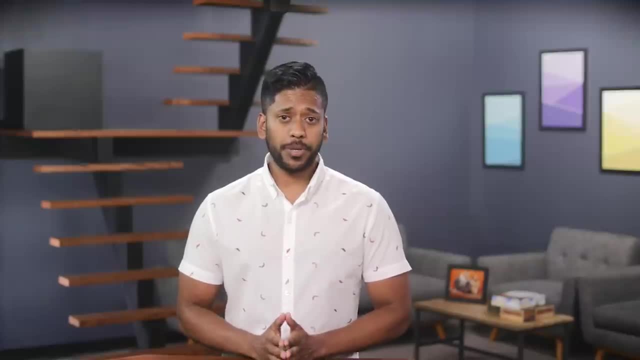 so our first midpoint value is 4. we'll perform our first check. is the value at the midpoint equal to the target? not true, so we go to our else clause. we'll perform another check here. is the value at the midpoint less than the target? now, in our case, this is: 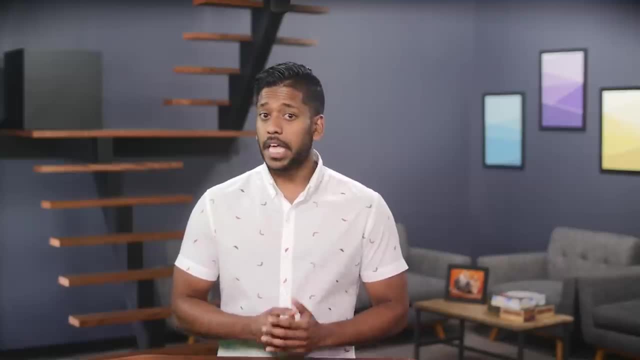 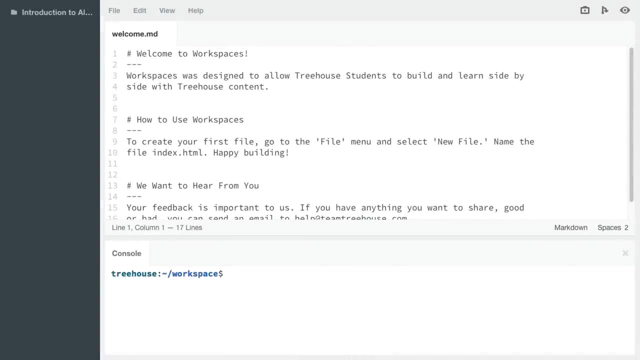 true. earlier, when we evaluated this condition, we simply changed the value of first. here we're going to call the recursive binary search function again and give it a new list to work with. the list starts at midpoint plus 1, so at index position 5, all the way to the end. 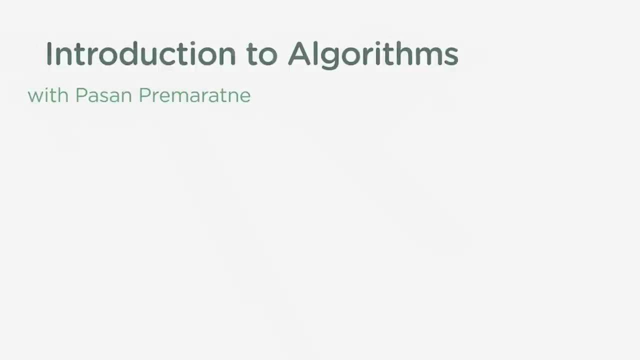 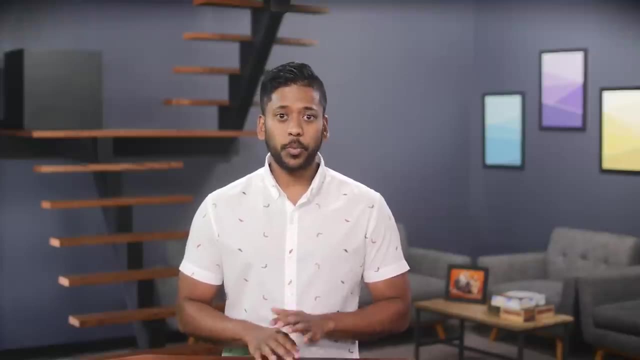 and write code in the next video. So far we've spent a lot of time in theory and, while these things are all important things to know, you get a much better understanding of how algorithms work when you start writing some code. As I mentioned earlier, 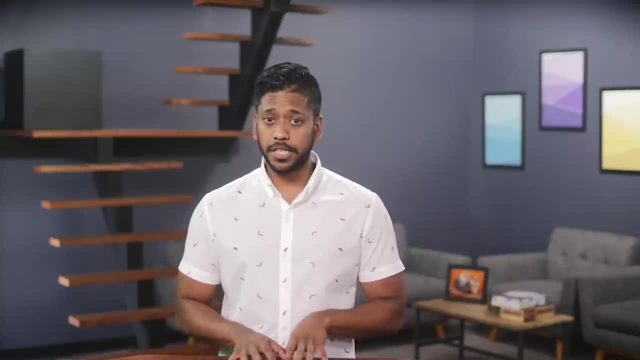 we're going to be writing Python code in this and all subsequent algorithm courses. If you do have programming experience, but in another language, check the notes section of this video for an implementation in your language. If you don't have any experience, I'll try my best to explain as we go along. 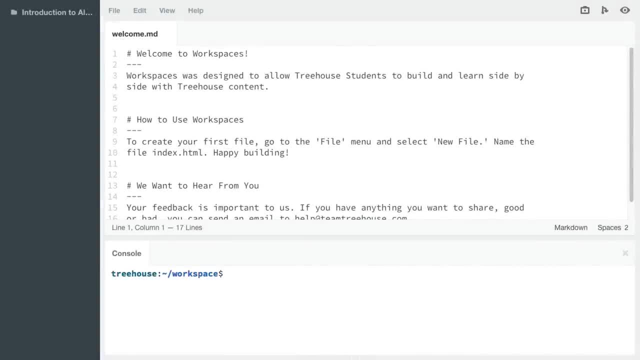 On the video you're watching right now, you should see a launch workspaces button. We're going to use a treehouse coding environment called workspaces to write all of our code. If you're familiar with using Python in a local environment, then feel free to keep doing so. 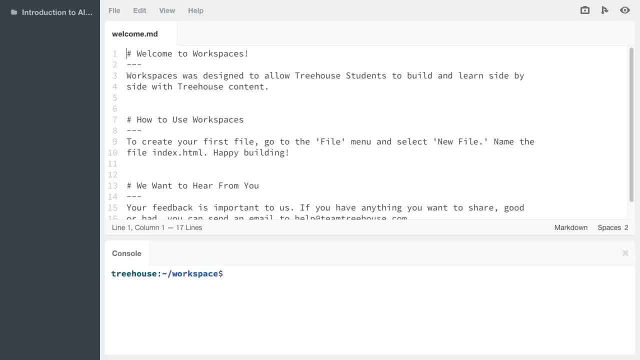 Workspaces is an in-browser coding environment and will take care of all the setup and installation, so you can focus on just writing and evaluating code. Workspaces is quite straightforward to use. On the left here we have a file navigator pane which is currently empty. 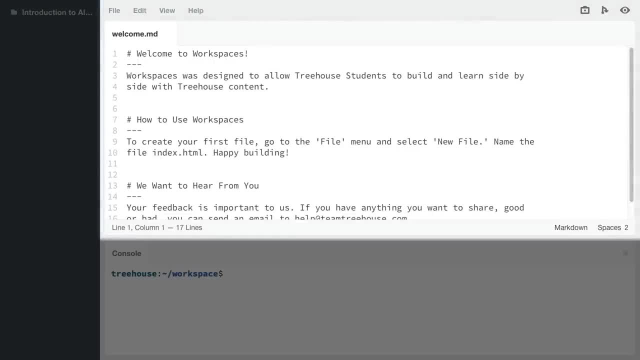 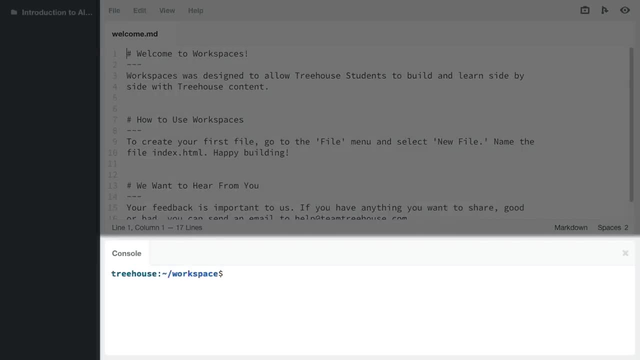 since we haven't created a new file. On the top we have an editor where we write all our code, and then below that we have a terminal or a command line prompt where we can execute the scripts that we write. Let's add a new file here. 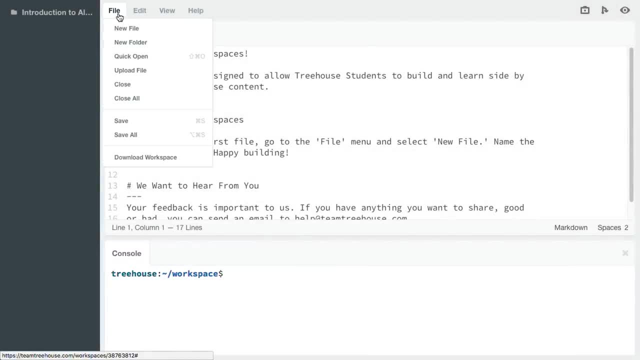 so at the top in the editor area we're going to go to file new file and we'll name this linear underscore search dot pi. In here we're going to define our linear search algorithm as a stand-alone function. We start with the keyword def. 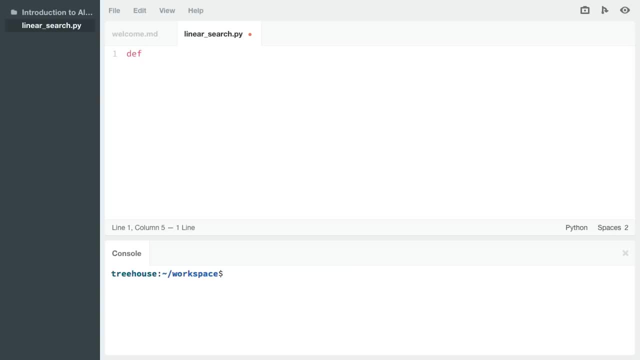 which defines a function or a block of code and then we give it the name linear underscore search. This function will accept two arguments: First the list we're searching through and then the target value we're looking for. Both of these arguments are enclosed. 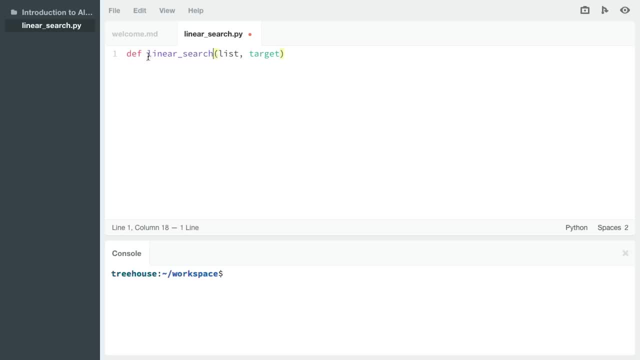 in a set of parentheses and there's no space between the name of the function and the arguments. After that we have a colon. Now there might be a bit of confusion here, Since we already have this target value. what are we searching for? 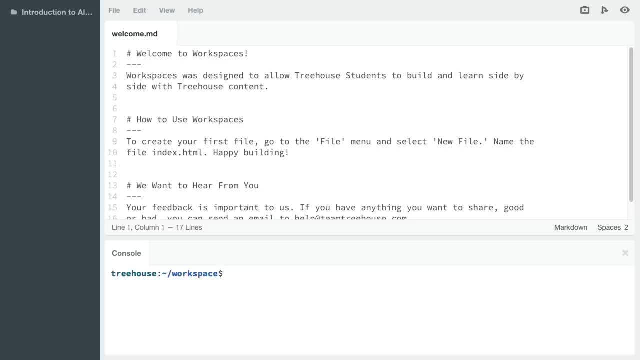 notice that this call to recursive binary search, inside of recursive binary search, includes a return statement. this is important and we'll come back to that in a second. so now we're back at the top of a new call to recursive binary search with, effectively, a new list. 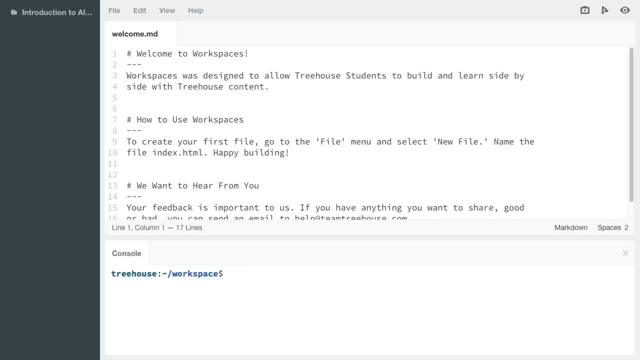 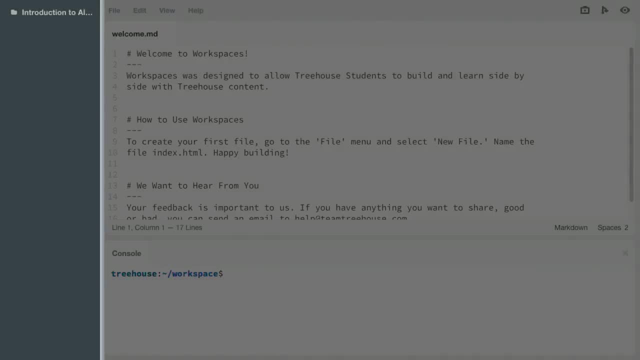 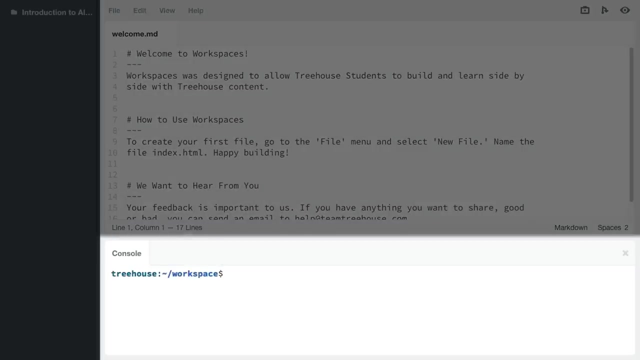 although technically just a sub list of the first one. the list here contains the numbers 6, 7 and 8, starting with the first check. the list is not empty, so we move to the else, the midpoint in this case. length of the list: 3 divided by 2, rounded down. 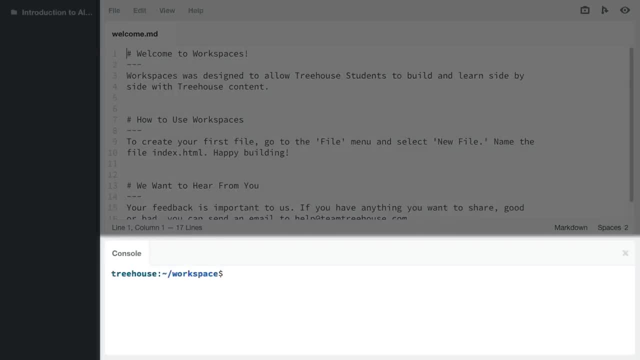 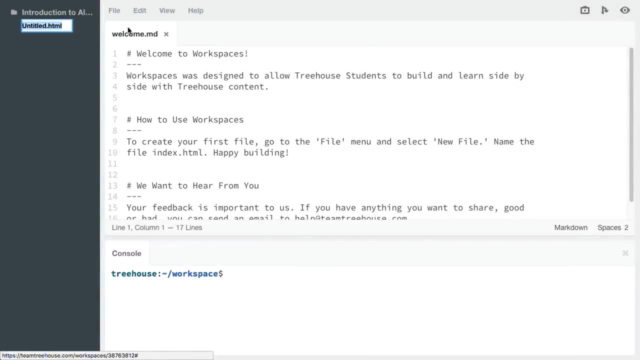 is 1. is the value of the midpoint equal to the target? well, the value at that position is 7, so no, in the else we perform the first check. is the value at the midpoint less than the target? indeed it is, so we call recursive binary search. 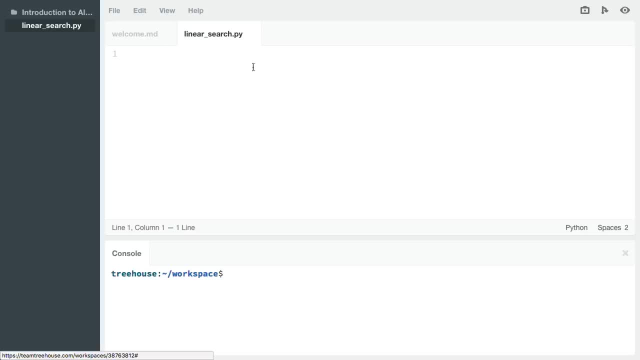 again and provide it a new list. this list starts at midpoint plus 1 and goes to the end, so in this case that's a single element list. since this is a new call to recursive binary search, we start back up at the top. is the list empty? no, the midpoint. 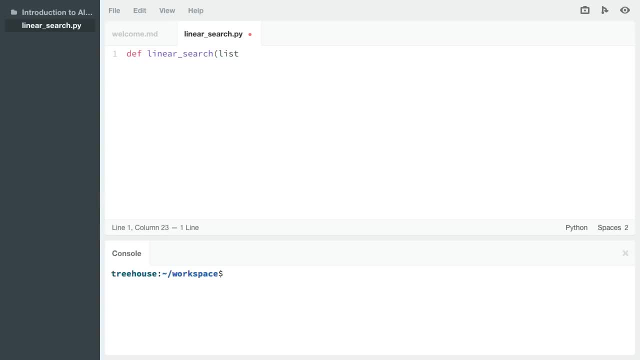 is 0, is the value at the midpoint the same as the target. it is, so now we can return true. remember a minute ago i pointed out that when we call recursive binary search from inside the function itself, it's preceded by a return statement that plays a. 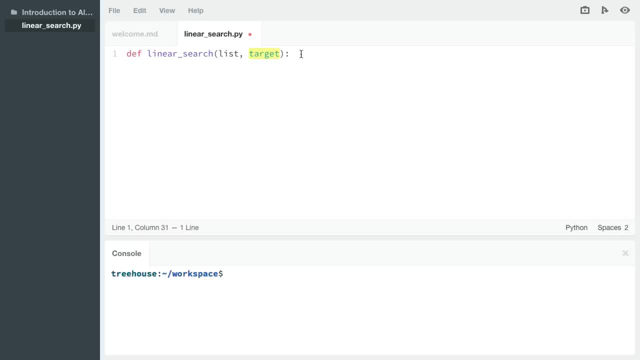 pretty important role here. so back to our visualization. we start at the top and we call binary search with a new list. but because that's got a return statement before it, what we're saying is, hey, when you run binary search on this, whatever value you get back. 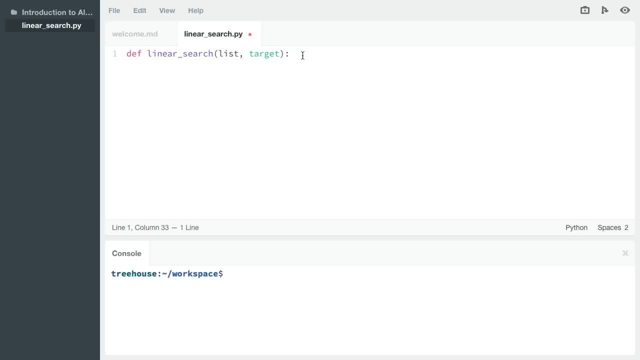 return it to the function that called you. then at the second level, we call binary search again, along with another return statement. like with the first call, we're instructing the function to return a value back to the code that called it. at this level we find the target, so the function returns. 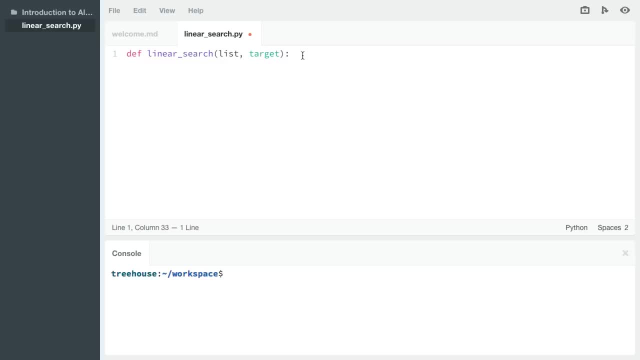 true back to the caller. but since this inner function was also called by a function with instruction to return, it keeps returning that true value back up until we reach the very first function that called it. going back to our book of answers, recursive binary search instructs itself to. 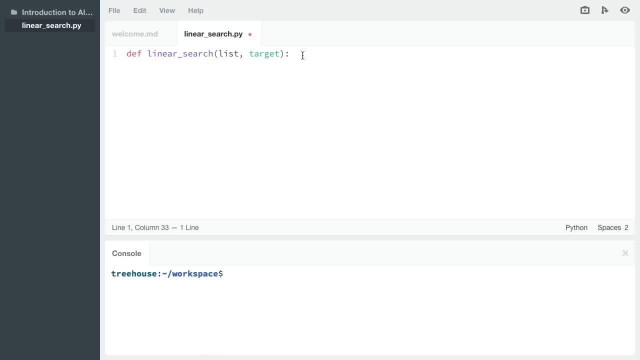 Unlike the game we played at the beginning, where John's job was to find the value, in a true implementation of linear search we're looking for the position in the list where the value exists. If the target is in the list, then we return its position. 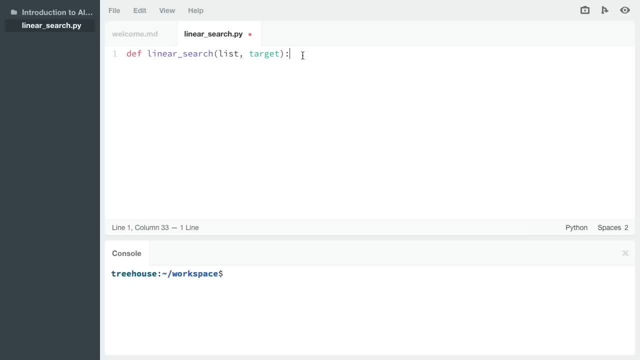 And since this is a list, that position is going to be denoted by an index value. Now, if the target is not found, we're going to return none. The choice of what to return in the failure case may be different in other implementations. 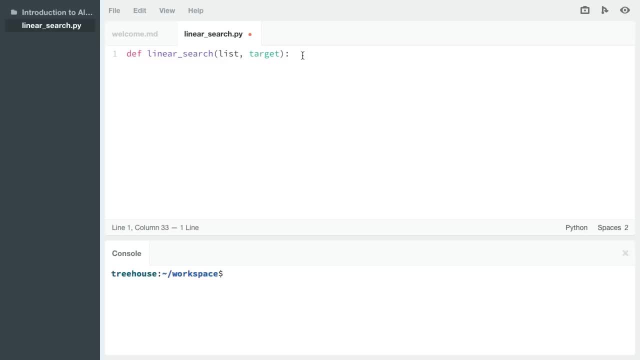 of linear search, You can return minus one, since that isn't typically an index value. You can also raise an exception, which is Python speak for indicating an error occurred. Now I think for us, the most straightforward value we can return here is none. 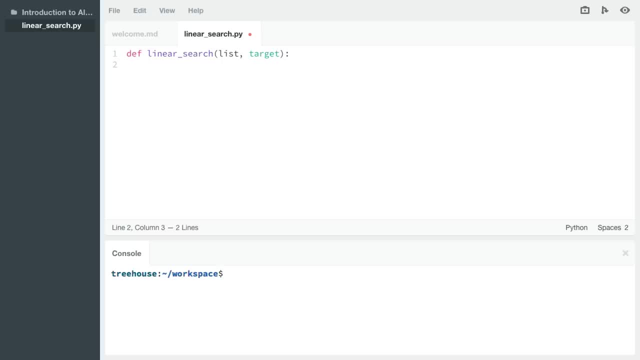 Now let's add a comment to clarify this. So hit enter to go to the next line, And then we're going to add three single quotes And then below that on the next line, we'll say: returns the position or the index position. 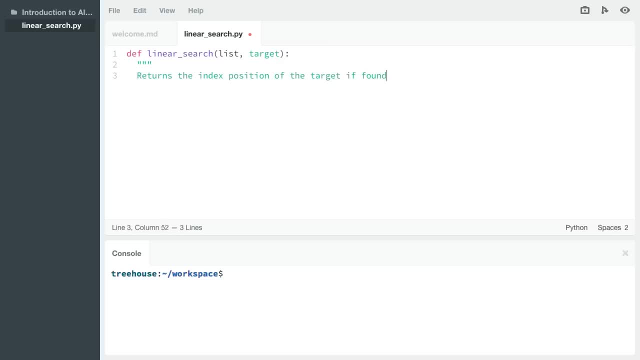 Of the target if found, else returns none. And then, on the next line, we'll close off those three quotes. This is called a doc string and is a Python convention for documenting your code. The linear search algorithm is a sequential algorithm that compares each item in the list. 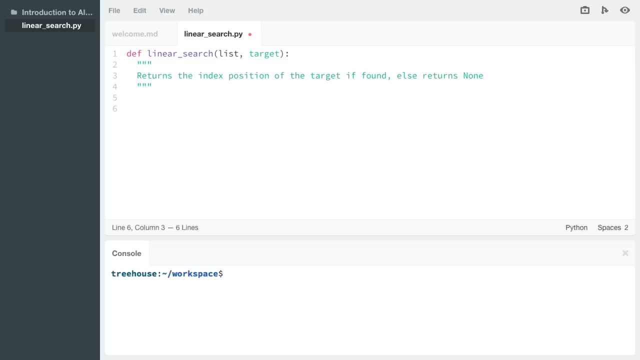 until the target is found To iterate or loop or walk through our list sequentially. we're going to use a for loop Now. typically when iterating over a list in Python we would use a loop like this. We'd say: for item in list. 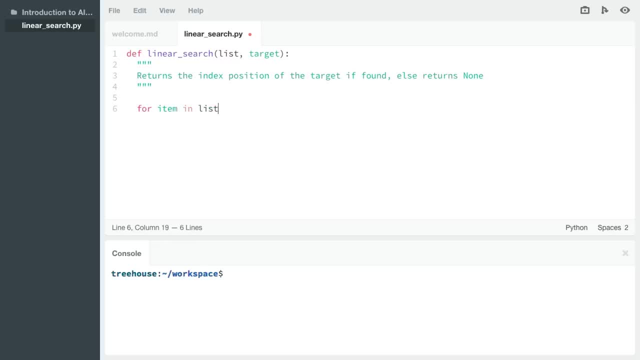 This assigns the value at each index position to that local variable item. We don't want this, though, since we primarily care about the index position. Instead, we're going to use the range function in Python to create a range of values that start at zero. 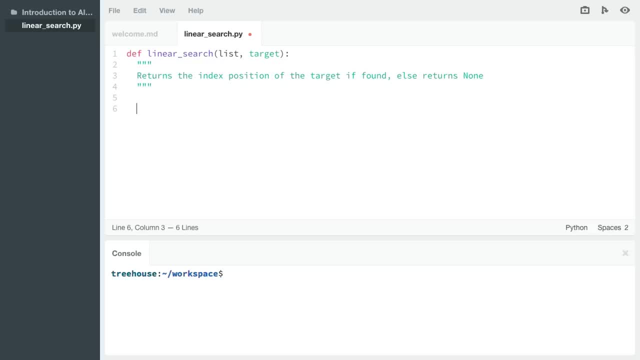 and end at the number of items in the list. So we'll say for i- i stands for index. here, in range starting at zero and going all the way up to the length of the list, We can get the number of items. 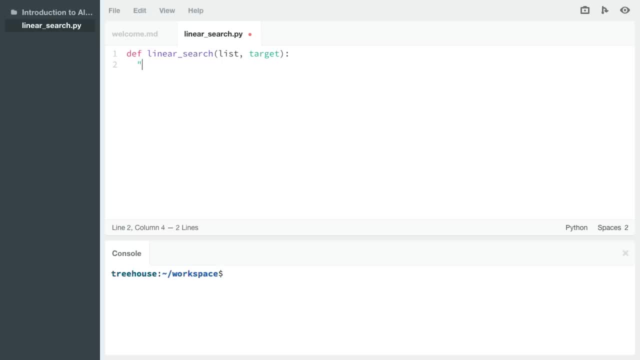 keep working on the problem until it has a concrete answer. once it does, it works its way backwards, giving the answer to every function that called it until the original caller has an answer. now, like i said at the beginning, this is pretty complicated, so you should not be concerned if this. 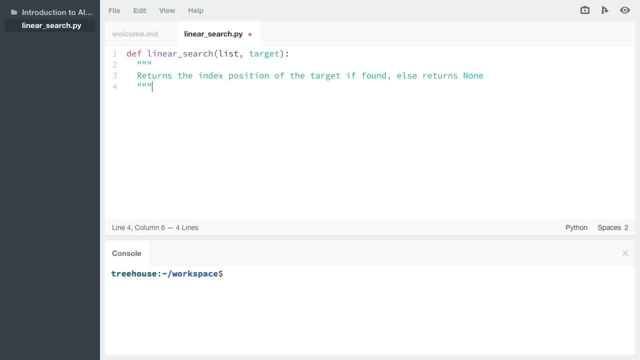 doesn't click. honestly, this is not one thing that you're going to walk away with knowing fully how to understand recursion after your first try. i'm really not lying when i say i have a pretty hard time with recursion. now, before we move on, i do want to point out one thing. 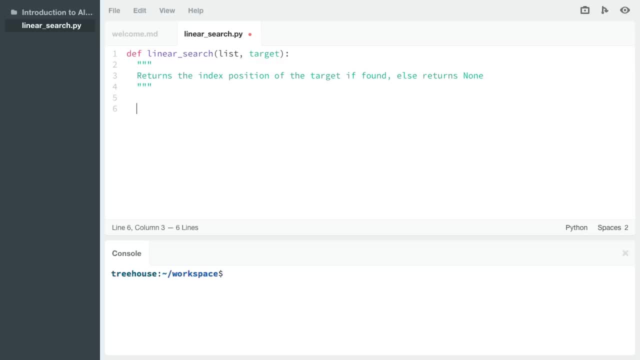 even though the implementation of recursion is harder to understand, it is easier in this case to understand how we arrive at the logarithmic runtime, since we keep calling the function with smaller lists. let's take a break here. in the next video, let's talk a bit more about. 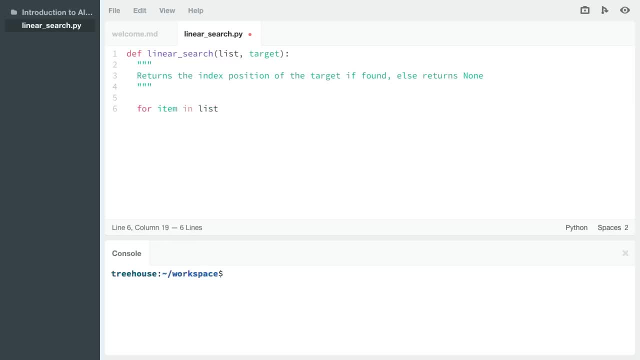 recursion and why it matters. in the last video, we wrote a version of binary search that uses a concept called recursion. recursion might be a new concept for you, so let's formalize how we use it. a recursive function is one that calls itself, in our example, the recursive. 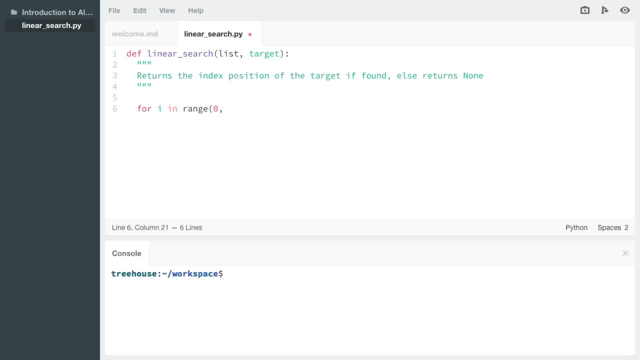 binary search function called itself inside the body of the function. when writing a recursive function, you always need a stopping condition and typically we start the body of the recursive function with this stopping condition. it's common to call this stopping condition the base case in our recursive binary search function. 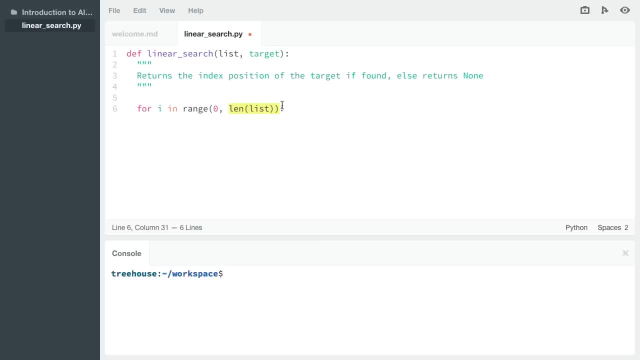 we had two stopping conditions. the first was what the function should return if an empty list is passed in. it seems weird to evaluate an empty list because you wouldn't expect to run search on an empty list. but if you look at how our function works- recursive binary search- 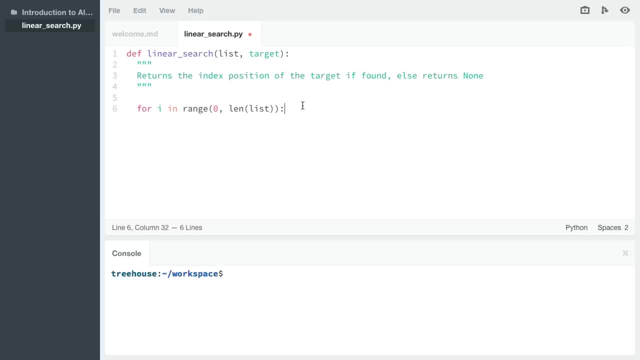 keeps calling itself and with each call to itself, the size of the list is cut in half. if we searched for a target that didn't exist in the list, then the function would keep halving itself until it got to an empty list. consider a three element list. 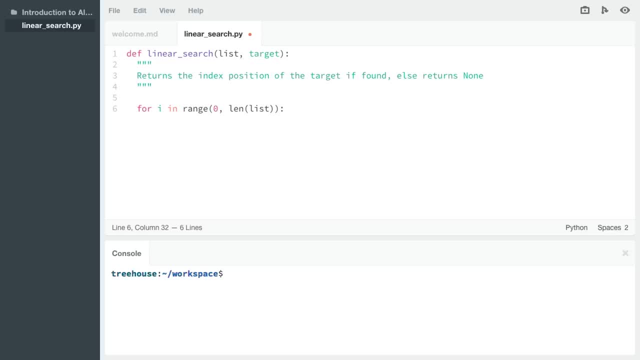 in the list using the len function. Now, going back to our talk on complexity and how individual steps in an algorithm can have its own run times, this is a line of code that we would have to be careful about. Python keeps track of the length of a list. 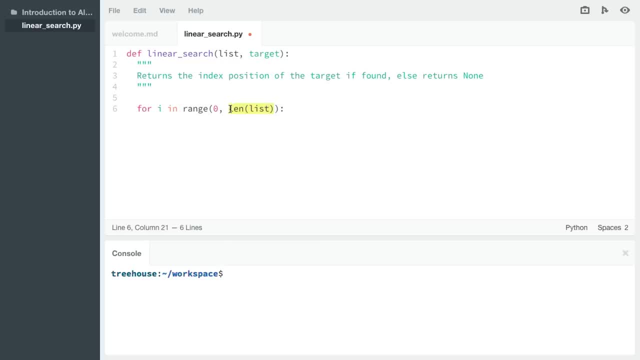 So this function- call here len list- is a constant time operation. Now if this were a naive implementation- let's say we wrote the implementation of the list and we iterate over the list every time we call this length function, then we've already incurred. 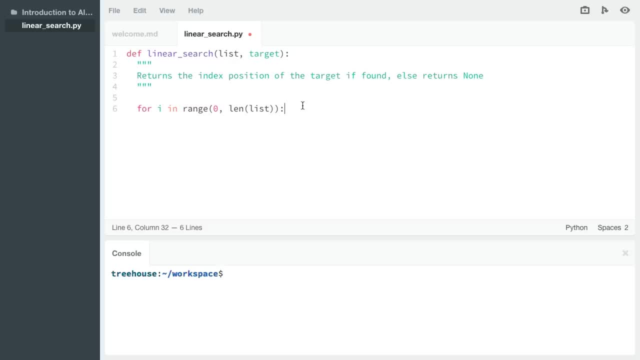 a linear cost. Okay, so once we have a range of values that represent index positions in this list, we're going to iterate over that using the for loop and assign each index value to this local variable. i Using this index value, we can obtain the item. 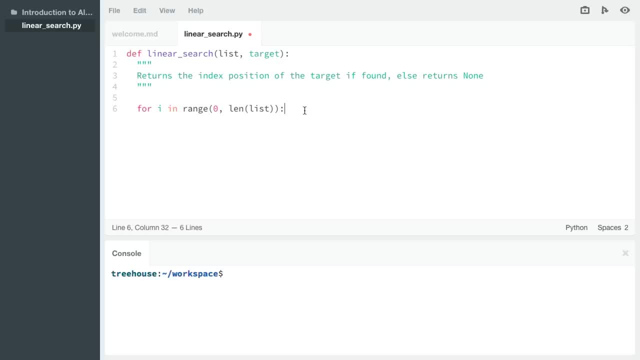 at that position using subscript notation on the list. Now, this is also a constant time operation because the language says so, So we'll do if list. So, once we have this value, which we'll get by using subscript notation, so we'll say list i. 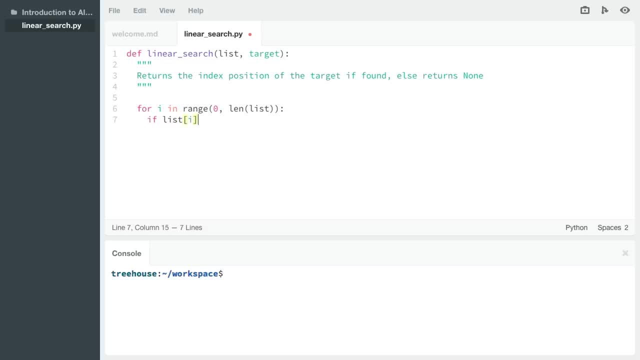 Once we have this value, we'll check if it matches the target. So if the value at i equals target, well, if it does, then we'll return that index value because we want the position And once we hit this return statement, 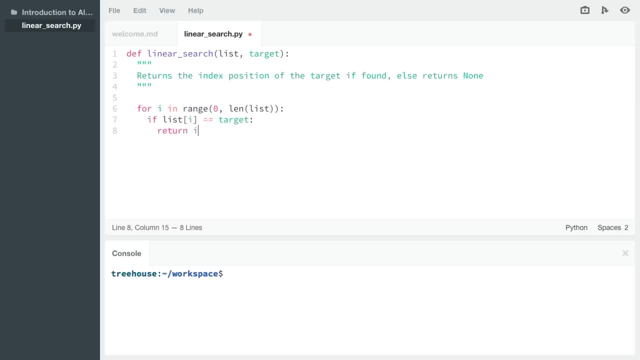 we're going to terminate our function. If the entire for loop is executed and we don't hit this return statement, then the target does not exist in the list. So at the bottom here we'll say: return none, Even though all the individual operations 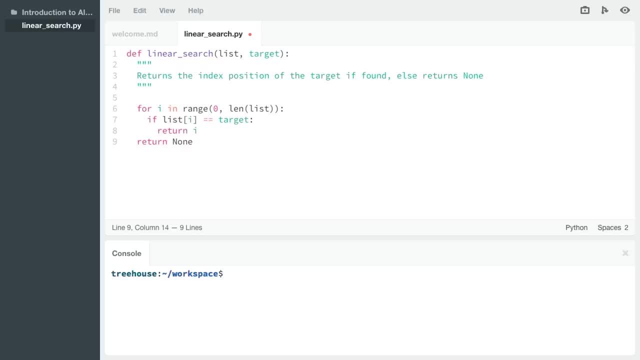 in our algorithm run in constant time. in the worst case scenario, this for loop here will have to go through the entire range of values and read every single element in the list, therefore giving the algorithm a big ol' value of n or running in linear time. 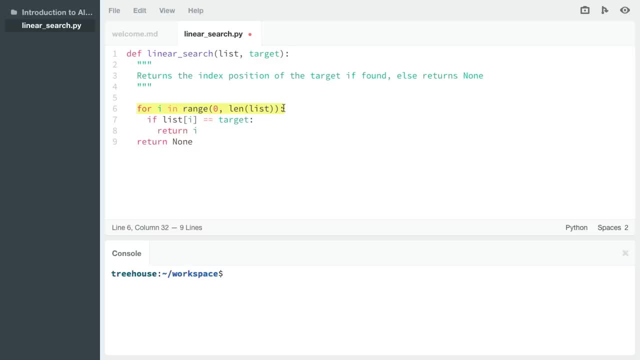 Now, if you've written code before, you've definitely written code like this a number of times and I bet you didn't know. but all along you were implementing what is essentially a well-known algorithm, So I hope this goes to show you. 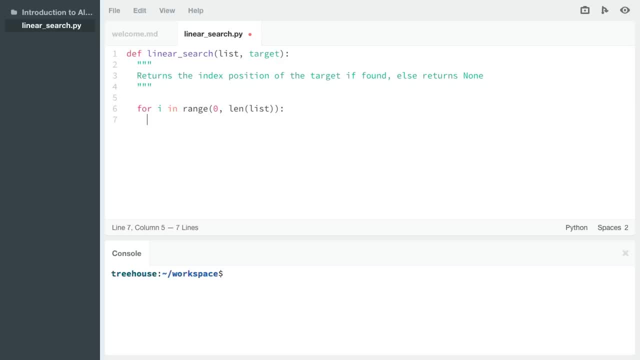 with numbers 1,2,3, where we're searching for a target of 4. on the first pass, the midpoint is 2, so the function would call itself with the list 3. on the next pass, the midpoint is 0 and the target is still greater. 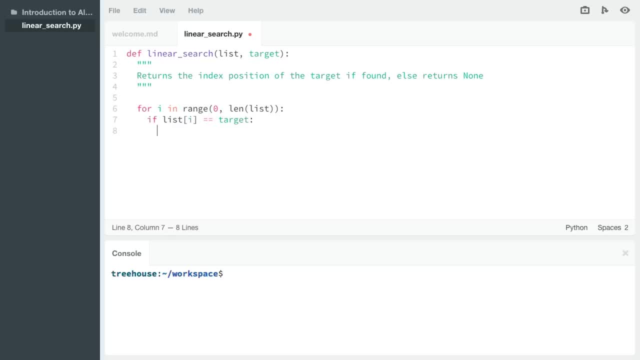 so the function would call itself, this time passing in an empty list, because an index of 0 plus 1 in a single element list doesn't exist. when we have an empty list, this means that after searching through the list, the value wasn't found. this is why we define an empty list. 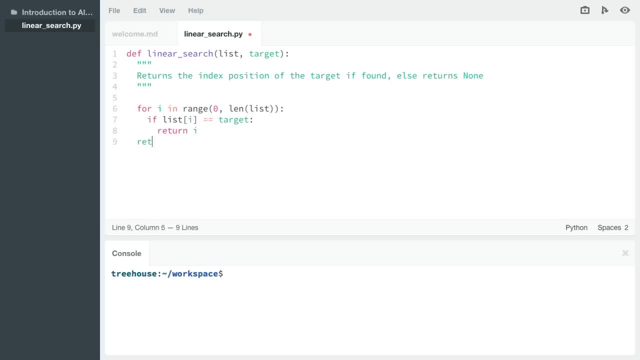 as a base case that returns false. if it's not an empty list, then we have an entirely different set of instructions we want to execute. first, we obtain the midpoint of the list. once we have the midpoint, we can introduce our next base case or stopping condition. if the value at the midpoint 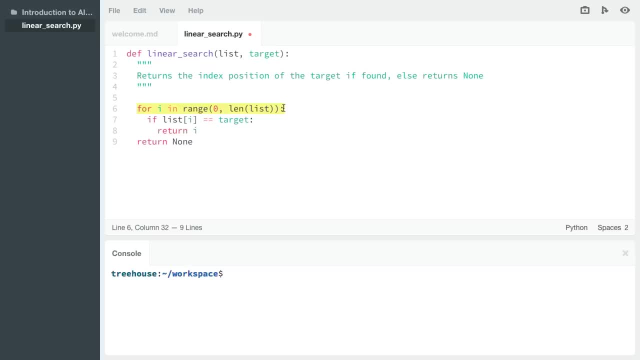 is the same as the target, then we return true. with these two stopping conditions, we've covered all possible paths of logic through the search algorithm. you can either find the value or you don't. once you have the base cases, the rest of the implementation of the recursive function. 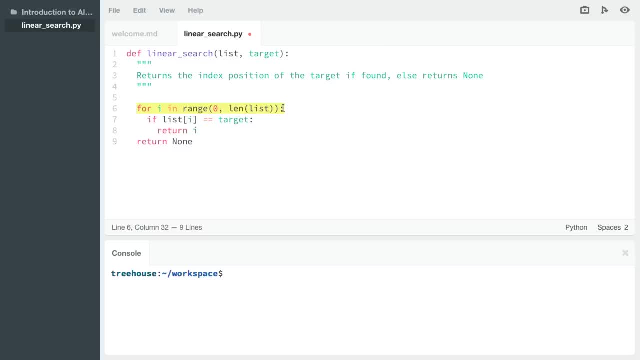 is to call the function on smaller sublists until we hit one of these base cases. going back to our visualization for a second, we see that recursive binary search calls itself a first time, which then calls itself again for the initial list we started with. the function only calls itself a few times. 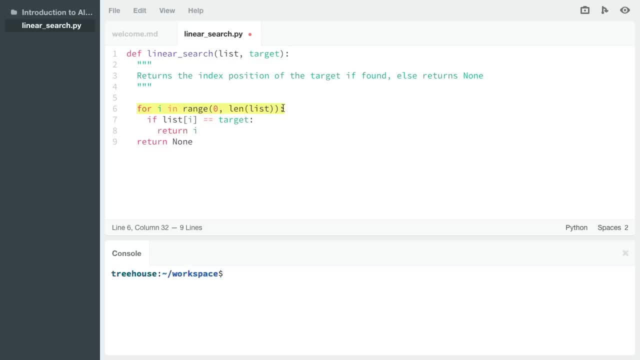 before a stopping condition is reached. the number of times a recursive function calls itself is called recursive depth. now, the reason I bring all of this up is because if, after you start learning about algorithms, you decide you want to go off and do your own research, you may start to see. 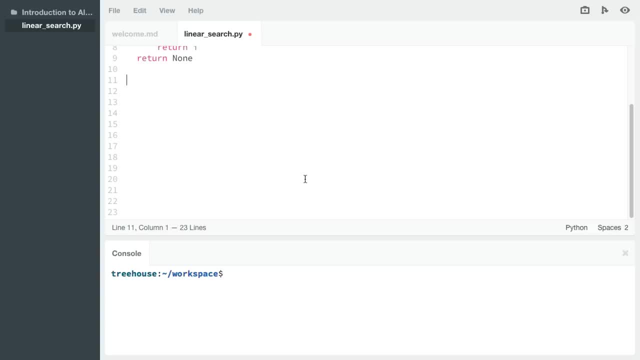 a lot of algorithms implemented using recursion, the way we implemented binary search. the first time is called an iterative solution. now, when you see the word iterative, it generally means the solution was implemented using a loop structure of some kind. a recursive solution, on the other hand, is one that involves 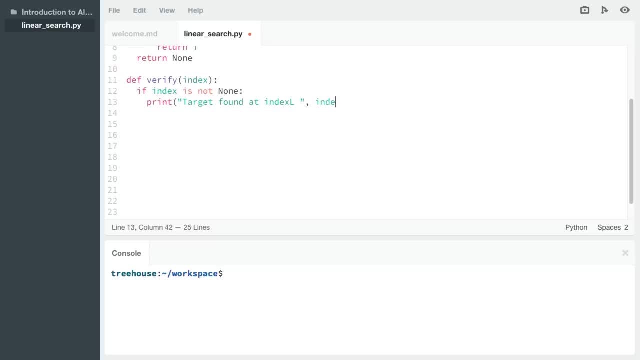 a set of stopping conditions and a function that calls itself computer scientists and computer science textbooks, particularly from back in the day, favor and are written in what are called functional languages. in functional languages we try to avoid changing data that is given to a function. in our first version of binary search, 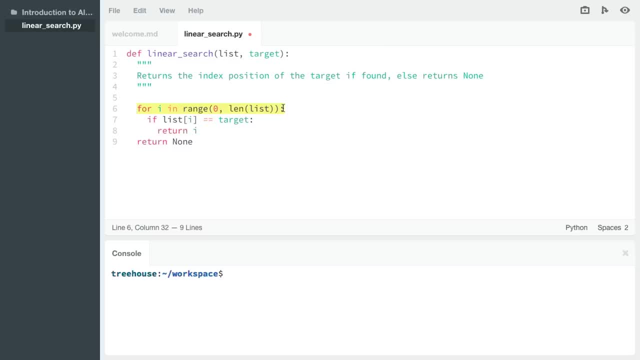 that algorithms are a pretty approachable topic. Like everything else, this does get advanced, but as long as you take things slow, there's no reason for it to be impossible. Remember that not any block of code counts as an algorithm To be a proper algorithm, 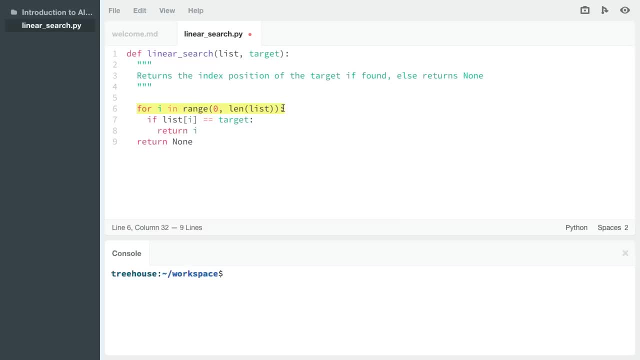 for implementation of linear search. this block of code must return a value, must complete execution in a finite amount of time and must output the same result every time for a given input set. So let's verify this with a small test. Let's write a function. 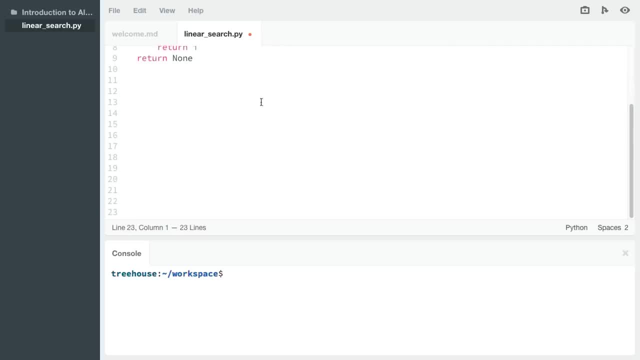 called verify. that accepts an index value. If the value is not none, it prints the index position. If it is none, it informs us that the target was not found in the list. So def verify, and this is going to take an index value. 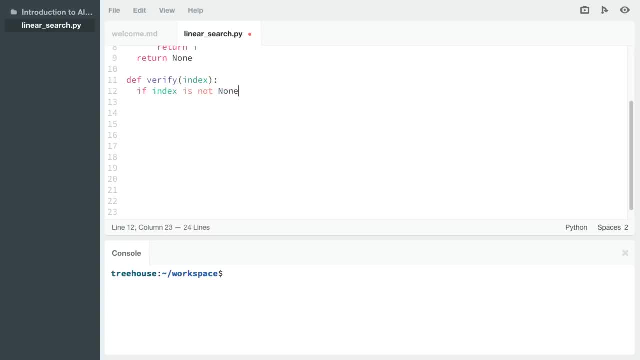 and we'll say: if index is not none, then we'll print target found at index. oops, that's a colon here, index, else that needs to go back. there we go, else we'll say: target not found in list. 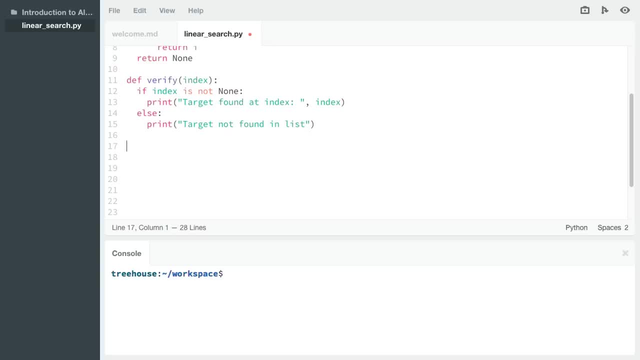 Okay, using this function, let's define a range of numbers now. so this will be a list numbers and we'll just go from 1 to, let's say, 10.. Now, if you've written Python code before, you know that I can use. 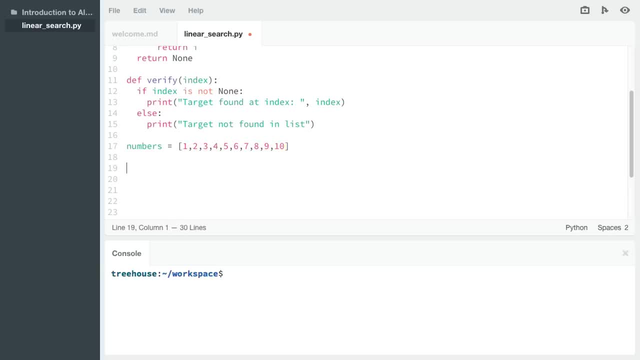 a list comprehension to make this easier. but we'll keep things simple. We can now use our linear search function to search for the position of a target value in this list. So we can say: result equal linear underscore search and we're going to pass in. 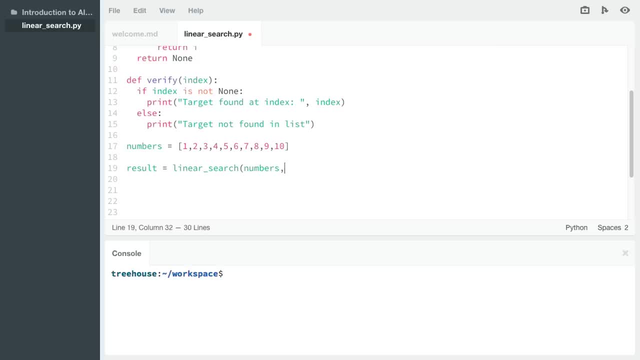 the numbers list. that's the one we're searching through, and we want to look for the position where the value 12 exists, and then we'll verify this result. If our algorithm works correctly, the verify function should inform us that the target 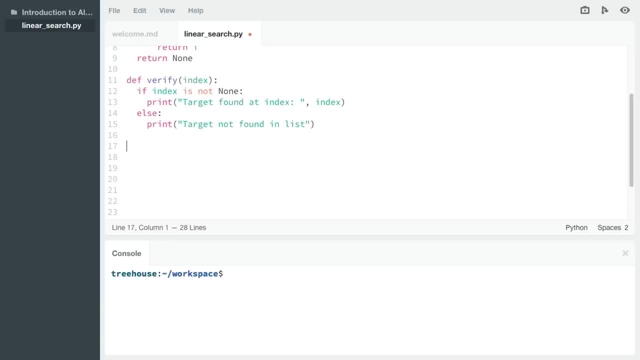 we created first and last variables using the list and then modified first and last as we needed to arrive at a solution. functional languages don't like to do this- all this modification of variables- and prefer a solution using recursion, a language like python, which is what we are using. 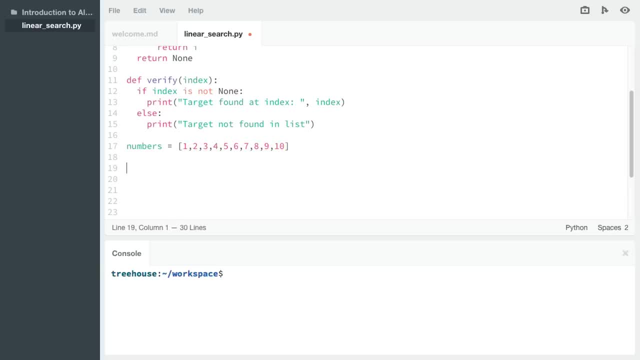 is the opposite and doesn't like recursion. in fact, python has a maximum recursion depth, after which our function will halt execution. python prefers an iterative solution. now, I mention all of this for two reasons. if you decide that you want to learn how to implement the algorithm in a language of your choice, 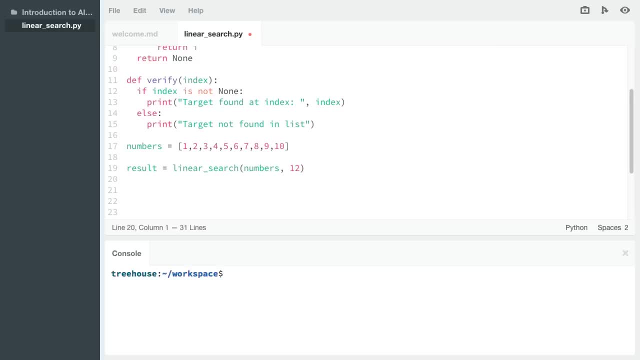 that's not python, then you might see a recursive solution as the best implementation in that particular language. I'm an ios developer, for example, and I work with a language called swift. swift is different from python in that it doesn't care about recursion depth and does some neat tricks. 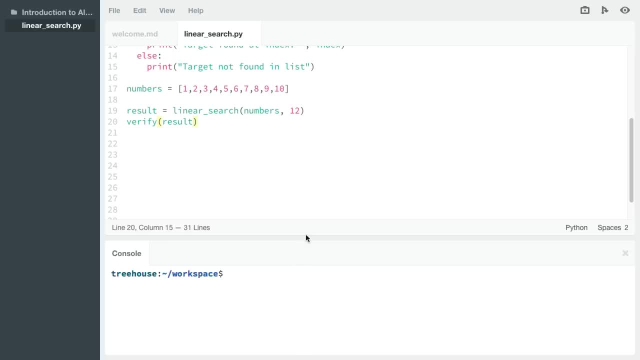 where it doesn't even matter how many times your function calls itself. so if you want to see this in swift code, then you need to know how recursion works well. and now you have some idea. now the second reason I bring it up is actually way more important. 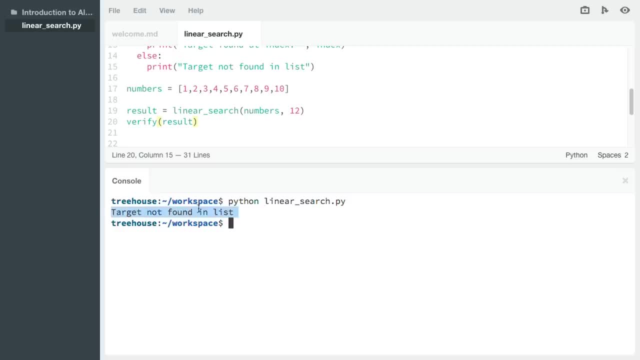 and to find out on to the next video. at the beginning of this series, I mentioned that there were two ways of measuring the efficiency of an algorithm. the first was time complexity, or how the runtime of an algorithm grows as n grows larger. the second is space complexity. 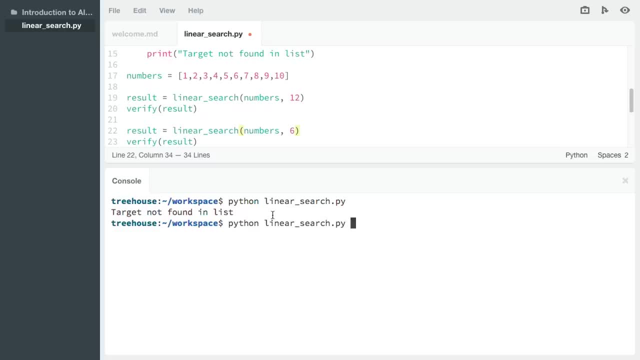 we took a pretty long route to build up this example, but now we're in a good place to discuss space complexity. space complexity is a measure of how much working storage, or extra storage, is needed as a particular algorithm grows. we don't think about it much these days. 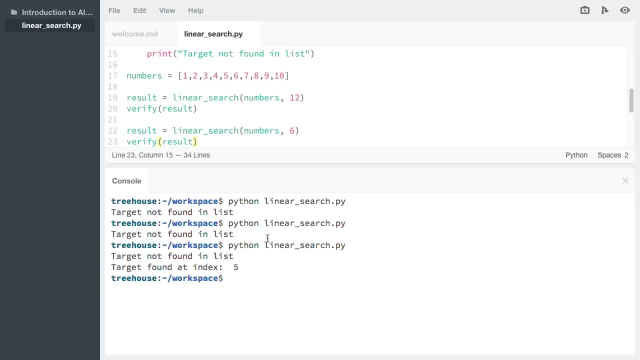 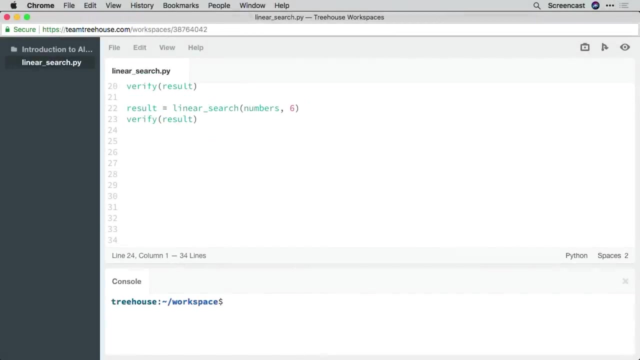 but every single thing we do on a computer takes up space in memory. in the early days of computing, considering memory usage was of paramount importance because memory was limited and really expensive. these days we're spoiled. our devices are rich with memory. this is okay when we write everyday code. 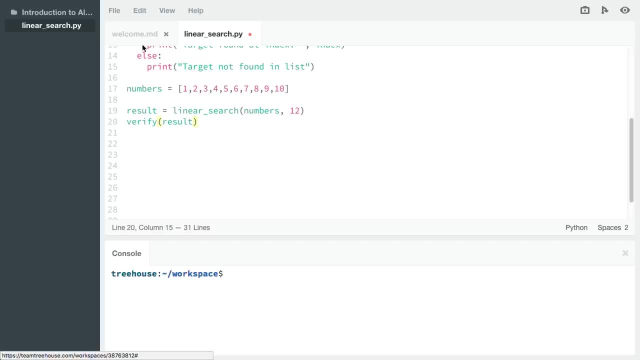 did not exist. So make sure you save the file, which you can do by going up to file and save or hitting command S and then below in the terminal you're going to type out Python linear search, or you can hit tab. 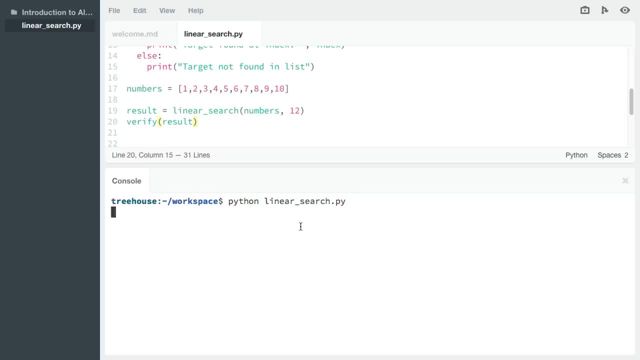 and it should auto-complete linear search dot pi. As you can see, correct the target was not found in the list, so the output of our script is what we expect. For a second test. let's search for the value 6. 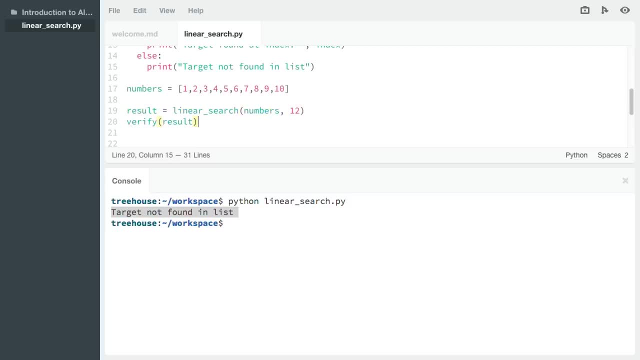 in the list. So you can call copy this command C to copy and then paste it again, and we'll just change 12 here to 6.. And then come back down to the terminal. hit the up arrow to execute the same command again. 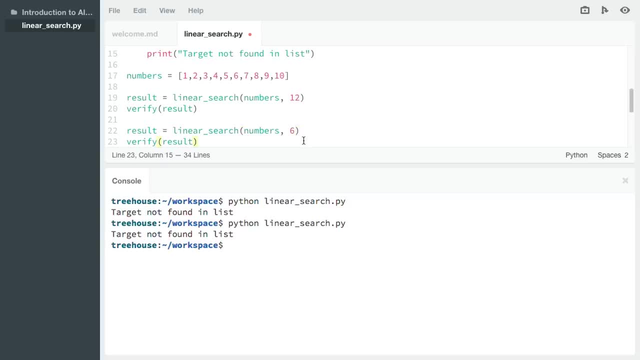 and hit enter, You'll notice that I forgot to hit save, so it did not account for that new change. we'll try that again and there you'll see that if it works correctly- which it did- the index should be number 5.. 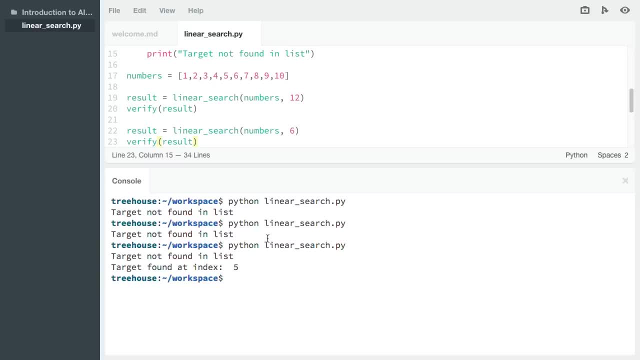 Run the program on your end and make sure everything works as expected. Our algorithm returned a result in each case. it executed in a finite time and the results were the ones we expect. In the next video, let's tackle binary search. 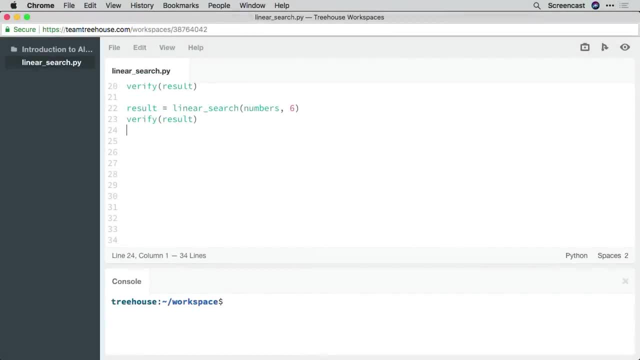 In the last video we left off with an implementation of linear search. Let's do the same for binary search so that we get an understanding of how this is represented in code. So we'll do this in a new file. back to file. 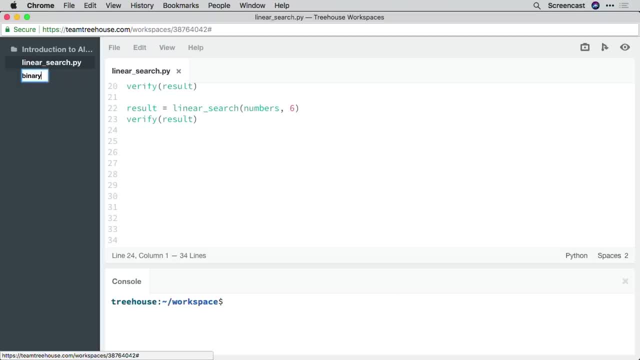 new file and we'll name this one binarysearchpy. Like before, we're going to start with a function named binarysearch, so we'll say def binary underscore search that takes a list and a target. If you remember, binary search works. 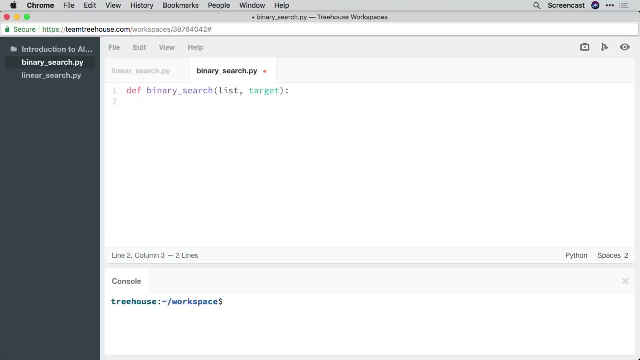 by breaking the array or list down into smaller sets until we find the value we're looking for. We need a way to keep track of the position of the list that we're working with, so let's create two variables, first and last. to point to the beginning, 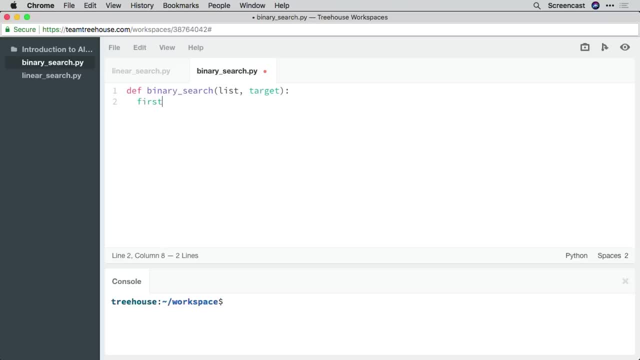 and end of the list. Now, if you're new to programming, list positions are represented by index values that start at zero instead of one. So here we're setting first to zero to point to the first element in the list. Last is going to point. 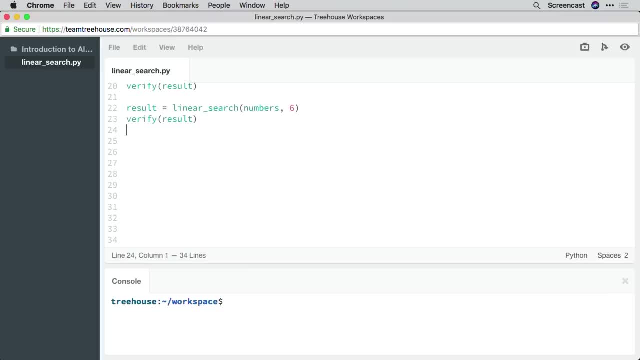 but most of us aren't dealing with enormously large data sets when we write algorithms. however, we need to think about this because we want to design our algorithms to perform as efficiently as it can, as the size of the data set n grows really large, like time, complexity. 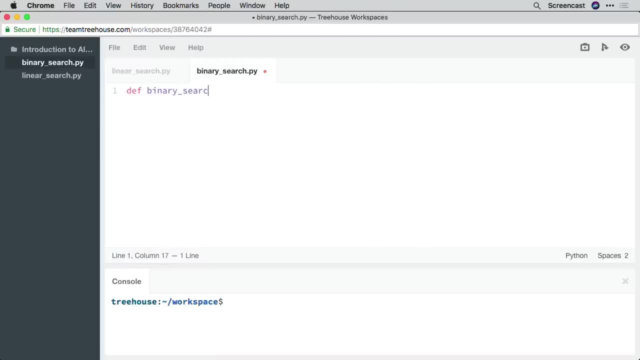 space complexity is measured, in the worst case scenario, using big O notation. since you are familiar with the different kinds of complexities, let's dive right into an example. in our iterative implementation of binary search- the first one we wrote that uses a while loop- let's look at what happens to our memory usage. 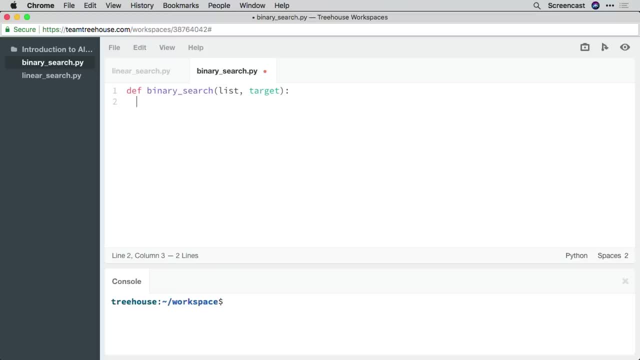 as n gets large. let's bring up that function. let's say we start off with a list of 10 elements. now, inspecting the code, we see that our solution relies heavily on these two variables: first and last. first points to the start of the list and last to the end. 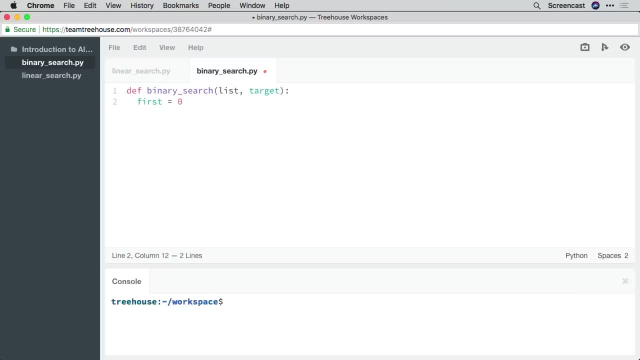 when we eliminate a set of values. instead, we just redefine first and last, as you see here to point to a different section of the list, since the algorithm only considers the values between first and last when determining the midpoint, by redefining first and last as the algorithm proceeds. 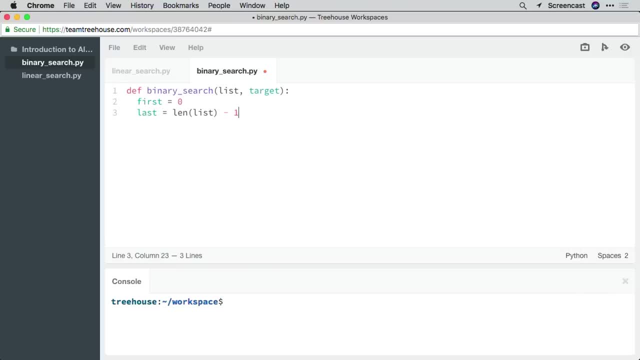 we can find a solution using just the original list. this means that for any value of n, the space complexity of the iterative version of binary search is constant, or that the iterative version of binary search takes constant space. remember that we would write this as O. this might seem confusing. 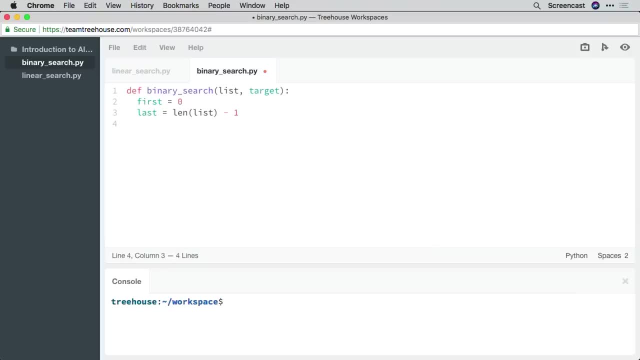 because as n grows, we need more storage to account for that larger list size. now, this is true, but that storage is not what space complexity cares about measuring. we care about what additional storage is needed as the algorithm runs and tries to find a solution. if we assume something simple, 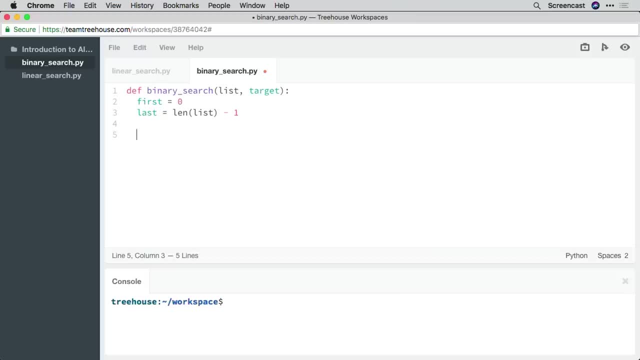 say that for a given size of a list represented by a value n, it takes n amount of space to store it. whatever that means then for the iterative version of binary search, regardless of how large the list is at the start, middle and end of the algorithm process. 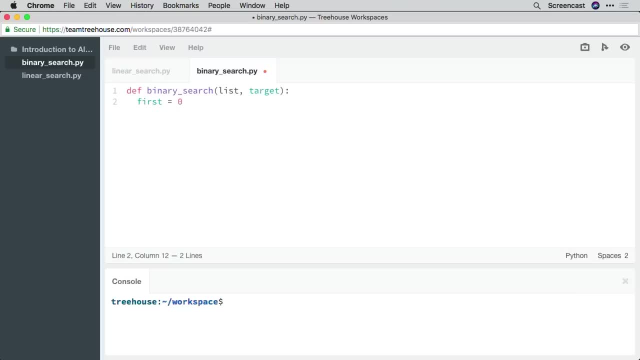 to the last element in the list. so we'll say: last equal lenlist minus one. Now this may be confusing to you, so a quick sidebar to explain what's going on. So let's say: last equals lenlist. Let's say: 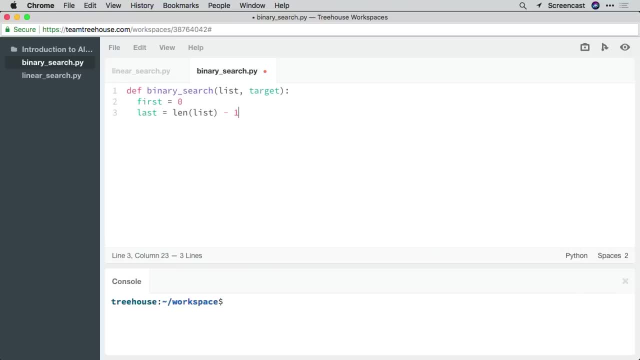 we have a list containing five elements. If we called len on that list, we should get five back because there are five elements. But remember that because the position numbers start at zero, the last value is not at position five but at four. 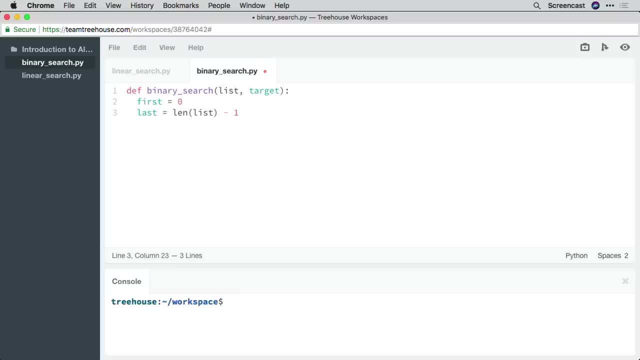 In nearly all programming languages, getting the position of the last element in the list is obtained by determining the length of the list and deducting one, which is what we're doing. Okay, so we know what the last positions are when we start the algorithm. 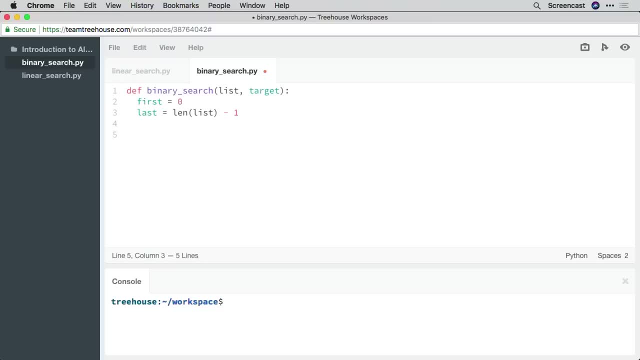 For our next line of code, we're going to create a while loop. A while loop takes a condition and keeps executing the code inside the loop until the condition evaluates to false. For our condition, we're going to say to keep executing this loop. 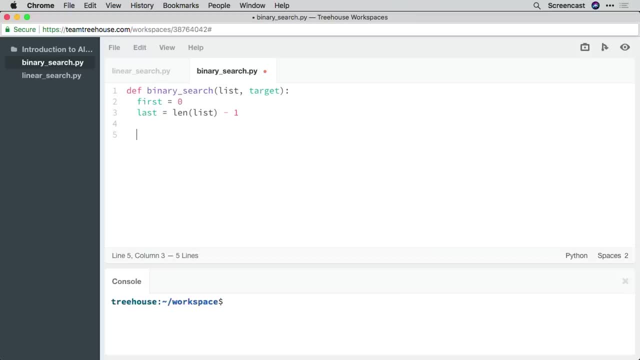 until the value of first is less than or equal to the value of last. So, while first less than or equal to last, well, you ask, why is this our condition? Well, let's work through this implementation, and then a visualization should help. 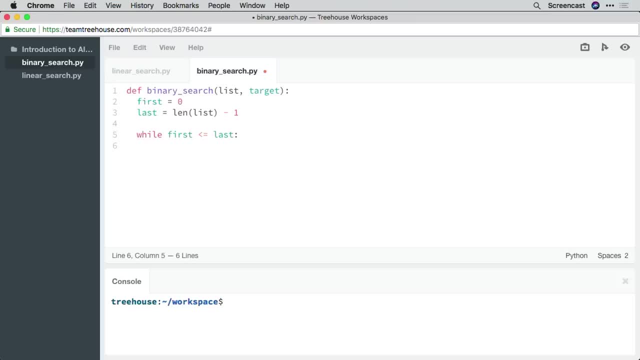 Inside the while loop we're going to calculate the midpoint of our list, since that's the first step of binary search: Midpoint equal. so we'll say first plus last, and then we'll use the floor division, double slash here, divided by two. 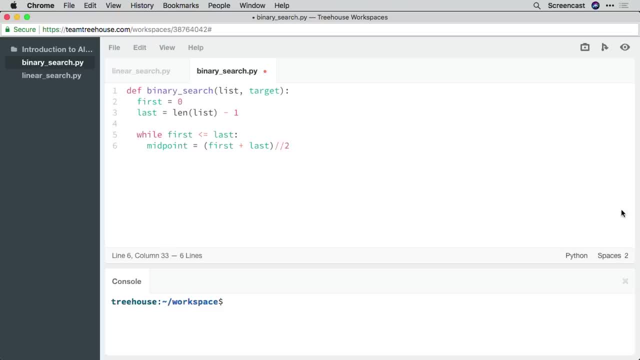 Now the two forward slashes. here are what Python calls a floor division operator. It rounds down to the nearest whole number. So if we have an eight element array, first is zero, last is seven. If we divided zero plus seven, which is seven, 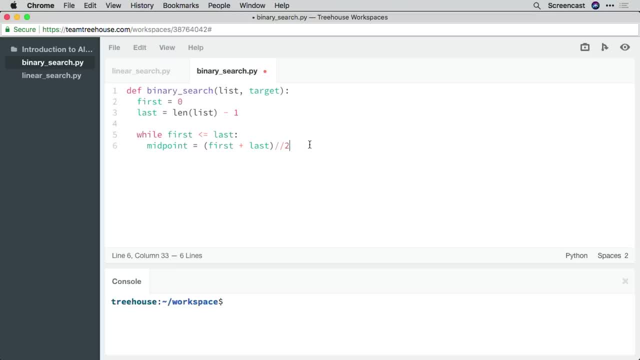 by two, we would get 3.5.. Now, 3.5 is not a valid index position, so we round that down to three using the floor division operator. Okay, so now we have a midpoint. The next step of binary search. 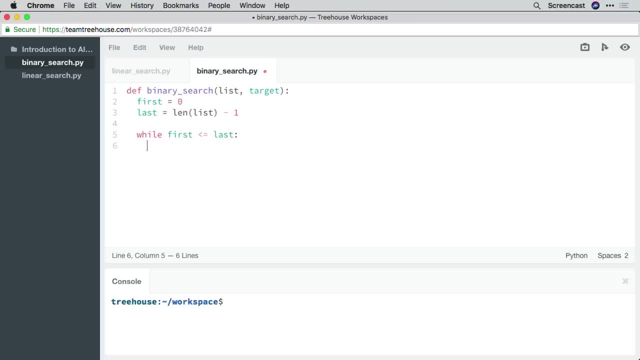 the amount of storage required does not get larger than n, and this is why we consider it to run in constant space. now this is an entirely different story with the recursive version of binary search. in the recursive version of binary search, we don't make use of variables. 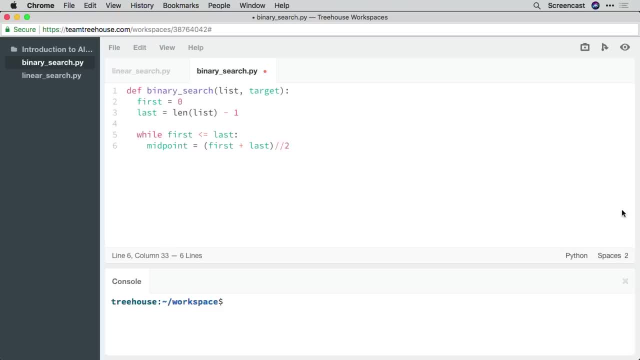 to keep track of which portion of the list we're working with. instead, we create new lists every time with a subset of values, or sublists with every recursive function call. let's assume we have a list of size n and in the worst case scenario the target element is the last in the list. 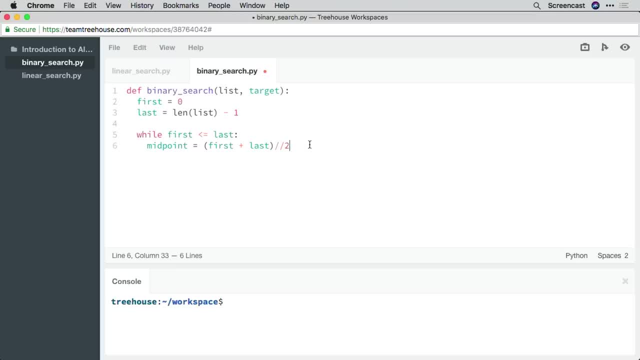 calling the recursive implementation of binary search on this list and target. the function would call itself and create a new list that goes from the midpoint to the end of the list. since we're discarding half the values, the size of the sublist is n by 2. 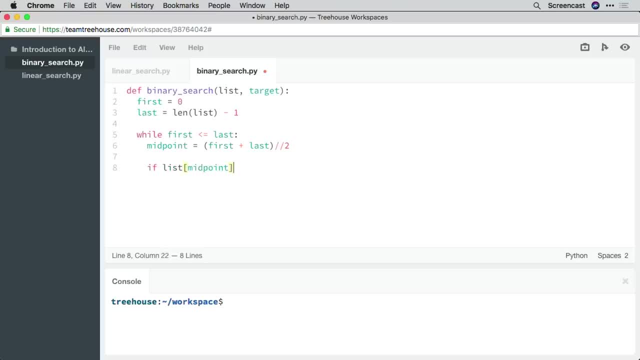 this function will keep calling itself, creating a new sublist that's half the size of the current one, until it arrives at a single element list and a stopping condition- this pattern that you see here, where the size of the sublist is reduced by a factor on each execution of the output. 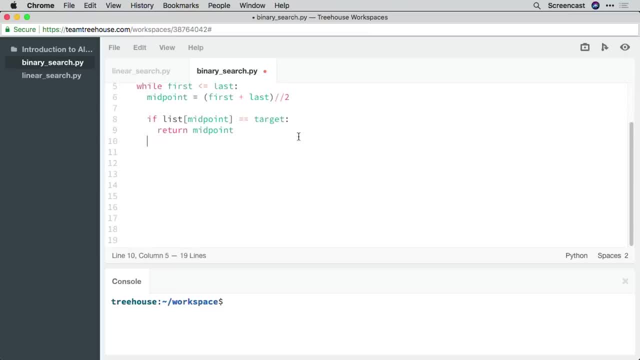 algorithmic logic. well, we've seen that pattern before. do you remember where? this is exactly how binary search works? it discards half the values every time until it finds a solution. now we know that because of this pattern, the running time of binary search is logarithmic. 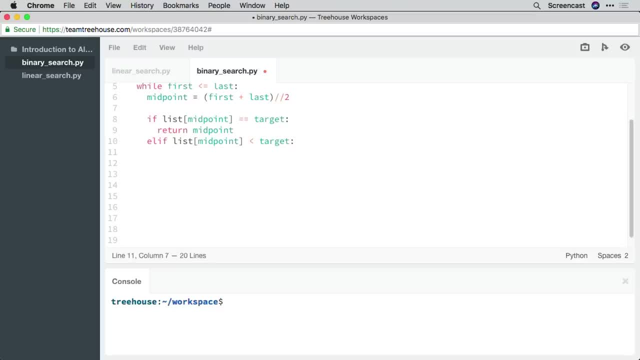 in fact, the space complexity of the recursive version of binary search is the same. if we start out with a memory allocation of size n that matches the list on each function call, we need to allocate additional memory of size n by 2, n by 4, and so on. 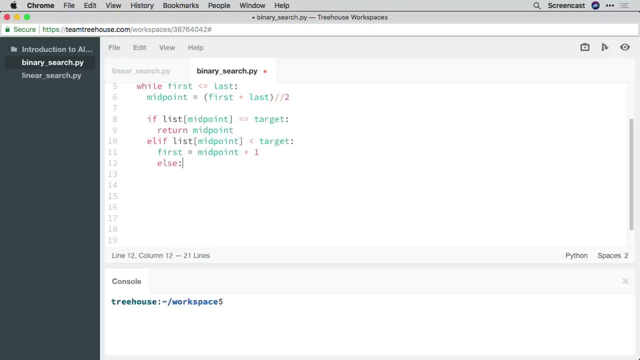 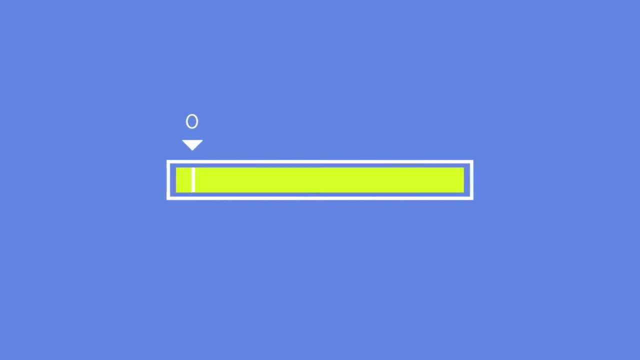 until we have a sublist that is either empty or contains a single value. because of this, we say that the recursive version of the binary search algorithm runs in logarithmic time with a big O of log n. now there's an important caveat here. this totally depends on the language. 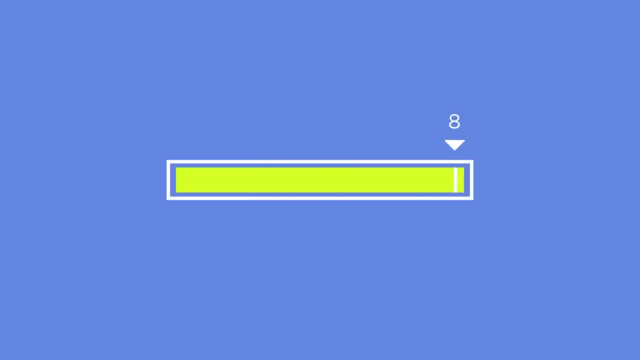 remember how I said that a programming language like swift can do some tricks to where recursion depth doesn't matter. the same concept applies here. if you care to read more about this concept, it's called tail optimization. it's called tail optimization because if you think of a function, 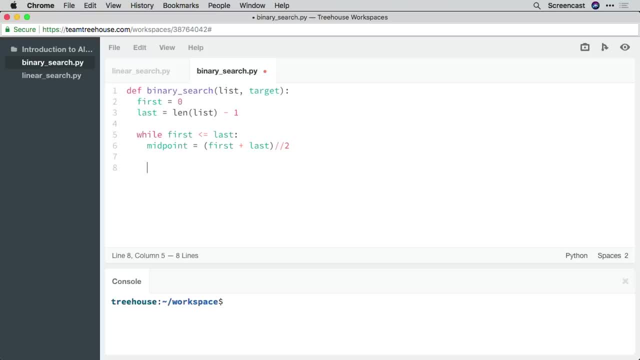 is to evaluate whether the value at this midpoint is the same as the target. if list and value at midpoint equals the target, Well, if it is, then we'll go ahead and return the midpoint. So we'll say: return midpoint The return statement. 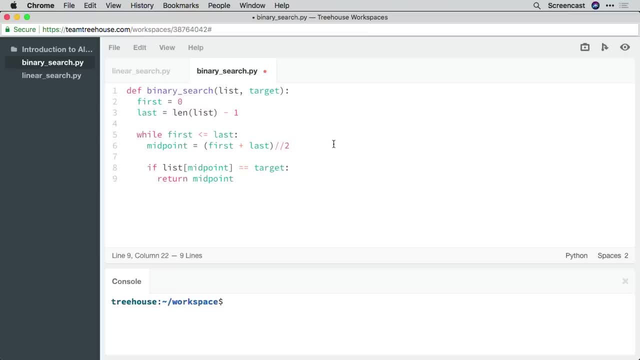 terminates our algorithm and over here we're done. This is our best case scenario. Next, we'll say else if list at midpoint or value at midpoint is less than the target. Now here, if the value is less, the value at midpoint is less than the target. 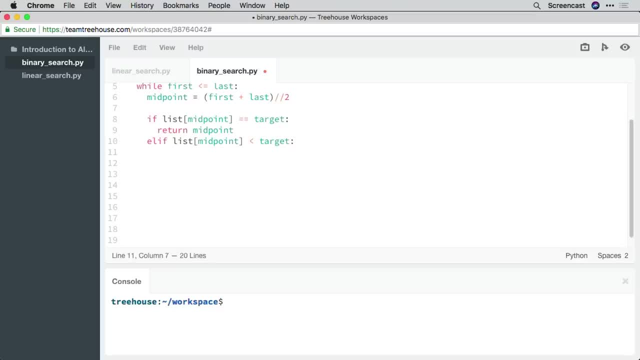 then we don't care about any of the values lower than the midpoint. So we redefine first to point to the value after the midpoint. So we'll say midpoint plus one. Now if the value at the midpoint is greater than the target, then we can discard. 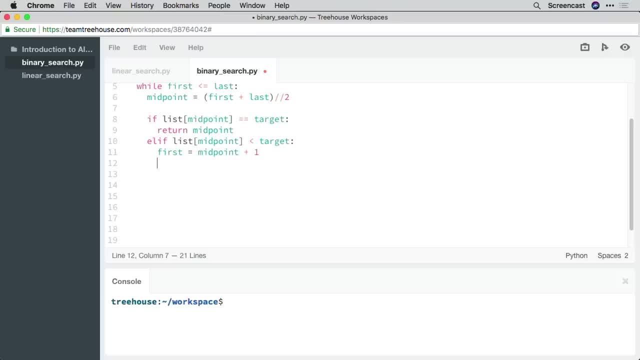 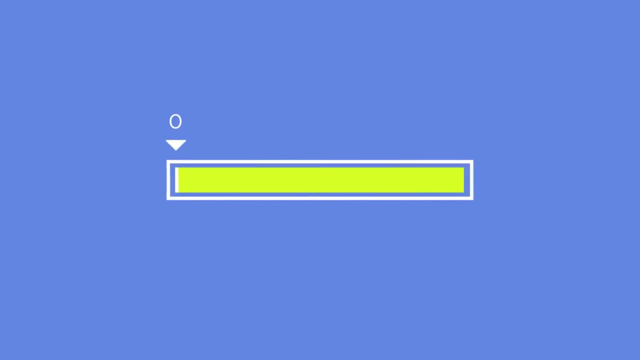 the values after the midpoint and redefine last to point to the value prior to the midpoint. Last equal midpoint minus one. Let's visualize this. We're going to start with a list of nine integers. To make this easier to understand, let's specify: 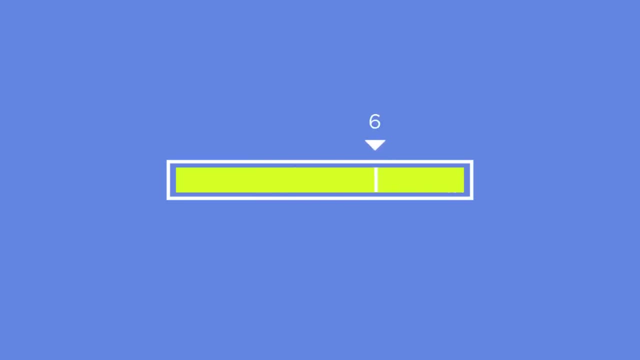 these integers to be of the same value as its index position. So we have a range of values from zero to eight. Our target is the worst case scenario. We're looking for the position of the value eight At the start. our algorithm sets first. 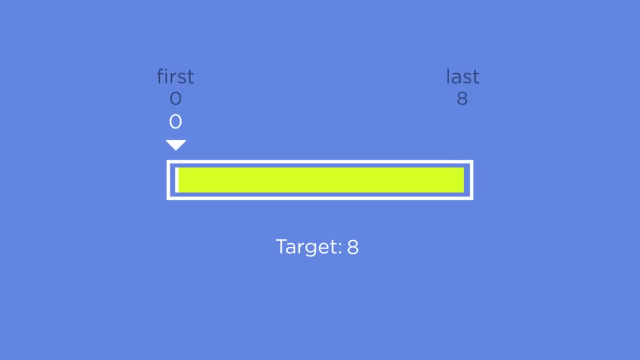 to point to zero and last, to point to the length of the list minus one, which is eight. Next, we hit our while loop. The logic of this loop is going to be executed as long as the value of first is not greater than the value. 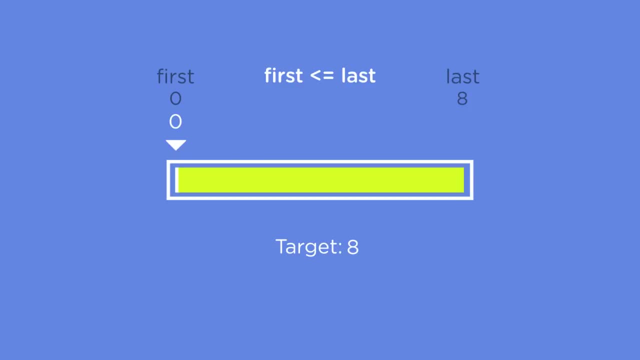 of last, Or as we've defined it. we're going to keep executing the contents of the loop as long as first is less than or equal to last. On the first pass we'll write two and round it down, so we get a nice even four. 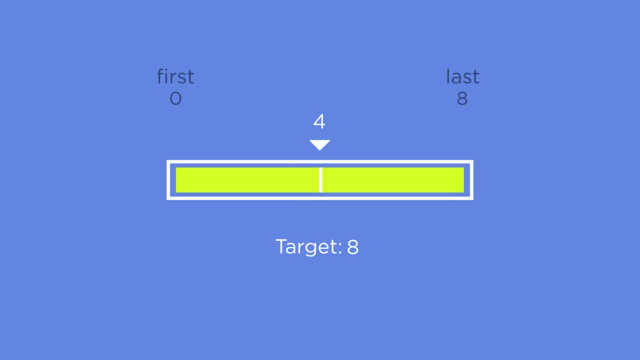 The value at this position is four. Now this is not equal to the target, so we move to the first, else if Four is less than eight. so now we redefine first to point to midpoint plus one, which is five. First is still less than last. 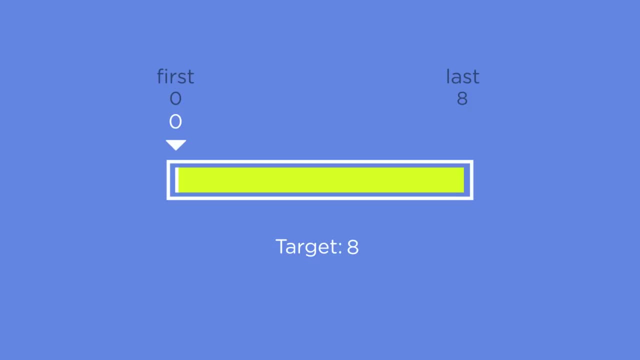 as having a head and a tail. if the recursive function call is the last line of code in the function, as it is in our case, we call this tail recursion, since it's the last part of the function that calls itself. now the trick that swift does to reduce 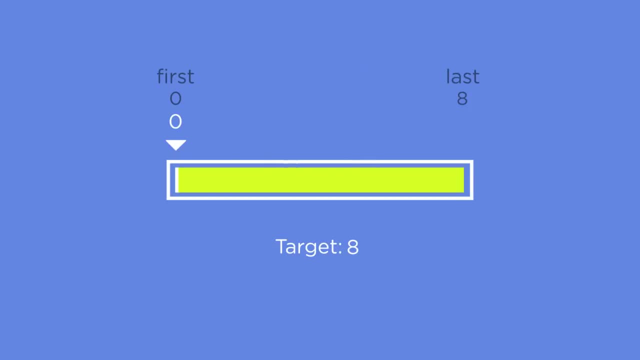 the amount of space and therefore computing overhead to keep track of these recursive calls is called tail call optimization or tail call elimination. it's one of those things that you'll see thrown around a lot in algorithm discussions but may not always be relevant to you. now what if any of this is relevant to us? 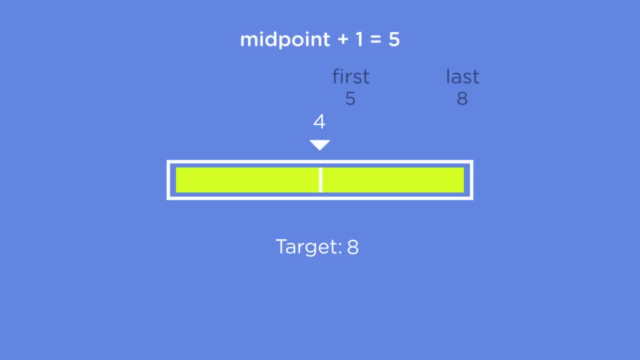 well, python does not implement tail call optimization, so the recursive version of binary search takes logarithmic space. if we had to choose between the two implementations, given that time, complexity or run time of both versions- the iterative and the recursive version- are the same, we should definitely go with the iterative implementation. 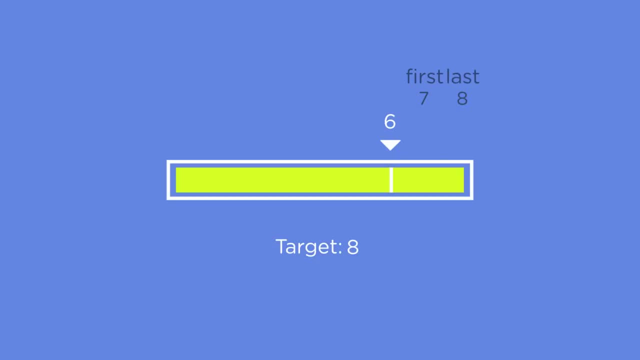 in python, since it runs in constant space. okay, that was a lot, but with all of this, we've now established two important ways to distinguish between algorithms that handle the same task and determine which one we should use. we've arrived at what I think is a good spot. 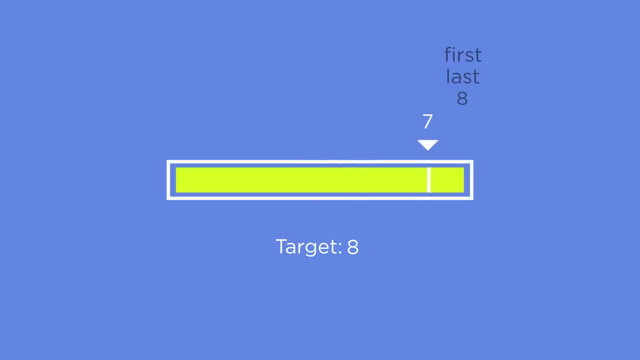 to take a long break and let all of these new concepts sink in. but before you go off to the next course, let's take a few minutes to recap everything we've learned so far. while we did implement two algorithms in this course in actual code, much of what we learned here was conceptual. 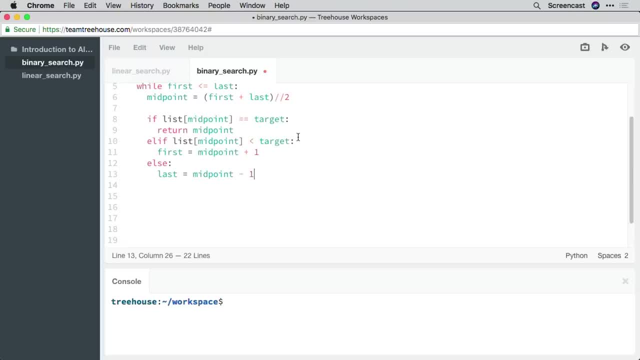 and will serve as building blocks for everything we're going to learn in the future. so let's list all of it out. the first thing we learned about, and arguably the most important, was algorithmic thinking. algorithmic thinking is an approach to problem solving that involves breaking a problem down. 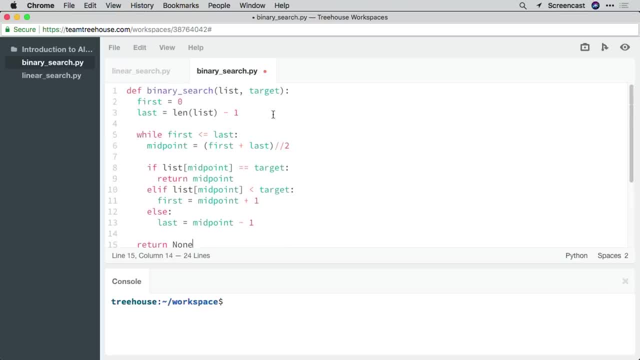 into a clearly defined input and output, along with a distinct set of steps that solves the problem by going from input to output. algorithmic thinking is not something you develop overnight by taking one course, so don't worry if you're thinking I still don't truly know how to apply. 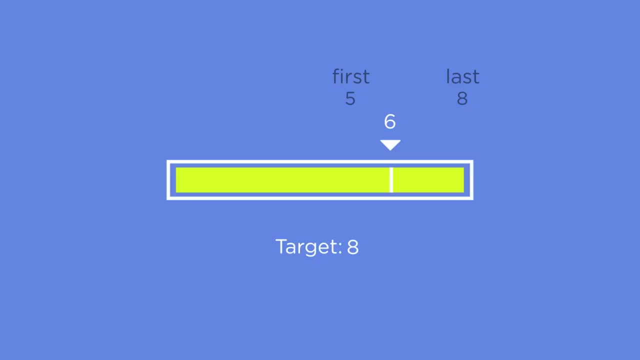 so we run through the body of the loop again. The midpoint is now six. Six is less than eight, so we move to seven. Seven is still less than or equal to eight, so we go for another iteration of the loop. The midpoint is seven. 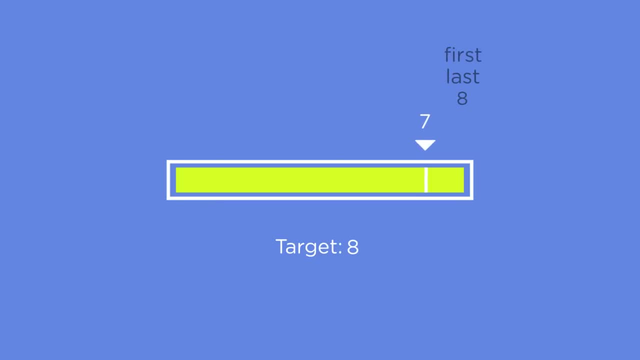 oddly enough, and seven is still less than the target. so we move first to point to eight. First is equal to last. now, but our condition says: keep the loop going as long as first is less than or equal to the target and we finally exit our algorithm. 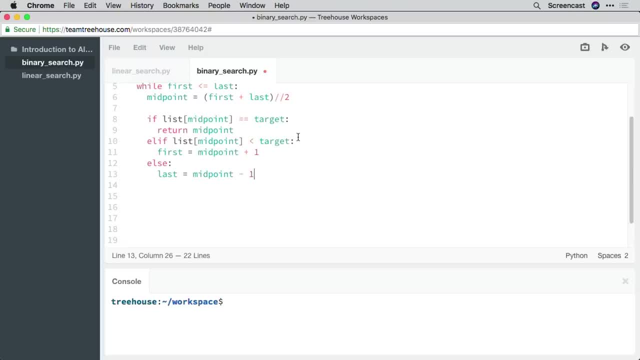 and return the position of the target. Now what if we had executed all this code and never hit a case where midpoint equal the target? Well, that would mean the list did not contain the target value. so after the while loop at the bottom, we'll return. 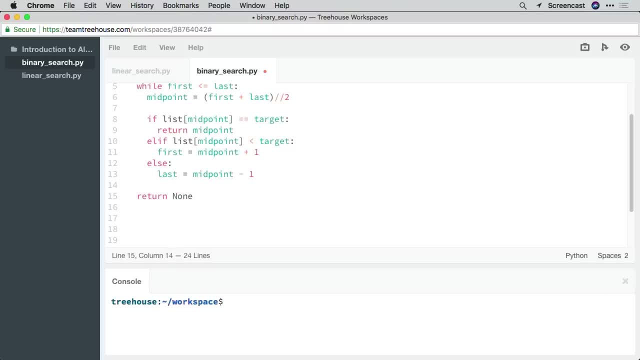 none. We have several operations that make up our binary search algorithm, so let's look at the runtime of each step. Let's start by assigning values to first and last. The value assigned to last involves a call to the len function to get the size. 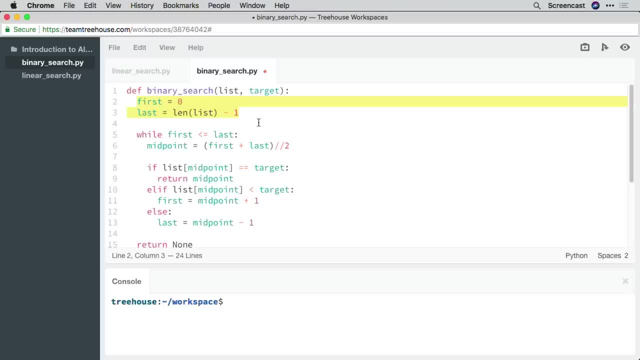 of the list. but we already know this is a constant time operation in Python, so both of these operations run in constant time. Inside the loop we have another value assignment and this is a simple division operation. so again, the runtime is constant. In the next line of code, 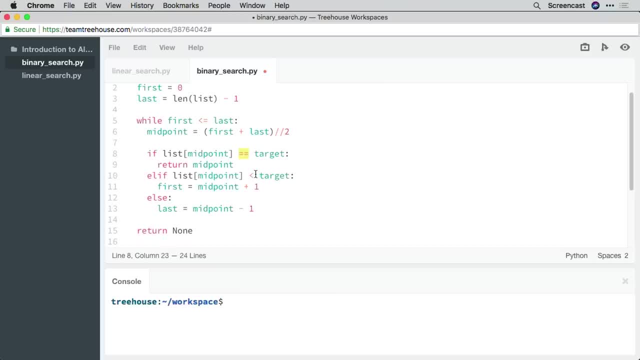 we're reading the value point to the target. Both of these, again, are constant time operations. The remainder of the code is just a series of comparisons and value assignments, and we know that these are all constant time operations as well. So if all we have 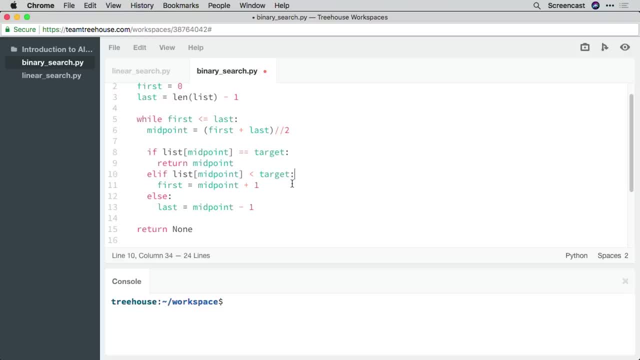 are a series of constant time operations. why does this algorithm have, in the worst case, a logarithmic runtime? It's hard to evaluate by just looking at the code, but the while loop is what causes the runtime, even though all we're doing is a comparison operation. 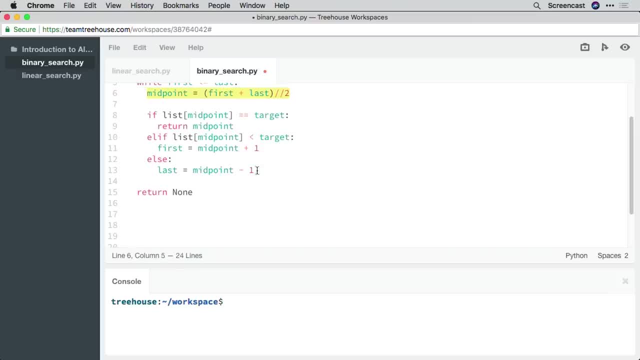 by redefining first and last over here, or rather in the last two steps over here, we're asking the algorithm to run as many times as it needs until first is equal or greater than last. Now, each time the loop does this the size of the dataset. 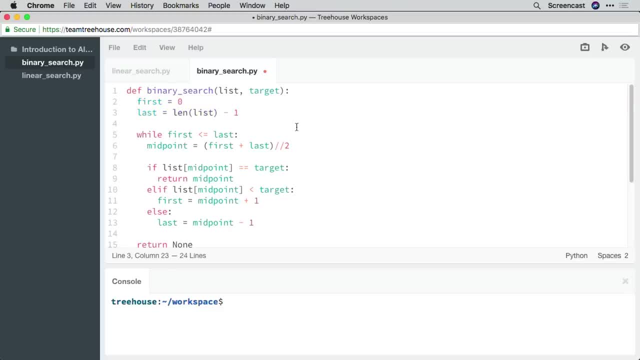 what I learned here. algorithmic thinking sinks in after you go through several examples, in a similar fashion to what we did today. it also helps to apply these concepts in the context of a real example, which is another thing we will strive to do. moving forward regardless, it is important to keep in mind. 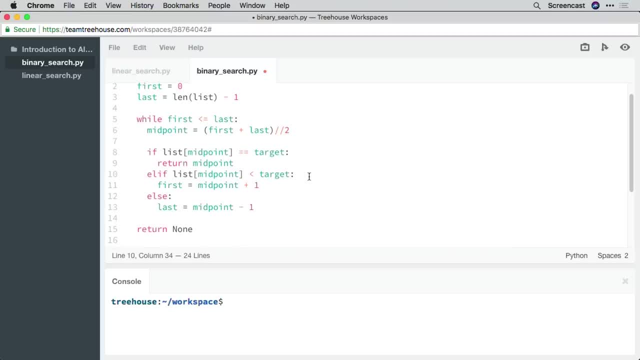 that the main goal here is not to learn how to implement a specific data structure or algorithm off the top of your head. I'll be honest, I had to look up a couple code snippets for a few of the algorithms myself in writing this course, but in going through this, 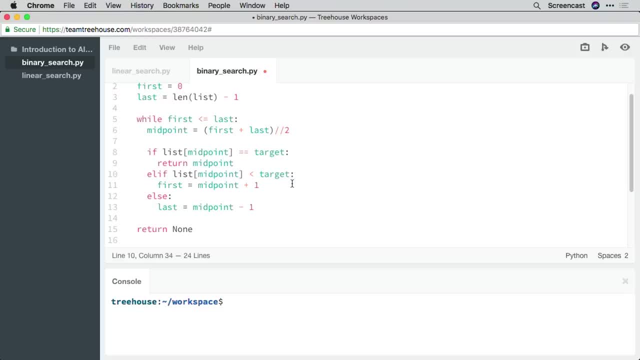 you now know that binary search exists and can apply to a problem where you need a faster search algorithm. unlike most courses where you can immediately apply what you have learned to build something cool, learning about algorithms and data structures will pay off more in the long run. the second thing: 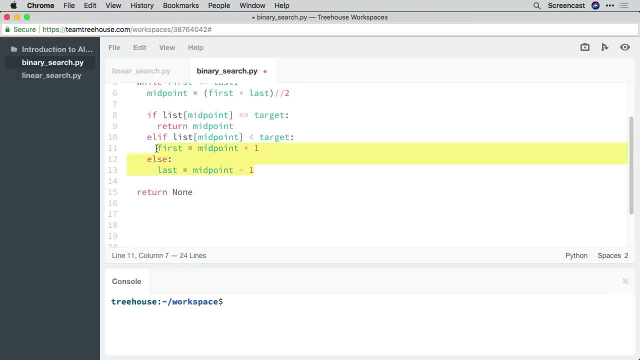 we learned about is how to define and implement algorithms. we've gone over these guidelines several times so I won't bore you here again at the end, but I will remind you that if you're often confused about how to effectively break down a problem in code, 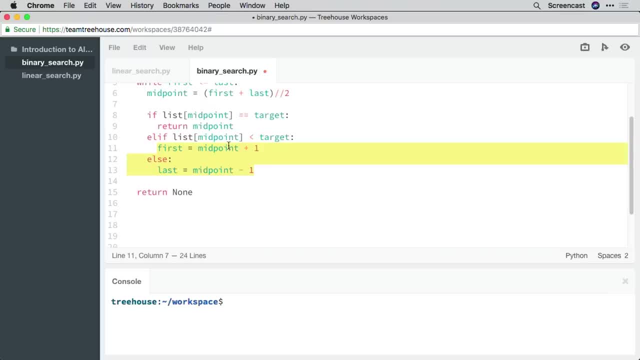 to something more manageable. following those algorithm guidelines is a good place to start. next we learned about Big O and measuring the time complexity of algorithms. this is a mildly complicated topic, but once you've abstracted the math away, it isn't as hazy a topic as it seems. 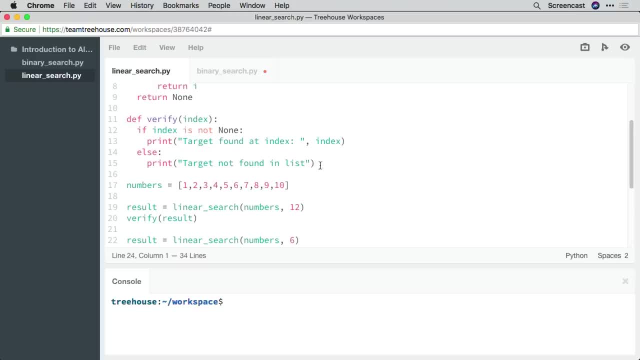 now, don't get me wrong. the math is pretty important, but only for those designing and analyzing algorithms. our goal is more about how to understand and evaluate algorithms. we learned about common run times like constant, linear, logarithmic and quadratic run times. these are all things that 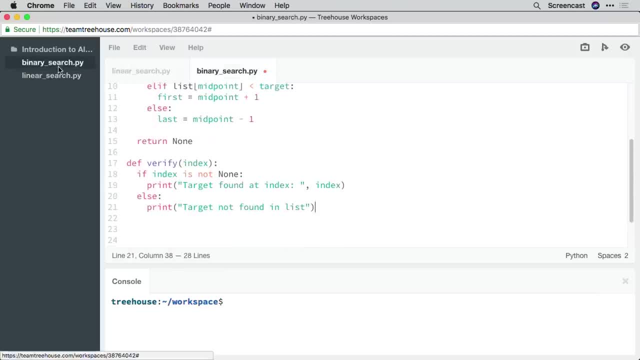 are fairly new concepts, but in time you will immediately be able to distinguish the run time of an algorithm based on the code you write and have an understanding of where it sits on an efficiency scale. you will also, in due time, internalize run times of popular algorithms. 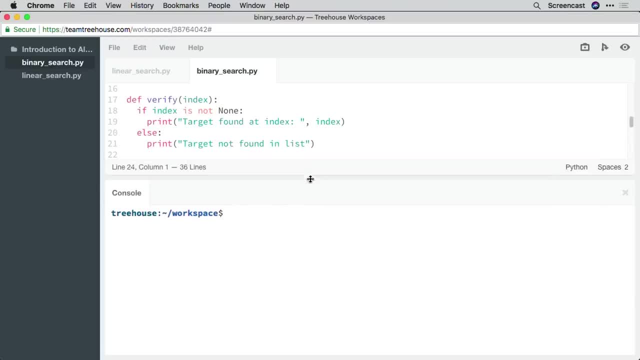 like the fact that binary search runs in logarithmic time and constant space and be able to recommend alternative algorithms for a given problem. all in all, over time, the number of tools in your tool belt will increase. now, next, we learned about two important search algorithms and the situations in which we select one over the other. 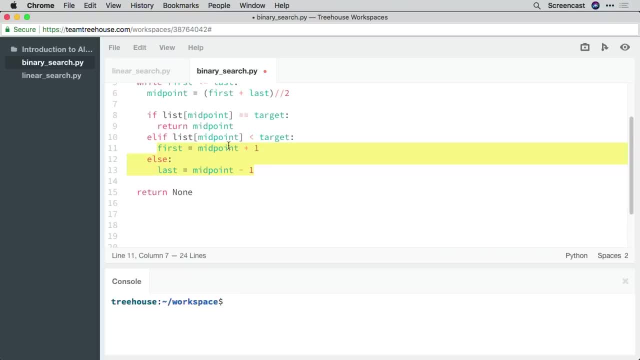 the size of the list grows smaller by a certain factor of the logarithmic runtime. Okay, just like with linear search, let's test that our algorithm works. So we'll go back to linearsearchpy and we're going to copy paste. so command c to copy. 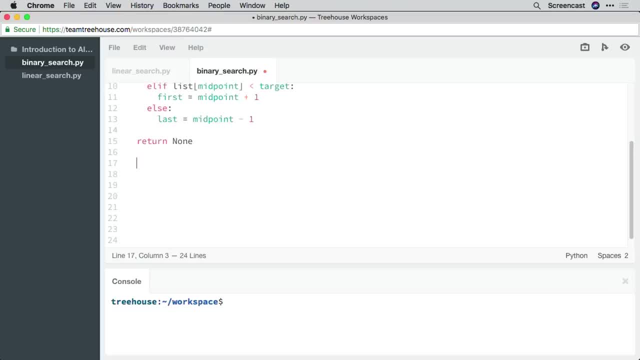 if you're on a Mac, then go back to binary search and at the bottom, oops, we're going to paste in that verify function. Okay, we'll also go back and grab this numbers. you know what? let's go ahead and do verify cases, we'll paste. 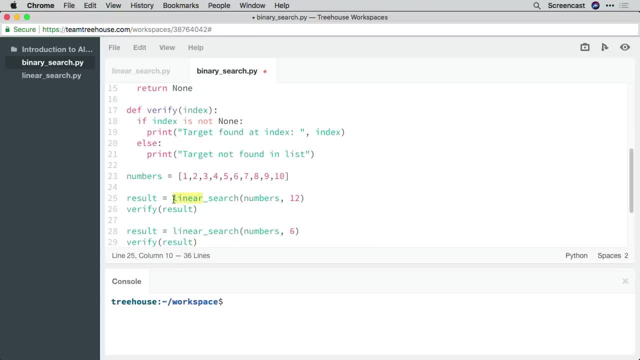 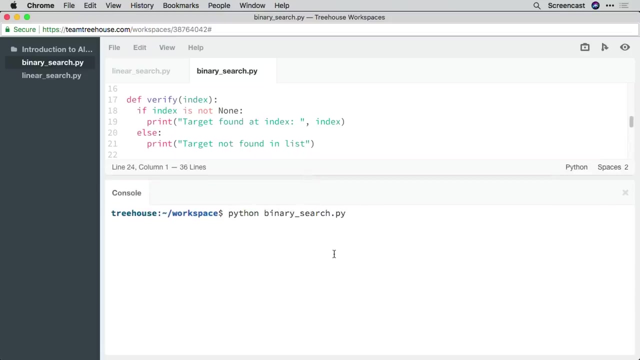 that in as well, and the only thing we need to change here is, instead of calling linear search, this is going to call binary search. Okay, we'll hit command s to save the file, and then I'm going to drag up my console and we'll run. 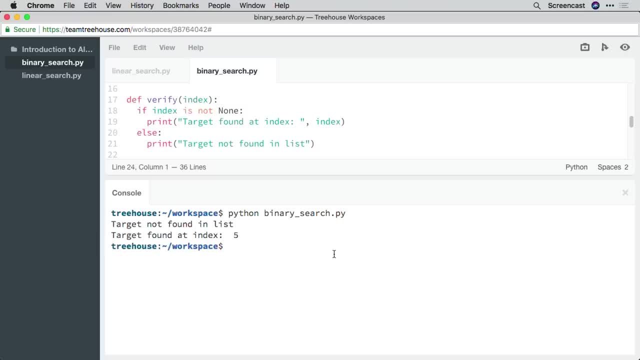 python binary search, dot pi and hit enter and you'll see, like just like before, we get the same results. the numbers list that we've defined for our test cases right here has to be sorted. The basic logic of binary search relies on the fact that if the target 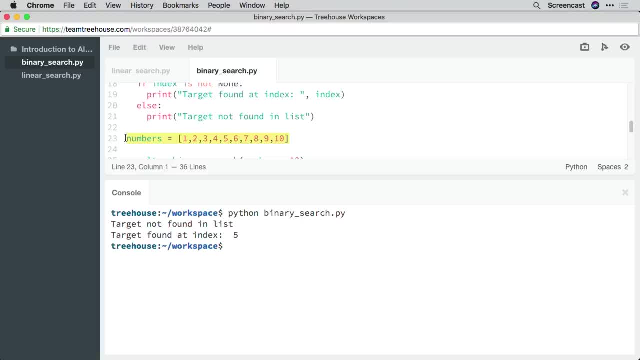 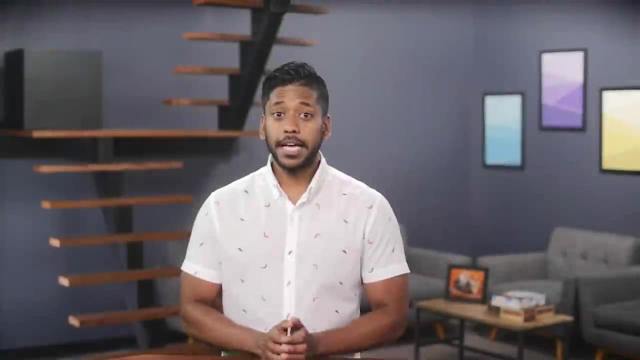 is greater than the midpoint, then our potential values lie to the left, or vice versa, since the values are sorted in ascending order. If the values are unsorted, our implementation of binary search may return none in the list. And just like that, you've written code. 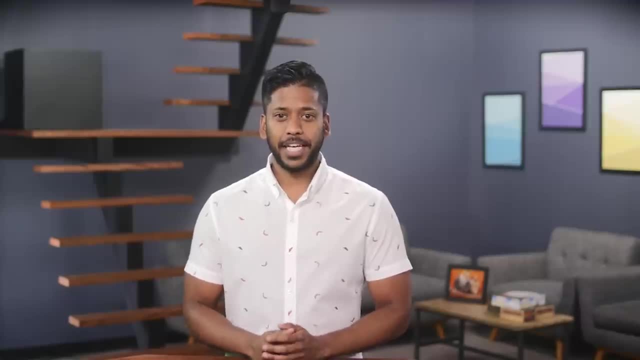 to implement two search algorithms. How fun was that. Hopefully, this course has shown you that it isn't a topic to be afraid of and that algorithms, like any other topic with code, can be broken down and understood piece by piece. Now we have a working implementation. 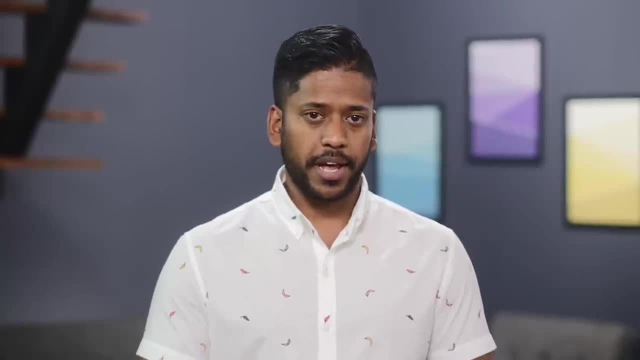 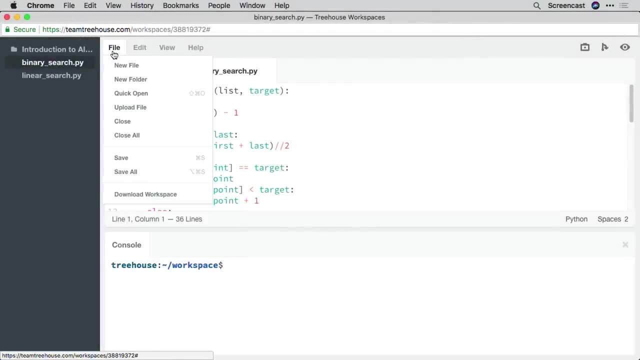 of binary search, but there's actually more than one way to write it, So in the next video let's write a second version. I'm going to create a new file, as always file, and we'll name this recursive underscore binary underscore search dot p, y. 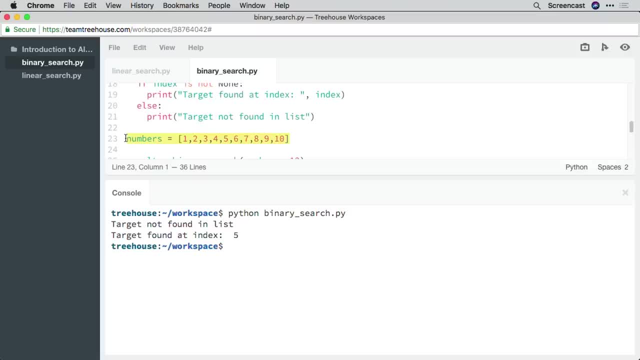 we also implemented these algorithms in code so that you got a chance to see them work. we did this in python, but if you are more familiar with a different language and haven't gotten the chance to check out the code snippets we've provided, you should try your hand at implementing it yourself. 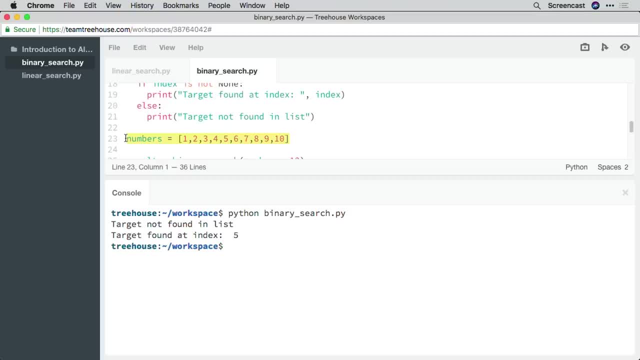 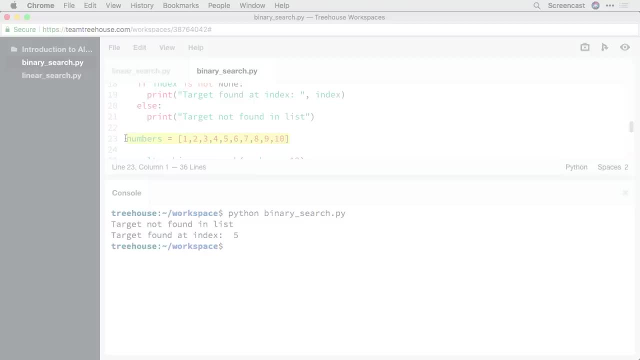 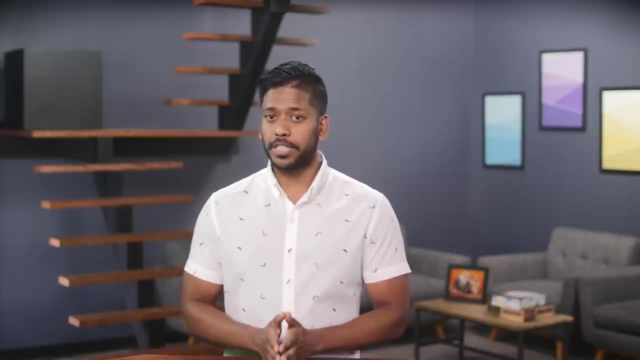 it's a really good exercise to go through. finally, we learned about an important concept and a way of writing algorithmic code through recursion. recursion is a tricky thing and, depending on the language you write code with, you may run into it more than others. it is also good to be aware of. 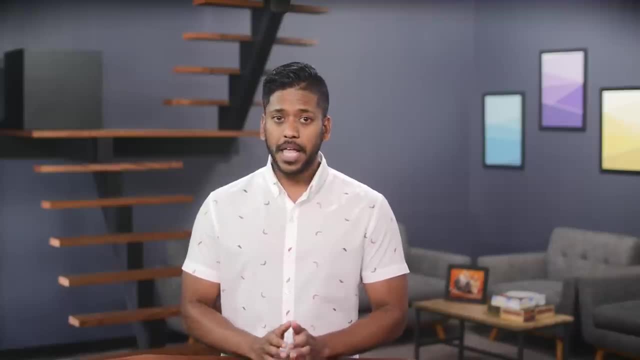 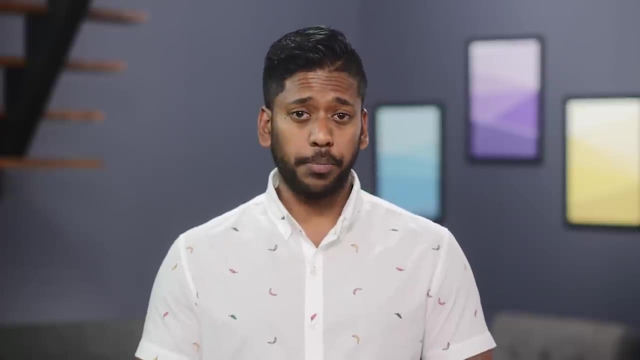 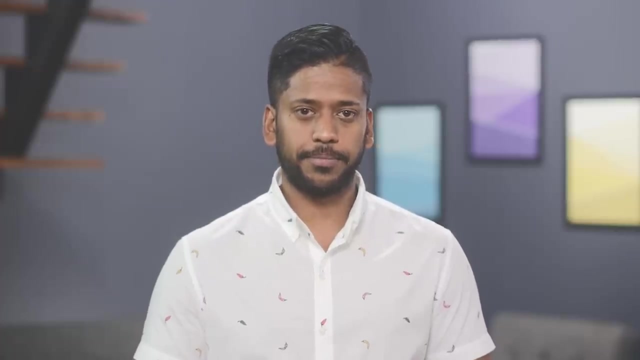 because, as we saw in our implementation of binary search, whether recursion was used or not affected the amount of space we used. don't worry if you don't fully understand how to write recursive functions. I don't truly know either. the good part is, you can always look these things up. 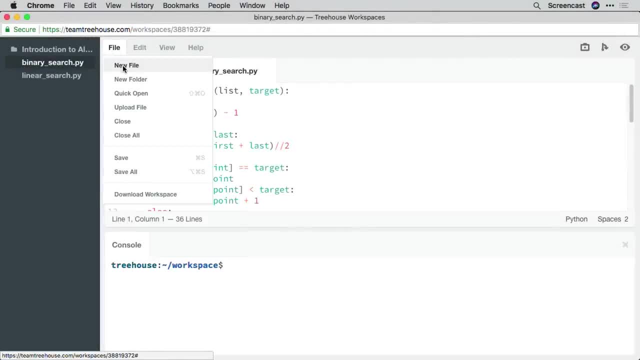 and understand how other people do it. anytime you encounter recursion in our courses moving forward, you'll get a full explanation of how and why the function is doing what it's doing. and that brings us to the end of this course. I'll stress again that the goal of this course 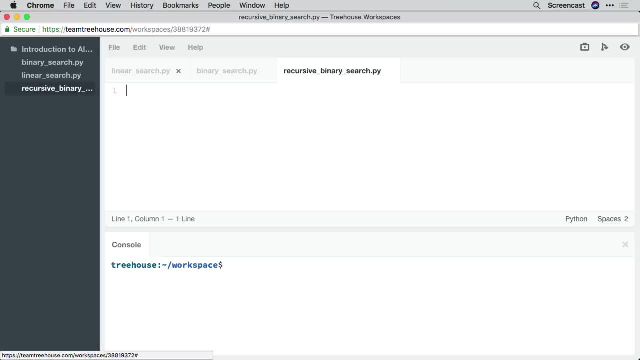 was to get you prepared for learning about more specific algorithms by introducing you to some of the tools and concepts you will need moving forward. so if you're sitting there thinking I still don't know how to write many algorithms or how to use algorithmic thinking, that's okay. 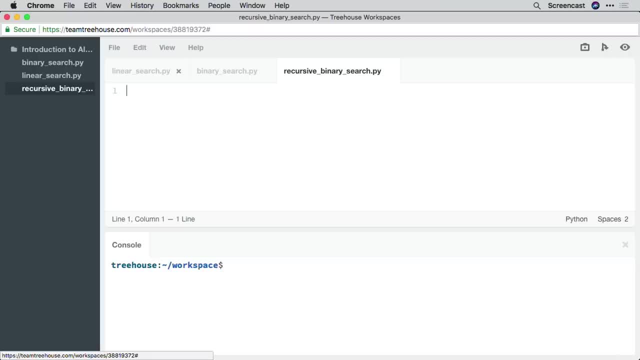 just stick with it as always. have fun and happy coding. Hi, my name is Pasan, I'm an instructor at Treehouse and welcome to the introduction to data structures course. in this course, we're going to answer one fundamental question: why do we need more data structures? 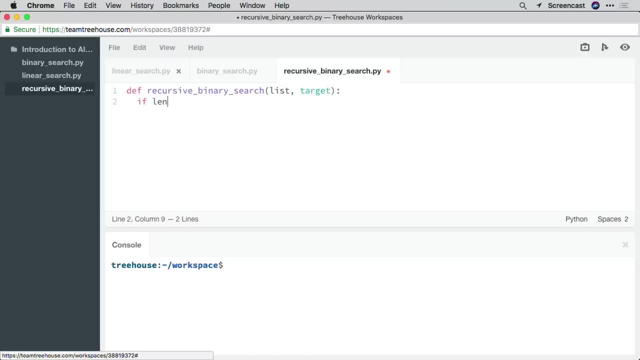 than a programming language provides. before we answer that question, if you will, in this course we're going to rely on concepts we learned in the introduction to algorithms course, namely big O, notation, space and time, complexity and recursion. if you're unfamiliar with those concepts or just need a refresher, 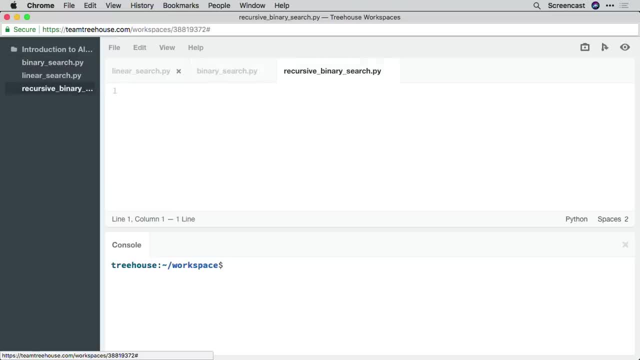 Okay, so we're going to add our new implementation here so that we don't get rid of that first implementation we wrote: Let's call this new function recursive binary search. Unlike our previous implementation, this version is going to behave slightly differently, in that it won't. 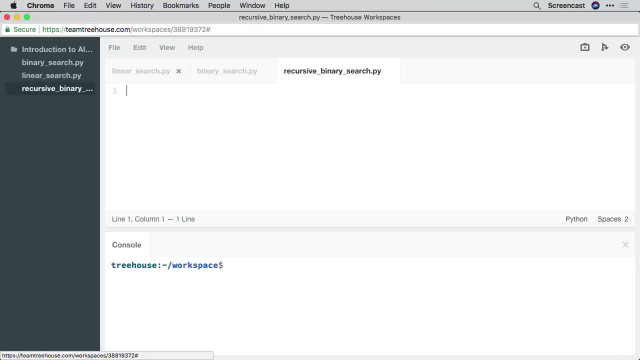 return the index value of the target. instead, it will just return a true value if it exists and a false if it doesn't. So recursive underscore, binary underscore search and, like before, this is going to take a list. it accepts a list and a target to look for. 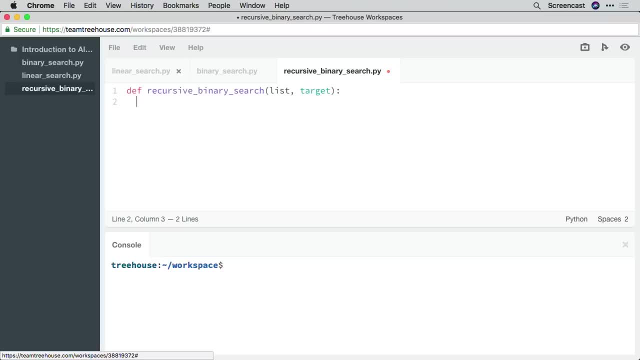 in that list. We'll start the body of the function by considering what happens if an empty list is passed in. In that case we would return false. So I would say, if the length is one way to figure it out, if it's empty, if it's equal. 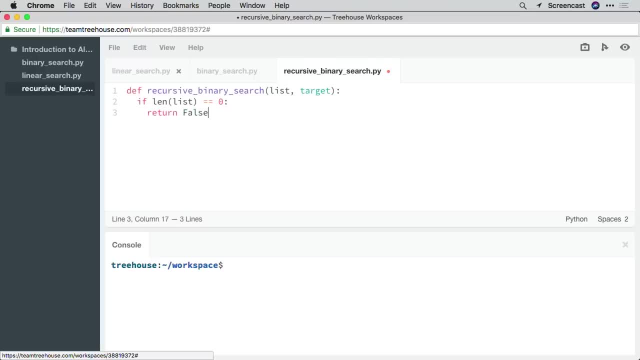 to zero, then we'll return false. Now you might be thinking that in the previous version of binary search we didn't care if the list was empty. Well, we actually did, but in a roundabout sort of way. So in the previous version of binary 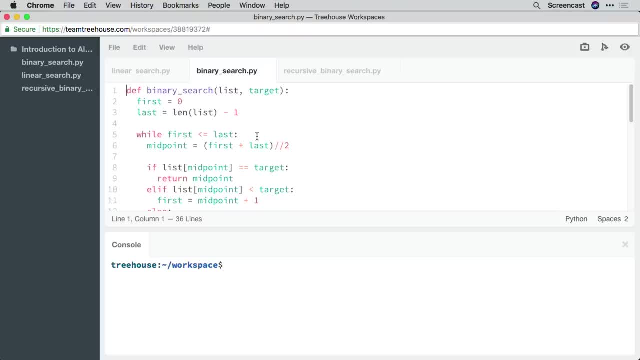 search. our function had a loop and that loop condition was true when first was less than or equal to last. Now, if we have an empty list, then first is greater than last and the loop would never execute and we return none at the bottom. So this is the same. 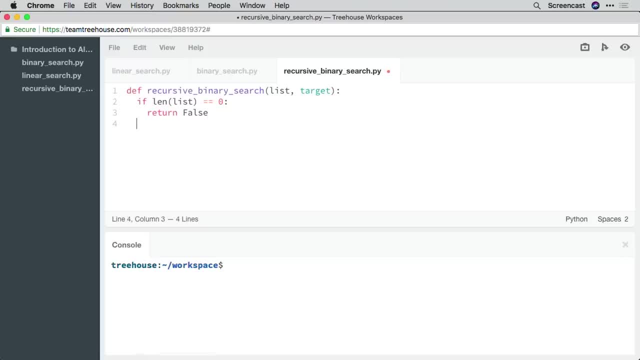 logic we're implementing here. we're just doing it in a slightly different way. If the list is not empty, we'll implement an else clause. Now, here we'll calculate the midpoint by dividing the length of the list by two and rounding down Again. there's no use. 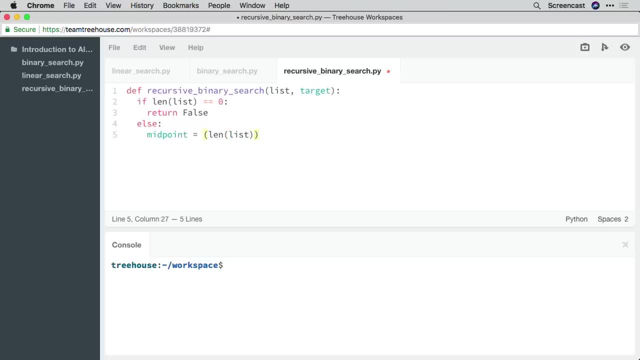 so we'll say length of list and then, using the floor division operator, we'll divide that by two. If the value at the midpoint, which we'll check by saying if list, using subscript notation, we'll say midpoint as the index. now, if this value at the midpoint, 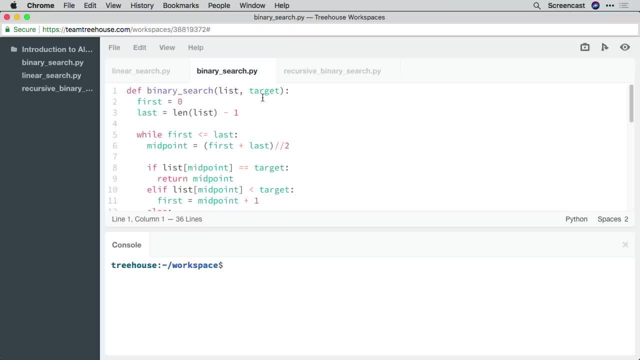 check out the prerequisites courses listed. in addition, this course does assume that you have some programming experience. we're going to use data structures that come built into nearly all programming languages as our point of reference. while we will explain the basics of how these structures work, we won't be going over 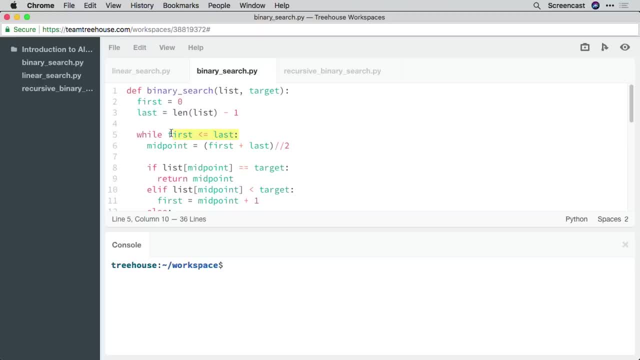 how to use them in practice. if you're looking to learn how to program, before digging into this content, check the notes section of this video for helpful links. if you're good to go, then awesome. let's start with an overview of this course, the first thing we're going to do. 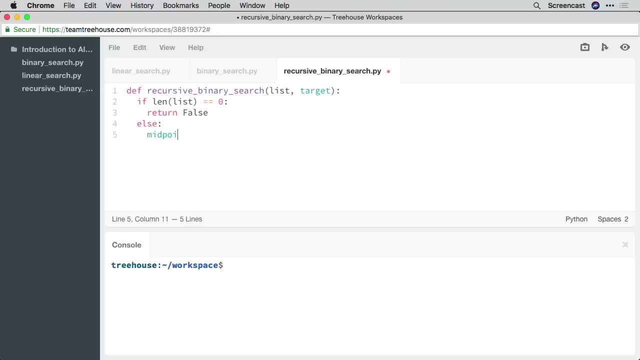 is to explore a data structure. we are somewhat already familiar with arrays. if you've written code before, there's a high chance you have used an array. in this course, we're going to spend some time exploring how arrays work. what are the common operations on an array? 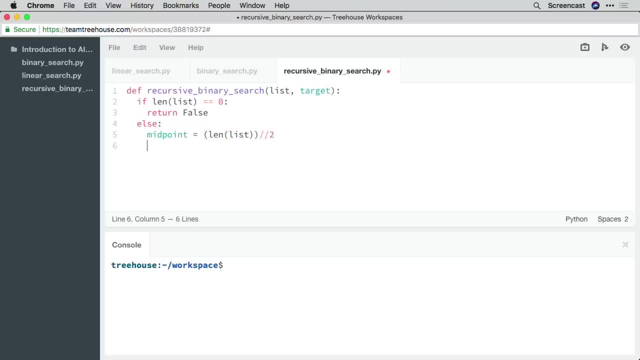 and what are the run times associated with those operations. once we've done that, we're going to build a data type of our own, called a linked list. in doing so, we're going to learn that there's more than one way to store data. in fact, there's way more than just one way. 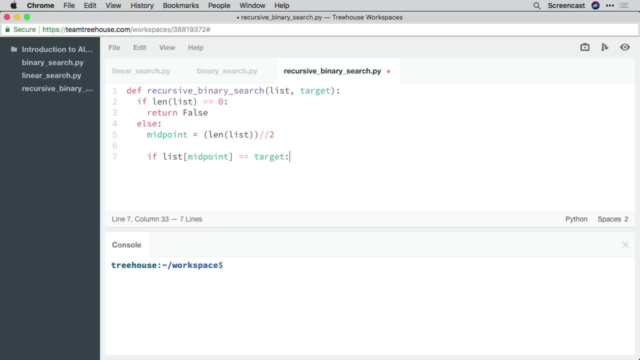 we're also going to explore what motivates us to build specific kinds of structures and look at the pros and cons of these structures. we'll do that by exploring four common operations: accessing a value, searching for a value, inserting a value and deleting a value. after that, 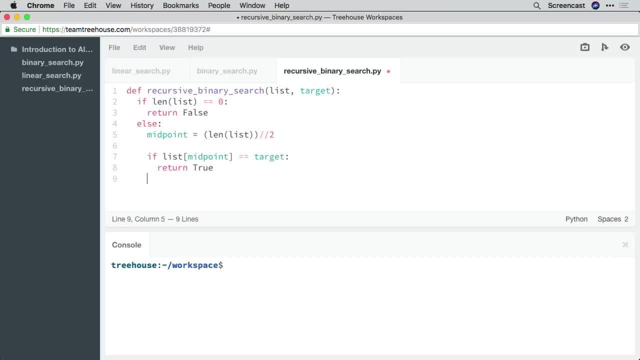 we're actually going to circle back to algorithms and implement a new one, a sorting algorithm. in the introductions to algorithms course, we implemented a binary search algorithm. a precondition to binary search was that the list needed to be sorted. we're going to try our hand. 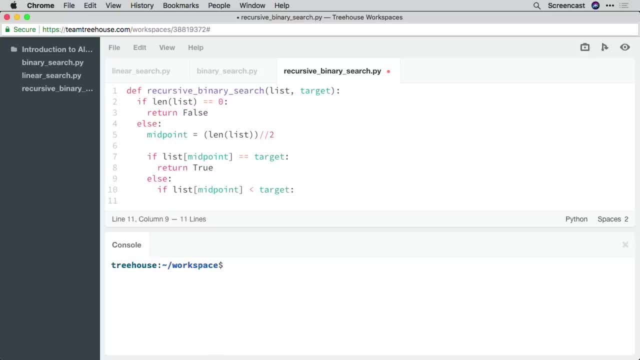 at sorting a list and open the door to an entirely new category of algorithms. we're going to implement our sorting algorithm on two different data structures and explore how the implementation of one algorithm can differ based on the data structure being used. we'll also look at 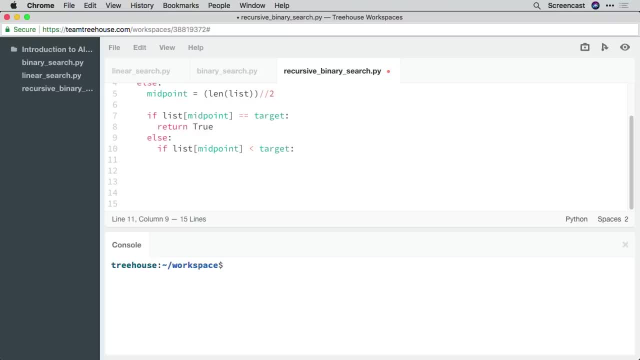 how the choice of data structure potentially influences the runtime of the algorithm. in learning about sorting, we're also going to encounter another general concept of algorithmic thinking called divide and conquer. along with recursion, divide and conquer will be a fundamental tool that we will use to solve complex 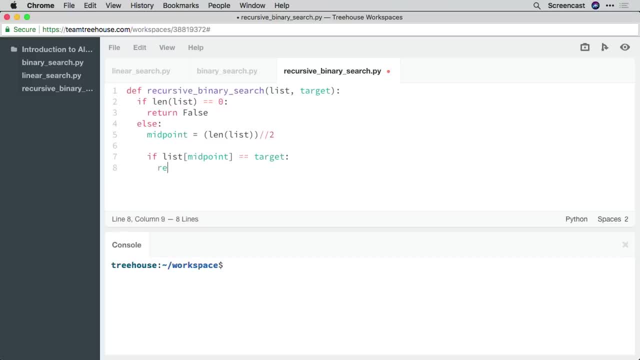 is the same as the target, then we'll go ahead and return. true, So far, this is more or less the same for the value that we're returning. Let me actually get rid of all that, Okay, Alright? So if this isn't the case, 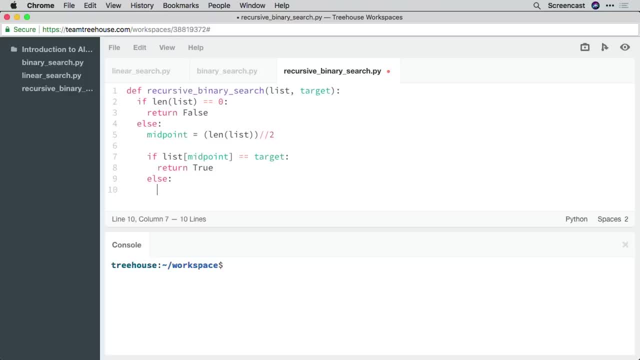 let's implement an else clause Now. here we have two situations. so, first, if the value at the midpoint is less than the target. so if value at midpoint is less than the target, then we're going to do something new, we're going to call this function. 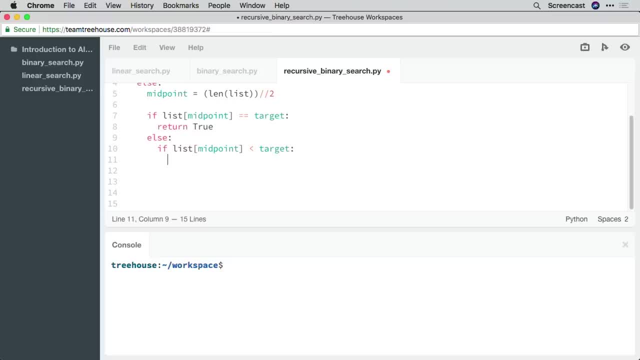 again This recursive binary search function that we're in the process of defining. we're going to call that again and we're going to give it the portion of the list that we want to focus on. In the previous version of binary search, we moved the first. 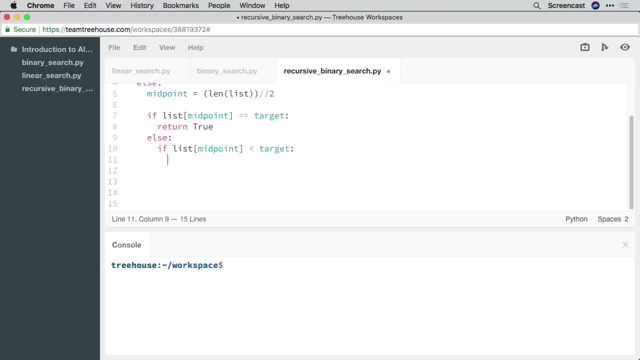 value, to point to the value after the midpoint. Now here we're going to specify the same target as the search target and when this function call is done, we'll return the value. So we'll say: return, the return is important, then we'll call this. 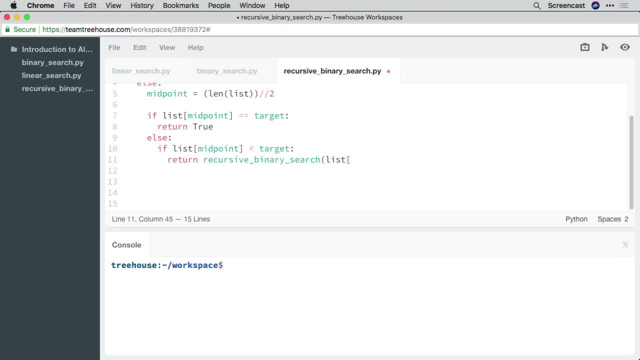 function, again recursive binary search, and this function takes a list, and here we're going to call it midpoint plus one, and then we'll go all the way to the end, and this is a python syntactic, sugar, so to speak, If I don't specify an. 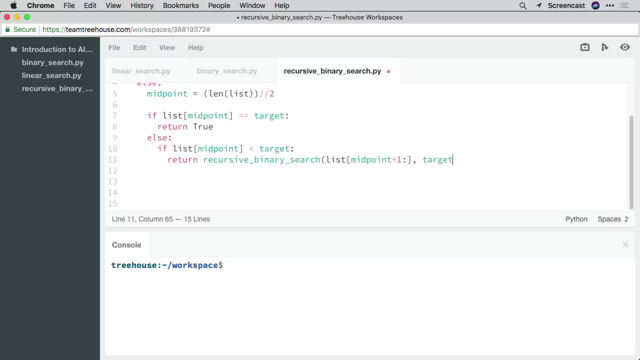 end index. python knows to just go all the way to the end. Alright, so this is our new list that we're working with, and we need a target. we'll just pass it through. The value at the midpoint is greater than the target, which means we only care. 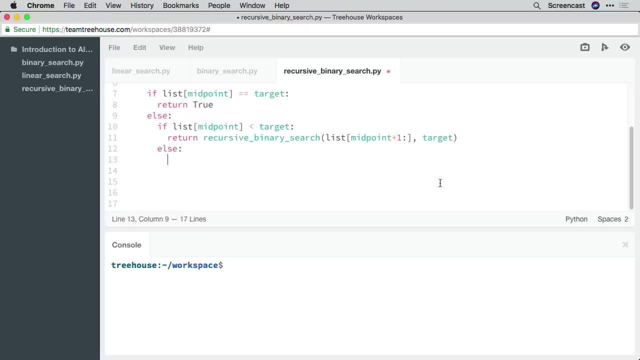 about the values in the list from the start, going up to the midpoint. Now, in this case as well, we're going to call the binary search function again and specify a new list to work with. This time, the list is going to start at the beginning. 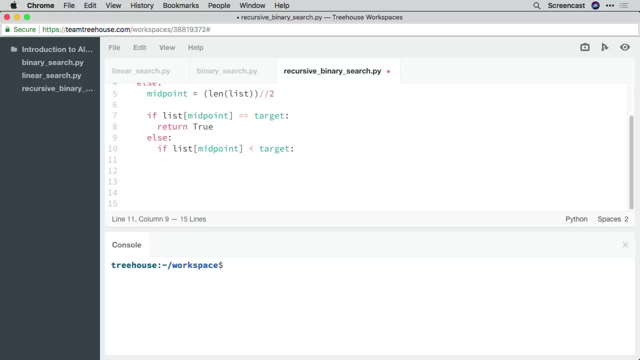 problems all in due time. in the next video, let's talk about arrays. a common data structure built into nearly every programming language is the array. arrays are a fundamental data structure and can be used to represent a collection of values, but it is much more than that: arrays are also. 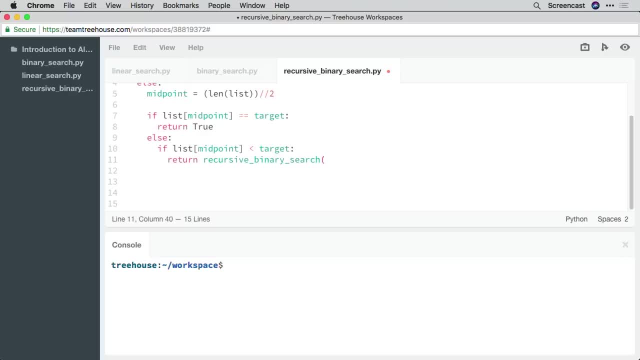 used as building blocks to create even more custom data types and structures. in fact, in most programming languages, text is represented using the string type and, under the hood, strings are just a bunch of characters stored in a particular order in an array. before we go further and dig into arrays, 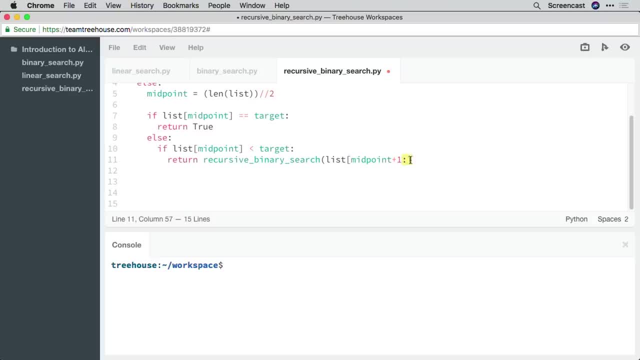 what exactly is a data structure? a data structure is a way of storing data when programming. it's not just a collection of values and the format they're stored in, but the relationship between the values in the collection, as well as the operations applied on the data stored in the structure. 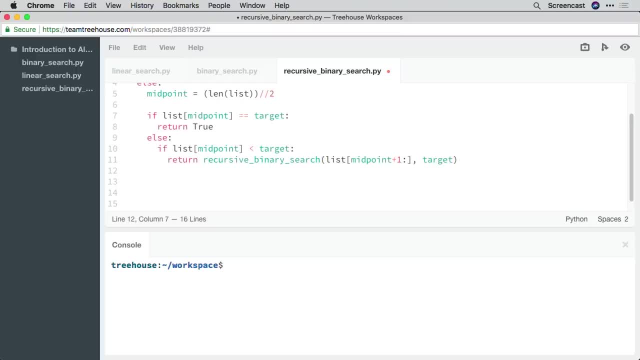 an array is one of very many data structures. in general, an array is a data structure that stores a collection of values, where each value is referenced using an index or a key. a common analogy for thinking about arrays is as a set of train cars: each car. 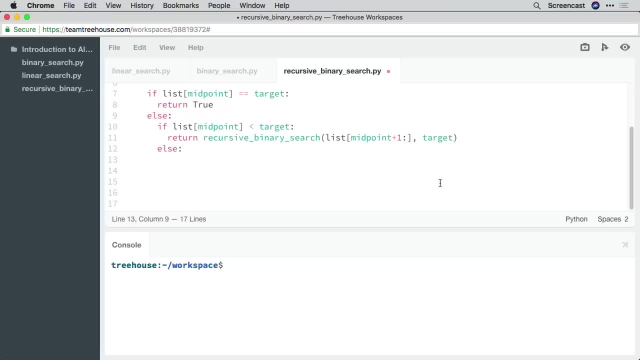 has a number and these cars are ordered sequentially. inside each car, the array- or the train in this analogy- stores some data. while this is the general representation of an array, it can differ slightly from one language to another, but for the most part, all these fundamentals remain the same. 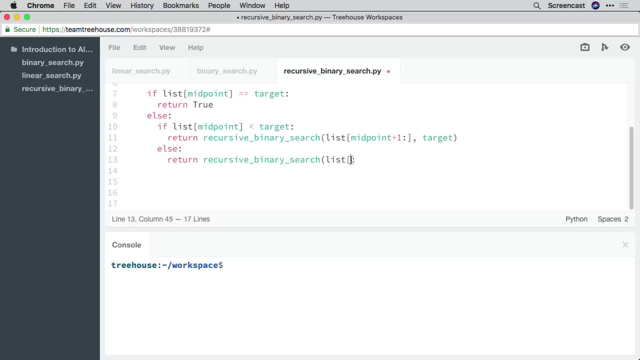 in a language like Swift or Java. arrays are homogenous containers, which means they can only contain values of the same type. if you use an array to store integers in Java, it can only store integers in other languages. arrays are heterogeneous structures that can store any kind of value. 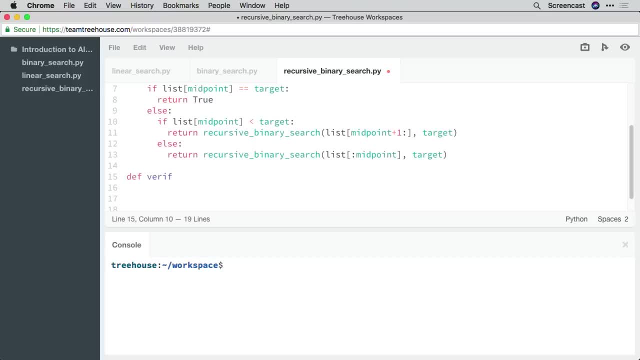 in Python, for example, you can mix numbers and text with no issues. now, regardless of this nuance, the fundamental concept of an array is the index. this index value is used for every operation on the array, from accessing values to inserting, updating and deleting. in Python, the language we're, 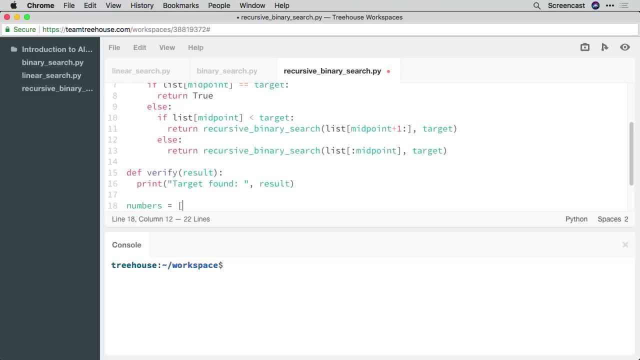 going to be using for this course. it's a tiny bit confusing. the type that we generally refer to as an array in most languages is best represented by the list type in Python. Python does have a type called array as well, but it's something different, so we're not going to use it. 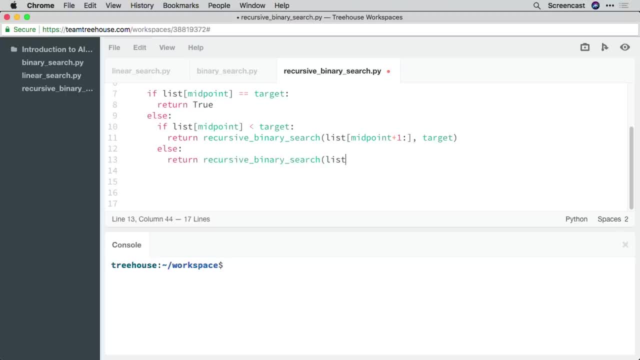 and then go all the way up to the midpoint. So it looks the same. so if we just put a colon here without a start index, python knows to start at the beginning and we're going to go all the way up to the midpoint. The target here. 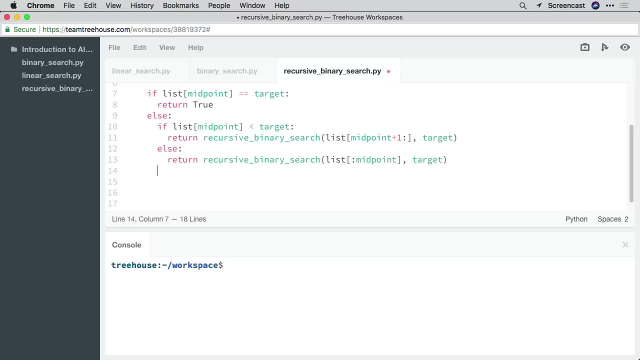 is the same and this is our new binary search function. So let's see if this works Actually. yes, Down here we'll make some space and we'll define a verify function. We're not going to copy paste the previous one because we're not returning. 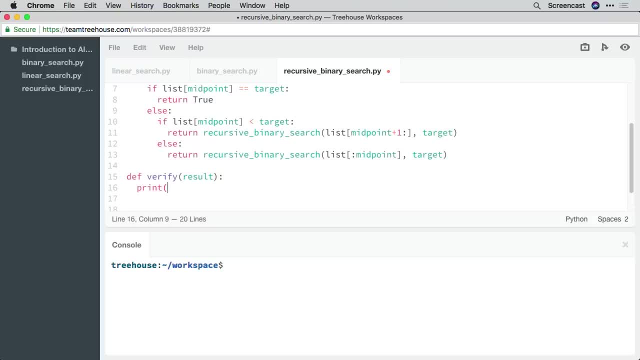 it. So we'll verify the result that we pass in and we'll say print target found and this is just going to say true or false, whether we found it. Okay, so, like before, we need a numbers list and we'll do something. 1, 2,, 3, 4. 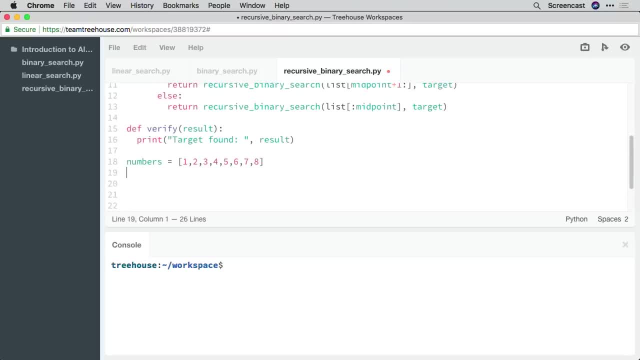 all the way up to 8.. Okay, and now let's test this out. So we'll call our recursive binary search function and we'll pass in the numbers list, and the target here is 12.. We're going to verify this. verify the result. 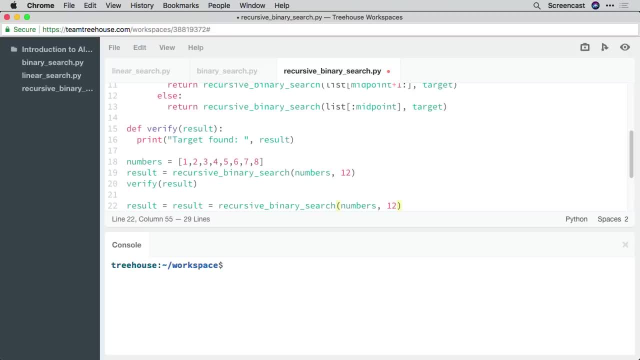 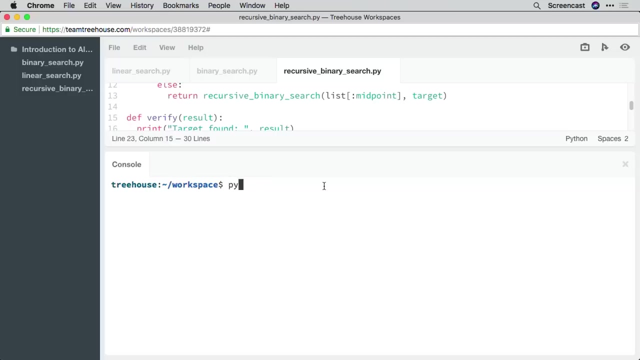 make sure it works and then we'll call it again, this time making sure that we give it a target that is actually in the list. so here we'll say 6 and we'll verify this again. Make sure you hit command s to save and then 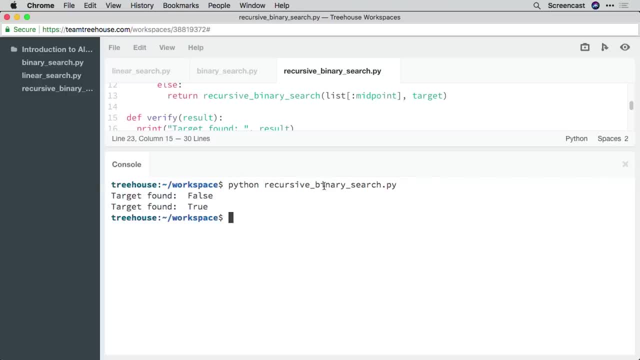 in the console dot pi. Run it and you'll see that we've verified that search works. While we can't verify the index position of the target value, which is a modification to how our algorithm works, we can guarantee, by running across all valid inputs, that search. 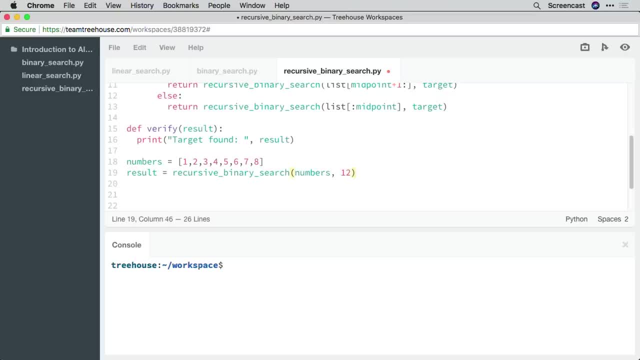 while Python calls it a list. when we use a list in this course, we'll be talking about concepts that apply to arrays as well in other languages, so definitely don't skip any of this. there's one more thing: in computer science, a list is actually a different data structure than an array. 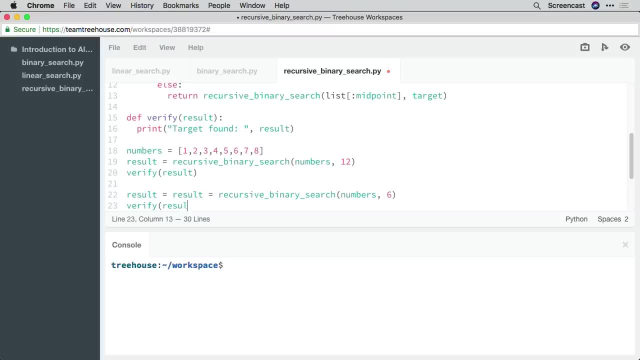 and in fact we're going to build a list later on in this course. generally, though, this structure is called a linked list as opposed to just list, so hopefully the terminology isn't too confusing. to properly understand how arrays work, let's take a peek at how arrays are stored. 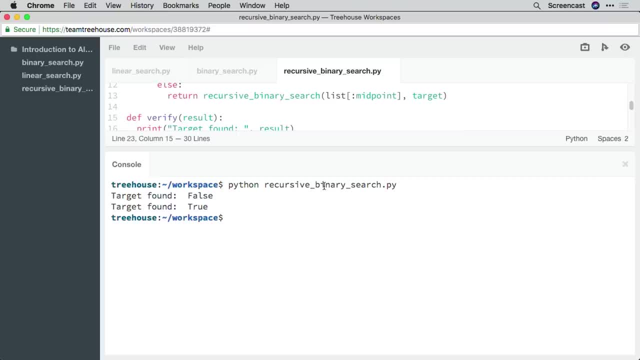 under the hood. an array is a contiguous data structure. this means that the array is stored in blocks of memory that are right beside each other with no gaps. the advantage of doing this is that retrieving values is very easy in a non-contiguous data structure we're going to build. 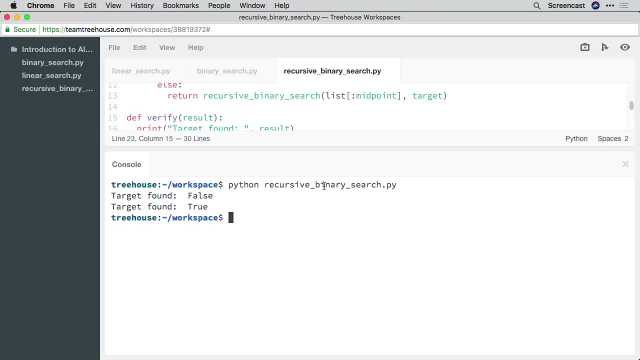 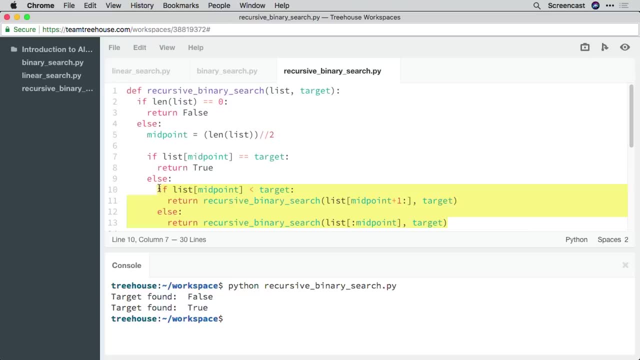 one soon. the structure stores a value as well as a reference to where the next value is. to retrieve that next value, the language has to follow that reference, also called a pointer to the next block of memory. this adds some overhead which, as you will see, 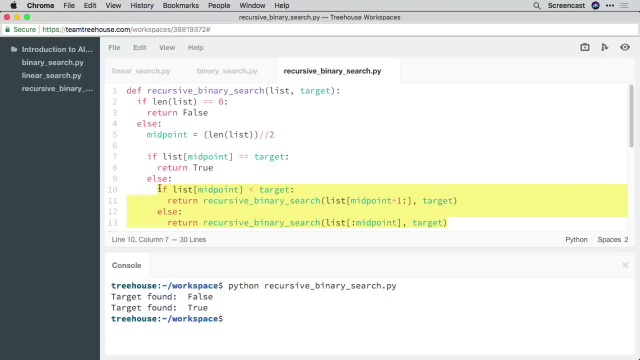 increases the runtime of common operations. a second ago I mentioned that, depending on the language, arrays can either be homogenous, containing the same type of value, or heterogeneous, where any kind of value can be mixed. this choice also affects the memory layout of the array. 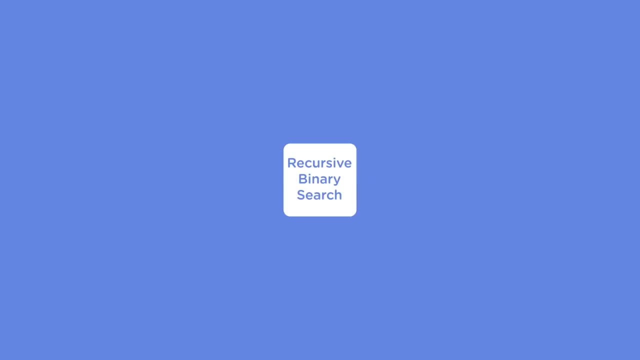 for example, in a language like C, Swift or Java, where arrays are homogenous. when an array is created, since the kind of value is known to the language compiler- and you can think of the compiler as the brains behind the language- it can choose a contiguous block of memory. 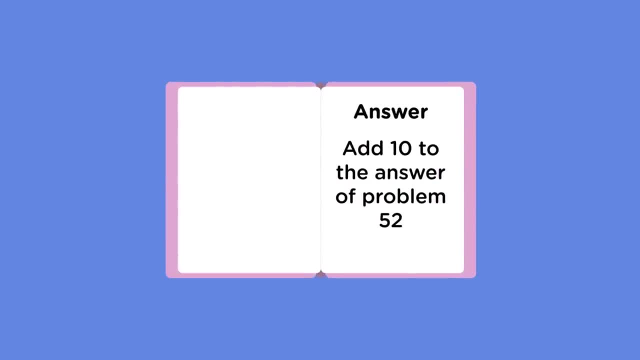 that fits the array size and values created. if the values were integers, assuming an integer took up space represented by one of these blocks, then for a five item array, the compiler can allocate five blocks of equally sized memory in Python. however, this is not the case. we can put any value in a Python list. 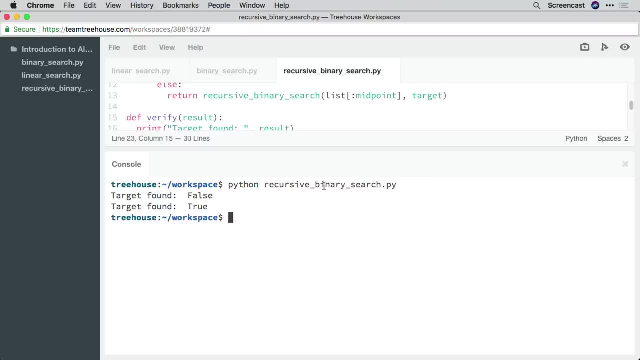 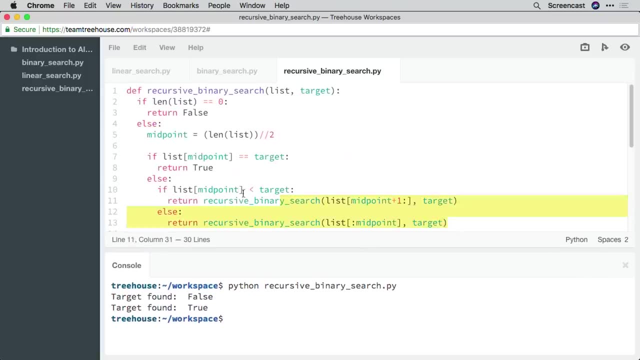 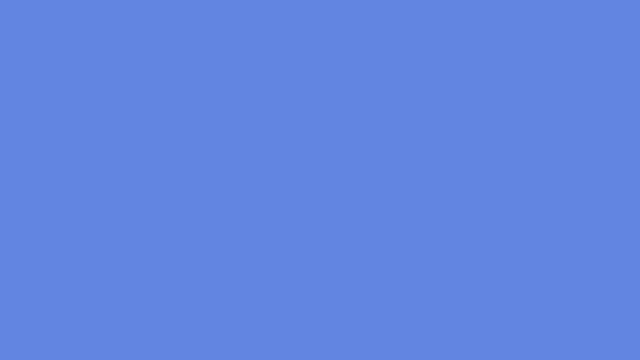 works as intended, So why write a different search algorithm here? a different version of binary search is a recursive binary search. a recursive function is one that calls itself a binary search, and this is a recursive binary search, a recursive binary search and that calls itself This is: 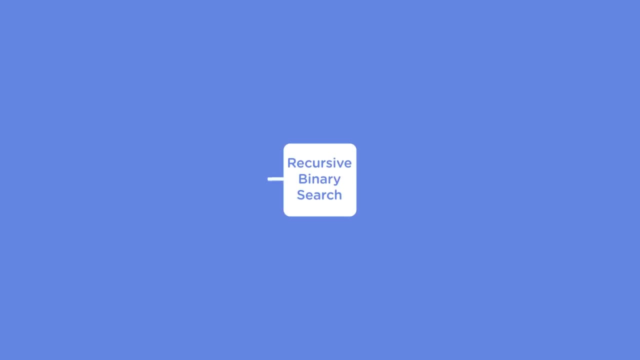 hard for people to grasp sometimes because there's few easy analogies that make sense. but you can think of it in sort of this way. So let's say, you have this book that contains answers to multiplication problems. You're working on a problem and you want. 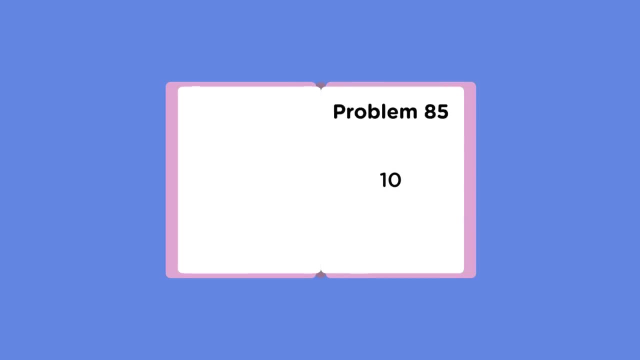 to add 12 to the answer for problem 85. Well, then you go and look up the answer to problem 85 and finally, instead of redirecting you somewhere else, that answer says 10.. So you take that 10 and then you go back to problem 52 because, remember, the answer for problem 52 was to add 12 to the answer for problem 85. So you take that 10 and then you now have the answer to problem 85. so you add 10 to 12 to get 22.. 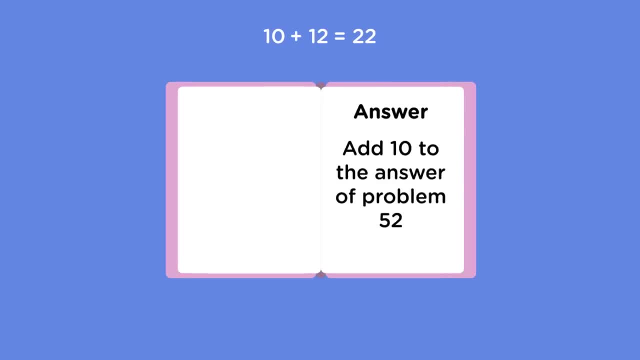 Then you go back to your original problem where it's said to add 10 to the answer for problem 52. so you add 10 to 22 and you get 32 to end up with your final answer. So that's a weird way of doing it, but this is an example of recursion. 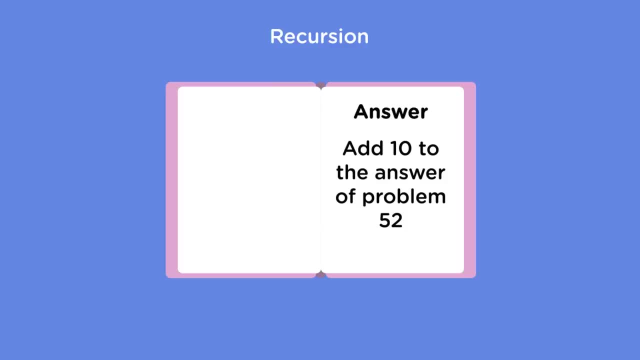 The solution to your first lookup in the book was the value obtained by another lookup in the same book, which was followed by yet another lookup in the same book. The book told you to check the book until you arrived at some base value. Okay, Our function works in a similar manner. 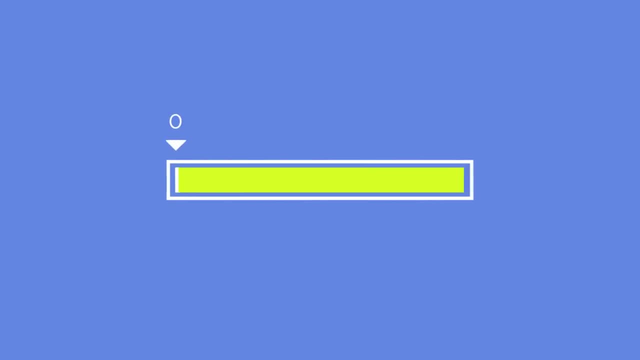 So let's visualize this with an example of a list. Like before, we have a 9 element list here with values 0 through 8.. The target we're searching for is the value 8.. We'll check if the list is empty by calling len on it. 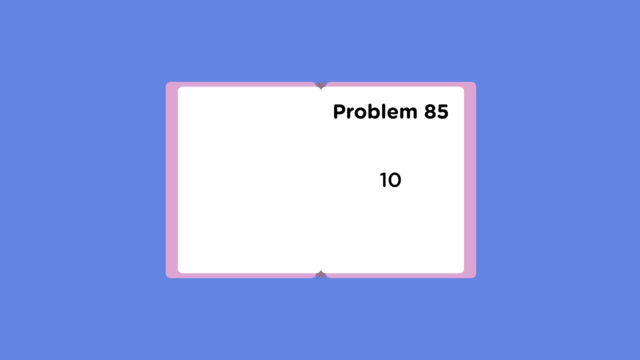 there's no restriction. what works is a combination of contiguous memory and the pointers or references I mentioned earlier. when we create a list in Python, there is no information about what will go into that array, which makes it hard to allocate contiguous memory of the same size. there are several advantages. 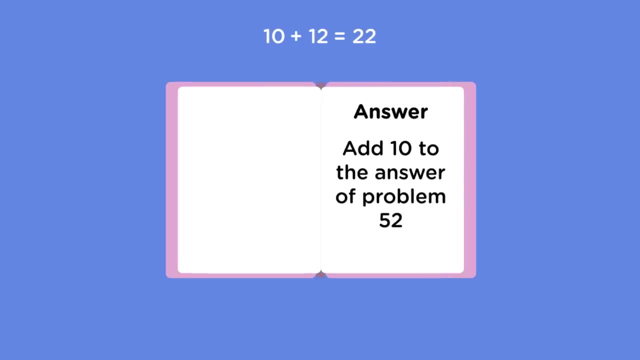 to having contiguous memory. since the values are stored beside each other, accessing the values happens in almost constant time. so this is a characteristic we want to preserve- is by allocating contiguous memory and storing in it not the value we want to store, but a reference or a pointer. 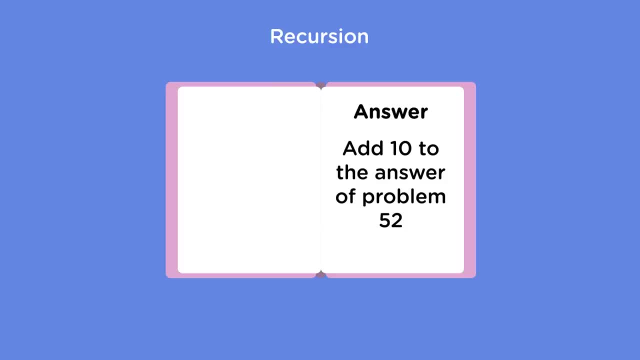 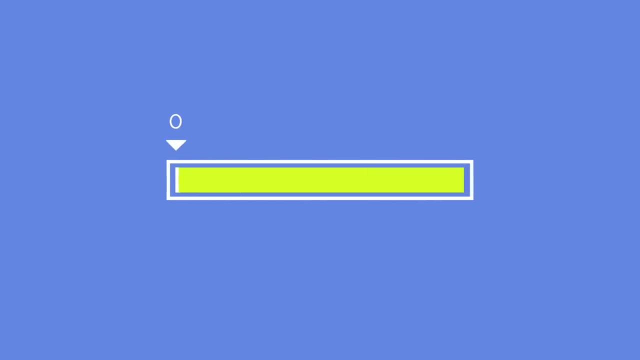 to the value that's stored somewhere else in memory. by doing this, it can allocate equally sized contiguous memory, since, regardless of the value size, the size of the pointer to that value is always going to be equal. this incurs an additional cost, in that when a value is accessed, 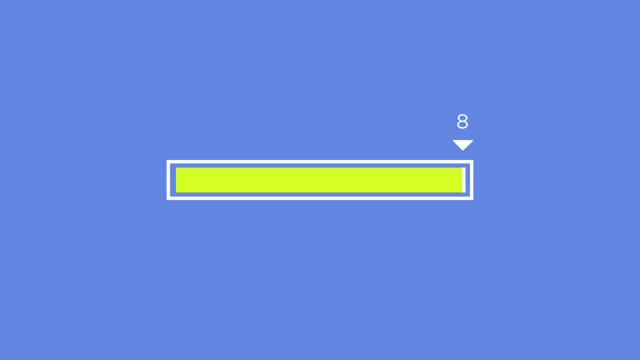 we need to follow the pointer to the block of memory where the value is actually stored, but Python has ways of dealing with these costs that are outside the scope of this course. now that we know how an array stores its values, let's look at common operations that we execute on an array. 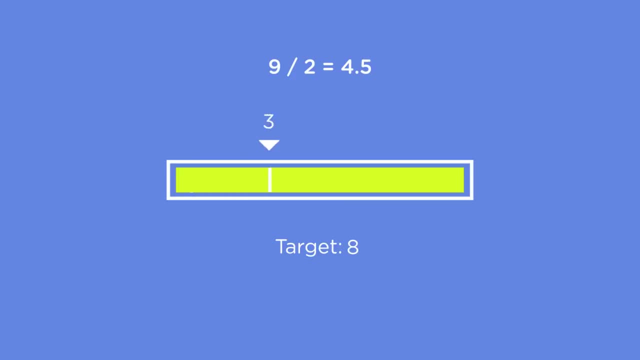 regardless of the kind of data structure you work with, all data structures are expected to carry out four kinds of operations at minimum. we need to be able to access and read values stored in the structure. we need to be able to search for an arbitrary value. we also need to be able to: 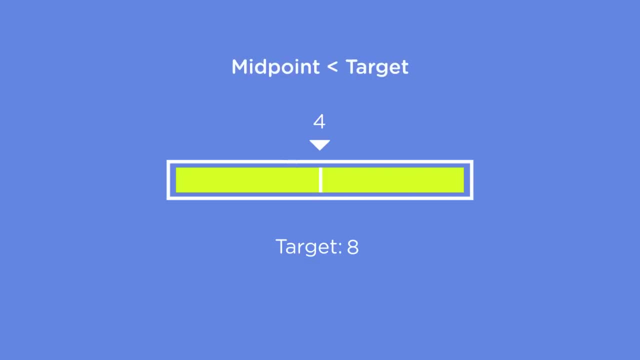 insert a value at any point into the structure and, finally, we need to be able to delete structures. let's look at how these operations are implemented on the array structure in some detail, starting with access. elements in an array are identified using a value known as an index. 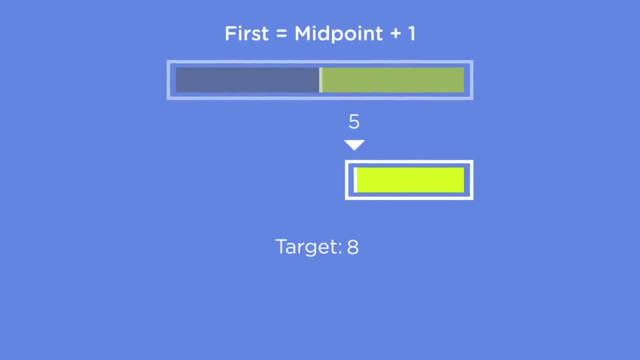 and we use this index to access and read the value. most programming languages follow a zero-based numbering system when it comes to arrays, and all this means is that the first index value is equal to zero, not one. generally speaking, when an array is declared a base amount of contiguous memory, 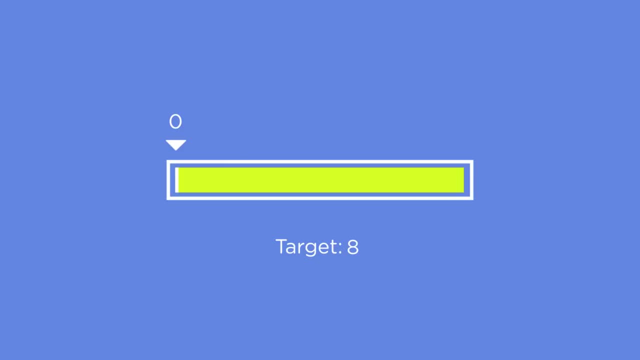 This list is not empty, so we go to the else clause. Next we calculate the midpoint: 9 divided by 2 is 4.5, rounded down is 4. so our first midpoint value is 4.. We'll perform our first check. 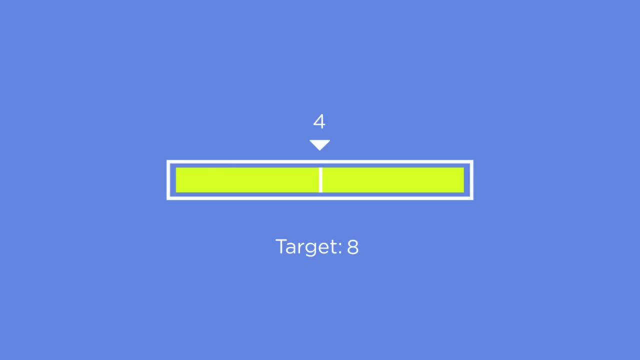 Is the value at the midpoint equal to the target? Not true, So we go to our else clause. We'll perform another check here. Is the value at the midpoint less than the target? Now, in our case, this is true. Earlier, when we evaluated this condition, we simply changed the value of first. 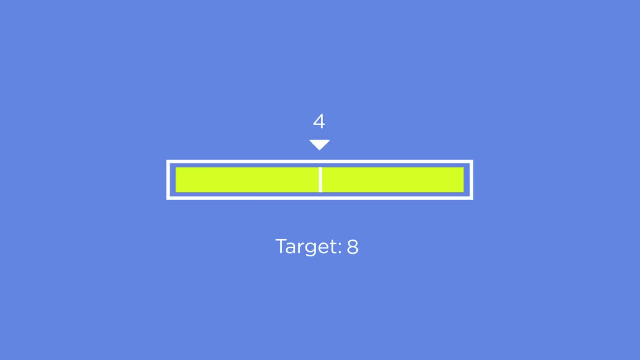 Here we're going to call the recursive binary search function again and give it a new list to work with. The list starts at midpoint plus 1. So at index position 5, all the way to the end. Notice that this call to recursive binary search, inside of recursive binary search, includes a return statement. 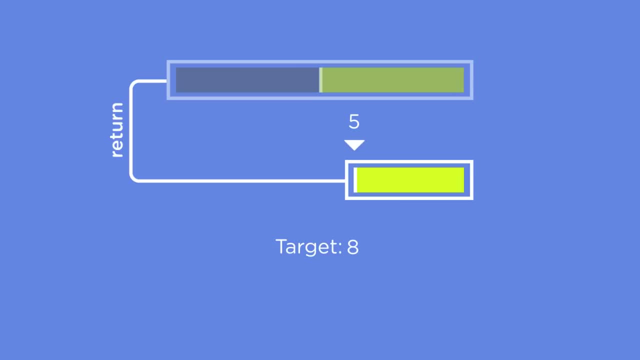 This is important and we'll come back to that in a second. So now we're back at the top of a new call to recursive binary search with, effectively, a new list, Although technically just a sub-list of the first one. The list here contains the numbers 6,, 7, 8.. 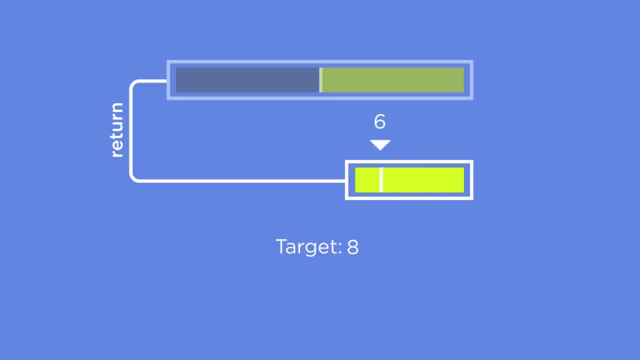 Starting with the first check, the list is not empty, so we move to the else. The midpoint, in this case length of the list, 3 divided by 2, rounded down, is 1.. Is the value at the midpoint equal to the target? Well, the value at that position is 7, so no. 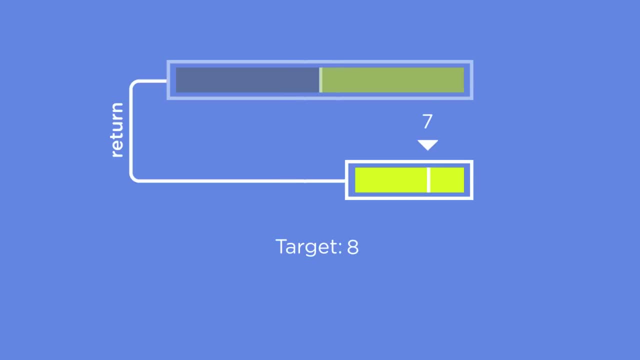 In the else we perform, the first check Is the value at the midpoint less than the target Indeed it is So we call recursive binary search again and provide it a new list. This list starts at midpoint plus 1 and goes to the end. 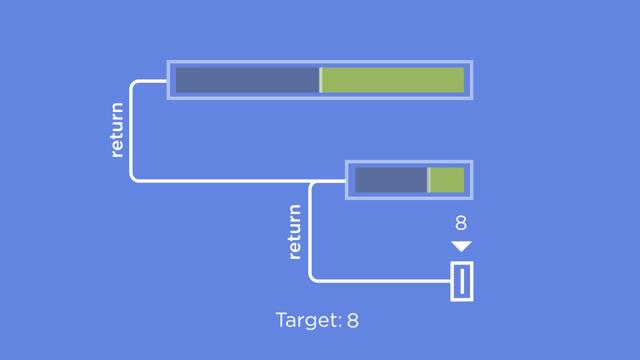 So in this case that's a single element list. Since this is a new call to recursive binary search, we start back up at the top. Is the list empty? No, The midpoint is 0.. Is the value at the midpoint the same as the target? 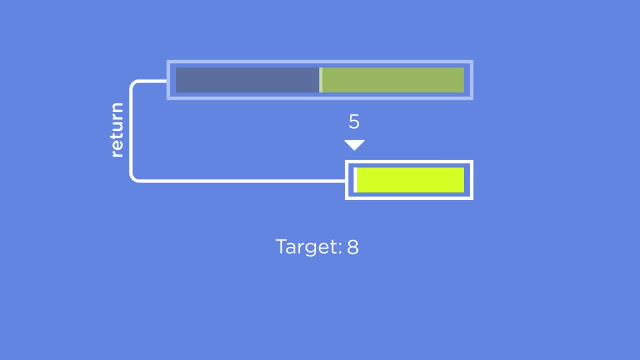 is allocated as the array storage. computers refer to memory through the use of an address, but instead of keeping a reference to all the memory allocated for an array, the array only has to store the address of the first location because the memory is contiguous using the base address. 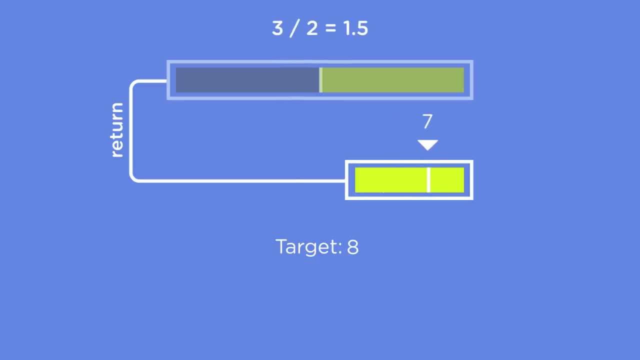 the array can calculate the address of any value by using the index position of that value as an offset. if you want to be more specific, think of it this way: let's say we want to create an array of integers, and then each integer takes up a certain amount. 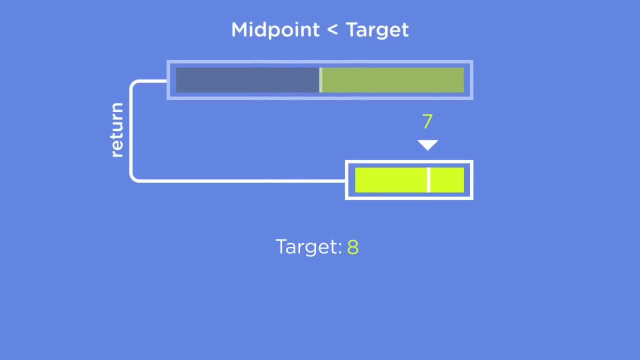 of space in memory that we'll call m. let's also assume that we know how many elements we're going to create, so the size of the array is some number of elements. we'll call n. the total amount of space that we need to allocate is n times the space per item, m. 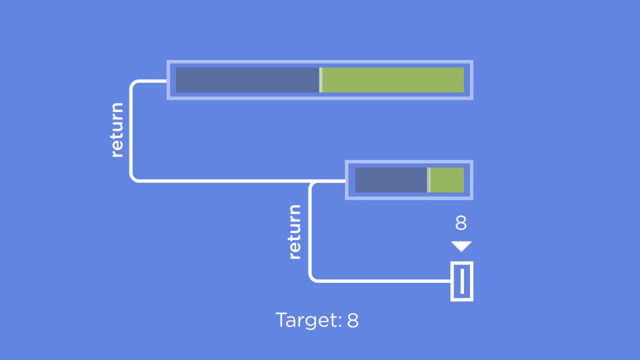 if the array keeps track of the location in memory where the first value is held, so let's label that m0- then it has all the information it needs to find any other element in the list. when accessing a value in an array, we use the index, so to get the first element in the list. 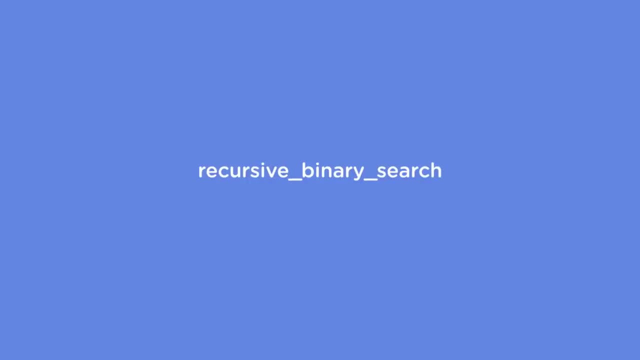 we use the zeroth index. to get the second, we use the index value 1, and so on. given that the array knows how much storage is needed for each element, it can get the address of any element by starting off with the address for the first element. 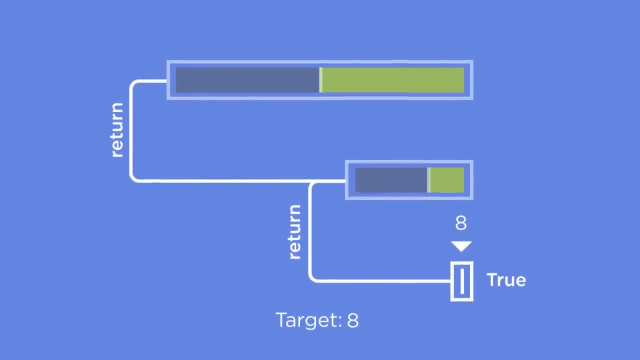 and adding to that the index value times the amount of storage per element. for example, to access the second value, we can start with m0 and to that add m times the index value 1, giving us m1 as the location in memory for the second address. 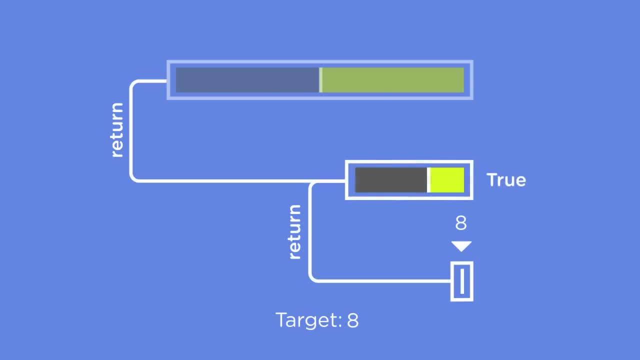 this is a very simplified model, but that's more or less how it works. this is only possible because we know that array memory is contiguous with no gaps. let's switch over to some code. as I mentioned earlier, we're going to be using python in this course. 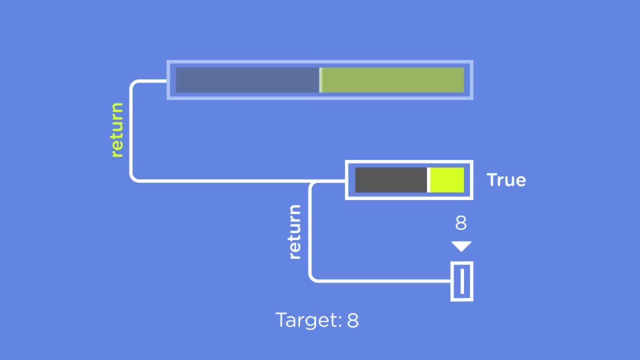 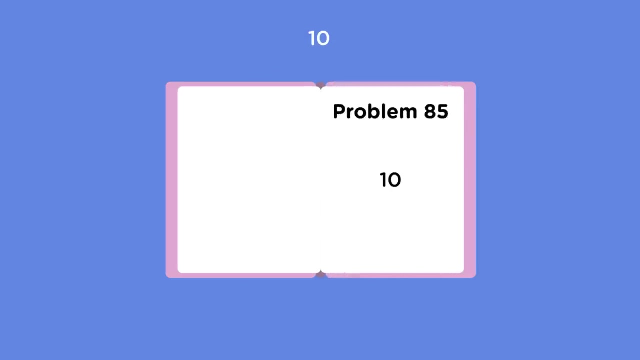 if you don't know how to code and are interested in this content, but know a language other than python, check the notes section of this video for more information. while the code will be in python, the concepts are universal and, more importantly, simple enough that you should have no issue. 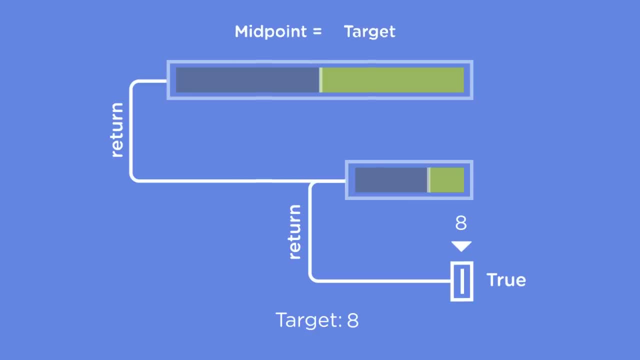 It is. So now we can return true. Remember, a minute ago I pointed out that when we call recursive binary search from inside the target, The function itself is preceded by a return statement. That plays a pretty important role here. So back to our visualization. 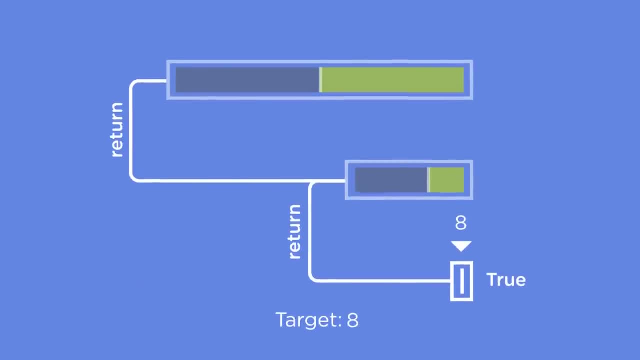 We start at the top and we call binary search with a new list, But because that's got a return statement before it. What we're saying is: hey, when you run binary search on this, Whatever value you get back, return it to the function that called you. 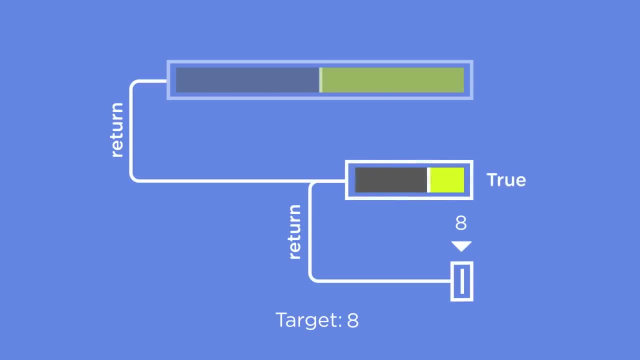 Then at the second level, we call binary search, again along with another return statement. Like with the first call, we're instructing the function to return a value back to the code that called it. At this level we find the target, so the function returns true back to the caller. 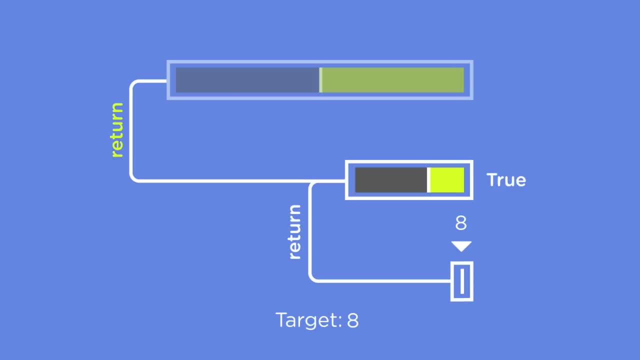 But since this inner function was also called by a function with instructions to return, It keeps returning that true value back up until we reach the very first function that called it. Going back to our book of answers, Recursive binary search instructs itself to keep working on the problem. 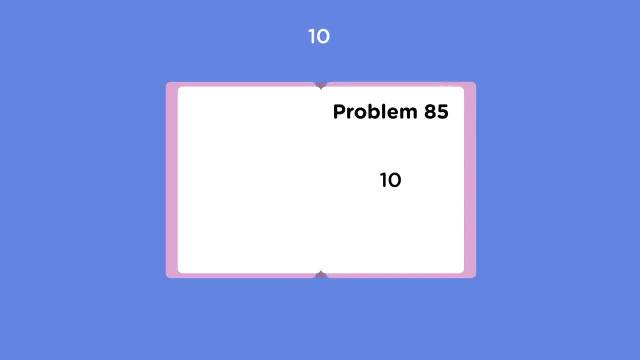 Until it has a concrete answer. Once it does, it works its way backwards, Giving the answer to every function that called it Until the original caller has an answer. Now, like I said at the beginning, this is pretty complicated, So you should not be concerned if this doesn't click. 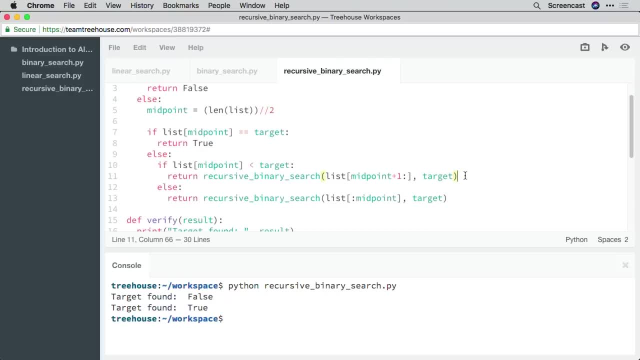 Honestly, this is not one thing that you're going to walk away with Knowing fully how to understand recursion after your first try. I'm really not lying when I say I have a pretty hard time with recursion. Now, before we move on, I do want to point out one thing. 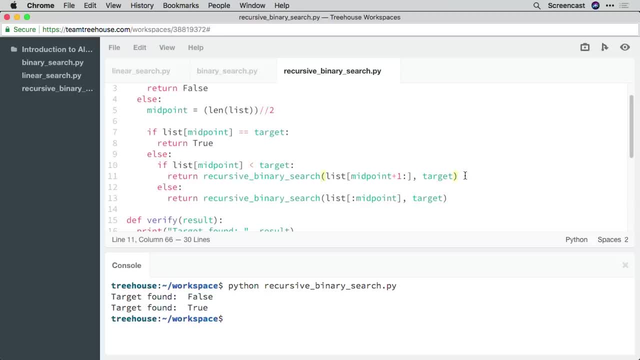 Even though the implementation of recursion is harder to understand, It is easier in this case to understand how we arrive at the logarithmic run time, Since we keep calling the function with smaller lists. Let's take a break here In the next video. 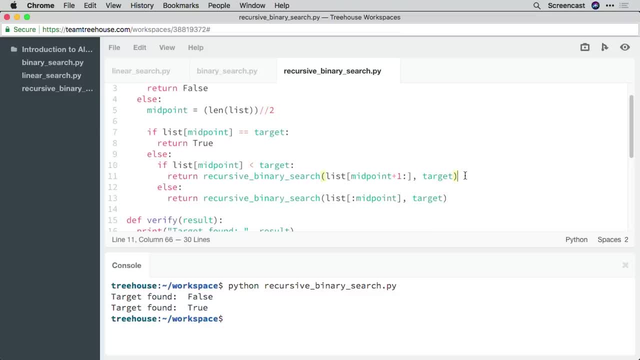 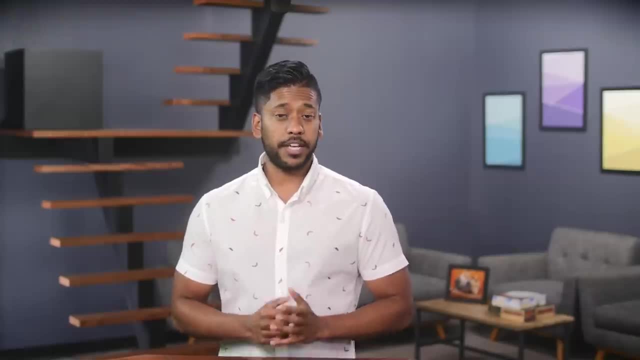 Let's talk a bit more about recursion and why it matters. In the last video, We wrote a version of binary search that uses a concept called recursion. Recursion might be a new concept for you, So let's formalize how we use it. 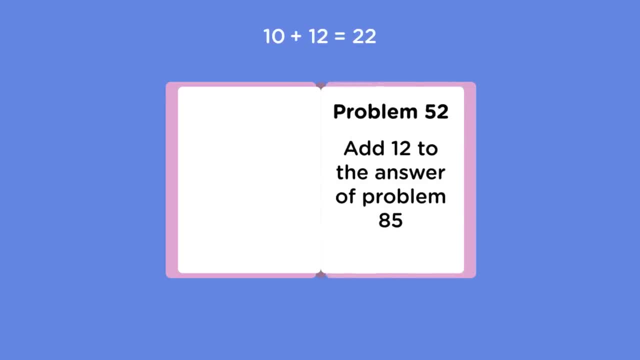 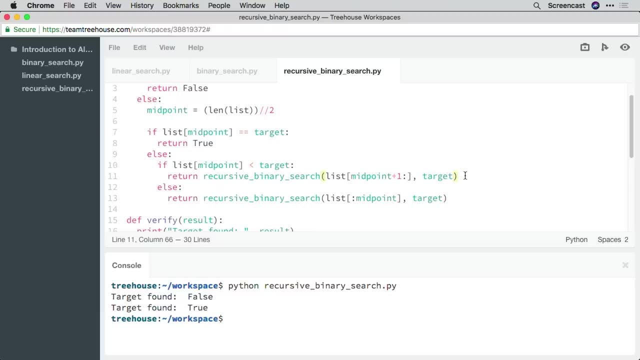 following along in your favorite programming language. now, to get started, click on the launch workspaces button on the video page that you're watching right now. this should spin up an instance of a treehouse workspace, an in-browser coding environment. your workspace should be empty and that's expected. 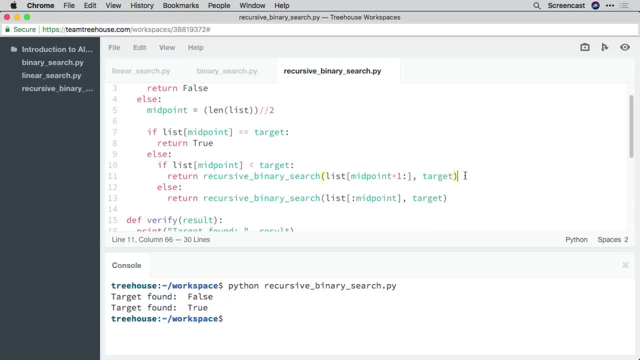 so let's add a new file in here. I'm going to go to file new file and we'll call this arrayspy. creating a list in python is quite simple, so we'll call this new underscore list. we use a set of square brackets around a set of values. 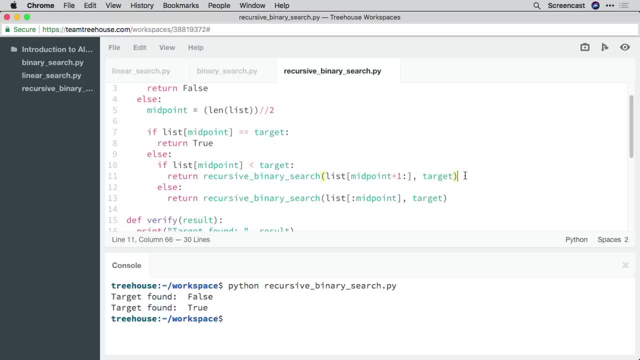 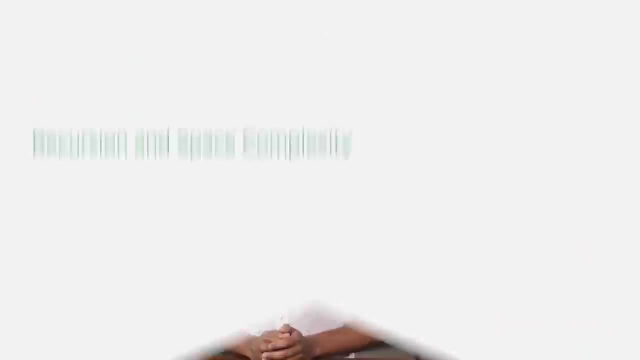 to create a list, so 1, and we comma separate them, so space 2 and space 3. this allocates a base amount of memory for the array to use. or when I say array, know that in python I mean a list. since this is python, the values aren't stored in memory. 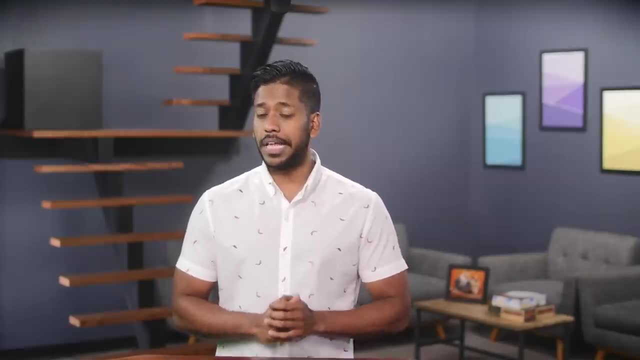 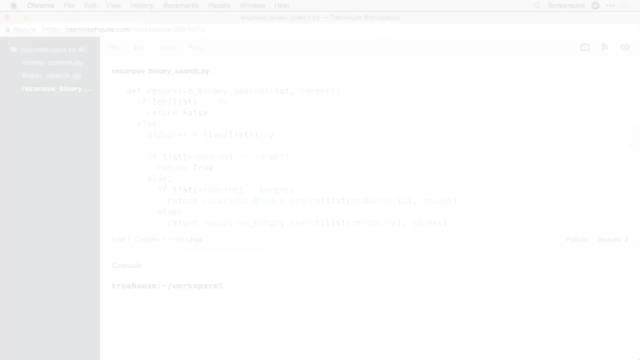 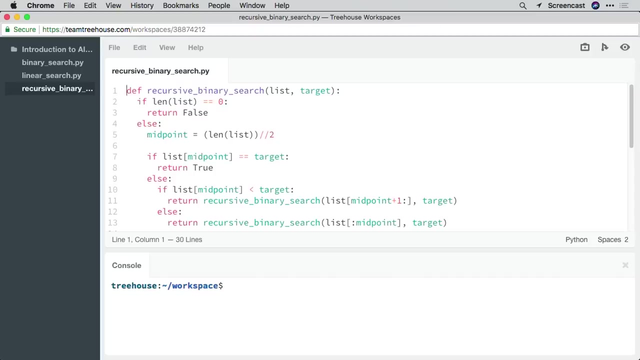 instead, the values 1,, 2 and 3 are stored elsewhere in memory and the array stores references to each of those objects. to access a value, we use a subscript along with an index value. so to get the first value, we use the index 0. 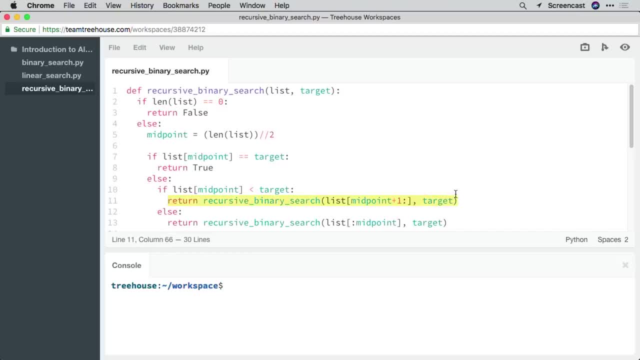 and if we were to assign this to another variable, we would say: result equal, new list. we write out new list, since this is the array that we're accessing the value from, and then a subscript notation, which is a square bracket, and then the index value, as we saw since the array. 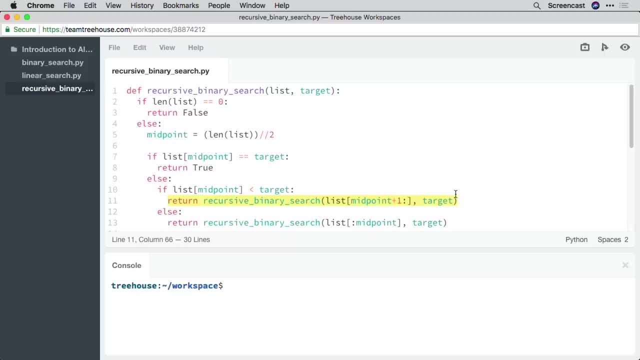 has a reference to the base location in memory, the position of any element can be determined pretty easily. we don't have to iterate over the entire list. all we need to do is a simple calculation of an offset from the base memory, since we're guaranteed that the memory 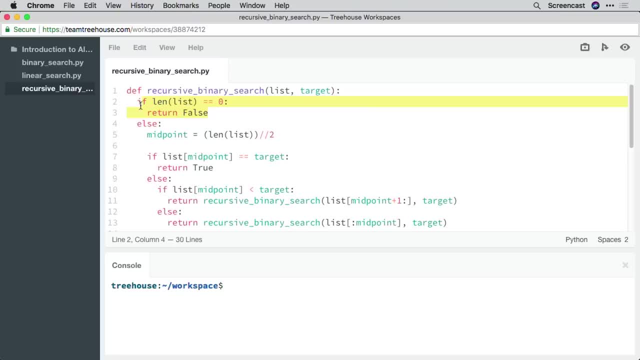 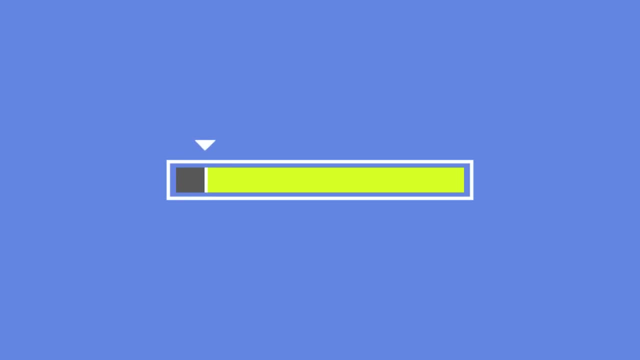 is contiguous. for this reason, access is a constant time operation on an array or a python list. this is also why an array crashes if you try to access a value using an index that is out of bounds of what the array stores. if you've used an array, 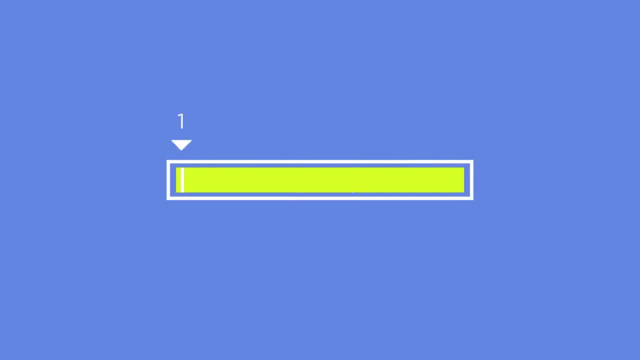 before. you've undoubtedly run into an error or a crash where you tried to access a value using an index that was larger than the number of elements in the array. since the array calculates the memory address on the fly, when you access a value with an out of bounds index. 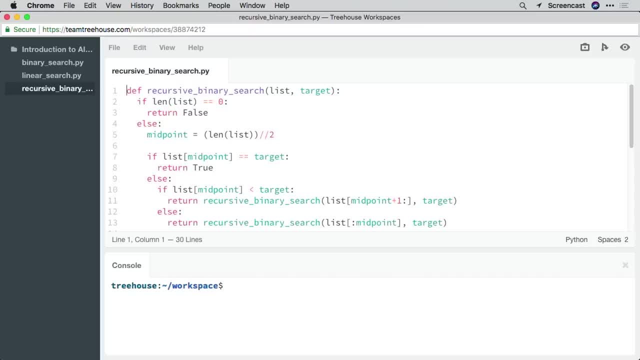 A recursive function is one that calls itself. In our example, the recursive binary search function Called itself inside the body of the function. When writing a recursive function, You always need a stopping condition And typically We start the body of the recursive function. 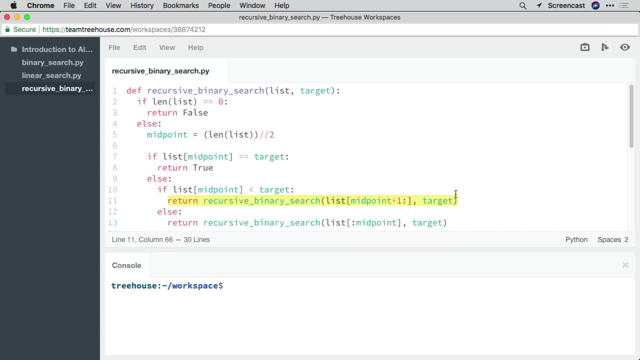 With this stopping condition. It's common to call this stopping condition the base case. In our recursive binary search function, We had two stopping conditions. The first was what the function should return If an empty list is passed in. It seems weird to evaluate an empty list. 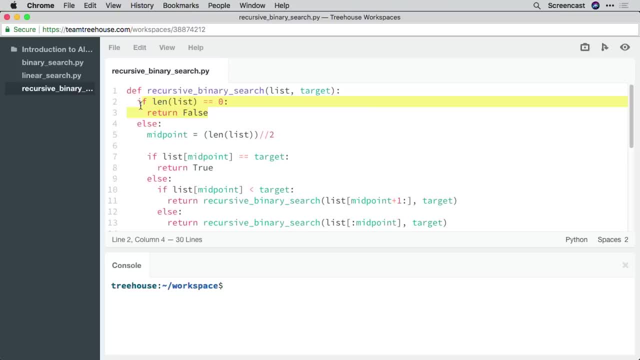 Because you wouldn't expect to run search on an empty list. But if you look at how our function works, Recursive binary search keeps calling itself And with each call to itself The size of the list is cut in half If we searched for a target. 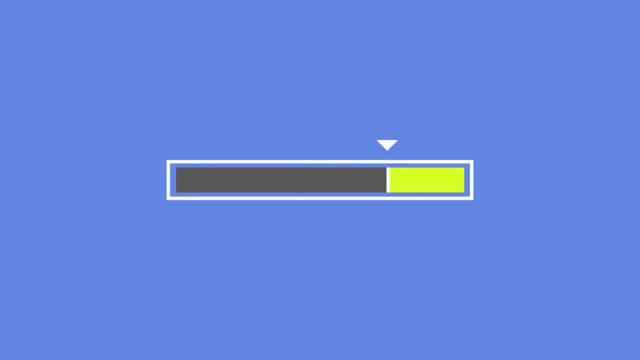 That didn't exist in the list, Then the function would keep having itself Until it got to an empty list. Consider a three element list With numbers one, two, three, Where we're searching for a target of four On the first pass. the midpoint is two. 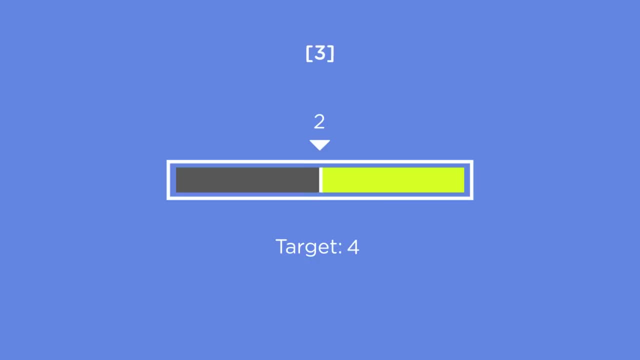 So the function would call itself with the list three On the next pass. the midpoint is zero And the target is still greater, So the function would call itself This time passing in an empty list, Because an index of zero plus one In a single element list doesn't exist. 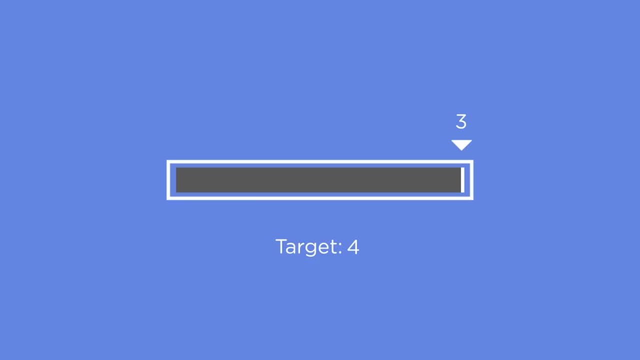 When we have an empty list. This means that after searching through the list, The value wasn't found. This is why we define an empty list As a stopping condition Or a base case that returns false If it's not an empty list. 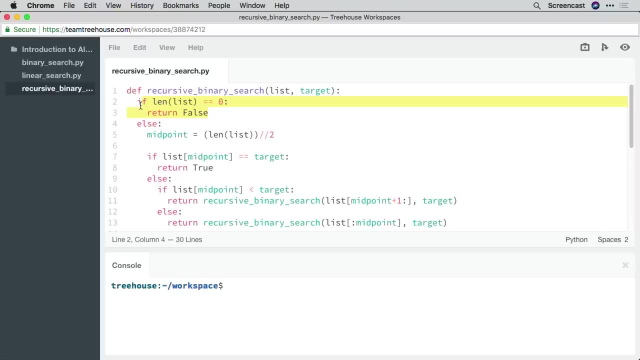 Then we have an entirely different set of instructions We want to execute. First, we obtain the midpoint of the list. Once we have the midpoint, We can introduce our next base case or stopping condition If the value at the midpoint is the same as the target. 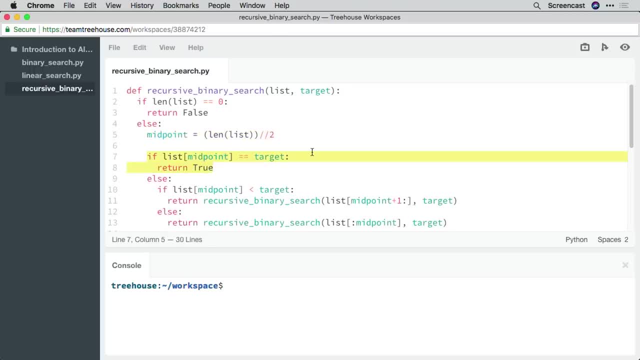 Then we return true. With these two stopping conditions, We've covered all possible paths of logic. Through the search algorithm, You can either find the value Or you don't. Once you have the base cases, The rest of the implementation of the recursive function. 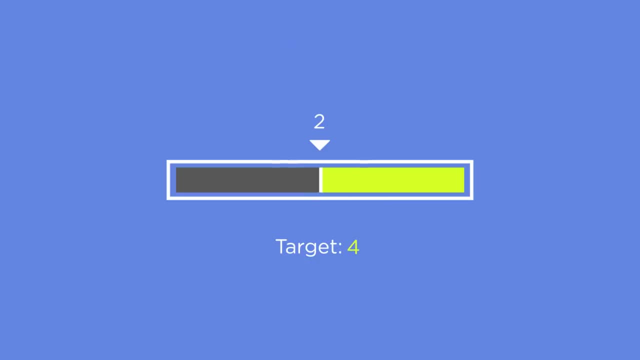 as it's called. the memory address returned is not one that's part of the array structure and therefore cannot be read by the array. now, in python this is represented by an index error and we can make this happen by using an index we know our array won't contain. 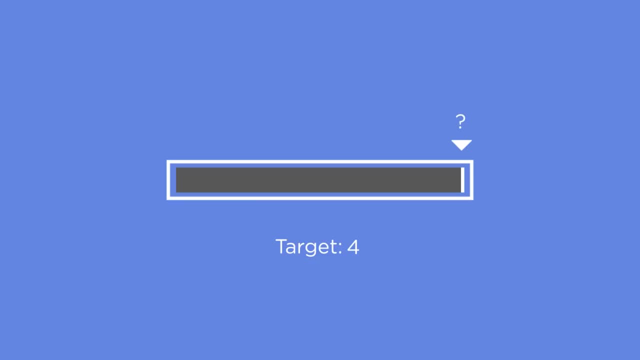 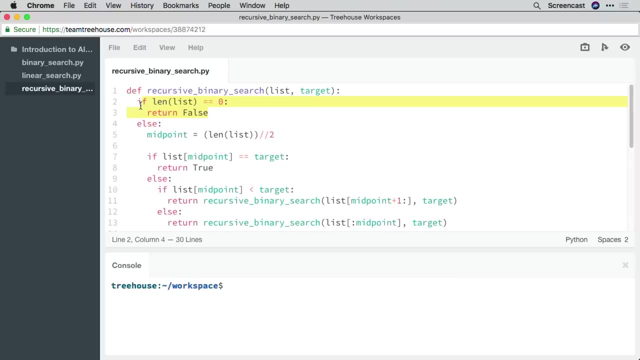 now I'm writing out my code here inside of a text editor which obviously doesn't run the code. so let's drag up this console area here and I'm going to write python to bring up the python interpreter and in here we can do the same thing. 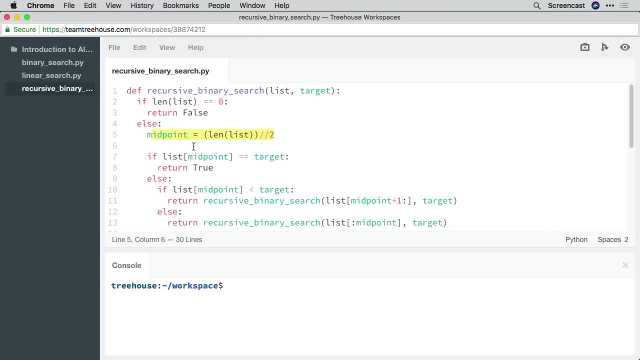 so I can say: new list equal 1 comma 2, comma 3, and now this is an interpreter, so it's actually going to evaluate our code alright, so now we have a new list. if I type out new list, it gets printed out into the console. 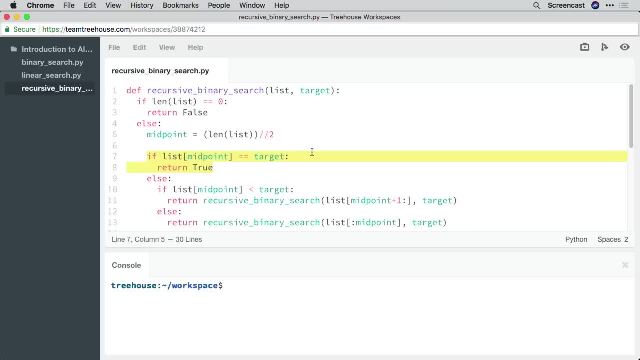 ok, I can also do new list, square bracket 0, and you'll see that I get the value 1, which is the value stored at the 0th index. now, to highlight that index error, we can do new list and inside the square brackets we can provide an index. 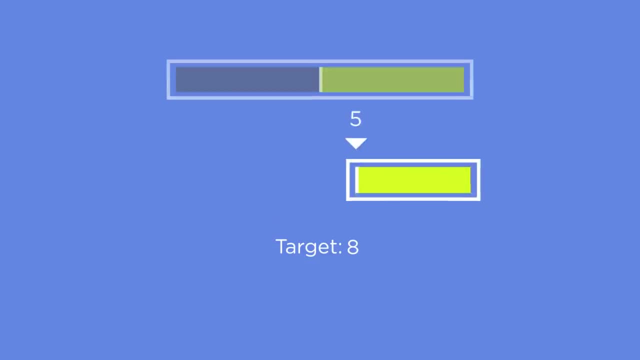 that we know our array doesn't contain. so here I'll say index 10 and if I hit enter you'll see it say index: error list, index out of range. and those are the basics of how we create and read values from an array. in the next video let's take a look. 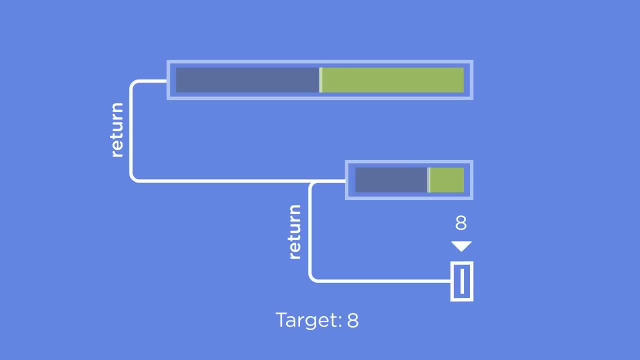 at searching. in the last video, we learned what happens under the hood when we create an array and read a value using an index. in this video, we're going to look at how the remaining data structure operations work on arrays. if you took the introduction to algorithms course, 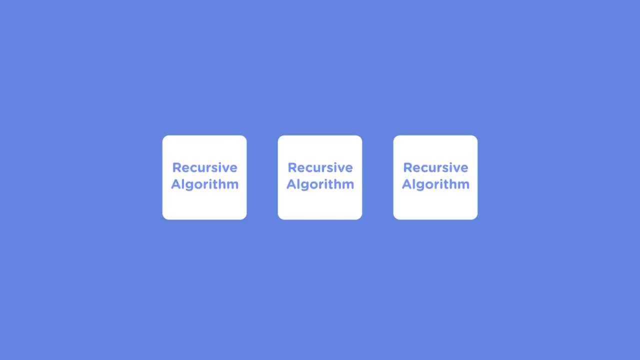 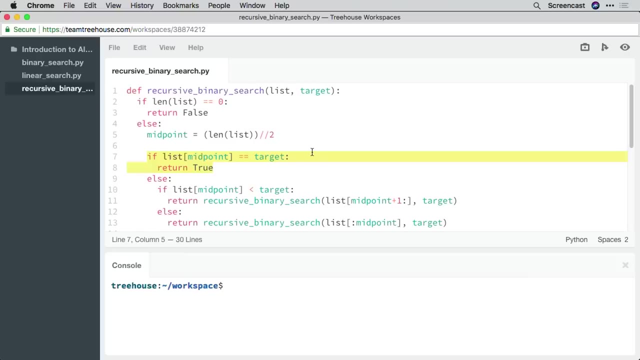 we spent time learning about two search algorithms: linear search and binary search. while arrays are really fast at accessing values, they're pretty bad at searching, taking an array as is. the best we can do is use linear search for a worst case, linear runtime. linear search works by accessing and reading each value. 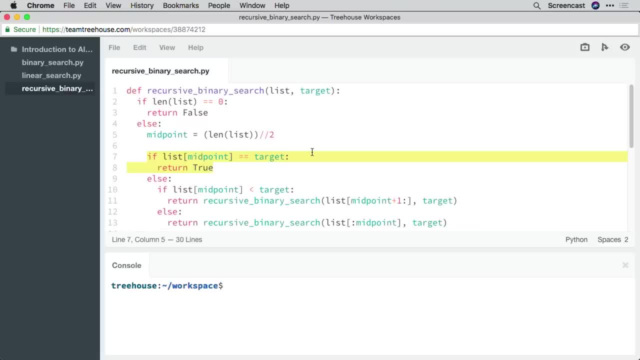 in the list until the element in concern is found. if the element we're looking for is at the end of the list, then every single element in the list will have been accessed and compared, even though accessing and comparing are constant time operations, having to do this for every element. 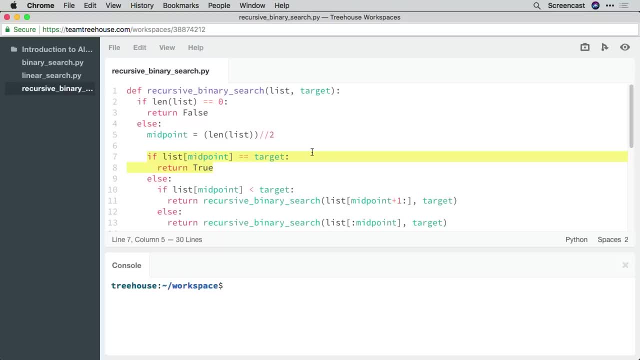 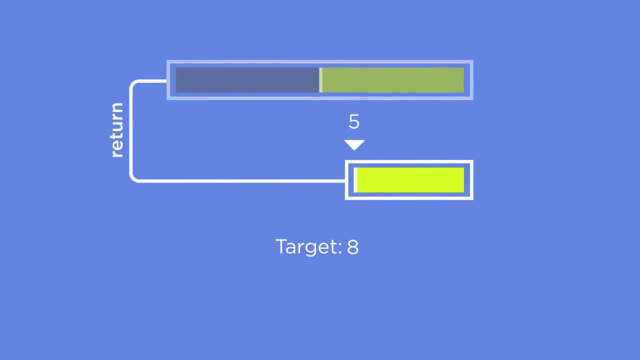 Is to call the function On smaller sub lists Until we hit one of these base cases. Going back to our visualization for a second, We see that recursive binary search Calls itself a first time, Which then calls itself again For the initial list we started with. 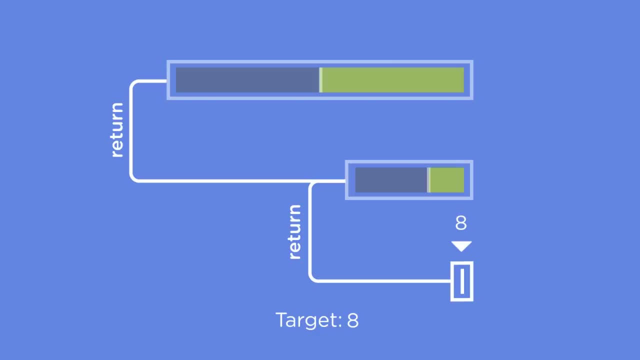 The function only calls itself a few times Before a stopping condition is reached. The number of times A recursive function calls itself Is called recursive depth. Now, the reason I bring all of this up Is because, If, after you start learning about algorithms, 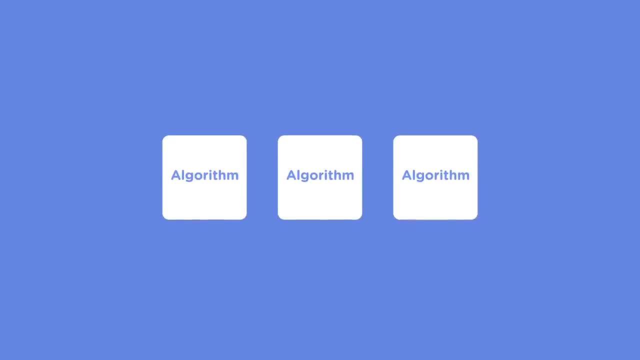 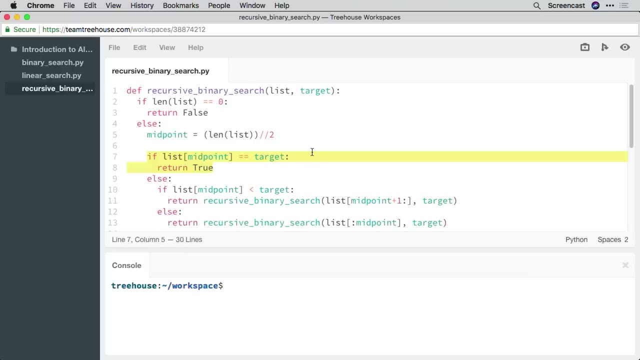 You decide you want to go off And do your own research, You may start to see a lot of algorithms Implemented using recursion, The way we implemented binary search The first time Is called an iterative solution. Now, when you see the word iterative, 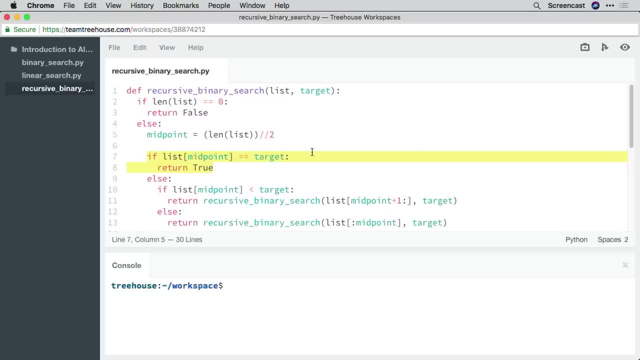 It generally means the solution Was implemented using a loop structure Of some kind. A recursive solution, on the other hand, Is one that involves A set of stopping conditions And a function that calls itself Computer scientists And computer science textbooks. 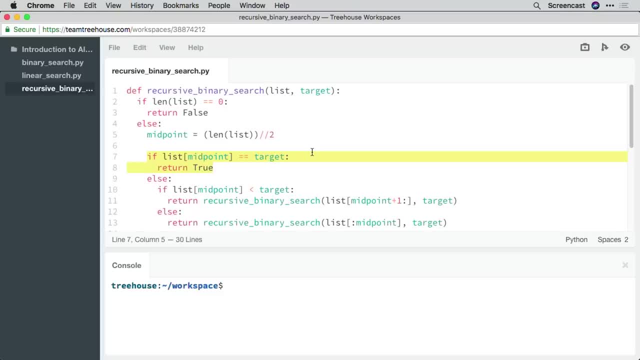 Particularly from back in the day Favor and are written in What are called functional languages. In functional languages We try to avoid changing data That is given to a function. In our first version of binary search We created first and last variables. 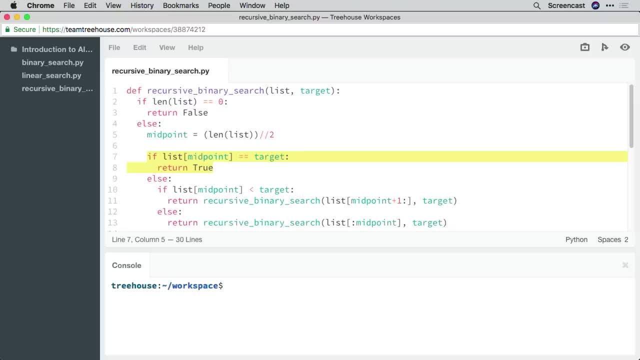 Using the list And then modified first and last As we needed to arrive at a solution. Functional languages don't like to do this Modification of variables And prefer a solution using recursion. Now, a language like python, Which is what we are using. 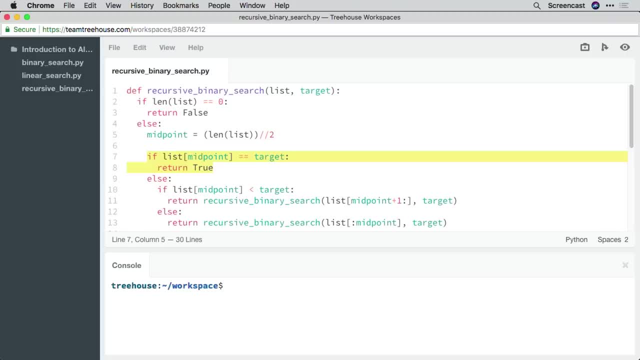 Is the opposite And doesn't like recursion. In fact, python has a maximum recursion depth, After which our function will halt execution. Python prefers an iterative solution. Now, I mention all of this For two reasons. If you decide That you want to learn, 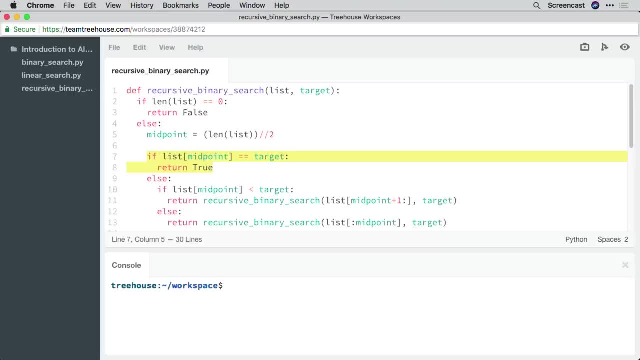 How to implement the algorithm In a language of your choice. Then you might see a recursive solution As the best implementation In that particular language. I'm an iOS developer, for example, And I work with a language called swift. Swift is different from python. 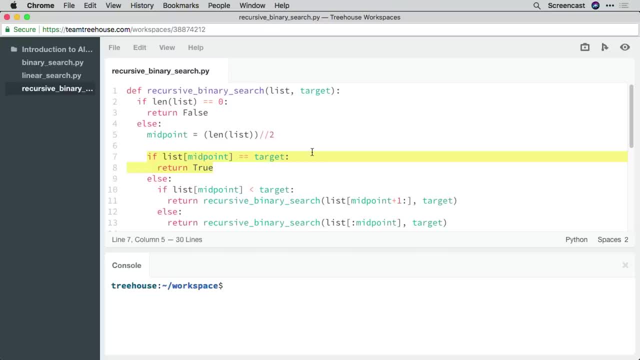 results in an overall linear time. let's look at how search works in code. in python we can search for an item in an array in one of two ways. we can use the in operator to check whether a list contains an item, so i can say if one. 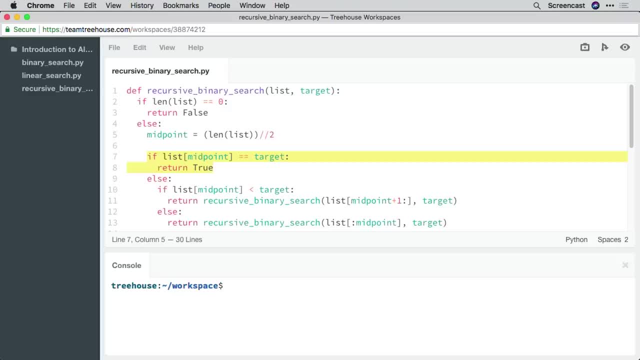 in new underscore list, then print true. the in operator actually calls a contains method that is defined on the list type which runs a linear search operation. in addition to this we can also use a for loop to iterate over the list manually and perform a comparison operation. so i can say: 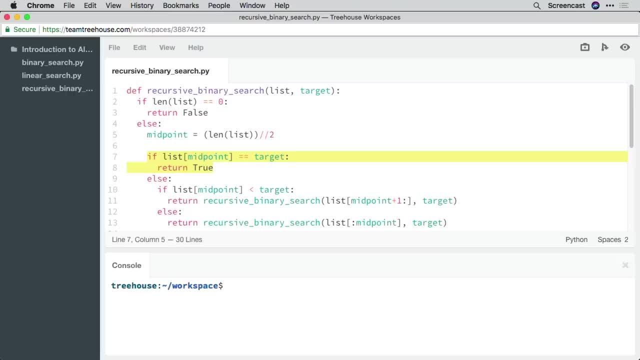 for n in new list. if n equals one, then print true and then after that break out of the loop. this is more or less the implementation of linear search. if the array were sorted, however, we could use binary search, but because sort operations incur a cost of their own languages usually. 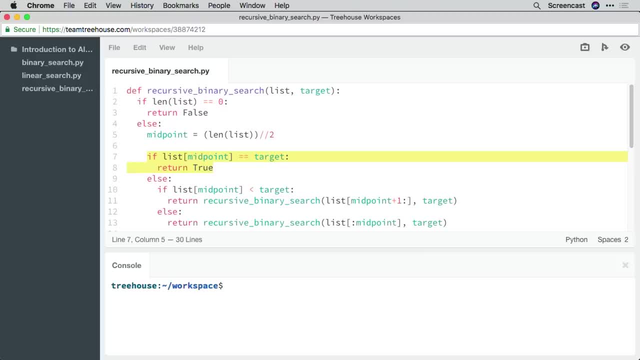 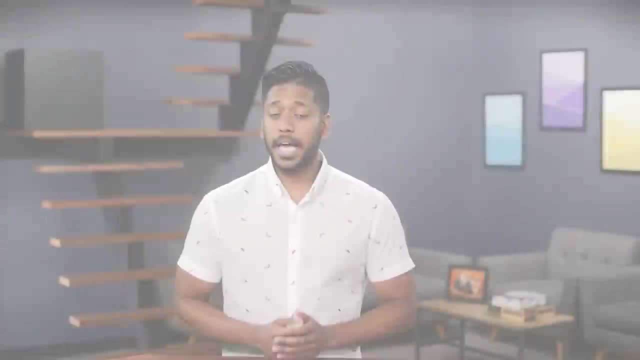 stay away from sorting the list and running binary search, since for smaller arrays, linear search on its own may be faster. now again, remember that, since this is an editor, this is just a text file. none of these lines of code are evaluated, so you can try that out in. 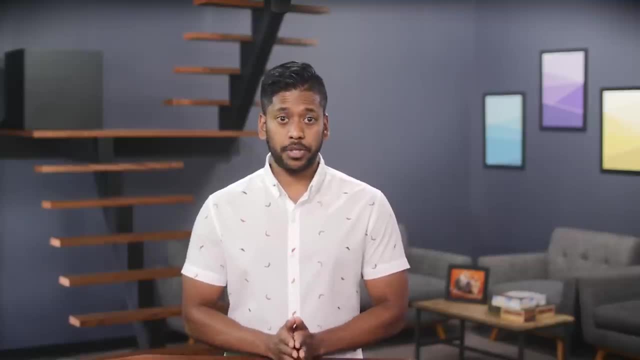 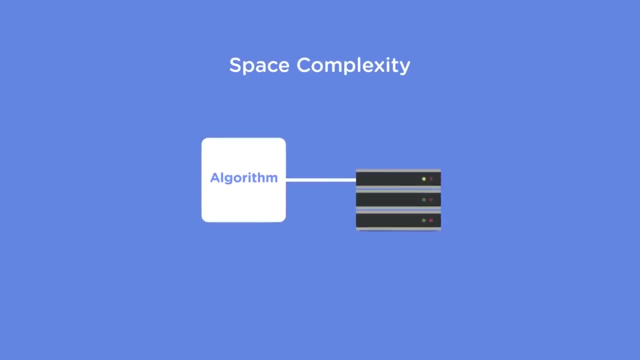 here, so we'll copy that. we can come down here and say python and hit enter and then when it starts up we can paste in our list and now we can try what we just did. so if one in new list print true, and there you go. it prints true now because we've 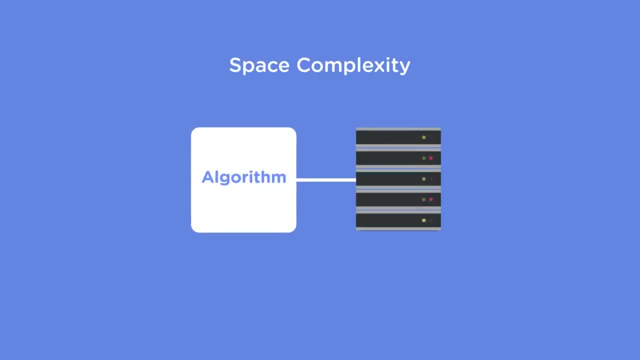 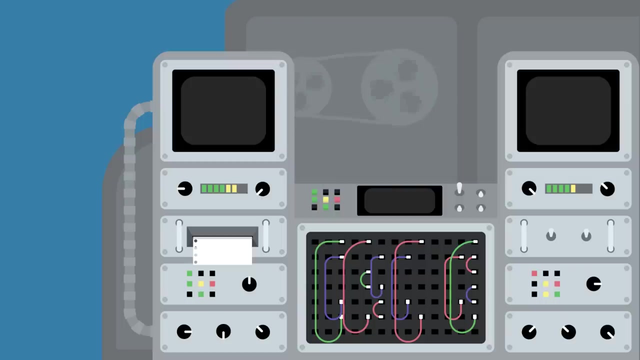 already learned about linear and binary search in a previous course. there's nothing new going on here. what's more interesting to look at, in my opinion, is inserting and deleting values in an array. let's start with inserting. in general, most array implementations support three types of insert. 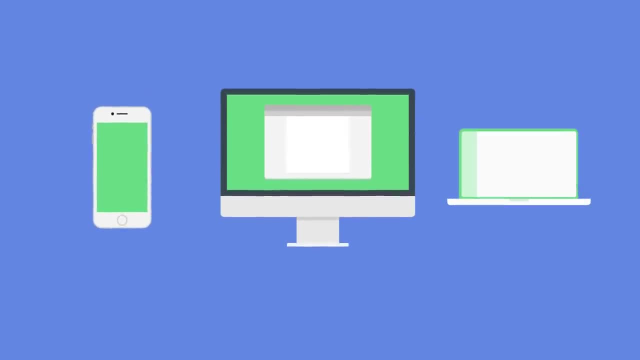 operations. the first is a true insert using an index value where we can insert an element anywhere in the list. this operation has a linear runtime. imagine you wanted to insert an item at the start of the list. when we insert into the first position, what happens to the item that is currently in? 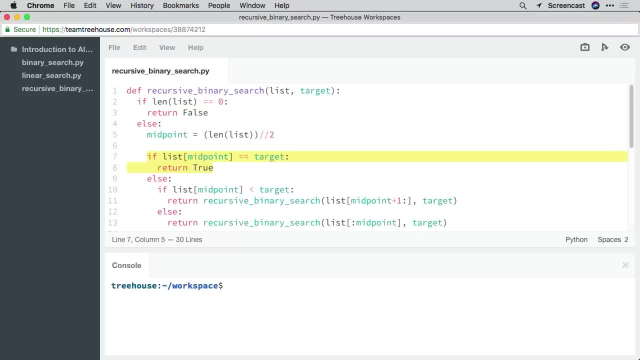 In that it doesn't care about recursion depth And does some neat tricks Where it doesn't even matter How many times your function calls itself. So if you want to see this in swift code, Then you need to know how recursion works. 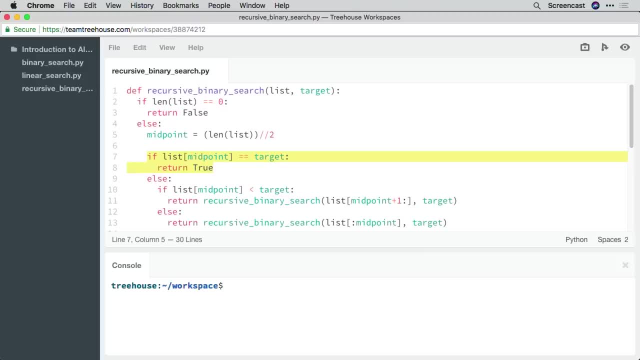 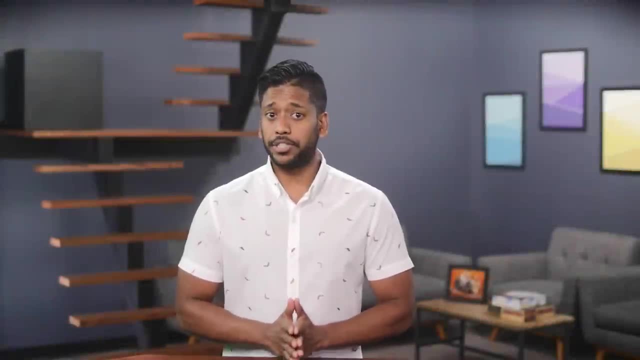 Well, and now you have some idea. Now, the second reason I bring it up Is actually way more important, And to find out On to the next video. At the beginning of this series, I mentioned that there were two ways Of measuring the efficiency of an algorithm. 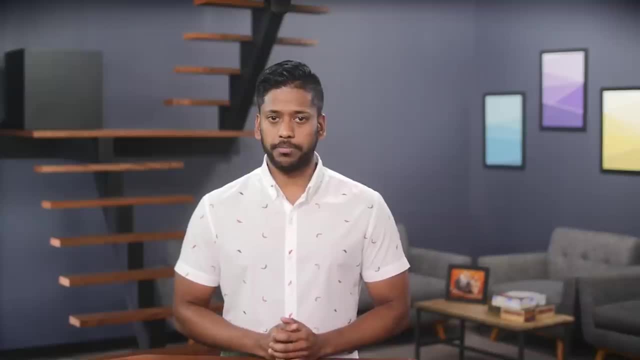 The first was time complexity, Or how the runtime of an algorithm Grows as n grows larger. The second is space complexity. We took a pretty long route To build up this example, But now we're in a good place To discuss space complexity. 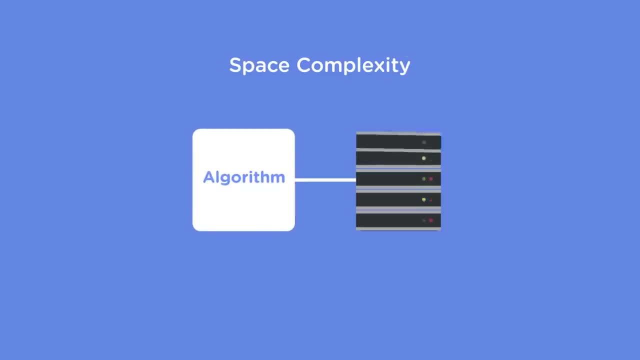 Space complexity is a measure Of how much storage is needed As a particular algorithm grows. We don't think about it much these days, But every single thing we do On a computer takes up space in memory In the early days of computing. 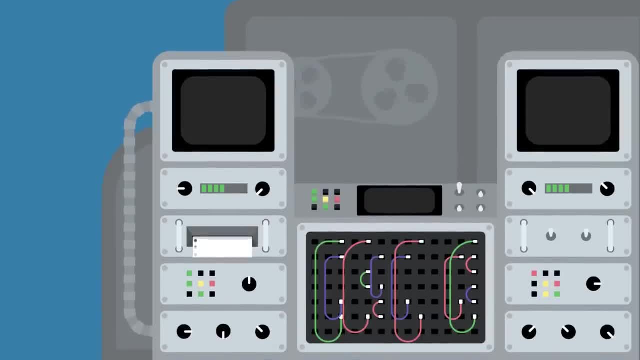 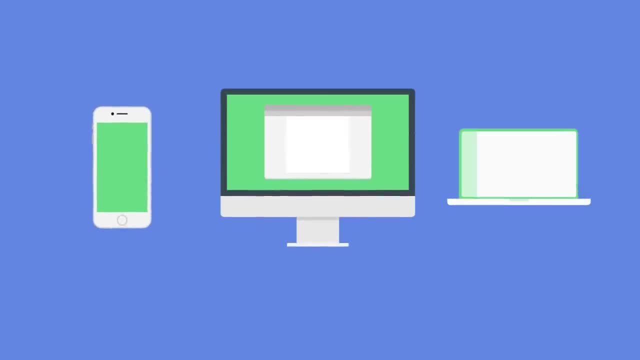 Considering memory usage Was of paramount importance, Because memory was limited And really expensive. These days, we're spoiled. Our devices are rich with memory. This is okay when we write everyday code, Because most of us aren't dealing with Enormously large data sets. 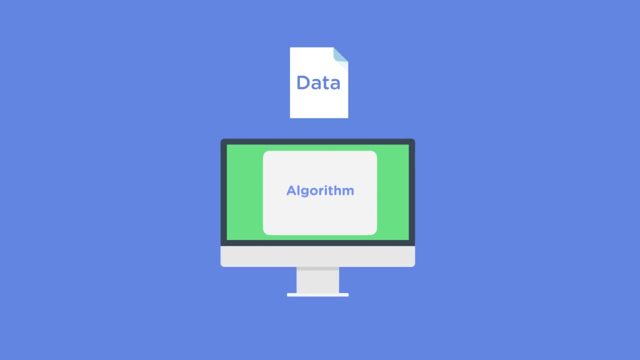 When we write algorithms, however, We need to think about this, Because we want to design our algorithms To perform as efficiently as it can, As the size of the data set n grows really large, Like time complexity, Space complexity is measured. 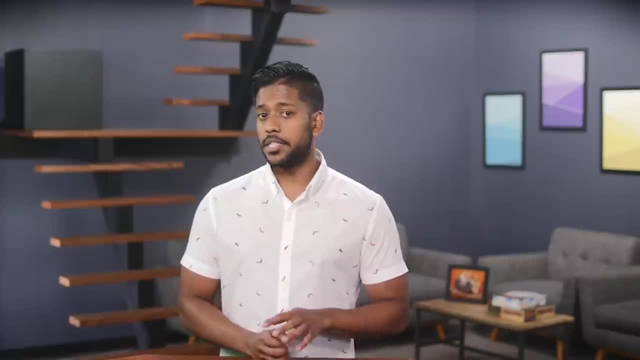 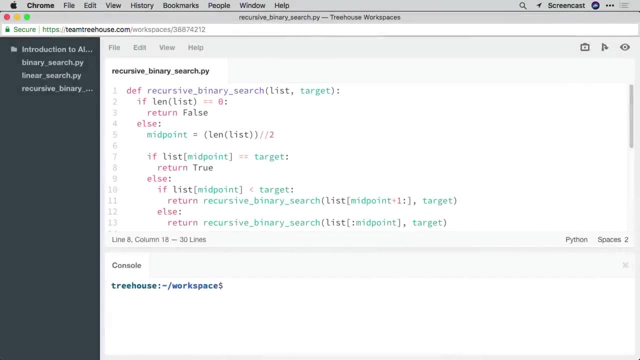 In the worst case scenario, Using big O notation. Since you are familiar with The different kinds of complexities, Let's dive right into an example. In our iterative implementation Of binary search That uses a while loop, Let's look at what happens to our memory usage. 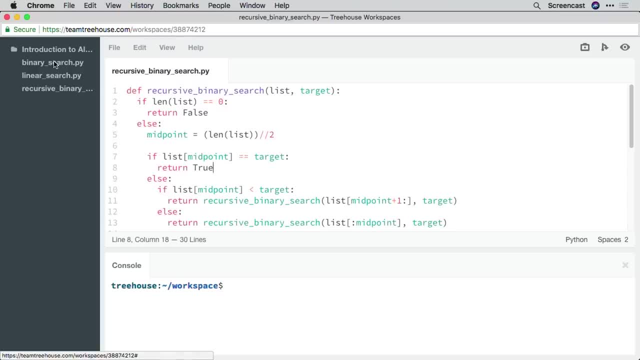 As n gets large, Let's bring up that function. Let's say We start off with a list of 10 elements. Now, inspecting the code, We see that our solution relies heavily On these two variables: First and last. First points to the start of the list. 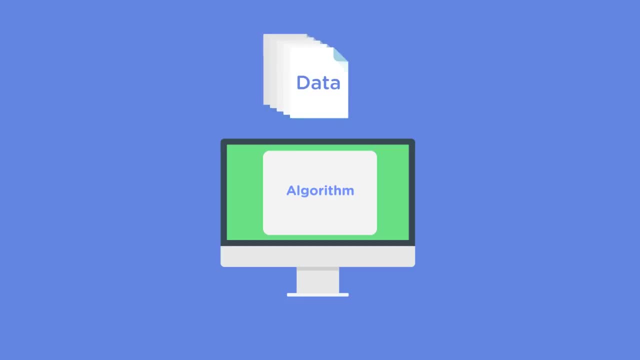 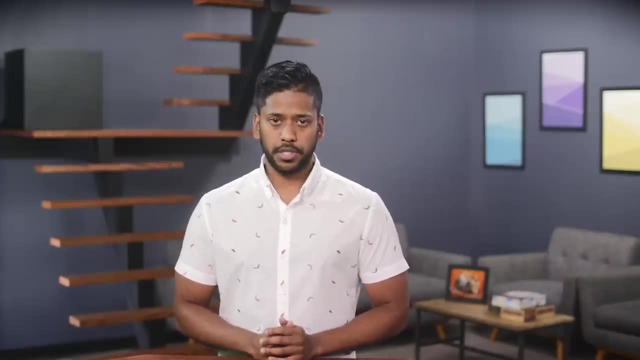 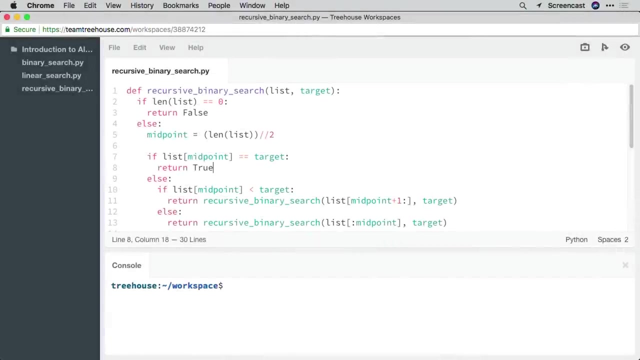 that spot. well, it has to move to the next spot at index value one. what happens to the second item at index position one? that one moves to the next spot at index position two. this keeps happening until all elements have been shifted forward. one index position. so in the 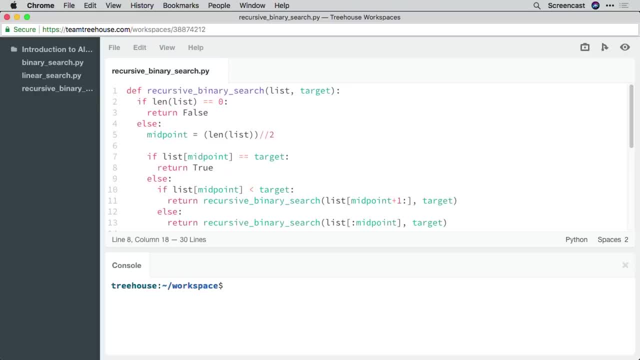 worst case scenario, inserting at the zeroth position of an array. every single item in the array has to be shifted forward and we know that any operation that involves iterating through every single value means a linear runtime. now the second way we can insert an item into an. 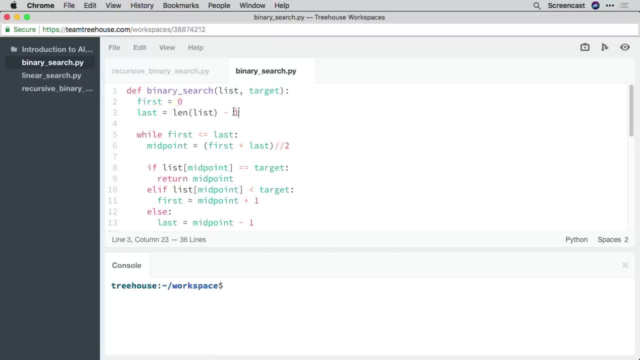 array is by appending. appending, although technically an insert operation, in that it inserts an item into an existing array, doesn't incur the same runtime cost, because appends simply add the item to the end of the list. we can simplify and say that this is constant time. this is a constant time. 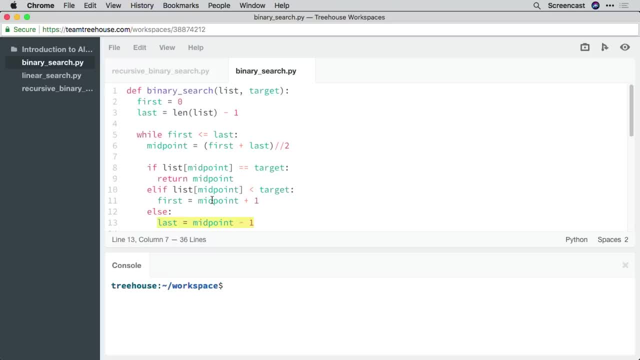 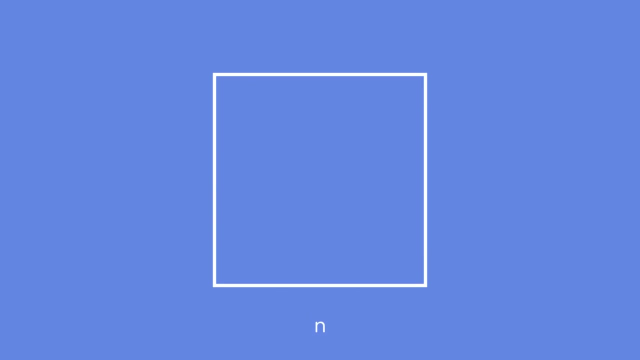 operation, but it depends on the language implementation of array. to highlight why that matters, let's consider how lists in python work. in python, when we create a list, the list doesn't know anything about the size of the list and how many elements we're going to store. 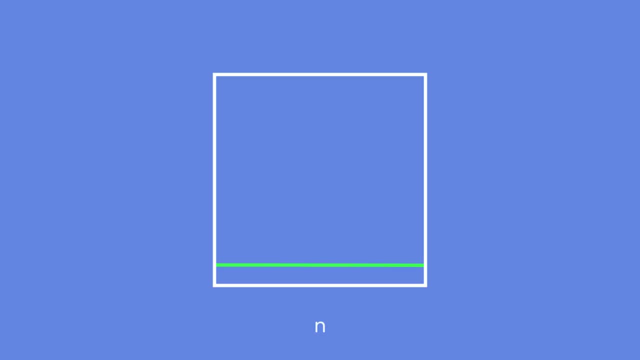 creating a new empty list like: so numbers equal and two empty brackets. so this creates a list and allocates a space of size n plus one. since n here is zero, there are no elements in this array. in this list, space is allocated for a one element list. to start off. 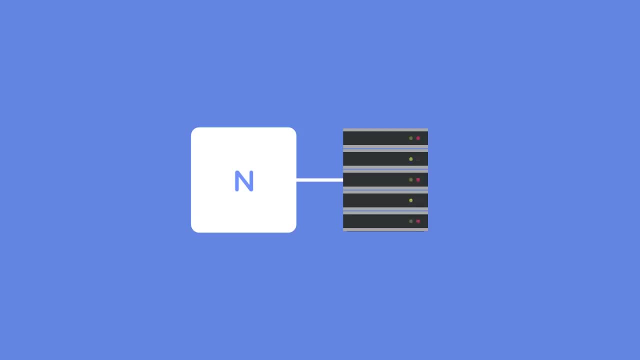 because the space allocated for the list and the space used by the list are not the same. what do you think happens when we ask python for the length of this list, so i can say len numbers? we correctly get zero back. this means that the list doesn't use the memory. 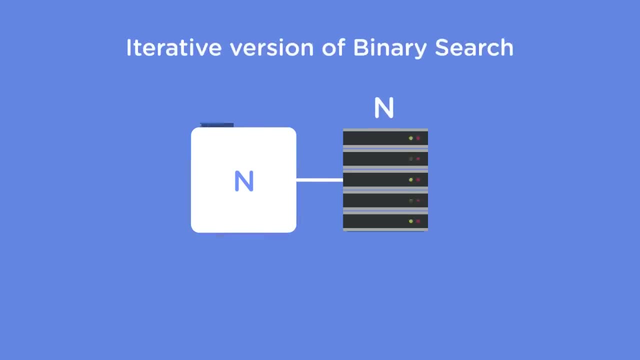 allocation as an indicator of its size, because, as i mentioned, it has allocated space for a one element list, but it returns zero, so it determines it in other ways. okay, so numbers. this list currently has space for one element. let's use the append method defined on the type to insert a number at the 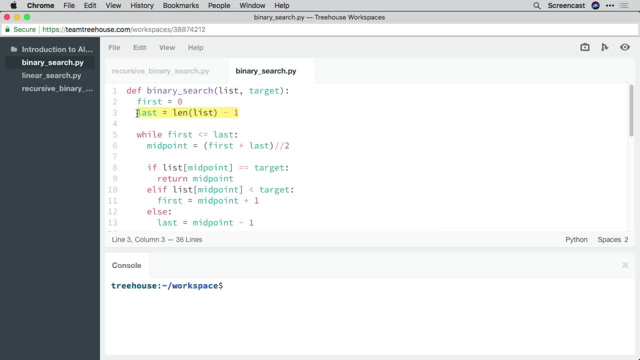 And last, to the end, When we eliminate a set of values, We don't actually create a sub list. Instead, we just redefine Last, as you see here To point to a different section of the list, Since the algorithm Only considers the values. 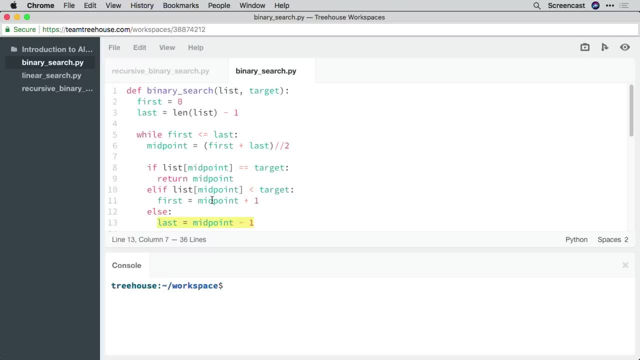 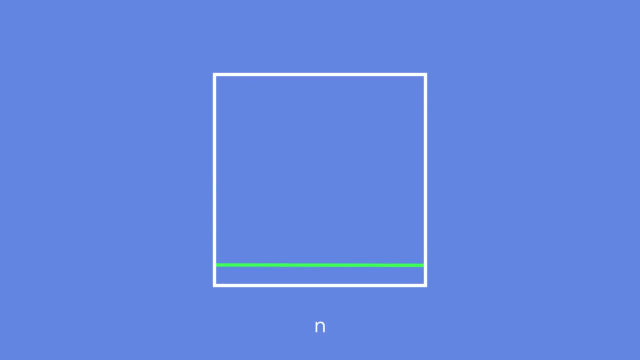 Between first and last When determining the midpoint, By redefining first and last As the algorithm proceeds, We can find a solution Using just the original list. This means that for any value of n, The space complexity Of the iterative version of binary search. 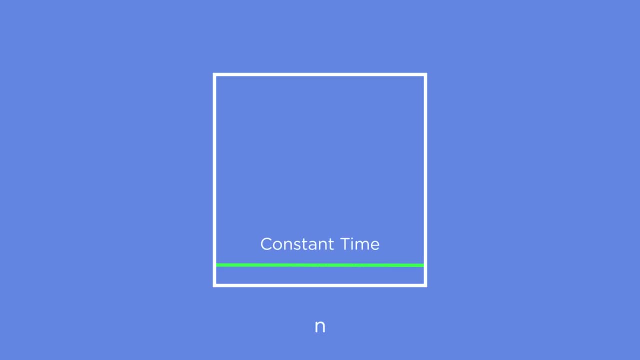 Is constant Or that the iterative version of binary search Takes constant space. Remember that we would write this as Big O of 1.. This might seem confusing Because as n grows We need more storage to account for that larger list size. 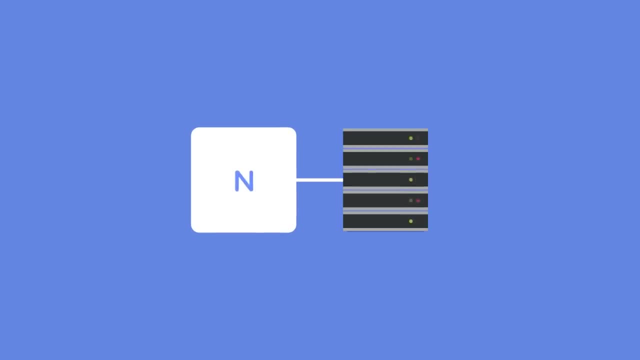 Now, this is true, But that storage is not what space complexity Cares about: measuring We care about what additional storage Is needed As the algorithm runs And tries to find a solution. If we assume something simple, Say that for a given size of a list. 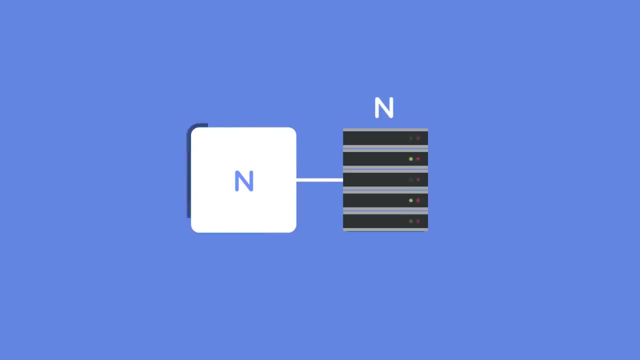 With value n, It takes n amount of space to store it. Whatever that means Then for the iterative version of binary search, Regardless of how large the list is At the start, Middle and end of the algorithm process, The amount of storage required. 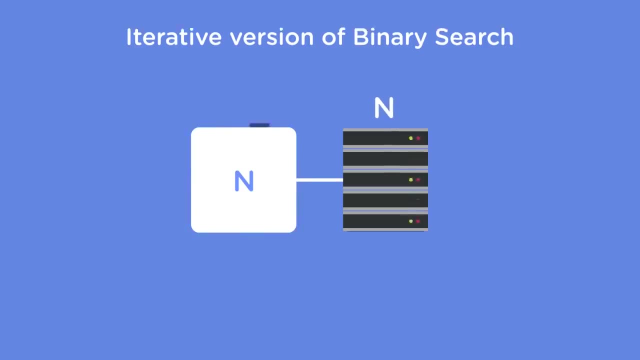 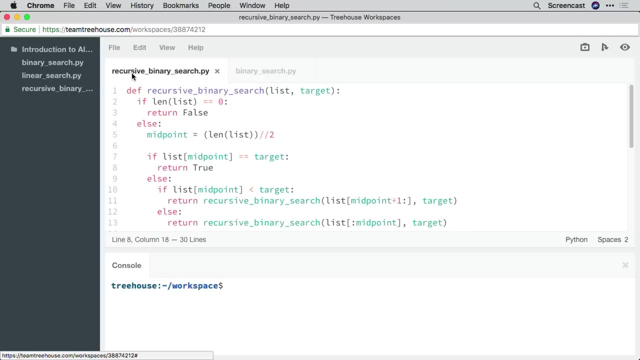 Does not get larger than n, And this is why We consider it to run in constant space. Now, This is an entirely different story With the recursive version, however. In the recursive version of binary search, We don't make use of variables. 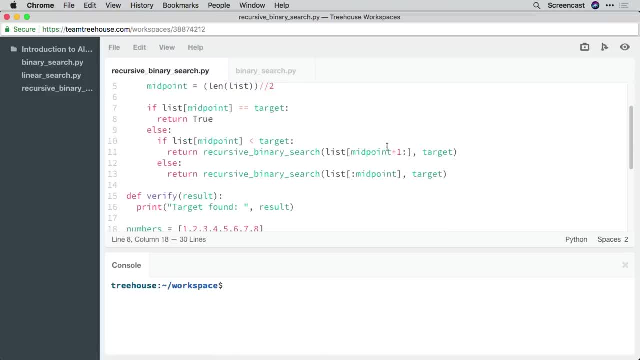 To keep track of which portion of the list We're working with. Instead, we create new lists Every time with a subset of values, Or sub lists With every recursive function call. Let's assume we have a list of size n And in the worst case scenario, 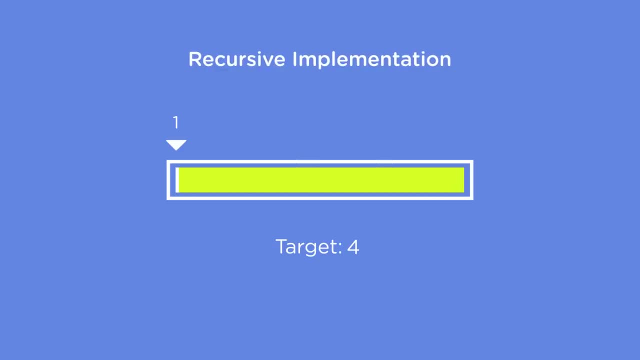 The target element is the last in the list. Calling the recursive implementation Of binary search on this list And target Would lead to a scenario like this. The function would call itself A new list That goes from the midpoint To the end of the list. 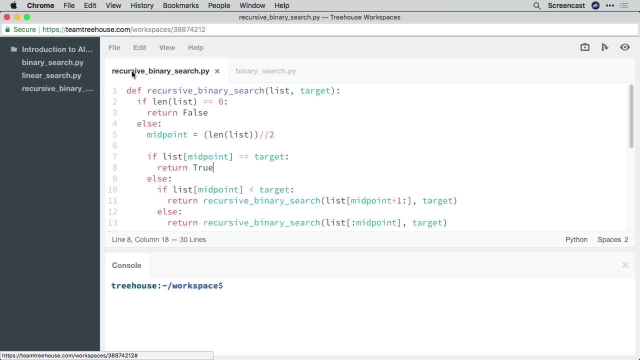 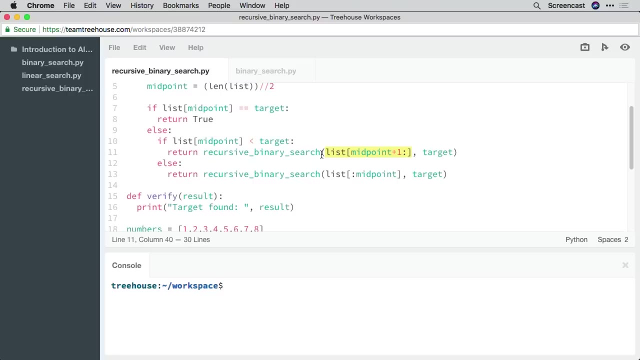 end of the list, so i can say numbers dot, append. and i'll pass in two. now the memory allocation and the size of the list are the same, since the list contains one element. now what if i were to do something like this: numbers dot, append. that needs to be a dot. 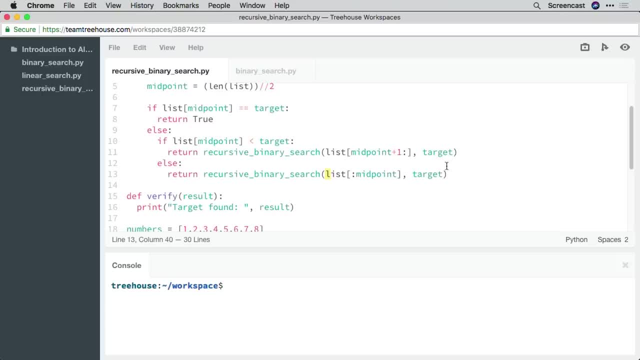 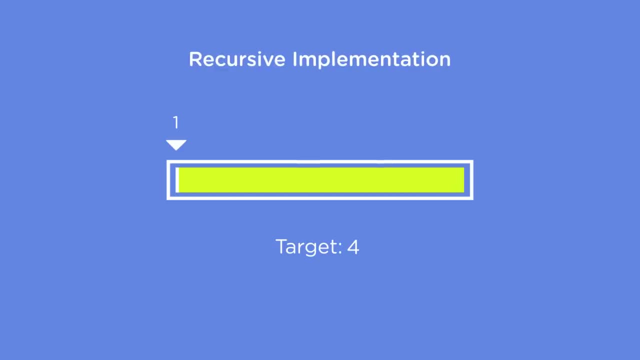 and i'll add another value, two hundred, now, since the list only has an allocation for one item at this point, before it can add the new element to the list, it needs to increase the memory allocation and thereby the size of the list. it does this by calling a list resize. 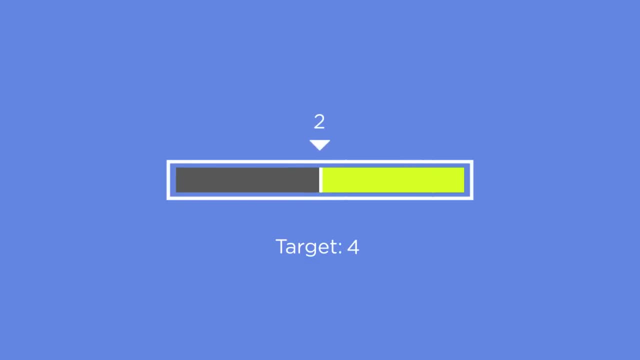 operation. list resizing is quite interesting because it shows the ingenuity in solving problems like this. python doesn't resize the list to accommodate just the element we want to add instead. in this case, it would allocate four blocks of memory to increase the size to a total of 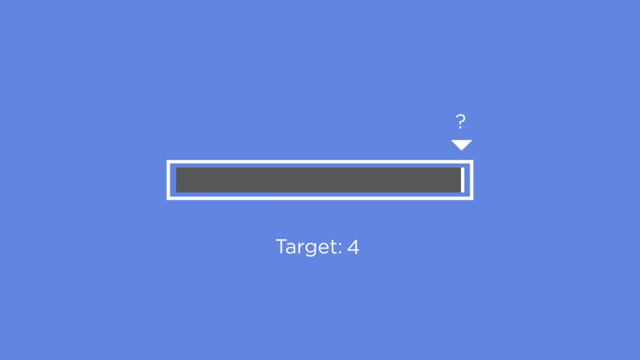 four contiguous blocks of memory. it does this so that it doesn't have to resize the list every single time we add an element, but at very specific points. the growth pattern of the list type in python is zero. four, eight, sixteen, twenty five, thirty five, forty six and so. 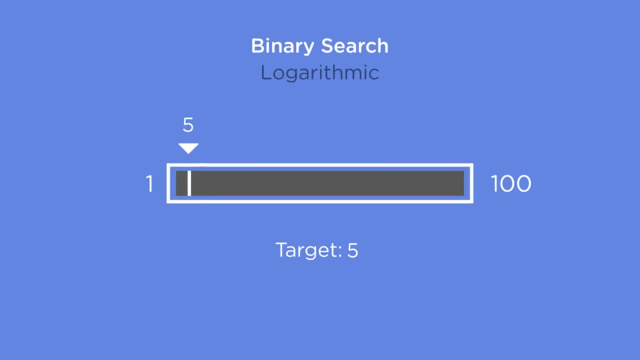 on. this means that as the list size approaches these specific values, resize is called again. if you look at when the size of the list is four, this means that when appending four more values until the size of eight, each of the those append operations do not increase the amount of space taken. 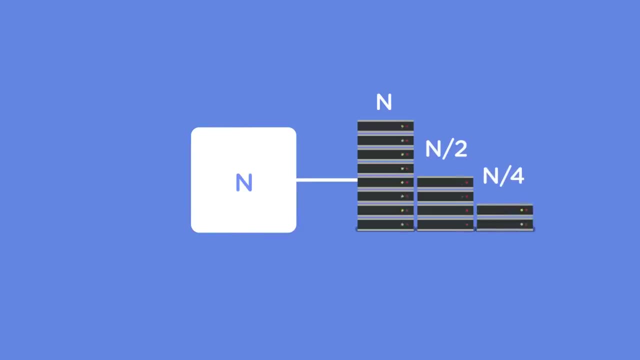 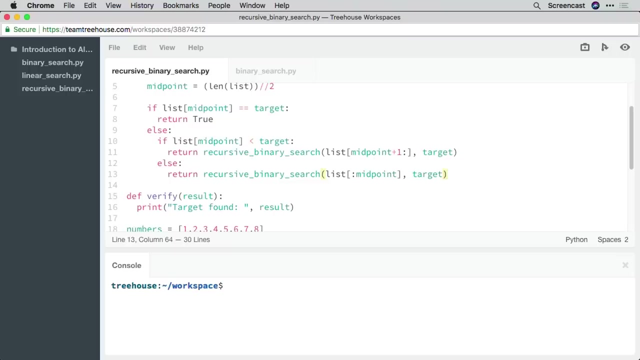 at specific points. however, when resizing is triggered, space required increases as memory allocation increases. this might signify that the append method has a non constant space complexity, but it turns out that, because some operations don't increase space and others do, when you average all of them out, append operations take: 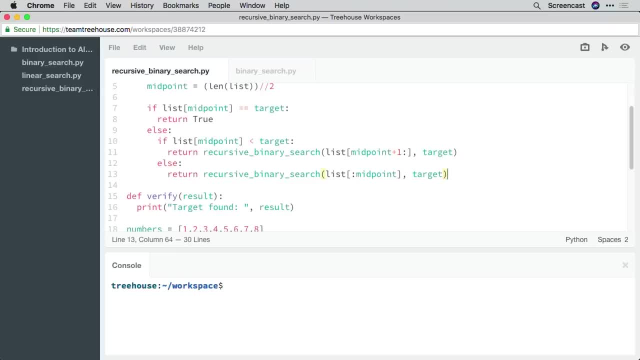 constant space. we say that it has an amortized constant space complexity. this also happens with insert operations. if we had a four element array, we would have four elements and a memory allocation of four. an insert operation at that point doesn't matter where it happens on the list. 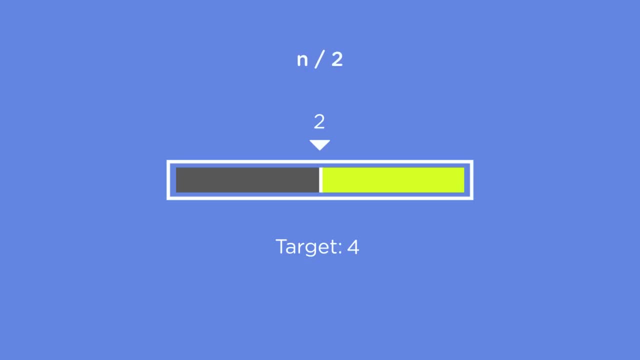 Since we're discarding half the values, The size of the sub list is n by 2. This function will keep calling itself Creating a new sub list That's half the size of the current one, Until it arrives at a single element list. 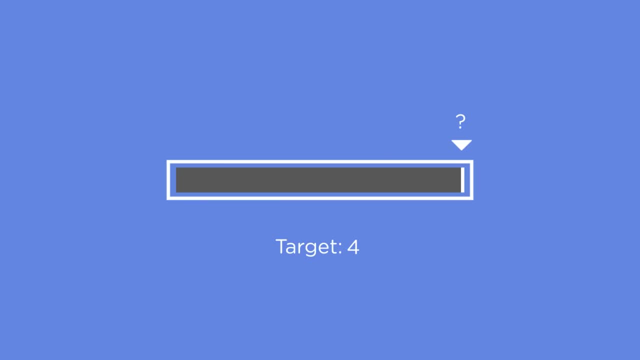 And a stopping condition, This pattern that you see here, Where the size of the sub list Is reduced by a factor On each execution of the algorithmic logic. Well, we've seen that pattern before. Do you remember where? This is exactly how binary search works. 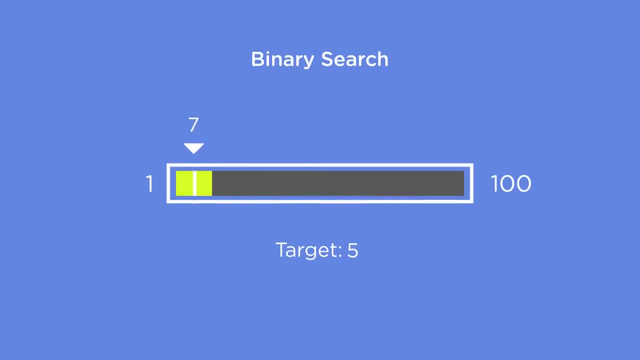 It discards half the values Every time until it finds a solution. Now we know that, because of this pattern, The running time of binary search Is logarithmic. In fact, the space complexity Of the recursive version of binary search Is the same. 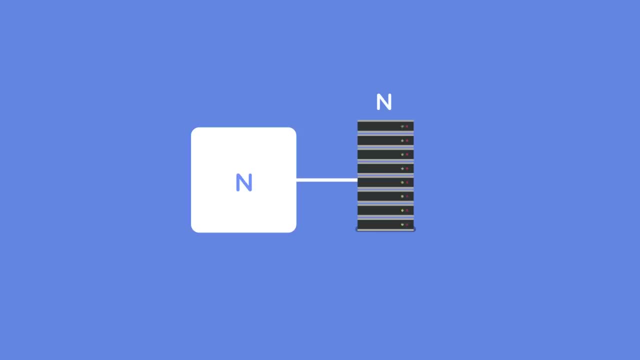 If we start out with a memory allocation Of size n that matches the list On each function call Of recursive binary search, We can allocate additional memory Of size n by 2, n by 4 and so on, Until we have a sub list. 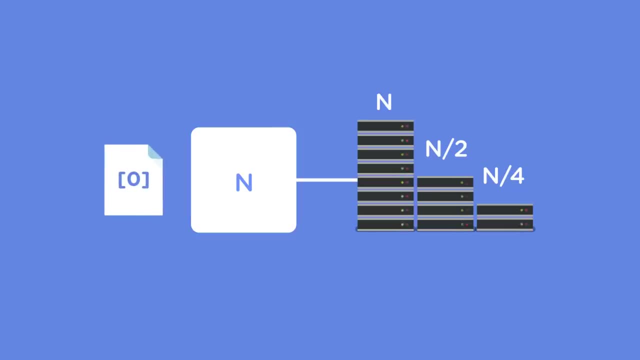 That is either empty or contains a single value. Because of this We say that the recursive version Of the binary search algorithm Runs in logarithmic time With a big O of log n. Now there's an important caveat here. This totally depends on the language. 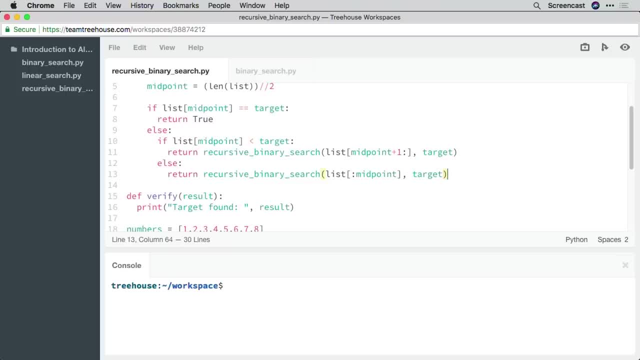 Remember how I said that A programming language like swift Can do some tricks to where Recursion depth doesn't matter. The same concept applies here. If you care to read more about this concept, It's called tail optimization. It's called tail optimization. 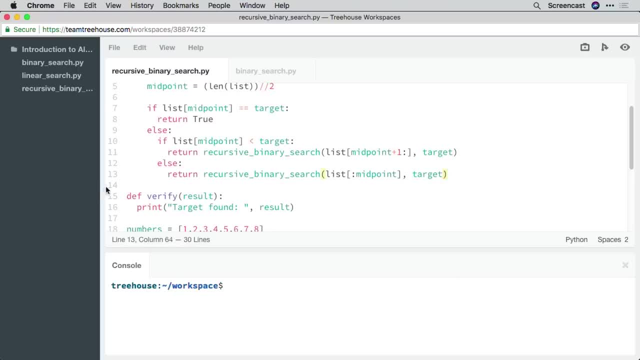 Because, if you think of a function As having a head and a tail, If the recursive function call Is the last line of code In the function, As it is in our case, We call this tail recursion, Since it's the last part of the function. 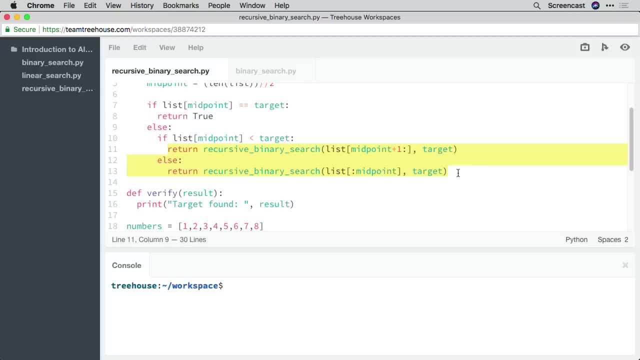 That calls itself. Now the trick that swift does To reduce the amount of space For computing overhead. To keep track of this, recursive calls Is called tail call optimization Or tail call elimination. It's one of those things That you'll see thrown around a lot. 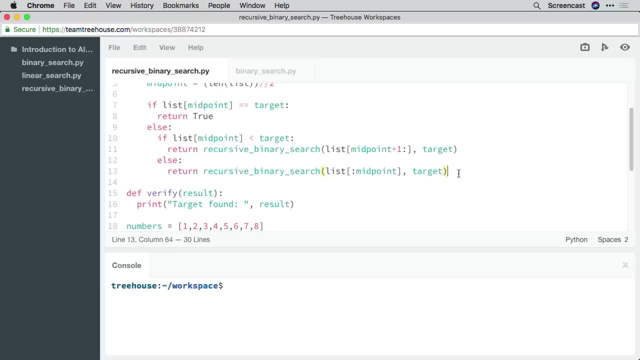 but at that point it would trigger a resize. inserting is still more expensive, though, because after the resize, every element needs to be shifted over one. the last insert operation that is supported in most languages is the ability to add one list to another. in python, this is called an extend and looks: 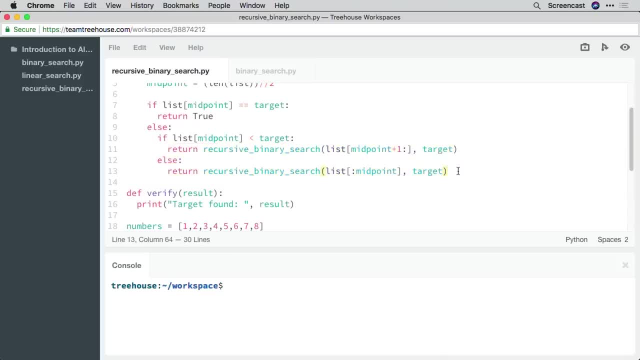 like this. so i'll say numbers now, if you let me actually clear out the console. oh actually, well, let's exit python. we'll clear this out. so we're back at the top and we'll start again. so i'll say numbers and we'll set it to an empty list. and now 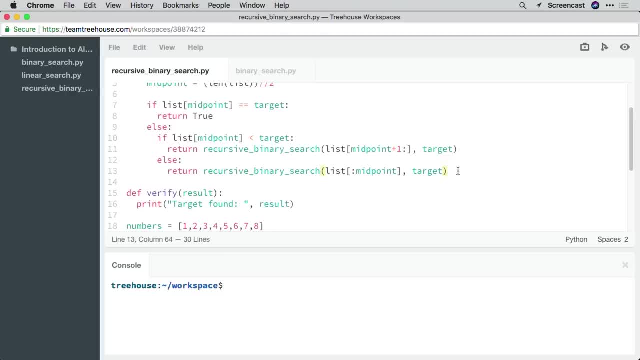 we can say numbers, dot, extend, and as an argument we're going to pass in a new list entirely. so here we'll say four comma five, comma six, and then, once i hit enter, if i were to print out numbers, you'll see that it now contains the values four, five. 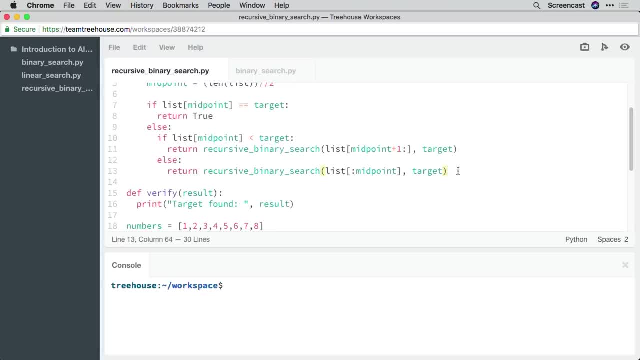 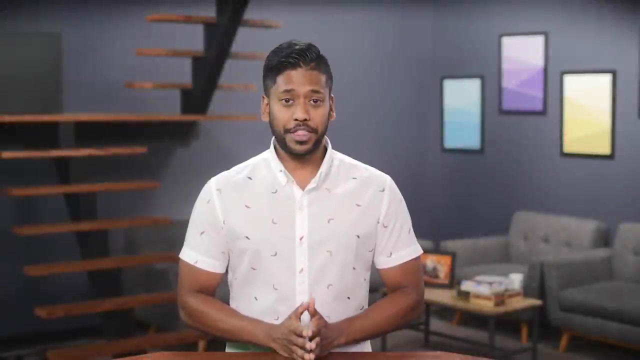 and six. so extend takes another list to add. extend effectively makes a series of append calls on each of the elements in the new list until all of them have been appended to the original list. this operation has a runtime of big O of k, where k represents the number of elements in the 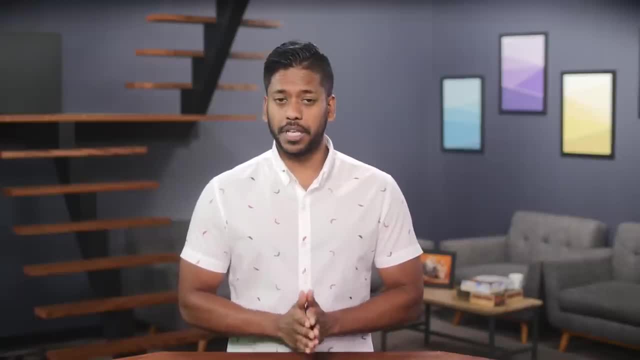 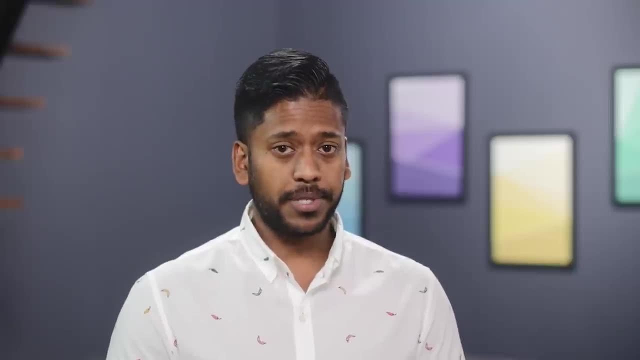 list that we're adding to our existing list. the last type of operation we need to consider are delete operations. deletes are similar to inserts in that when a delete operation occurs, the list needs to maintain correct index values. so where an insert shifts every element to the right, a delete operation shifts. 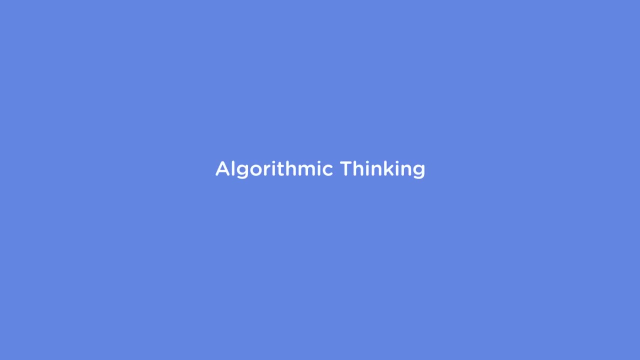 every element to the left, just like an insert as well. if we delete the first element in the list, every single element in the list needs to be shifted to the left. delete operations have an upper bound of big O of n, also known as a linear runtime. now that we've seen how common 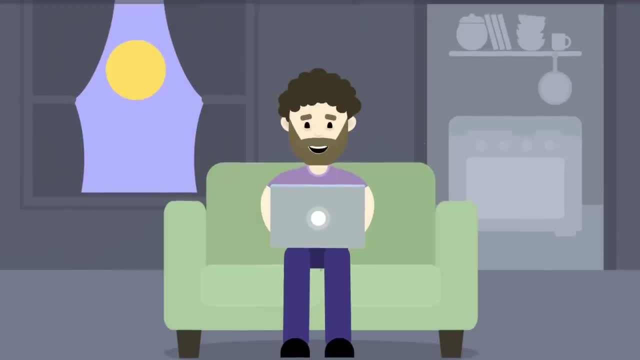 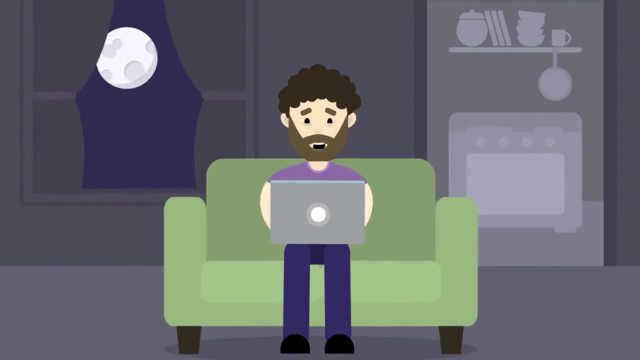 operations work on a data structure that we're quite familiar with. let's switch tracks and build our own data structure. over the next few videos, we're going to build a data structure that you may have worked with before- a linked list. before we get into what a linked list is, let's talk. 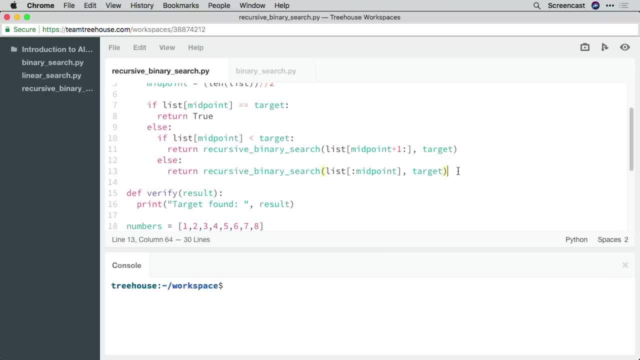 In algorithm discussions, But may not always be relevant to you. Now what if any of this is relevant to us? Well, python does not Implement tail call optimization, So the recursive version of binary search Takes logarithmic space. If we had to choose, 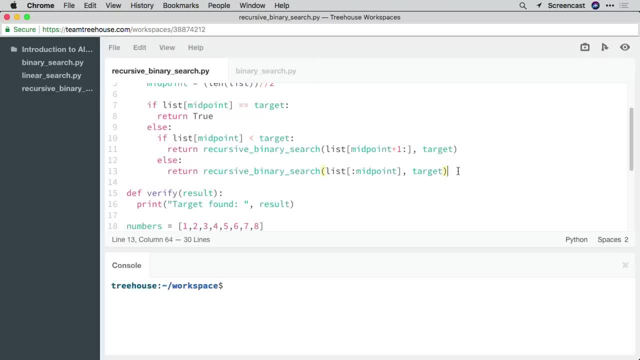 Between the two implementations. Given that time, complexity Or run time of both versions, The iterative and the recursive version Are the same. We should definitely go with the iterative implementation In python, Since it runs in constant space. Okay, that was a lot. 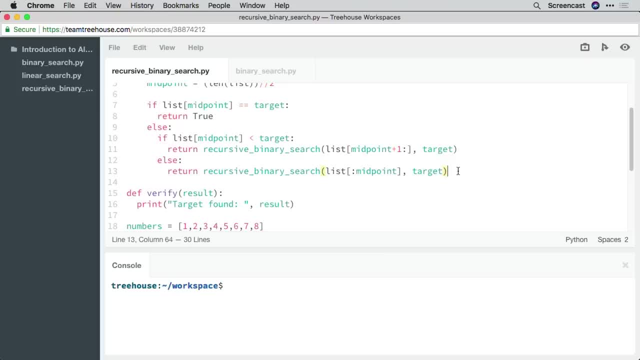 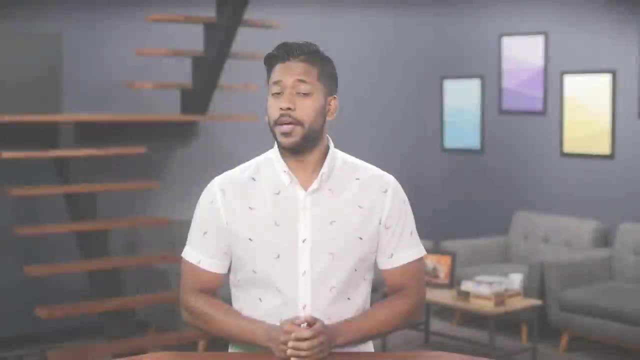 But with all of this, We've now established two important ways To distinguish between algorithms That handle the same task And determine which one we should use. We've arrived at what I think Is a good spot to take a long break. 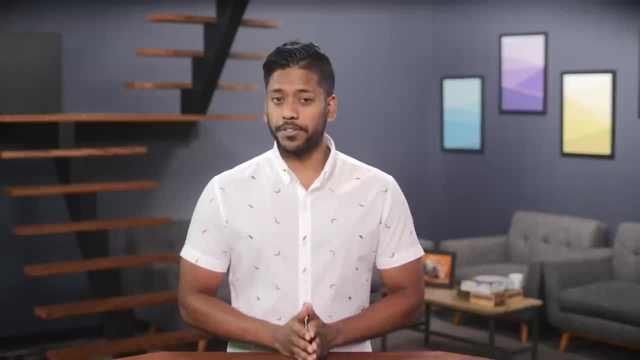 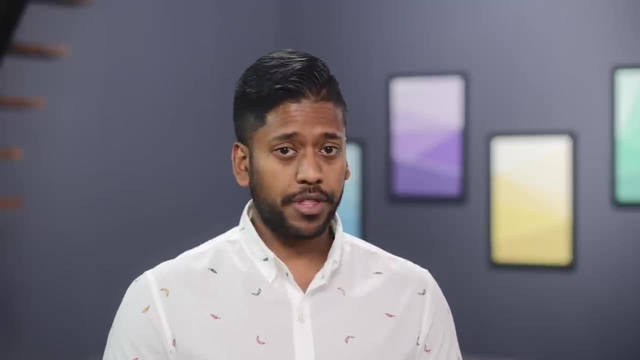 And let all of these new concepts sink in. But before you go off to the next course, Let's take a few minutes To recap everything we've learned so far, While we did implement two algorithms In this course In actual code. 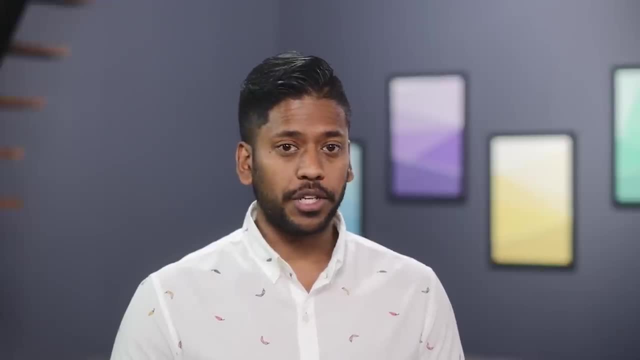 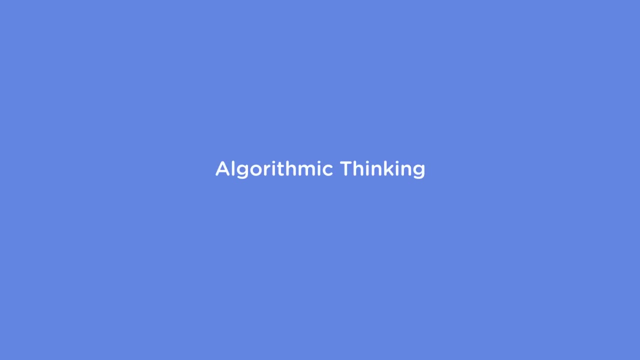 Much of what we learned here was conceptual And will serve as building blocks For everything we're going to learn in the future. So let's list all of it out. The first thing we learned about, And arguably the most important, Was algorithmic thinking. 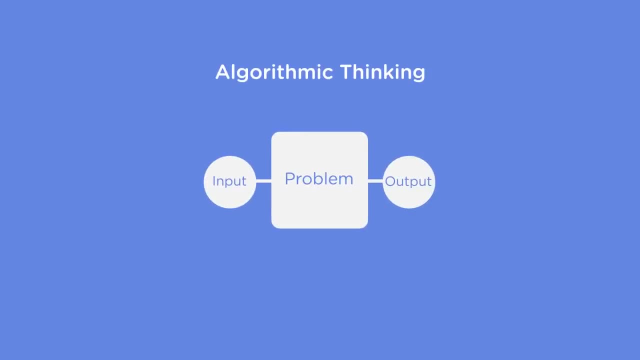 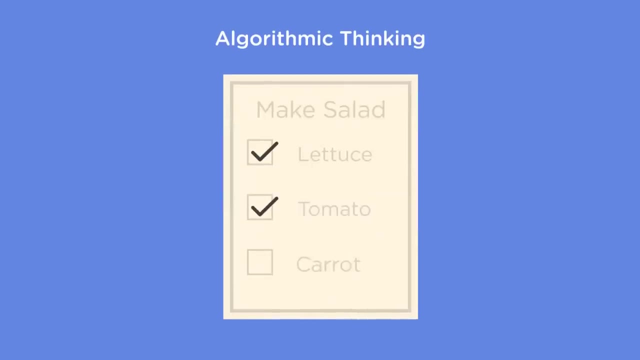 Algorithmic thinking is an approach To breaking a problem down Into a clearly defined input and output, Along with a distinct set of steps That solves the problem By going from input to output. Algorithmic thinking is not something You develop overnight. 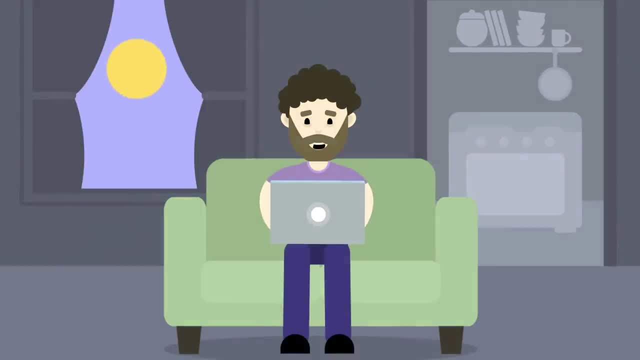 By taking one course, So don't worry if you're thinking, I still don't truly know how to apply What I learned here. Algorithmic thinking sinks in After you go through several examples In a similar fashion to what we did today. 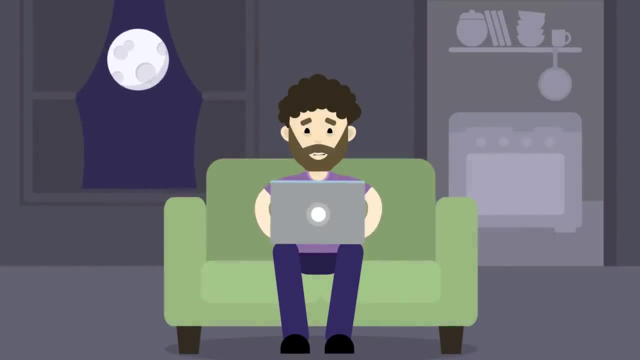 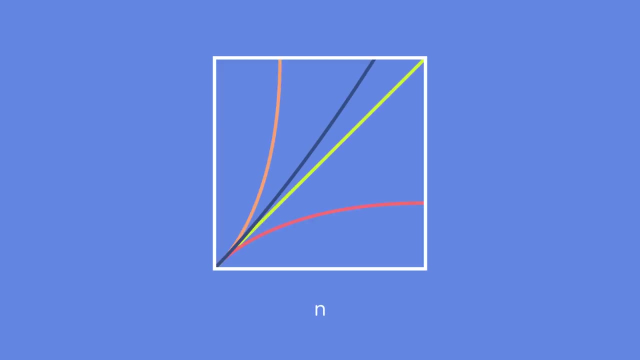 We're going to look at three steps In the context of a real example, Which is another thing We will strive to do moving forward. Regardless, it is important to keep in mind That the main goal here Is not to learn how to implement. 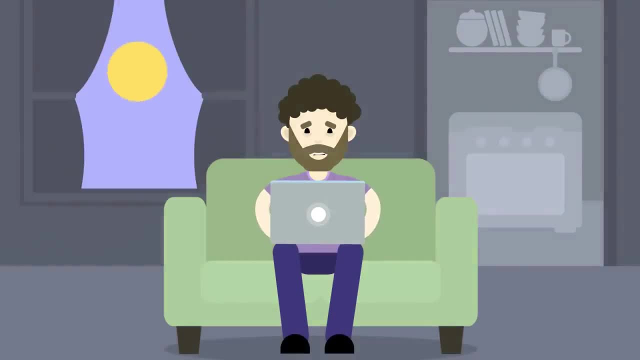 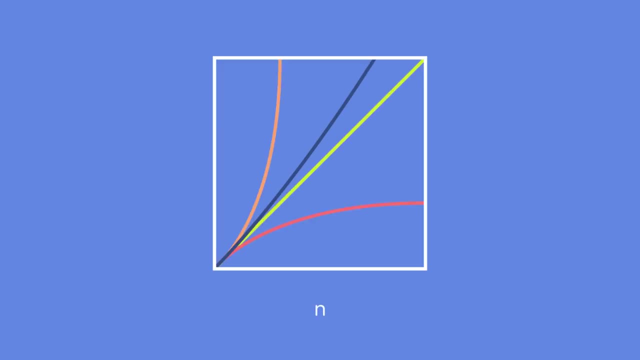 about why we build data structures instead of just using the ones that come built in to our languages. each data structure solves a particular problem. we just went over the basics of the array data structure and looked at the cost of common operations that we carry out on arrays. 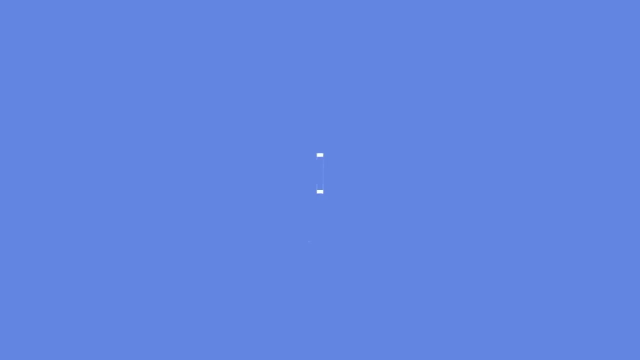 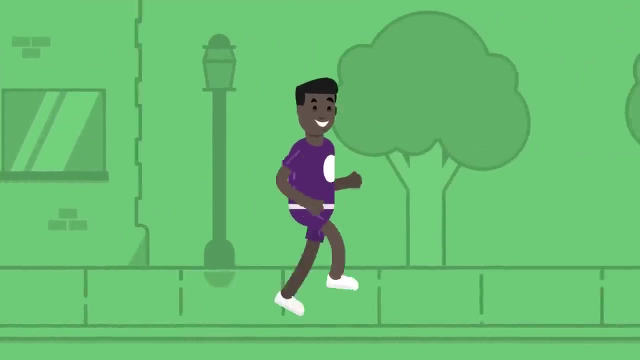 we found that arrays were particularly good at accessing reading values happens in constant time, but arrays are pretty bad at inserting and deleting, both of which run in linear time. linked lists, on the other hand, are somewhat better at this, although there are some caveats, and if we're trying to solve a problem that involves 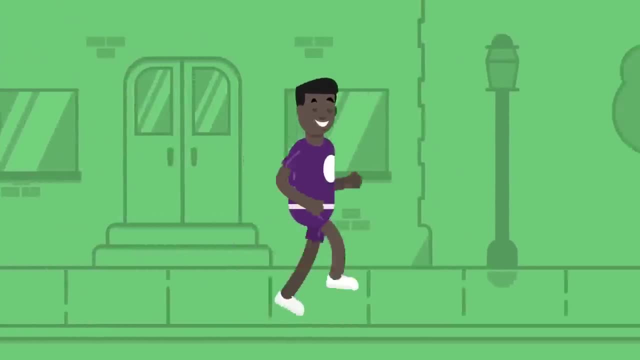 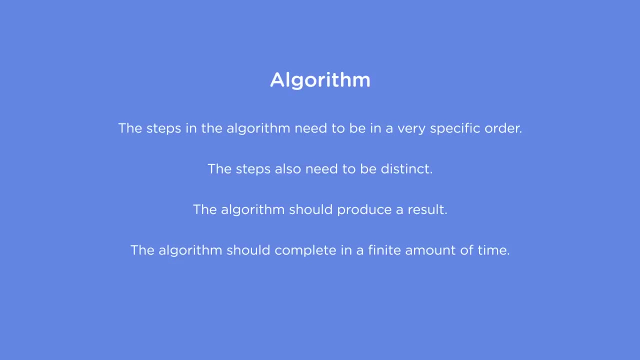 far more inserts and deletes than accessing. a linked list can be a better tool than an array. so what is a linked list? a linked list is a linear data structure where each element in the list is contained in a separate object called a node. a node models two pieces of information: an individual. 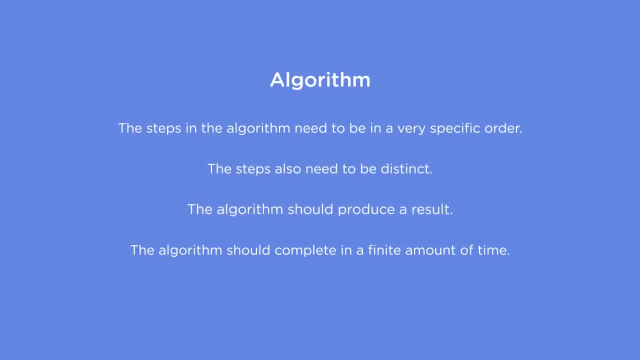 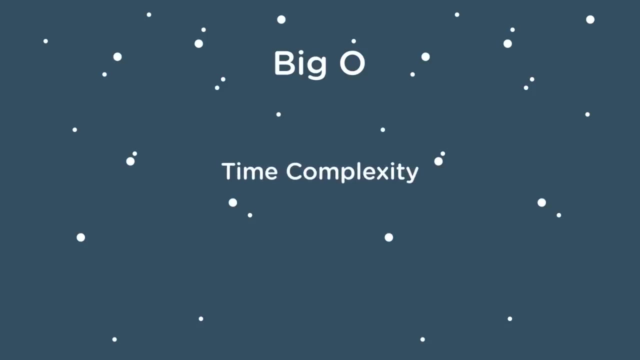 item of the data we want to store and a reference to the node in the list. the first node in the linked list is called the head of the list, while the last node is called the tail. the head and the tail nodes are special. the list only maintains a. 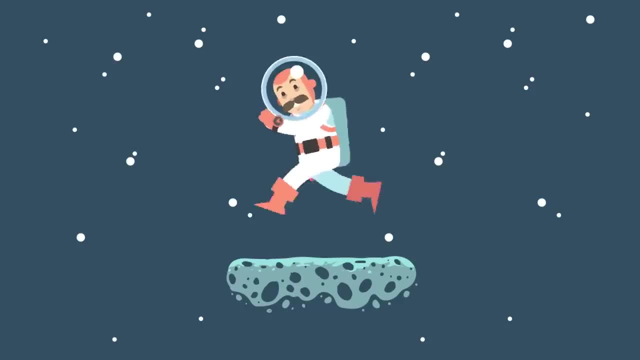 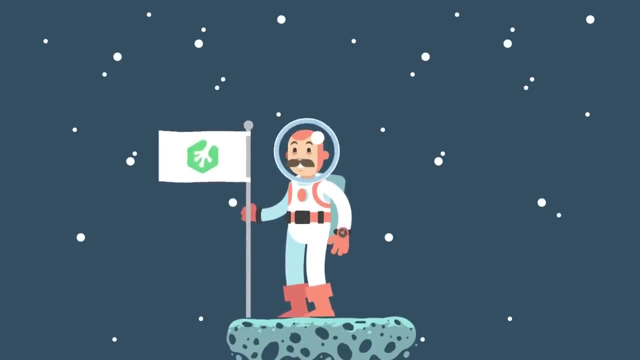 reference to the head, although in some implementations it keeps a reference to the tail as well. this aspect of linked lists is very important and, as you'll see, most of the operations on the list need to be implemented quite differently compared to an array. the opposite of the head, the tail. 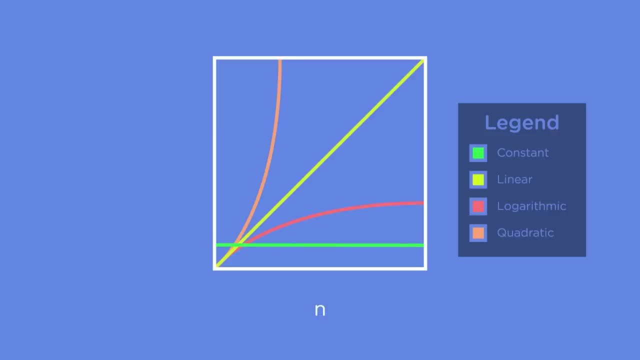 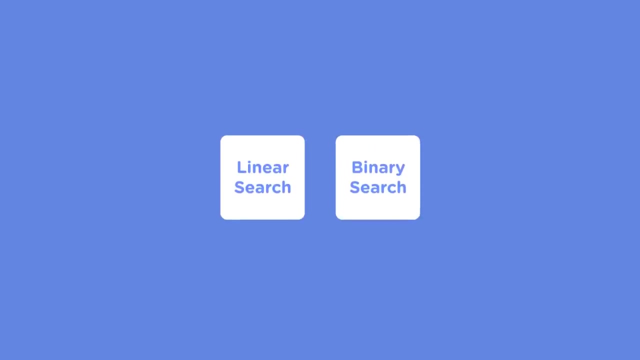 denotes the end of the list. every node other than the tail points to the next node in the list, but tail doesn't point to anything. this is basically how we know it's the end of the list. nodes are what are called self-referential objects. the definition of a node includes: 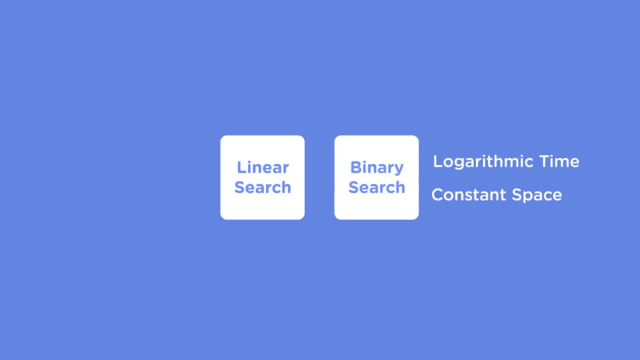 a link to another node, and self-referential here means the definition of node includes the node itself. linked lists often come in two forms: a singly linked list, where each node stores a reference to the next node in the list, and a doubly linked list or a doubly linked. 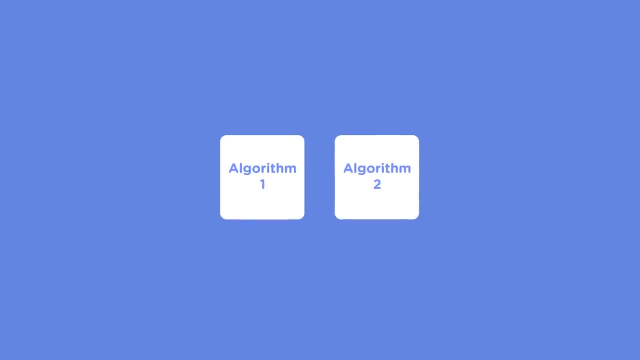 list where each node stores a reference to both the node before and after. if an array is a train with a bunch of cars in order, then a linked list is like a treasure hunt. when you start the hunt, you have a piece of paper with the location of the first treasure. 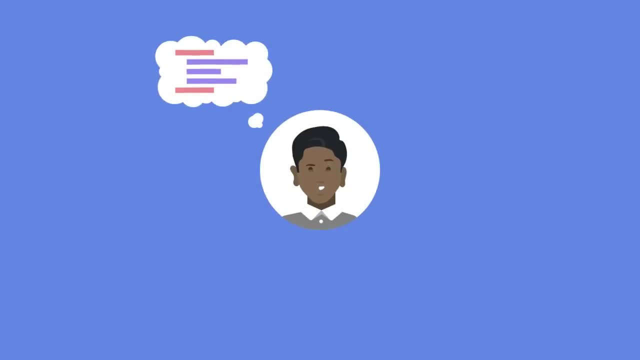 A specific data structure or algorithm Off the top of your head. I'll be honest, I had to look up a couple code snippets For a few of the algorithms myself In writing this course, But in going through this It's a faster search algorithm. 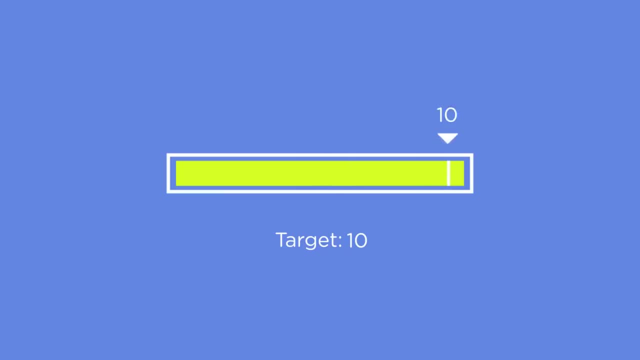 Unlike most courses, Where you can immediately apply what you have learned To build something cool. Learning about algorithms and data structures Will pay off more in the long run. The second thing we learned about Is how to define and implement algorithms. We've gone over these guidelines several times. 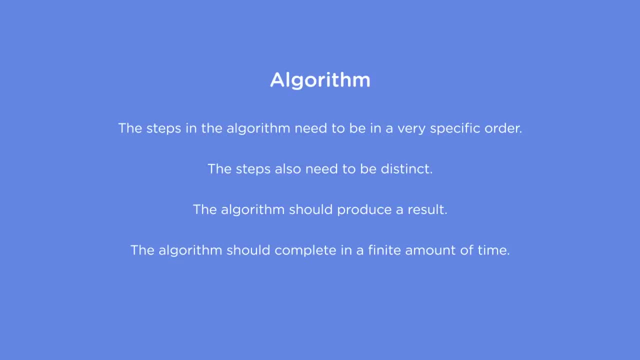 So I won't bore you here again At the end, But I will remind you That if you're often confused About how to effectively break down a problem in code To something more manageable, Then algorithm guidelines Is a good place to start. 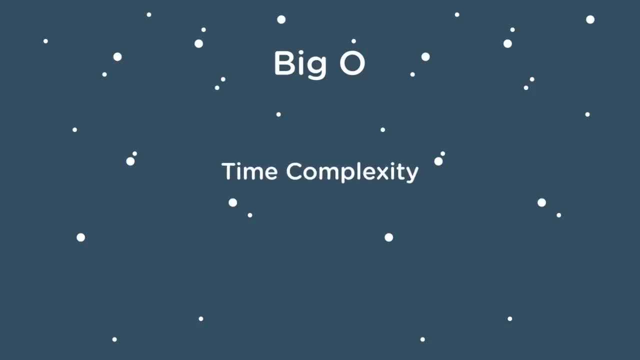 Next we learned about Big O And measuring the time. complexity of algorithms. This is a mildly complicated topic, But once you've abstracted the math away It isn't as hazy a topic as it seems Now, don't get me wrong. 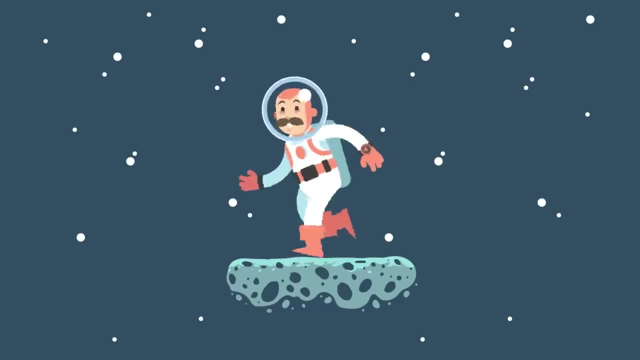 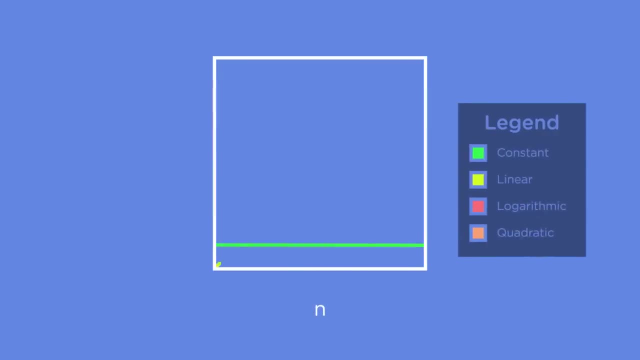 The math is pretty important, But only for those designing and analyzing algorithms. Our goal is more about How to understand and evaluate algorithms. We learned About common run times Like constant, Logarithmic And quadratic run times. These are all fairly new concepts. 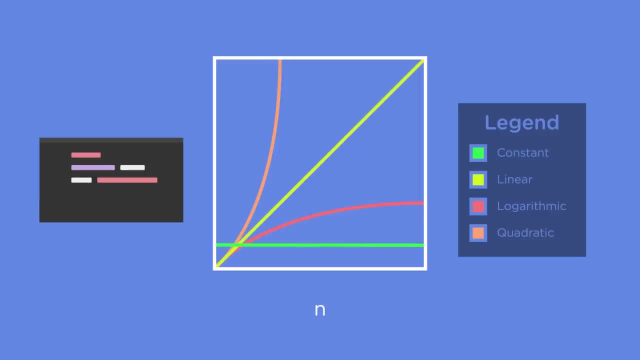 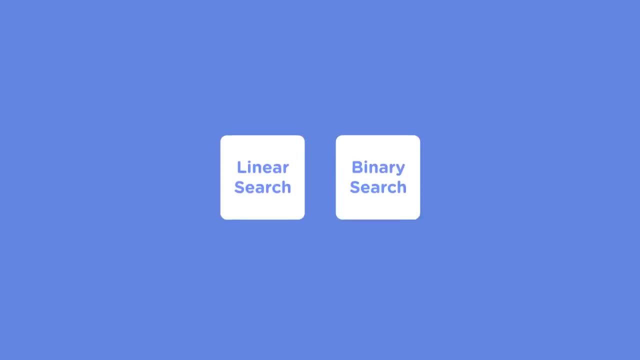 But in time You will immediately be able to distinguish the run time of an algorithm Based on the code you write And have an understanding of where it sits on an efficiency scale. You will also, In due time, Internalize run times of popular algorithms. 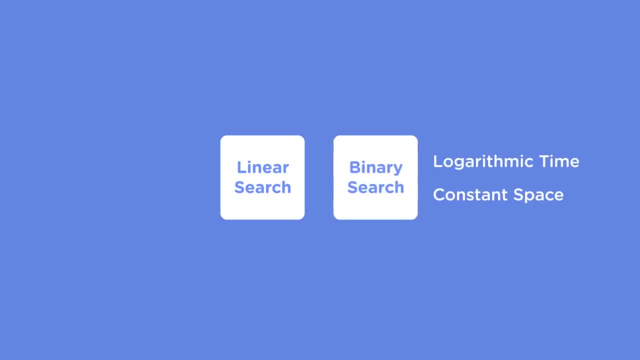 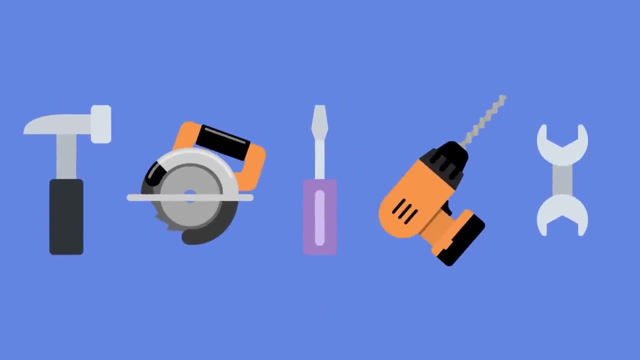 Like the fact that binary search runs in logarithmic time And constant space, And be able to recommend alternative algorithms For a given problem. All in all, The number of tools in your tool belt will increase Now. next, We learned about two important search algorithms. 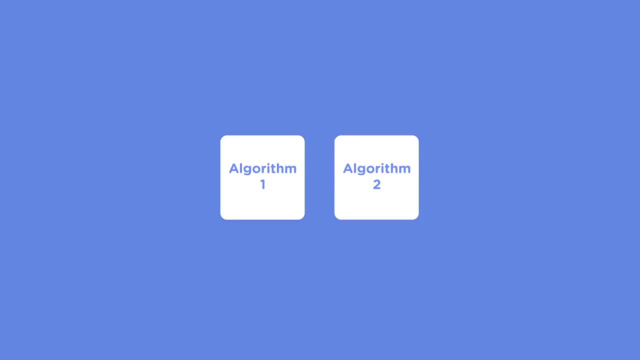 And the situations in which we select One over the other. We also implemented these algorithms in code So that you got a chance to see them work. We did this in Python, But if you are more familiar with a different language And haven't gotten the chance, 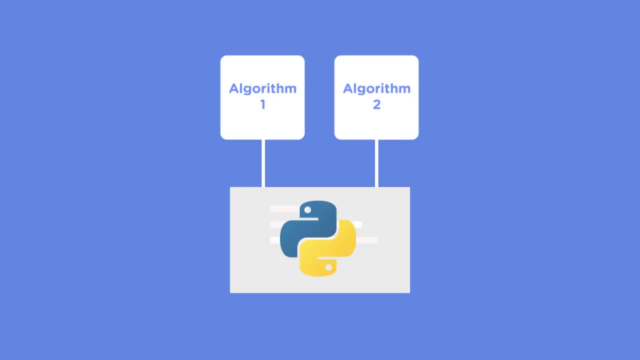 To check out the code snippets we've provided. You should try your hand At implementing it yourself. It's a really good exercise to go through. Finally, An important concept And a way of writing algorithmic code Through recursion. Recursion is a tricky thing. 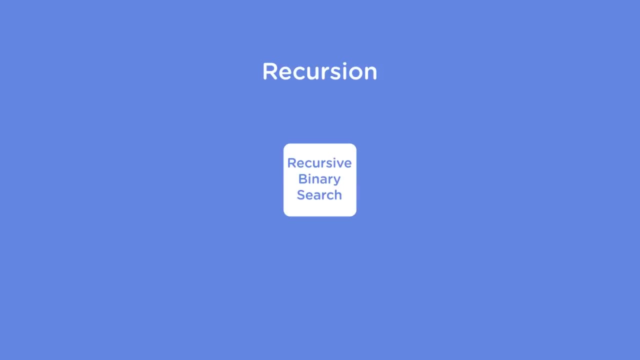 And, depending on the language you write code with, You may run into it more than others. It is also good to be aware of Because, as we saw in our implementation of binary search, Whether recursion was used or not Affected the amount of space we used. 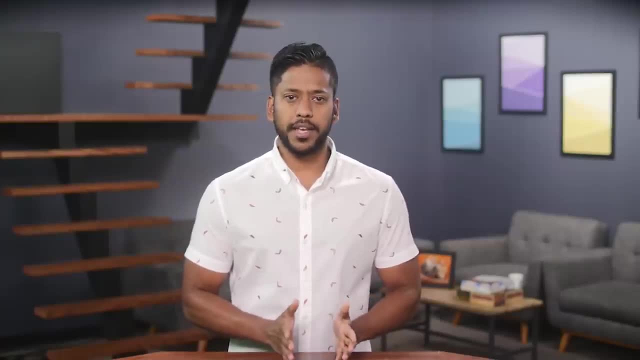 Don't worry If you don't fully understand How to write recursive functions- I don't truly know either. The good part is You can pick it up And understand how other people do it Anytime you encounter recursion In our courses. moving forward, 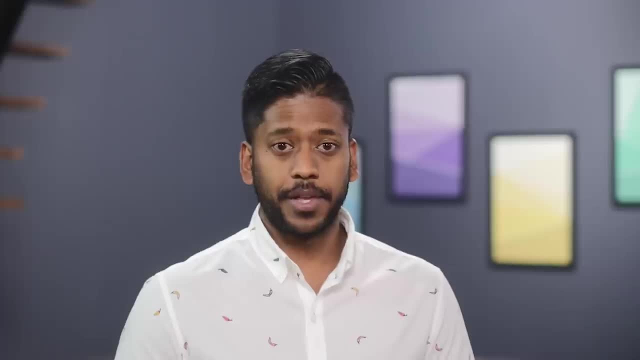 You'll get a full explanation Of how and why the function is doing What it's doing. And that brings us to the end of this course. I'll stress again That the goal of this course Was to get you prepared For learning about more specific algorithms. 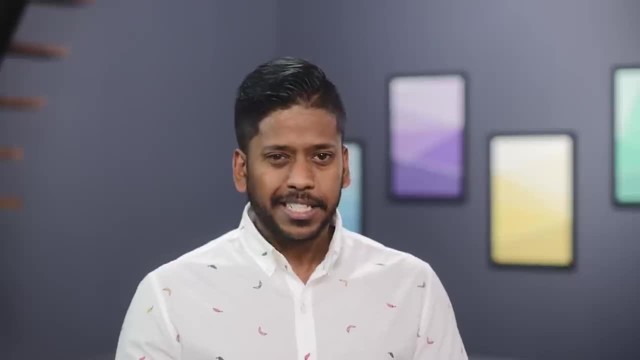 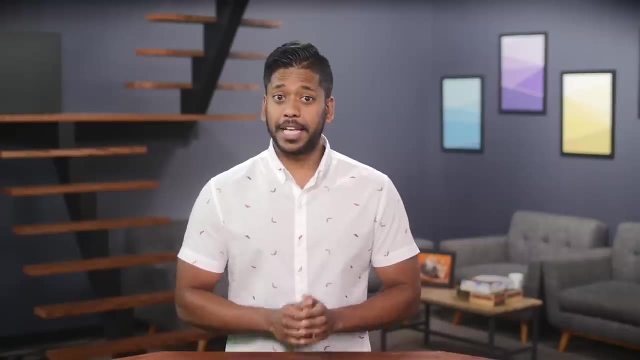 By introducing you to some of the tools And concepts you will need moving forward. So if you're sitting there thinking Algorithmic thinking, That's okay, We'll get there. Just stick with it. As always, have fun and happy coding. 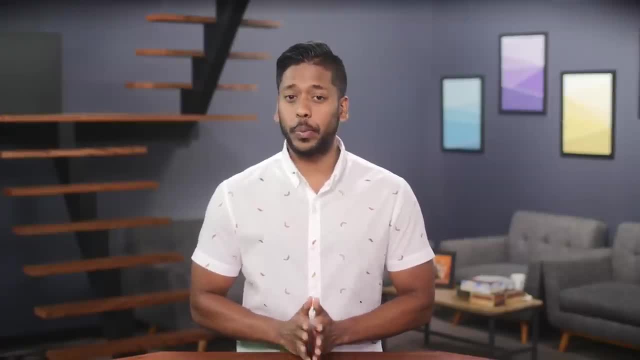 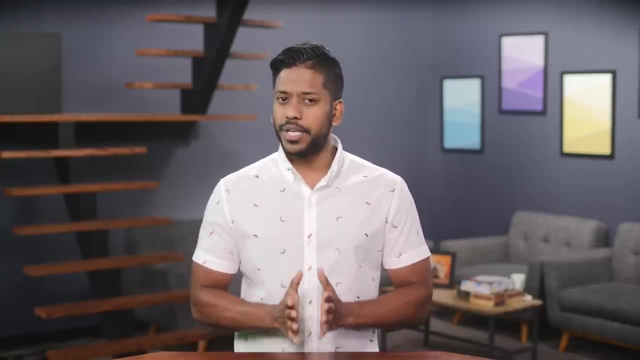 Hi, my name is Pasan, I'm an instructor at Treehouse And welcome to the introduction to data structures course. In this course, We're going to answer one fundamental question: Why do we need more data structures Than a programming language provides? 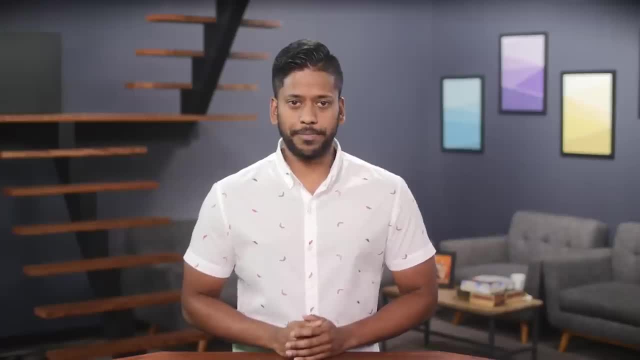 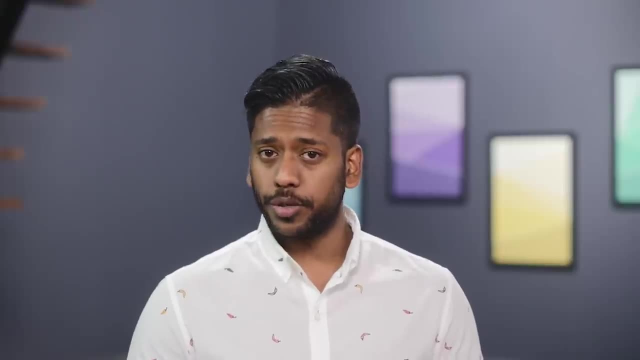 Before we answer that question, Some housekeeping, if you will. In this course We're going to rely on concepts We learned in the introduction to algorithms course, Namely big O, notation, Space and time, complexity And recursion. If you're unfamiliar with those concepts, 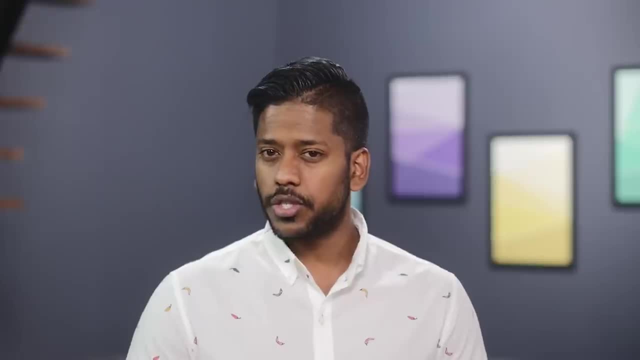 Or just need a refresher? Check out the prerequisites courses listed. In addition, this course does assume That you have some programming experience. We're going to use data structures In primarily all programming languages As our point of reference, While we will explain the basics. 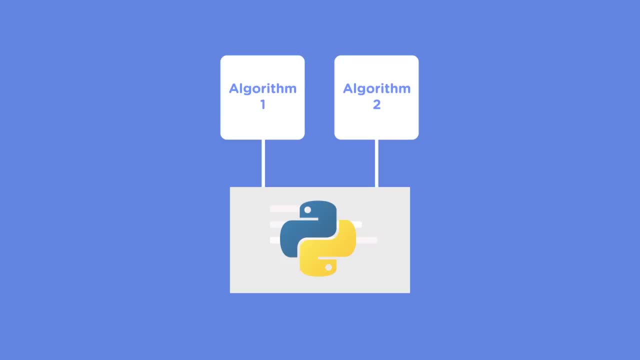 you go to that location and you find an item along with the location to the next item of treasure. when you finally find an item that doesn't also include a location, you know that the hunt has ended. now that we have a high level view of what a linked 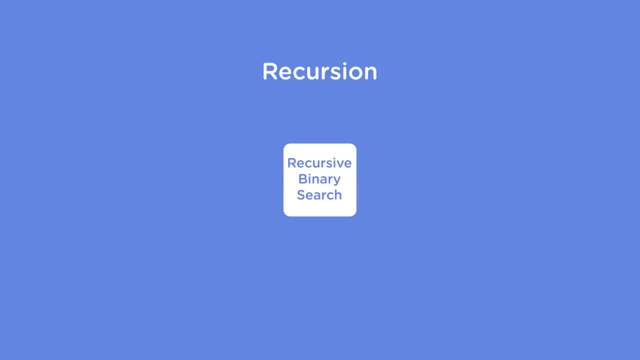 list is. let's jump into code and build one together. we'll focus on building a singly linked list for this course. there are advantages to having a doubly linked list, but we don't want to get ahead of ourselves. let's start here by creating a new file. 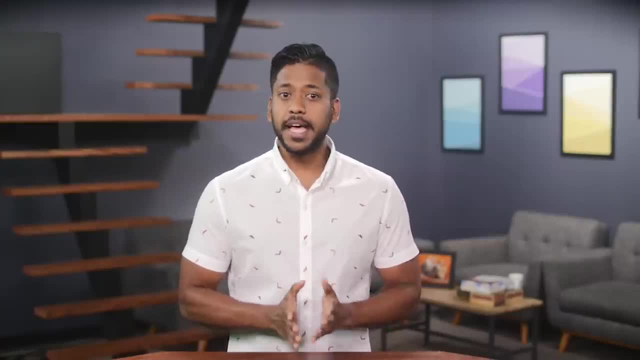 where we're going to put all our code for our linked list. so we'll call this linked underscore list dot pi. and first we're going to create a class to represent a node, say class node. now, node is a simple object in that it won't model much. 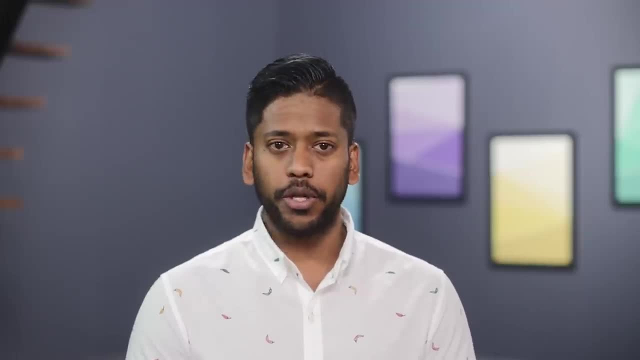 so first we'll add a data variable- it's an instance variable here called data- and we'll assign the value none initially, and then we'll add one more. we'll call this next node and to this we'll assign none as well. so we've created two instance. 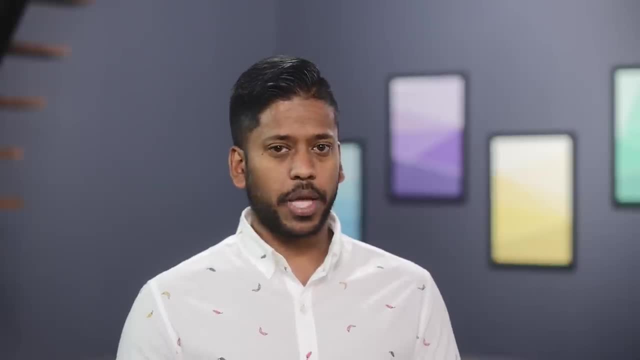 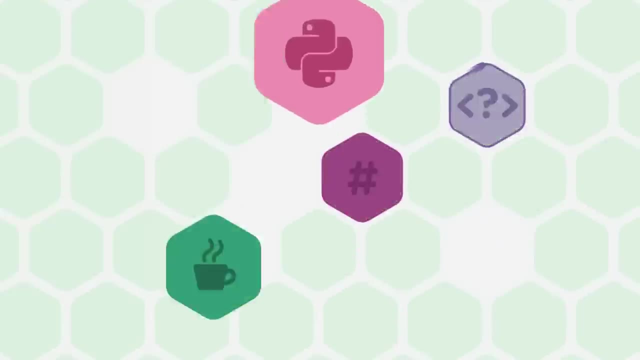 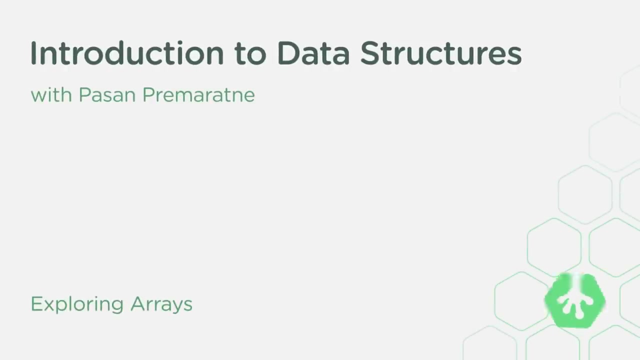 variables: data to hold on to the data that we're storing, and next node to point to the next node in the list. now we need to add a constructor to make this class easy to create, so we'll add an init method here that takes self and some data. 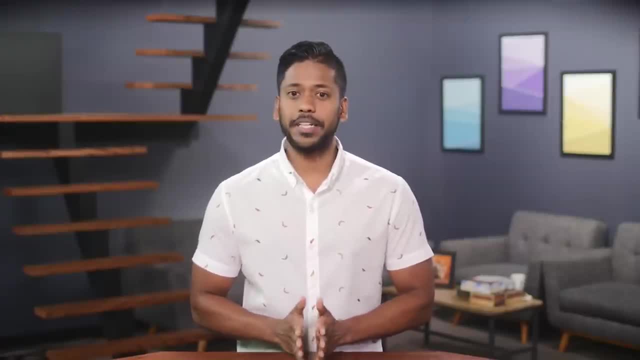 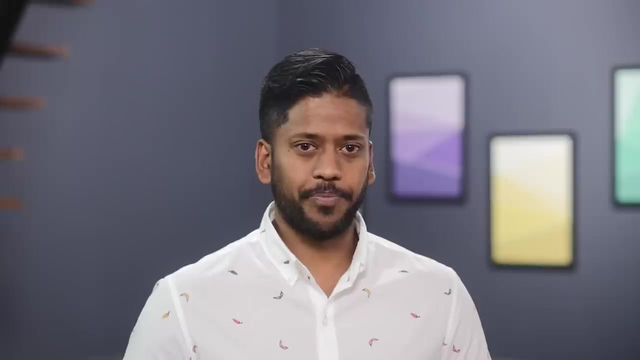 to start off, and all we're going to do is assign data to that instance variable we created. so that's all we need to model node. before we do anything else, though, let's document this. so, right after the class definition, let's create a doc string. so three quotes. 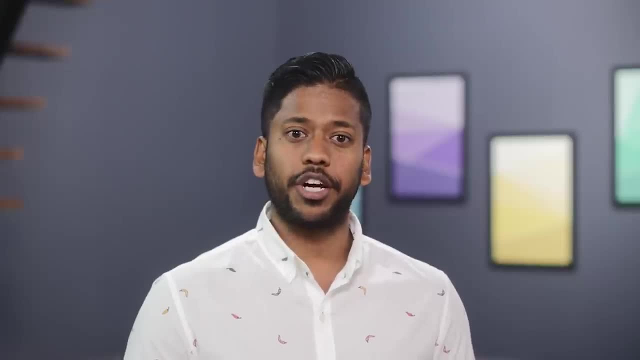 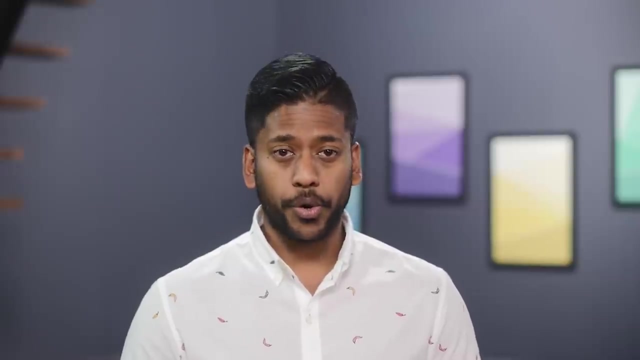 next line and we'll say an object for storing a single node of a linked list, and then on the next line we'll say models, two attributes, data and the link to the next node in the list, and then we'll close this doc string off with three more quotation marks. 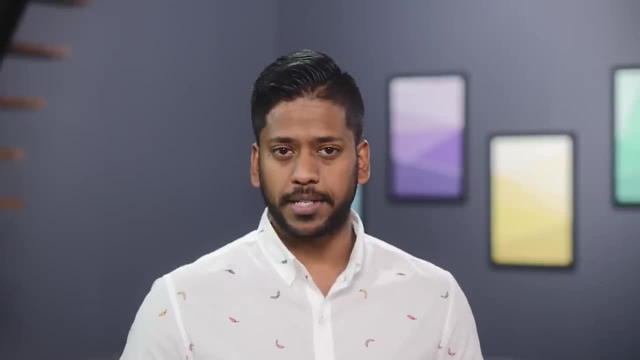 Of how these structures work. We won't be going over how to use them in practice. If you're looking to learn how to program Before digging into this content, Check the notes section of this video For helpful links. If you're good to go, then awesome. 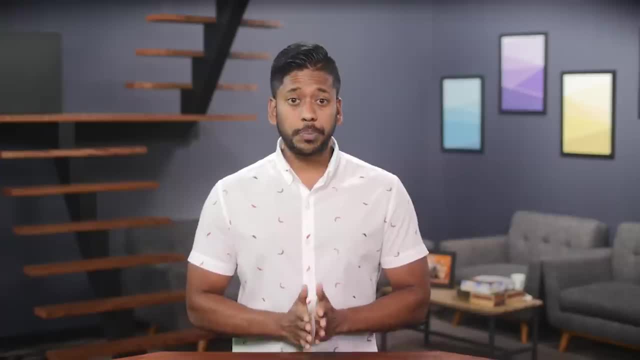 Let's start with an overview of this course. The first thing we're going to do Is to explore a data structure. We are somewhat already familiar with arrays. If you've written code before, You have used an array. In this course, we're going to spend some time. 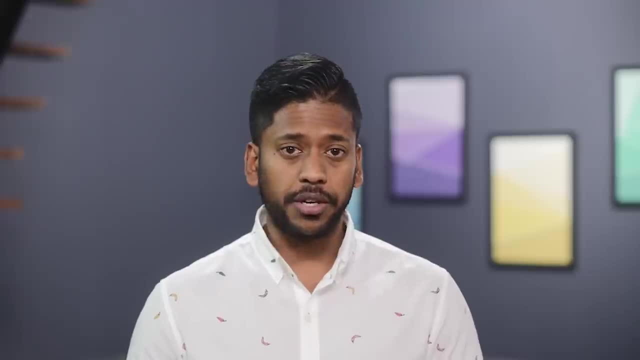 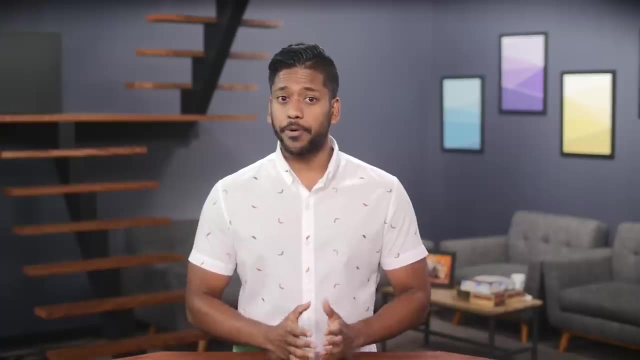 Understanding how arrays work, What are the common operations on an array And what are the run times associated With those operations. Once we've done that, We're going to build a data type of our own, Called a linked list. In doing so, we're going to learn. 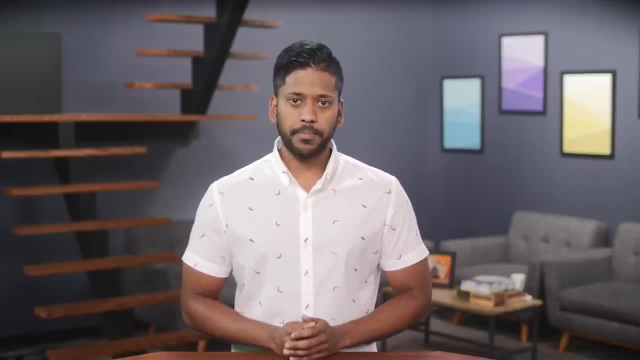 That there's more than one way to store data. In fact, there's way more than just one way. We're also going to explore What motivates us to build specific kinds of structures And look at the pros and cons Of these structures. 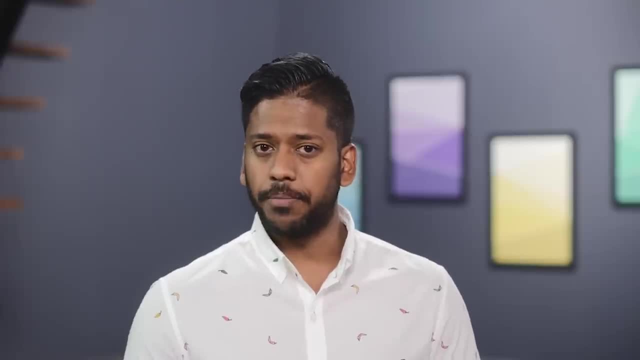 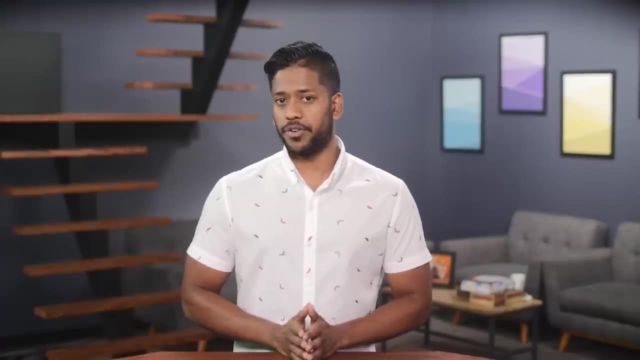 We'll do that by exploring four common operations: Accessing a value, Searching for a value, Inserting a value And deleting a value. After that, we're actually going to circle back to algorithms And implement a new one, A sorting algorithm. 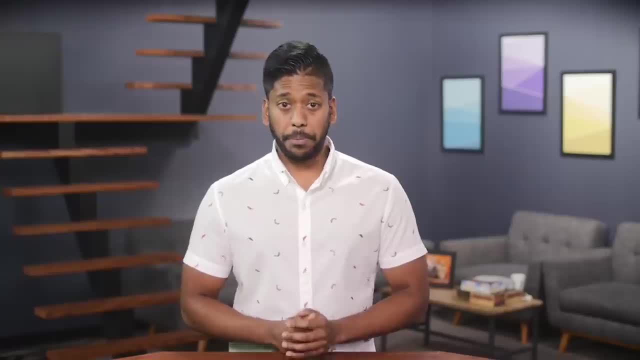 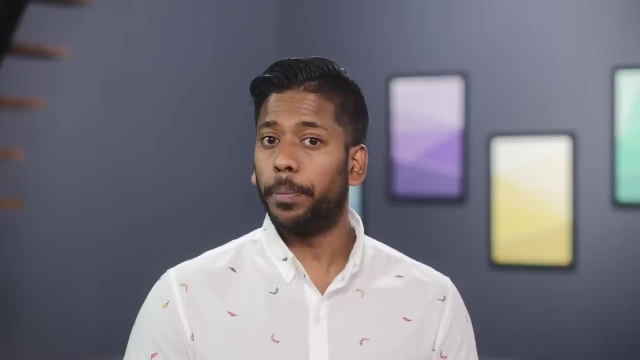 In the introductions to algorithms course, We implemented a binary search algorithm. A precondition to binary search Was that the list needed to be sorted. We're going to try our hand at sorting a list And open the door to an entirely new. 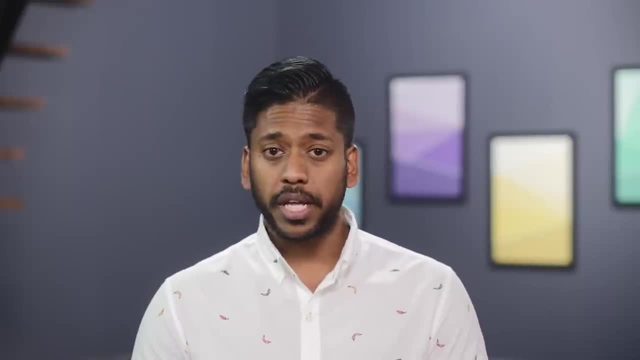 Category of algorithms. We're going to implement our sorting algorithm On two different data structures And explore how the implementation of one algorithm Can differ Based on the data structure being used. We'll also look at how the choice of data structure. 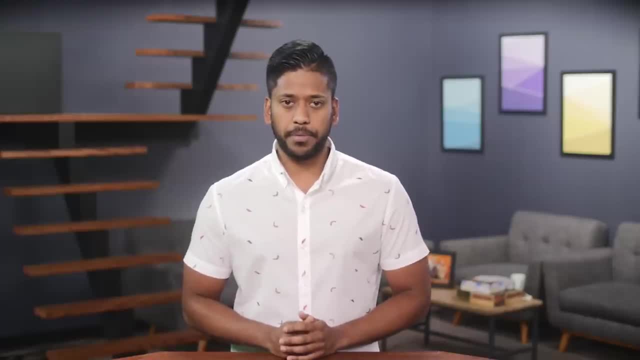 Potentially influences The run time of the algorithm. In learning about sorting, We're also going to encounter another general concept Of algorithmic thinking, Called divide and conquer, Along with recursion, Which will be a fundamental tool That we will use to solve complex problems. 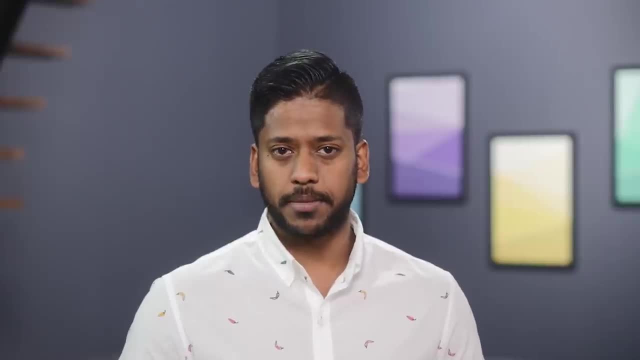 okay, using the node class is fairly straightforward, so we can create a new instance of node with some data to store. now, the way we're going to do this is we're going to bring up the console and we're going to type out like we've been typing out before. 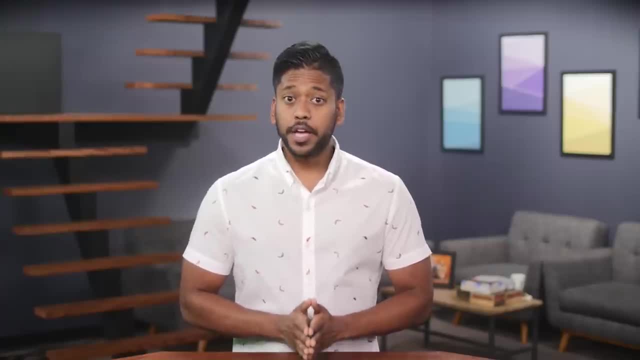 python, followed by the name of the script that we wrote which is linked list. linked underscore. list dot pi. but before we do that, we're going to pass an argument to the python command. we're going to say dash or python i, and then the name of the script linked underscore. 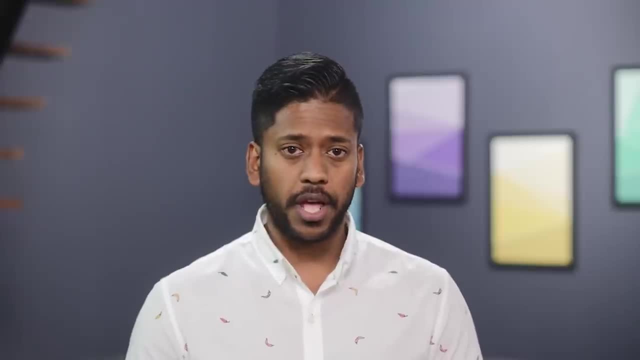 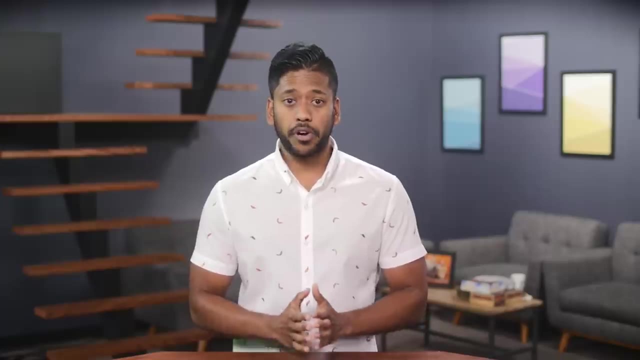 list dot pi. so what this does is this is going to run the python repl, the read evaluate print loop in the console, but it's going to load the contents of our file into that so that we can use it. so I'll hit enter and we have a new instance going. 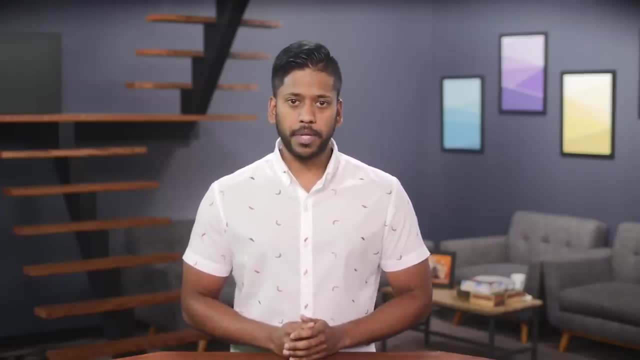 and now we can use the node in here, so we can say n1 equal node. and since we defined that constructor, we can pass it some data, so we'll say 10 here. now, if we try to inspect this object, the representation return isn't very useful. 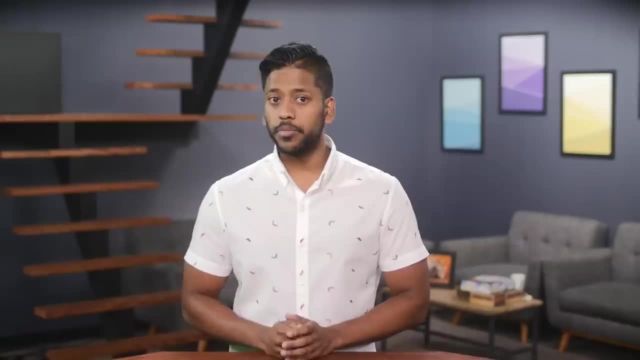 which will make things really hard to debug as our code grows. so, for example, if I type out n1, you'll see that we have a valid instance here, but it's not very helpful the way it's printed out. so we can customize this by adding a. 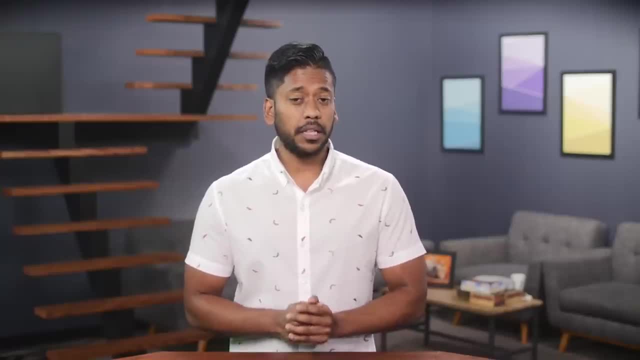 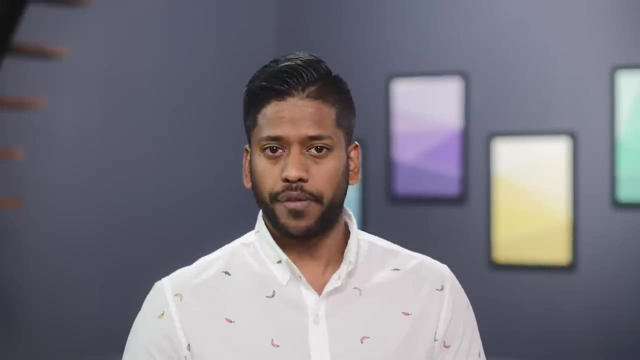 representation of the object using the repr function. now in the terminal, still, we'll type out exit like that: hit enter to exit the console. and then down here let's add in some room: ok, and here we'll say: def, double underscore, repr, another set of double underscores, and then this function. 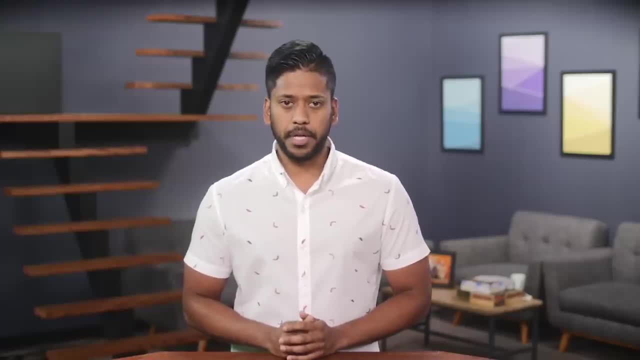 takes the argument self, and in here we can provide a string representation of what we want printed to the console when we inspect that object inside of it, inside of the console. so here we'll say: return again, this is a string representation. so inside quotes we'll say: 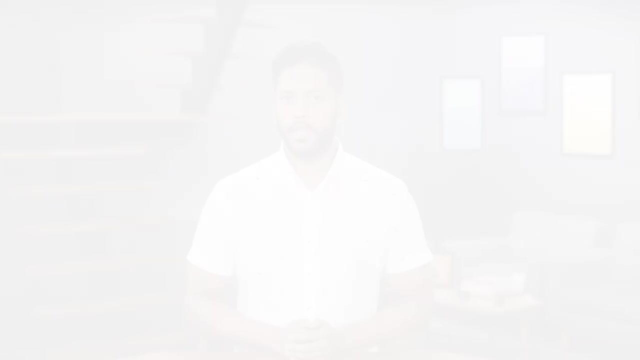 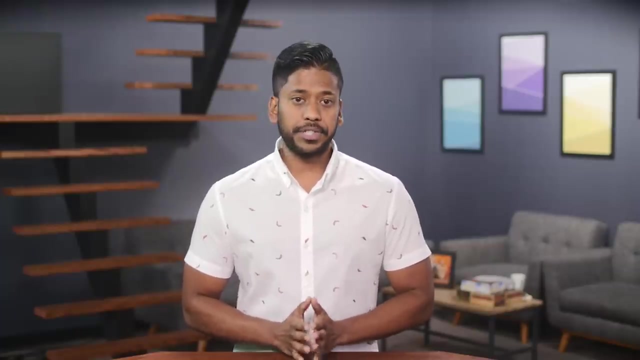 node. so this represents a node instance and the data it contains. here we'll say %s, which is a python way of substituting something into a string- string interpolation- and outside of the string we can say % again, and here we're saying we want to replace. 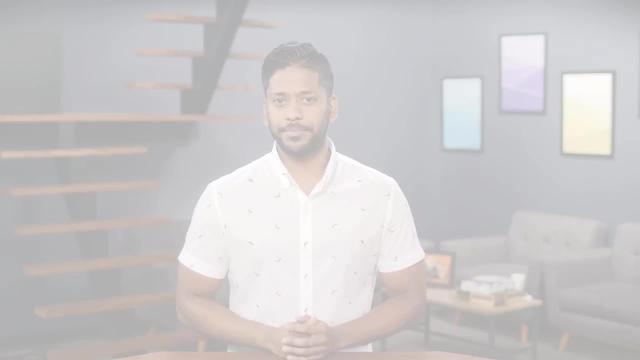 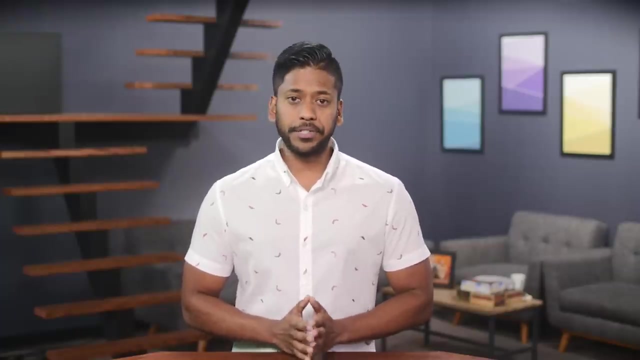 All in due time. In the next video, let's talk about arrays. A common data structure Built into nearly every programming language Is the array. Arrays are a fundamental data structure And can be used to represent a collection of values, But it is much more than that. 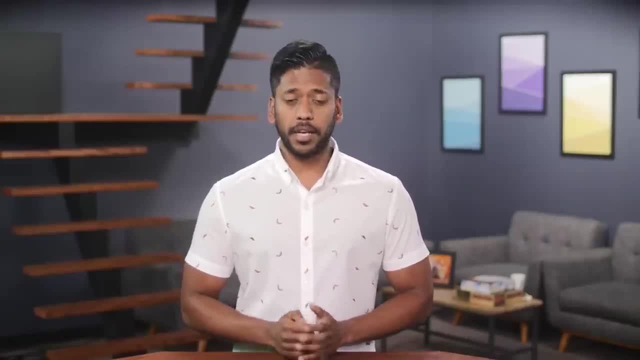 Arrays are also used as building blocks To create even more custom data types And structures. In fact, in most programming languages, Text is represented using the string type And under the hood, Strings are just a bunch of characters Stored in a particular order in an array. 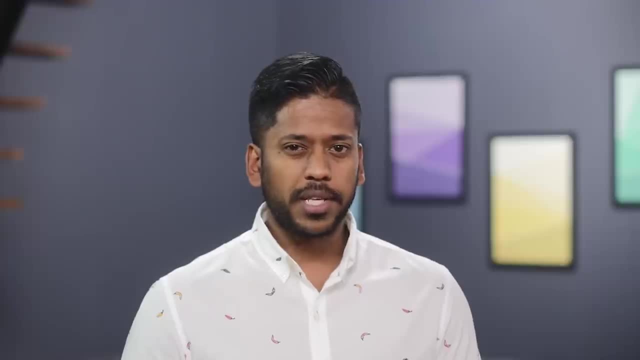 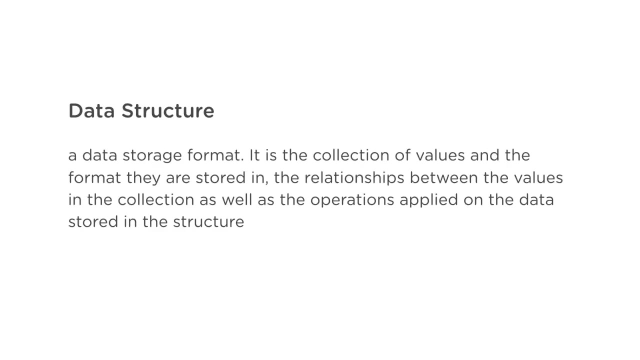 Before we go further And dig into arrays, What exactly is a data structure? A data structure is a way of storing data When programming. It's not just a collection of values And the format they're stored in, But the relationship between the values. 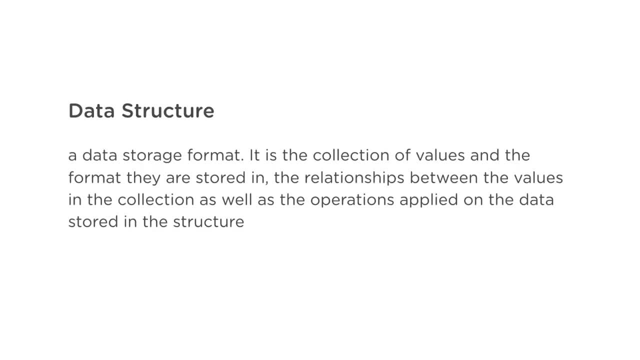 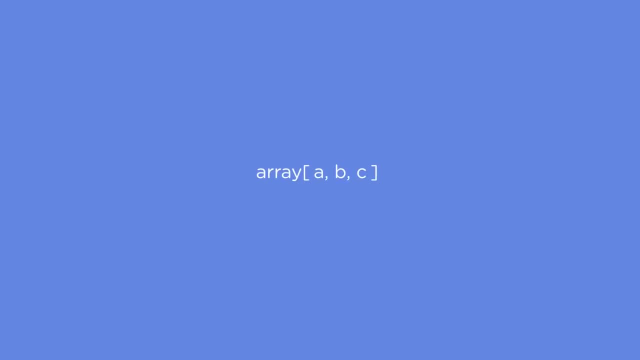 In the collection, As well as the operations applied on the data Stored in the structure. Arrays are one of very many data structures. In general, An array is a data structure That stores a collection of values, Where each value is referenced. 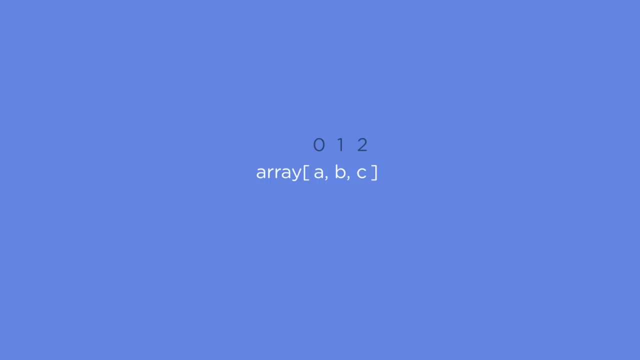 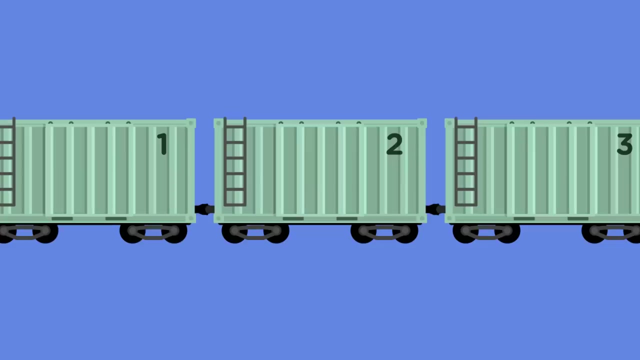 Using an index or a key. A common analogy for thinking about arrays Is as a set of train cars. Each car has a number And these cars are ordered sequentially Inside each car. The array or the train in this analogy Stores some data. 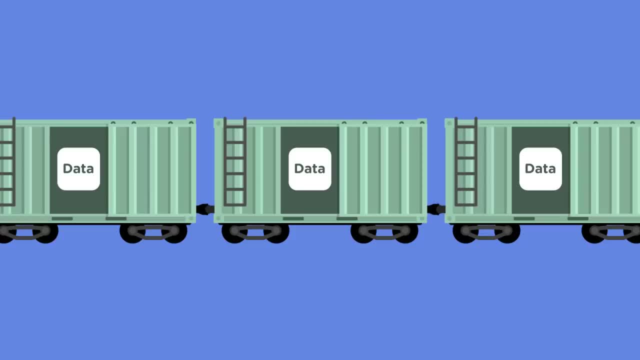 While this is the general representation Of an array, Slightly from one language to another, But for the most part, All these fundamentals remain the same. In a language like Swift or Java, Arrays are homogenous containers, Which means they can only contain values. 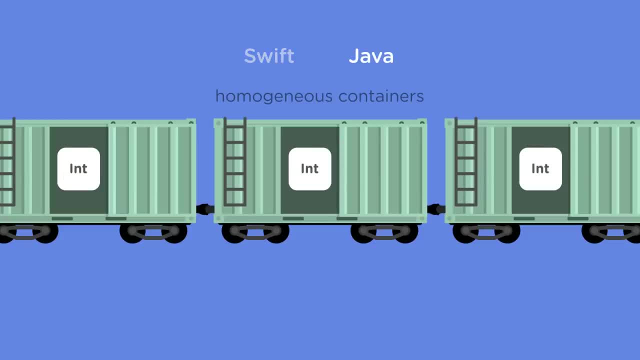 Of the same type. If you use an array to store integers in Java, It can only store integers In other languages. Arrays are heterogeneous structures That can store any kind of value. In Python, for example, You can mix numbers and text. 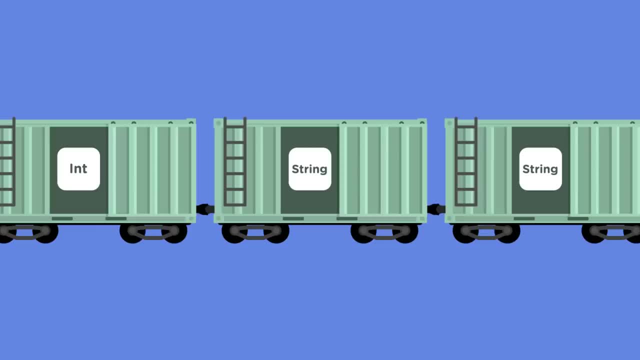 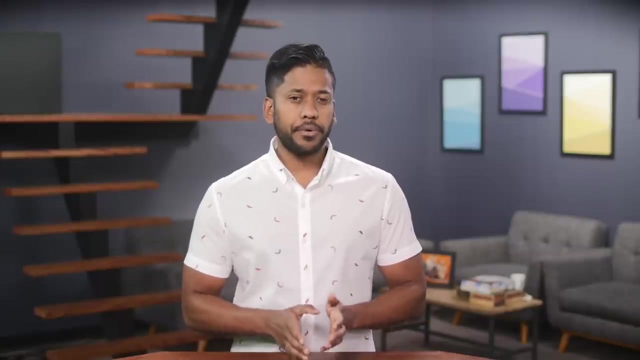 With no issues. Regardless of this nuance, The fundamental concept of an array Is the index. This index value is used for every operation on the array, From accessing values To inserting, updating and deleting In Python, The language we're going to be using for this course. 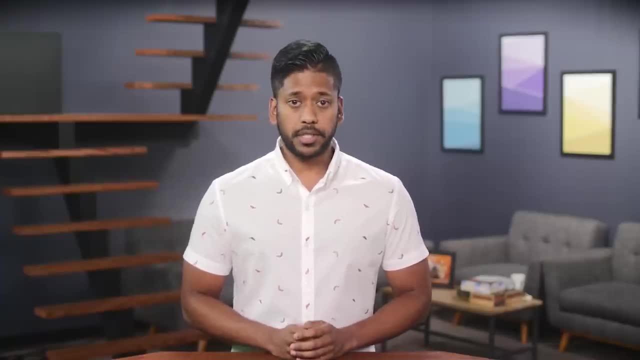 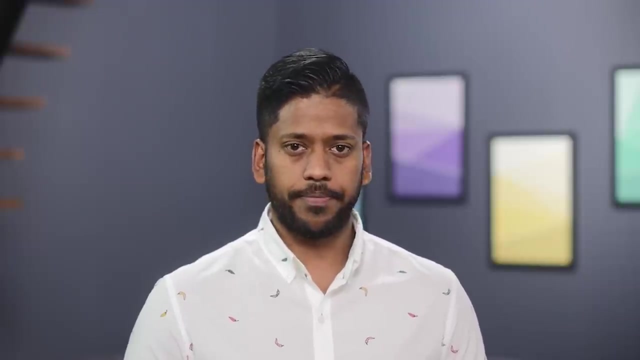 this %s with selfdata. ok, let's hit save and before we move on, let's verify that this works. so I'm going to come in here, type clear to get rid of everything, and then we'll do what we did again, and you can just hit the up arrow a couple times. 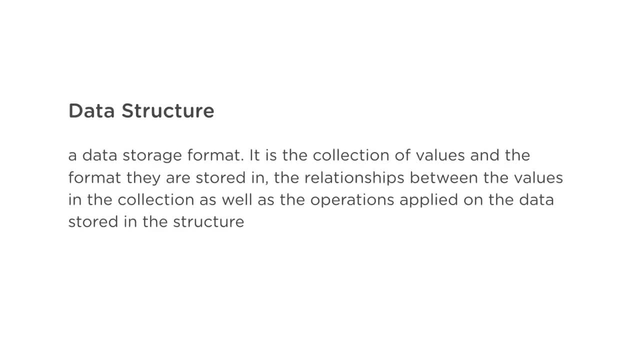 to get that command. alright. so hit enter. and now, just so you know, every time you run this you start off. you know from scratch. so n1 that we created earlier not there anymore, so let's go ahead and create it. n1 equal node 10 and we can type. 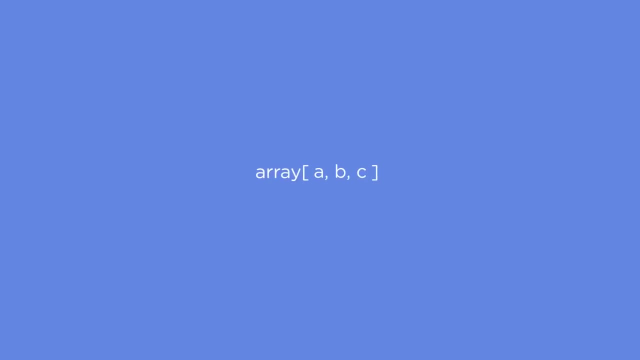 n1 again and hit enter and you have a much better representation now. so we can see that we have a node and it contains the data 10. we can also create another one n2 equal node that contains the data 20, and now we can say n1- dot- next node. 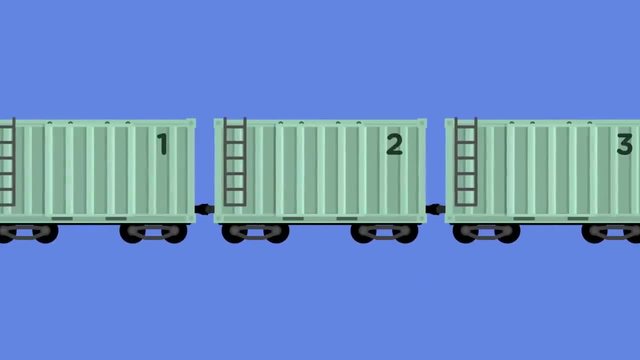 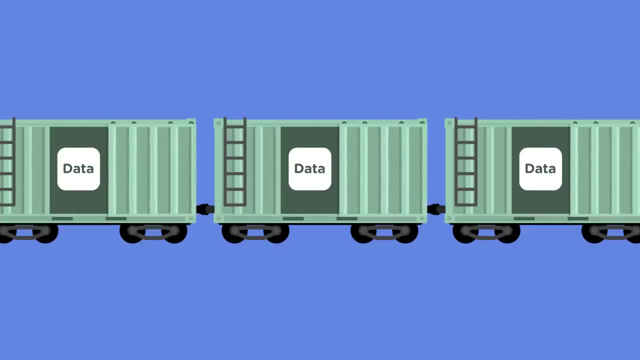 equal n2. so n1 now points to n2 and if we say n1 dot next node, you'll see that it points to that node. the node containing 20 nodes are the building blocks for a list and now that we have a node object, we can use it to create. 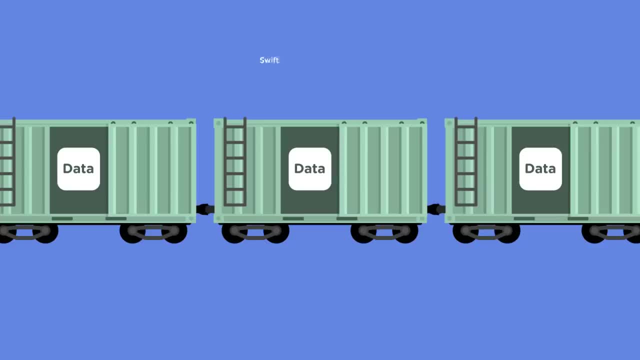 a singly linked list. so again, I'm going to exit out of this and then go back to the text editor and here we'll create a new class. so class linked list. the linked list class is going to define a head and this attribute models the only node. 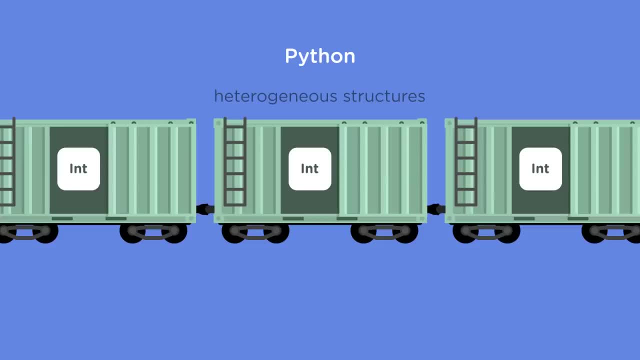 that the list is going to have a reference to. so here we'll say head and we'll assign none initially, and then, like we did earlier, let's create a constructor. so double underscore, init, double underscore. this takes self, and then inside, like before, we'll say self, dot head. 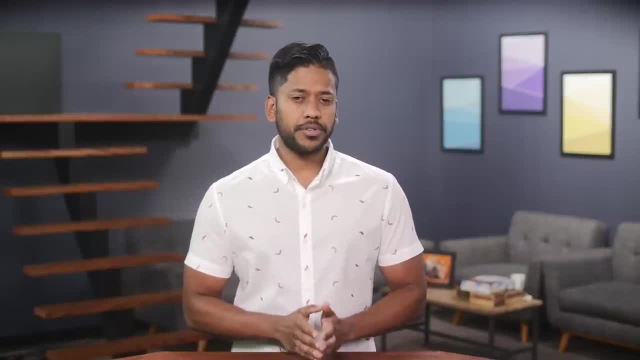 equal none. this is the same as doing this, so we can actually get rid of that and just use the constructor. ok, so again, this head attribute models the only node that the list will have a reference to, since every node points to the next node to find a particular 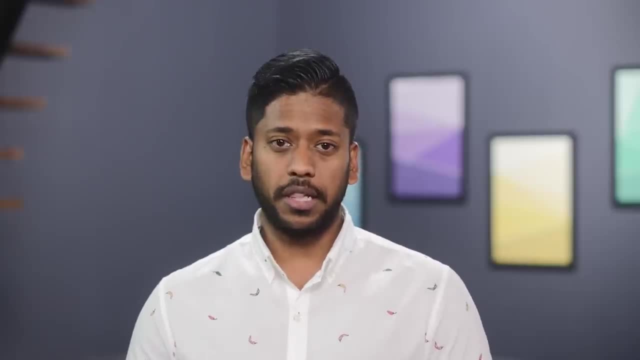 node. we can go from one node to the next in a process called list traversal. so in the class constructor here we've set the default value of head to none, so that new lists created are always empty again. you'll notice here that I didn't explicitly declare the head. 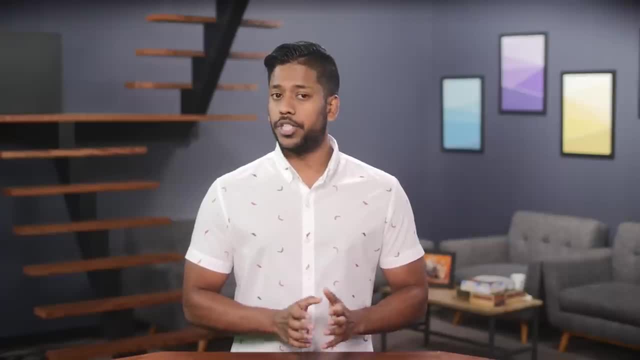 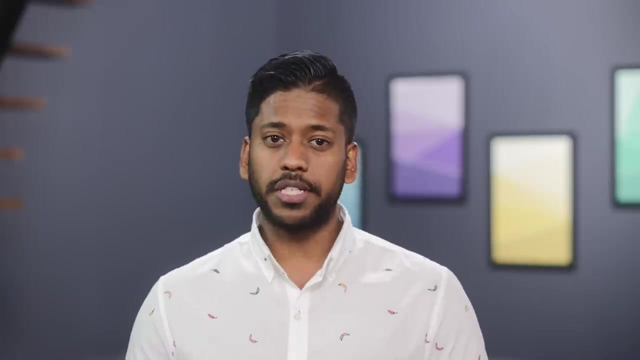 It's a tiny bit confusing. The type that we generally refer to As an array in most languages Is best represented By the list type in Python. Python does have a type called Array as well, But it's something different, So we're not going to use it. 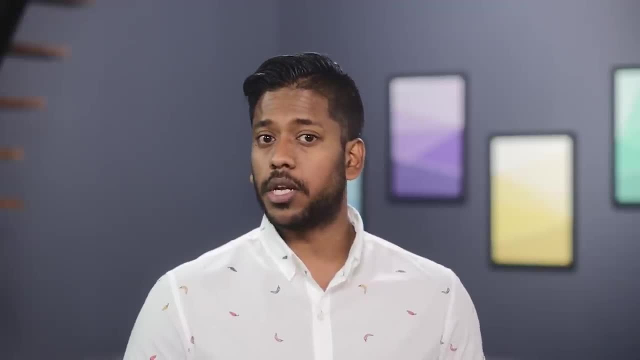 While Python calls it a list. When we use a list in this course, We'll be talking about concepts That apply to arrays as well In other languages, So definitely don't skip any of this. There's one more thing In computer science. 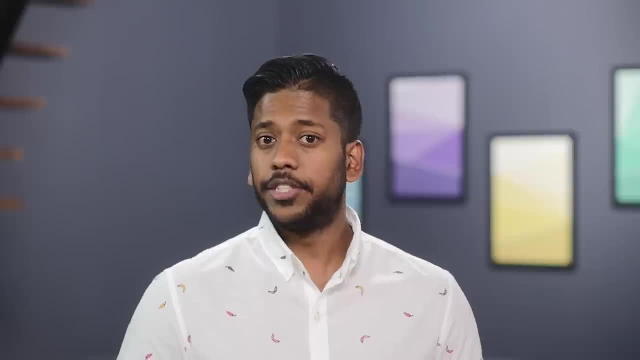 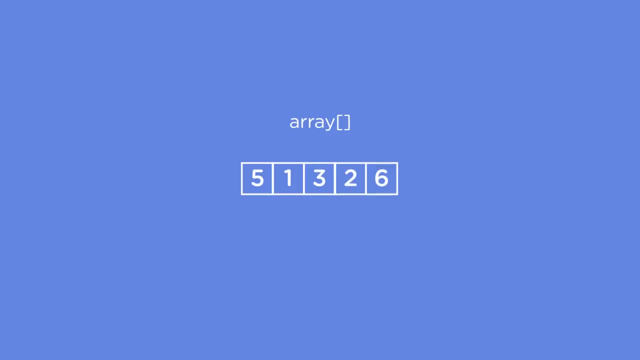 A list is actually a different data structure Than an array, And in fact we're going to build a list Later on in this course, So hopefully the terminology Isn't too confusing. To properly understand How arrays work, Let's take a peek at how arrays. 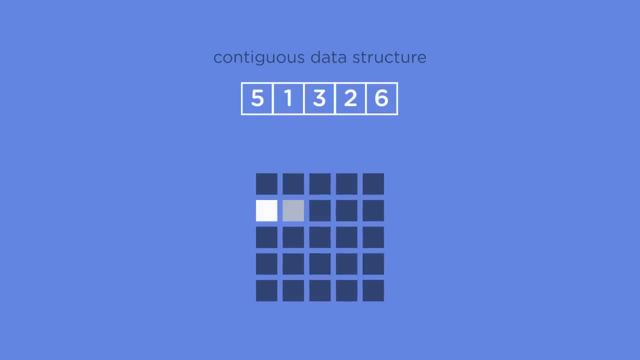 Are stored under the hood. An array is a contiguous data structure. This means that the array Is stored in blocks of memory That are right beside each other With no gaps. The advantage of doing this Is that retrieving values is very easy. 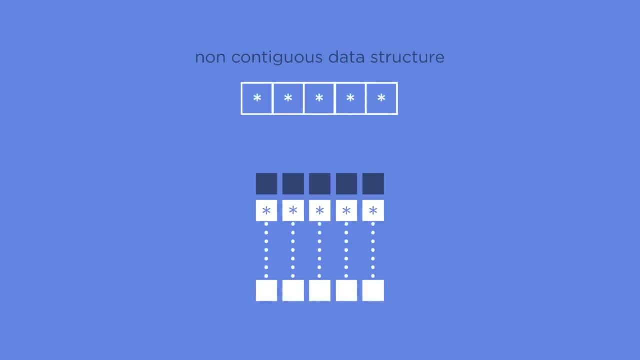 In a non-contiguous data structure. We're going to build one soon- A reference to where the next value is. To retrieve that next value, The language has to follow that reference, Also called a pointer To the next block of memory. 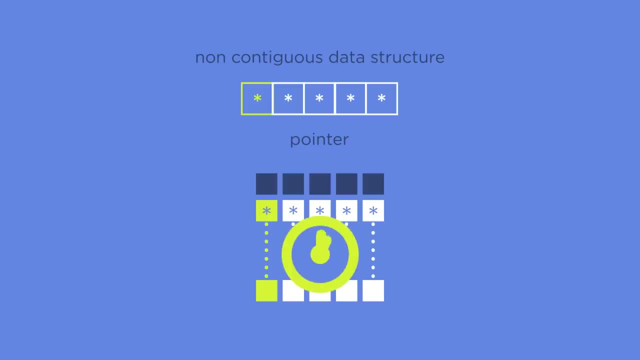 This adds some overhead Which, as you will see, Increases the runtime of common operations. A second ago I mentioned that, depending on the language, Arrays can either be homogenous, Containing the same type of value, Or heterogeneous, Where any kind of value can be mixed. 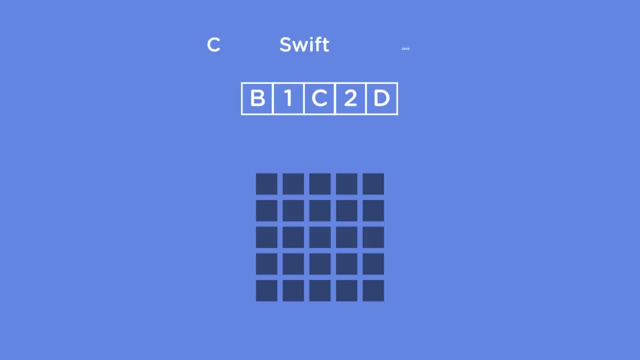 This choice also affects the memory layout. For example, In a language like C, Swift or Java, Where arrays are homogenous. When an array is created, Since the kind of value Is known to the language compiler, And you can think of the compiler. 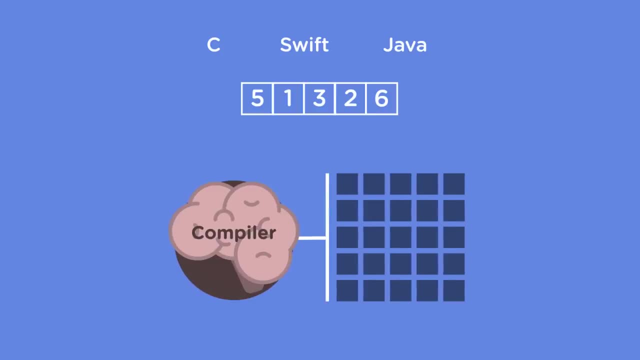 As the brains behind the language. It can choose a contiguous block of memory That fits the array size And values created. If the values were integers, Assuming an integer took up space Represented by one of these blocks, Then for a five item array, 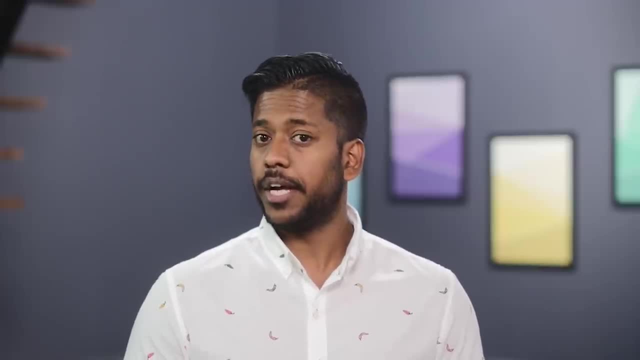 attribute at the top of the class definition- and don't worry, that's not an oversight- the self dot head in the initializer means that it's still created. ok, so that's all there is to modeling a linked list. now we can add methods that make it easier to use this data structure. 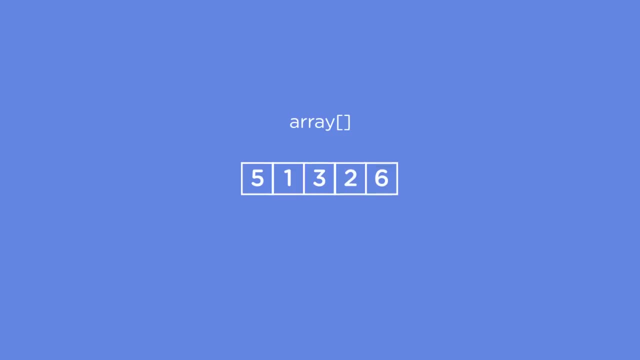 first a really simple doc string to provide some information. so here we'll create a doc string, three quotation marks, and then we'll say singly linked list and then close it off. a common operation carried out on data structures is checking whether it contains any data or whether it's. 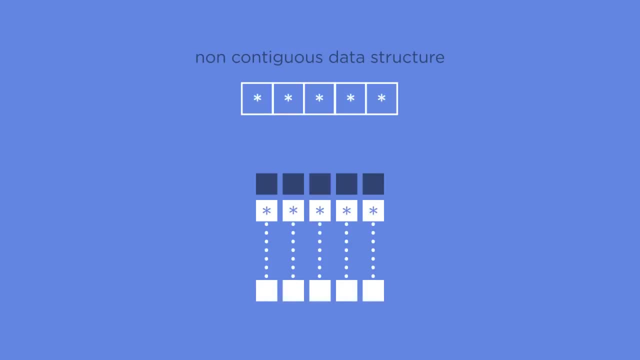 empty at the moment. to check if a list is empty, we would need to query these instance variables, head and so on every time. ideally, we would like to not expose the inner workings of our data structure to code that uses it. instead, let's make this operation more explicit. 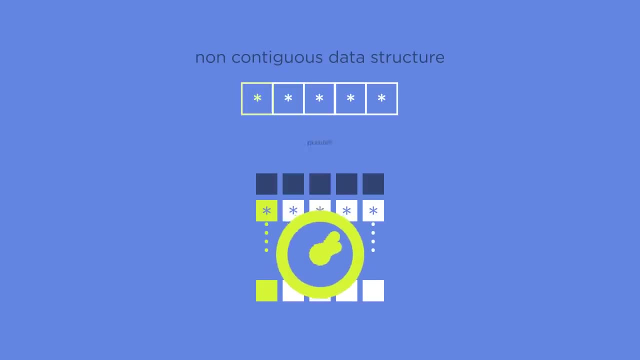 by defining a method. so we'll say def is empty and this method takes self as an argument, and here we'll say: return self dot head double equal none. all we're doing here is checking to see if head is none. if it is, this condition evaluates to true, which indicates the list is. 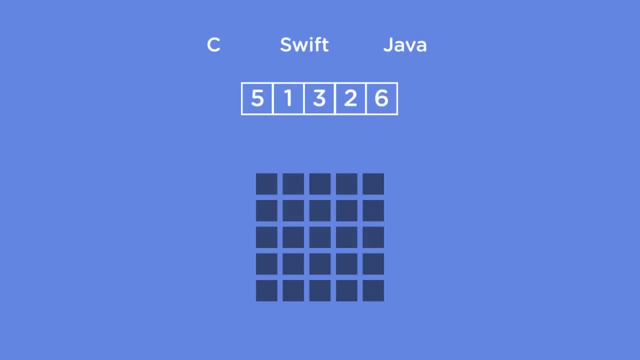 empty. now, before we end this video, let's add one more convenience method to calculate the size of our list. the name convenience method indicates that what this method is doing is not providing any additional functionality that our data structure can't handle right now, but instead making existing functionality. 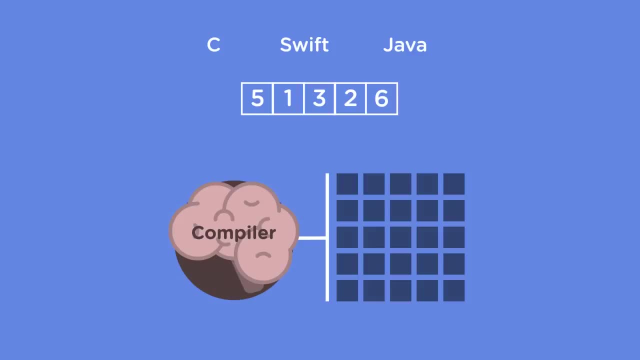 easier to use. we could calculate the size of our linked list by traversing it every time, using a loop, until we hit a tail node, but doing that every time is a hassle. okay, so we'll call this method size and, as always, it takes self, unlike calling len on a python. 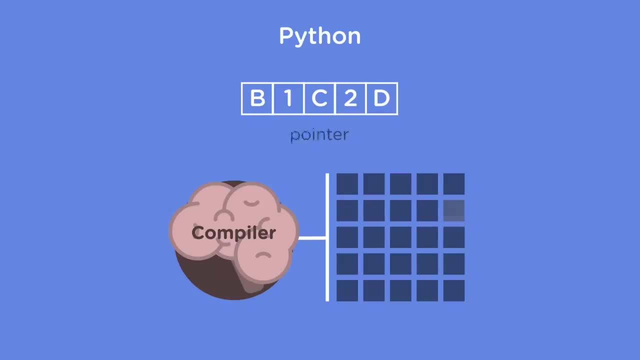 list not to be confused with a linked list, which is a constant time operation. our size operation is going to run in linear time. the only way we can count how many items we have is to visit each node and call next until we hit the tail node. so we'll start by getting a reference. 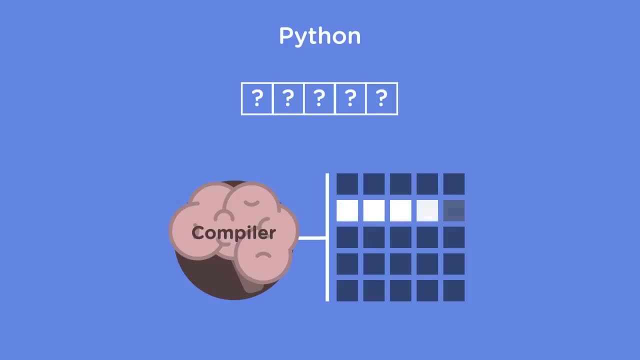 to the head we'll say current equal self dot head. let's also define a local variable named count, with an initial value of zero that will increment every time we visit a node. once we hit the tail, count will reflect the size of that list. next we'll define a while. 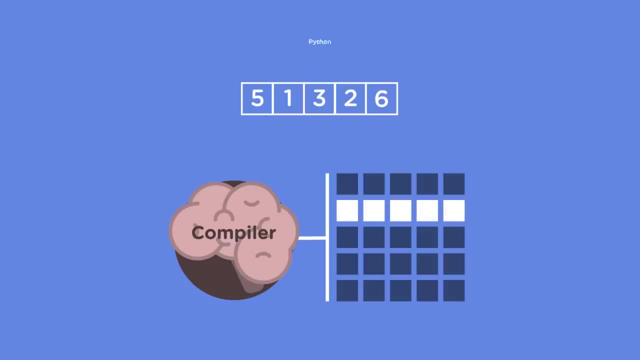 Five blocks of equally sized memory In Python. however, This is not the case. We can put any value in a Python list. There is no restriction. The way this works Is a combination of contiguous memory And the pointers or references I mentioned earlier. 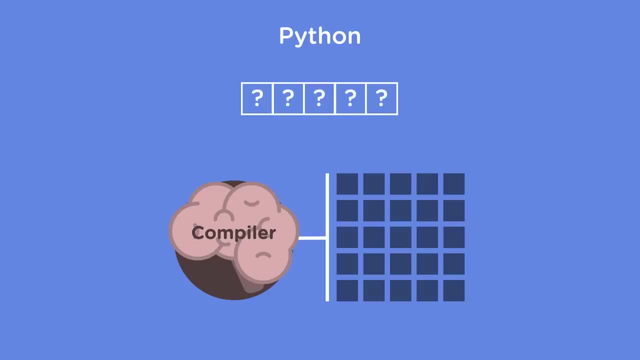 When we create a list in Python, There is no information About what will go into that array, Which makes it hard to allocate contiguous memory Of the same size. There are several advantages, Since the values are stored beside each other. Accessing the values. 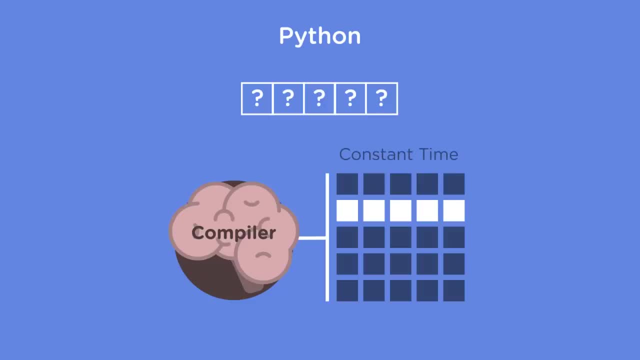 Happens in almost constant time, So this is a characteristic We want to preserve. The way Python gets around this Is by allocating contiguous memory And storing in it Not the value we want to store, But a reference or a pointer to the value. 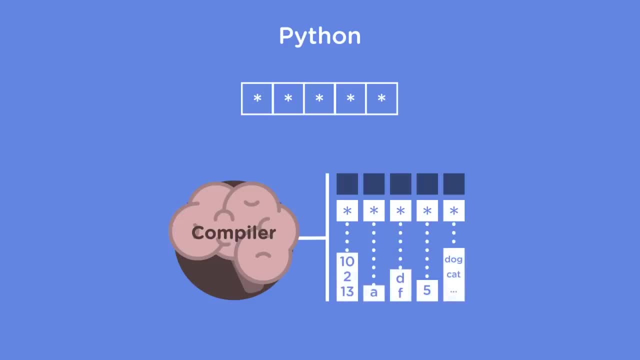 That's stored somewhere else in memory. By doing this, It can allocate equally sized contiguous memory, Since, regardless of the value size, The size of the pointer To that value Is always going to be equal. This incurs an additional cost. 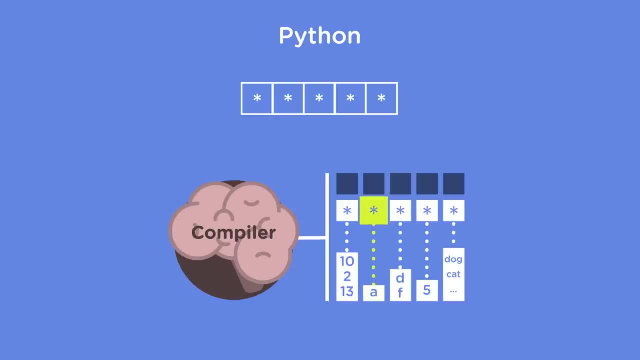 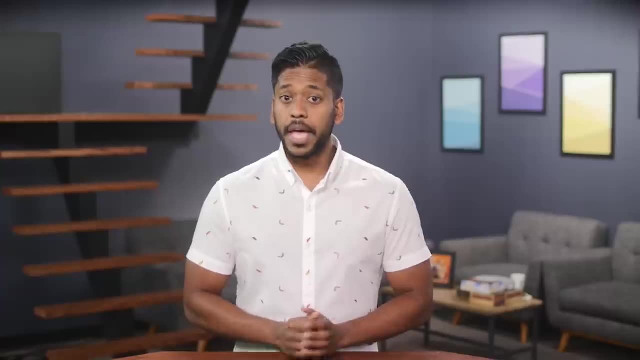 In that when a value is accessed, We need to follow the pointer To the block of memory Where the value is actually stored. But Python has ways of dealing with these costs That are outside the scope of this course. Now that we know. 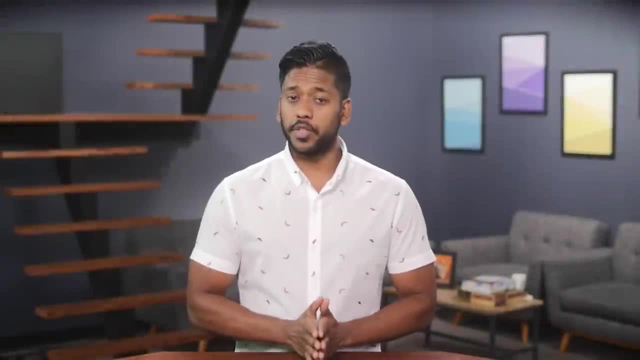 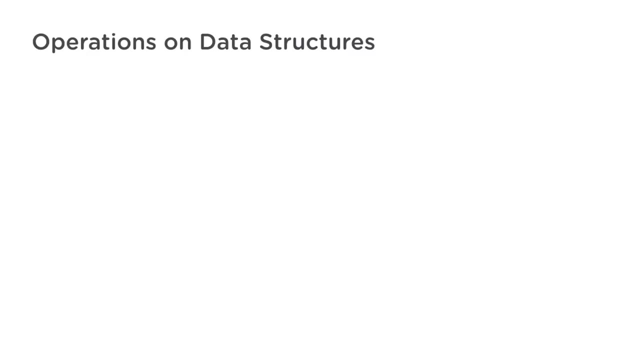 How an array stores its values. Let's look at common operations That we execute on an array. Regardless of the kind of data structure You work with, We need to be able to access And read values stored in the structure. We need to be able to search. 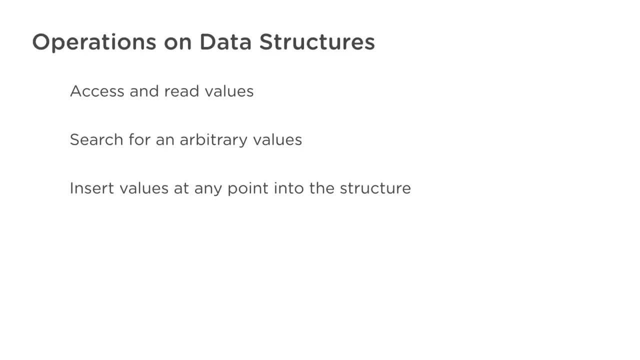 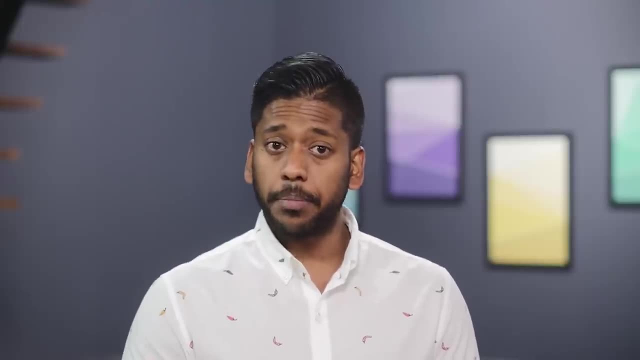 For an arbitrary value. We also need to be able to insert a value At any point into the structure And, finally, we need to be able to delete structures. Let's look at how these operations Are implemented on the array structure In some detail, starting with access. 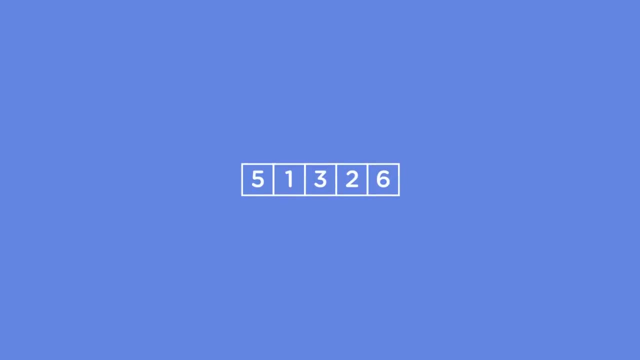 Elements in an array Are identified using a value Known as an index, And we use this index to access And read the value. Most programming languages Follow a zero based numbering system When it comes to arrays, And all this means. 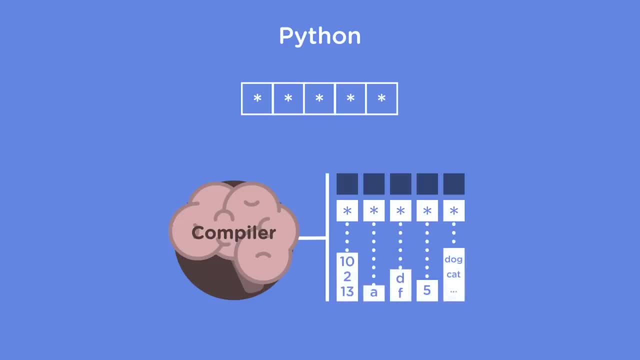 loop that will keep going until there are no more nodes. so we'll say while current. while current is the same as writing out. while current does not equal none, but it's more succinct, so we'll go with this former if the latter is more precise for you. 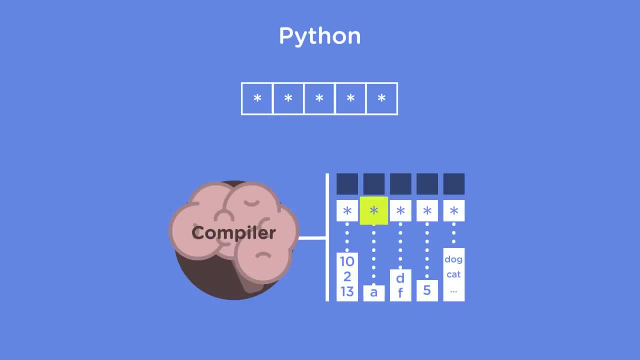 you can go with that. now, inside this loop we'll increment the count value. so count plus equal, one plus equal- if you haven't encountered it before- is the same as writing count equal, count plus one. so if count is zero initially, zero plus one is one and then. 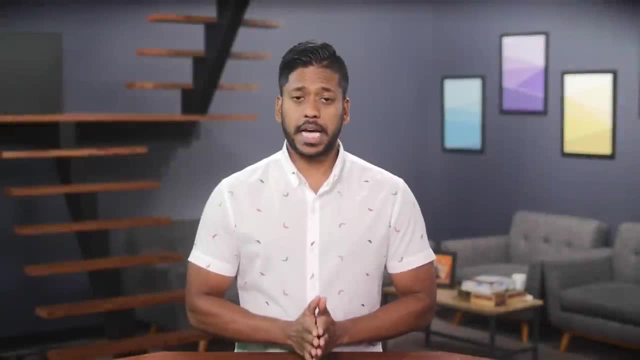 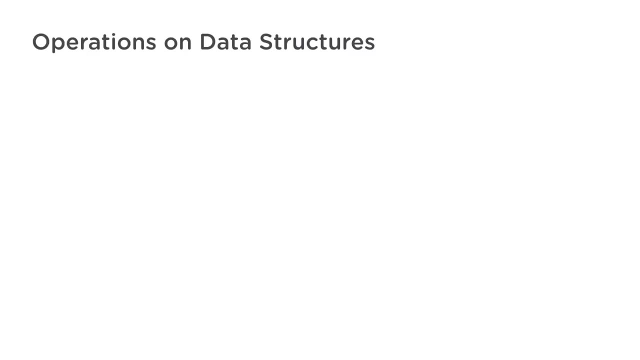 we'll assign that back to count. okay, so count plus equal one. next, we're going to assign the next node in the list to current. so current equal current dot next node. this way, once we get to the tail and call next node, current will equal none and the while. 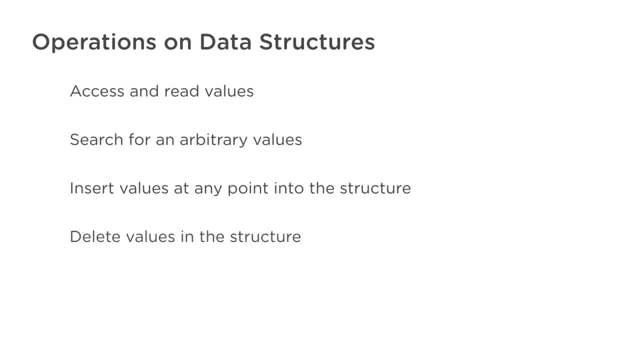 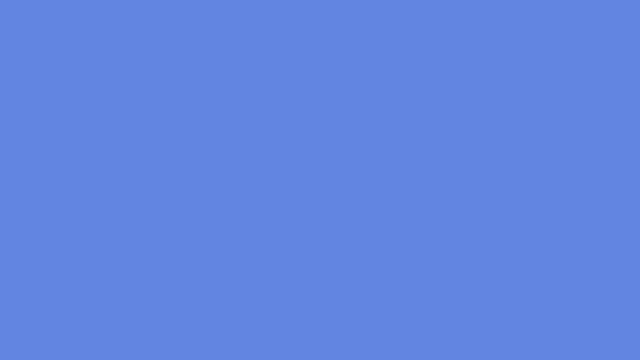 loop terminates, so at the end we can return count. as you can see, we need to visit every node to determine the size, meaning our algorithm runs in linear time. so let's document this up in our doc string, which we'll add now to size, we'll say: 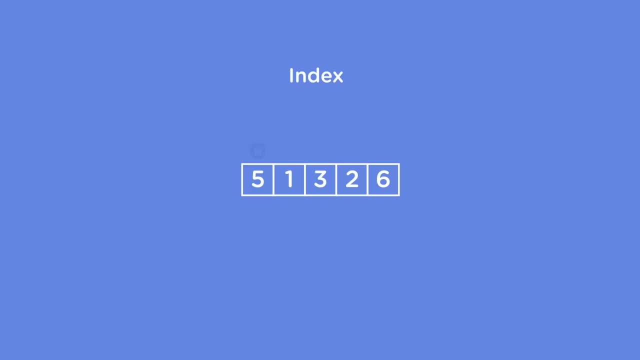 returns the number of nodes in the list takes linear time. let's take a break here. we can now create lists, check if they're empty and check the size. in the next video, let's start implementing some common operations. at the moment, we can create an empty list, but nothing else. 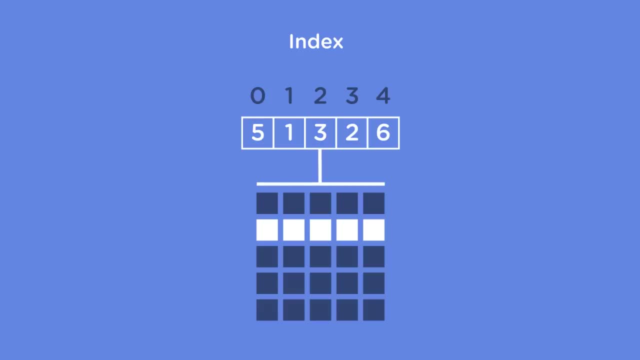 let's define a method to add data to our list. technically speaking, there are three ways we can add data to a list. we can add nodes at the head of the list, which means that the most recent node we created will be the head and the first node we created will be. 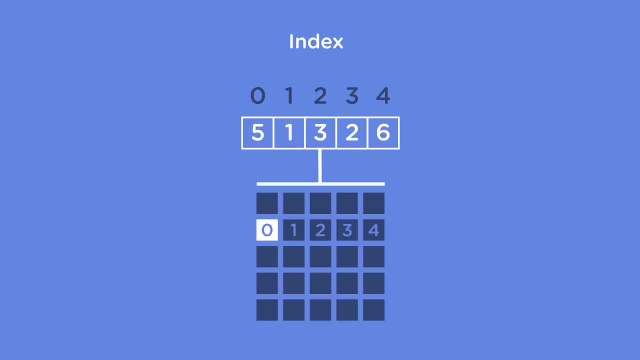 the tail, or we could flip that around: most recent nodes are the tail of the list and the first node to be added is the head. i mentioned that one of the advantages of linked lists over arrays is that inserting data into the list is much more efficient than to the. 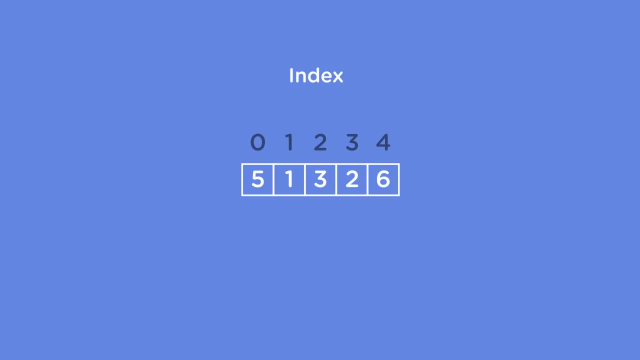 Is that the first index value Is equal to zero, not one. Generally speaking, When an array is declared, A base amount of contiguous memory Is allocated as the array storage. Computers refer to memory Through the use of an address, But instead of keeping a reference. 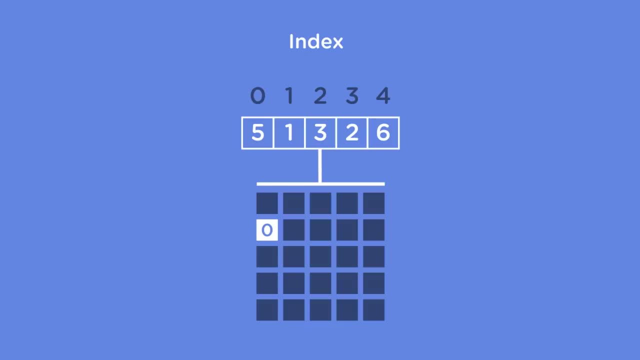 To all the memory allocated for an array. The array only has to store Contiguous using the base address. The array can calculate the address Of any value by using the index position Of that value as an offset, If you want to be more specific. 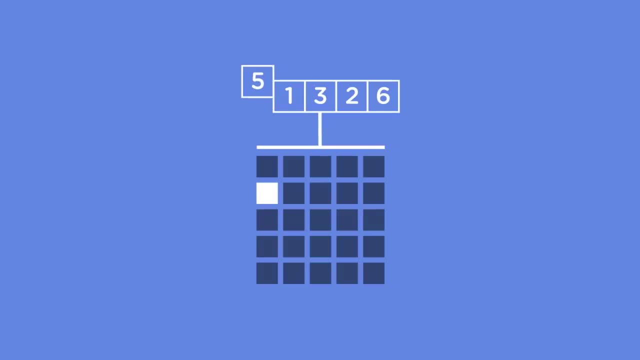 Think of it this way: Let's say we want to create an array of integers, And then each integer takes up A certain amount of space in memory That we'll call m. Let's also assume that we know How many elements we're going to create. 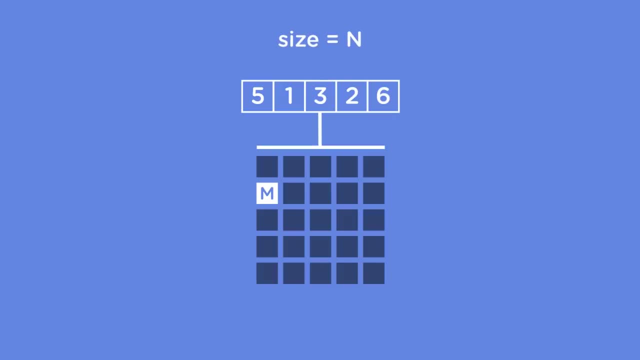 So the size of the array Is some number of elements. we'll call n. The total amount of space Is n times the space per item, m If the array keeps track Of the location in memory Where the first value is held. 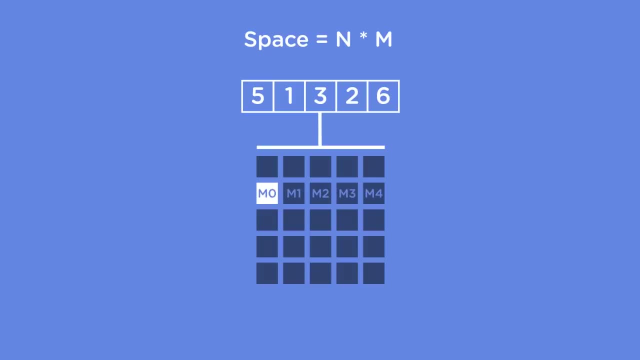 So let's label that m zero. Then it has all the information it needs To find any other element in the list. When accessing a value in an array We use the index. So to get the first element in the list We use the zeroth index. 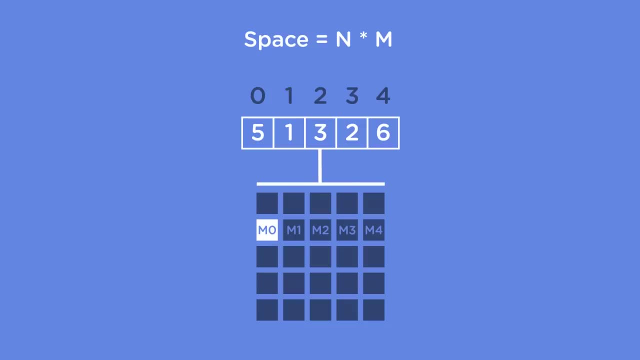 To get the second, we use the index value one, And so on. Given that the array knows how much storage Is needed for each element, We can add the address of any element By starting off with the address For the first element. 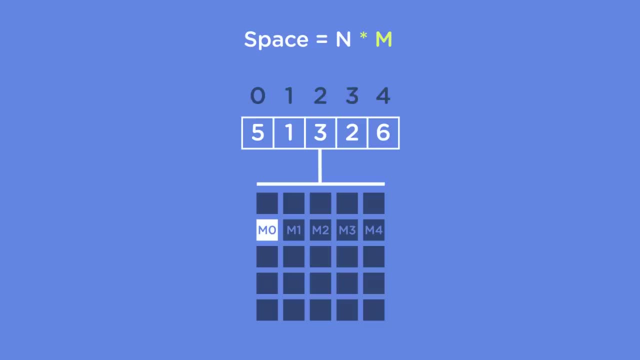 And adding to that the index value Times the amount of storage per element. For example, To access the second value, We can start with m zero And to that add m times the index value one, Giving us m one as the location in memory. 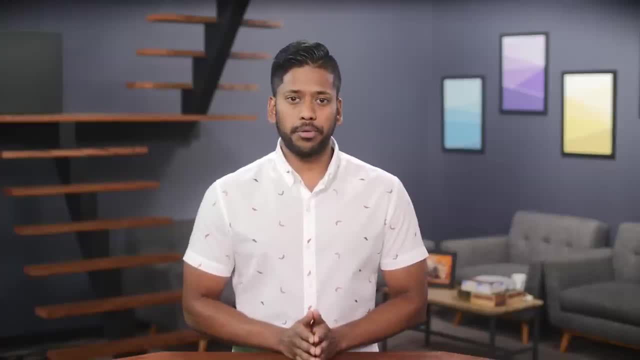 For the second address. This is a very simplified model, But that's more or less how it works. This is only possible Because we know that array memory Has no gaps. Let's switch over to some code, As I mentioned earlier. 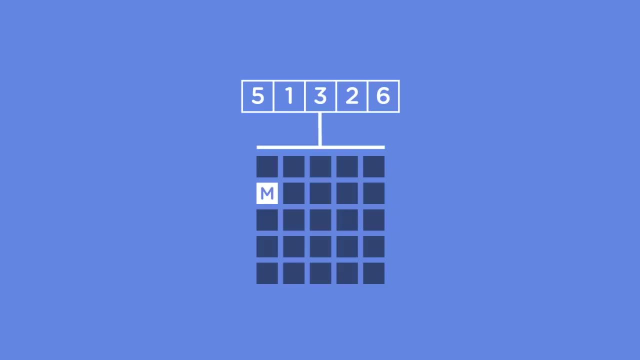 array. this is only true if we're inserting at the head or the tail. technically speaking, this isn't an insert, and you'll often see this method called add, prepend if the data is added to the head, or append if it's added to the tail. a true insert is: 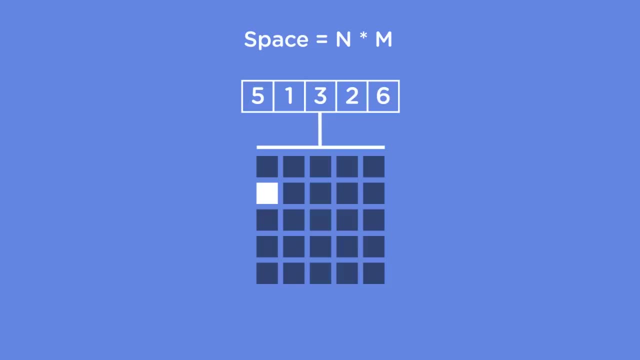 where you can insert the data at any point in the list, which is our third way of adding data. we're going to circle back on that. if we wanted to insert at the tail, then the list needs a reference to the tail node, otherwise we would have to start at the head. 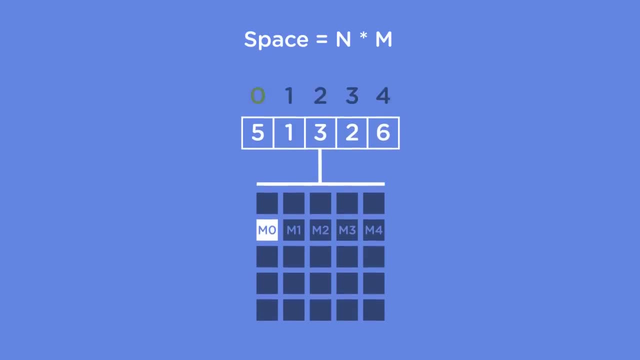 and walk down the length of the list or traverse it to find the tail. since our list only keeps a reference to the head, we're going to add new items at the head of the list now, before we add our new method. i forgot that i didn't show you in the last. 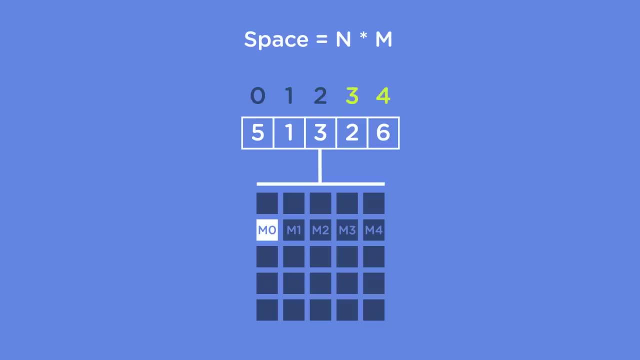 video how to actually use the code we just added and how to check every time. you know, when we add new code that works correctly. so, like before, we're going to bring up the console and here we're going to say python dash. i linked underscore list: dot pi. 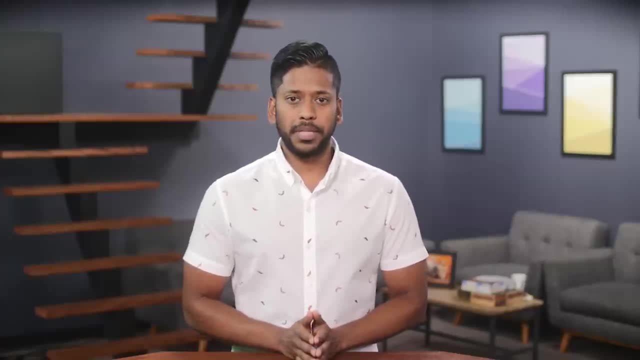 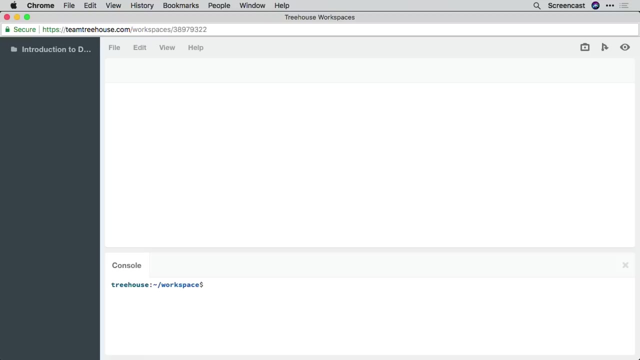 which should load. it, load the contents of our file. and now we'll start here by creating a linked list, so l- equal linked list, and then we'll use a node, so n1, equal node- with the value 10, and now we can assign n1 to the nodes. 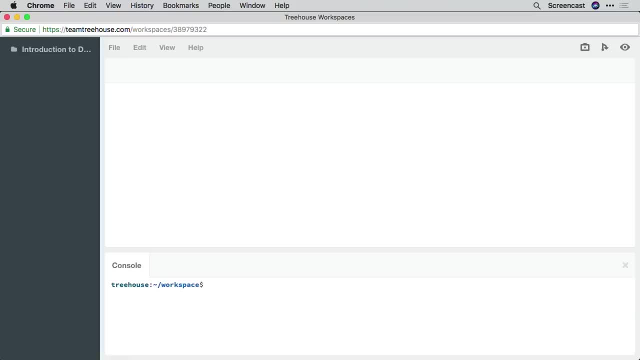 or to the linked list's head attribute. so l1 dot head equal n1 and then we can see if size works correctly. so if we call l1 dot size- and since this is a method, we need a set of parentheses at the end- and enter, you'll see that we get back. 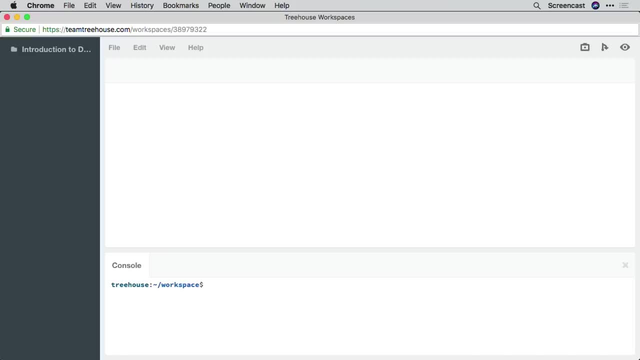 one correctly. okay, so it works. now let's add our new method, which we're going to call add. add is going to accept some data to add to the list inside of a node. so we'll say def add and every python method takes self as an argument. 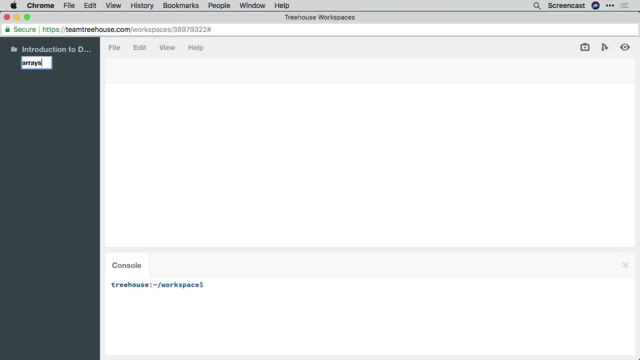 and then we want to add some data to this node. so we're going to say data for the second argument inside the method. first we'll create a new node to hold onto the data, so new underscore node, equal node with the data. before we set the new node as the head of the list: 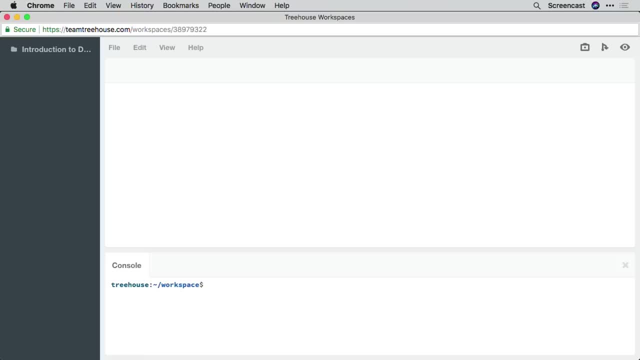 We're going to be using python in this course. If you don't know how to code, Or you're interested in this content But know a language other than python, Check the notes section of this video For more information, While the code will be in python. 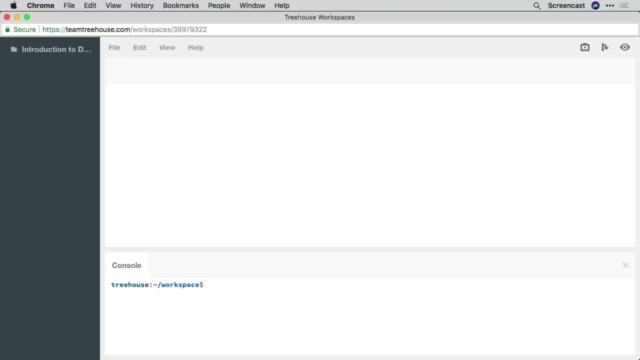 The concepts are universal And, more importantly, Simple enough that you should have no issue following along In your favorite programming language. And to get started, Click on the workspaces button On the video page that you're watching right now. This should spin up an instance. 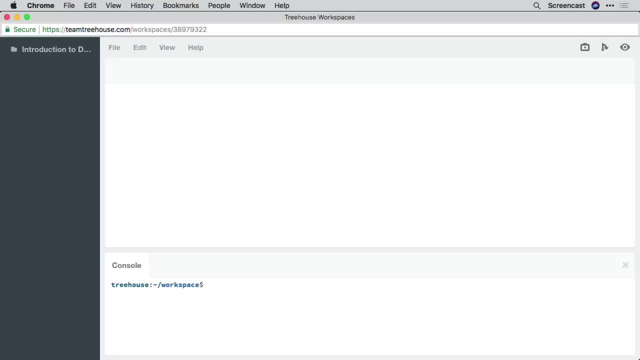 Of a treehouse workspace, An in browser coding environment. Right now your workspace should be empty, And that's expected, So let's add a new file in here. I'm going to go to file New file And we'll call this arrayspy. 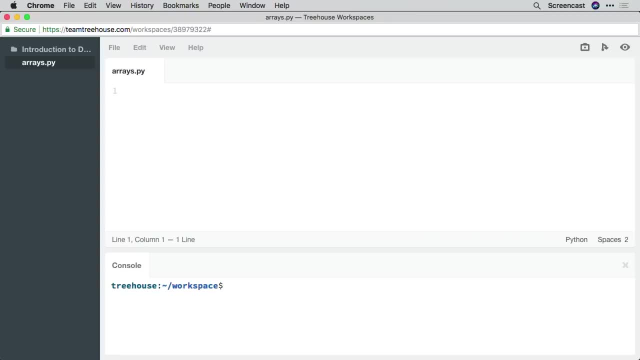 Creating a list in python Is quite simple, So we'll call this new underscore list. We'll use a set of Square brackets around a set of values To create a list, So 1, and we comma separate them, So space 2 and space 3.. 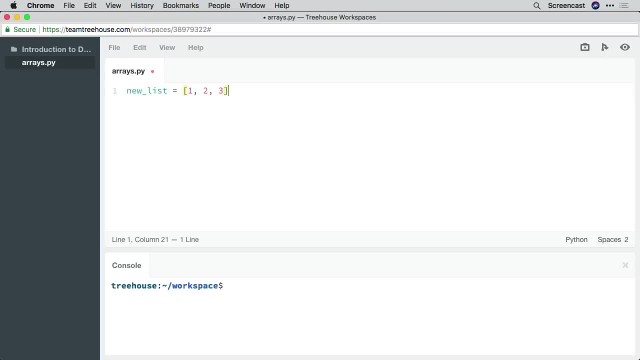 This allocates A base amount of memory for the array to use. Or when I say array, Know that in python I mean a list. Since this is python, The values aren't stored in memory. Instead, the values 1,, 2 and 3.. 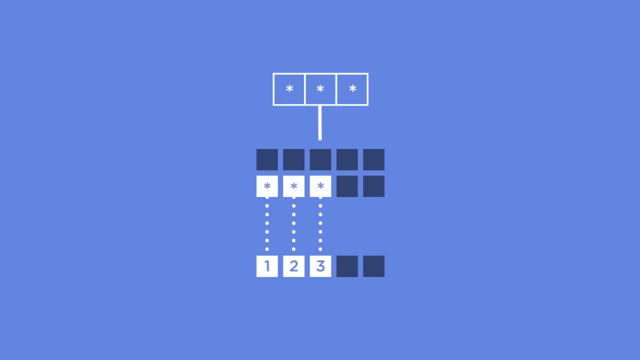 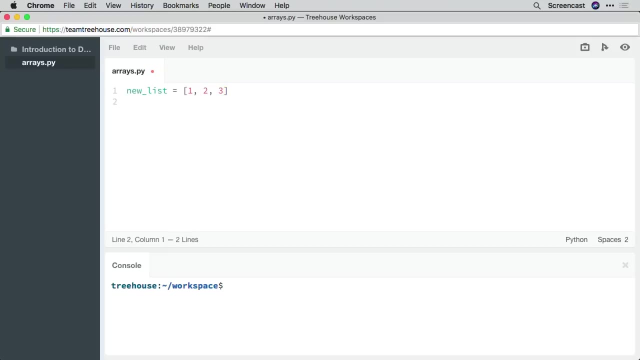 Are stored elsewhere in memory And the array stores references To each of those objects. So to access a value, We use a subscript Along with an index value. So to get the first value, We use the index 0.. And if we were to assign this to another variable? 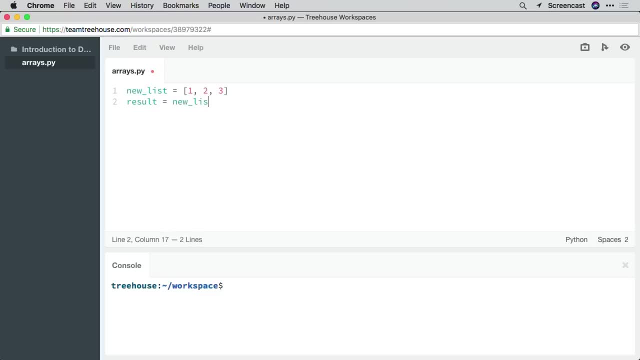 We would say: result Equal new list. We write out new list, since this is the array That we're accessing the value from, And then a subscript notation, Which is a square bracket, And then the index value, As we saw, since the array has a reference. 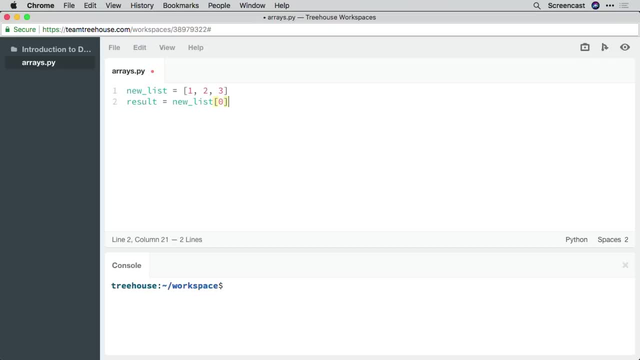 To the base location in memory, The position of any element Can be determined pretty easily. We don't have to iterate Over the entire list. All we need to do is a simple calculation Of an offset from the base memory. Since we're guaranteed 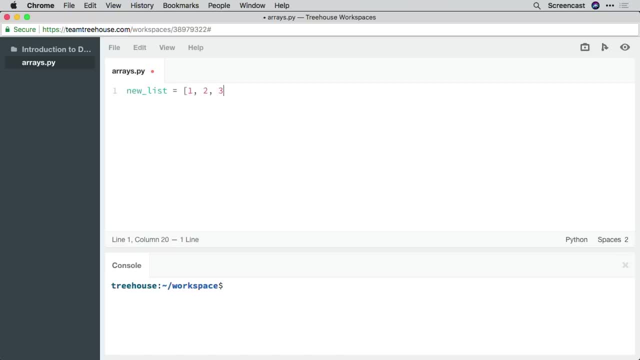 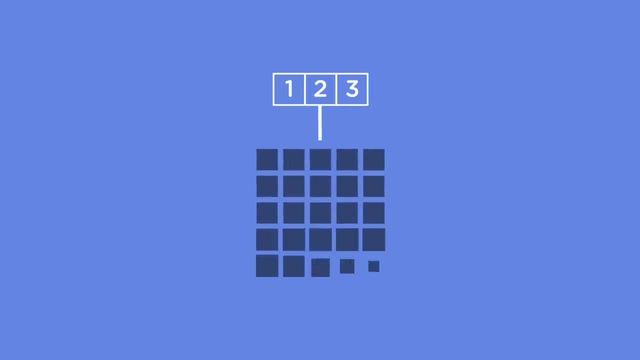 we need to point the new node's next property at whatever node is currently at head. this way, when we set the new node as the head of the list, we don't lose a reference to the old head. so new underscore node dot. next node equal self dot head. 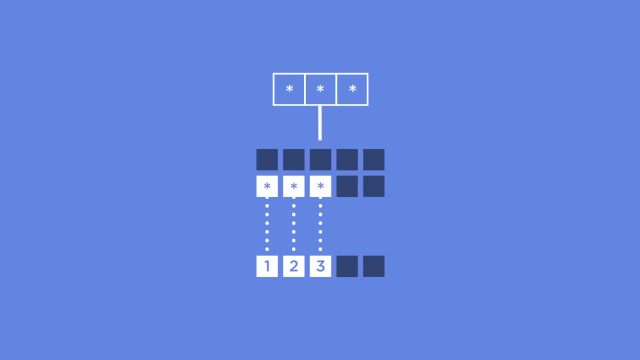 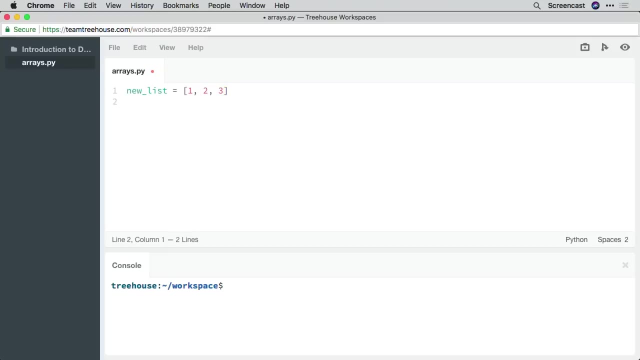 now, if there was no node at head, this correctly sets next node to none. now we can set the new node as the head of the node. so we'll say self dot head equal new underscore node. because the insert operation is simply a reassignment of the head and next node properties. 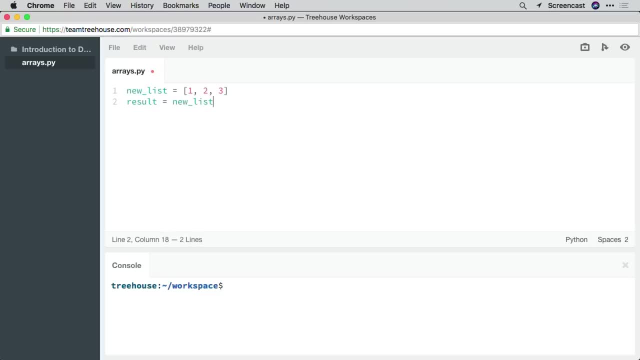 this is a constant time operation, so let's add that in as a doc string first, what the method does. so it adds a new node containing data at the head of the list. this operation takes constant time, which is our best case scenario. okay, let's test this out. so I'm going to bring the console back up. 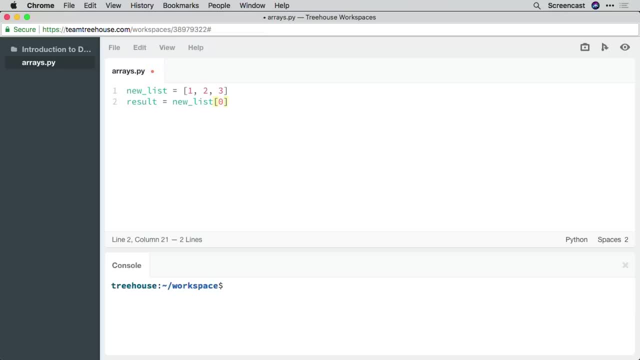 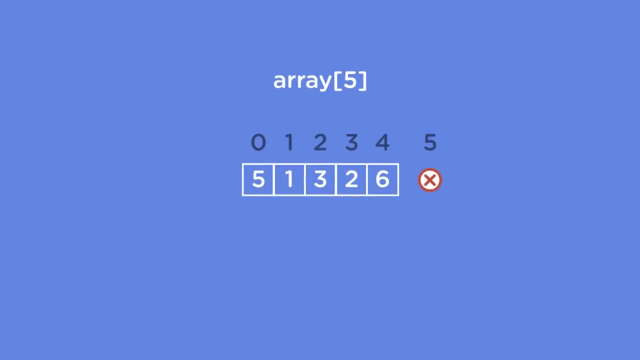 we'll exit out of our current repl and we'll load the contents of the file again. and now we don't need to create a node like we did earlier, so we can say: l equal linked list, l dot add one. okay, let's see if this works. 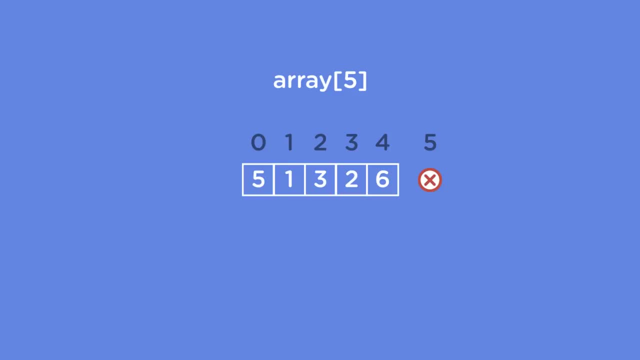 we'll call size and if it worked, the linked list should now have a size of one. there we go. we can also do l dot add two, l dot add three and l dot size should now be three. there we go. now. if I were to type l, 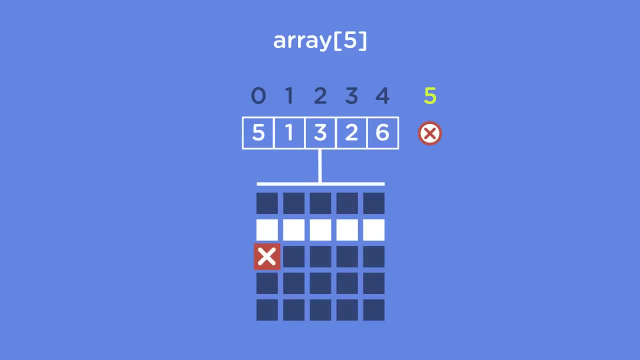 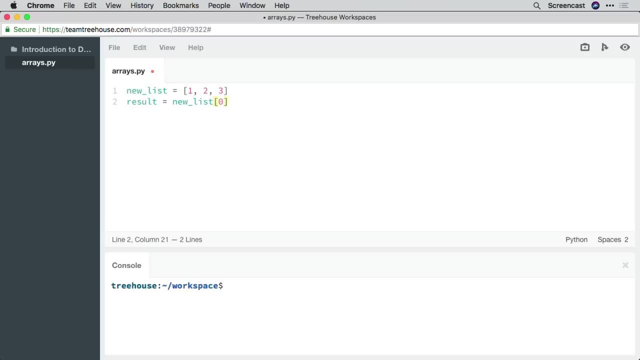 and just hit print again. what we get in the repl is nothing useful. so, like before, we'll implement the repper function for our linked list. now I'm just going to copy paste this in and we'll walk through it. okay, so this is what our implementation. 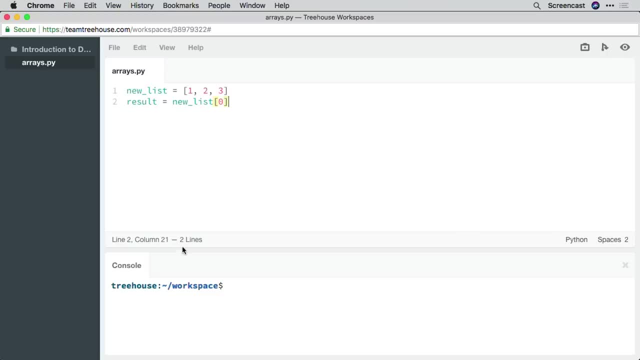 of repper looks like for the linked list object. you can grab this code from the notes section of this video. okay, so at the top you'll see a doc string where it says it returns a string representation of the list and like everything we need to do. 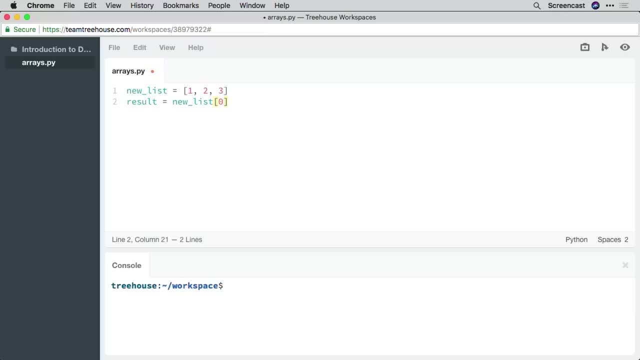 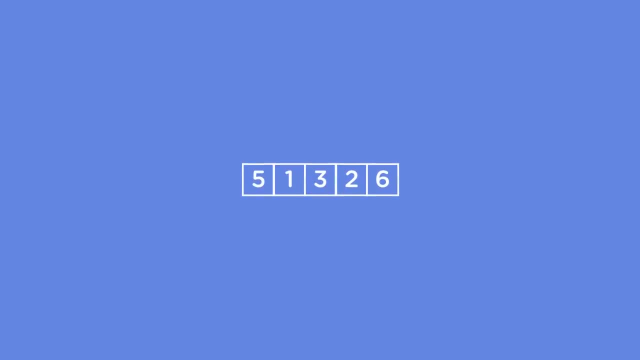 That the memory is contiguous. For this reason, Access is a constant time operation On an array Or a python list. This is also why an array crashes If you try to access a value Using an index that is out of bounds. 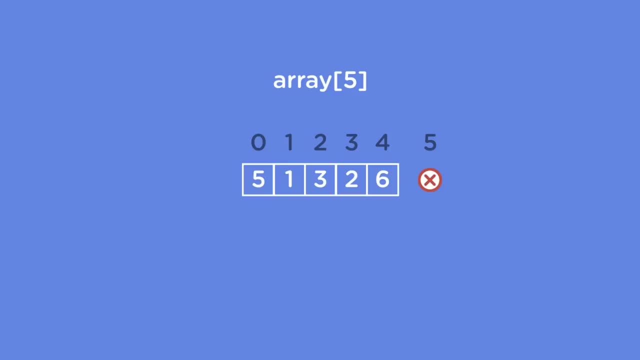 Of what the array stores. If you've used an array before, You've undoubtedly run into an error Or a crash Where you tried to access a value Using an index that was larger Than the number of elements in the array, Since the array calculates the memory address on the fly. 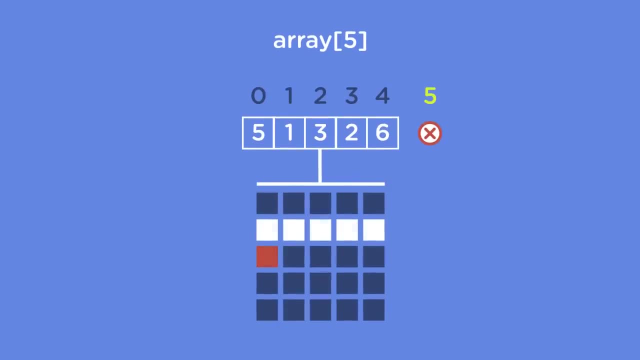 When you access a value With an out of bounds index, As it's called, The memory address returned Is not one that's part of the array structure And therefore cannot be read by the array. This is represented by an index error. 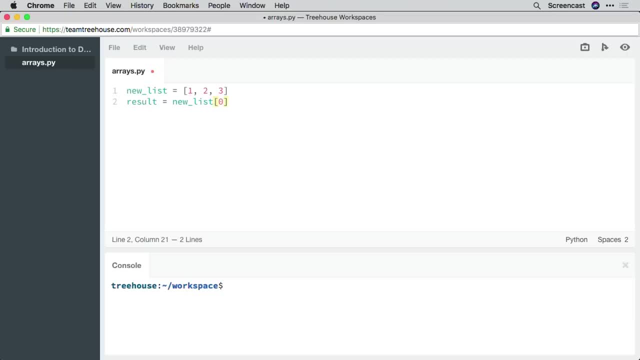 And we can make this happen By using an index We know our array won't contain. Now I'm writing out my code here, Inside of a text editor Which obviously doesn't run the code, So let's drag up this console area here. 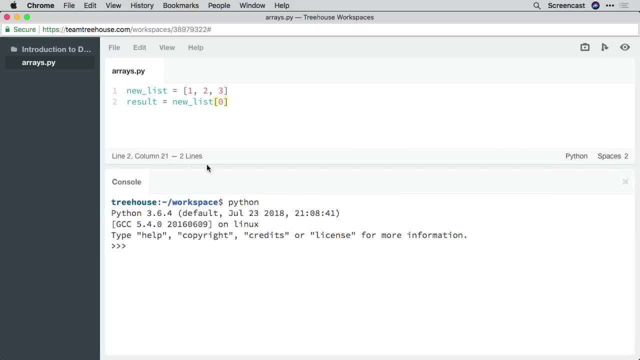 And I'm going to write python To bring up the python interpreter And in here We can do the same thing. So I can say: new list equal 1 comma 2 comma 3.. And now this is an interpreter Which is actually going to evaluate our code. 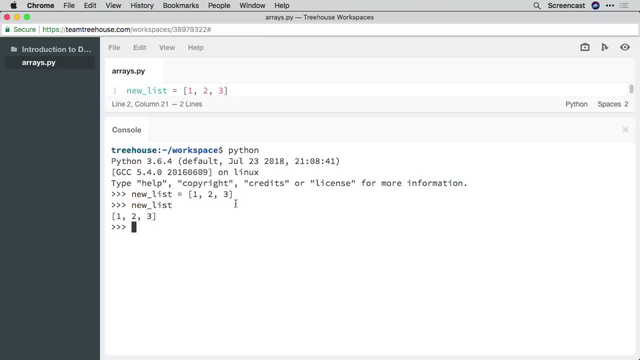 Alright, so now we have a new list. If I type out new list, It gets printed out into the console. Okay, I can also do new list, Square bracket 0. And you'll see that I get the value 1.. Which is the value stored at the 0th index. 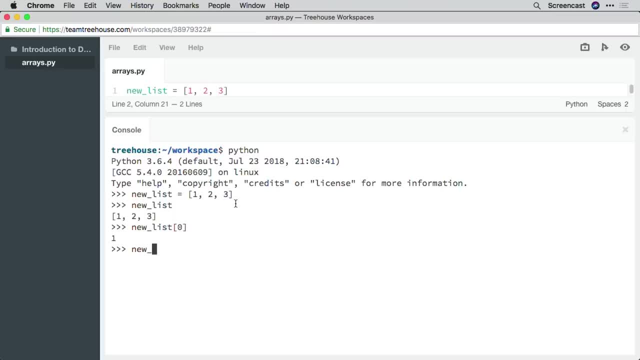 Now to highlight that index error, We can do new list And inside the square brackets We can provide an index That we know our array doesn't contain. So here I'll say index 10. And if I hit enter, We get index error. 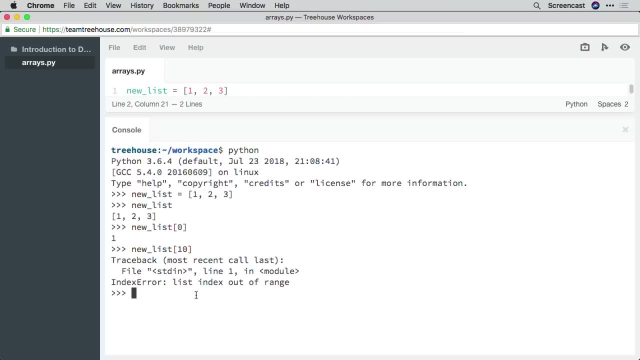 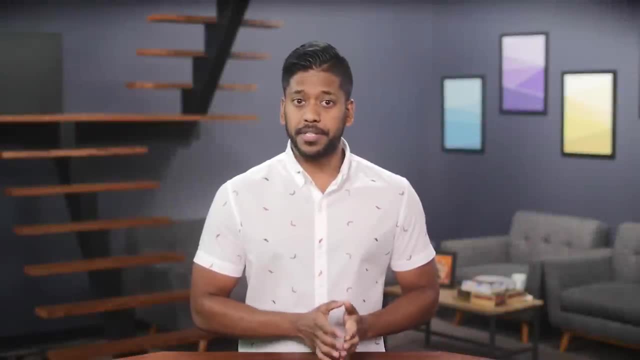 List index out of range. And those are the basics of how we create And read values from an array. In the next video, Let's take a look at searching. In the last video We learned what happens under the hood When we create an array. 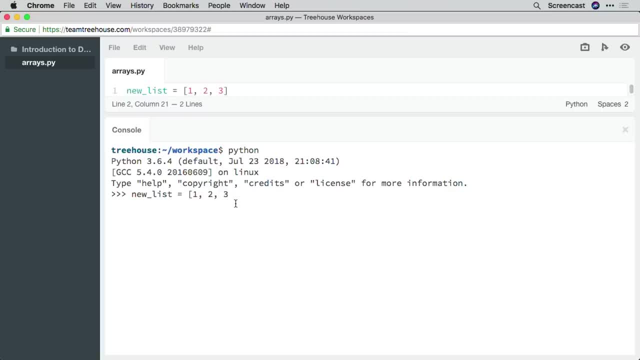 with a linked list. we need to traverse it, so this is going to take linear time. we start by creating an empty list. now I need to distinguish: this is a python list, not a linked list. so we create an empty list called nodes, and to nodes we're going to add strings that 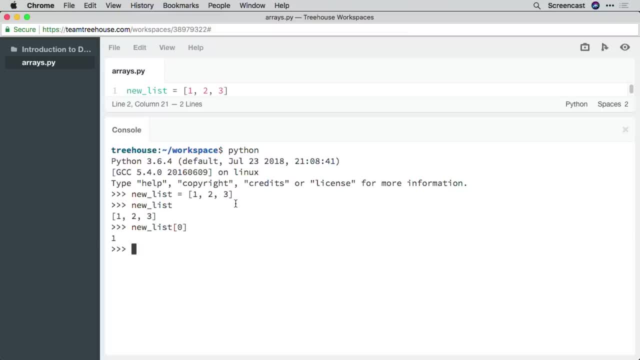 have a description that provide a description of each node, but we're not going to use the description that we implemented in the node class because we're going to customize it a bit here. next we start by assigning selfhead to current, so we sort of have a pointer to the 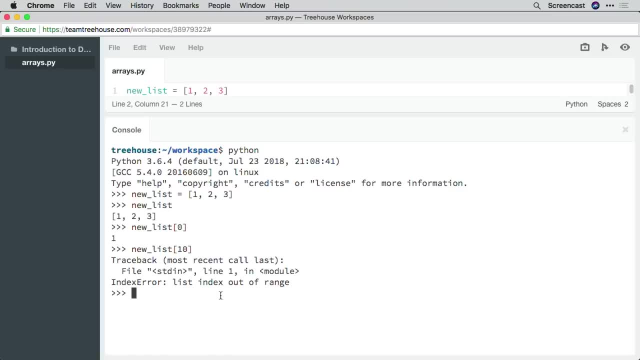 head node, as long as current does not equal none, which means we're not at the tail, we're going to implement some logic. so in the first scenario, if the node assigned to current is the same as the head, then we're going to append this string to our 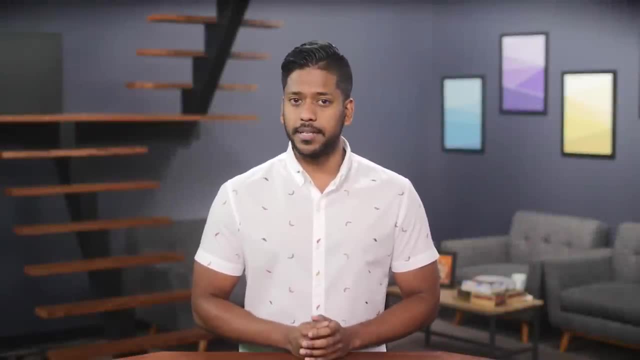 nodes list and this string is simply going to say that, hey, this is a head node and it contains some data which we'll extract using currentdata. next scenario is if the node assigned to current's next node is none, meaning we're at the tail node, then we'll assign a different kind of string. 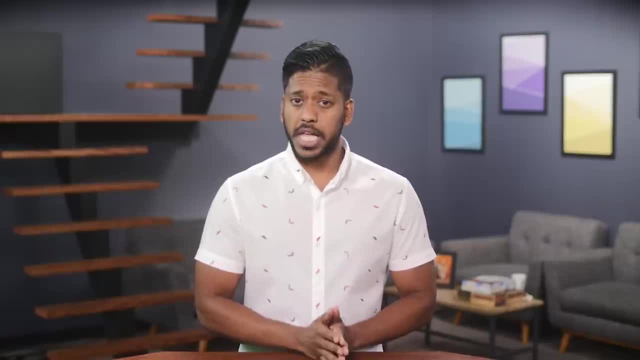 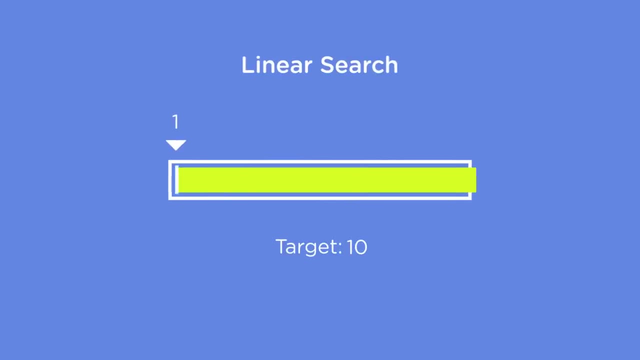 so it's the same as earlier, except we're saying tail here. and then, finally, in any other scenario, which means we're not at the head or not at the tail, we'll simply print the nodes value inside and again we'll extract it using currentdata with every iteration of the loop. 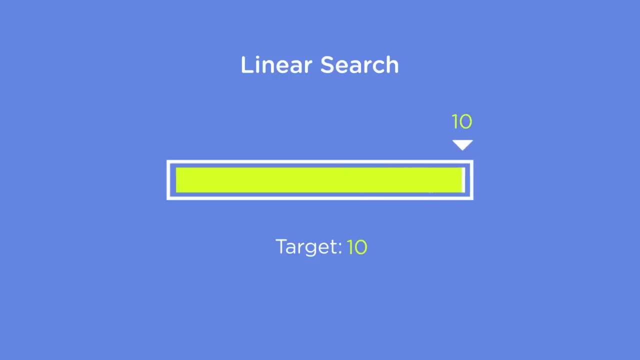 we'll move current forward by calling currentnextNode and reassigning it and then, at the very end when we're done, we'll join all the strings that are inside the nodes list together using the python join method, and we'll say that with every join. 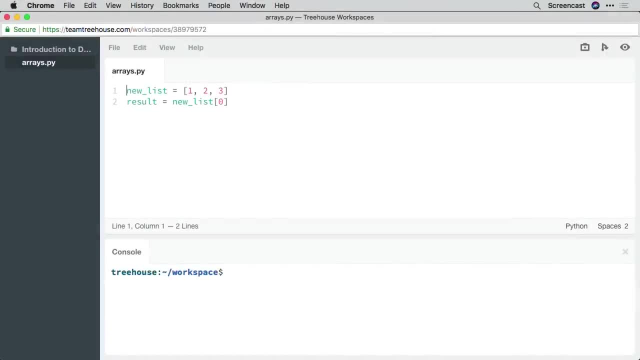 so when you join these two strings together to make one string, you need to put this set of characters in between. alright, so let's see what this looks like. so I'm going to come down here. exit out of the console again. clear it out. load the contents of the file again. 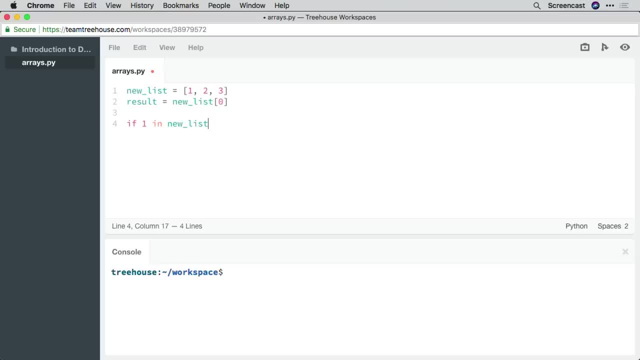 and let's try that. so we'll say l- equal linked list. alright, so ladd1, ladd2, ladd3. that seems enough. and then now, if I type out l and hit enter, we get a nice string representation of the list. so you can see that we add every. 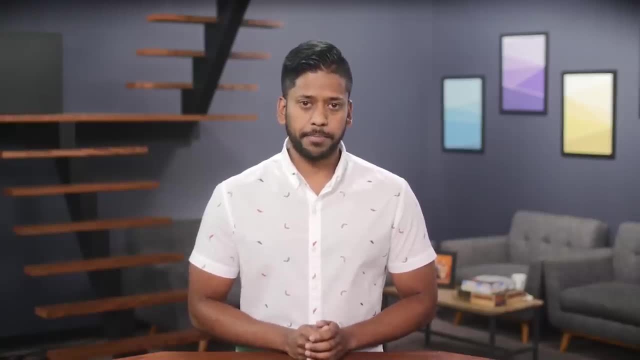 And read a value using an index. In this video, We're going to look at how the remaining data structure operations Work on arrays. If you took the introduction to algorithms course, We spent time learning about two search algorithms, While arrays are really fast. 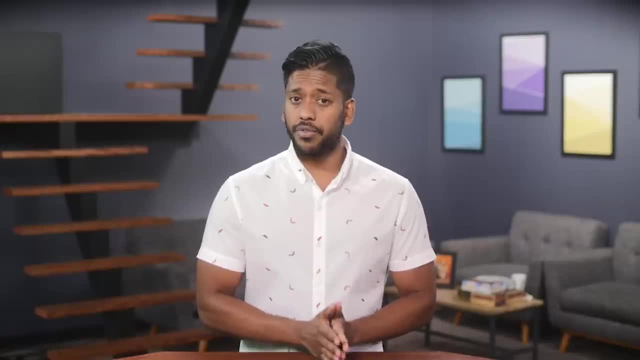 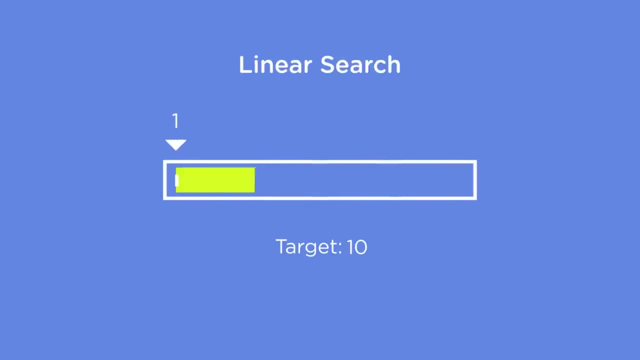 At accessing values. They're pretty bad at searching, Taking an array as is. The best we can do is use linear search For a worst case, linear run time. Linear search works by accessing And reading each value in the list Until the element in concern is found. 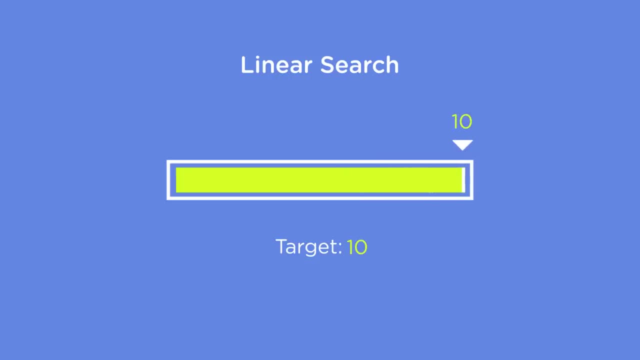 If the element we're looking for Is at the end of the list, Then every single element in the list Will have been accessed and compared. Even though accessing and comparing Are constant time operations For every element results In an overall linear time. 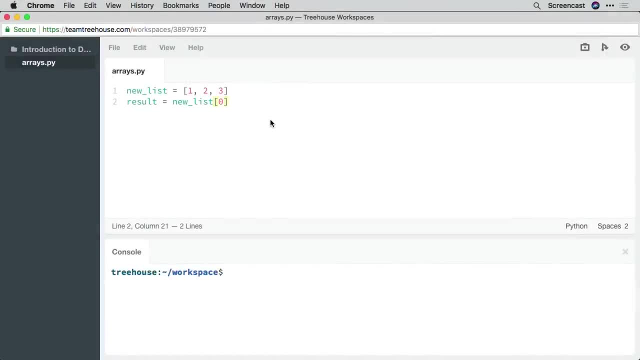 Let's look at how search works in code. In Python, We can search for an item in an array In one of two ways. We can use the in operator To check whether a list contains an item, So I can say if one. 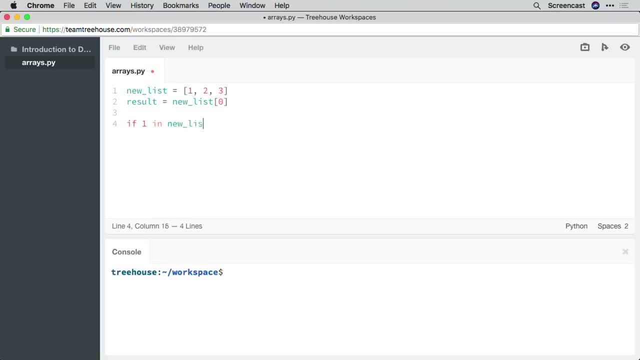 In new Underscore list, Then print True. The in operator actually calls A contains method That is defined on the list type Which runs a linear search operation. In addition to this, We can also use a for loop. 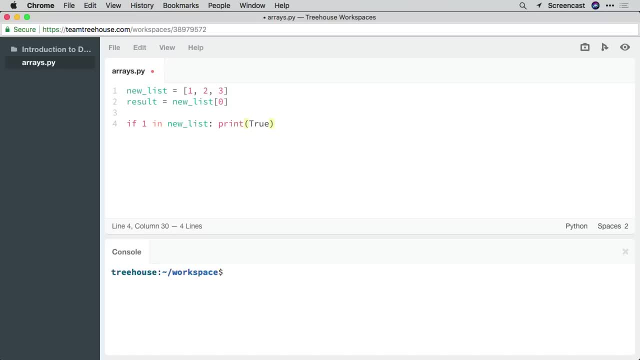 To iterate over the list manually And perform a comparison operation. So I can say For N in new list, If n equals one, Then print True And then after that Break out of the loop. That's the implementation of linear search. 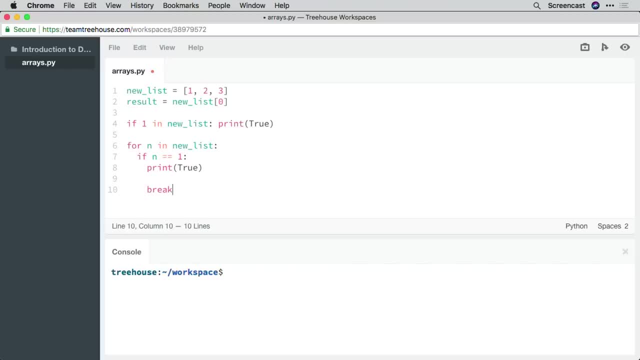 If the array were sorted, However, We could use binary search, But because sort operations incur a cost of their own, Languages usually stay away from sorting the list And running binary search, Since for smaller arrays, Linear search on its own may be faster. 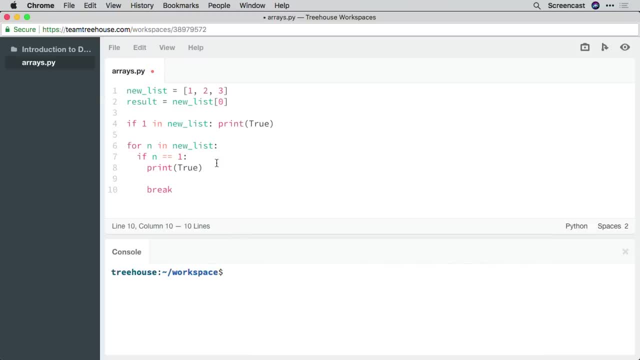 Now again, remember that, Since this is an editor, This is just a text file. None of these lines of code are evaluated, So you can try that out in here. So we'll copy that. Let's say python and hit enter And then when it starts up, 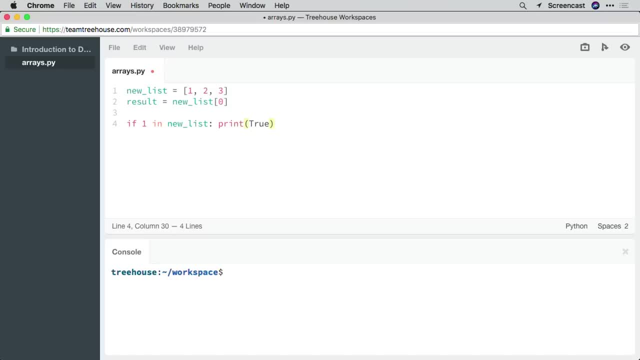 new node to the head. so we added one first- one ends up being the tail because it keeps getting pushed out- then two and then finally three. so three is at the head. so far we've only implemented a single method which functions much like the append method on a python list or an array. 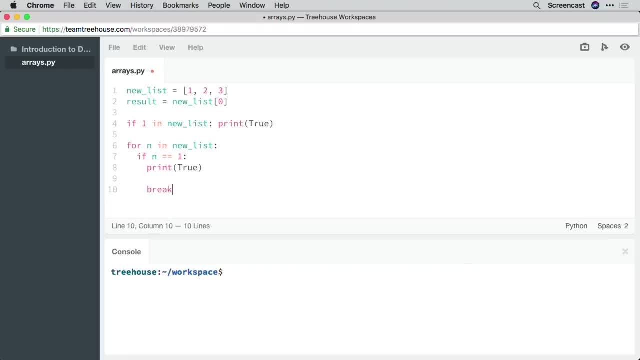 except it adds it to the start of the linked list. it prepends it like append. this happens in constant time. in the next video let's add the ability to search through our list. for the search operation, we're going to define a method that takes a value to search for. 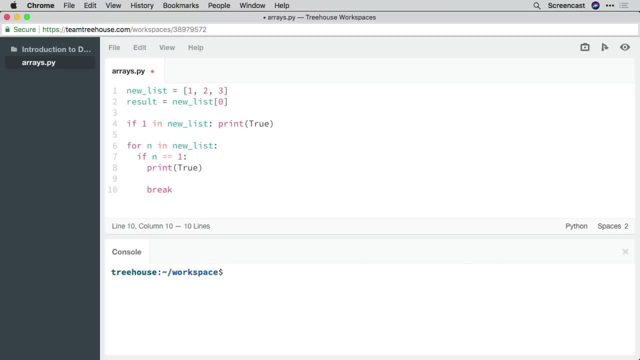 and returns either the node containing the value, if the value is found, or none, if it isn't. so right after, actually, you know what we'll make sure repper is the last function or last method in our class, so we'll add it above it. so here we'll say: 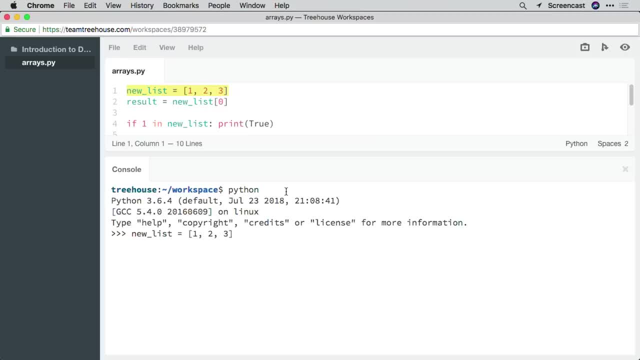 def, search, self and then key. in the last video we implemented the repper method to provide a string representation of the list, so we're going to use similar logic here to implement the search function. we'll start by setting a local variable current to point to the head. 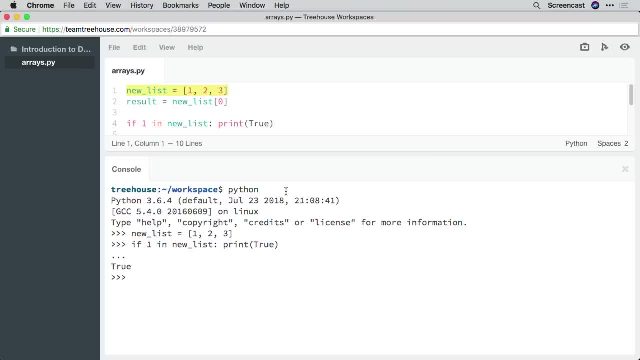 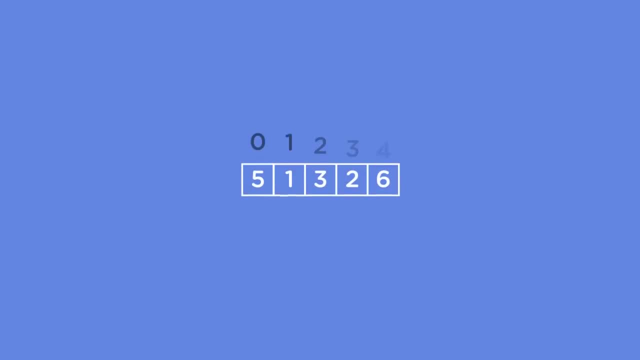 of the list. while the value assigned to current is a valid node, that is, if it isn't none, we'll check if the data on that node matches the key that we're searching for. so, while current, we'll say if current dot data is the key, then we'll 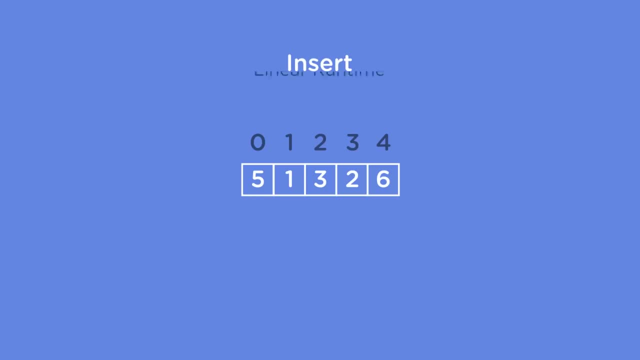 return current. if it does match, we'll go ahead and return it, like we've done here. but if it doesn't, we'll assign the next node in the list to current and check again. so we'll say else: current, equal current dot next node. once we hit the tail. 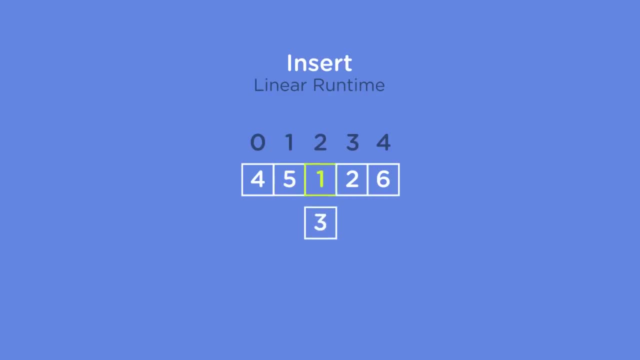 node and haven't found the key. current gets set to none and the while loop exits. at this point we know the list doesn't contain the key, so we can return none. okay, that completes the body of our method. let's add a doc string to document this. 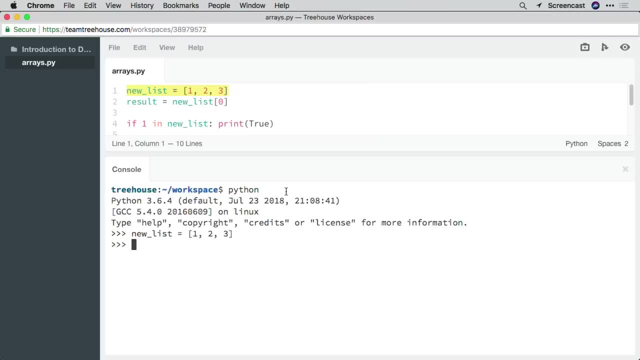 We can paste in our list And now we can try what we just did. So if one in new list, Print True, And there you go, It prints true Now, because we've already learned about linear and binary search In a previous course. 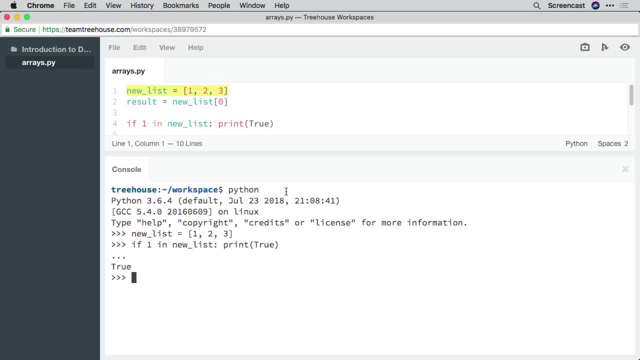 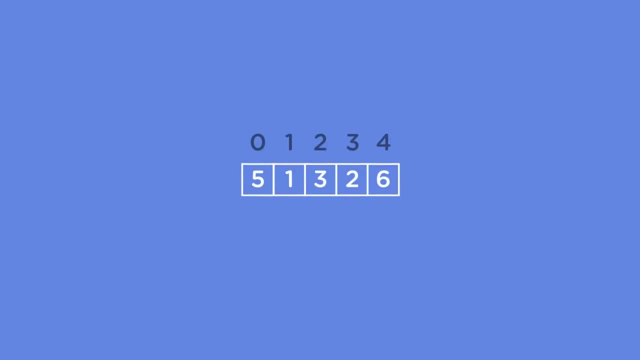 There's nothing new going on here. What's more interesting to look at, In my opinion, Is inserting and deleting values in an array. In general, Most array implementations Support three types of insert operations. The first is a true insert Using an index value. 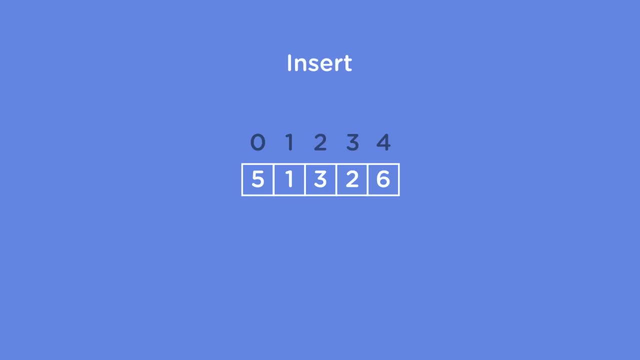 Where we can insert an element Anywhere in the list. This operation has a linear run time. Imagine you wanted to insert an item At the start of the list. When we insert into the first position, What happens to the item That is currently in that spot? 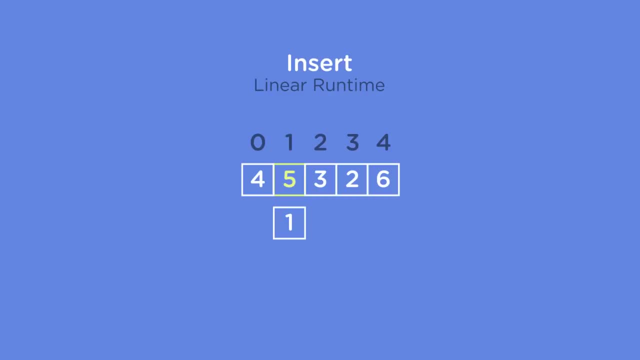 Well, it has to move to the next spot At index value one And it moves to the second item At index position one. That one moves to the next spot At index position two. This keeps happening Until all elements have been shifted forward. 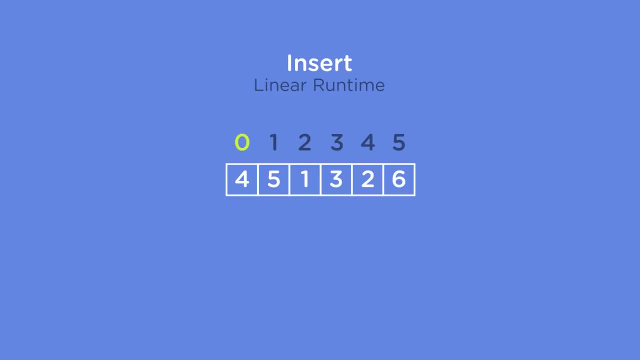 One index position. So in the worst case scenario, Inserting at the zeroth position of an array, Every single item in the array Has to be shifted forward, And we know that any operation That involves iterating through every single value Means a linear run time. 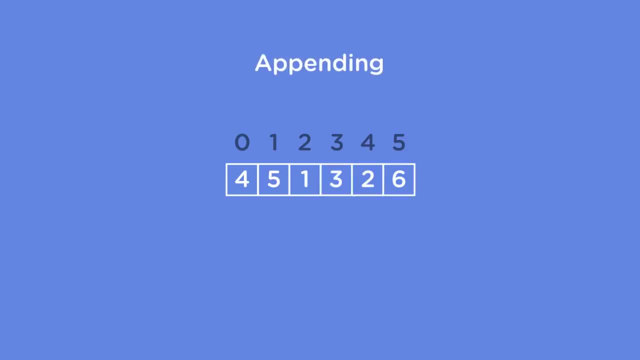 Now the second way To insert an item into an array Is by appending. Appending, Although technically an insert operation, In that it inserts an item into an existing array, Doesn't incur the same run time cost, Because appends Simply add the item to the end of the list. 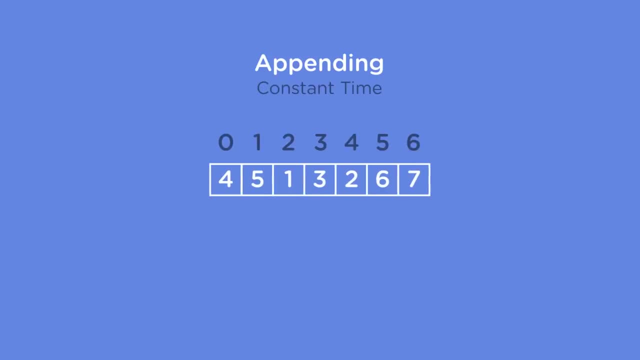 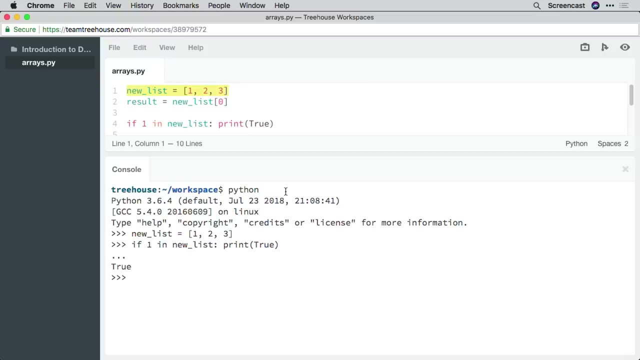 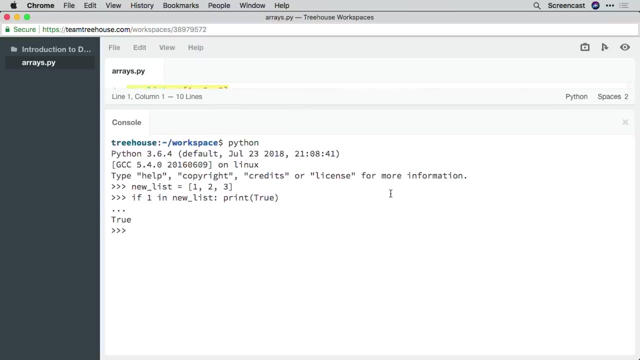 We can simplify And say that this is constant time. This is a constant time operation, But it depends on the language implementation Of array. To highlight why that matters, Consider how lists in python work. In python When we create a list. 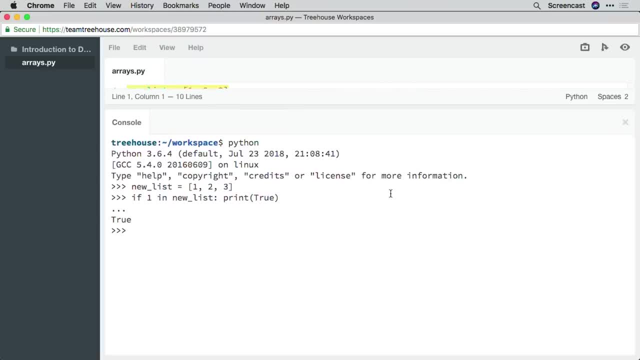 The list doesn't know anything about the size of the list And how many elements we're going to store. Creating a new empty list Like so: Numbers equal And two empty brackets. So this creates a list And allocates a space of size n plus one. 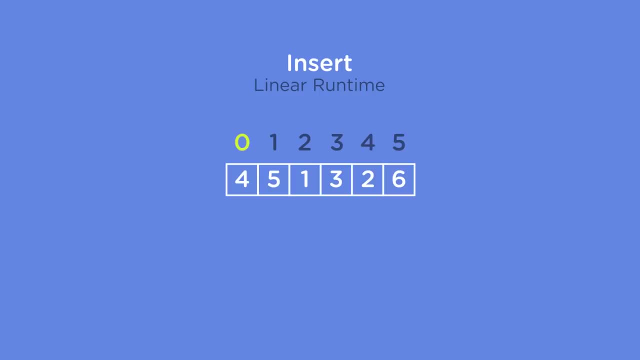 so up at the top, we'll say: search for the first node containing data that matches the key. now, this is important because if our linked list contains more than one node with the same value, it doesn't matter. we're going to return the first one with this implementation. 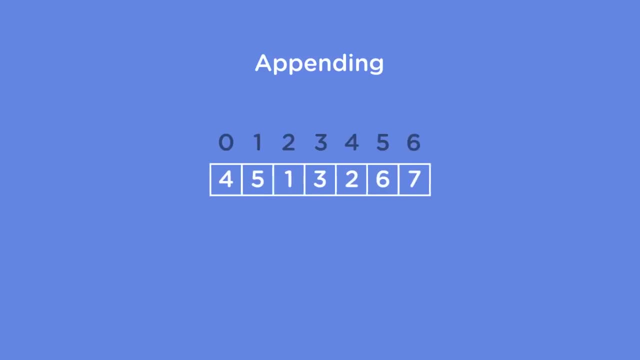 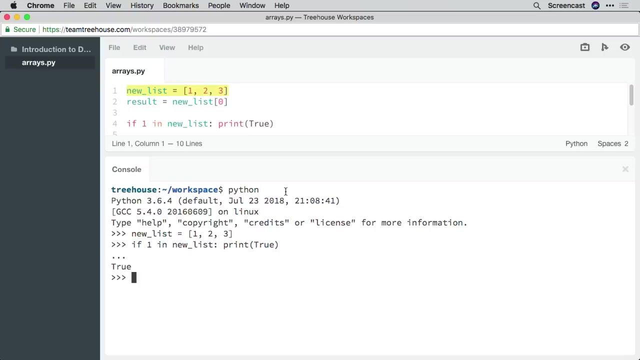 we'll also say here that if it returns the node or none, if not found, in the worst case scenario we'll need to check every single node in the list before we find the key or fail, and as a result, this operation runs in linear time. so we'll say: takes. 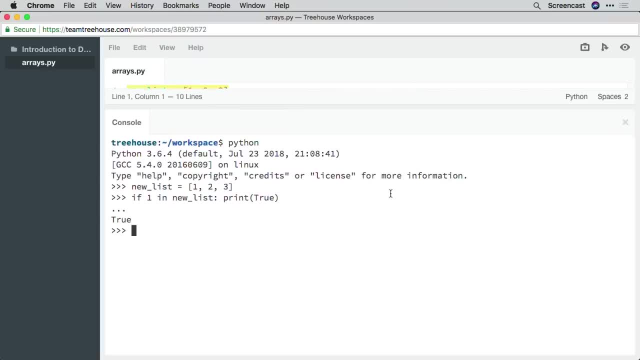 o of n or linear time. so far we haven't seen anything that indicates this data structure has any advantage over an array or a python list, but we knew that I mentioned the strength of linked lists. comes in inserts and deletes at specific positions. we'll check that out in the next video. 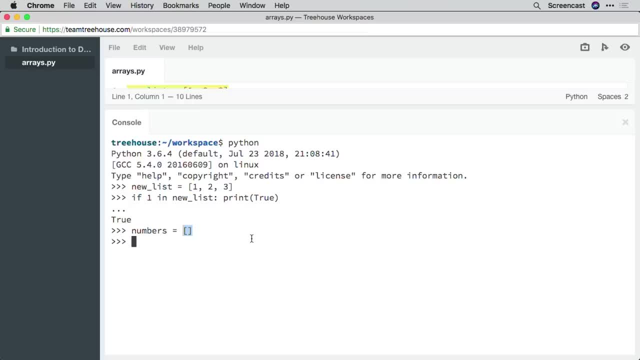 but as always, before we end this one, let's make sure everything works. so we'll load the contents of the file again, l equal linked list, and then we'll say: l dot add 10, l dot add 20, 2, doesn't matter, l dot add 45. 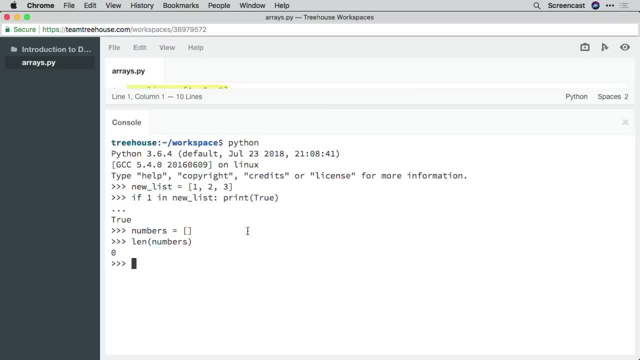 and one more: l dot add 15. now we can say l dot search and we need to give it a value. so we'll say 45 and this returns a node or none, so we'll say n- equal, and then we'll hit enter. if this works, n should be. 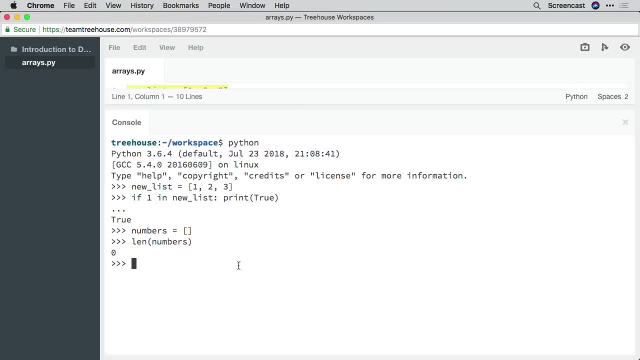 a node. okay, weirdly, n does not work here, at least it says it's not a node, which means I made a mistake in typing out our code and looking at it immediately, it's fairly obvious. so this return none needs to be outside of the while loop. 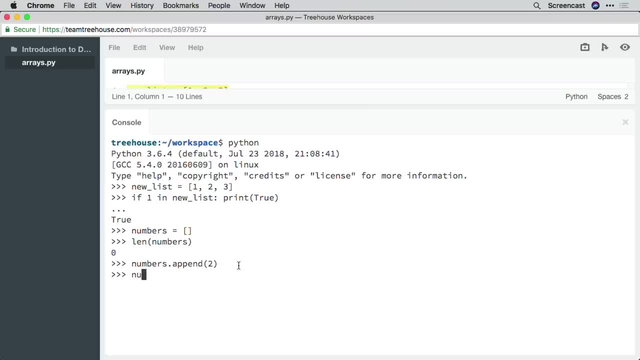 okay, so I'm going to hit save now. so make sure it's on the same indentation here, which means it's outside the while loop, and then we'll run through this again. okay, so l is linked list. l dot add 10. l dot add 2. 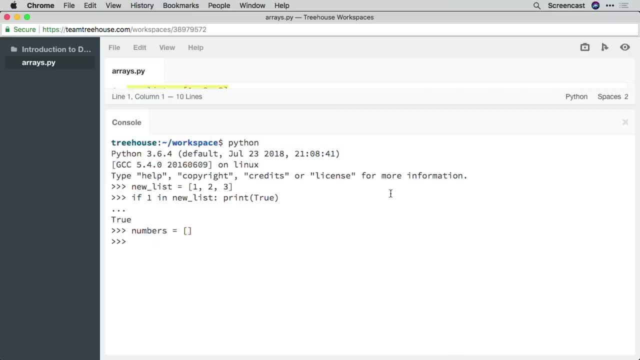 Since n here is zero, There are no elements in this array. In this list Space is allocated One element list to start off, Because the space allocated for the list And the space used by the list Are not the same. What do you think happens when we ask? 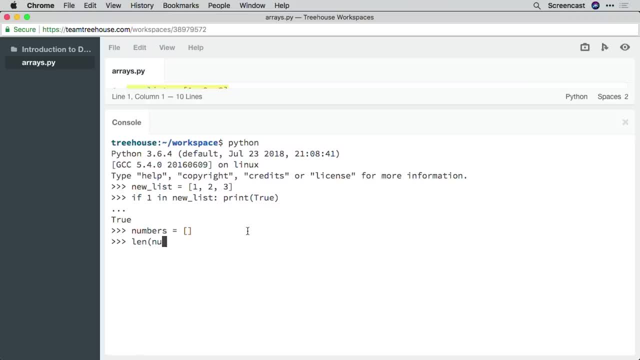 Python for the length of this list. So I can say len Numbers, We correctly get zero back. This means that the list doesn't use The memory allocation As an indicator of its size Because, as I mentioned, It has allocated space for a one element list. 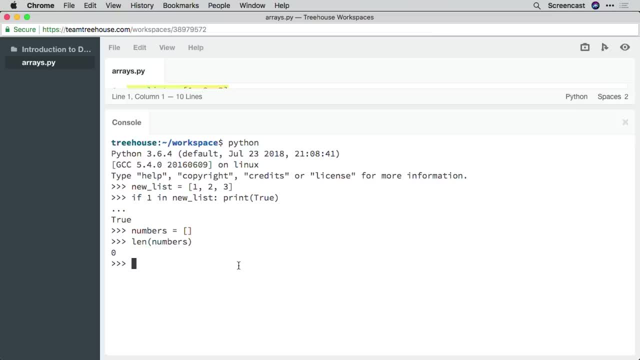 But it returns zero In other ways. Okay so numbers. this list Currently has space for one element. Let's use the append method Defined on the type To insert a number at the end of the list, So I can say numbersappend. 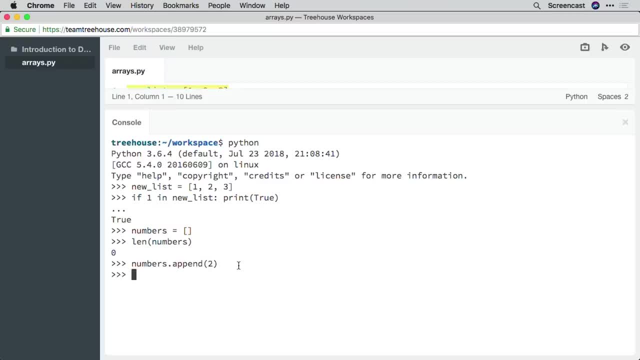 And I'll pass in two. Now, the memory allocation And the size of the list Are the same, Since the list contains one element. Now what if I were to do something like this: Numbersappend, That needs to be a dot. 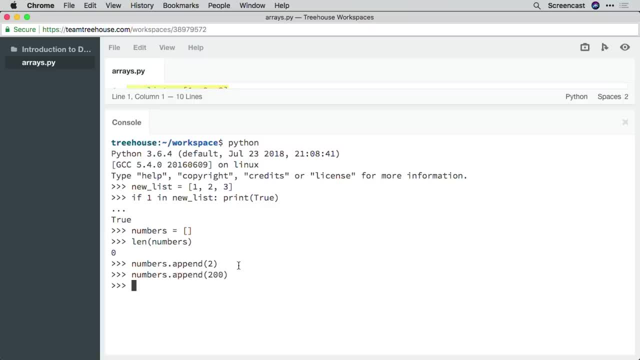 And I'll add another value, 200.. Now, since the list only has an allocation For one item at this point, Before it can add the new element To the list It needs to increase the memory allocation And thereby the size of the list. 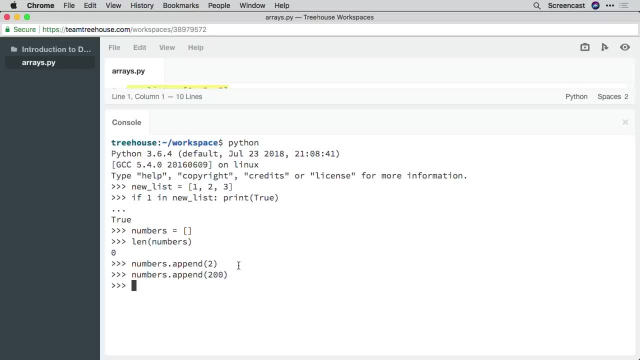 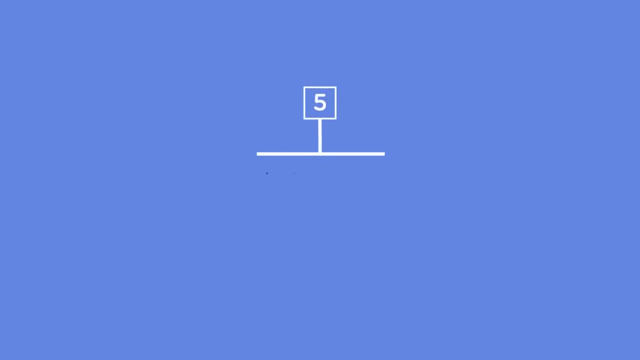 It does this by calling a list Resize operation. List resizing is quite interesting Because it shows the ingenuity In solving problems like this. Python Doesn't resize the list To accommodate just the element We want to add Instead, in this case, 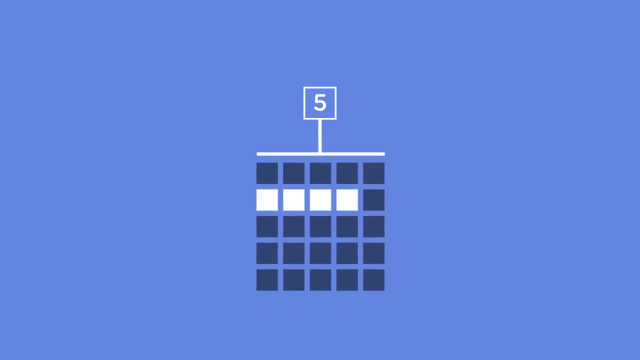 It would allocate four blocks of memory To increase the size To a total of four contiguous blocks of memory. It does this So that it doesn't have to resize the list Every single time. we add an element, But at very specific points. 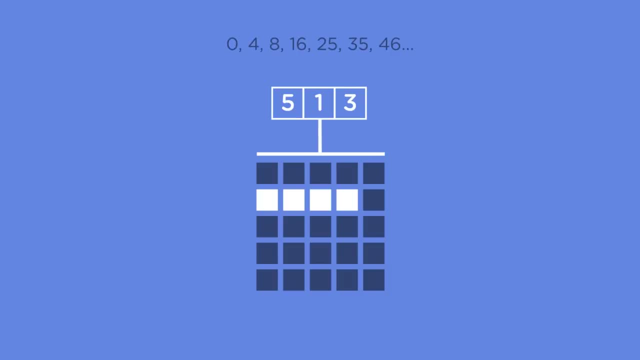 The growth pattern Of the list type in Python Is 0., 4., 8., 16., 25., 35., 46. And so on. This means that as the list size Approaches these specific values, 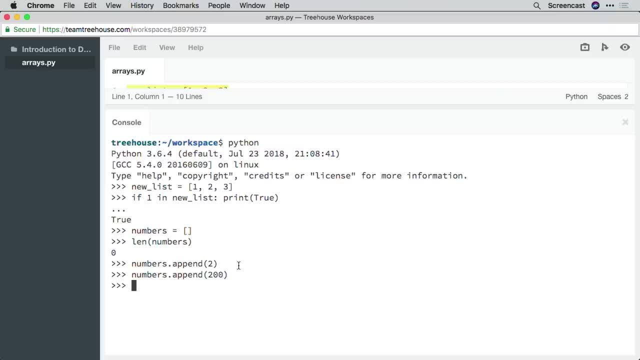 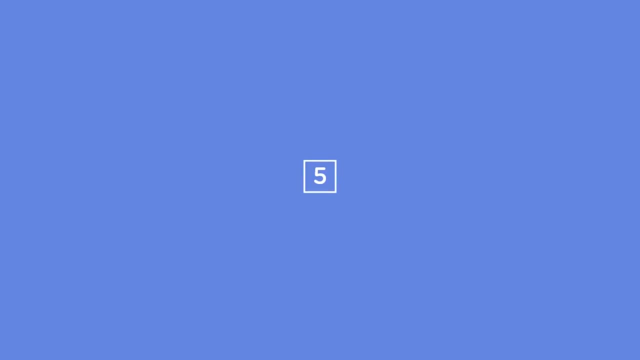 l dot add 45. and what was the last one we did? I believe it was 15, and now we should be able to say l dot search. remember, we're assigning this to a node, to a variable. so l dot search 45. and there you go, we get that node. 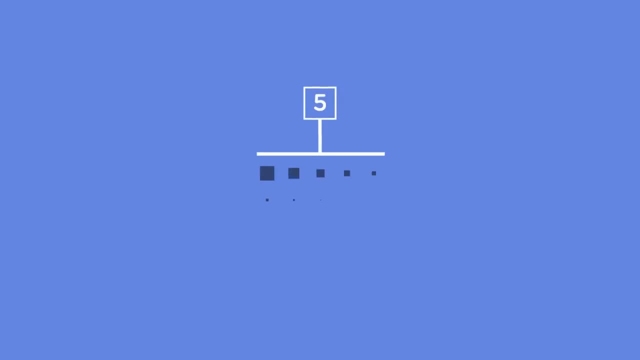 back and we can hit l and we'll see a representation of our list. okay, so again in the next video, inserts and deletes at specific positions. insert operations on linked lists are quite interesting, unlike array, where when you insert an element into the array, all elements after the. 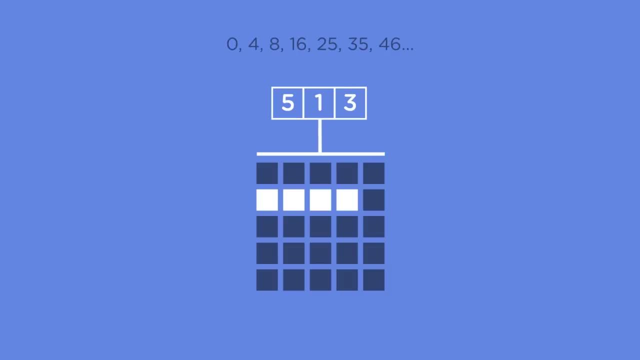 particular index need to be shifted with a linked list. we just need to change the references to next on a few nodes and we're good to go, since each node points to the next one. by swapping out these references, we can insert a node at any point in the list in constant. 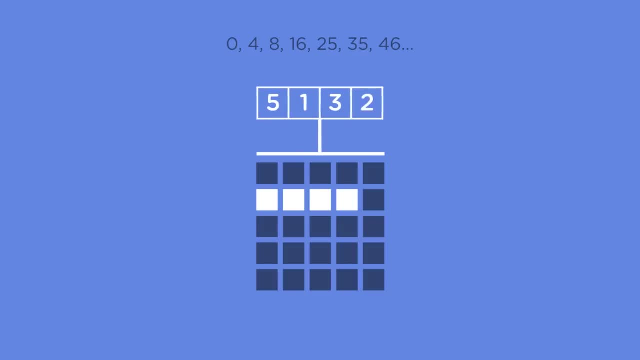 time, much like binary search, though there's a catch. to find the node at that position we want to insert, we need to traverse the list and get to that point. we just implemented our search algorithm for the linked list type and we know that this runs in linear. 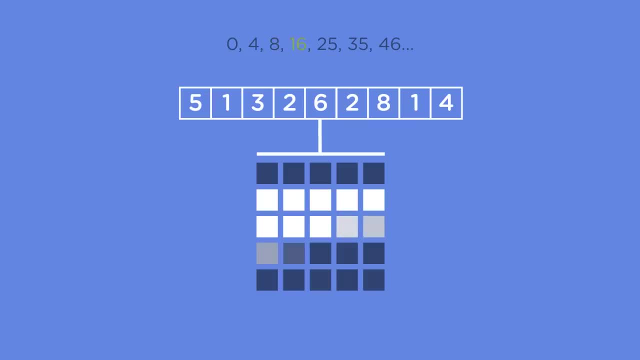 time. so, while actually inserting is fast, finding the position in the list you want to insert, it is not. this is why i mentioned that there were some caveats to inserting. anyway, let's see what this looks like in code. we'll define a method named insert that takes data to insert along. 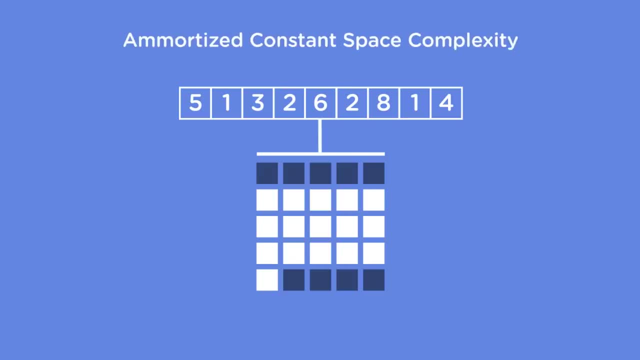 with an index position. so we'll do this after search right here, say, def, insert, and this takes some data to insert and a position to insert it at. you may be thinking wait a minute, linked lists don't have index positions. right, and you're correct. but we can mimic that behavior by just 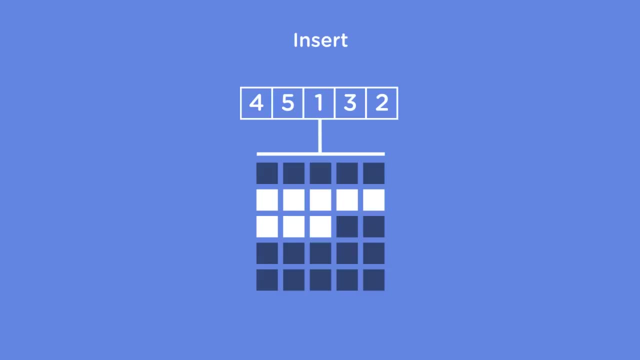 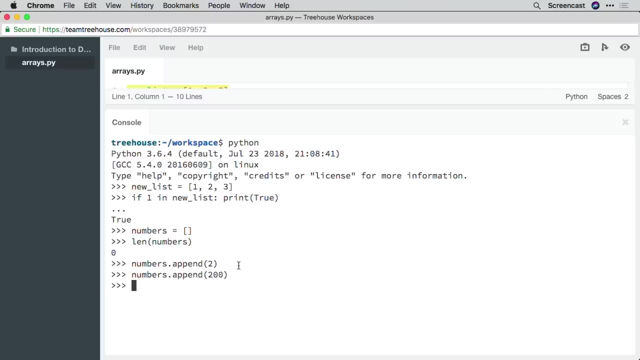 counting the number of times we access next node. if the index value passed into this argument is zero, that means we want to insert the new node at the head of the list. this is a method that is effectively the same behavior as calling add, which means the logic is the same, so we don't need 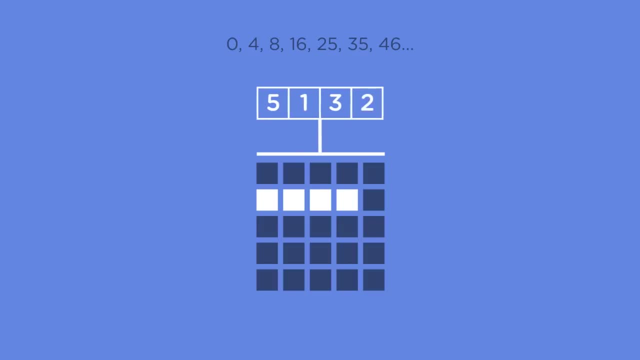 Resize is called again If you look at when the size Of the list is 4.. This means that when appending 4 more values Until the size of 8. Each of those append operations Do not increase the amount Of space taken. 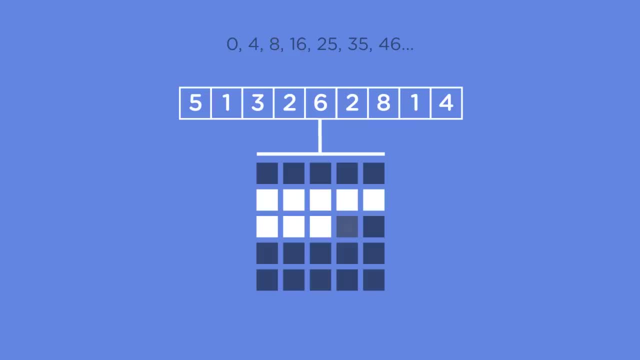 At specific points. however, When resizing is triggered, Space required increases As memory allocation increases. This might signify That the append method Has a non constant space complexity, But it turns out That, because some operations Don't increase space And others do, 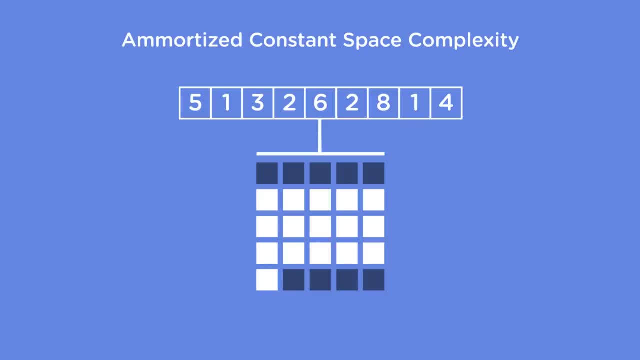 When you average all of them out. Append operations. take constant space. We say that it has an amortized Constant space complexity. This also happens with insert operations. If we had a 4 element array, We would have 4 elements And a memory allocation of 4.. 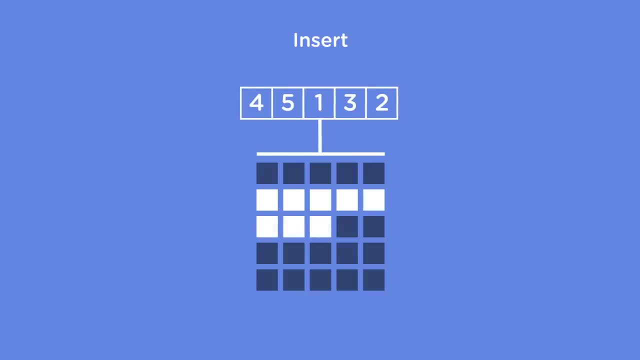 An insert operation at that point Happens on the list, But at that point it would trigger a resize. Inserting is still more expensive, though, Because after the resize, Every element needs to be shifted over. 1. The last insert operation. 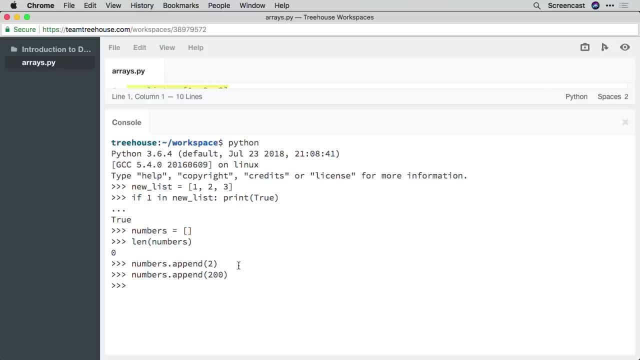 That is supported in most languages Is the ability to add One list to another. In Python, this is called an extend And looks like this, So let's say numbers. Let me actually clear out the console. Oh, actually, well, Let's exit Python. 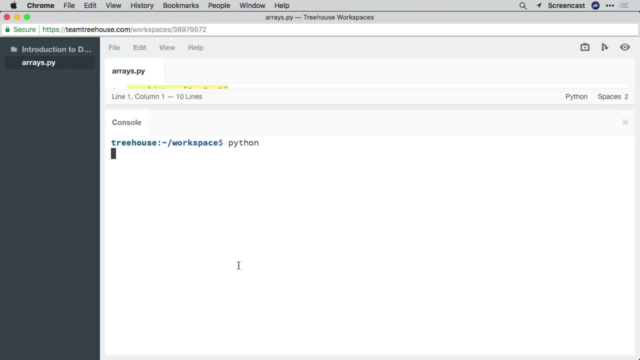 We'll clear this out. So we're back at the top And we'll start again. So I'll say numbers And we'll set it to an empty list, And now we can say numbersextend And as an argument We're going to pass in a new list entirely. 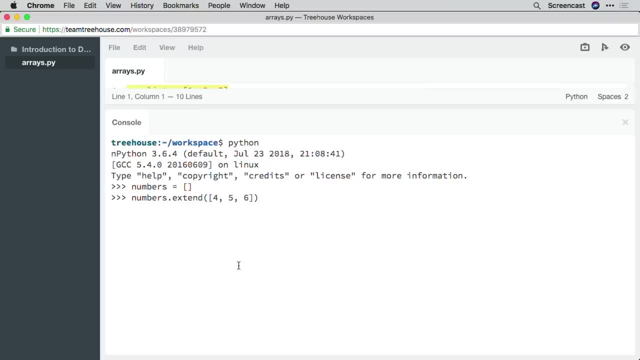 So here we'll say 4,, 5,, 6. And then, once I hit enter, If I were to print out numbers, You'll see that it now contains the values 4,, 5, and 6.. Extend takes another list to add. 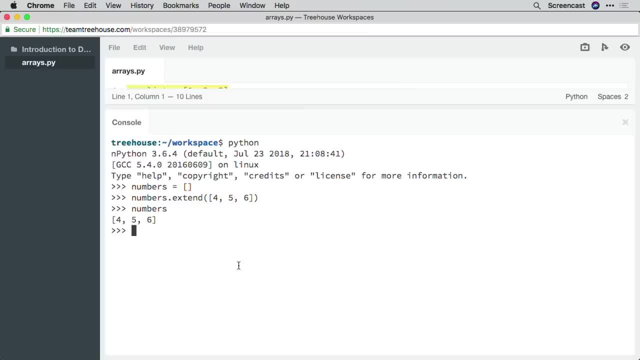 Extend effectively Makes a series of append calls On each of the elements in the new list, Until all of them Have been appended to the original list. This operation has a run time Of big O of k, Where k represents the number of elements. 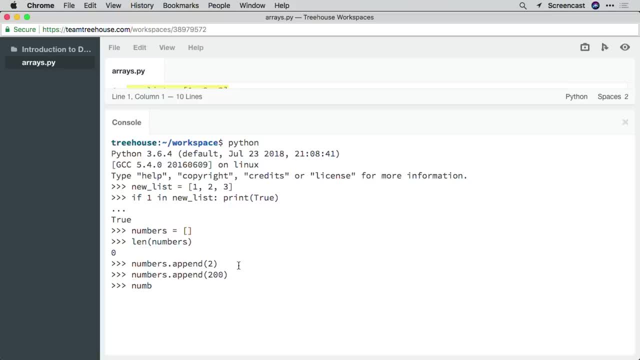 to repeat it, we can call the add method we wrote earlier. so we'll say: if index, if index equals zero, or if index is zero, then self dot add data. if the index is greater than zero, then we need to traverse the list to find the current node. 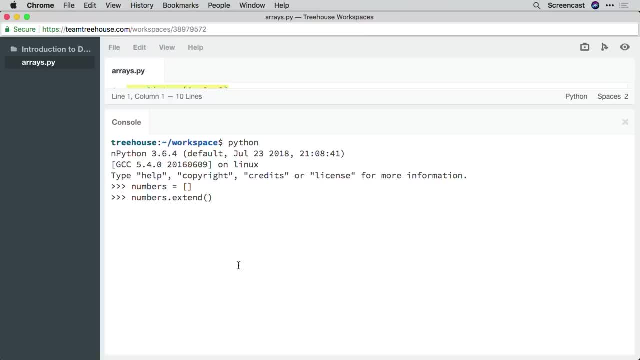 at that index. so if index is greater than zero, now, before we do that we need to create a new node containing the data we want to insert. so we'll say new equal node with some data. I'm going to assign index- the argument passed to our function- to a local variable. 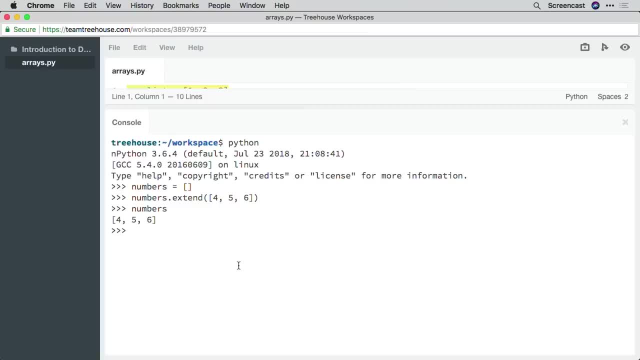 named position and the head of the list to a variable named current position, equal index. current equals self dot head. every time we call current dot, next node, meaning we're moving to the next node in the list, we'll decrease the value of position by one when position is zero. 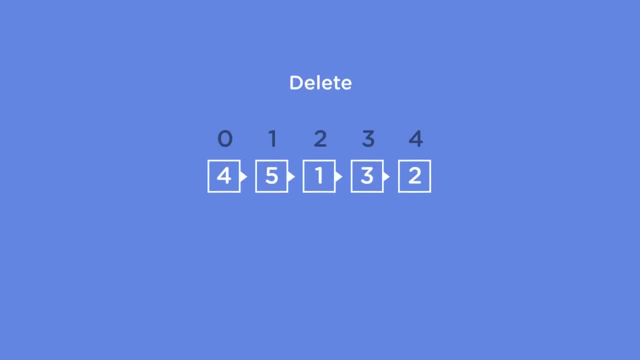 we'll have arrived at the node. that's currently at the position we want to insert in. in reality, though, we don't want to decrease it all the way to zero. imagine we have a list with five nodes and we want to insert a node at position three. to insert a node. 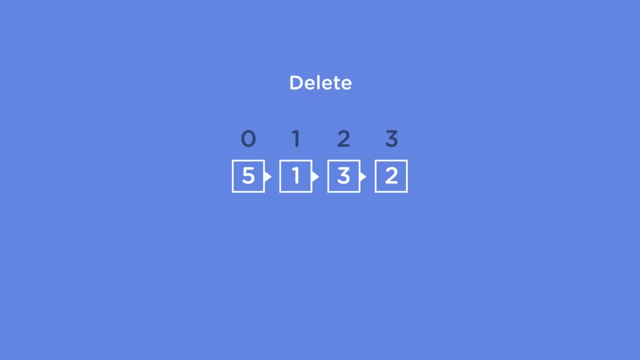 at position three. we need to modify the nodes at positions two and three. node two's next node attribute is going to point to the new node and the new node's next node attribute will point to node three. in this way, an insert is a constant time operation. we don't need to shift every. 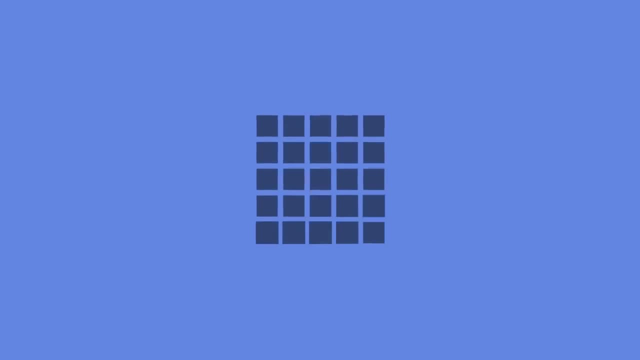 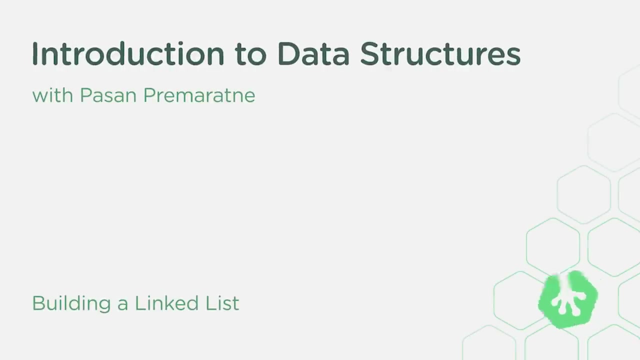 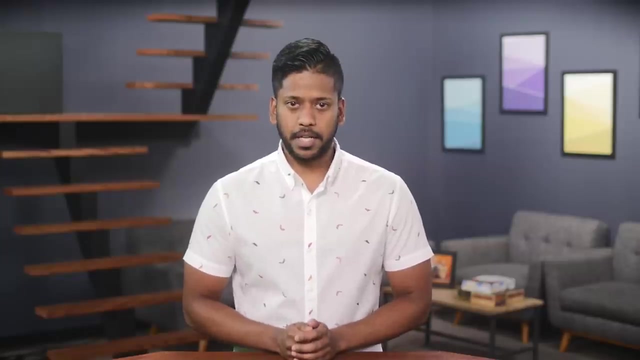 single element. we just modify a few next node references in a doubly linked list we can use node three to carry out both of these operations. node three in a doubly linked list would have a reference to node two and we can use this reference to modify all the unnecessary. 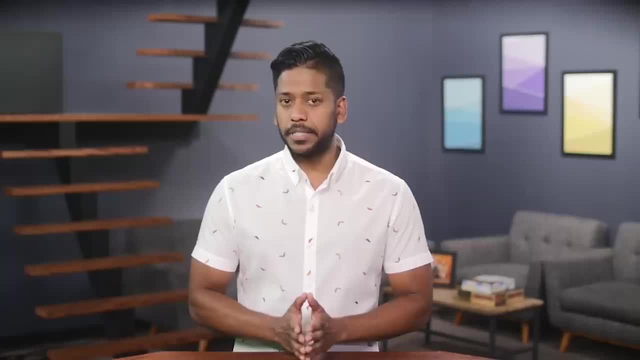 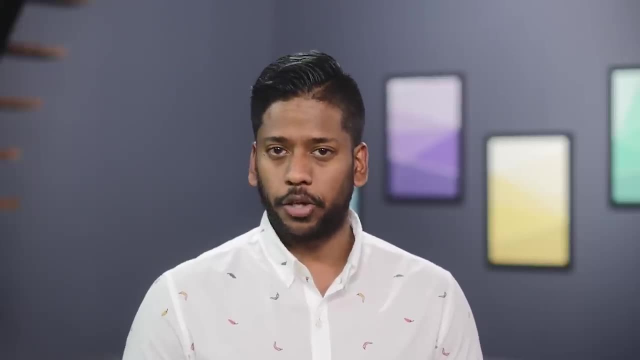 links and a singly linked list, though, which is what we have. if we kept decreasing position until we're at zero, we arrive at node three. we can then set the new node's next node property to point to node three, but we have no way of getting a. 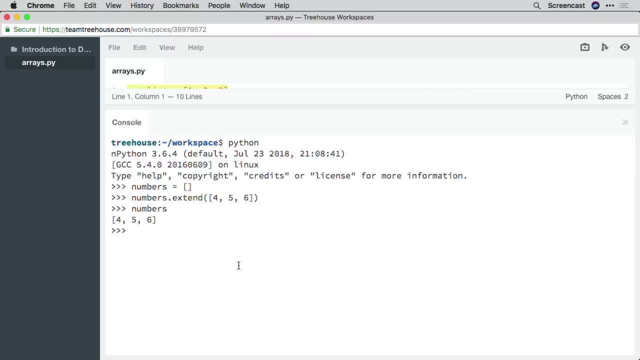 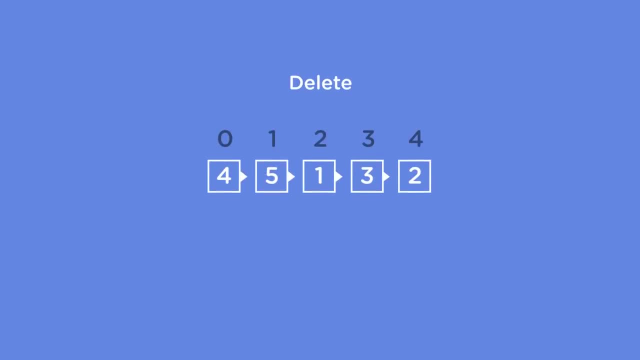 In the list that we're adding To our existing list. The last type of operation we need to consider Are delete operations. Deletes are similar to inserts In that when a delete operation Occurs, The list needs to maintain correct index values. 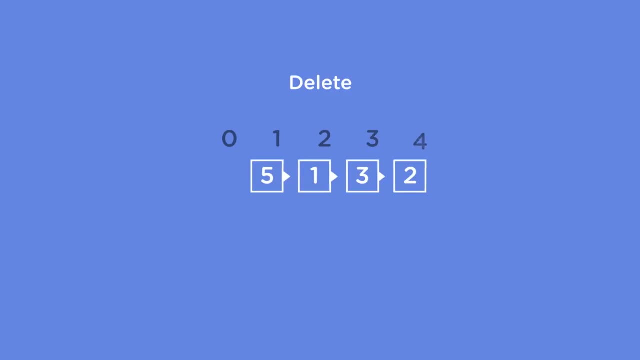 So where an insert shifts Every element to the right, A delete operation shifts every element to the left, Just like an insert as well. If we delete the first element In the list, Every single element in the list Needs to be shifted to the left. 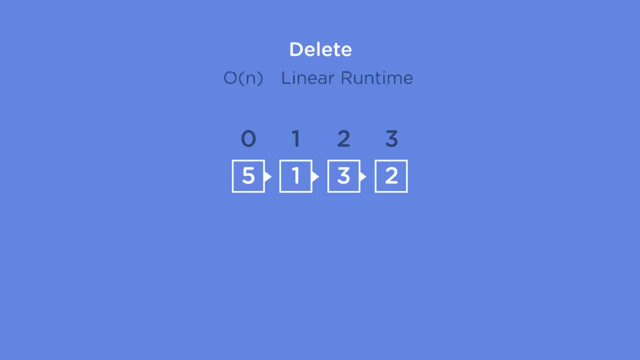 Delete operations have an upper bound Of big O of n, Also known as a linear run time. Now that we've seen how common operations work On a data structure That we're familiar with, Let's switch tracks And build our own data structure. 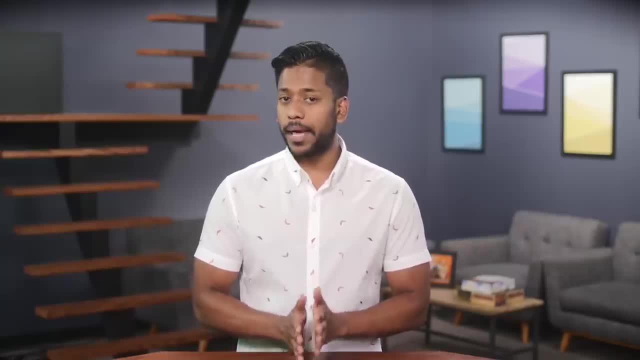 Over the next few videos, We're going to build a data structure That you may have worked with before- A linked list. Before we get into what a linked list is, Let's talk about why we build data structures Instead of just using the ones. 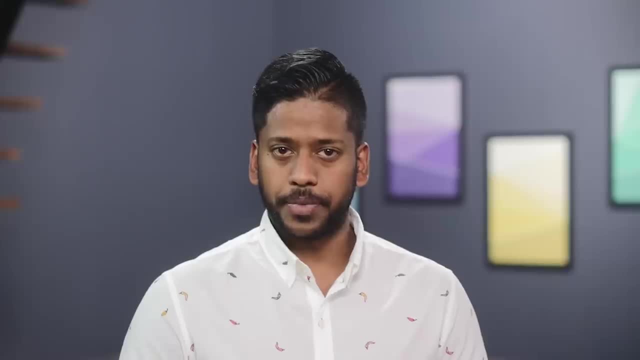 That come built into our languages. Each data structure solves a particular problem. We just went over the basics Of a linked data structure And looked at the cost of common operations That we carry out on arrays. We found that arrays were particularly good. 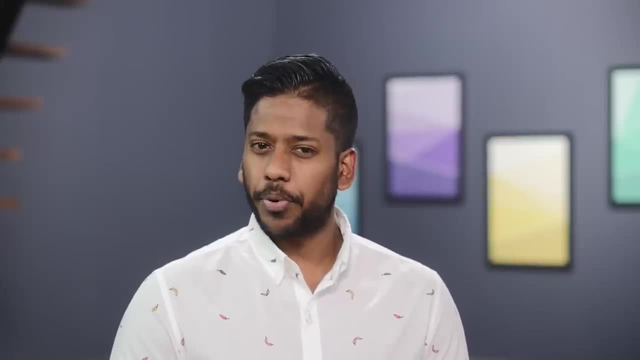 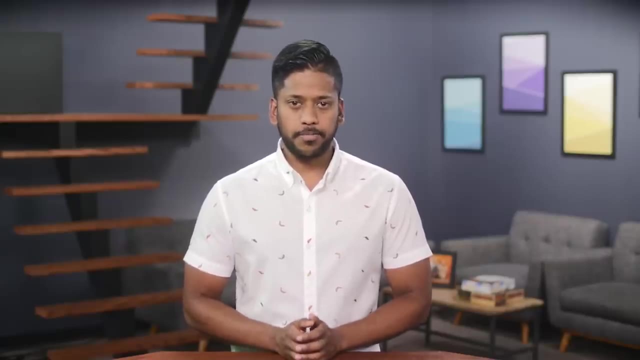 At accessing Reading values happens in constant time, But arrays are pretty bad at inserting and deleting, Both of which run in linear time. Linked lists, on the other hand, Are somewhat better at this, Although there are some caveats And if we're trying to solve a problem. 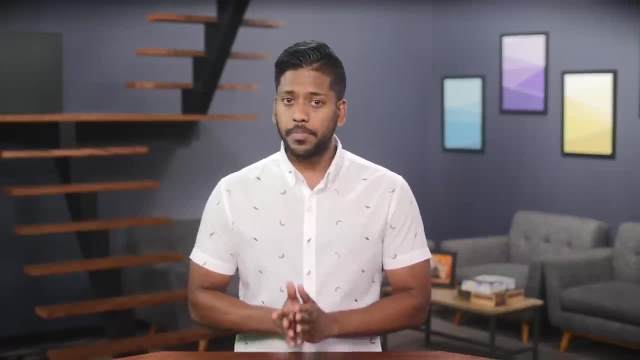 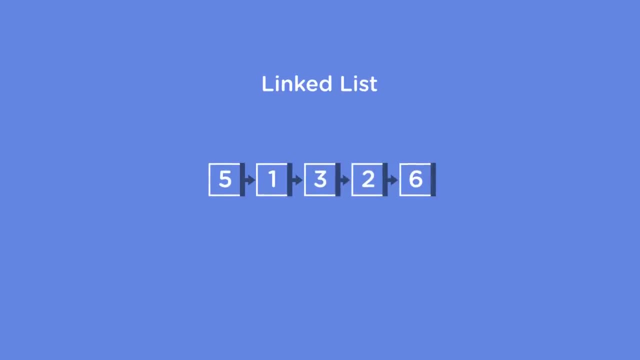 That involves far more inserts and deletes Than accessing. So what is a linked list? A linked list Is a linear data structure Where each element in the list Is contained in a separate object Called a node. A node models two pieces of information. 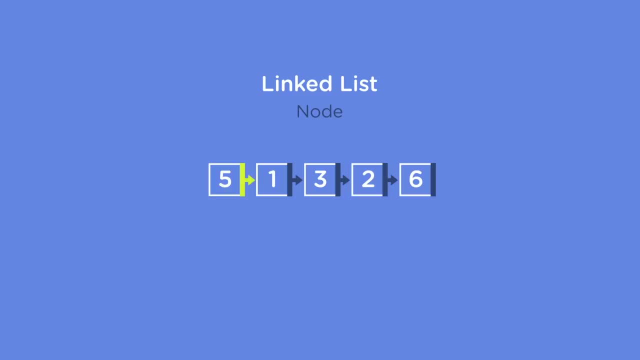 An individual item of the data We want to store And a reference to the next node in the list. The first node in the linked list Is called the head of the list, While the last node is called the tail. The head and the tail nodes are special. 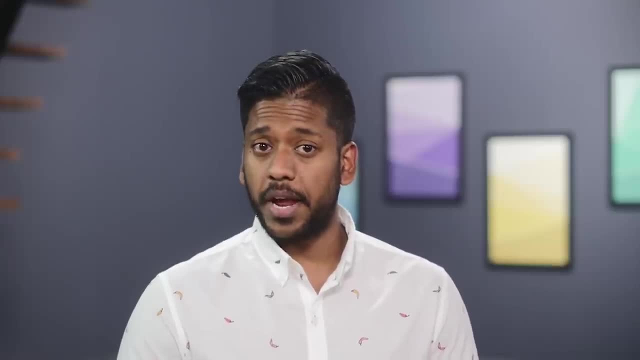 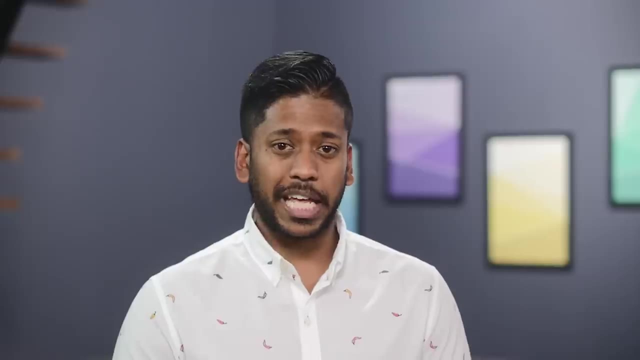 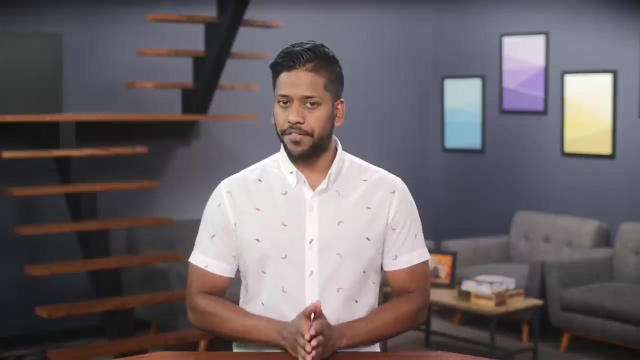 reference to node two, which we also need. for this reason, it's easier to decrease position to just one when it equals one and stop at node two. so in here we'll say: while position is greater than one, now, while the position is greater than one, we'll keep. 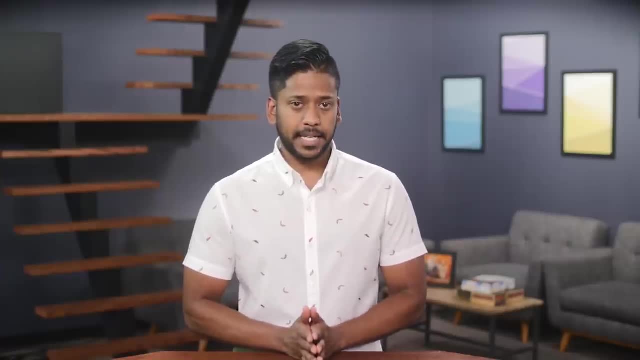 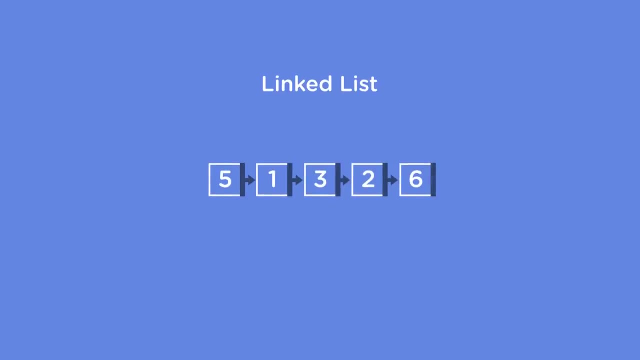 calling next node and reassigning the current node. so current equal node dot next node, and at the same time we'll decrement position, so position equal to position minus one, which you can also succinctly write as minus equal one. this way, when the position equals one, 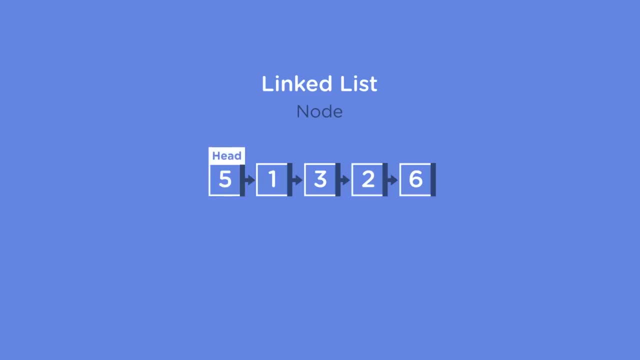 the loop exits, and current will refer to the node at the position before the insert point. so outside the while loop we'll say previous equal current and next equal current dot. next node. to make things more clear, what I've done here is name the node before the new one. 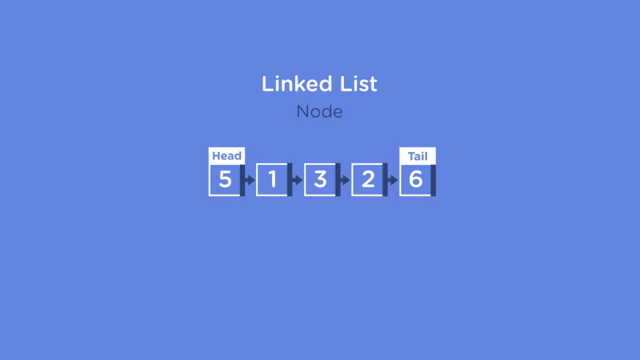 previous and the node after the new one next. all that's left to do now is to insert the new node between previous and next. so we'll say: previous dot, next node equal new, and then new dot, next node equal next. now it seems like there's an issue with 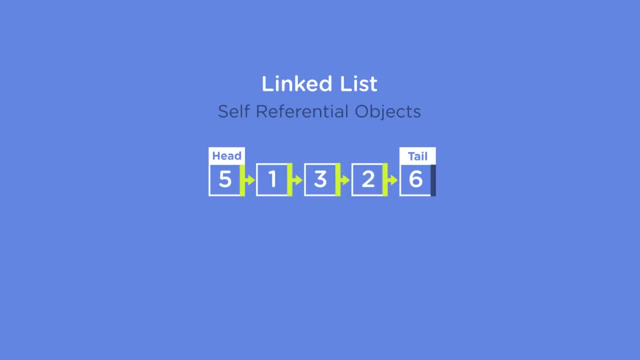 variable naming here and I'm most probably conflicting with some globally named next variable. so I should go ahead and call this next node and previous node, so that we don't mess things up here. previous node. so the dot next node is obviously the attribute on a node. 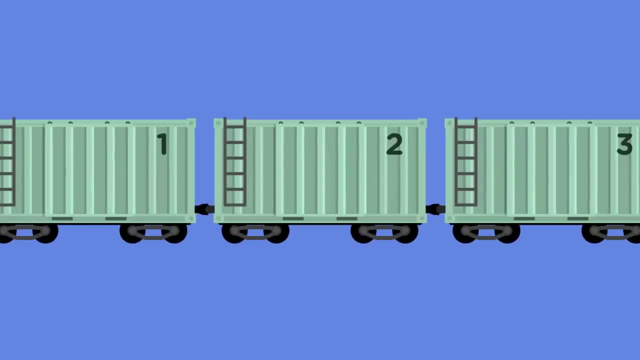 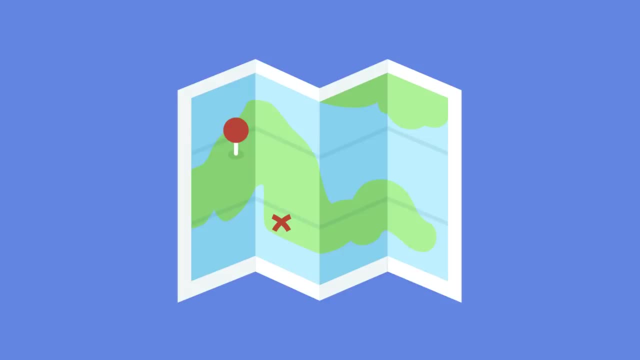 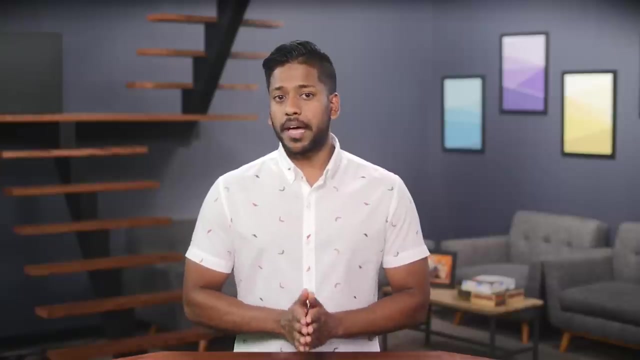 but this is just a local variable. let's document this method. so up at the top we'll add a doc string and it will say: inserts a new node containing data at index position. insertion takes constant time, but finding the node at the insertion point takes linear time. 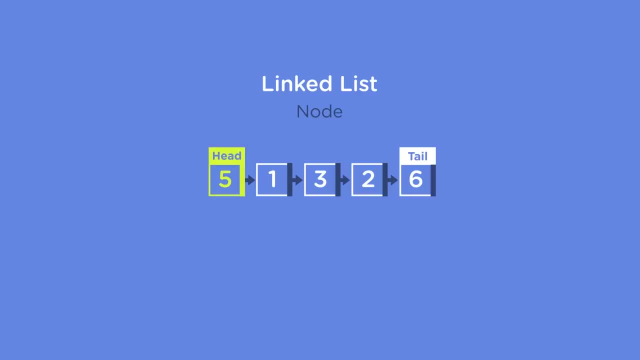 The list only works Because it only maintains a reference to the head, Although in some implementations It keeps a reference to the tail as well. This aspect of linked lists Is very important And, as you'll see, Most of the operations on the list. 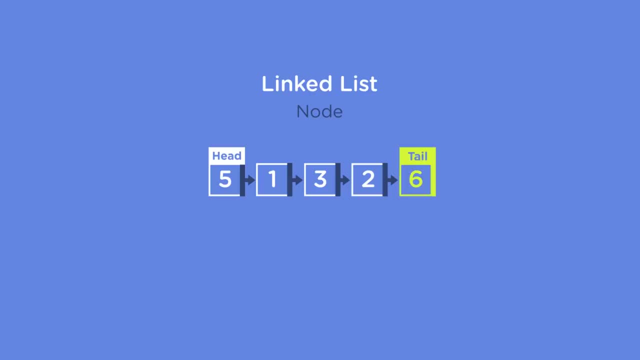 Need to be implemented quite differently. Compared to an array, The opposite of the head, The tail Denotes the end of the list. Every node other than the tail Points to the next node in the list, But tail doesn't point to anything. 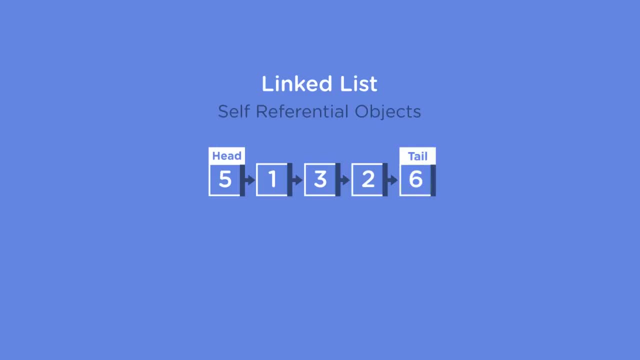 They're called self-referential objects. The definition of a node Includes a link to another node, And self-referential here Means the definition of node Includes the node itself. Linked lists often come in two forms: A singly linked list. 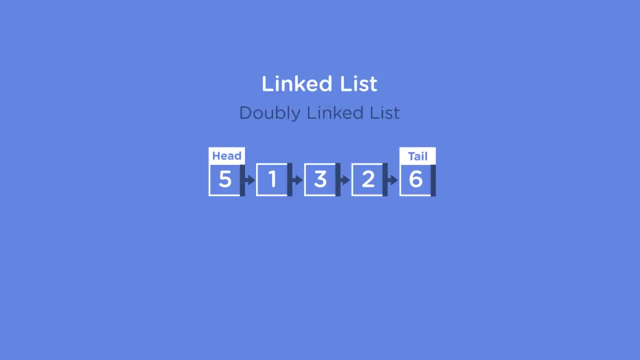 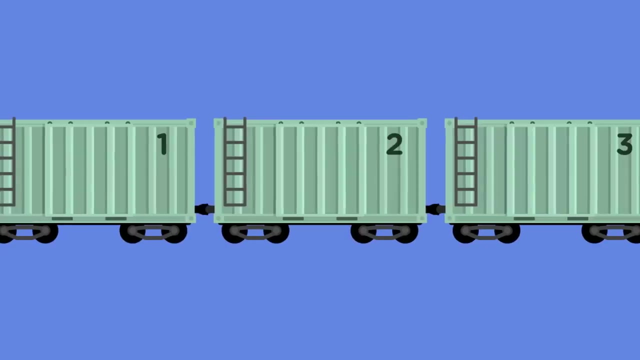 Where each node stores a reference To the next node in the list. Or a doubly linked list Where each node stores a reference To both the node before and after, If an array is a train With a bunch of cars in order. 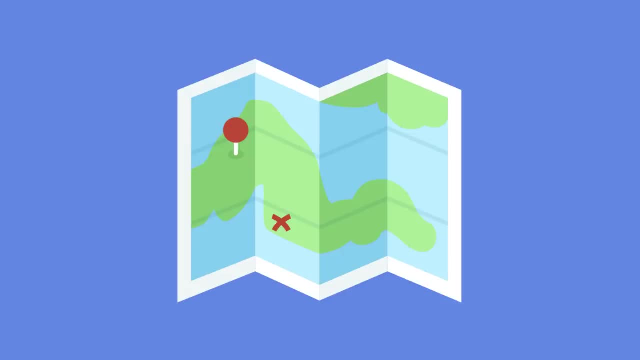 Like a treasure hunt. When you start the hunt, You have a piece of paper With the location of the first treasure. You go to that location And you find an item Along with the location to the next item of treasure. When you finally find an item, 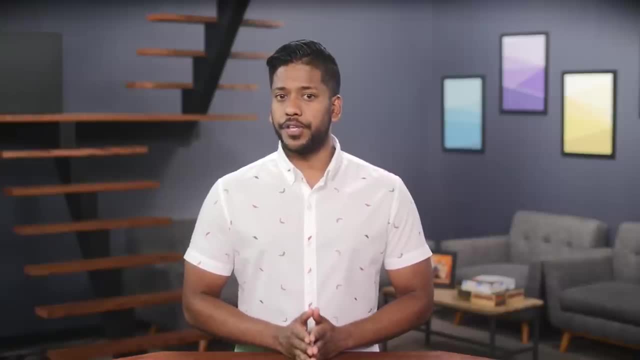 That doesn't also include a location. You know that the hunt has ended. Now that we have a high level view Of what a linked list is, Let's jump into code and build one together. We'll focus on building a singly linked list. 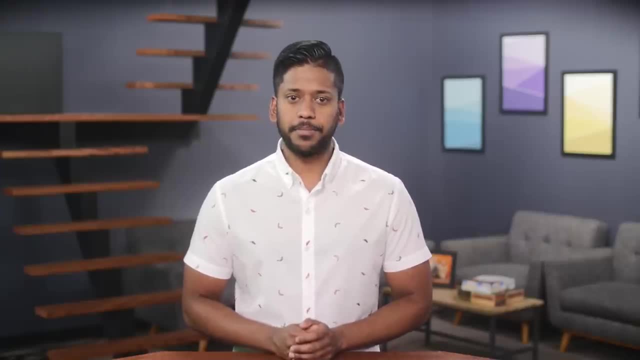 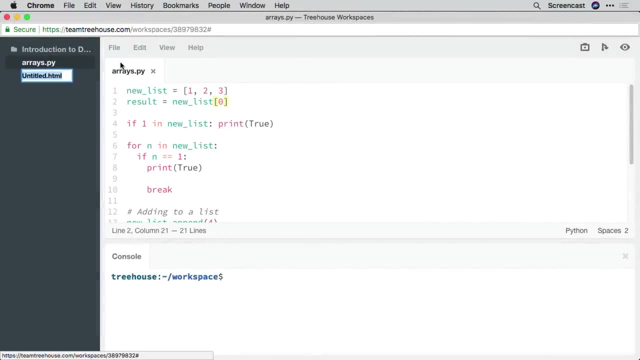 For this course. We don't want to get ahead of ourselves. Let's start here By creating a new file Where we're going to put all our code For our linked list. So we'll call this linked underscore list Dot pi. 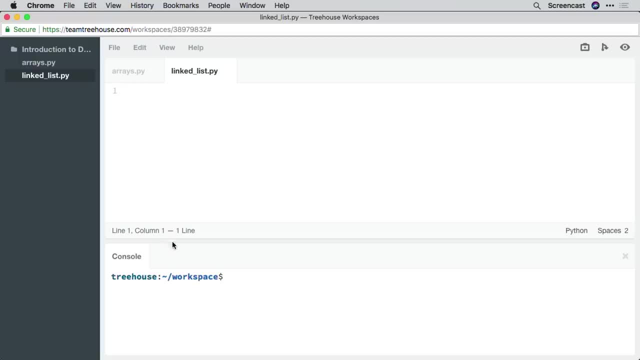 And first We're going to create a class To represent a node, Say class Node. Now, node is a simple object In that it won't model much, So first we'll add A data variable. It's an instance variable here. 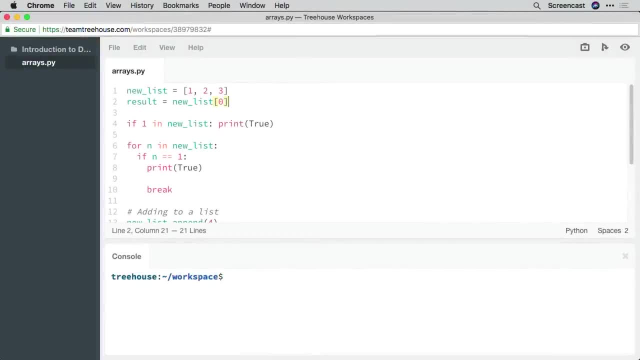 let's add this to the next line. there we go and then we'll say: therefore, it takes an overall linear time. this is why, even though we can easily insert a new node without having to shift the rest, ultimately adding to either the head or the tail, if you have a reference, is much. 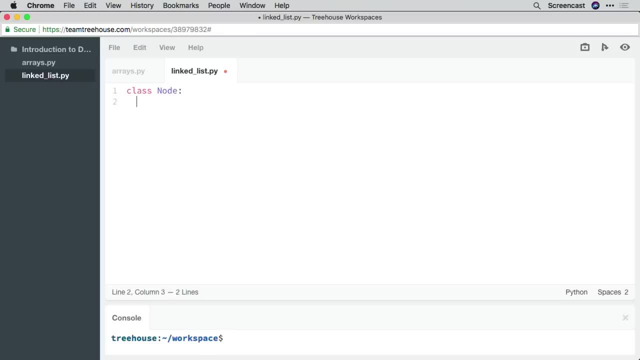 more efficient. we have one more operation to add to our linked list that will make it a robust data structure. much like inserts, removing a node is actually quite fast and occurs in constant time. but to actually get to the node that we want to remove and modify the next connections: 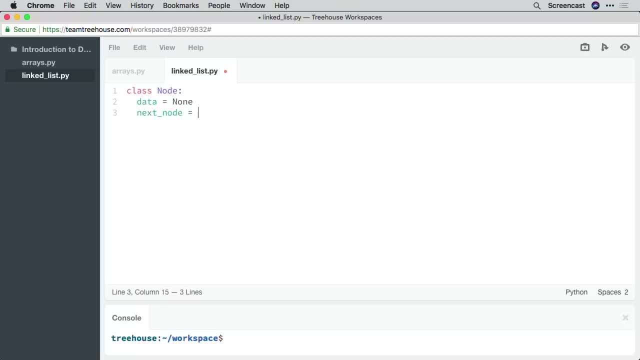 we need to traverse the entire list in our worst case. so in the worst case, this takes linear time. let's add this operation to our data structure. there are two ways we can define the remove method: one where we provide a key to remove as an argument, and one where we provide an index. 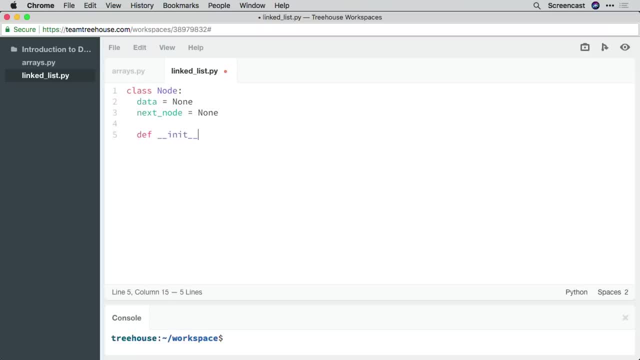 now, in the former, the key refers to the data the node stores. so in order to remove that node, we would first need to search for data that matches the key. I'm going to implement that first method, which we'll call remove, and I'll leave it up to you to get some practice. 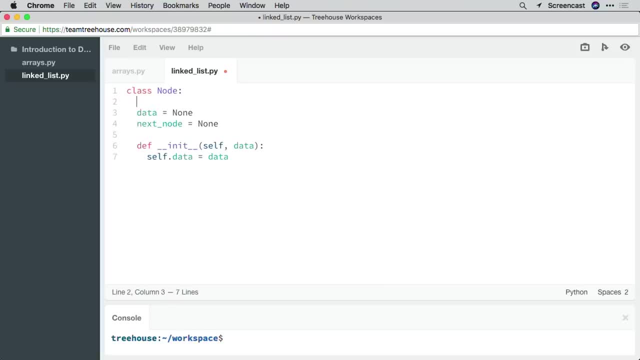 in and implement a remove at index method to complete our data structure. so we'll add this after the insert method right here. remove is going to accept a key which we'll need to search for before we can remove a node. earlier we defined a search method that found a node. 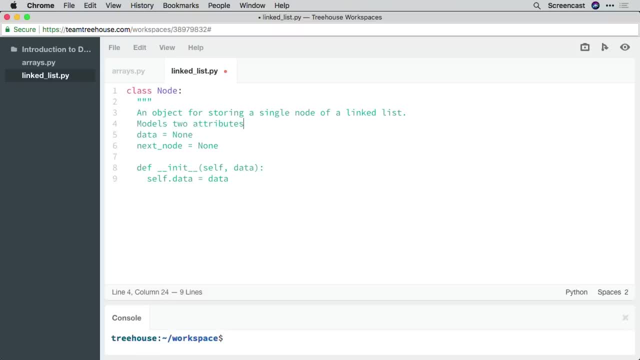 containing data that matches a key, but we can't use that method, as is for the implementation of remove. when we remove a node, much like the insert operation, we need to modify: the next node references. the node before the match needs to point to the node after the match. 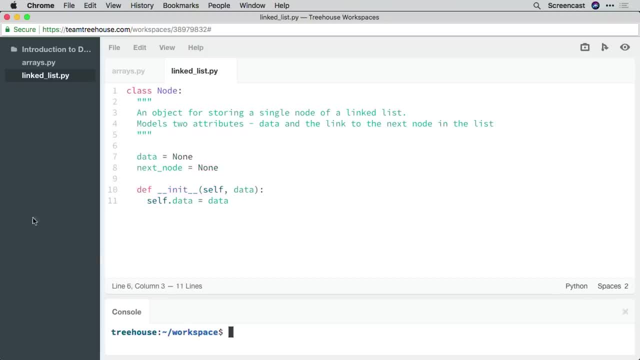 if we use the search method we defined earlier, we get the node we want to remove as a return value, but because this is a singly linked list, we can't obtain a reference to the previous node. like I said earlier, if this was a doubly linked list, we could use the search method. 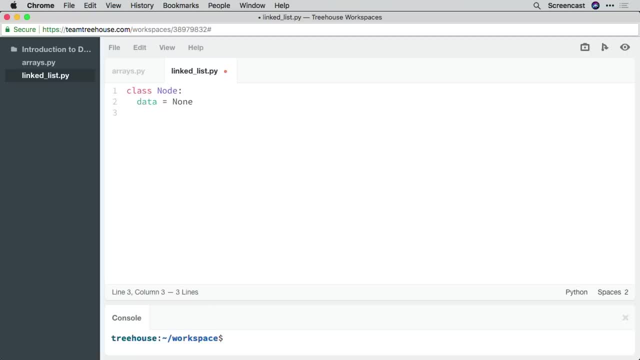 Called data And we'll assign the value none initially, And then we'll add one more. We'll call this next node And to this we'll assign none as well. So we've created two instance variables- Data- to hold on to the data that we're storing. 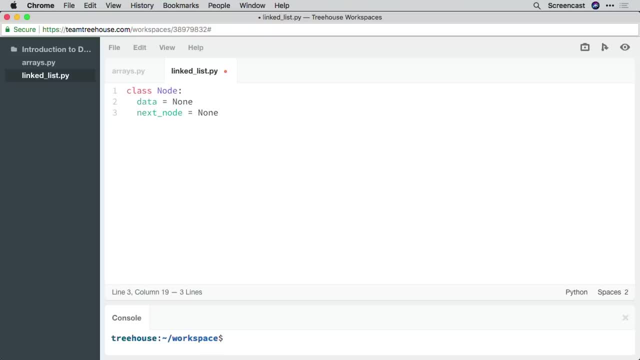 And next node. To point to the next node In the list, Now we need to add a constructor To make this class easy to create. So we'll add an init That takes self And some data to start off, And all we're going to do is assign. 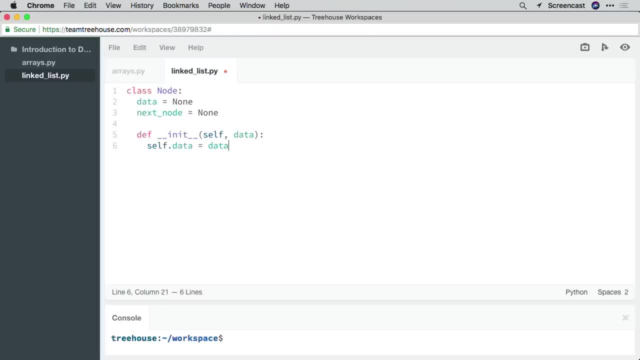 Data to that instance variable We created. So that's all we need to model node. Before we do anything else, though, Let's document this. So, right after the class definition, Let's create a doc string. So three quotes Next line and we'll say an object. 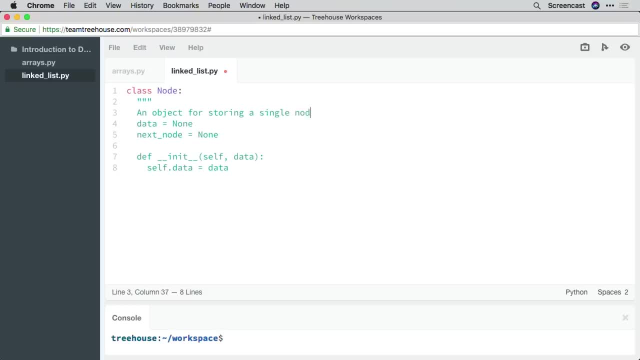 For storing A single node Of a linked list And then on the next line We'll say models Two attributes, Data And The link To the next node In the list, And then we'll close this doc string off. 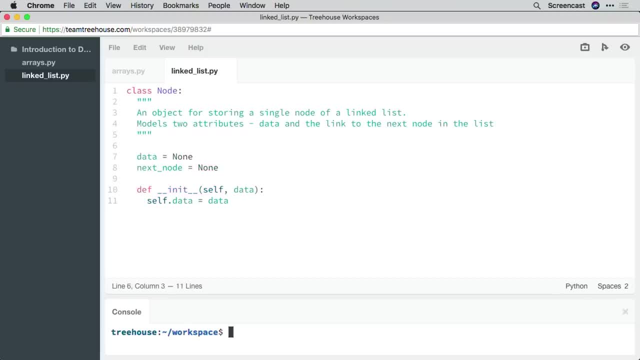 With three more quotation marks. Okay, using the node class Is fairly straight forward, So we can create a new instance of node With some data to store. Now, the way we're going to do this Is we're going to type out: 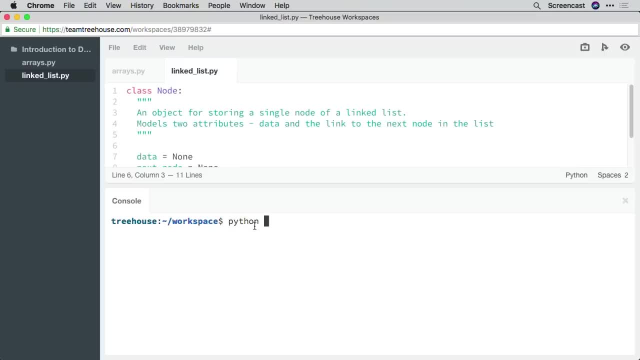 Like we've been typing out before: Python, followed by the name of the script that we wrote, Which is linked list. Linked underscore, list dot pi. But before we do that, We're going to pass an argument to the python command. We're going to say dash or python. 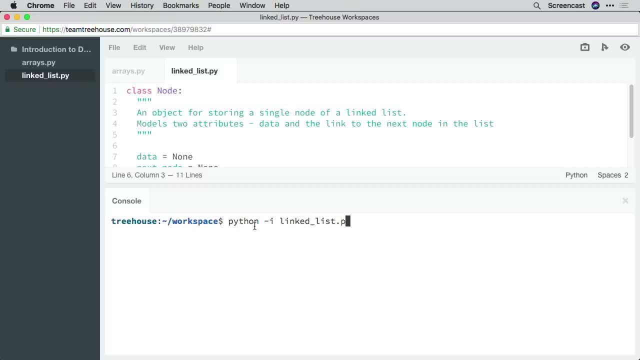 I and then the name of the script Linked underscore list dot pi. So what this does Is this is going to run the python repl, The read, evaluate print loop In the console, But it's going to load the contents of our file. 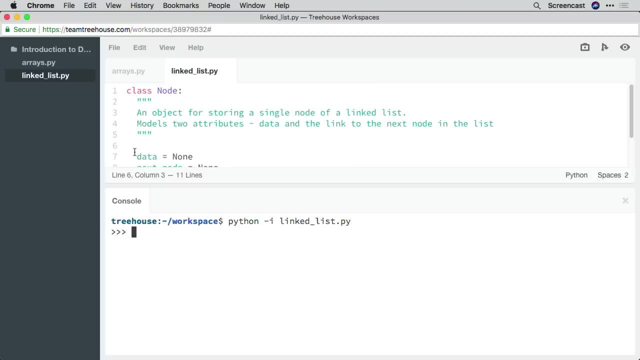 Into that so that we can use it. So I'll hit enter And we have a new instance going And now we can use the node in here So we can say n1, equal node, And since we defined that constructor, We can pass it some data. 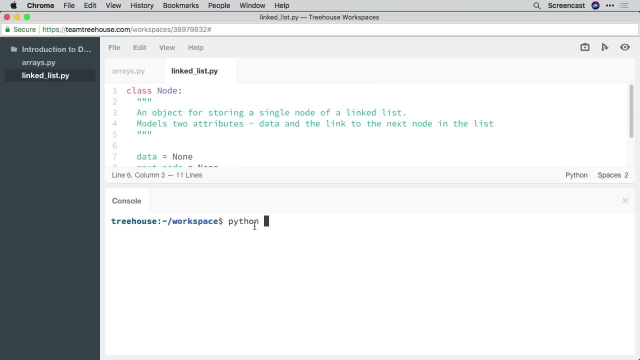 since we would have a reference to that previous node, we'll start here by setting a local variable named current to point to the head. let's also define a variable named previous that we'll set to none to keep track of the previous node as we traverse the list. 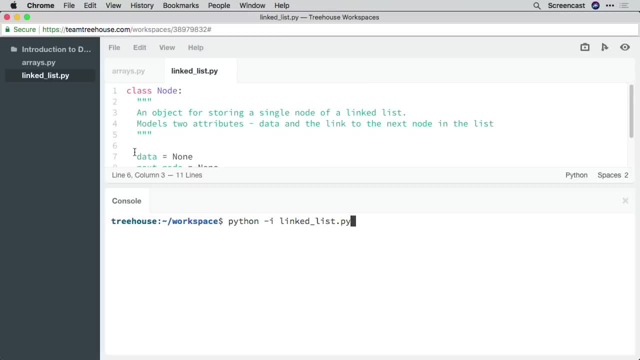 finally, let's declare a variable named found that we'll set to false. found is going to serve as a stopping condition for the loop that we'll define. we'll use the loop to keep traversing the linked list as long as found is false, meaning we haven't found the key that we're 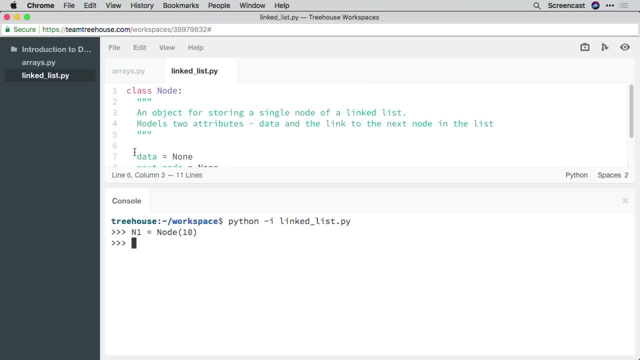 looking for once we found it, we'll set found to true and the loop terminates. so let's set up our loop. so we'll say: while current and not found. here we're defining a while loop that contains two conditions. first, we tell the loop to keep iterating. 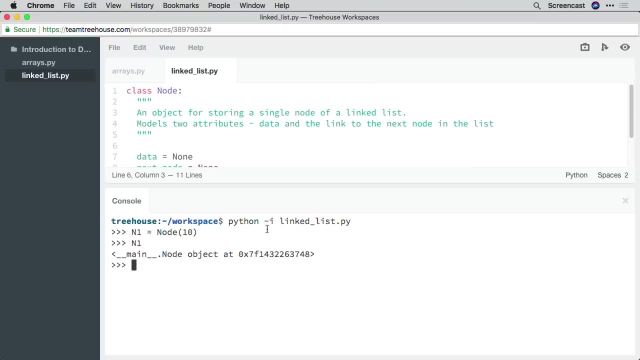 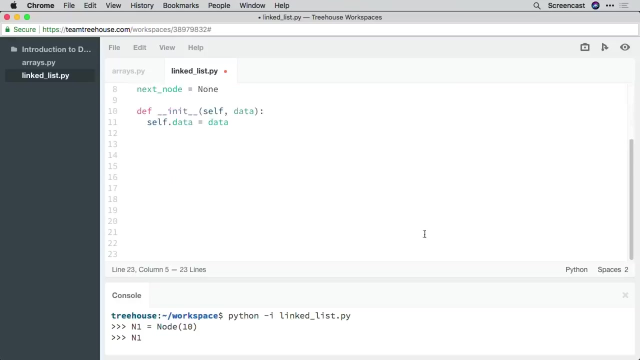 as long as current does not equal none. when current equals none, this means we've gone past the tail node and the key doesn't exist. the second condition asks the loop to keep evaluating as long as not found equals true. now this might be tricky because it involves a negation here. 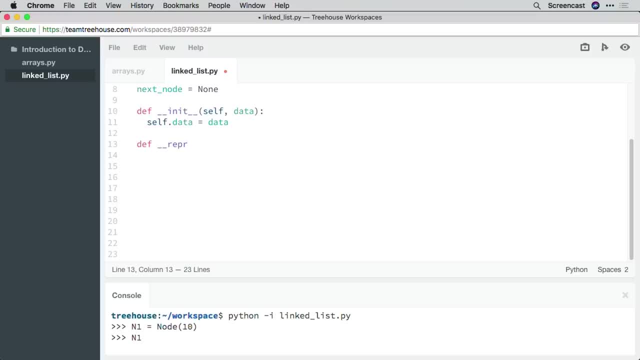 right now, found is set to false, so not found, not false equals true. this not operator flips the value. when we find the key and we set found to true, not true, not found will equal false then and the loop will stop. the and in the while loop means that both conditions current. 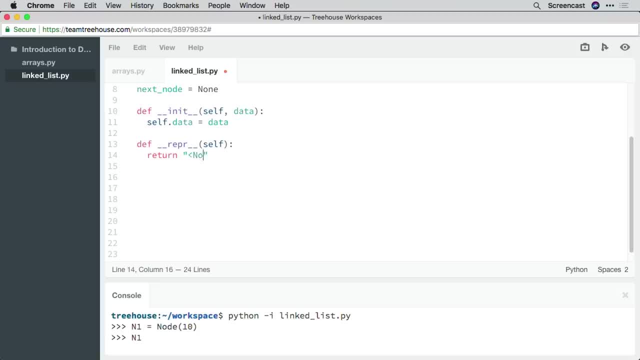 being a valid node and not found equaling true. both have to be true. if either one of them evaluates to false, then the loop will terminate. now, inside the loop, there are three situations that we can run into. first, the key matches the current node's data and 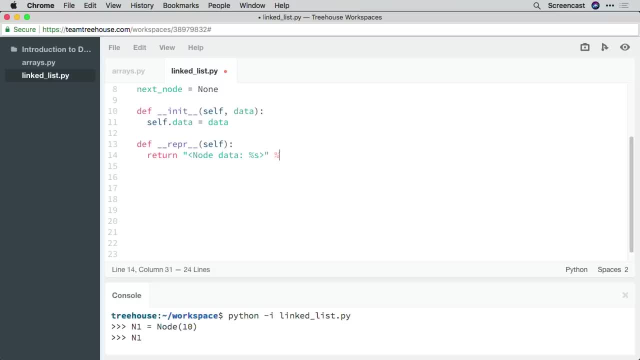 current is still at the head of the list. this is a special case because the head doesn't have a previous node and it's the only node being referenced by the list. let's handle this case so we'll say: if current dot data double equals the key and 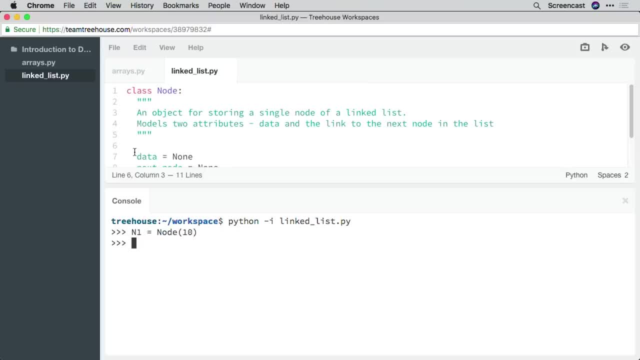 So we'll say 10 here. Now, if we try to inspect this object, The representation return isn't very useful, Which will make things Really hard to debug As our code grows. So, for example, if I type out n1. You'll see that we have a valid instance here. 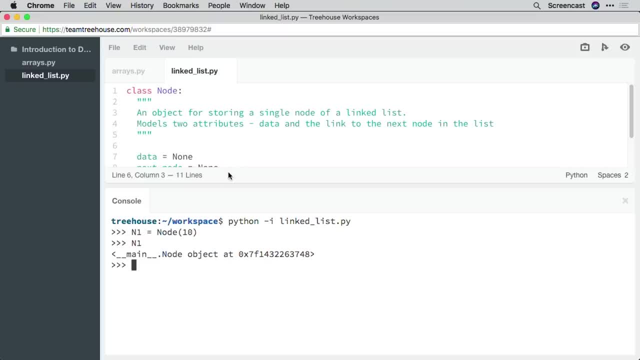 Which is not very helpful The way it's printed out. So we can customize this By adding a representation of the object Using the repr function. Now in the terminal, still, we'll type out exit Like that: Hit enter To exit the console. 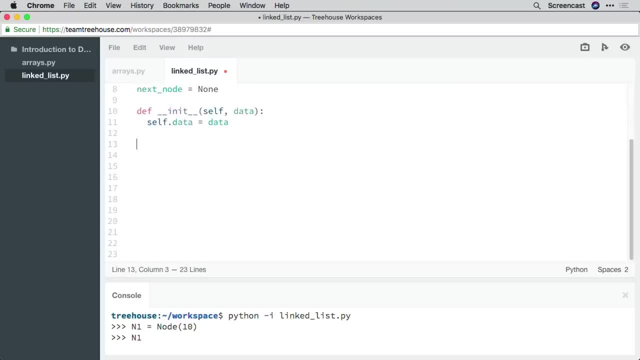 And then down here Let's add in some room, Okay, and here we'll say: def- Double underscore, Repr- Another set of double underscores, And in here we can provide a String representation Of what we want printed to the console. 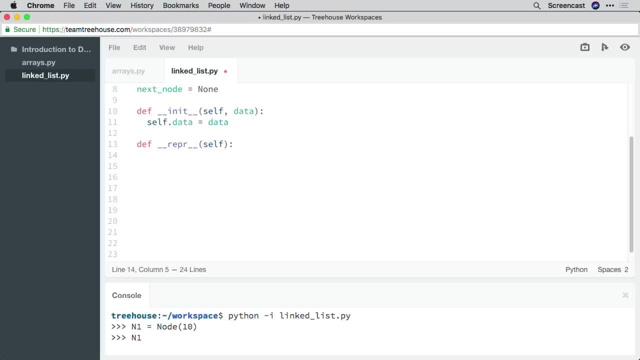 When we inspect that object Inside of it, Inside of the console, So here we'll say return. Again, this is a string representation. So inside quotes we'll say node. So this represents a node instance And the data it contains. Here we'll say percent s. 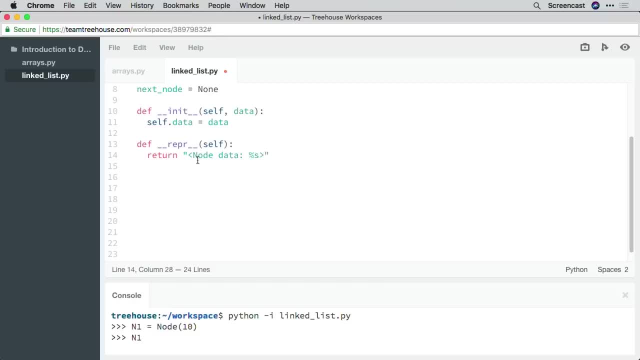 Which is a Python way of substituting something Into a string- String- interpolation- And outside of the string we can say percent again. And here we're saying We want to replace this percent s With selfdata. Okay, Let's hit save. 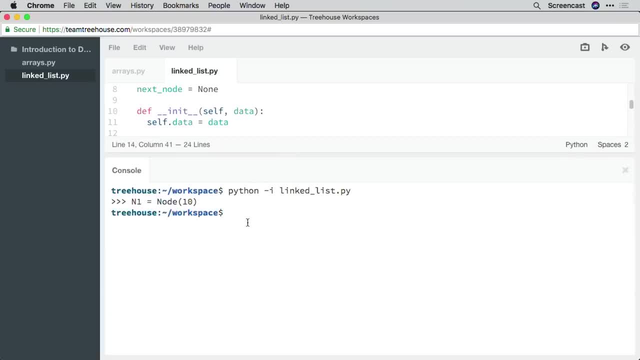 And before we move on, let's verify that this works. So I'm going to come in here, Type clear To get rid of everything, And then we'll do what we did again, And you can just hit the up arrow a couple times. 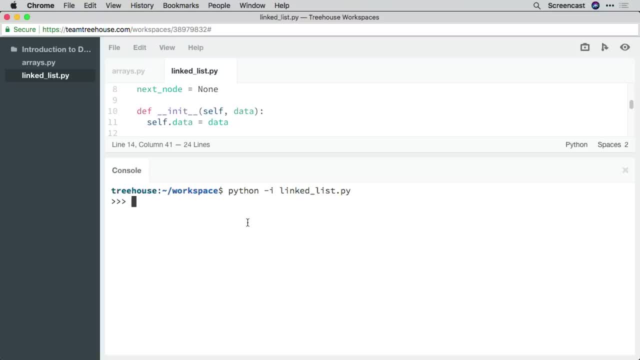 To get that command Alright. so hit enter. You start off from scratch. So n1 that we created earlier Not there anymore, So let's go ahead and create it. n1 equal node 10. And we can type n1 again and hit enter. 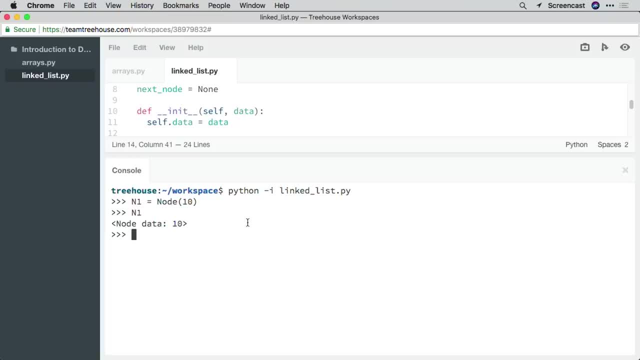 And you have a much better representation now. So we can see that we have a node And it contains the data 10. We can also create another one n2 equal node that contains the data 20.. And now we can say: 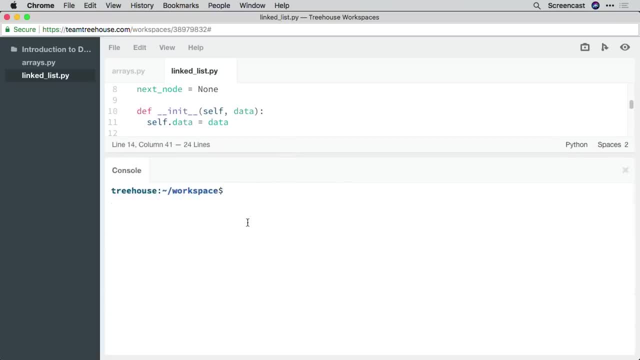 current is self dot head, which you can write out as current equals self dot head or current is self dot head. now, if we hit this case, we'll indicate that we found the key by setting found to true and then this means that on the next pass, this is going to evaluate to false. 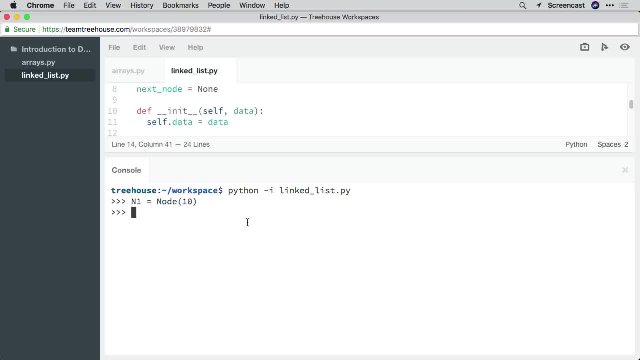 because not true will be false and then the loop terminates. once we do that, we want to remove the current node and since it's the head node, all we need to do is point head to the second node in the list, which we can get by referencing the. 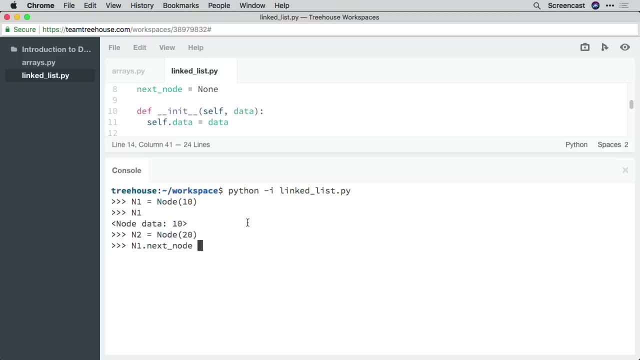 next node. attribute on current self dot head: equal current dot next node. so when we do this, there's nothing pointing to that first node, so it's automatically removed. the next scenario is when the key matches data in the node and it's a node that's not the head. 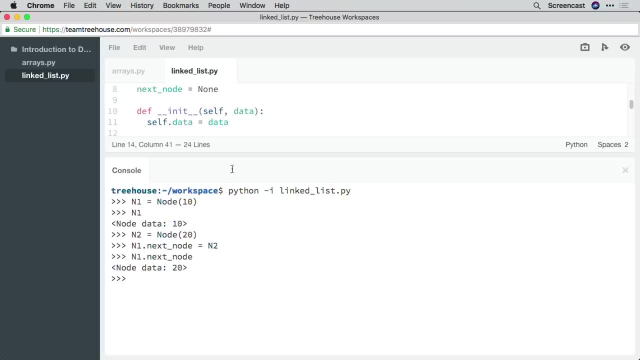 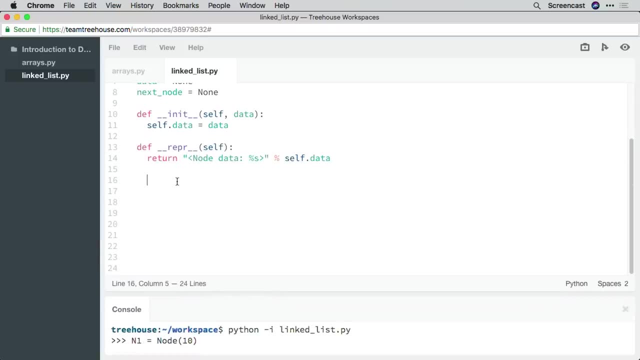 so here we'll say else. if current dot data equal key, if the current node contains the key we're looking for, we need to remove it. to remove the current node, we need to go to the previous node and modify its next node reference to point to the node after current. 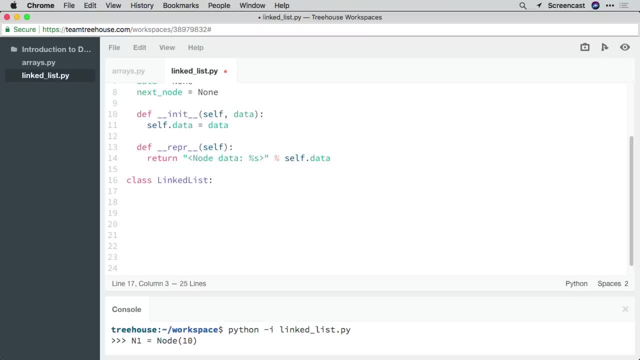 but first we'll set found to true and then we'll switch out the references. so: previous dot, next node, equal current dot, next node. so far we haven't written any code to keep track of the previous node. we'll do that in our else case here. so if we hit the else case, 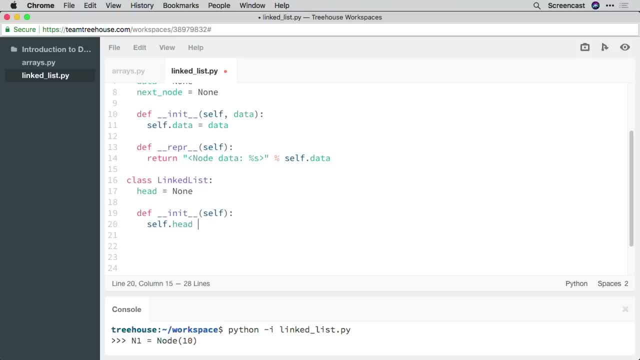 it means that the current node we're evaluating doesn't contain the data that matches the key. so in this case we'll make previous point to the current node and then set current to the next node. so previous equal current and current equal current dot next node, and that's it. 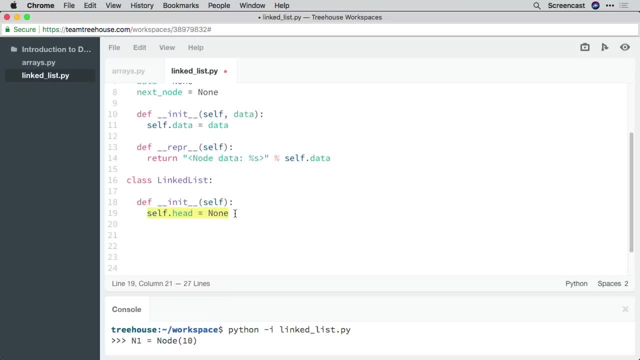 for the implementation of remove. now we're not doing anything at the moment with the node we're removing, but it's common for remove operations to return the value being removed. so at the bottom outside the while loop, let's return current and with that we have a minimal implementation. 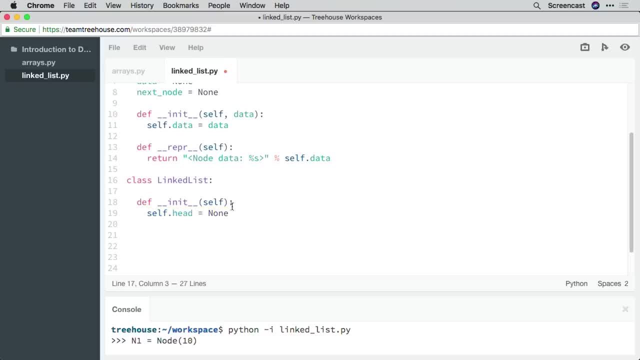 of a linked list and your first custom data structure. how cool is that? there's quite a bit we can do here to improve our data structure, particularly in making it easy to use, but this is a good place to stop before we move on to the next topic. 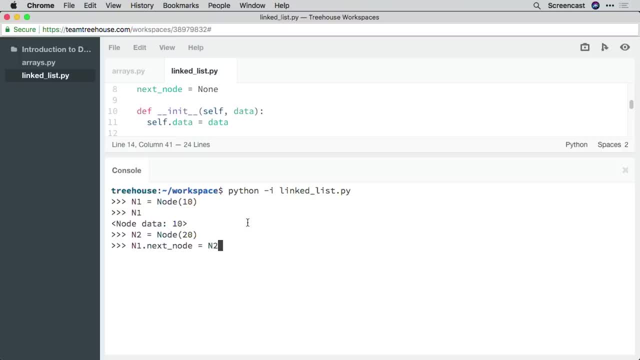 n1 dot next node, Equal n2.. So n1 now points to n2.. So we say n1 dot next node. You'll see that it points To that node, The node containing 20.. Nodes are the building blocks for a list. 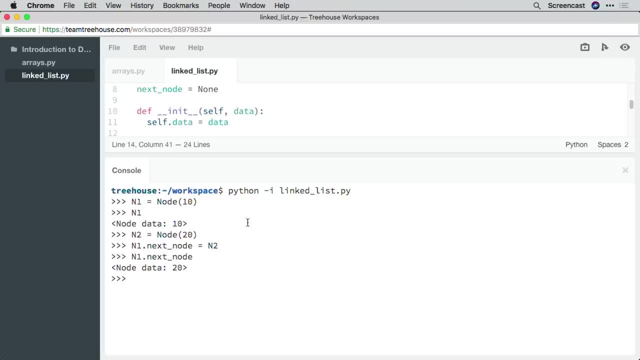 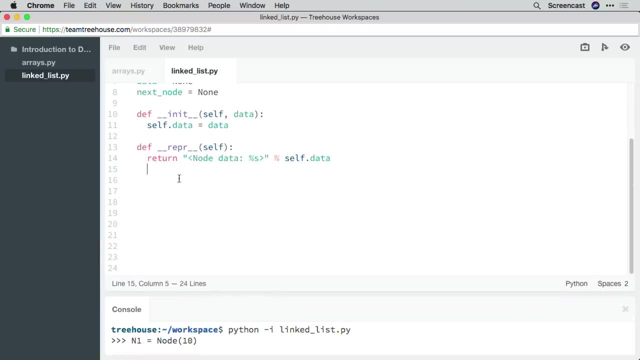 And now that we have a node object, We can use it to create a singly linked list. So again, I'm going to exit out of this And then go back to the text editor And here We'll create a new class. So, class linked list. 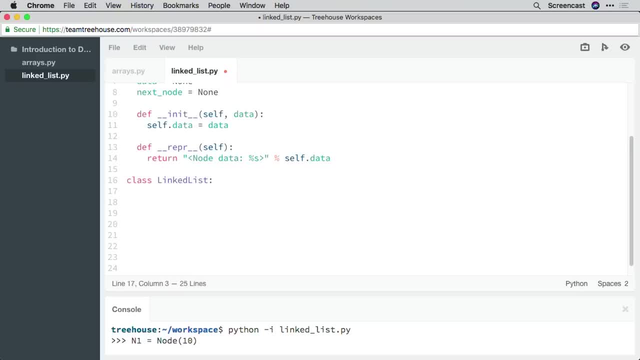 The linked list class Is going to define a head, And this attribute models The only node that the list is going to have a reference to. So here we'll say head And we'll assign none initially And then, like we did earlier, 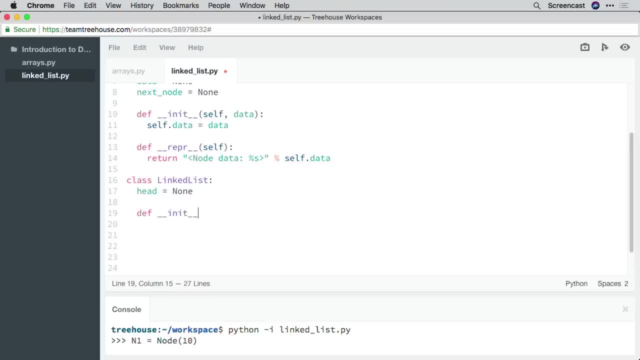 Let's create a constructor. So double underscore, init. Double underscore. This takes self And then inside, Like before, we'll say self dot, head, Equal none. This is the same as doing this, So we can actually get rid of that. 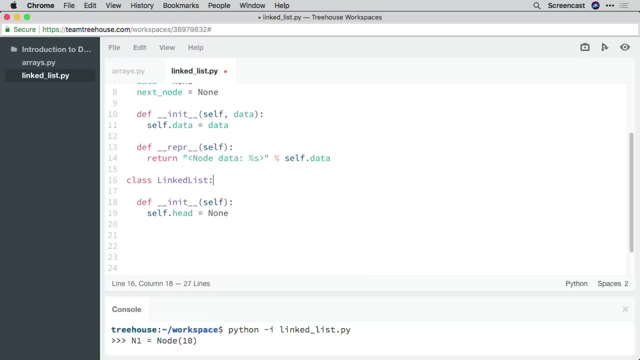 And just use the constructor. Okay, so again, This head attribute models the only node That the list will have a reference to. Since every node Points to the next node, To find a particular node We can go from one node to the next. 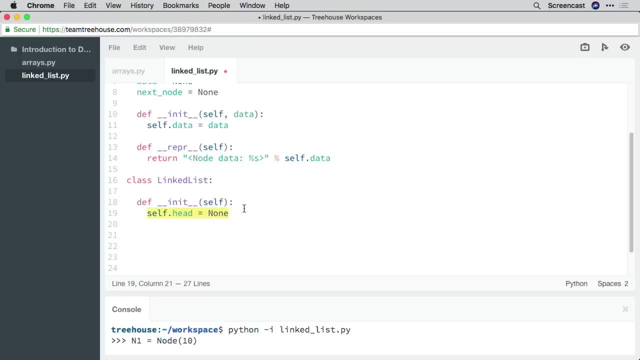 In a process called list traversal. So in the class constructor here We've set the default value of head to none, So that new lists created Are always empty Again. you'll notice here That I didn't explicitly declare the head attribute. 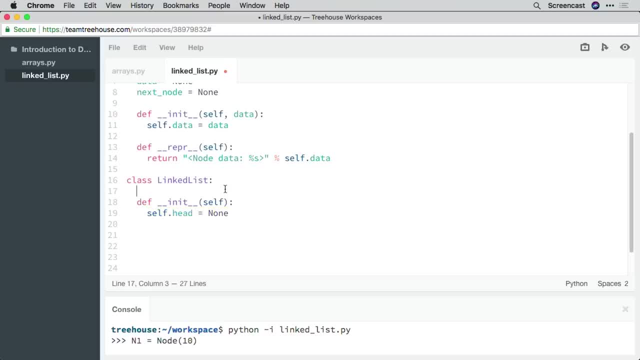 At the top of the class definition. Don't worry, that's not an oversight. The self dot head in the initializer Means that it's still created. Okay, so that's all there is to modeling A linked list. Now we can add methods that make it easier. 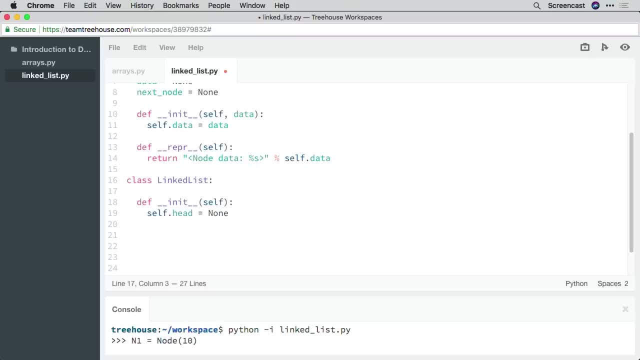 To use this data structure. First a really simple doc string To provide some information. So here we'll create a doc string, Three quotation marks, And then we'll say singly linked list And then close it off. A common operation carried out. 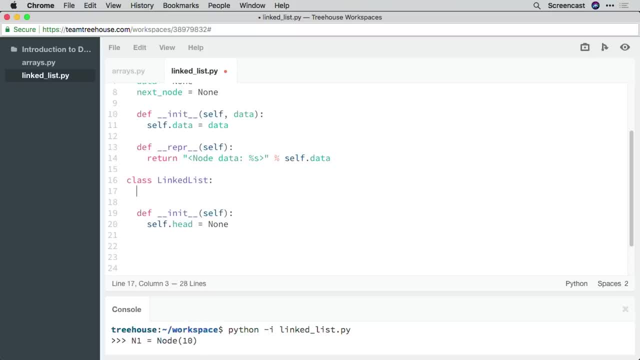 let's document our method. so the top another doc string here we'll say, removes node containing data that matches the key. also, it returns the node or none if the key doesn't exist. and finally, this takes linear time because in the worst case scenario we need to search the entire. 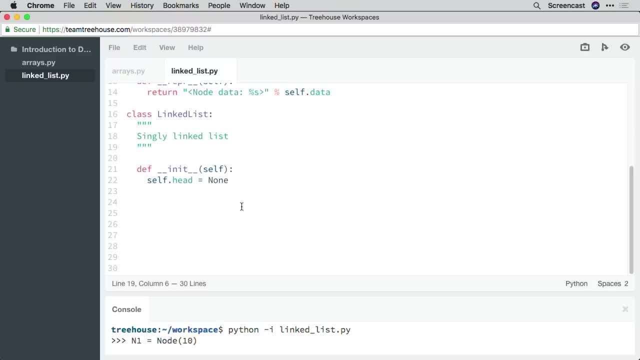 list. if you'd like to get in some additional practice implementing functionality for linked lists, two methods you can work on are remove it index and node at index to allow you to easily delete or read values in a list at a given index. now that we have a linked list, let's talk about 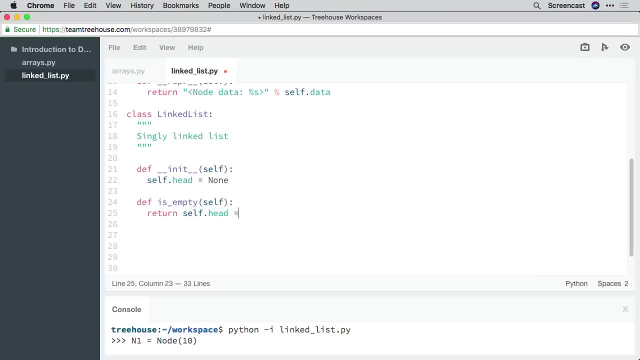 where you can use them. the honest answer is not a lot of places. linked lists are really useful structures to build for learning purposes because they're relatively simple and are a good place to start to introduce the kinds of operations we need to implement for various data structures. it is 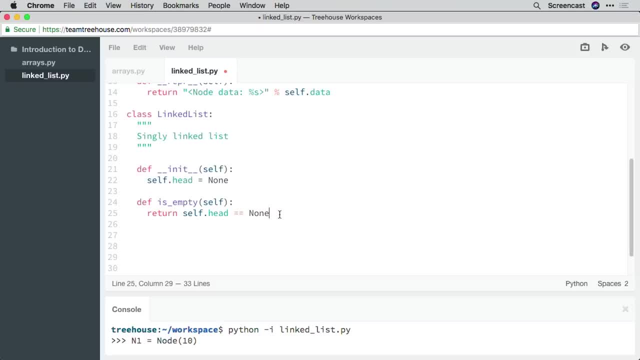 quite rare, however, that you will need to implement a linked list on your own. there are typically much better- and by that i mean much more efficient- data structures that you can use. in addition, many languages, like java, for example, provide an implementation of a linked list already. now that we have a 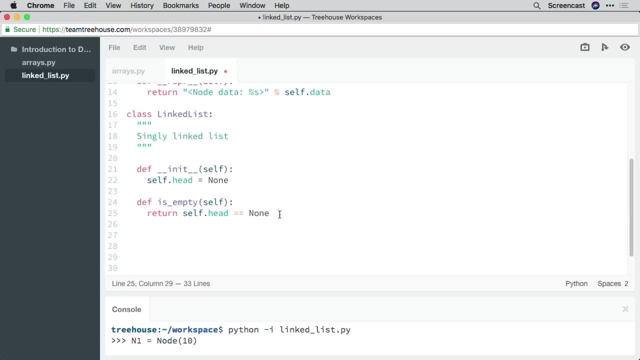 custom data structure. let's do something with it. let's combine the knowledge we have and look at how a sorting algorithm can be implemented across two different data structures. now that we've seen two different data structures, let's circle back and apply what we know about algorithms to these new concepts. 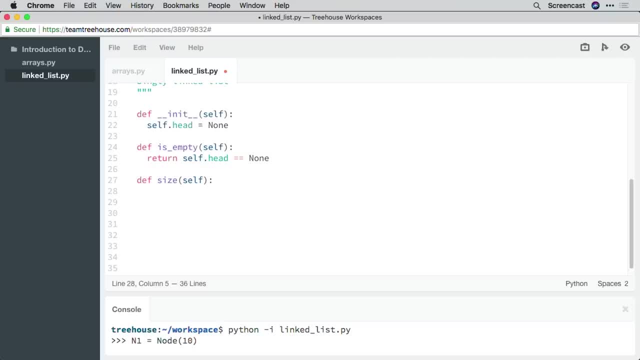 one of the first algorithms you learned about was binary search, and we learned that with binary search, there was one precondition: the data collection needs to be sorted. over the next few videos, let's implement the merge sort algorithm, which is one of many sorting algorithms, on both arrays or python. 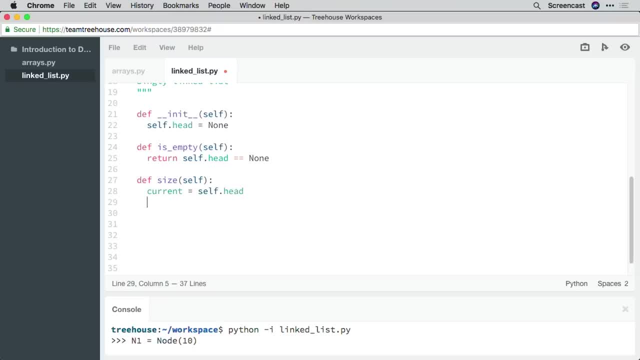 lists and the singly linked list we just created. this way, we can learn a new sorting algorithm that has real-world use cases and see how a single algorithm can be implemented on different data structures. before we get into code, let's take a look at how merge sort works conceptually and we'll use 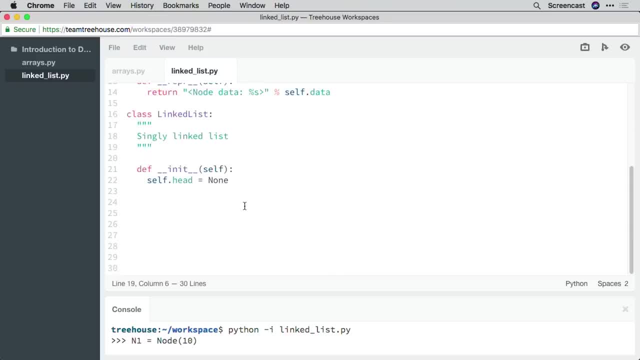 On data structures By defining whether it contains any data Or whether it's empty At the moment. to check if a list is empty, We would need to query These instance- variables, Head and so on- every time. Ideally, we would like to not expose. 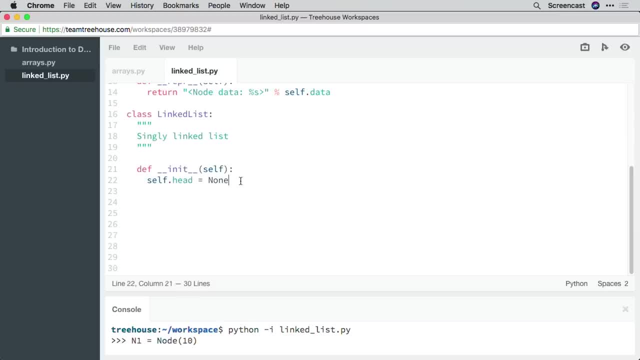 The inner workings of our data structure To code that uses it. Instead, let's make this operation More explicit by defining a method. So we'll say def is empty, And this method Takes self as an argument, And here we'll say return. 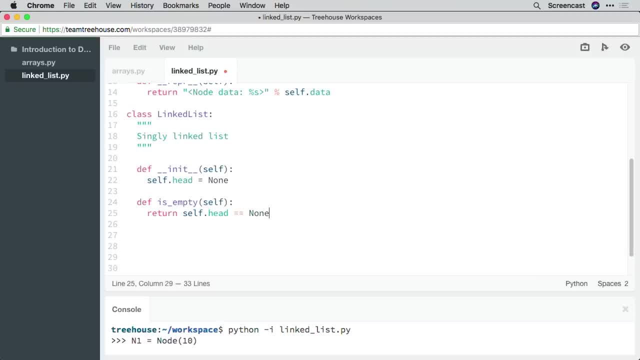 Self dot head Double equal none. All we're doing here Is checking to see if head is none. If it is, This condition evaluates to true, Which indicates the list is empty. Now, before we end this video, Let's add one more convenience method. 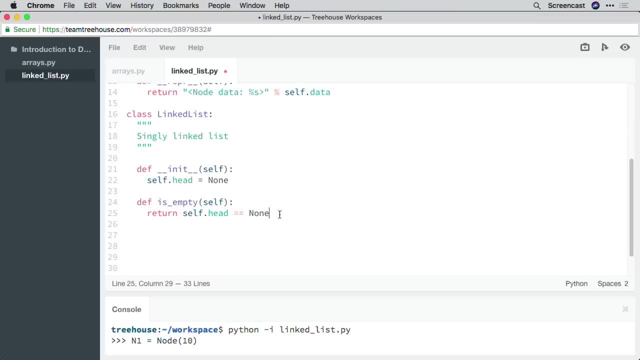 To calculate the size of our list. The name convenience method Indicates that what this method is doing Is not providing any additional functionality That our data structure can't handle right now, But instead making existing functionality To use. We could calculate the size of our linked list. 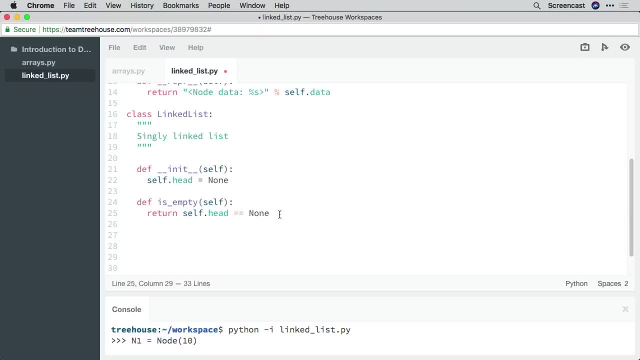 By traversing it every time using a loop Until we hit a tail node, But doing that every time is a hassle. Okay, so we'll call this method Size, And as always, it takes self, Unlike calling len On a python list. 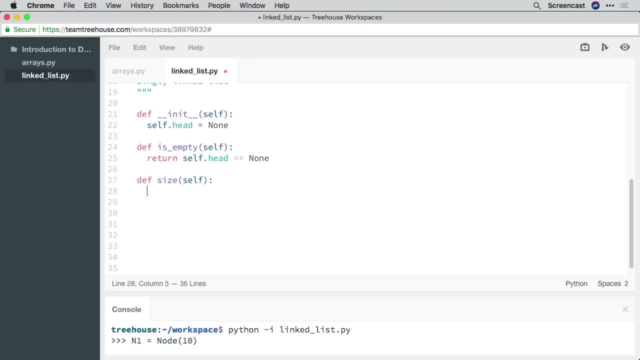 Not to be confused with a linked list, Which is a constant time operation. Our size operation is going to run In linear time. The only way we can count how many items we have Is to visit each node And call next, Until we hit the tail node. 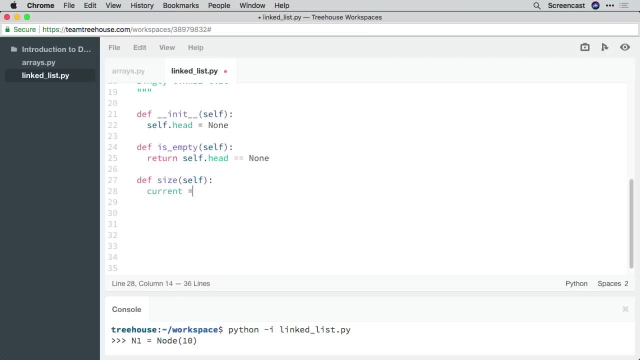 So we'll start by getting a reference to the head. We'll say current Equal selfhead. Let's also define a local variable, Named count, with an initial value of zero That will increment Every time we visit a node. Once we hit the tail, 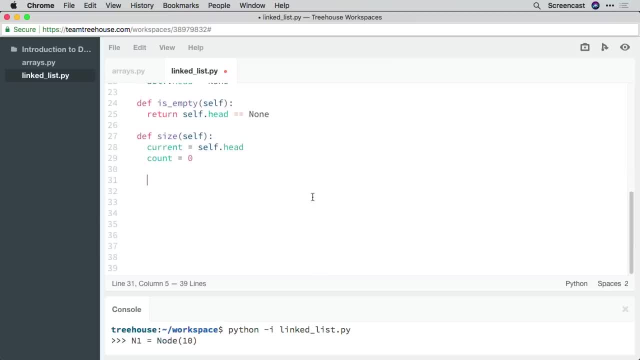 Count will reflect the size of that list. Next, We'll define a while loop And we'll keep going Until there are no more nodes. So we'll say while current, While current is the same as writing out, While current does not equal none. 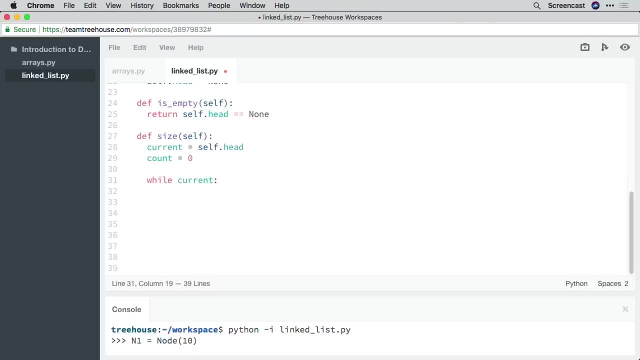 an array to work through this. we start with an unsorted array of integers and our goal is to end up with an array sorted in ascending order. merge sort works like binary sort by splitting up the problem into sub problems, but it takes the process one step further. 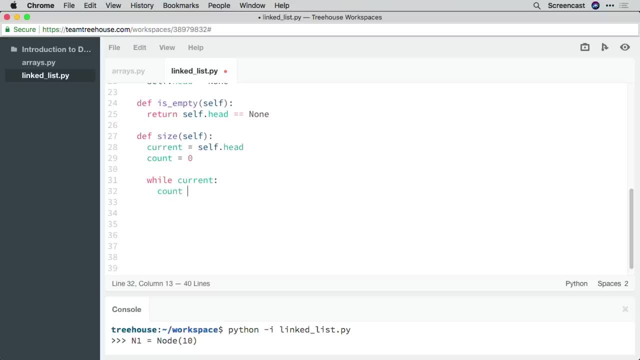 on the first pass, we're going to split the array into two smaller arrays. now in binary search, one of these sub arrays would be discarded, but that's not what happens here. on the second pass, we're going to split each of those sub arrays into further smaller. 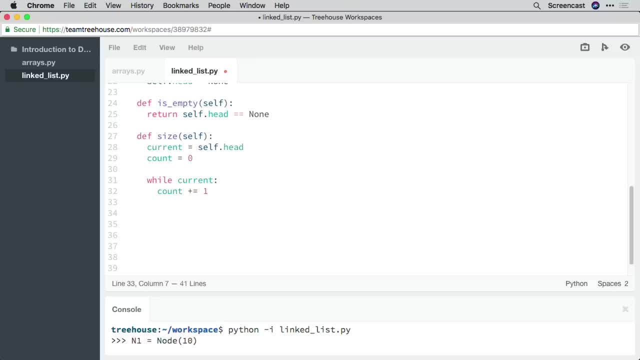 evenly sized arrays, and we're going to keep doing this until we're down to single element arrays. after that, the merge sort algorithm works backwards, repeatedly merging these single element arrays and sorting them at the same time. since we start at the bottom by merging two single element arrays, we 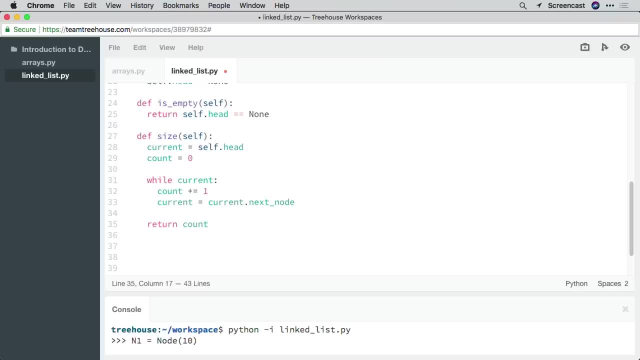 only need to make a single comparison. to sort the resulting merge array by starting with smaller arrays that are sorted as they grow, merge sort has to execute fewer sort operations than if it sorted the entire array at once. solving a problem like this by recursively breaking down the 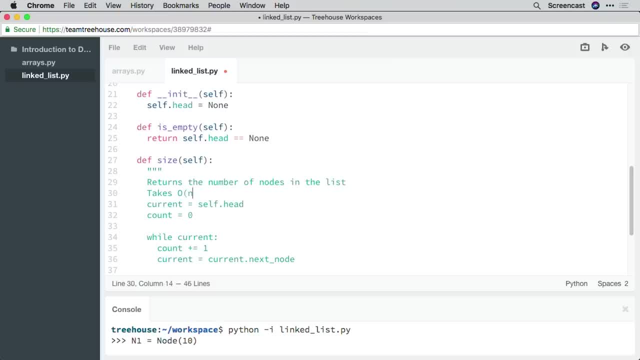 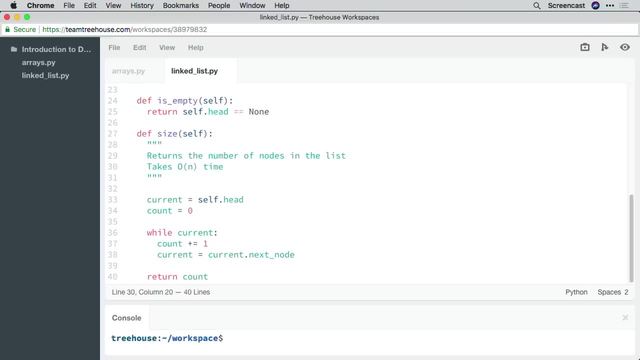 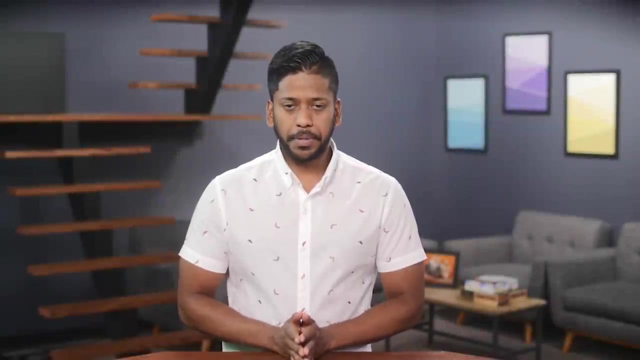 problem into sub parts until it is easily solved is an algorithmic strategy known as divide and conquer. but instead of talking about all of this in the abstract, let's dive into the code. this way we can analyze the run time as we implement it. for our first implementation of merge sort. 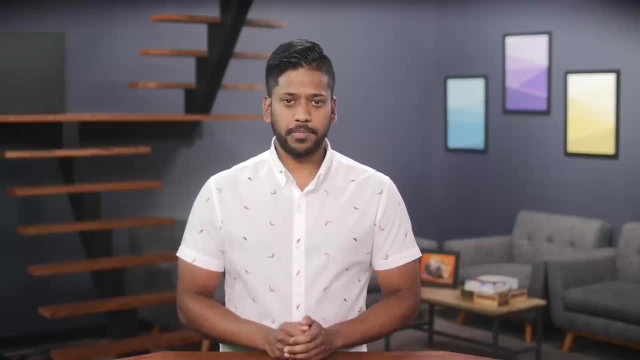 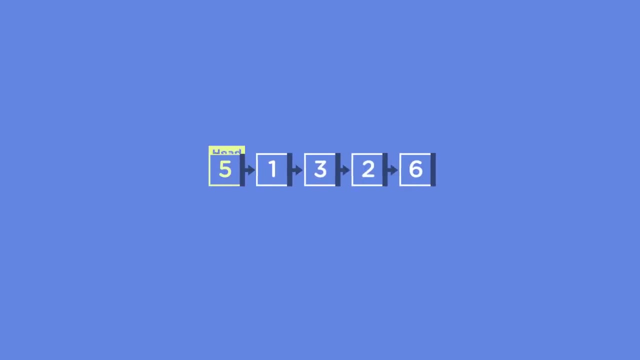 we're going to use an array or a python list. while the implementation won't be different conceptually for a linked list, we will have to write more code because of list traversal and how nodes are arranged. so once we have these concepts squared away, we'll come back to that. 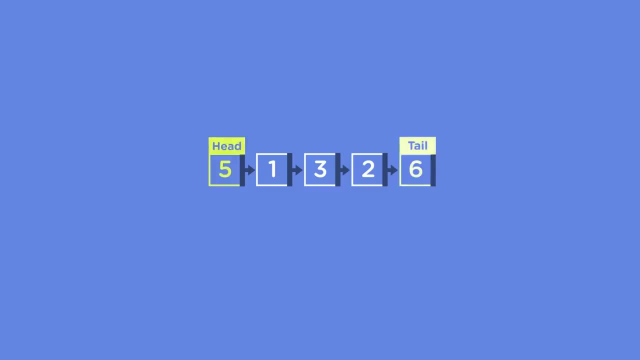 let's add a new file here. we'll call this merge- underscore sort- dot pi. in our file let's create a new function named merge sort that takes a list. and remember, when I say list, unless I specify linked list, I mean a python list, which is the equivalent of an array. 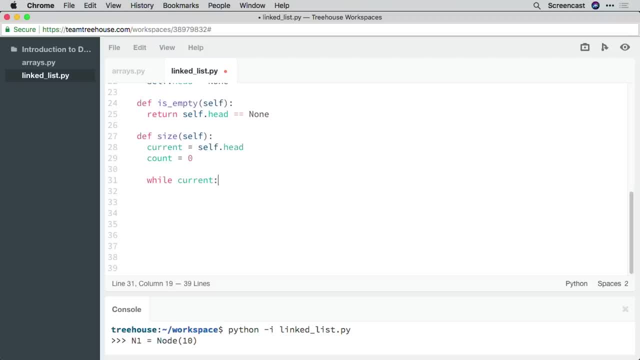 But it's more succinct, So we'll go with this former. If the latter is more precise for you, You can go with that. Now, inside this loop, We'll increment the count value. So count plus equal, one Plus equal, if you haven't encountered it before. 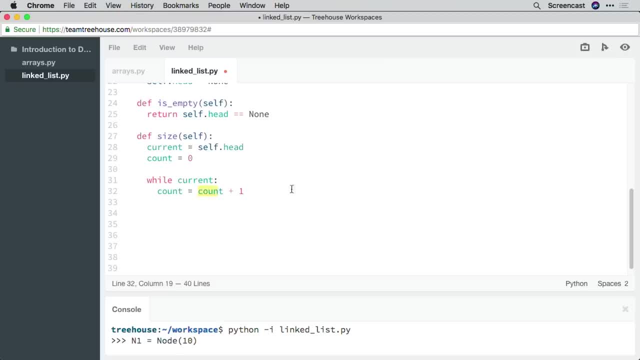 Is the same as writing. count equal, count plus one. So if count is zero initially, Then we'll assign that back to count. Okay, So count plus equal one. Next, we're going to assign the next node In the list to current. 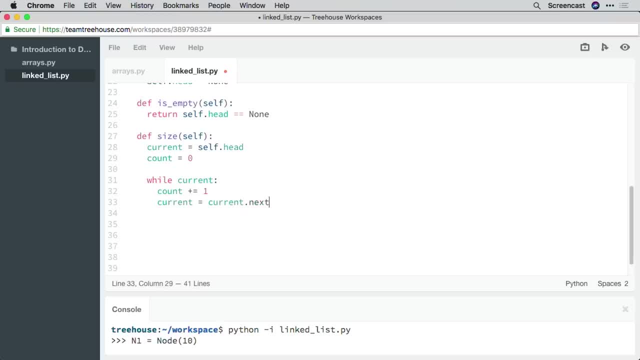 So current equal Current dot next node. This way, Once we get to the tail And call next node, Current will equal none And the while loop terminates To the end. we can return count. As you can see, We've created a new node. 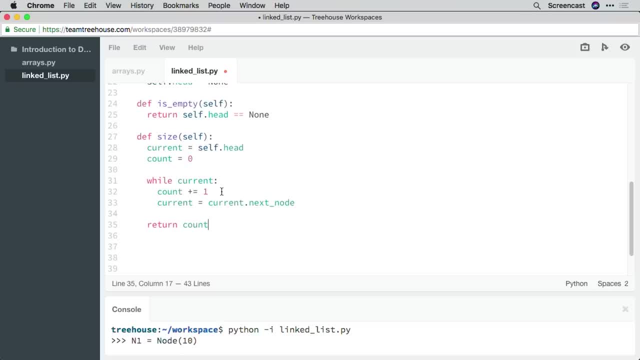 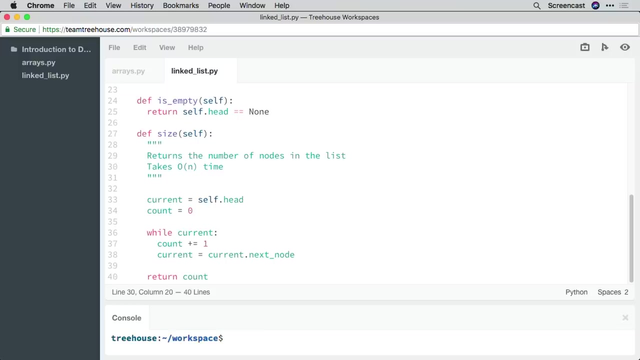 To determine the size Meaning. our algorithm runs in linear time, So let's document this Up in our doc string, Which we'll add now to size, We'll say: Returns the number of nodes In the list. Takes linear time. 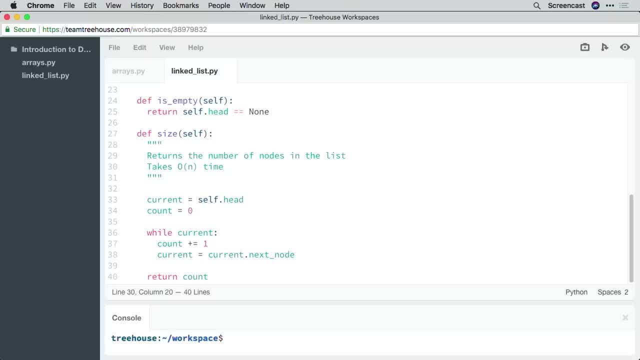 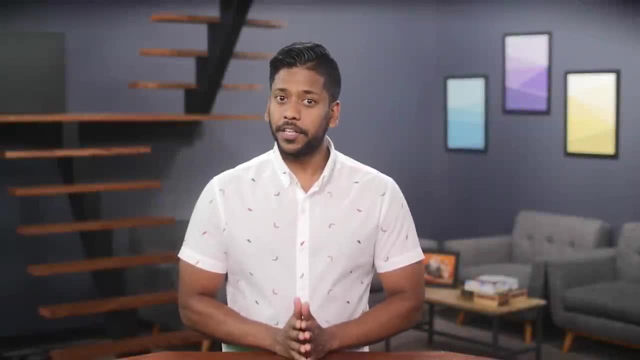 Let's take a break here. We can now create lists, Check if they're empty And check the size. At the moment, We can create an empty list, But nothing else. Let's define a method to add data to our list. 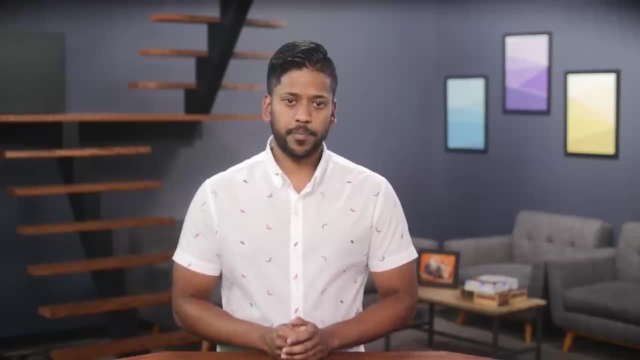 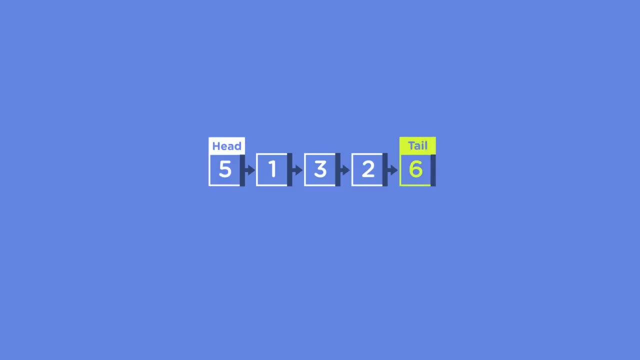 Technically speaking, There are three ways we can add data to a list. We can add nodes at the head of the list, Which means that the most recent node we created Will be the head And the first node we created will be the tail. 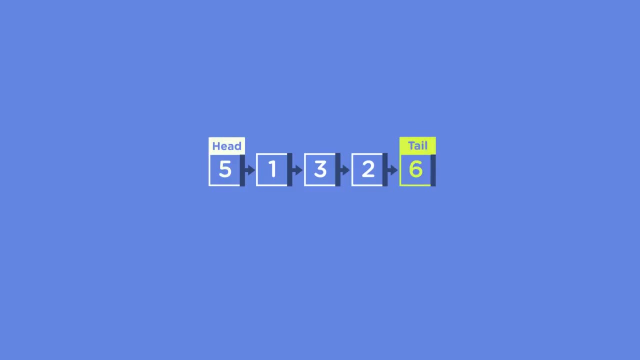 Or we could flip that around: Most recent nodes are the tail of the list And the first node to be added is the head. I mentioned that one of the advantages Of linked lists over arrays Is that adding data into the list Is much more efficient than to the array. 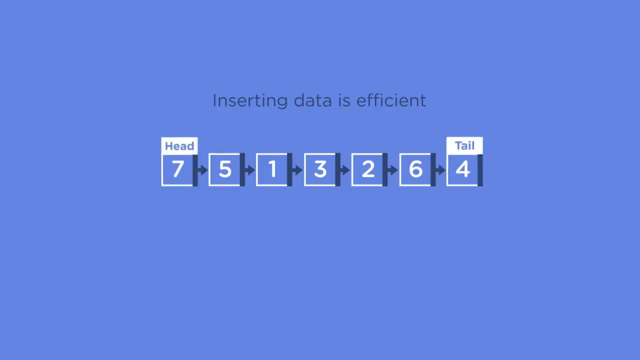 This is only true If we're inserting at the head or the tail. Technically speaking, This isn't an insert, And you'll often see this method called add, Prepend, if the data is added to the head, Or append, if it's added to the tail. 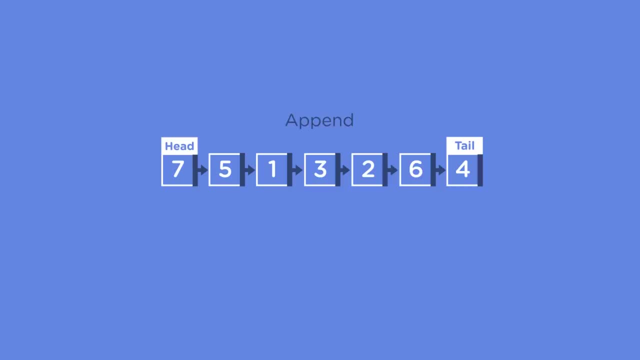 so we'll say def, merge, underscore, sort. that takes a list. in the introduction to algorithms course we started our study of each algorithm by defining the specific steps that comprise the algorithm. let's write that out as a doc string in here, the steps of the algorithm, so that we can refer to it. 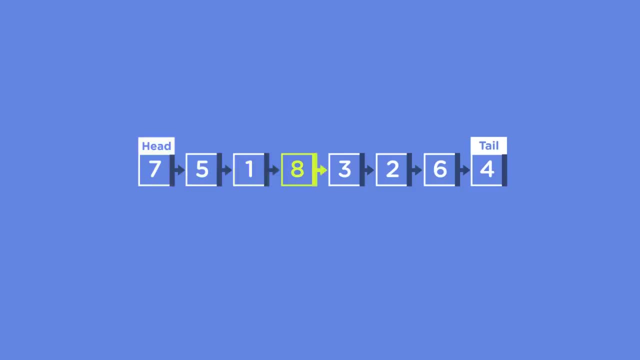 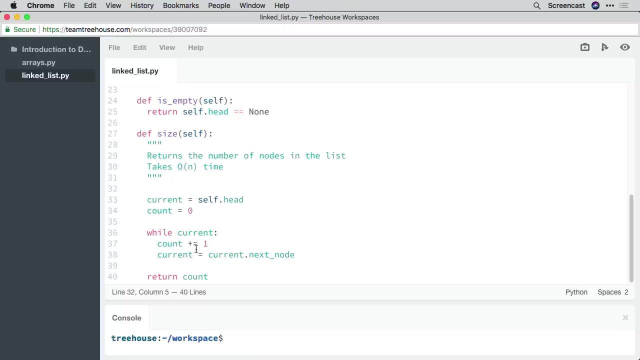 right in our code. this algorithm is going to sort the given list in an ascending order, so we'll start by putting that in here, as a simple definition sorts a list in ascending order. there are many variations of merge sort, and in the one we're going to implement, 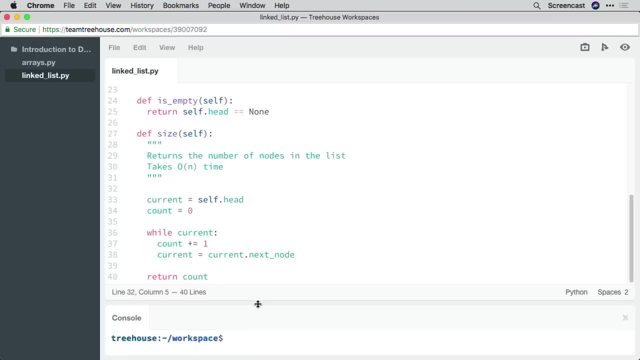 we'll create and return a new sorted list. other implementations will sort the list we pass in, and this is less typical in an operation known as sort in place, but I think that returning a new list makes it easier to understand the code. now these choices do have. 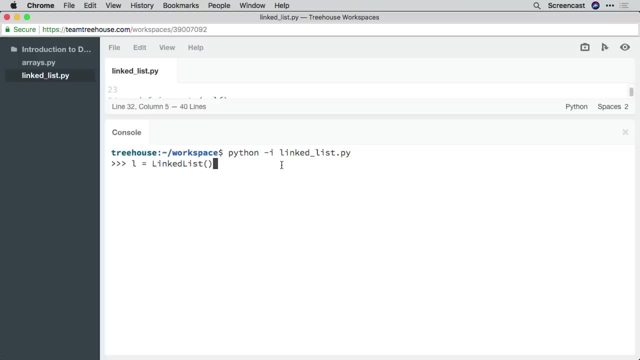 implications, though, and we'll talk about them as we write this code. for our next bit of the doc string, let's write down the output of this algorithm. so returns a new sorted list. merge sort has three main steps. the first is the divide step, where we find the midpoint. 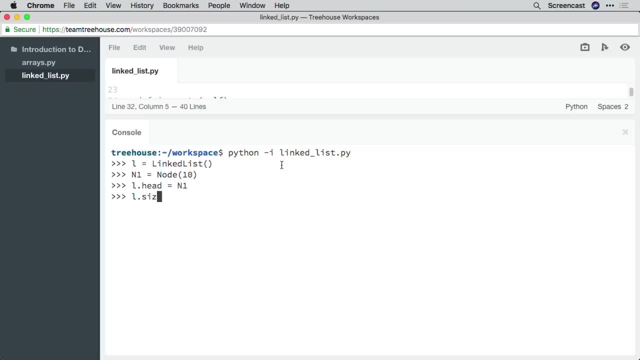 of the list. so we'll say divide, find the midpoint of the list and divide into sublists. the second step is the conquer step, where we sort the sublists that we created in the divide step. so we'll say recursively sort the sublists created in previous. 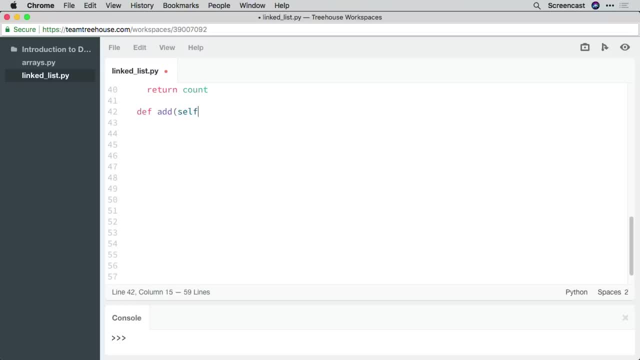 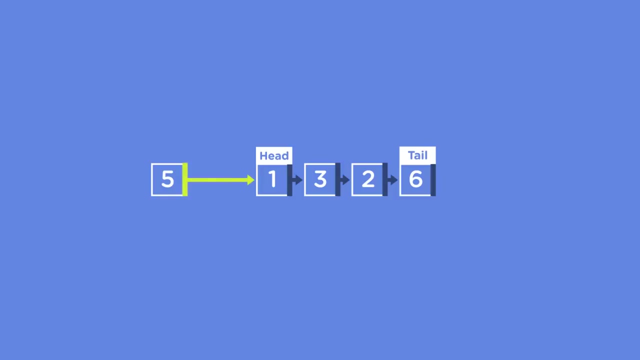 step. and finally, the combine- the combine- step, where we merge these recursively sorted sublists back into a single list. so merge the sorted sublists created in previous step. when we learned about algorithms, we learned that a recursive function has a basic pattern. first we start with a base case. 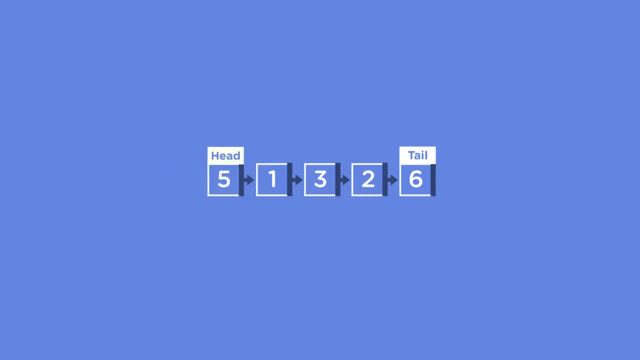 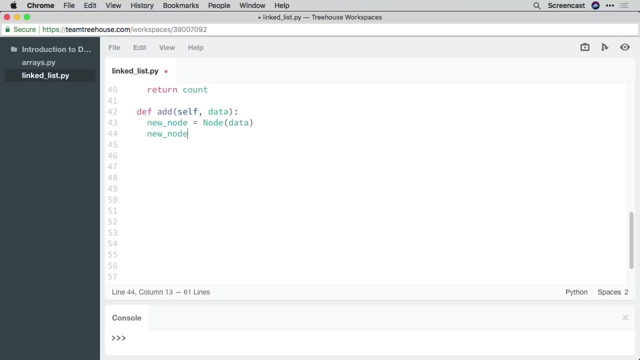 that includes a stopping condition. after that we have some logic that breaks down the problem and recursively calls itself: our stopping condition. is our end goal, a sorted array now to come up with a stopping condition or a base case. we need to come up with the simplest condition that satisfies. 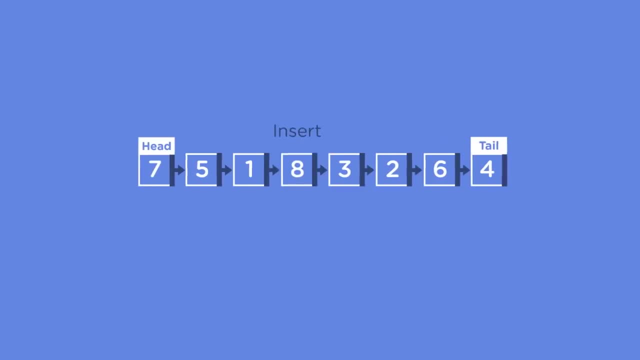 A true insert Is where you can insert the data At any point in the list, Which is our third way of adding data. We're going to circle back on that If we wanted to insert at the tail, Otherwise we would have to start at the head. 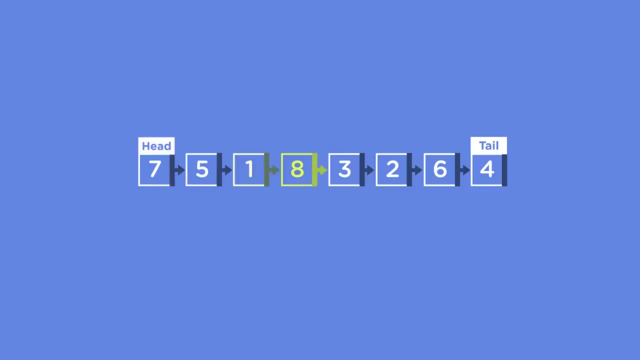 And walk down the length of the list Or traverse it To find the tail. Since our list only keeps a reference to the head, We're going to add new items at the head of the list Now, before we add our new method. 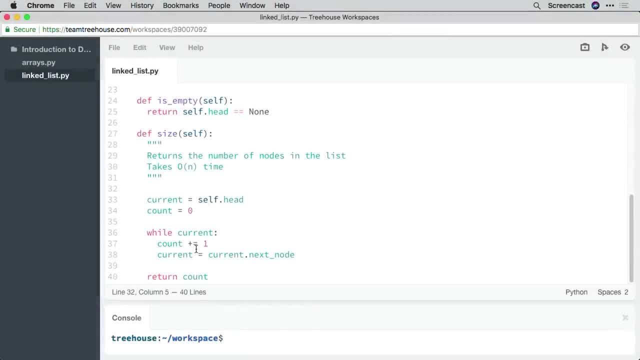 I forgot that. I didn't show you in the last video How to actually use the code we just added And how to check every time You know, when we add new code, That it works correctly. So, like before, We're going to bring up the console. 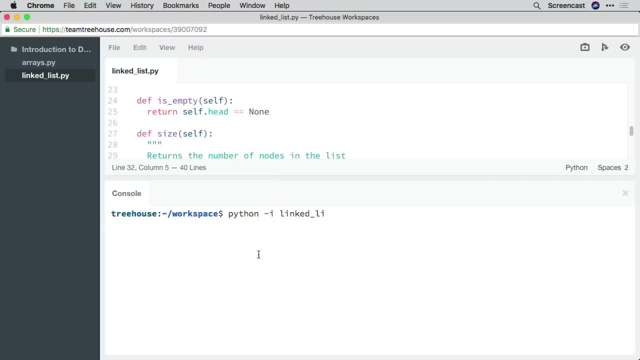 And we're going to add a new function. We're going to call it Python-i linked underscore list dot pi, Which should load. it, Load the contents of our file. And now we'll start here by creating a linked list, So l equal linked list. 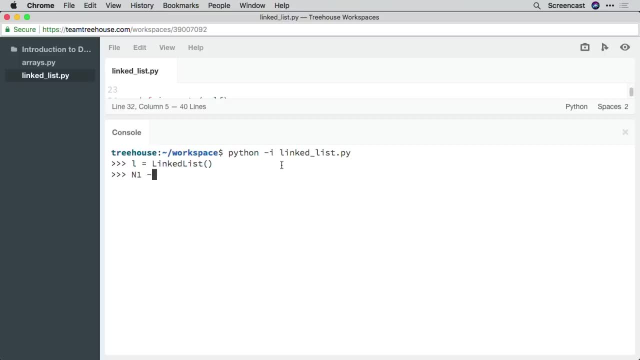 And then we'll use a node, So n1 equal node, With the value 10.. And now we can assign n1. To the nodes Or to the linked list's head attribute, So l1 dot head, equal n1.. And then 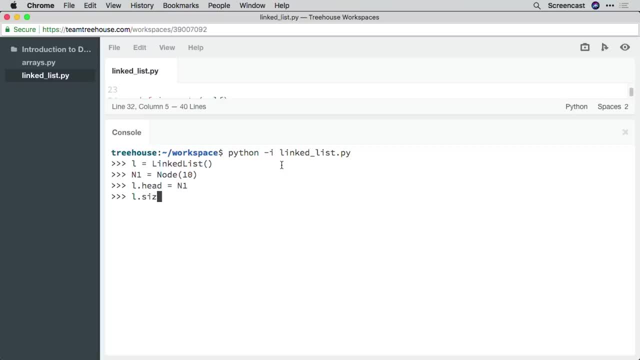 We can see if size works correctly. So if we call l1 dot size- And since this is a method, We need a set of parentheses at the end- And enter, You'll see that we get back one correctly. Okay, so it works. 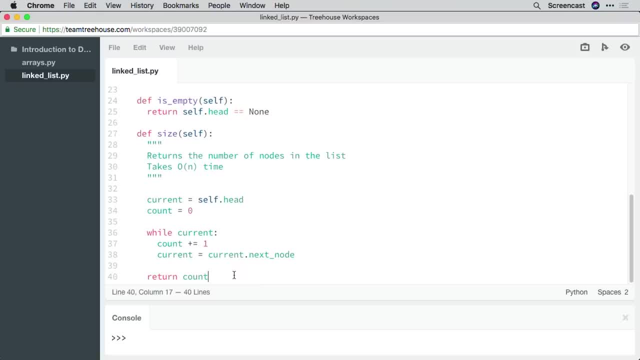 Now let's add our new method, Which we're going to call add. Add is going to accept some data To add to the list Inside of a node. So we'll say def, Add, And every Python method Has an argument. 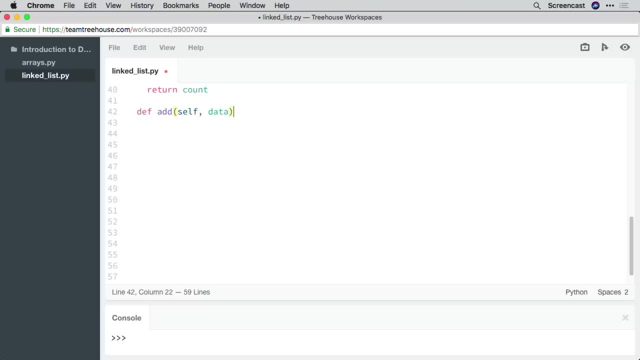 And then we want to add some data to this node. So we're going to say data for the second argument Inside the method. First we'll create a new node To hold onto the data, So new underscore node, equal Node with the data. 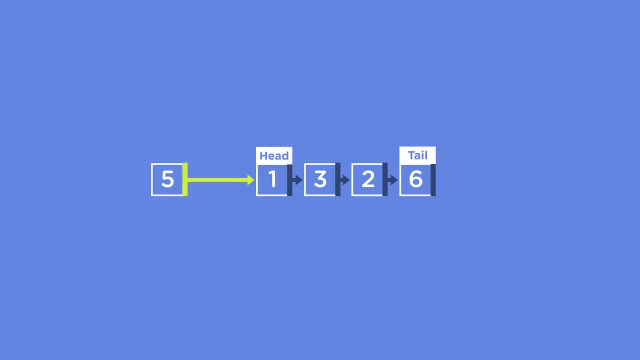 Before we set the new node As the head of the list, We need to point the new node's next property At whatever node is currently at head. This way, when we set the new node As the head of the list, We don't lose a reference to the old head. 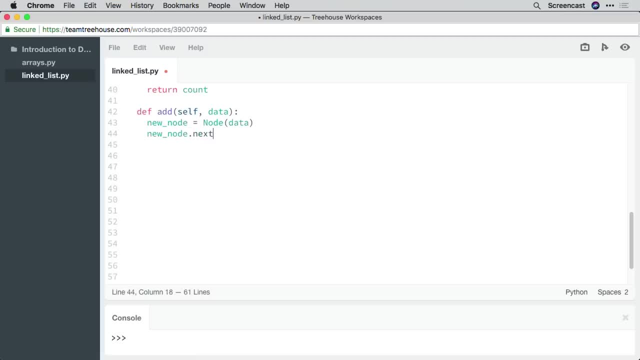 So new underscore: node Dot. next node Equal- self dot head. Now, if there was No node at head, This correctly sets Next node to none. Now we can set the new node As the head of the node. So say self dot head equal. 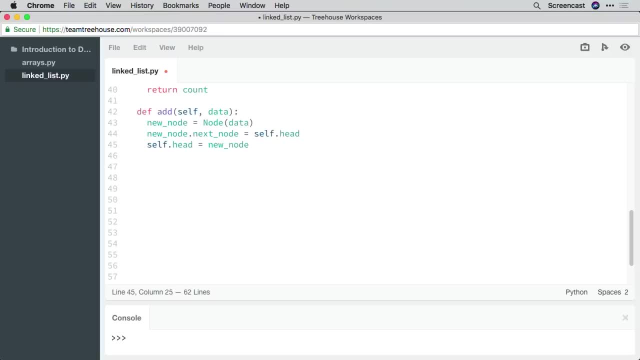 New underscore node, Because the insert operation Is simply a reassignment Of the head and next node Properties. This is a constant time operation, So let's add that in as a doc string First, what the method does. So it adds a new node. 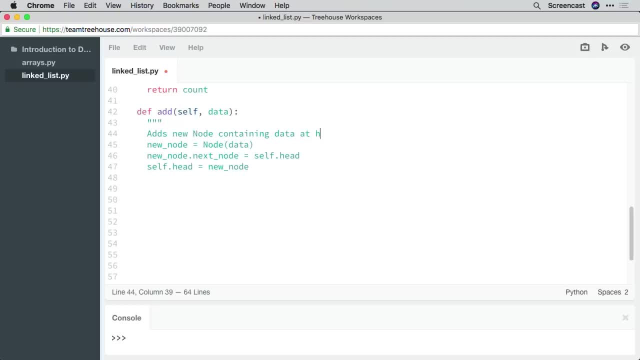 Containing data At the head of the list. This operation takes Constant time, Which is our best case scenario. Okay, Let's test this out. So I'm going to bring the console back up Out of Our current repl. 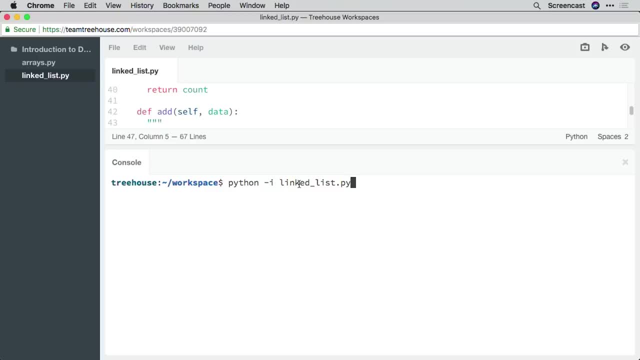 And we'll load The contents of the file again. And now we don't need to create a node Like we did earlier, So we can say: l equal linked list, L dot, add one. Okay, Let's see if this works. 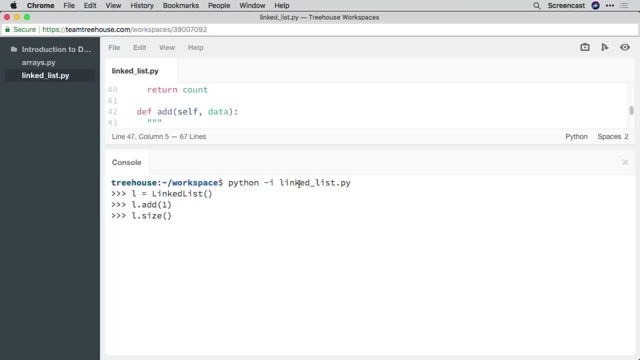 We'll call size And, if it worked, The linked list should now have a size of one. There we go. L dot add three, And l dot size Should now be three. There we go Now. if I were to type l and just hit print. 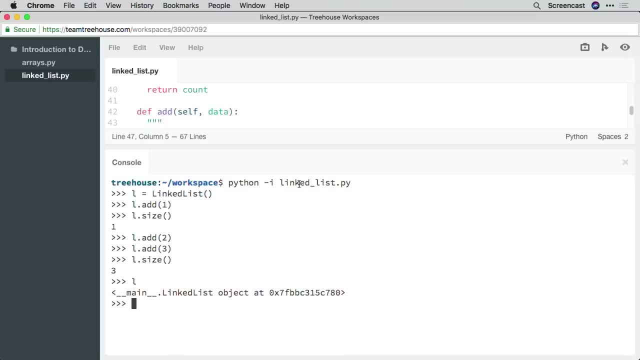 Again, what we get in the repl Is nothing useful. So, like before, we'll implement The repper function For our linked list. Now I'm just going to copy paste this in And we'll walk through it. Okay, so this is what our 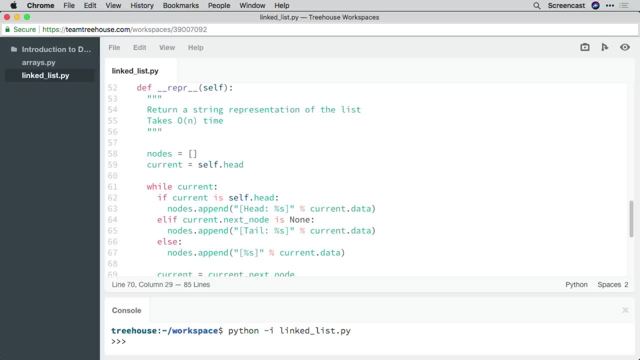 Implementation of repper looks like For the linked list object. You can grab this code from the Notes section of this video. Okay, so at the top you'll see a doc string Where it says it returns a string representation Of the list. 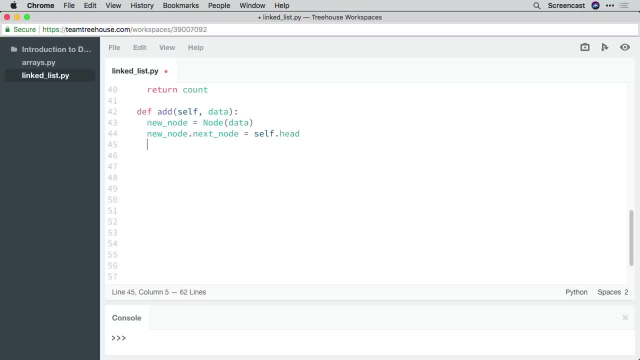 this end result. so there are two possible values that fit: a single element list or an empty list. now, in both of these situations we don't have any work to do. if we give the merge sort function an empty list or a list with one element, it's technically already sorted. 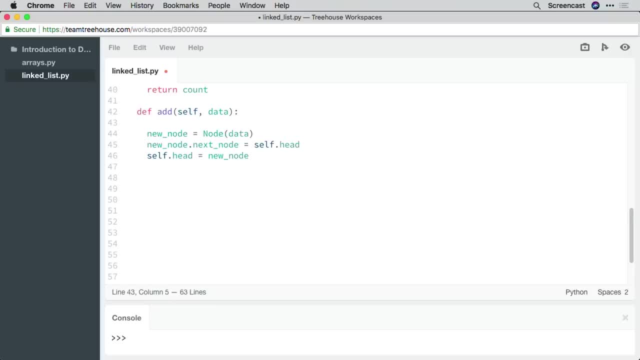 we call this naively sorting. so let's add that as our stopping condition we'll say: if len list, if the length of the list is less than or equal to one, then we can return the list. okay, so this is our stopping condition, and now that we have a stopping, 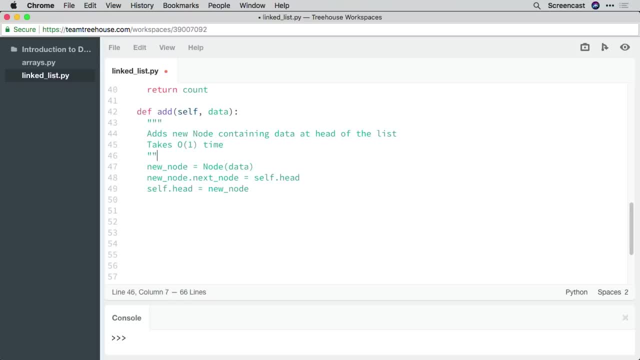 condition we can proceed with the list of steps. first we need to divide the list into sublists to make our functions easier to understand. we're going to put our logic in a couple different functions instead of one large one, so I'll say it: left half, comma right half. 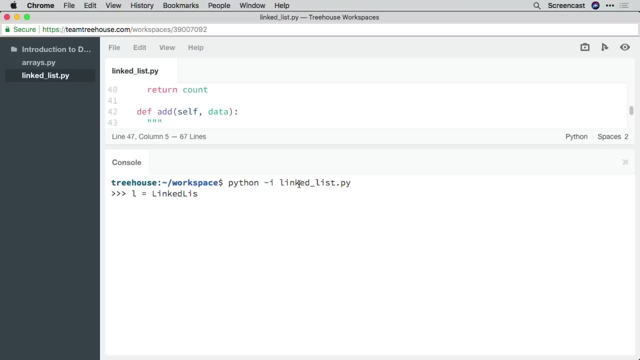 equal split list. so here we're calling a split function that splits the list we pass in and returns two lists, split at the midpoint. because we're returning two lists, we can capture them in two variables. now you should know that this split function is not something that comes built. 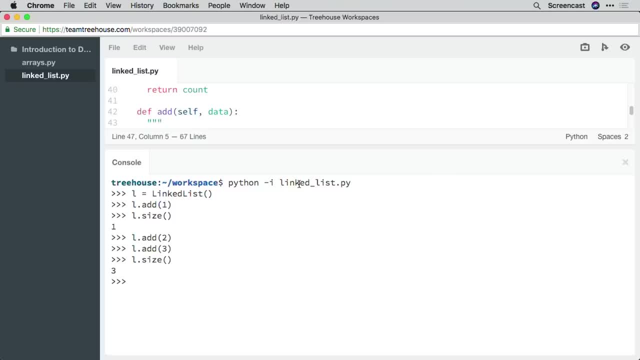 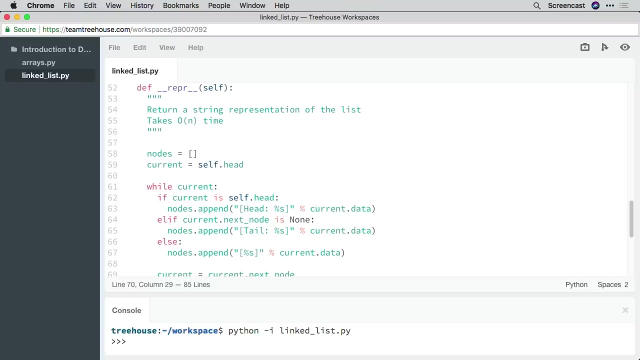 into python. this is a global function that we're about to write. next is the conquer step, where we sort each sublist and return a new sorted sublist. so we'll say: left equal merge- sort left half and right equal merge- sort right half. this is the recursive portion of our function. 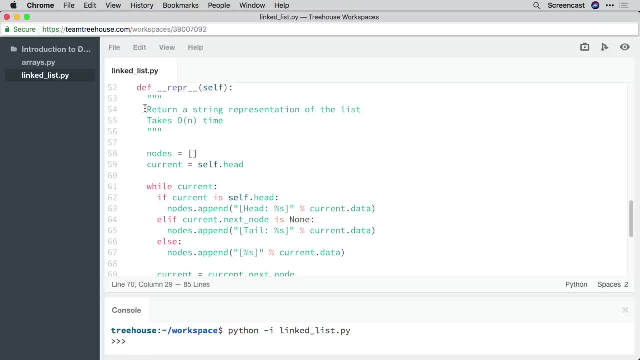 so here we're calling merge sort on this divided sublist. so we divide the list into two here and then we call merge sort on it again. this further splits that sublist into two. in the next pass through of merge sort this is going to be called again and again, and again until we 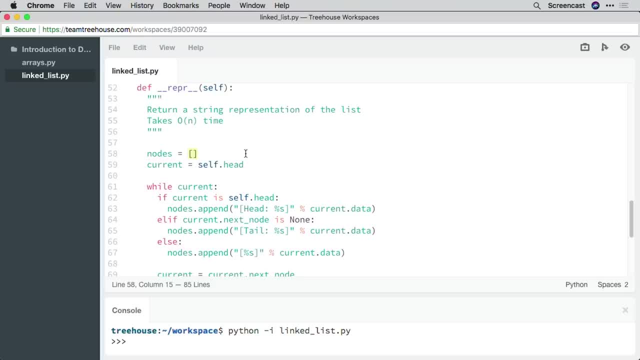 reach our stopping condition where we have single element lists or empty lists. when we've subdivided until we cannot divide anymore, then we'll end up with a left and a right half and we can start merging backwards. so we'll say: return, merge, left and right. that brings 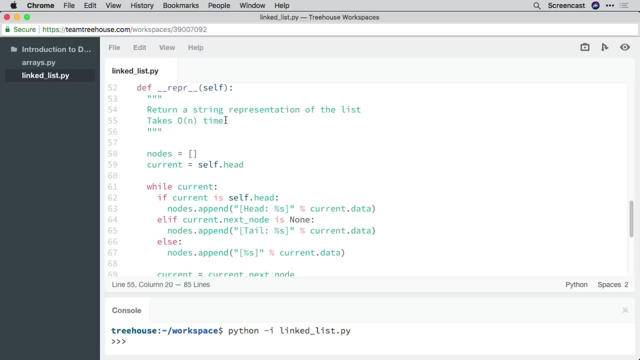 And, like everything we need to do with a linked list, We need to traverse it, So this is going to take linear time. We start by creating an empty list. Now I need to distinguish: this is a python list, Not a linked list. 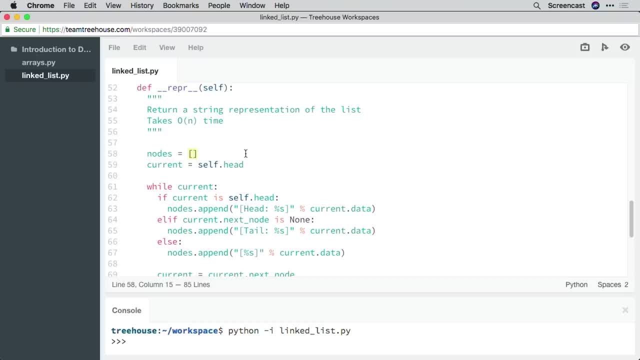 So we create an empty list called nodes, And to nodes we're going to add strings That have a description, That provide a description To the node, But we're not going to use the description That we implemented in the node class. 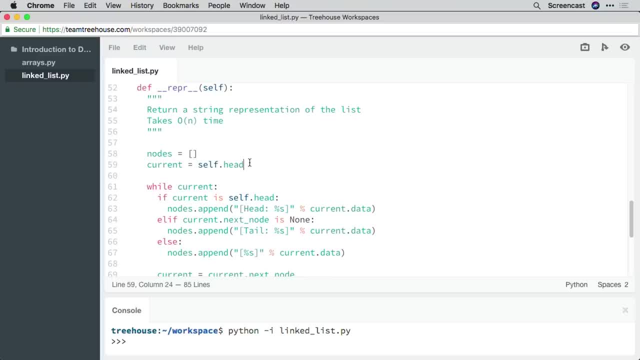 Because we're going to customize it a bit here. Next, we start by assigning selfhead to current, So we sort of have a pointer To the head node As long as current does not equal none, Which means we're not at the tail. 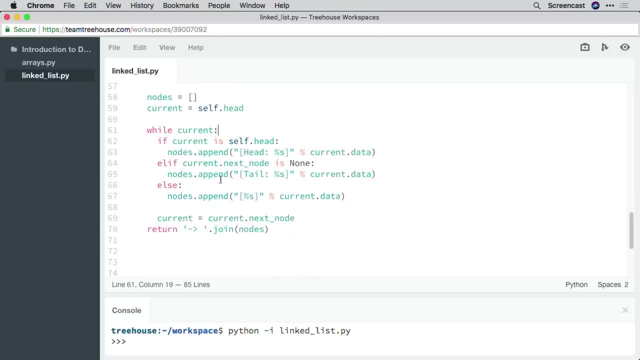 We're going to implement some logic. So in the first scenario, If the node assigned to current Is the same as the head, Then we're going to append this string To our nodes list And this string is simply Going to say that, hey, this is a head node. 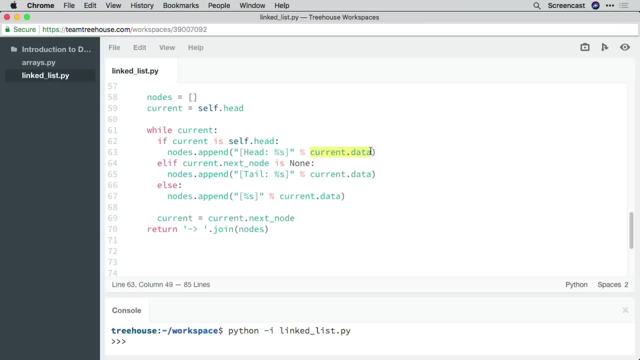 And it contains some data Which we'll extract using currentdata. Next scenario Is: if the node assigned to Current's next node Is none Meaning we're at the tail node, Then we'll assign a different kind of string. So it's the same as earlier. 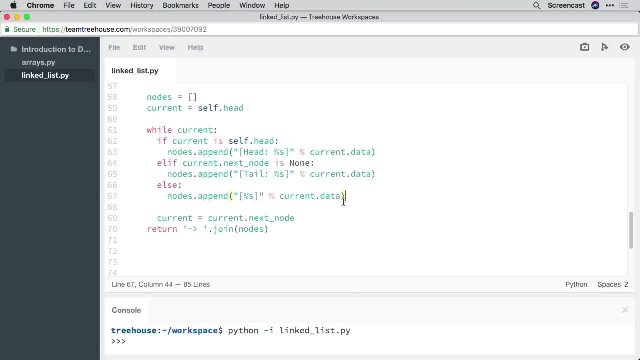 Except we're saying tail here, And then finally in any other scenario, Which means we're not at the head Inside, And again we'll extract it using currentdata. With every iteration of the loop We'll move current forward By calling currentnextnode and reassigning it. 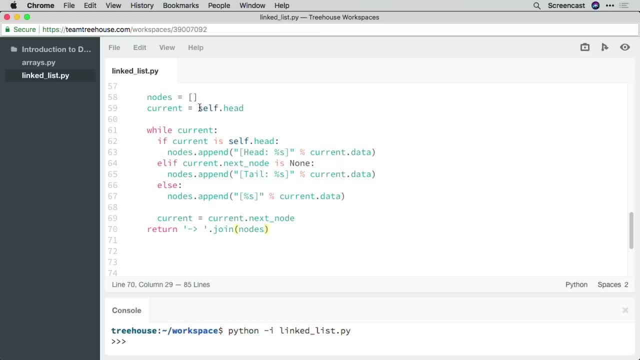 And then at the very end, when we're done, We'll join all the strings That are inside the nodes list together Using the python join method, And we'll say that With every join. So when you join these two strings together, 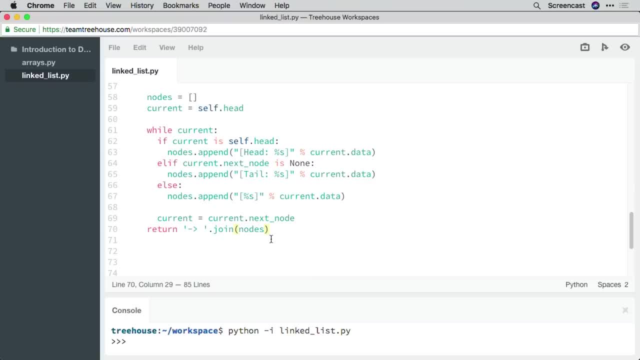 To make one string, You need to put this set of characters in between. Alright, So when I come down here, Exit out of the console again, Clear it out, Load the contents of the file again And let's try that. So we'll say l equal linked list. 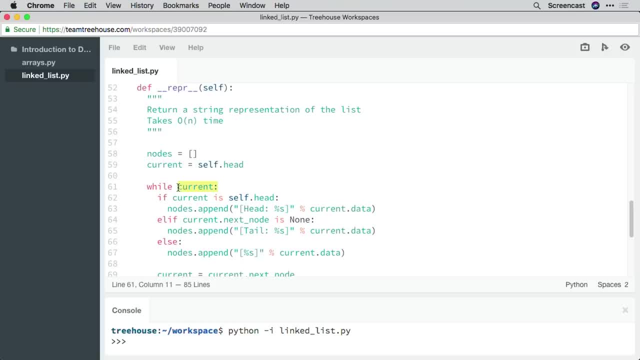 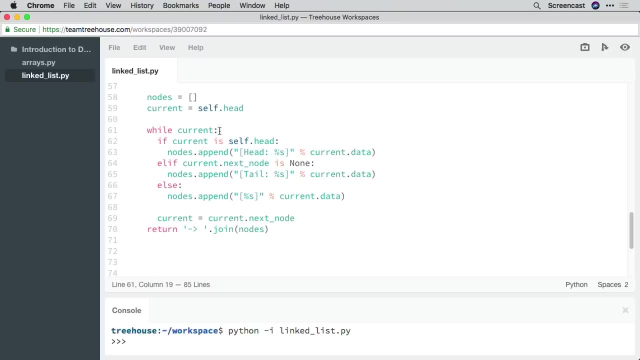 us to the combine step. once two sublists are sorted and combined, we can return it. now, obviously, none of these functions- merge, merge, sort. well, merge, sort is written, but merge and split haven't been written. so all we're going to do here, if we run it, is raise and 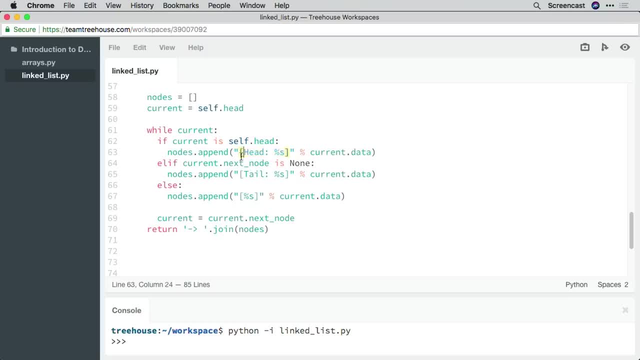 error. so in the next video let's implement the split operation. the first bit of logic we're going to write is the divide step of the algorithm. this step is fairly straightforward and only requires a few lines of code, but is essential to get the sorting process going. 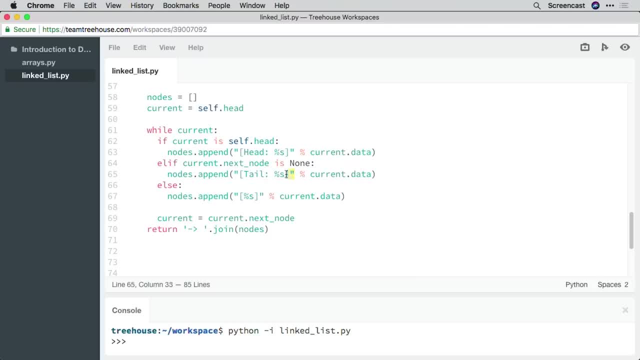 alright. so, as we saw earlier, we're going to call the function for the divide step split. so we'll say def split and split is going to take as an argument a list to split up. let's document how this function works. so we'll say: divide, the. 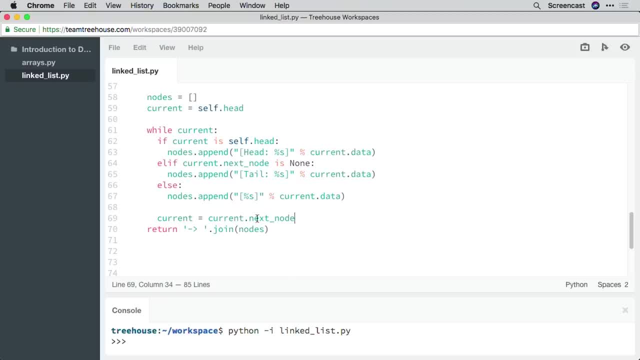 unsorted list at midpoint into sublists, and it's always good to say what we're returning as well, so we'll say returns to sublists, left and right. alright. so the first step is to determine the midpoint of this list, of this array we're going. 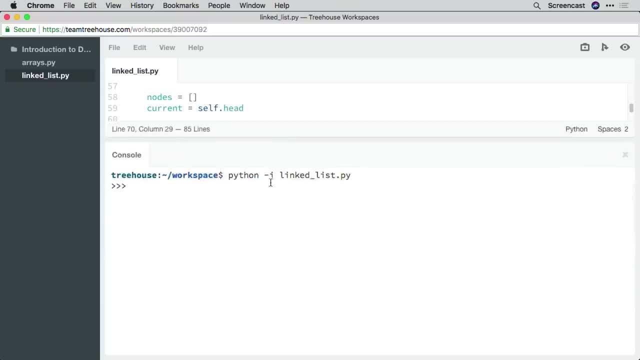 to use the floor division operator, for this floor division carries out a division operation and if we get a non integer value like 2.5 back, it just gets rounded down to 2. we'll define the midpoint to be the length of the list divided by 2 and then rounded down. 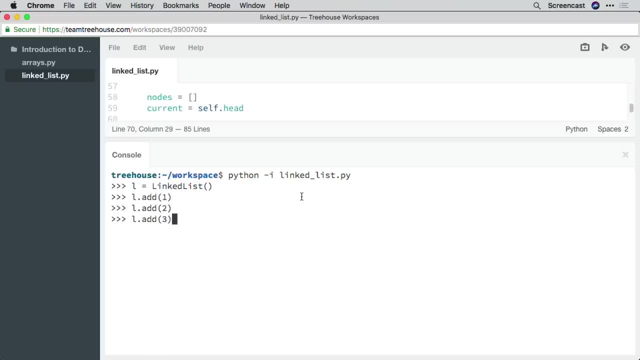 so len list and using the two forward slashes for the floor division operator, we'll put number 2 after it. ok, once we have the midpoint, we can use the slicing notation in python to extract portions of the list we want to return. for instance, we can define left. 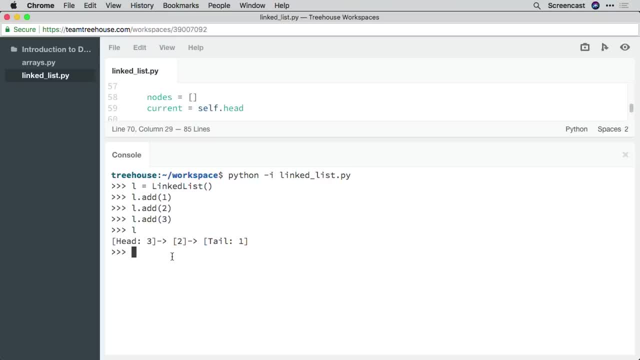 as the left sublist. that goes all the way from the start of the list all the way up to the midpoint, without including the midpoint. now, over here we're using the slicing syntax, where it's like using the you know subscript notation to access a value from a list, but instead 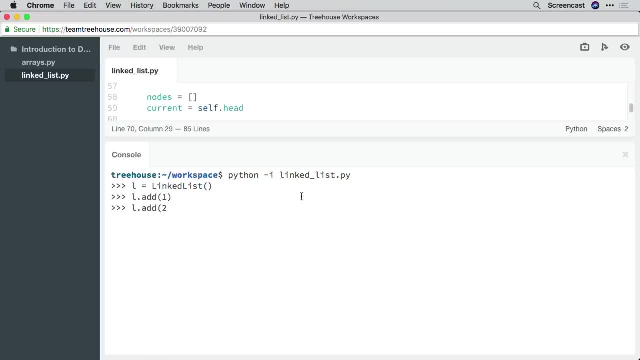 Alright. So l dot add one, L dot add two, L dot add three. That seems enough. And then now, if I type out l and hit enter, We get a nice string representation of the list, So you can see that we add every new node to the head. 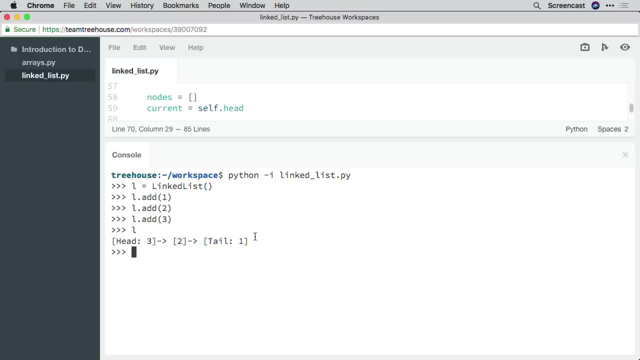 So we added one first, That being the tail Because it keeps getting pushed out- Then two And then finally three. So three is at the head. So far, we've only implemented a single method, Which functions much like the append method. 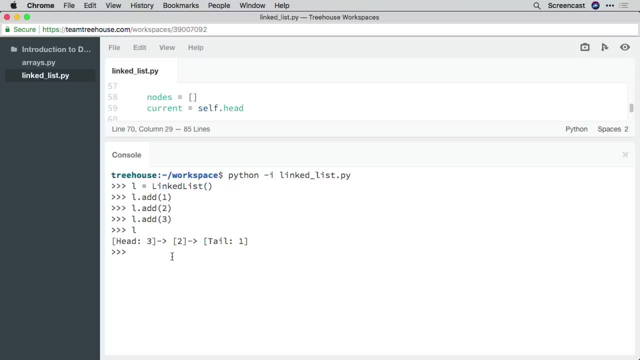 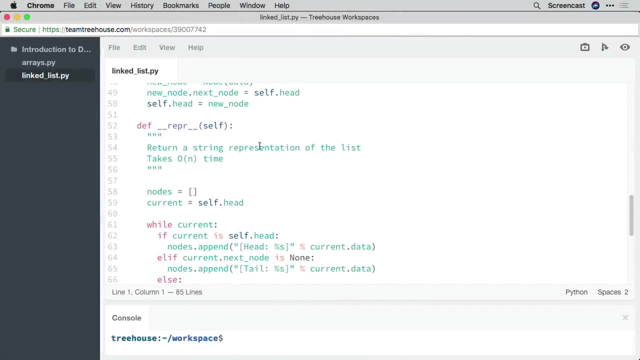 On a python list Or an array, Except it adds it to the start of the linked list, It prepends it Like append. This happens in constant time In the next video For the search operation We're going to define a method. 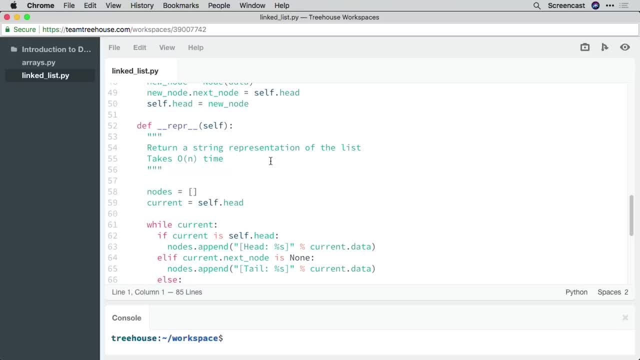 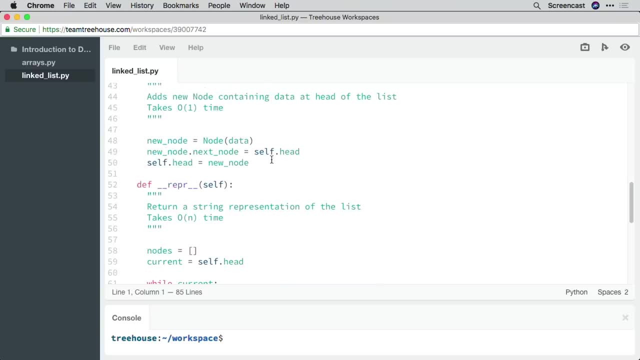 That takes a value to search for And returns either the node containing the value, If the value is found, Or none if it isn't. So right after, Actually, you know what We'll make sure? repr is the last function Or last method in our class. 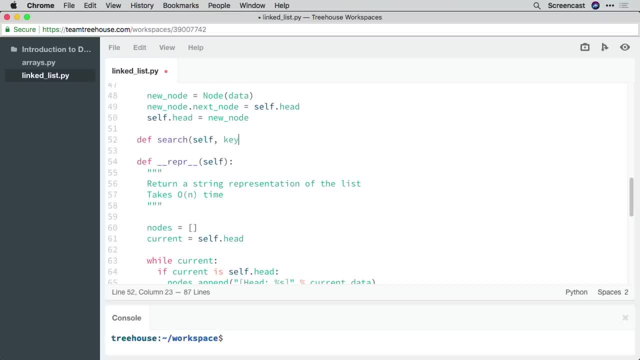 So we'll add it above it. So here we'll say def, search, self And then key. In the last video We'll use this method To provide a string representation of the list. So we're going to use similar logic here. 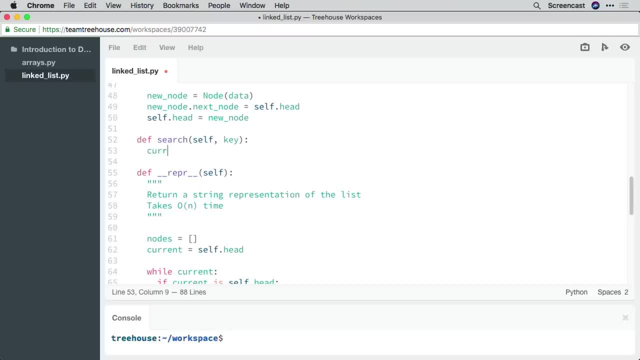 To implement the search function, We'll start by setting a local variable, Current, To point to the head of the list, While the value assigned to current Is a valid node, That is. if it isn't none, We'll check if the data on that node 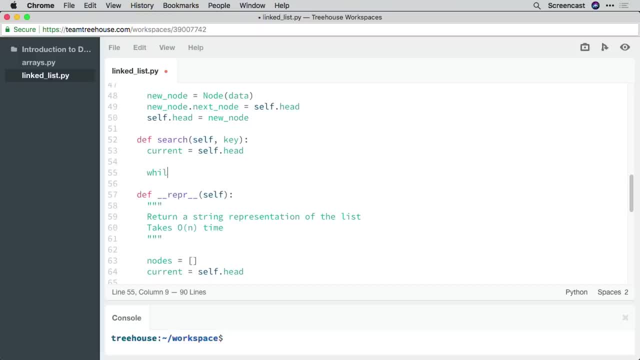 Matches the key that we're searching for. So, while current, We'll say If current dot data Is the key, Then we'll return current. If it does match, We'll go ahead and return it, Like we've done here. 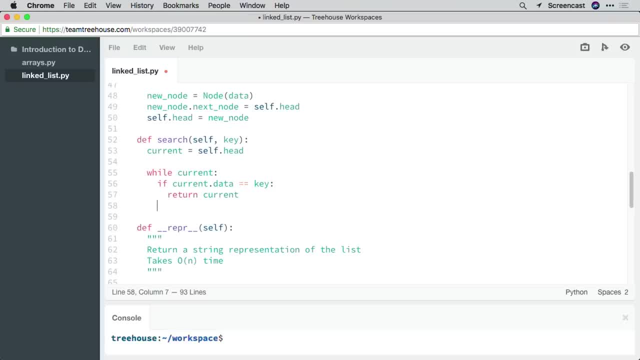 But if it doesn't, We'll assign the next node in the list To current and check again. So we'll say else: Current equal current dot. next node. Once we hit the tail node And haven't found the key, Current gets set to none. 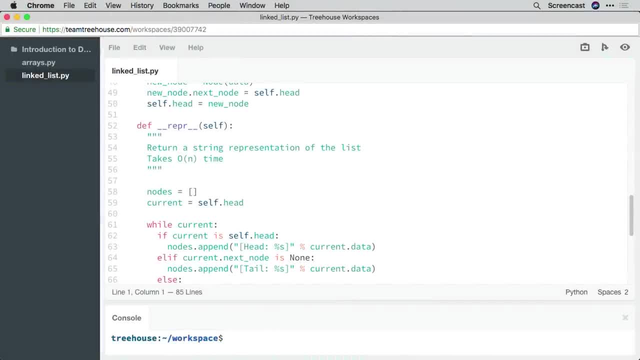 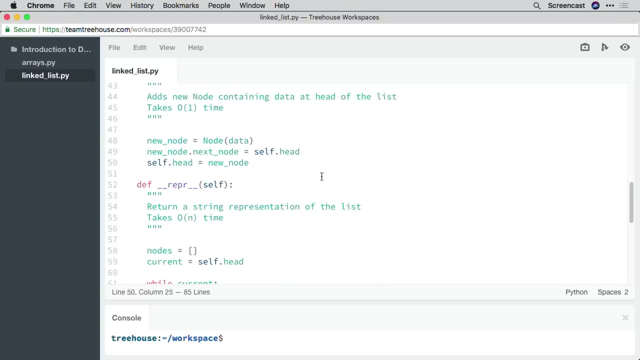 we give two index values as a start and stop. so if we don't include a start value, as I've done here, python interprets that as starting from the 0th index or the start of the list now. similarly, we can define right to be values on the. 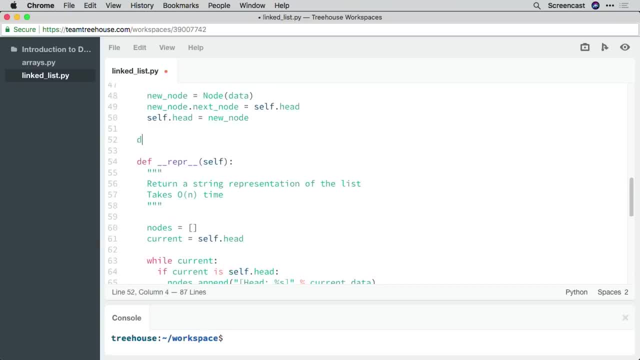 right of the midpoint. so starting at the midpoint and going all the way up to the end of the list. so couple things to note. as I said earlier, when you don't include the starting index, it interprets it as to start at the very beginning of the list, the index you give. 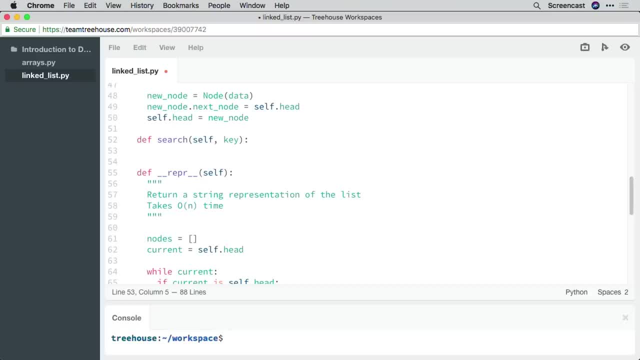 as the stopping condition. that value is not included in the slice. so over here we're starting at the very beginning of list and we go all the way up to midpoint, but not including midpoint, and then right starts at midpoint. so it includes that value and then goes all. 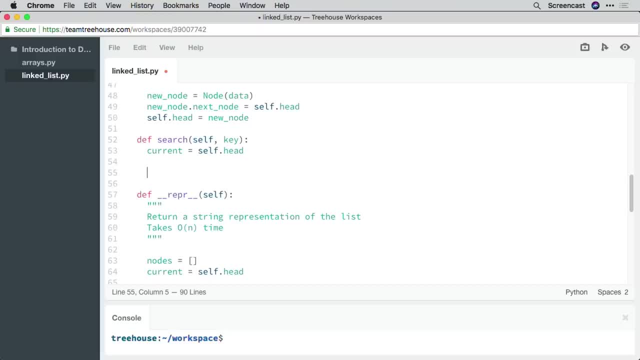 the way to the end of the list. now, once we have these two sublists, we can return them. so we return left and right. notice that we're returning two values here and then in the merge sort function, when we call that split function, we're declaring two. 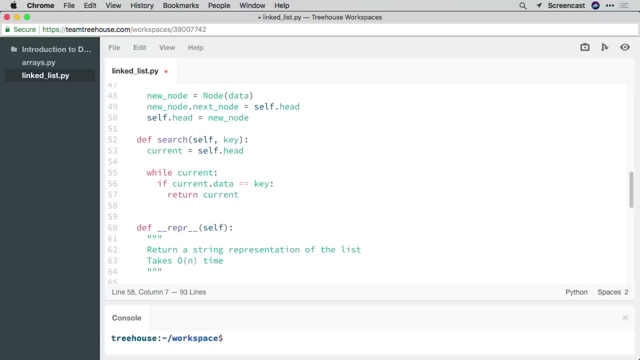 variables left half and right half- to assign, so that we can assign these two sublists to them. okay, and that's all there is to the split function. in the next video let's implement the crucial portion of the merge sort logic once we run the split function. 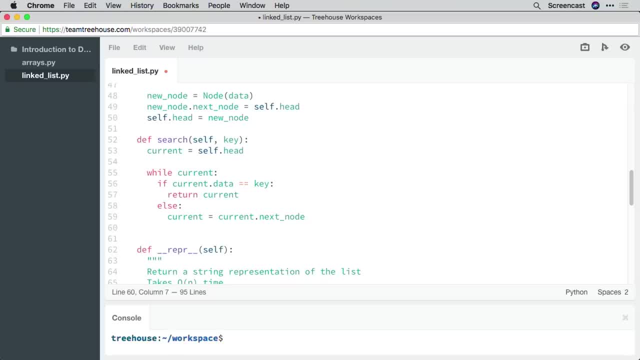 recursively over the array, we should end up with several single member or empty arrays. at this point we need to merge them all back and sort them in the process, which is what our merge function is for. the merge function is going to take two arrays or lists as arguments and to match the 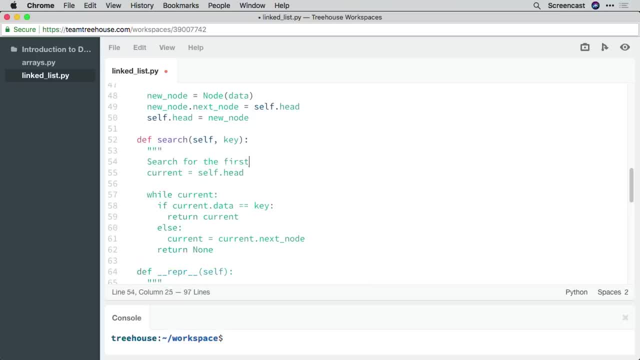 naming conventions we used in the split function. we'll call this left and right as well. so we'll say: def merge takes a left and a right list. now, like before, let's add some documentation to our function. so this function merges two lists or arrays, sorting them in the 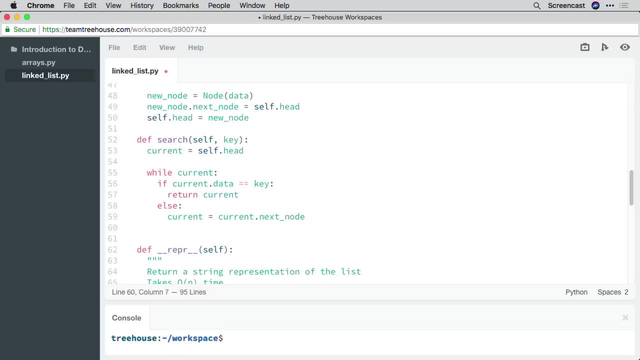 And the while loop exits And we know the list doesn't contain the key, So we can return None. That completes the body of our method. Let's add a doc string to document this. So up at the top We'll say search. 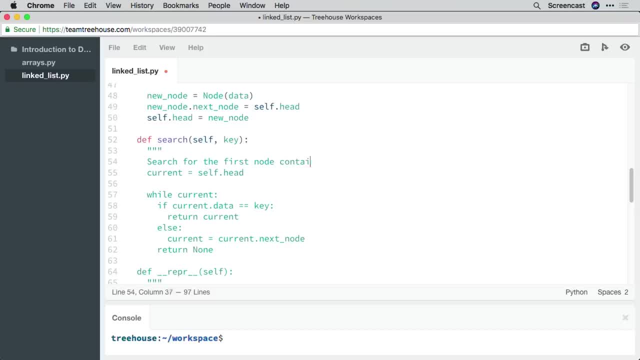 For the first node Containing data That matches The key. Now, this is important Because if our linked list Contains more than one node With the same value, We're going to return the first one. With this implementation, We'll also say here: 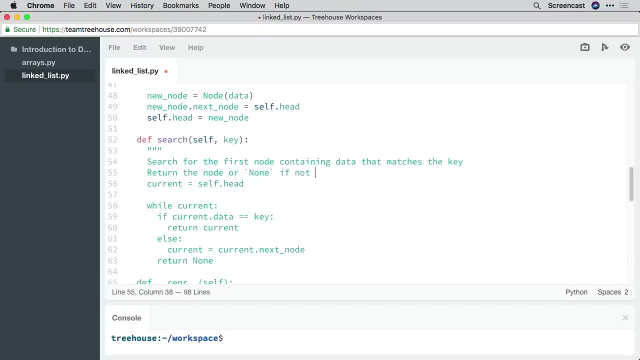 That it returns the node Or none, If not found. In the worst case scenario, We'll need to check every single node in the list Before we find the key or fail, And as a result, This operation runs in linear time. 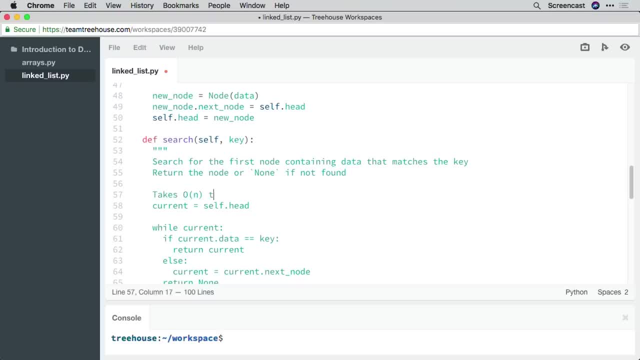 So we'll say takes O of n Or linear time. So far It indicates this data structure Has any advantage over an array Or a Python list. But we knew that I mentioned the strength of linked lists. Comes in inserts and deletes. 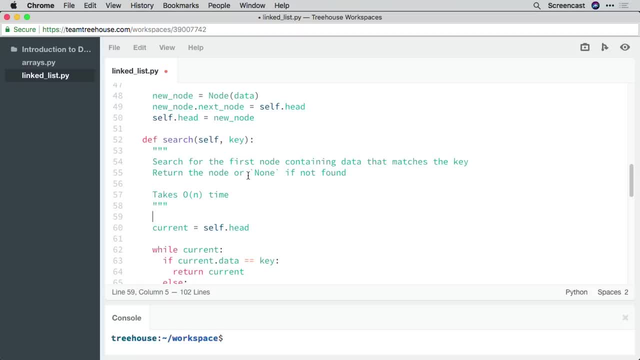 At specific positions. We'll check that out in the next video, But as always, before we end this one, Let's make sure everything works. So we'll load the contents Of the file again- L equal linked list- And then we'll say: 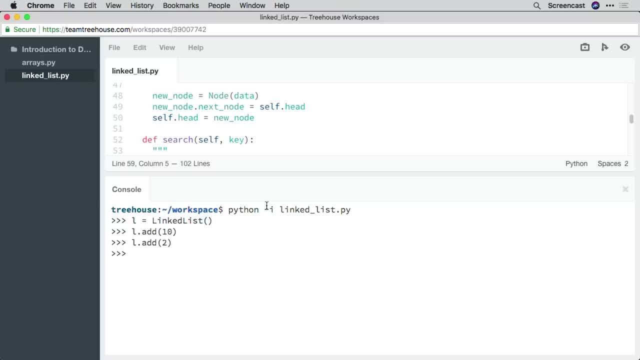 L dot add 10.. L dot add 20.. 2 doesn't matter. L dot add 45. And one more L dot add 15.. Now we can say l dot search And we need to give it a value. 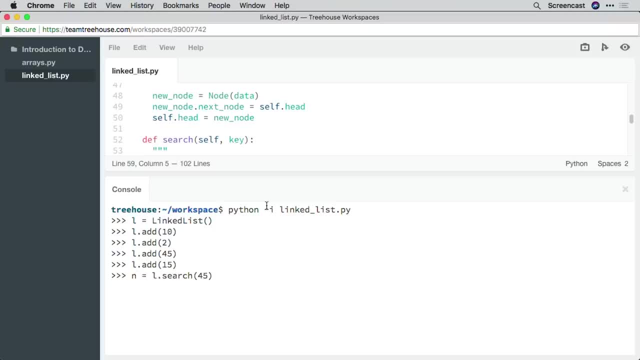 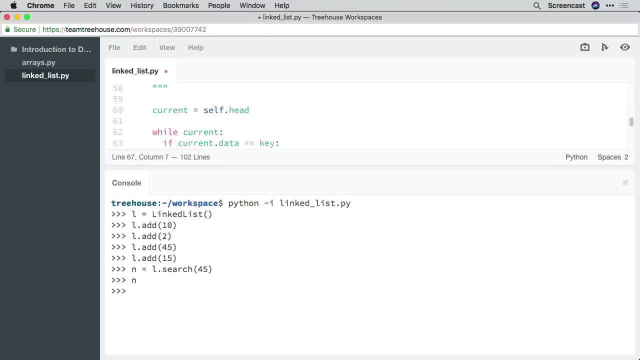 So we'll say 45. And this returns a node or none. So we'll say n- equal, And then we'll hit enter If this works Okay. weirdly n Does not work here. At least it says it's not a node. 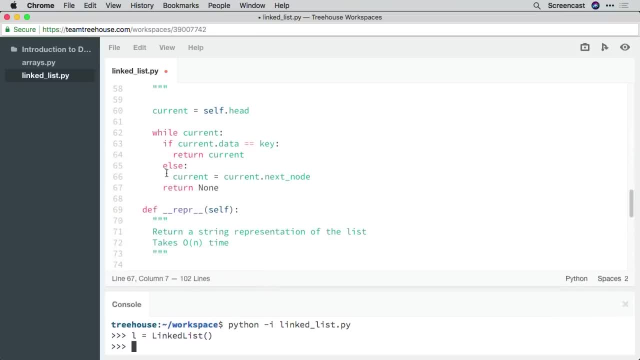 Which means I made a mistake in typing out our code And looking at it immediately, It's fairly obvious. So this return none needs to be outside Of the while loop. Okay, so I'm going to hit save now, So make sure it's on the same indentation here. 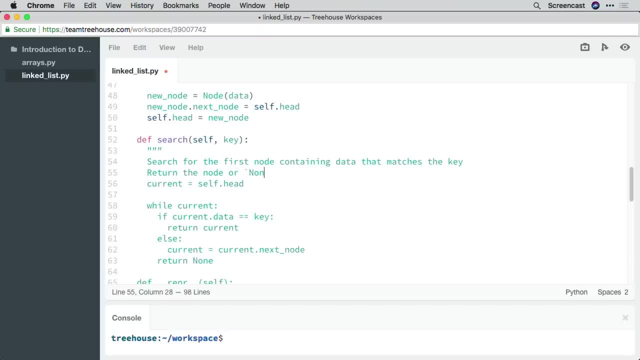 process and then it returns a new merged list. since our function is going to return a new list, let's start by creating one. now. in the process of merging, we need to sort the values in both lists. to sort, we need to compare values from each array or each list. 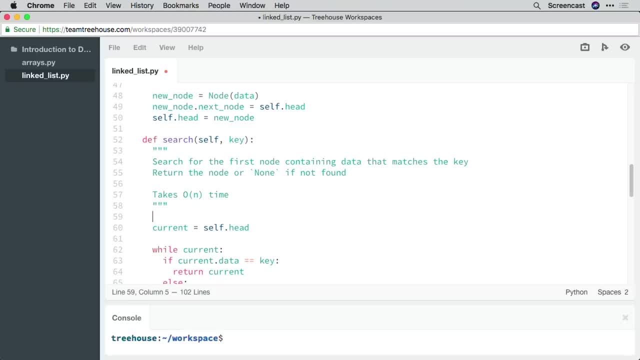 so next let's create two local variables to keep track of index values that we're using for each list. so the convention here is i and j, so we'll stick to it. so i equals zero, j equals zero. as we inspect each value in either list, we'll use the variables. 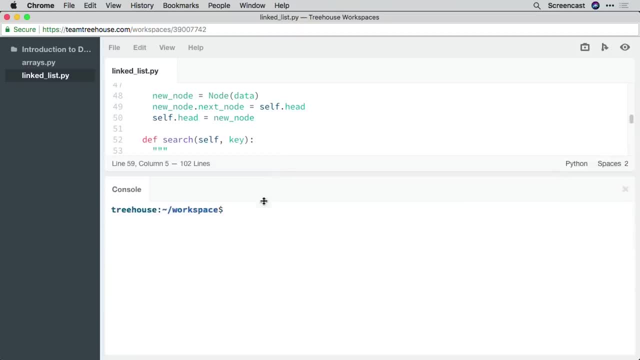 to keep track of the indexes of those values. so we'll use i to keep track of indexes in the left list and j for indexes in the right list. when merging, we want to keep sorting the values until we've worked through both lists. so for our loop, let's set up: 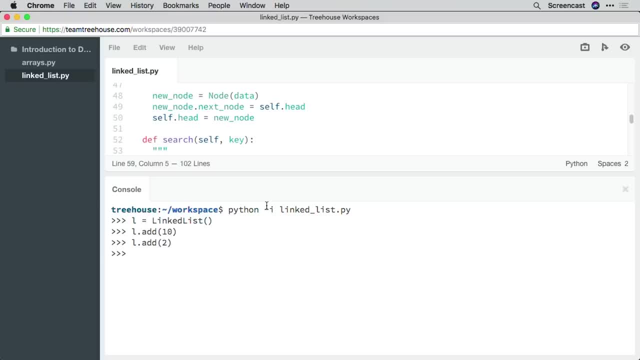 two conditions with an and operator. so we'll say: while, let's just stay up here. while i is less than, while i is less than the length of the left list and j is less than the length of the right list, then we'll keep executing our loop. 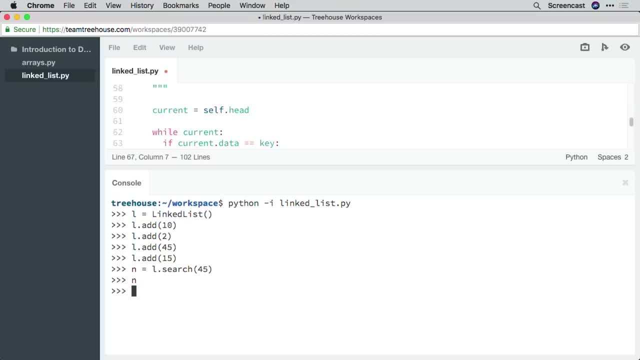 so here we're ensuring that as long as i is less than the length of the left list- and the and is important- and j is less than the length of the right list, we're going to keep executing the code. now i and j are both set to zero. 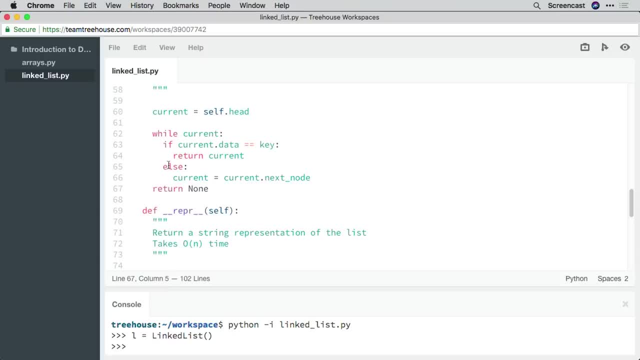 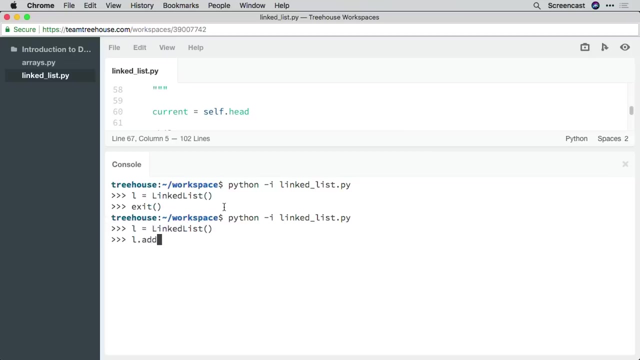 initially, which means that our first comparison operation will be on the first element of each list respectively. so we'll say: if left i, so i is zero, so this is going to get the first value out of the left list is less than right j. and again, here j is. 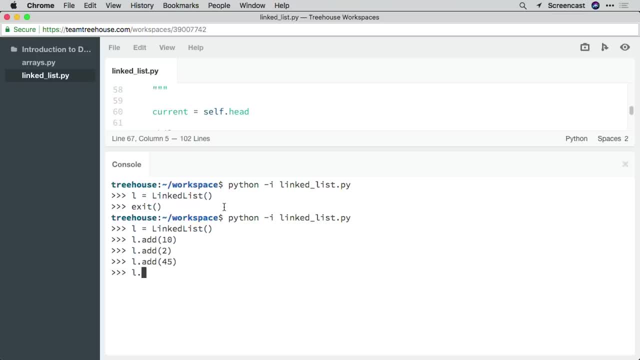 zero. so we're going to get the first value out of the right list. now, if the value at index i in the left list is less than the value at index j in the right list, what do we do? well, that means the value being compared in left. 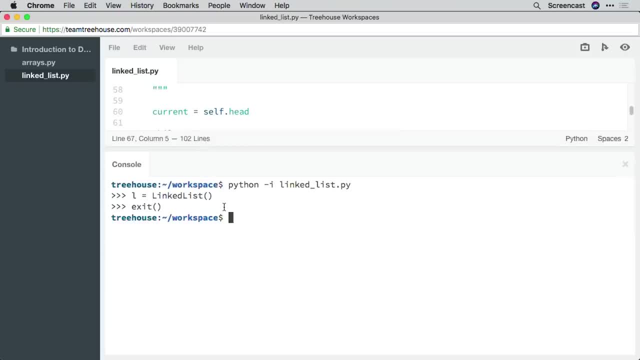 Which means it's outside the while loop, And then we'll run through this again. Okay, So l is linked list. L dot add 10.. L dot add 2.. L dot add 45.. And what was the last one we did? 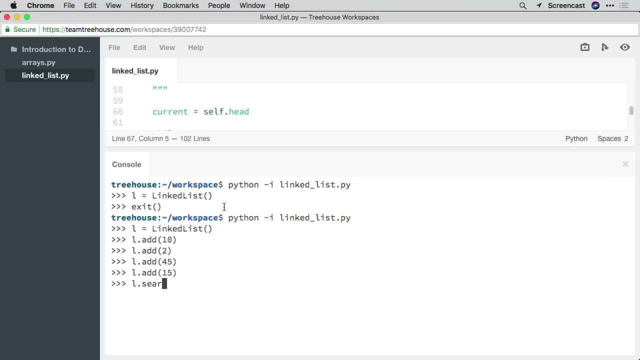 I believe it was 15.. And now we should be able to say l dot search. Remember, we're assigning this to a node, To a variable. So l dot search 45. And there you go, We get that node back. 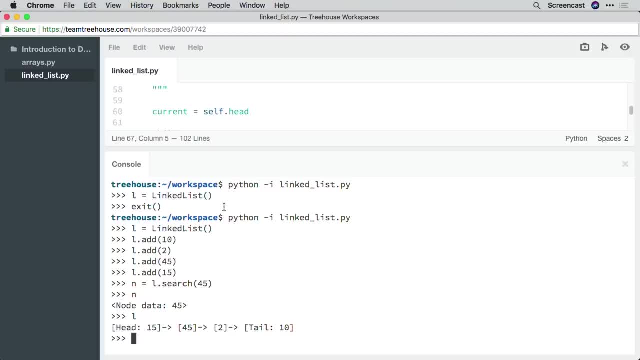 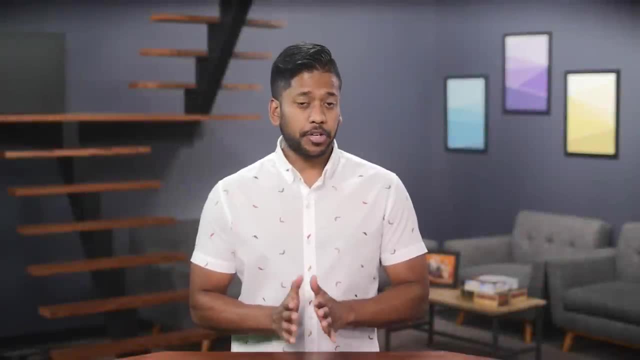 And we can hit l And we'll see a representation of our list. Okay, so again in the next video We're going to look at how to insert and delete At specific positions. Insert operations on linked lists are quite interesting, Unlike arrays. 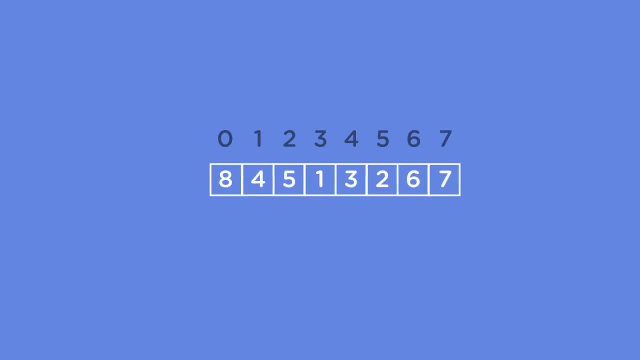 Where, when you insert an element into the array, All elements after the particular index Need to be shifted, With a linked list. We just need to change the references to next On a few nodes And we're good to go, Since each node points to the next one. 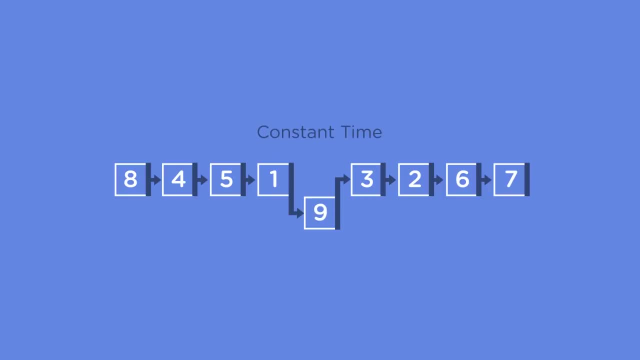 By swapping out these references, We can insert a node at any point in the list In constant time. To find the node at that position We want to insert, We need to traverse the list And get to that point. We just implemented our search algorithm. 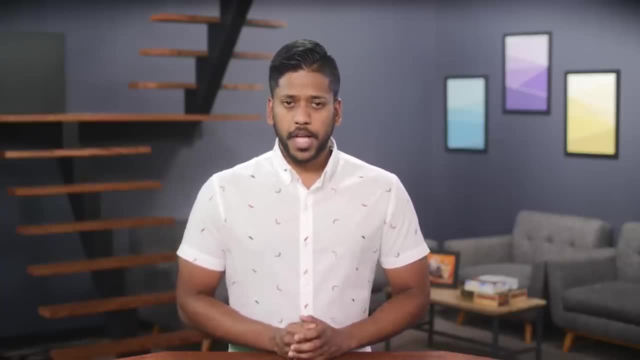 For the linked list type And we know that this runs in linear time. So while actually inserting is fast, Finding the position in the list You want to insert, it is not. This is why I mentioned that There were some caveats to inserting. 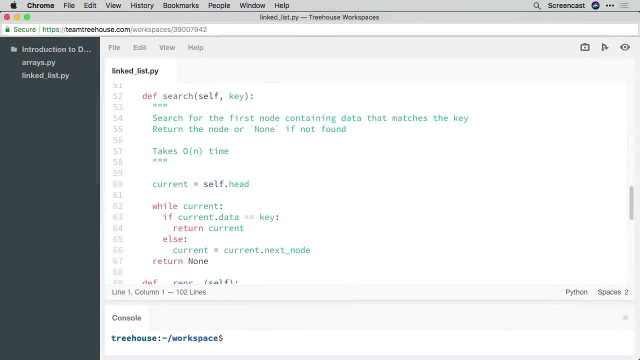 Anyway, let's see what this looks like in code. We'll define a method Named insert, Along with an index position. So we'll do this after search, Right here Say def, Insert, And this takes some data to insert And a position. 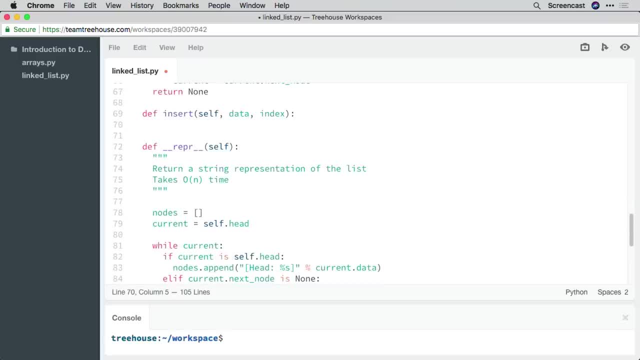 To insert it at. You may be thinking, Wait a minute, Linked lists don't have index positions, And you're correct. But we can mimic that behavior By just counting the number of times we access next node: If the index value 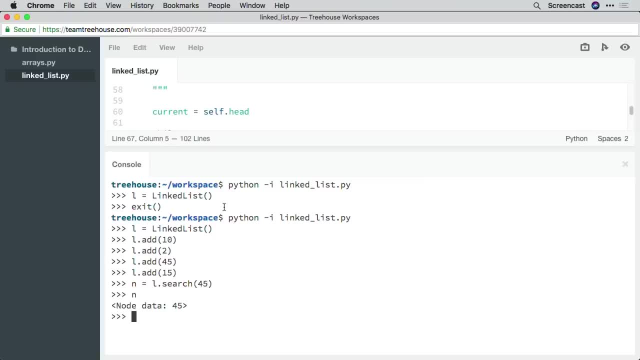 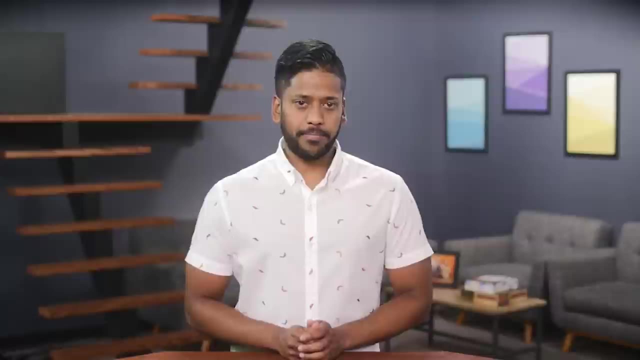 is less than the value in the right and can be placed at position zero in the new array l that we created earlier. so here we'll say l dot append left i. since we've read and done something with the value at position i, let's increment that value. 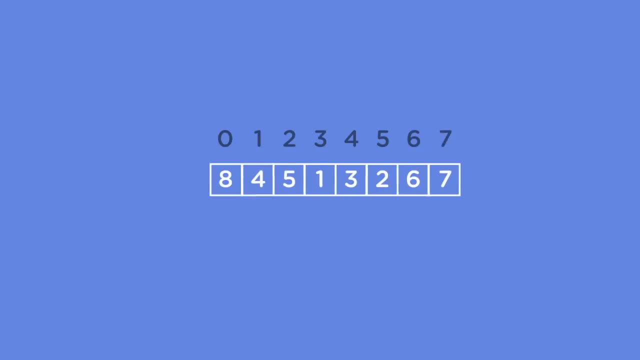 so we move forward to evaluate the next item in the left list: i plus one, or we can say i plus equal one. okay, next is an else statement and here we'll say if the value at index i. so i don't have to write out the actual logic, because 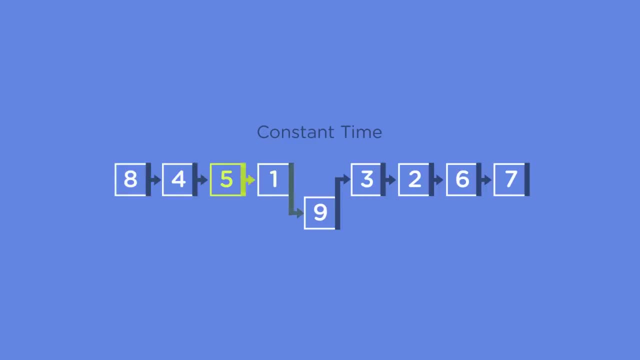 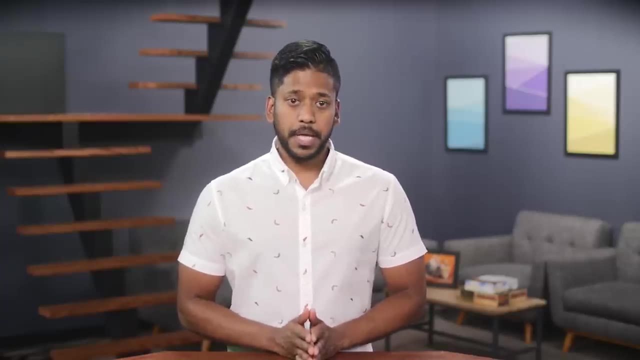 it's implied. so here we're saying that left, the value at left, is less than the value at right now in the else clause, if the value at- so i equal- is greater- and i haven't written out that condition because it's implied- so here we're saying: if the value 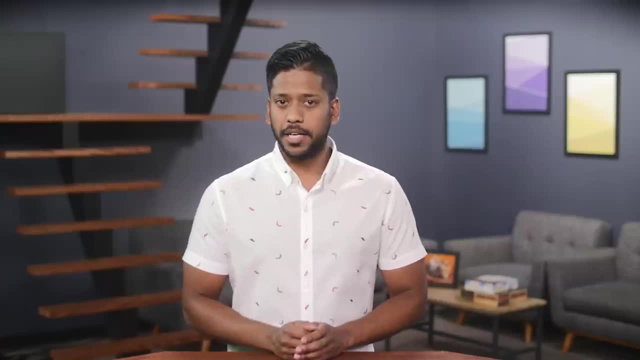 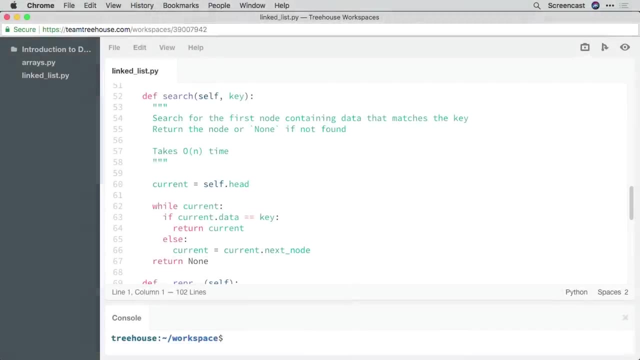 in the left is less than the value in the right. so in the else clause it's going to mean that the value in the left is either greater than or equal to the value in the right. but when we hit the else clause, if the value at index 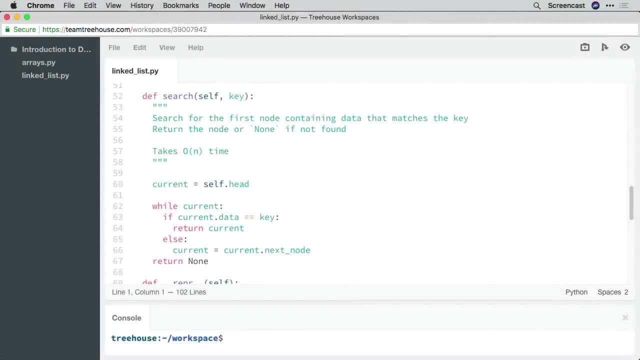 i in the left list is greater, then we place the value at index j from the right list at the start of the new one list, l, and similarly increment j. so here we'll say l, dot, append, write j, and then j equal j plus one. doing this, 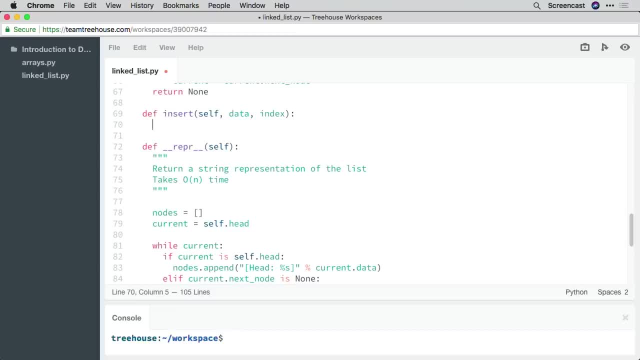 doesn't necessarily mean that in one step we'll have a completely sorted array. but remember that because we start with single element arrays and combine with each merge step, we will eventually sort all the values more than one time, and by the time the entire process is done, all the values are. 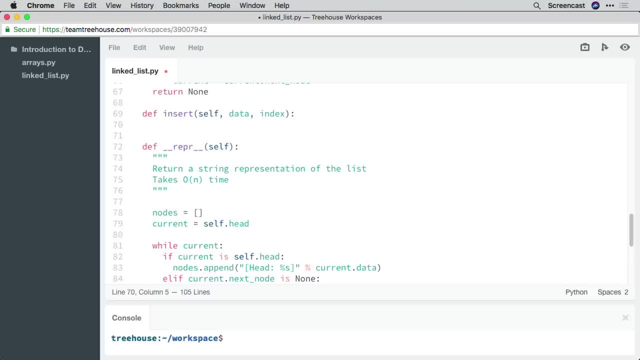 correctly sorted. now this isn't all we need to do in the merge step. however, there are two situations we can run into: one where the left array is larger than the right, and vice versa. so this can occur when an array containing an odd number of elements needs to be split. so how do you split? 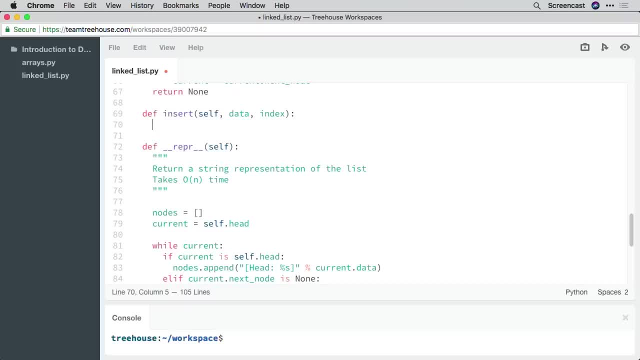 Into this argument is zero, That means we want to insert the new node At the head of the list. This is effectively the same behavior As calling add, Which means the logic is the same, So we don't need to repeat it. 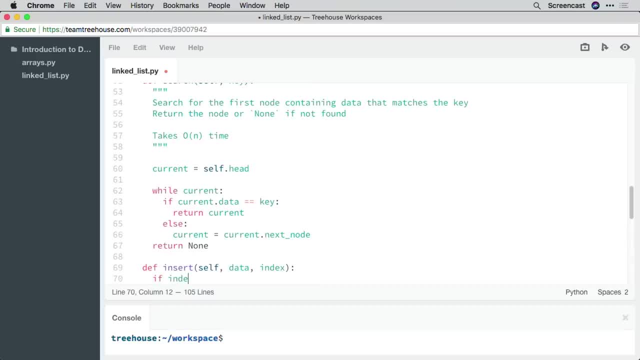 We can call the add method we wrote earlier. So we'll say: if index, If index equals zero, Or if index is zero, Then selfadd Data. If the index is greater than zero, Then We need to traverse the list. 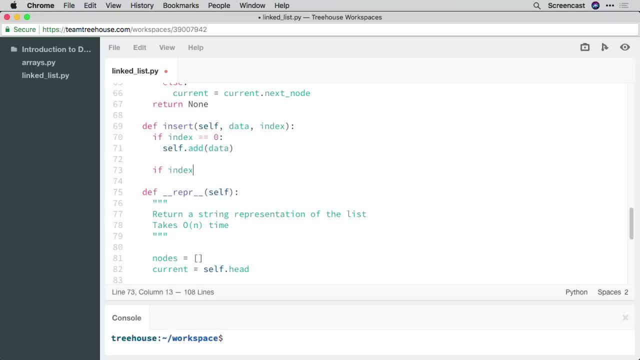 To find the current node at that index. So if index Is greater than zero. Now before we do that We need to create a new node Containing the data we want to insert. So we'll say new Equal node with some data. 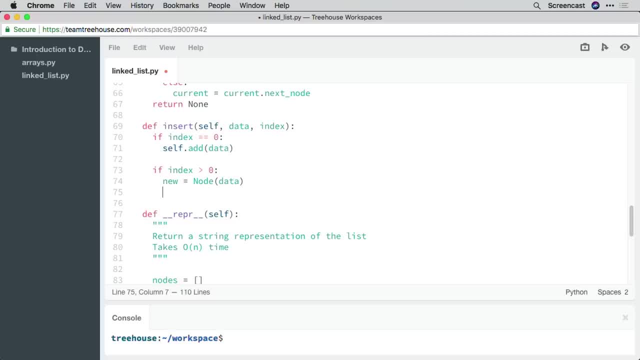 I'm going to assign index The argument passed to our function To a local variable named position And the head of the list To a variable named current Position. Current Equals selfhead Every time we call Currentnextnode. 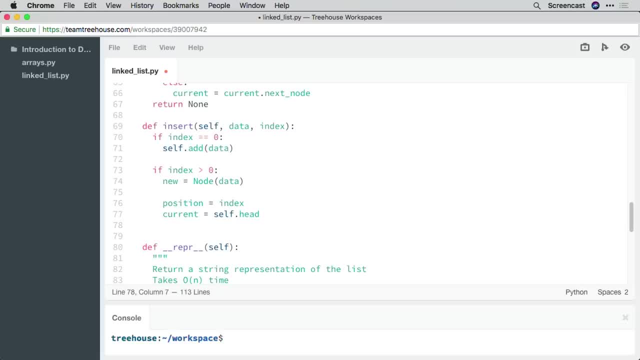 Meaning we're moving to the next node in the list. We'll decrease the value of position By one. When position is zero, We'll have arrived at the node. That's currently at the position we want to insert it. In reality, though, 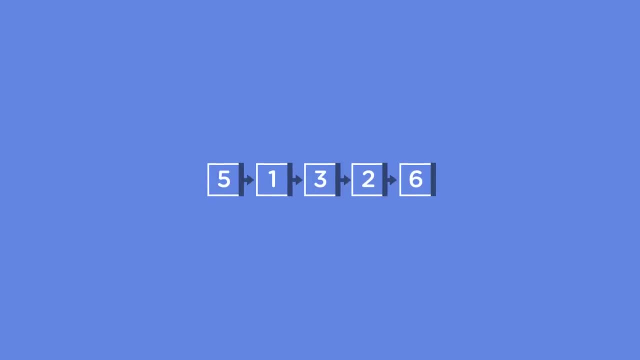 We don't want to decrease it all the way to zero. Imagine we have a list with five nodes And we want to insert a node At position three. To insert a node at position three, We need to modify the nodes At positions two and three. 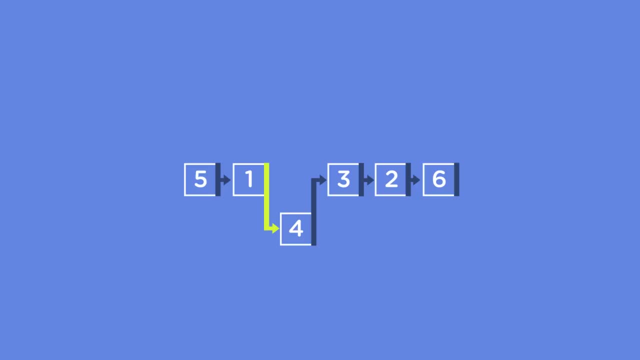 Node two's next node attribute Is going to point to the new node And the new node's next node attribute Will point to node three. In this way, An insert is a constant time operation. We don't need to shift every single element. 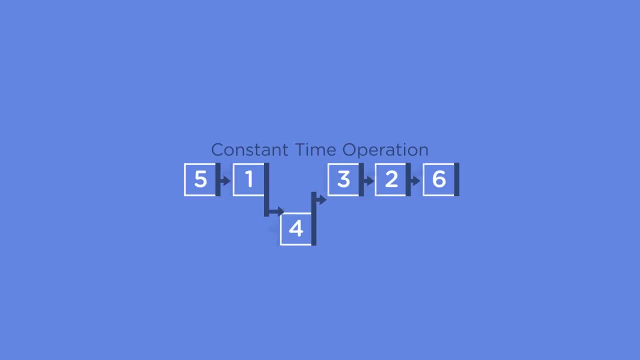 We just modify a few next node references In a doubly linked list. We can use node three In a doubly linked list Would have a reference to node two And we can use this reference To modify all the unnecessary links And a singly linked list though. 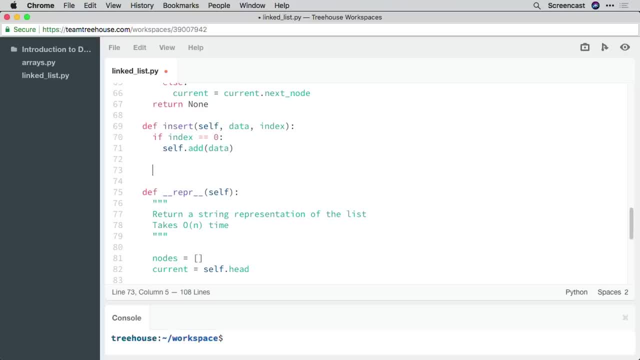 a three element array or list. well, the left can have two elements and the right can have one, or the other way around. in either case, our while loop uses an and condition where the variables used to store the indexes need to be less than the length of the lists. 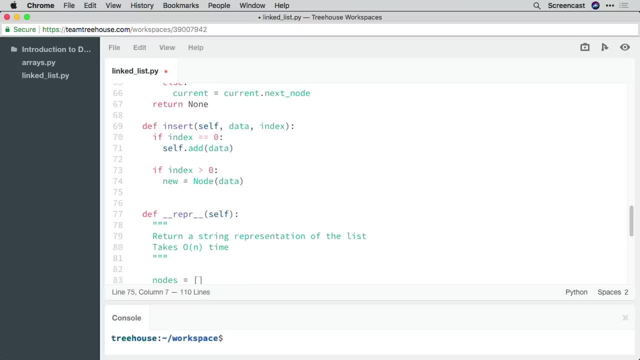 if the left list is shorter than the right, then the first condition returns false and the entire loop returns false because it's an and condition. this means that in such an event, when the while loop terminates, not all the values in the right list will have been moved over to the new. 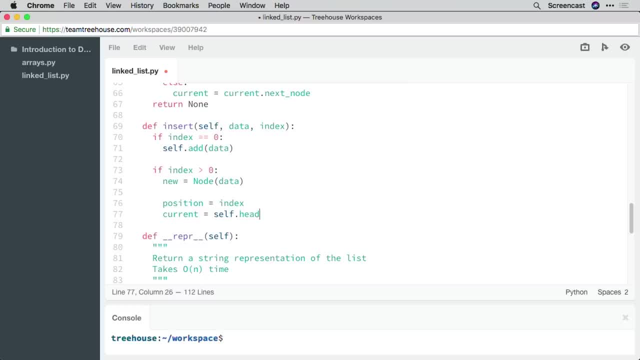 combined list. so to account for this, let's add two more while loops. the first while loop is going to account for a situation where the right list is shorter than the left and the previous loop terminated because we reached the end of the right list first. so in this case, 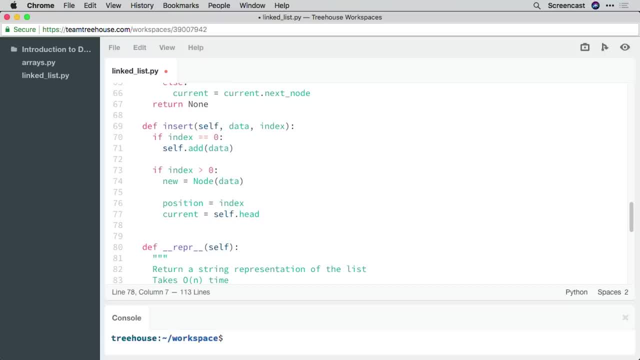 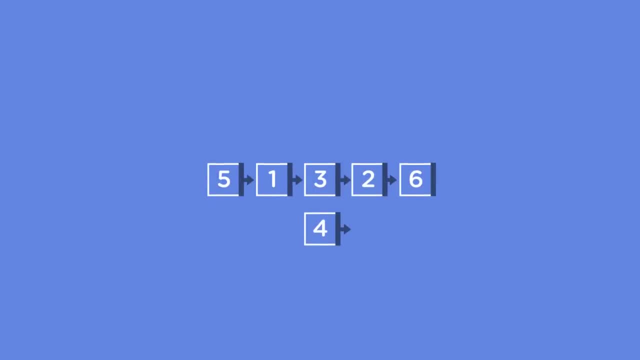 what we're going to do is simply add the remaining elements in the left to the new list. we're not going to compare elements because we're going to assume that within a list the elements are already sorted. so while i is less than length of left, then 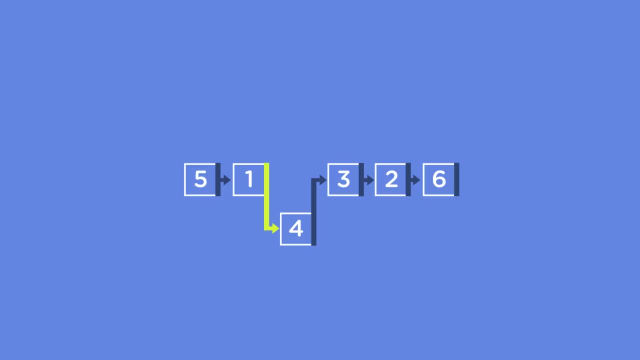 it's the same logic lappend left: i and i plus equal one, so the while loop is going to have the similar condition. keep the loop going until it's at the last index inside the body. we're incrementing the index with every iteration of the loop. our final loop accounts. 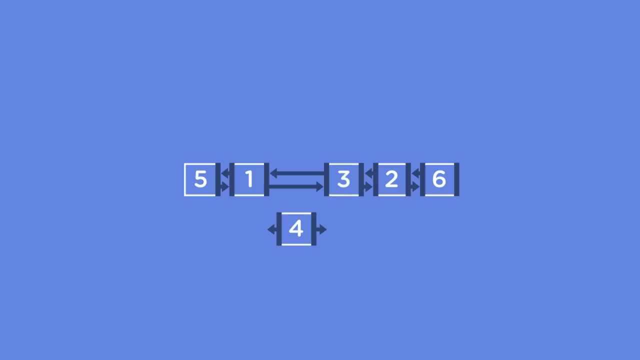 for the opposite scenario, where the left was shorter than the right. the only difference here is that we're going to use the variable j along with the right list. so we'll say: while j is less than length of right lappend right, j and j plus equal one. okay, let's stop. 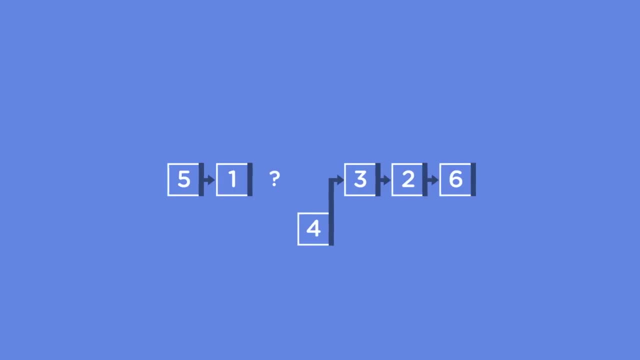 here. in the next video, let's test out merge sort, make sure our code is running correctly and everything is written well, and then we'll wrap up this stage by documenting our code and evaluating the run time of our algorithm. in the last video, we completed our implementation for the merge. 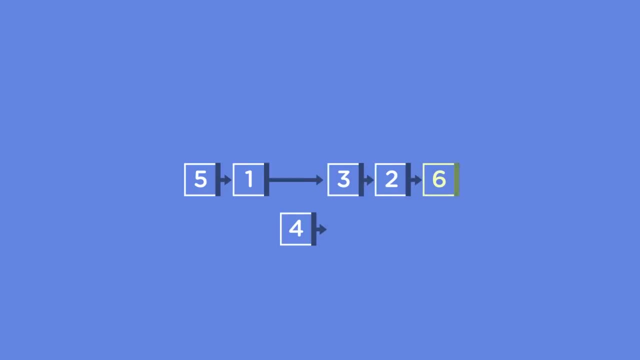 Which is what we have. If we kept decreasing position Until we're at zero, We arrive at node three. We can then set the new node's Next node property To point to node three, But we have no way of getting a reference to node two. 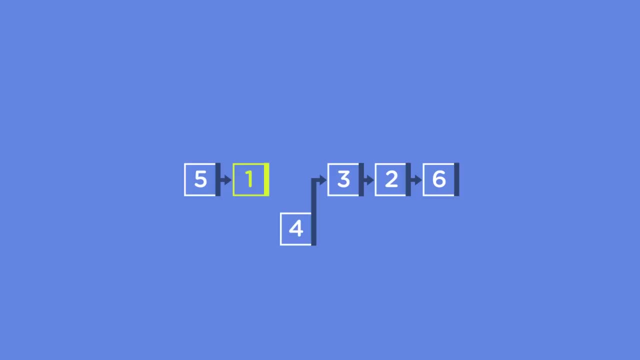 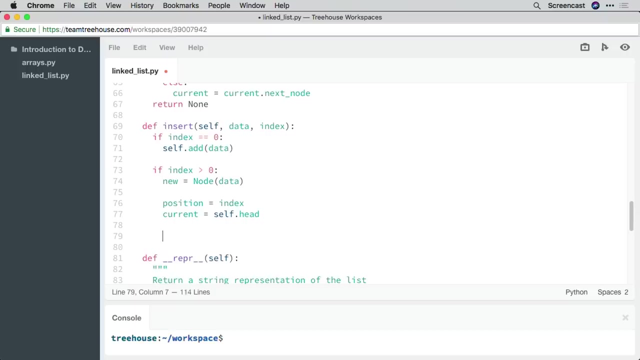 Which we also need. For this reason We can use position to just one When it equals one And stop at node two. So in here we'll say: While position Is greater than one, Now, while the position is greater than one. 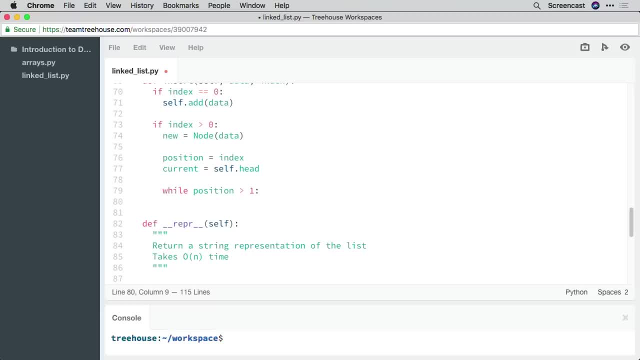 We'll keep calling next node And reassigning the current node. So current Equal node dot next node, And at the same time We'll decrement position. So position Equal to position Minus one, Which you can also succinctly write as: 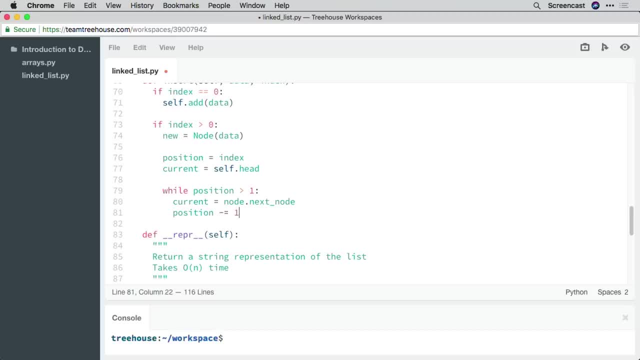 Minus equal one. This way, When the position equals one, The loop exits, And current will refer to the node at the position Before the insert point. So outside the while loop We'll say previous equal current And next Equal current dot. next node. 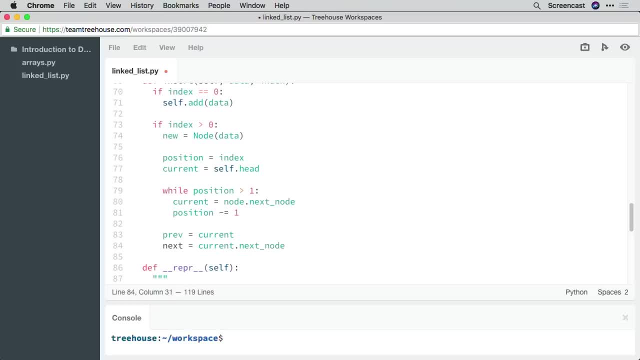 To make things more clear, What I've done here Is insert the new one previous And the node after the new one next. All that's left to do now Is to insert the new node Between previous and next, So we'll say previous dot next. 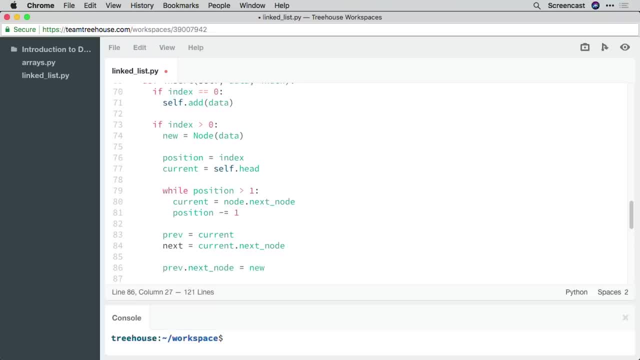 Node Equal new And then new dot next, node Equal next. Now it seems like There's an issue with variable naming here And I'm most probably Conflicting with some globally named next variable. So we'll actually go ahead and call this. 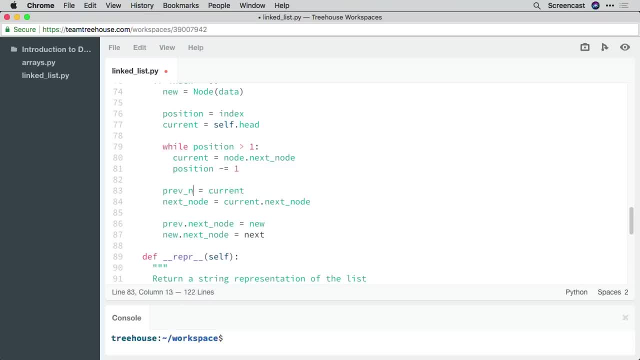 Previous node And Previous node, So that we don't mess things up here. Previous node, So the dot. next node Is obviously the attribute on a node, But this is just a local variable. Let's document this method So up at the top. 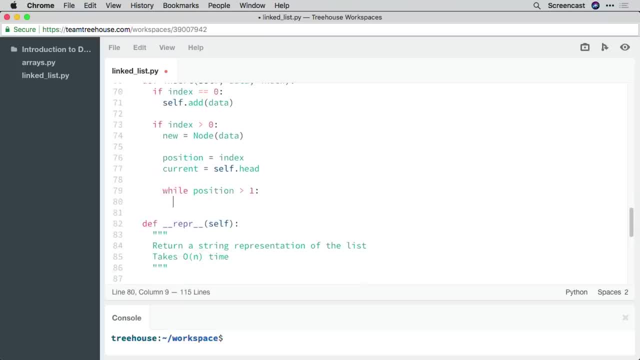 sort algorithm, but we didn't test it in any way. let's define a new list at the bottom that contains several numbers. you can put whatever you want in there, but make sure that the numbers are not in order. i'll call mine a list and here we'll say: 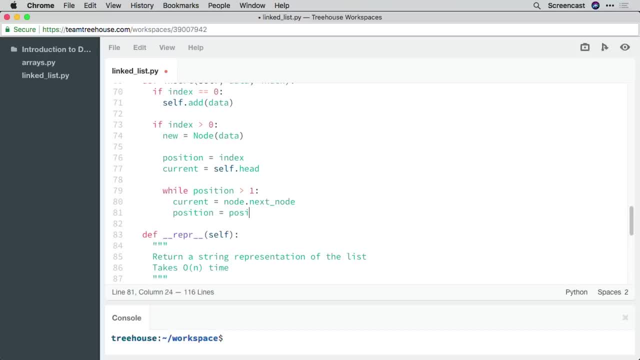 54, 26 or 62, doesn't matter. 93, 17, 77, 31, just add enough so that you can make out that it's sorted. okay, next we're going to call the merge sort algorithm and pass in our list. let's assign this to some. 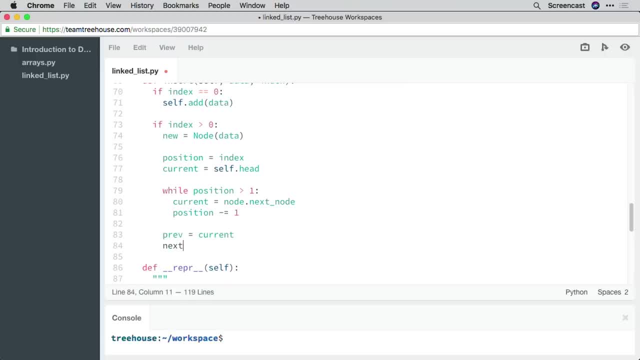 variables. so we'll say l equal, merge, underscore, sort a list and then, if it works correctly, we should be able to print this list and see what it looks like. so i'm going to hit save down here in the console we'll type out: python, merge, sort. 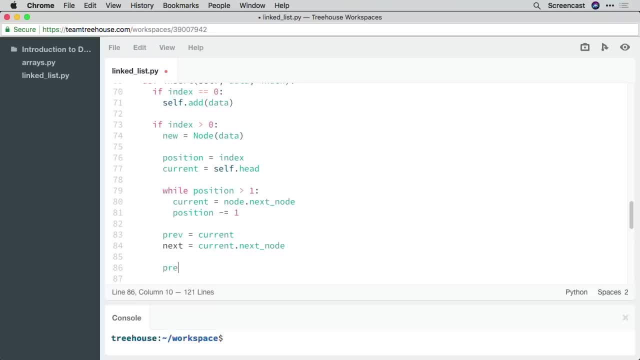 dot pi, and before i hit enter, i actually noticed i made an error in the last video, but i'll hit enter anyway and you should see the error pop up, okay? so what i forgot to do, which is a pretty crucial part of our algorithm, is in the merge function. i forgot to. 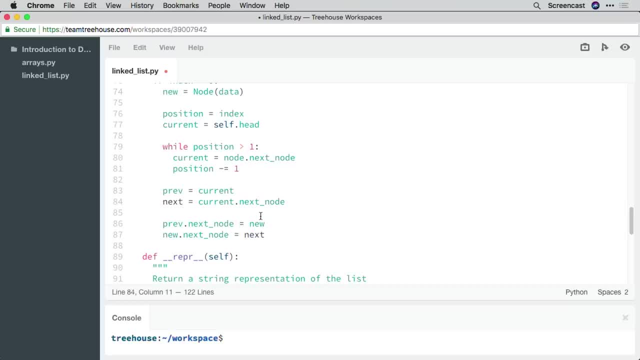 return the list containing the sorted numbers after carrying out all this logic. so here at the bottom we'll say: return l, alright, we'll save again. and now we'll clear this out and try that one more time. and there we go. you should see a sorted list printed out. 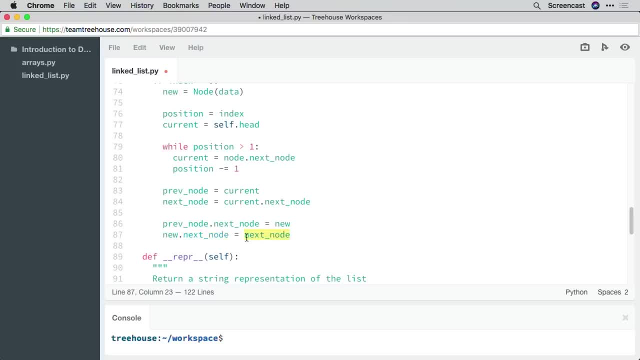 we can write out a more robust function to test this, because with bigger arrays, visually evaluating that printed list won't always be feasible. so we'll bring this back down. let's get rid of this and we'll call our function verify sorted and this will take a list. 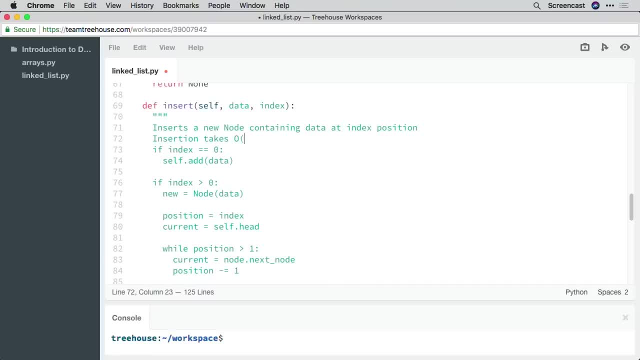 first we're going to check inside the body of the function. we'll check the length of the list. if the list is a single element list or an empty list, we don't need to do any unnecessary work because- remember, it is naively sorted. so we'll say: if n. 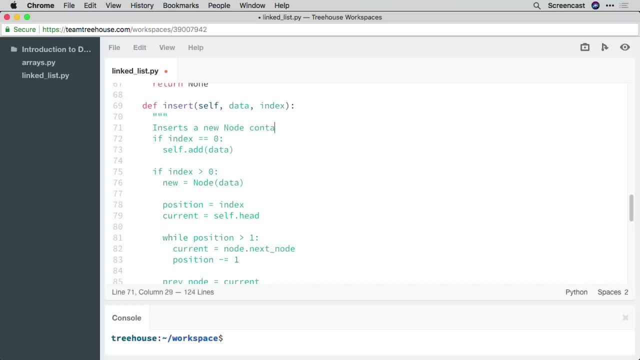 We'll add a doc string And it will say: inserts a new node Containing data At index Insertion. Insertion takes Constant time, But finding the node At the insertion Point Takes linear Time. Let's add this to the next line. 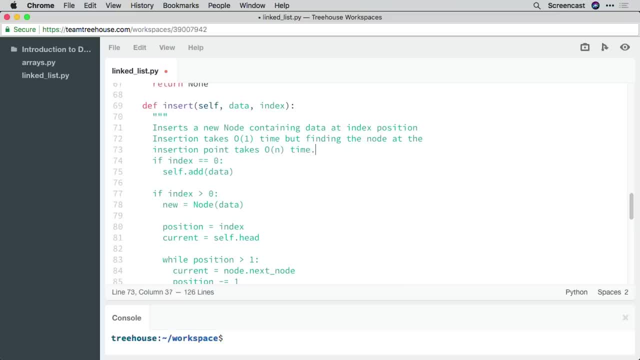 There we go And then we'll say: Therefore, it takes an overall Linear Time. This is why, Even though we can easily insert a new node Without having to shift the rest, Ultimately Adding to either the head or the tail. 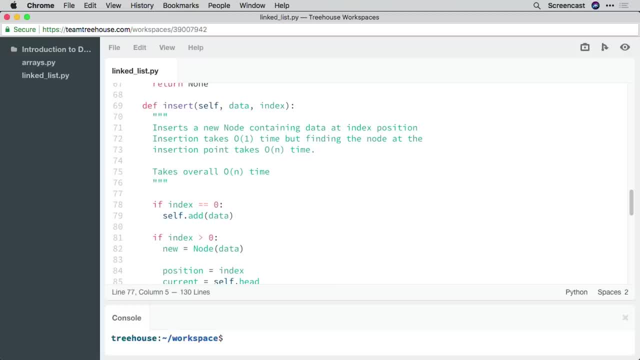 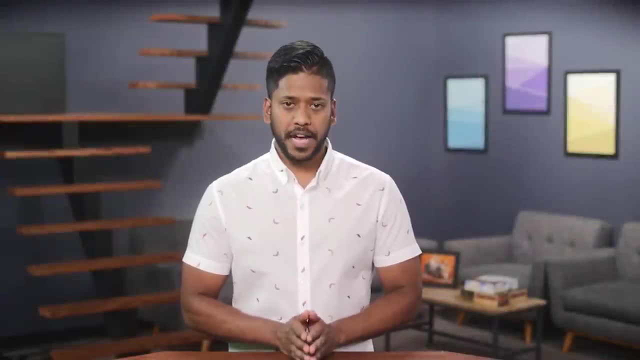 If you have a reference, Is much more efficient. We have one more operation to add to our linked list That will make it a robust data structure, Much like inserts. Removing a node is actually quite fast And occurs in constant time To actually get to the node that we want to remove. 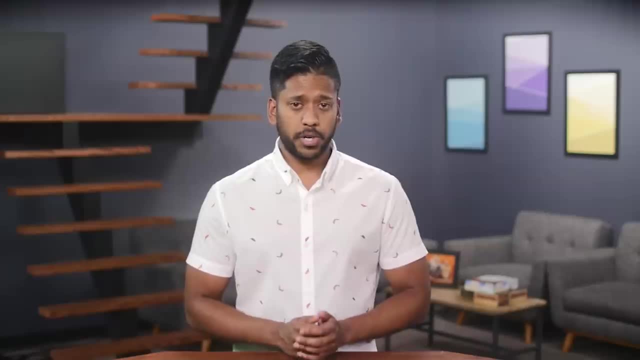 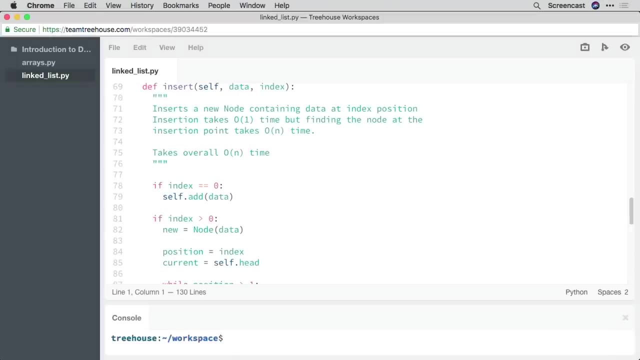 The next connections: We need to traverse the entire list In our worst case. So in the worst case This takes linear time. Let's add this operation to our data structure. There are two ways we can define the remove method: One where we provide a key. 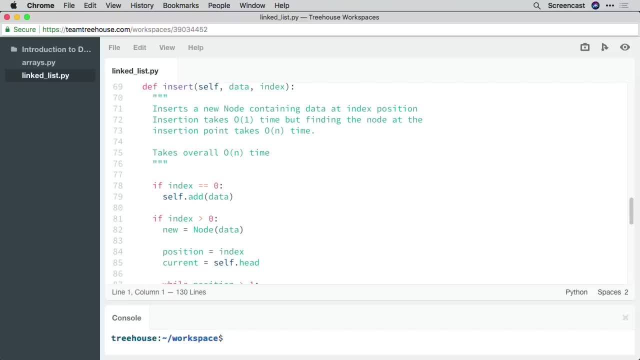 To remove as an argument, And one where we provide an index. Now, in the former, The key refers to the data the node stores. So in order to remove that node, We would first need to search for data, Which is the key. 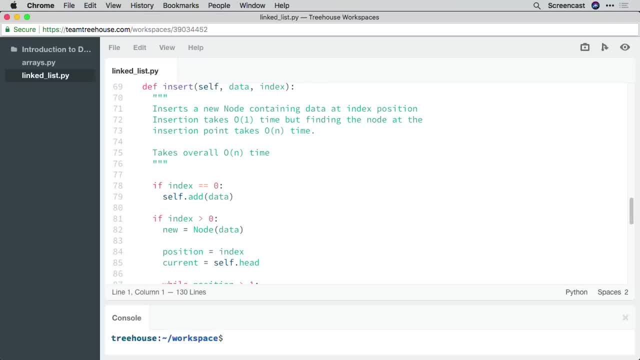 I'm going to implement that first method, Which we'll call remove, And I'll leave it up to you to get some practice in And implement a remove at index method To complete our data structure. So we'll add this after the insert method. 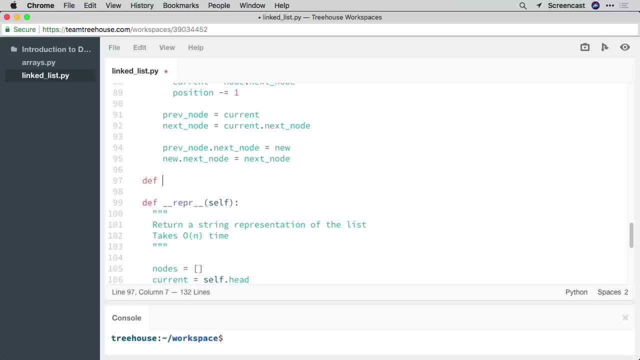 Right here. Remove Is going to accept a key Which we'll need to search for Before we can remove a node. Earlier we defined a search method That found a node containing data That matches a key, So we'll use that method as is. 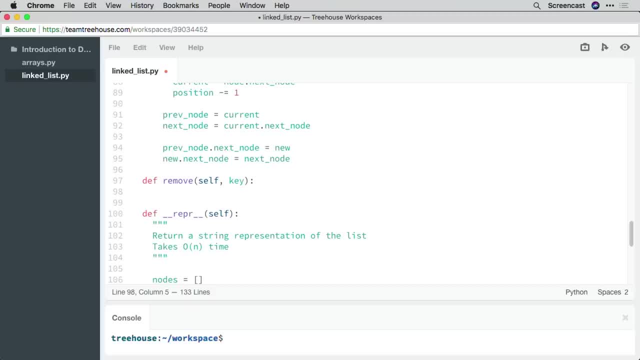 For the implementation of remove. When we remove a node, Much like the insert operation, We need to modify: the next node references. The node before the match Needs to point to the node after the match If we use the search method We defined earlier. 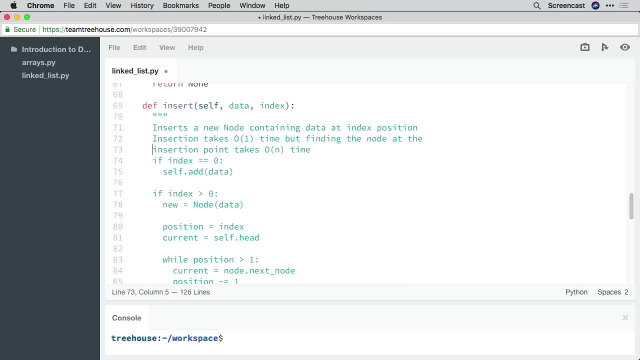 equals 0, or if n equals 1, then we'll return true, we've verified that. it's sorted. now, to conclude our function, we're going to write out one line of code that will actually do quite a bit of work, so first we'll say return list. 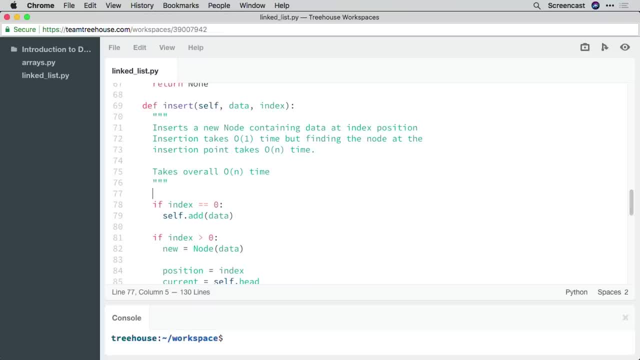 0. so we'll take the first element out of the list and we'll compare and see if that's less than the second element in the list. ok, so first we'll check that the first element in the list is less than the second element in the list. this returns either. 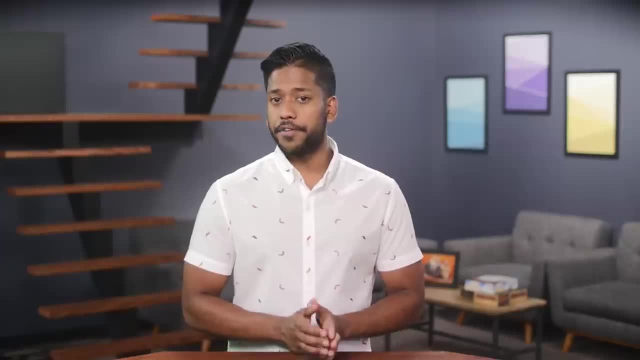 true or false, so we can return that directly. but this isn't sufficient. if it were, we could trick the verify function by only sorting the first two elements in the list. so to this return statement we're going to use an and operator to add on one more condition. 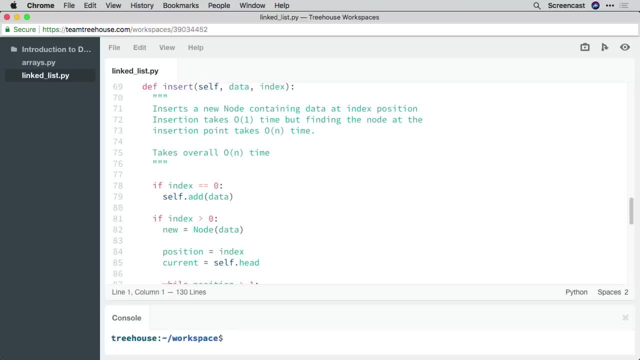 for this condition, we're going to make a recursive function call back to verify sorted. and for the argument, we're going to pass in the list, going from the second element all the way to the end. let's visualize how this would work. we'll use a five element. 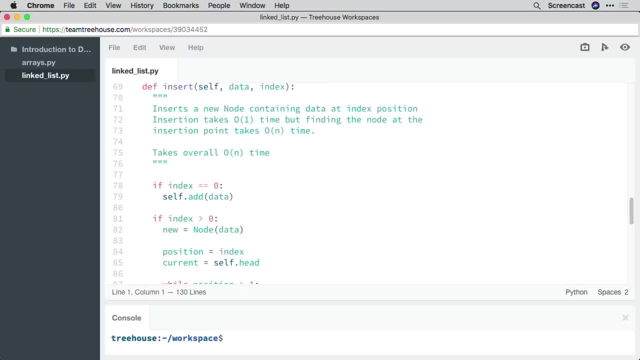 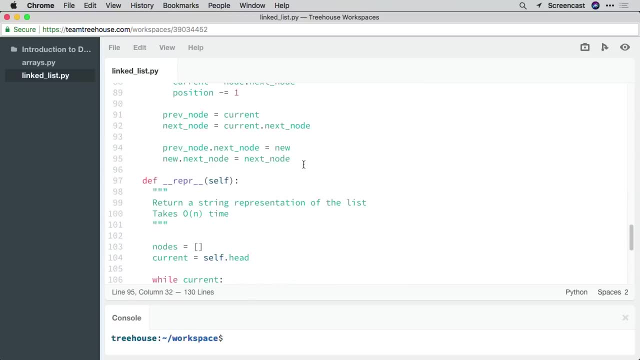 list as an example. so we'll call, verify, sorted and pass in the entire list. this list is not one or zero elements long, so we skip that first. if statement there's only one line of code left in the function and first we check that the element at index zero. 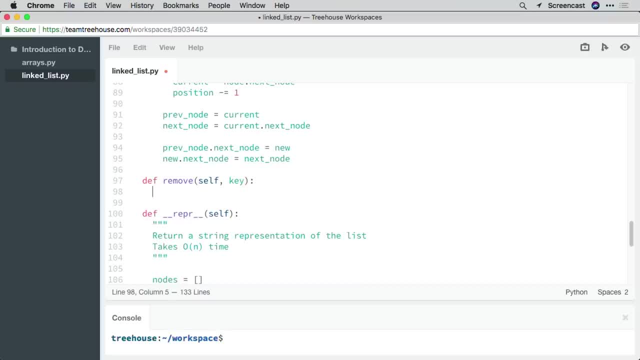 is less than the element at index one. if this is false, the function returns immediately with a false value. an and operator requires both conditions to be true for the entire line of code to return true. since the first condition evaluates to false, we don't need to bother evaluating. 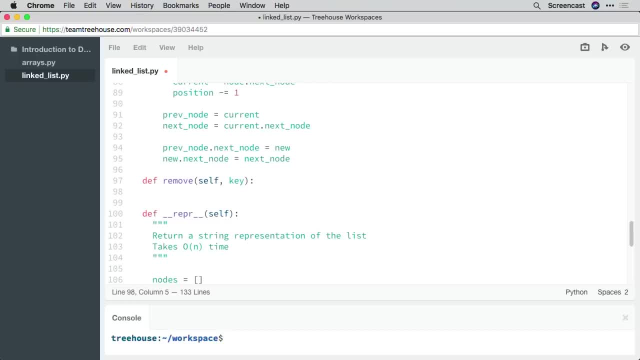 the second. the second condition is a recursive call with a sub list containing elements from the original list, starting at position one and going to the end. so, on the second call again, we can skip that first if statement and proceed to check whether the value at element zero is less than the value. 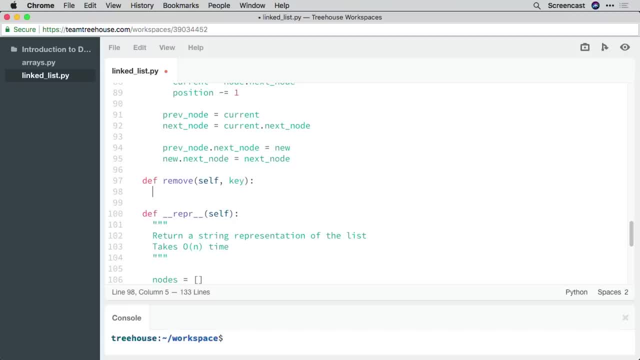 at element one. remember that because this list is a sub list of the original, starting at the element that was the second element in the original list, by comparing the elements at position zero and one in the sub list, we're effectively comparing the elements at position one and two in the original. 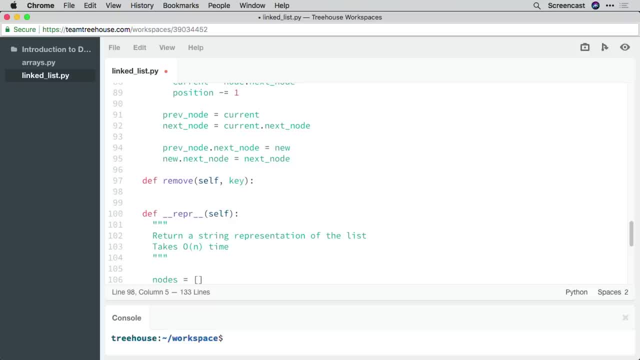 We get the node we want to remove As a return value, But because this is a singly linked list, We can't obtain a reference to the previous node. Like I said earlier, If this was a doubly linked list, We can't use the search method. 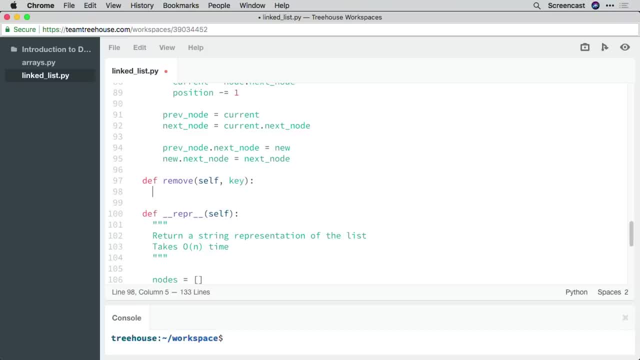 Since we would have a reference to that previous node, We'll start here by setting a local variable Named current To point to the head. Let's also define a variable Named previous That we'll set to none To keep track of the previous node. 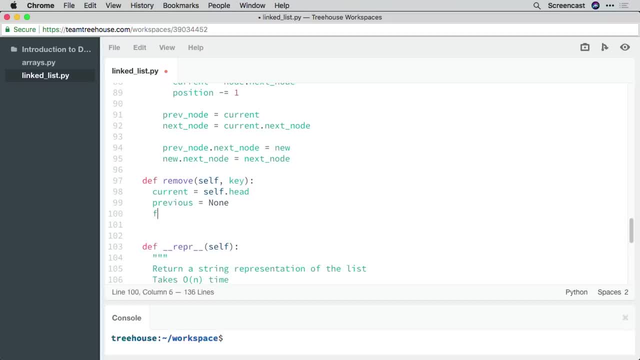 As we traverse the list. Finally, let's declare a variable Named found, That we'll set to false. Found is going to serve as a stopping condition For the loop that we'll define. We'll use the loop to keep traversing the linked list. 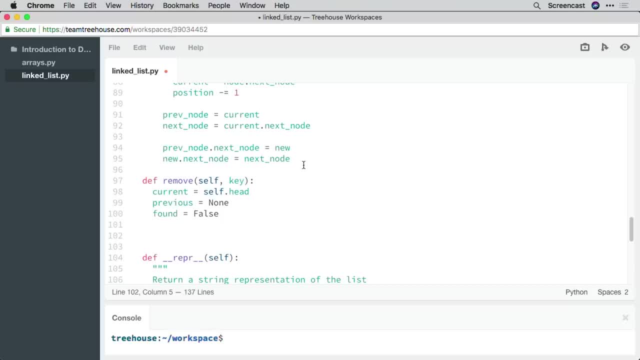 As long as found is false Meaning we haven't found the key That we're looking for. Once we've found it, We'll set found to true And the loop terminates. So let's set up our loop. So we'll say: while current. 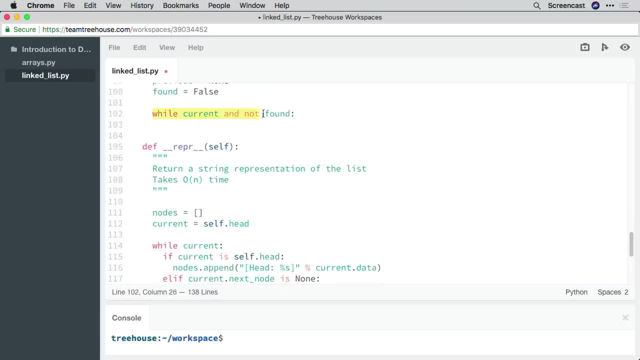 And not found Here. we're defining a while loop That contains two conditions. First, we tell the loop To keep iterating As long as current does not equal none. When current equals none, This means we've gone past the tail node. 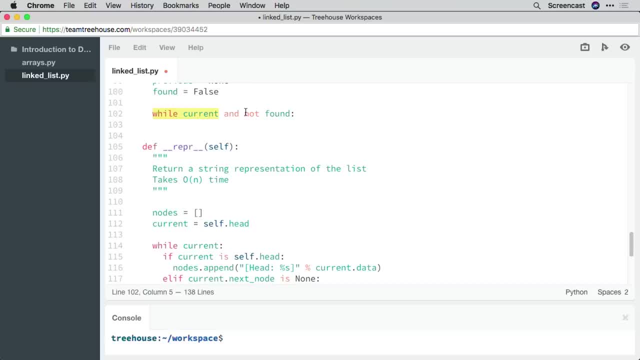 And the key doesn't exist. The second condition Asks the loop to keep evaluating As long as not found equals true. Now, this might be tricky Because it involves a negation here Right now. found is set to false, So not found. 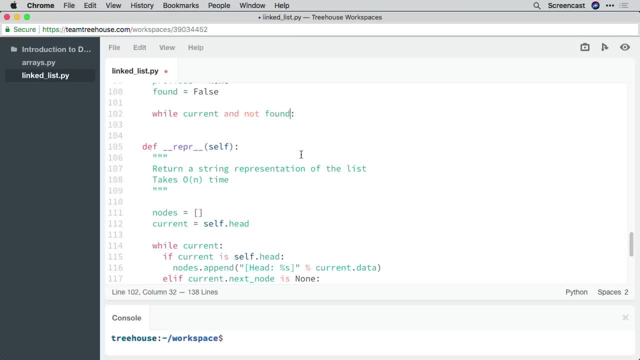 Not false equals true. This not operator Flips the value. When we find the key And we set found to true. Not found Will equal false then And the loop will stop. The and in the while loop Means that both conditions. 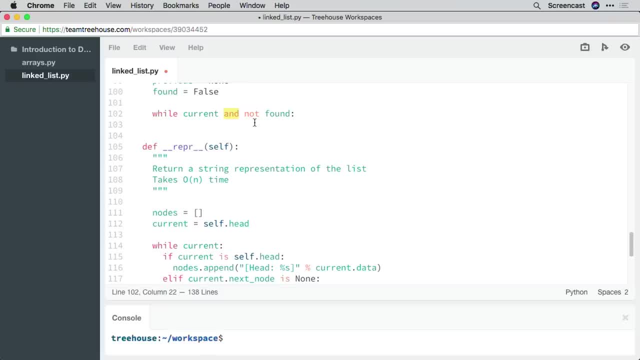 Current being a valid node And not found equaling true. Both have to be true. If either one of them evaluates to false, Then the loop will terminate. Now, inside the loop, There are three situations that we can run into. First, the key matches the current nodes- data. 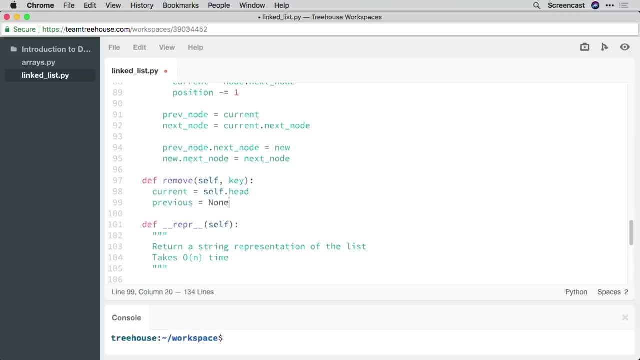 list. with each recursive call, as we create new sub lists that start at index position one, we're able to check the entire list without having to specify any checks other than the first two elements. since this is a recursive function, it means we need a stopping condition, and we have it already. 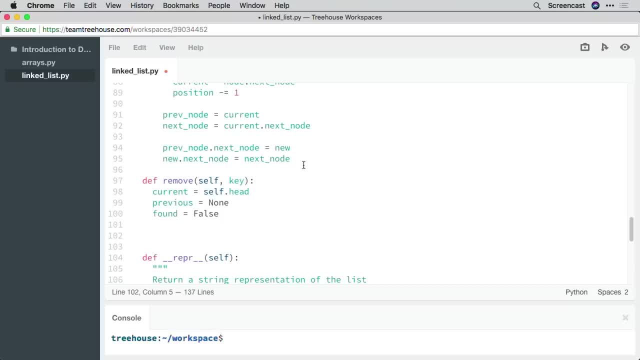 it's that first if condition. as we keep making sub lists, once we reach a single element list, that element is already sorted by definition, so we can return true. since this recursive function call is part of an and condition, it means that every single recursive call has to. 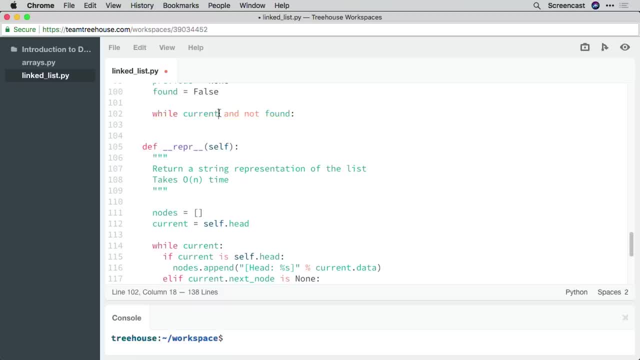 return true all the way back to the beginning, for our top level function to return true and for the function to say yes, this is sorted now. we could have easily done this using an iterative solution and a for loop, but this way you get another example of recursion to work. 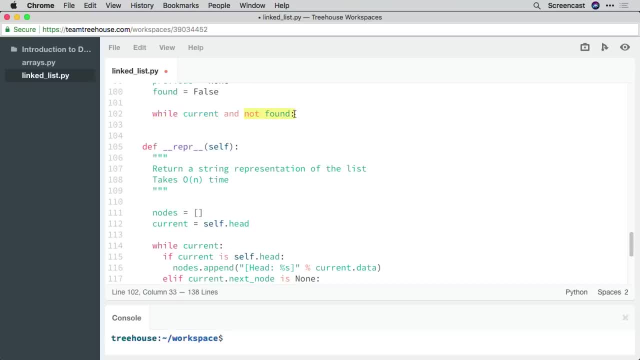 through and understand. so let's use this function. at the bottom we'll say print, verify, sorted, and first we'll pass in a list. oops, we got rid of that, didn't we? okay, let me write it out again. so a list equal, and i think i have those original. 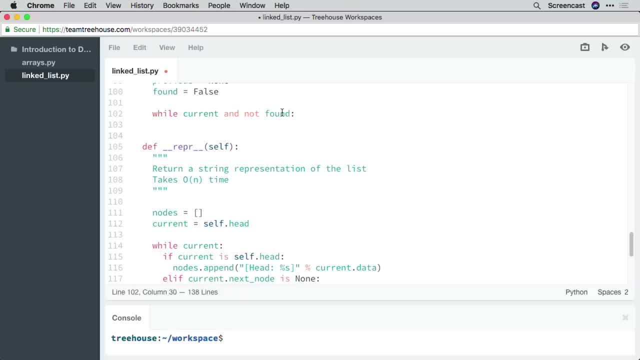 numbers here somewhere. so we'll say 54, 26, 93, okay, and then we assign it to l. the result of calling merge sort on a list: okay. so now here we're going to use the verify sorted function and we'll check first that a list is sorted. 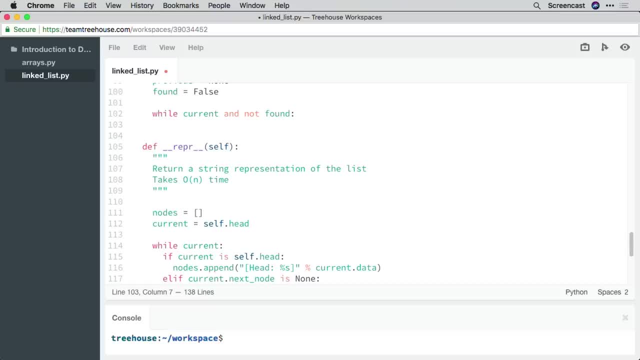 that should return false and then we'll check the same call on, we'll pass in l and this should return true. okay, so now at the bottom here in the console we'll call python, merge, sort, dot, pi. and there we go. it returned false for a list, meaning it's not sorted. 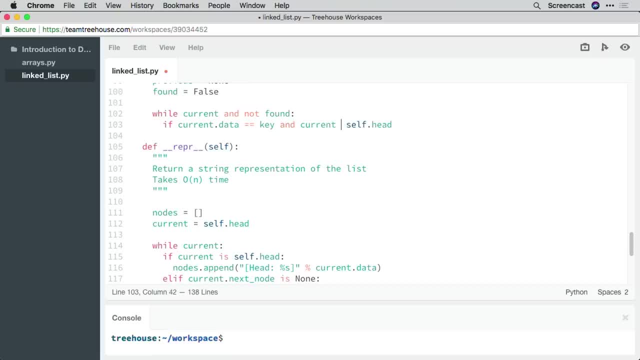 but l is sorted, cool, so our merge sort function works. in the next video let's talk about the cost of this algorithm. if we go back to the top level, the merge sort function, what does the run time of this function look like and what about space complexity? 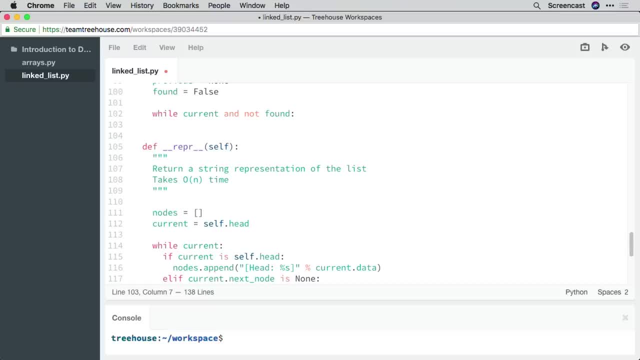 And current is still at the head of the list. This is a special case. We have a previous node And it's the only node being referenced by the list. Let's handle this case. So we'll say if current dot data Double equals the key. 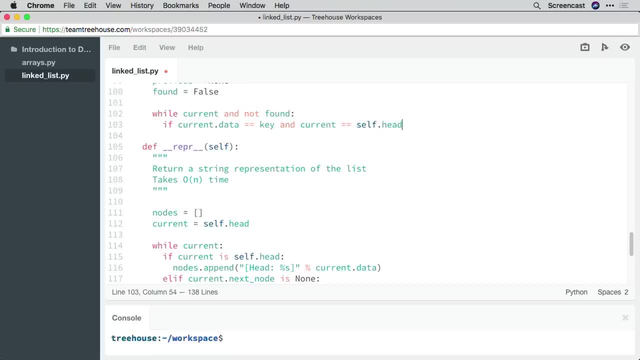 And current Is self dot head, Which you can write out as current equals self dot head Or current is self dot head. Now, if we hit, this case Will indicate that we found the key By setting found to true And then this means that on the next pass, 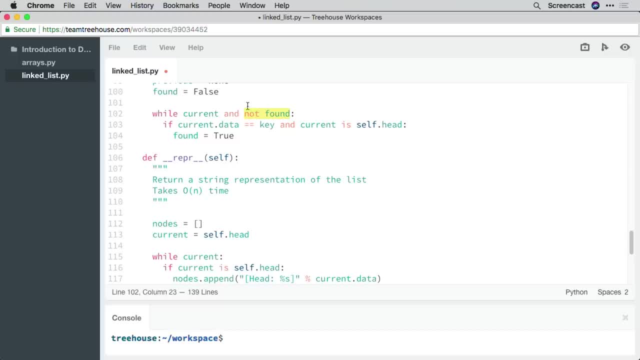 This is going to evaluate To false, Because not true will be false, And then the loop terminates. Once we do that, We want to remove the current node And since it's the head node, All we need to do is point head. 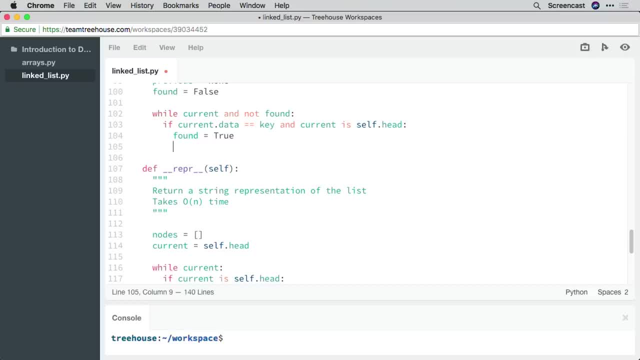 To the second node in the list Which we can get by referencing the next node attribute On current Self dot head equal current dot next node. So when we do this There's nothing pointing to that first node, So it's automatically removed. 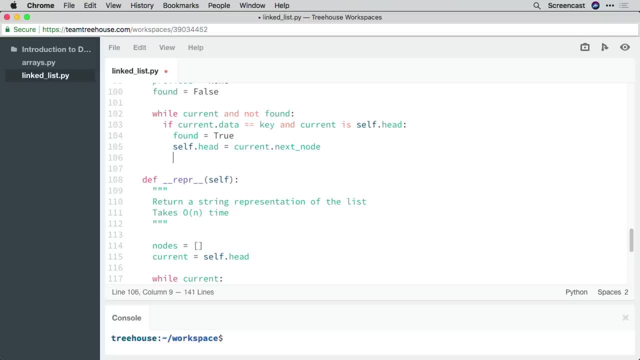 The next scenario Is when the key matches data in the node, And it's a node, that's not the head. So here we'll say else: if Current dot data Equal key, If the current node Contains the key we're looking for. 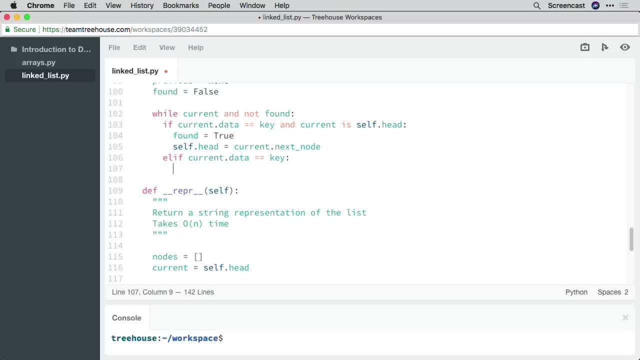 We need to remove it. To remove the current node, We need to go to the previous node And modify it's next node reference To point to the node after current. But first we'll set found To true And then we'll switch out the references. 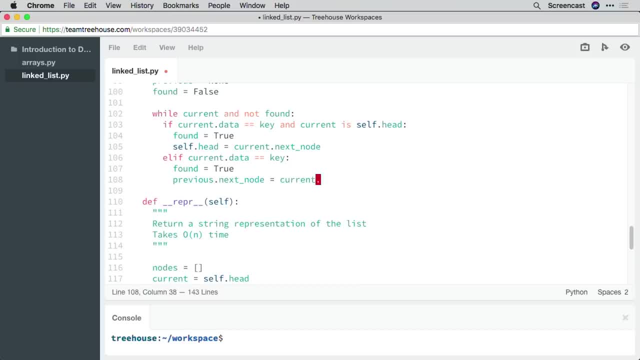 To the previous dot next node Equal current dot next node. So far We haven't written any code To keep track of the previous node. We'll do that in our else case here. So if we hit the else case It means that the current node 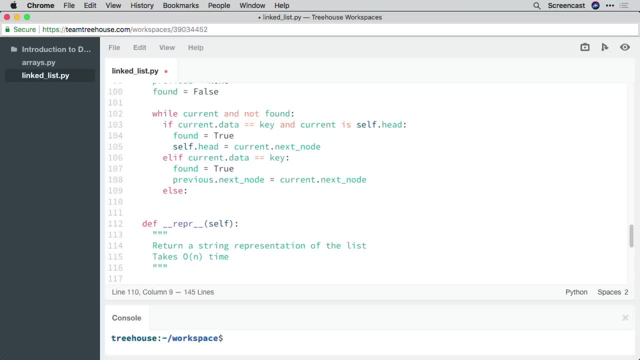 We're evaluating doesn't contain the data That matches the key. So in this case We'll make previous point to the current node And then set current to the next node. So previous equal current And current equal current Dot. next node. 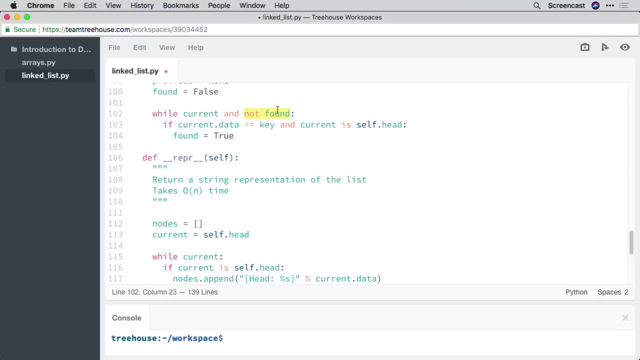 how does memory usage grow as the algorithm runs? to answer those questions, let's look at the individual steps, starting with the split function. in the split function, all we're doing is finding the midpoint of the list and splitting the list at the midpoint. this seems like a constant time operation. 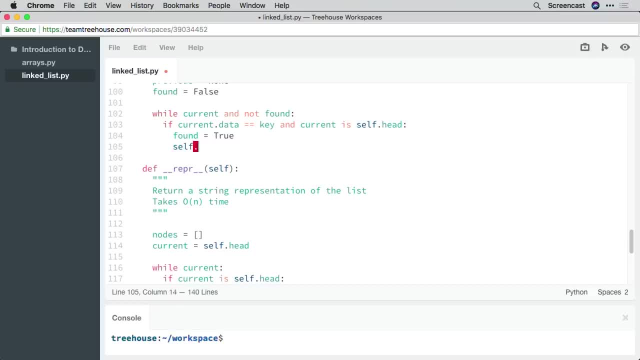 but remember that the split function isn't called once. it's called as many times as we need it to to go from the initial list down to a single element list. now, this is a pattern we've seen a couple times now and we know that overall this runs in logarithmic. 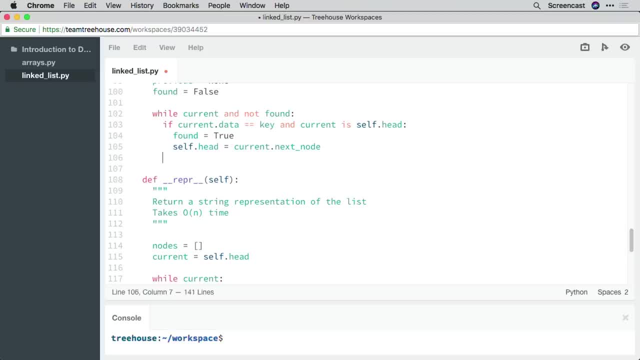 time. so let's add that as a comment. so here I'll say: takes overall big O of log n time. now there's a caveat here, but we'll come back to that. so next up is the merge step. in the merge step we've broken the original list down into single. 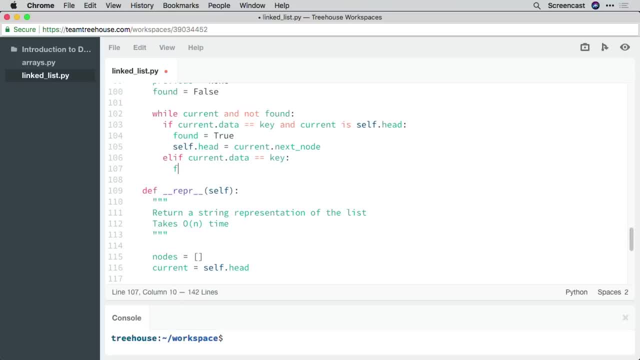 element lists and now we need to make comparison operations and merge them back in the reverse order. for a list of size n, we'll always need to make an n number of merge operations to get back from single element lists to a merge list. this makes our overall run time. 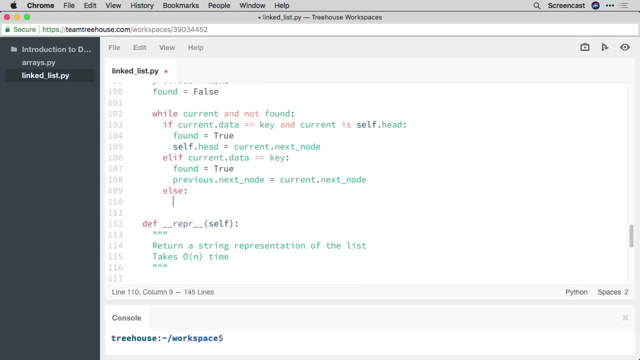 big O of n times log n, because that's an n number of merge steps multiplied by log n, number of splits of the original list. so to our merge step here let's add a comment. we'll say it runs in overall. oops, there we go. runs in overall. 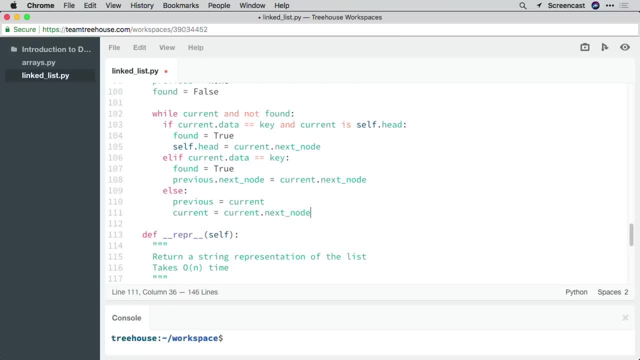 linear time. right, it takes an n number of steps, number of merge steps. but now that we have these two so linear here and logarithmic here, we can multiply these and say that the merge sort function, the top level function, we can conclude that the run time of the overall sorting process 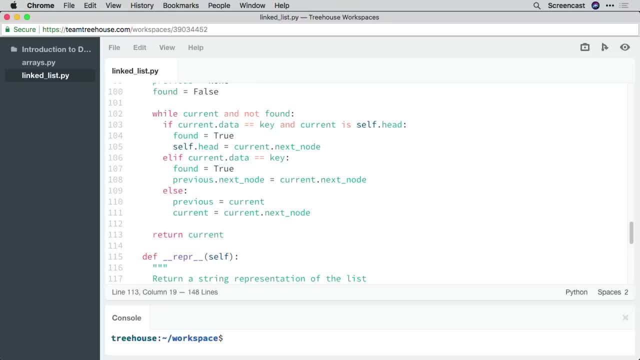 is big O of n times. log n. now what about that caveat I mentioned earlier? so if we go back to our split function here, right here there we go. let's take a look at the way we're actually splitting the list. so we're using Python's. 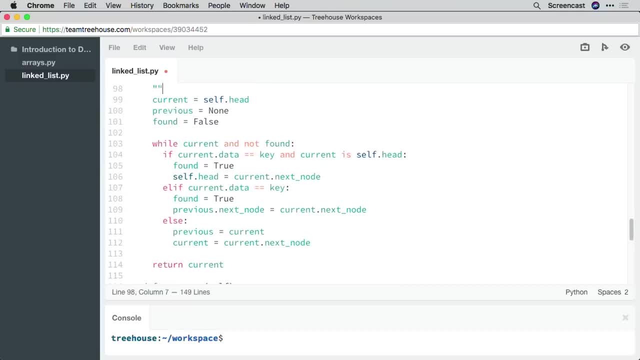 list slicing operation here and passing in two indexes where the split occurs. now, if you go and poke around the Python documentation, which I've done, it says that a slicing operation is not a constant time operation and in fact has a run time of big O of k. 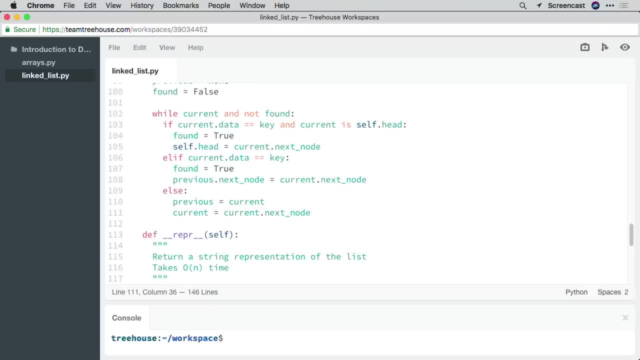 And that's it for the implementation Of remove. Now we're not doing anything at the moment With the node we're removing, But it's common for remove operations To return the value being removed. So at the bottom, Outside the while loop, 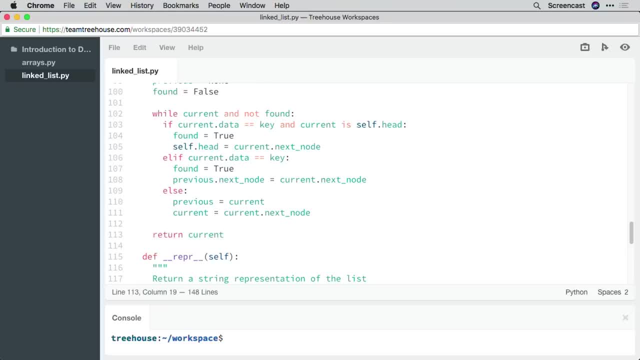 Let's return current And with that we have a minimal implementation Of a linked list And your first custom data structure. How cool is that? There's quite a bit we can do here To improve our data structure, Particularly in making it easy to use. 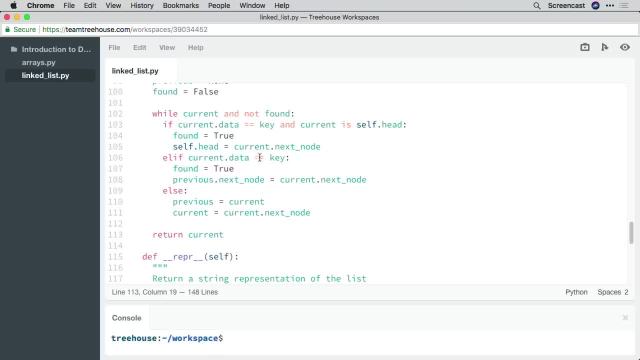 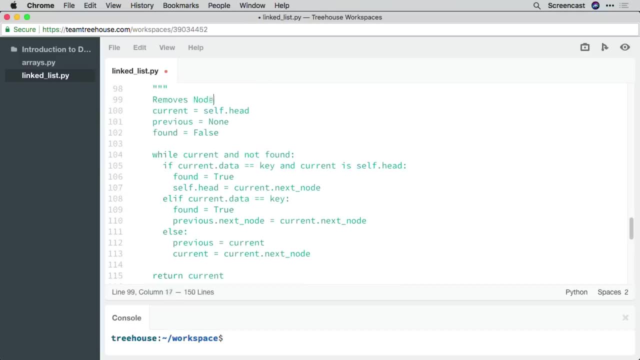 But this is a good place to stop. Before we move on to the next topic, Let's document our method. So the top another doc string, And here we'll say: removes node Containing data That matches the key. Also, It returns the node. 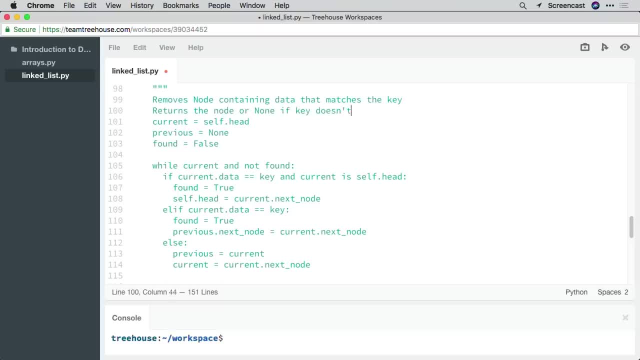 Or none If the key doesn't exist. And finally, It takes linear time Because, in the worst case scenario, We need to search the entire list. If you'd like to get in some additional practice Implementing functionality for linked lists, 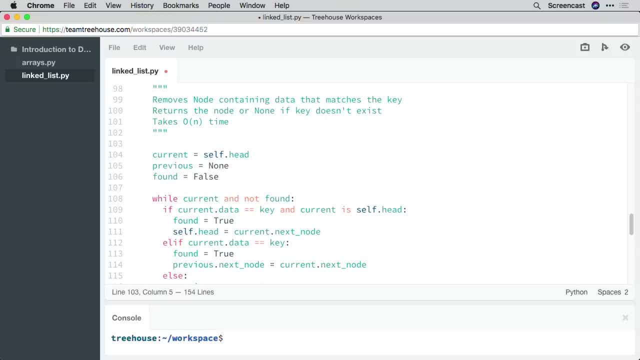 Two methods you can work on Are remove at index And node at index To allow you to easily delete Or read values in a list At a given index. Now that we have a linked list, Let's talk about where you can use them. 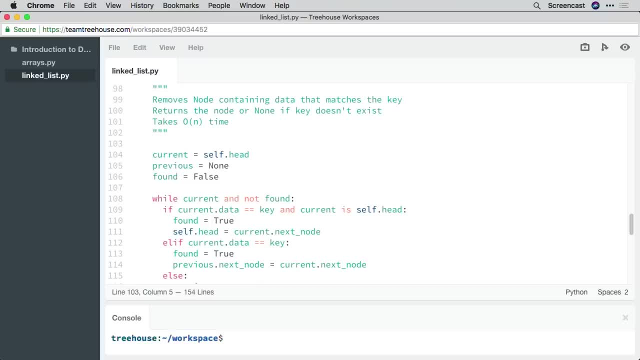 The honest answer is Not. a lot of places Are really useful structures to build For learning purposes Because they're relatively simple And are a good place to start to introduce The kinds of operations We need to implement for various data structures. 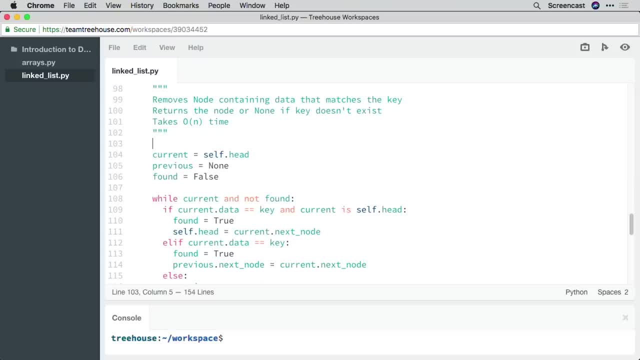 It is quite rare, however, That you will need to implement a linked list On your own. There are typically much better- And by that I mean much more efficient- data structures That you can use. In addition, many languages Like Java, for example. 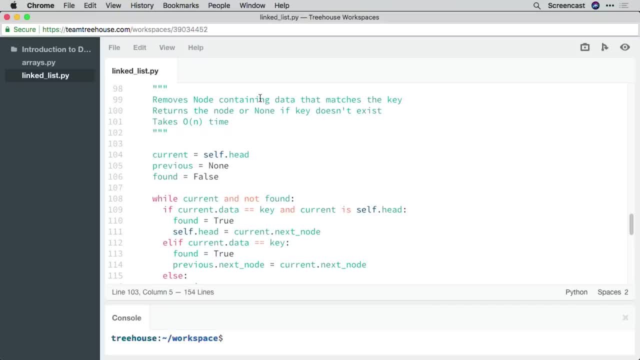 Provide an implementation of a linked list already. But if we have a custom data structure, Let's do something with it. Let's combine the knowledge we have And look at how a sorting algorithm Can be implemented Across two different data structures. 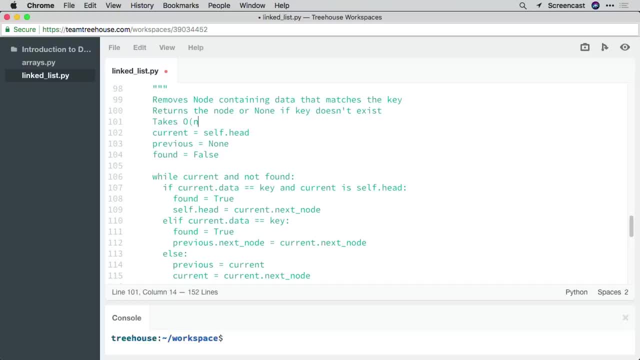 where k represents the slice size. this means that in reality, our implementation of split, this implementation of split- does not run in logarithmic time, but k times logarithmic time, because there's a slice operation for each split. this means that our implementation is much more expensive. so, overall, 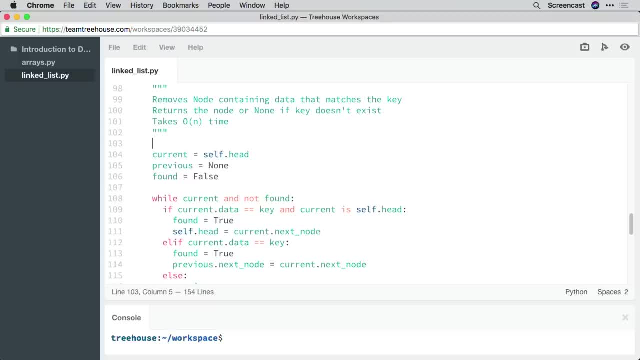 that makes our overall top level merge sort function not n times log n, but k n times log n, which is much more expensive. now let's get rid of all that. to fix this, we would need to remove this slicing operation. now we can do that by using a technique. 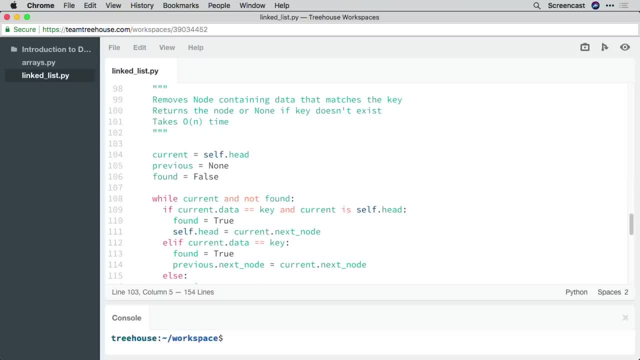 we learned in a previous course. in the introduction to algorithms course we looked at two versions of binary search in Python: a recursive and an iterative version. in the recursive one, we use list slicing with every recursion call, but we achieved the same end result using an iterative approach without using list slicing. 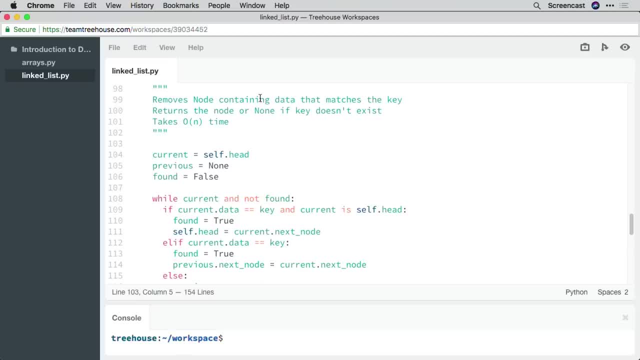 over there. we declared two variables to keep track of the starting and ending positions in the list. we could rewrite merge sort to do the same, but I'll leave that as an exercise for you. if you want some hints, if you want any action, I've included a link in the notes. 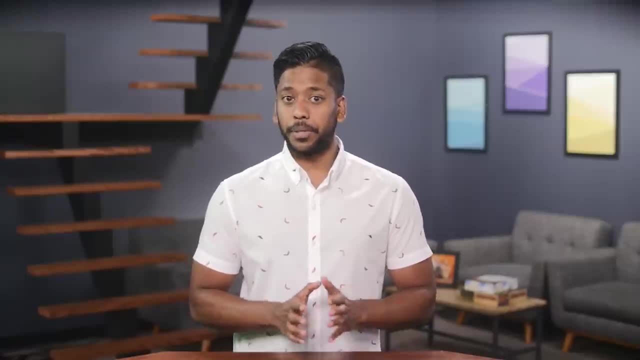 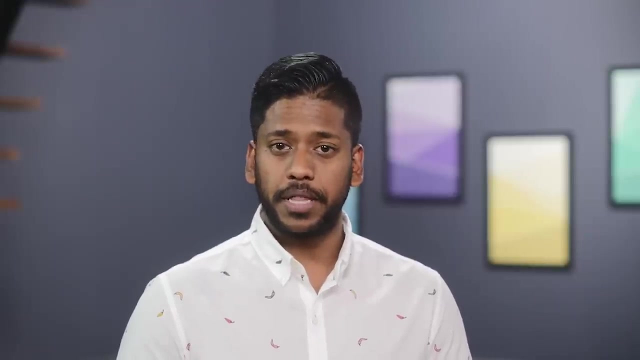 with an implementation. so that is time complexity. now, just so we know before moving on for Python here, our overall run time is not what I've listed here, but this is what the actual run time of the merge sort algorithm looks like. so the merge step runs in linear time. 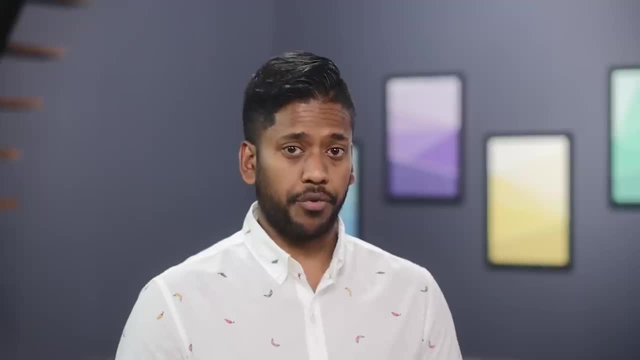 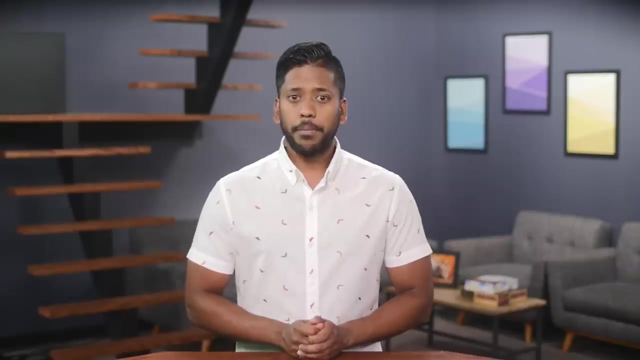 and the split step takes logarithmic time for an overall n times log n, and that is how merge sort actually works. okay, so what about space complexity? the merge sort algorithm takes linear space, and this is weird to think about at first, but, as always, a visualization helps. 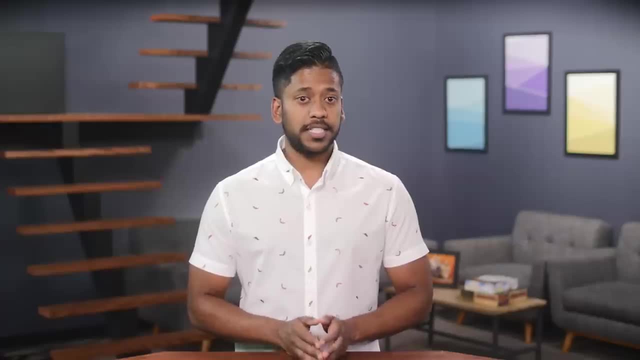 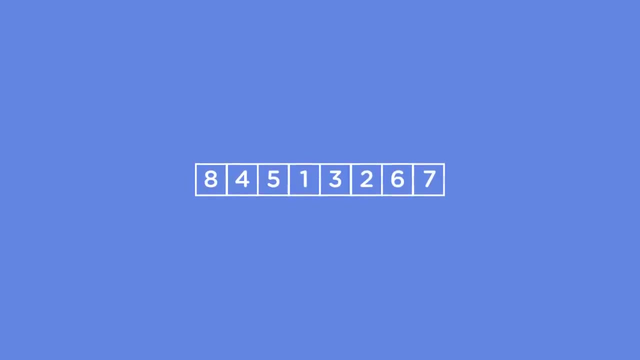 so if we start at the top again with our full list and carry out the split method until we have single element lists, each of these new lists take up a certain amount of space. so the second level. here we have two lists where each take up an n by. 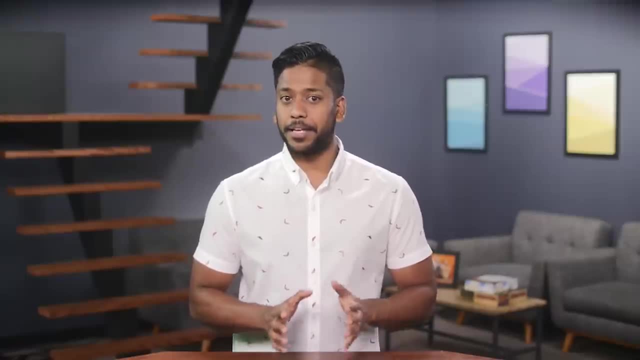 Now that we've seen two different data structures, Let's circle back And apply what we know about algorithms To these new concepts. One of the first algorithms you learned about Was binary search, And we learned that with binary search, The selection needs to be sorted. 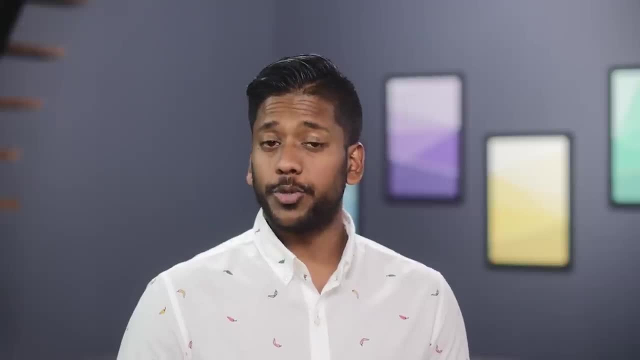 Over the next few videos, Let's implement the merge sort algorithm, Which is one of many sorting algorithms, On both arrays Or Python lists And the singly linked list we just created. This way, we can learn a new sorting algorithm That has real world use cases. 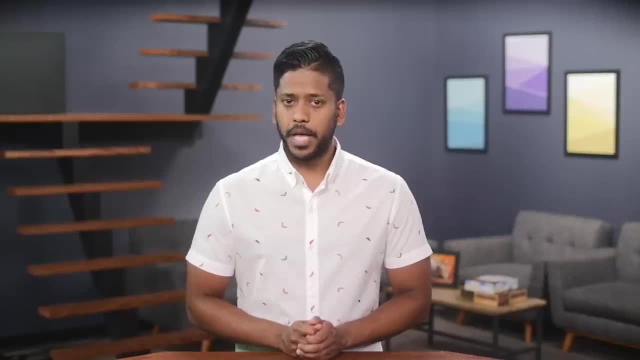 And see how a single algorithm Can be implemented on different data structures. Before we get into code, Let's take a look at how merge sort works conceptually, And we'll use an array to work through this. We start With an unsorted array of integers. 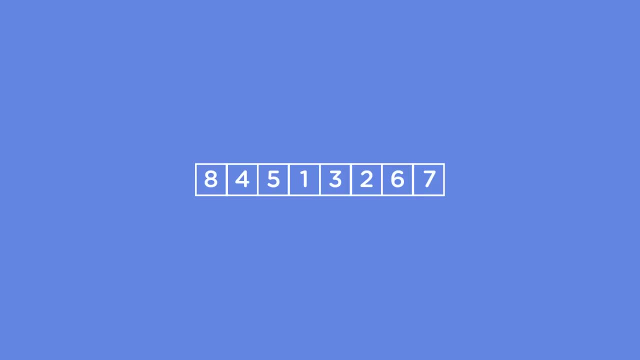 And our goal Is to end up with an array sorted in ascending order. Merge sort works Like binary sort By splitting up the problem into sub problems, But it takes the process one step further. On the first pass, We're going to split the array into two smaller arrays. 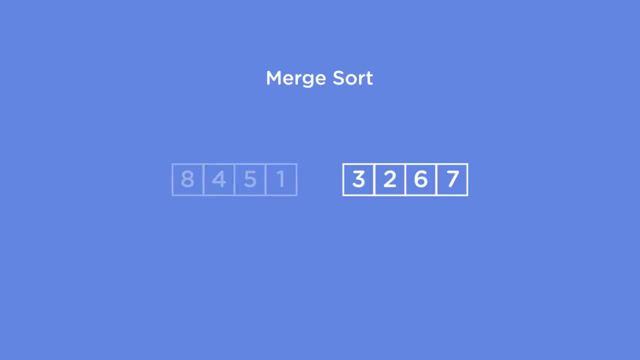 Now in binary search, One of these sub arrays would be discarded. But that's not what happens here. On the second pass, We're going to split each of those sub arrays Into smaller, evenly sized arrays, And we're going to keep doing this. 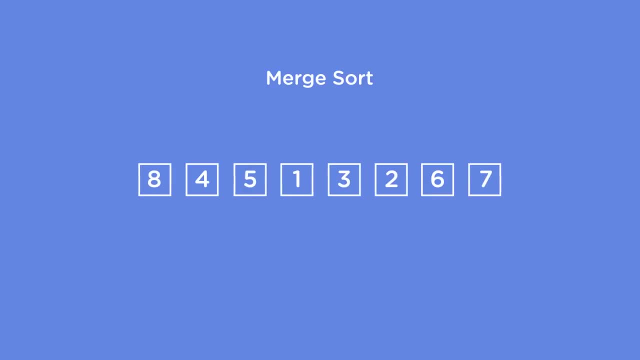 Until we're down to single element arrays. After that, The merge sort algorithm works backwards, Repeatedly, merging the single element arrays And sorting them At the same time, Since we start at the bottom By merging two single element arrays. 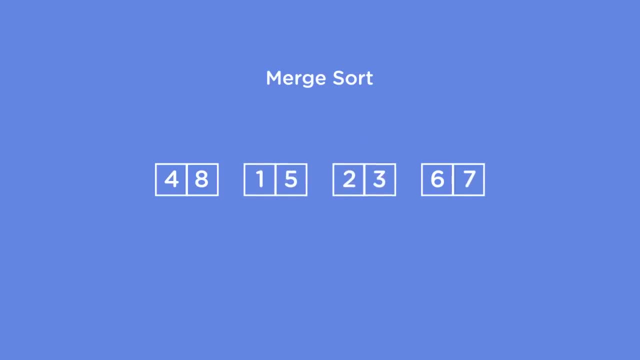 We only need to make a single comparison To sort the resulting merge array By starting with smaller arrays That are sorted As they grow. This allows us to execute Fewer sort operations Than if it sorted the entire array at once. 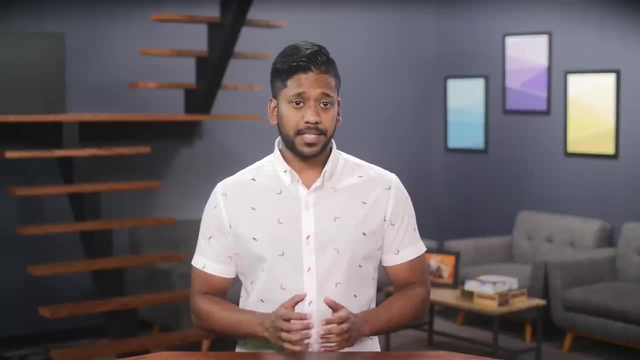 Solving a problem like this, By recursively breaking down the problem Into sub parts Until it is easily solved, Is an algorithmic strategy Known as divide and conquer. But instead of talking about all of this in the abstract, Let's dive into the code. 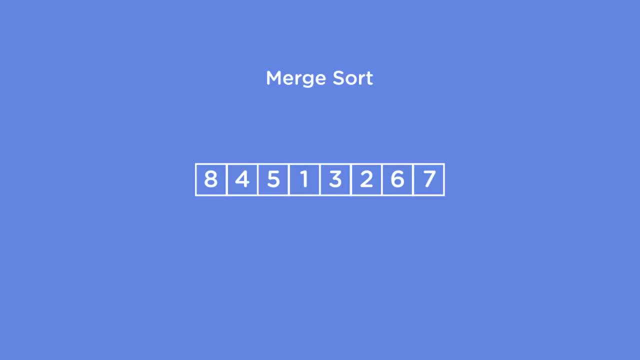 two amount of space. now, this makes it seem that the sum of all this space is the additional space needed for merge sort, but that's not actually the case in reality. there are two factors that make a difference. first, not every single one of these sublists are created. 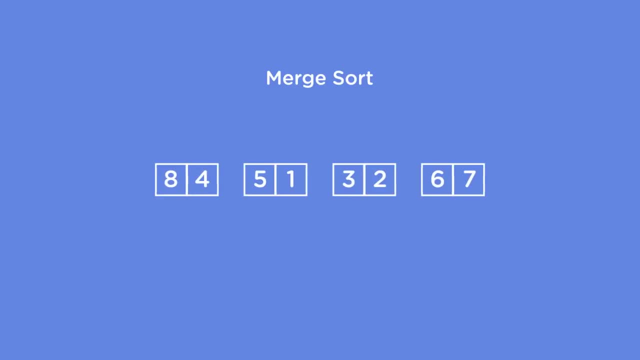 simultaneously. at step two, we create two n by two size sublists. when we move to the next step, however, we don't hold on to the n by two sublists and then create four n by four size sublists for the next split. instead, after the four, n by four. 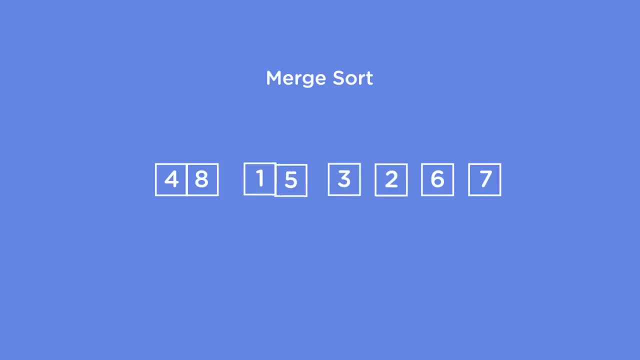 size sublists are created, the n by two ones are deleted from memory. there's no reason to hold on to them any longer now. the second point is that our code doesn't execute every path simultaneously. think of it this way: when we pass our list to the 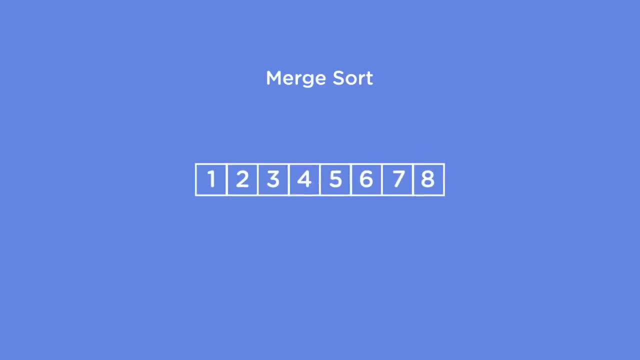 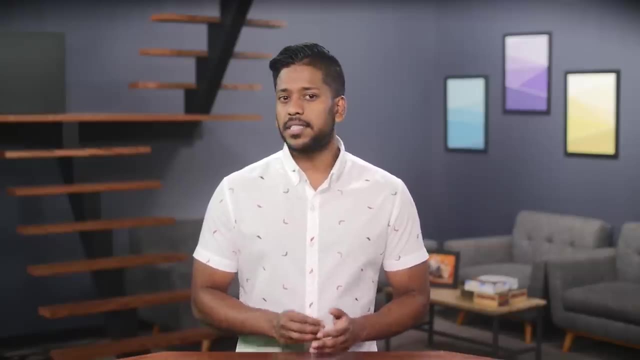 top level merge sort function. our implementation calls split, which returns a left half and a right half. the next line of code then calls merge sort on the left half again. this runs the function, the merge sort function, again with a new list. in that second run of the function, split is called again. 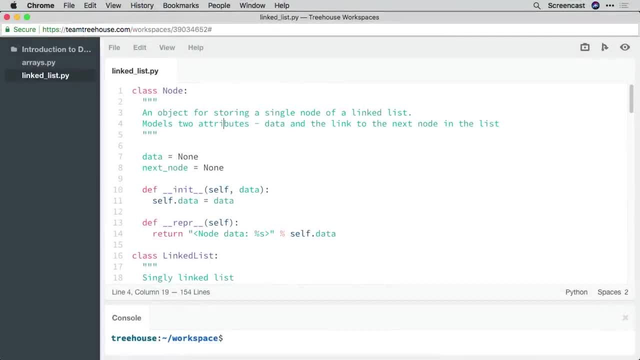 we get a second left and right half and then again, like before, we call merge sort on this left half as well. what this means is that the code walks down the left path all the way down until that initial left half is sorted and merged back into one. 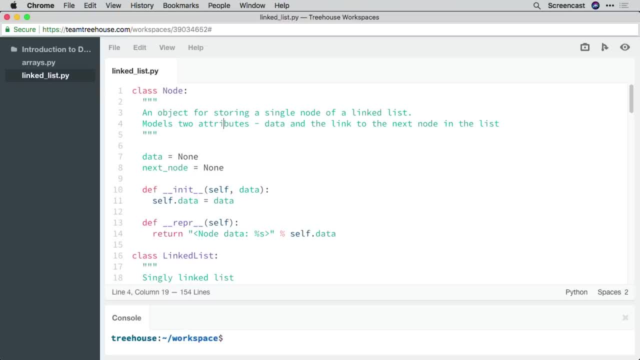 array, then it's going to walk all the way down the right path and sort that until we're back to that first split with two n by two sized sublists. essentially we don't run all of these paths of code at once, so the algorithm doesn't need additional. 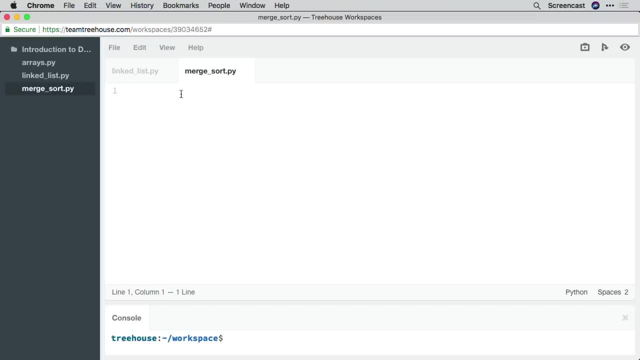 space for every sublist. in fact, it is the very last step that matters. in the last step, the two sublists are merged back into the new sorted list and returned. that sorted list has an equal number of items as the original unsorted list and since this is a new list, 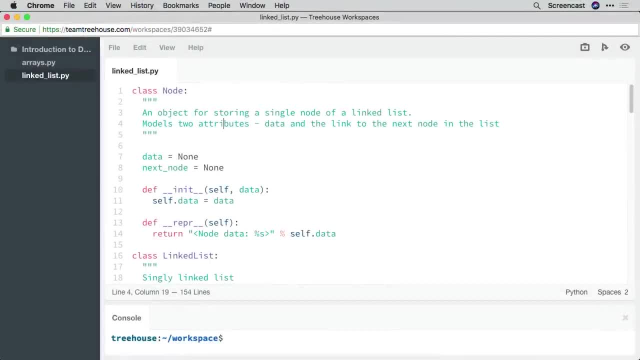 This way we can analyze the runtime As we implement it. For our first implementation of merge sort, We're going to use an array. While the implementation Won't be different conceptually, For a linked list We will have to write more code. 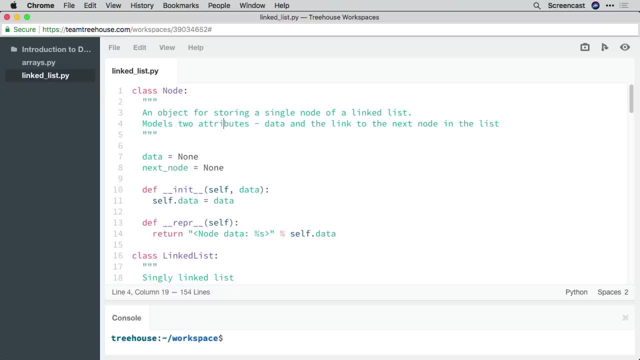 Because of list traversal And how nodes are arranged. So once we have these concepts squared away, We'll come back to that. Let's add a new file here. We'll call this: Merge underscore sort dot pipe In our file. Let's create a new function. 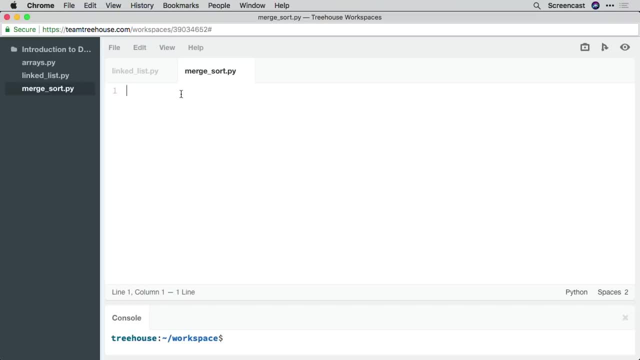 Named merge sort List unless I specify linked list I mean a python list Which is the equivalent of an array. So we'll say def Merge underscore sort. That takes a list. In the introduction to algorithms course We started our study. 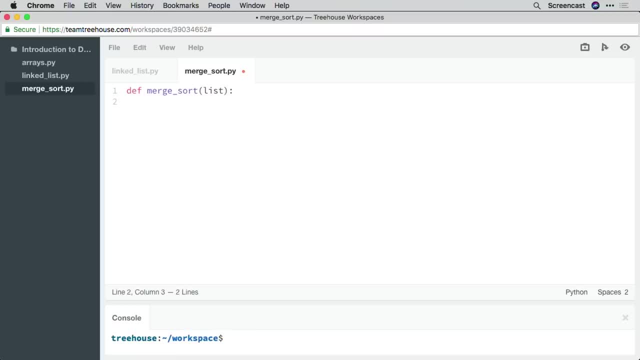 Of each algorithm By defining the specific steps That comprise the algorithm. Let's write that out as a doc string In here- the steps of the algorithm, So that we can refer to it Right in our code. This algorithm is going to sort the given list. 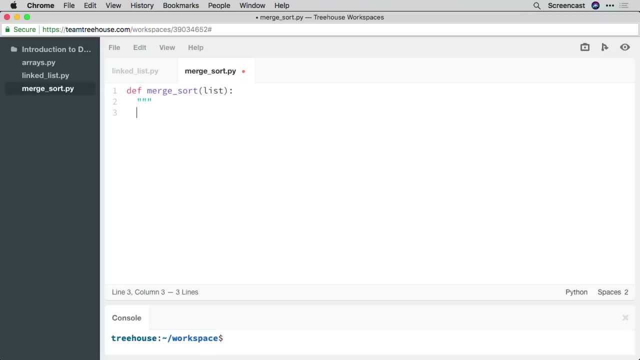 In an ascending order. So we'll start by putting that in here As a simple definition Sorts a list In ascending order. There are many variations Of merge sort And in the one we're going to implement We'll create and return a new sorted list. 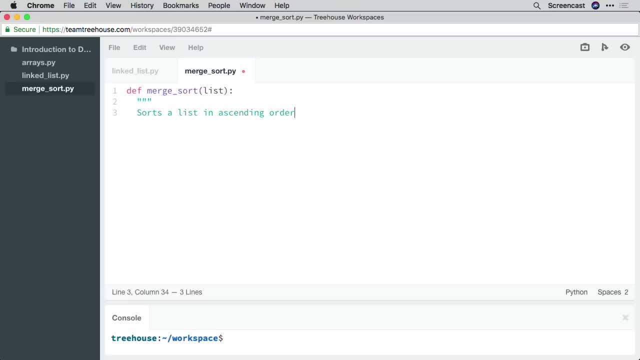 Other implementations Will sort the list we pass in, And this is less typical In an operation known as sort in place, But I think that Sorting a new list Makes it easier to understand the code. Now, these choices do have implications, though. 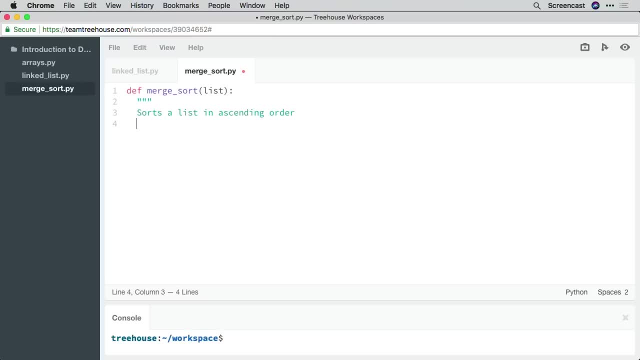 And we'll talk about them As we write this code For our next bit of the doc string, Let's write down the output of this algorithm. So returns A new sorted list. Merge sort has three main steps. The first Is the divide step. 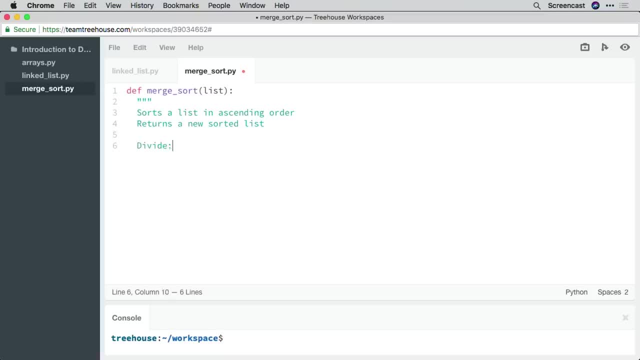 Where we find the midpoint of the list. So we'll say divide, Find the midpoint Of the list And divide Into Sublists. The second step is the conquer step, Where we sort the sublists That we created in the divide step. 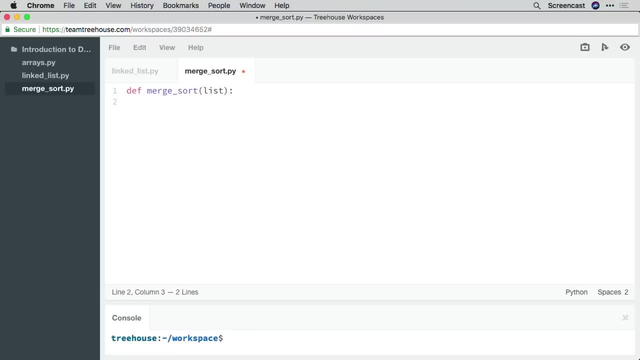 it means that at most the additional space the algorithm will require at a given time is n. yes, at different points in the algorithm we require log n amount of space. but log n is smaller than n, and so we consider the space complexity of merge sort to be linear. 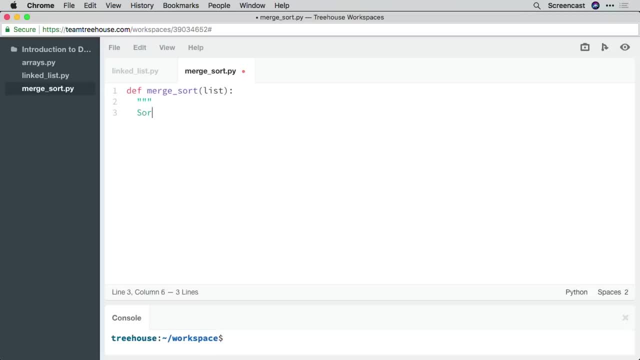 because that is the overall factor. okay, that was a lot, so let's stop here. don't worry if you've got questions about merge sort, because we're not done yet. over the next few videos, let's wrap up this course by implementing merge sort on a linked 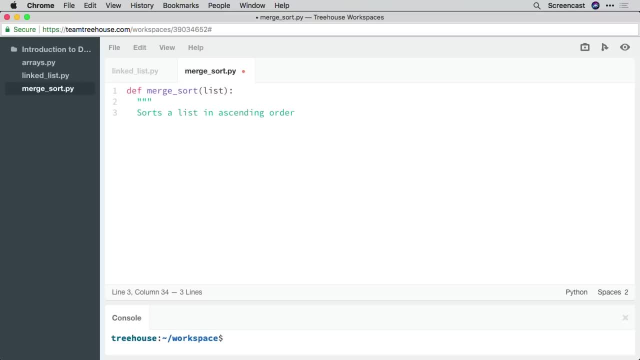 list. over the last few videos we implemented the merge sort algorithm on the array or list type in python. merge sort is probably the most complicated algorithm we've written so far, but in doing so we learned about an important concept: divide and conquer. we also concluded the last video by figuring out the run. 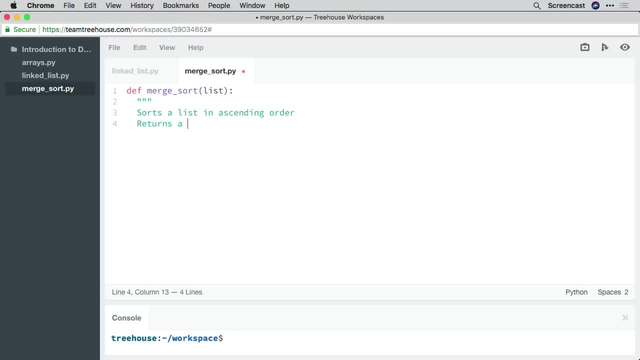 time of merge sort, based on our implementation. over the next few videos, we're going to implement merge sort again, this time on the linked list type. in doing so, we're going to get a chance to see how the implementation differs based on the data structure, while still keeping the fundamentals. 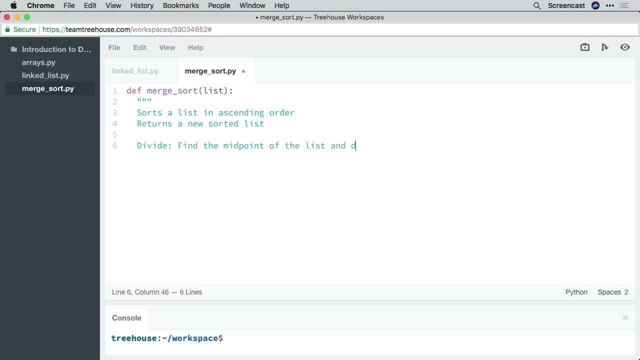 of the algorithm the same, and we'll also see how the run time may be affected by the kinds of operations we need to implement. let's create a new file to put our second implementation of merge sort in. so file over here, new file, and it's going to have a rather long name. we'll call 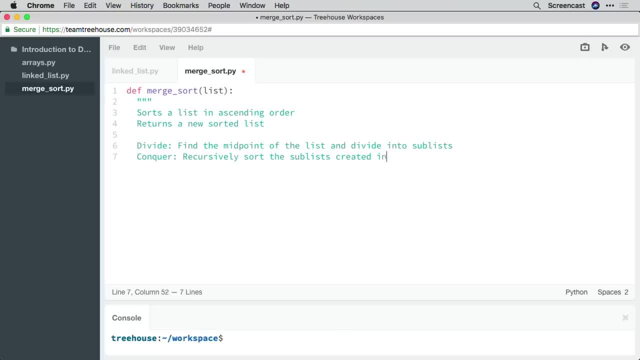 this linked list merge sort with underscores everywhere, py. we're going to need the linked list class that we created earlier, so we'll start at the top by importing the linked list class from the linked listpy file. the way we do that is, we'll say from: 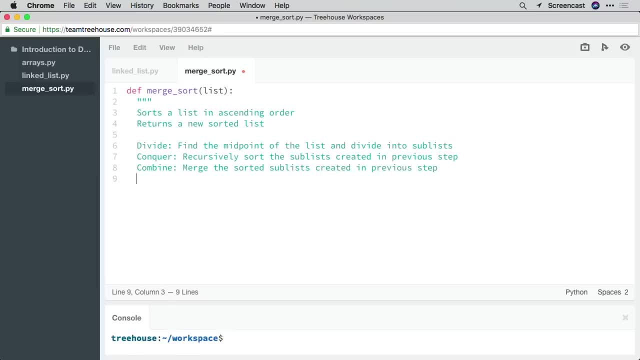 linked list: import linked list. right, so that imports the class. let's test if this works really quick. we'll just do something like l: equal linked list, l dot add ten or one, doesn't matter, print l okay, and if i hit save and then down here we'll say: 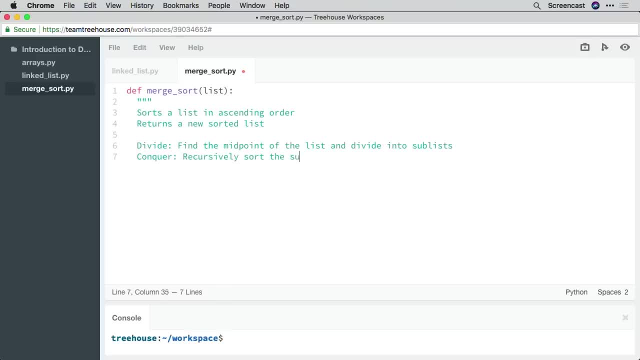 So we'll say recursively Sort the sublists Created in Previous step And finally the combine, The combine step Where we merge these recursively sorted sublists Back into a single list, So merge The sorted sublists Created in. 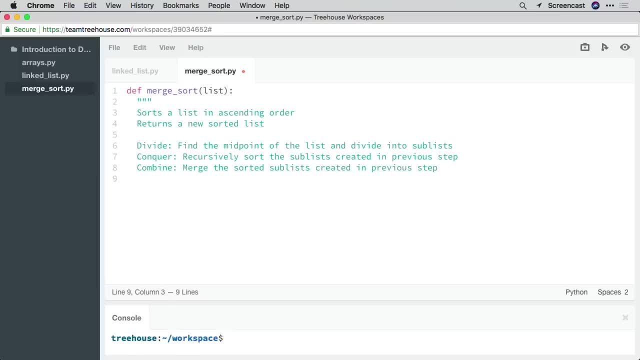 Previous step. When we learned about algorithms, We learned that a recursive function Has a basic pattern. First we start with a base case That includes a stopping condition. After that we have some logic That breaks down the problem And recursively calls itself. 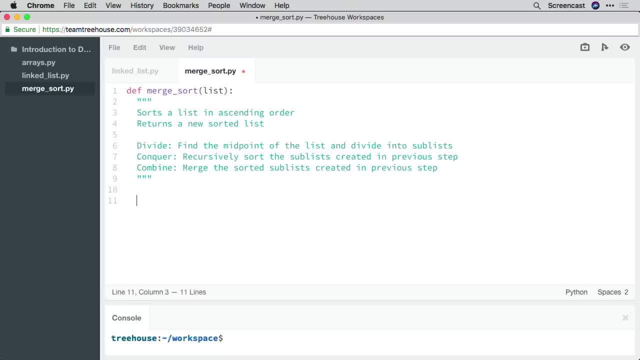 Our stopping condition Is our end goal, A sorted array To come up with a stopping condition Or a base case. We need to come up with the simplest condition That satisfies this end result. So there are two possible values That fit. 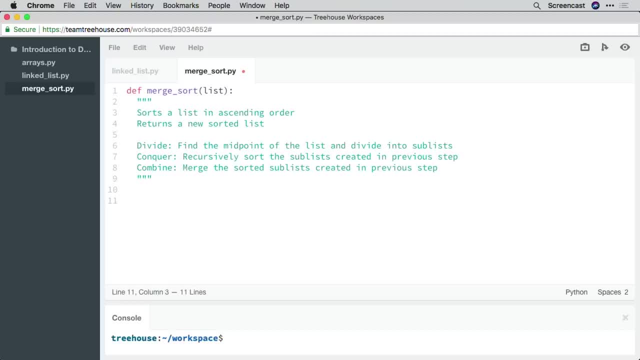 A single element list Or an empty list. Now, in both of these situations We don't have any work to do. If we give the merge sort function an empty list Or a list with one element, It's technically already sorted. We call this naively sorting. 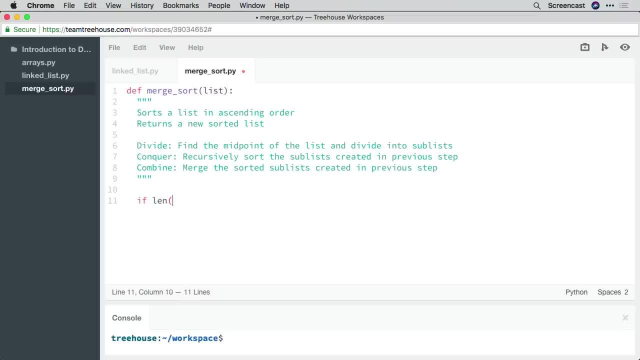 Let's add that as our stopping condition. We'll say: if len list, If the length of the list Is less than or equal to one, Then we can return the list. Okay, so this is our Stopping condition. And now that we have a stopping condition, 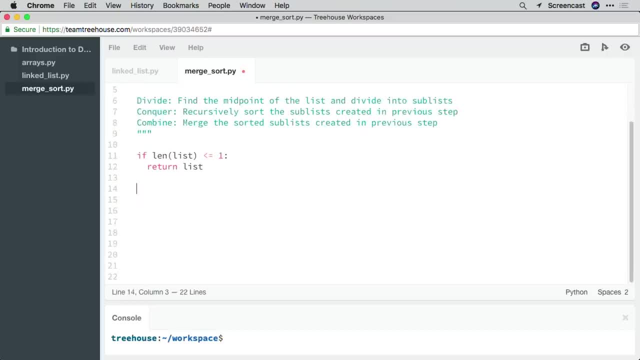 We can proceed with the list of steps. First, we need to divide the list Into sub lists To make our functions easier to understand. We're going to put our logic In a couple different functions. One large one, So I'll say it left half. 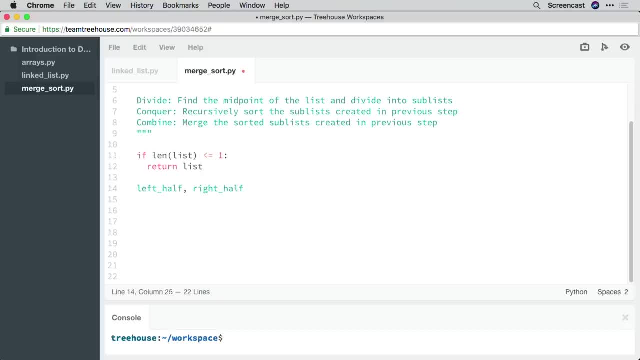 Comma right, half Equal Split List. So here we're calling a split function That splits the list we pass in And returns two lists, split at the midpoint. Because we're returning two lists, We can capture them in two variables. 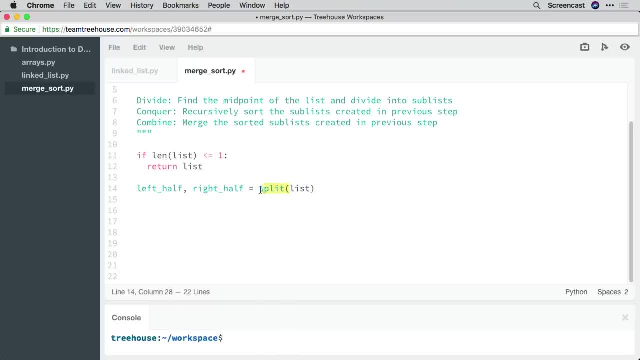 Now You should know that this split function Is not something that comes built into python. This is a global function. Right Next is the conquer step, Where we sort each sub list And return a new sorted sub list. So we'll say: left equal. 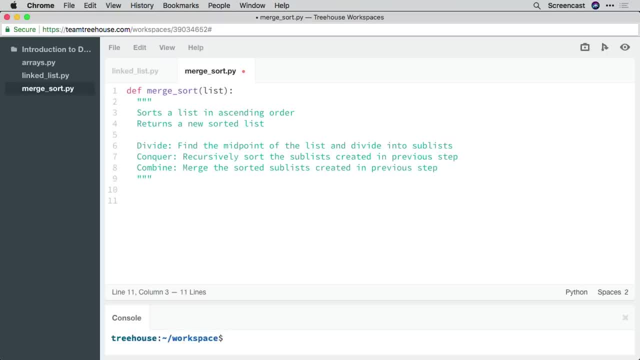 python linked list: merge sort dot py. okay, it works. so this is how we get some of the code, how we reuse the code that we've written in other files into this current file. we can get rid of this now, okay, like we did with the first implementation of merge sort. 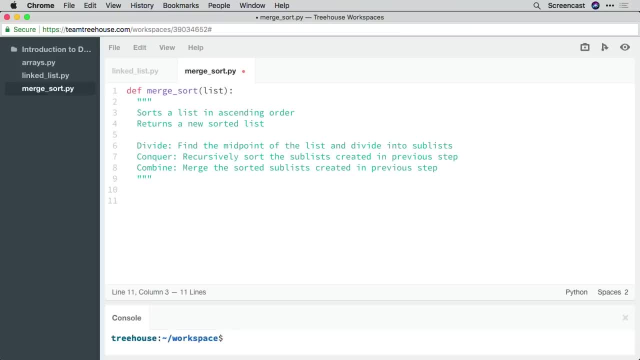 we're going to split the code up across three functions: the main function, merge sort, a split function and a merge function. now, if you were to look up a merge sort implementation in python, both for a regular list and array or a linked list, you would find much more. 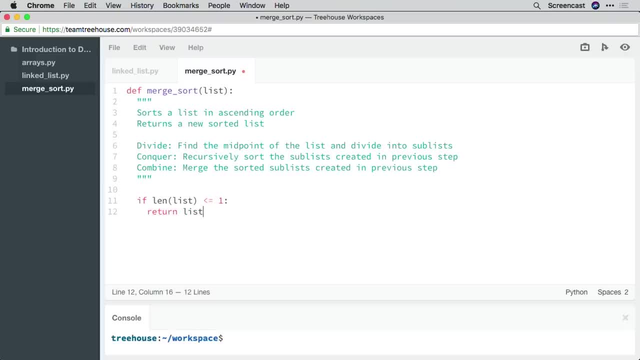 concise versions out there, but they're kind of hard to explain. so splitting it up into three will sort of help it, you know, be easier to understand. we'll call this merge sort at the top level, and this time it's going to take a linked list. let's add a doc. 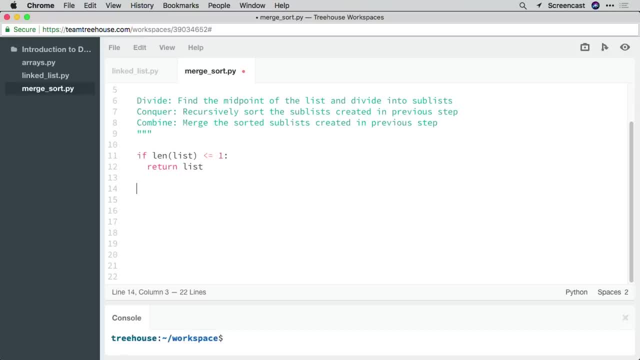 string to document the function. so we'll say that this function sorts a linked list in ascending order and, like before, we'll add the steps in here. so we'll say you first recursively divide the linked list into sub lists containing a single node, then we repeatedly merge the sub lists. 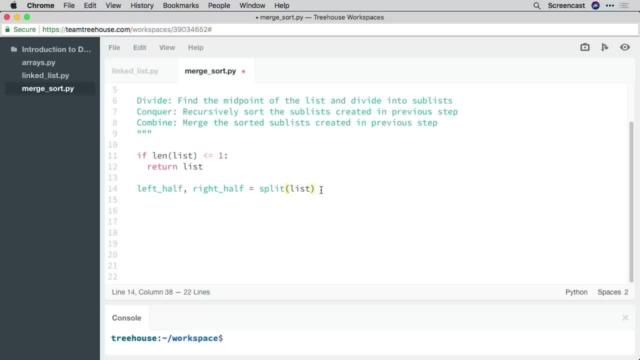 to produce sorted sub lists until one remains, and then finally, this function returns a sorted linked list. the implementation of this top level merge function is nearly identical to the array or list version we wrote earlier. so first we'll provide a stopping condition or two, if the size of the list is one or it's. 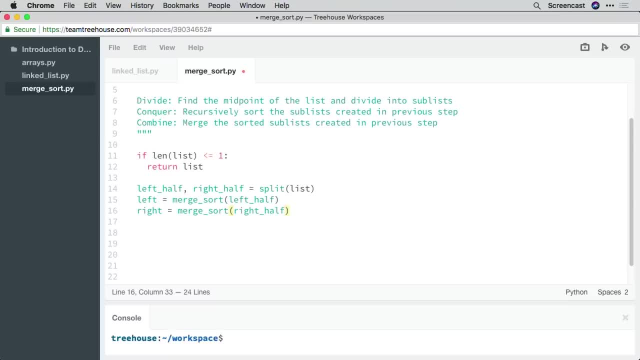 an empty list, we'll return the linked list, since it's naively sorted. so if linked list dot size- remember that function we wrote equal one- then we'll return linked list. else, if linked list dot head is none, meaning it's an empty list, then we'll return linked 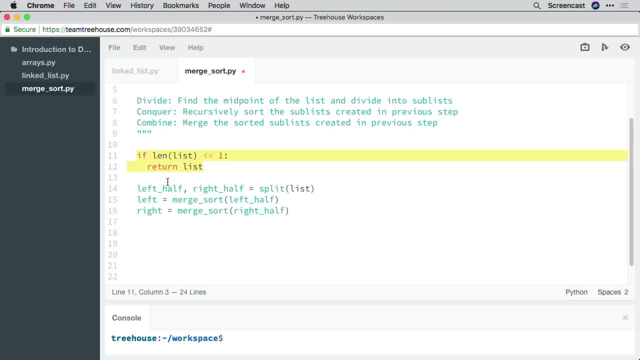 list as well. okay, next let's split the linked list into a left and right half. conceptually this is no different, but in practice we need to actually traverse the list. we'll implement a helper method to make this easier, but we'll say: left half, comma, right half. 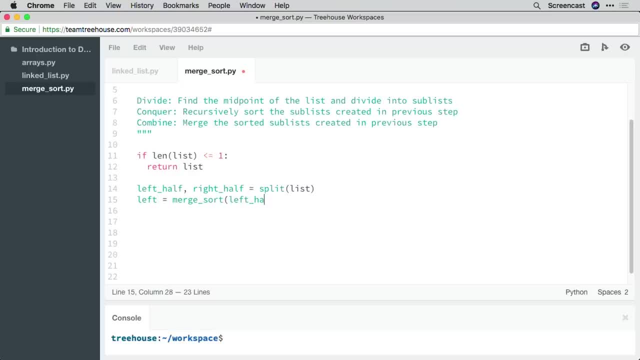 Merge sort Left half And Right equal. Merge sort Right half. This is the recursive Portion of our function. So here we're calling merge sort Sub list. So we divide the list into two here And then we call merge sort on it again. 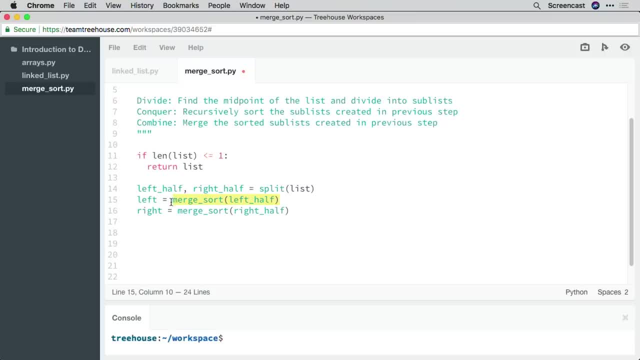 This further splits that sub list Into two. In the next pass through of merge sort, This is going to be called again, And again, And again, Until we reach our stopping condition Where we have single element lists Or empty lists. 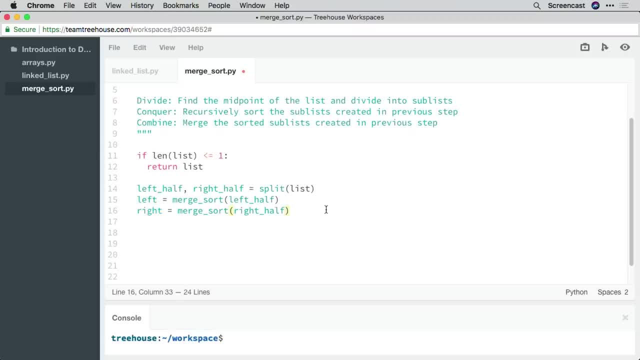 When we've subdivided Until we cannot divide anymore, We can start merging backwards. So we'll say: return, Merge Left and right. That brings us to the combine step. Once two sub lists are sorted And combined, We can return it. 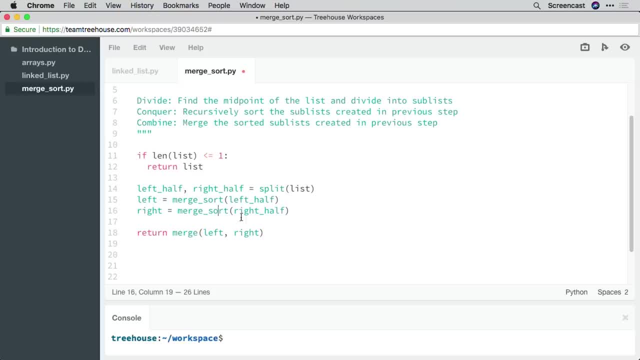 Now, obviously none of these functions- Merge, merge, sort. well, merge, sort is written, But merge and split haven't been written. So all we're going to do here, if we run it, Is raise an error. So in the next video. 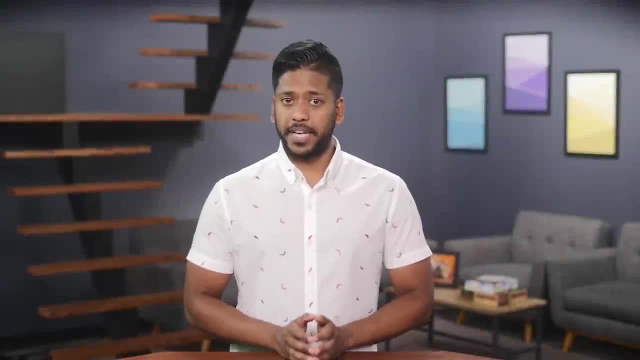 Let's implement the split operation. The first bit of logic we're going to write Is the divide step of the algorithm. This step is fairly straight forward And only requires a few lines of code, But is essential to get the sorting process going. 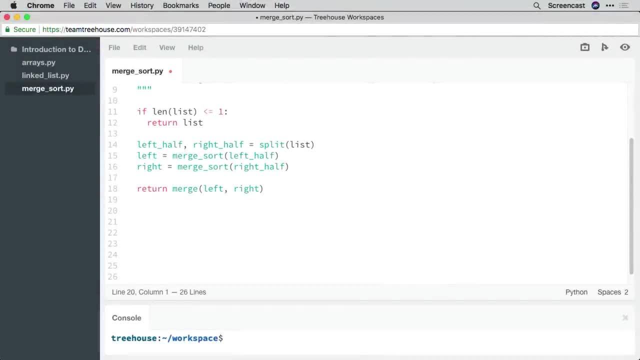 Alright. so, as we saw earlier, We're going to call the function for the divide step Split. So we'll say def, split And split is going to take as an argument A list to split up. Let's document how this function works. 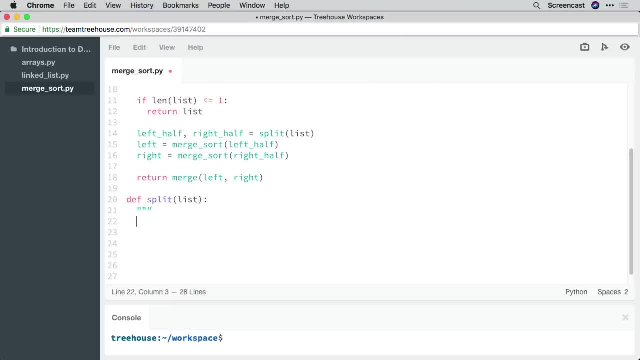 So we'll say: Divide The unsorted List at midpoint Into sub lists. And it's always good to say What we're returning as well. So we'll say: returns To sub lists Left and right. Alright, so the first step. 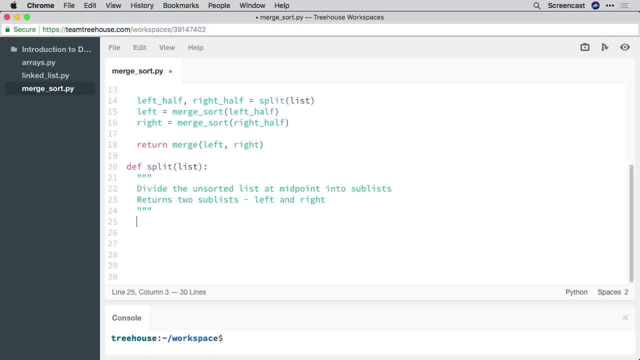 Is to determine the midpoint Of this list, Of this array. We're going to use the floor division operator, for this Floor division carries out a division operation And if we get a non integer value Like 2.5. It just gets rounded down to 2.. 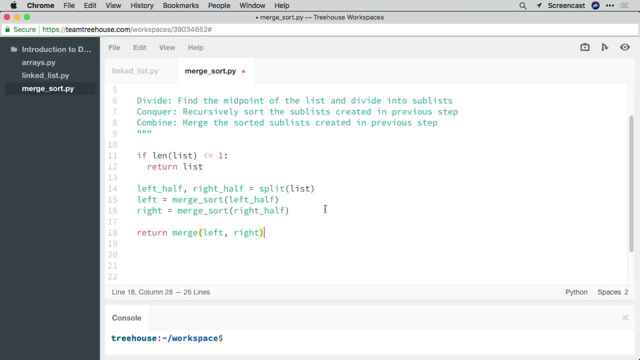 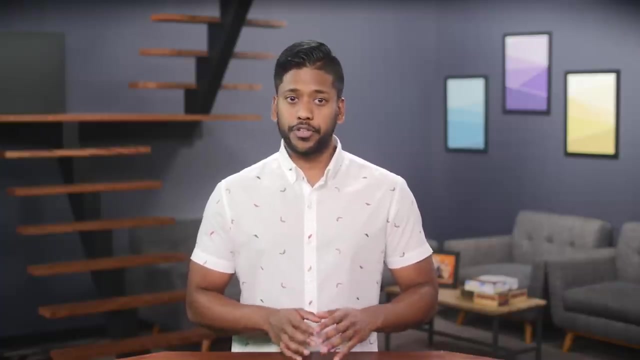 equal split linked list. and once we have two sub lists, like before, we can call merge sort the top level function on each. so left equal merge- sort- left half and right equal merge- sort on the right half. finally, we'll merge these two top level sub lists and return it, so merge. 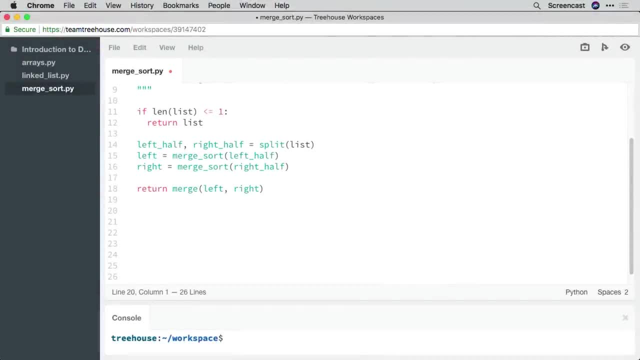 left and right. okay, nothing new here, but in the next video let's implement the split logic. the next step in the merge sort algorithm is the divide step, or rather an implementation of the split function. so down here we'll call this split like before, and this is going to take a linked. 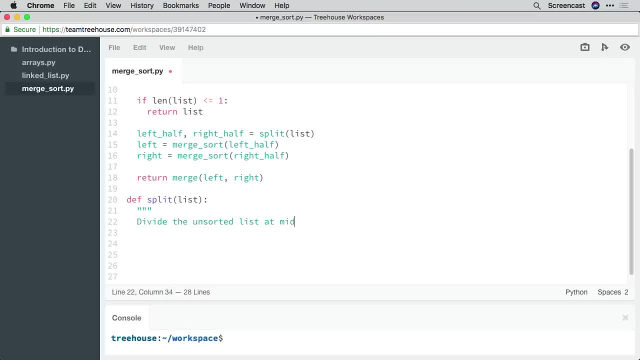 list. documenting things is good, and we've been doing it so far, so let's add a doc string, divide the unsorted list at midpoint into sub lists. now, of course, when I say sub lists here I mean sub linked lists, but that's a long word to say. 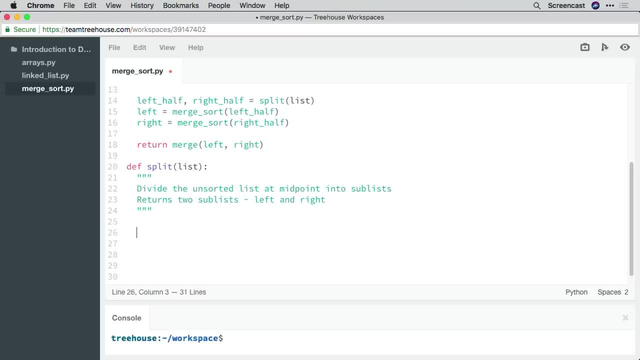 now here's where things start to deviate from the previous version. with the list type, we could rely on the fact that finding the midpoint using an index and list slicing to split into two lists would work even if an empty list was passed in, since we have no automatic behavior like that. 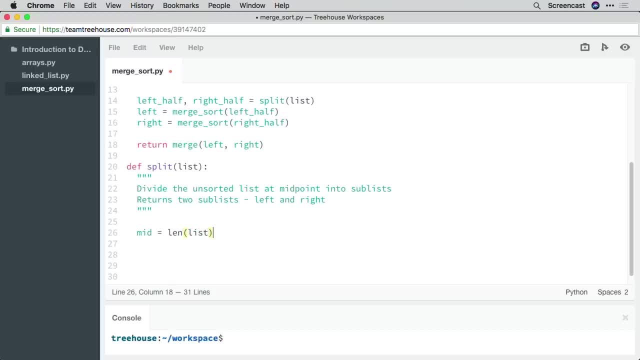 we need to account for this when using a linked list. so our first condition is: if the linked list is none or if it's empty, that is, if head is equal to none, so we'll say: if linked list equal none or you can write: is there, doesn't matter. 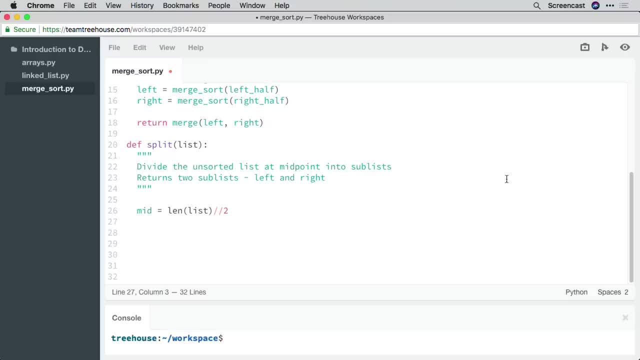 or linked list. dot head is none. well, linked list can be none. for example, if we call split on a linked list containing a single node, a split on such a list would mean left would contain the single node, while right would be none. now, in either case, we're going to assign the entire list. 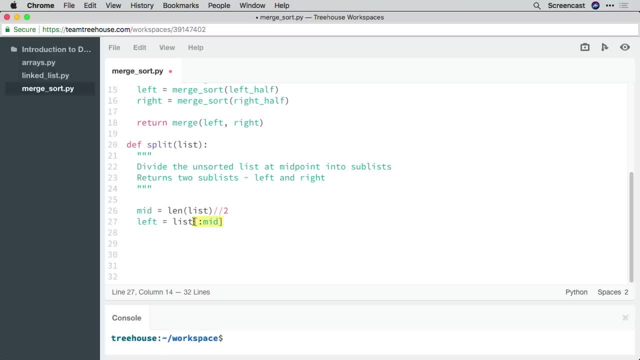 to the left half and assign none to the right. so we'll say left half equal linked list and then right half equal none. you could also assign the single element list or none to left and then create a new empty linked list assigned to the right half. but that's unnecessary. 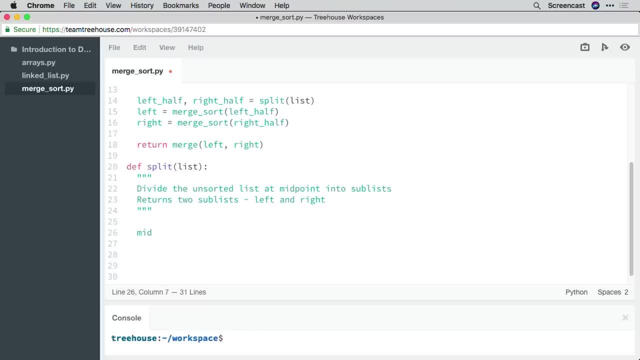 We'll define the midpoint To be the length of the list Divided by 2.. And then rounded down So: len list And using the two forward slashes For the floor division operator, We'll put number 2 after it. 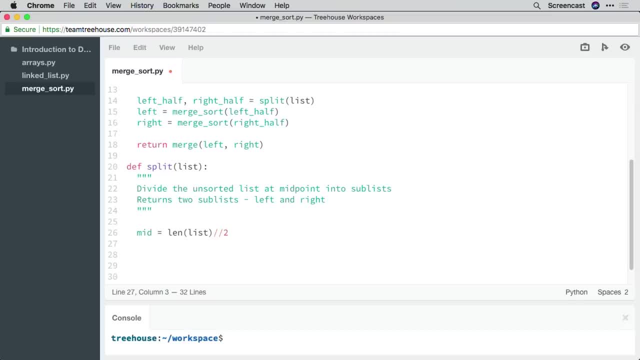 Okay, Once we have the midpoint, We can use the slicing notation In Python To extract portions of the list we want to return, For instance, Left As the left sub list. That goes all the way from the start of the list. 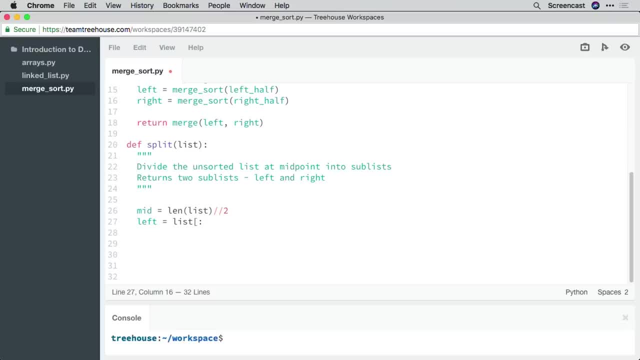 All the way up to the midpoint, Without including the midpoint. Now, over here We're using the slicing syntax Where it's like using the You know subscript notation To access a value from a list, But instead we give two index values. 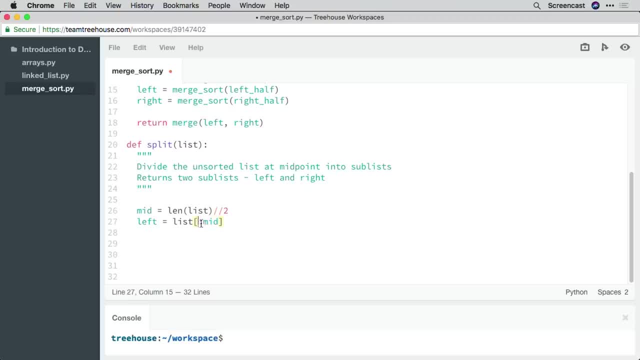 As a start and stop. If we don't include a start value, As I've done here, Python interprets that As the zeroth index Or the start of the list Now. similarly, We can define right To be values on the right of the midpoint. 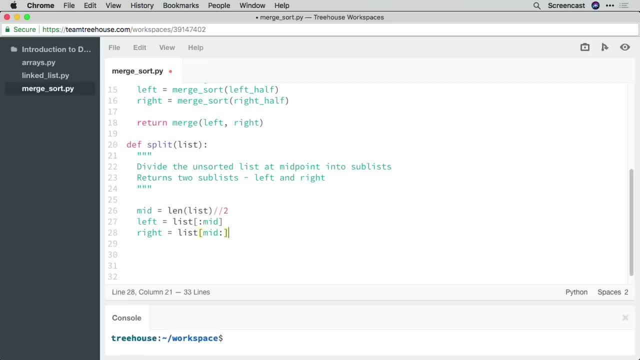 So starting at the midpoint And going all the way up to the end of the list. So Couple things to note. As I said earlier, When you don't include the starting index, It interprets it as to start at the very beginning of the list. 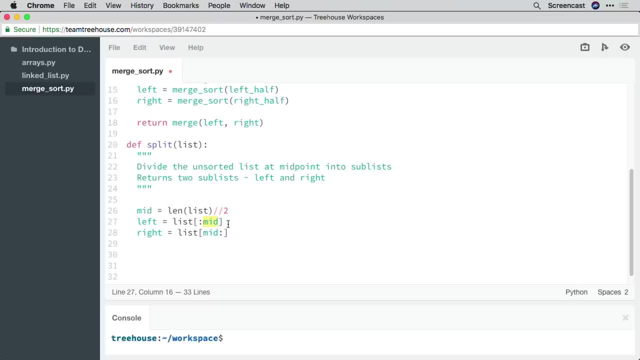 The index you give as the stopping condition. That value is not included In the slice Over here. We're starting at the very beginning of list And we go all the way up to midpoint, But not including midpoint, And then right starts at midpoint. 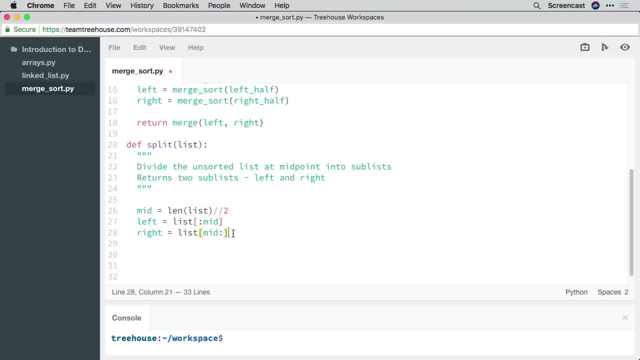 So it includes that value And then goes all the way to the end of the list. Now, once we have these two sub lists, We can return them. So we return left and right. Notice that we're returning two values here And then in the merge sort function. 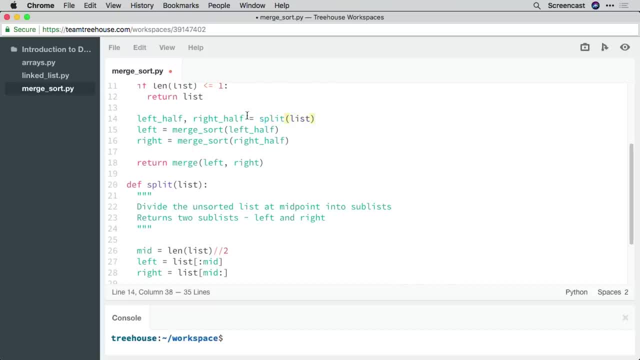 When we call that split function, We're declaring two variables, Left half and left half, And then right half To assign, So that we can assign these two sub lists to them. Okay, And that's all there is to the split function. 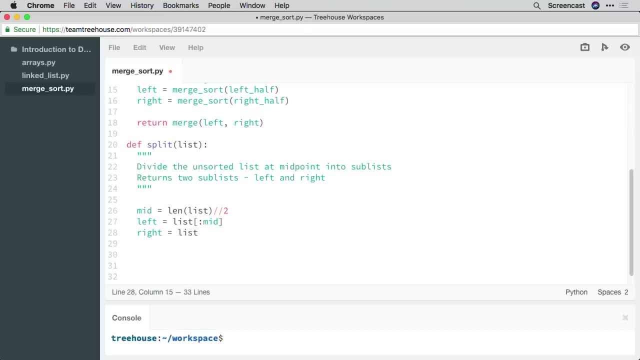 work. so now that we've done this, we can return left half and right half. so that's our first condition. let's add an else clause to account for non empty linked lists. first we'll calculate the size of the list. now this is easy because we've done. 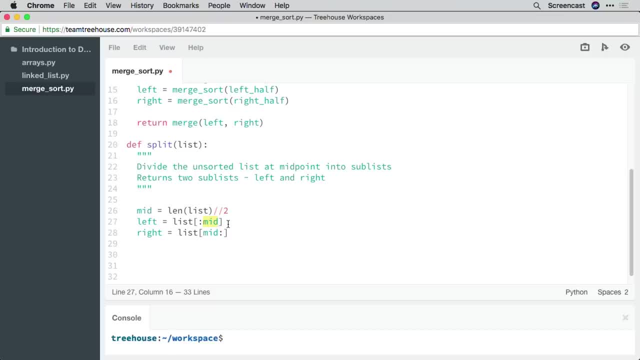 the work already and we can just call the size method that we've defined. we'll say: size equal linked underscore list: dot size. using the size we can determine the midpoint. so mid equals size, and here we'll use that floor division operator to divide it by two. once we have 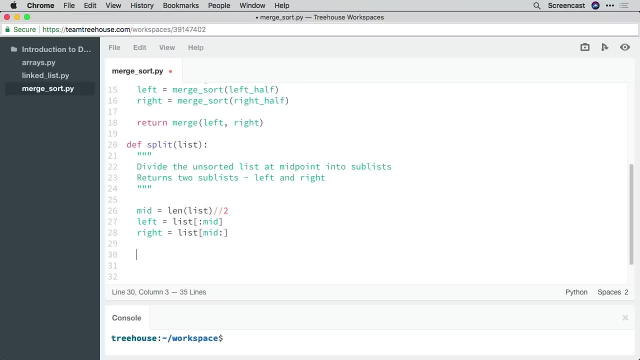 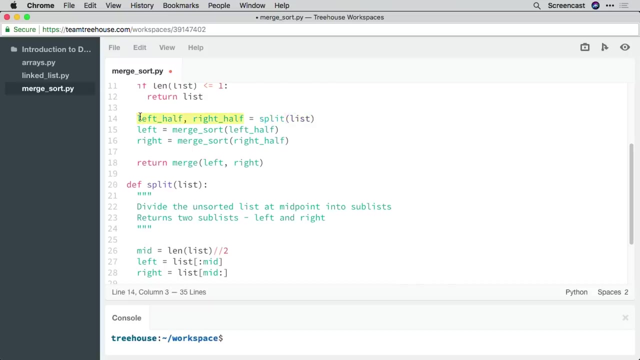 the midpoint. we need to get the node at that midpoint now. make sure you hit command s to save here and we're going to navigate back to linked list dot pi. in here we're going to add a convenience method at the very bottom right before the repper function. right, 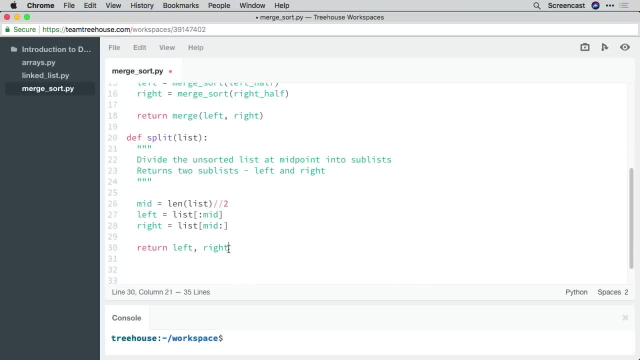 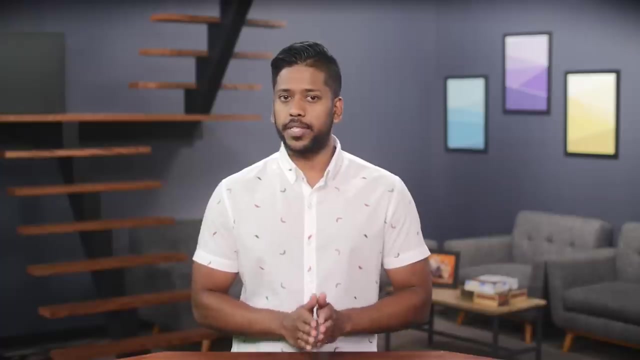 here, and this convenience method is going to return a node at a given index, so we'll call this node at index and it's going to take an index value. this way, instead of having to traverse the list inside of our split function, we can simply call node at index. 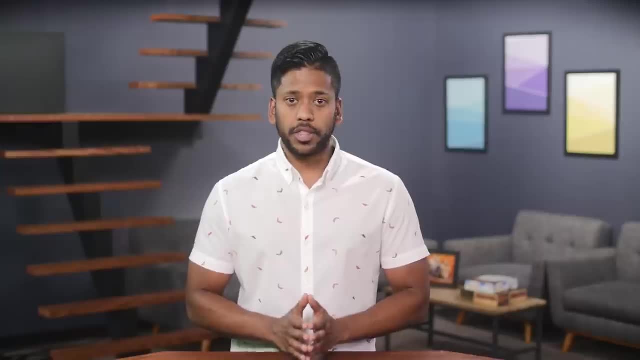 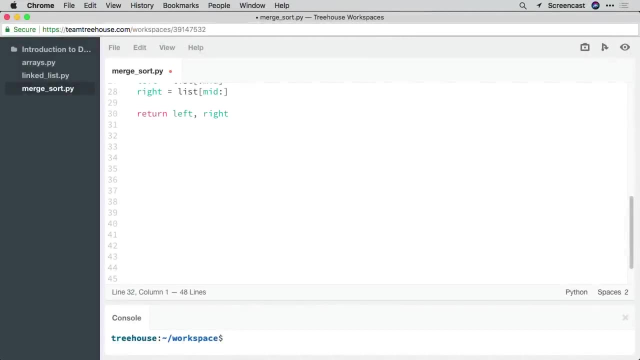 and pass it the midpoint index we calculated to give us the node right there so we can perform the split. okay, so this method accepts as an argument the index we want to get the node for. if this index is zero, then we'll return the head of the list. so if 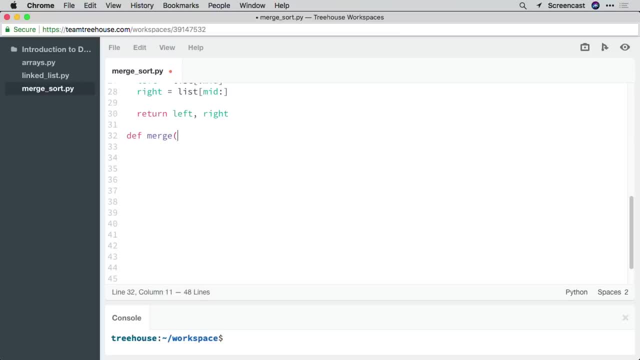 index double equals zero return self dot head. the rest of the implementation involves traversing the linked list and counting up to the index as we visit each node. the rest of the implementation involves traversing the linked list and counting up to the index as we visit each node. 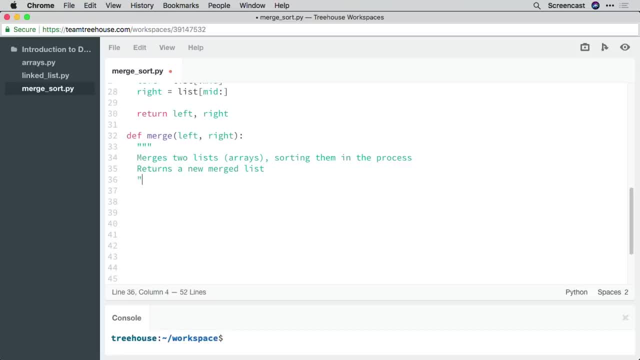 so I'll add an else clause here and we'll start at the head. so we'll say current equal self dot head. let's also declare a variable called position to indicate where we are in the list. we can use a while loop to walk down the list. 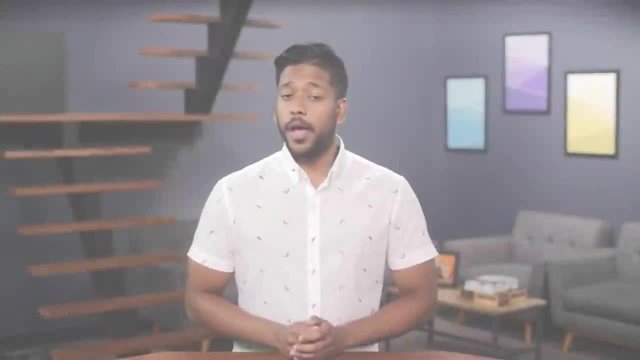 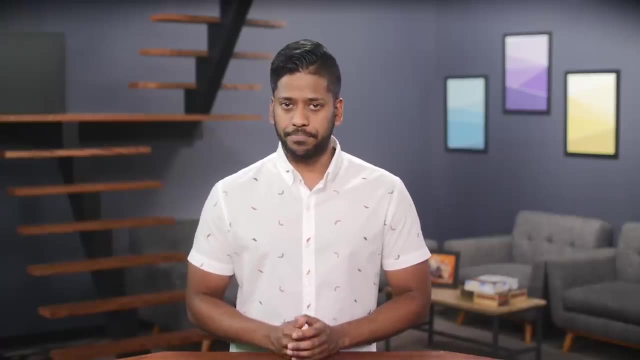 In the next video Let's implement the crucial portion of the merge sort logic. Once we run the split function recursively Over the array, We should end up with several single member or empty arrays. At this point We need to merge them all back. 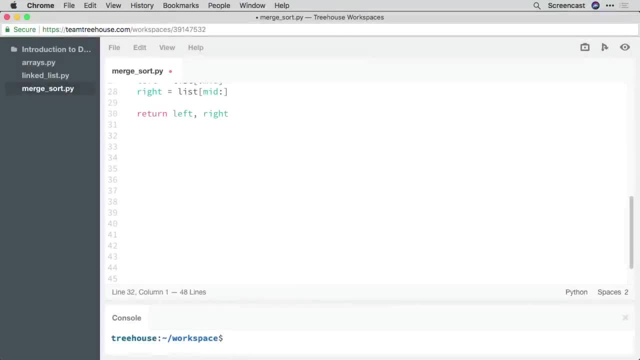 And sort them in the process, Which is what our merge function is for. So our merge function is going to take two arrays Or lists As arguments And to match the naming conventions we used in the split function. We'll call this left and right as well. 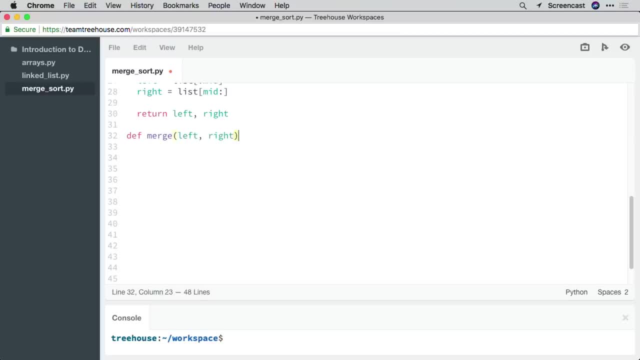 So we'll say: def. merge Takes a left and a right list And, like before, Let's add some documentation to our function. So this function Merges two lists Or arrays, Sorting them In the process, And then it returns a new. 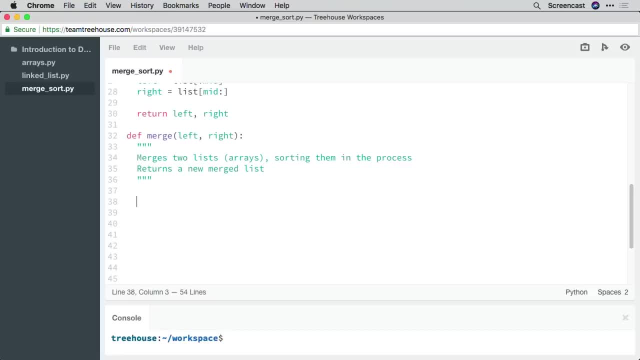 Merged list. Since our function Is going to return a new list, Let's start by creating one. Now, in the process Of merging, We need to sort the values in both lists. To sort, We need to compare values from each array. 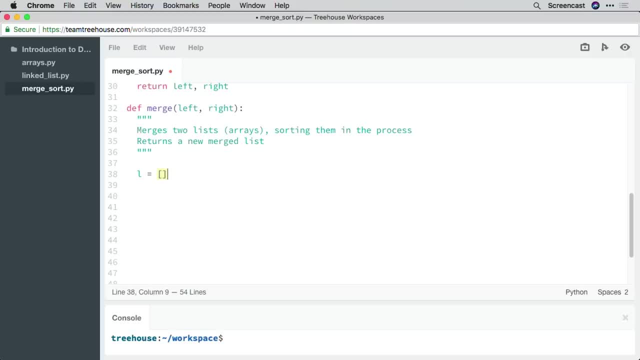 Or each list. So next let's create two local variables To keep track of index values That we're using for each list. So the convention here is i and j, So we'll stick to it. j equals zero As we inspect each value. 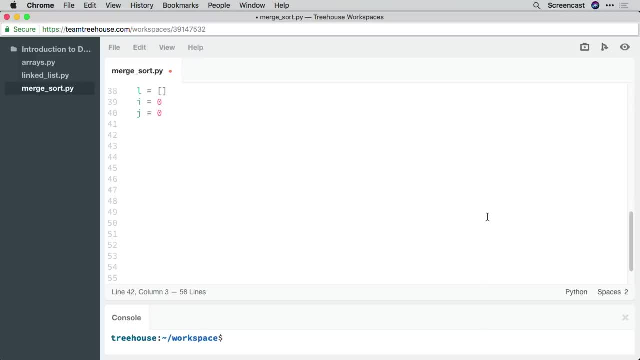 In either list, We'll use the variables To keep track of the indexes Of those values. So we'll use i to keep track of indexes in the left list And j for indexes in the right list. When merging, We want to keep sorting the values. 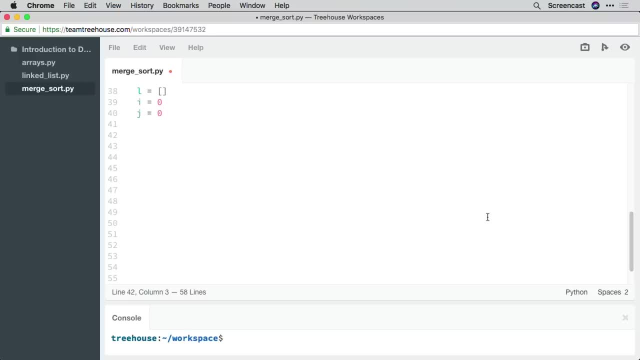 Until we've worked through both lists. So for our loop Let's set up two conditions With an and operator. So we'll say: while, While i is less than, While i is less than the length Of the left list And j. 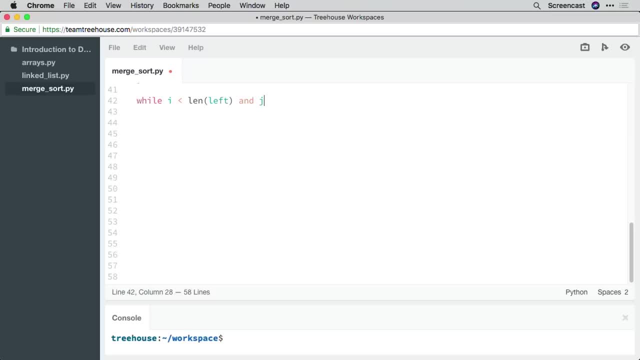 Is less than the Length Of the right list, Then we'll keep executing our loop. So here we're ensuring that As long as i is less than the length Of the left list And the and is important- And j is less than the length, 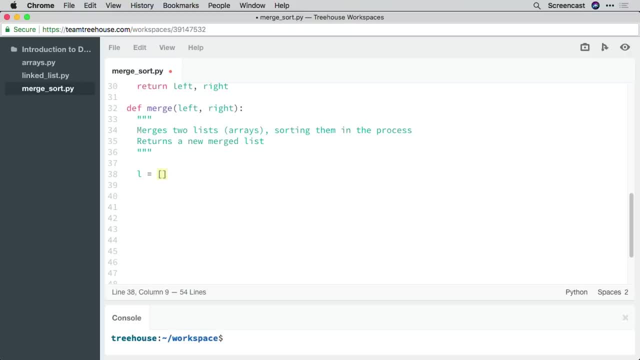 our condition here is as long as the position is less than the index value. so I'll say, while position is less than index, inside the loop we'll assign the next node to current and increment the value of position by one. so current, equal current dot. next node. 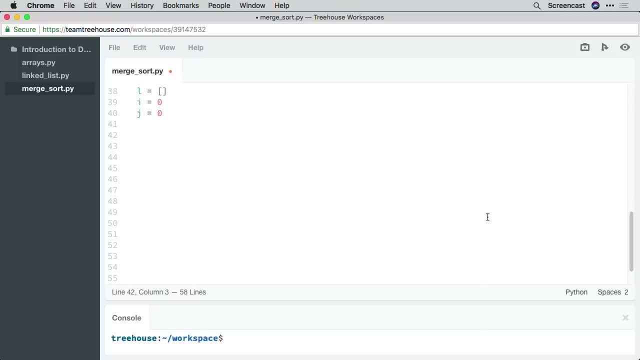 position plus equal one. once the position value equals the index value, current refers to the node we're looking for and we can return it. we'll say return current. let's get rid of all this empty space there. we go now back in linked list: merge sort dot pi. 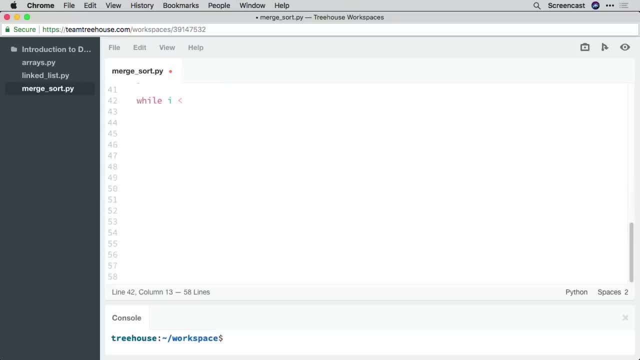 we can use this method to get at the node after we've calculated the midpoint, to get the node at the midpoint of the list. so we'll say mid node equal linked list, dot node at index. and here I'm going to do something slightly confusing. I'm going to do mid minus one. 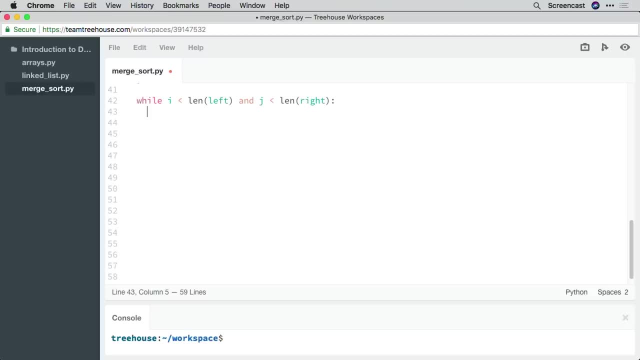 remember we're subtracting one here, because we used size to calculate the midpoint and, like the len function, size will always return a value greater than the maximum index value. so think of a linked list with two nodes. size would return two, the midpoint though, and the way we're calculating the index. 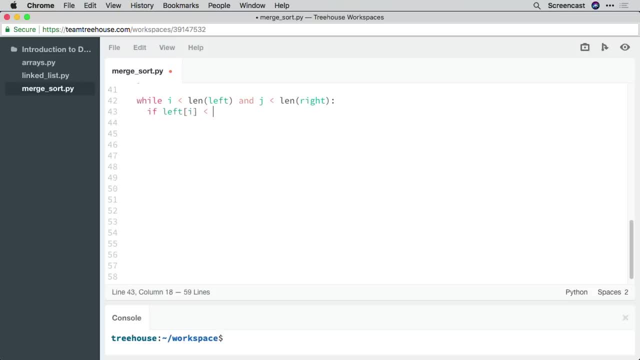 we always start at zero, which means size is going to be one greater than that. so we're going to deduct one from it to get the value we want. but we're using the floor division operator, so it's going to round that down even more. no big deal with the node at. 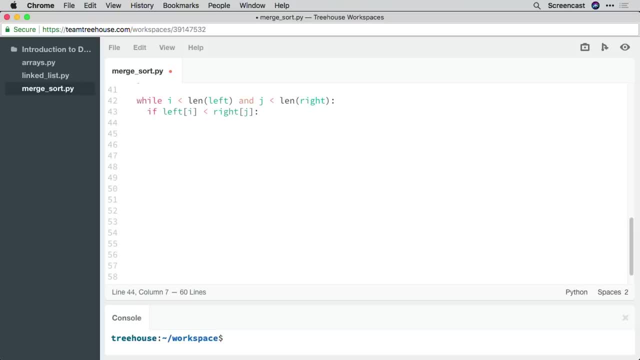 the midpoint. now that we have this mid node we can actually split the list. so first we're going to assign the entire linked list to a variable named left half. so left half, equal linked list. this seems counterintuitive, but it will make sense in a second for the right half. 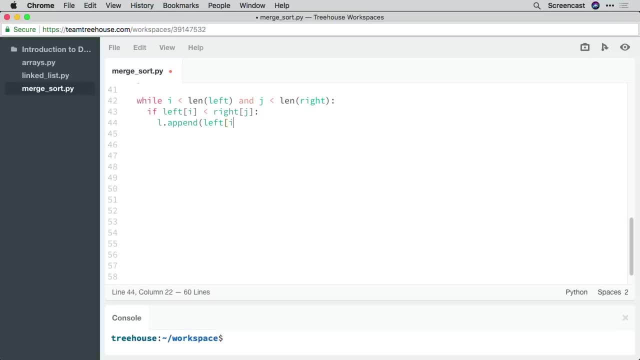 we're going to assign a new instance of linked list. so right, half equal linked list. this newly created list is empty, but we can fix that by assigning the node that comes after the midpoint. so after the midpoint of the original linked list, we can assign the node that comes after that. 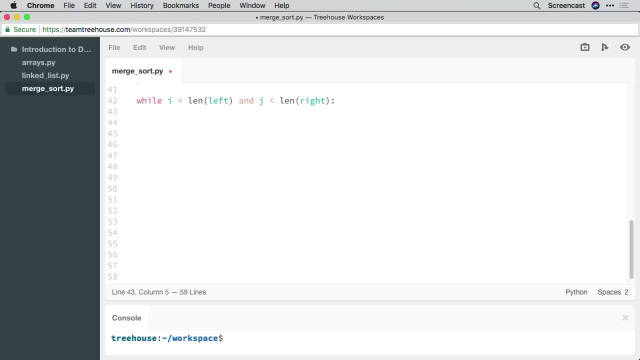 Of the right list. We're going to keep executing The code Now. i and j are both set to zero initially, Which means that our first comparison operation Will be on the first element Of each list respectively. So we'll say: 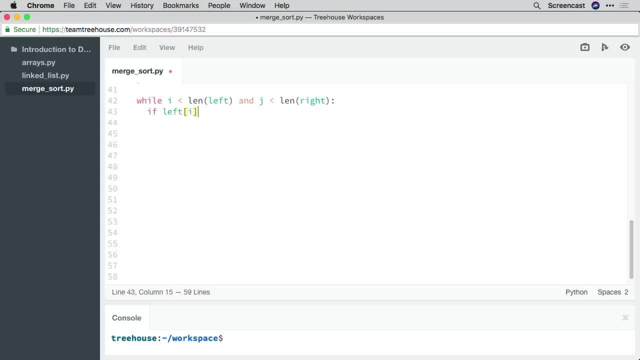 If left i, So i is zero. So this is going to get the first value out of the left list Is less than Right j, And again here J is zero. So we're going to get the first value out of the right list. 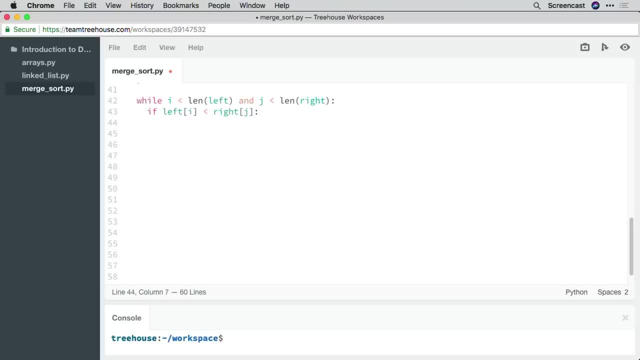 Now, if the value In the left list Is less than the value at index j In the right list, What do we do? Well, that means the value being compared in left Is less than the value in the right And can be placed at position zero. 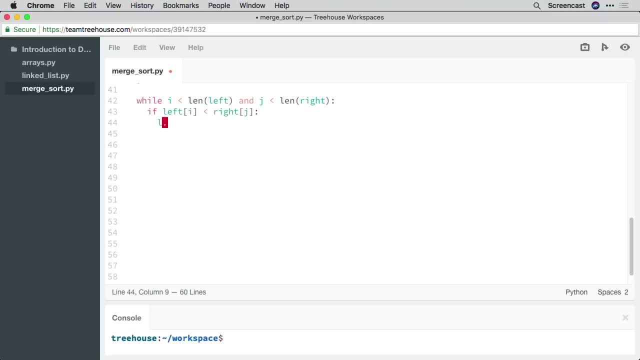 In the new array l That we created earlier. So here we'll say: lappend Left i. Since we've read And done something With the value at position i, Let's increment that value And evaluate the next item In the left list. 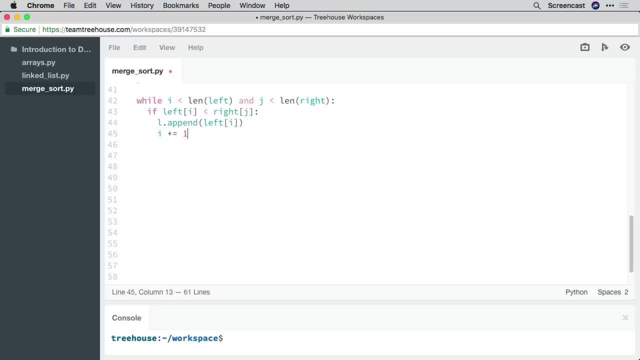 i plus one, Or we can say i plus equal one. Okay, Next is an else statement, And here we'll say: If the value at index i. So I don't have to write out the actual logic, Because it's implied. 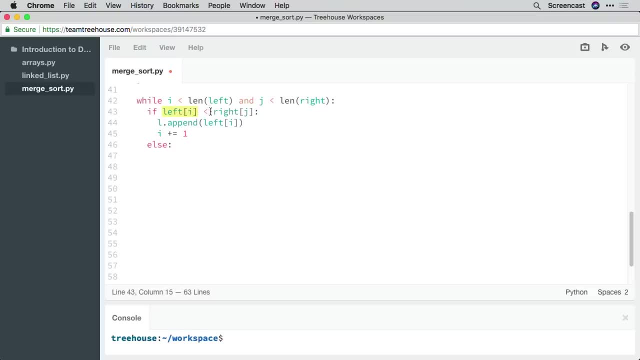 So here we're saying that left, The value at left, Is less than the value at right. Now in the else clause, Equal Is greater, And I haven't written out that condition Because it's implied. So here we're saying: if the value in the left, 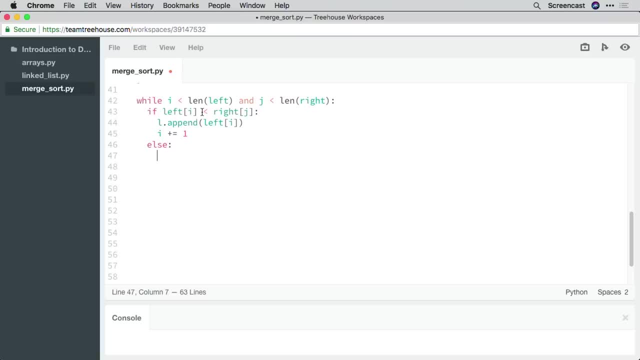 Is less than the value in the right. So in the else clause It's going to mean that the value in the left Is either greater than or equal To the value in the right. But when we hit the else clause, If the value at index i 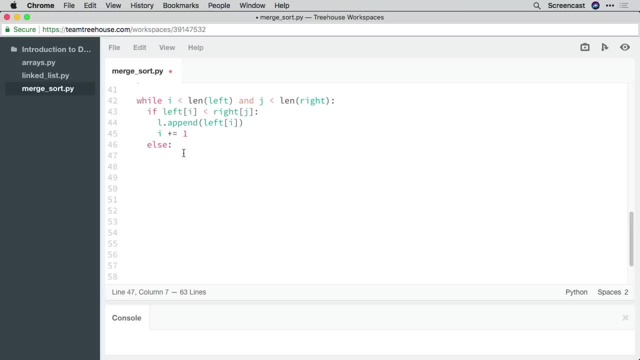 In the left list is greater, Then we place the value at index j, List l, And similarly increment j. So here we'll say l dot, append, Write j, And then j Equal j plus one. Doing this doesn't necessarily mean. 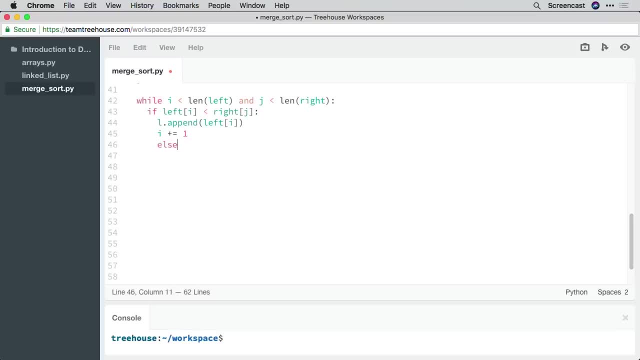 midpoint node as the head of this newly created right linked list. so here we'll say: right, half dot head equal mid node, dot next node. once we do that, we can assign none to the next node property on mid node to effectively sever that connection and make what was the mid 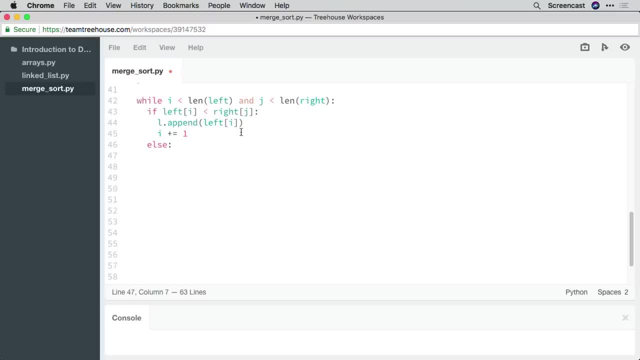 node, now the tail node of the left linked list. so I'll say mid node, dot, next node equal none. if that's confusing, here's a quick visualization of what just happened. we start off with a single linked list and find the midpoint, the node that comes after the node. 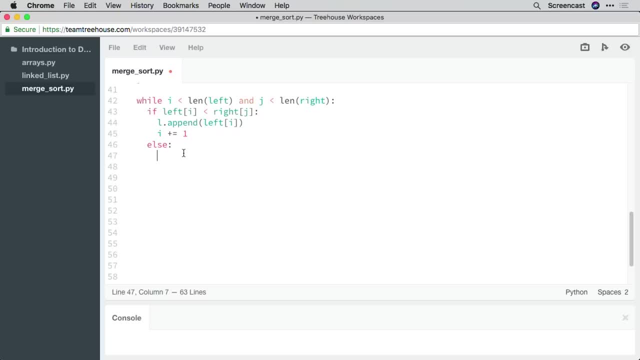 at midpoint is assigned to the head of a newly created linked list and the connection between the midpoint node and the one after is removed. we now have two distinct linked lists split at the midpoint, and with that we can return the two sublists. so we'll return left half. 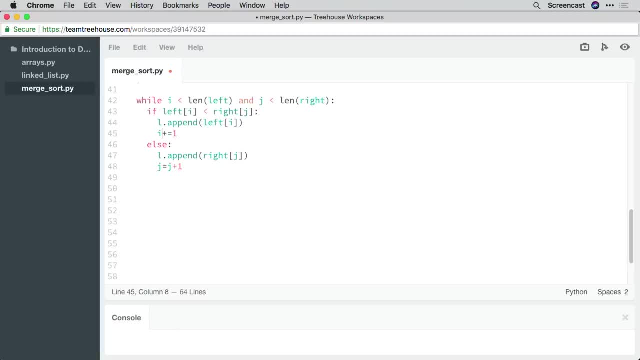 and right half. in the next video let's tackle our merge function. in the last video we defined an implementation for the version of the split function that works on linked lists. it contained a tiny bit more code than the array or list version, and that was expected. the merge function is. 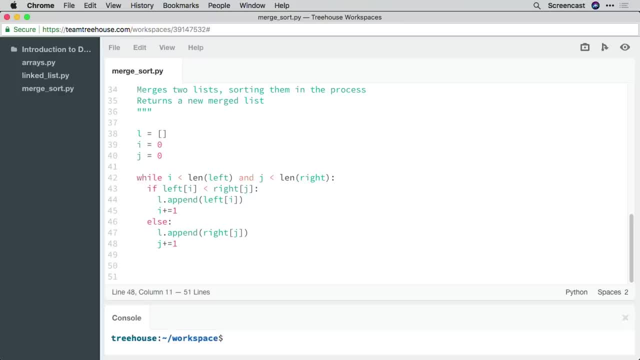 no different because, like with the split function, after we carry out a comparison operation, we also need to swap references to corresponding nodes. alright, let's add our merge function over here at the bottom below these split functions. we'll call this merge and it's going to take a. 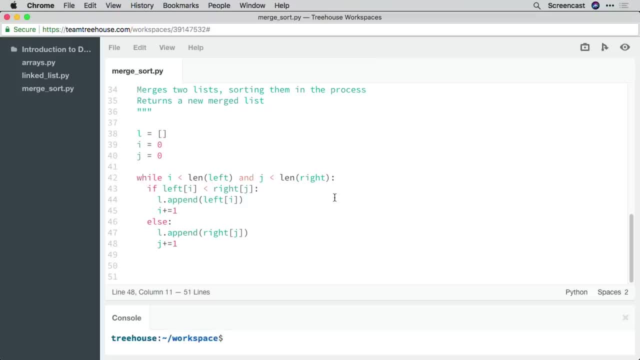 left and a right. now, because this can get complicated, we're going to document this function extensively and, as always, we're going to start with a doc string. so we'll say that this function merges two linked lists, sorting by data in the nodes, and it returns a new 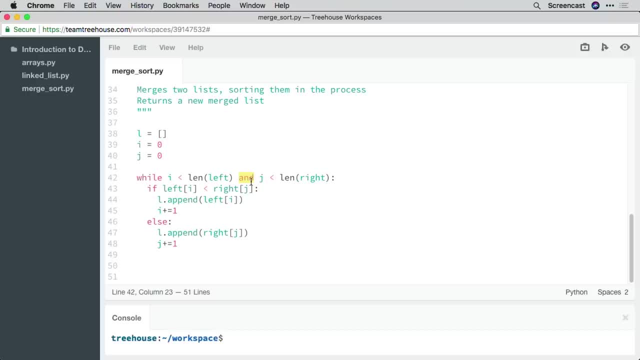 merged list. remember that in the merge step we're going to compare values across two linked lists and then return a new linked list with nodes where the data is sorted. so first we need to create that new linked list. let's add a comment in here. we'll say: 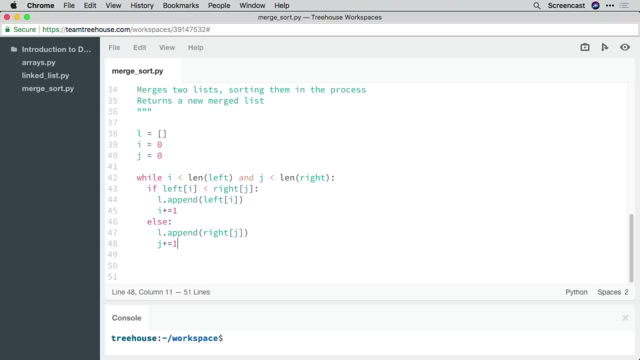 That in one step We'll have a completely sorted array. But remember that because we start with single element arrays And combine with each merge step, We will eventually Sort all the values more than one time And by the time The entire process is done. 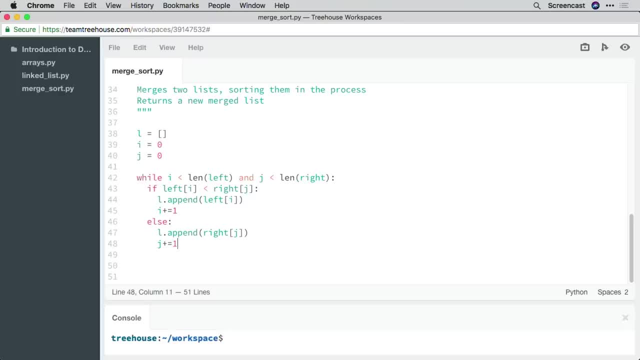 All the values are correctly sorted. Now. this isn't all we need to do In the merge step, however, There are two situations we can run into: One where the left array Is larger than the right, And vice versa. So this can occur when an array containing 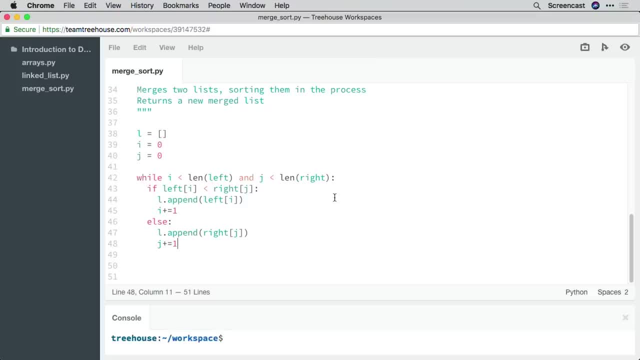 An odd number of elements needs to be split. So how do you split a three element array Or list, While the left can have two elements And the right can have one, Or the other way around? The first condition Is an AND condition. 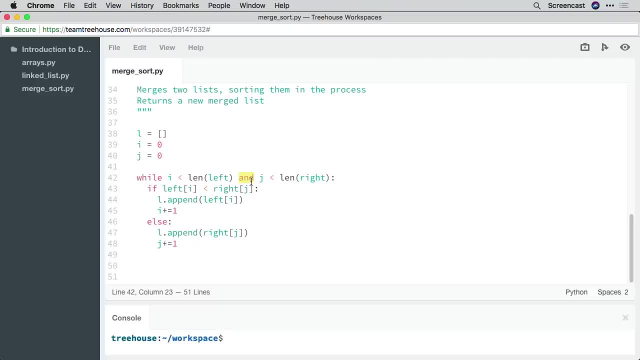 Where the variables used to store the indexes Need to be less than the length of the lists. If the left list is shorter than the right, Then the first condition returns false And the entire loop returns false Because it's an AND condition. 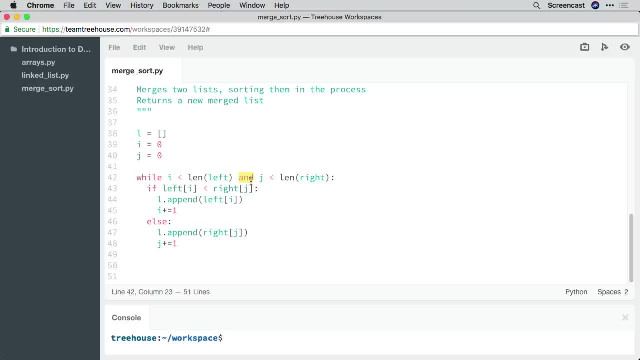 This means that in such an event, When the while loop terminates, Not all the values in the right list Will have been moved over to the new combined list. So to account for this, Let's add two more while loops. The first while loop 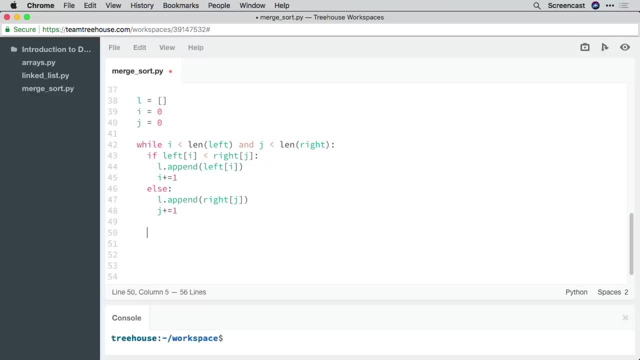 Is going to account for a situation Where the right list Is shorter than the left And the previous loop terminated Because we reached the end of the right list first. So in this case, What we're going to do Is simply add the remaining elements in the left. 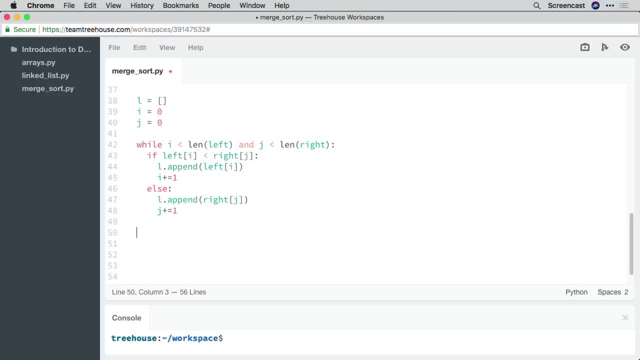 To the new list. We're not going to compare elements Because we're going to assume that within a list The elements are already sorted. So while i Is left, Then it's the same logic: L dot, append left, i And i. 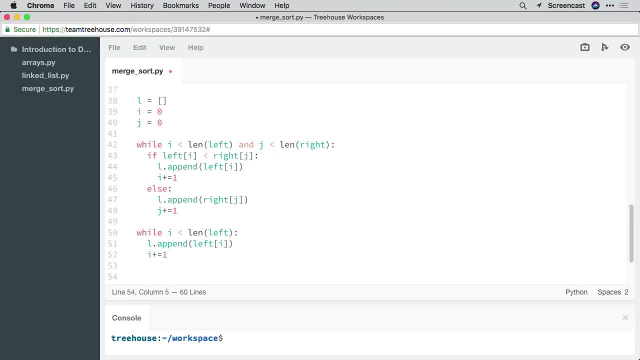 Plus equal one. So the while loop Is going to have the similar condition. Keep the loop going until it's at the last index Inside the body. We're incrementing the index With every iteration of the loop. Our final loop accounts for the opposite scenario. 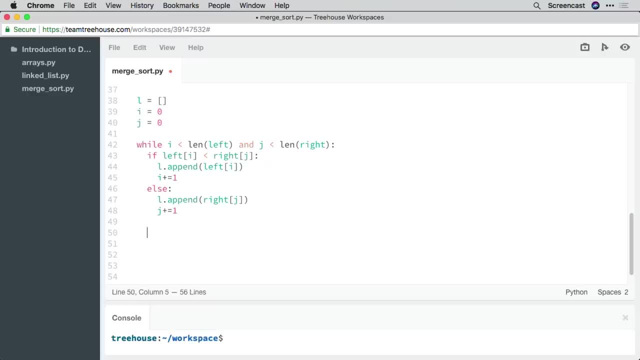 create a new linked list that contains nodes from: let's add on a new line merging left and right, okay, and then create the list so merged equal new linked list to this list. we're going to do something unusual. we're going to add a fake head. this is: 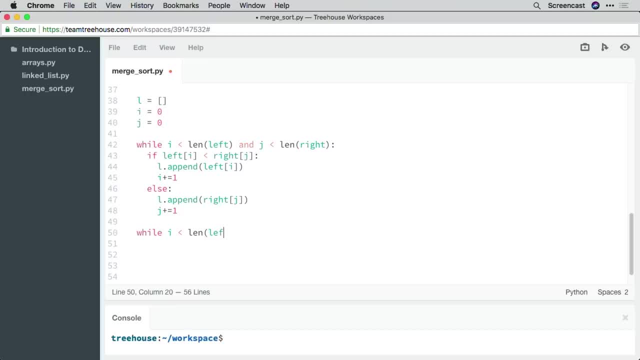 so that when adding sorted nodes, we can reduce the amount of code we have to write by not worrying about whether the head of the list. once we're done, we can assign the first sorted node as the head and discard the fake head. now, this might not make sense at first, but not having to 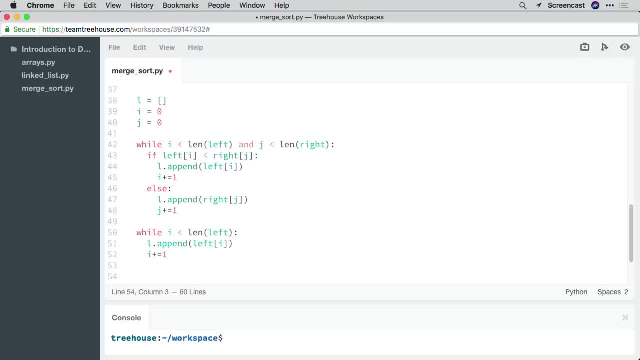 worry about whether the new linked list already contains a head or not, makes the code simpler. we'll add another comment, add a fake head that is discarded. later we'll say merged dot add zero, like we've been doing so far. we'll declare a variable named current to point to the head. 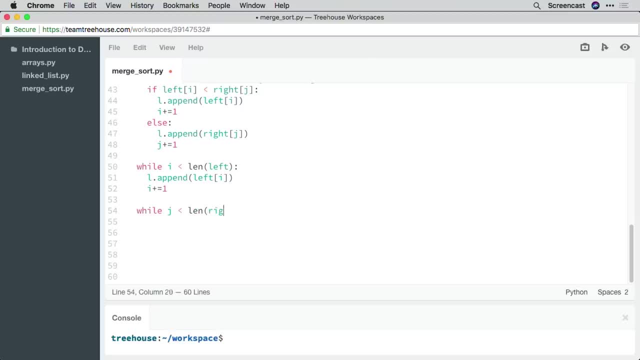 of the list set current to the head of the linked list and then current equal merged dot head. next we'll get a reference to the head on each of the linked lists, left and right. so we'll say: obtain head nodes for left and right linked lists and. 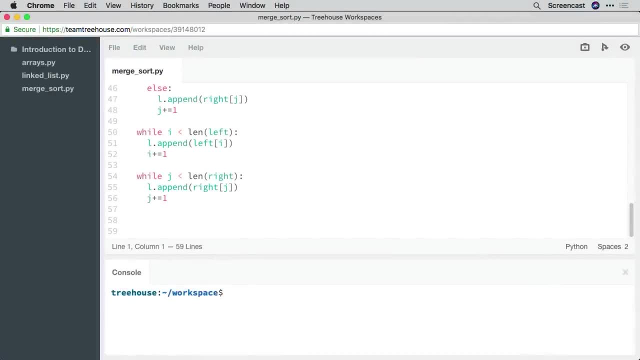 here we'll call this: left head equal left dot head and right head equal right dot head. okay, so with that setup out of the way, let's start iterating over both lists. so another comment: iterate over left and right as long, or we'll say until the until we. 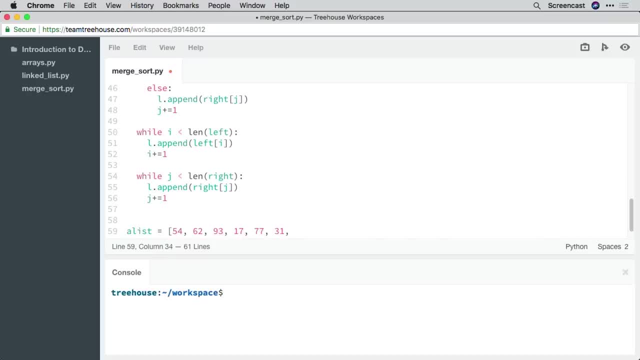 reach the tail node of either, and we'll do that by saying: while left head or right head. so this is a pattern that we've been following all along. we're going to iterate until we hit the tail nodes of both lists and we'll move this pointer. 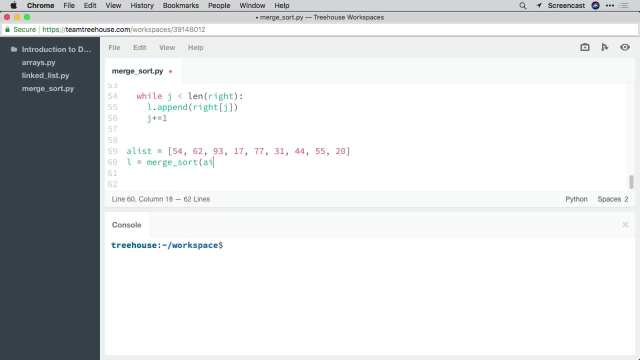 forward every time so that we traverse the list with every iteration. if you remember the logic behind this from the earlier version, once we hit the tail node of one list, if there are nodes left over in the other linked list, we don't need to carry out a comparison operation anymore. 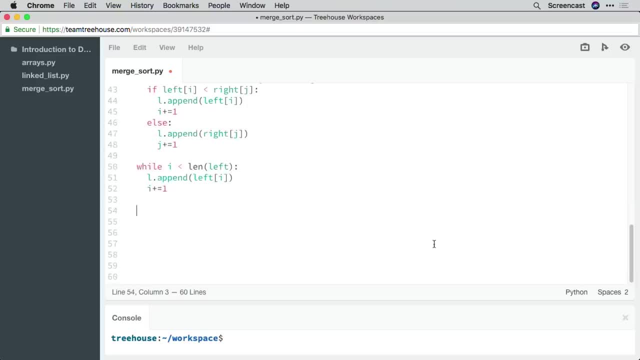 Where the left was shorter than the right. The only difference here Is that we're going to use the variable j Along with the right list. So we'll say: while j Is less than length of right L dot append Right j. 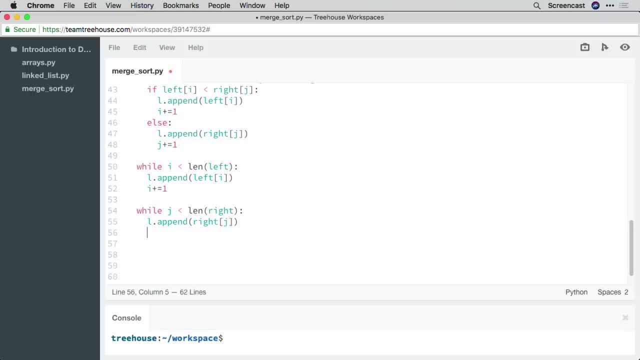 And j Plus equal one. Okay, Let's stop here. In the next video Let's test out merge sort, Make sure our code is running correctly And everything is written well, And then we'll wrap up this stage By documenting our code. 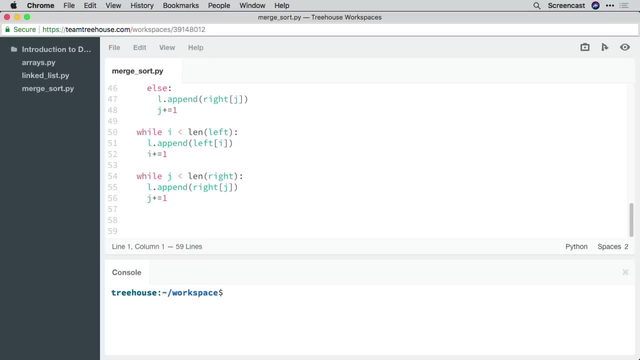 We completed our implementation For the merge sort algorithm, But we didn't test it in any way. Let's define a new list at the bottom That contains several numbers. You can put whatever you want in there, But make sure that the numbers are not in order. 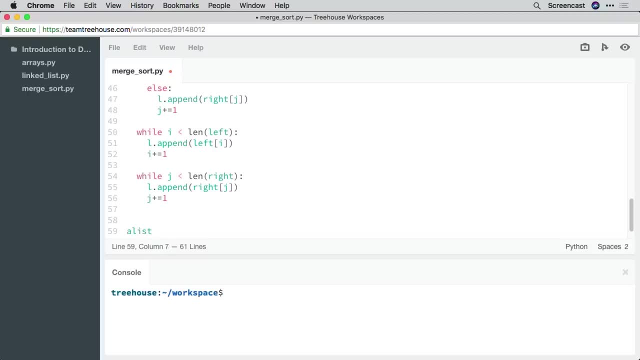 I'll call mine A list And in here We'll say 54.. 26 or 62. Doesn't matter. 93,, 17,, 77., 31.. Just add enough So that you can make out. 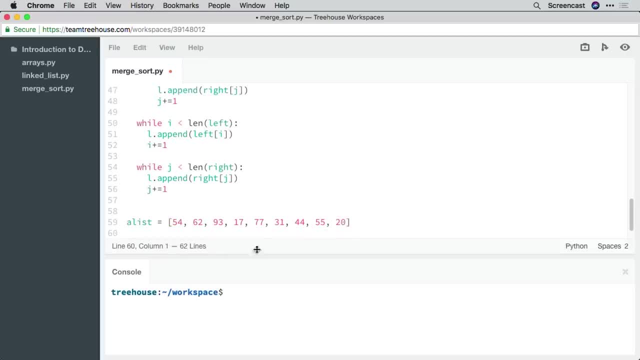 That it's sorted. Okay. Next we're going to call the merge sort algorithm And pass in our list. Let's assign this to some variables. We'll say: l, equal, merge, Underscore, sort A list And then, if it works correctly, 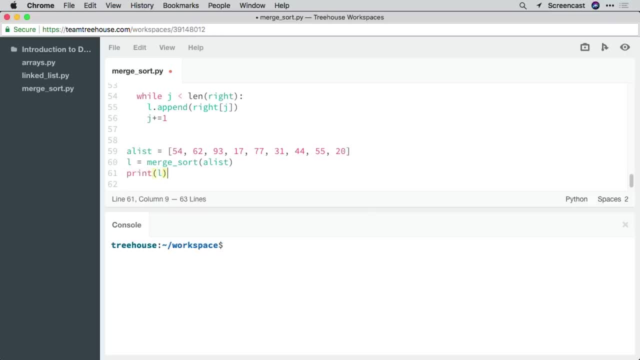 We should be able to print this list And see what it looks like. So I'm going to hit save Down here in the console, Merge, sort dot pi And before I hit enter- Actually notice, I made an error in the last video. 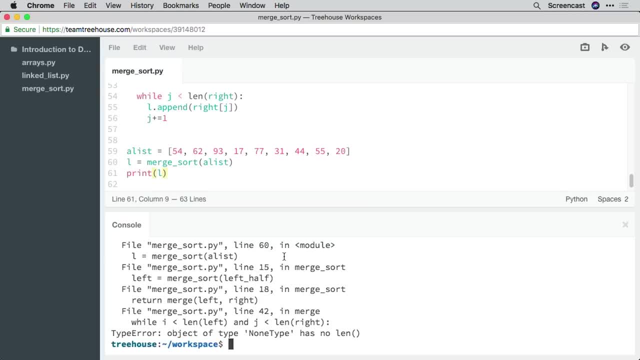 But I'll hit enter anyway And you should see the error pop up. Okay, so what I forgot to do- Which is a pretty crucial part of our algorithm- Is in the merge function. I forgot to return the list Containing the sorted numbers. 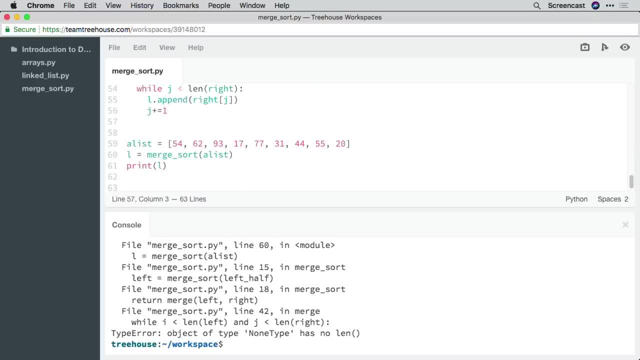 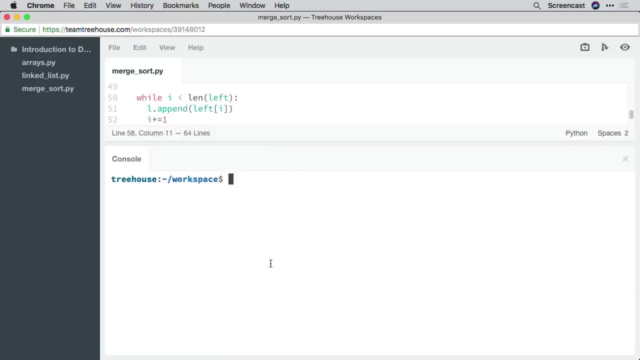 After carrying out all this logic. So here at the bottom We'll say: return l, Alright, we'll save again. And now we'll clear this out And try that one more time. And there we go. You should see a sorted list. 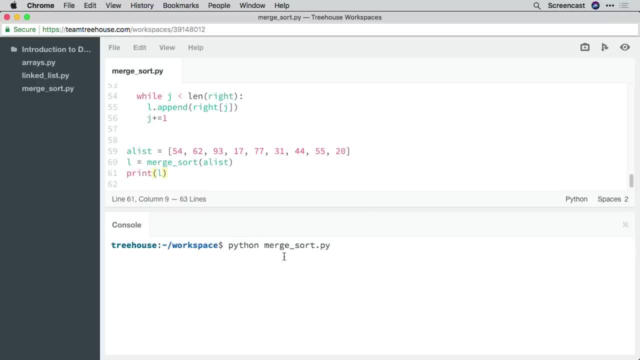 and we can simply add those nodes to the merged list. the first scenario we'll consider is if the head of the left linked list is none, this means we're already past the tail of left and we can add all the nodes from the right linked list to the final merged list. 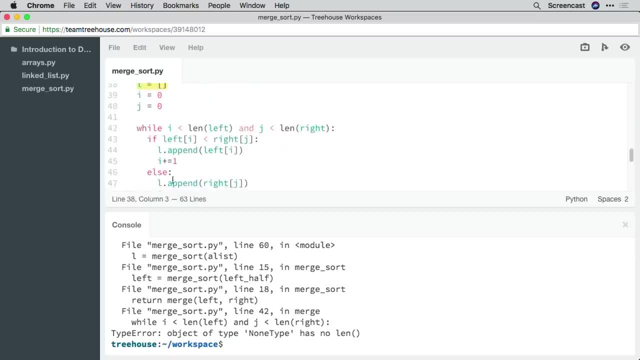 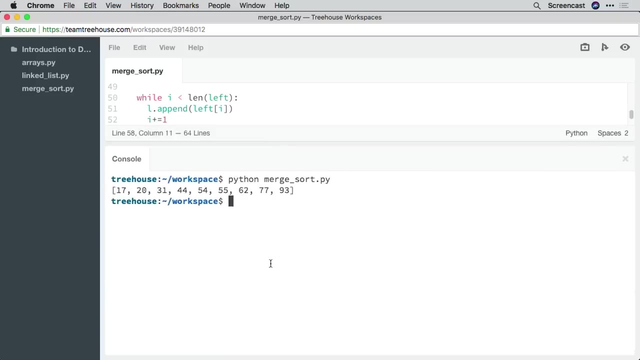 so here I'll say: if the head node of left is none, we're past the tail, add the node from the right to merged linked list. so here we'll say: if left head is none, current dot, next node, remember current points to the head of the merged list that we're going to return. 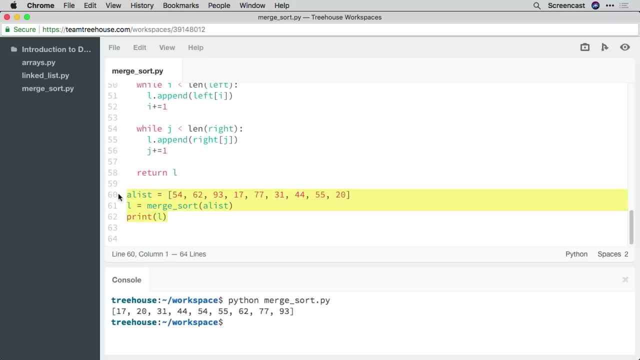 so here we're setting its next node, reference to the head node on the right linked list. so here we'll say right head. then when we do that we'll move the right head forward to the next node. so we'll say right head, equal right head dot. next node. 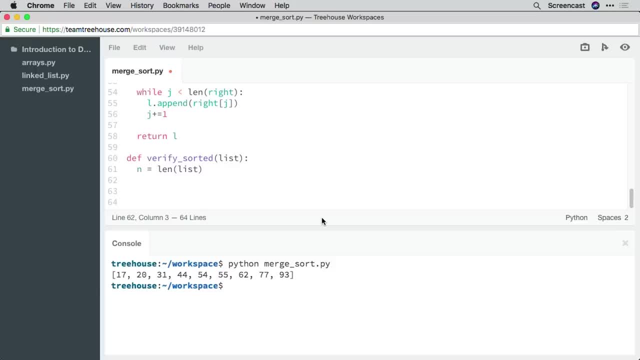 this terminates the loop. on the next iteration, let's look at a visualization to understand why. let's say we start off with a linked list containing four nodes, so we keep calling split on it until we have lists with just a single head, single node, linked list, essentially. so let's focus on 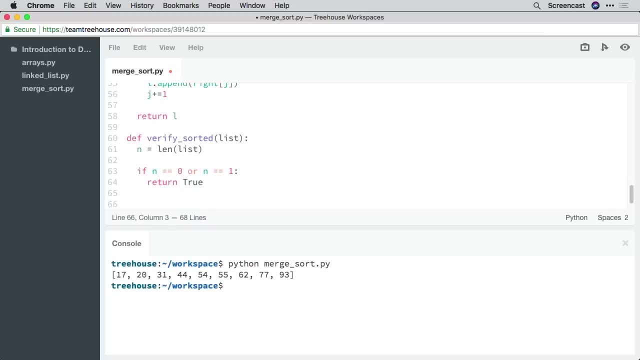 these two down here that we'll call left and right. we haven't implemented the logic for this part yet, but here we would compare the data values and see which one is less than the other. so we'll assume that left's head is lesser than right's head, so we'll set this. 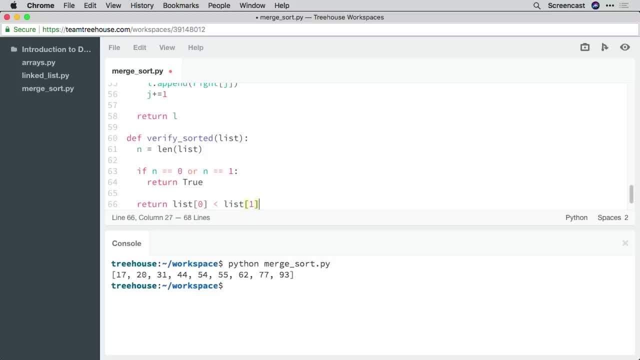 as the next node in the final merged list. left is now an empty linked list, so left dot head equals none. on the next pass through the loop, left head is none, which is the situation we just implemented here. we can go ahead and now assign right head as the next node in the 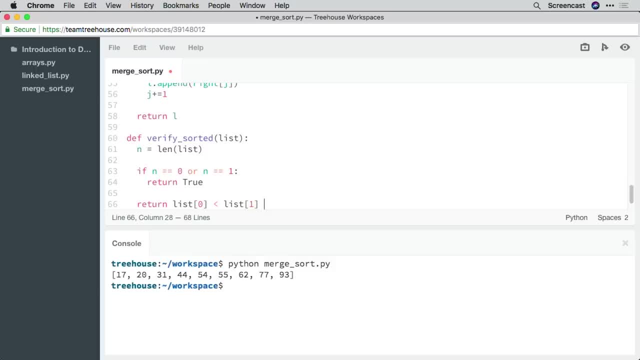 merged linked list. we know that right is also a singly linked list. here's the crucial bit: when we move the pointer forward by calling next node on the right node there is no node and the right linked list is also empty now, which means that both left head and right head are none. 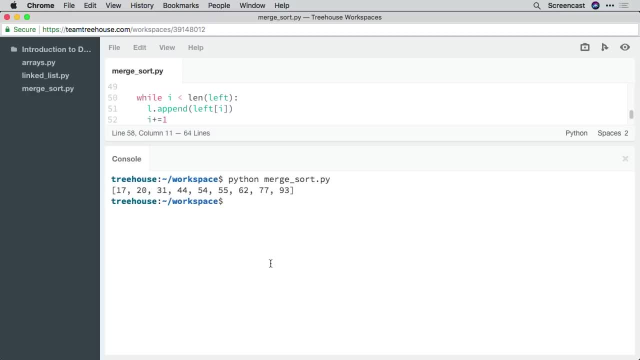 Printed out. We can write out a more robust function to test this, Because with bigger arrays, Visually evaluating that printed list Won't always be feasible. So we'll bring this back down. Let's get rid of this And we'll call our function. 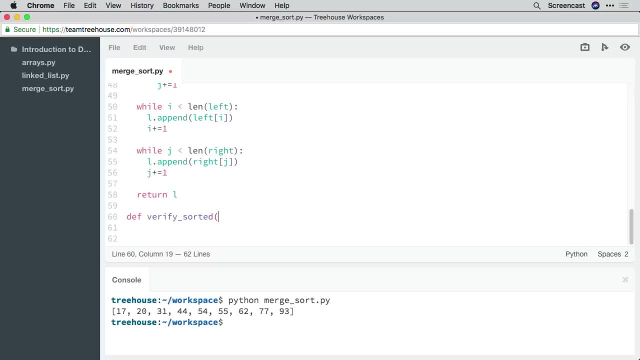 Verify, sorted And this will take a list. And this will take a list. First we're going to check Inside the body of the function. We'll check the length of the list If the list is a single element list Or an empty list. 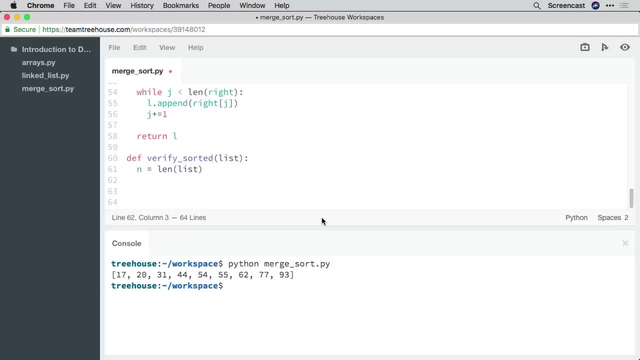 We don't need to do any unnecessary work Because, remember, it is naively sorted. So we'll say if n Equals 0. Or if n Equals 1.. Then we'll return: true, We've verified that it's sorted. 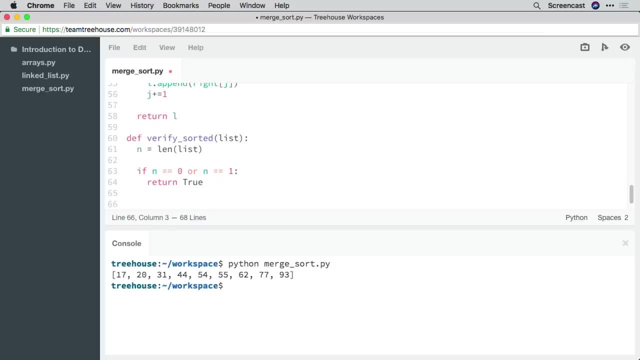 Now to conclude our function. We're going to write out one line of code That will do quite a bit of work. So first we'll say Return list 0. So we'll take the first element out of the list And we'll compare and see if that's less than. 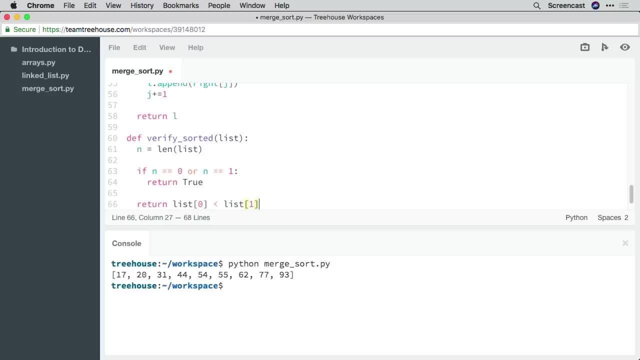 The second element in the list. Okay, So first we'll check that the first element in the list Is less than the second element in the list. This returns either true or false, So we can return that directly, But this isn't sufficient. 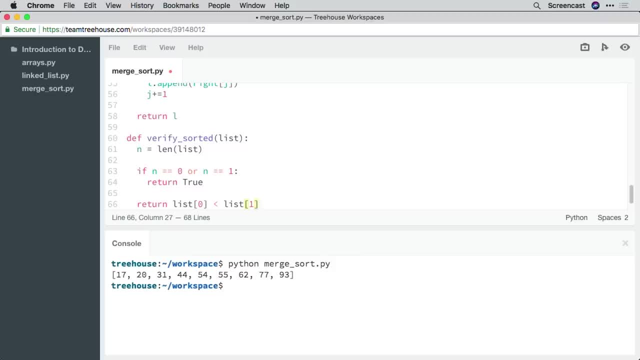 If it were, We could trick the verify function By only sorting the first two elements in the list. So to this return statement We're going to use an And operator To add on one more condition. For this condition, We're going to make a recursive function call. 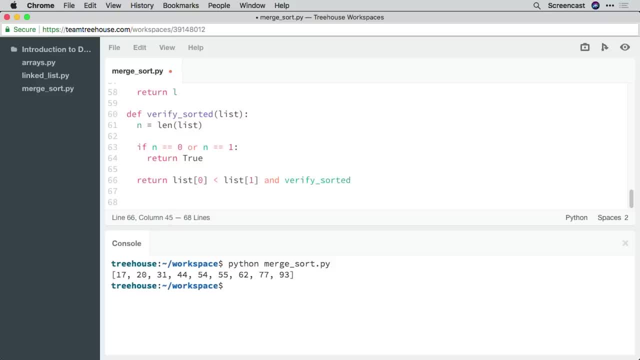 Back to verify sorted And for the argument We're going to pass in the list, Going from the second element All the way To the end. Let's visualize how this would work. We'll use a five element list as an example. 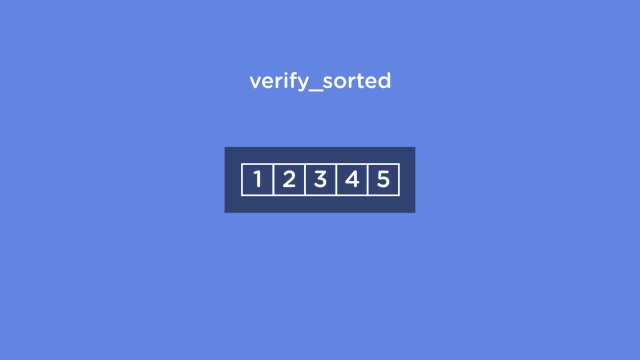 So we'll call verify, sorted And pass in the entire list. This list is not one or zero elements long, So we skip that first if statement There's only one line of code Left in the function And first we check that the element at index zero. 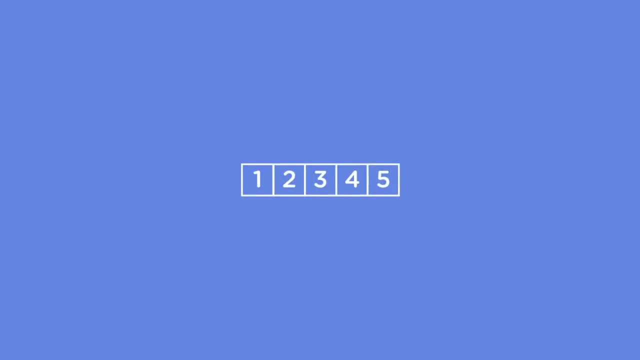 and either one of these would cause our loop condition to terminate. so what we've done here is encoded a stopping condition for the loop. so we need to document this because it can get fuzzy. so right above that line of code, I'll say call next on right. 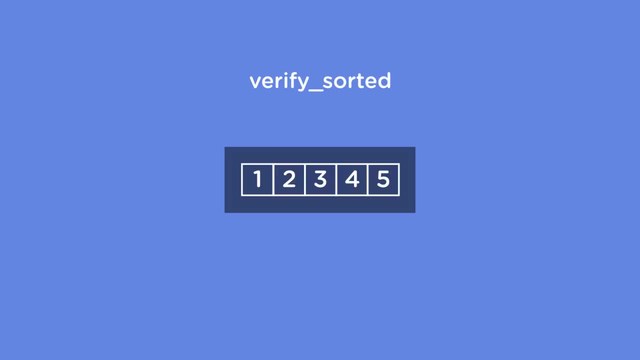 to set loop condition to false. okay, there's another way we can arrive at this stopping condition, and that's in the opposite direction, if we start with the right head being none. so here we'll say: I'm going to add another comment, if oops, not there. 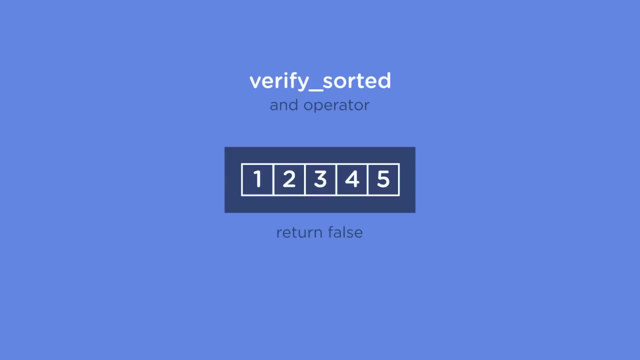 there. if the head node of right is none, we're past the tail. then we'll say: add the tail node from left to merged linked list and then we'll add that condition. we'll say else, if right head is none, now remember, we can enter these even if left head is none. 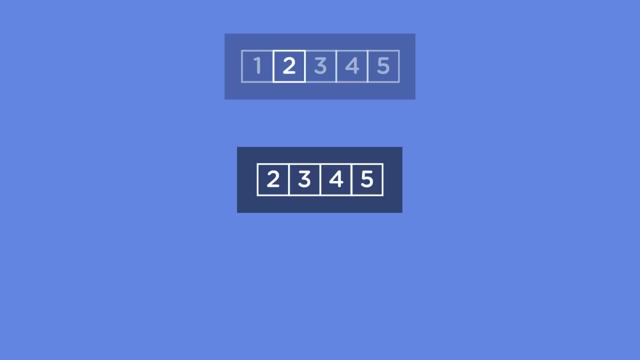 we can still go into this condition. we can still enter this if statement and execute this logic, because, while loop, the loop condition here is an or statement. so even if left head is false, if this returns true because there's a value there, there's a node there, the loop. 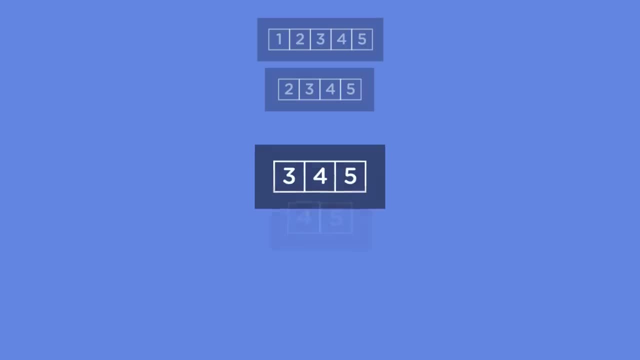 will keep going. okay, now, in this case, we want to set the head of the left linked list as the next node on the merged list. so this is simply the opposite of what we did over here. we'll set current dot next node equal to left head and then we'll 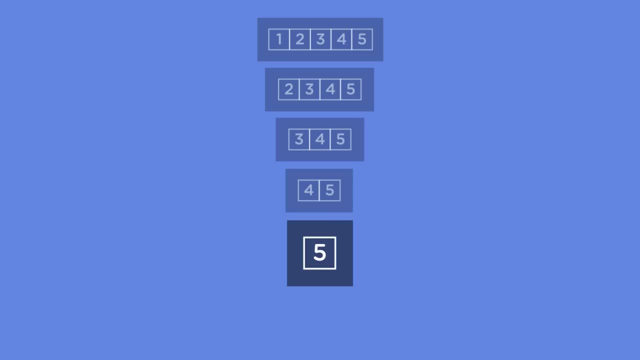 move. so after doing that we can move the variable pointing to left head forwards which, as we saw earlier, is past the tail node and then results in the loop terminating. so we'll say: left head equal left head dot next node and we'll add that comment here as well. 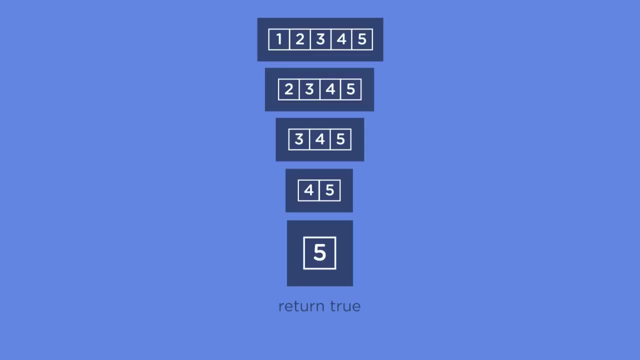 so we'll say: call next on left to set loop condition to false, because here right head is none and now we make left head none. these two conditions we looked at were either the left head or right head. were at the tail nodes of our respective lists. those are conditions. 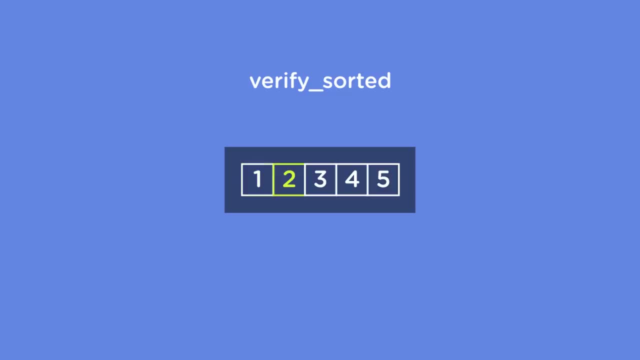 Is less than the element at index one. If this is false, The function returns immediately With a false value. An and operator Requires both conditions to be true For the entire line of code to return true, Since the first condition evaluates to false. 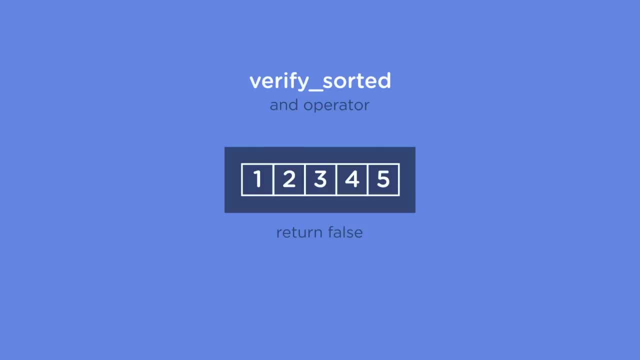 We don't need to bother Evaluating the second. The second condition is a recursive call With a sub list Containing elements from the original list, Starting at position one And going to the end. So on the second call, Again, we can skip that first if statement. 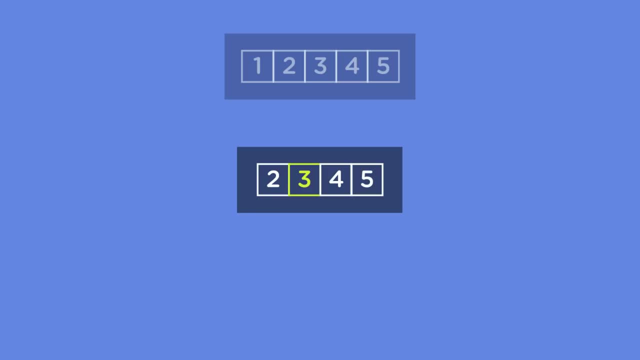 And proceed to check whether the value at element zero Is less than the value at element one. Remember that, because this list Is a sub list of the original, Starting at the element that was the second element In the original list, By comparing the elements at position zero. 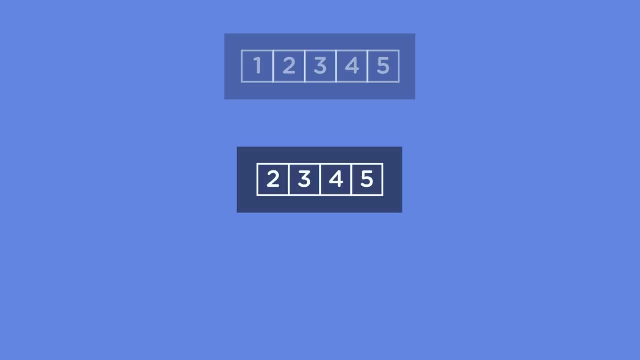 And one in the sub list. We're effectively comparing the elements At position one and two In the original list. With each recursive call As we create new sub lists That start at index position one, We're able to check the entire list. 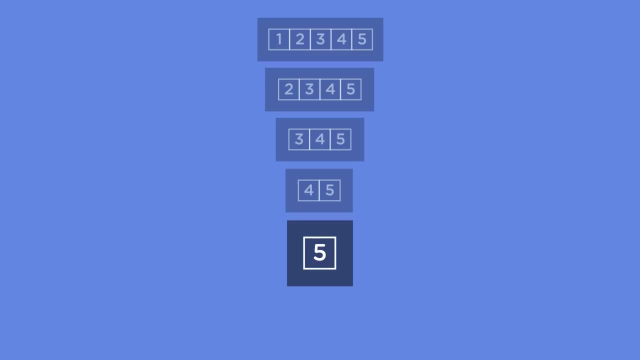 Without having to specify Any checks other than the first two elements. Since this is a recursive function, It means We need a stopping condition And we have it already. It's that first if condition In the sub lists Once we reach a single element list. 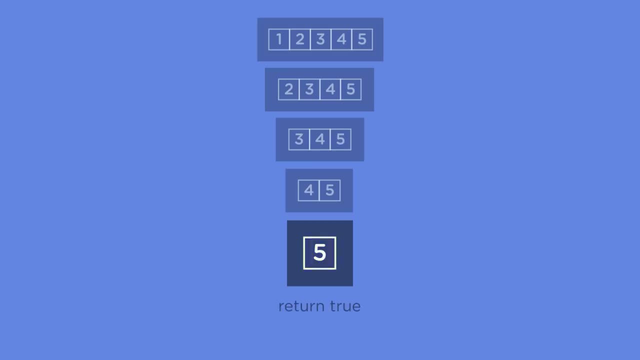 That element is already sorted by definition, So we can return true. Since this recursive function call Is part of an and condition, It means that every single recursive call Has to return true All the way back to the beginning For our top level function to return true. 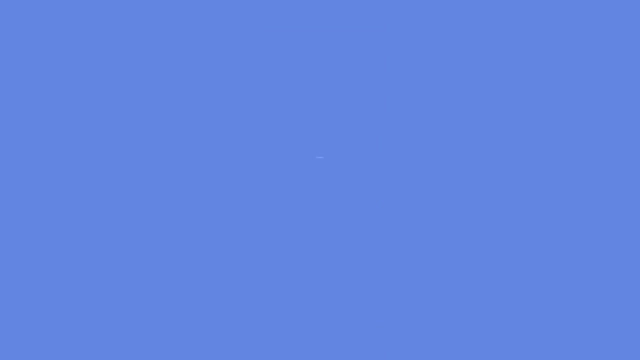 And for the function to say: Yes, this is sorted Now. we could have easily done this Using an iterative solution and a for loop, But this way We have a recursion to work through And understand, So let's use this function. 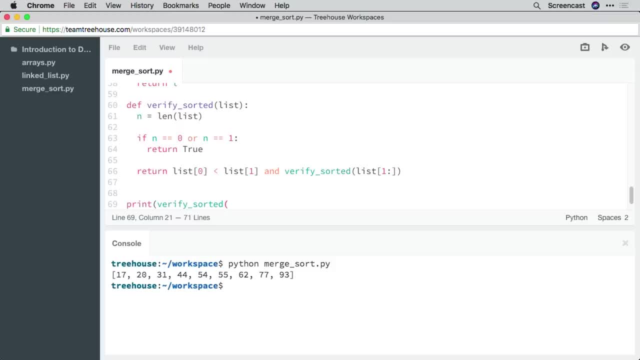 At the bottom we'll say print, Verify, sorted, And first we'll pass in a list. Oops, we got rid of that, didn't we? Okay, Let me write it out again. So a list equal, And I think I have those original numbers. 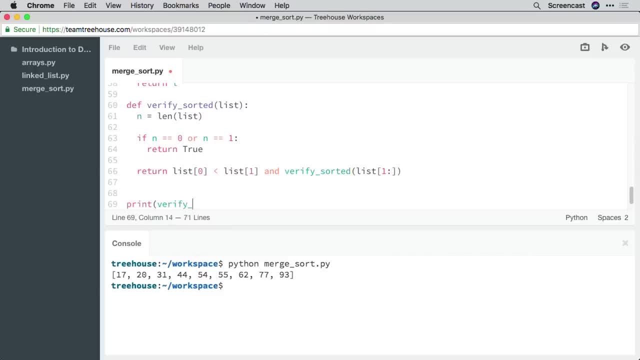 we run into when we've reached the bottom of our split, where we have single element linked lists or empty linked lists, let's account for our final condition, where we're evaluating a node that is neither the head nor the tail of the list, and this condition we need to reach into the 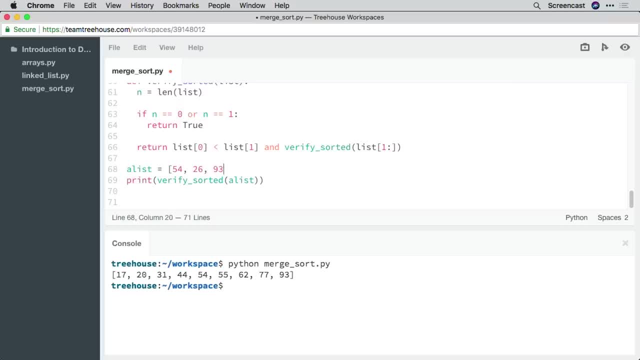 nodes and actually compare the data values to one another before we can decide which node to add first to the merged list. so here this is an else, because we've arrived at our third condition, third and final, and here we'll say not at either tail node obtain. 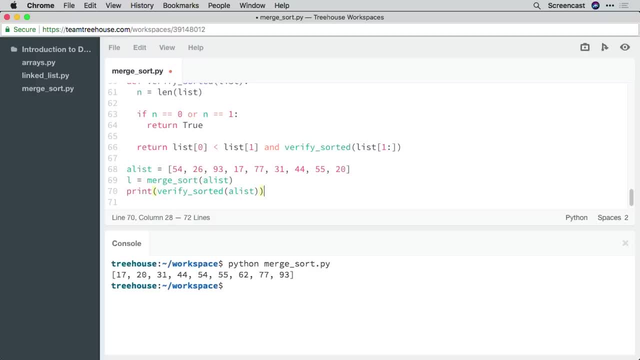 node data to perform comparison operations. so let's get each of those data values out of the respective nodes so that we can compare it. so we'll say: left data equal left head dot data and right data equal right head dot data. okay, what do we do next? 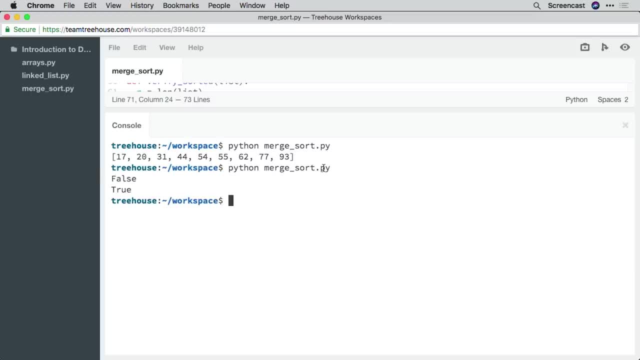 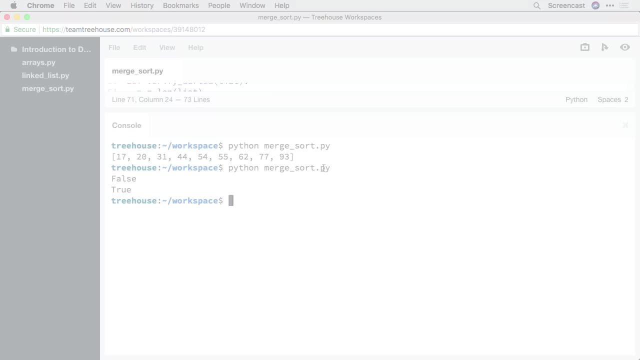 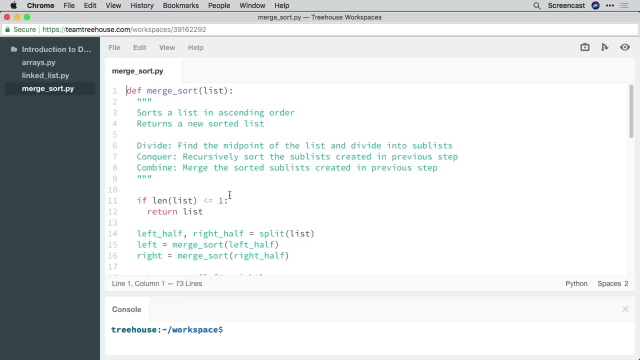 well, we compare. but first let's add a comment. so we'll say: if data on left is less than right, set current to left node and then move. actually we'll add this in a second. so here we'll say: if left data is less than right data, then 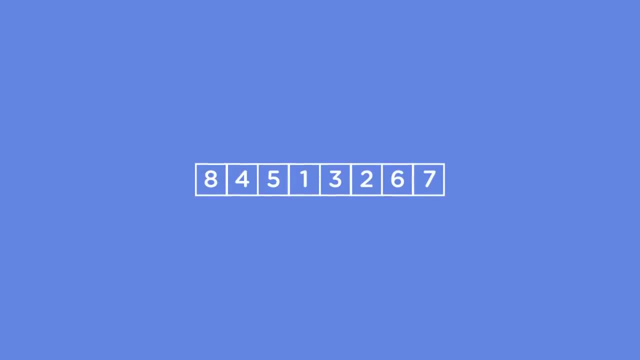 current dot. next node: equal left head. and then we'll add a comment and we'll say: move left head to next node on that list. so we'll say: left head equal left head dot next node. just as our comment says. we'll check if the left data is less. 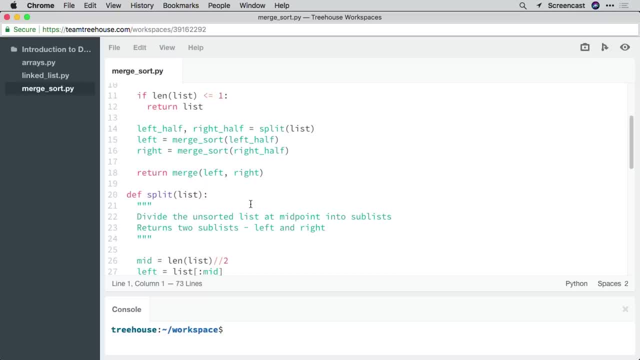 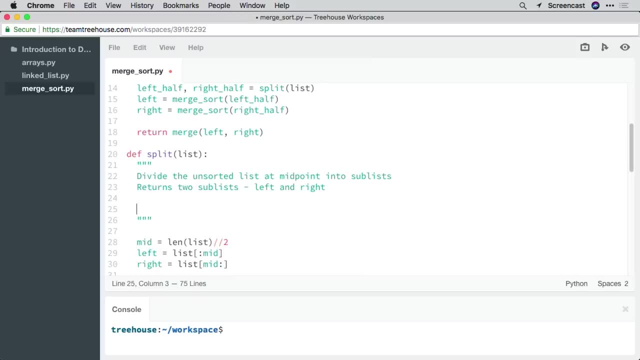 than the right data. if it is, since we want a list in ascending order, we'll assign the left node to be the next node in the merged list. we'll also move the left head forward to traverse down to the next node in that particular list. now, if left is large, 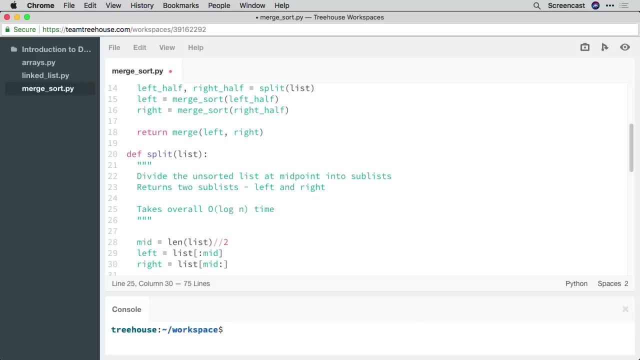 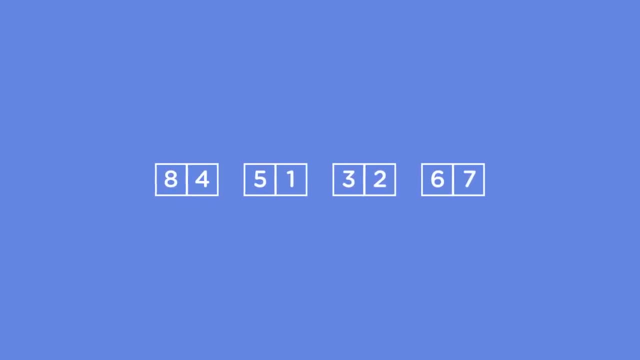 than right, then we want to do the opposite, so we'll go back two spaces. add another comment: if data on left is greater than right, set current to right node. okay, so else here we assign the right head to be the next node in the merged list, so current dot. 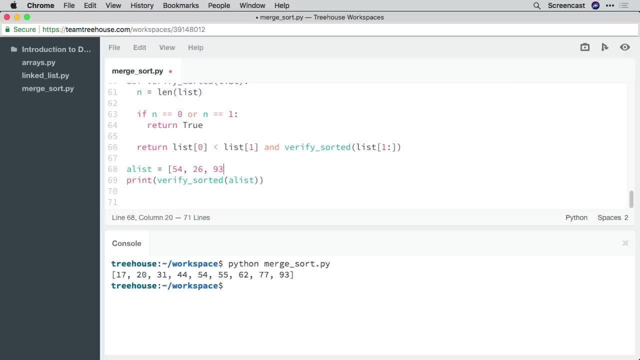 Here somewhere. So we'll say 54,, 26,, 93.. Okay, And then we assign it to l, The result of calling merge Sort On a list. Okay, so now here We're going to use the verify sorted function. 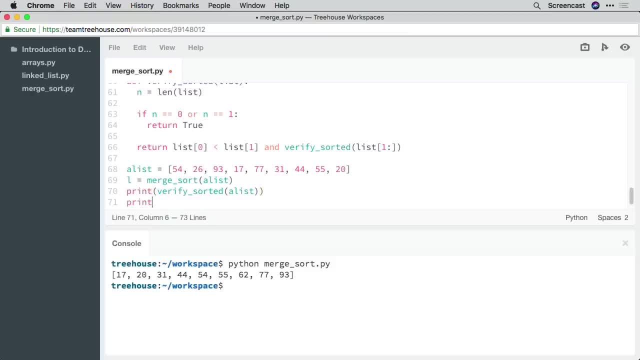 And we'll check first that a list Is sorted. That should return false And then we'll check the same call on. We'll pass in l And this should return true. Okay, so now at the bottom here in the console, We'll call python. 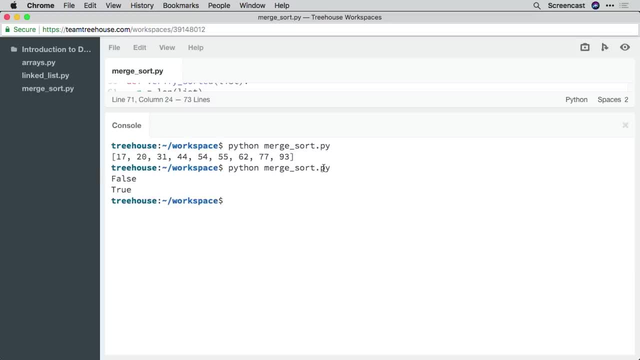 And there we go. It returned false for a list, Meaning it's not sorted, But l is sorted. Cool, So our merge sort function works. In the next video let's talk about the cost of this algorithm If we go back to the top level. 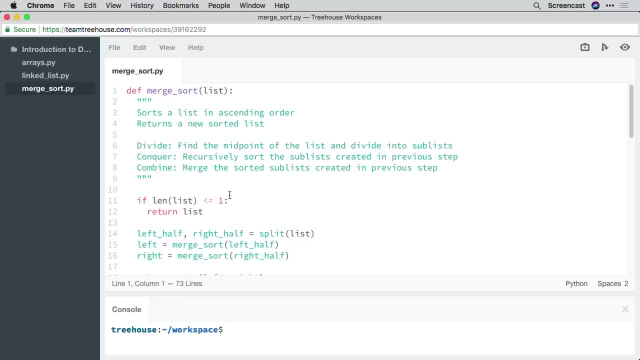 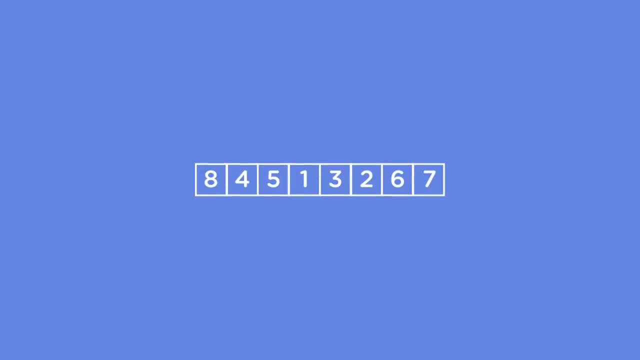 The merge sort function. What does the run time of this function look like? And what about space complexity? How does memory usage grow as the algorithm runs? To answer those questions, Let's look at the individual steps, Starting with the split function. 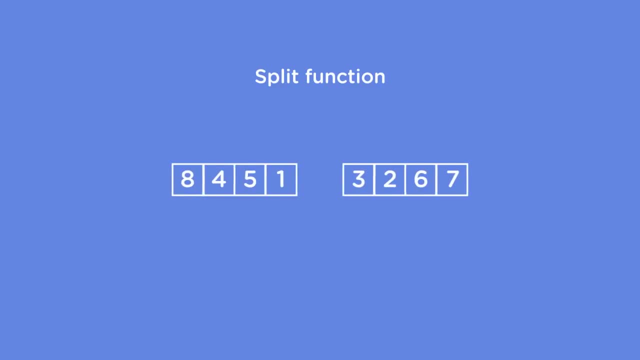 In the split function. All we're doing is finding the midpoint of the list And splitting the list at the midpoint. This seems like a constant time operation, But remember that the split function Isn't called once. It's called as many times as we need it to. 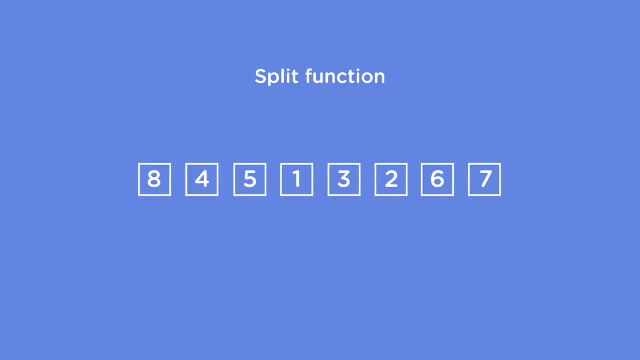 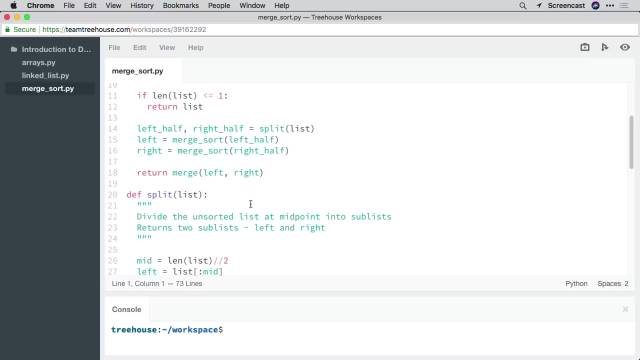 To go from the initial list Down to a single element list. Now, this is a pattern We've seen a couple times now And we know that overall This runs in logarithmic time. So let's add that as a comment. So here I'll say: 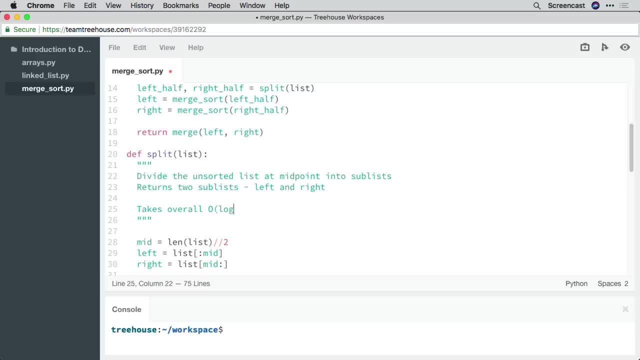 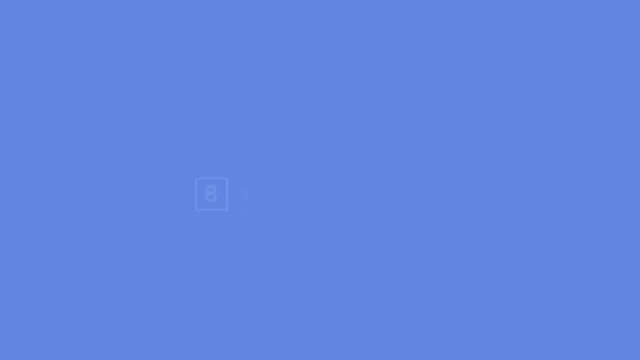 Overall Big O of log n time. Now there's a caveat here, But we'll come back to that. So next up is the merge step. In the merge step We've broken the original list down Into single element lists And now we need to make comparison operations. 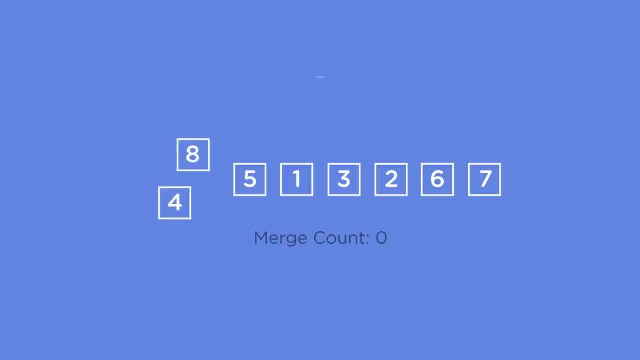 And merge them back in the reverse order. For a list of size n, We'll always need to make An n number of merge operations To get back from single element lists To a merge list. This makes our Overall runtime Big O of n times log n. 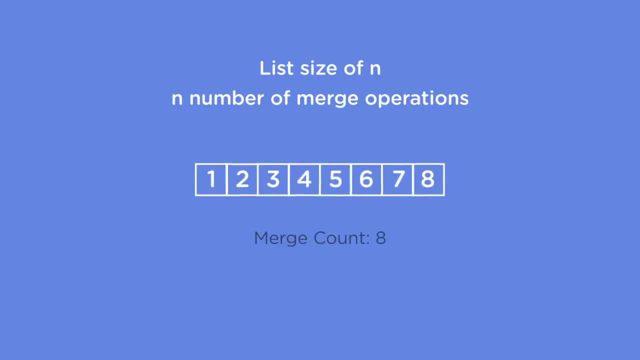 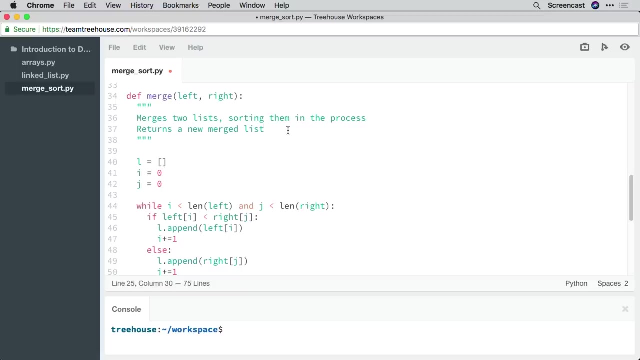 next node: equal right head. and then comment: move right head to next node. so right head, equal right head dot next node. okay, after doing that, we move the right head pointer to reference the next node in the right list and finally, at the end of each iteration of the while loop, so not 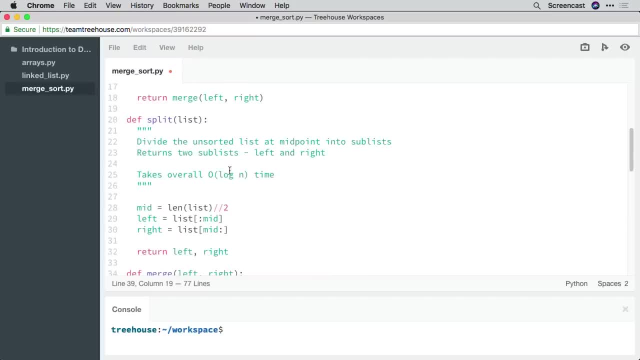 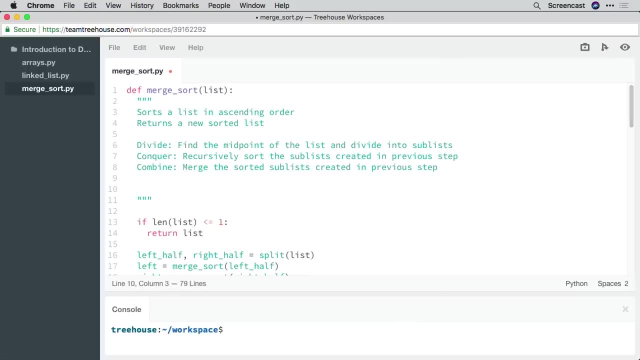 here but two spaces back, make sure we're indented at the same level as the while. so we gotta go yup or not, the same level as the while, but the same outer scope. and then there we're going to say: move current to next node. so current, equal current dot. 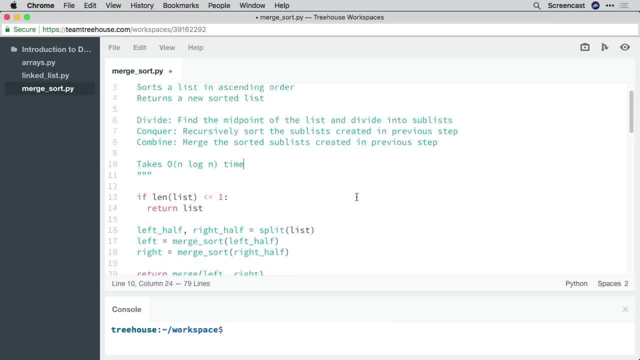 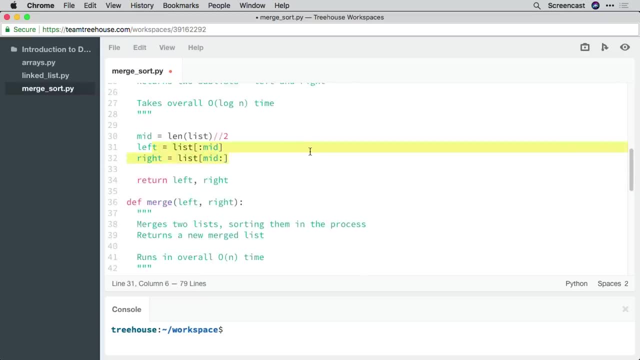 next node. okay, don't worry if this is confusing. as always, we'll look at a visualization in just a bit. so we'll wrap up this function by discarding that fake head we set earlier, setting the correct node as head and returning the linked list. so we'll add a comment. 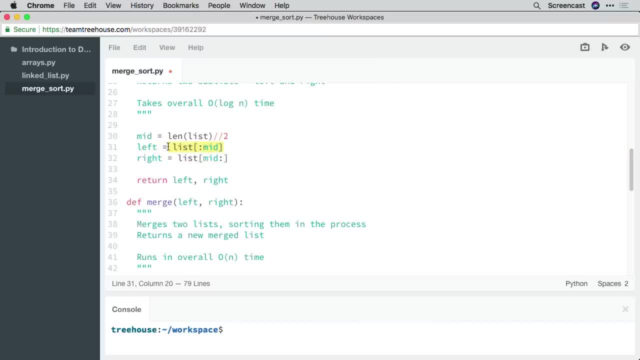 discard fake head and set first merged node as head. so here we'll say: head equal, merged dot, head dot next node, and then merged dot, head equal head and finally return merged. okay, we wrote a lot of code here. a lot of it was comments, but still it's a bunch. let's take a quick. 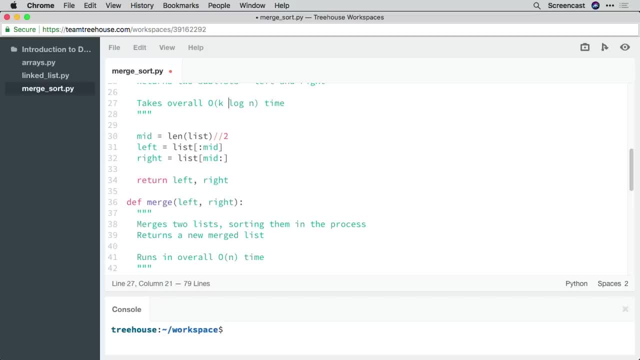 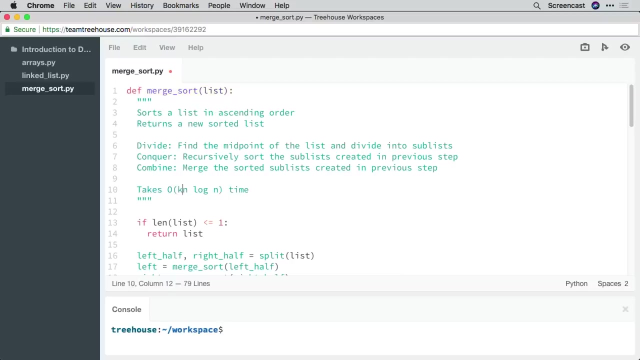 break. in the next video, we'll test this out, evaluate our results and determine the run time of our algorithm. okay, first things first. let's test out our code now. we'll keep it simple, because writing a robust verify function would actually take up this entire video. instead, I'll leave that up to you to try. 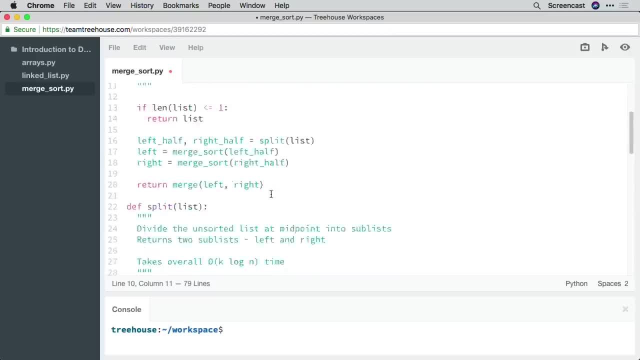 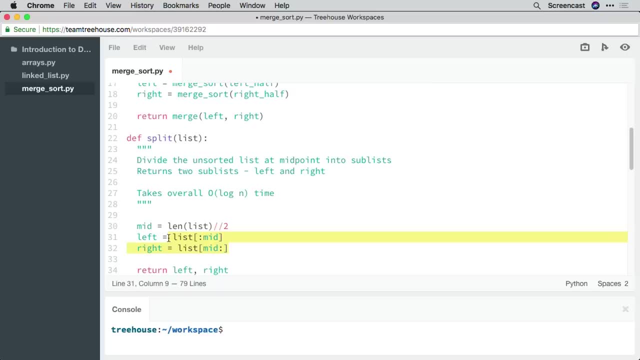 as homework. okay, so at the very end, let's create a new linked list. let's add a few nodes to this, so I'll add- I'm gonna copy paste this so it makes it easier for me not to have to retype a bunch. so I'll add 10. 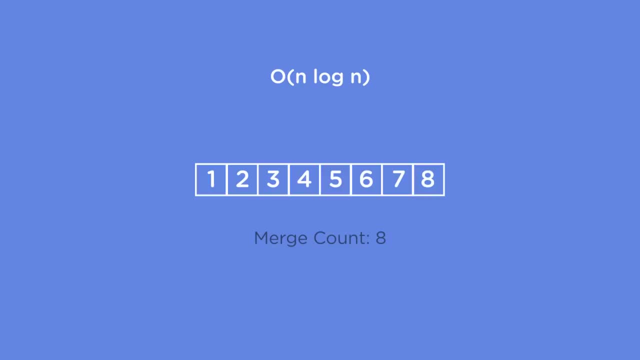 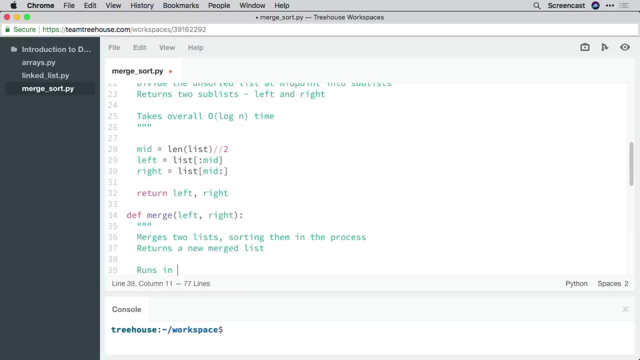 Because that's an n number of merge steps Multiplied by a log, n number of splits Of the original list. So to our merge step here Let's add a comment. We'll say it runs in overall. Whoops, There we go. 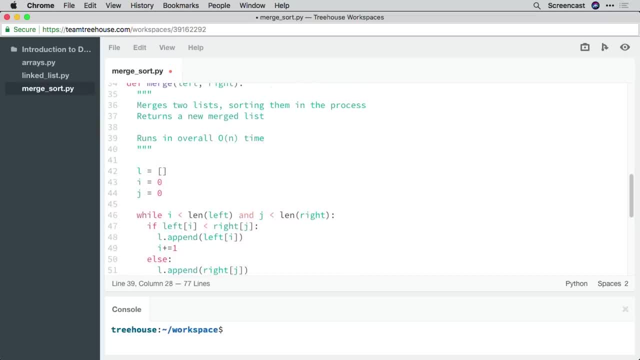 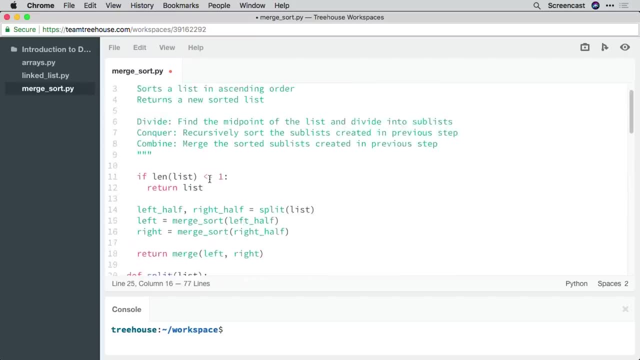 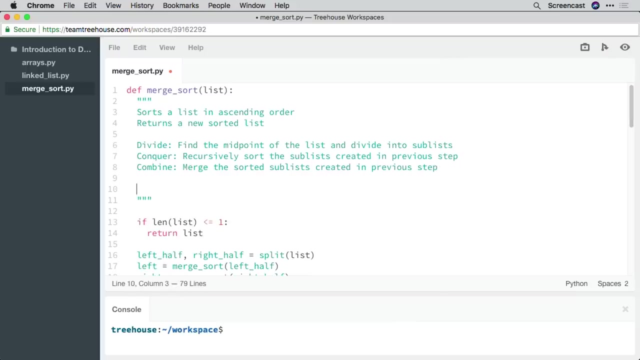 Runs in overall linear time. It takes an n number of steps. Number of merge steps Of these two, So linear here and logarithmic here. We can multiply these And say that the merge sort function, The top level function. We can conclude that the runtime 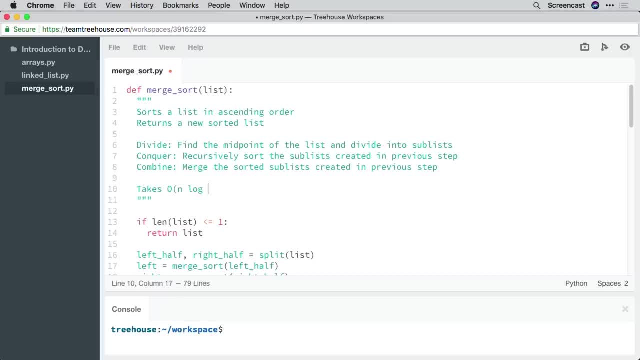 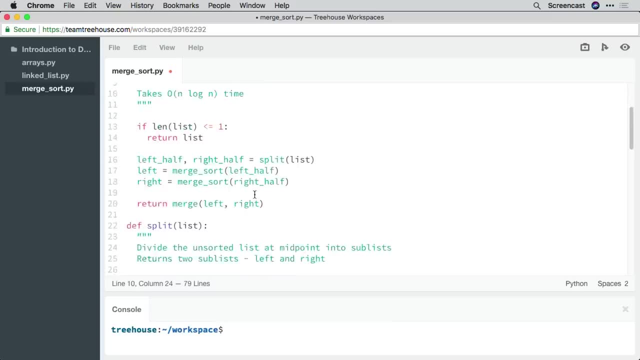 Of the overall sorting process is: We go of n times, log n. Now what about that caveat I mentioned earlier? So if we go back to our Split function here, Right here, There we go. Let's take a look at the way. 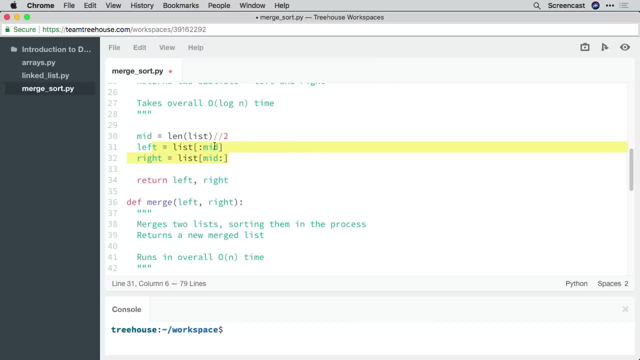 We're splitting the list, So we're using Python's List slicing operation here And passing in two indexes Where the split occurs. Now, if you go and poke around The Python documentation, Which I've done, It says that a slicing operation 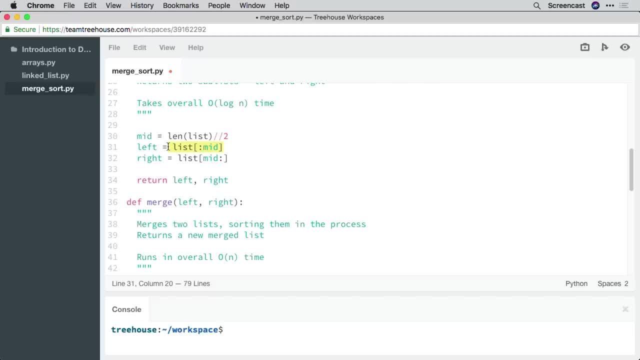 Is not a constant time operation And in fact has a runtime Of big O of k, Where k represents the slice size. This means that in reality, Our implementation of split Is not done in logarithmic time But k times logarithmic time. 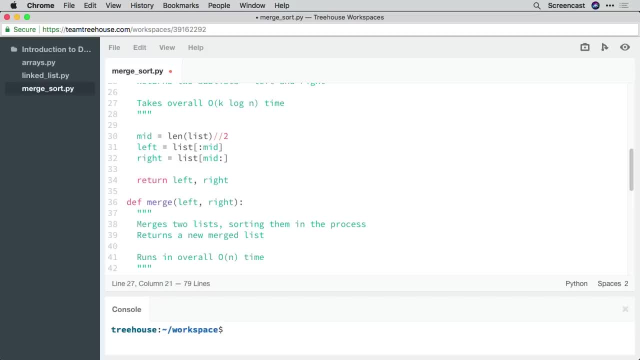 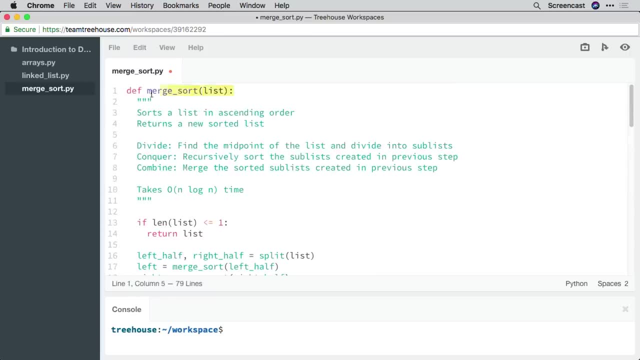 Because there's a slice operation For each split. This means that our implementation Is much more expensive. So overall That makes our overall top level merge sort function Not n times log n But k n times log n, Which is much more expensive. 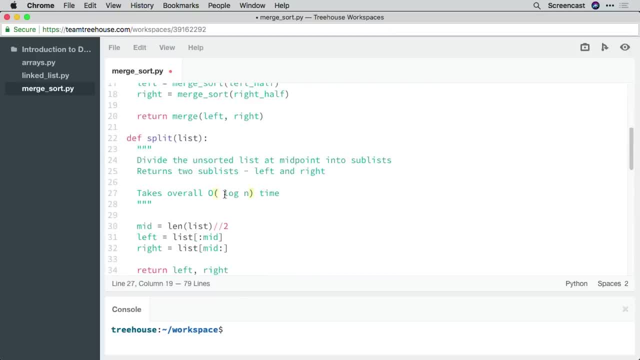 Now let's get rid of all that. To fix this, We need to remove this slicing operation. Now we can do that By using a technique We learned in a previous course. In the introduction to algorithms course, We looked at two versions of binary search in Python. 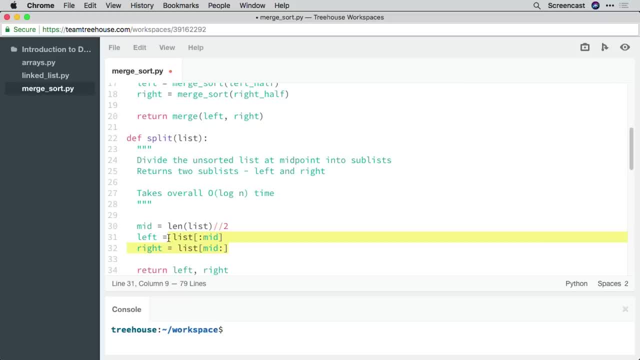 A recursive And an iterative version. In the recursive one We use list slicing with every recursion call, But we achieved the same end result Using an iterative approach Without using list slicing. Over there we declared two variables To keep track of the starting. 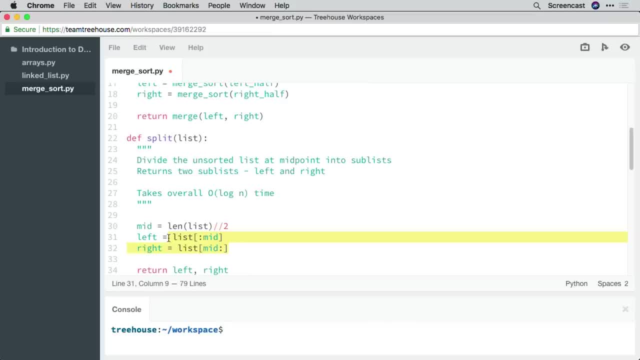 then say 2, 44, 15 and something like 200. okay, then we'll go ahead and print L so that we can inspect this list. next let's create a declare, a variable here. so we'll call this sorted linked list and to this we're going to assign. 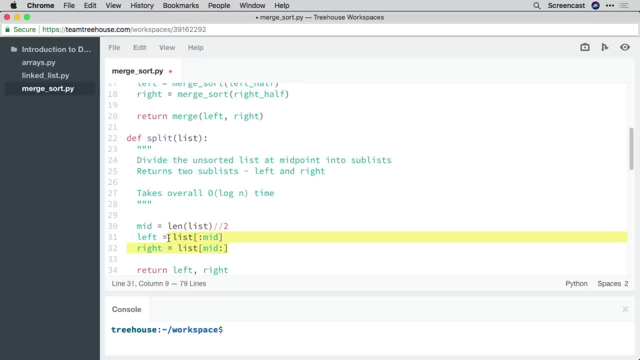 the result of calling merge: sort on L, and then we'll print this: so sorted linked list. okay, since we've taken care of all the logic, we know that this gets added in as nodes, and then let's see what this looks like. alright, so hit save and. 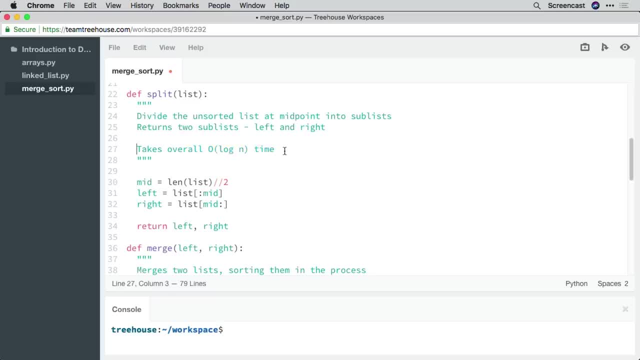 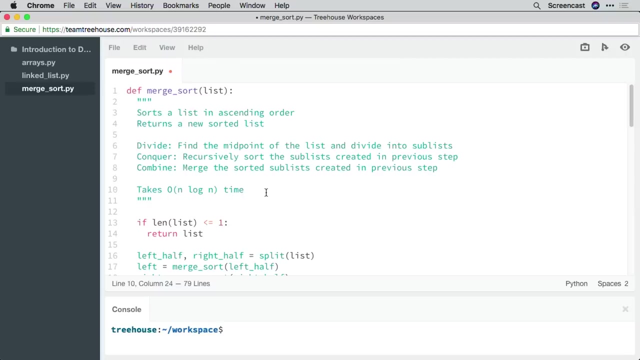 then bring up the console. we're gonna type out python: linked list, underscore, merge, sort, dot, pi and then enter okay, so we see that linked list we first created. remember that what we add first is right. that eventually becomes a tail. yeah, so 10 is the tail. 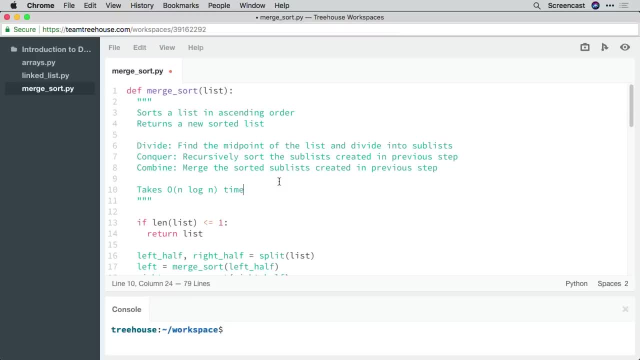 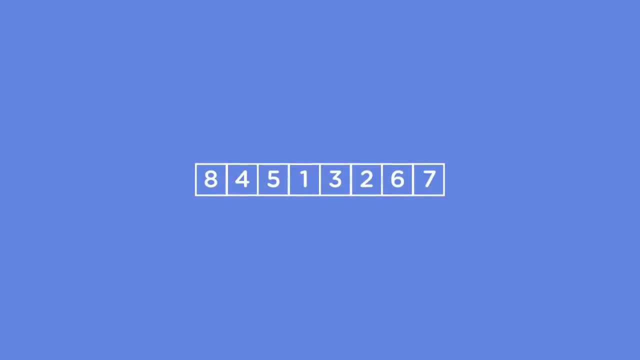 200 is the last one, so 200 is the head, because I'm calling add. it simply adds each one to the head of the list. so here we have 10, 2, 44, 15 and 200, in the order we added, and then the sorted linked list sorts it out. 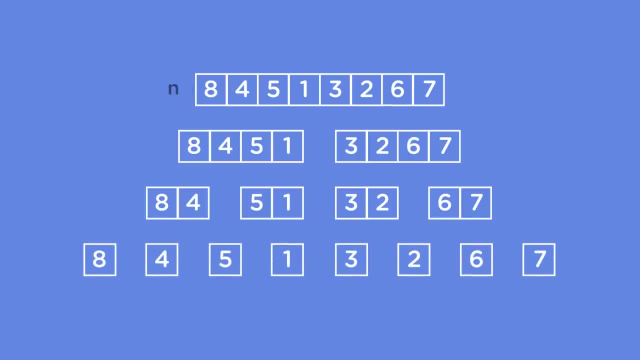 so it's 2, 10, 15, 44 and 200. look at that- a sorted linked list. okay, so let's visualize this from the top. we have a linked list containing 5 nodes with integers 10, 2, 44, 15 and 200. 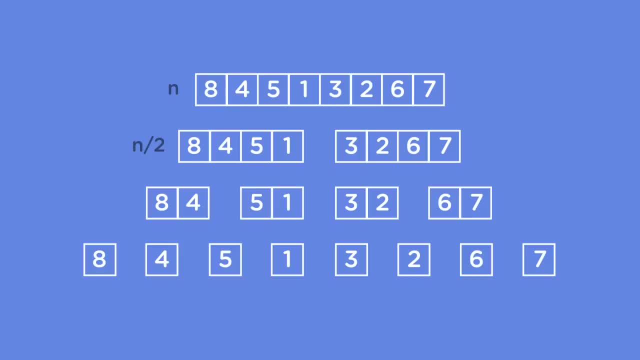 as data respectively. our merge sort function calls split on this list. the split function calls size on the list and gets back 5, which makes our midpoint 2. using this midpoint, we can split the list using the node at index method. remember that when doing this, we deduct. 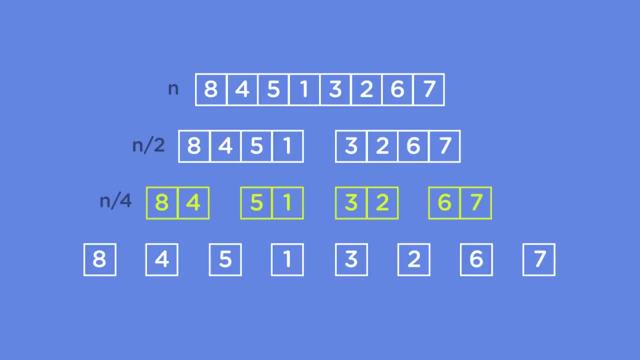 1 from the value of mid. so we're going to split here using an index value of 1. effectively, this is the same. since we're starting with an index value of 0. 1 means we split. after node 2, we assign the entire list to left. 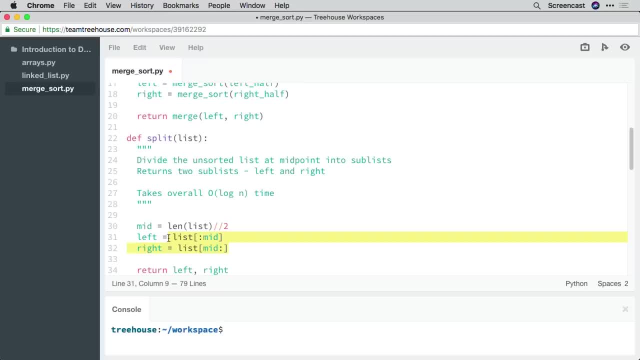 In the list. We could rewrite, merge, sort To do the same, But I'll leave that as an exercise for you. If you want some hints, If you want any direction, I've included a link in the notes With an implementation. 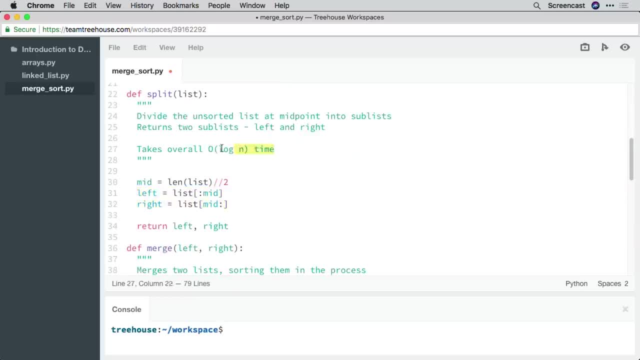 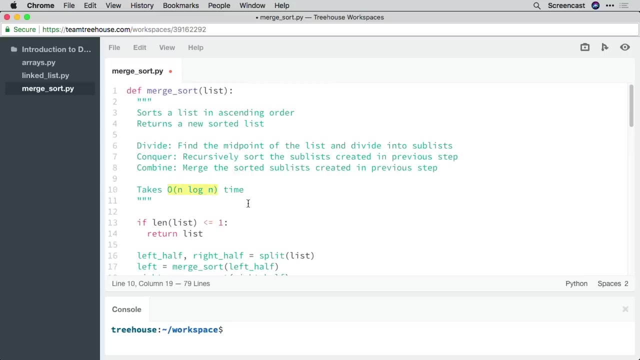 So that is time complexity. Now, just so we know Before moving on For Python here, Our overall run time Is not what I've listed here, But this is what the actual run time Takes: logarithmic time For an overall n times. log n. 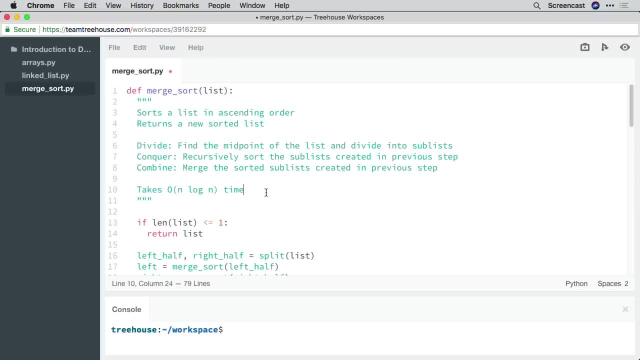 And that is how merge sort Actually works. Okay, so what about space complexity? The merge sort algorithm Takes linear space, And this is weird to think about at first, But as always, a visualization helps. So if we start at the top again, 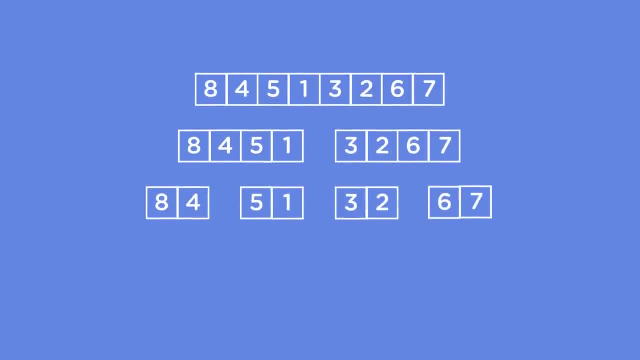 With our full list And carry out the split method Until we have single element lists. Each of these new lists Take up a certain amount of space. We have two lists Where each take up an n by two amount of space. Now this makes it seem: 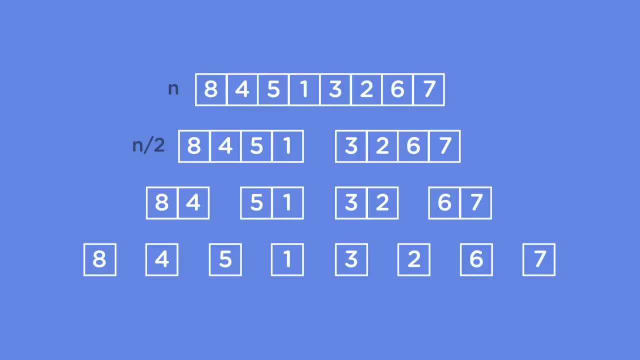 That the sum of all this space Is the additional space needed for merge sort, But that's not actually the case In reality. there are two factors that make a difference. First, Not every single one of these sub lists Are created simultaneously. 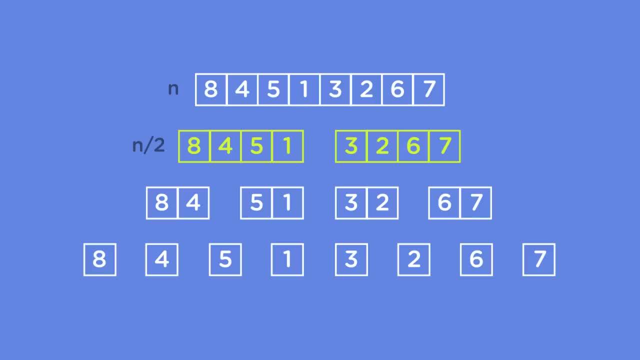 At step two, We create two n by two size sub lists. When we move to the next step, however, We don't hold on to the N by two sub lists. We can create four N by four size sub lists For the next split. 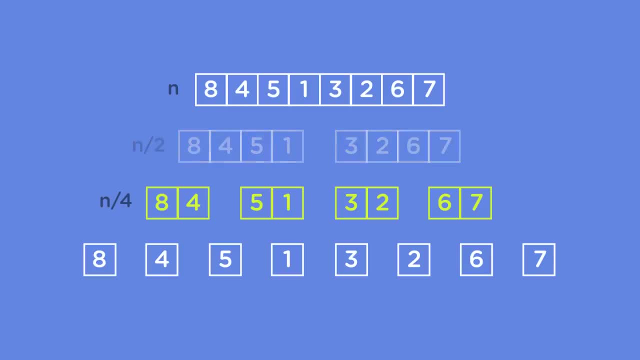 Instead, after the four N by four size sub lists are created, The n by two ones are deleted from memory. There's no reason to hold on to them any longer Now. the second point Is that our code doesn't execute Every path simultaneously. 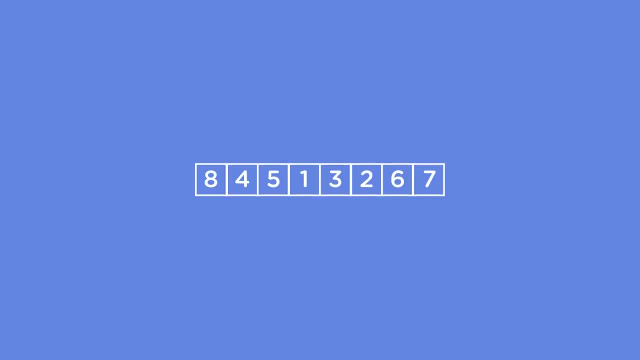 Think of it this way: When we pass our list to the Top level merge sort function, Our implementation calls split, Which returns A left half and a right half. The next line of code Then calls merge sort on the left half. 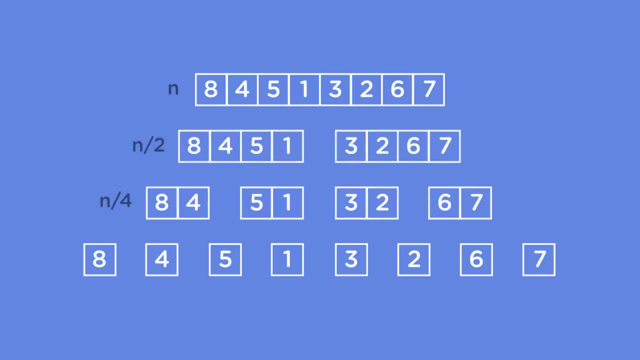 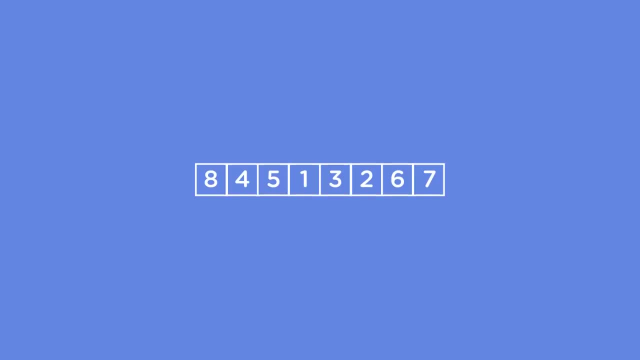 half, then create a new list and assign that to right half. we can assign node 3 at index value 2 as the head of the right list and remove the references between node 2 and node 3. so far so good, right, okay, so now we're back. 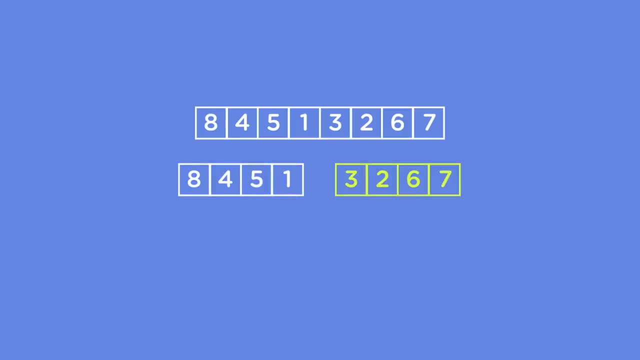 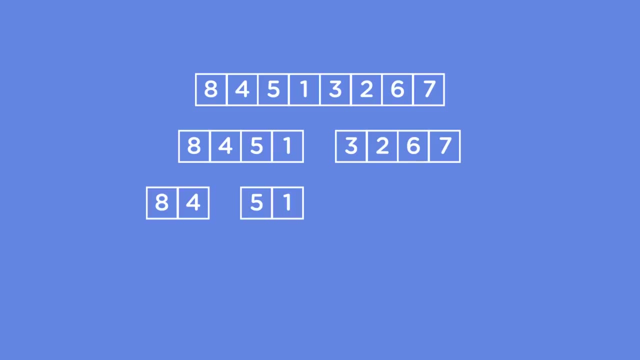 in the merge sort function after having called split and we have 2 linked lists. let's focus on just the left half because if you go back and look at our code we're going to call merge sort on the left linked list again. this means the next thing we'll do is run through that split. 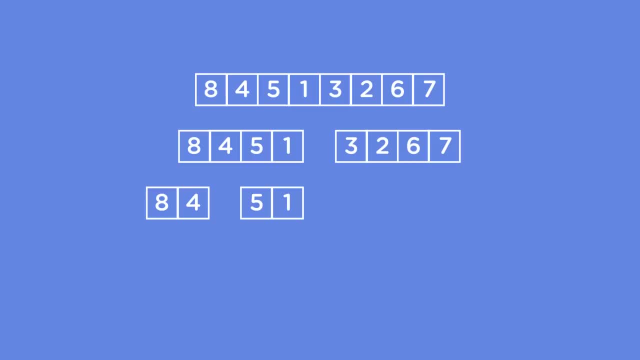 process. since this is a linked list containing 2 nodes, this means that split is going to return a new left and right list, each with 1 node. again we're back in the merge sort function, which means that we call merge sort on this left list again. 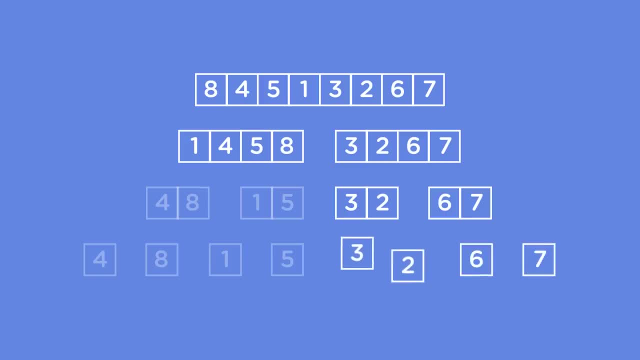 since this is a single node linked list on calling merge sort on it, we immediately return the list before we split, since we hit that stopping condition. so we go to the next line of code, which is calling merge sort on the right list as well, but again we'll get back immediately because 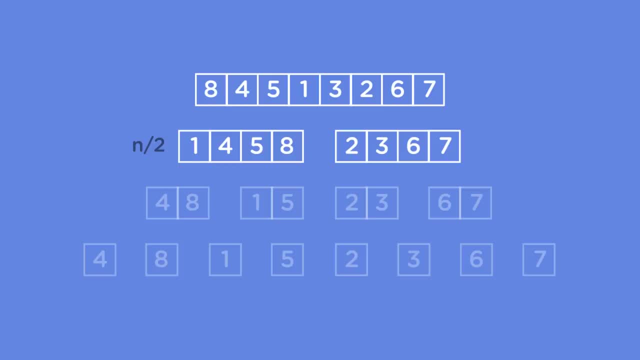 we hit that stopping condition. now that we have a left and right that we get back from calling merge sort, we can call merge on them inside the merge function. we start by creating a new linked list and attaching a fake head. then we evaluate whether either the left or the 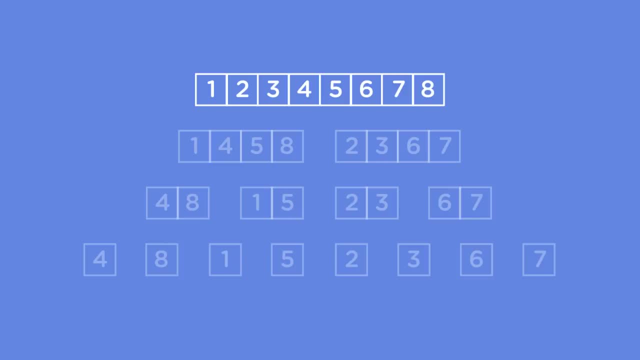 right head is none. since neither condition is true, we go to the final step where we evaluate the data in each node. in this case, the data in the right node is less than the left node, so we assign the right node as the next node in the merge linked list and move the right 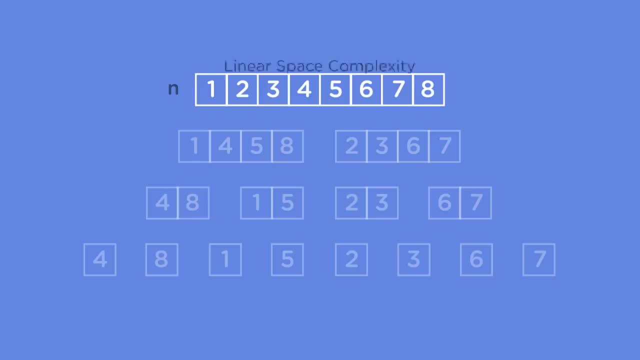 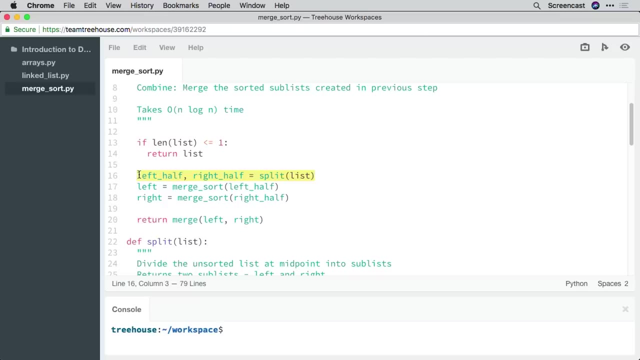 head pointer forward in the merge linked list, we move our current pointer forward to this new node we've added and that completes one iteration of the loop. on the next iteration, right head now points to none, since that was a single node list and we can assign the rest of the 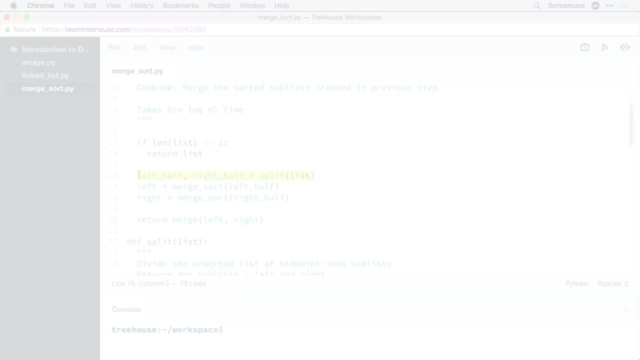 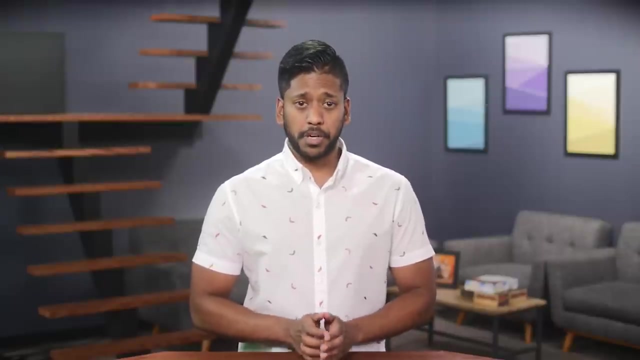 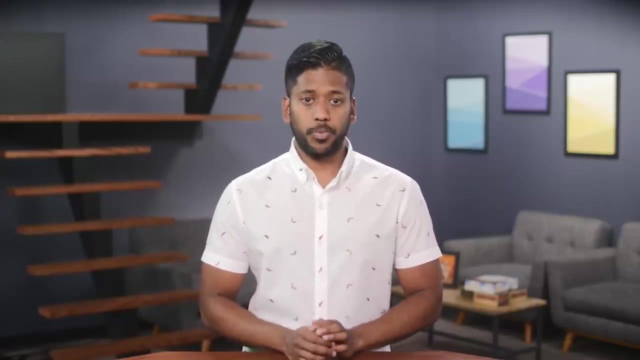 left linked list, which is effectively the single node, over to the merge linked list. here we discard the fake head, move the next node up to be the correct head and return the newly merged sorted linked list. remember that at this point because right head and left head pointed to: 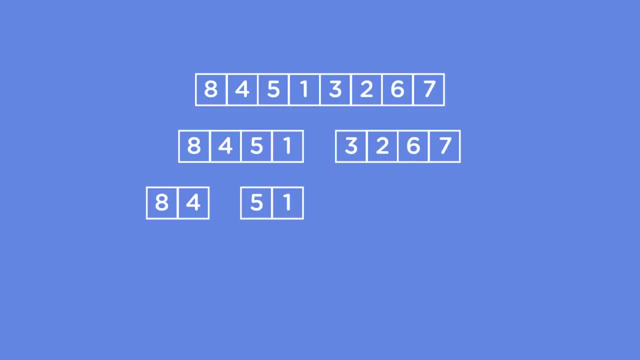 Again This runs the function, The merge sort function, again with a new list. In that second run of the function, Split is called again We get a second left and right half And then again, like before, We call merge sort on this left half as well. 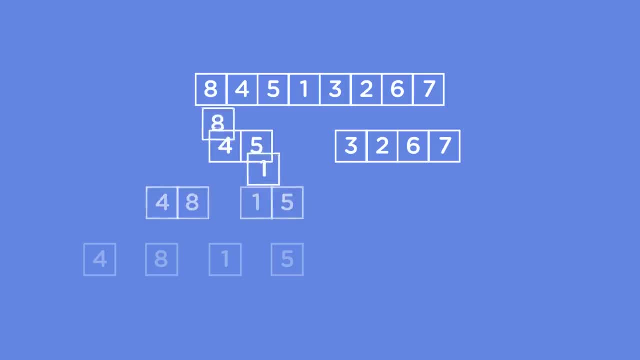 What this means Is that the code walks down the left path All the way down Until the initial left half is sorted And merged back into one array. Then it's going to walk all the way down the right path And sort that. 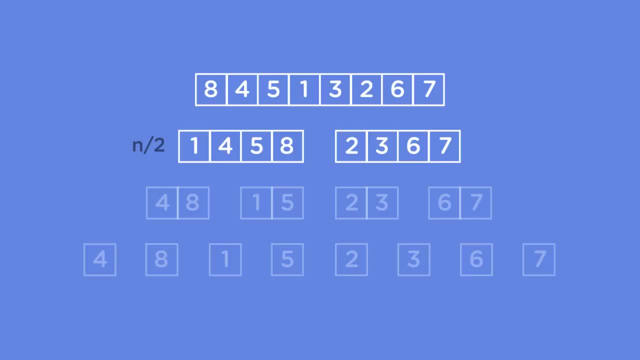 Until we're back to that first split With two n by two sized sub lists. Essentially, We don't run all of these paths of code at once, So the algorithm Doesn't need additional space for every sub list. In fact, It is the very last step that matters. 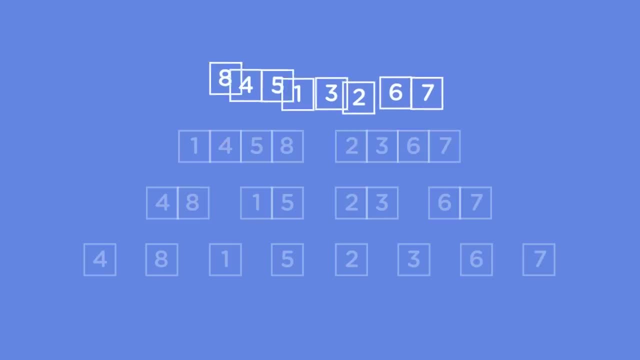 In the last step, The two sub lists are merged back Into the new sorted list And returned. That sorted list Has an equal number of items As the original unsorted list And since this is a new list, It means that at most, 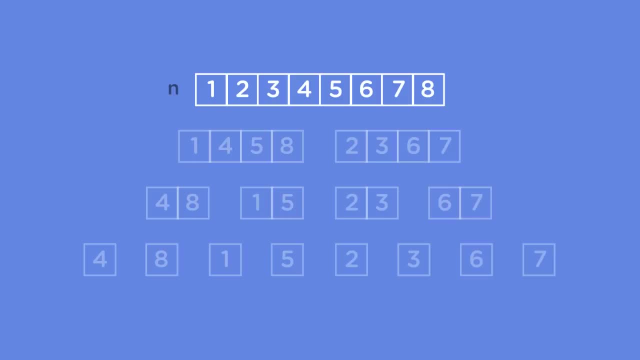 The additional space The algorithm will require at a given time Is n. Yes, at different points in the algorithm We require log n- amount of space, But log n is smaller than n, And so we consider the space complexity of merge sort. 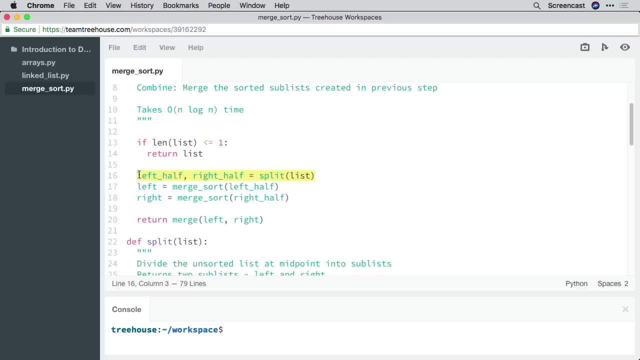 To be linear As the overall factor. Okay, that was a lot, So let's stop here. Don't worry if you've got questions about merge sort, Because we're not done yet. Over the next few videos, Let's wrap up this course. 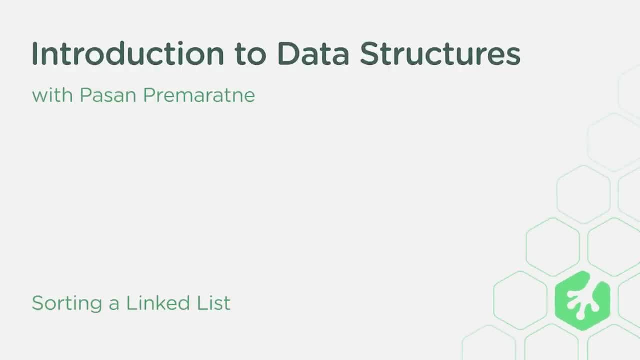 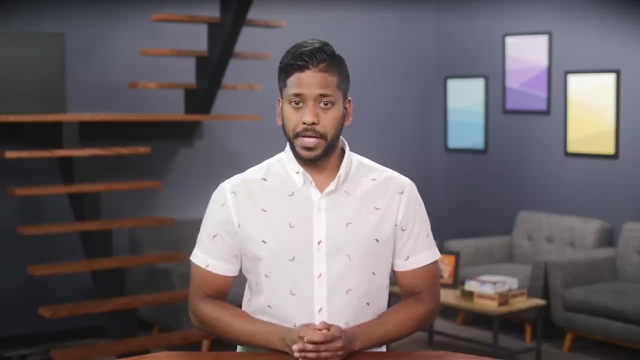 By implementing merge sort on a linked list. Over the last few videos We implemented the merge sort algorithm On the array or list type in python. Merge sort is probably The most complicated algorithm We've written so far. We learned about an important concept. 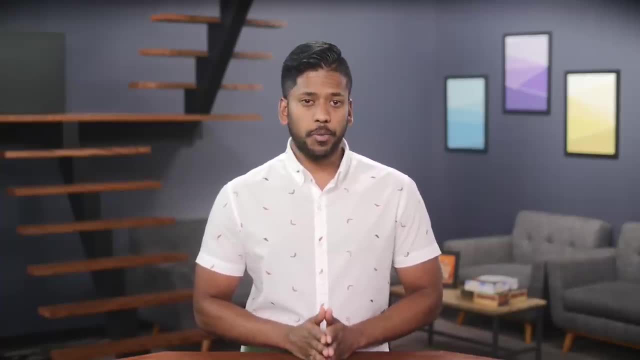 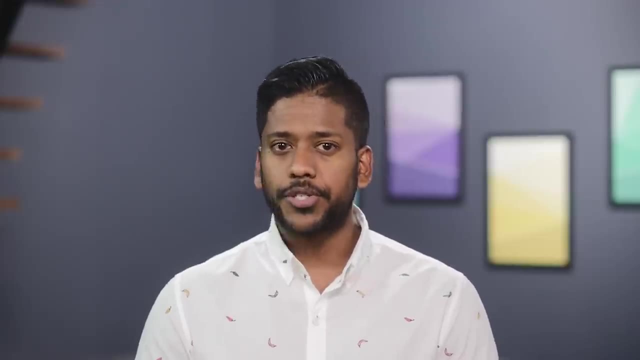 Divide and conquer. We also concluded the last video By figuring out the run time of merge sort Based on our implementation. Over the next few videos, We're going to implement merge sort again, This time on the linked list type. In doing so, we're going to get a chance. 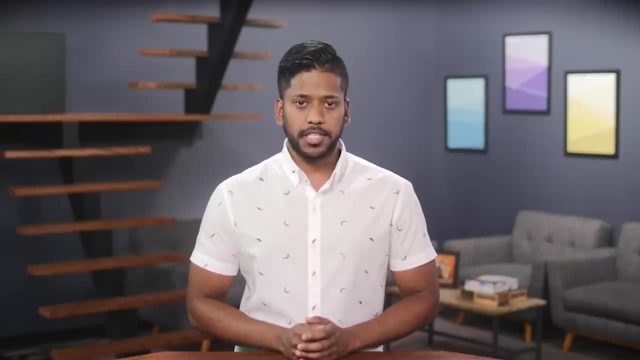 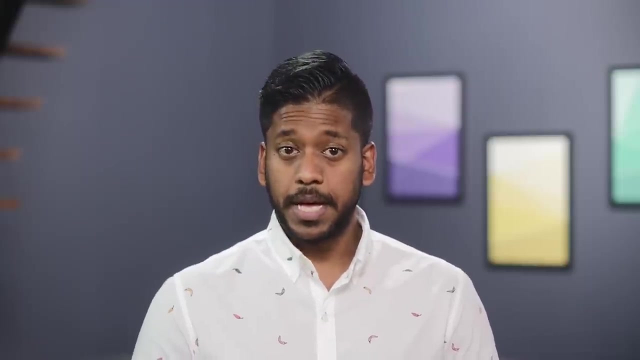 none are while loop terminated. so in this way we recursively split and repeatedly merge sublists until we're back with one sorted linked list. the merge sort algorithm is a power full sorting algorithm but ultimately it doesn't really do anything complicated, it just breaks the problem down until it's really simple to solve. 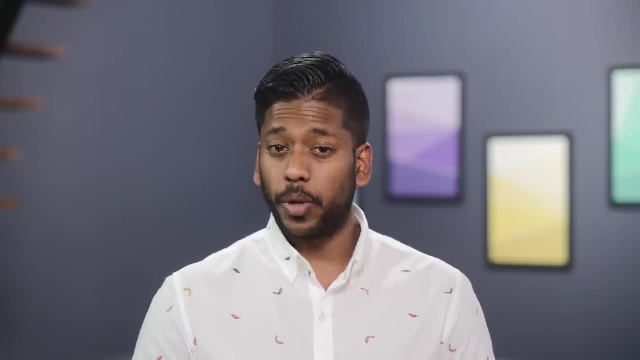 remember the technique here which we've talked about before, is called divide and conquer, so i like to think of merge sort in this way: there's a teacher at the front of the room and she has a bunch of books that she needs to sort into alphabetical order instead of. 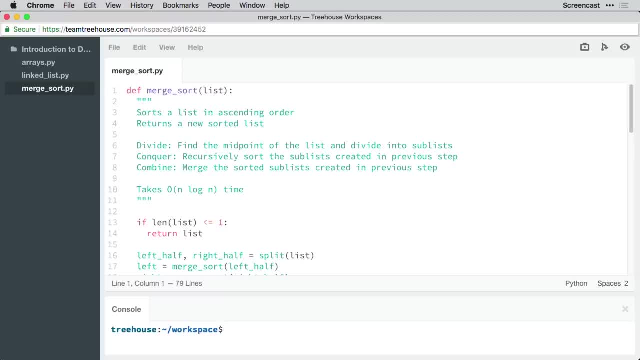 doing all that work herself. she splits that pile into two and hands it to two students at the front. each of those students split it into more and hand it to the four students seated behind them. as each student does this, eventually a bunch of single students has two books to compare and they can sort. 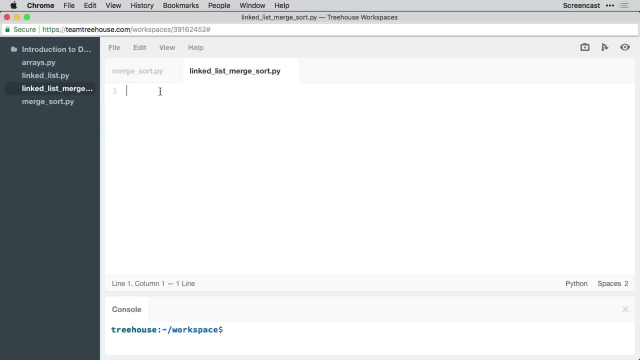 it very easily and hand it back to the student who gave it to them in front of them, who repeats the process backwards. so ultimately it's really simple work. it's just efficiently delegated. now back to our implementation. here let's talk about run time. so far other 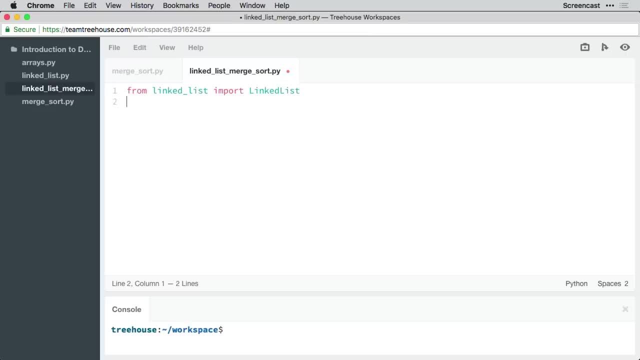 than the node swapping we had to do. it seems like most of our implementation is the same right. in fact it is including the problems that we ran into in the list version as well. so in the first implementation of merge sort, we thought we had an algorithm that ran in big O of. 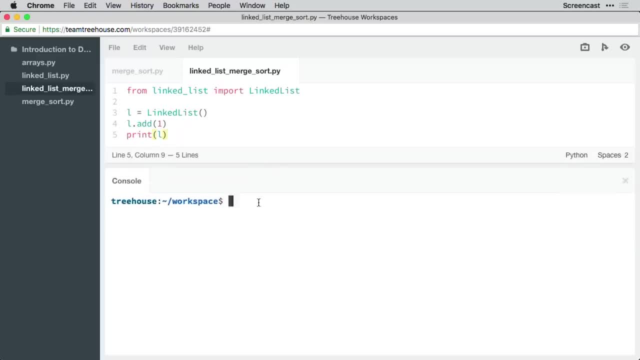 n, log n, but turns out we didn't why? well, the python list slicing operation, if you remember, actually takes up some amount of time amounting to big O of k. a true implementation of merge sort runs in quasi-linear or log-linear time, that is, n times. 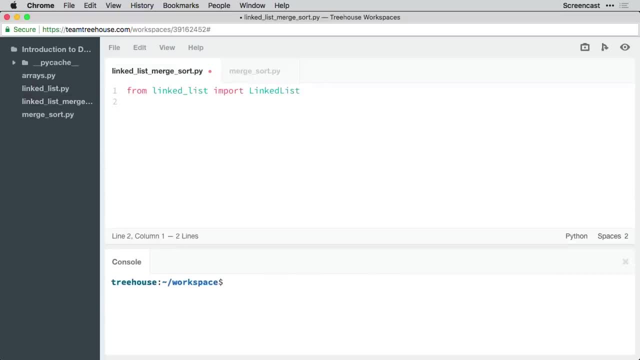 log n. so we almost got there, but we didn't. now, in our implementation of merge, sort on a linked list, we introduced the same problem. so if we go back up to the merge, or rather the split function, this is where it happens now, swapping node references. that's a constant time operation. no, 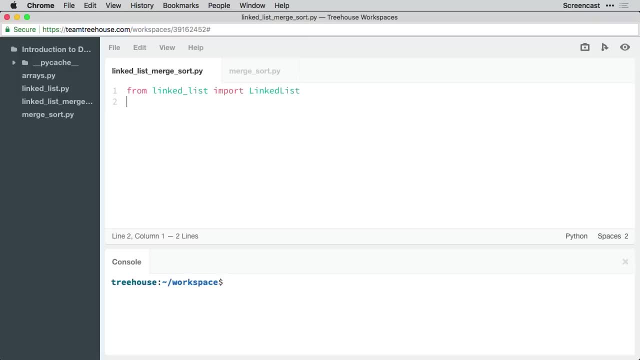 big deal comparing values, also constant time. the bottleneck here, like list slicing, is in splitting a linked list at the midpoint. if we go back to our implementation, you can see here that we use the node at index method, which finds the node we want by traversing the list. 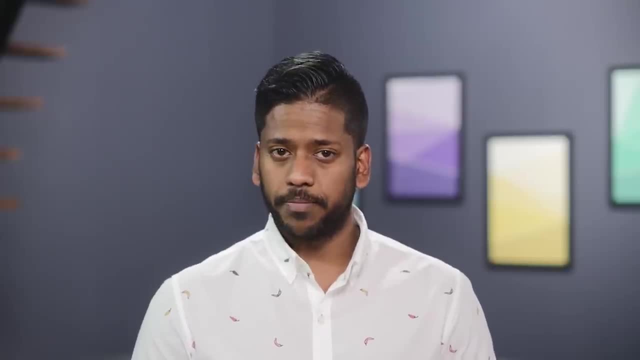 To see how the implementation differs Based on the data structure, While still keeping the fundamentals Of the algorithm the same, And we'll also see how the run time May be affected by the kinds of operations. Let's create a new file. 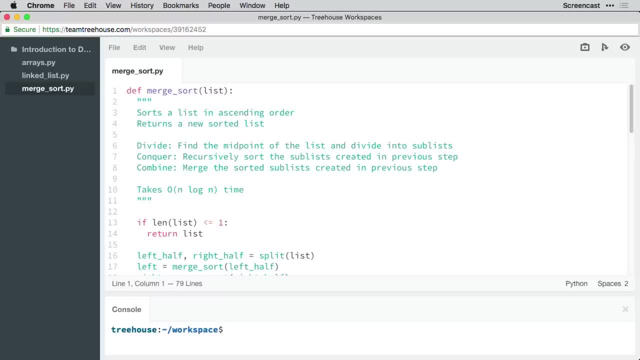 To put our second implementation Of merge sort in So file over here. New file And this is going to have a rather long name. We'll call this linked list merge sort With underscores everywhere, Dot pi. We're going to need the linked list class. 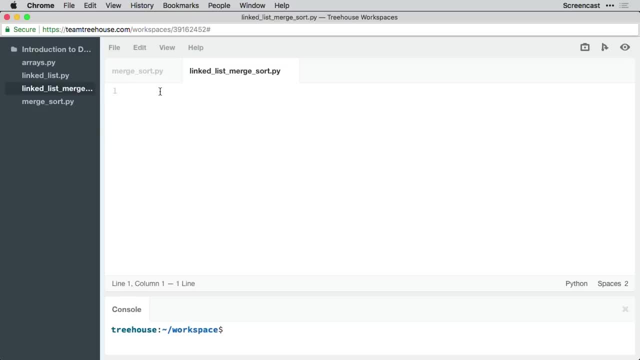 That we created earlier. So we'll start at the top By importing the linked list class From the linked list dot pi file. The way we do that. We'll say from linked List, Import, linked list, Right, so that imports the class. 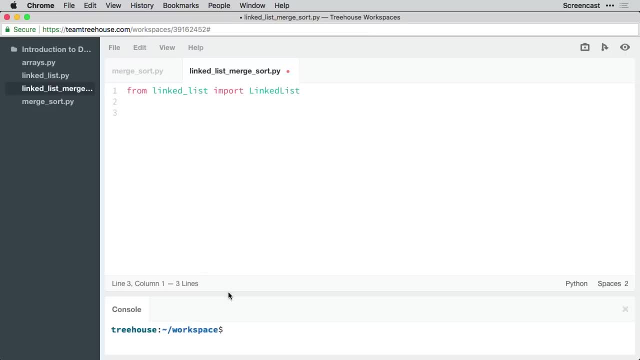 Let's test if this Works really quick. We'll just do something like L equal linked list, L dot add Ten, or one Doesn't matter, print l Okay, and if I hit save And then Down here we'll say python. 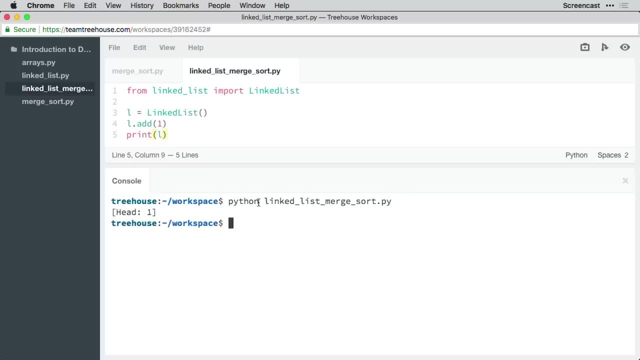 Linked list: Sort dot pi. Okay, it works. So this is how we get some of the code, How we reuse the code that we've written in other files Into this current file And get rid of this now. Okay, Like we did with the first implementation of merge sort. 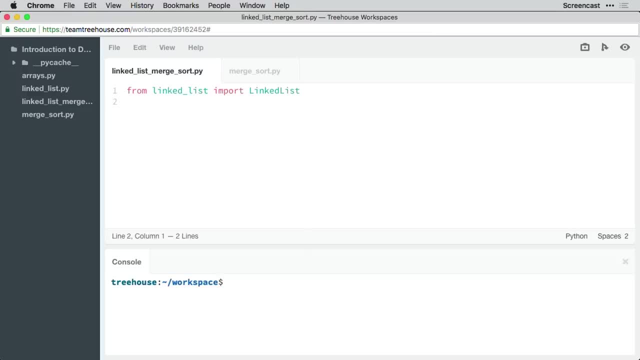 We're going to split the code up across three functions: The main function, merge sort, A split function And a merge function. Now, if you were to look up A merge sort implementation in python, Both for a regular list Or a linked list, 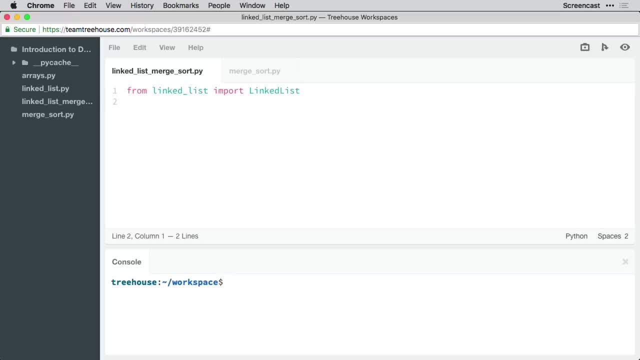 You would find much more concise versions out there, But they're kind of hard to explain, So splitting it up into three will sort of Help it, you know, Be easier to understand. We'll call this merge sort at the top level, And this time it's going to take a linked list. 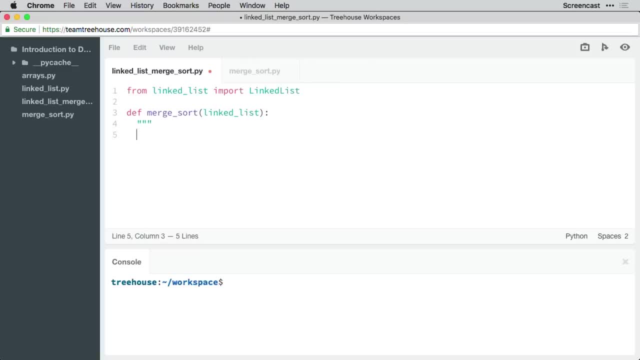 Let's add a doc string to document the function. So we'll say that this function sorts A linked list In ascending order And, like before, we'll add the steps in here. So we'll say: You first recursively Divide the linked list. 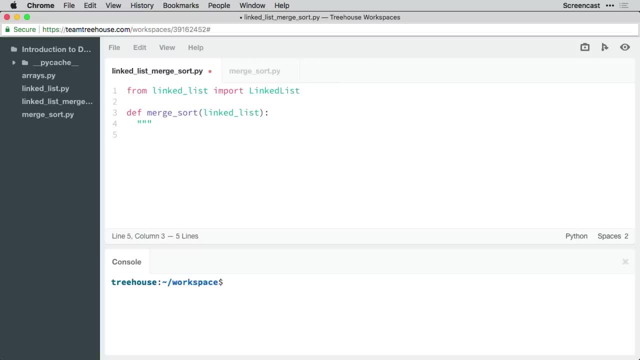 this means that every split operation incurs a big O of k cost, where k- here is the midpoint of the list- effectively n by 2, because we have to walk down the list, counting up the index, until we get to that node, given that overall splits take logarithmic time. 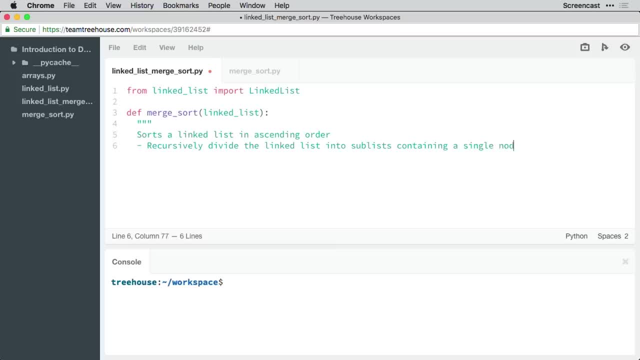 our split function, just like the one we wrote earlier, incurs a cost of big O of k log n. so here we'll say: it takes big O of k times log n. now the merge function, also like the one we wrote earlier, takes linear time. so that one is good, that one runs in the expected. 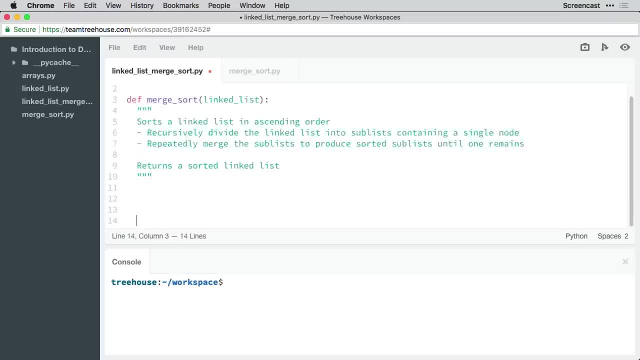 amount of time. so here we'll say it runs in linear time, and that would bring our overall run time so up at the merge sort function. we can say this runs in big O of k? n times log n. it's okay, though. this is a good start and one. 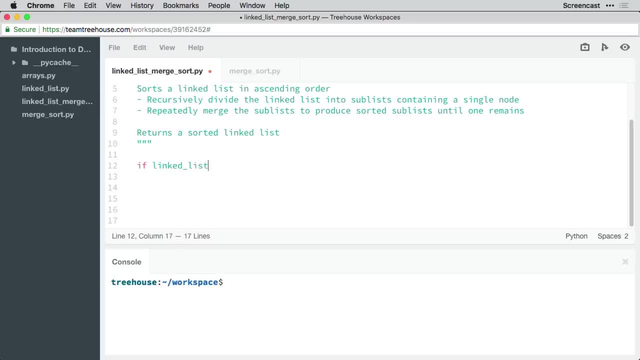 day when we talk about constant factors and look at ways we can reduce the cost of these operations using different strategies, we can come back and reevaluate our code to improve our implementation. for now, as long as you understand how merge sort works conceptually, what the run time and space complexities- 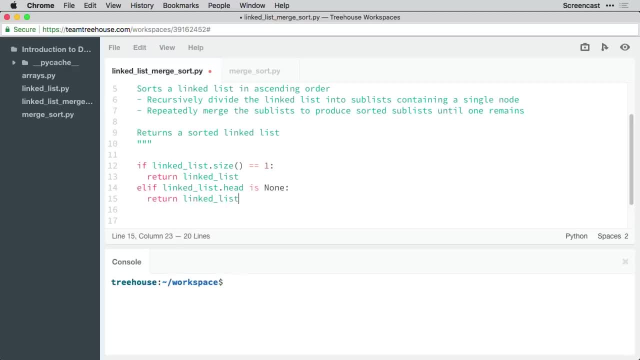 look like and where the bottlenecks are in your code. that's plenty of stuff. if you're interested in learning more about how we would solve this problem, check out the notes in the teachers video. in the next video, let's wrap this course up, and with that, let's wrap up this course. 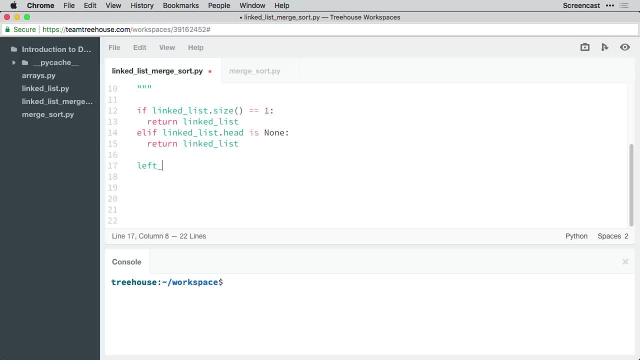 in the prerequisite to this course, introduction to algorithms, we learned about basic algorithms, along with some concepts like recursion and big O that set the foundation for learning about implementing and evaluating algorithms. in this course, we learned what a data structure is and how data structure go hand in hand with algorithms. 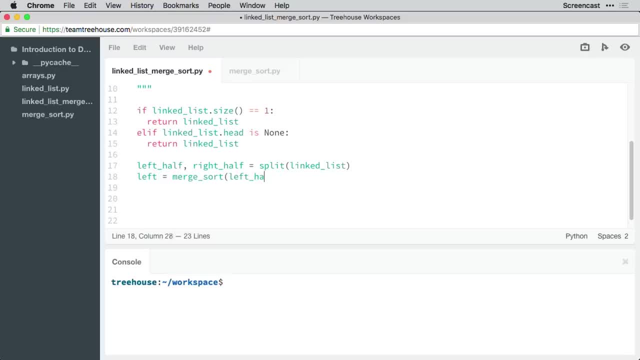 we started off by exploring a data structure that many of us use in our day to day programming: arrays, or lists as they are known in python. we took a peek under the hood at how arrays are created and stored, and examined some of the common operations carried out on arrays. 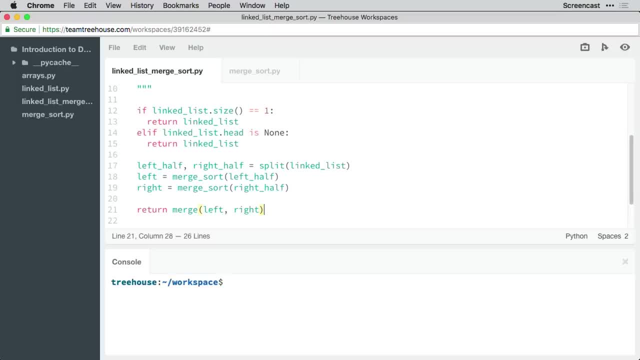 these are operations that we write and execute all the time, but here we took a step back and evaluated the run times of these operations and how they effect the performance of our code. after that we jumped into an entirely new world where we wrote our own data structure, a singly linked list. 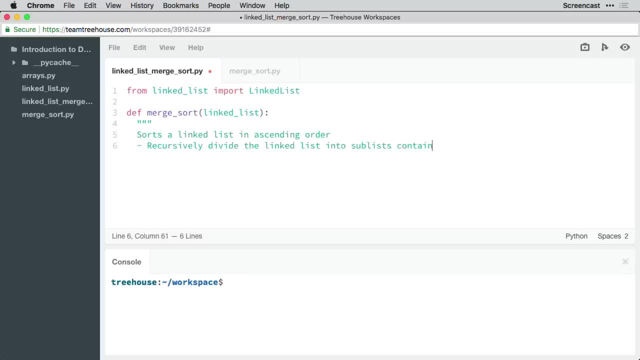 Into sub lists Containing A single node. Then We repeatedly Merge the sub lists To produce Sorted sub lists Until one remains And then, finally, This function returns A sorted, linked list. The implementation Of this top level merge function. 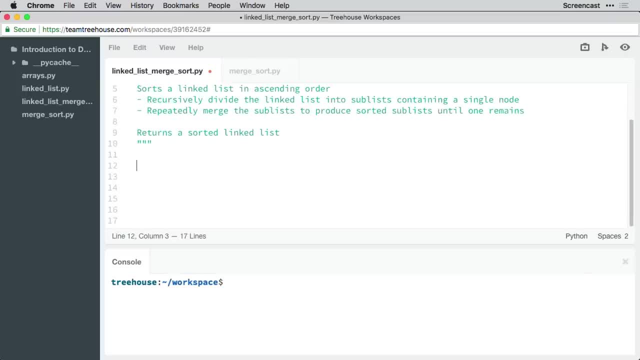 Is nearly identical To the array or list version We wrote earlier. So first we'll provide a stopping condition or two. If the size of the list is one Or it's an empty list, We'll return the linked list, Since it's naively sorted. 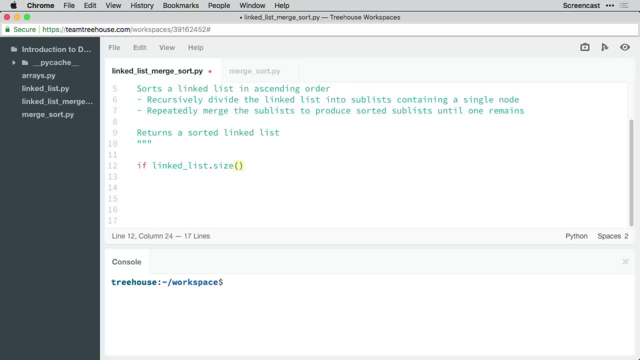 So if linked listsize- Remember that function we wrote- Equal one, Then we'll return Linked list. Else, if Linked listhead Is none Meaning, it's an empty list, Then we'll return linked list As well. Okay. 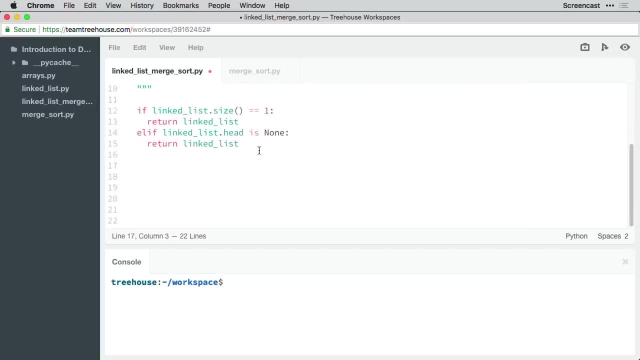 Next, let's split the linked list Into a left and right half. Conceptually this is no different, But in practice We need to actually traverse the list. We'll implement a helper method To make this easier. So, left Equal split- linked list. 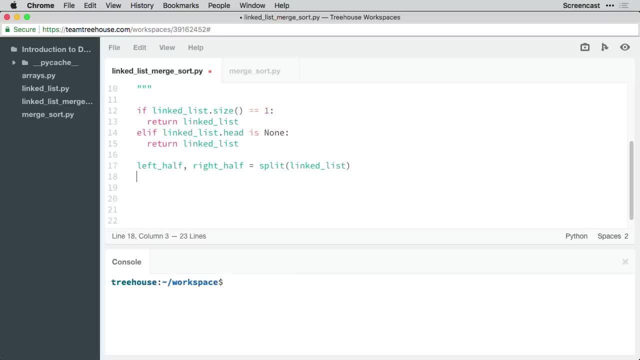 Now, once we have two sub lists, Like before, We can call merge sort, The top level function On each. So left equal merge sort, Left half And right Equal merge sort On the right half. Finally, We'll merge these two top level sub lists. 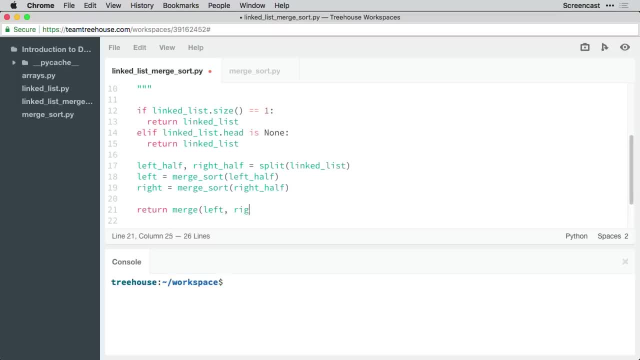 And return it. So merge left and right. Okay, Nothing new here, But in the next video Let's implement the split logic. The next step in the merge sort algorithm Is the divide step, Or rather An implementation of the split function. 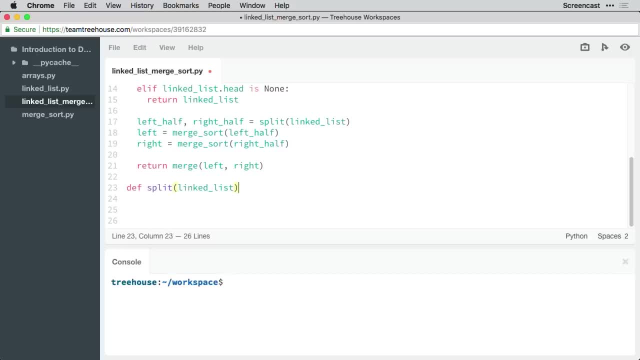 So down here We'll call this split Like before, And this is going to take a linked list. Documenting things is good, So we'll divide The unsorted list At midpoint Into sub lists. Now, of course, When I say sub lists here, 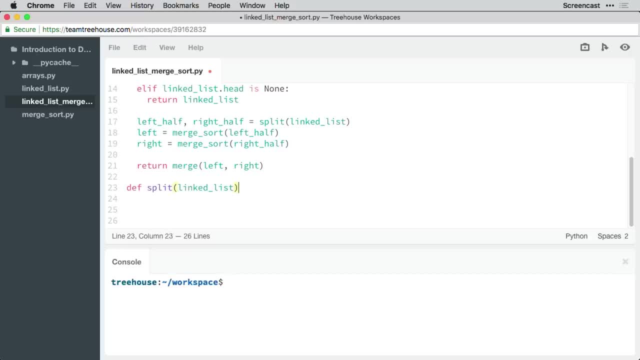 admittedly, linked lists aren't used much in day to day problem solving, but it is a good data structure to start off with because it is fairly straight forward to understand and not that much different from an array. we carried out the same exercise as we did on arrays. 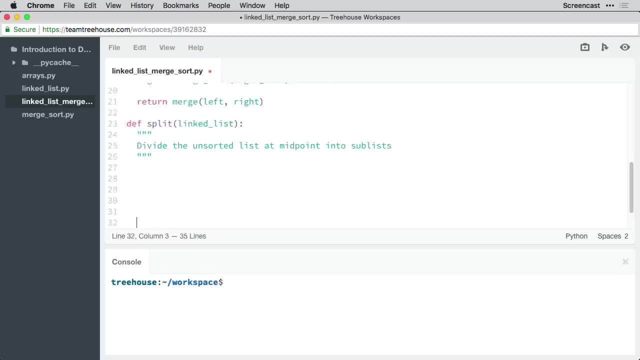 in that we looked at common data operations, but since this was a type we defined on our own, we implemented these operations ourselves and got to examine, with a fine tooth comb, how our code and the structure of the type effected the run time of these operations. the next: 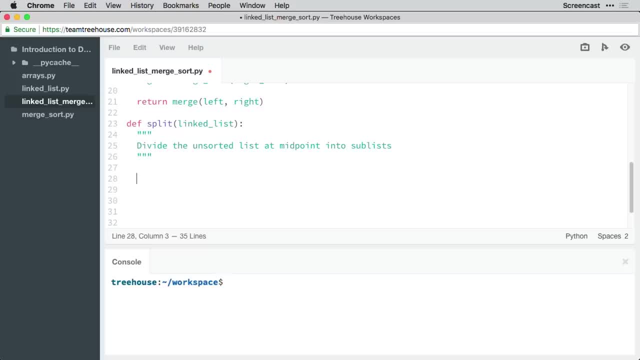 topic we tackled was essentially worlds colliding. we implemented a sorting algorithm to sort two different data structures. here we got to see how all of the concepts we've learned so far- algorithmic thinking, time and space, complexity and data structures- all come together to tackle the problem of 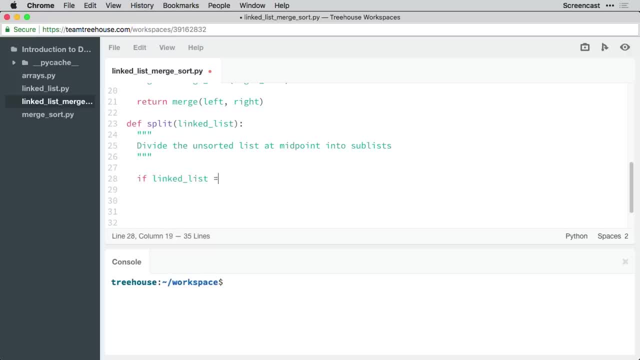 sorting data. this kind of exercise is one we're going to focus on moving forward as we try to solve more real world programming problems using different data structures and algorithms. if you stuck with this content so far, keep up the great work. this can be a complex topic, but a really interesting one. 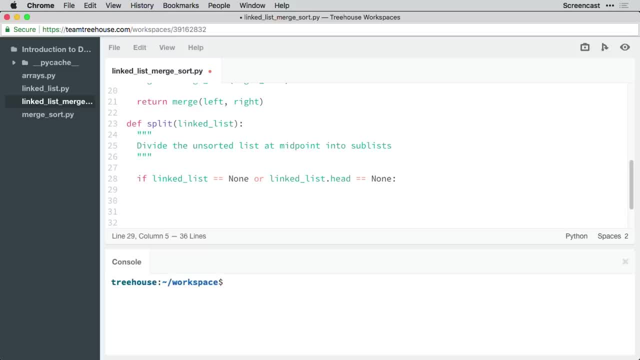 and if you take your time with it, you will get a deeper understanding of programming and problem solving. as always, check the notes for more resources and happy coding. you may have heard that algorithms and computer science are boring or frustrating. they certainly can be hard to figure out, especially the way 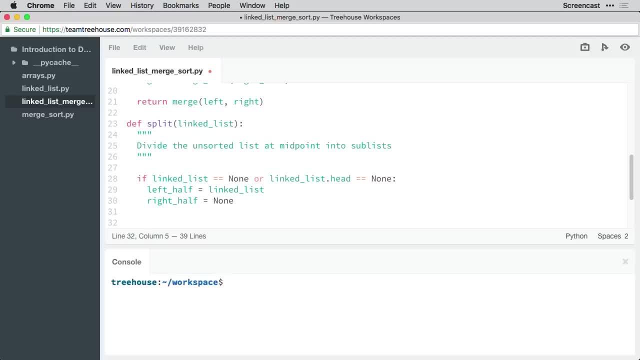 some textbooks explain them, but once you understand what's going on, algorithms can seem fascinating, clever or even magical. to help further your understanding of algorithms, this course is going to look at two categories: sorting algorithms and searching algorithms. you could argue that these are the easiest kinds of algorithms to learn, but in the 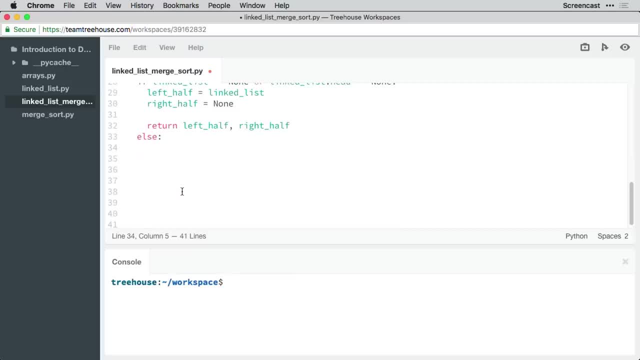 learning how these algorithms are designed. we'll cover useful concepts like recursion and divide and conquer that are used in many other sorts of algorithms and can even be used to create brand new ones. by the way, all the code samples i'm going to show in the videos will be in: 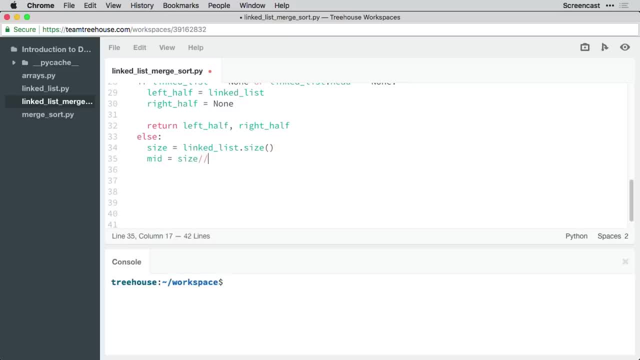 python because it's a popular language that's relatively easy to read. but you don't need to know python to benefit from this course. you can see the teacher's notes for each video for info on implementing these algorithms in your own favorite language. our goal with this course is to give you 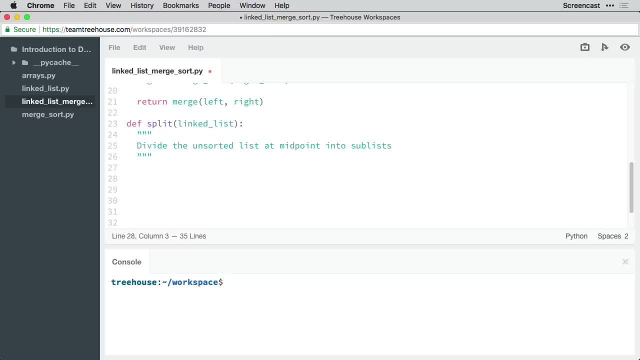 I mean sub linked lists, But that's a long word to say. Now, here's where things start to deviate From the previous version. With the list type, We could rely on the fact That finding the midpoint Using an index. 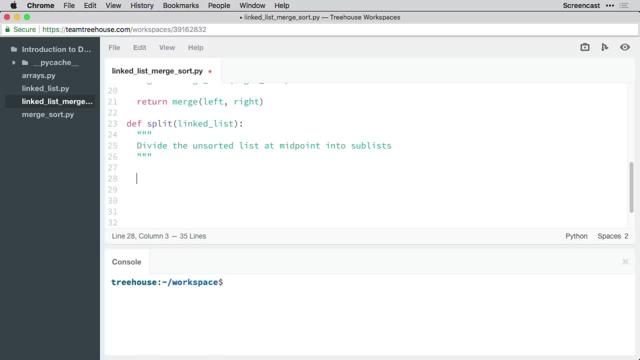 Since we have no automatic behavior Like that, We need to account for this When using a linked list. So our first condition Is if the linked list is none Or if it's empty, That is, if head is equal to none. 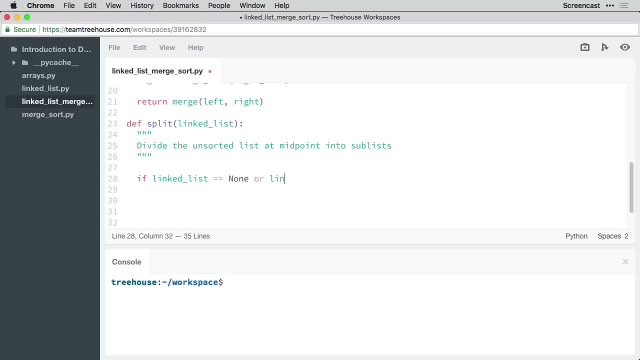 So we'll say: if linked list Equal none, Or you can write: is there Doesn't matter, Or linked listhead is none. Well, linked list can be none. For example, A split on such a list Would mean left would contain the single node. 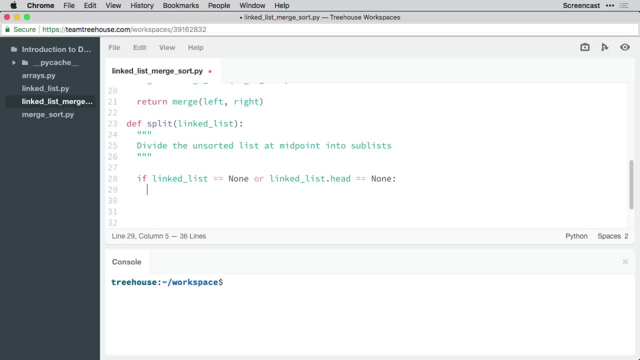 While right would be none. Now, in either case, We're going to assign the entire list To the left half And assign none to the right. So we'll say: left half Equal linked list And then right half Equal none. 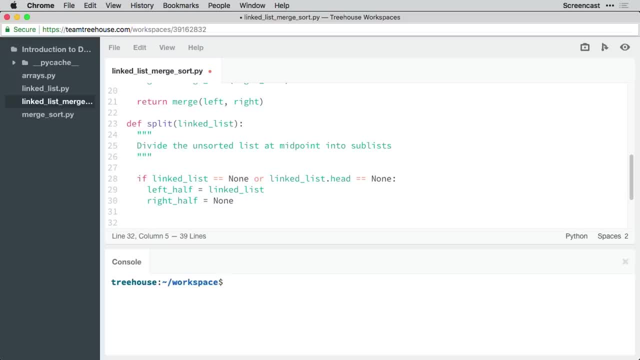 You could also assign the single element list, Or none, to left And then create a new empty linked list Assigned to the right half. That's unnecessary work. So now that we've done this, We can return Left half And right half. 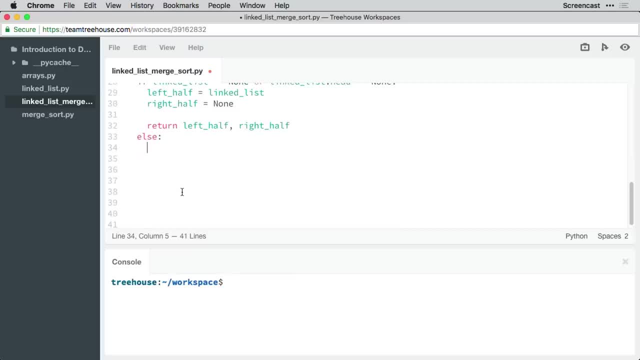 So that's our first condition. Let's add an else clause To account for non empty linked lists. First we'll calculate the size of the list. Now this is easy Because we've done the work already And we can just call the size method. 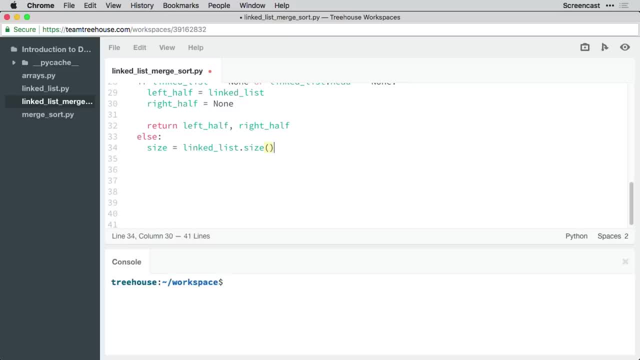 That we've defined. We'll say: size equal. Using the size We can determine the midpoint. So mid equal size, And here we'll use that floor division operator To divide it by two. Once we have the midpoint, We need to get the node at that midpoint. 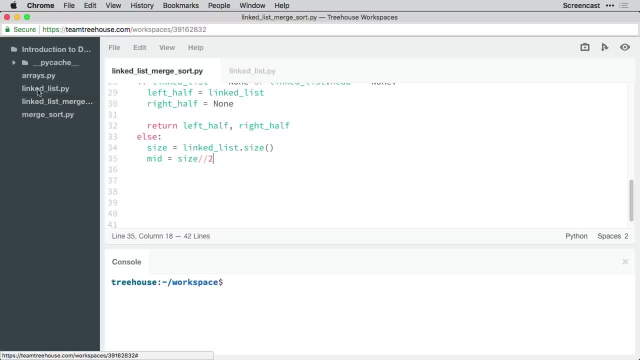 Now make sure you hit command s to save here And we're going to navigate back to Linked list. dot pi. In here We're going to add a convenience method At the very bottom, Right before the repper function, Right here. 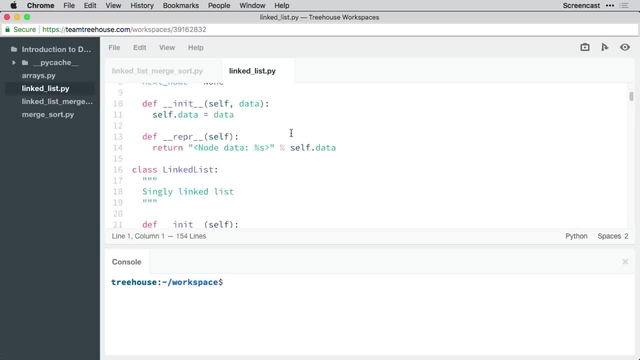 an overview of how sorting and searching algorithms work, but many algorithms have details that can be handled in different ways. some of these details may distract from the big picture, so we put them in the teacher's notes instead. you don't need to worry about these when completing the course for the first time. 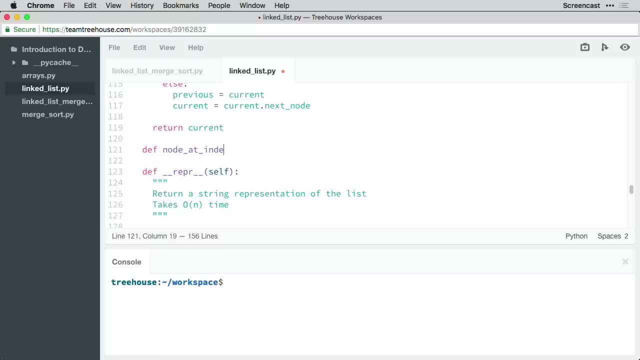 but if you're going back and referring to it later, be sure to check the teacher's notes for additional info. suppose we have a list of names. it's a pretty big list, a hundred thousand names long. this list could be part of an address book or social media app. 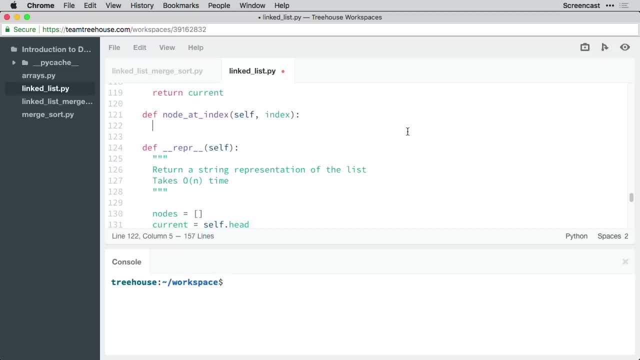 and we need to find the locations of individual names within the list, possibly to look up additional data that's connected to the name. let's assume there's no existing function in our programming language to do this or that the existing function doesn't suit our purpose in some way. 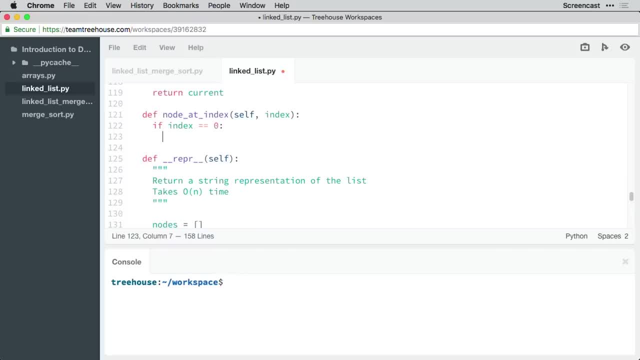 for an unsorted list. our only option may be to use linear search, also known as sequential search. linear search is covered in more detail elsewhere on our site. check the teacher's notes for a link. if you want more details. you start at the first element, you compare it to the value you're searching. 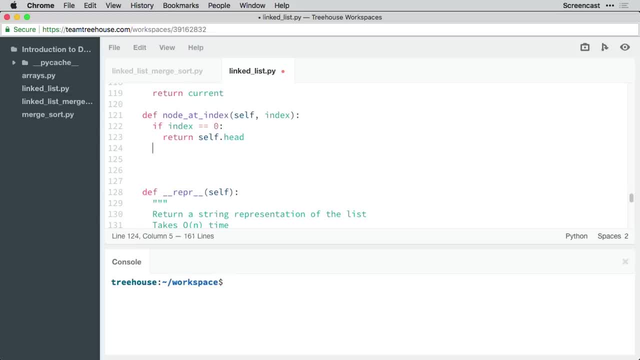 for if it's a, If it's a match, you return it. If not, you go to the next element. You compare that to your target. If it's a match, you return it, If not, you go to the next element. 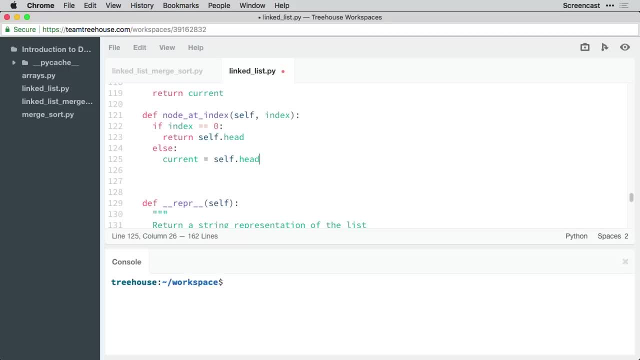 And so on through the whole list. The problem with this is that you have to search the entire list every single time. We're not doing anything to narrow down the search. each time We have to search all of it If you're searching a big list or searching it repeatedly. 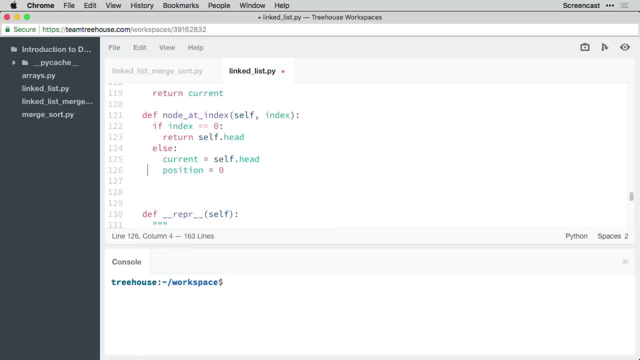 this amount of time can slow your whole lap down to the point that people may not want to use it anymore. That's why it's much more common to use a different algorithm for searching lists: binary search. Binary search is also covered in more detail elsewhere on our site. 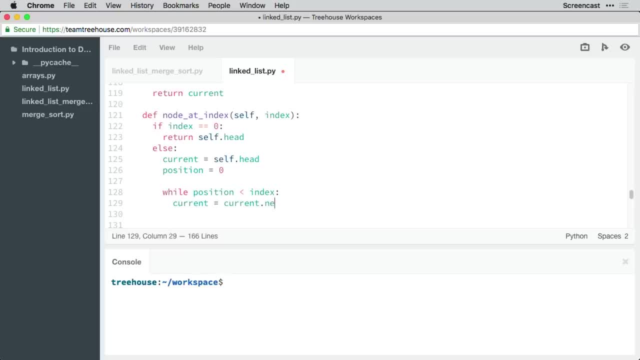 Check the teacher's notes for a link. Binary search does narrow the search down for us. Specifically, it lets us get rid of half the remaining items we need to search through each time. It does this by requiring that the list of values be sorted. 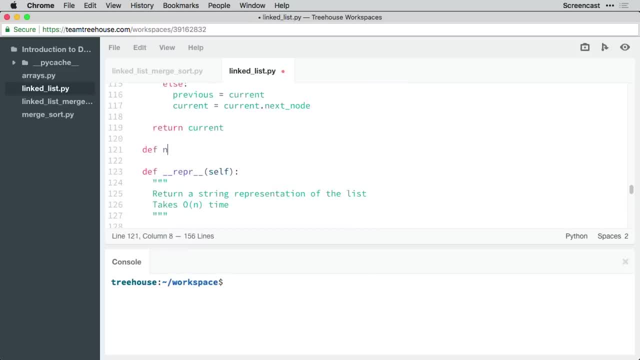 We're going to return a node At a given index, So we'll call this node At index And it's going to take an index value. This way, Instead of having to traverse the list Inside of our split function, We can simply call node at index. 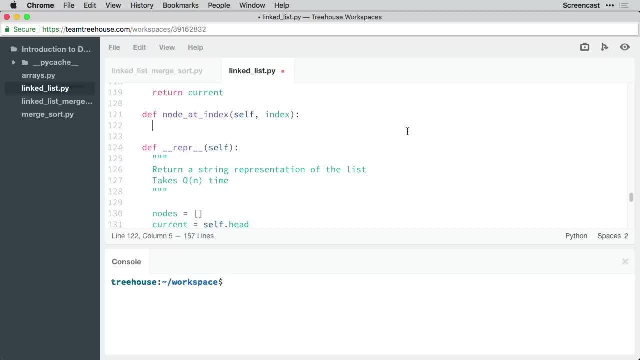 And pass it the midpoint index we calculated To give us the node right there, So we can perform the split. Okay, so this method accepts as an argument The index we want to get the node for. If this index is zero, We'll return the head of the list. 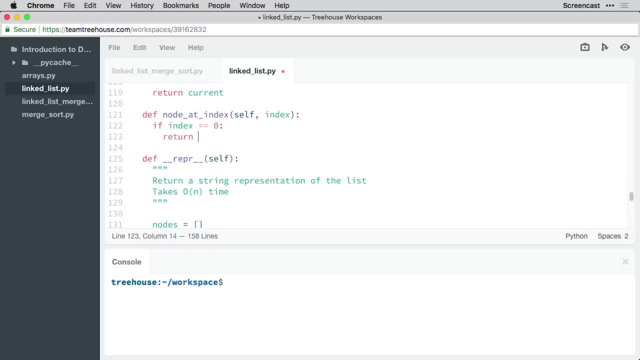 So if Index double equals zero Return, self dot head. The rest of the implementation Involves traversing the linked list And counting up to the index As we visit each node. The rest of the implementation Involves traversing the linked list. 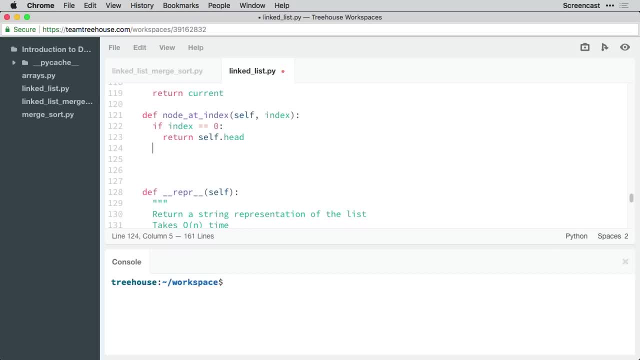 And counting up to the index As we visit each node. So I'll add an else clause here And we'll start at the head Equal self dot head. Let's also declare a variable Called position To indicate where we are. 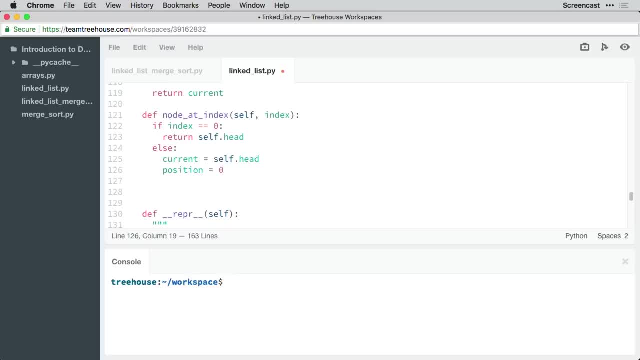 In the list. We can use a while loop to walk down the list. Our condition here Is as long as the position Is less than the index value. So I'll say, While position Is less than index, Inside the loop. 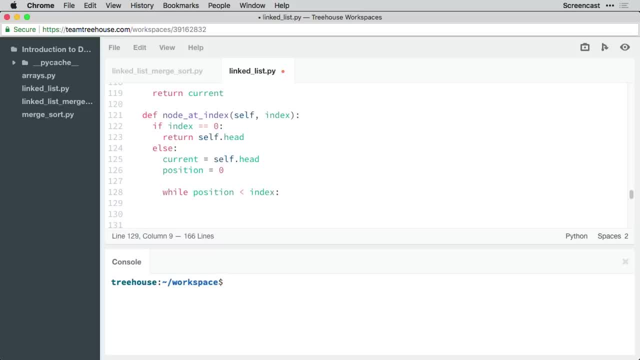 We'll assign the next node to current And increment the value of position By one. So current equal current, dot. next node: Position Plus equal one. Once the position value Equals the index value, Current refers to the node we're looking for. 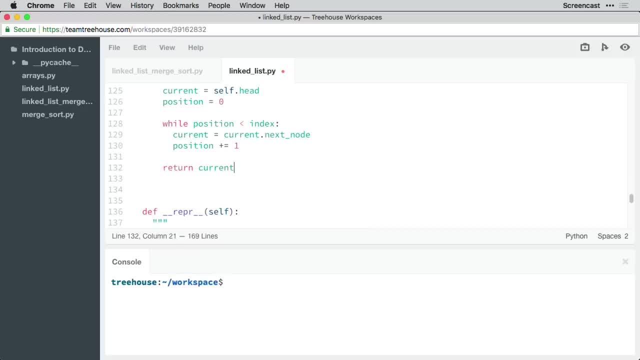 And we can return it. We'll say: return current. Let's get rid of all this Empty space. There we go Now back in linked list: merge sort Dot pi. We'll use this method To get at the node After we've calculated the midpoint. 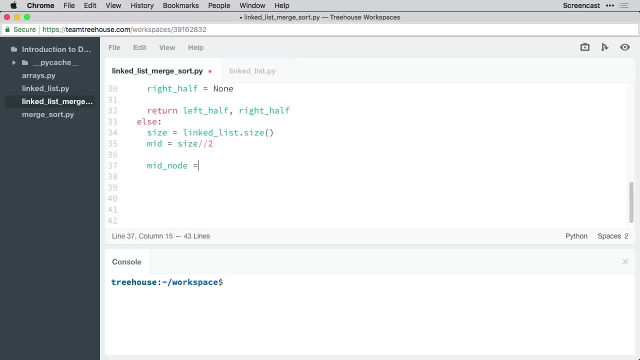 To get the node at the midpoint of the list. So we'll say mid node, Equal Linked list, Dot node at index. And here I'm going to do something Slightly confusing. I'm going to do mid minus one. Remember, we're subtracting one here. 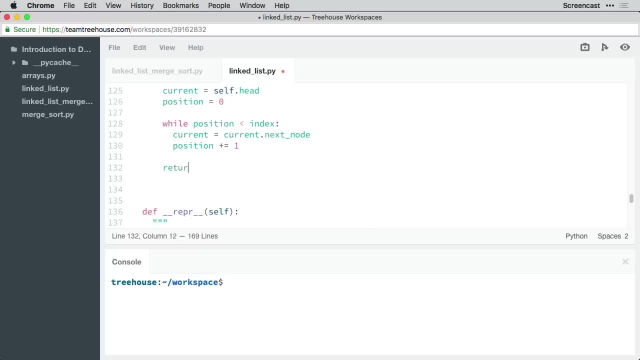 It looks at the value in the middle of the list. If the value it finds is greater than the target value, it ignores all values after the value it's looking at. If the value it finds is less than the target value, it ignores all values before the value it's looking at. 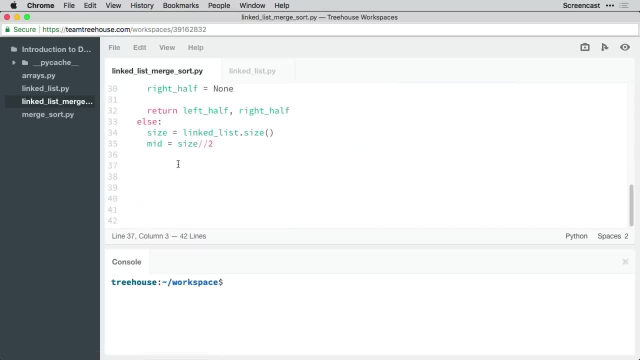 Then it takes the set of values that remain and looks at the value in the middle of that list. Again, if the value it finds is greater than the target value, it ignores all values after the value it's looking at. If the value it finds is less than the target value, 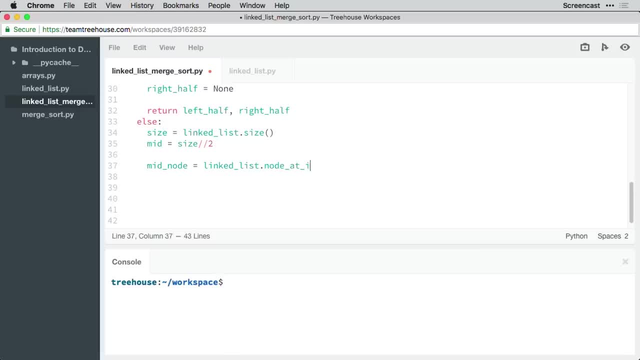 it ignores all values before the value it's looking at. But, as we mentioned, binary search requires the list of values you're searching through to be sorted. If the list weren't sorted, you would have no idea which half of the values to ignore. 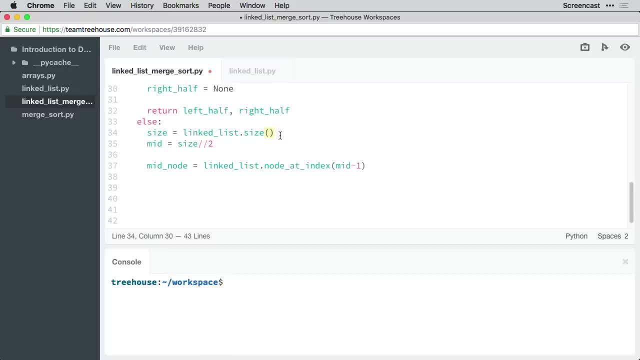 because either half could contain the value you're looking for. You'd have no choice but to use linear search. So before we can use binary search on a list, we need to be able to sort that list. We'll look at how to do that next. 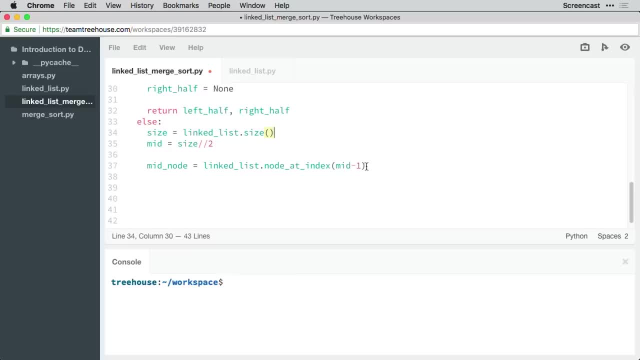 Our end goal is to sort a list of names, but comparing numbers is a little easier than comparing strings, so we're going to start by sorting a list of numbers. I'll show you how to modify our examples to sort strings at the end of the course. 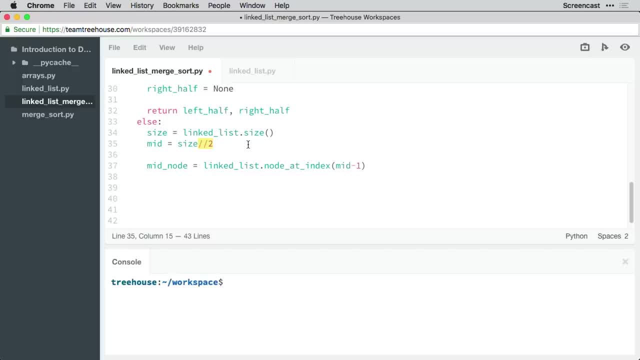 To help make clear the importance of choosing a good sorting algorithm, we're going to start with a bad one. It's called bogosort. Basically, bogosort just randomizes the order of the list repeatedly until it's sorted. Here's a Python code file where we're going to implement bogosort. 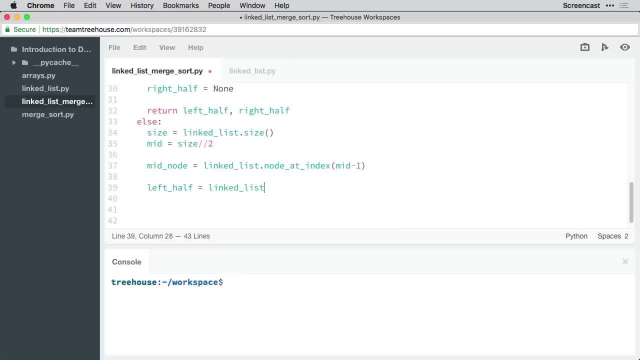 It's not important to understand this code here at the top, although we'll have info on it in the teacher's notes if you really want it. All you need to know is that it takes the name of a file that we pass on the command line. 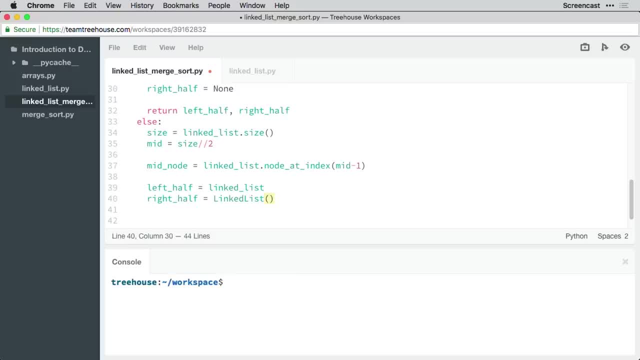 loads it and returns a Python list, which is just like an array in other languages, containing all the numbers that it read from the file. Let me have the program print out the list of numbers it loads so you can see it. We'll call the print method and we'll pass it the list of numbers. 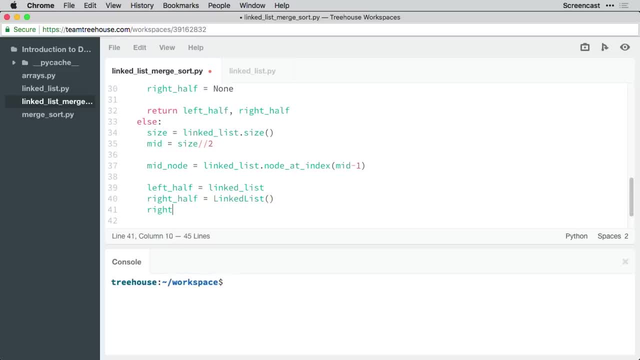 Save that. Let's run it real quick with python bogosortpy. Oh whoops. And we need to provide it the name of the file here on the command line that we're going to load. So it's in the numbers directory. 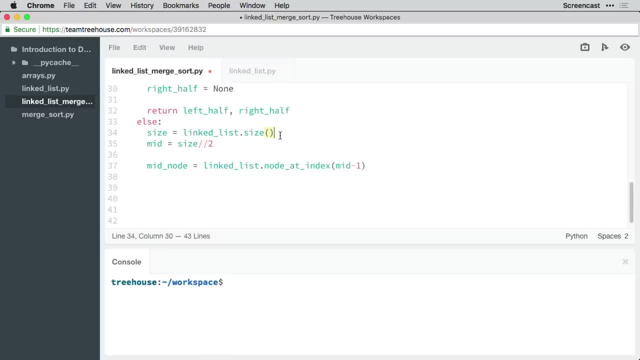 Because we used size To calculate the midpoint And, like the len function, Size will always return a value Greater than the maximum index value. So think of a Linked list with two nodes. Size would return two. The midpoint, though, And the way we're calculating the index. 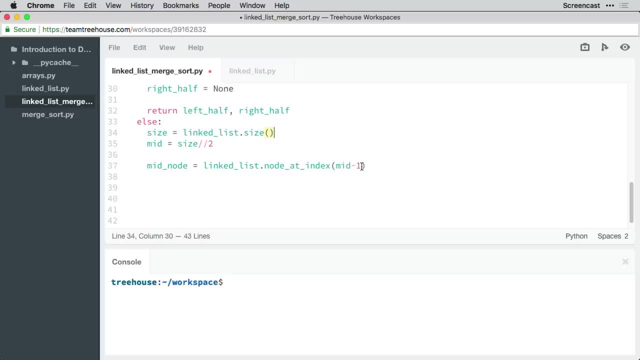 We always start at zero, Which means size is going to be one greater than that. So we're going to deduct one from it To get the value we want. But we're using the floor division operator, So it's going to round that down even more. 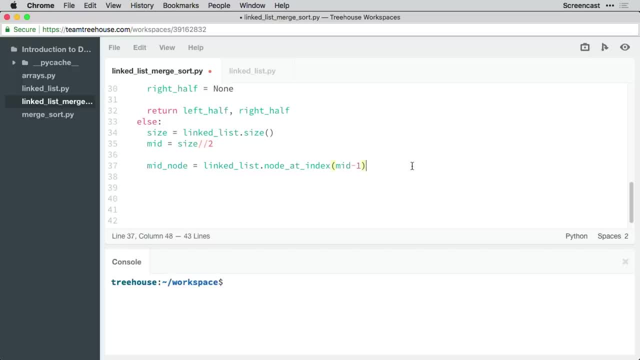 No big deal Because we have this mid node, We can actually split the list. So first we're going to assign the entire linked list To a variable named left half. So left half Equal linked list. This seems counter intuitive, But it will make sense in a second. 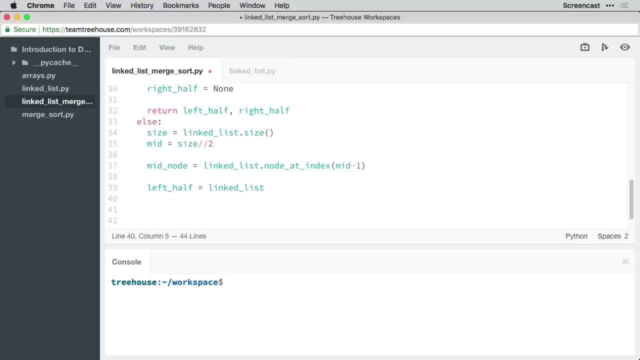 For the right half, We're going to assign a new instance of linked list. So right half Equal linked list. This newly created list Is empty, But we can fix that. So after the midpoint: So after the midpoint of the original linked list. 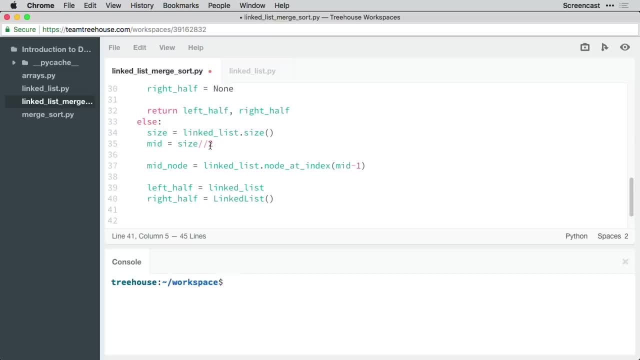 We can assign the node that comes After that midpoint node As the head of this newly created Right linked list. So here we'll say right, half Dot head, Equal mid node, Dot next node. Once we do that, We can assign none to the next node property. 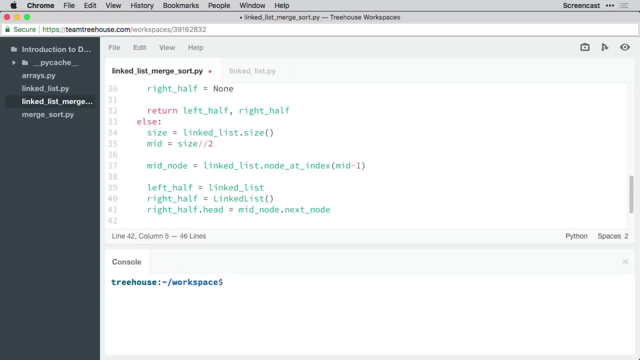 On mid node To effectively sever that connection And make what was the mid node The tail node Of the left linked list. So I'll say mid node Dot, next node Equal none. If that's confusing, Here's a quick visualization of what just happened. 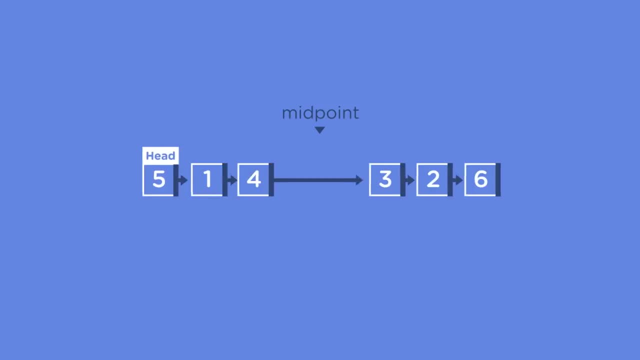 We start off with a single linked list And find the midpoint. The node that comes after the node at midpoint Is assigned to the head of a newly created linked list And the connection Between the midpoint node And the one after is removed. 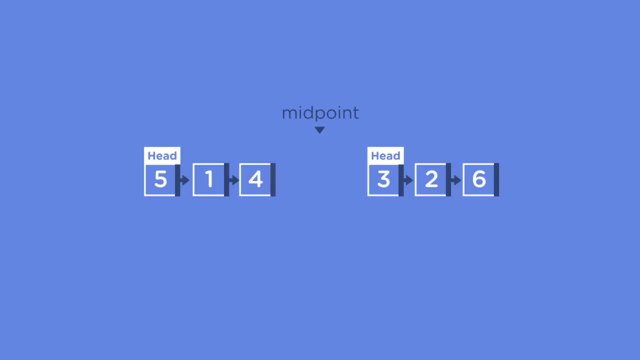 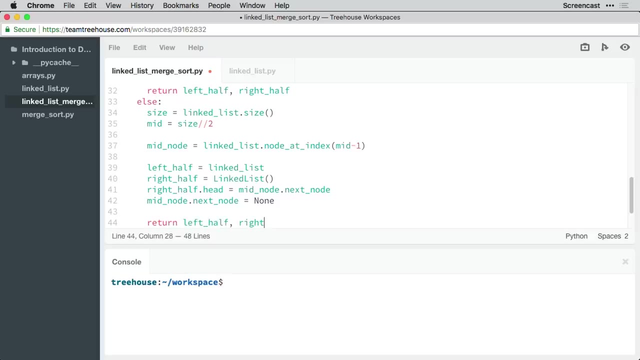 We now have two distinct linked lists, Split at the midpoint, And with that We can return the two sub lists. So we'll return left half And right half In the next video. Let's tackle our merge function In the last video. 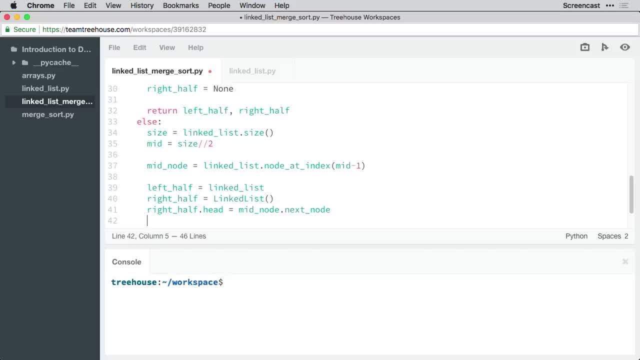 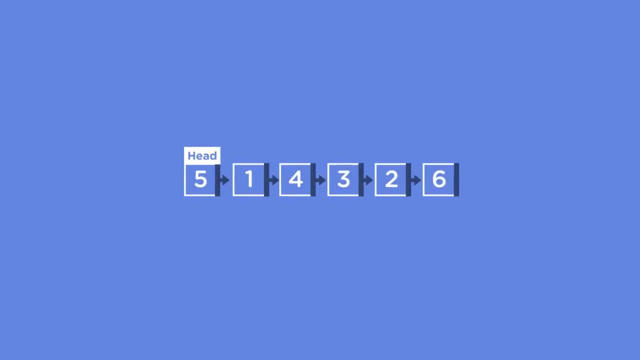 A slash separates the directory name from the file name. Five dot text, And there's our list of numbers that was loaded from the file. Okay, let me delete that print statement and then we'll move on. Bogosort just randomly rearranges the list of values over and over. 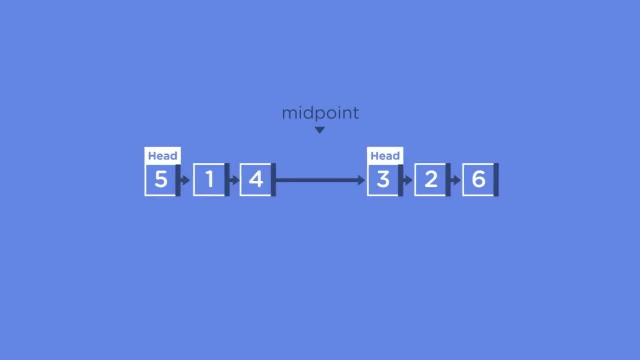 So the first thing we're going to need is is a function to detect when the list is sorted. We'll write an is sorted function that takes a list of values as a parameter. It'll return true if the list passed in is sorted or false if it isn't. 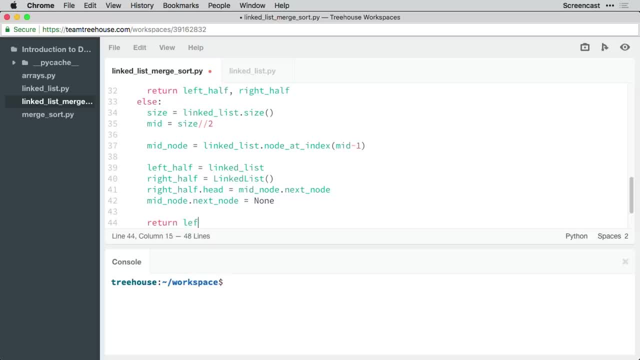 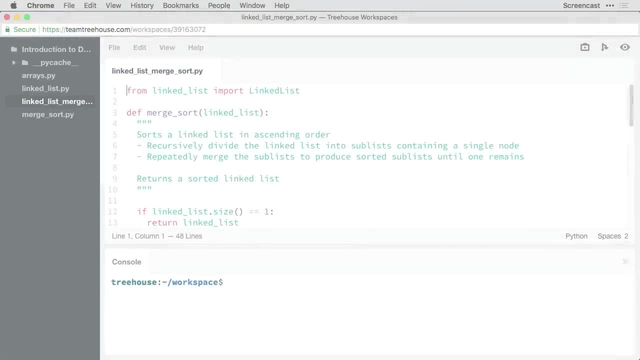 We'll loop through the numeric index of each value in the list from zero to one less than the length of the list. Like many languages, Python list indexes began at zero, so a list with a length of five has indexes going from zero through four. 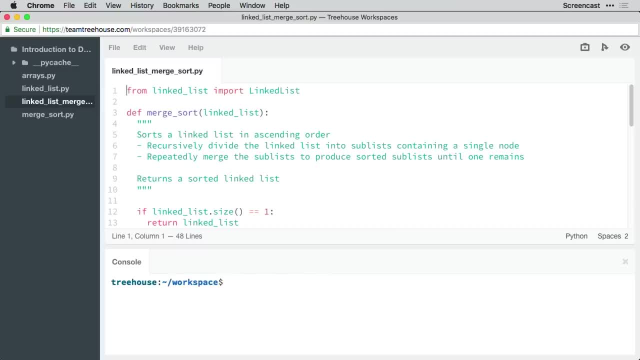 If the list is sorted, then every value in it will be less than the one that comes after it. So we test to see whether the current item is greater than the one that follows it. If it is, it means the whole list is not sorted. so we can return false. 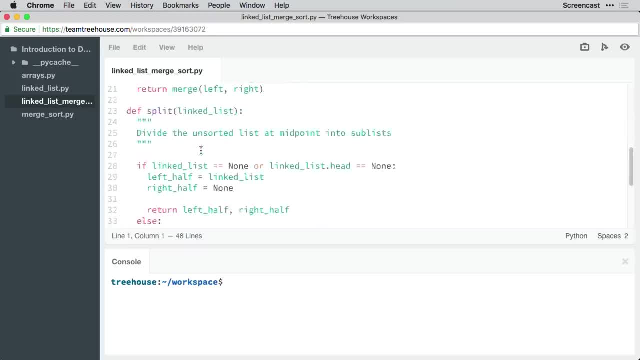 If we get down here, it means the loop completed without finding any unsorted values. Python uses whitespace to mark code blocks, so, unintenting, the code like this marks the end of the loop. Since all the values are sorted, we can return true. 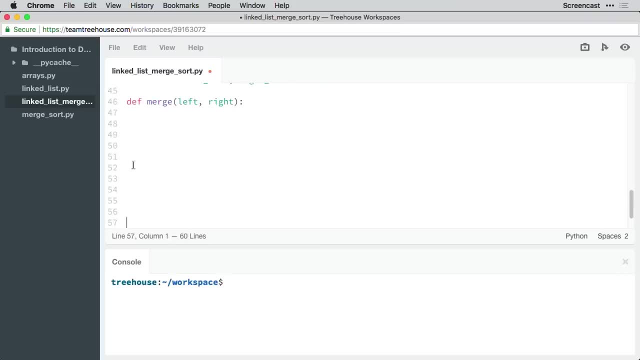 Now we need to write the function that will actually do the so-called sorting. The bogosort function will also take the list of values it's working with as a parameter. We'll call our is sorted function to test whether the list is sorted. 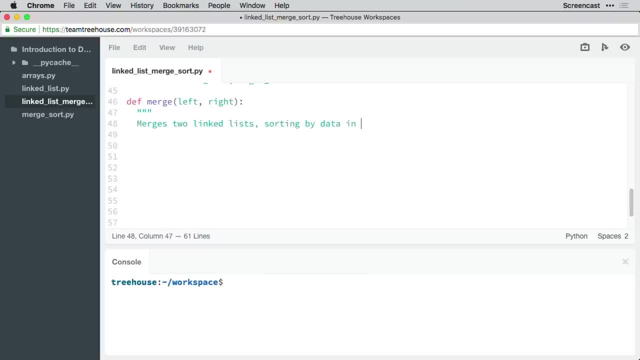 We'll keep looping until is sorted. returns true. Python has a ready-made function that randomizes the order of elements in the list. Since the list isn't sorted, we'll call that function here, And since this is inside the loop, it'll be randomized over and over. 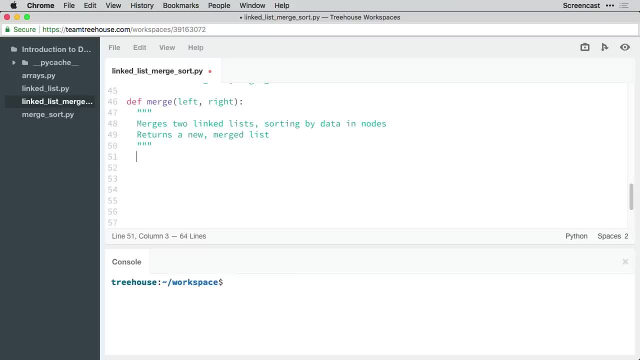 until our is sorted function returns true. If the loop exits, it means is sorted returns true and the list is sorted. so we can now return the sorted list. Finally, we need to call our bogosort function, pass it the list we loaded from the file and print the sorted list it returns. 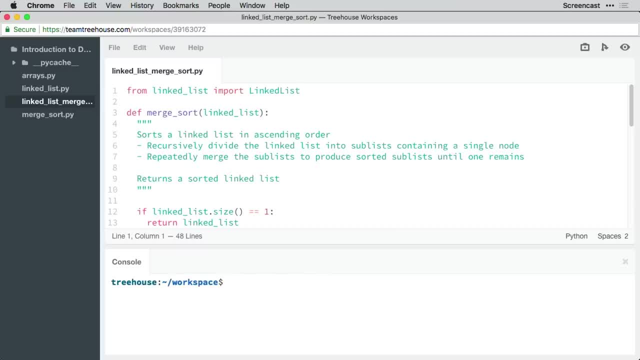 We defined an implementation For the version of the split function That works on linked lists. It contained a tiny bit more code Than the array or list version, And that was expected. After we carry out a comparison operation, We also need to swap references. 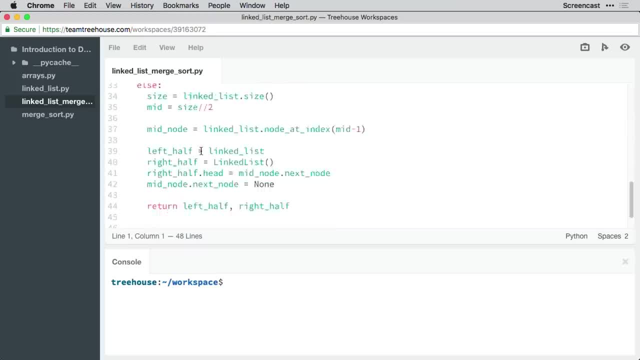 To corresponding nodes. Alright, let's add our merge function Over here at the bottom Below The split function. We'll call this merge And it's going to take a left And a right Now because this can get complicated. We're going to document this function extensively. 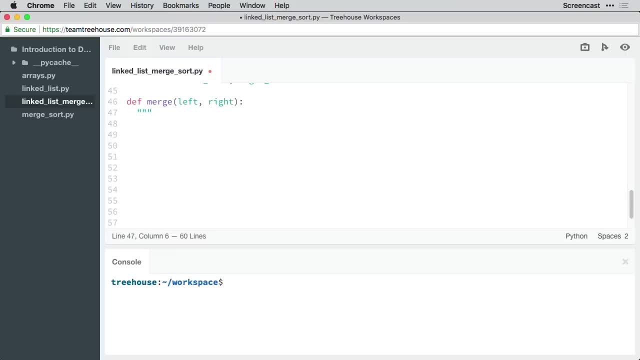 And, as always, we're going to start with a doc string. So we'll say that this function Merges Two linked lists, Sorting By data In the nodes, And it returns a new Merged list. Remember that in the merge step. 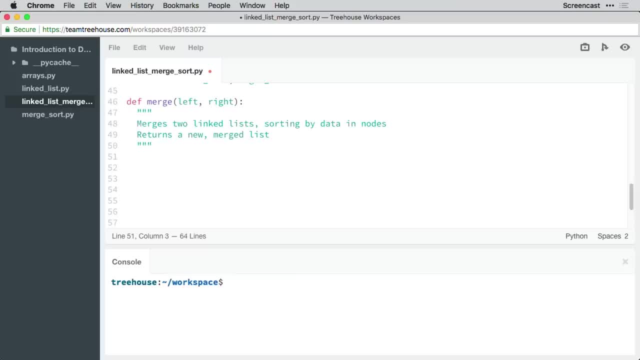 We're going to compare values across two linked lists And then return a new linked list With nodes where the data is sorted. So first We need to create that new linked list. Let's add a comment in here. We'll say create. 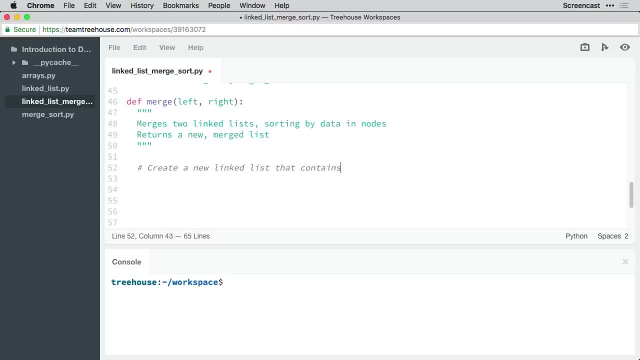 A new linked list That contains nodes From Merging left And right. Okay, and then create the list So merged, equal. New linked list To this list. We're going to do something unusual. We're going to add a fake head. 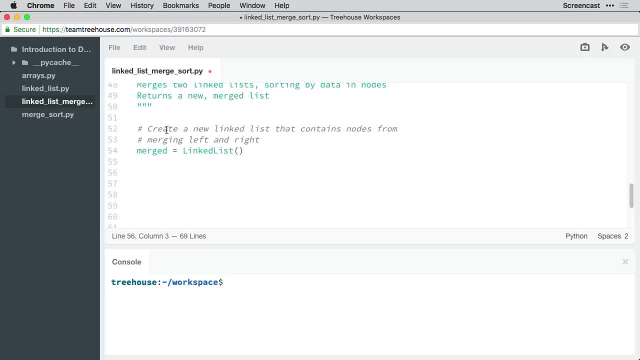 This is so that when adding sorted nodes, We can reduce the amount of code we have to write By not worrying about whether we're at the head of the list. Once we're done, We can assign the first sorted node As the head. 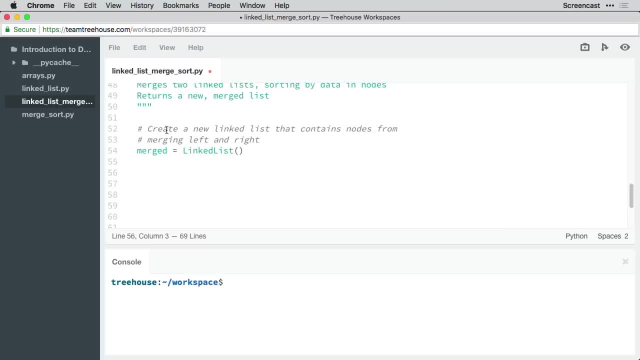 And discard the fake head Now. this might not make sense at first, But not having to worry about whether the new linked list Already contains a head or not Makes the code simpler. We'll add another comment. Add a fake head. that is discarded. 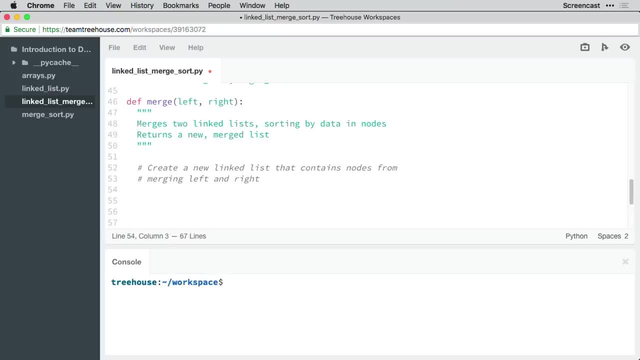 Okay, let's save this and try running it. We do so with Python. the name of the script- bogosortpy, and the name of the file. we're going to run it on: numbers, directory 5.txt. It looks like it's sorting our list successfully. 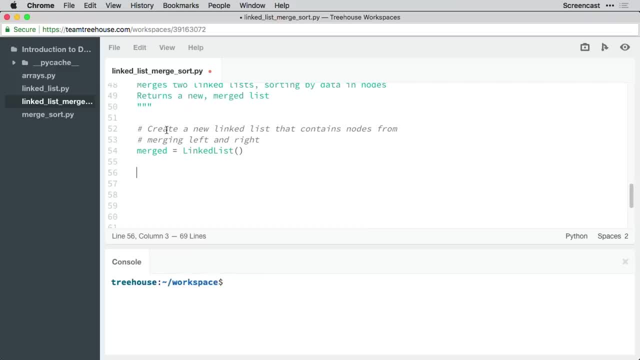 But how efficient is this? Let's add some code to track the number of times it attempts to sort the list. Up here at the top of the bogosort function we'll add a variable to track the number of attempts it's made. 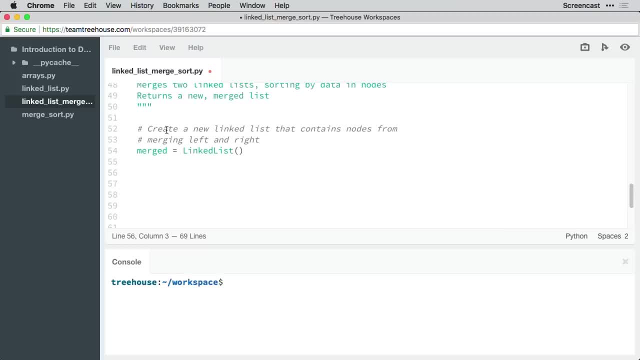 We'll name it attempts and we'll set its initial value to zero, since we haven't made any attempts yet. With each pass through the loop, we'll print the current number of attempts And then here at the end of the loop, after attempting to shuffle the values. 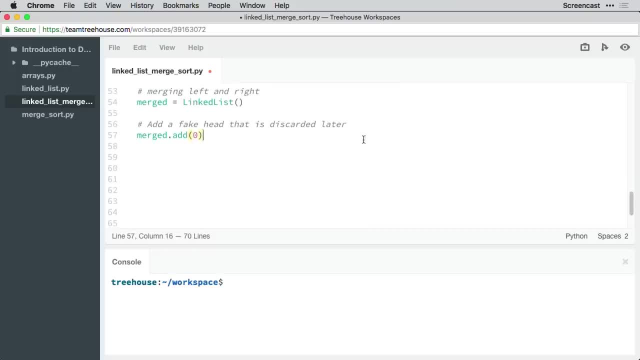 we'll add one to the count of attempts. Let's save this and let's try running it again a couple times. In the console I can just press the up arrow to bring up the previous command and rerun it. So it looks like this first run to sort this five element list took 363 attempts. 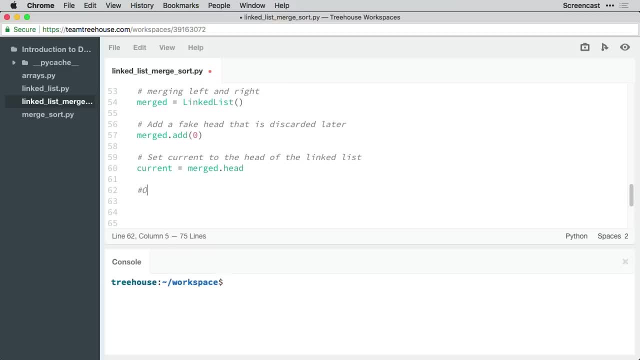 Let's try it again. This time it only took 91 attempts. We're simply randomizing the list with each attempt, so each run of the program takes a random number of attempts. Now let's try this same program with a larger number of items. 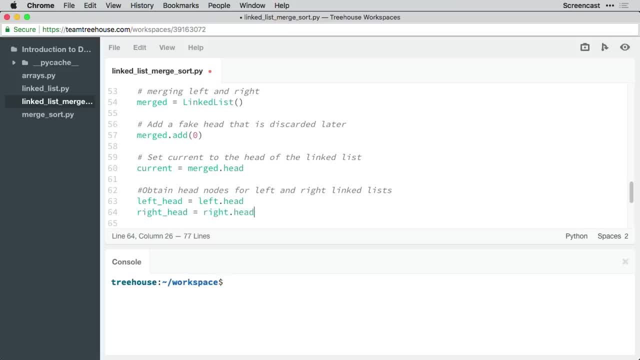 Python bogosort numbers. I have a list of eight items set up here in this other file. This time it takes 11,000 attempts, Only 487.. This time, 13,000.. You can see that the trend is increasing steadily. 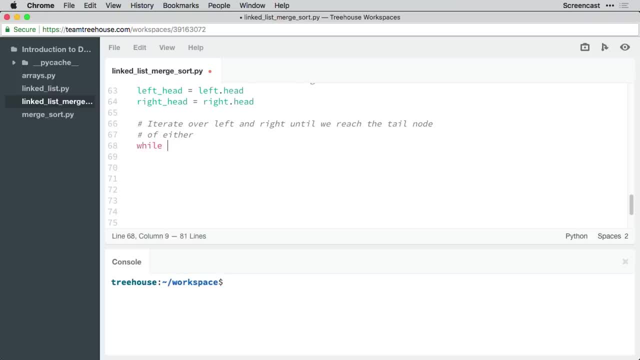 The problem with bogosort is that it doesn't make any progress toward a solution. with each pass, It could generate a list where just one value is out of order, but then on the next attempt it could generate a list where all the elements are out of order again. 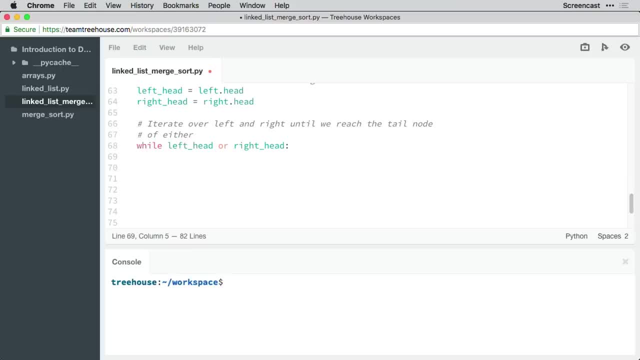 Stumbling on a solution is literally a matter of luck, and for lists with more than a few items it might never happen. Up next We'll look at selection sort. It's a sorting algorithm that's still slow, but it's better than bogosort. 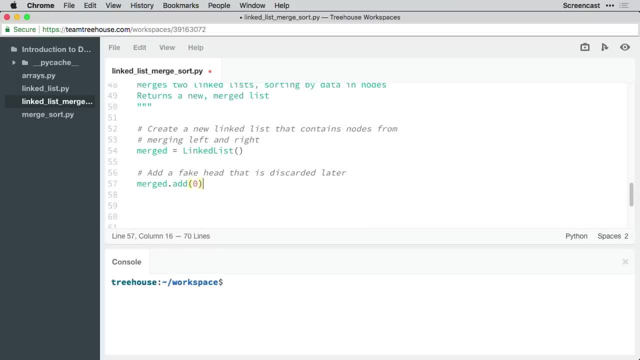 Later We'll say merged- Add zero, Like we've been doing so far, And point to the head of the list, Set current To the head Of the linked list And then current, equal Merged dot head. Next we'll get a reference to the head. 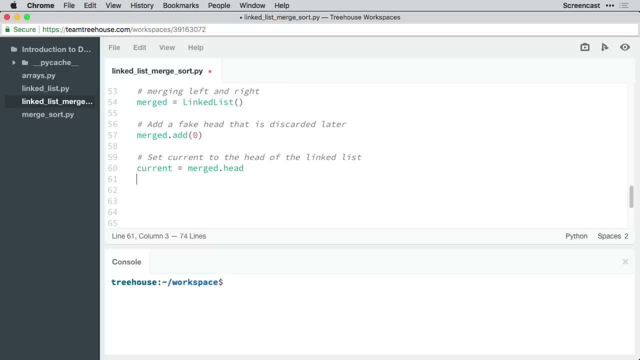 On each of the linked lists, Left and right. So we'll say: obtain Head nodes For left and right Linked lists, And here we'll call this: left head Equal Left dot head And right head Equal right dot head. 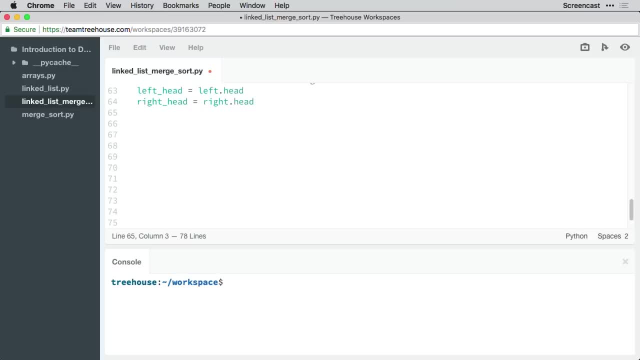 Okay. so with that setup out of the way, Let's start iterating over both lists. So another comment: Iterate Over left and right As long, Or we'll say until Until we reach The tail node Of either, Or we'll do that. 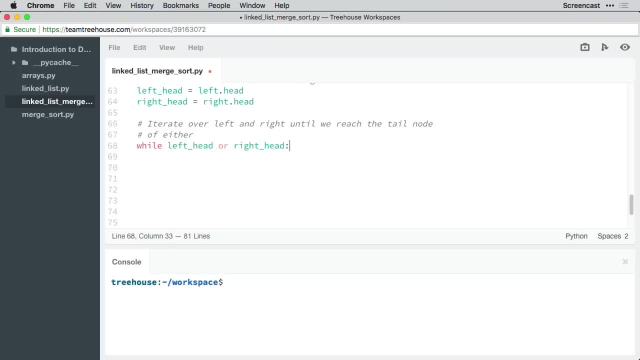 By saying: while Left head Or right head. So this is a pattern that we've been following all along. We're going to iterate until we hit the tail nodes of both lists And we'll move this pointer forward every time So that we traverse the list. 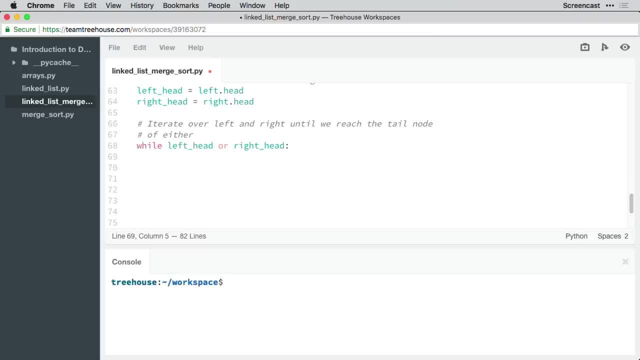 With every iteration. If you remember the logic behind this From the earlier version, Once we hit the tail node of one list, If there are nodes left over in the other linked list, We don't need to carry out a comparison operation anymore. 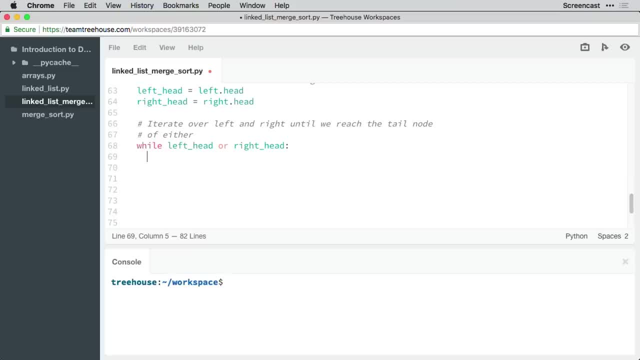 And we can simply add Those nodes to the merged list. The first scenario we'll consider Is if the head of the left linked list Is none, This means we're already past the tail of left And we can add all the nodes. 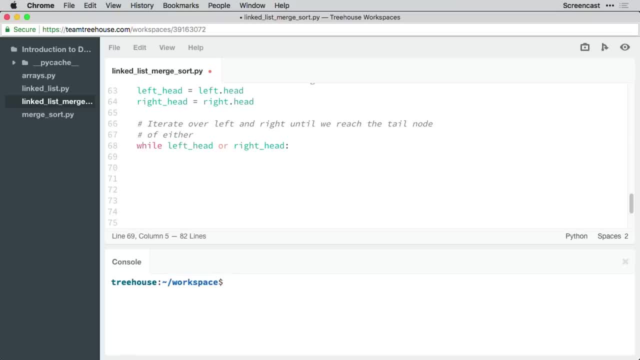 From the right linked list To the final merged list. So we'll say: if The head node of left Is none, We're past the tail. Add the node From the right, From right To the merged linked list. So here we'll say: 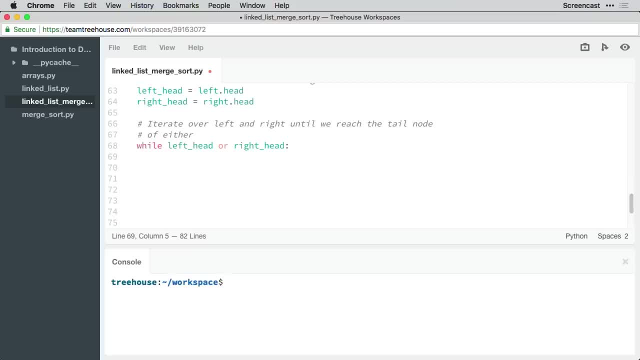 Previously, we showed you bogosort, a terrible sorting algorithm that basically randomizes the order of a list and then checks to see if it happens to be sorted. The problem with bogosort is that it doesn't get any closer to a solution with each operation. 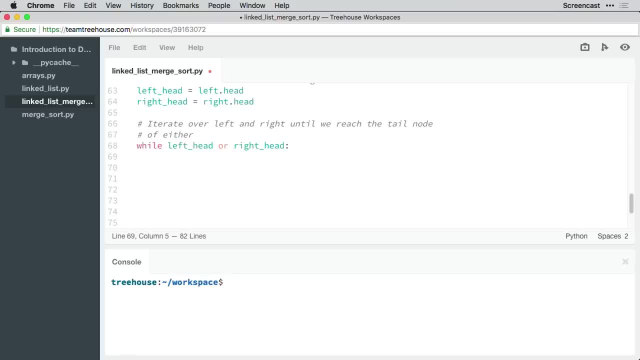 and so with lists that have more than a few items, it'll probably never finish sorting them. Now we're going to look at an algorithm named selection sort. It's still slow, but at least each pass through the list brings it a little closer to completion. 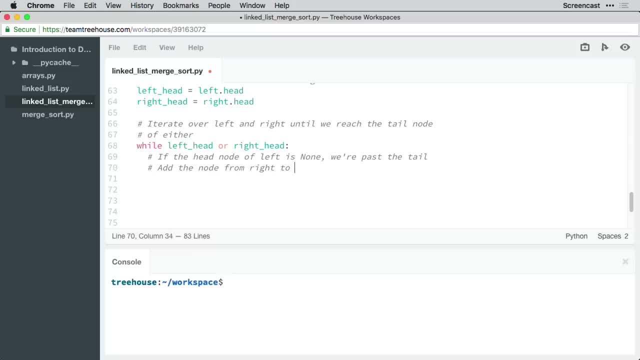 Our implementation of selection sort is going to use two arrays: an unsorted array and a sorted one. Some versions move values around within just one array, but we're using two arrays to keep the code simpler. The sorted list starts out empty, but we'll be moving values from the unsorted list to the sorted list, one at a time. 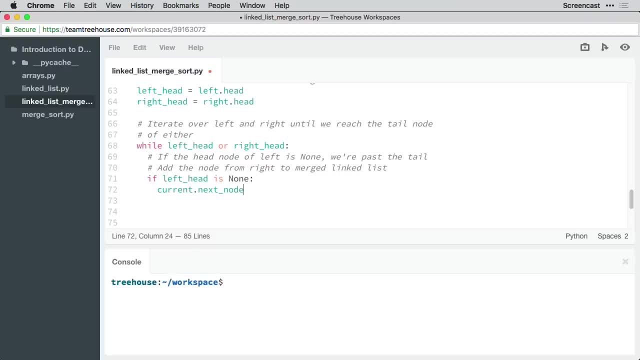 With each pass we'll look through each of the values in the unsorted list, find the smallest one and move that to the end of the sorted array. We'll start with the first value in the unsorted array and say that's the minimum or smallest value we've seen so far. 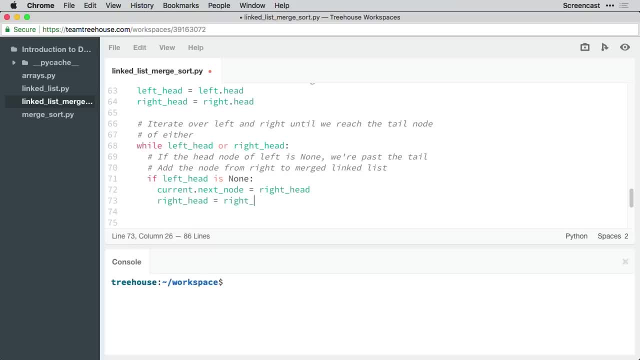 Then we'll look at the next value and see if that's smaller than the current minimum. If it is, we'll mark that as the new minimum. Then we'll move to the next value and compare that to the minimum. again, If it's smaller, that becomes the new minimum. 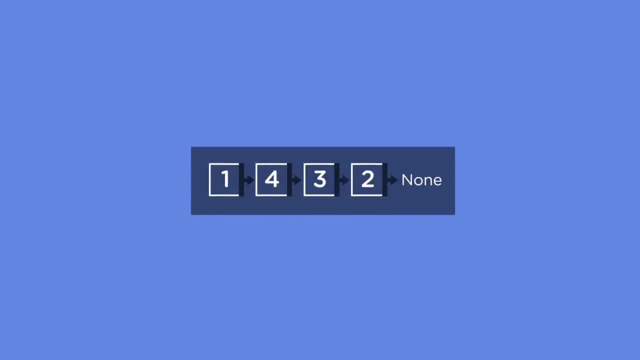 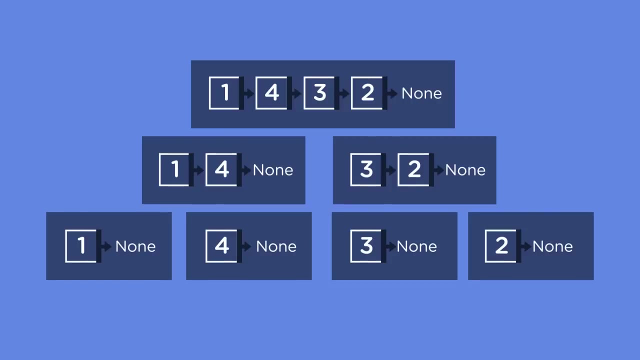 We continue that way until we reach the end of the list. At that point we know whatever value we have, it's going to be the minimum. Whatever value we have marked as the minimum is the smallest value in the whole list. Now here's the part that makes selection sort better than BOGO sort. 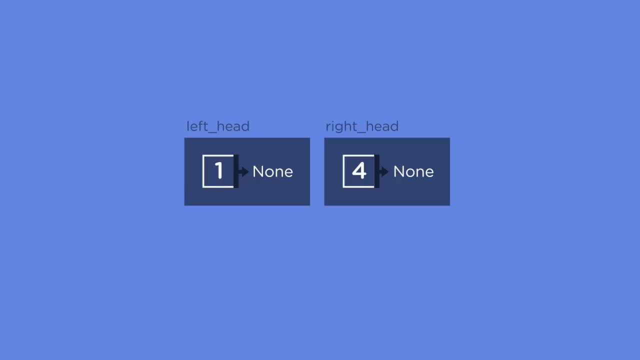 We then move that minimum value from the unsorted list to the end of the sorted list. The minimum value isn't part of the unsorted list anymore, so we don't have to waste time looking at it anymore. All our remaining comparisons will be on the remaining values in the unsorted list. 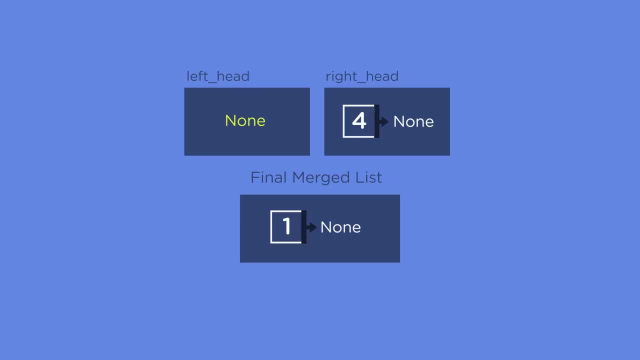 Then we start the process over. At this point, our list consists of the numbers 8,, 5, and 6.. 8,, 5,, 4, and 7.. Our first minimum is 8.. We start by comparing the minimum to 5.. 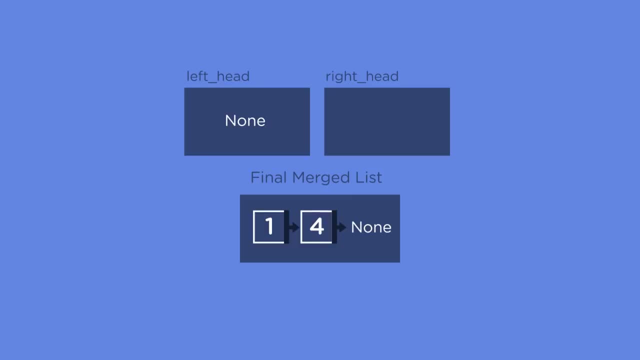 5 is smaller than 8, so 5 becomes the new minimum. Then we compare 5 with 4, and 4 becomes the new minimum. 4 is not smaller than 7, though, so 4 remains the minimum. 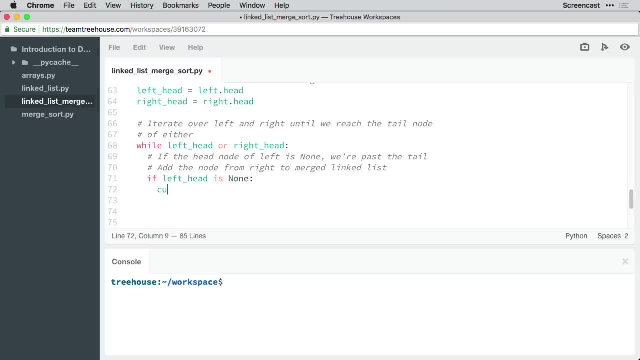 If left head Is none, Current dot. next node: Remember current Points to the head of the merged list That we're going to return. So here we're setting it's next node. reference To the head node On the right linked list. 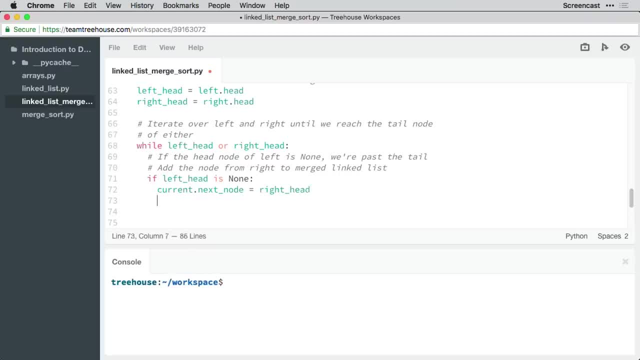 So we'll say right head. Then when we do that, We'll move the right head forward To the next node. Right head Equal right head Dot next node. This terminates The loop. on the next iteration. Let's look at a visualization. 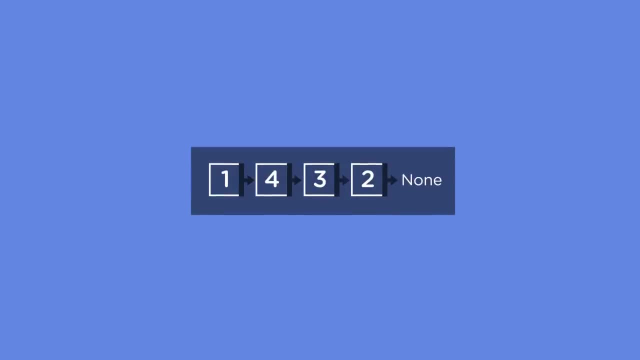 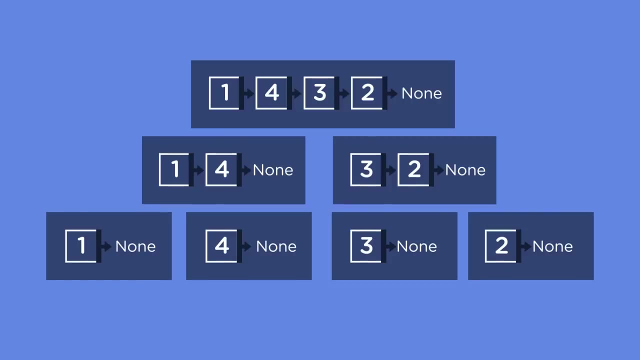 To understand why. Let's say, we start off with a linked list Containing four nodes, So we keep calling split on it Until we have lists with just a single head, Single node, linked lists essentially. So let's focus on these two down here. 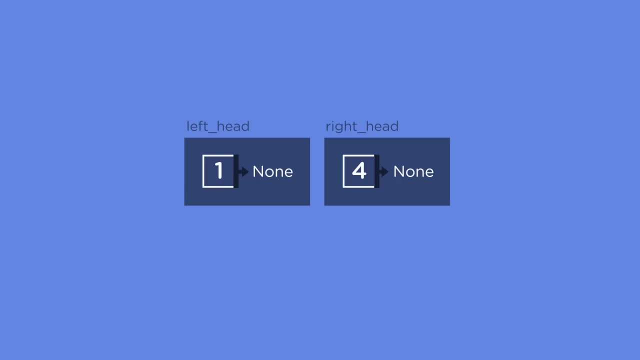 That we'll call left and right. We haven't implemented the logic for this part yet, But here we would compare the data values And see which one is less than the other. So we'll assume that left's head Is lesser than right's head. 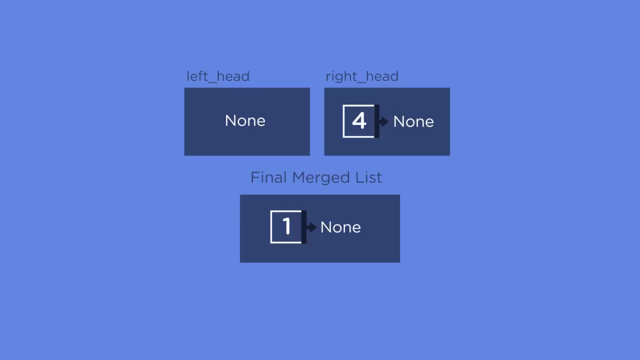 So we'll set this as the next node In the final merged list. Left is now an empty linked list, So left dot head equals none. On the next pass through the loop, Left head is none, Which is the situation we just implemented. 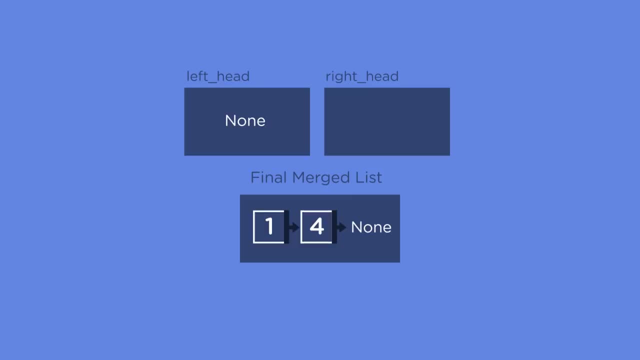 Here we can go ahead And now assign right head As the next node in the merged linked list. We know that right is also a singly linked list. Here's the crucial bit When we move the pointer forward By calling next node. 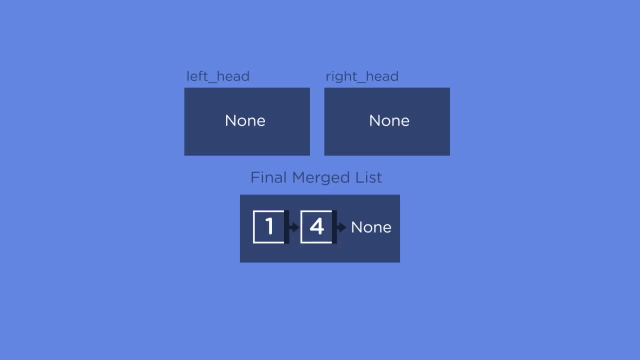 On the right node. There is no node, And the right linked list Is also empty now, Which means that both left head and right head are none, And either one of these Would cause our loop condition to terminate. So what we've done here? 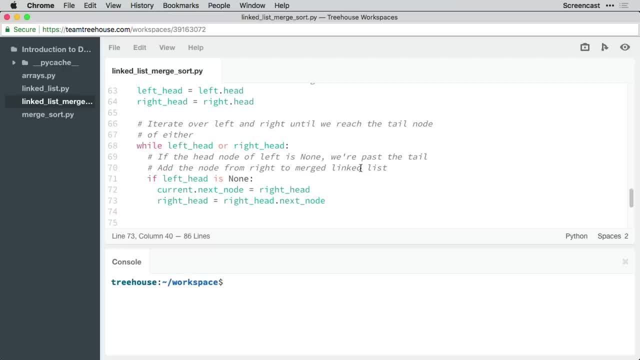 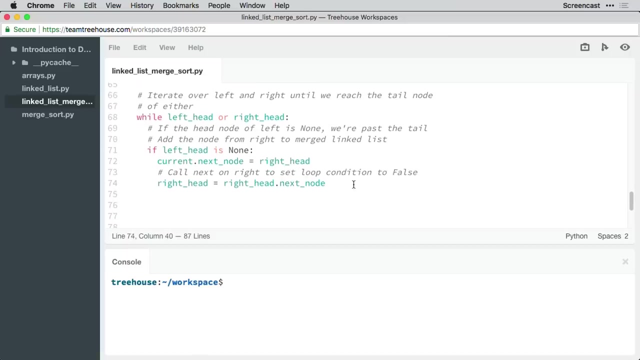 Is encoded a stopping condition for the loop. So we need to document this Because it can get fuzzy. So right above that line of code, I'll say: call next On right To set loop condition To false. Okay, there's another way we can arrive. 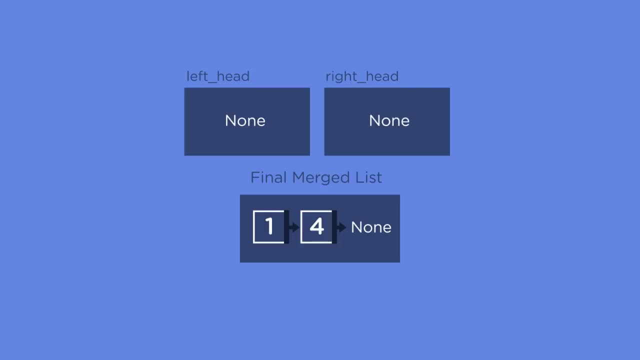 4 gets moved to the end of the sorted array, becoming its second element. The process repeats again. 8 is the first minimum, but 5 is smaller, so that becomes the minimum. 7 is larger, so 5 stays as the minimum. 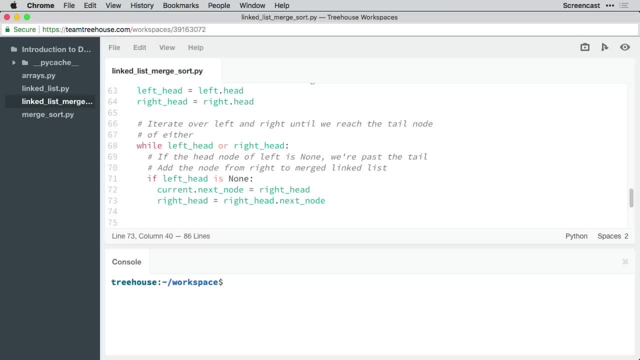 1, 1, 0, 1, 0,, 5,, 5,, 4,, 4,, 4, 4, 4,, 5,, 5,, 6,, 7.. And 5 is what gets moved over to the sorted array. 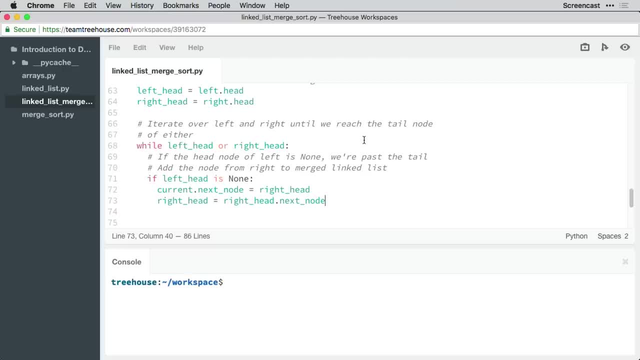 And so on, until there are no more items left in the unsorted array, and all we have left is the sorted array. So that's how selection sort works in general. Now let's do an actual implementation of it. This code here at the top is the same as we saw in the BOGO sort example. 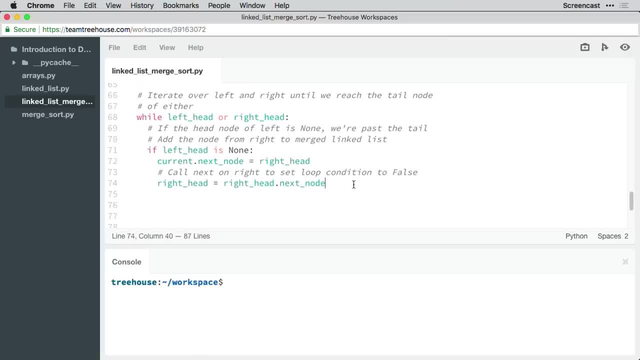 It just loads a Python list of numbers from a file. Let's implement the function that will do our selection sort. We're going to pass in our Python list containing all the unsorted numbers. We'll create an empty list that will hold all our sorted values. 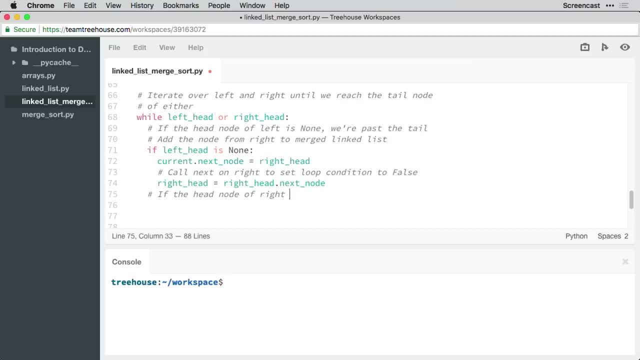 We'll loop once for each value in the list. We call a function named index of min- which we're going to write in just a minute- that finds the minimum value in the unsorted list and returns its index. Then we call the pop method on the list and pass it the index of the minimum value. 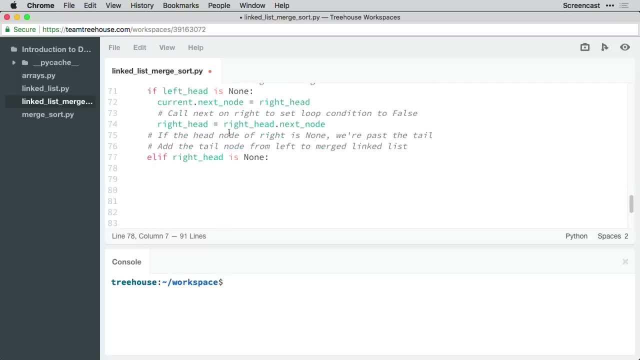 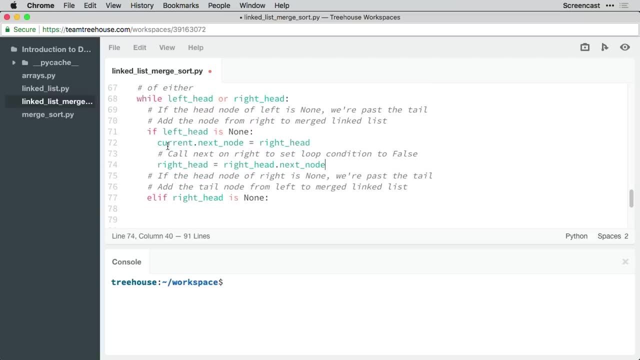 Pop will remove that item from the list and return it. We then add that value to the end of the sorted list. Going up a level of indentation signals to Python that we're ending the loop. After the loop finishes, we return the sorted list. 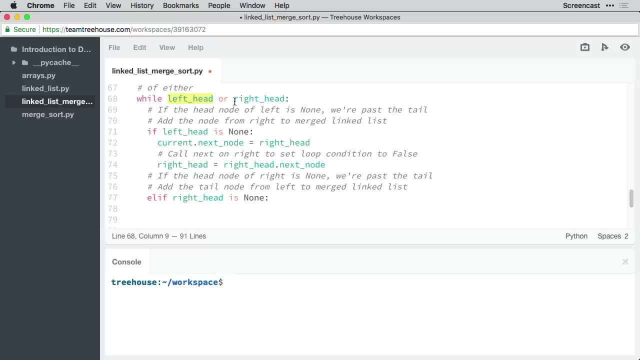 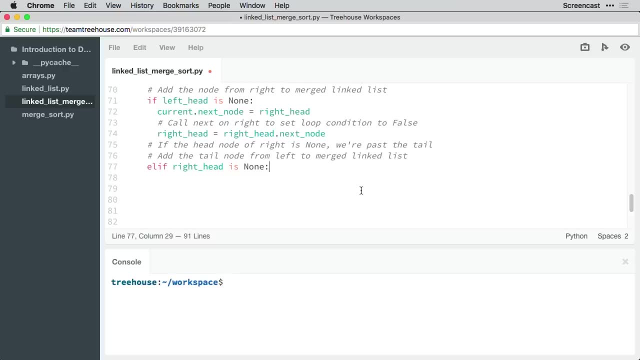 Now we need to write the function that picks out the minimum value We pass in the list we're going to search. We mark the first value in the list as the minimum. It may or may not be the actual minimum, but it's the smallest we've seen on this pass. through the list. It's also the only value we've seen on this. pass through this, the list …. It's the smallest we've seen on this. pass through the list …. It's also the only value we've seen on this. pass through this list. 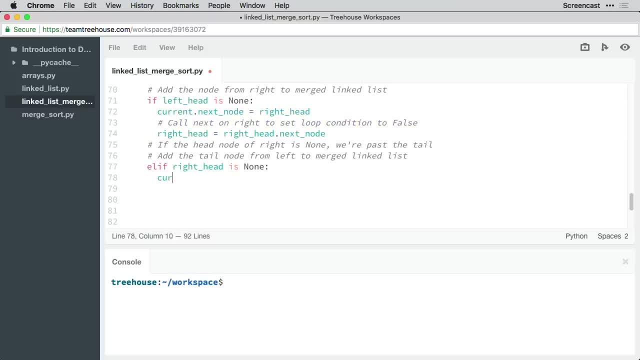 …. … list so far. Now we loop through the remaining values in the list. after the first, We test whether the value we're currently looking at is less than the previously recorded minimum. If it is, then we set the current index as the new index of the minimum value. 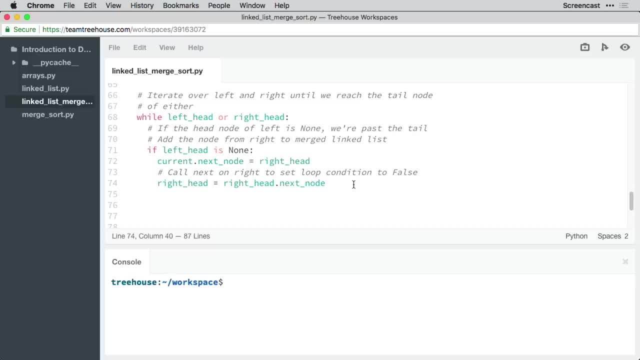 At this stopping condition, And that's in the opposite direction, If we start with the right head being none. So here we'll say- I'm going to add another comment: If, If The head node Of right Is none. 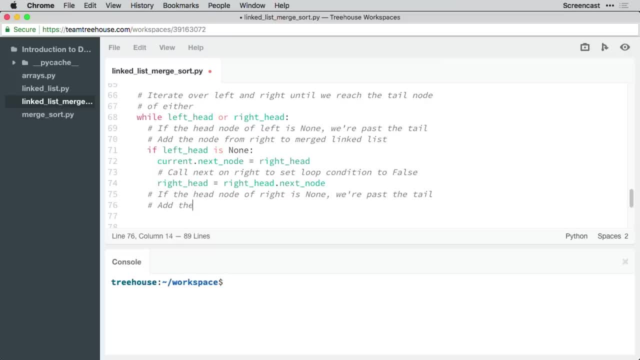 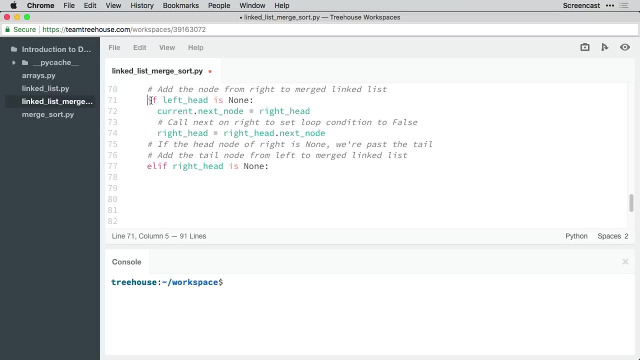 We're past the tail, Then we'll say: Add the tail node From left To merged linked list And then we'll add that condition. We'll say else, if right head Is none, Now remember we can enter these Even if left head is none. 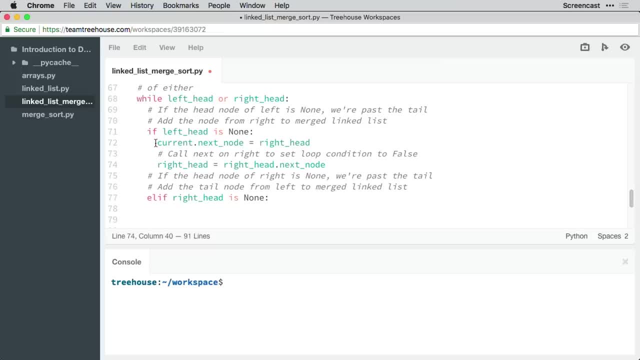 We can still go into this condition. We can still enter this if statement And execute this logic. The loop condition here Is an or statement. So even if left head is false, If this returns true, Because there's a value there. 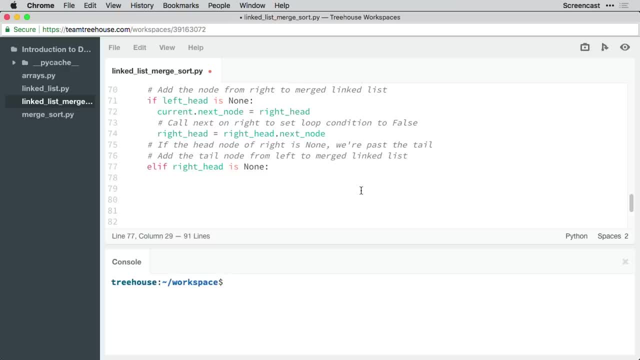 There's a node there, The loop will keep going. Okay, now, in this case, We want to set the head of the left linked list As the next node on the merged list. So this is simply the opposite Of what we did over here. 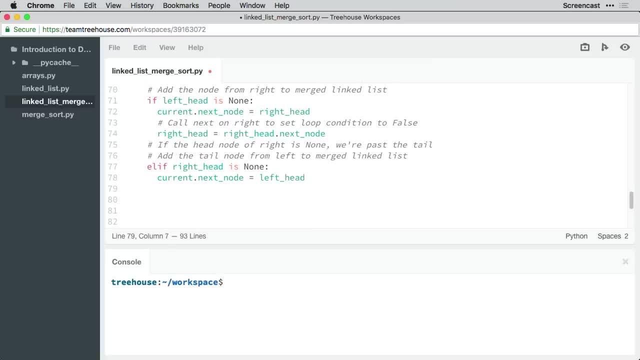 We'll set currentnext node Equal to left head, And by doing that we can move the variable Pointing to left head forwards, Which, as we saw earlier, is past the tail node And then results in the loop terminating. So we'll say left head. 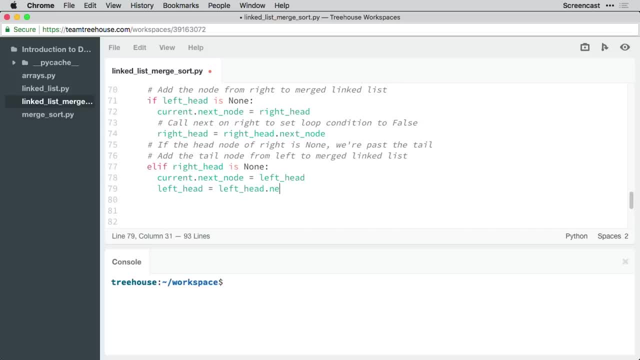 Equal Left head dot next node, And we'll add that comment here as well. So we'll say: call next On left to set Loop condition To false, Because here right head is none And now we make left head none. 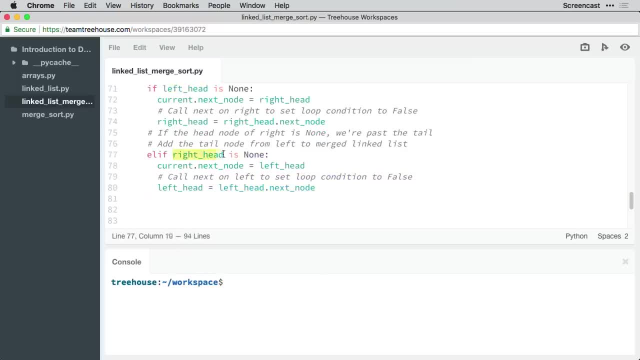 These two conditions- we looked at Left head Or right head- Were at the tail nodes of our respective lists. Those are conditions that we run into When we've reached the bottom of our split, Where we have single element linked lists Or empty linked lists. 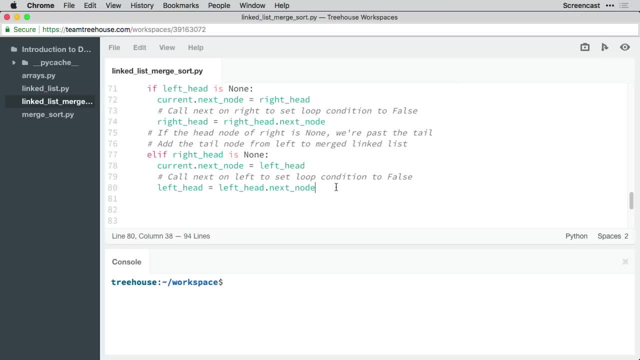 Let's account for our final condition, Where we're evaluating a node That is neither the head Nor the tail of the list, And this condition: We need to reach into the nodes And actually compare the data values to one another Before we can decide. 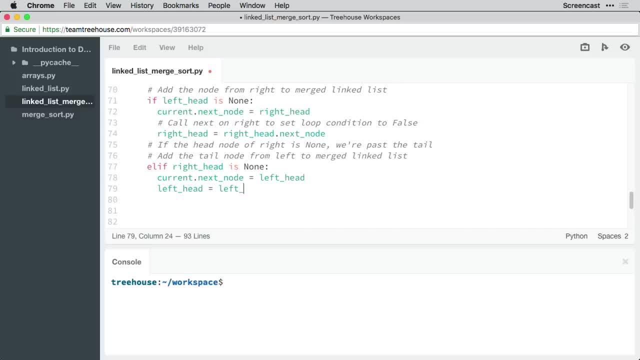 After we've looped through all the values, we return the index of the smallest value we found. Lastly, we need to actually run our selection sort method and print the sorted list it returns. Let's save this and now let's try running it. We run the python command and pass it the name of. 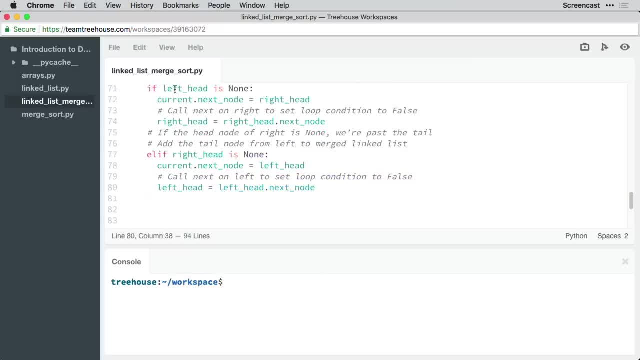 our script selection sortpy. In the numbers directory, I've saved several data files filled with random numbers, one on each line. 5.txt has five lines, 8.txt has eight lines and, to help us really measure the speed of our algorithms, 10,000.txt has 10,000 lines. I've even created 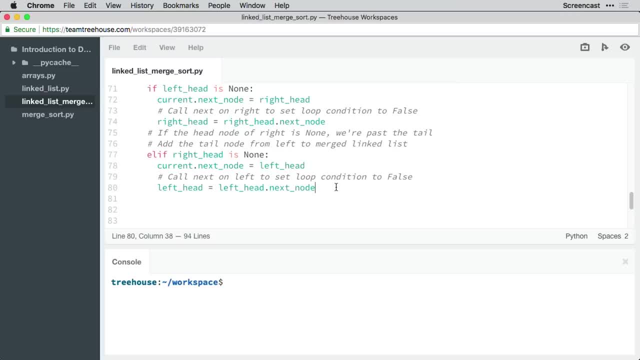 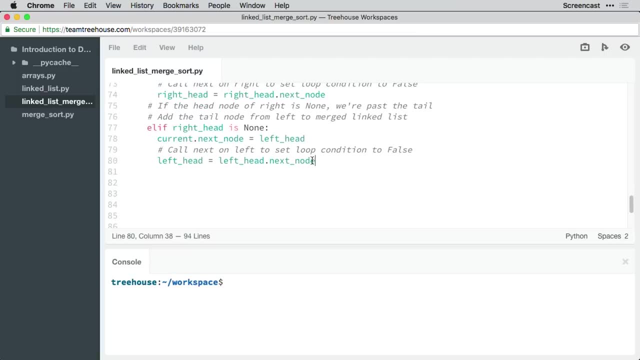 a file with a million numbers. Our script takes the path of a file to load as an argument, so I'll give it the path of our file with five numbers, numbers, slash, 5.txt. The script runs. reads the numbers in the file into a list. calls our selection sort. 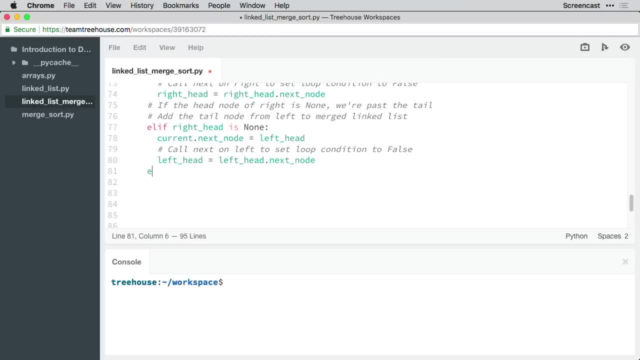 method with that list and then prints the sorted list. Let me add a couple print statements within the selection sort function so you can watch the sort happening. Don't worry about figuring out the python formatting string that I use. it's just there to keep the two lists neatly aligned. 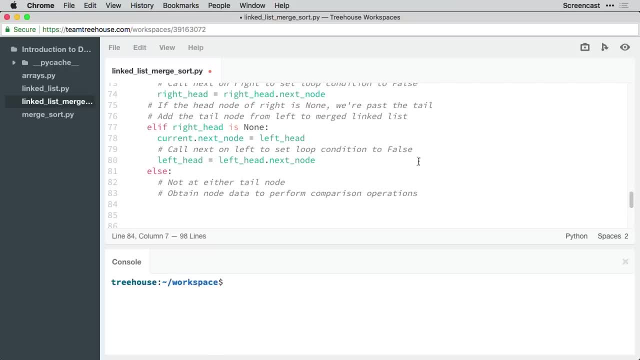 I'll add the first print statement before the loop runs at all. I'll have it print out the unsorted list and the sorted list. I'll add an identical print statement within the loop so we can watch values moving from the unsorted list to the sorted. 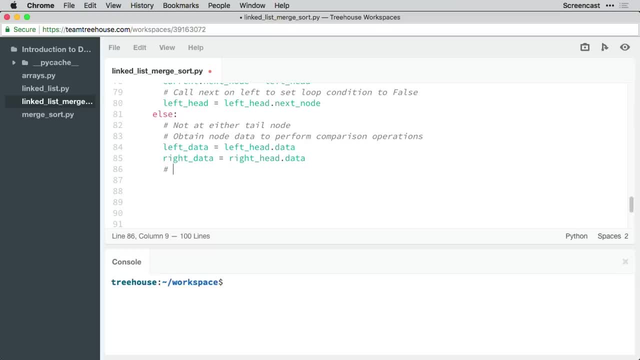 list. Let's save this and we'll try running the same command again. The output looks like this. You can see the unsorted list on the left and the sorted list on the right. Initially, the sorted list is empty. On the first pass it selects the lowest number 1 and moves it to the 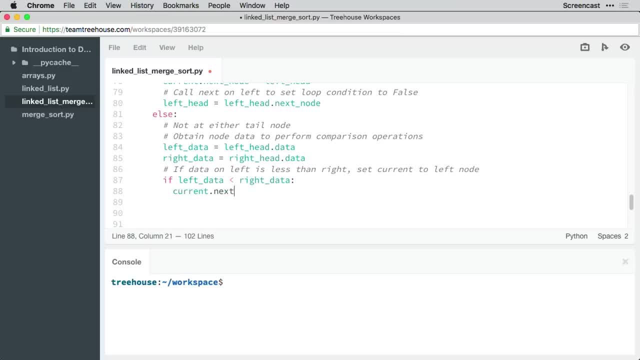 sorted list. Then it moves the next lowest number over 4.. This repeats until all the numbers have been moved to the sorted list. I have another file with 8 different numbers in it. Let's try our program with that python selection: sortpy numbers 8.txt. You can see the same process at: work here. Notice that this file has 8 different numbers in it. This file has the same numbers as the first one and you can see that it's moved to the sorted list. You can use that to make the other file and you can also use the first one to move the lowest number over 4.5.. The sorted list is empty. The. 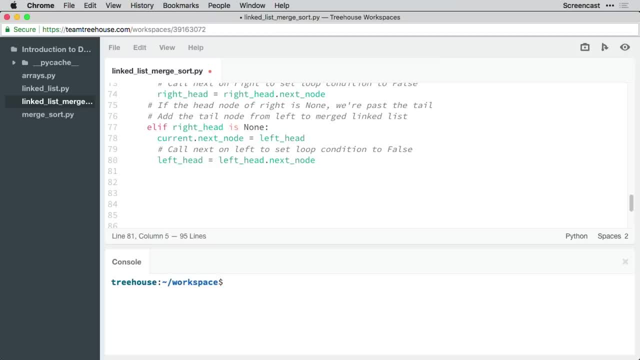 Add first to the merge list. So here this is an else, Because we've arrived at our third condition. Third and final, And here we'll say not at either, Tail node Obtain Node data To perform comparison operations. So let's get each of those data values. 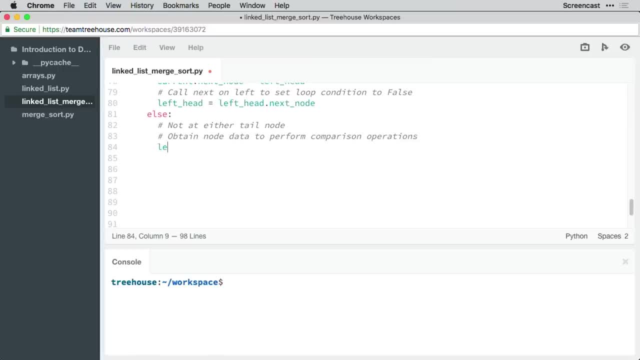 Out of the respective nodes So that we can compare it. So we'll say: left data Equal left head dot data And right data Equal right head Dot data. Okay, what do we do next? Well, we compare, But first let's add a comment. 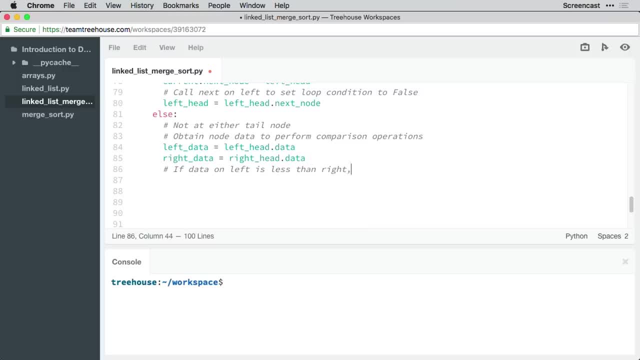 So we'll say: if data On left Is less than right, Set current to left node And then move. Actually we'll add this in a second. So here we'll say: if left data Is less than right data, Then current. 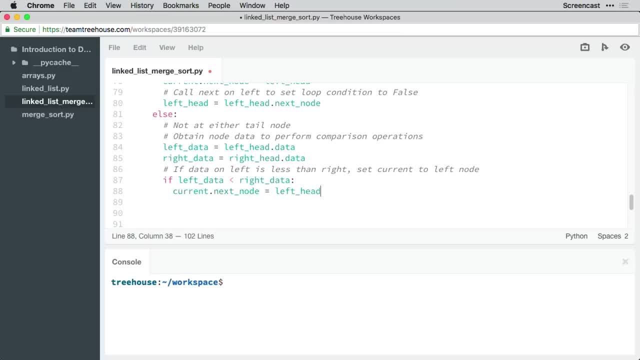 Dot next node: Left head. And then we'll add a comment And we'll say: move left head To next node On that list. So we'll say: left head Equal left head Dot next node, Just as our comment says. 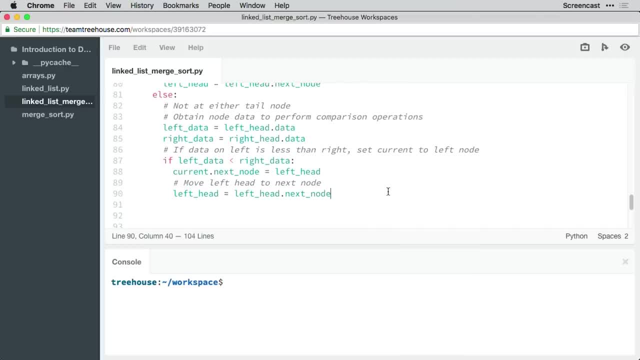 We'll check if the left data Is less than the right data. If it is, Since we want a list in ascending order, We'll assign the left node to be the next node In the merged list. So left head forward To traverse down to the next node. 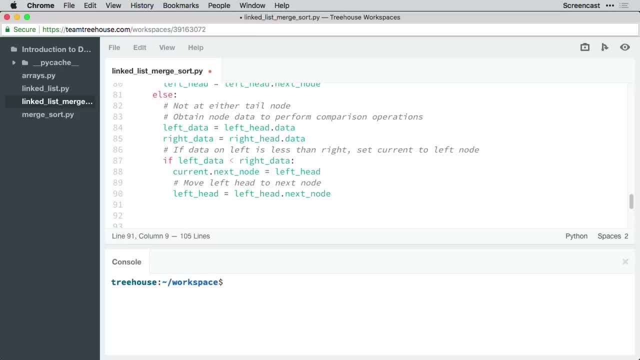 In that particular list. Now, if left is larger than right, Then we want to do the opposite, So we'll go back two spaces. Add another comment. If data on left is greater than right, Set current To right node Okay. 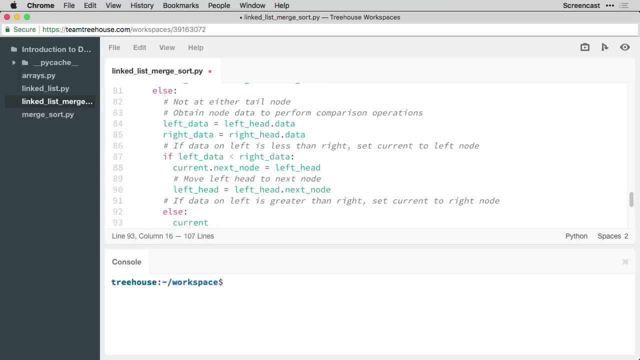 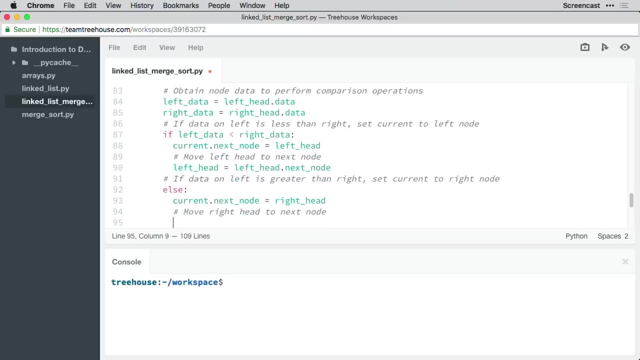 So else Here we assign the right head To be the next node in the merged list. So current dot. next node Equal right head. And then Comment: Move right head To next node. So right head Equal right head. 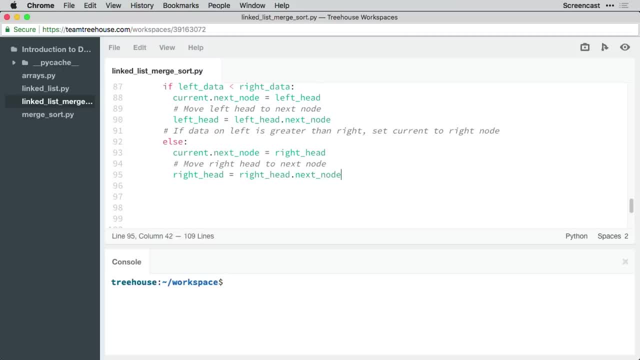 Dot, next node. Okay, After doing that, We move the right head pointer To reference the next node in the right list And finally At the end of each iteration of the while loop. So not here, Two spaces back Right. 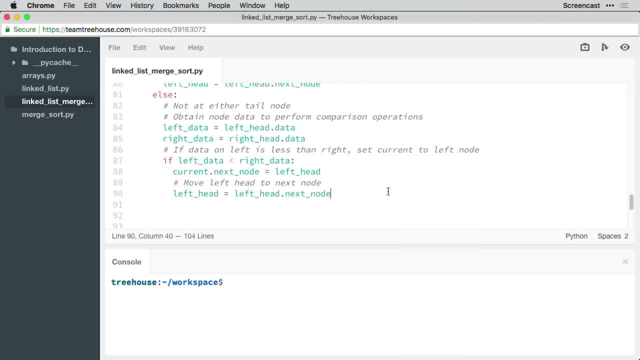 This file had some duplicate values too. That's okay, though, because the index of min function only updates the minimum index if the current value is less than the previous minimum. If they're equal, it just keeps the first minimum value it found and waits to move. 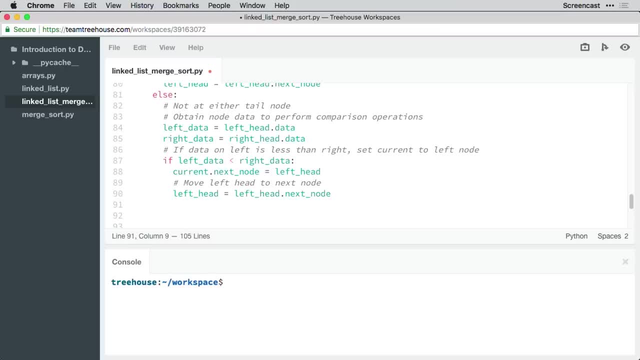 the duplicate value over until the next pass through the list. So now we know that the selection sort algorithm works, But the datasets we've been giving it to sort are tiny. In the real world, algorithms need to work with datasets of tens of thousands or even. 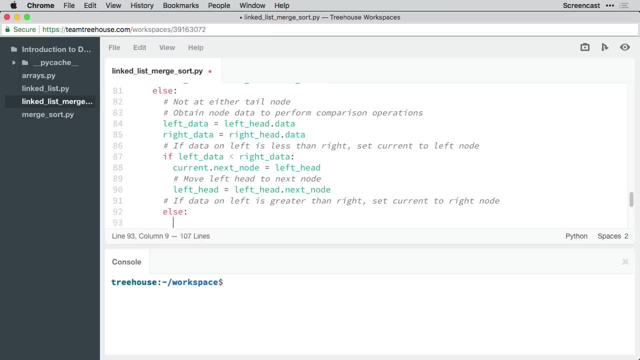 millions of items and do it fast. I have another file with 10,000 random numbers in it. Let's see if selection sort can handle that. If I run this as it is now, though, it'll print out a lot of debug info as it sorts. 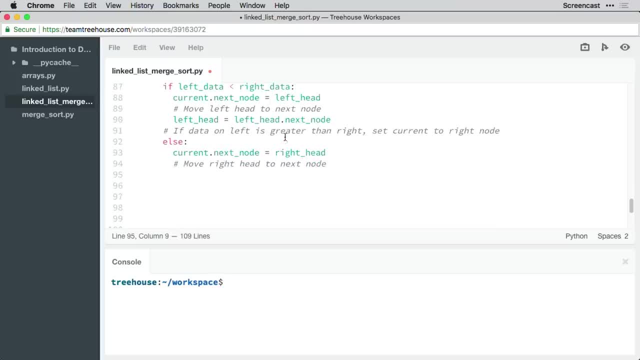 the list. So first I'm going to go into the program and remove the two print statements in the selection sort function. Okay, Now let's run the program again on the 10,000.txt file and see how long it takes. 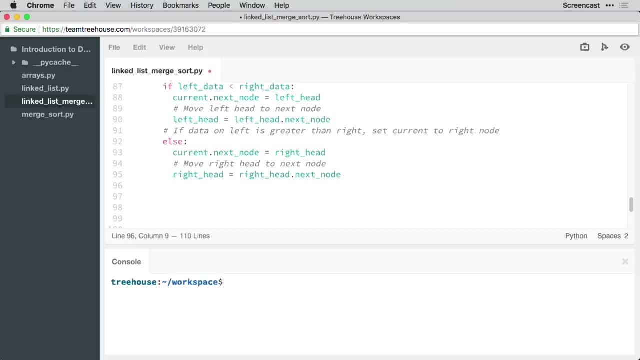 Python selection sortpy numbers: 10,000.txt. 1 1,000,, 2 1,000,, 3 1,000,, 4 1,000,, 5 1,000,, 6 1,000, 7 1,000,, 8 1,000,, 9 1,000,, 10 1,000,, 11 1,000,, 12 1,000,, 13 1,000,. and it prints: 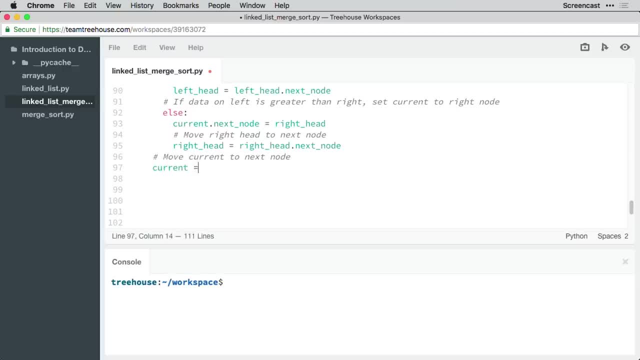 out all 10,000.. It took a little bit, though. How long? Well, counting the time off vocally isn't very precise, and other programs running on the system can skew the amount of time your program takes to complete. Let me show you a Unix command that's available here in workspaces which can help. 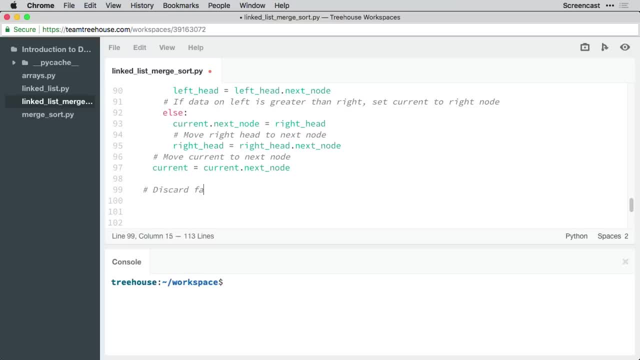 You type time, followed by a space, and then the command you want to run. So this command by itself will print the contents of our 5.txt file, cat, as in concatenate numbers 5.txt- And this command will do the same thing, but it'll also keep track of how long it takes. 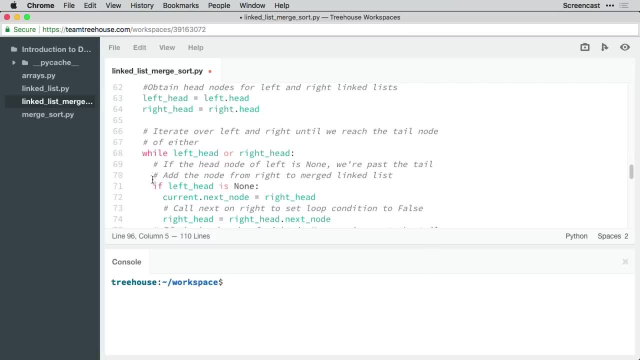 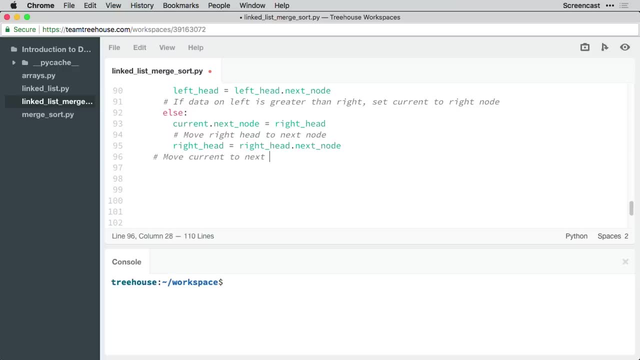 Make sure we're indented at the same level as the while. So we gotta go Yep Or not the same level as the while, But the same outer scope. And then there We're going to say: Move current to next node. 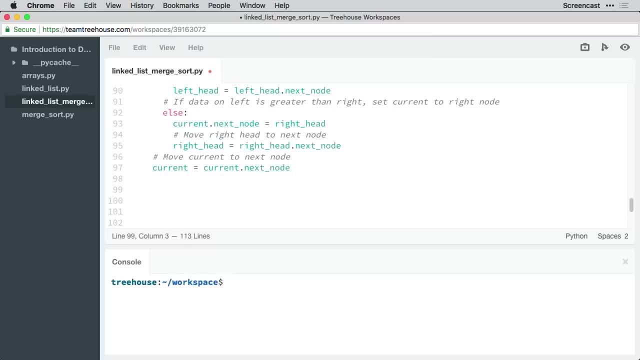 So current Equal, current dot. next node: Okay, Don't worry if this is confusing. As always, Setting the correct node as head And returning the linked list. So we'll add a comment. Discard fake head And set first. 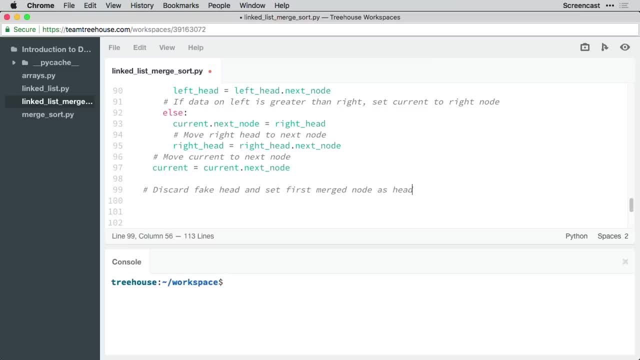 Merged node As head. So here we'll say: head equal, Merged dot, head, Dot next node, And then merged dot, head Equal head And finally return Merged. Okay, We wrote a lot of code here. Some of it was comments. 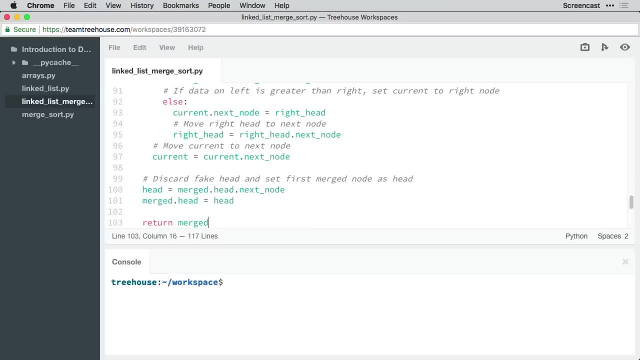 But still it's a bunch. Let's take a quick break. In the next video We'll test this out, Evaluate our results And determine the runtime of our algorithm. Okay, First things first. Let's test out our code Now. we'll keep it simple. 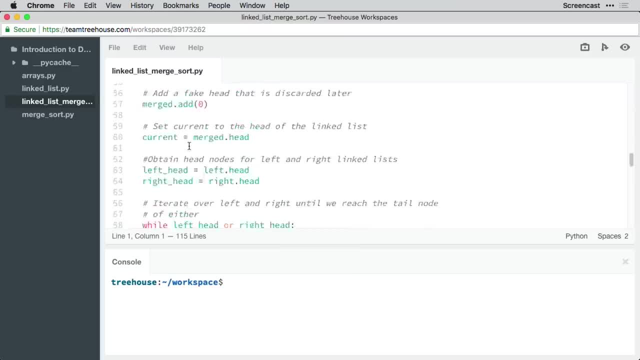 Because writing a robust verify function Would actually take up this entire video. Instead, I'll leave that up to you To try as homework. Okay, Let's add a few nodes to this. So l add, I'm going to copy paste this: 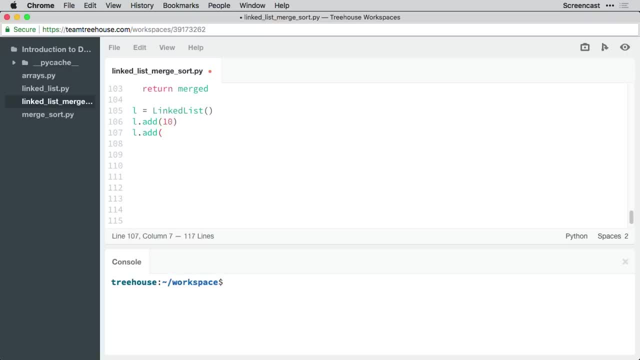 So it makes it easier for me Not to have to retype a bunch. So I'll add 10. Then say 2.. 44., 15. And something like 200.. Okay, Then we'll go ahead and print l. 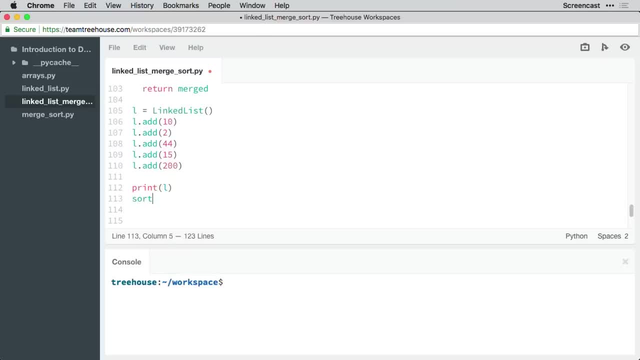 So that we can inspect this list. Next, Let's create a declare variable here, And to this we're going to assign The result of calling merge sort On l, And then we'll print this So sorted, Linked list. Okay, Since we've taken care of all the logic, 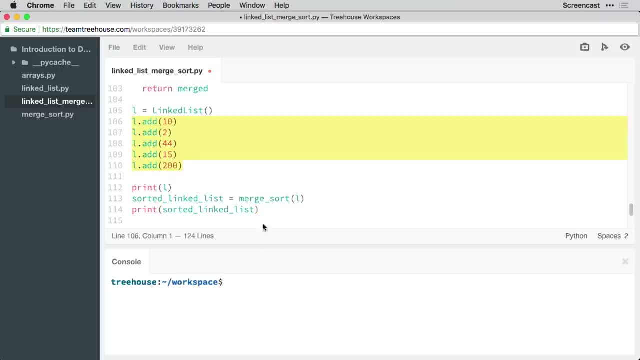 We know that this gets added in as nodes, And then Let's see what this looks like. Alright, So hit save And then bring up the console. We're going to type out python. Linked list. Underscore: merge sort dot pi. 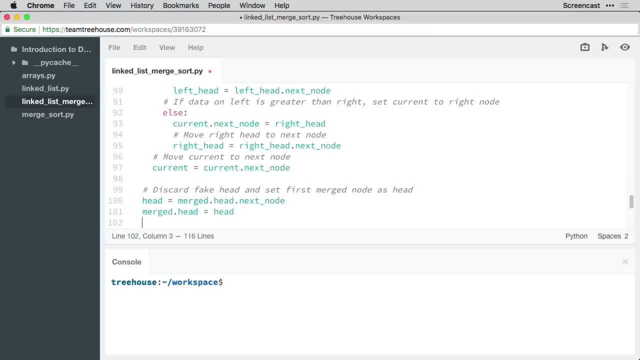 the cat program to complete and report the result. time cat numbers 5.txt. The real row in the results is the actual amount of time for when the program started running to when it completed. We can see it finished in a fraction of a second. 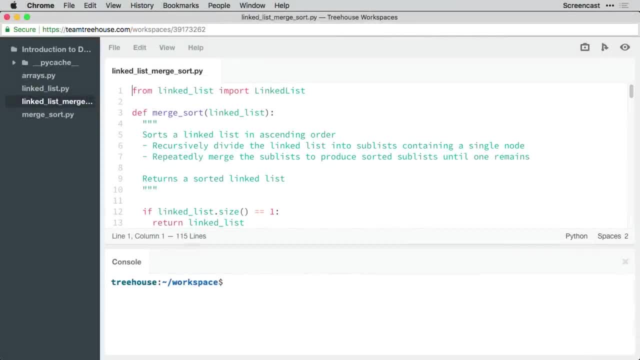 But, as we said, other programs running on the system can take CPU resources, resources, in which case your program will seem slower than it is. so we generally want to ignore the real result. The user result is the amount of time the CPU actually spent running the program code. 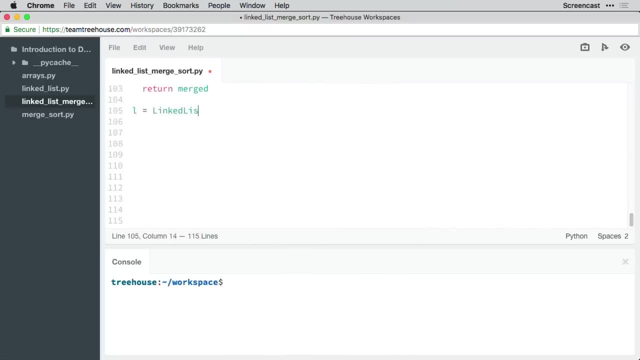 so this is the total amount of time the code inside the cat program took to run The sys. result is the amount of time the CPU spent running Linux kernel calls that your code made. The Linux kernel is responsible for things like network communications and reading files. 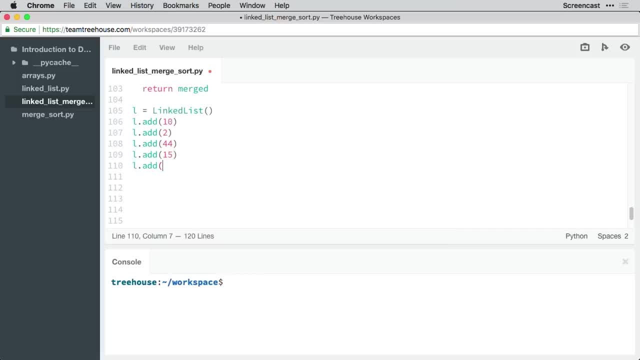 so loading the 5.txt file is probably included in this result. In evaluating code's performance, we're generally going to want to add together the user and sys results. but Cat is a very simple program. Let's try running the time command on our code and see if we get a more interesting. 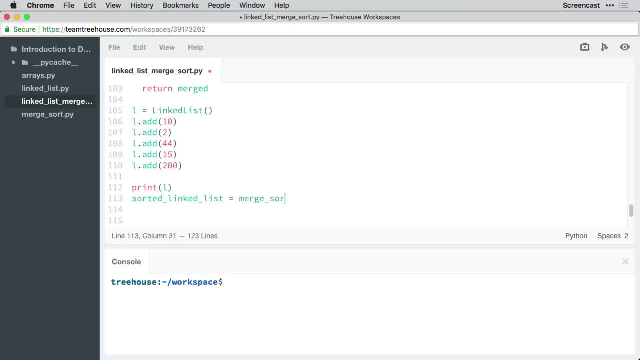 result: time: python selection-sortpy numbers 10000.txt. This takes much longer to complete- Nearly 12 seconds according to the real time measurement. But, as we said, the real result is often skewed, so let's disregard that. If we add the user and sys runtimes together, we get about 6 seconds. 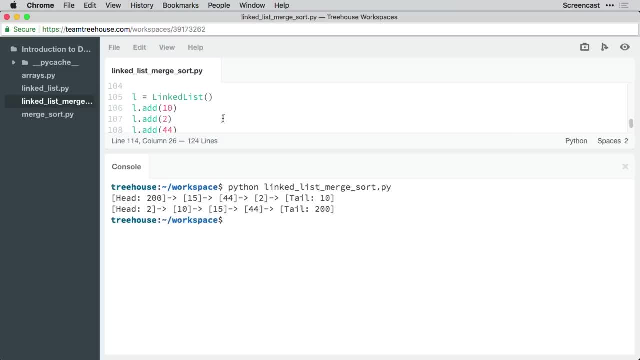 The time for the program to complete will vary a little bit each time you run it, but if it's doing the same operations it usually won't change more than a fraction of a second. If I run our selection sort script on the same file, you can see it completes in roughly. 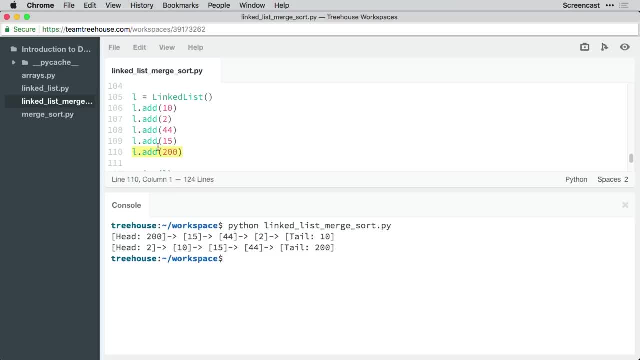 the same time. Now let's try it on another file with one million numbers: time python selection-sortpy numbers- 10000.txt. How long does this one take? I don't even know. While designing this course, I tried running this command and my workspace connection. 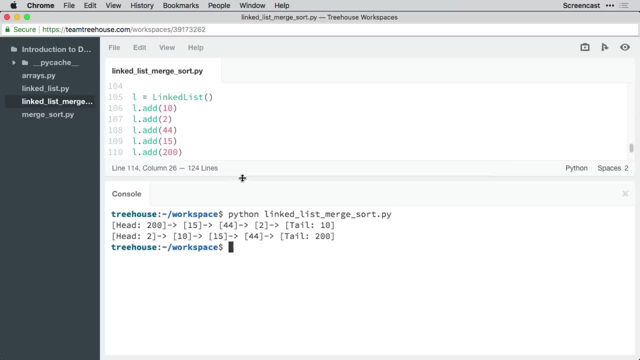 Enter. Okay, So we see that linked list we first created. Remember that what we add first, Right That eventually becomes a tail. Yeah, So 10 is the tail, 200 is the last one, So 200 is the head. 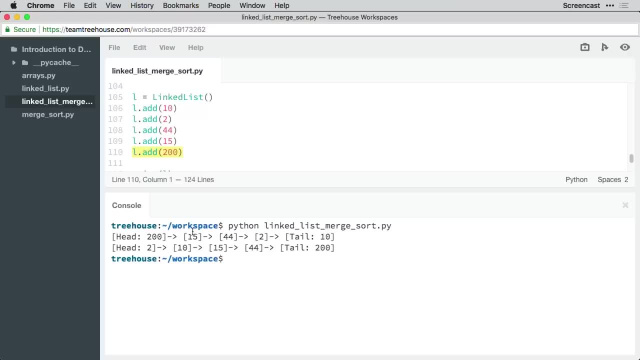 Because I'm calling add. It simply adds each one to the head of the list. So here we have 10,, 2,, 44,, 15, and 200. In the order we added, And then the sorted linked list sorts it out. 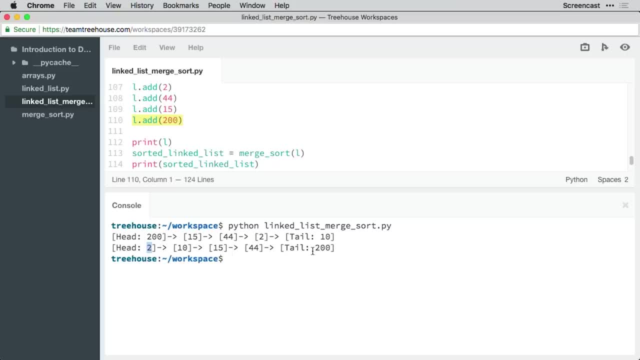 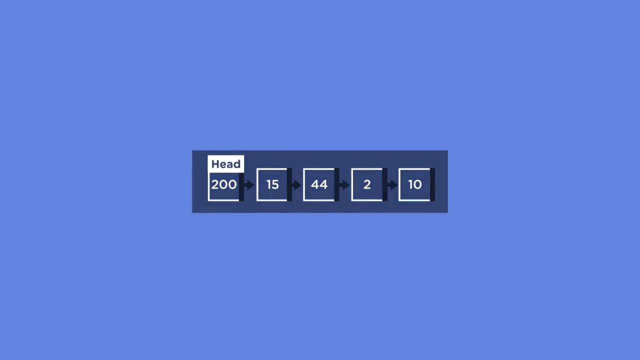 So it's 2,, 10,, 15,, 44, and 200.. Look at that, Okay. So let's visualize this from the top. We have a linked list containing 5 nodes With integers 10,, 2,, 44,, 15, and 200.. 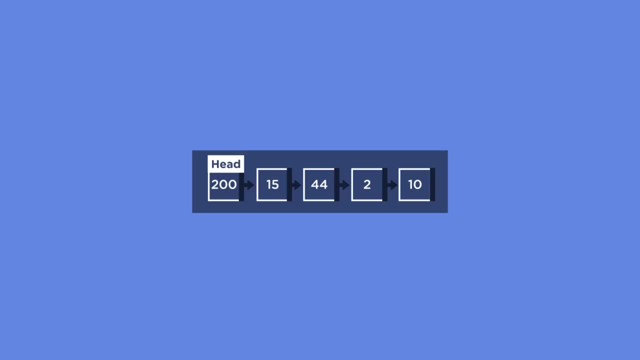 As data respectively. Our merge sort function calls split on this list. The split function calls size on the list And gets back 5. Which makes our midpoint 2.. Using this midpoint, We can split the list using the node at index method. 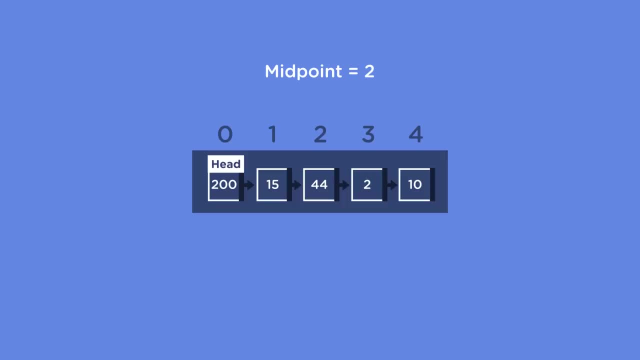 Remember that when doing this, We deduct 1 from the value of mid, So we're going to split here Using an index value of 1.. Effectively, this is the same, Since we're starting with an index value of 0.. 1 means we split after node 2. We assign the entire list to left half. Then create a new list And assign that to right half. We can assign node: 3. At index value. 2. As the head of the right list. 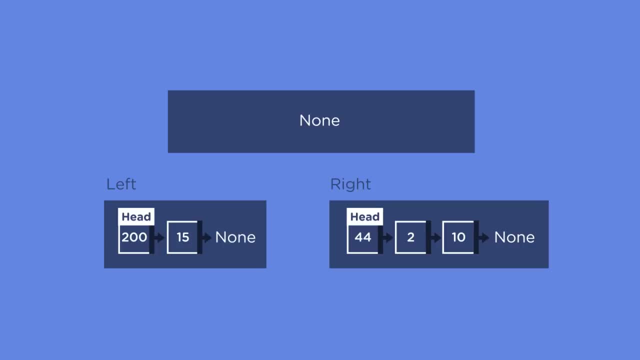 And remove the references between node 2. And node 3.. So far so good, Right. So now we're back in the merge sort function After having called split, And we have 2 linked lists. Let's focus on just the left half. 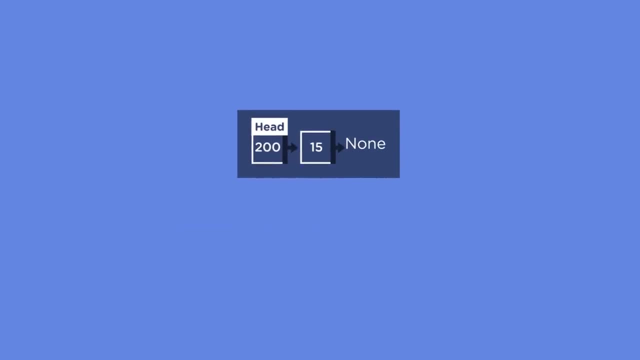 Because if you go back and look at our code, We're going to call merge sort On the left linked list again. This means the next thing we'll do Is run through that split process, Since this is a linked list containing 2 nodes. 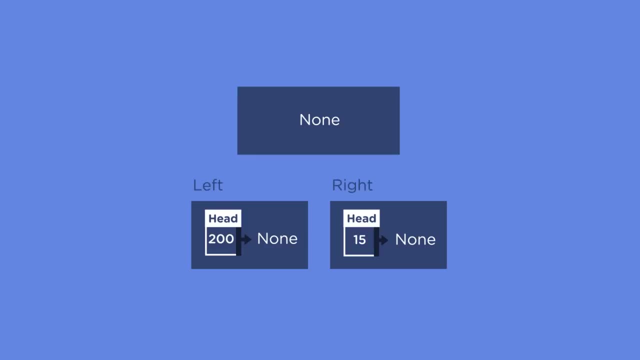 This means that split is going to return A new left and right list, Each with 1 node. Again we're back in the merge sort function, Which means that we call merge sort On this left list again, Since this is a single node linked list. 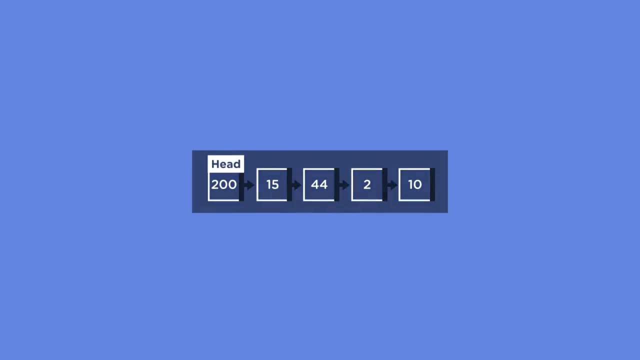 timed out before it completed. So we'll just say that selection sort takes a very, very long time to sort a million numbers. If we're going to sort a list that big, we're going to need a faster algorithm. We'll look into alternative sorting algorithms shortly. 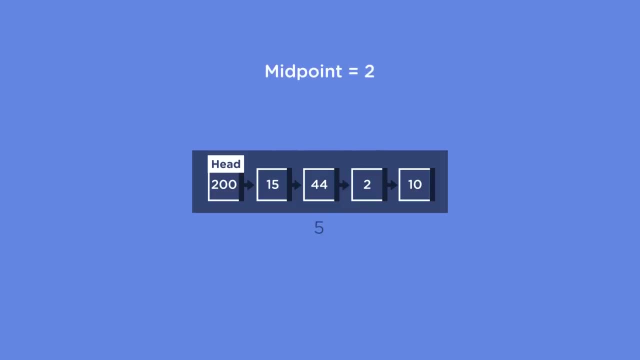 The next two sorting algorithms we look at will rely on recursion, which is the ability of a function to call itself. So before we move on, we need to show you how recursion works. Recursive functions can be very tricky to understand. Imagine a row of dominoes stood on end where one domino falling over causes the next domino. 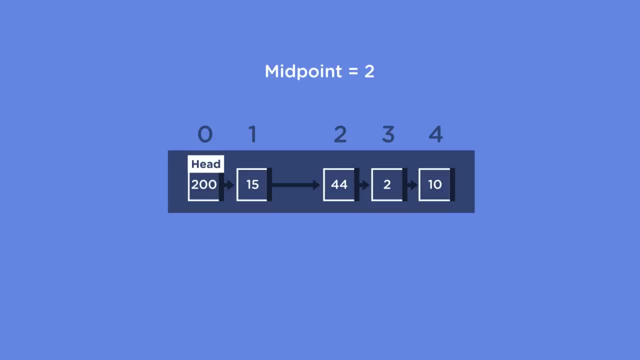 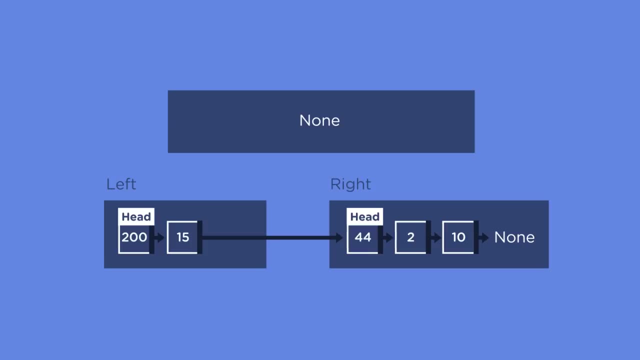 to fall over, which causes the next domino to fall over, causing a chain reaction. It's kind of like that. Let's suppose we need to write a function that adds together all the numbers in an array or, in the case of Python, a list. 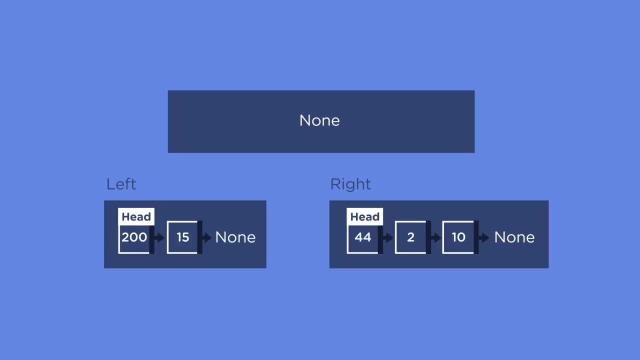 Normally we'd probably use a loop for this sort of operation. The function takes a list of the numbers we want to add. the total starts at 0,. we loop over every number contained in the list and we add the current number to the total. 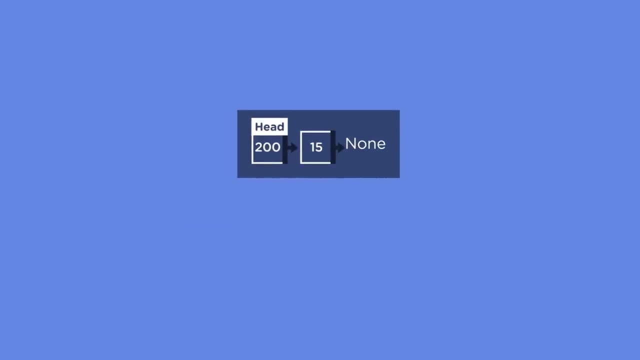 Once we're done looping, we return the accumulated total. If we call this sum function with a list of numbers, we'll get the sum function and the total. In other words, it'll return the total. When we run this program it'll print out that return value 19.. 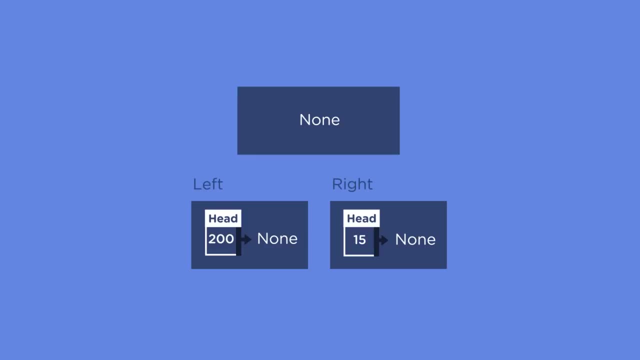 Let's try it real quick: Python recursionpy. oh, whoops, mustn't forget to save my work here And run it, and we see the result 19.. To demonstrate how recursion works, let's revise the sum function to use recursion instead. 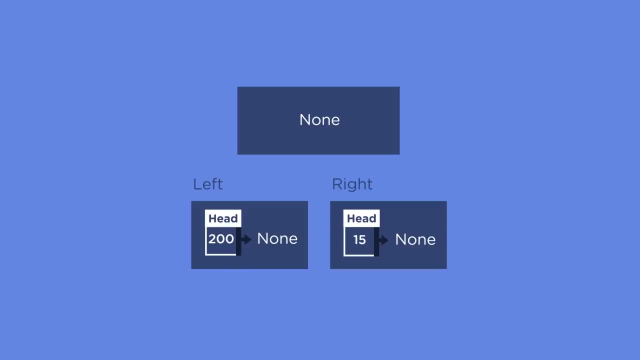 Note that recursion is not the most efficient way to add a list of numbers together, But this is a good problem to use to demonstrate recursion because it's so simple. One thing before I show you the recursive version, though: This example is going to use the Python slice syntax, so I need to take a moment to explain. 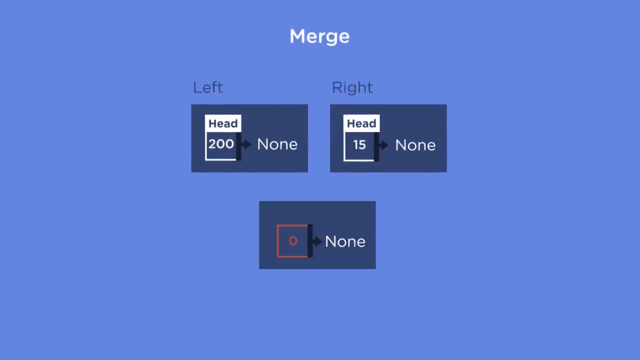 that, for those not familiar with it, A slice is a way to get a series of values from a list. Let's load up the Python REPL or read-evaluate-print loop so I can demonstrate. We'll start by creating a list of numbers to work with. 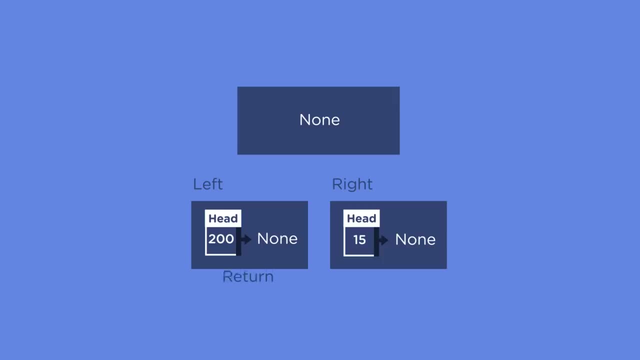 On calling merge sort on it. We immediately return Before we split, Since we hit that stopping condition. So we go to the next line of code, Which is calling merge sort on the right list as well, But again, we'll get back immediately. 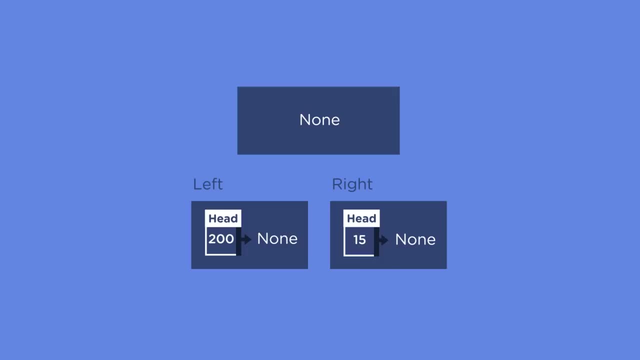 Because we hit that stopping condition. Now that we have a left and right That we get back from calling merge sort, We can call merge on them Inside the merge function. We start by creating a new linked list And attaching a fake head. 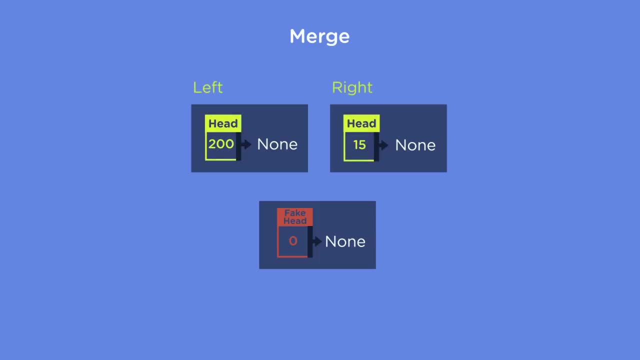 Then we evaluate whether either the left Or the right head is none. Since neither condition is true, We go to the final step, Where we evaluate the data in each node. In this case, the data in the right node Is less than the left node. 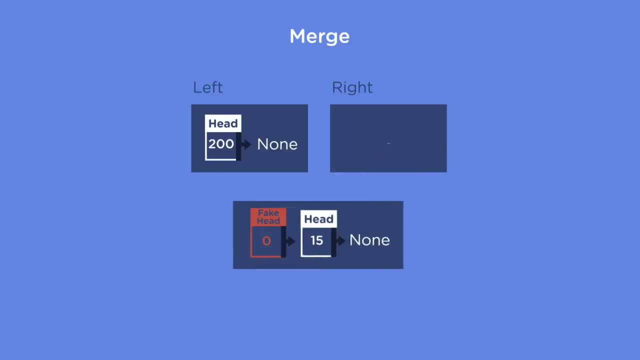 So we assign the right node As the next node in the merge linked list And move the right head pointer forward In the merge linked list. We move our current pointer forward To this new node we've added, Which completes one iteration of the loop. 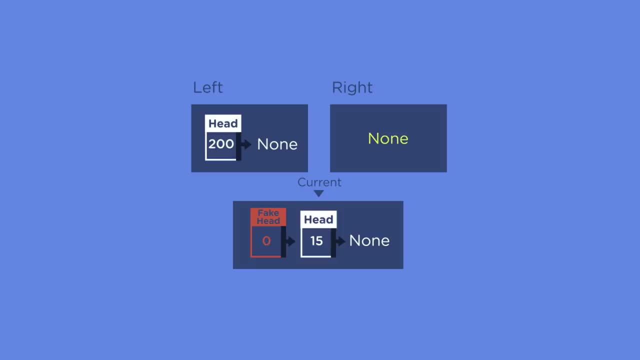 On the next iteration. Right head now points to none, Since that was a single node list And we can assign the rest Of the left linked list, Which is effectively the single node, Over to the merge linked list. Here we discard the fake head. 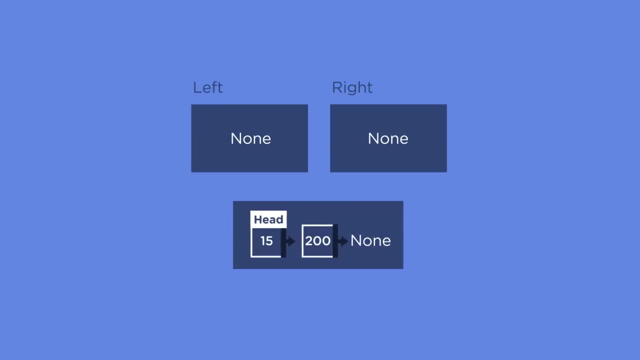 Move the next node up To be the correct head And return the newly merged, sorted linked list. Remember that at this point, Because right head and left head Pointed to, none Is terminated. So in this way we recursively split And repeatedly merge sub lists. 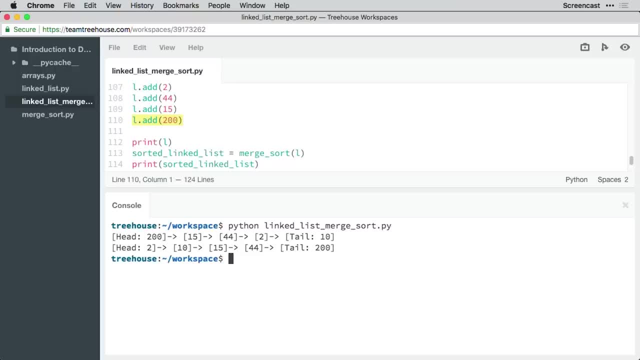 Until we're back with one sorted linked list. The merge sort algorithm Is a powerful sorting algorithm But ultimately it doesn't really do Anything complicated, It just breaks the problem down Until it's really simple to solve. Remember the technique here. 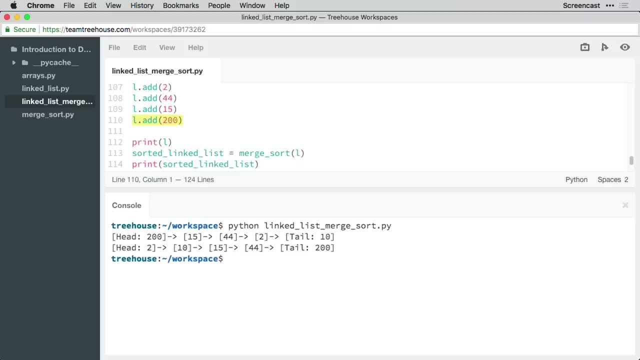 Which we've talked about before, Is called divide and conquer, So I like to think of merge, sort in this way. As a simple example, I've been working with a student Who has a bunch of books That she needs to sort. 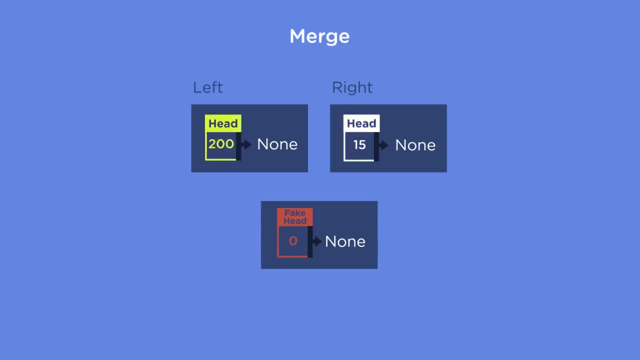 Numbers equals a list. We'll create a list of numbers. Number equals a list. Number equals a list, With 0,, 1,, 2,, 3, and 4 containing those numbers Like arrays. in most other languages, Python list indexes start at 0.. 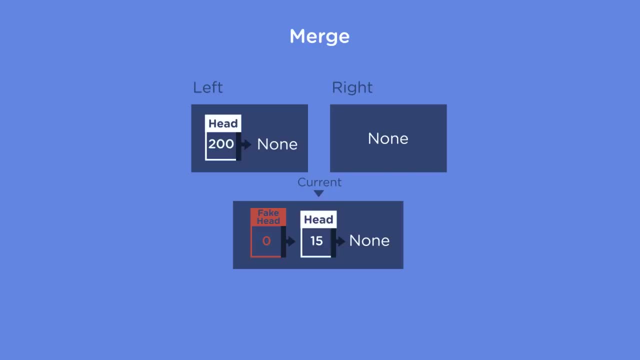 So numbers will actually get the second item from the list. With slice notation I can actually get several items back. It looks just like accessing an individual index of a list, But then I type a colon followed by the list index that I want up to but not including. 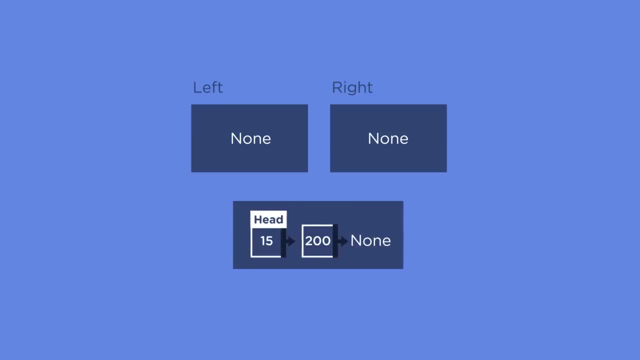 So numbers 1, colon 4 would get us the second up to, but not including the fifth items from the list, That is, it'll get us the second through the fourth items. Now I know what you're thinking and you're right. 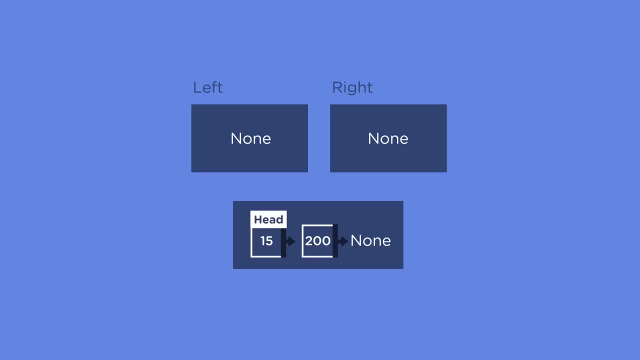 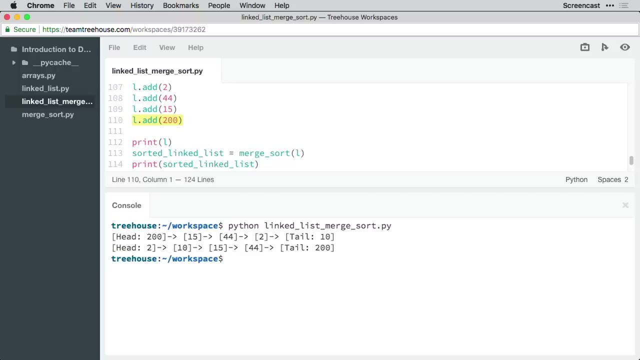 That up to, but not including rule is a little counterintuitive, but you can just forget all about it for now, because we won't be using a second index with any of our Python slice operations in this course. Here's what we will be using. 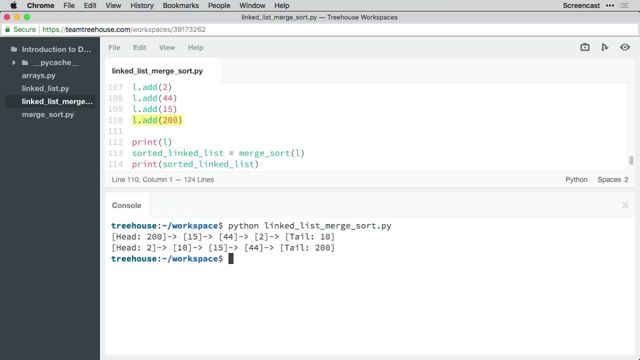 When you leave the second index off of a Python slice, it gives you the items from the first index up through the end of the list, wherever that is So numbers 1, colon with no index following. it will give us items from the second index. 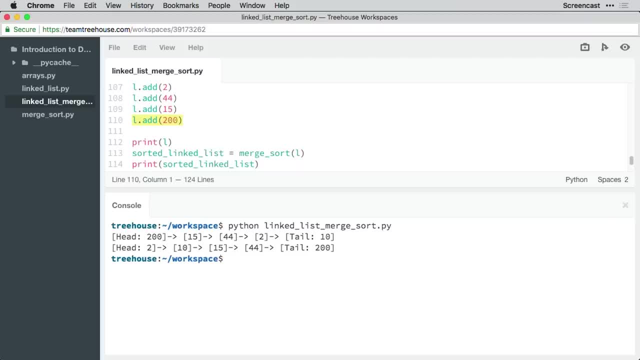 up through the end of the list. Numbers 2, colon will give us items from the third index up through the end of the list. You can also leave the first index off to get everything from the beginning of the list. Numbers colon 3 will get us everything from the beginning of the list. 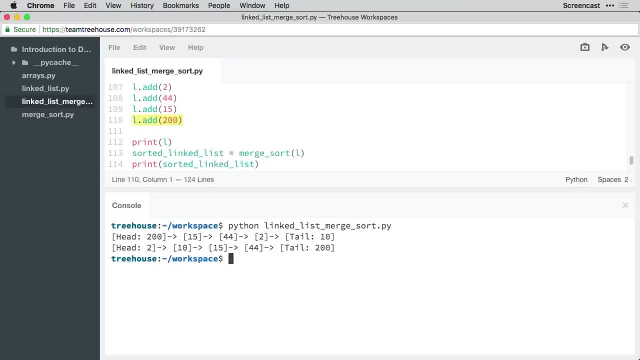 It's also worth noting that if you take a list with only one item and you try to get everything from the non-existent second item onwards, the result will be an empty list. So if I create a list with just one item in it and I try to access from the second element, 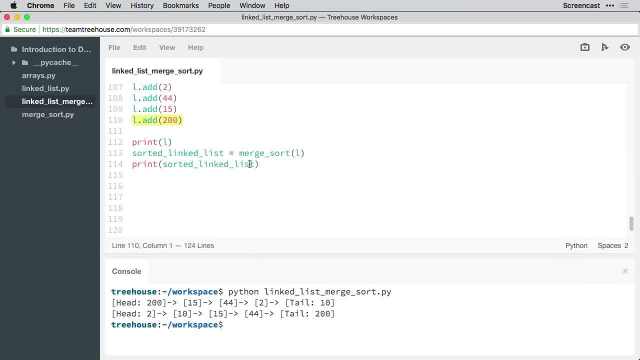 onwards. the second element doesn't exist, so the result will be an empty list. Don't worry too much. Don't worry too much about remembering Python slice syntax. It's not an essential part of sorting algorithms or recursion. I'm only explaining it to help you read the code you're about to see. 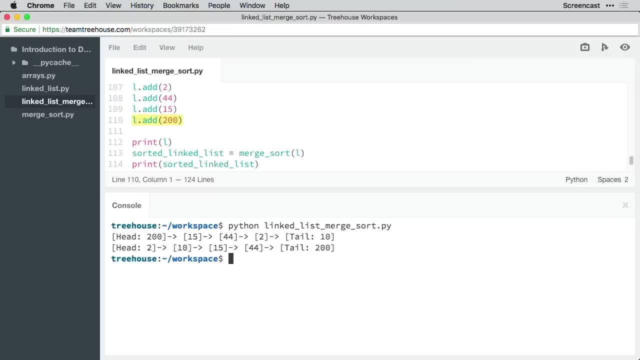 Into alphabetical order. Instead of doing all the work herself, She splits that pile into two And hands it to two students at the front. Each of those students Split it into two more And hand it to the four students Seated behind them. 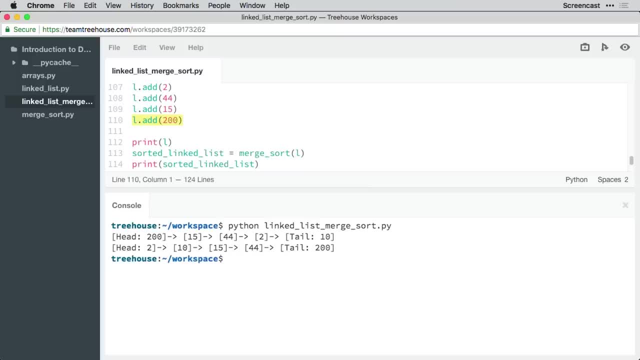 As each student does this, Eventually a bunch of single students Start to move this backwards. So ultimately It's really simple work. It's just efficiently delegated. Now back to our implementation. here Let's talk about run time So far, other than the node swapping, 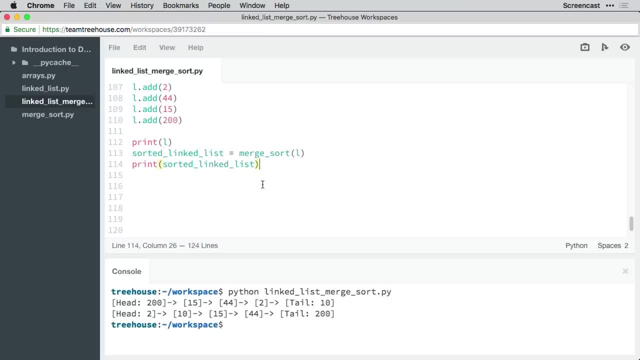 We had to do. It seems like most of our implementation Is the same right. In fact it is Including the problems that we ran into In the list version as well. So in the first implementation of merge sort, We thought we had an algorithm. 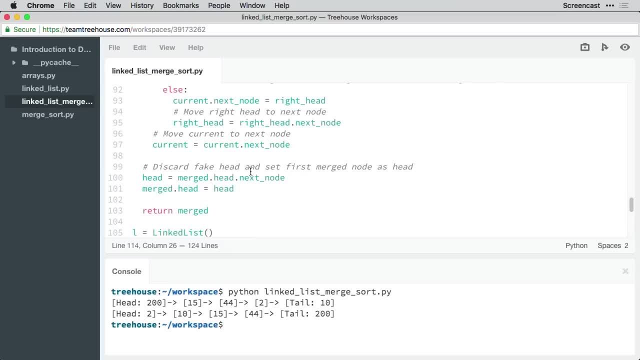 Well, the python list slicing operation, If you remember, Actually takes up some amount of time Amounting to big O of k. A true implementation of merge sort Runs in quasi linear Or log linear time, That is n times log n. 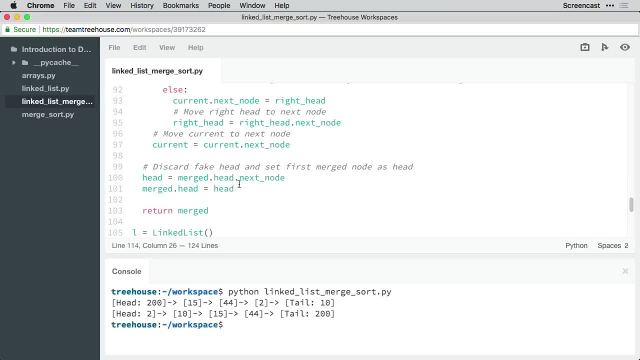 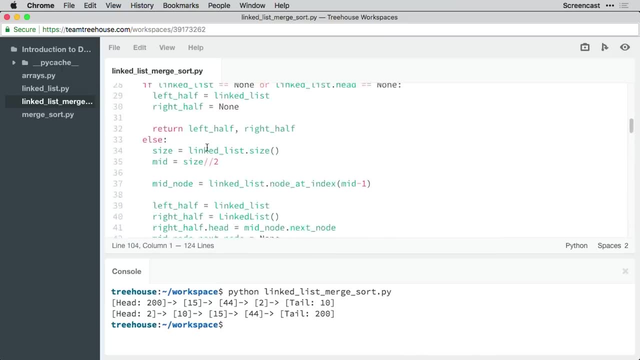 So we almost got there But we didn't. Now in our implementation of merge, sort On a linked list, We introduce the same problem. So if we go back up to the merge, Or rather the split function, The node references, That is a constant time operation. 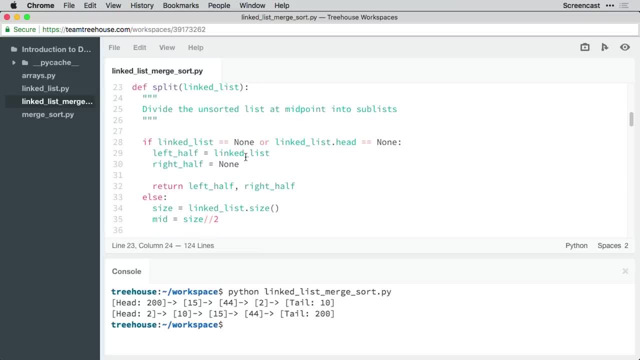 No big deal Comparing values. Also constant time. The bottleneck here, Like list slicing, Is in splitting a linked list At the midpoint. If we go back to our implementation, You can see here That we use the node at index method. 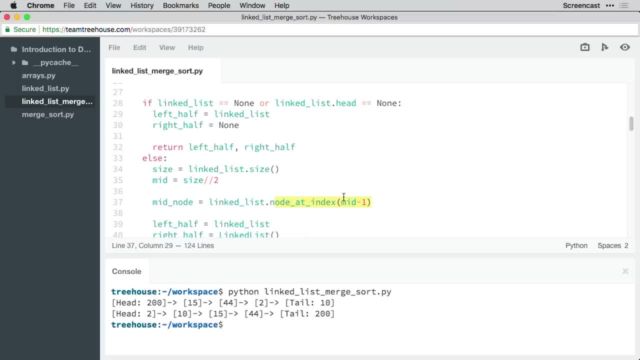 Which finds the node we want By traversing the list, Where k- here Is the midpoint of the list, Effectively n by 2.. Because we have to walk down the list, Counting up the index, Until we get to that node. 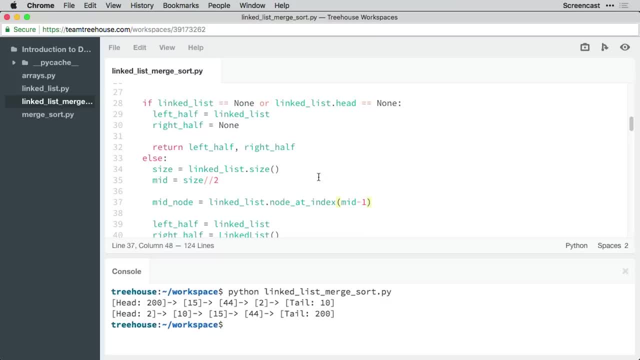 Given that overall splits Take logarithmic time, Our split function, Just like the one we wrote earlier, Incurs a cost of Big O of k log n. So here we'll say it takes Big O of k times log n. 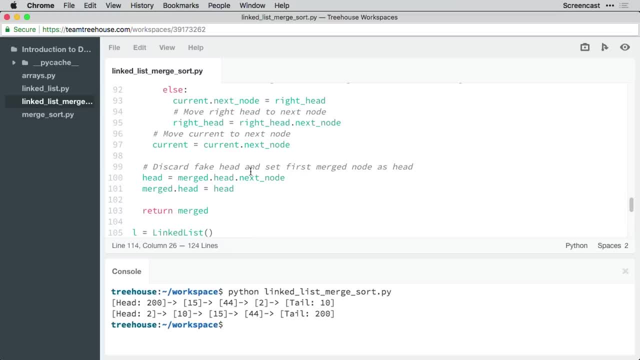 So I'm going to exit the Python REPL. Now that we've covered recursion, we can convert our SUM function to a recursive function. It'll take the list of numbers to add, just like before. Now here's the recursive part. We'll have the SUM function call itself. 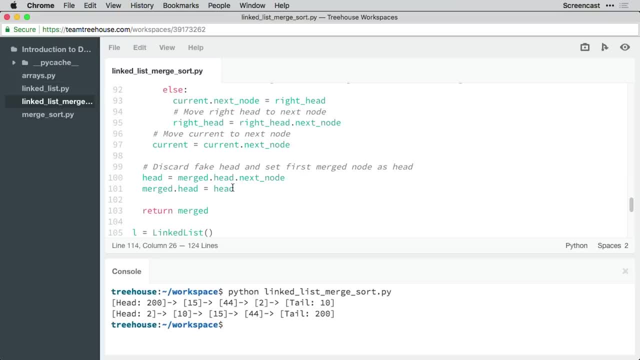 We use slice notation to pass the entire list of numbers Except the first one. Then we add the first number in the list to the result of the recursive function call and return the result. So if we call SUM with four numbers first, it'll call itself with the remaining three. 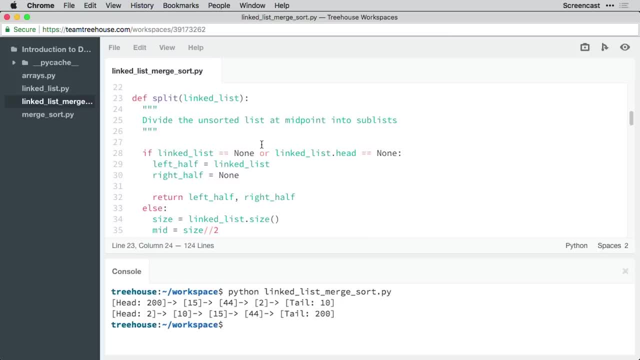 numbers That call to SUM will then call itself with the remaining two numbers and so on. But if we save this and try to run it python recursionpy- well first we get a syntax error. It looks like I accidentally did that. 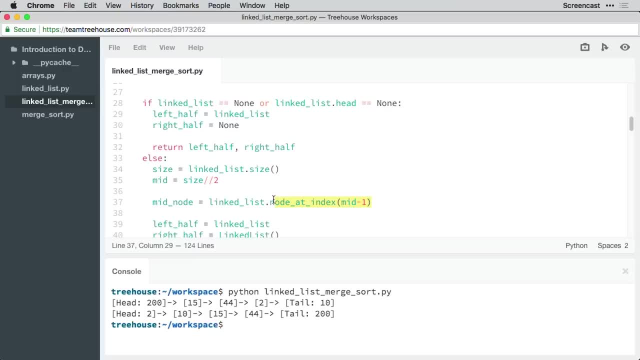 I accidentally indented something I shouldn't have, So let me go fix that real quick. There we go. That suggested to Python that there was a loop or something there when there wasn't. So let's go back to the terminal and try running this again. 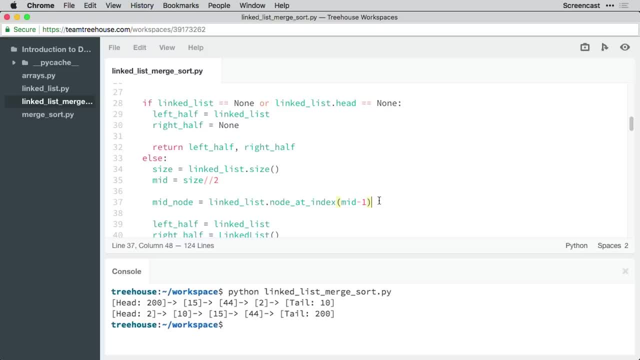 There we go. Now we're getting the error I was expecting: Recursion error. Maximum recursion depth exceeded. This happens because SUM gets into an infinite loop. It keeps calling itself over and over. The reason is that when we get down to a list of just one else, 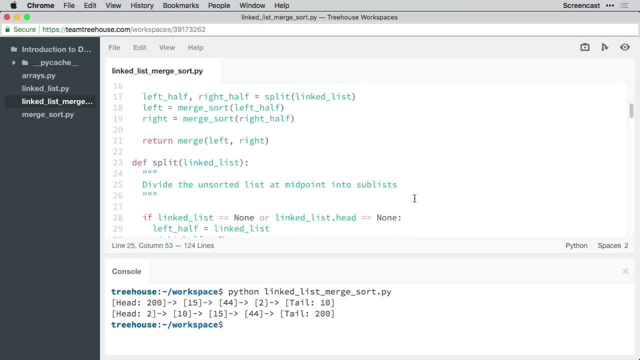 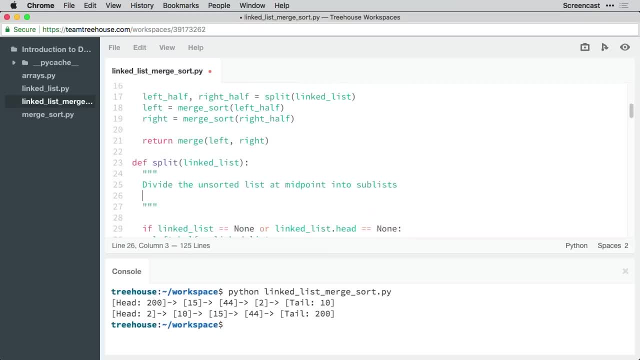 And we take a slice from the non-existent second element to the end. the result is an empty list. That empty list gets passed to the recursive call to SUM, which passes an empty list in its recursive call to SUM, and so on until the Python interpreter detects too many recursive. 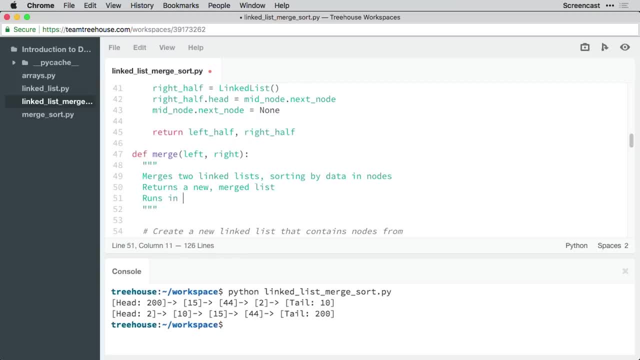 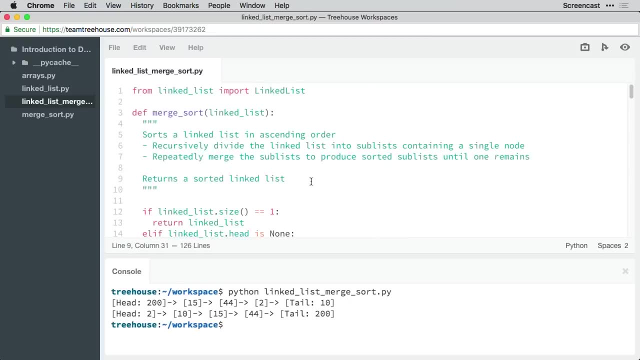 calls and shuts the program down. What we need is to add a base case to this recursive function, a condition where the recursion stops. This will keep it from getting into an infinite loop With the SUM function. the base case is when there are no elements. 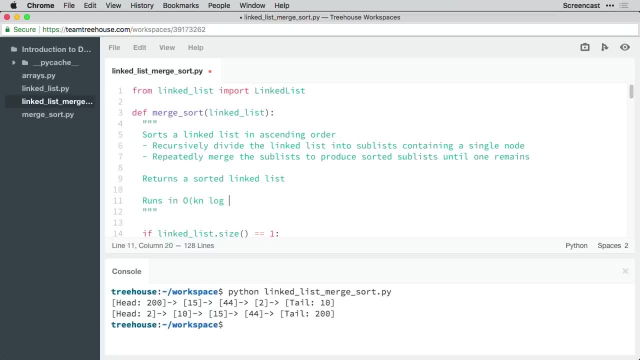 In that case, there is nothing left to add and the recursion can stop. A base case is the alternative to a recursive case, a condition where recursion should occur For the SUM function. the recursive case is when there are still elements in the list. 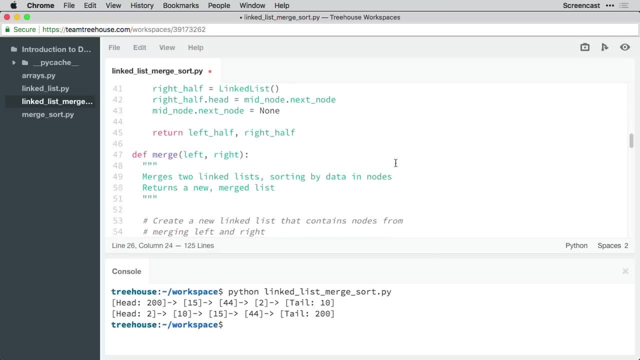 Now the merge function, Just like the one we wrote earlier, Takes linear time. So that one is good, That one runs in the expected amount of time. So here we'll say it runs in Linear time And that would bring our overall run time. 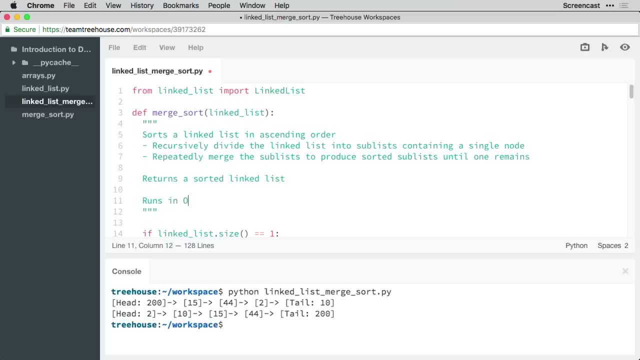 So up at the merge sort function, We can say this runs in Big O of k? n Times log n. It's okay, though. This is a good start, And one day, when we talk about constant factors And look at ways we can reduce. 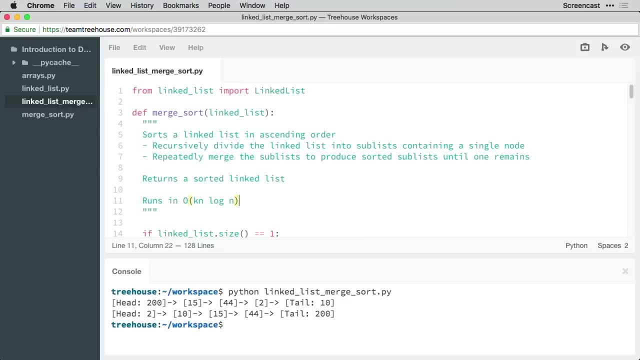 Our operations using different strategies. We can come back and reevaluate our code To improve our implementation. For now, as long as you understand How merge sort works conceptually, What the run time and space Complexities look like And where the bottlenecks are in your code, 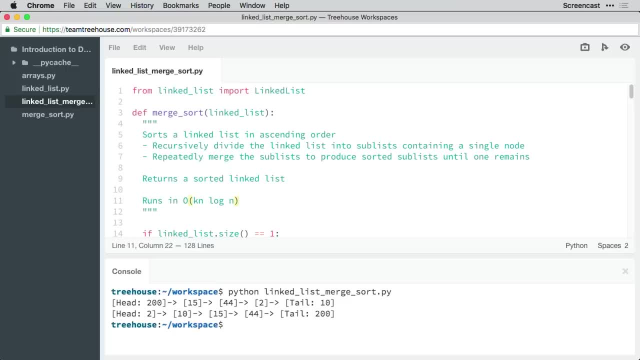 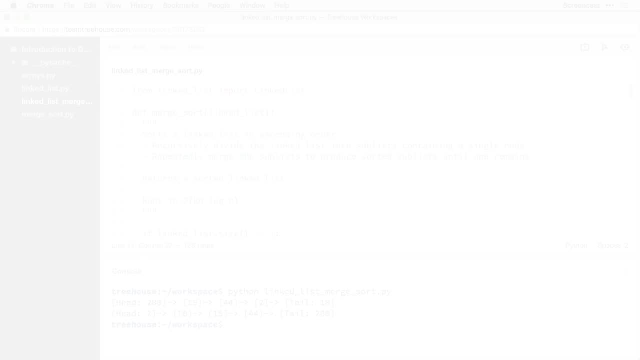 That's plenty of stuff. If you're interested in learning more About how we would solve this problem, Check out the notes in the teacher's video. In the next video, let's wrap this course up. And with that, Let's wrap up this course. 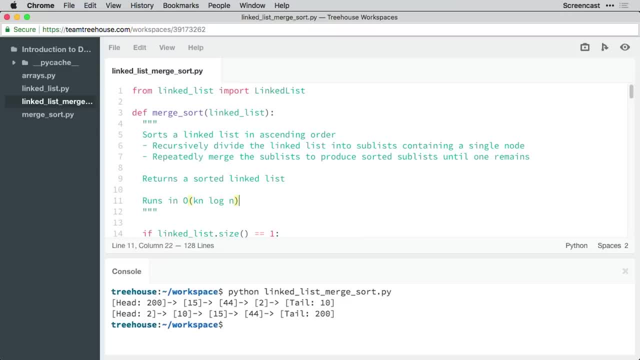 to add together. Let's add a base case at the top of the function. Python treats a list that contains one or more values as a true value and it treats a list containing no values as a false value. So we'll add an if statement that says: if there are no numbers in the list, we should 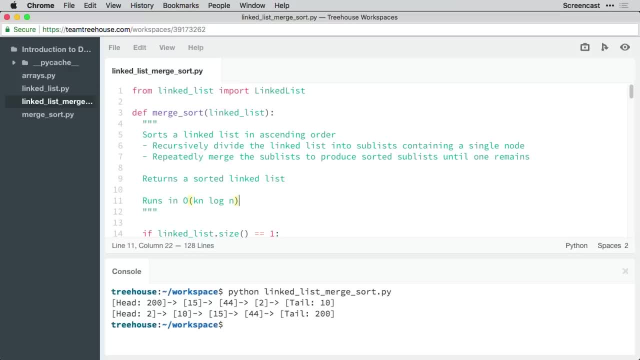 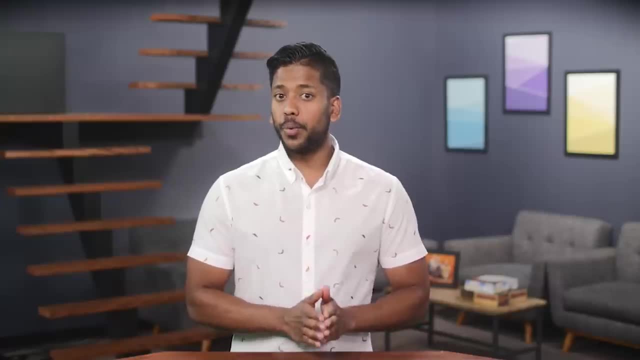 return a SUM of 0.. That way, the function will exit immediately without making any further recursive calls to itself. We'll leave the code for the recursive case unchanged. If there are still numbers in the list, the function will call itself with any numbers. after the first, then add the return value to the first number in the list. Let's save this and try running it again. Python recursionpy. Let's save this and try running it again. Python recursionpy. Let's save this and try running it again. 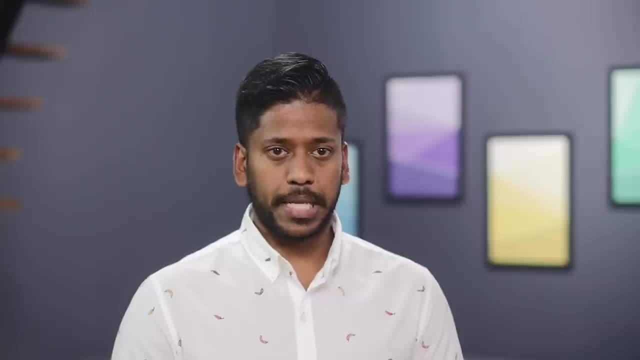 It'll output the sum of the numbers in the list 19.. But it's still not really clear how this worked. Let's add a couple print statements that will show us what it's doing. We'll show the recursive call to SUM and what it's being called with. 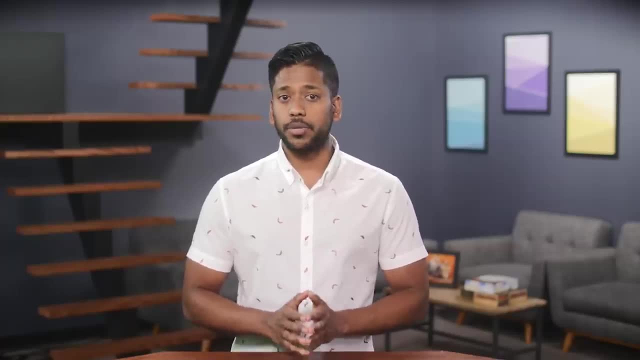 We'll also add a call to print right before we return, showing which of the calls to SUM is returning and what it's returning. Let's save this and try running it again. Let's save this and try running it again. 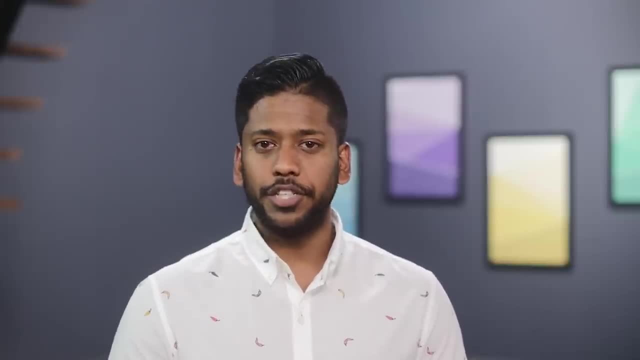 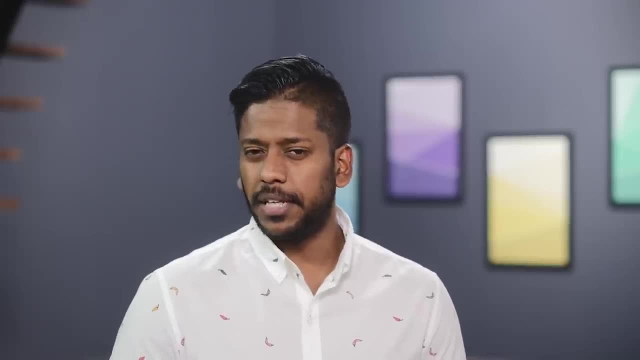 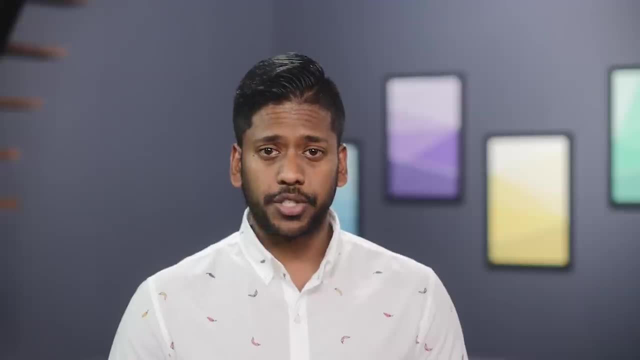 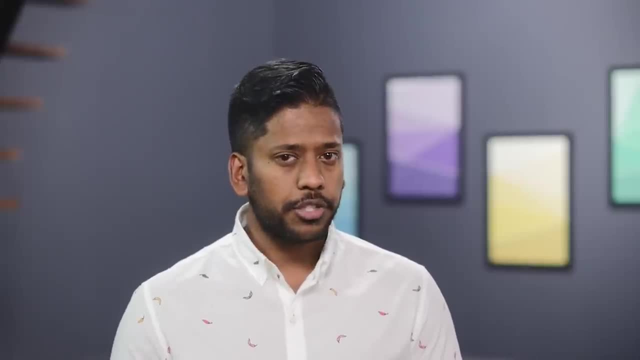 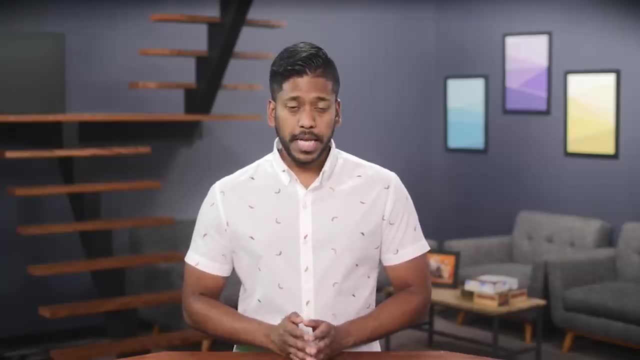 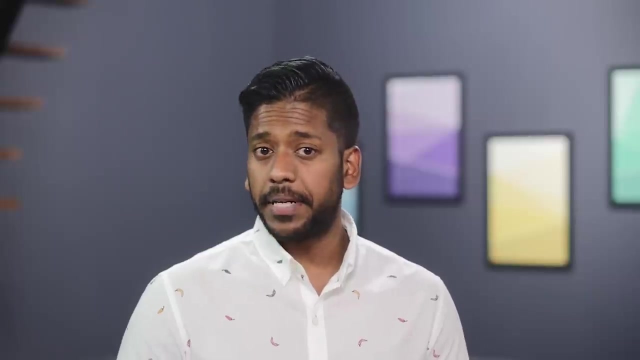 recursively. It passes the remaining items from the list 2,, 7, and 9.. That call to sum again ignores the first item in the list it receives, 2, and again calls itself recursively. It passes the remaining items in the list 7 and 9.. That call ignores the 7 and calls itself with a 9.. 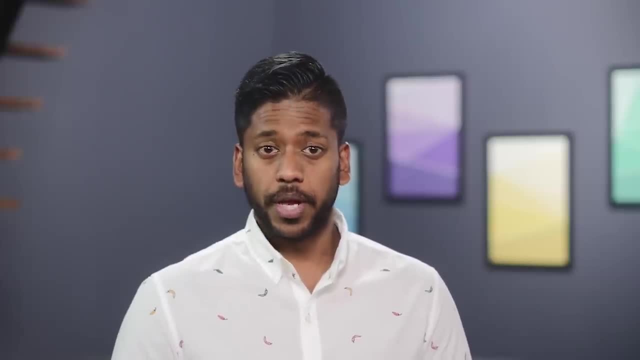 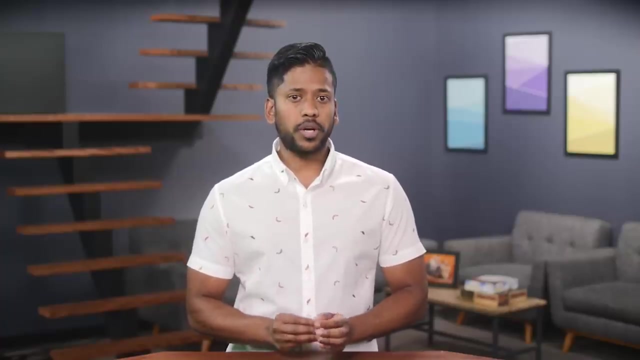 And the last call shown here ignores the 9 and calls itself with an empty list. At this point, none of our recursive calls to sum have returned yet. Each of them is waiting on the recursive call it made to sum to complete. Python and other programming languages use something called a call stack to keep track of this series of function calls. 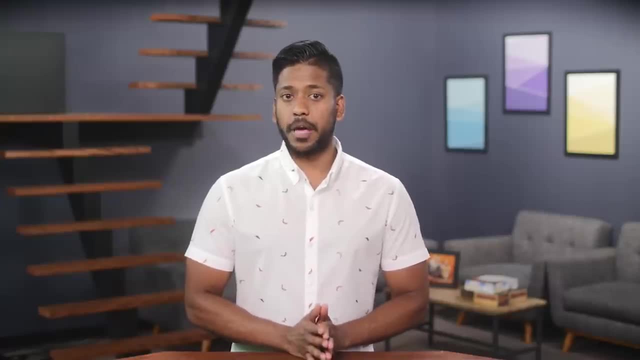 As an requisite to this course, Introduction to algorithms. We learned about basic algorithms, Along with some concepts like recursion And Big O that set the foundation For learning about implementing and evaluating algorithms. In this course, We learned what a data structure is. 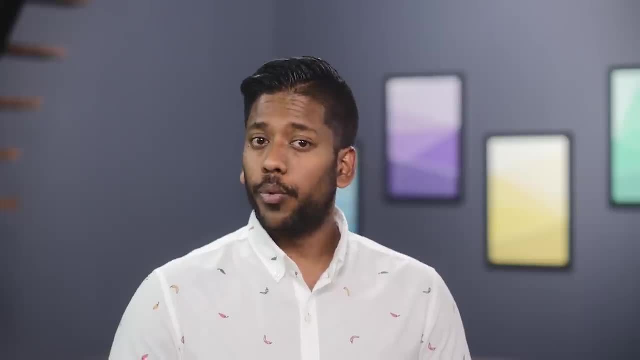 And how data structures go hand in hand With algorithms. We started off by exploring a data structure That many of us use in our day to day programming- Arrays, Or lists as they're known in Python. We took a peek under the hood. 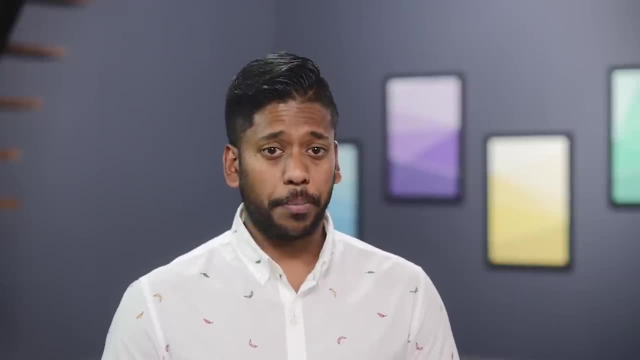 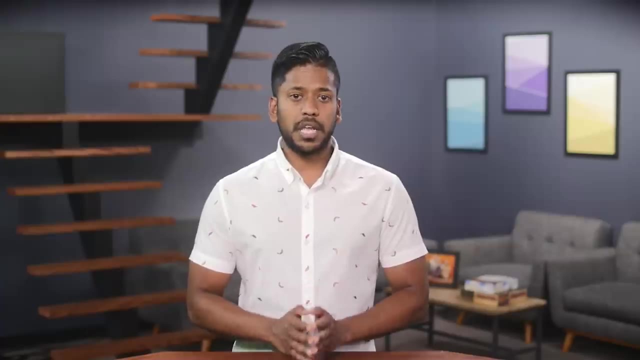 At how arrays are created and stored And examined some of the common operations Carried out on arrays. These are operations that we write And execute all the time, But here we took a step back And evaluated the run times of these operations. 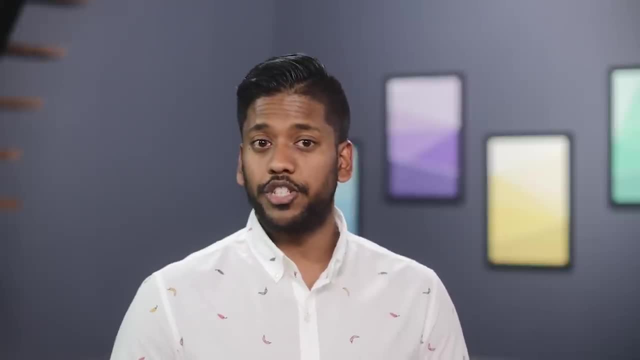 And how they affect the performance of our code. After that We jumped into an entirely new world Where we wrote our own data structure, A singly linked list. Admittedly, linked lists aren't used much In day to day problem solving. 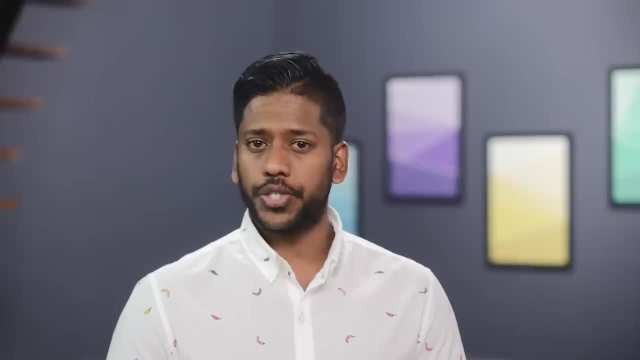 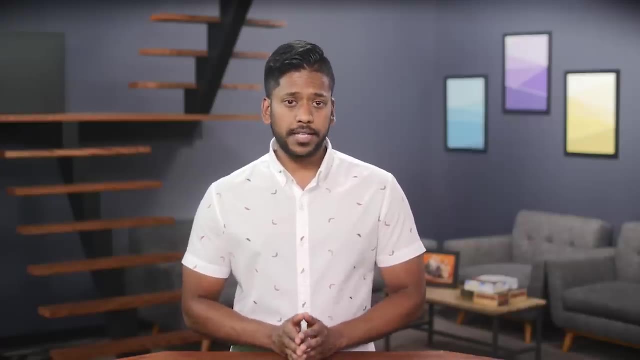 We needed a good data structure To start off with, Because it is fairly straight forward to understand And not that much different from an array. We carried out the same exercise As we did on arrays, In that we looked at common data operations. 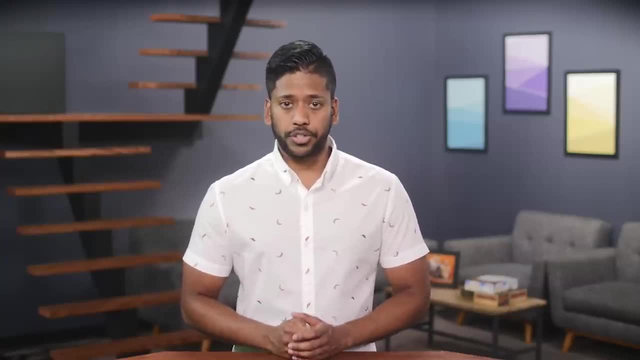 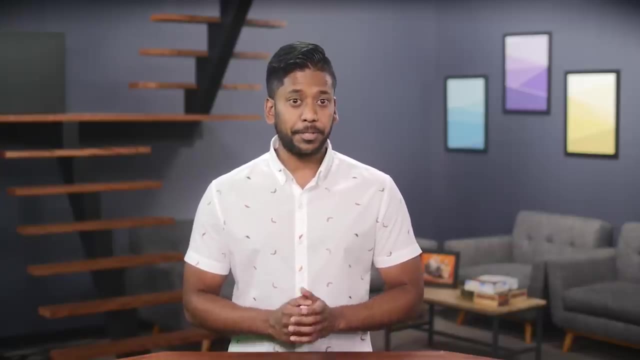 But since this was a type we defined on our own, We implemented these operations ourselves And got to examine, with a fine tooth comb, How our code And the structure of the type Affected the run time of these operations- The next topic we tackled. 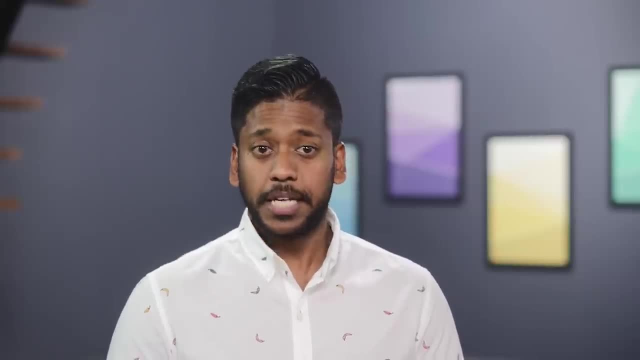 Was essentially worlds colliding With a sorting algorithm To sort two different data structures. Here we got to see How all of the concepts we've learned so far- Algorithmic thinking, Time and space, complexity And data structures- All come together to tackle the problem of sorting data. 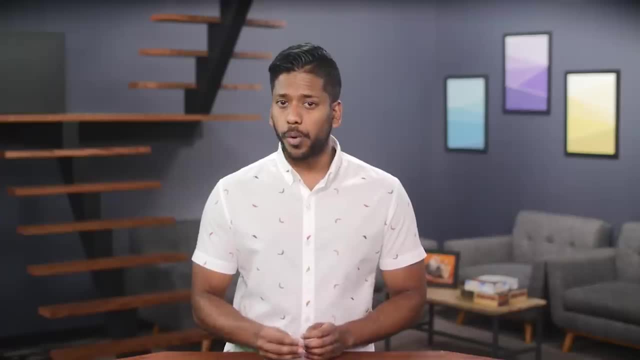 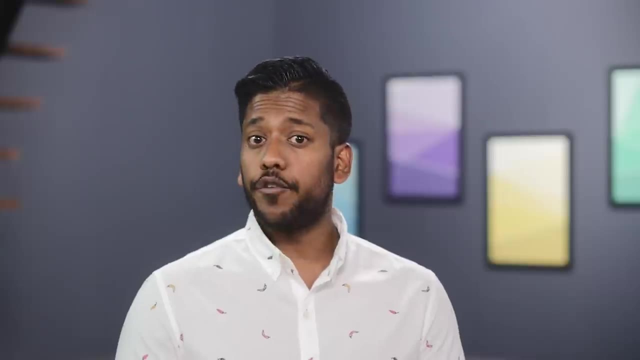 This kind of exercise Is one we're going to focus on moving forward As we try to solve more real world programming problems Using different data structures And algorithms. If you've stuck with this content so far, Keep up the great work. 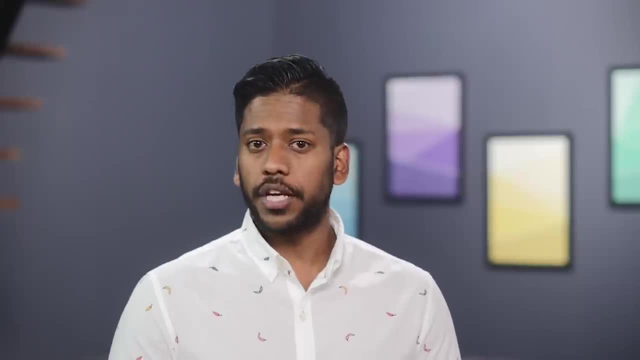 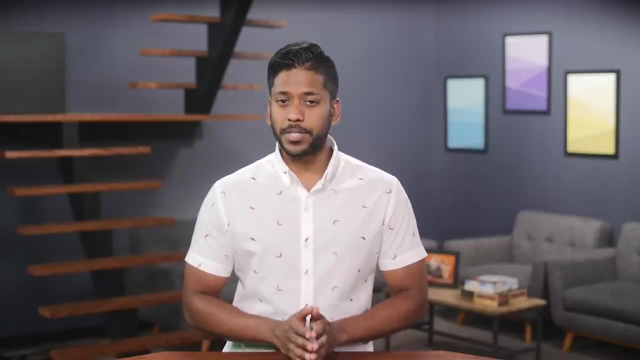 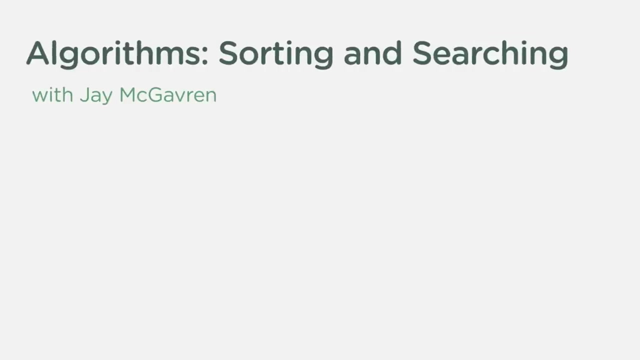 This can be a complex topic, But a really interesting one, And if you take your time with it, You will get a deeper understanding of programming And problem solving. As always, check the notes for more resources And happy coding. You may have heard that algorithms 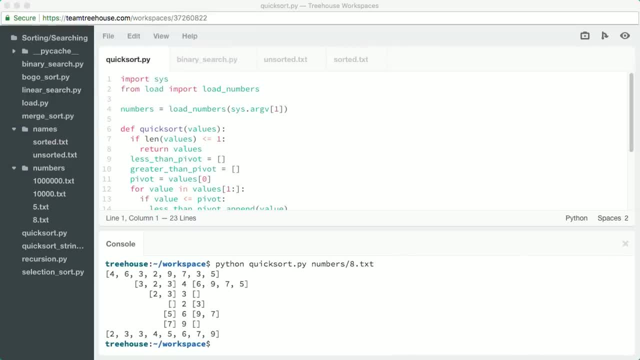 And computer science are boring Or frustrating, Especially the way some textbooks explain them. But once you understand what's going on, Algorithms can seem fascinating, Clever Or even magical. To help further your understanding of algorithms, This course is going to look at two categories. 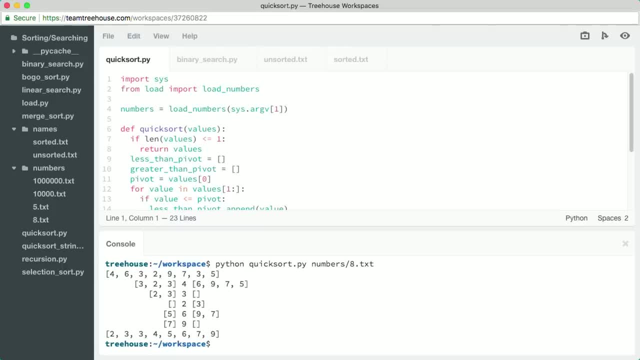 Sorting algorithms And searching algorithms. You could argue that these are the easiest kinds of algorithms to learn, But in learning how these algorithms are designed, We'll cover useful concepts Like recursion And divide and conquer That are used in many other sorts of algorithms. 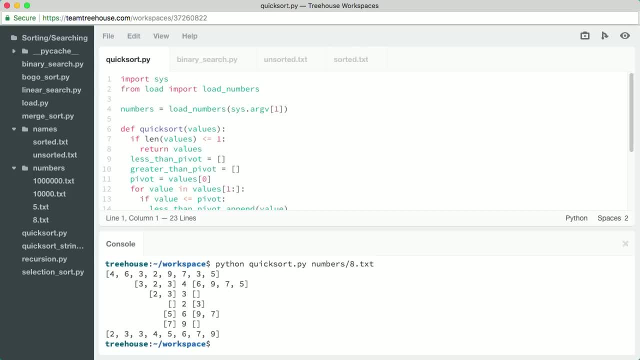 To create brand new ones. By the way, All the code samples I'm going to show in the videos Will be in Python, Because it's a popular language that's relatively easy to read, But you don't need to know Python to benefit from this course. 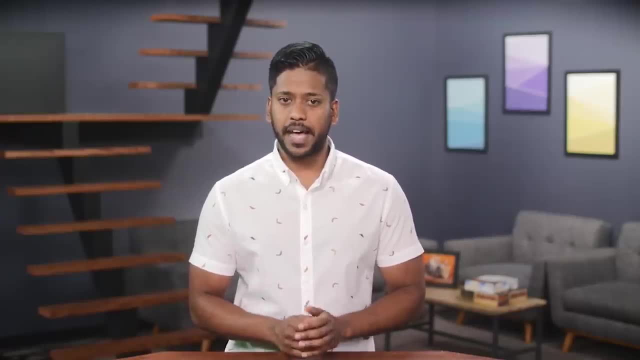 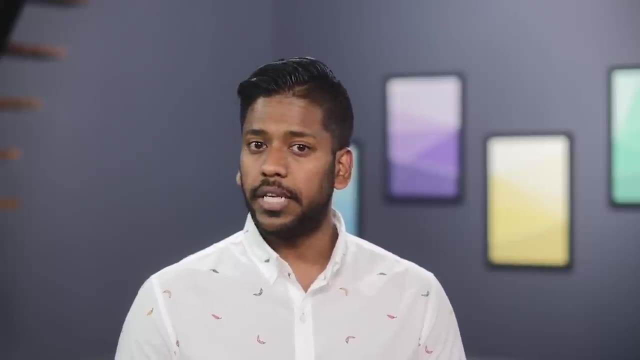 Each function call is added to the stack along with a place in the code that it needs to return when it completes. But now the empty list triggers the base case, causing the recursion to end and the sum function to return zero. That zero value is returned to its caller. 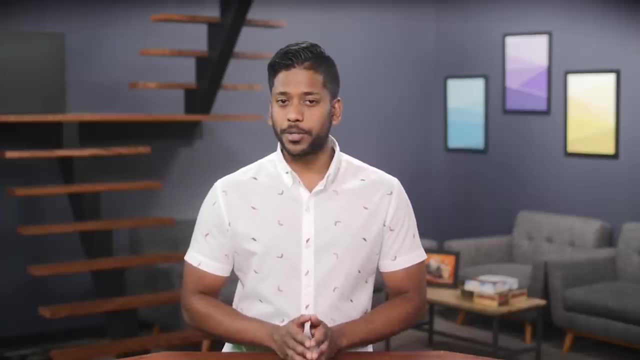 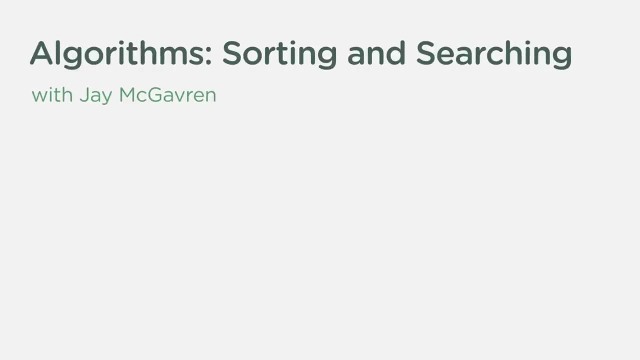 The caller adds the zero to the first and only value in its list. nine: The result is nine. That nine value gets returned to the caller, which adds it to the first value in the list it received. seven: The result is sixteen. 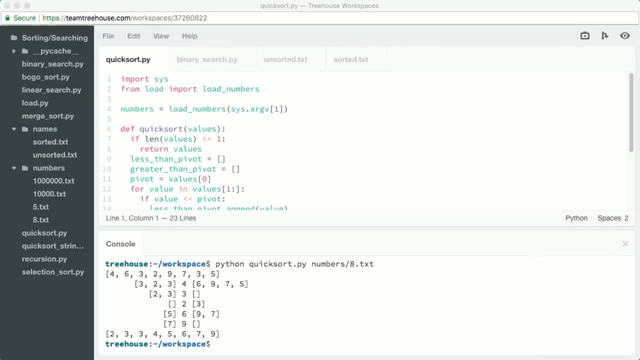 That sixteen value is returned to the caller, which adds it to the first value in the list it received. two. The result is eighteen. That eighteen value is returned to the caller caller, which adds it to the first value in the list it received, 1.. The result is 19.. 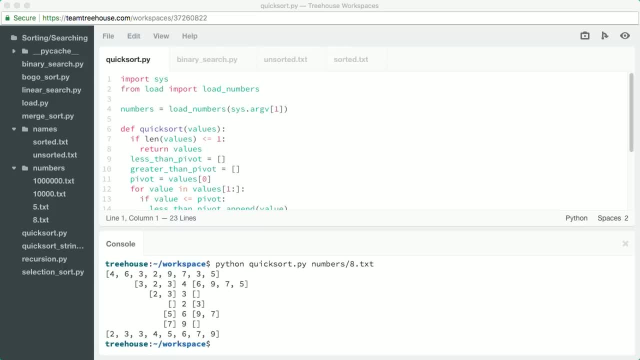 That 19 value is returned to the caller, which is not the SUM function recursively calling itself, but our main program. This is our final result, which gets printed. It's the same result we got from the loop-based version of our program. The end. We don't want the. 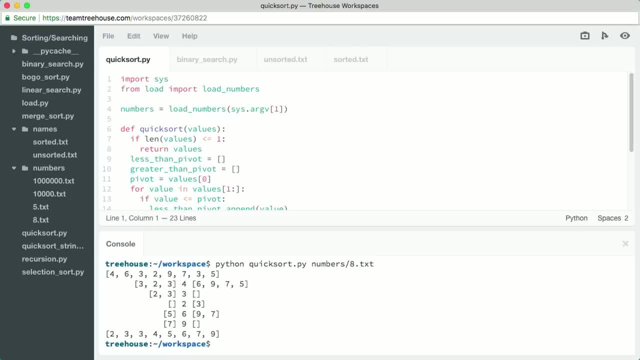 print statements in our final version of the program. so let me just delete those real quick. And there you have it: A very simple recursive function. Well, the function is simple but, as you can see, the flow of control is very complex. Don't worry if you didn't. 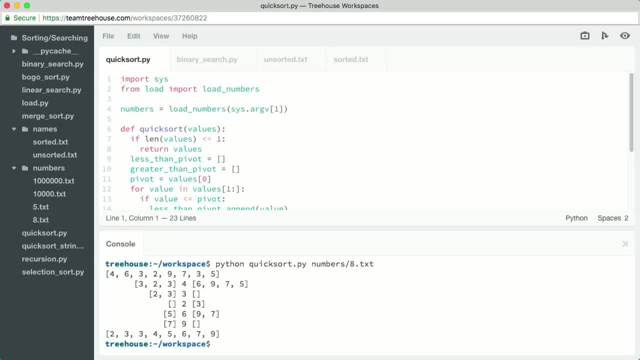 understand every detail here, because we won't be using this particular example again. There are two fundamental mechanisms you need to remember: A recursive function needs a recursive case that causes it to call itself, and it also needs to eventually reach a base case that causes the recursion to stop. 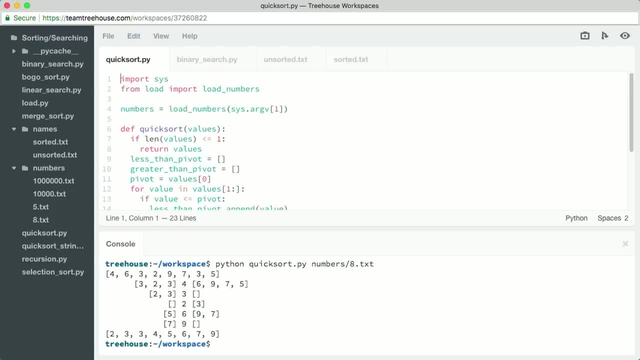 You've seen both the recursive function and the recursive function. They're both very BOGO sort which doesn't make any progress towards sorting a list. with each pass Either it's entirely sorted or it isn't. You've seen selection sort which moves one value over to a sorted list with. 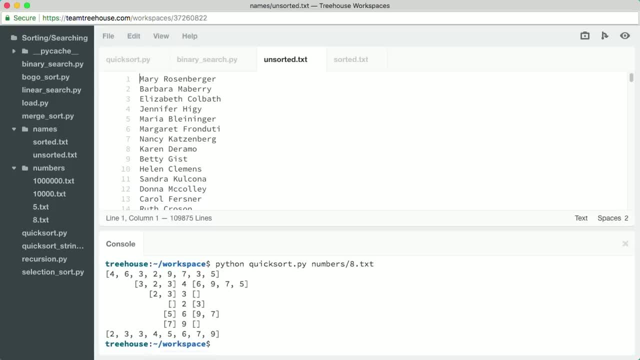 each pass so that it has fewer items to compare each time. Now let's look at an algorithm that speeds up the process further by further reducing the number of comparisons it makes. It's called quicksort. Here's some Python code where we'll implement quicksort. Again, you can ignore these. 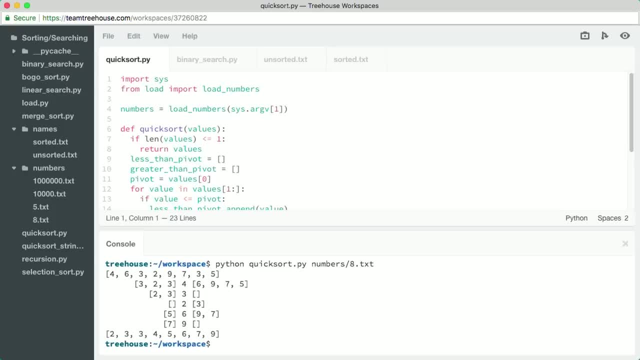 You can see the teacher's notes for each video For info on implementing these algorithms In your own favorite language. Our goal with this course Is to give you an overview of how sorting and searching algorithms work, But many algorithms Have details that can be handled in different ways. 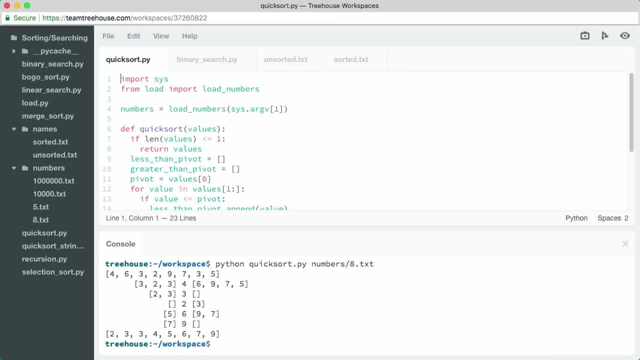 Some of these details May distract from the big picture, So let's put them in the teacher's notes instead. You don't need to worry about these When completing the course for the first time, But if you're going back and referring to it later. 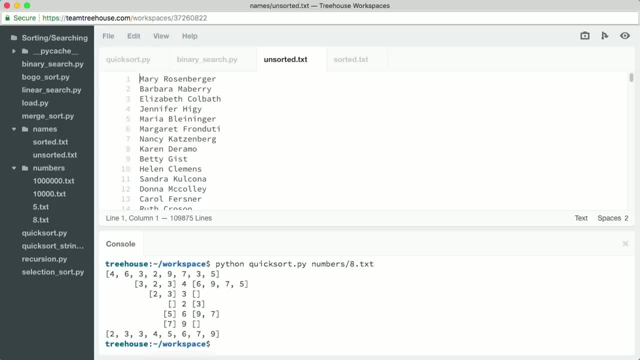 Be sure to check the teacher's notes for additional info. Suppose we have a list of names. It's a pretty big list, 100,000 names long. This list could be part of an address book Or social media app And we need to find the locations of individual names within the list. 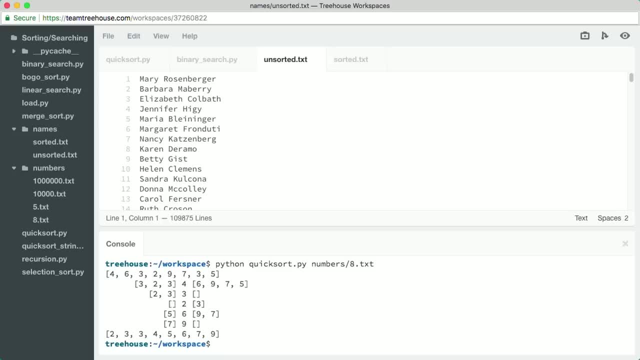 Possibly to look up additional data That's connected to the name. Let's assume there's no existing function In our programming language to do this. We want to make sure that the existing function Doesn't suit our purpose in some way For an unsorted list. 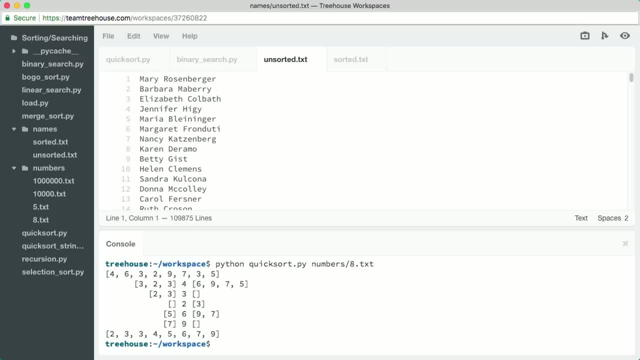 Our only option may be to use linear search, Also known as sequential search. Linear search is covered in more detail elsewhere on our site. Check the teacher's notes for a link. If you want more details, You start at the first element, You compare it to the value you're searching for. 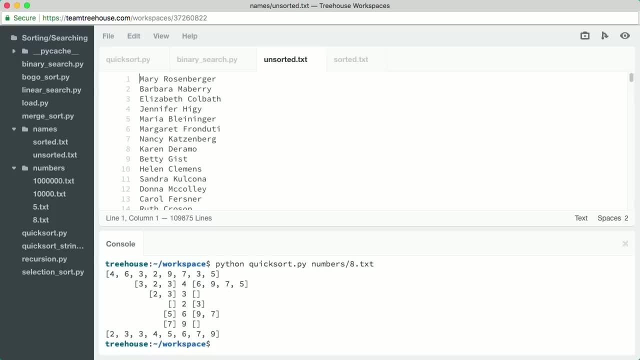 lines at the top. We're just using them to load a file full of numbers into a list. The quicksort algorithm relies on recursion. To implement it, we'll write a recursive function. We'll accept the list of numbers to sort as a parameter. Quicksort is recursive because it keeps calling itself with. 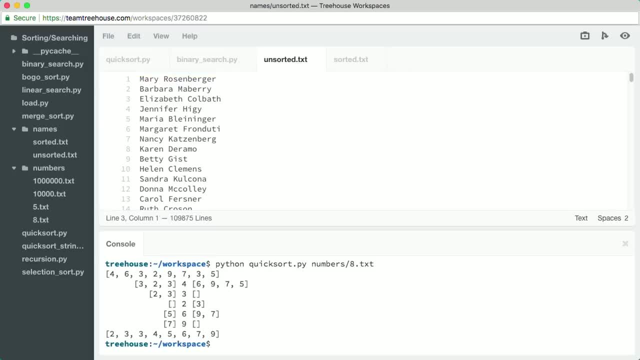 smaller and smaller subsets of the list you're trying to sort. We're going to need a base case where the recursion stops so it doesn't enter an infinite loop. Lists that are empty don't need to be sorted, and lists with just a number of numbers don't need to be sorted. We're going to need a. 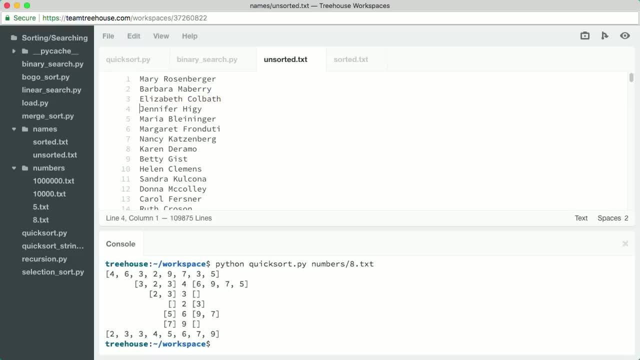 recursive case where just one element don't need to be sorted either. In both cases there's nothing to flip around, so we'll make that our base case. If there are zero or one elements in the list passed to the quicksort function, we'll return the unaltered list to the caller. Lastly, we need to 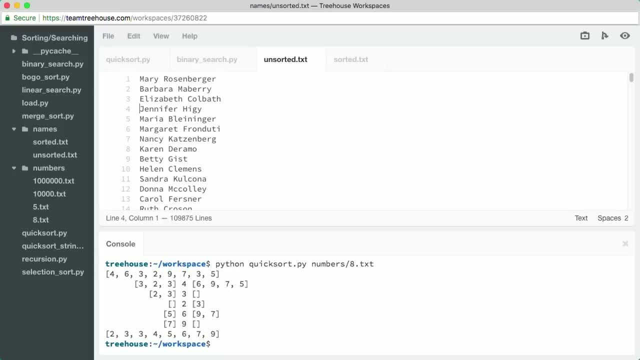 call our quicksort function with our list of numbers and print the list it returns. That takes care of our base case. Now we need a recursive case. We're going to rely on a technique that's common in algorithm design called divide-and-conquer. Basically, we're going 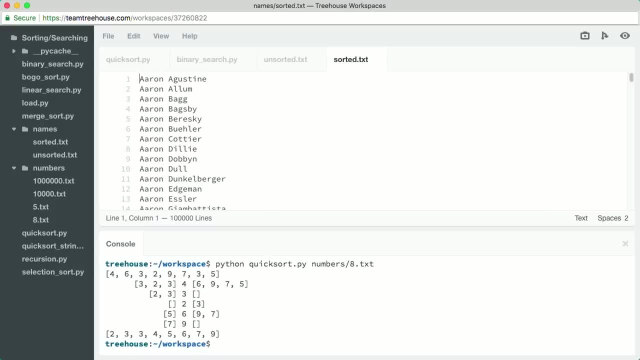 to take our problem and split it into smaller and smaller problems until they're easy to solve. In this case, that means taking our list and splitting it into smaller lists. Viewers, a suggestion. The process I'm about to describe is complex. There's just no way. 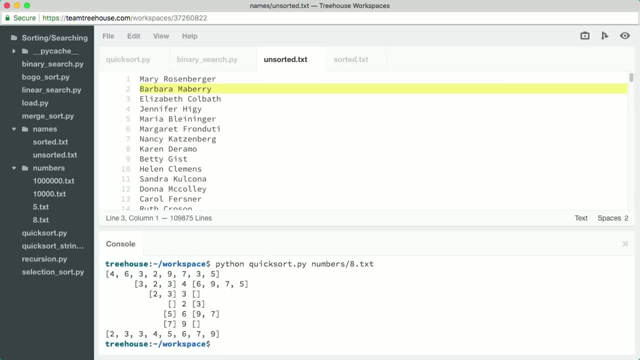 If it's a match, You return it, If not, You go to the next element, You compare that to your target And you go on through the whole list. The problem with this Is that you have to search the entire list. 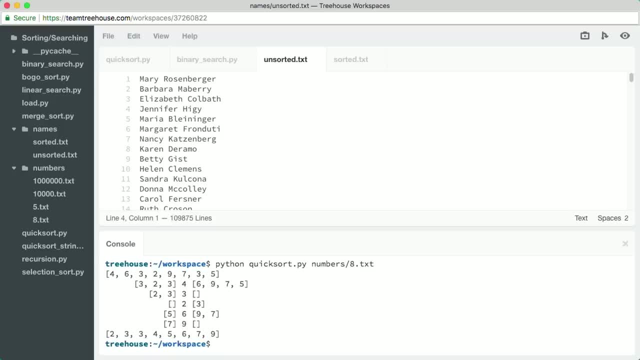 Every single time We're not doing anything to narrow down the search. each time We have to search all of it. If you're searching a big list Or searching it repeatedly, This amount of time can slow your whole lap down To the point that people may not want to use it anymore. 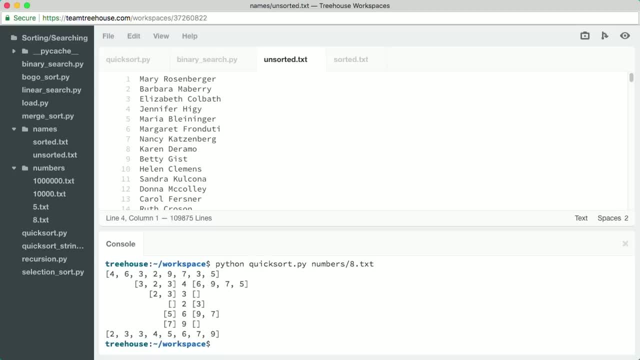 That's why it's much more common To use a different algorithm for searching lists: Binary search. Binary search is also covered in more detail elsewhere on our site. Binary search is also covered in more detail elsewhere on our site. Check the teacher's notes for a link. 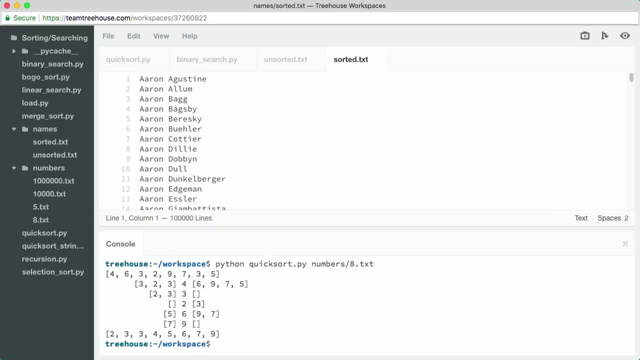 Binary search does narrow the search down for us. Binary search does narrow the search down for us. Specifically, it lets us get rid of half the remaining items we need to search through each time. Specifically, it lets us get rid of half the remaining items we need to search through each time. 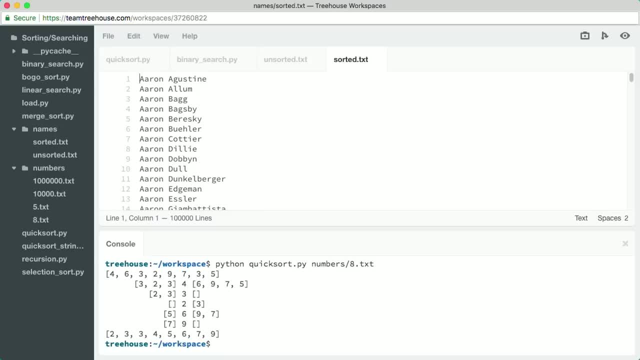 It does this by requiring that the list of values be sorted. It does this by requiring that the list of values be sorted. It looks at the value in the middle of the list. It looks at the value in the middle of the list If the value it finds is greater than the target value. 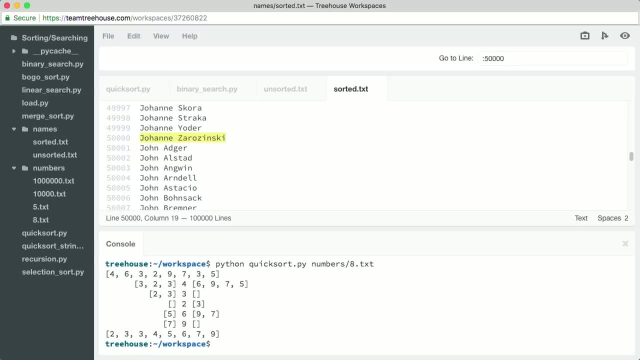 It ignores all values after the value it's looking at. It ignores all values after the value it's looking at. If the value it finds is less than the target value. It ignores all values before the value it's looking at. the value it's looking at, Then it takes the set of values that remain and looks at the value in. 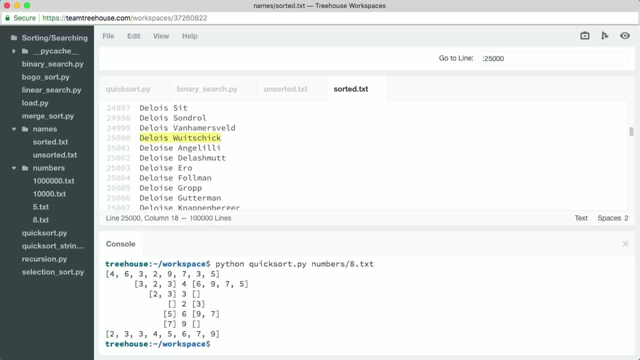 the middle of that list. Again, if the value it finds is greater than the target value, it ignores all values after the value it's looking at. If the value it finds is less than the target value, it ignores all values before the value it's looking at. But, as we mentioned, binary search: 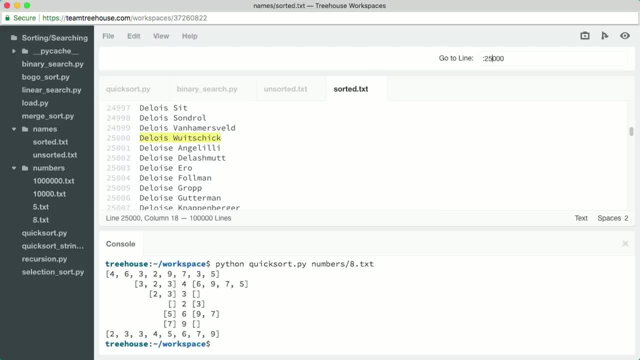 requires the list of values you're searching through to be sorted. If the list weren't sorted, you would have no idea which half of the values to ignore, because either half could contain the value you're looking for. You'd have no choice but to use linear search. So before we can use 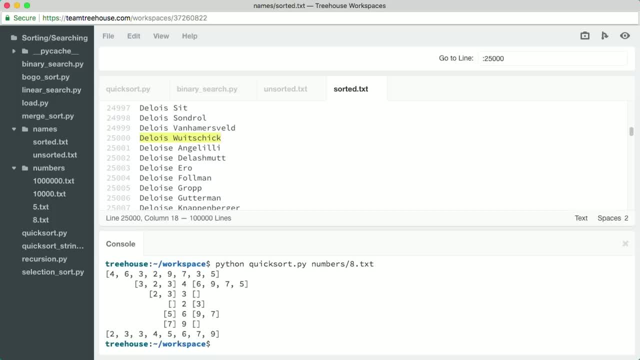 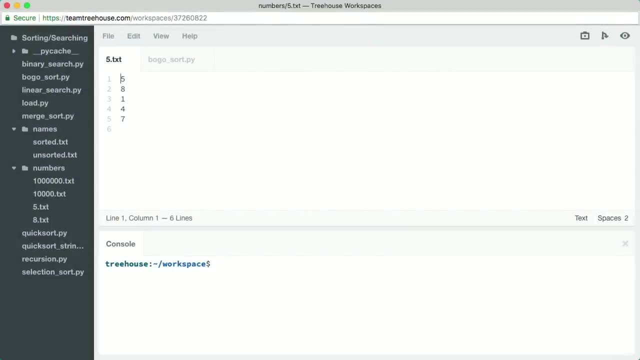 binary search on a list, we need to be able to sort that list. We'll look at how to do that next. Our end goal is to sort a list of names, but comparing numbers is a little easier than comparing strings, so we're going to start by sorting a list of numbers. 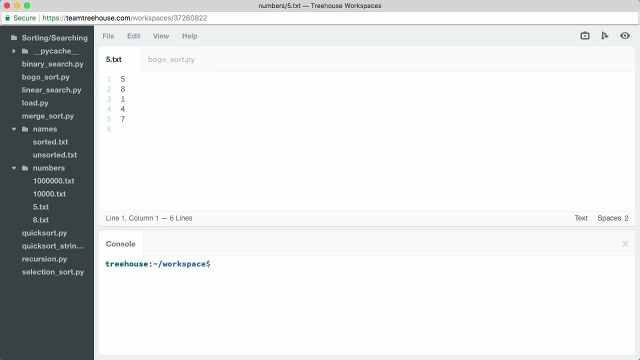 I'll show you how to modify our examples to sort strings at the end of the course, To help make clear the importance of choosing a good sorting algorithm. we're going to start with a bad one. It's called bogosort. Basically, bogosort just randomizes. 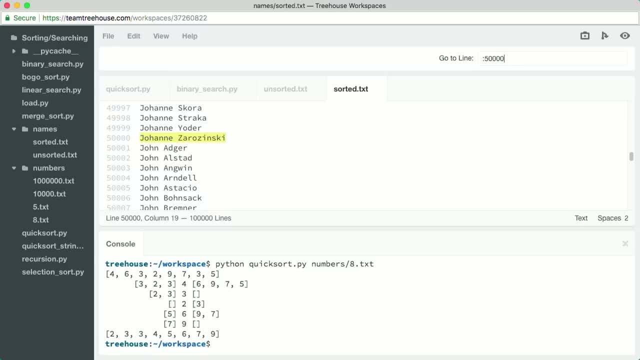 around it. If you're having trouble following along, remember the video playback controls. Feel free to slow the playback down, rewind or pause the video as needed. Watch this the first time. You may also find it helpful to rewind and make your own diagram of the. 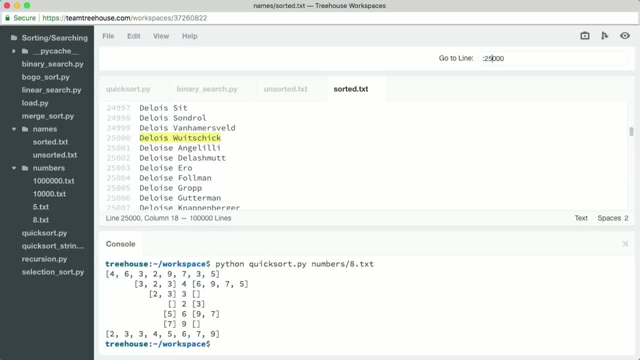 process as we go. Okay, ready, Here goes. Suppose we load the numbers from our eattxt file into a list, How do we divide it? It would probably be smart to have our quicksort function divide the list in a way that brings it closer to being sorted. Let's pick an item from the list, We'll just 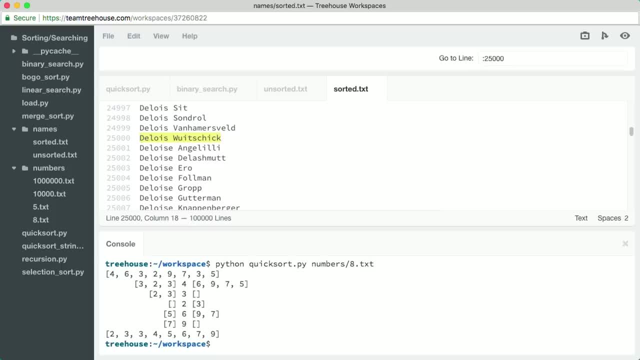 pick the first item for now four. We'll call this value. we've picked the pivot, like the center of a seesaw on a playground. We'll break the list into two sublists. The first sublist will contain all the items in the original list that are smaller than the pivot. The second sublist 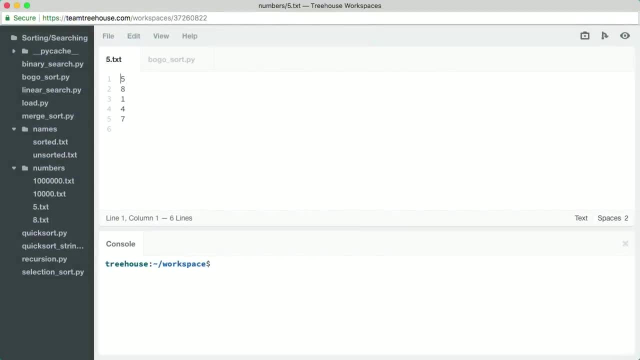 will contain all the items in the original list that are greater than the pivot. The sublists of values less than and greater than the pivot aren't sorted. But what if they were? You could just join the sublists and the pivot all together into one list and the whole thing would be sorted. 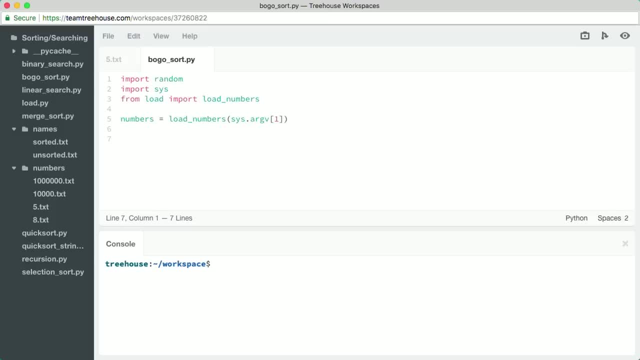 So how do we sort the sublist? We call our quicksort recursively on them. This may seem like magic, but it's not. It's the divide-and-conquer algorithm design technique at work. If our quicksort function works on the big list, then it will work on the. 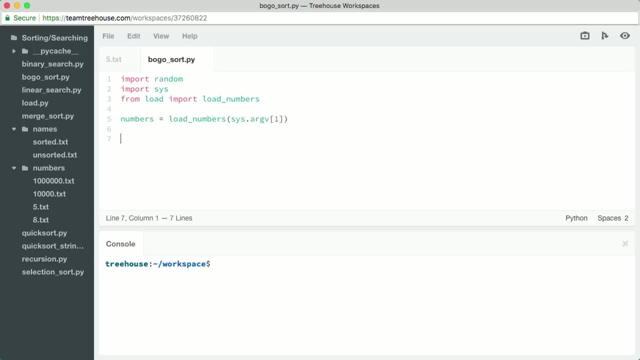 smaller list too. For our first sublist we take the first item as the pivot. again, That's three. We break the sublist into two sublists: one with everything less than the pivot and one with everything greater than the pivot. Notice that there's a value equal to the pivot that gets put. 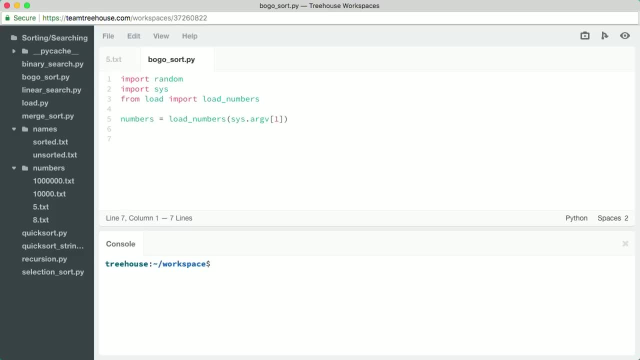 in the first sublist. Our finished quicksort function is actually going to put everything that's less than or equal to the pivot in the first sublist. But I don't want to say less than or equal to over and over, so I'm just referring to it as the less than pivot sublist. Also notice. 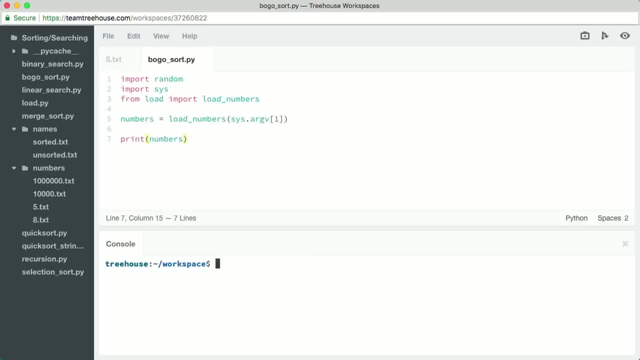 that there are no values greater than the pivot, That's okay. When we join the sublists back together, that just means nothing will be in the return list after the pivot. We still have one sublist that's more than one element long, so we call our quicksort function on that too. 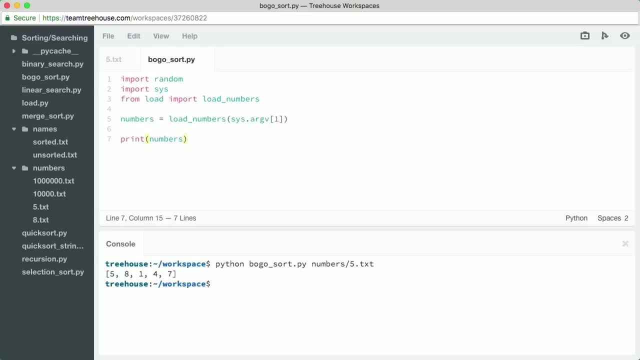 You and I can see that it's already sorted, but the computer doesn't know that, so it'll call it anyway, just in case It picks the first element two as a pivot. There are no elements less than the pivot and only one element greater than the pivot. That's it for the recursive case. 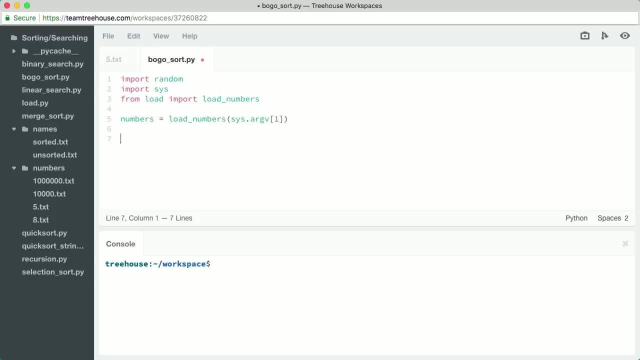 We've finally hit the base case for our quicksort function. It'll be called on both the empty list of elements less than the pivot and the one-item list of elements greater than the pivot. But both of these lists will be returned as they are because there's nothing to sort. 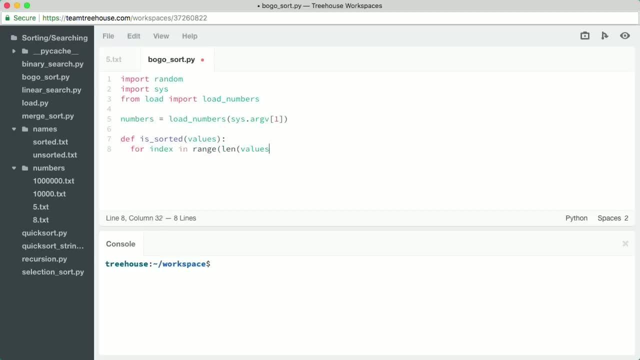 So now, at the level of the call stack, above this, the return sorted lists are used in place of the unsorted sublist that's less than the pivot and the unsorted sublist that's greater than the pivot. These are joined together into one sorted list. Remember that any empty lists 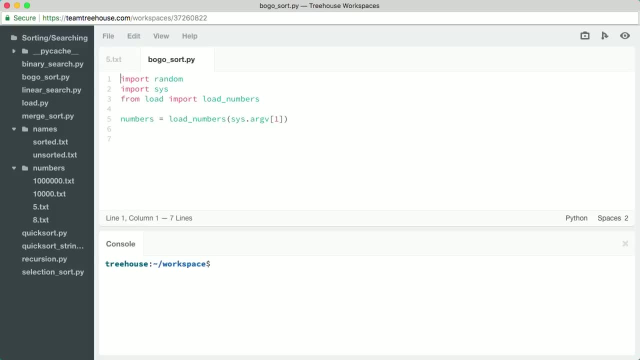 the order of the list repeatedly until it's sorted. Here's a Python code file where we're going to implement bogosort. It's not important to understand this code here at the top, although we'll have info on it in the teacher's notes if you really want it. All you need to know. 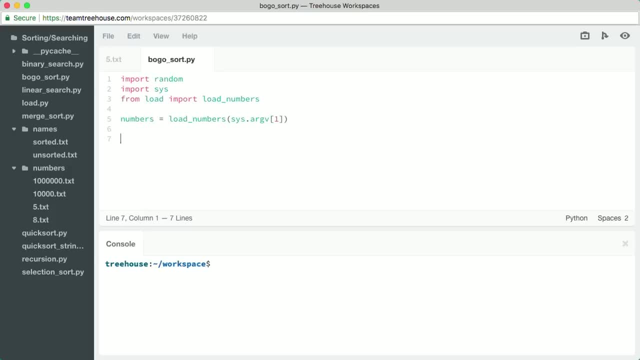 is that it takes the name of a file that we pass on the command line, loads it and returns a list of numbers- It's called a Python list, which is just like an array in other languages- containing all the numbers that it read from the file. Let me have the program print out the list. 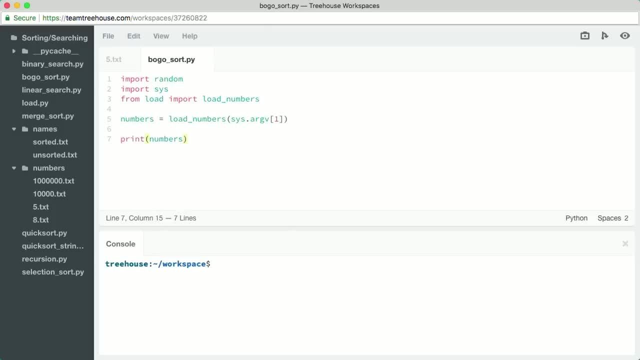 of numbers it loads so you can see it. We'll call the print method and we'll pass it. the list of numbers. Save that. Let's run it real quick with python bogosortpy. Oh whoops, and we need to load the list of numbers we're going to load. So it's in the numbers directory, A slash separates. 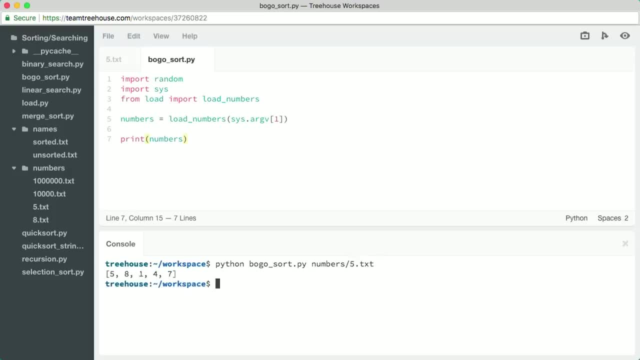 the directory name from the file name 5.text. And there's our list of numbers that was loaded from the file. Okay, let me delete that print statement and then we'll move on. Bogosort just randomly rearranges the list of values over and over, So the first thing we're going to need is: 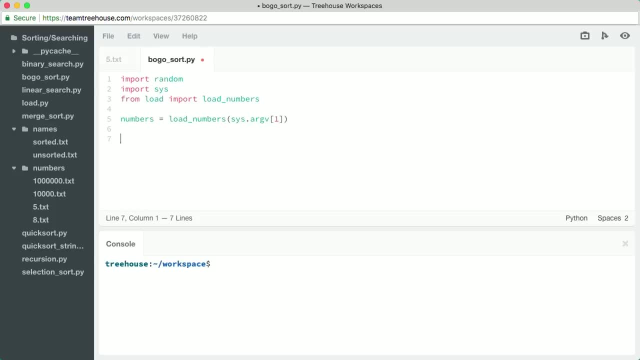 a function to detect when the list is sorted. We'll write an isSorted function that takes a list of parameters. It'll return true if the list passed in is sorted or false if it isn't. We'll loop through the numeric index of each value in the list from zero to one less than. 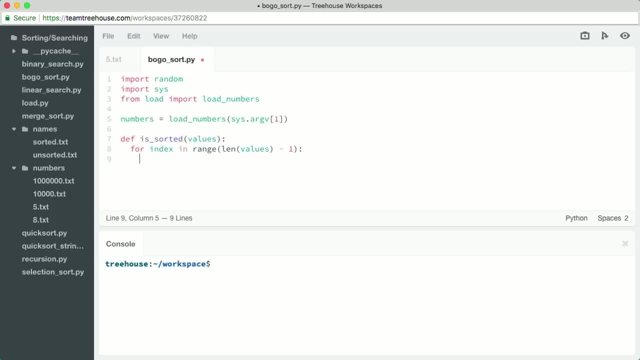 the length of the list. Like many languages, Python list indexes begin at zero. so a list with a length of five has indexes going from zero through four. If the list is sorted, then every value in it will be less than the one that comes after it. So we test to see whether the 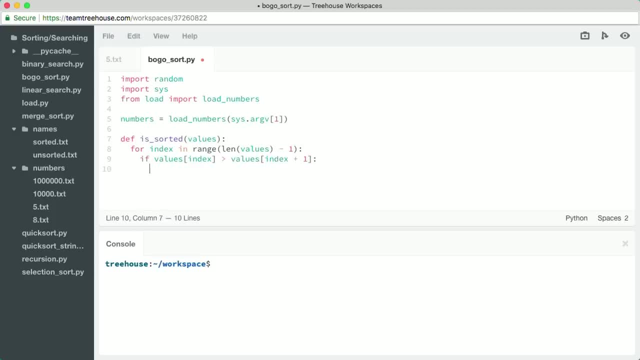 current item is greater than the one that follows it. If it is, it means the whole list is not sorted, so we can return false. If we get down here, it means the loop completed without finding any unsorted values. Python uses whitespace to mark code blocks, so, unintenting, the code like this: 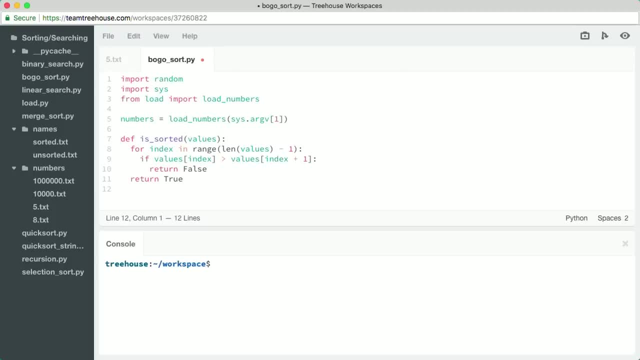 marks the end of the loop. Since all the values are sorted, we can return true. Now we need to write the function that will actually do the so-called sorting. The bogosort function will also use the values it's working with as a parameter. We'll call our isSorted function to test whether 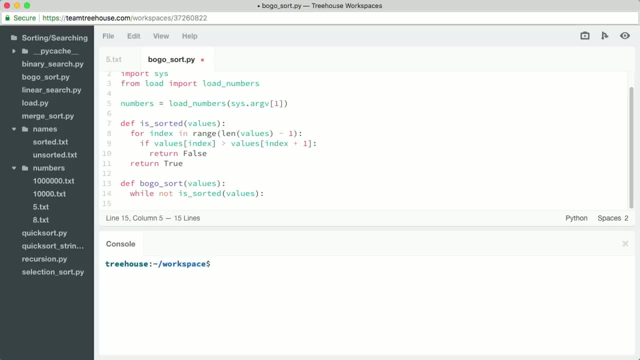 the list is sorted, We'll keep looping until isSorted returns true. Python has a ready-made function that randomizes the order of elements in the list. Since the list isn't sorted, we'll call that function here And since this is inside the loop, it'll be randomized over and over until our 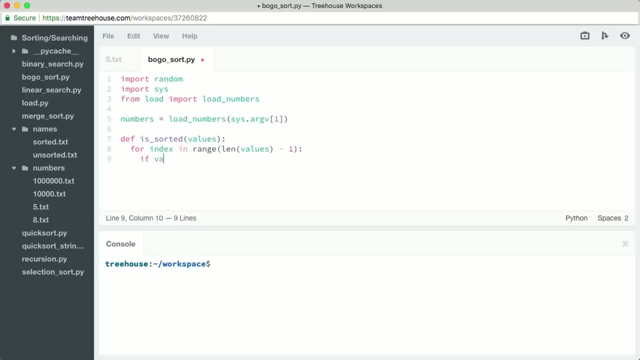 get discarded. Then at the level of the call stack above that, the return sorted lists are used in place of the unsorted sublists. there Again, they were already sorted, but the quicksort method was called on them anyway, just in case The sublists are joined. 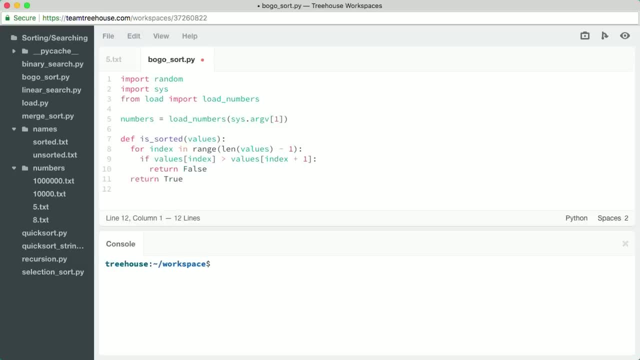 together into one sorted list At the level of the call stack. above that, the return sorted list is used in place of the unsorted sublist that's less than the pivot. So now everything that's less than or equal to the pivot is sorted. Now we call quicksort on the unsorted sublist. 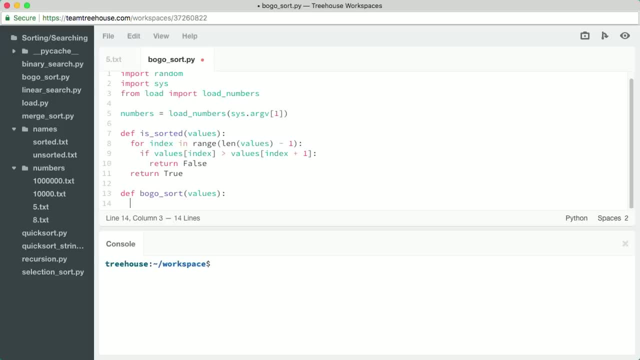 that's greater than the pivot and the process repeats for that sublist. We pick the first element, 6,, as the pivot, We split the sublist into sublists of elements that are less than and greater than this pivot And we recursively call the quicksort function. 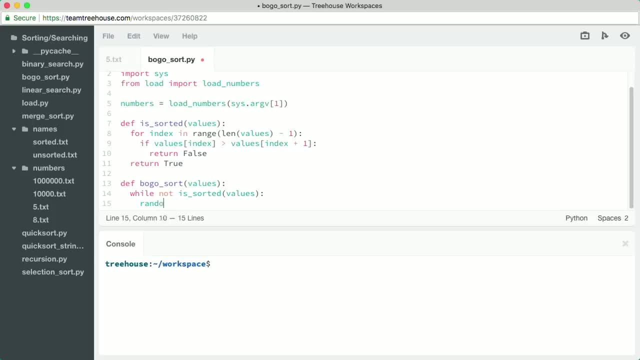 until those sublists are sorted. Eventually a sorted sublist is returned to our first quicksort function call. We combine the sublist that's less than or equal to the pivot, the pivot itself and the sublist that's greater than the pivot into a single list. 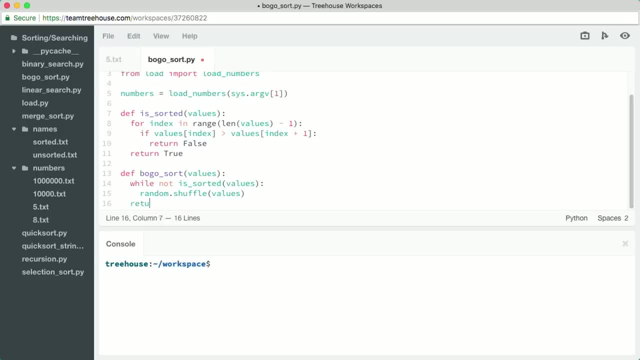 And because we recursively sorted the sublists, the whole list is sorted. So that's how the quicksort function is going to work. In the next video we'll show you the actual code. Quicksort works by picking a pivot value. 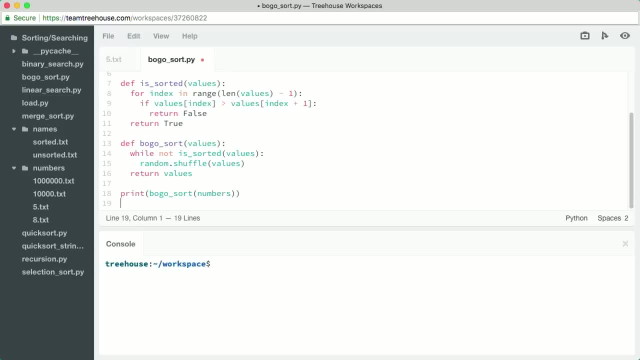 then splitting the full list into two sublists. The first sublist has all the values less than or equal to the pivot, and the second sublist has all the values greater than the pivot. The quicksort function recursively calls itself to sort these sublists. 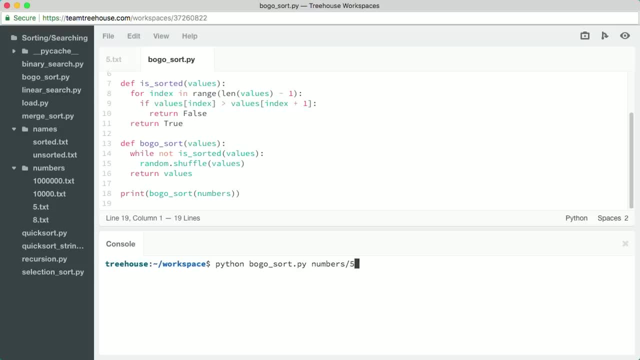 and then to sort the sublists of those sublists until the full list is sorted. Now it's time to actually implement this in code. We already have the base case written. Any list passed in that consists of 0 or 1 values will be returned as is, because there's 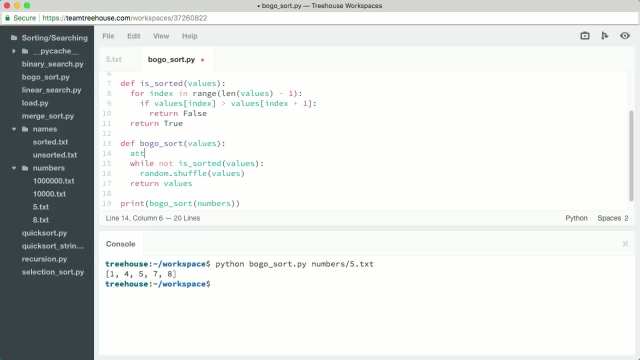 nothing to sort Now we need to create a list that will hold all the values less than the pivot. That list will be empty at first. We do the same for values greater than the pivot. Next we need to choose the pivot value. For now, we just grab the first item from the list. 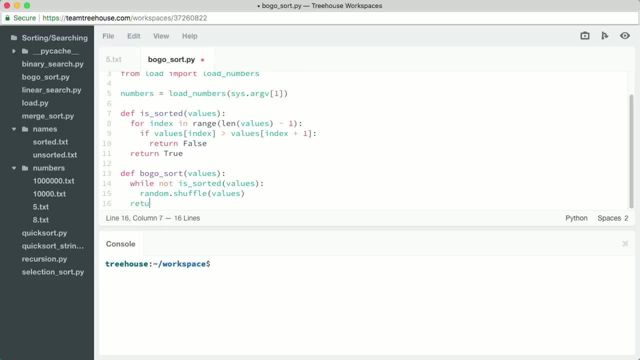 isSorted function returns true. If the loop exits, it means isSorted returned true and the list is sorted. So we can now return the sorted list. Finally, we need to call our bogosort function, pass it the list we loaded from the file and print the sorted list it returns. 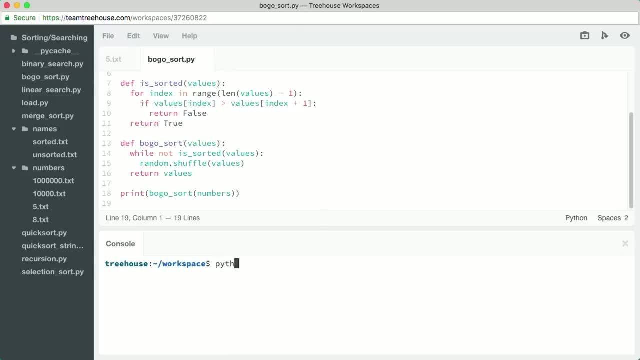 Okay, let's save this and try running it. We do so with Python. the name of the script- bogosortpy, and the name of the file. we're going to run it on: numbers, directory 5.txt. It looks like it's sorting our list successfully. 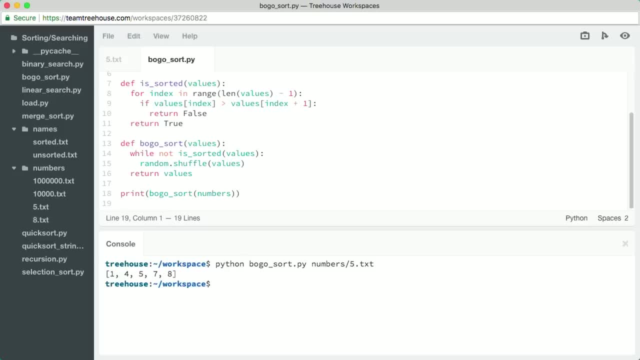 but how efficient is this? Let's add some code to track the number of times it attempts to sort the list Up here at the top of the bogosort function we'll add a variable to track the number of attempts it's made. We'll name it attempts and we'll set its initial value to 0,. 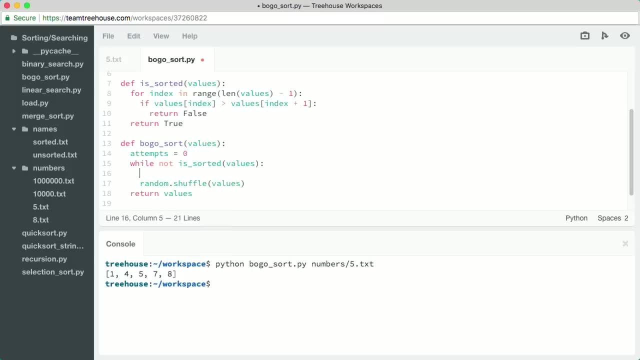 since we haven't made any attempts yet, With each pass through the loop, we'll print the current number of attempts And then, here at the end of the loop, after attempting to shuffle the values, we'll add one to the count of attempts. 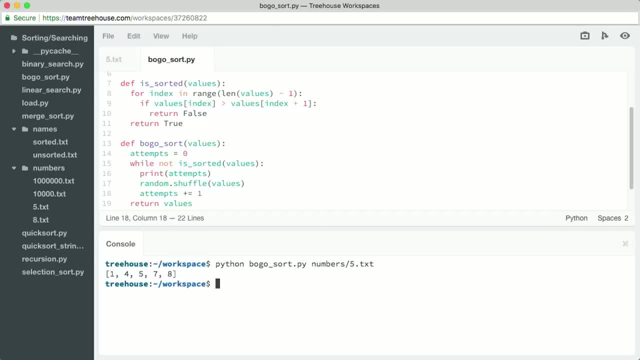 Let's save this and let's try running it again a couple times. In the console I can just press the up arrow to bring up the previous command and rerun it. So it looks like this first run to sort this five element list took 363 attempts. Let's try it again. 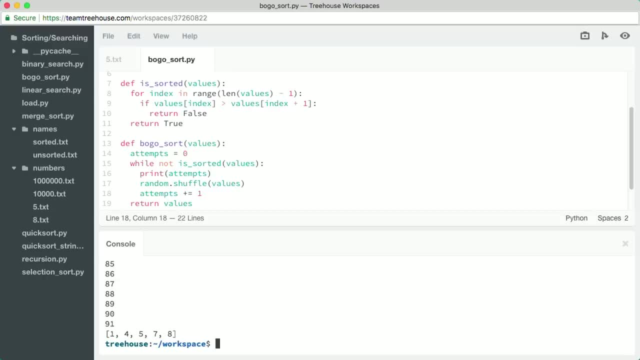 This time it only took 91 attempts. We're simply randomizing the list with each attempt, so each run of the program takes a random number of attempts. Now let's try this again. Same program with a larger number of items: Python, bogosort numbers. 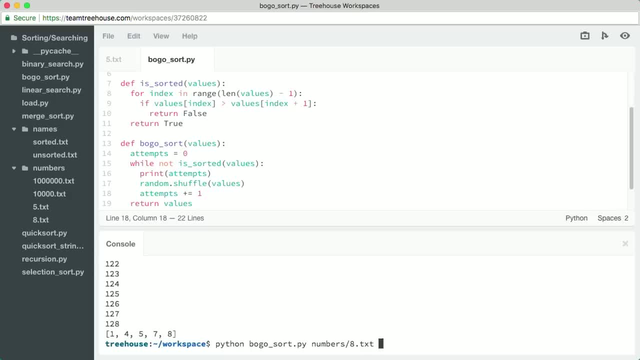 I have a list of eight items set up here in this other file. This time it takes 11,000 attempts, only 487 this time, And this time 13,000.. You can see that the trend is increasing steadily. The problem with bogosort. 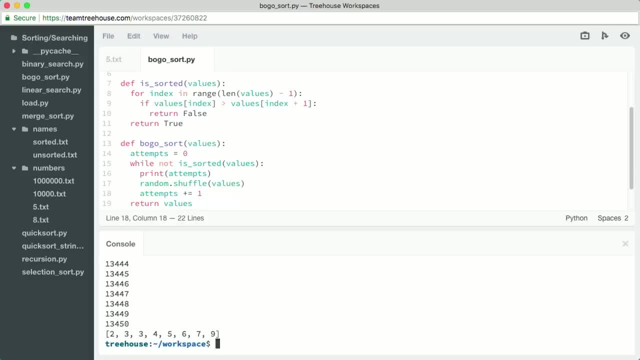 is that it doesn't make any progress toward a solution. with each pass, It could generate a list where just one value is out of order, but then on the next attempt it could generate a list where all the elements are out of order again. Stumbling on a solution is literally a matter of luck. 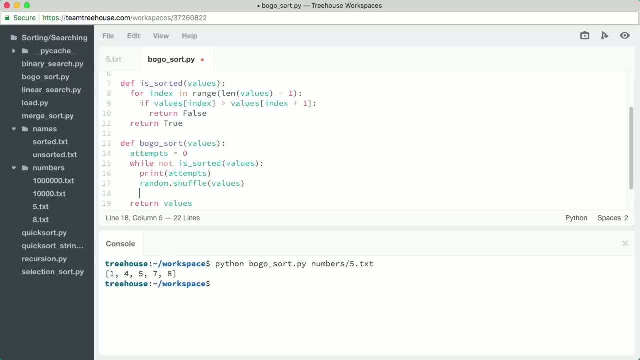 Then we loop through all the items in the list following the pivot. We check to see whether the current value is less than or equal to the pivot. If it is, we copy it to the sublist of values less than the pivot. Otherwise, the current value must be greater than the pivot, so we copy it to the other list. 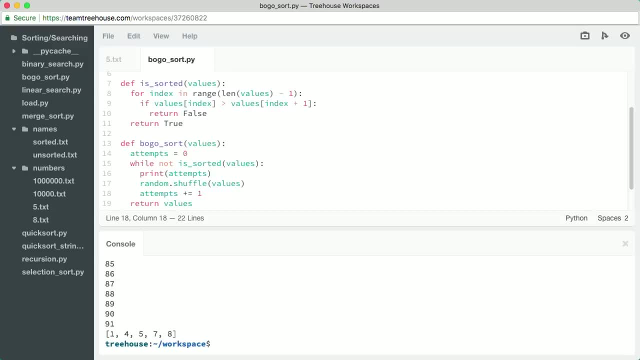 This last line is where the recursive magic happens. We call quicksort recursively on the sublist that's less than the pivot. We do the same for the sublist that's greater than the pivot. Those two calls will return sorted lists. so we combine the sorted values less than the pivot. 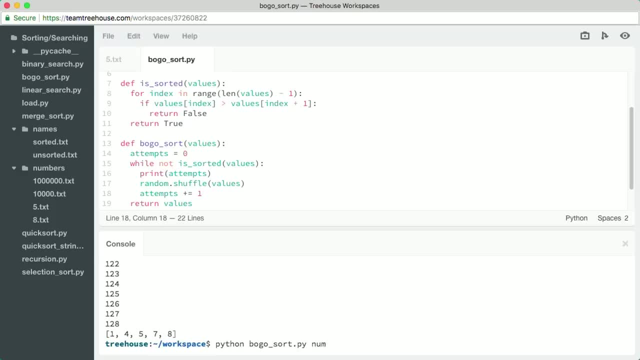 the pivot itself and the sorted values greater than the pivot. This gives us a complete sorted list which we return. This took a lot of prep work. Are you ready? Let's try running it. It outputs our sorted list. I don't know about you, but this whole thing still. 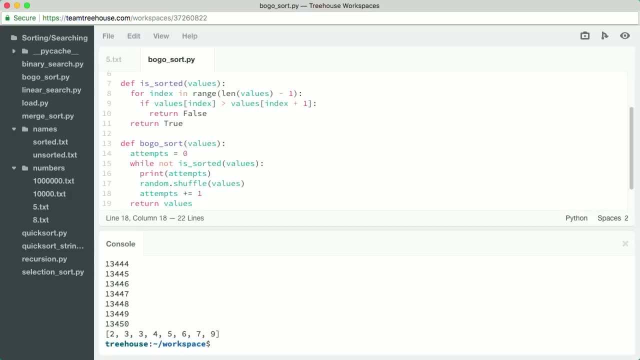 seems a little too magical to me. Let's add a couple of print statements to the program so we can see what it's doing. First let's add a print statement right call to the quicksort function so we can see the unsorted list. we'll also add a. 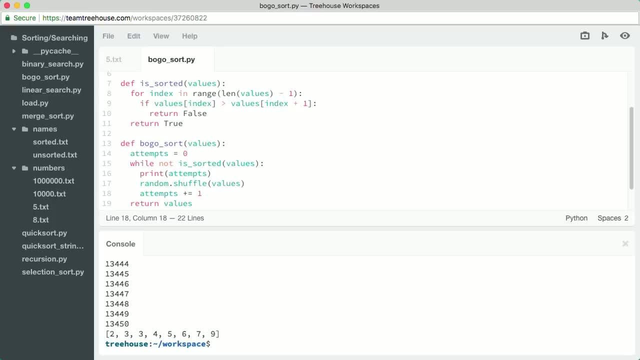 print right within the quicksort function right before the recursive calls. again, this string formatting code is just to keep the info aligned in columns. let's try running this again, and now you can see our new debug output. each time quicksort goes to call itself recursively, it prints out the pivot as: 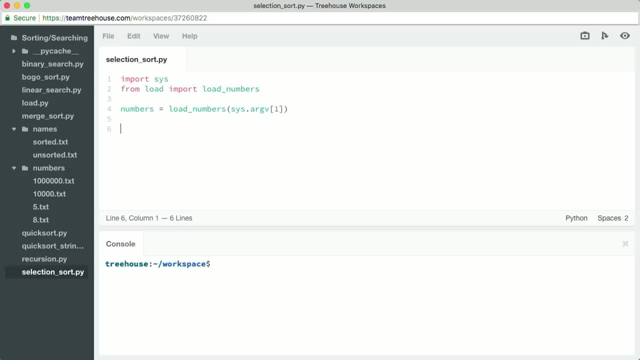 well as the sub list of items less than or equal to the pivot, if any, and the sub list of items greater than the pivot, if any. you can see that first it sorts the sub list of items less than the pivot at the top level. it goes through a couple. 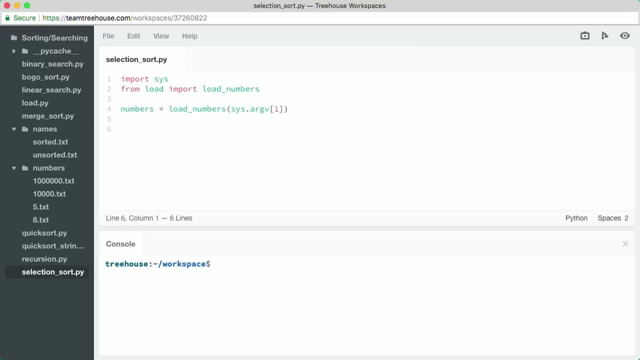 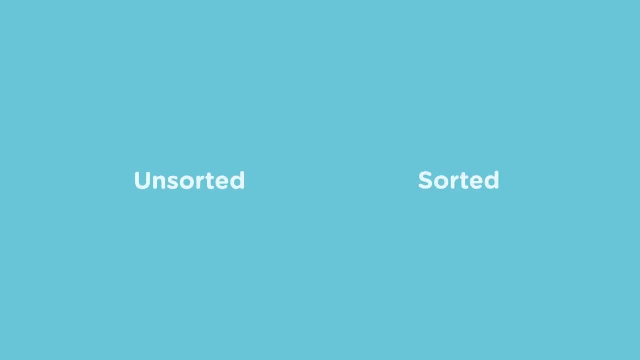 levels of recursion to do that. there are actually additional levels of recursion, but they're from calls to quicksort with a list of zero or one elements and those calls return before the print statement is reached you. then it starts sorting the second sub list from the top level with items. 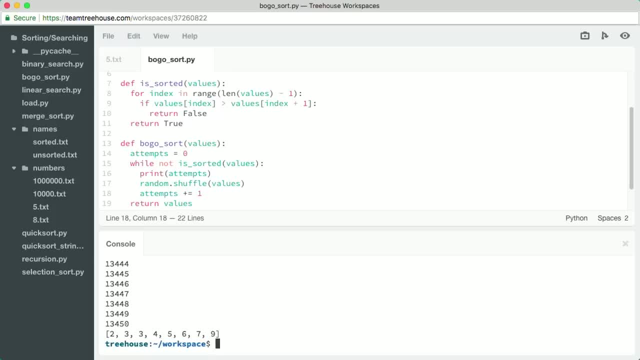 and for lists with more than a few items, it might never happen. Up next we'll look at selection sort. It's a sorting algorithm that's still slow, but it's better than bogosort. Previously we showed you bogosort. 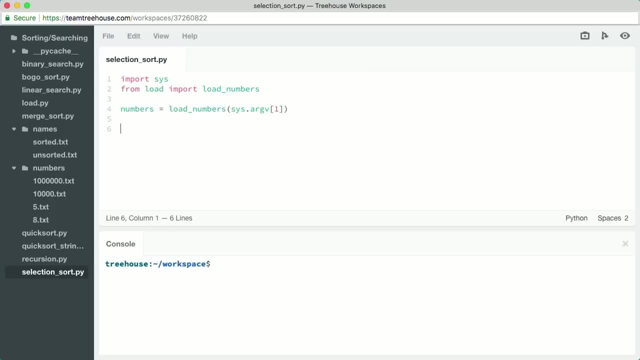 a terrible sorting algorithm that basically randomizes the order of a list and then checks to see if it happens to be sorted. The problem with bogosort is that it doesn't get any closer to a solution with each operation, and so with lists that have more than a few items, it'll 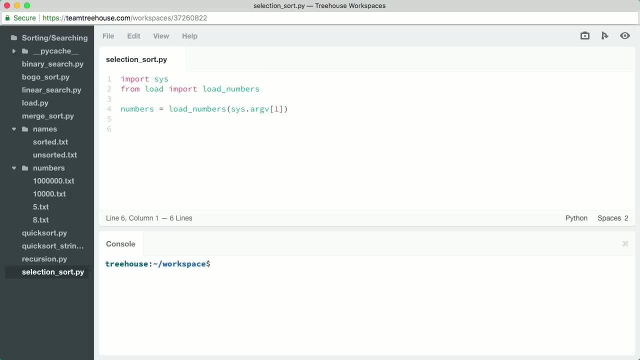 probably never finish sorting them. Now we're going to look at an algorithm named selection sort. It's still slow, but at least each pass through the list brings it a little closer to completion. Our implementation of selection sort is very similar to that of bogosort, but it's a little slower. 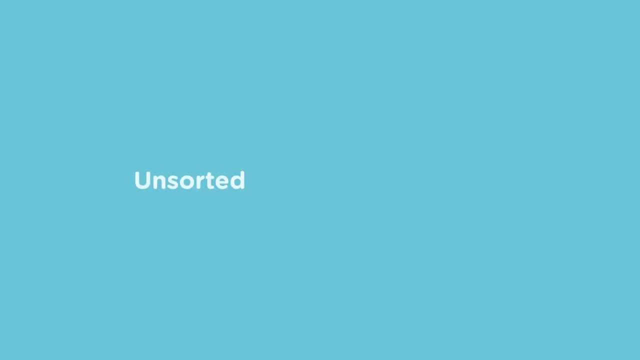 We're going to use two arrays, an unsorted array and a sorted one. Some versions move values around within just one array, but we're using two arrays to keep the code simpler. The sorted list starts out empty, but we'll be moving values from the unsorted list to the sorted list, one at a time. 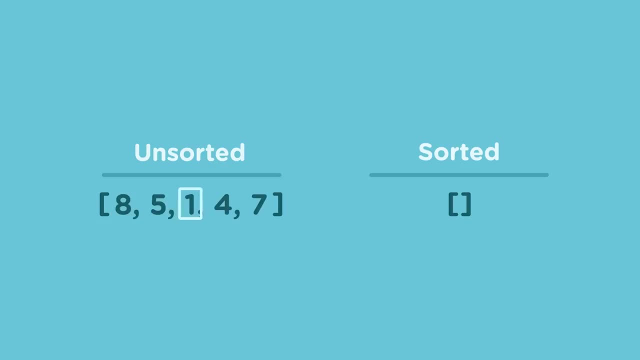 With each pass we'll look through each of the values in the unsorted array, find the smallest one and move that to the end of the sorted array. We'll start with the first value in the unsorted array and say that's the minimum. 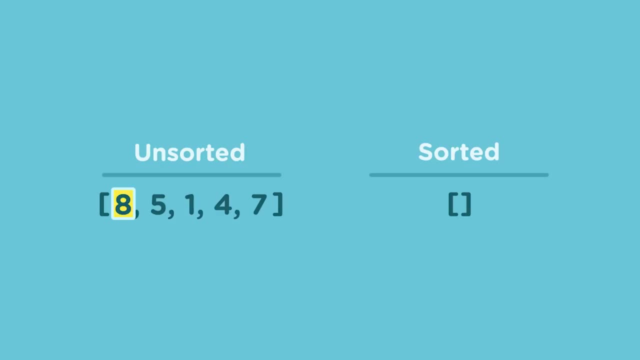 or smallest value we've seen so far. Then we'll look at the next value and see if that's smaller than the current minimum. If it is, we'll mark that as the new minimum. Then we'll move to the next value and compare that to the minimum again. 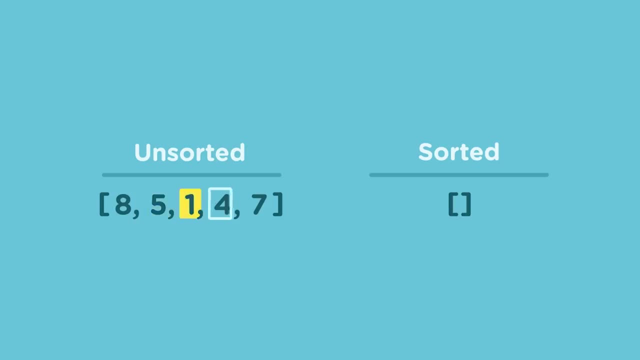 If it's smaller, that becomes the new minimum. We continue that way until we reach the end of the list. At that point we know whatever value we have marked as the minimum is the smallest value in the whole list. Now here's the part that makes selection sort better than bogosort. We then 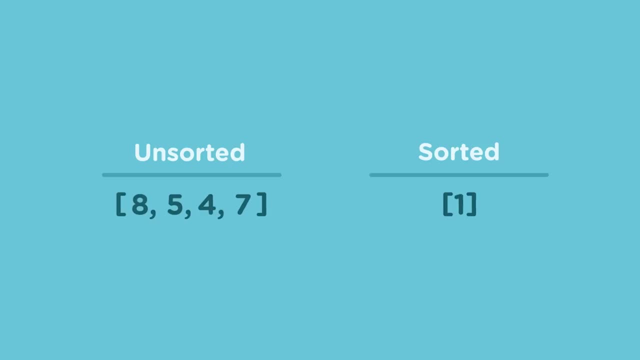 move that minimum value from the unsorted list to the end of the sorted list. The minimum value isn't part of the unsorted list anymore, so we don't have to waste time looking at it anymore. All our remaining comparisons will be on the remaining values in the unsorted list. 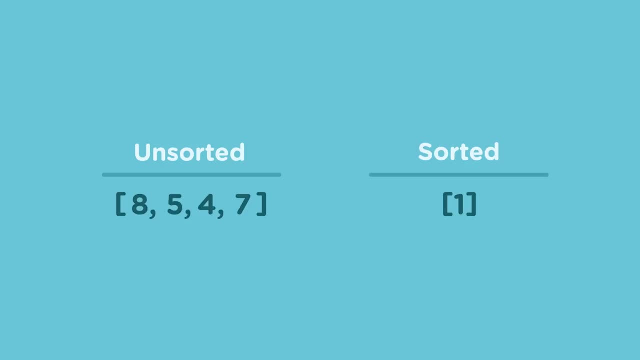 Then we start the process over. At this point, our list consists of the numbers 8,, 5,, 4, and 7.. Our first minimum is 8.. We start by comparing the minimum to 5.. 5 is smaller than 8, so 5 becomes the. 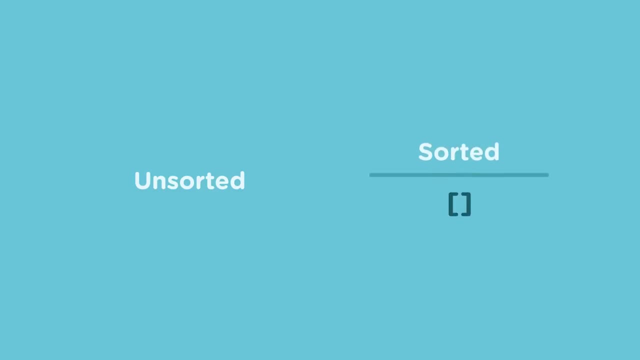 greater than the original pivot. you can see a couple levels of recursion for that sort as well. finally, when both sub lists are recursively sorted, the original call to the quicksort function returns and we get the sorted list back. so we know that it works. the next question is: how well does it work? let's 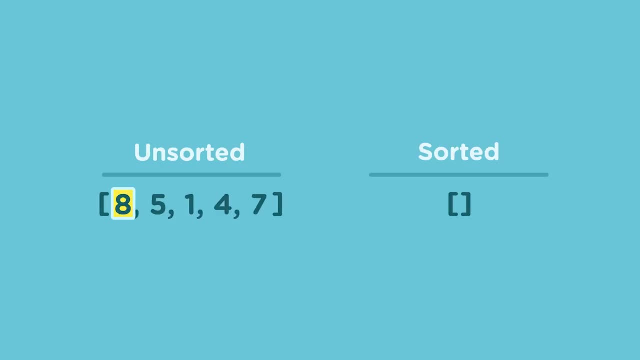 go back to our file of 10,000 numbers and see if it can sort those. first, though, I'm going to remove our two debug calls to print so it doesn't produce unreadable output. a quick note: if you try running this on a file with a lot of repeated values, it's possible you'll get a runtime error. 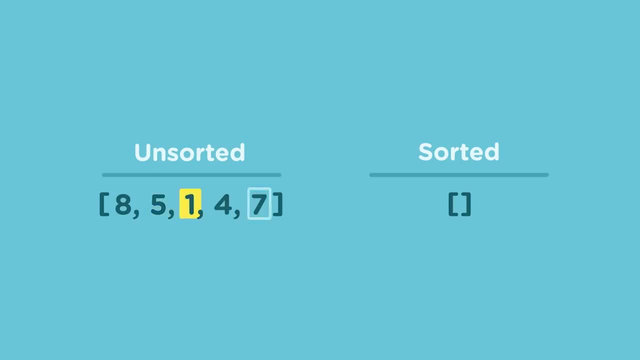 maximum recursion depth exceeded. if you do see the teachers notes for a possible solution. now let's try running our quicksort program against the 10,000 dot-text file. Python, quicksortpy numbers: 10,000 dot-text. there we go and it seems pretty fast. but how fast exactly? let's run it with the time. 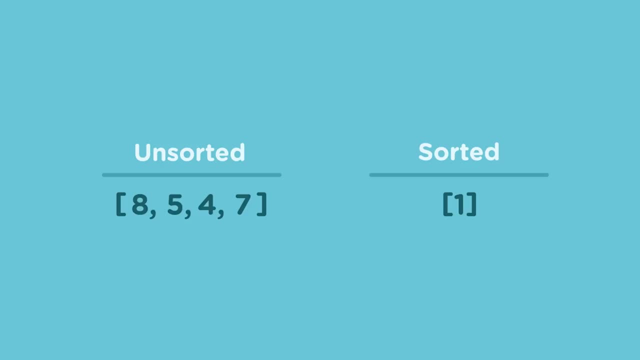 command to see how long it takes time. Python quicksortpy numbers: 10,000 dot-text. remember we need to ignore the real result and add the user and sys results. it took less than a second of CPU time to sort 10,000 numbers with. 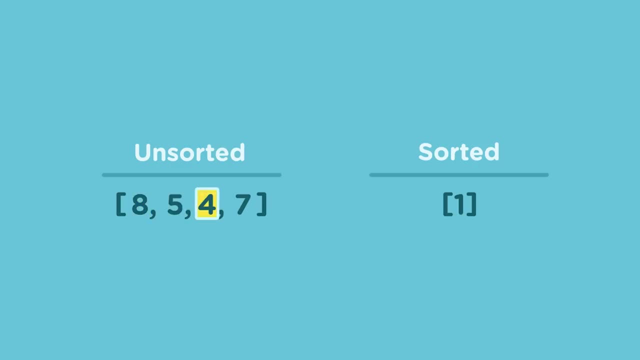 quicksort. remember that selection sort took about 13 seconds. that's a pretty substantial improvement. and with a million numbers, selection sort took so long that it never even finished successfully. let's see if quicksort performs any better time. Python, quicksortpy numbers 1 million dot-text. 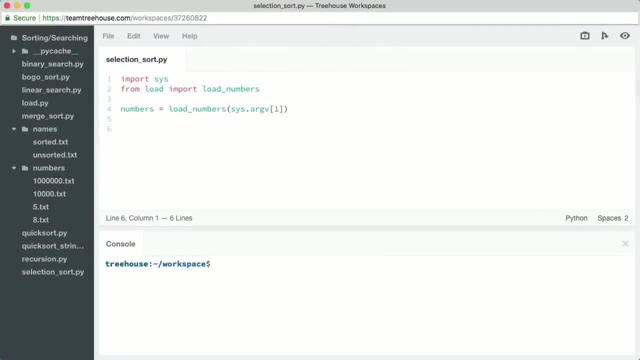 not only did quicksort sort a million numbers successfully, it only took about 11 seconds of CPU time. quicksort is clearly much, much faster than selection sort. how much faster, that's something we'll discuss in a later video. what we've shown you here is just one way to implement quicksort, although the basic 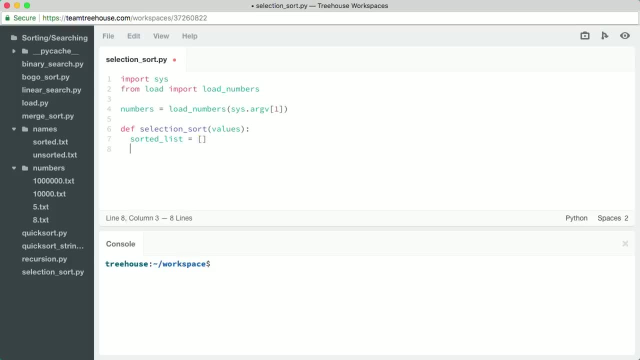 algorithm is always the same. the details can vary, like how you pick the pivot. see the teachers notes for more details. let's review another sorting algorithm, merge sort, so that we can compare it with quicksort. merge sort is already covered elsewhere on the site so we won't go into as much detail about it. 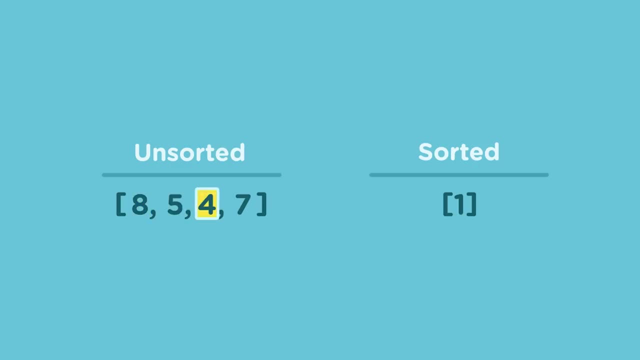 minimum. Then we compare 5 with 4, and 4 becomes the new minimum. 4 is not smaller than 7, though, so 4 remains the minimum. 4 gets moved to the end of the sorted array, becoming its second element. 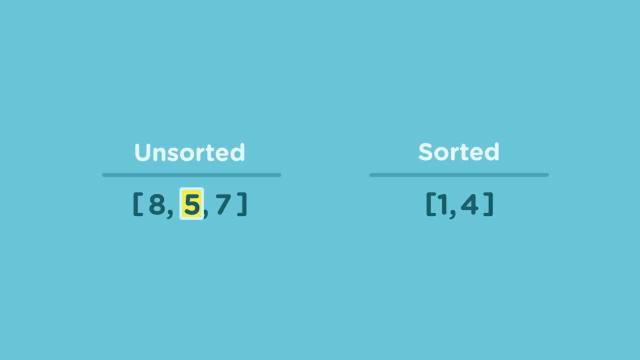 The process repeats again. 8 is the first minimum, but 5 is smaller, so that becomes the minimum. 7 is larger, so 5 stays as the minimum, and 5 is what gets moved over to the sorted array, and so on, until there are no more items left in the unsorted array and all we have left is the. 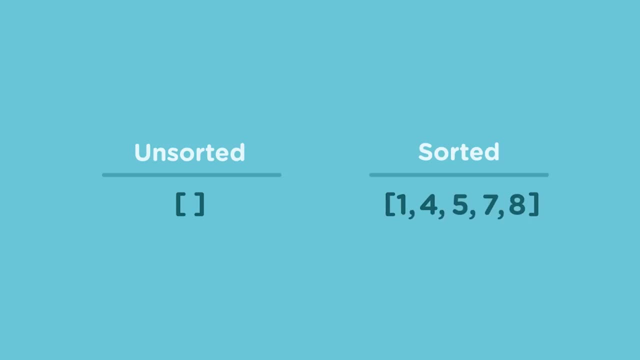 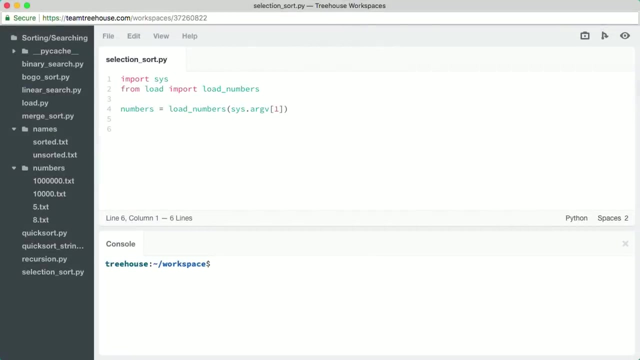 sorted array. That's how selection sort works in general. Now let's do an actual implementation of it. This code here at the top is the same as we saw in the BOGO sort example. It just loads a Python list of numbers from a file. 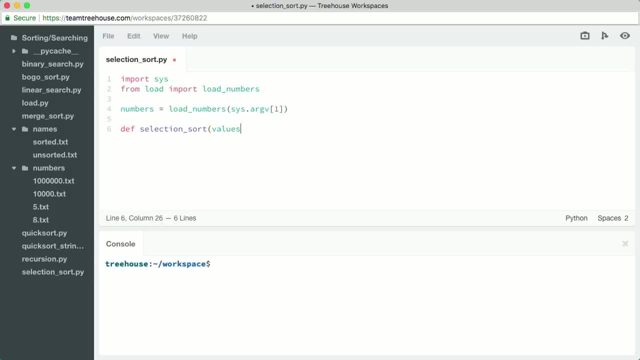 Let's implement the function that will do our selection sort. We're going to pass in our Python list containing all the unsorted numbers. We'll create an empty list that will hold all our sorted values. We'll loop once for each value in the list. 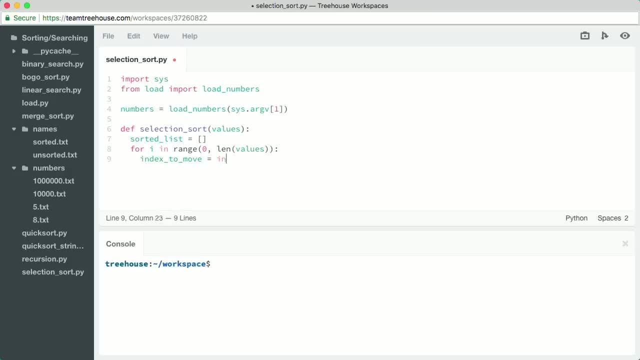 We call a function named indexSubmin, which we're going to write in just a minute, that finds the minimum value in the unsorted list and returns its index. Then we call the pop method on the list and pass it the index of the minimum value. 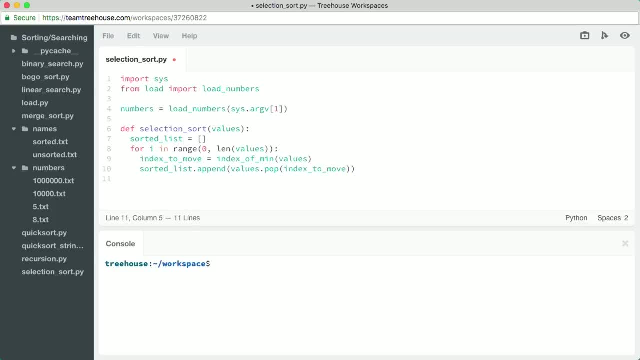 Pop will remove that item from the list and return it. We then add that value to the end of the sorted list. Going up a level of indentation signals to Python that we're ending the loop. After the loop finishes, we return the sorted list. 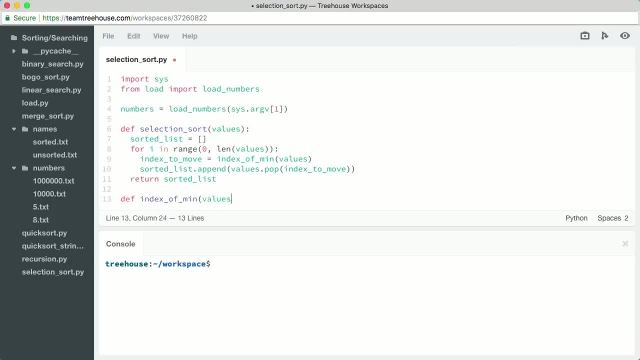 Now we need to write the function that picks out the minimum value We pass in the list we're going to search. We mark the first value in the list as the minimum. It may or may not be the actual minimum, but it's the smallest we've seen on this pass. 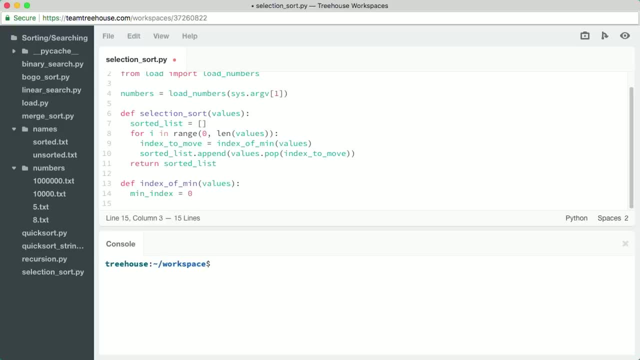 through the list. It's also the only value we've seen on this pass through the list so far. Now we loop through the remaining values in the list after the first. We test whether the value we're currently looking at is less than or equal to the number. 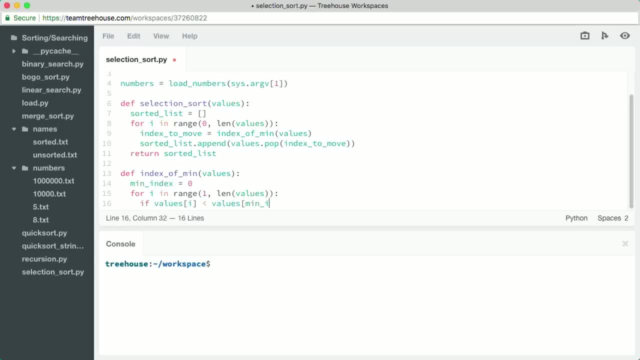 that we're look at less than the previously recorded minimum. If it is, then we set the current index as the new index of the minimum value. After we've looped through all the values, we return the index of the smallest value we found. 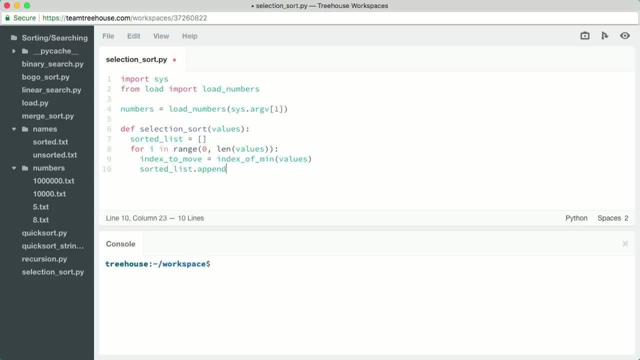 but we'll have more info in the teachers notes if you want it. both quicksort and merge sort are recursive. the difference between them is in the sorting mechanism itself. whereas quicksort sorts a list into two sub lists that are less than or greater than a pivot value, merge sort simply splits list in half recursively. 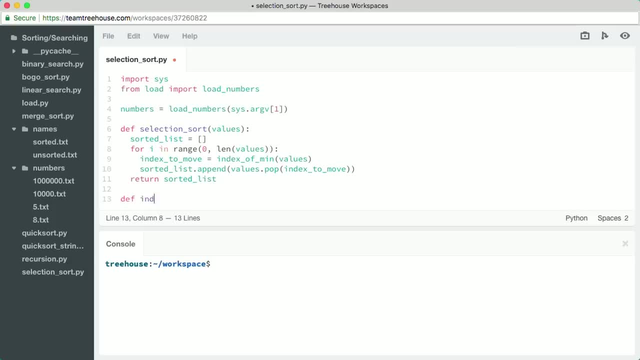 and then sorts the halves as it merges them back together. that's why it's called merge sort. you may recognize this code at the top by now. it just loads a file full of numbers into a list. let's define a recursive merge sort function. as usual, it'll take the list or sub list. 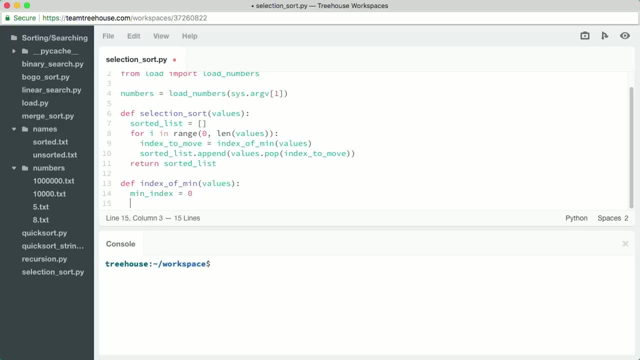 that we want it to sort. our base case is the same as with quicksort: if the list has 0 or 1 values, there's nothing to sort, so we return it as is. if we didn't return, it means we're in the recursive case. so first we need to split the list. 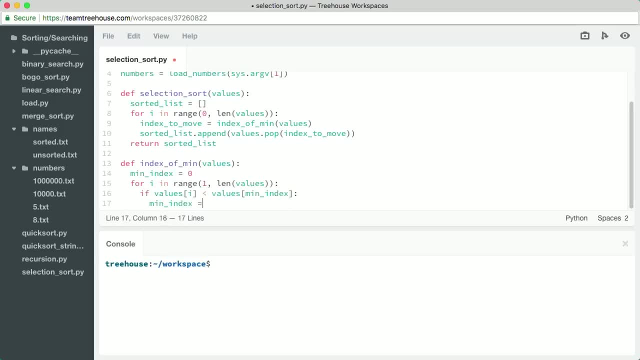 in half. we need to know the index we should split on. so we get the length of the list and divide it by 2. so, for example, if there are 8 items in the list, will one an index of 4? but what if there were an odd number of items in the list? 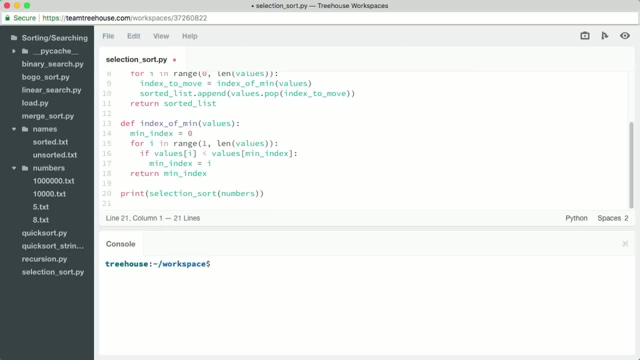 like 7, we can't have an index of 3.5, so we'll need to round down in that case. since we're working in Python currently, we can take advantage of a special Python operator that divides and rounds the result down: the floor division operator. it consists of a double slash. now we'll use the Python slice syntax to 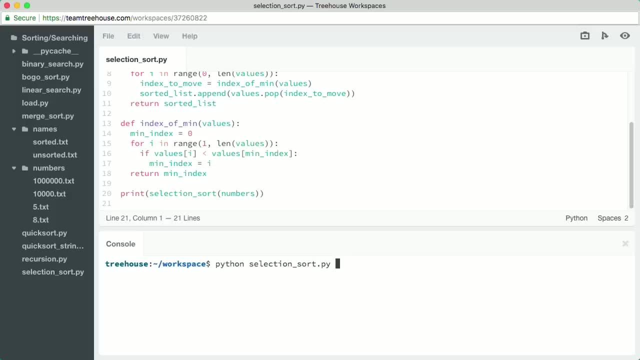 get the left half of the list, we'll pass that list to a recursive call to the merge sort function. we'll also use slice syntax to get the right half of the list and pass that to merge sort as well. now we need to merge the two halves together. 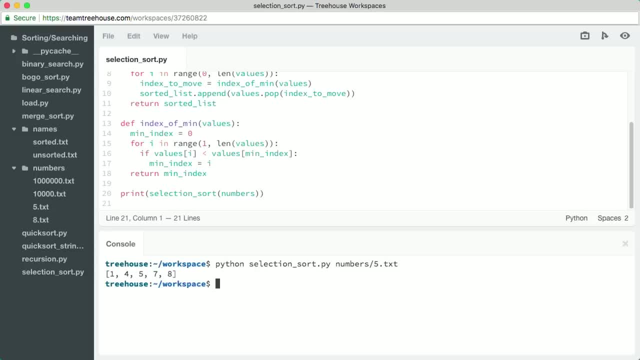 and sort them as we do it, we'll create a list to hold the sorted values. and now we get to the complicated part: merging the two halves together and sorted them as we do it. we'll be moving from left to right through the left half of the list. 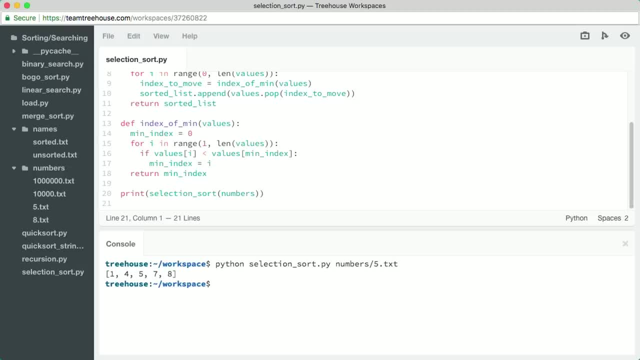 copying values over to the sorted values list. as we go, this left index variable will help us keep track of our position. at the same time, we'll also be moving from left to right through the right half of the list and copying values over, so we need a separate right index variable to track that position as 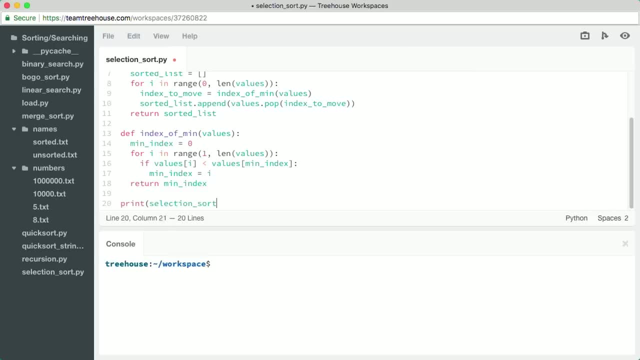 Lastly, we need to actually run our selection sort method and print the sorted list it returns. Let's save this and now let's try running it. We run the Python command and pass it the name of our script: selection sortpy. 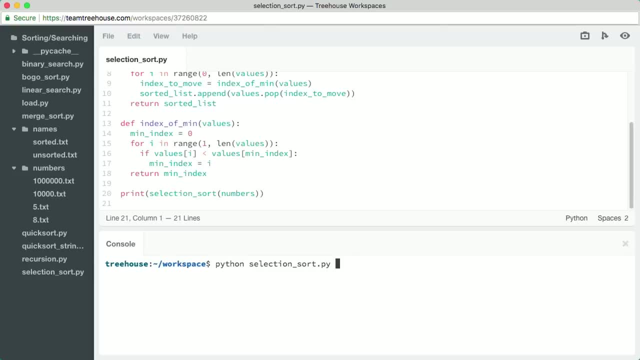 In the numbers directory I've saved several data files filled with random numbers, one on each line. Five dot text has five lines. eight dot text has eight lines. and to help us really measure the speed of our algorithms, ten thousand dot text has ten thousand lines. 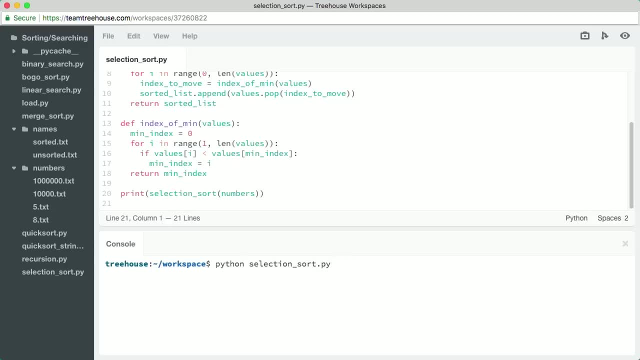 I've even created a file with a million numbers. Our script takes the path of a file to load as an argument, so I'll give it the path of our file with five numbers: Numbers slash, five numbers, Five dot text. The script runs, reads the numbers in the file into a list. calls our selection sort. 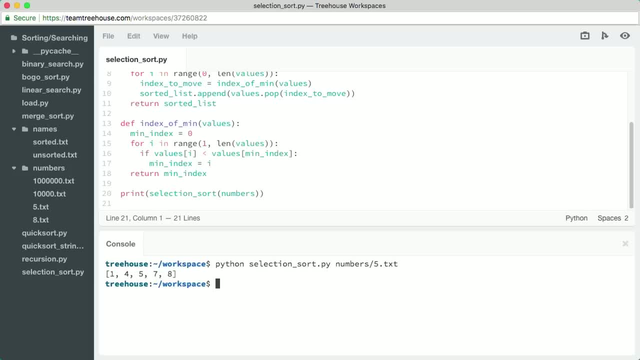 method with that list and then prints the sorted list. Let me add a couple print statements within the selection sort function so you can watch the sort happening. Don't worry about figuring out the Python formatting string that I use. It's just there to keep the two lists neatly aligned. 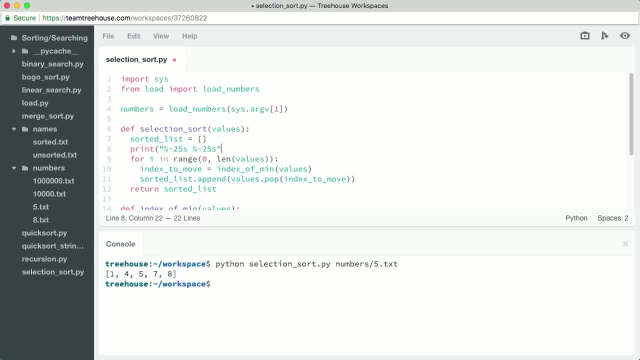 I'll add the first print statement before the loop runs at all. I'll have it print out the unsorted list and the sorted list. I'll add an identical print statement within the loop so we can watch values moving from the unsorted list to the sorted list. 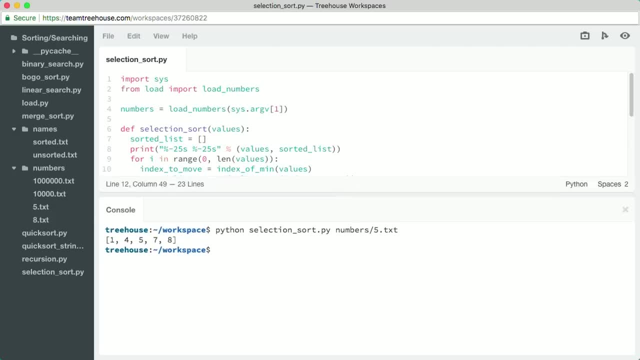 Let's save this And we'll try running the same command again. The output looks like this. You can see the unsorted list on the left and the sorted list on the right. Initially, the sorted list is empty. On the first pass it selects the sorted list. 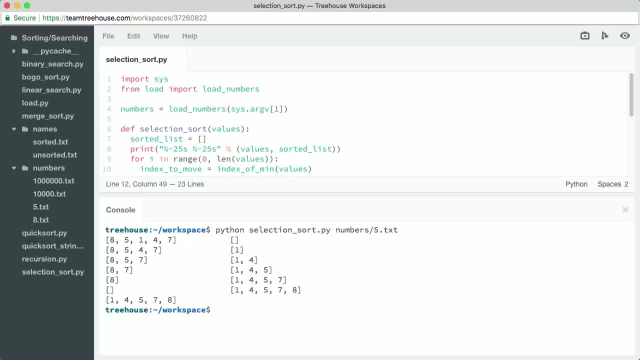 Then it selects the lowest number, 1, and moves it to the sorted list. Then it moves the next lowest number over 4.. This repeats until all the numbers have been moved to the sorted list. I have another file with 8 different numbers in it. 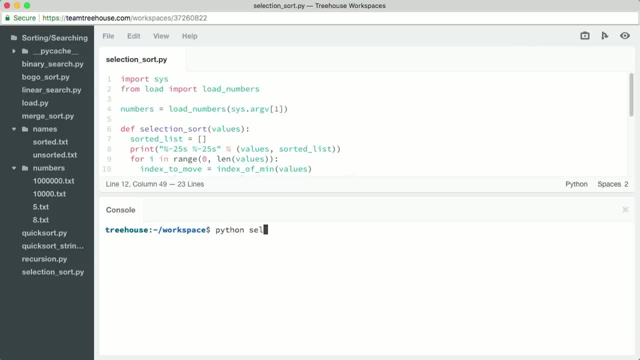 Let's try our program with that Python selection: sort dot pi numbers, 8 dot text. You can see the same process at work here. Notice that this file had some duplicate values too. That's okay. It's okay, though, because the index of min function only updates the minimum index if 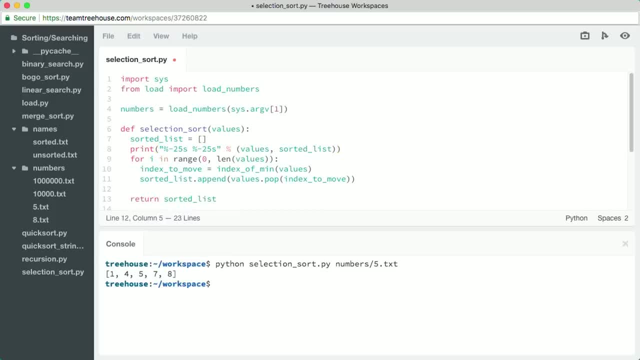 well, we'll keep looping until we've processed all of the values. in both halves of the list we're looking to copy over the lowest values first. so first we test whether the current value on the left side is less than the value on the right side. if the left side value is less, that's what we'll copy over to the sorted list. 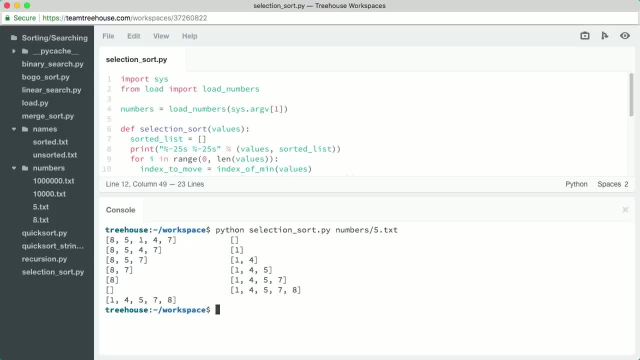 and then we'll move to the next value in the left half of the list. otherwise the current value from the right half must have been lower, so we'll copy that value value to the sorted list instead, And then we'll move to the next value in the right half of the list. 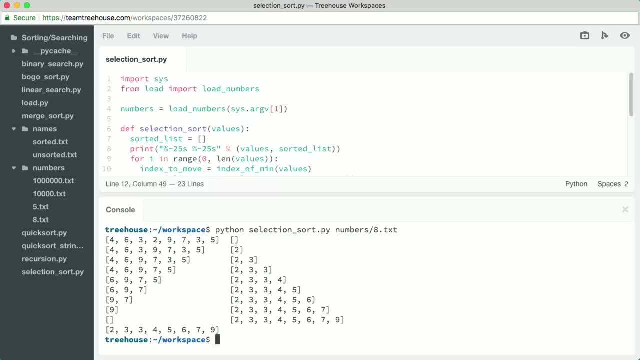 That ends the loop. At this point, one of the two unsorted halves still has a value remaining and the other is empty. We won't waste time checking, which is which We'll just copy the remainder of both lists over to the sorted list. 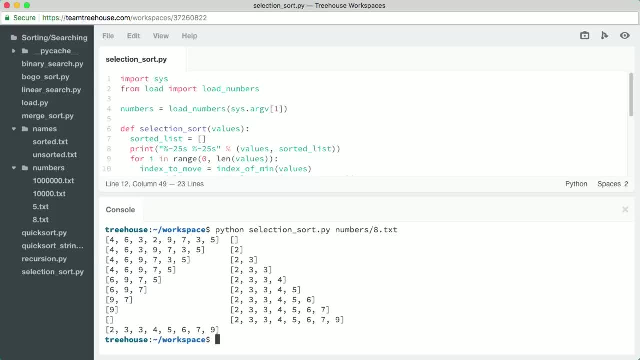 The one with the value left will add that value, and the empty one will add nothing. All the numbers from both halves should now be copied to the sorted list so we can return it. Finally, we need to kick the whole process off. 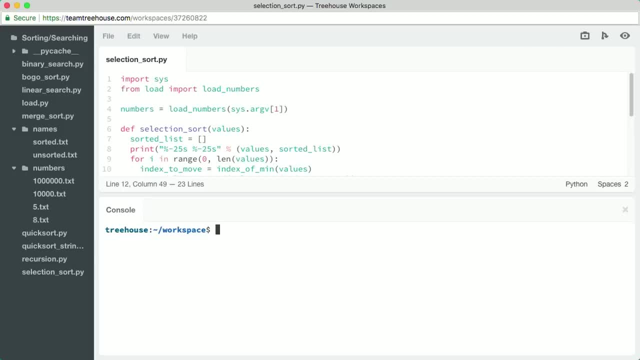 We'll call the merge sort function with the list of numbers we loaded and print the result. Let's save this And we'll try it out on our file with eight numbers- Python, munungsortpy numbers eighttxt- And it prints out the sorted list. 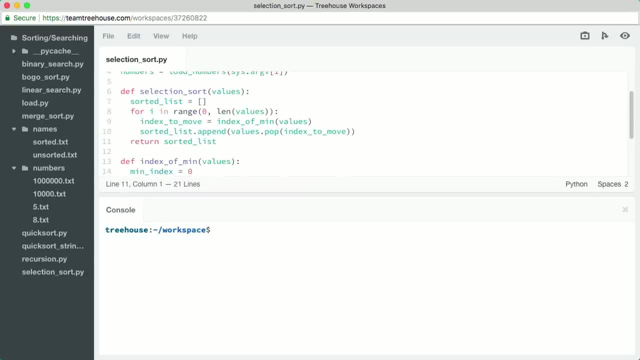 But again, this seems pretty magical. Let's add some print statements to get some insight into what it's doing. First we'll print the unsorted list so we can refer to it. We'll add a print statement right before we call the merge sort function for the first time. 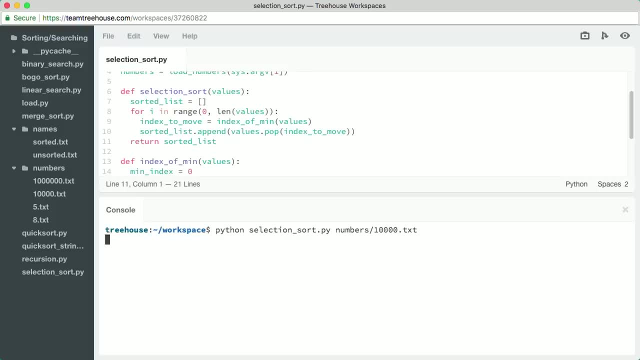 Then we'll add another print statement within the merge sort function right after the recursive list, after the recursive calls. This will show us the sorted left half and right half that it's returning Again. don't worry about the fancy Python formatting string, It just keeps the. 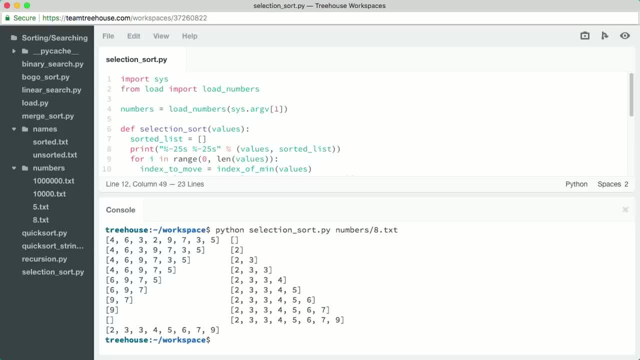 the current value is less than the previous minimum. If they're equal, it just keeps the first minimum value it found and waits to move the duplicate value over until the next pass through the list. So now we know that the selection sort algorithm works. 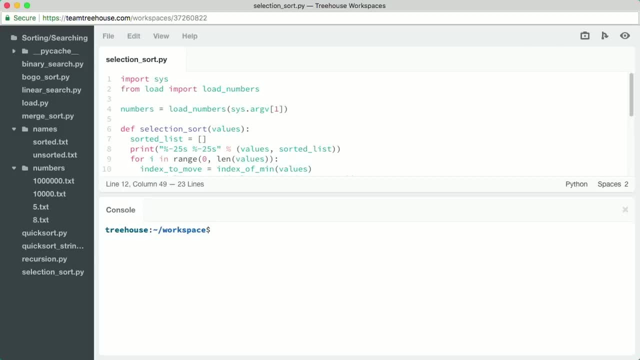 But the datasets we've been giving it to sort are tiny In the real world. algorithms need to work with datasets of tens of thousands or even millions of items and do it fast. I have another file with 10,000 random numbers in it. 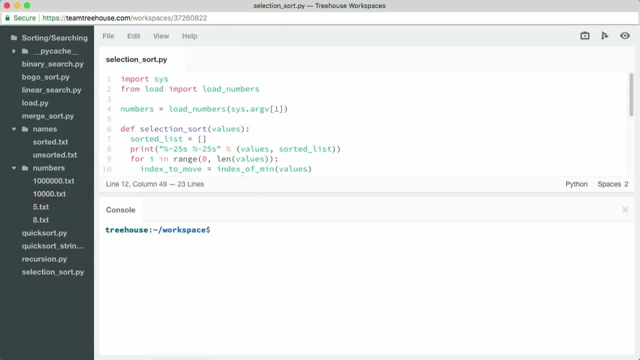 Let's see if selection sort can handle that. If I run this as it is now, though, it'll print out a lot of debug info as it sorts the list. So first I'm going to go into the program and remove the two print statements in the. 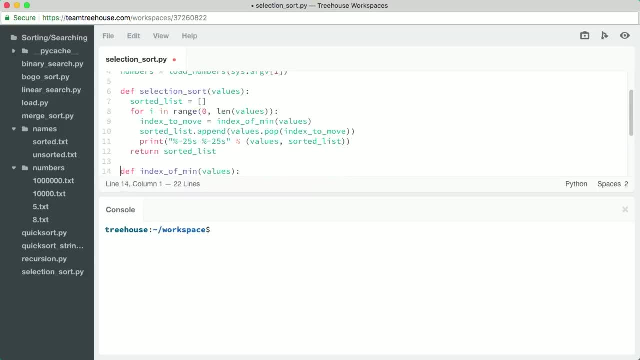 selection sort function. Now let's run the program again on the 10,000 dot text file and see how long it takes. I'm going to go into the program and remove the two print statements in the selection sort function. Now let's run the program again on the 10,000 dot text file and see how long it takes. 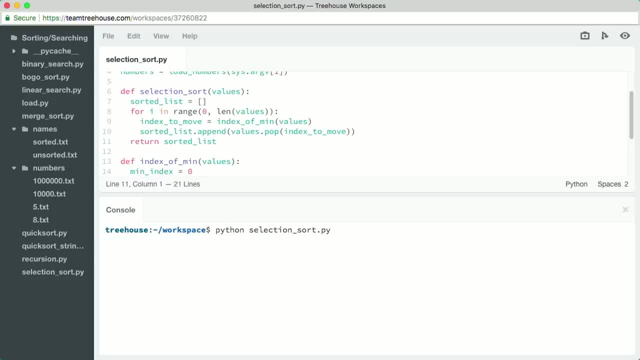 It's a little bit though. Let's see how long it takes to get to the 10,000 number. Let's go back to the program. I'm going to go to the Python Selections: sort dot pi Numbers: 10,000 dot text. 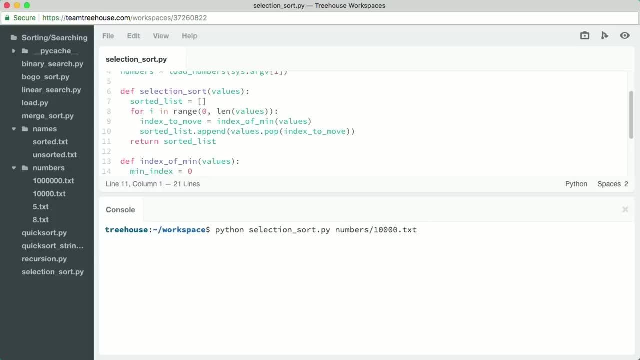 One, one thousand Two, one thousand Three, one thousand Four, one thousand Five, one thousand Six, one thousand Seven, one thousand Eight, one thousand Nine, one thousand Ten, one thousand Eleven, one thousand Twelve, one thousand Thirteen one thousand. 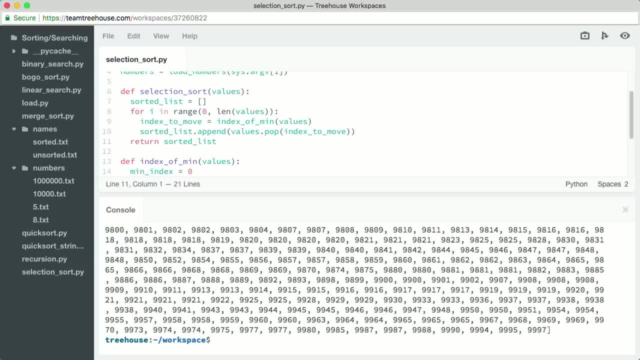 And it prints out all 10,000 of those numbers, neatly sorted. It took a little bit, though. How long? Well, counting the time off vocally isn't very precise. I'm going to go back to the program and see how long this takes. 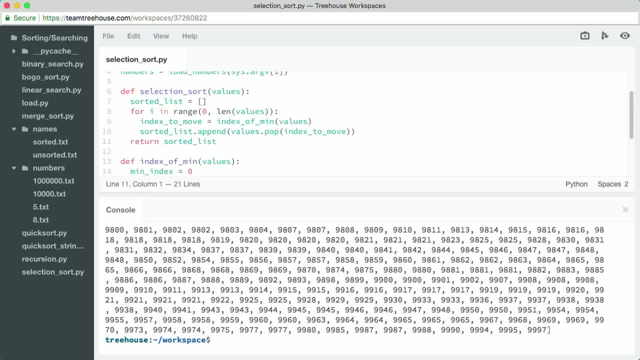 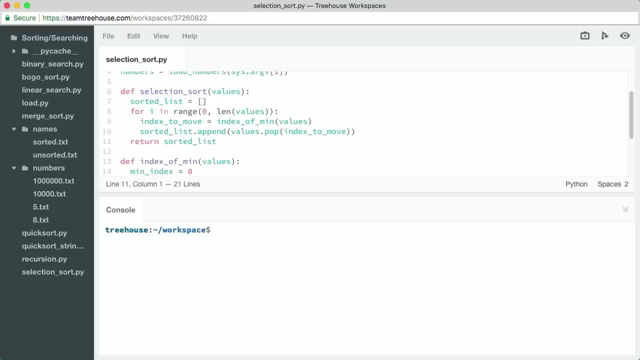 size and other programs running on the system can skew the amount of time your program takes to complete. Let me show you a unix command that's available here in workspaces which can help You type time followed by a space and then the command you want to run. 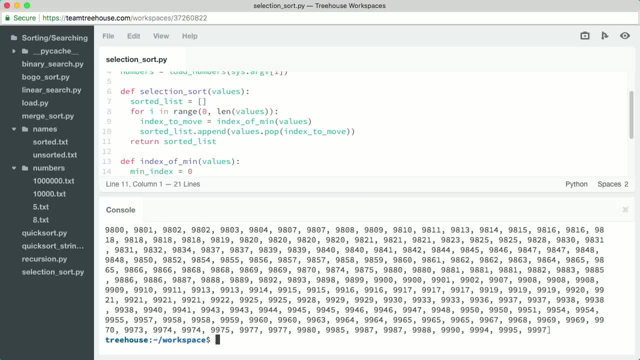 values neatly aligned. Let me resize my console, clear the screen and then we'll try running this again. What we're seeing are the values being returned from the recursive merge sort function calls, not the original calls to merge sort. So what you see here is after we reach the base case. 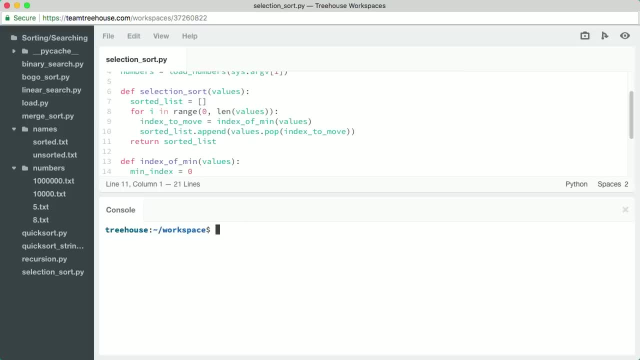 with a list that's only one item in length and the recursive calls start returning, the original list gets split into two unsorted halves: 4, 6,, 3, and 2, and 9,, 7,, 3, and 5.. 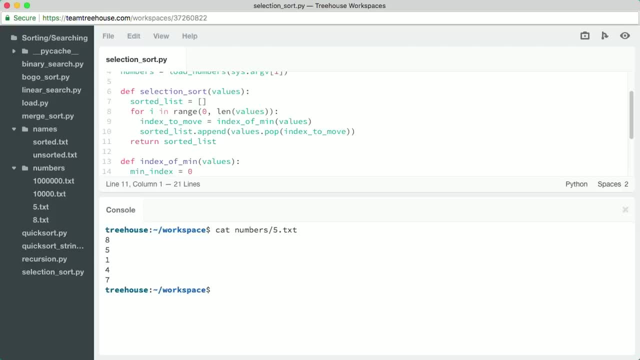 The first half gets split in half again: 4 and 6, and 3 and 2. And each of those halves is halved again into single element lists. There's nothing to sort in the single element list, so they're returned from the merge sort function as is Those single. 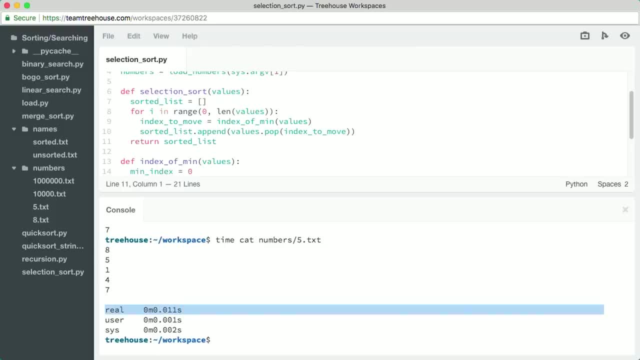 element lists are returned from the merge sort function, as is. Those two lists get merged into two sublists and sorted as they do. so The 4 and 6 sublist looks the same after sorting as it did before sorting, but the 3 and the 2 get sorted as they're combined. 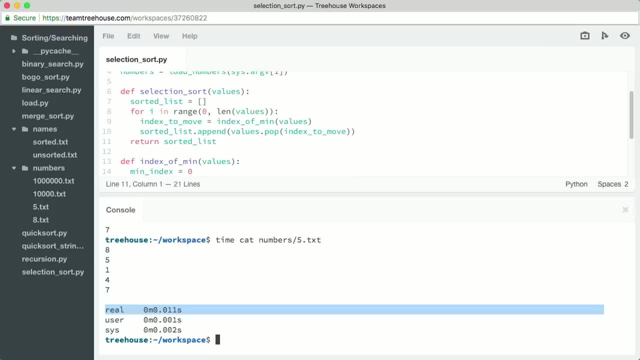 into a sublist. The new order is 2, 3.. The order is shifted again when those two sublists get combined back into a single list: 2, 3,, 4, 6. Then we recursively sort the right half of the. 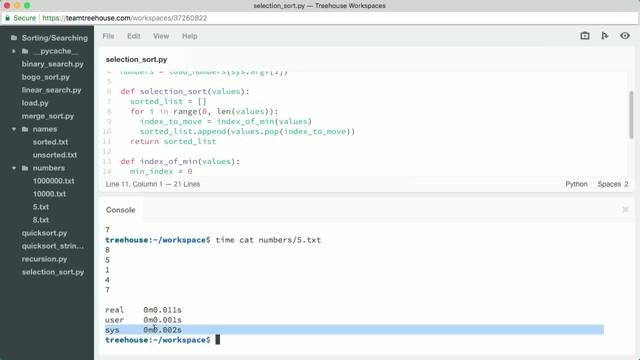 original list: 9,, 7,, 3, 5.. It gets split in half again: 9,, 7,, 3,, 5.. And the new order is 2, 3, 5.. It gets split in half again 9,, 7,, 3, 5.. It gets split in half again 9,, 7,, 3,, 5.. And each of those 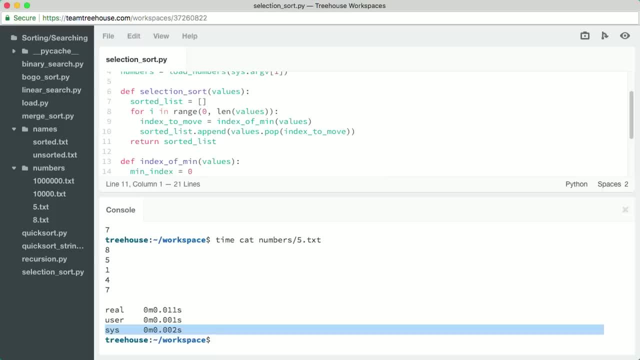 halves get broken into single element lists. There's nothing to sort there, so the single element lists are returned as is. The first. two are sorted as they're merged: 7, 9.. And so are the second: 3, 5.. And then those two sublists get sorted as they're combined into another sublist. 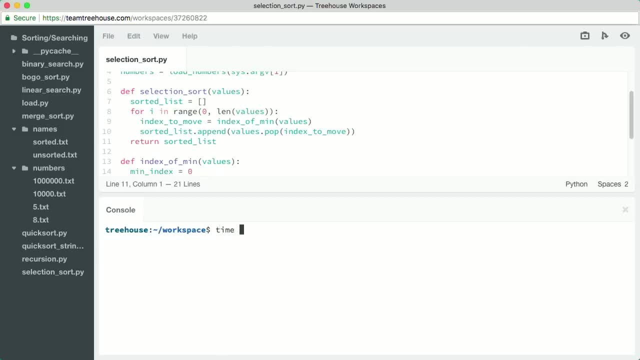 3, 5,, 7, 9.. And finally, everything is sorted as it's merged back into the full sorted list: 2, 3,, 3,, 4,, 5, 6, 7, 9.. That's how merge sort works on a list of eight numbers. 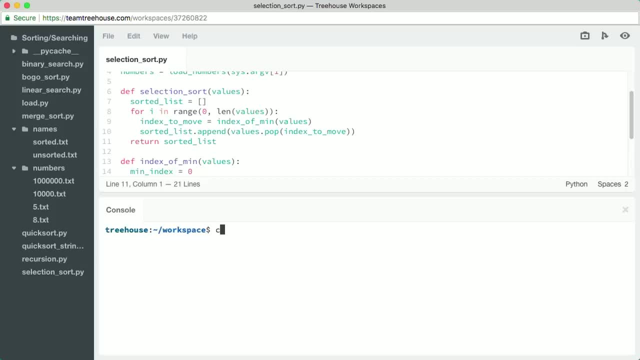 So this command by itself will print the contents of our 5.txt file cat as in concatenate numbers 5.txt. And this command will do the same thing, but it'll also keep track of how long it takes the cat program to complete and report the result time: cat numbers 5.txt. 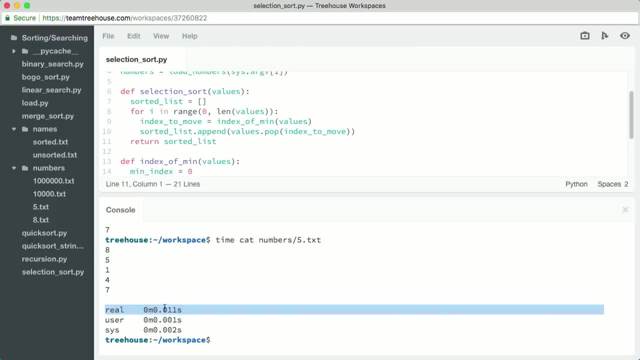 The real row in the results is the actual amount of time for when the program started running to when it completed. We can see it finished in a fraction of a second. But, as we said, other programs running on the system can take CPU resources in which 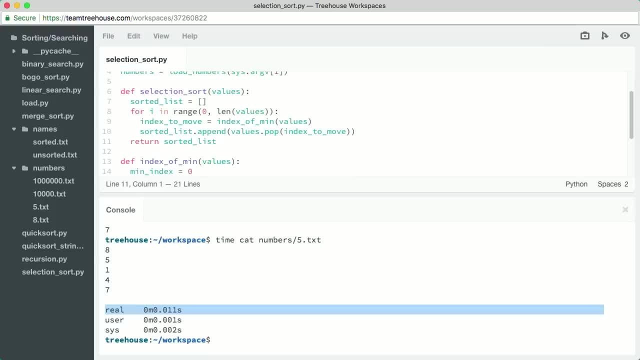 case your program will seem slower than it is. so we generally want to ignore the real result. The user result is the amount of time the CPU actually spent running the program code. So this is the total amount of time the code inside the cat program took to run. 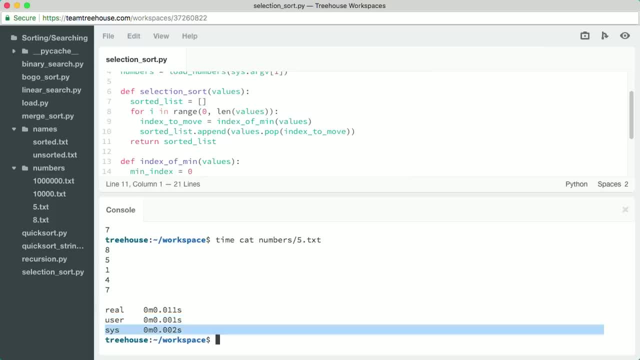 The sys result is the amount of time the CPU spent running Linux kernel calls that your code made. The Linux kernel is responsible for things like network communications and reading files, so loading the 5.txt file is probably included in this result. In evaluating code's performance, we're generally going to want to add together the: 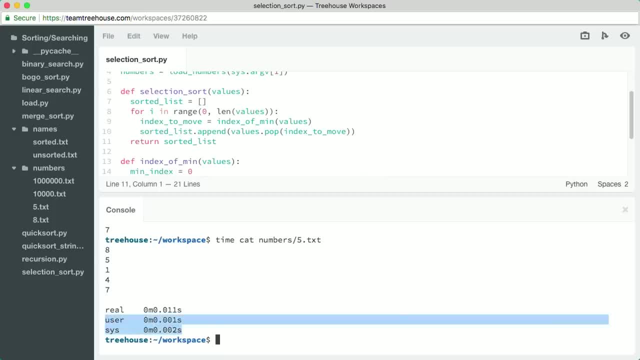 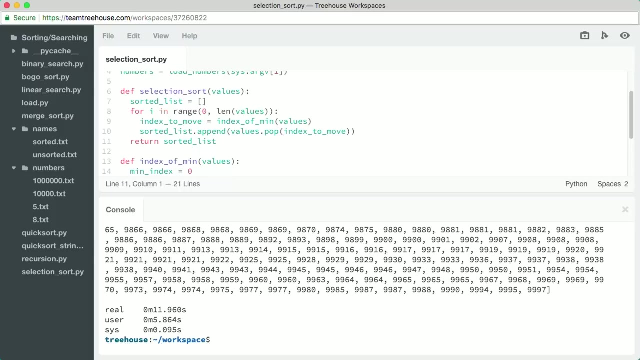 user and sys results. But cat is a very simple program. Let's try running the time command on our code and see if we get a more interesting result. time python selection-sortpy numbers- 10,000.txt. This takes much longer to complete- nearly 12 seconds according to the real time measurement. 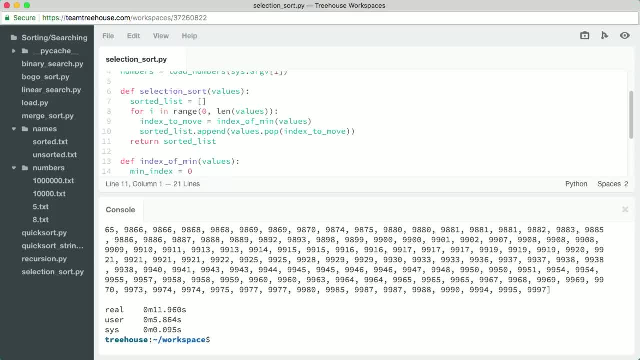 But, as we said, the real result is often skewed. so let's disregard that. It's a very simple program. It's a very simple program. If we add the user and sys runtimes together, we get about 6 seconds. The time for the program to complete will vary a little bit each time you run it. 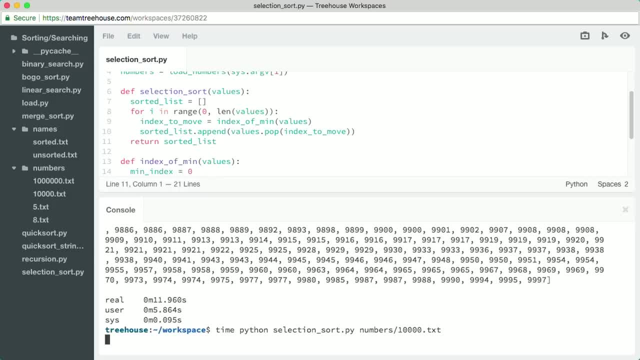 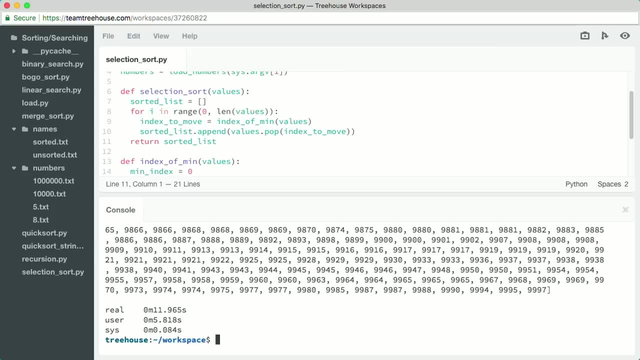 But if it's doing the same operations it usually won't change more than a fraction of a second. If I run our selection-sort script on the same file, you can see it completes in roughly the same time. Now let's try it on another file with 1 million numbers. 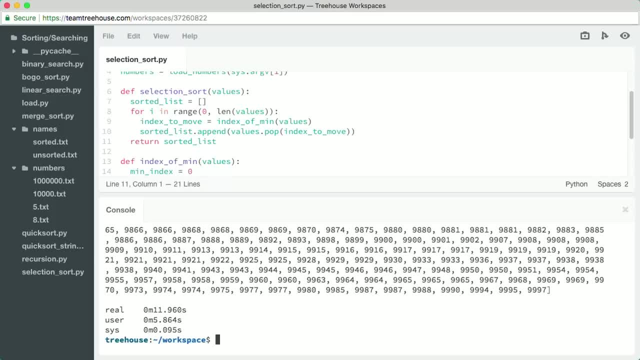 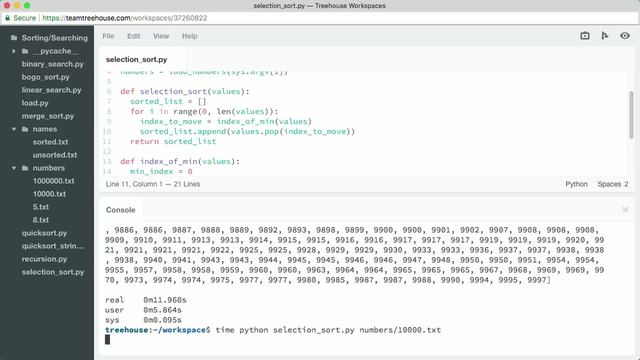 Let's see if it works on a bigger list. First I'll remove the two print statements so we don't get an overwhelming amount of debug output. Then I'll run it on a list of 10,000 items. Python merge sort, dot, pi numbers: 10,000, dot text. 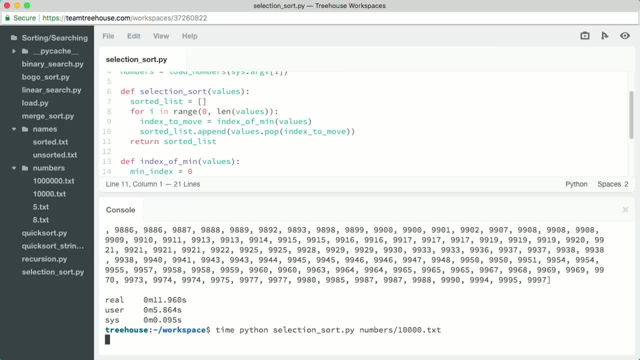 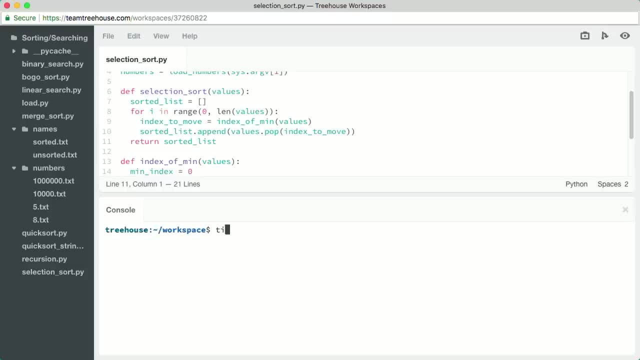 Not only did it work, it was pretty fast. But which is faster: merge sort or quick sort? We'll look at that next. I've removed the call to print that displays the sorted list at the end of our selection sort, quick sort and merge sort scripts. That way it'll still run the sort. 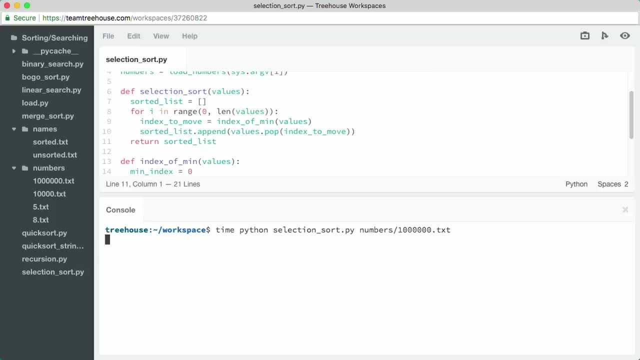 but the output won't get in the way of our comparing runtimes. Let's try running each of these scripts and see how long it takes Time. Python Selection- Sort. We'll do that one first Numbers 10,000, dot text. 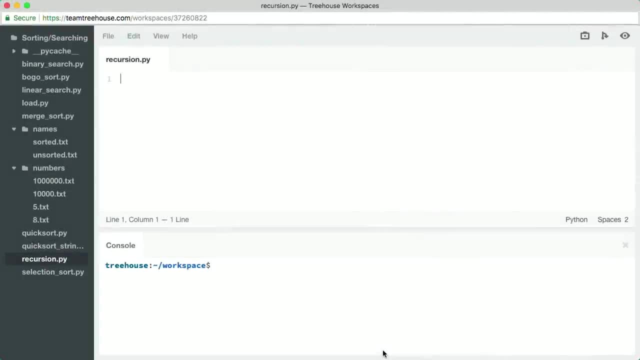 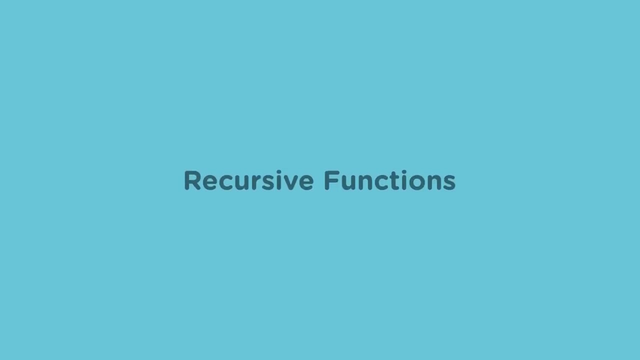 We combine the user and sys results and that gives us about six seconds. Now let's try quick sort, Time Python. Quick sort dot pi numbers 10,000, dot text Much faster, less than a second. And finally time Python. 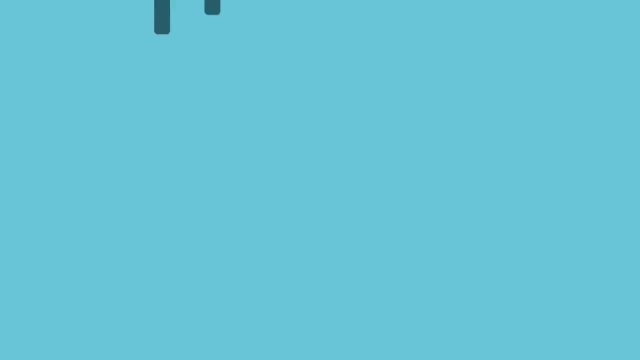 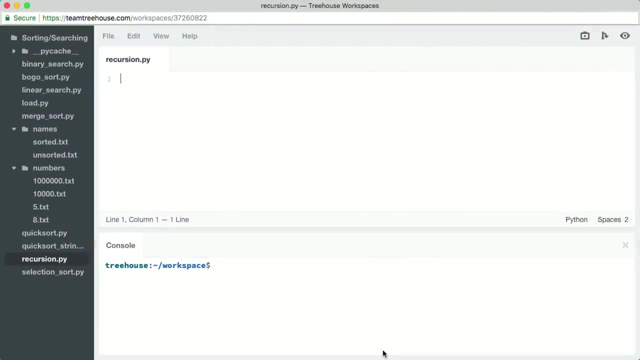 Merge sort: dot pi numbers: 10,000, dot text: A little longer, but far less than a second. So even on a list with just 10,000 numbers, selection sort takes many times as long as quick sort and merge sort. 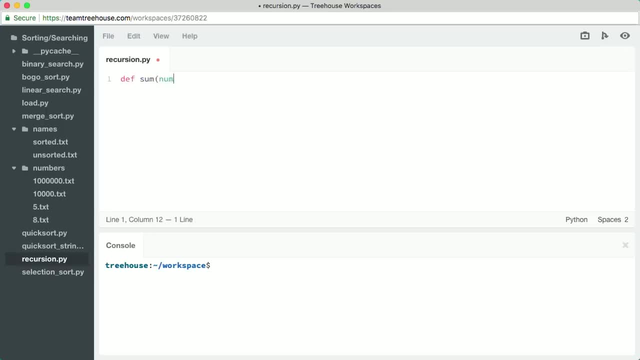 And remember I ran the selection sort script on a file with a million numbers and it took so long that my workspace timed out before it completed. It looks like selection sort is out of the running. It's a viable sorting algorithm. It may be easy to understand and implement, but it's just too slow to handle the huge data sets that are out in the real world. 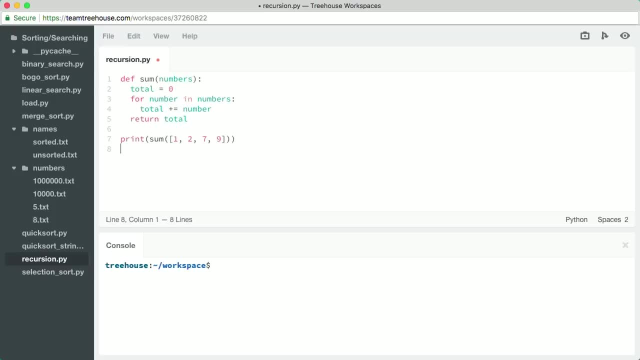 Now let's try quick sort and merge sort on our file with a million numbers and see how they compare there. Time Python: Quick sort dot pi numbers- 1,000, dot text. Time Python: Quick sort dot pi numbers- 1,000, dot text. 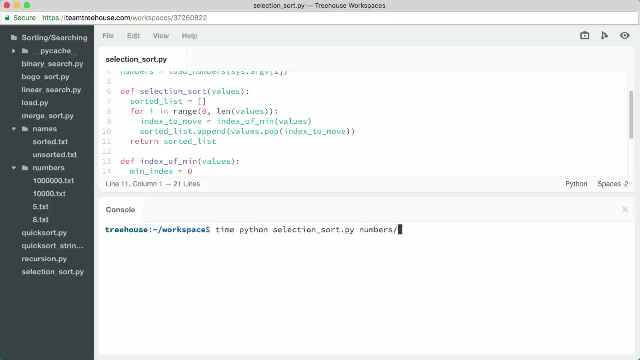 time python- selection-sortpy numbers- 1,000,000.txt. Let's try it on another file with 1,000,000 numbers. time python- selection-sortpy numbers- 1,000,000.txt. Let's try it on another file with 1,000,000 numbers. 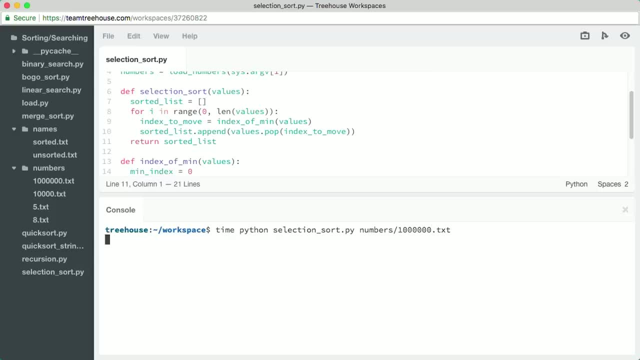 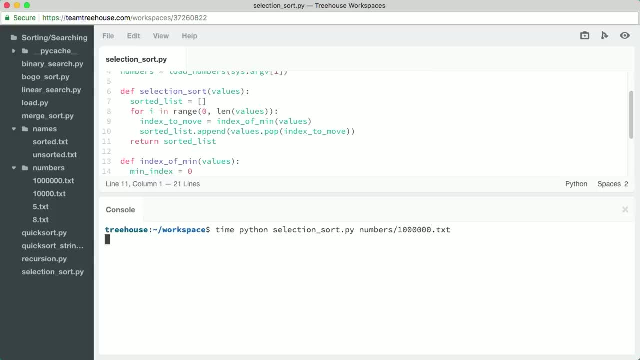 Let's try it on another file with 1,000,000.txt. How long does this one take? I don't even know. While designing this course, I tried running this command and my workspace connection timed out before it completed, So we'll just say that selection sort takes a very, very long time to sort a million numbers. 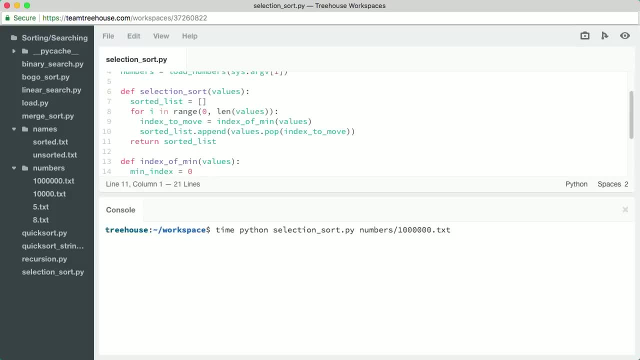 If we're going to sort a list that big, we're going to need a faster algorithm. We'll look into alternative sorting algorithms shortly. The next two sorting algorithms we look at will rely on recursion, which is the ability of a function to call itself. 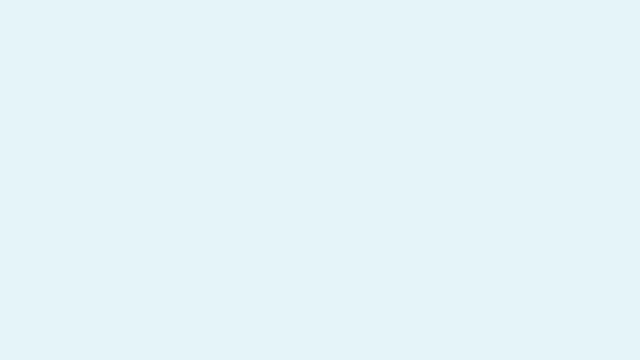 So, before we move on, we need to show you how recursion works. Recursive functions can be very tricky to understand. Imagine a row of dominoes stood on end where one domino falling over causes the next domino to fall over, which causes the next domino to fall over, causing a chain reaction. 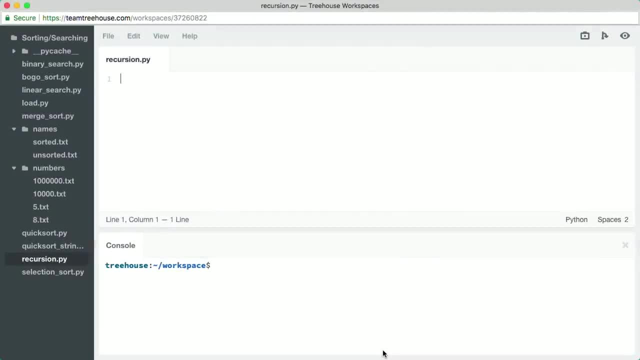 It's kind of like that. Let's suppose we need to write a function that adds together all the numbers in an array or, in the case of Python, a list. Normally we'd probably use a list, But we're going to use a loop for this sort of operation. 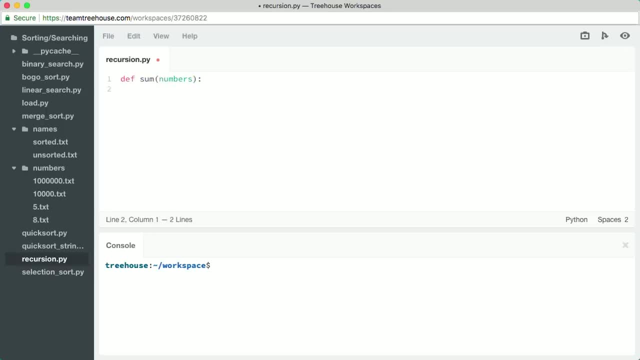 The function takes a list of the numbers we want to add. The total starts at zero. We loop over every number contained in the list and we add the current number to the total. Once we're done looping, we return the accumulated total. 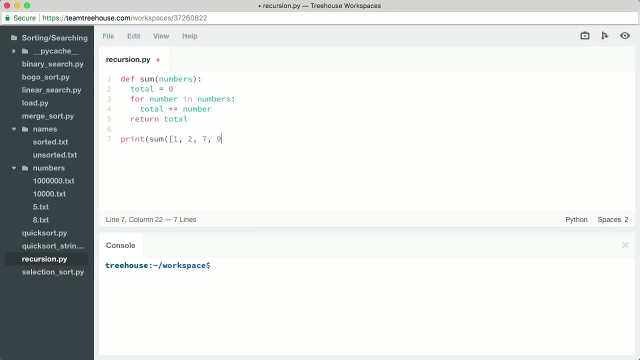 If we call this sum function with a list of numbers, it'll return the total. When we run this program, it'll print out that return value 19.. Let's try it real quick: Python Recursionpy. Oh whoops. 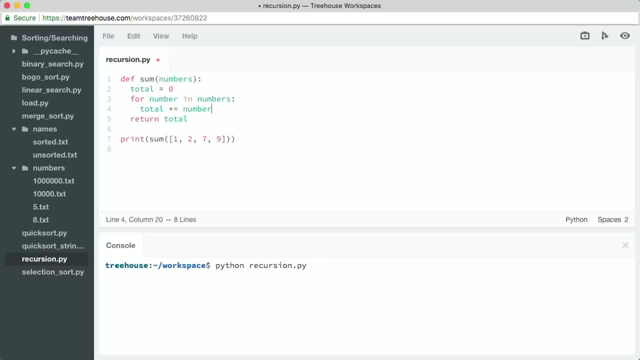 I mustn't forget to save my work here And run it, and we see the result 19.. To demonstrate how recursion works, let's revise the sum function to use recursion instead. Note that recursion is not the most efficient way to add a list of numbers together. 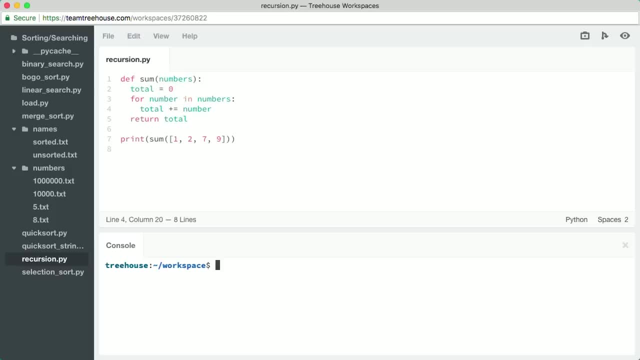 But this is a good problem to use to demonstrate recursion because it's so simple. One thing before I show you the recursive version: though: This example is going to use the Python recursion. It uses the Python slice syntax, so I need to take a moment to explain that for those. 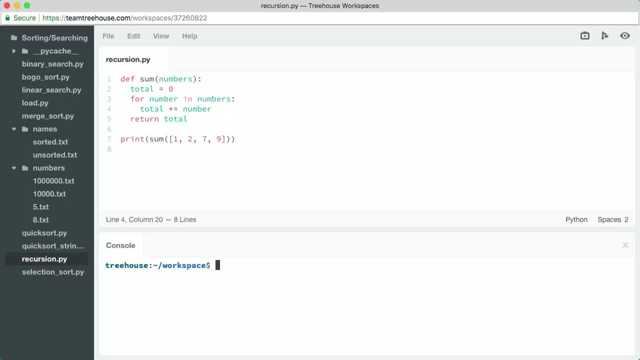 Time Python. Quick sort dot pi numbers- 1,000, dot text. Looks like it took about a second, So now we only have 11 seconds of CPU time. Now let's try merge sort Time Python. merge sort dot pi numbers- 1,000, dot text. 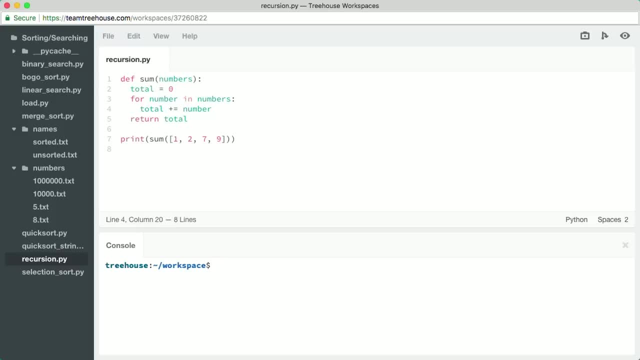 That took about fifteen seconds of CPU time. It looks like quick sort is marginally faster than merge sort on this sample data. We have to learn a lot of details for each algorithm we've covered in this course. Developers who need to implement their own algorithm follow them. 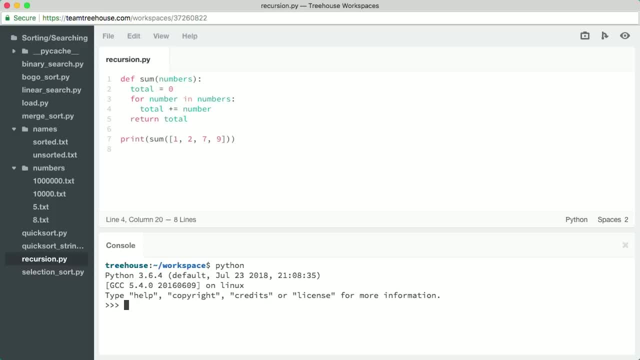 So here's something I can tell you often need to choose an algorithm for each and every problem they need to solve, And they often need to discuss their decisions with other developers. Can you imagine needing to describe all the algorithms in this same level of detail all the time? 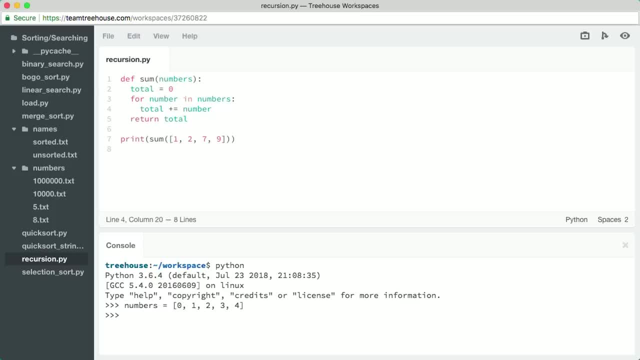 You'd spend all your time in meetings rather than programming. That's why Big O Notation was created: as a way of quickly describing how an algorithm performs as the dataset it's working on increases in size. Big O Notation lets you quickly compare several algorithms. 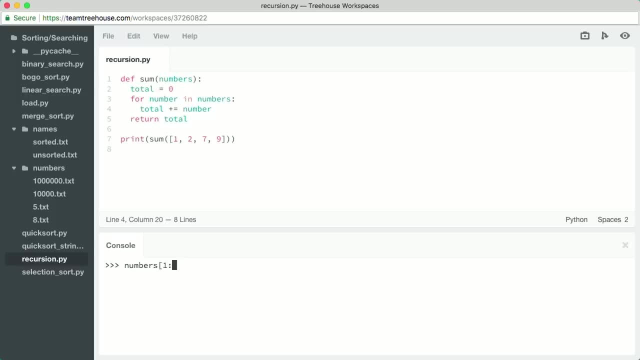 to choose the best one for your problem. The algorithms we've discussed in this course are very well known. Some job interviewers are going to expect you to know their Big O runtimes, So let's look at them. Remember that the N in Big O Notation. 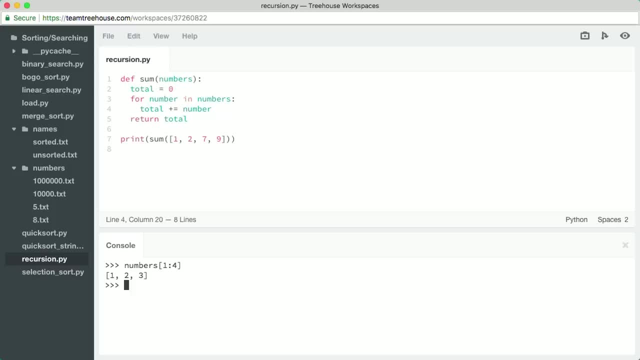 refers to the number of elements you're operating on With Selection Sort. you need to check each item in the list to see if it's the lowest so you can move it over to the sorted list. So that's N operations, Suppose you're doing Selection Sort. 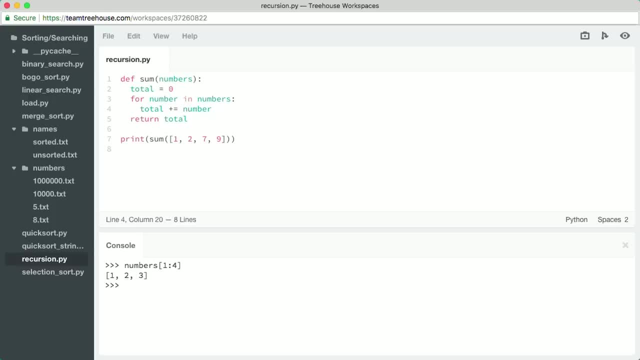 on a list of five items and N in this case would be five. So that's five operations before you can move an item to the sorted list. But with Selection Sort you have to loop over the entire list for each item you want to move. 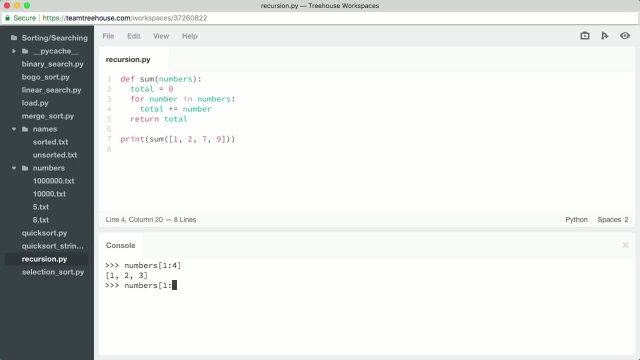 There are five items in the list and you have to do five comparisons to move each one. So it's more like five times five operations. Or if we replace five with N, it's N times N or N squared. But wait, you might say. 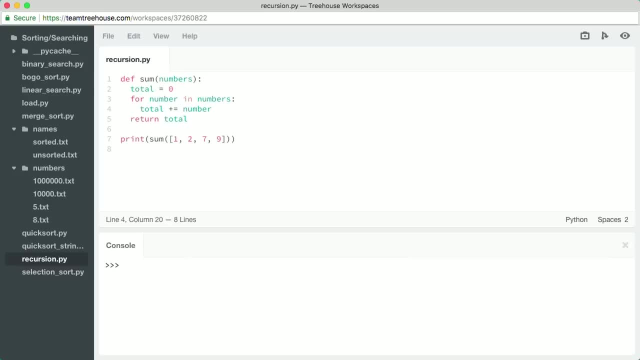 half of that five by five grid of operations is missing because we're testing one fewer item in the unsorted list with each pass. So isn't it more like one half times N times N? And this is true. We're not doing a full N squared operations. 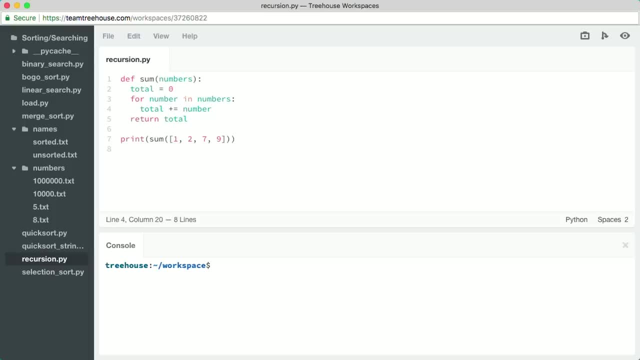 not familiar with it. A slice is a way to get a series of values from a list. Let's load up the Python REPL or read-evaluate-print loop so I can demonstrate. We'll start by creating a list of numbers to work with. 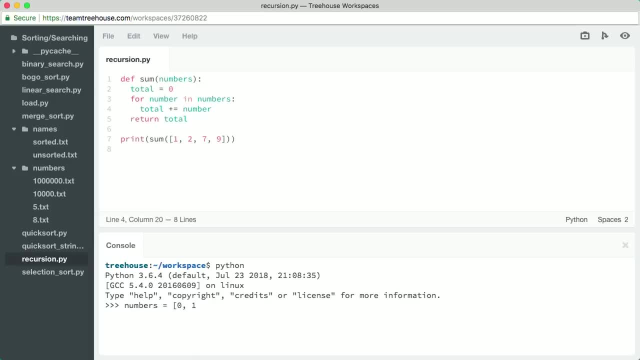 Numbers equals a list with 0,, 1,, 2,, 3, and 4, containing those numbers. Like arrays in most other languages, Python list indexes are a set of numbers. They're not a set of numbers. They're a set of numbers. 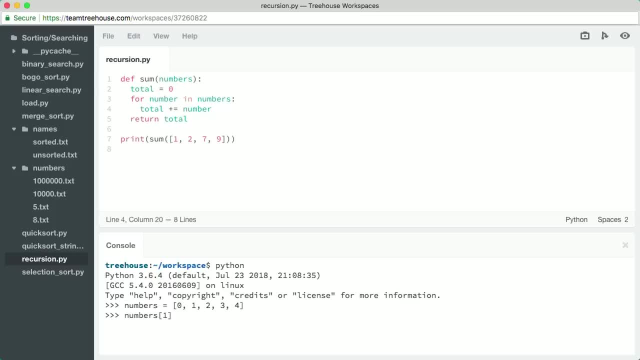 They start at 0. So numbers 1 will actually get the second item from the list. With slice notation I can actually get several items back. It looks just like accessing an individual index of a list, But then I type a colon followed by the list index that I want up to but not including. 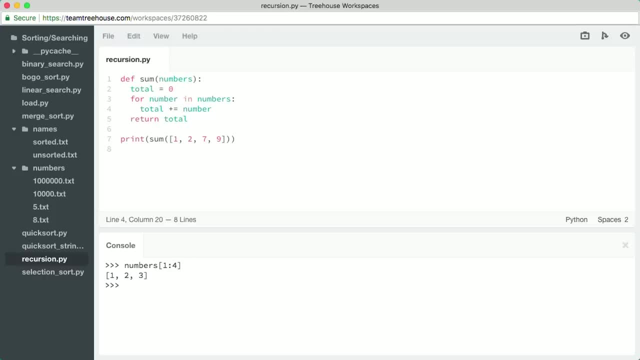 So numbers 1, colon 4 would get us the second up to, but not including the fifth items from the list, That is, It will get us the second through the fourth items. Now I know what you're thinking and you're right. 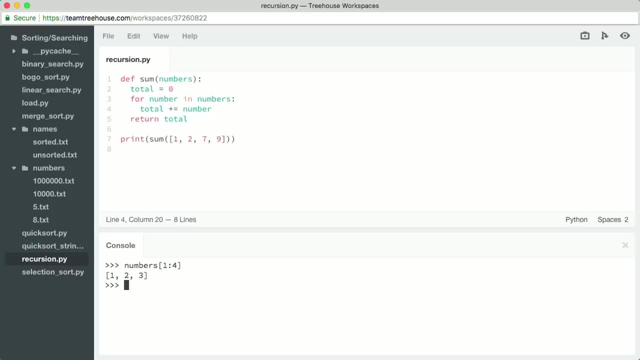 That up to, but not including rule is a little counter-intuitive, But you can just forget all about it for now, because we won't be using a second index with any of our Python slice operations in this course. Here's what we will be using. 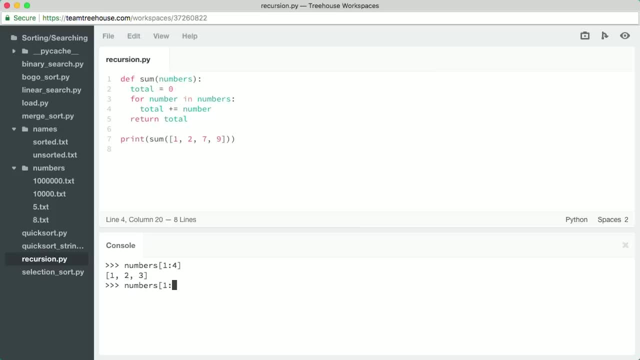 When you leave the second index off of a Python slice, it gives you the items from the first index up through the end of the list, wherever that is. So numbers 1, colon with no index following. it will give us the second index followed. 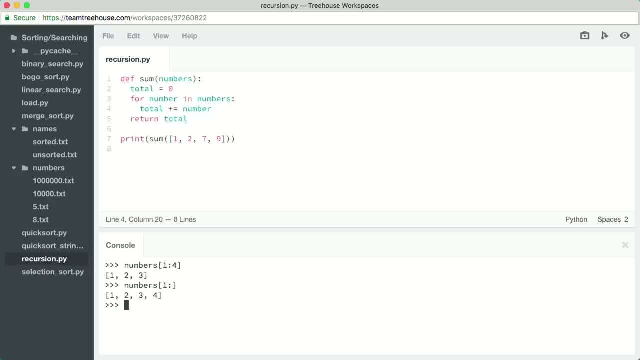 by the second index up through the end of the list. Numbers 2, colon will give us items from the third index up through the end of the list. You can also leave the first index off to get everything from the beginning of the list. 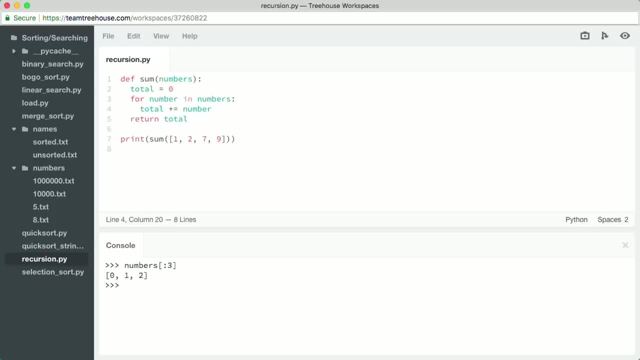 Numbers, colon 3, will get us everything from the beginning of the list up to, but not including, the third index. It's also worth noting that if you take a list with only one item and you try to get everything from the non-existent second item onwards, the result will be the same as the. 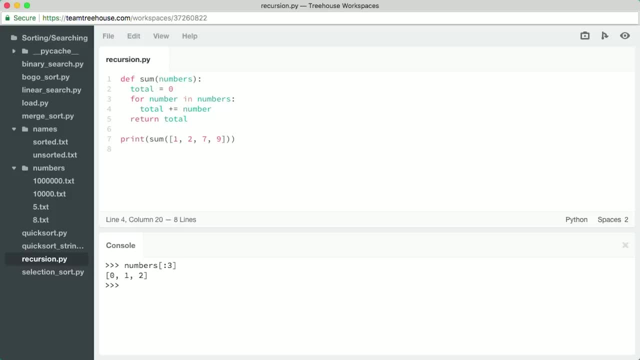 But remember, in Big O notation, as the value of N gets really big, constants like one half become insignificant And so we discard them. The Big O runtime of Selection Sort is widely recognized as being O- N squared. Quicksort requires one operation. 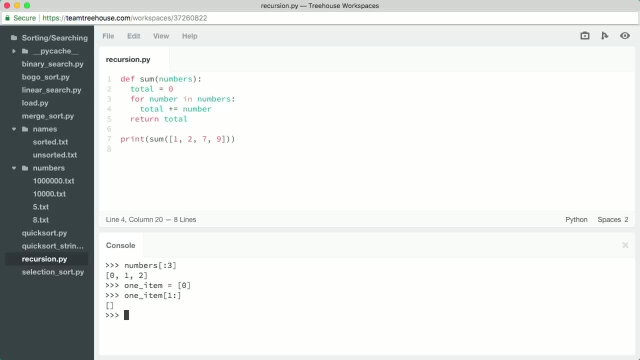 for each element of the list it's sorting. It needs to select a pivot first, and then it needs to sort elements into lists that are less than or greater than the pivot. So that's N operations. To put that another way, if you have a list of eight items, 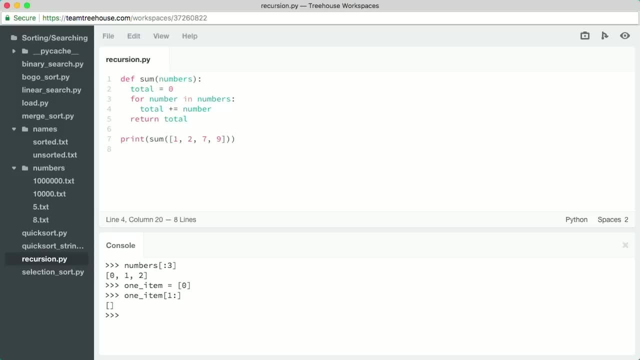 then N is eight. So it will take eight operations to split the list around the pivot. But of course the list isn't sorted after splitting it around the pivot, just once. You have to repeat those eight operations several times, In the best case. 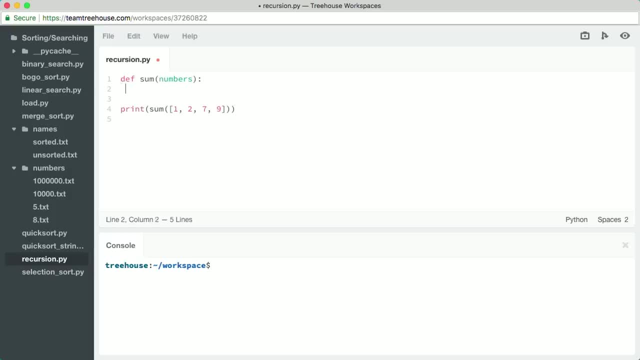 you'll pick a pivot that's right in the middle of the list, so that you're dividing the list exactly in half. Then you keep dividing the list in half until you have a list with a length of one. The number of times you need to divide N in half. 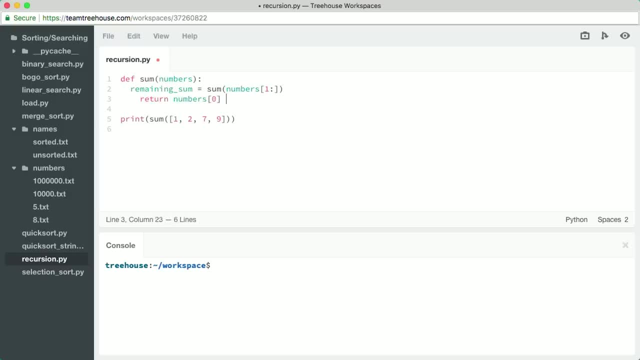 until you reach one is expressed as log N, So you need to repeat N sorting operations, log N times. That leaves us with the best case: runtime for Quicksort of O N log N. But that's the best case. What about the worst case? 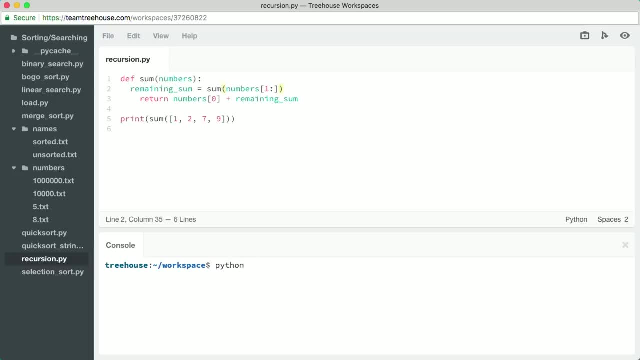 Well, if you pick the wrong pivot, you won't be dividing the list exactly in half. If you pick a really bad pivot pivot, the next recursive call to quicksort will only reduce the list length by one. Since our quicksort function simply picks the first item to use as a pivot, we can make it pick the worst. 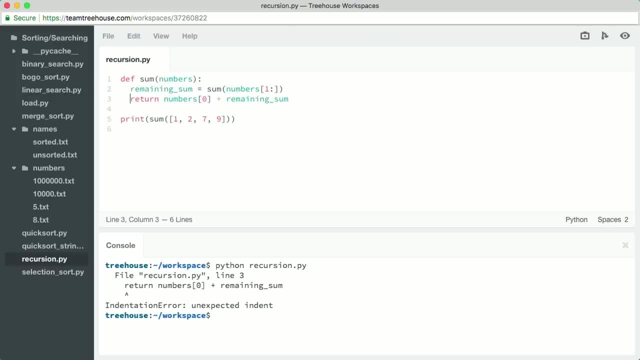 possible pivot repeatedly, simply by giving it a list that's sorted in reverse order. If we pick the worst possible pivot every time, we'll have to split the list once for every item it contains and then do end sorting operations on it. You already know another sorting algorithm that only 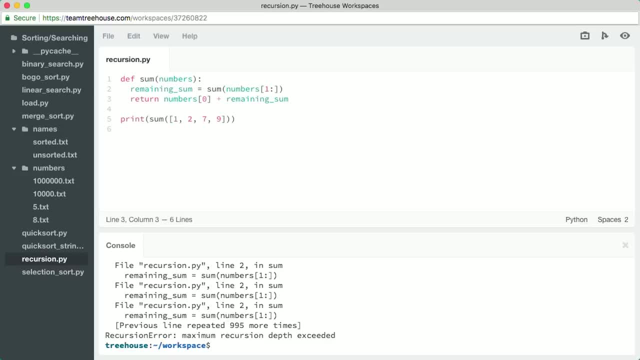 manages to reduce the list by one element with each pass: selection sort. Selection sort has a runtime of o n squared, and in the worst case that's the runtime for quicksort as well. So which do we consider when trying to decide whether to use quicksort- the best case or the worst case? 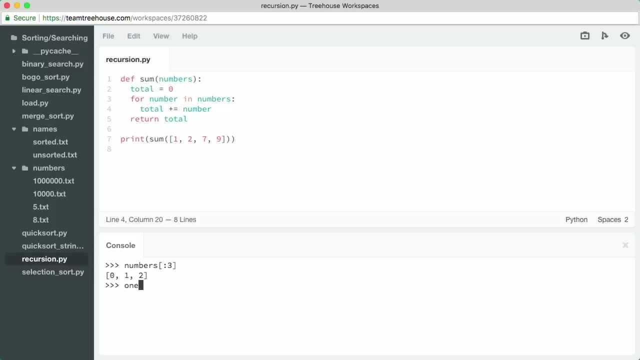 first item. So if I create a list with just one item in it and I try to access from the second element onwards, the second element doesn't exist, so the result will be an empty list. Don't worry too much about remembering Python slice syntax. 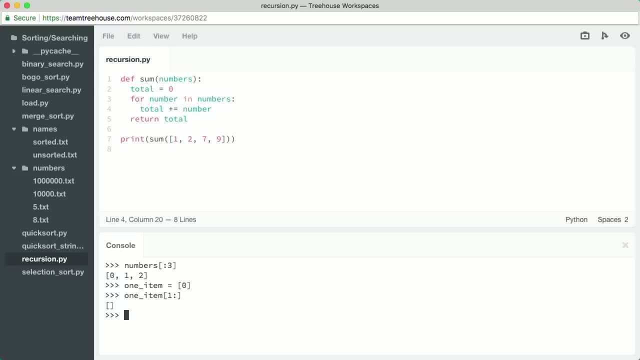 It's not an essential part of sorting algorithms or recursion. I'm only explaining it to help you read the code you're about to see. I'm only explaining it to help you read the code you're about to see. I'm only explaining it to help you read the code you're about to see. 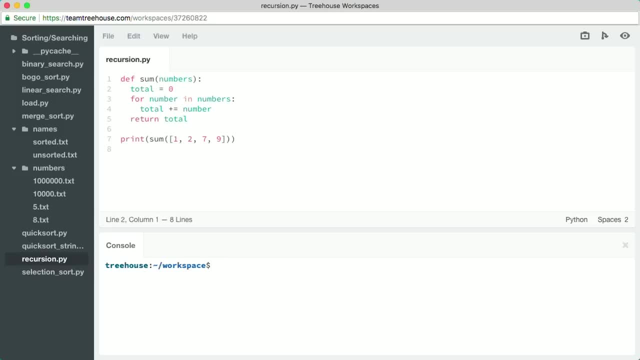 So I'm going to exit the Python REPL. Now that we've covered recursion, we can convert our sum function to a recursive function. It'll take the list of numbers to add, just like before. Now here's the recursive part. We'll have the sum function call itself. 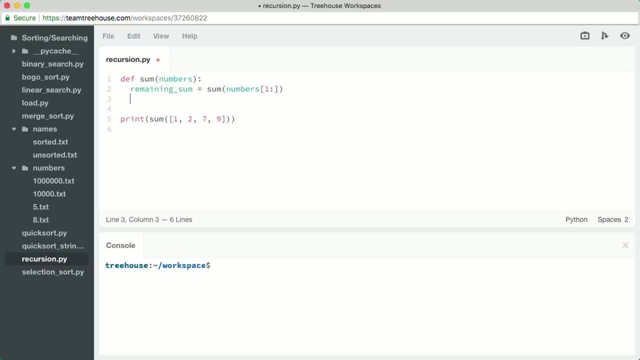 We use slice notation to pass the entire list of numbers except the first one. Then we add the first number in the list to the result of the recursive function call and return the result. Okay, Okay, four numbers first. it'll call itself with the remaining three numbers That call to sum will. 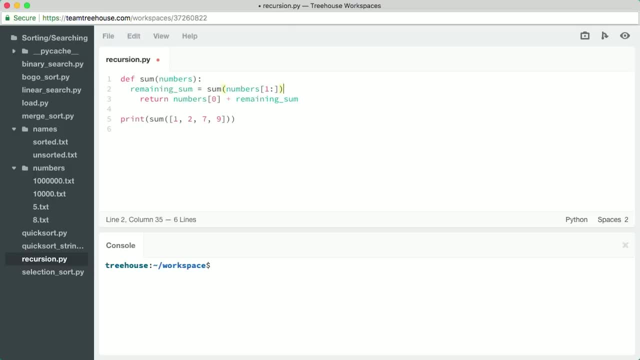 then call itself with the remaining two numbers and so on. But if we save this and try to run it python, recursionpy, well, first we get a syntax error. It looks like I accidentally indented something I shouldn't have, so let me go fix that real quick. 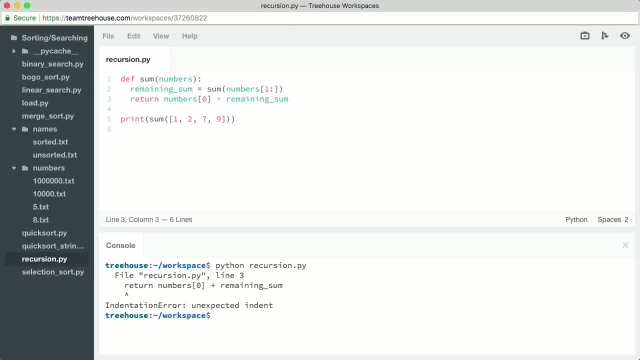 There we go. That suggested to python that there was a loop or something there when there wasn't. So let's go back to the terminal and try running this again. There we go. Now we're getting the error I was expecting: Recursion error. maximum recursion depth exceeded. This happens because 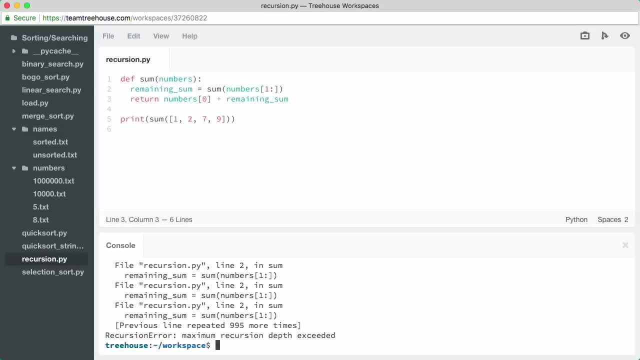 sum gets into an infinite loop. It keeps calling itself over and over. The reason is that when we get down to a list of just one element and we take a slice from the non-existent second element to the next element, we get a slice from the non-existent second element to the next element. 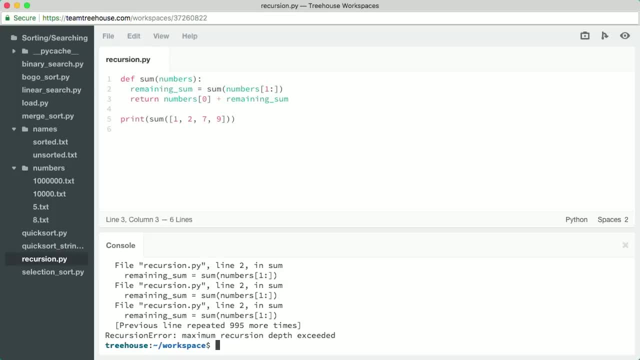 It keeps calling itself over and over. The reason is that when we get down to a list of just one element end, the result is an empty list. That empty list gets passed to the recursive call to sum, which passes an empty list in its recursive call to sum, and so on, until the Python interpreter 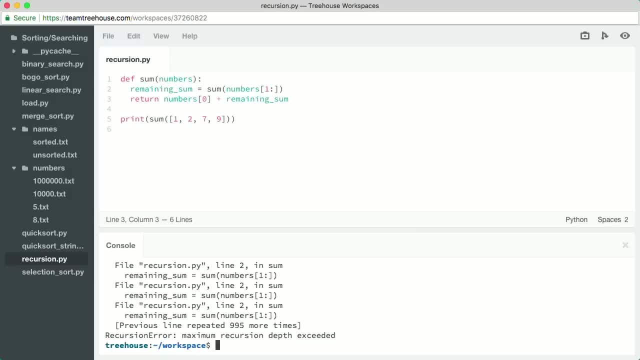 Well, as long as your implementation doesn't just pick the first item as a pivot, which we did so we could demonstrate this issue. it turns out that, on average, quicksort performs closer to the best case. Many quicksort implementations accomplish this simply by picking a pivot at random on each. 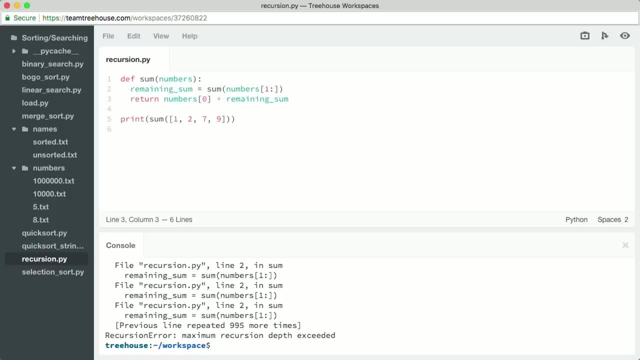 recursive loop. Here we are sorting our reverse sorted data again, but this time we pick pivots at random, which reduces the number of recursive operations needed. Sure, random pivots sometimes give you the best case, and sometimes you'll randomly get the worst case, but it all averages. 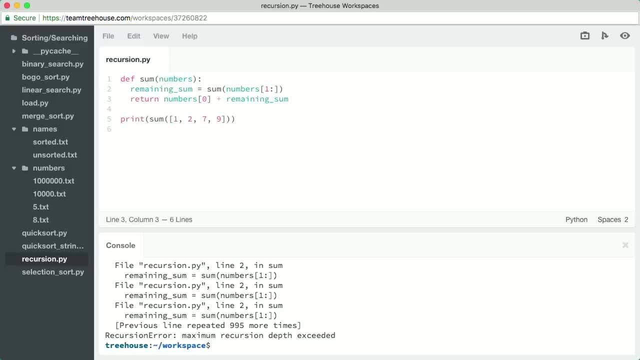 out over multiple calls to the quicksort function. Now, with merge sort, there's no increases as the data set it's operating on gets really, really big. But you can't always choose between two algorithms based just on their big O runtimes. 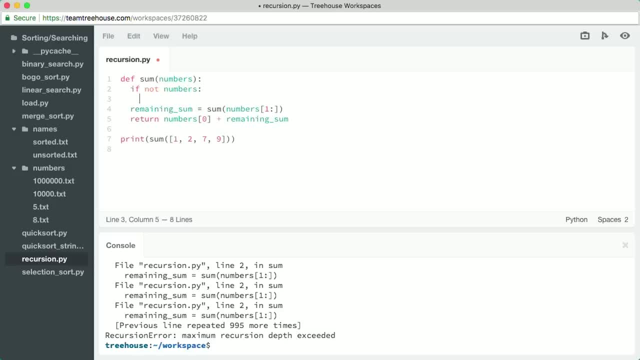 Sometimes there's additional info. you need to know about an algorithm to make a good decision. Now that we can sort a list of items, we're well on our way to being able to search a list efficiently as well. We'll look at how to do that in the next stage. 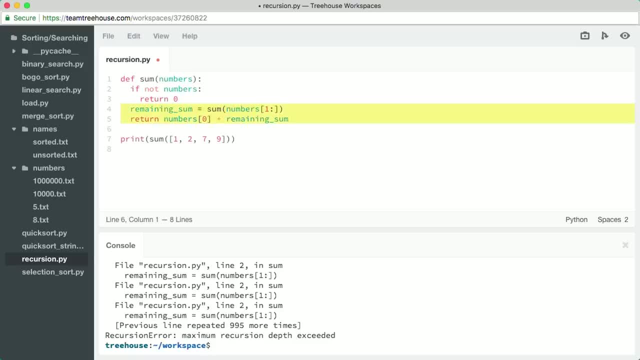 Now that we've covered sorting algorithms, the groundwork has been laid to talk about searching algorithms. If you need to search through an unsorted list of items, binary search isn't an option, because you have no idea which half of the list contains the item you're looking for. 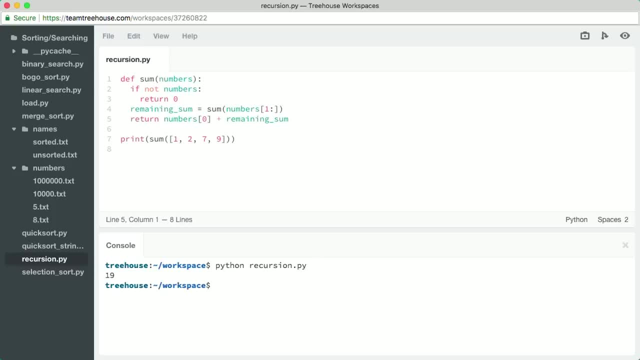 Your only real option is to start at the beginning and compare each item in the list to your target value, one at a time, until you find the value you're looking for. This algorithm is called linear search or sequential search, because the search proceeds in a straight line or sequence. 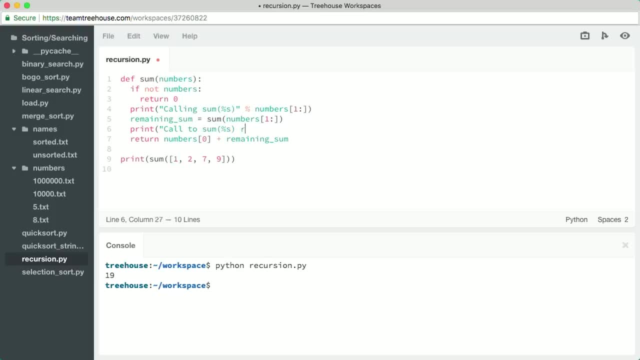 Even though linear search is inefficient, searching for just one name will happen so fast that we won't be able to tell anything useful about the algorithm's runtime. So let's suppose we had a hundred different names and that we needed to know where they appear in a list of unsorted names. Here's some code that demonstrates: 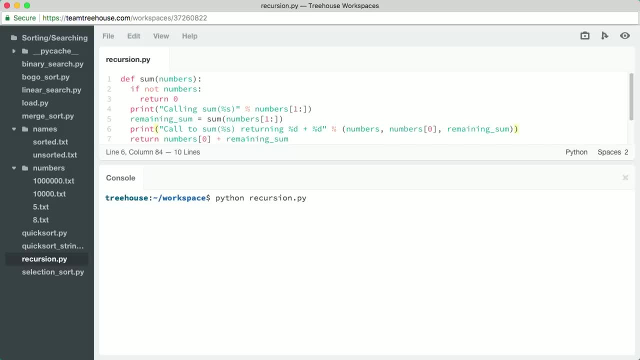 As usual, this code at the top isn't relevant to the search algorithm. It's just like the code that loaded a list of numbers from a file in the previous stage. but this code calls a different function, loadStrings. that loads a list of strings in. If you want, the loadStrings Python code. 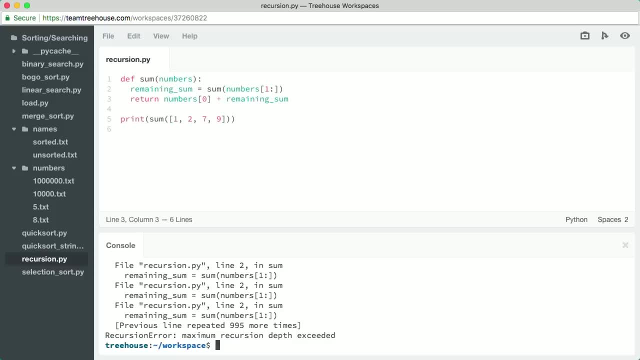 detects too many recursive calls and shuts the program down. What we need is to add a base case to this recursive function, a condition where the recursion stops. This will keep it from getting into an infinite loop With the sum function. the base case is when there are no elements left in. 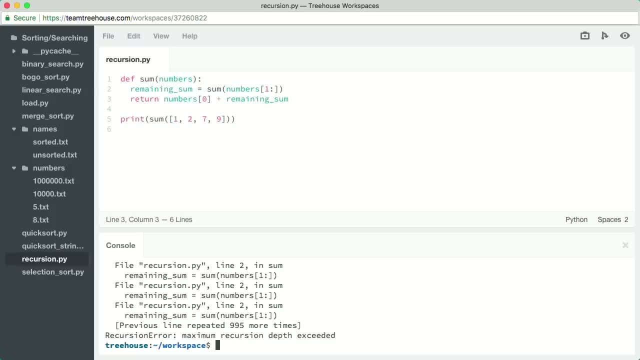 the list. In that case there is nothing left to add and the recursion can stop. A base case is the alternative to a recursive case, a condition where recursion should occur For the sum function. the recursive case is when there are still elements in the list to add together. 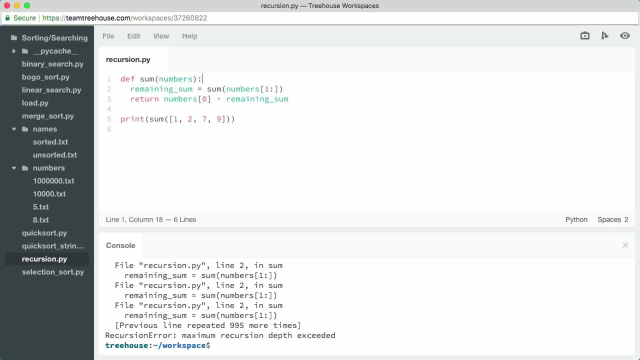 Let's add a base case at the top of the function. Python treats a list that contains one or more values as a true value and it treats a list containing no values as a false value. So we'll let an if statement that says: if there are no numbers in the list, we should return a sum of zero. 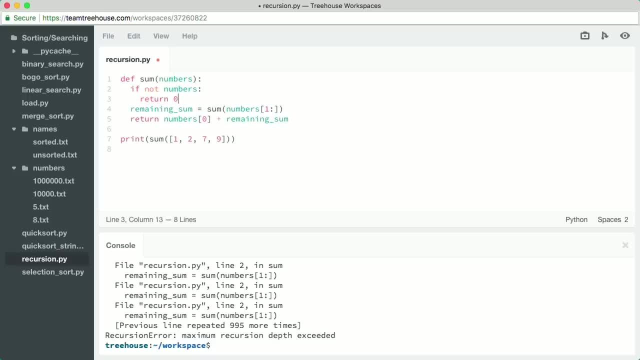 That way, the function will exit immediately without making any further recursive calls to itself. We'll leave the code for the recursive case unchanged. If there are still numbers in the list, the function will call itself with any numbers after the first, then add the return. 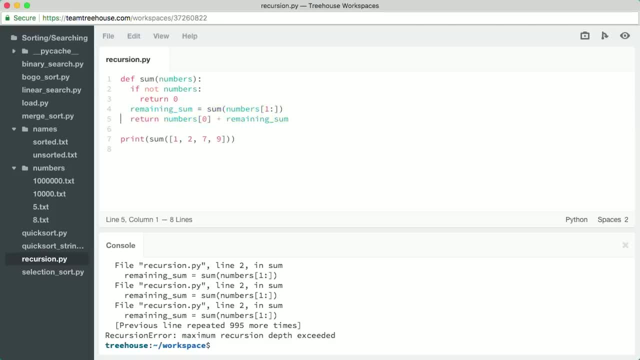 value to the first number in the list. Let's save this and try running it again. Python recursionpy. It'll output the sum of the numbers in the list 19.. But it's still not really clear how this worked. Let's add a couple print statements that will show us what it's doing. 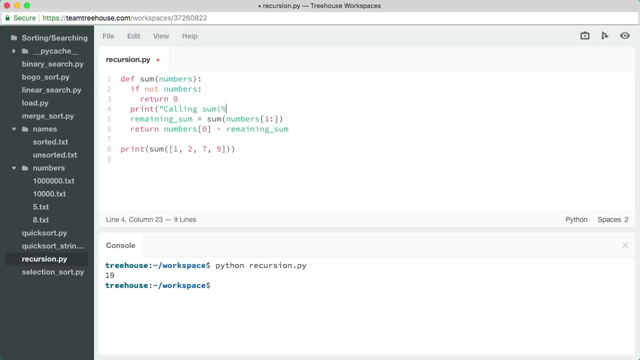 We'll show the recursive call to sum and what it's being called with. We'll also add a call to print right before we return, showing which of the calls to sum is returning and what it's returning. Let me save this and resize it. 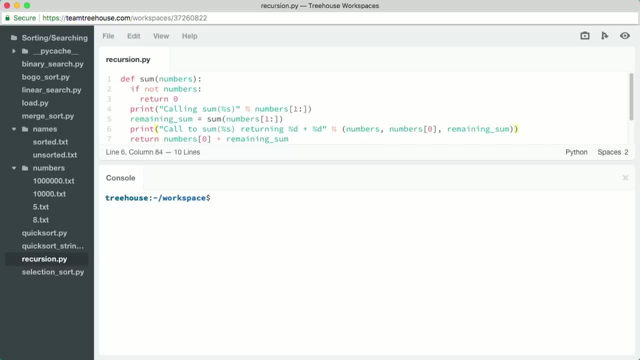 And let's try running it again. Python recursionpy. Since the print calls are inside the sum function, the first call to sum- 1279, isn't shown, only the recursive calls are. This first call to sum ignores the first item in the list, 1,. 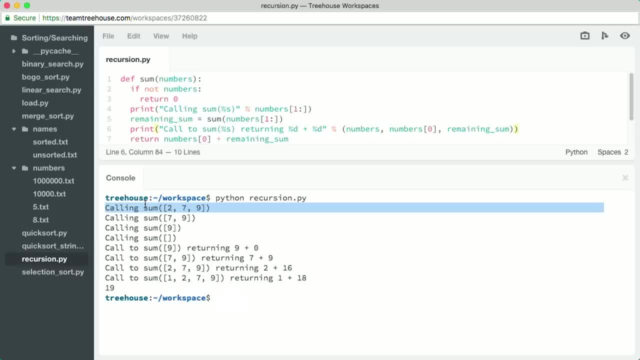 and calls itself recursively. It passes the remaining items from the list 2,, 7, and 9.. That call to sum again ignores the first item in the list it received, 2,, and again calls itself recursively. It passes the remaining items in the list 7, and 9.. 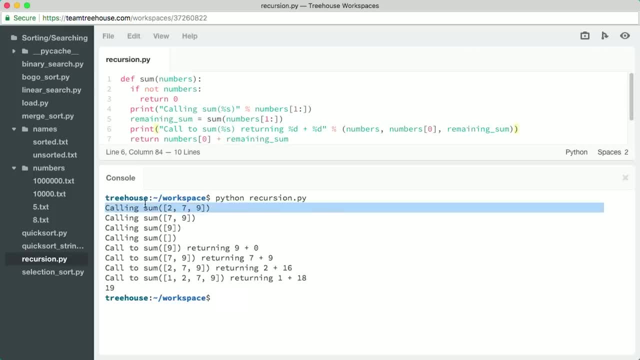 we'll have it for you in the teachers. Here's a separate hard-coded list containing the 100 names we're going to search for. We'll loop through each name in this list and pass it to our search function to get the index within the full list where it appears. 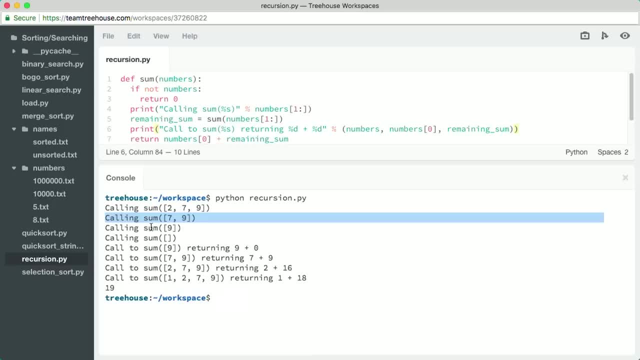 Now let's implement the search function. Compared to the sorting algorithms, this is going to be short. The indexOfItem function takes the Python list you want to search through and a single target value you want to search for. Now we need to loop over each item in the list: The range function. 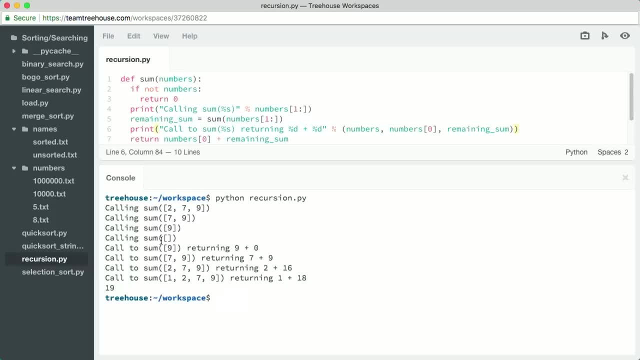 gives us a range of numbers from its first argument up to, but not including its second argument. So if our list had a length of 5, this would loop over the indexes 0 through 4.. We test whether the list item at the current index matches our target. 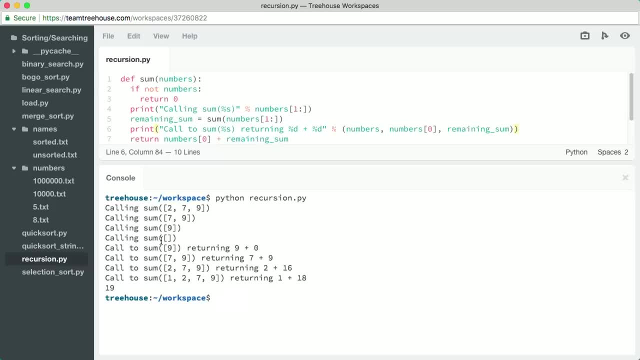 If it does, then we return the index of the current item. This will exit the indexOfItem function without looping over the remaining items in the list. If we reach the end of the loop without finding the target value, that means it wasn't in the list. So instead of 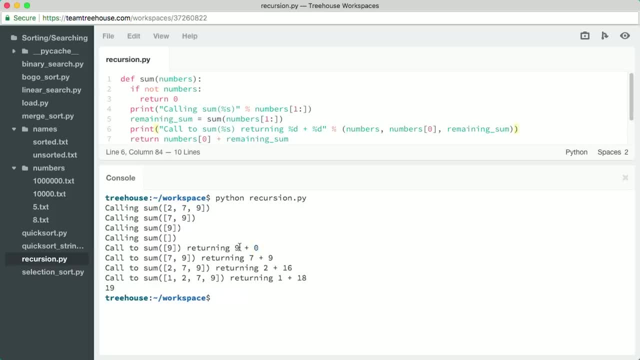 returning an index, we return the special python value, none, which indicates the absence of a value. Other languages have similar values, like nil or null, but if yours doesn't, you might have to return a value that would otherwise be impossible, like an index of negative 1.. 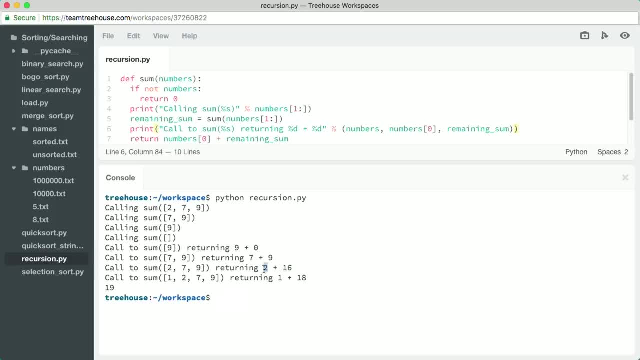 Now let's call our new search function. We start by looping over the list of 100 values we're looking for. We're using the values themselves this time, not their indexes within the list, so there's no need to mess with Python's range function. 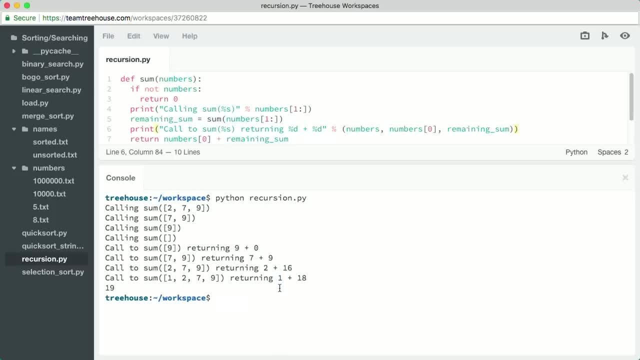 Here's the actual call to the indexOfItem function. We pass it the full list of names that we loaded from the file, plus the name we want to search for within that list. Then we store the index. it returns in a variable And, lastly, we print the index we get back from the indexOfItem function. 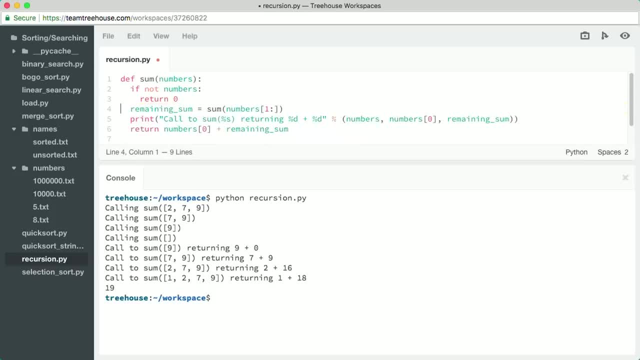 Let's save this and go to our console and see if it works. Python linearSearchpy names unsortedtxt, And it'll print out the list of indexes for each name. I actually set it up so that the last two items in the list of names we're going to. 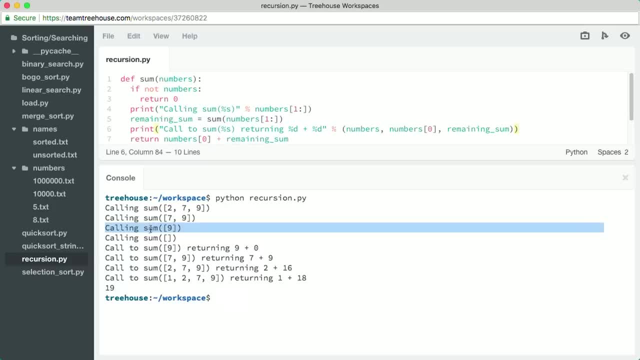 That call ignores the 7, and calls itself with a 9.. And the last call shown here ignores the 9, and calls itself with an empty list. At this point, none of our recursive calls to sum have returned yet. Each of them is waiting on the recursive call it made to sum to complete. 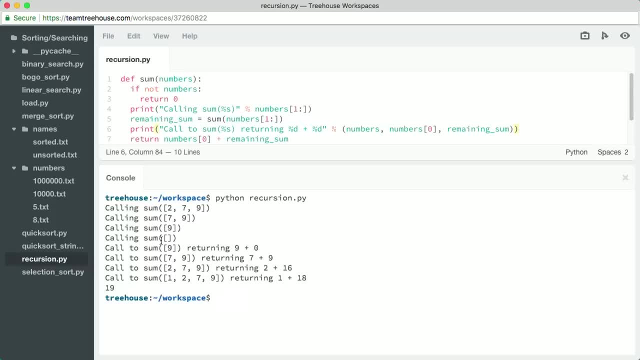 Python and other programming languages use something called a call stack to keep track of this series of functions. Python and other programming languages use something called a call stack to keep track of this series of functions. Python and other programming languages use something called a call stack to keep track of this series of functions. 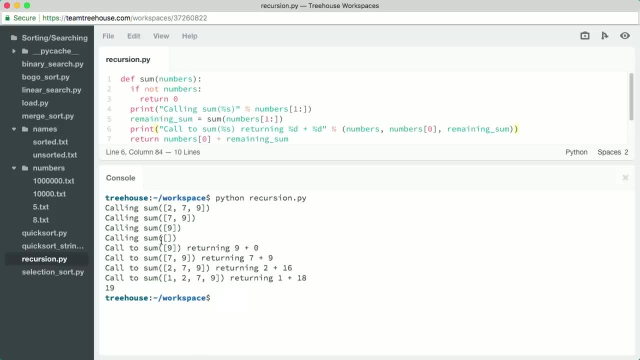 Each function call is added to the stack along with a place in the code that it needs to return when it completes. But now the empty list triggers the base case, causing the recursion to end and the sum function to return 0.. That 0 value is returned to its caller. The caller adds the 0 to the first and. 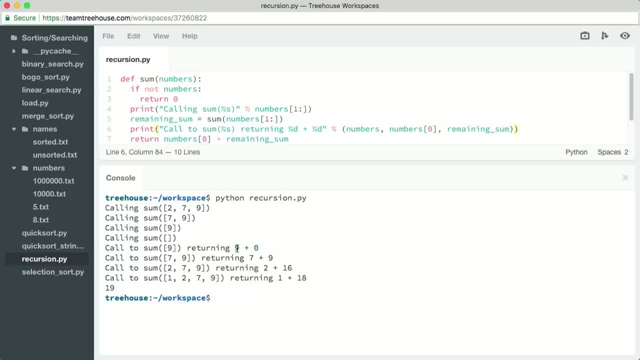 only value in its list 9.. The result is 9.. That 9 value gets returned to the caller, which adds it to the first value in the list it received, 7.. The result is 16.. That 16 value is returned to the caller. 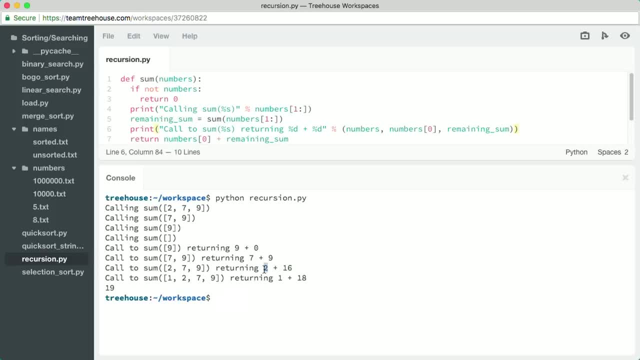 which adds it to the first value in the list it received, 2.. The result is 18.. That 18 value is returned to the caller, which adds it to the first value in the list it received, 1.. The result is 19.. That 19 value is returned to the caller, which is not the sum function. 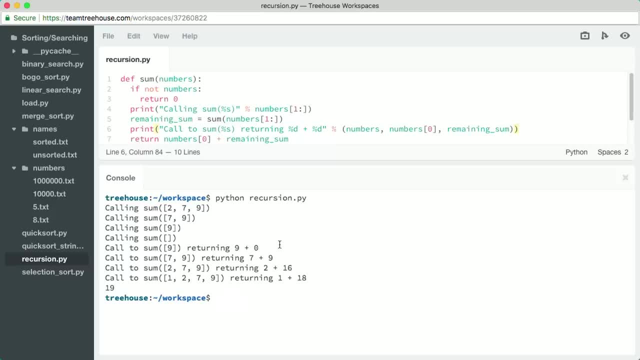 recursively calling itself but our main program. This is our final result which gets printed. It's the same result we got from the loop-based version of our program: The end. We don't want the print statements in our final version of the program. 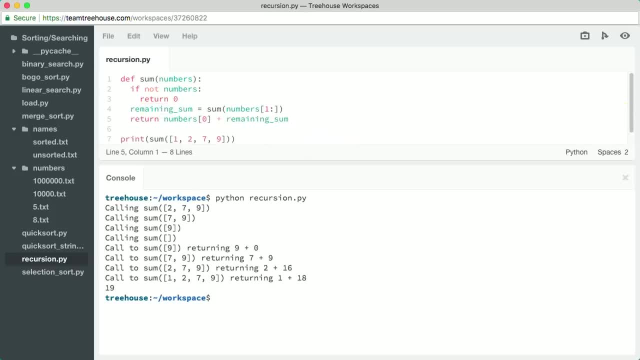 so let me just delete those real quick. And there you have it: a very simple recursive function. Well, the function is simple, but, as you can see, the flow of control is very complex. Don't worry if you didn't understand every detail here, because we won't be using this particular example again. 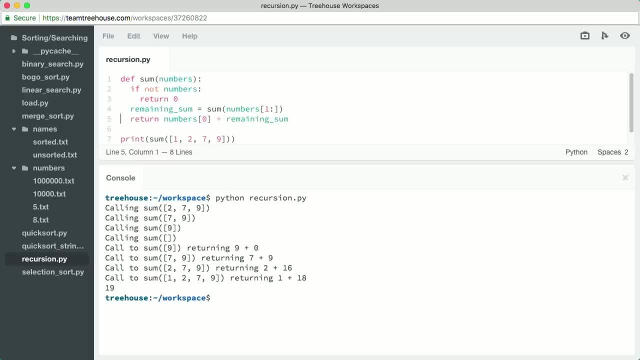 There are two fundamental mechanisms you need to remember: A recursive function needs a recursive case that causes it to call itself, and it also needs to eventually reach a base case that causes the recursion to stop. You've seen bogosort, which doesn't. 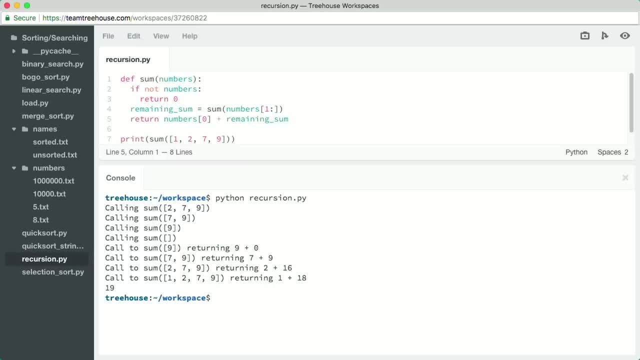 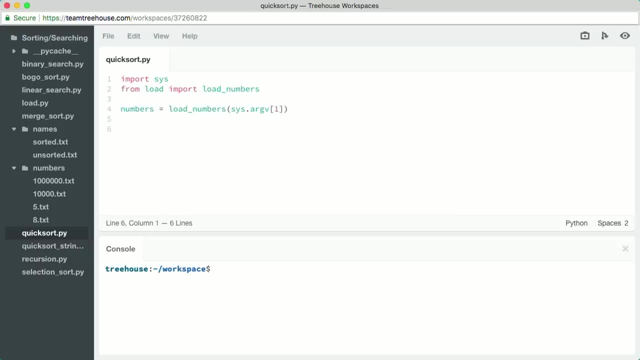 search for corresponded to the first and last name within the file. So if we open up our unsortedtxt file, we'll see Mary Rosenberger is the first name and Alonso Viviano is the last name. And those are the last two values in our list of names we're searching for. 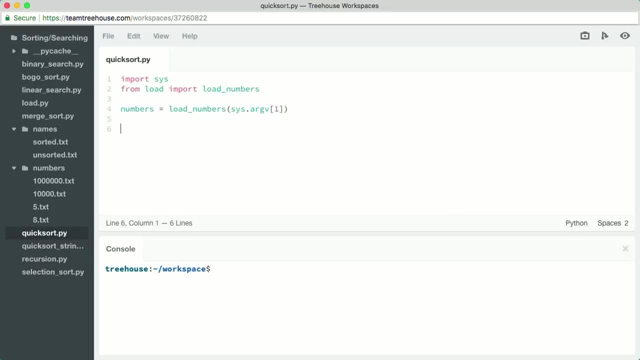 So it returned an index of zero for that second-to-last name, And you can see that name here on line 1 of the file. The line numbering starts at 1, and the Python list indexes start at 0. So that makes sense. 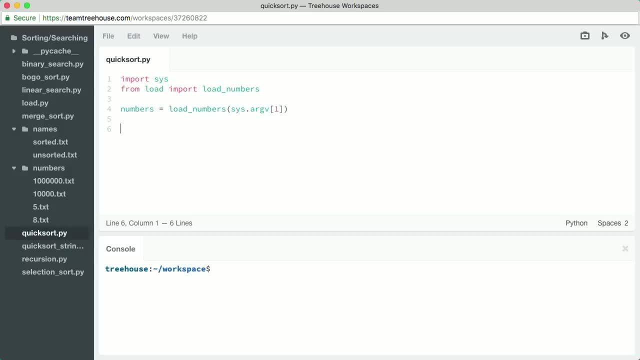 And for the last name it returned an index of 109873.. And you can see that name here on line 109874.. So we can see that it's returning the correct indexes, But right now we're just searching for 100 different names in a list of 100,000 names. 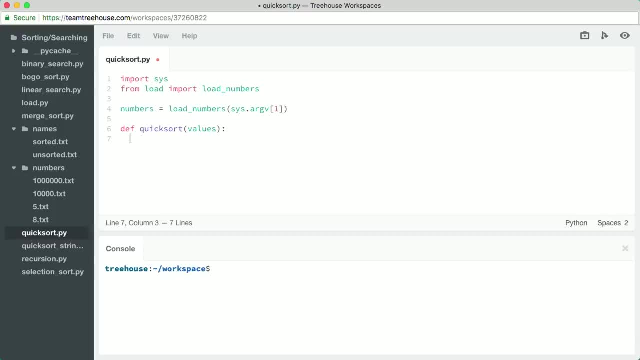 In the real world. we're going to be looking for many more names, And we'll be looking for many more names than that within much bigger lists than that. Can we do this any faster? Yes, but we'll need to use the binary search algorithm. 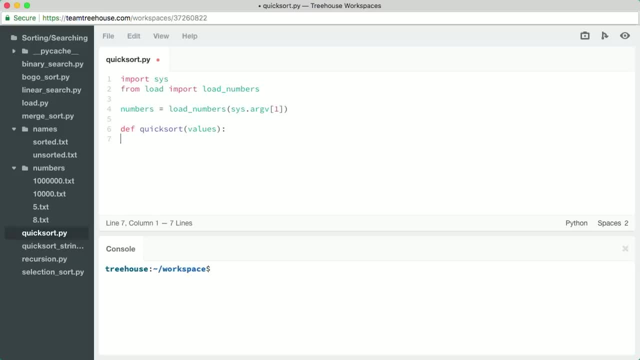 And for that to work we need to sort our list of strings. We'll do that in the next video. Before we can use the binary search algorithm on our list of names, we need to sort it. Let's do that now. We need to load our unsorted list of names from a file sorted and write the sorted. 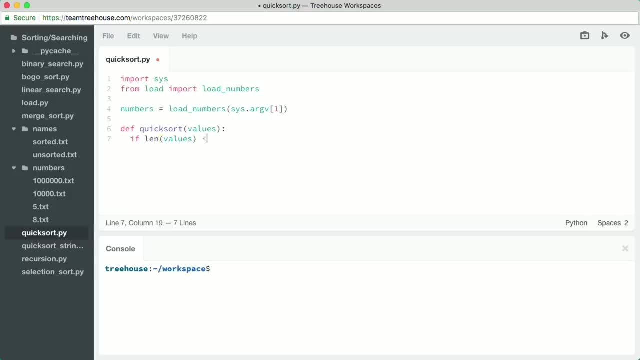 names back out to a new file Again. this code at the top just loads a file full of strings into a new file, And that's what we're going to do here. Let's do that now. We'll use our quicksort method to sort the list of names. 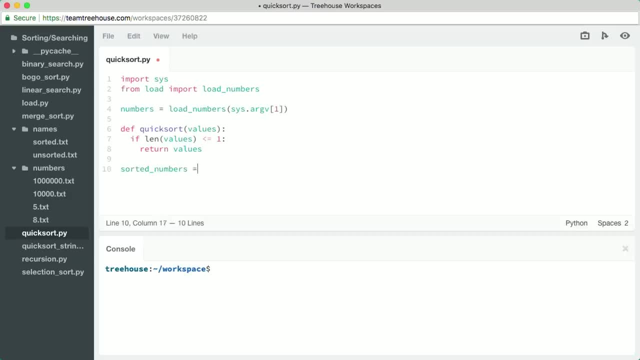 Its code is completely unchanged from when you saw it in the previous stage. We just call our quicksort function on the list of names loaded from the file and save the list to a variable. Then we loop through each name in the sorted list and we print that name. 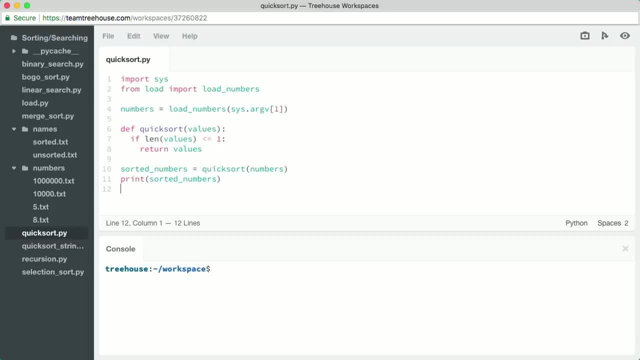 That's all there is to it. Let's save this script and try running it. Python, Quicksort, Stringspy, And we'll pass it the namesunsortedtxt file. Let me resize the console window here a little bit. That prints the sorted list of names out to the terminal, but we need it in a file. 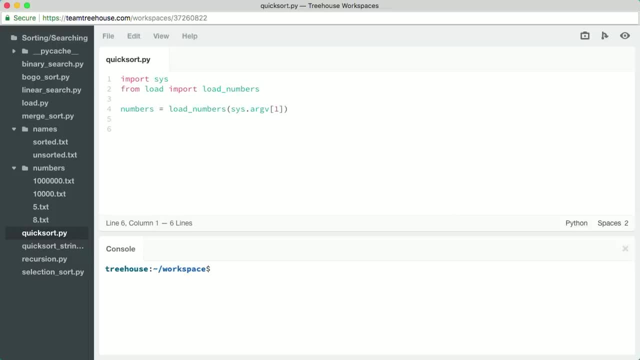 make any progress toward sorting a list with each pass. either it's entirely sorted or it isn't. You've seen selectionsort, which moves one value over to a sorted list with each pass so that it has fewer items to compare each time. Now let's look at an algorithm that speeds up the process. 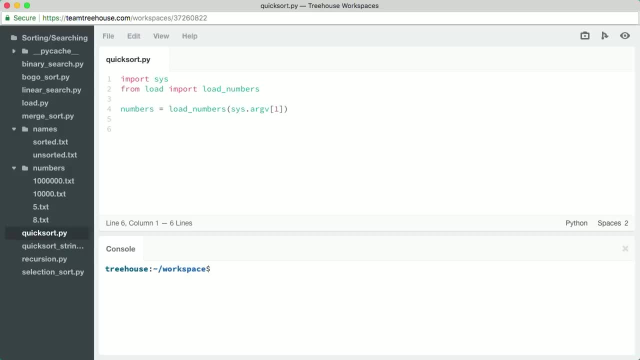 further by further reducing the number of items that are sorted with each pass. So let's look at the number of comparisons it makes. It's called Quicksort. Here's some Python code where we'll implement Quicksort Again, you. 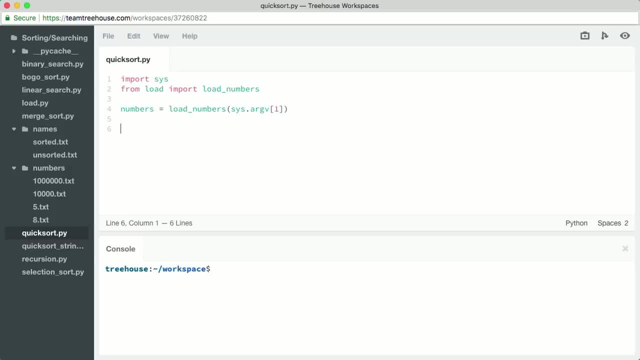 can ignore these lines at the top. We're just using them to load a file full of numbers into a list. The Quicksort algorithm relies on recursion. To implement it, we'll write a recursive function. We'll accept the list of numbers to sort as a parameter. 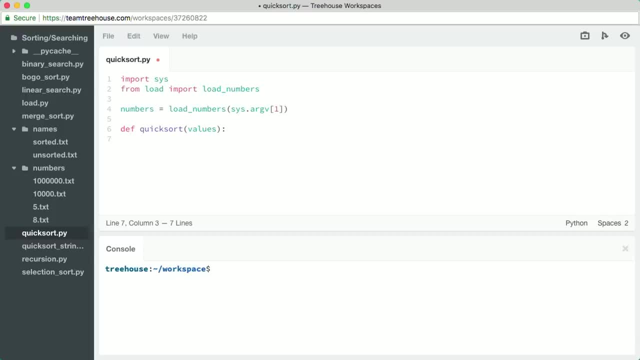 Quicksort is recursive because it keeps calling itself with smaller and smaller subsets of the list you're trying to sort. We're going to need a base case where the recursion stops so it doesn't enter an infinite loop. Lists that are empty don't need to be sorted. 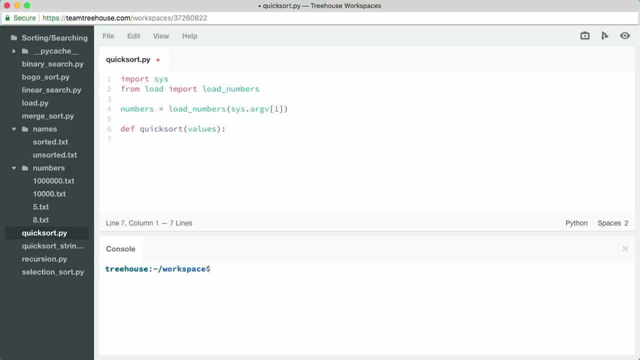 and lists with just one element don't need to be sorted either. In both cases there's nothing to flip around, so we'll make that our base case. If there are zero or one elements in the list passed to the Quicksort function. 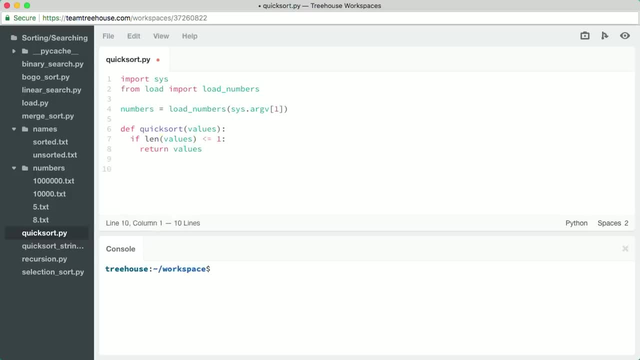 we'll return the unaltered list to the caller. Lastly, we need to call our Quicksort function with our list of numbers and print the list as it returns. That takes care of our base case. Now we need a recursive case. We're going to 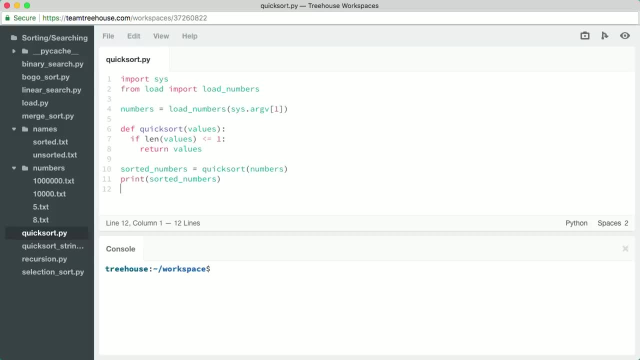 rely on a technique that's common in algorithm design called divide and conquer. Basically, we're going to take our problem and split it into smaller and smaller problems until they're easy to solve. In this case, that means taking our list and splitting. 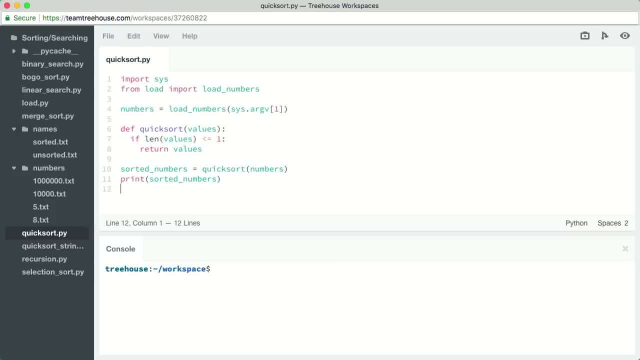 it into smaller lists. Viewers. a suggestion: The process I'm about to describe is complex. There's just no way around it. If you're having trouble following along, remember the video playback controls. Feel free to slow the playback down. 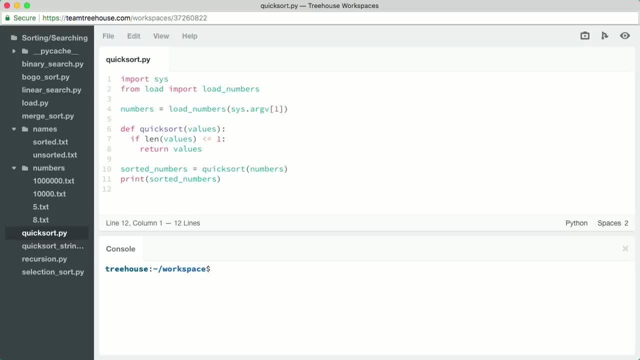 rewind or pause the video as needed. After you watch this the first time, you may also find it helpful to rewind and make your own diagram of the process as we go. Okay, ready, Here goes. Suppose we load the numbers from our eattxt file into: 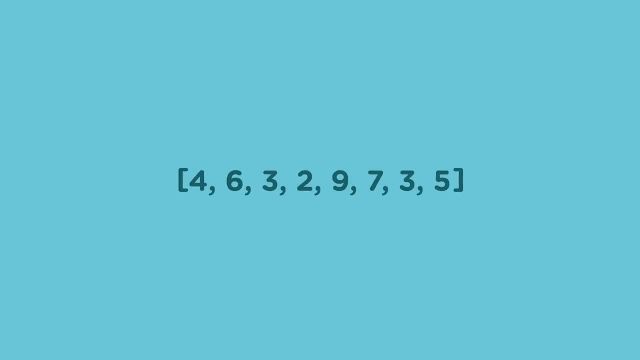 a list. How do we divide it? It would probably be smart to have our Quicksort function divide the list in a way that brings it closer to being sorted. Let's pick an item from the list. We'll just pick the first item for now 4.. 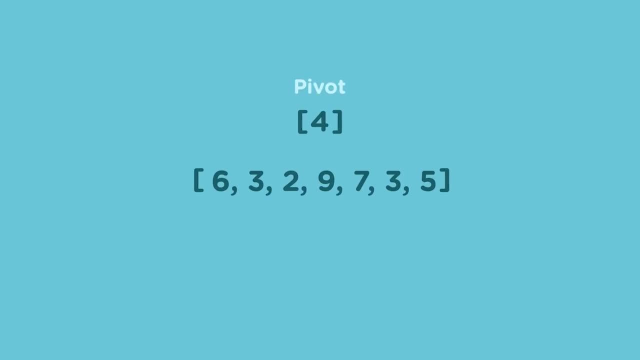 We'll call this value. we've picked the pivot like the center of a seesaw on a playground. We'll break the list into two sublists. The first sublist will contain all the items in the original list that are smaller than the pivot. 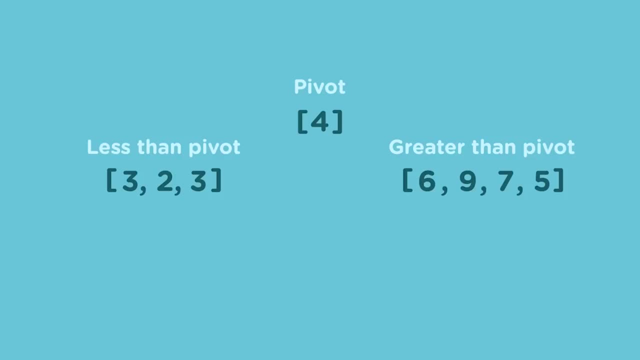 The second sublist will contain all the items in the original list that are greater than the pivot. The sublists of values less than and greater than the pivot aren't sorted, But what if they were? You could just join the sublists and the pivot all. 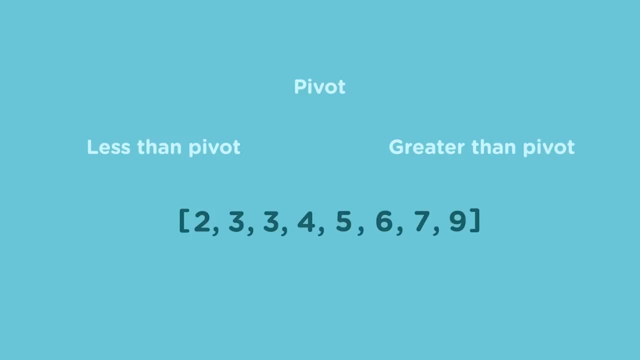 together into one list and the whole thing would be sorted. So how do we sort the sublist? We call our Quicksort function recursively on them. This may seem like magic, but it's not. It's the divide and conquer algorithm design technique at work. 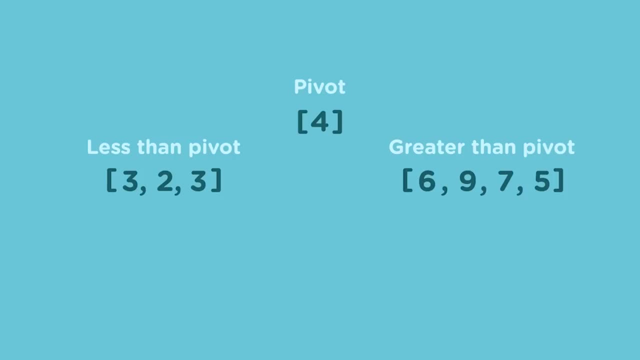 If our Quicksort function works on the big list, then it will work on the smaller list too. For our first sublist we take the first item as the pivot again, That's 3.. We break the sublist into two sublists. 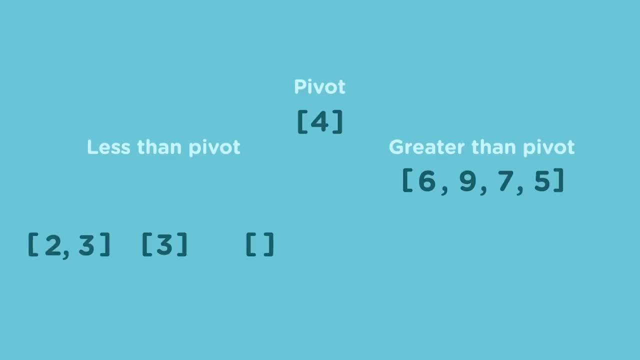 one with everything less than the pivot and one with everything greater than the pivot. Notice that there's a value equal to the pivot that gets put into the less than sublist. Our finished Quicksort function is actually going to put everything that's less than or equal. 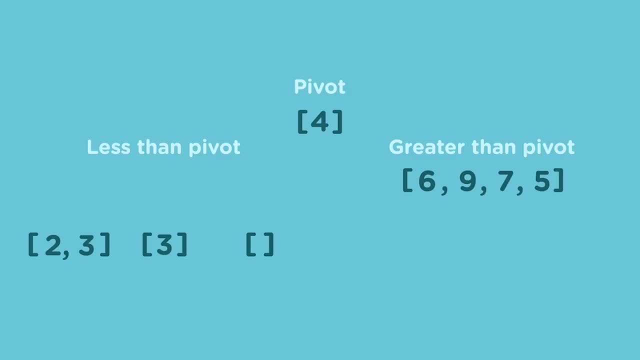 to the pivot in the first sublist, But I don't want to say less than or equal to over and over, so I'm just referring to it as the less than pivot sublist. Also, notice that there are no values greater than the pivot. That's okay When we do. 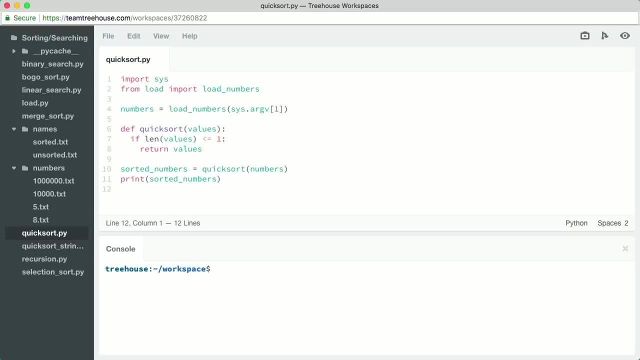 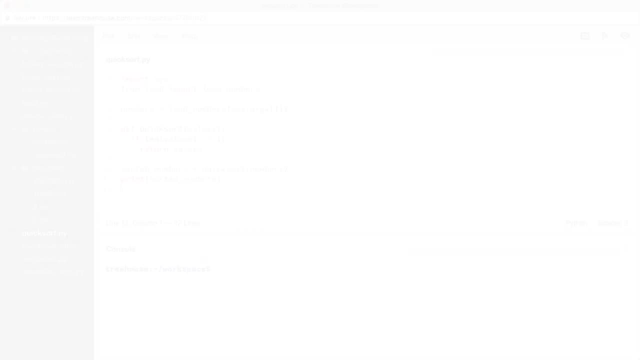 So we'll do what's called a redirect of the program's output. We'll run the same command as before, but at the end we'll put a great event sign, followed by the path to a file that we want the program output written to. 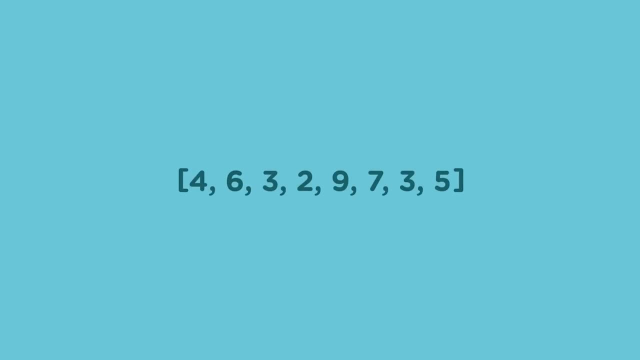 namessortedtxt. Redirecting works not only on Linux-based systems like workspaces, but also on Macs and even on Windows machines. You just need to be careful, because if you redirect to an existing file, its contents will be overwritten without asking you. 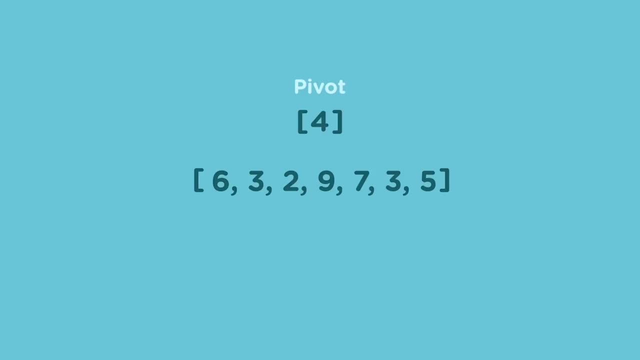 Let me refresh the list of files in the sidebar And you'll see that we now have a new sortedtxt file in the names directory. It's the same number of lines as the unsortedtxt file, but all the names are sorted now. 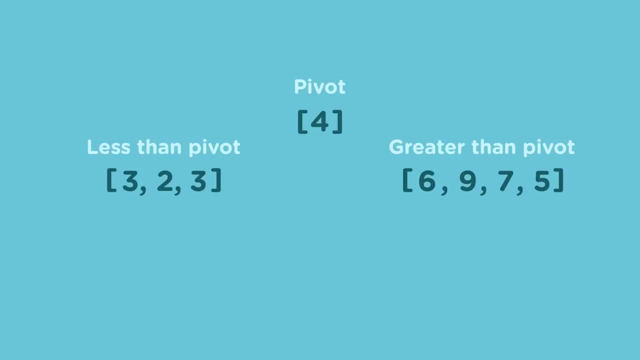 Now we can load this file of sorted names into a list and we'll be able to use that list with the binary search algorithm. We'll see how to do that next, Now that we have our list of names sorted, we can use the binary search algorithm on. 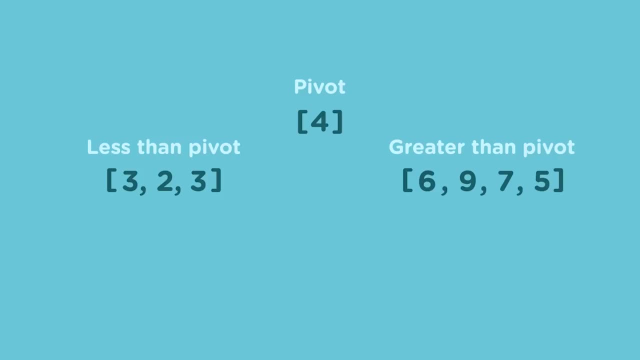 it. Let's see if we can use it to speed up our search for the indexes of 100 names. Binary search keeps narrowing down the list until it has the value it's looking for. It's faster than linear search because it discards half the potential matches each time. 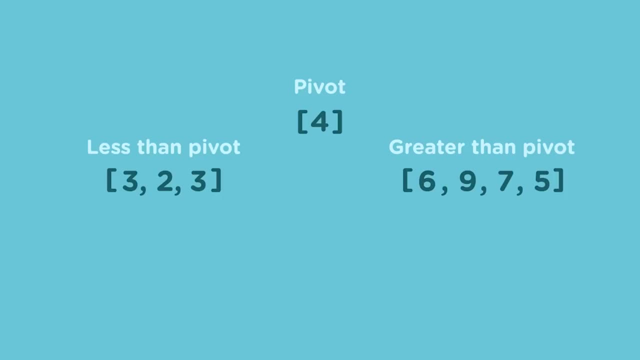 Our code here at the top of our binary search script is unchanged from the previous scripts. We just called the loadStrings function to load our 100,000 sorted names from a file. Here we've hardcoded the list of 100 names we're going to search for again. 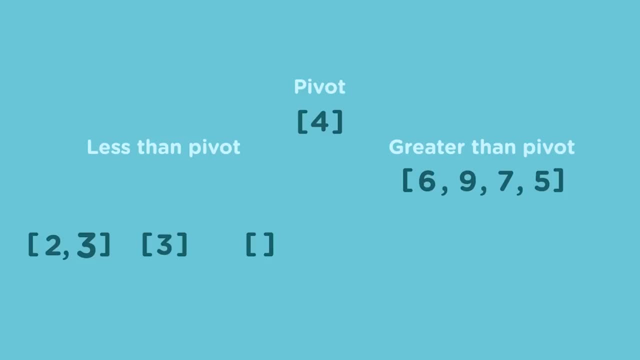 It's identical to the list from the linear search script, except that I've again changed the last two names to correspond to the names on the first and last lines of the file we'll be loading. Now let's write the function that we'll implement on the first and last lines of the file we'll 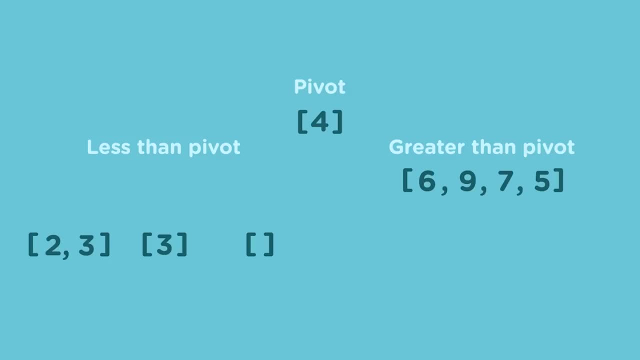 be loading. It's called our binary search algorithm, Like the linear search function. before. it'll take two arguments. The first is the list we're going to search through and the second is the target value we'll be searching for. Again, the binary search function will return the index it found the value at or the special. 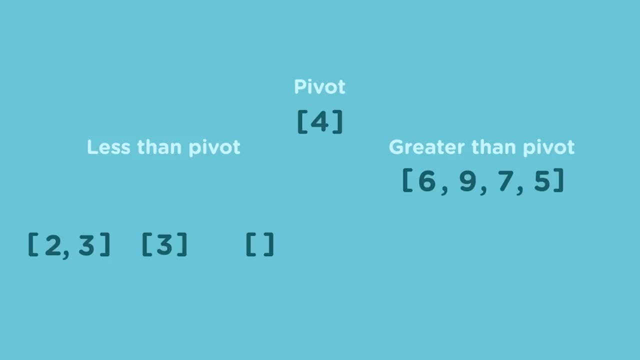 value none if it wasn't found. Binary search is faster than linear search because it discards half the values it has to search through each time. To do this, it needs to keep track of a range that it still needs to search through. To start, that range is going to include the full list. 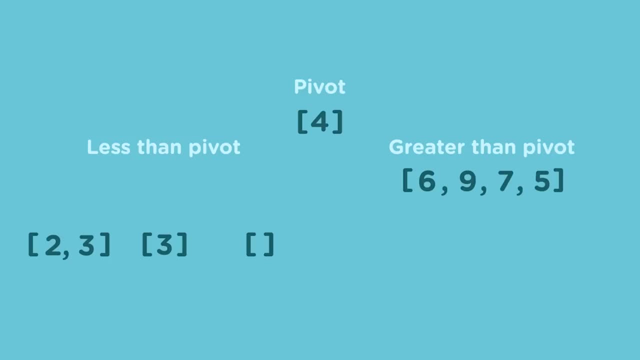 join the sublists back together, that just means nothing will be in the return list after the pivot. We still have one sublist that's more than one element long, so we call our Quicksort function on that too, You and I can. 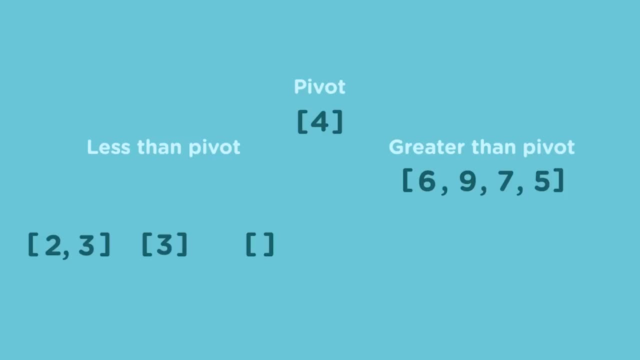 see that it's already sorted, but the computer doesn't know that, so it'll call it anyway, just in case It picks the first element 2, as a pivot. There are no elements less than the pivot and only one element greater than the pivot. 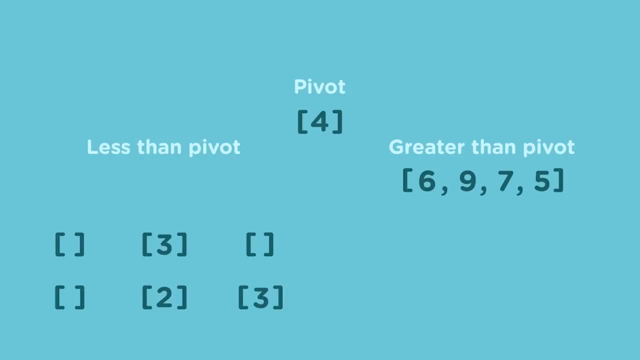 That's it for the recursive case. We've finally hit the base case for our Quicksort function. It'll be called on both the empty list of elements less than the pivot and the one-item list of elements greater than the pivot, But both of these lists will be. 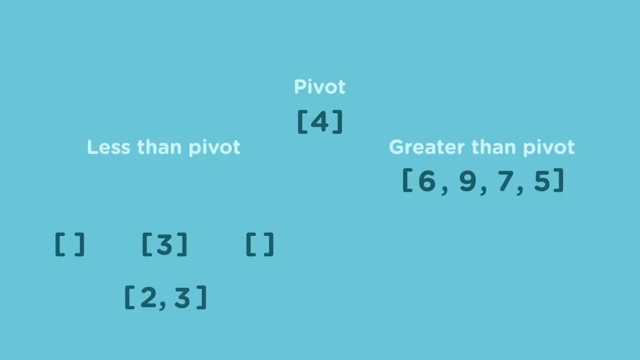 returned as they are because there's nothing to sort. So now, at the level of the call stack, above this, the returned sorted lists are used in place of the unsorted sublist. that's less than the pivot and the unsorted sublist, that's. 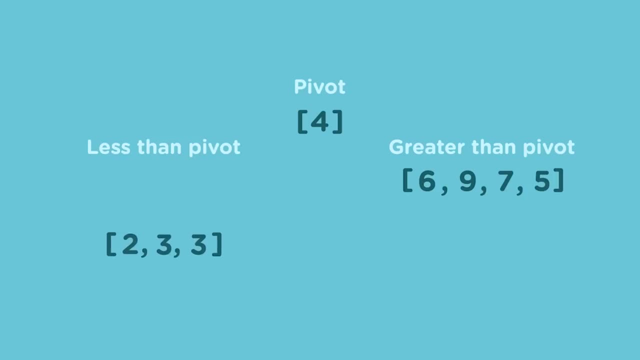 greater than the pivot, These are joined together into one sorted list. Remember that any empty lists get discarded Then, at the level of the call stack above that, the returned sorted lists are used in place of the unsorted sublists. there Again, they were already sorted, but the 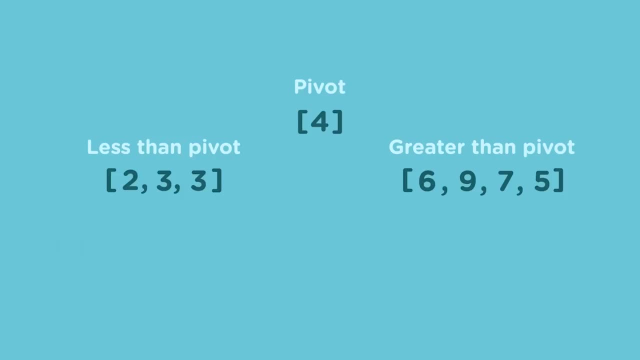 Quicksort method was called on them anyway, just in case The sublists are joined together into one sorted list At the level of the call stack. above that, the returned sorted list is used in place of the unsorted sublist. that's less than the pivot. 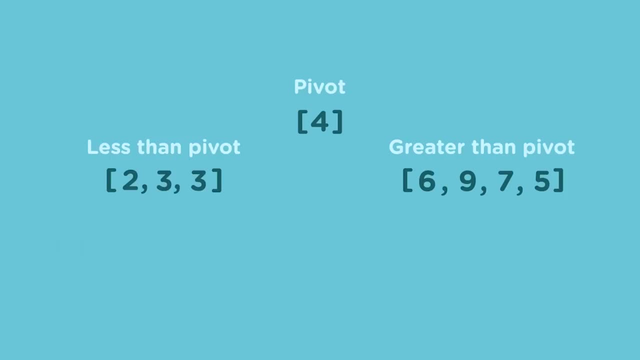 So now everything that's less than or equal to the pivot is sorted. Now we call Quicksort on the unsorted sublist that's greater than the pivot and the process repeats for that sublist We pick the first element, 6, as the pivot We split the. 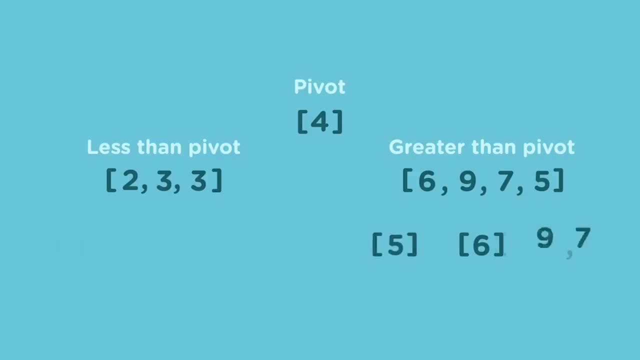 sublist into sublists of elements that are less than and greater than this pivot And we recursively call the Quicksort function until those sublists are sorted. Eventually a sorted sublist is returned to our first Quicksort function call. We combine the sublist that's less than or equal. 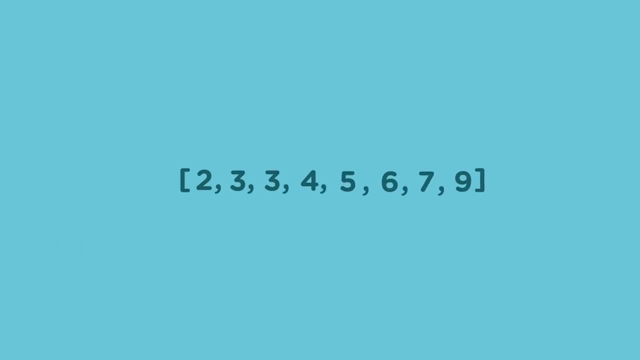 to the pivot, the pivot itself and the sublist that's greater than the pivot into a single list, And because we recursively sorted the sublists, the whole list is sorted. So that's how the Quicksort function is going to work In the next video. 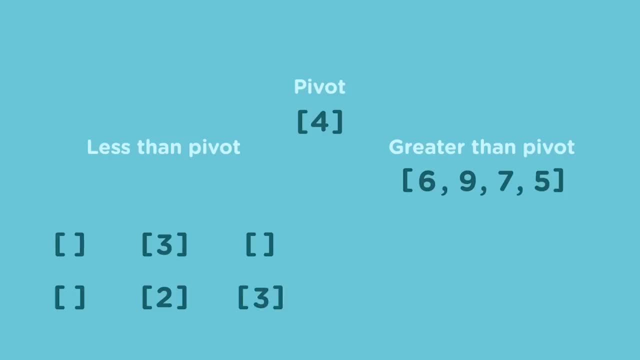 The first variable will track the lowest index in the range we're searching To start. it's going to be zero, the first index in the full list. Likewise, the last variable will track the highest index in the range we're searching To start. we'll set it to the highest index in the full list. 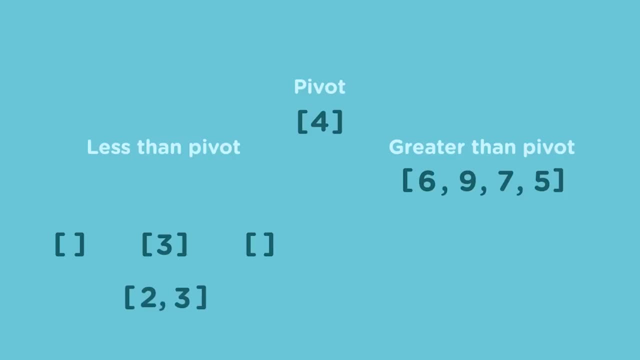 If the first and last variables are equal, then it means the size of the search range has shrunk to zero and there is no match. Until that happens, though, we'll keep looping to continue the search. We want to divide the list of potential matches in half each time. 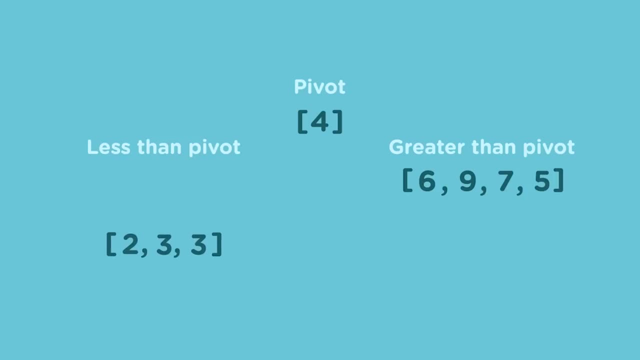 To do that we need to check the value that's in the middle of the range we're searching in. We add the indexes in the first and last variables, then divide by two to get their average. We might get a fractional number which can't be used as a list index. so we also round. 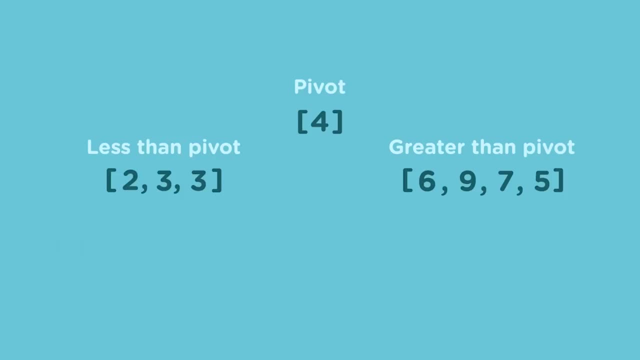 down using Python's double-slash-floor-division operator. All this will give us the index of the list element. that's the midpoint of the range we're searching. Now we test whether the list element at the midpoint matches the target value. If it does, we return the midpoint index without looping any further. 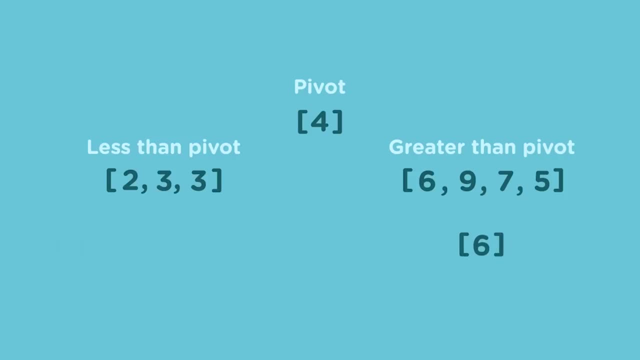 Our search is complete. Otherwise, if the midpoint element's value is less than the target value, then we know that our target value is less than the target value of the target value of the list element. That's it. Thanks for watching. Our target value can't be at the midpoint or any index prior to that, so we move the. 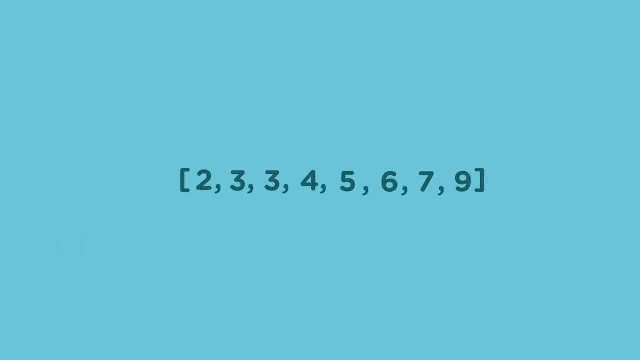 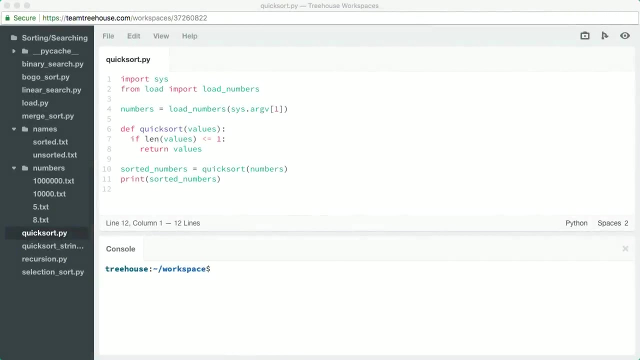 new start of our search range to just after the old midpoint. Otherwise the midpoint element's value must have been greater than the target value. We know that our target value can't be at the midpoint or any index after that, so we move the new end of our search range to just before the old midpoint. 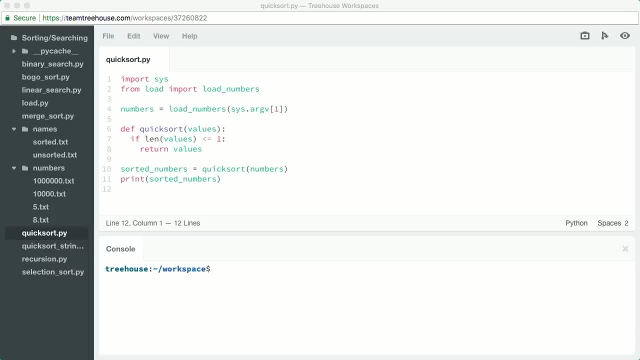 By unindenting here we mark the end of the loop. If the loop completes, it means the search range shrank to nothing without our finding a match. That means there's no matching value in the list, So we return the special Python value NONE to indicate this. 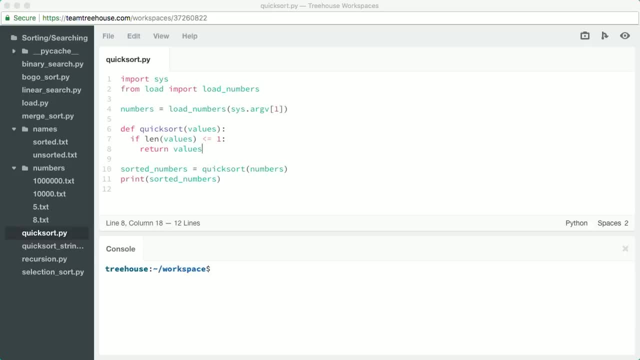 Lastly, just as we did in our linear search script, we need to search for each of the 100 names. We loop over each name in our hardcoded list And we call the binary search function with the sorted list of names we're going to. 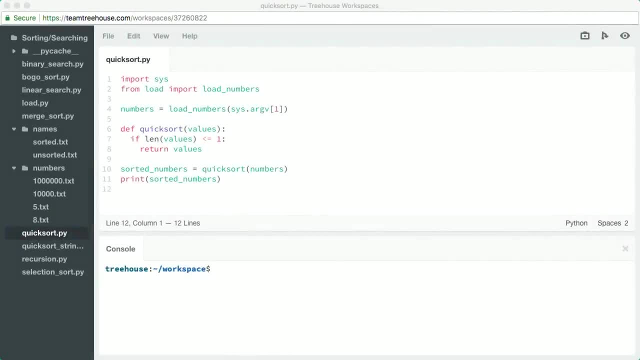 we'll show you the actual code. Quicksort works by picking a pivot value, then splitting the full list into two sublists. The first sublist has all the values less than or equal to the pivot, and the second sublist has all the values greater than the pivot. 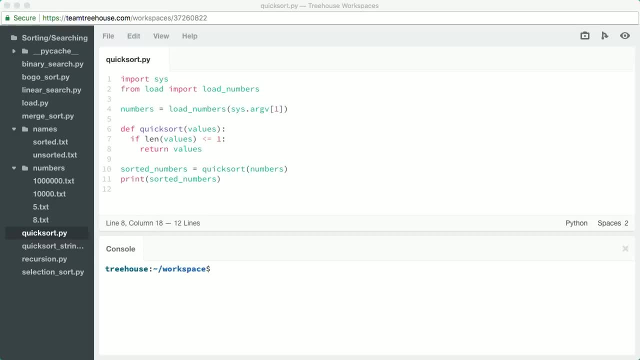 The Quicksort function recursively calls itself to sort these sublists and then to sort the sublists of those sublists until the full list is sorted. Now it's time to actually implement this in code. We already have the base case written: Any list passed. 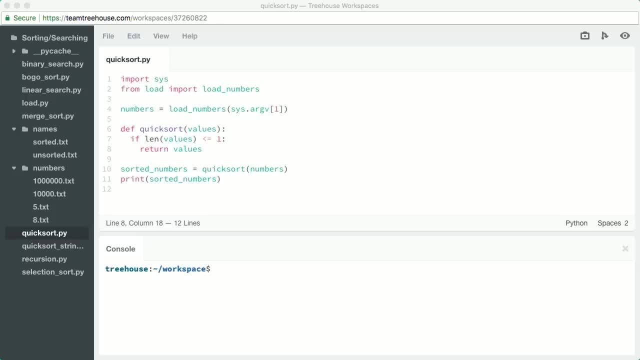 in that consists of 0 or 1, values will be returned as is, because there's nothing to sort. Now we need to create a list that will hold all the values less than the pivot. That list will be empty at first. We do the same for values greater than. 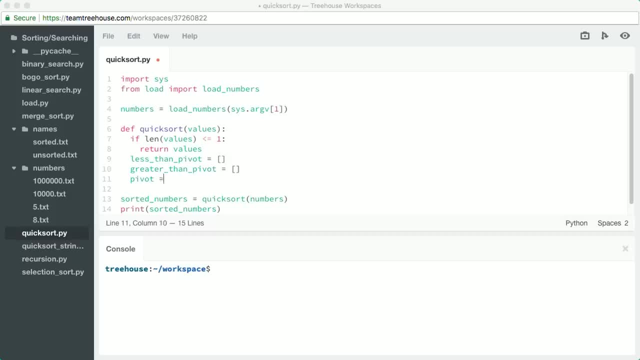 the pivot. Next we need to choose the pivot value. For now we just grab the first item from the list. Then we loop through all the items in the list. following the pivot We check to see whether the current value is less than or equal to the pivot. 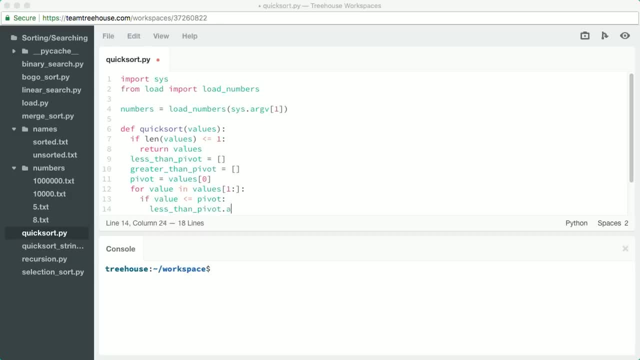 If it is, we copy it to the sublist of values less than the pivot. Otherwise, the current value must be greater than the pivot, so we copy it to the other list. This last line is where the recursive magic happens. We call Quicksort. 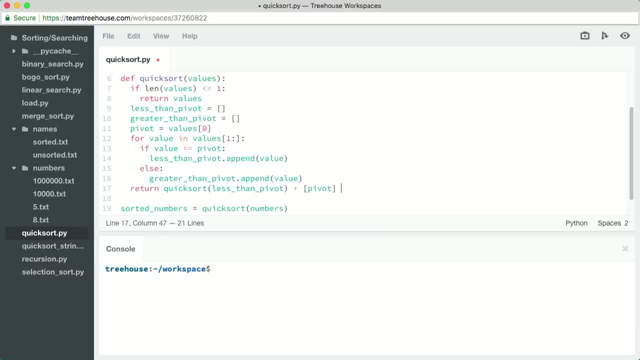 recursively on the sublist that's less than the pivot. We do the same for the sublist that's greater than the pivot. Those two calls will return sorted lists. so we combine the sorted values less than the pivot, the pivot itself and the sorted values. 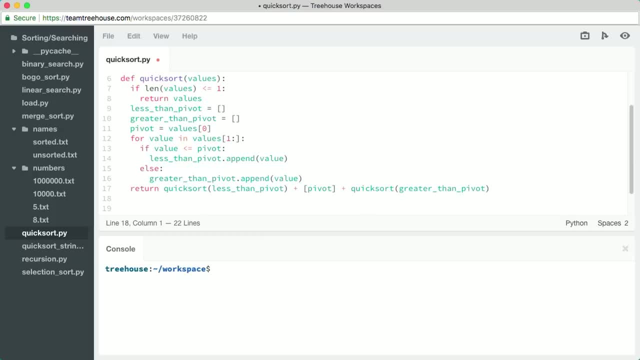 greater than the pivot. That gives us a complete sorted list which we return. This took a lot of prep work. Are you ready? Let's try running it Python quicksortpy- numbers8.text. It outputs our sorted list. I don't know. 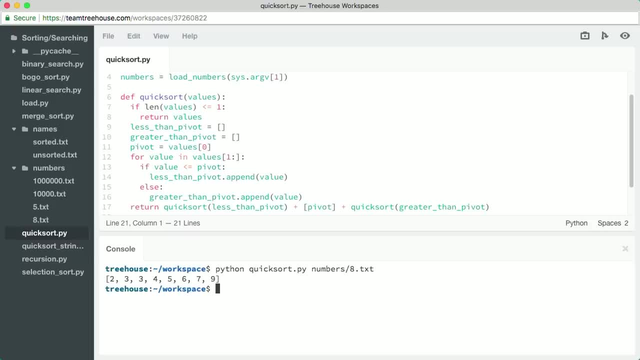 about you, but this whole thing still seems a little too magical to me. Let's add a couple print statements to the program so we can see what it's doing. First, we'll add a print statement right before the first call to the quicksort function. 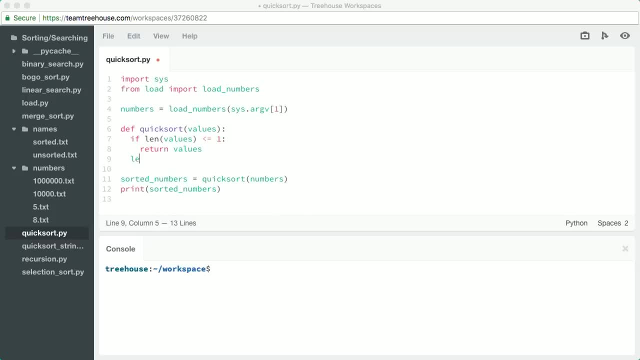 load from the file and the current name we're searching for, We store the returned list index in the index variable And finally we print that variable. Let's save this and go to our console and try running it. Python: binarysearchpy. 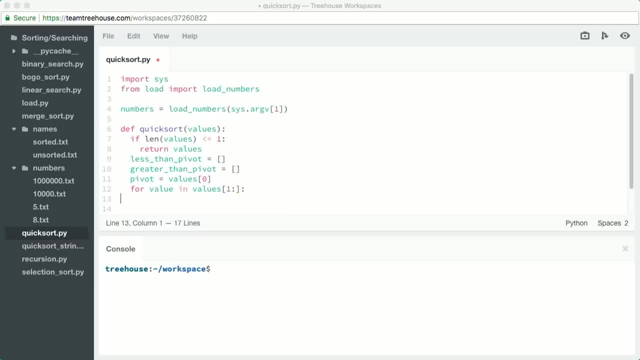 And it's important to give it the name of the sorted file. If it loads the unsorted file, the binary search won't work. So names sortedtxt. Again it prints out the list of indexes for each name. I once again set it up. so the last two items in the list of names we're going to search. 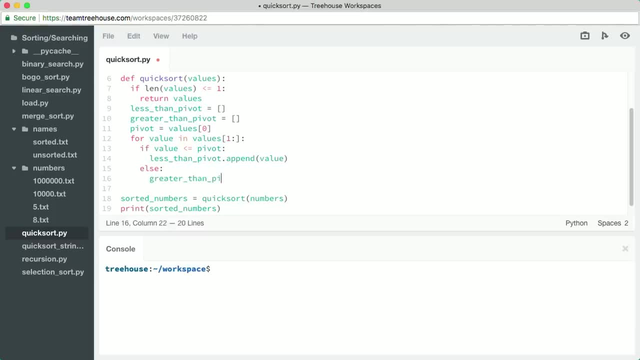 for corresponded to the first and last name in the file And we're good to go. So it returned an index of 0 for the second-to-last name And you can see that name. Here's the second-to-last name: Erin Augustine. 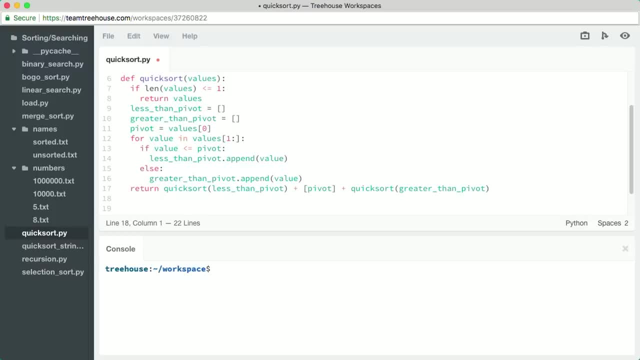 You can see that name here on line 1 of the file. And for the last name it returned an index of 109873.. And you can see that name here on line 109874.. Let's check the third-to-last name for good measure. 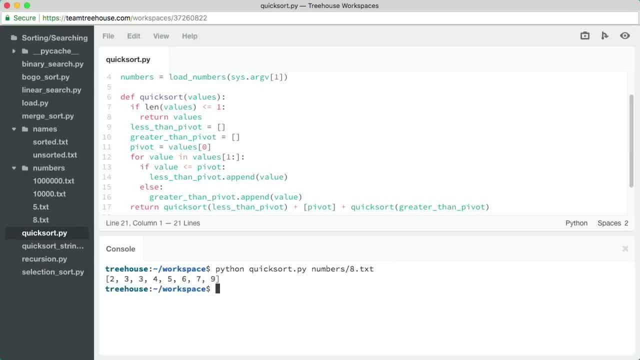 It looks like an index of 97022 was printed for that name, Stephen Derriss. Let's search for Stephen Derriss within the file, And here it is, on line 97023.. Remember that line numbers start on 1 instead of 0, so this actually matches up with the. 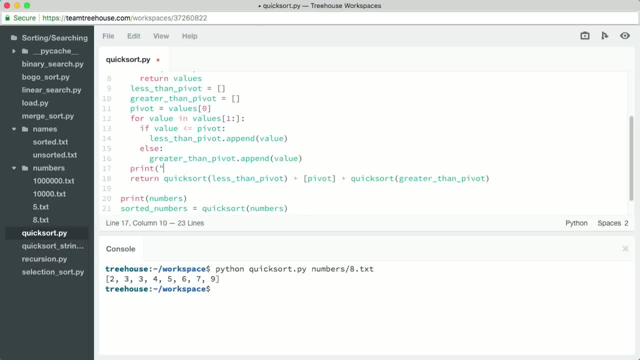 printed list index of 97023.. And here it is, on line 97023.. Remember that line numbers start on 1 instead of 0, so this actually matches up with the printed list index of 97023.. And here it is, on line 97023.. 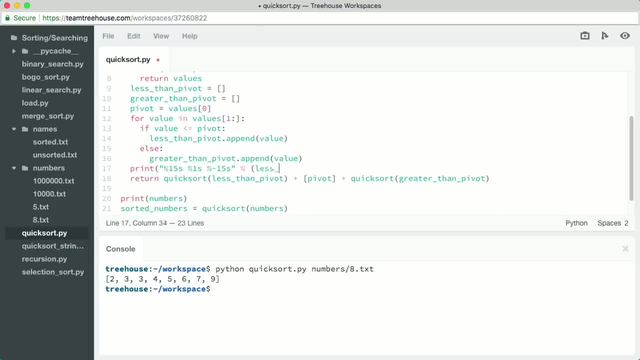 It looks like our binary search script is working correctly. Let's try our linear search and binary search scripts out with the time command and see how they compare. I've commented out the lines that print the indexes of matches in the two scripts. That way they'll still call their respective search functions with the 100 names we're. 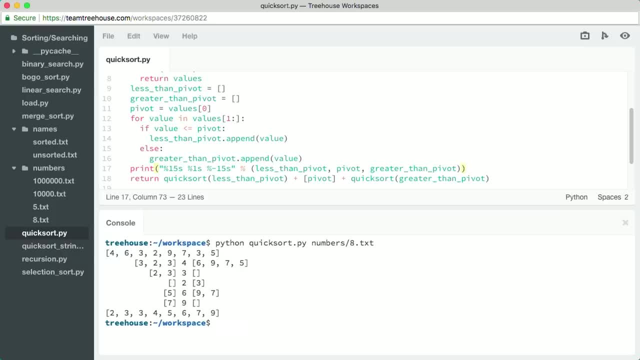 searching for, but they won't actually print the indexes out, so we won't have a bunch of output obscuring the results of the time command. First let's try the linear search Time Python, linearSearchpy names, and we can just use the unsorted list of names. 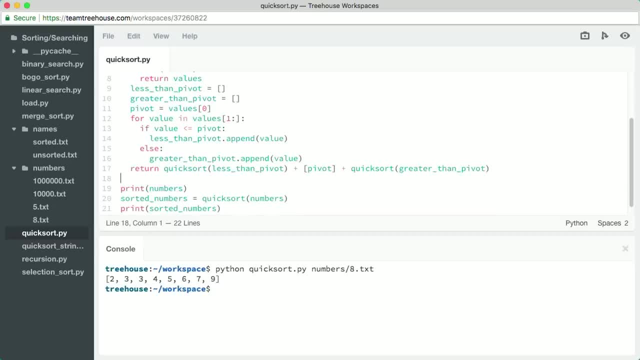 so we can see the unsorted list. We'll also add a print right within the quicksort function right before the recursive calls. Again, this string formatting code is just to keep the info aligned in columns. Let's try running this again, and now you. 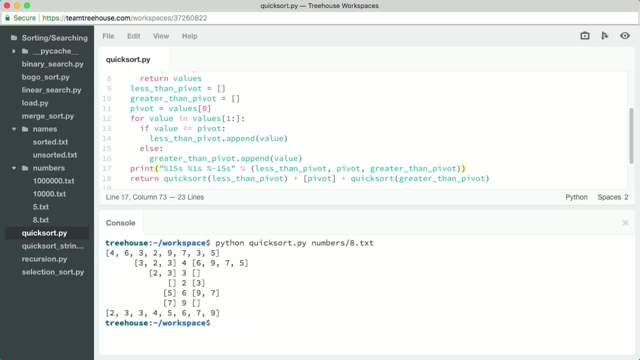 can see our new debug output. Each time quicksort goes to call itself recursively, it prints out the pivot, as well as the sublist of items less than or equal to the pivot, if any, and the sublist of items greater than the pivot, if any. You can. 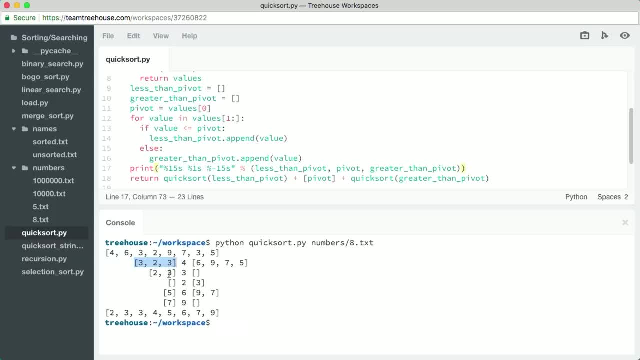 see that first it sorts the sublist of items less than the pivot at the top level. It goes through a couple levels of recursion to do that. There are actually additional levels of recursion, but they're from calls to quicksort with a list of zero or one elements. 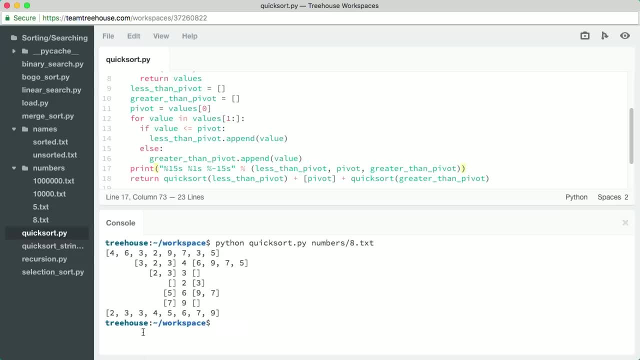 and those calls return before the print statement is reached. Then it starts sorting the second sublist from the top level with items greater than the original pivot. You can see a couple levels of recursion for that sort as well. Finally, when both sublists are recursively, 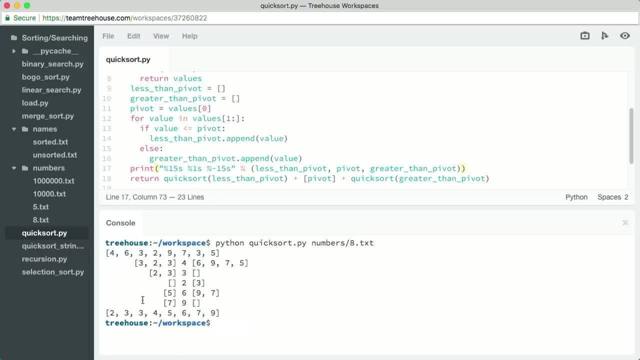 sorted. the original call to the quicksort function returns and we get the sorted list back. So we know that it works. The next question is: how well does it work? Let's go back to our file of 10,000 numbers. 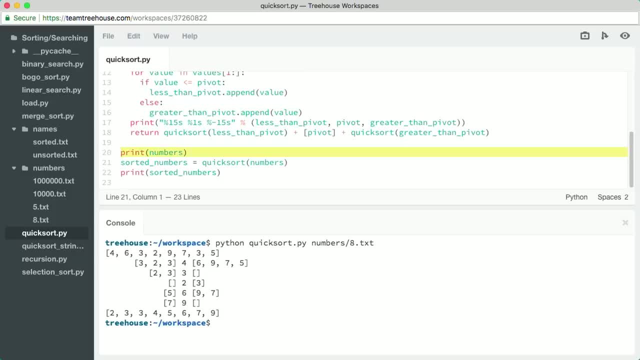 and see if it can sort those. First, though, I'm going to remove our two debug calls to print so it doesn't produce unreadable output. A quick note: if you try running this on a file with a lot of repeated values, it's possible you'll get a runtime. 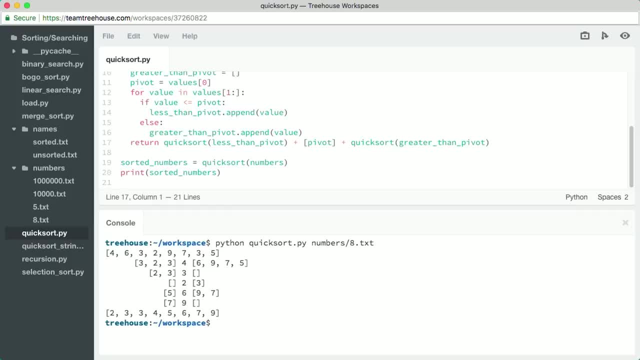 error and maximum recursion depth exceeded, If you do see the teacher's notes for a possible solution. Now let's try running our quicksort program against a 10,000 dot text file Python. quicksort dot pi numbers: 10,000 dot text. 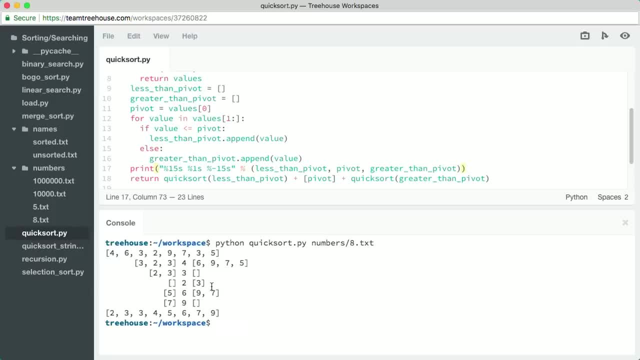 for linear search. Remember we want to ignore the real result and add the user and sys results together. It looks like it took about .9 seconds for linear search to find the 100 names in a list of 100,000.. Now let's try timing the binary search script. 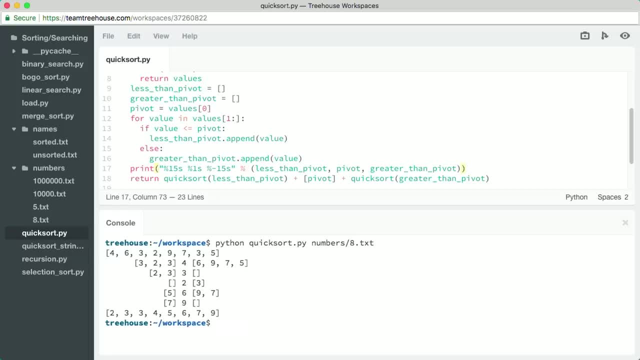 Time Python binarySearchpy names, and for this one we need to use the sorted list of names. Looks like that took around a quarter second, so less than half as long. Bear in mind that part of this time is spent loading the file of names into a list. 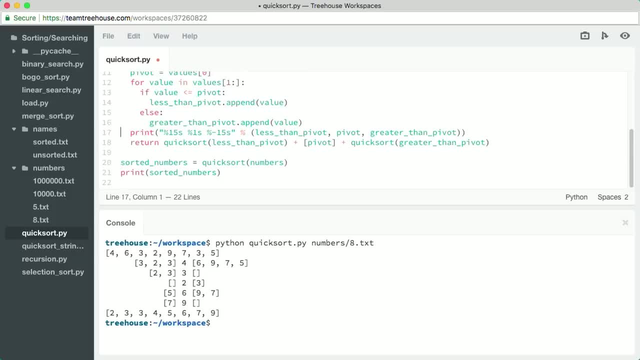 The difference between linear search and binary search will be even more pronounced as you search through bigger lists or search for more items. Let's wrap up the course by looking at the Big O runtimes for linear search and binary search. These are going to be much simpler to calculate than the sorting algorithms were. 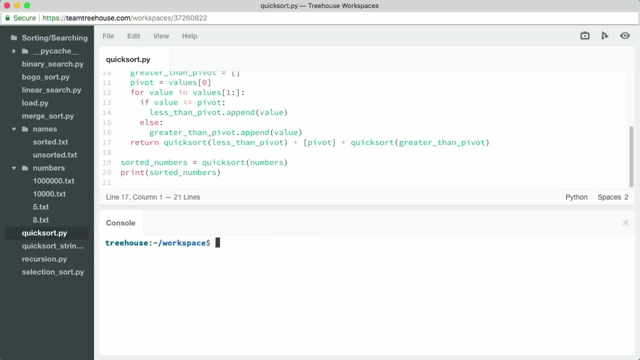 For linear search you need to do one comparison to the target value for each item in the list. Again, theoretically we could find the target value before searching the whole list. but Big O notation is only concerned with the worst case, where we have to search the entire. 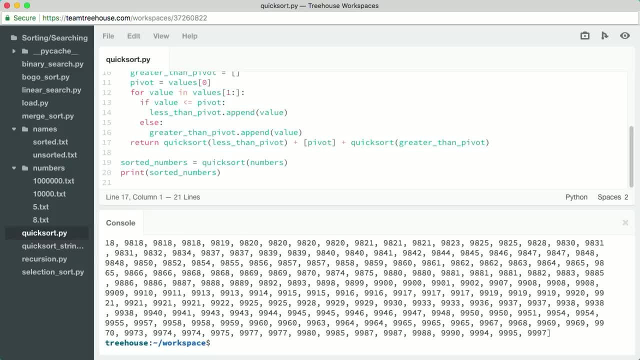 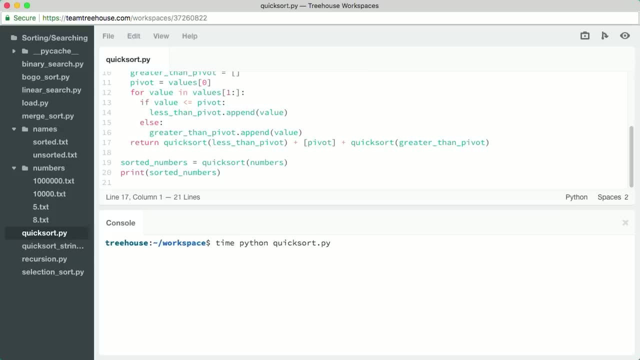 list. So for a list of 8 items that means 8 operations. The Big O runtime for linear search is O, where N is the number of items we're searching. This is also known as linear time, because when the number of items and number of operations 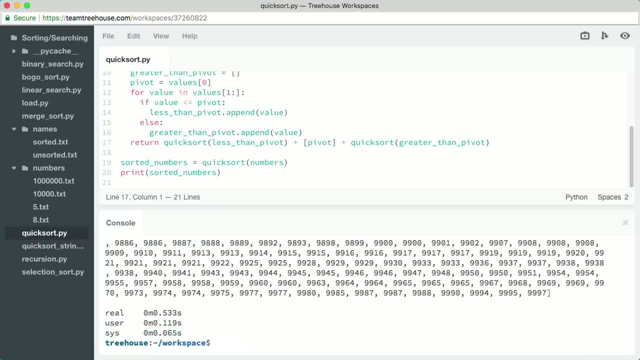 are compared on a graph, the result is a straight line. Linear search looks pretty good until you compare it to binary search. For binary search, the number of items you have to search through, and therefore the number of operations, is cut in half with each comparison. 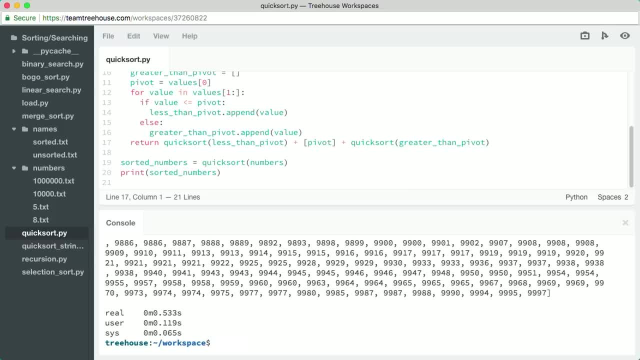 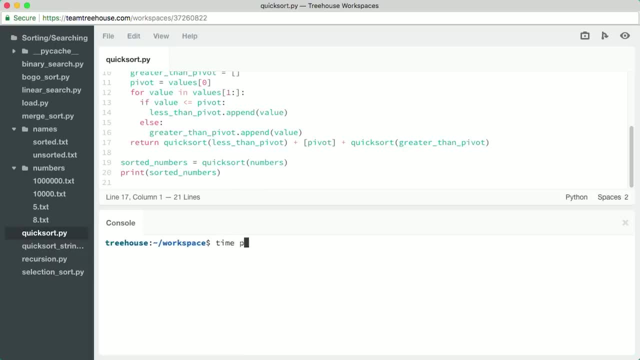 Remember the number of times you can divide N by 2 until you reach 1 is expressed as log N. So the runtime of binary search in Big O notation is O, where N is the number of items you have to search through, Even for very large values of N, that is, very large lists you have to search through. 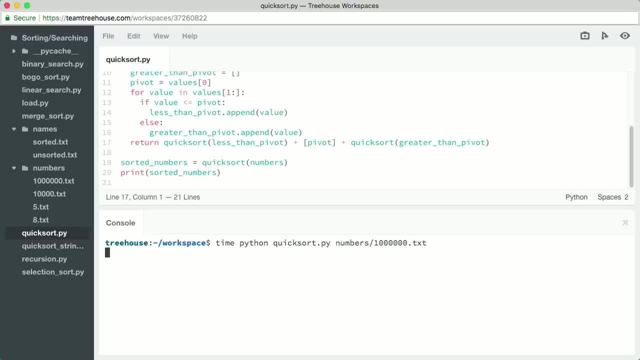 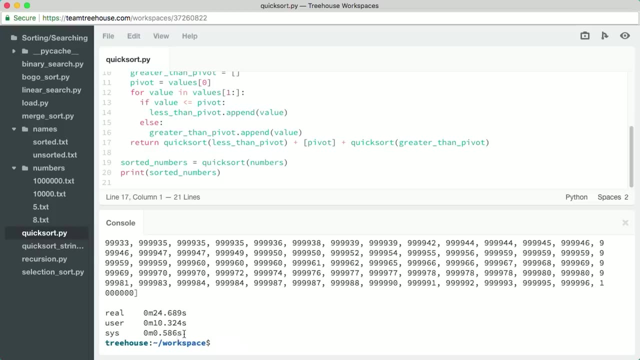 the number of operations needed to search is very small. Binary search is a very fast, efficient algorithm. That's our tour of sorting and searching algorithms. Be sure to check the teacher's notes for opportunities to learn more. Thanks for watching. 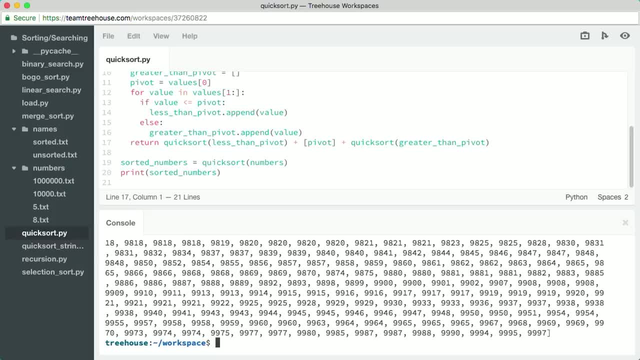 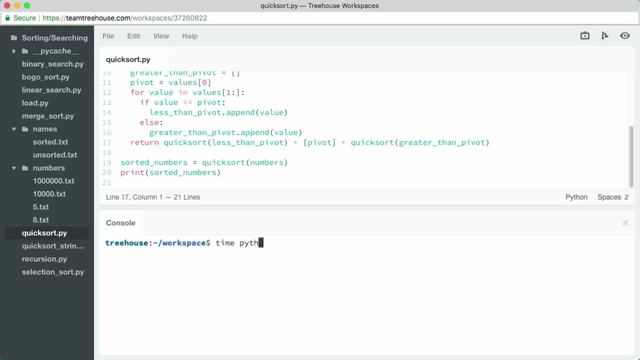 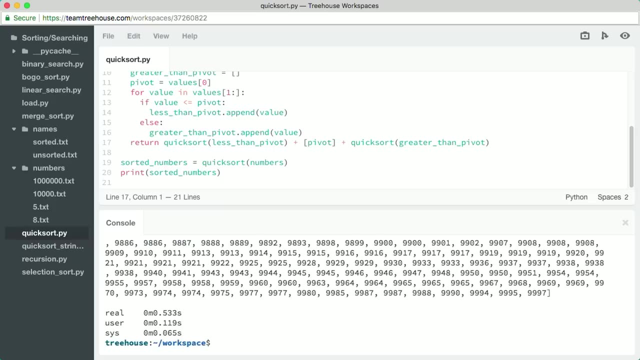 There we go And it seems pretty fast, But how fast exactly? Let's run it with the time command to see how long it takes Time. Python quicksort dot pi numbers 10,000 dot text. Remember we need to ignore the real result. 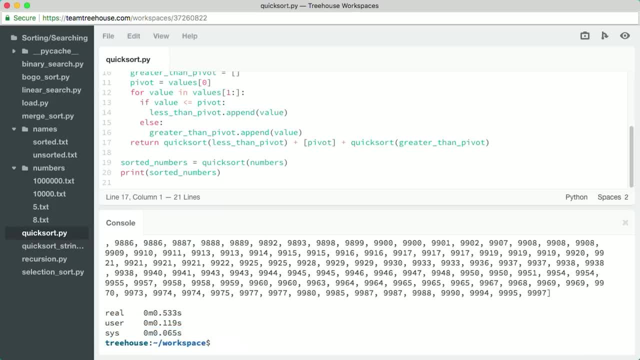 and add the user and sys results. It took less than a second of CPU time to sort 10,000 numbers with quicksort. Remember that selection sort took about 13 seconds. That's a pretty substantial improvement. And with a million numbers, 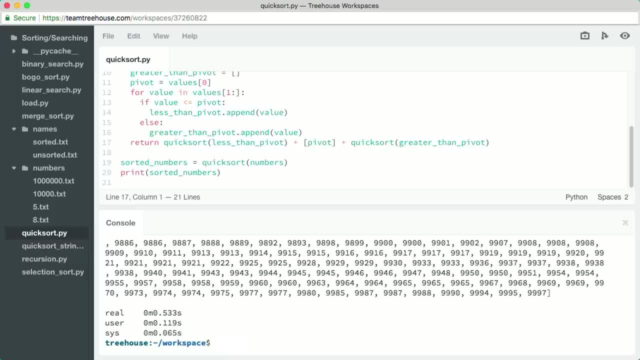 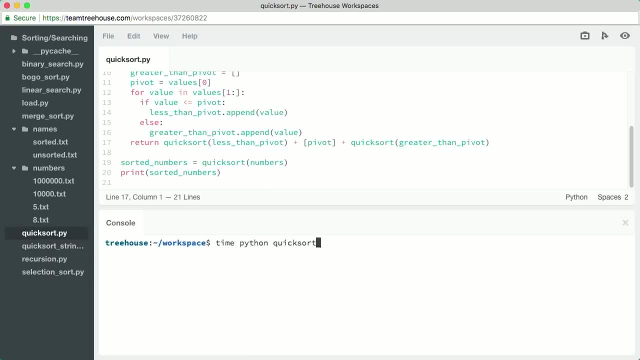 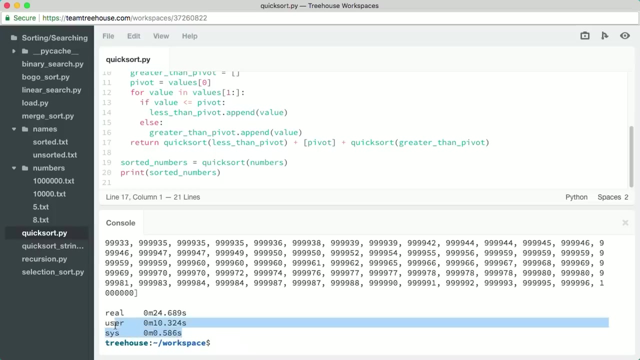 selection sort took so long that it never even finished successfully. Let's see if quicksort performs any better Time. Python quicksort dot pi numbers 1 million dot text. Not only did quicksort sort a million numbers successfully, it only took about 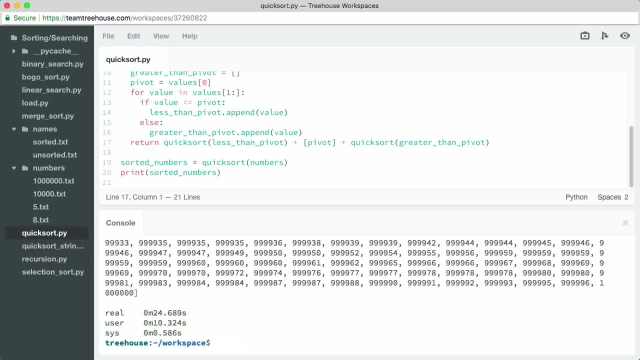 11 seconds of CPU time. Quicksort is clearly much, much faster than selection sort. How much faster, That's something we'll discuss in a later video. What we've shown you here is just one way to implement quicksort, Although the basic algorithm is always. 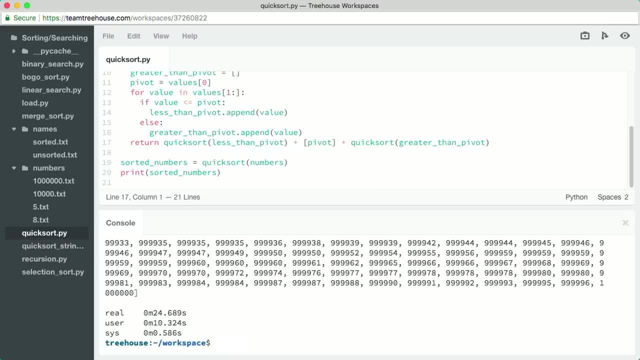 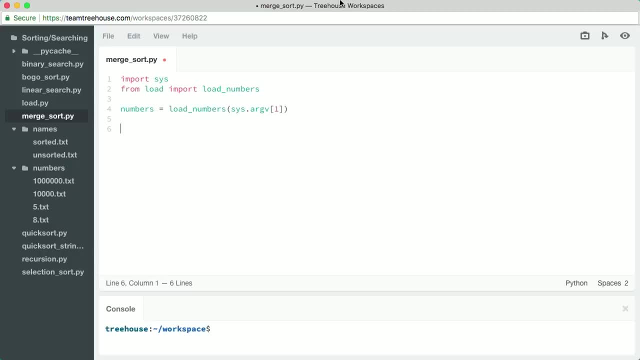 the same. the details can vary, like how you pick the pivot. See the teacher's notes for more details. Let's review another sorting algorithm, merge sort, so that we can compare it with quicksort. Merge sort is already covered elsewhere on the site so we won't go into as much. 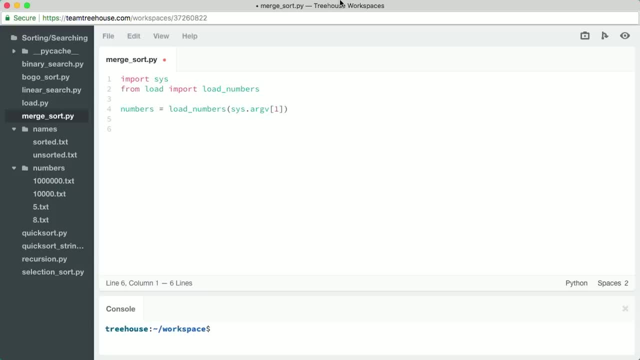 detail about it, but we'll have more info in the teacher's notes if you want it. Both quicksort and merge sort are recursive. The difference between them is in the sorting mechanism itself, Whereas quicksort sorts a list into two sublists that are less than or greater than a. 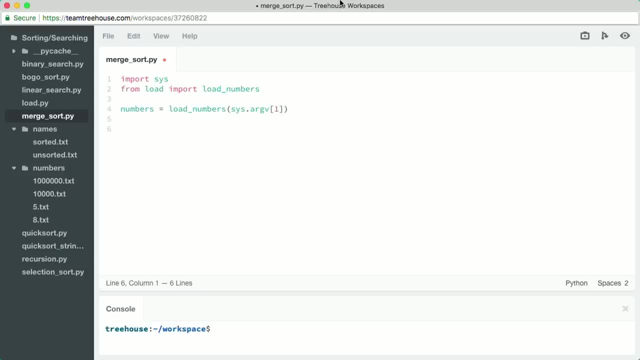 pivot value. merge sort simply splits the list in half recursively and then sorts the halves as it merges them back together. That's why it's called merge sort. You may recognize this code at the top by now. It just loads a file full. 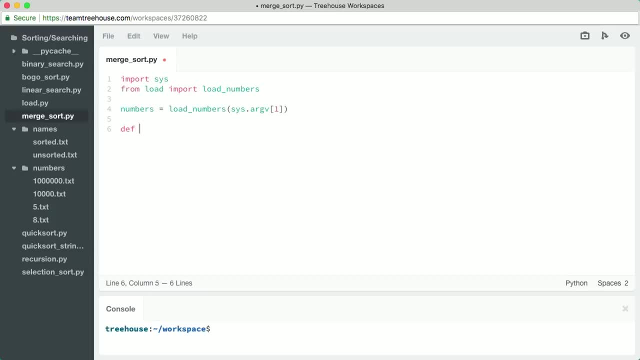 of numbers into a list. Let's define a recursive merge sort function. As usual, it'll take the list or sublist that we want it to sort. Our base case is the same as with quicksort, If the list has zero or one values. 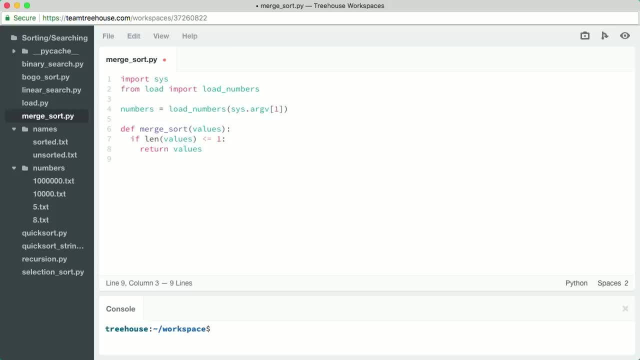 there's nothing to sort, so we return it as is. If we didn't return, it means we're in the recursive case. so first we need to split the list in half, We need to know the index we should split on. so 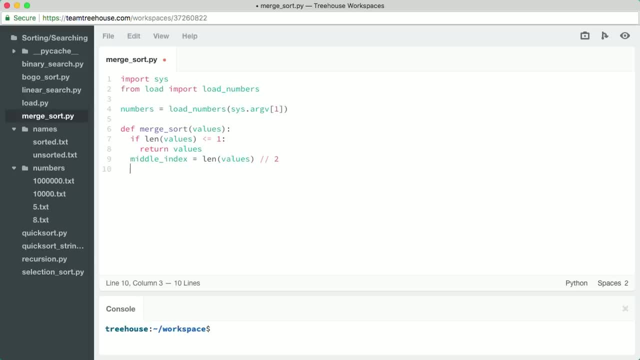 we get the length of the list and divide it by two. So, for example, if there are eight items in the list, we'll want an index of four. But what if there were an odd number of items in the list, like seven? We can't have an index. 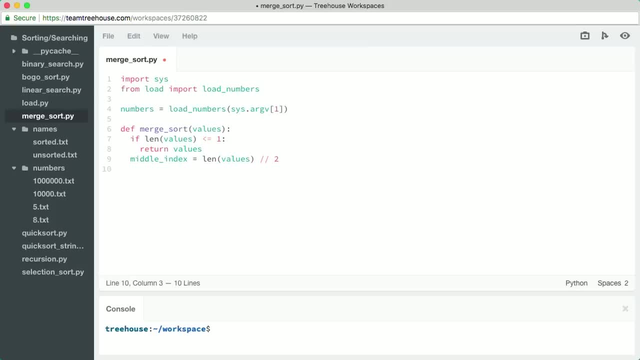 of 3.5, so we'll need to round down in that case. Since we're working in Python currently, we can take advantage of a special Python operator that divides and rounds the result down: the floor division operator. It consists of a double. 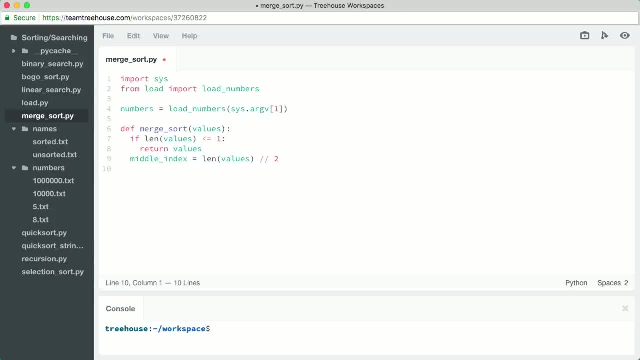 slash. Now. we'll use the Python slice syntax to get the left half of the list. We'll pass that list to a recursive call to the merge sort function. We'll also use slice syntax to get the right half of the list and pass that to merge sort. 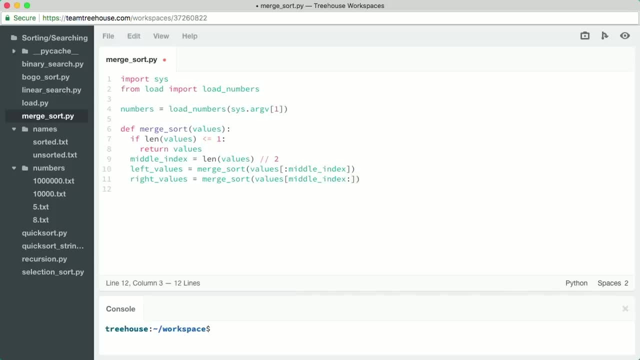 as well. Now we need to merge the two halves together and sort them. as we do it, We'll create a list to hold the sorted values. And now we get to the complicated part: merging the two halves together and sorting them as we do it. 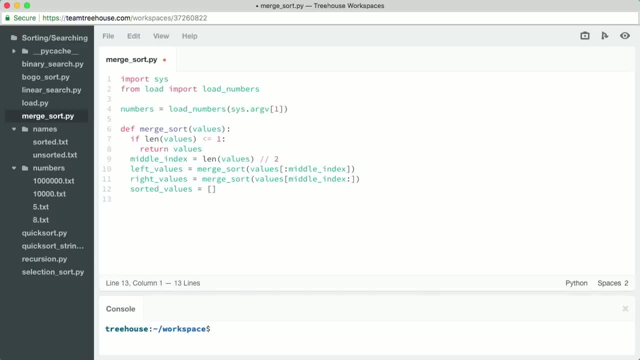 We'll be moving from left to right through the left half of the list, copying values over to the sorted values list. as we go, This left index variable will help us keep track of our position. At the same time, we'll also be moving from left to. 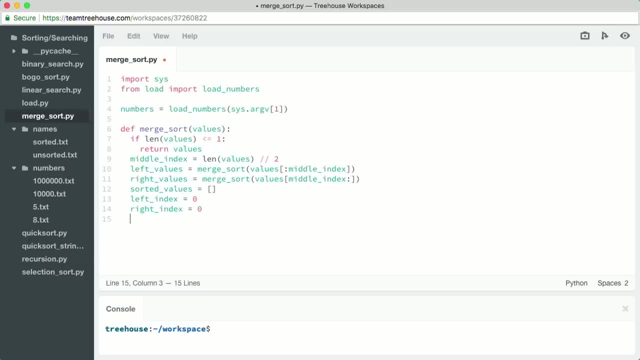 right through the right half of the list and copying values over. so we need a separate right index variable to track that position as well. We'll keep looping until we've processed all of the values in both halves of the list We're looking to copy over the. 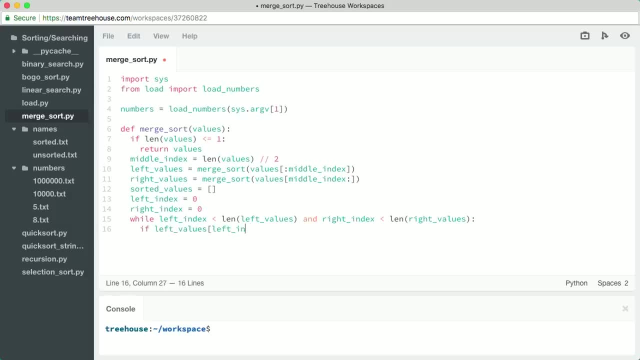 lowest values first. so first we test whether the current value on the left side is less than the value on the right side. If the left side value is less, that's what we'll copy over to the sorted list, And then we'll move to the next value in the left. 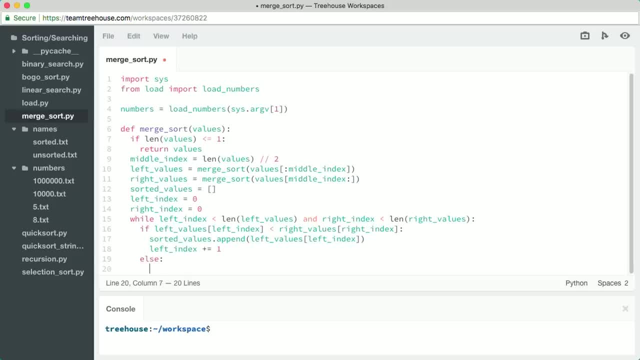 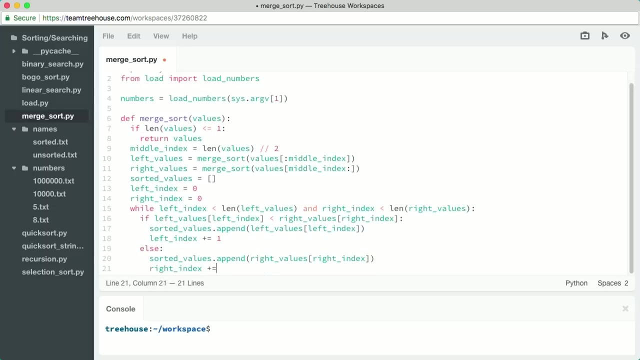 half of the list. Otherwise the current value from the right half must have been lower. So we'll copy that value to the sorted list instead, And then we'll move to the next value in the right half of the list. That ends the loop At this. 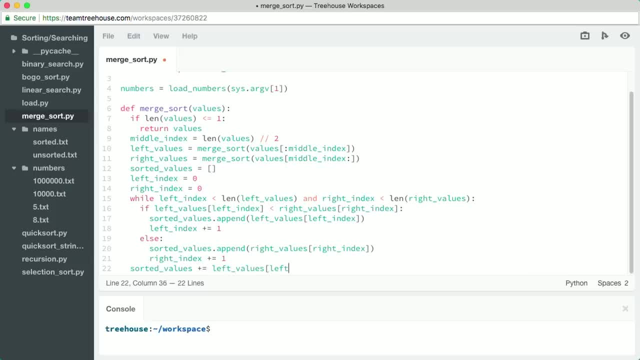 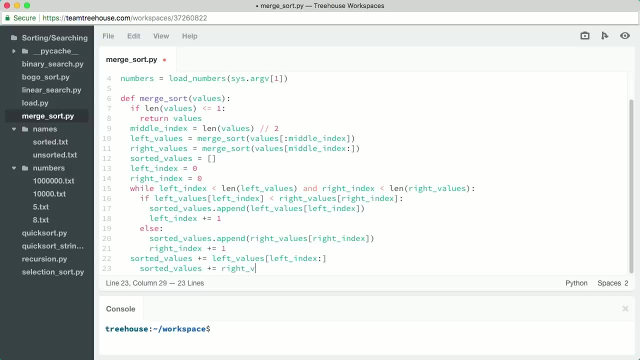 point. one of the two unsorted halves still has a value remaining and the other is empty. We won't waste time checking which is which. We'll just copy the remainder of both lists over to the sorted list. The one with the value left will. 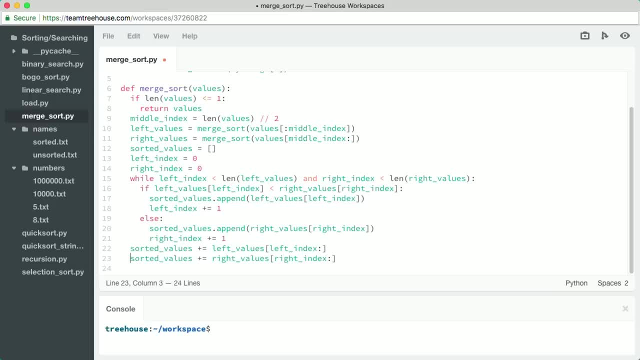 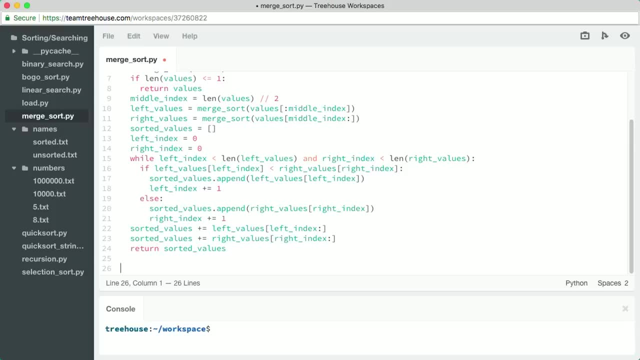 add that value and the empty one will add nothing. All the numbers from both halves should now be copied to the sorted list so we can return it. Finally, we need to kick the whole process off. We'll call the merge sort function with the list of numbers we loaded. 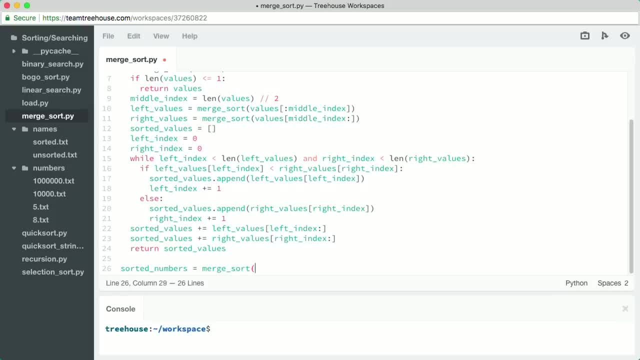 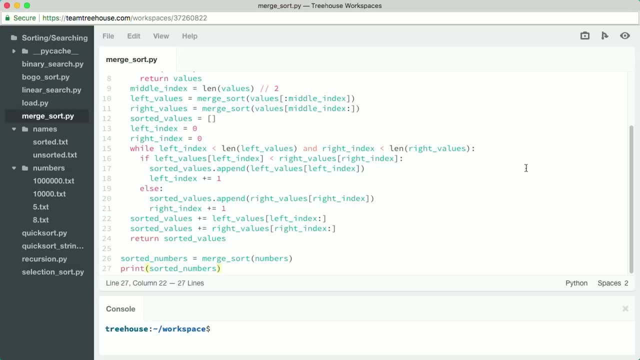 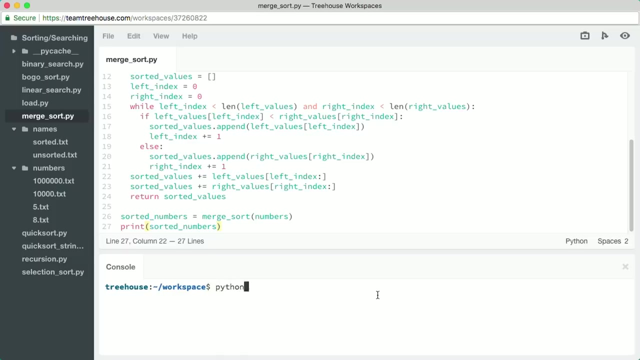 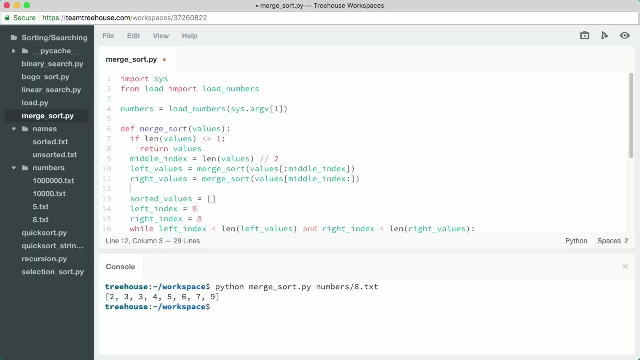 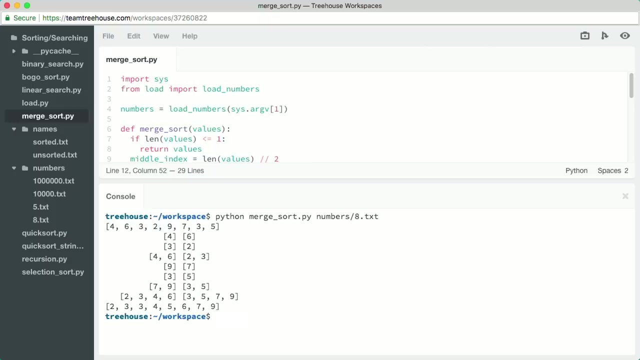 and print the result. Let's save this. 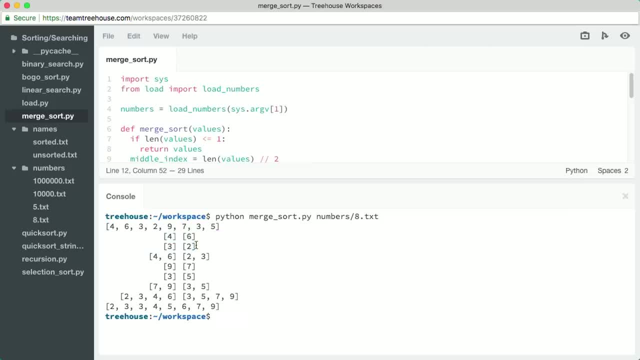 Then I'll run it on a list of 10,000 items. 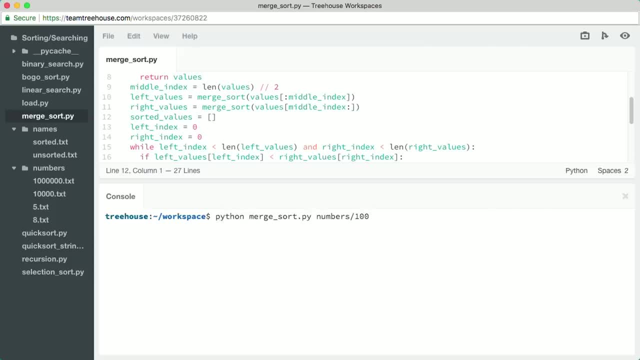 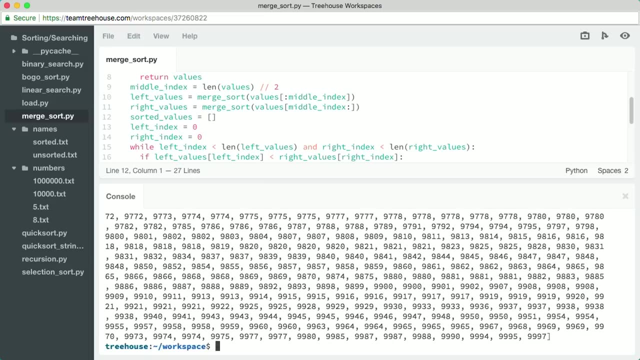 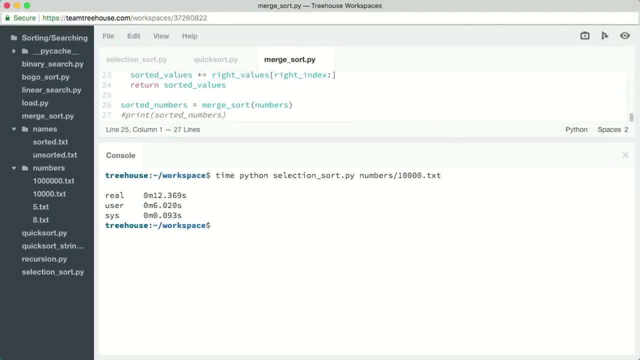 Python merge sortpy numbers 10,000, text. Not only did it work, it was pretty fast. But which is faster: merge, sort or quick sort? We'll look at that next. I've removed the call to print. that displays the sorted list. 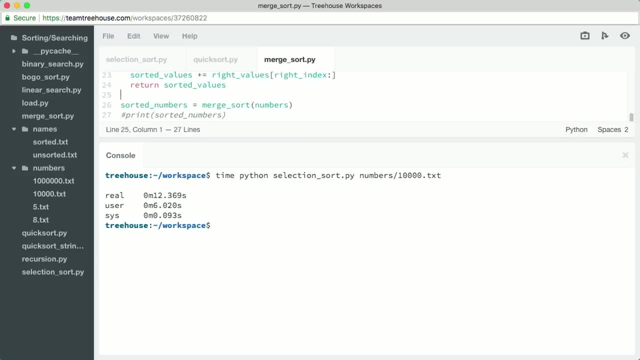 at the end of our selection sort, quick sort and merge sort scripts. That way it'll still run the sort but the output won't get in the way of our comparing runtimes. Let's try running each of these scripts and see how long it takes. 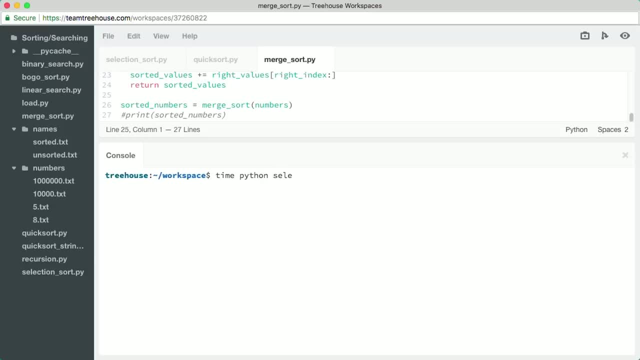 Time Python selection sort. We'll do that. one first Numbers 10,000, text. We combine the user and sys results and that gives us about six seconds. Now let's try quick sort Time Python. quick sort py: numbers: 10,000, text. 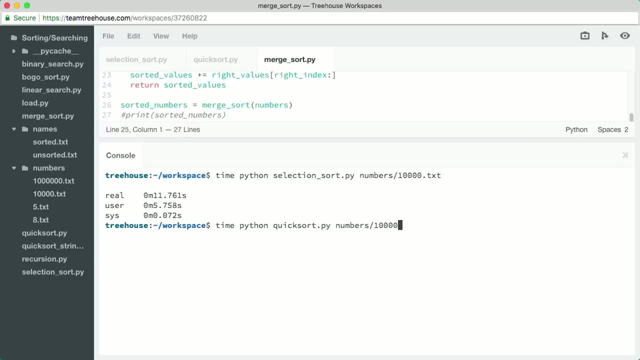 Time Python quick sort py numbers- 10,000, text. Time Python: quick sort py numbers- 10,000, text Much faster, less than a second. And finally, time Python merge: sort py numbers: 10,000, text. 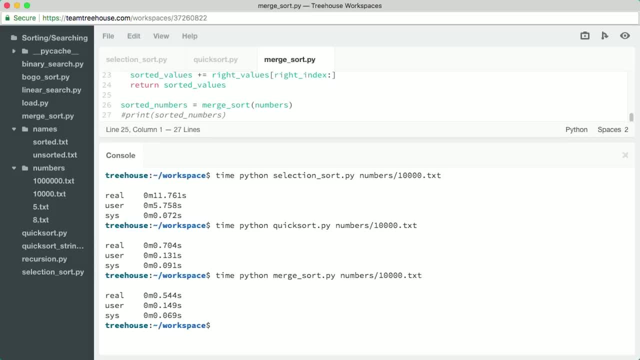 A little longer but far less than a second. So even on a list with just 10,000 numbers selection sort takes many times as long as quick sort and merge sort, And remember I ran the selection sort script on a file with a million numbers. 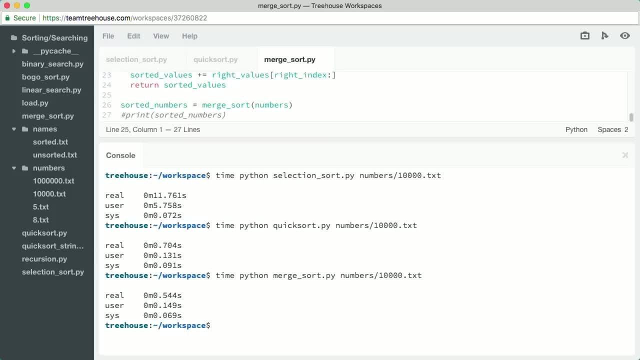 and it took so long that my workspace timed out before it completed. It looks like selection sort is out of the running. It's a viable sorting algorithm. It may be easy to understand and implement, but it's just too slow to handle the huge data sets. 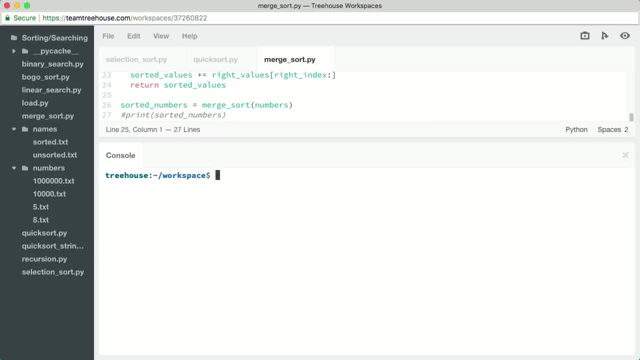 that are out in the real world. Now let's try quick sort and merge sort on our file with a million numbers and see how they compare there. Time Python- quick sort- py numbers 10,000, text. 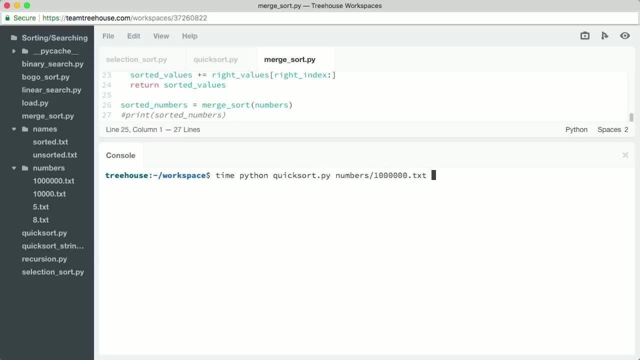 Numbers- 1,000,000, text. Looks like it took about 11 seconds of CPU time. Now let's try merge sort Time Python. merge sort py: numbers- 1,000,000, text. 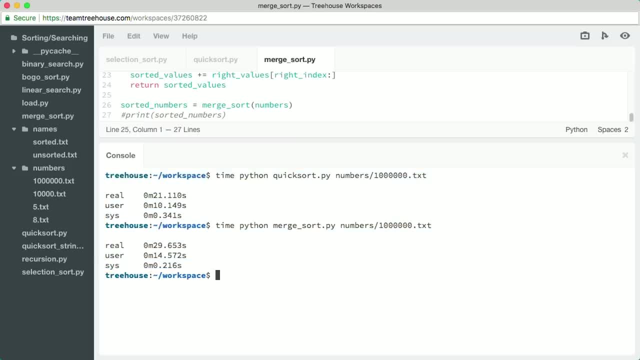 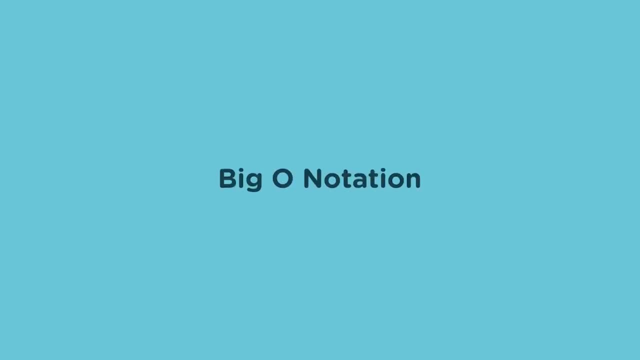 That took about 15 seconds of CPU time. It looks like quick sort is marginally faster than merge sort. on this sample data. We had to learn a lot of details for each algorithm. we've covered in this course Developers who need to implement their own algorithms. 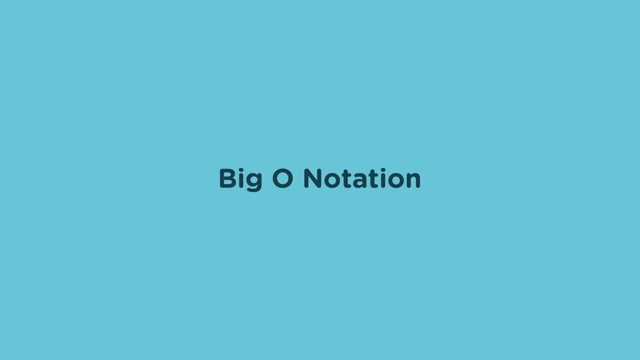 often need to choose an algorithm for each and every problem they need to solve, And they often need to discuss their decisions with other developers. Can you imagine needing to describe all the algorithms in this same level of detail all the time? You'd spend all your time in meetings rather than programming. 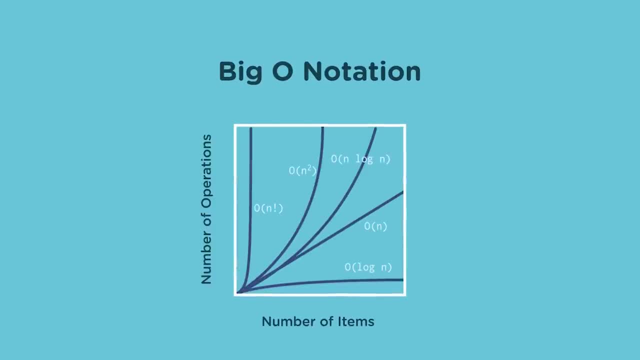 That's why big O notation was created, as a way of quickly describing how an algorithm performs as the data set it's working on increases in size. Big O notation lets you quickly compare several algorithms to choose the best one for your problem. The algorithms we've discussed in this course are very well known. 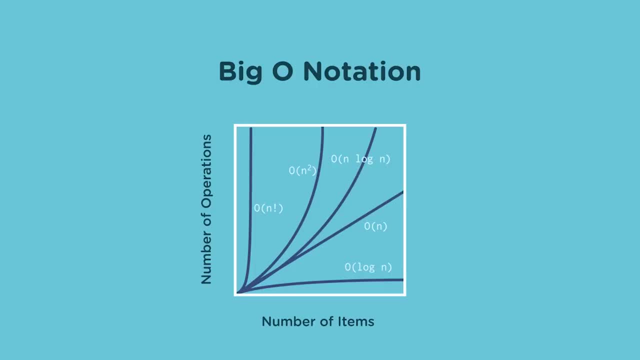 Some job interviewers are going to expect you to know their big O runtimes, So let's look at them. Remember that the N in big O notation refers to the number of elements you're operating on With selection sort. you need to check each item in the list. 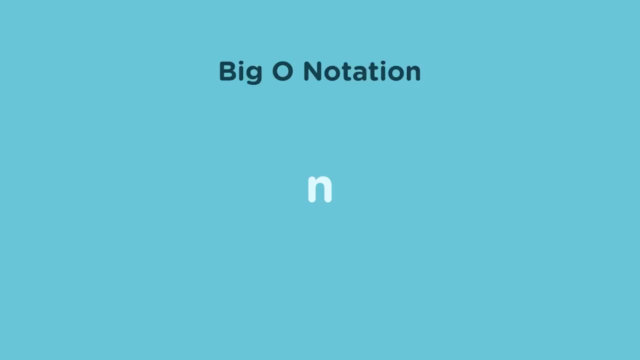 to see if it's the lowest, So you can move it over to the sorted list. So that's N operations. Suppose you're doing selection sort on a list of five items. N in this case would be five, So that's five operations before you can move an item. 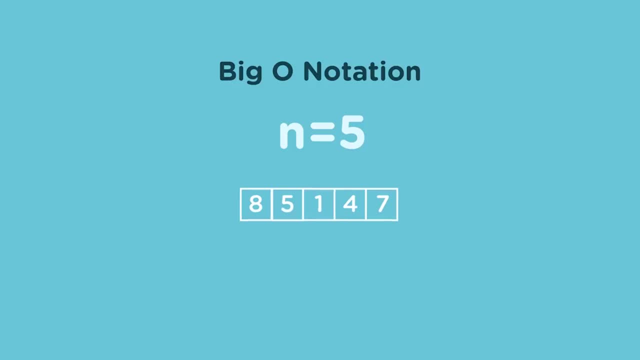 to the sorted list. But with selection sort you have to loop over the entire list for each item you want to move. There are five items in the list and you have to do five comparisons to move each one. So it's more like five times five operations. 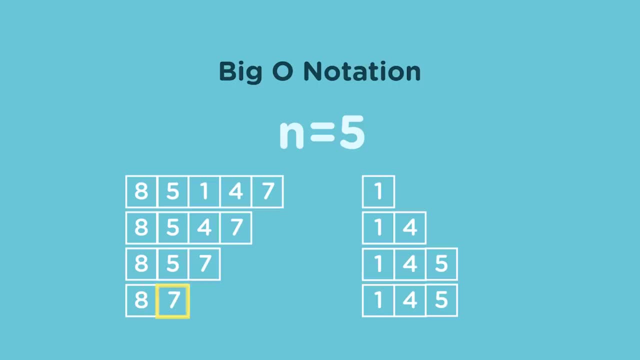 Or if we replace five with N, it's N times N Or N squared. But wait, you might say Half of that five by five grid of operations is missing because we're testing one fewer item in the unsorted list with each pass. 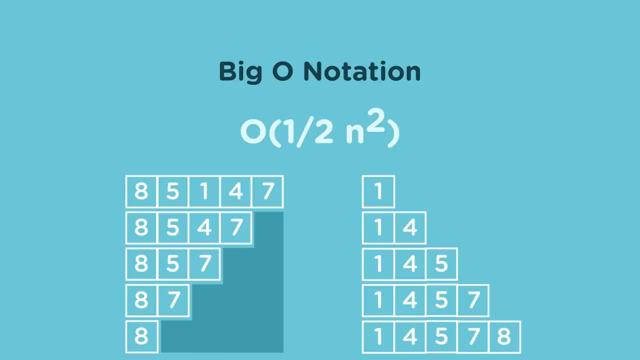 So isn't it more like one half times N times N? And this is true. We're not doing a full N squared operations. But remember, in big O notation, as the value of N gets really big, constants like one half become insignificant. 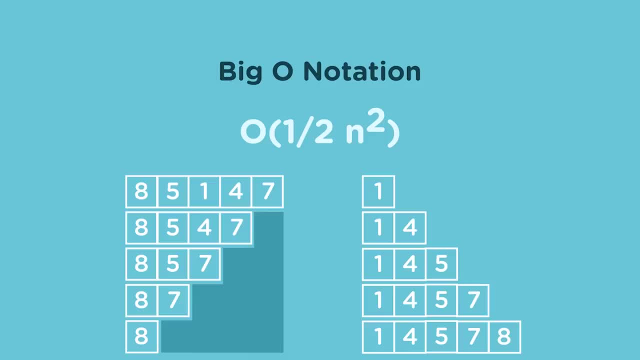 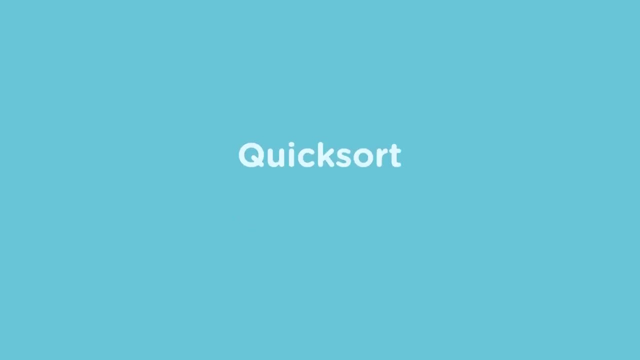 And so we discard them. The big O runtime of selection sort is widely recognized as being O N squared. Quicksort requires one operation for each element of the list it's sorting. It needs to select a pivot first, and then it needs to sort elements into lists. 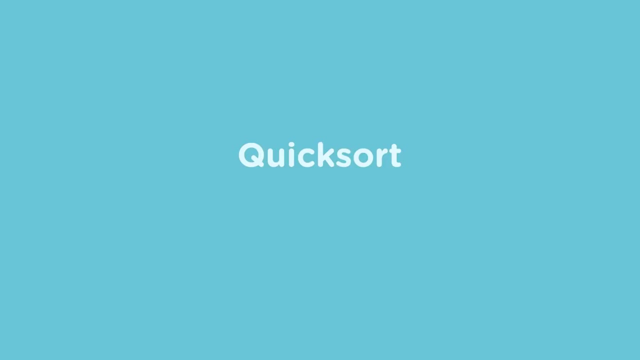 that are less than or greater than the pivot. So that's N operations. To put that another way: if you have a list of eight items, then N is eight. So it will take eight operations to split the list around the pivot, But of course the list isn't sorted. 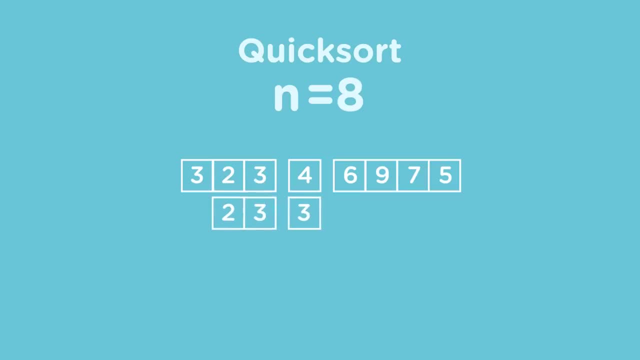 after splitting it around the pivot just once. You have to repeat them. you have to repeat those eight operations several times. In the best case you'll pick a pivot that's right in the middle of the list, so that you're dividing the list exactly in half. 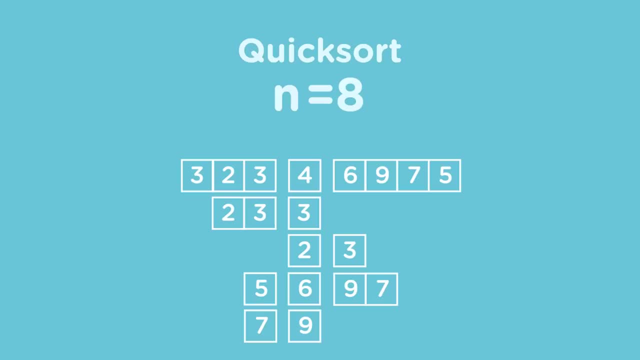 Then you keep dividing the list in half until you have a list with a length of one. The number of times you need to divide N in half until you reach one is expressed as log N, So you need to repeat N sorting operations, log N times. 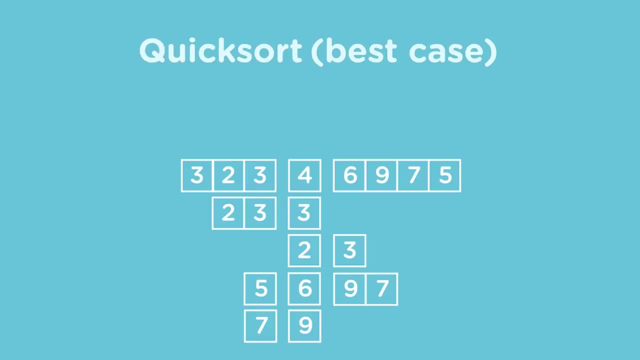 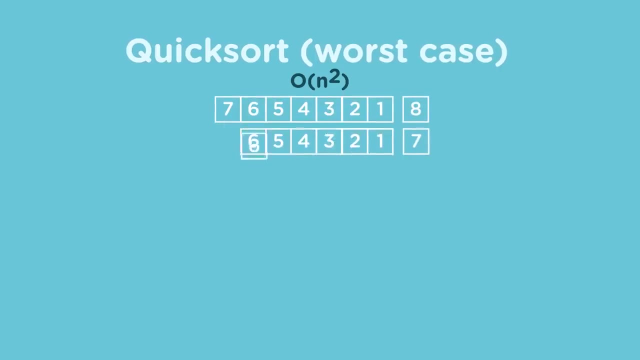 That leaves us with the best case: runtime for quicksort of O N log N. But that's the best case. What about the worst case? Well, if you pick the wrong pivot, you won't be dividing the list exactly in half. If you pick a really bad pivot. 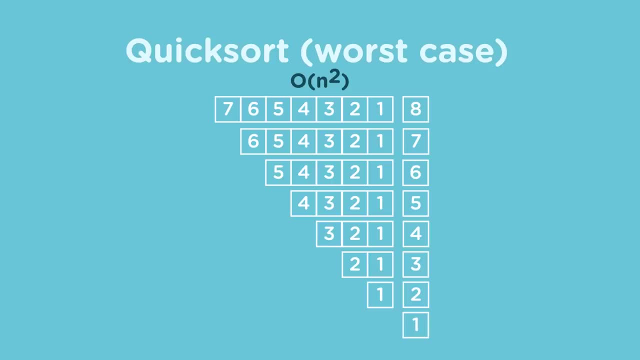 the next recursive call to quicksort will only reduce the list length by one. Since our quicksort function simply picks the first item to use as a pivot. we can make it pick the worst possible pivot repeatedly simply by giving it a list that's sorted in reverse order. 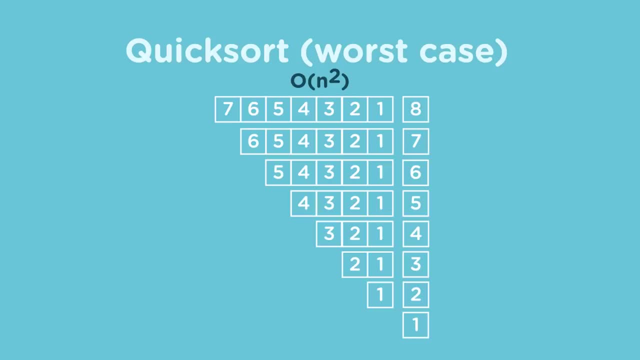 If we pick the worst possible pivot every time, we'll have to split the list once for every item it contains. we'll have to split the list once for every item it contains. we'll have to split the list once for every item it contains. 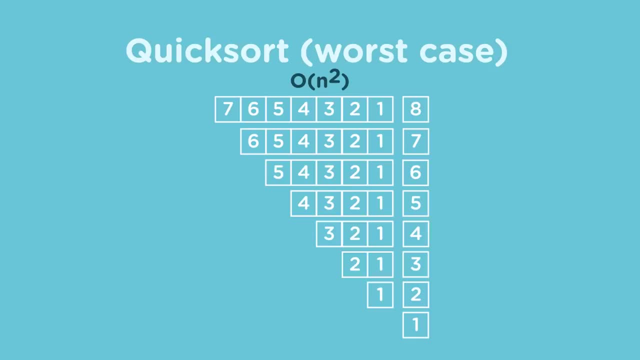 and then do N sorting operations on it. You already know another sorting algorithm that only manages to reduce the list by one element with each pass selection sort. Selection sort has a runtime of O N squared And in the worst case that's the runtime for quicksort as well. 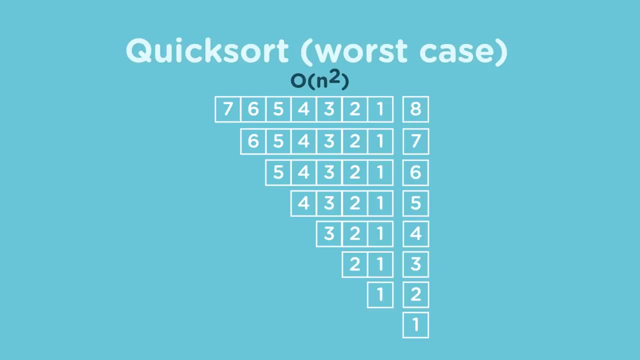 So which do we consider when trying to decide whether to use quicksort, the best case or the worst case? Well, as long as your implementation doesn't just pick the first item as a pivot, which we did so we could demonstrate this issue- 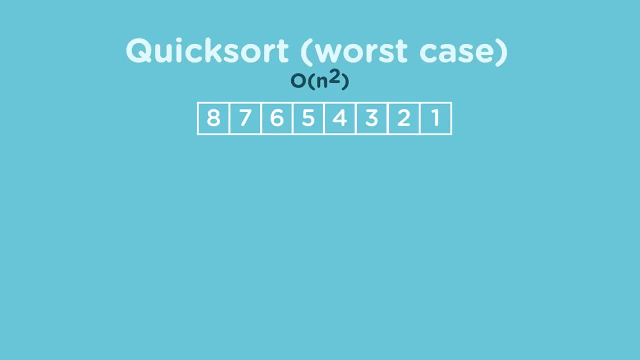 it turns out that, on average, quicksort performs closer to the best case. Many quicksort implementations accomplish this simply by picking a pivot at random on each recursive loop. Here we are sorting our reverse sorted data again, but this time we pick pivots at random. 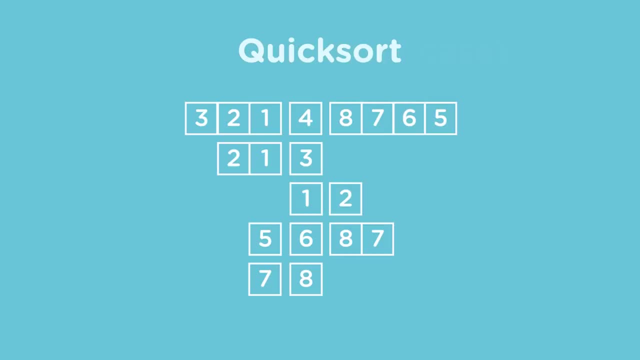 which reduces the number of recursive operations needed. Sure, random pivots sometimes give you the best case and sometimes you'll randomly get the worst case, but it all averages out over multiple calls to the quicksort function In merge sort. there's no pivot to pick. 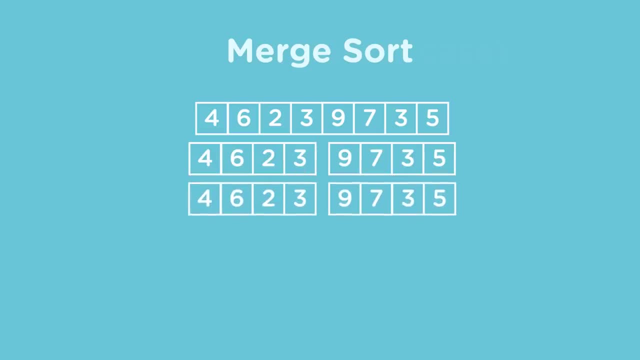 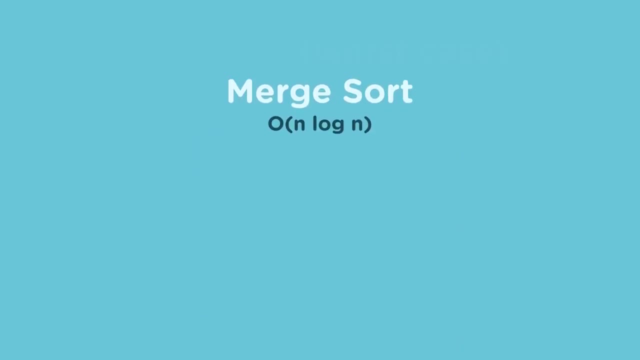 Your list of N items always gets divided in half log N times. That means merge sort always has a big O runtime of O N log N. Contrast that with quicksort, which only has a runtime of O N log N in the best case. 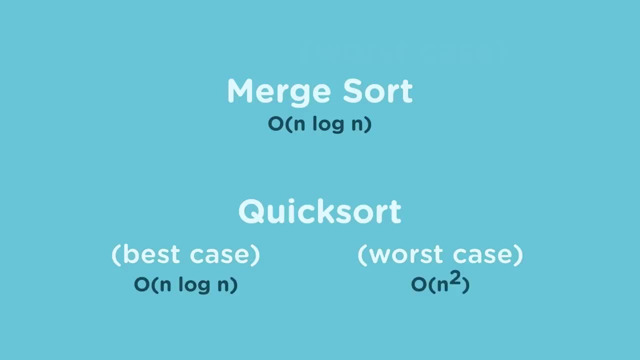 In the worst case, quicksort's runtime is O N squared. And yet out in the real world, quicksort is more commonly used than merge sort. Now why is that if quicksort's big O runtime can sometimes be worse than merge sorts? 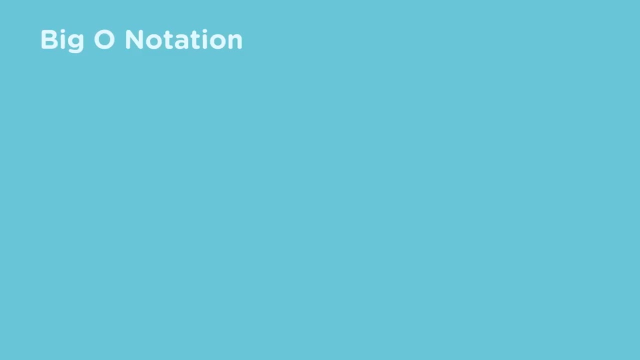 This is one of those situations where big O notation doesn't tell you the whole story. All big O can tell you is the number of times an operation is performed. It doesn't describe how long that operation takes And the operation merge sort performs repeatedly. 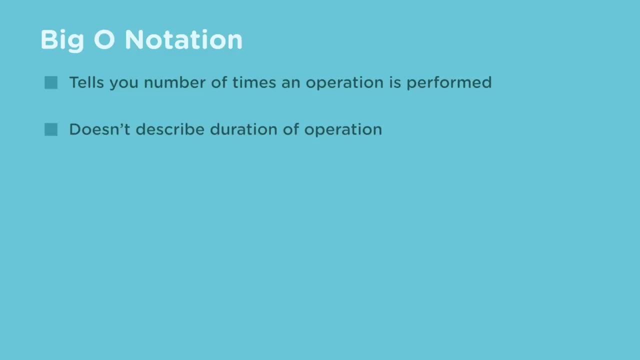 takes longer than the operation quicksort performs repeatedly. Big O is a useful tool for quickly describing how the runtime of an algorithm increases as the data set it's operating on gets really, really big. But you can't always choose between two algorithms based just on the runtime. 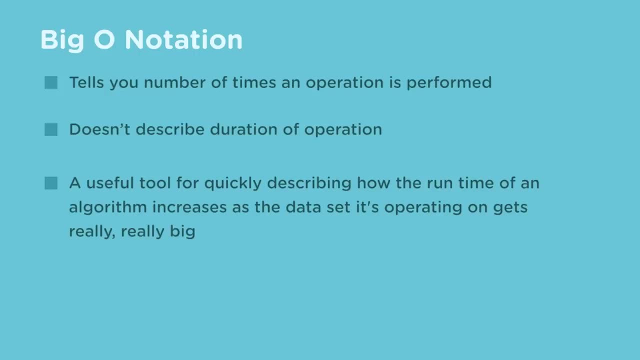 Sometimes there's additional info. you need to know about an algorithm to make a good decision. Now that we can sort a list of items, we're well on our way to being able to search a list efficiently as well. We'll look at how to do that in the next stage. 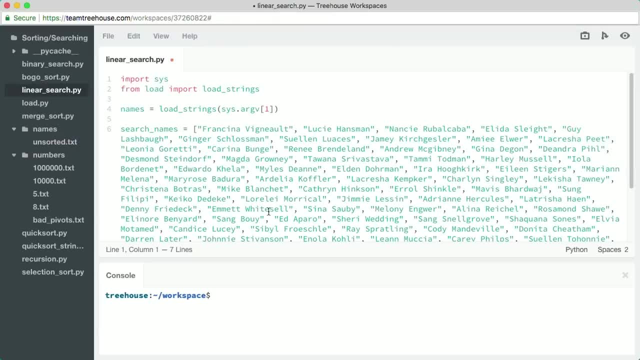 Now that we've covered sorting algorithms, the groundwork has been laid to talk about searching algorithms. If you need to search through an unsorted list of items- binary searches- you can use an option because you have no idea which half of the list contains the item you're looking for. 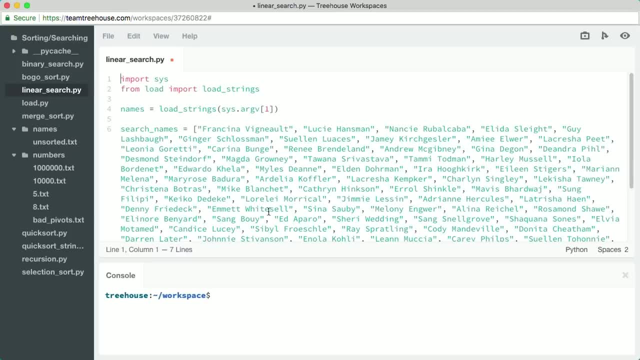 Your only real option is to start at the beginning and compare each item in the list to your target value, one at a time, until you find the value you're looking for. This algorithm is called linear search or sequential search, because the search proceeds in a straight line or sequence. 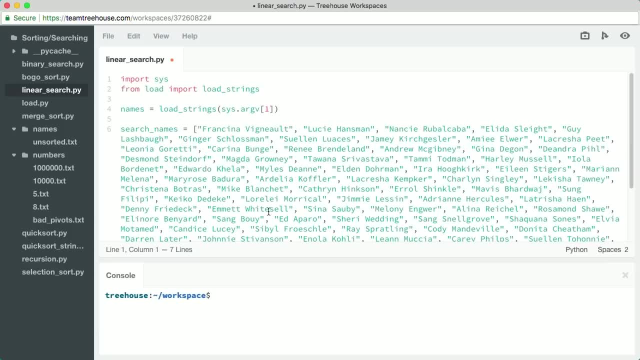 Even though linear search is inefficient, searching for just one name will happen so fast that we won't be able to tell anything useful about the algorithms runtime. So let's suppose we had a hundred different names and that we needed to know where they appear in a list of unsorted names. 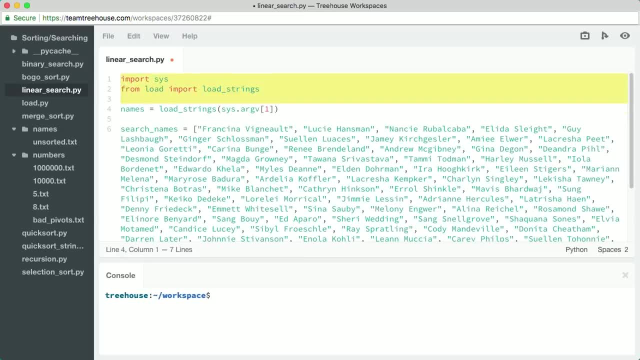 Here's some code that demonstrates, As usual, this code at the top isn't relevant to the search algorithm. It's just like the code that loaded a list of numbers from a file in the previous stage, but this code calls a different function: load strings. 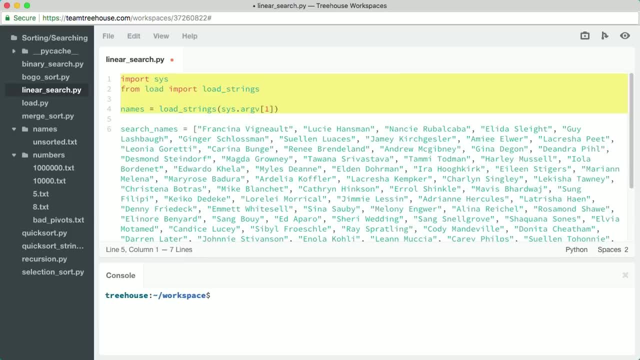 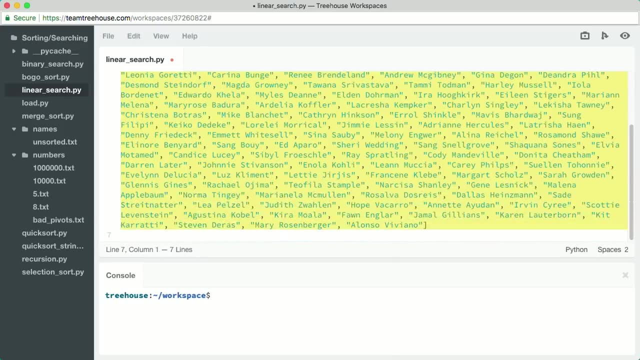 that loads a list of strings in. If you want the load strings Python code, we'll have it for you. in the teacher's notes. Here's a separate hard-coded list containing the 100 names we're going to search for. We'll loop through each name in this list. 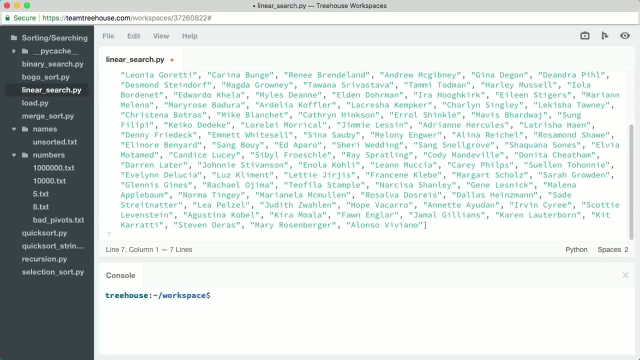 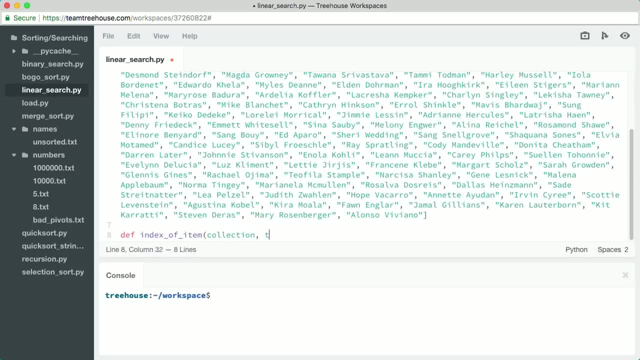 and pass it to our search function to get the index within the full list where it appears. Now let's implement the search function. Compared to the sorting algorithms, this is going to be short. The index of item function takes the Python list you want to search through. 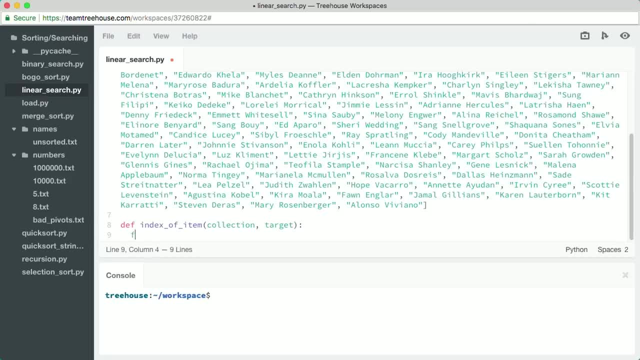 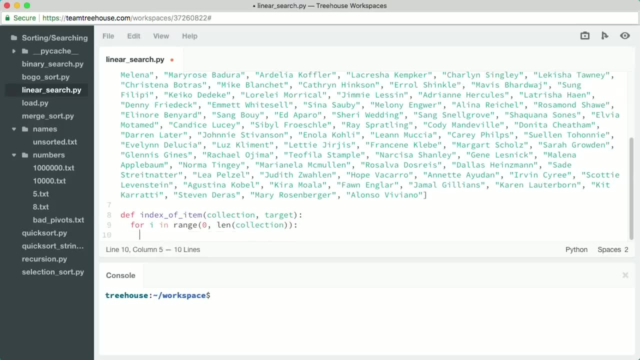 and a single target value you want to search for. Now we need to loop over each item in the list. The range function gives us a range of numbers from its first argument to, but not including its second argument. So if our list had a length of five, 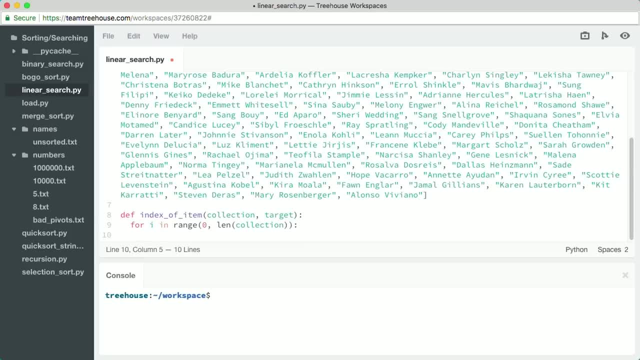 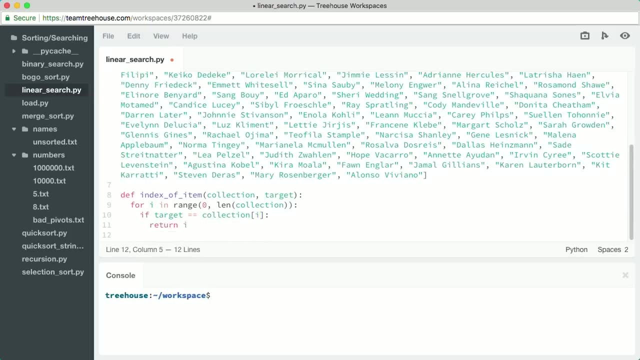 this would loop over the indexes zero through four. We test whether the list item at the current index matches our target. If it does, then we return the index of the current item. This will exit the index of item function without looping over the remaining items in the list. 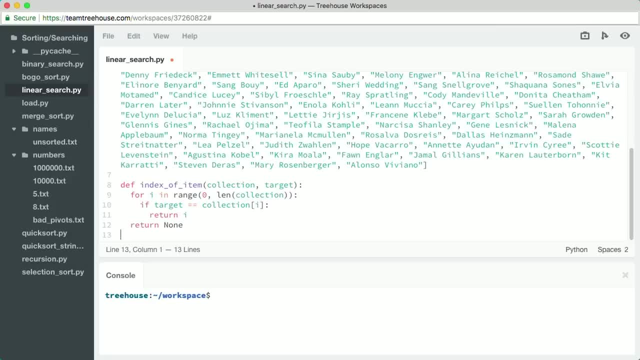 If we reach the end of the loop without finding the target value, that means it wasn't in the list. So instead of returning an index, we return the special Python value none, which indicates the absence of a value. Other languages have similar values, like nil or null. 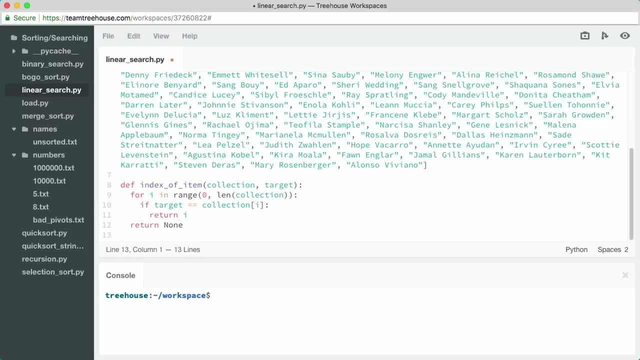 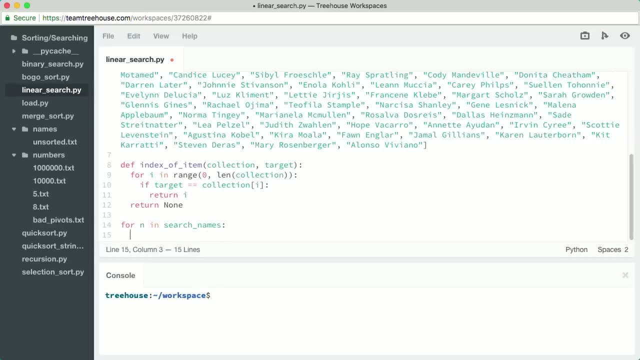 but if yours doesn't, you might have to return a value that would otherwise be impossible, like an index of negative one. Now let's call our new search function. We start by looping over the list of 100 values we're looking for. 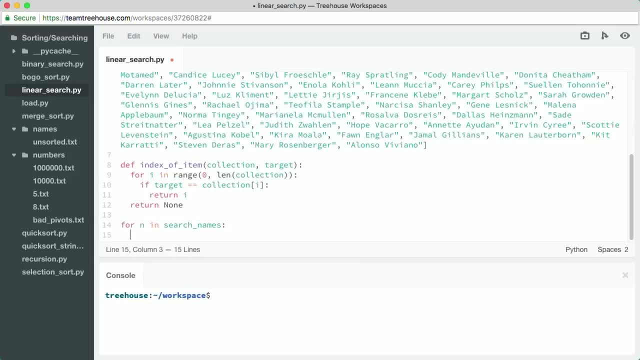 We're using the values themselves this time, not their indexes within the list, So there's no need to mess with Python's range function. Here's the actual call to the index of item function. First, we set the full list of names that we loaded from the file. 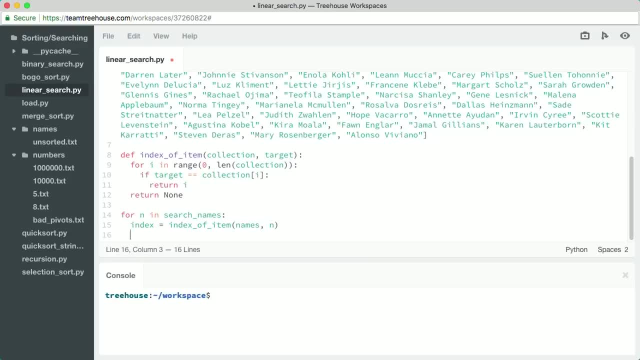 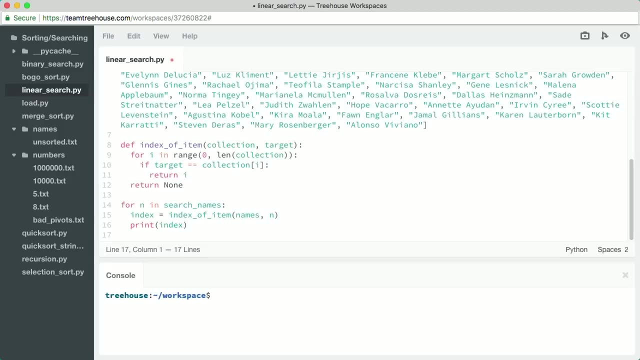 plus the name we want to search for within that list. Then we store the index. it returns in a variable And lastly we print the index we get back from the index of item function. Let's save this and go to our console and see if it works. 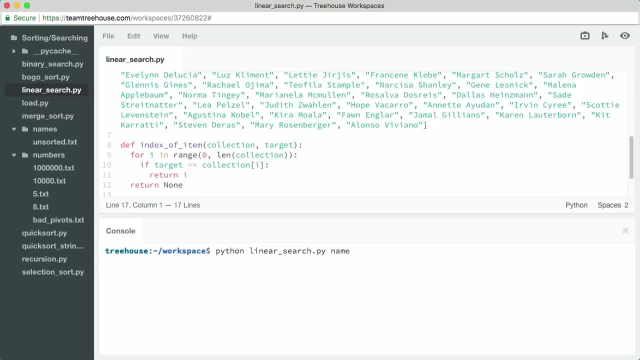 Python linearsearchpy names unsortedtxt And it'll print out the list of indexes for each name. We've actually set it up so that the last two items in the list of names we're going to search for corresponded to the first and last name within the file. 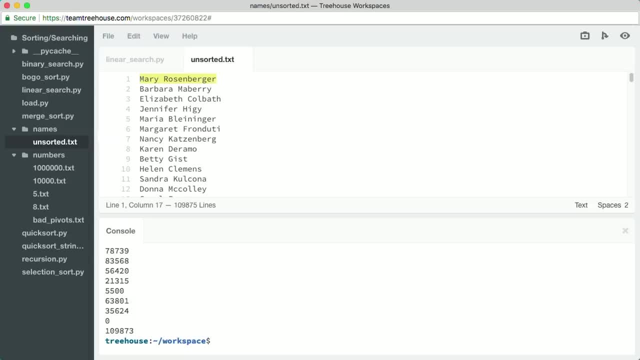 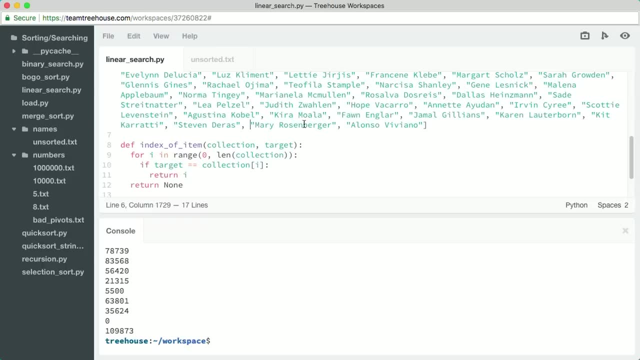 So if we open up our unsortedtxt file, we'll see Mary Rosenberger is the first name and Alonso Viviano is the last name, And those are the last two values in our list of names we're searching for. So it returned an index of zero. 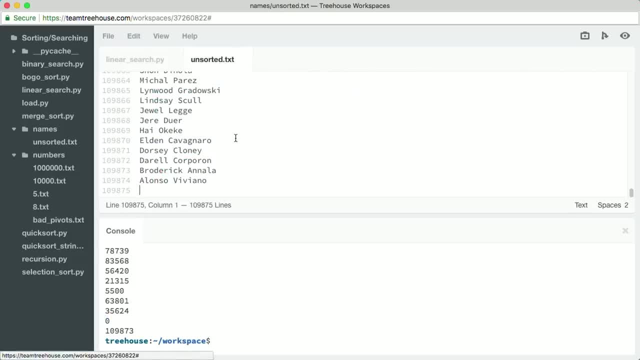 for that second to last name- And you can see that name here on line one of the file- Everything starts at one and the Python list indexes start at zero, So that makes sense. And for the last name it returned an index of 109873.. 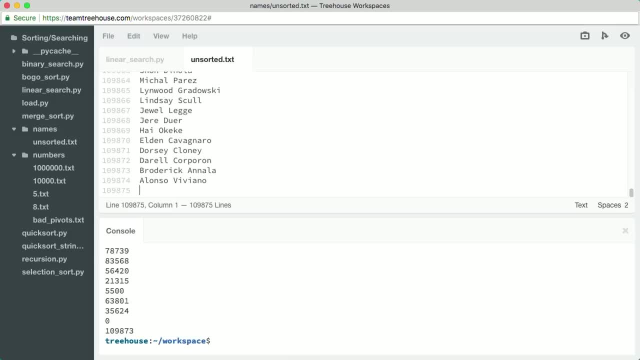 And you can see that name here on line 109874.. So we can see that it's returning the correct indexes, But right now we're just searching for a hundred different names in a list of 100,000 names In the real world. we're going to be looking. 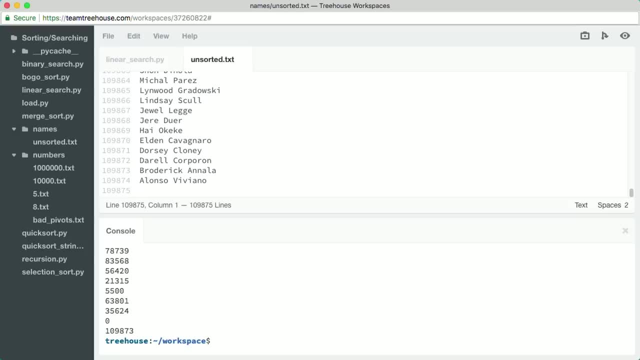 for many more names than that, within much bigger lists than that. Can we do this any faster? Yes, but we'll need to use the binary search algorithm And for that to work we need to sort our list of strings. We'll do that in the next video. 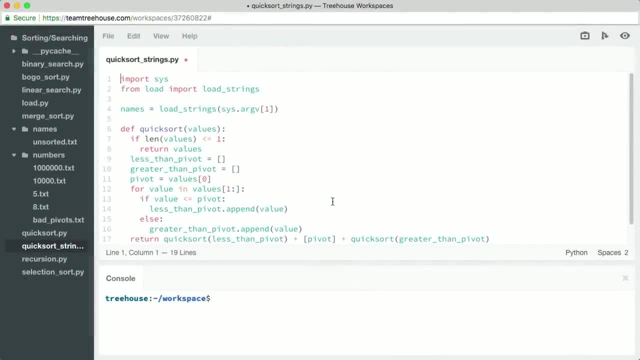 Before we can use the binary search algorithm on our list of names, we need to sort it. Let's do that now. We need to load our unsorted list of names from a file, sort it and write the sorted names back out to a new file. 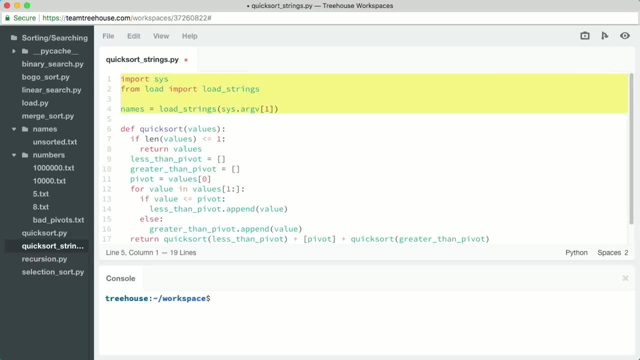 Again. this code at the top just loads a file full of strings into a list. We'll use our quick sort method to sort the list of names. Its code is completely unchanged from when you saw it in the previous stage. We just call our quick sort function. 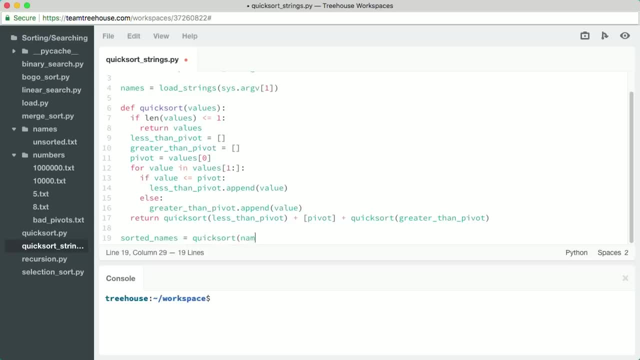 on the list of names loaded from the file and save the list to a variable. Then we loop through each name in the sorted list and we print that name. That's all there is to it. Let's save this script and try running it. 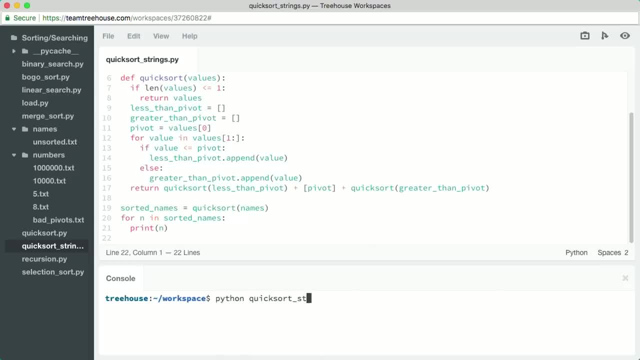 Python, quick sort stringspy and we'll pass it the names Un-sortedtxt file. Let me resize the console window here a little bit. That prints the sorted list of names out to the terminal, but we need it in a file. 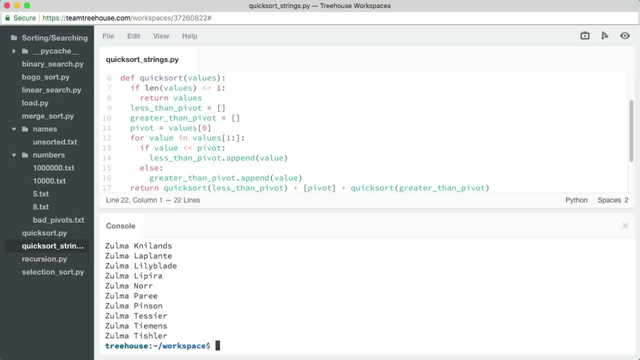 So we'll do what's called a redirect of the program's output. We'll run the same command as before, but at the end we'll put a great event sign followed by the path to a file that we want the program output written to names: sortedtxt. 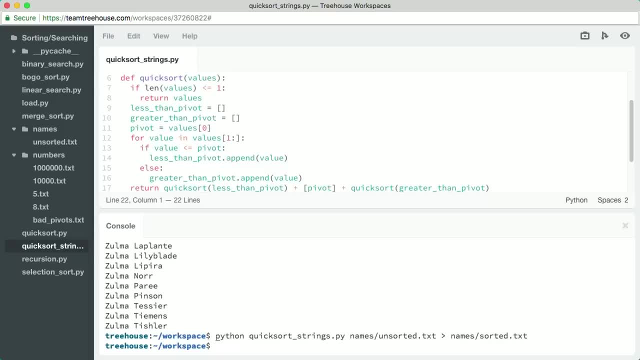 Redirecting works not only on Linux-based systems like workspaces, but also on Macs and even on Windows machines. You just need to be careful, because if you redirect to an existing file, its contents will be overwritten without asking you. Let me refresh the list of files in the sidebar. 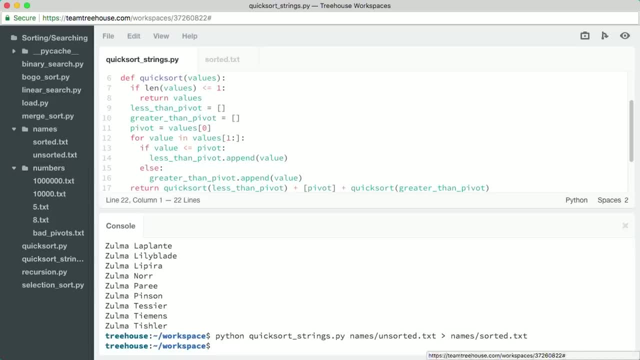 And you'll see that we now have a new sortedtxt file in the names directory. It's the same number of lines as the unsortedtxt file, but all the names are sorted now. Now we can load this file of sorted names into a list. 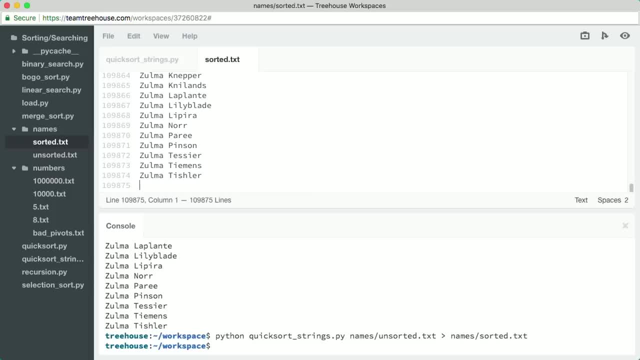 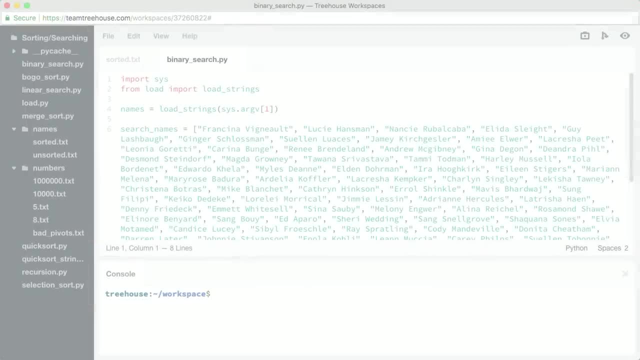 and we'll be able to use that list with the binary search algorithm. We'll see how to do that. next, Now that we have our list of names sorted, we can use the binary search algorithm on it. Let's see if we can use it to speed up our search. 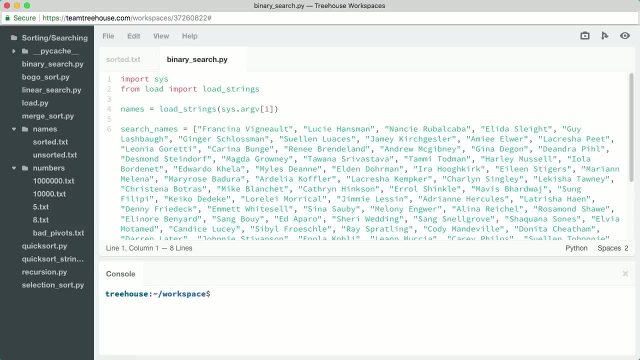 for the indexes of 100 names. Binary search keeps narrowing down the list until it has the value it's looking for. It's faster than linear search because it discards half the potential matches each time. Our code here at the top of our binary search script: 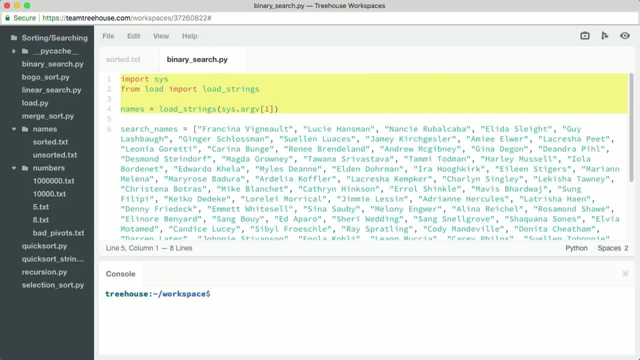 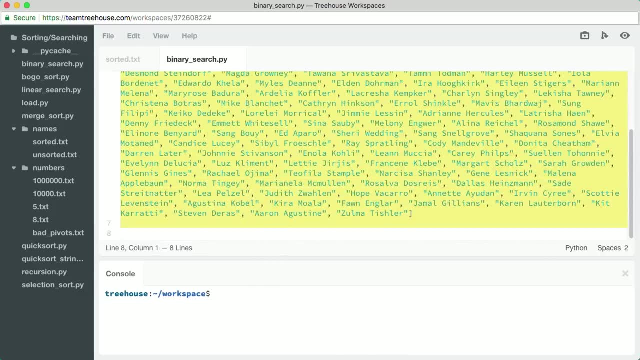 is unchanged from the previous scripts. We just called the loadStrings function to load our 100,000 sorted names from a file. Here we've hardcoded the list of 100 names we're going to search for again. It's identical to the list from the linear search script. 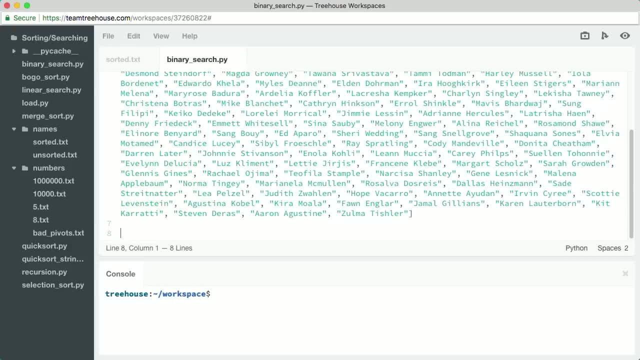 except that I've again changed the last two names to correspond to the names on the first and last lines of the file we'll be loading. Now let's write the function that will implement our binary search algorithm, Like the linear search function. before it'll take two arguments: 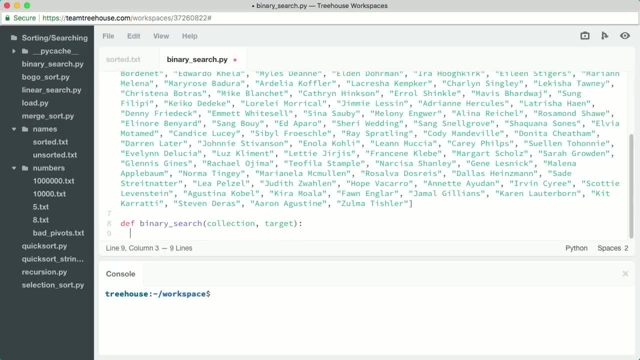 The first is the list we're going to search through and the second is the target value we'll be searching for. Again, the binary search function will return the index it found, the value at or the special value none if it wasn't found. 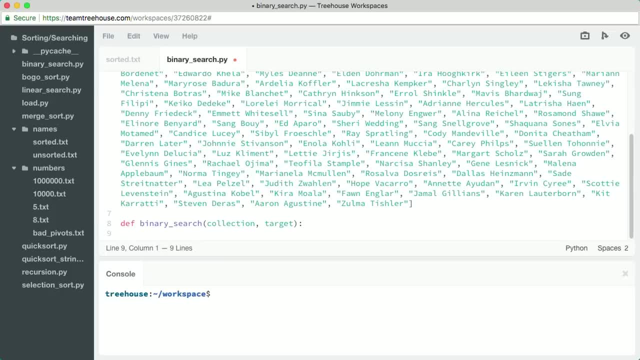 Binary search is faster than linear search because it discards half the values it has to search through each time. To do this, it needs to keep track of a range that it still needs to search through. To start, that range is going to include the full list. 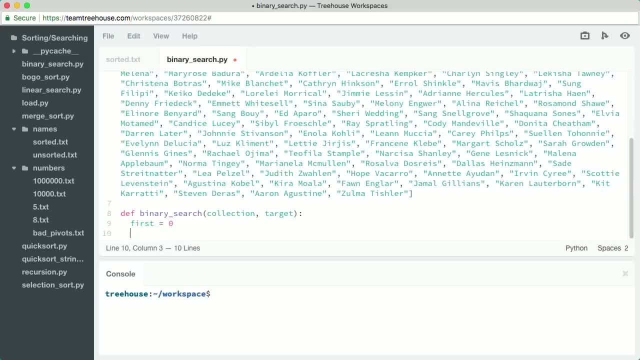 The first variable will track the lowest index in the range we're searching To start. it's going to be zero, the first index in the full list. Likewise, the last variable will track the highest index in the range we're searching To start. we'll set it to the highest index in the full list. 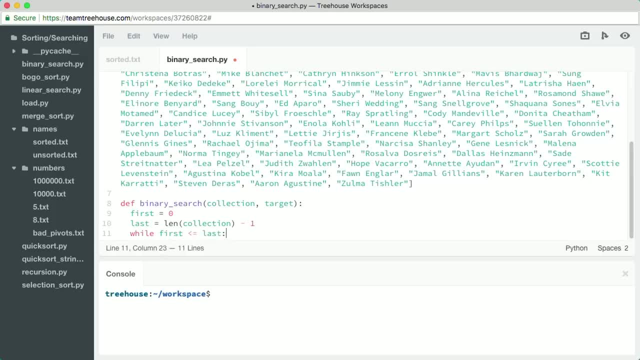 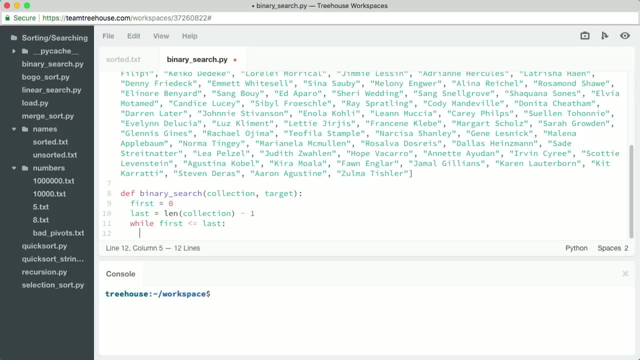 If the first and last variables are equal, then it means the size of the search range has shrunk to zero and there is no match. Until that happens, though, we'll keep looping to continue the search. We want to divide the list of potential matches. 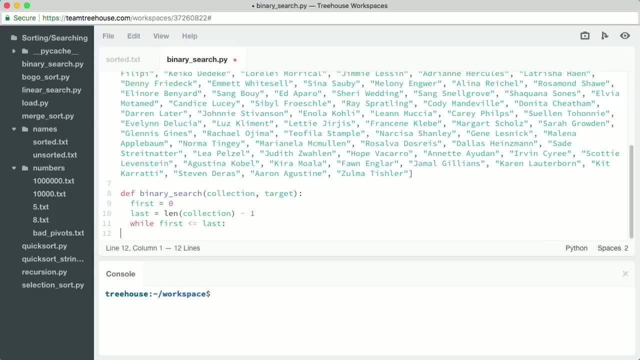 in half. each time To do that we need to check the value that's in the middle of the range we're searching in. We add the indexes in the first and last variables, then divide by two to get their average. We might get a fractional number. 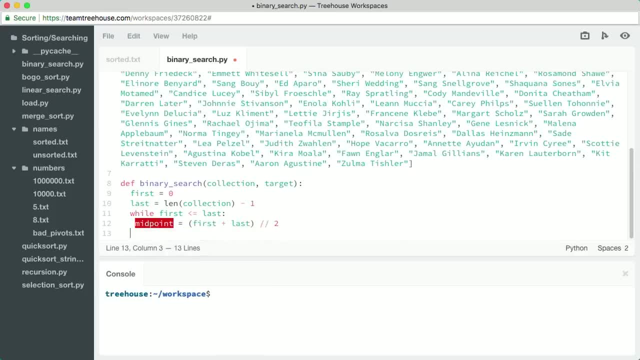 which can't be used as a list index. so we also round down using Python's double slash floor division operator. All this will give us the index of the list element. that's the midpoint of the range we're searching. We store that in the midpoint variable. 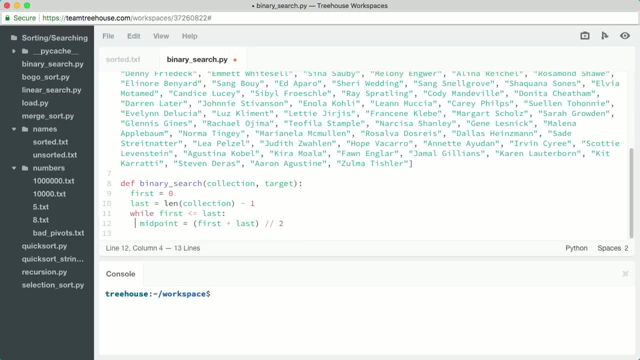 Whoops, looks like my indentation got mixed up there. Let me fix that real quick. There we go. Now we test whether the list element at the midpoint matches the target value. If it does, we return the midpoint index without looping any further. 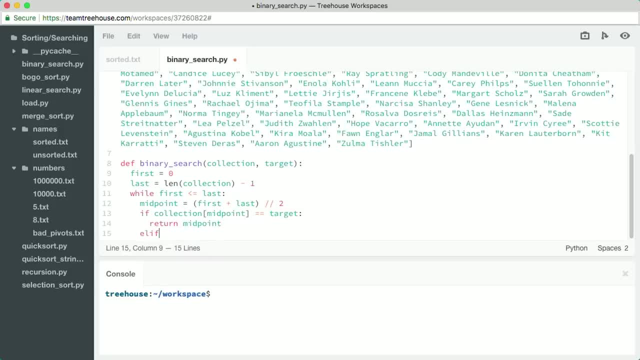 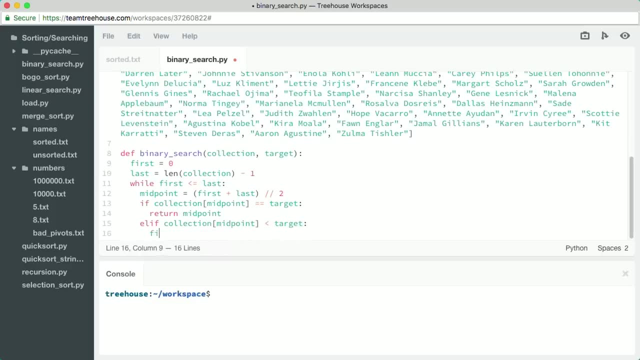 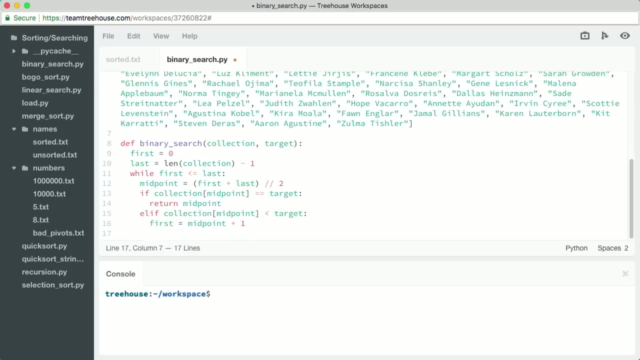 Our search is complete. Otherwise, if the midpoint element's value is less than the target value, then we know that our target value can't be at the midpoint or any index prior to that. so we move the new start of our search range to just after the old midpoint. 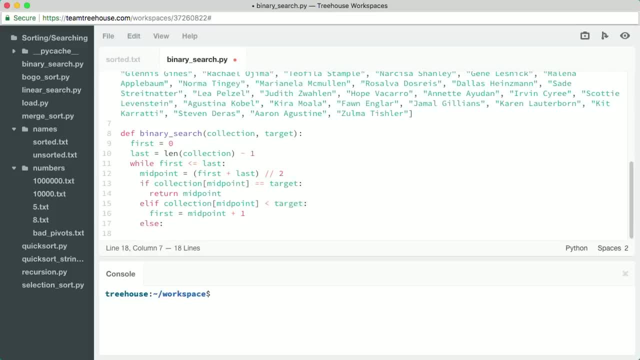 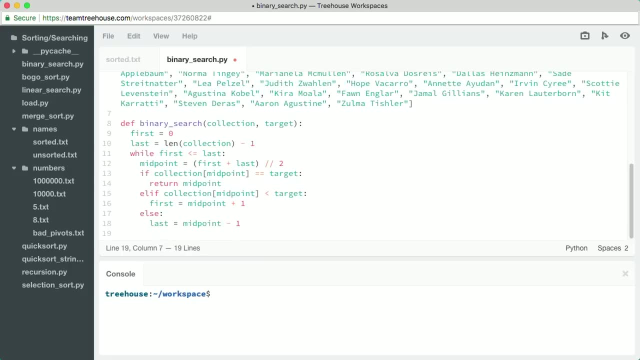 Otherwise the midpoint element's value must have been greater than the target value. We know that our target value can't be at the midpoint or any index after that, so we move the new end of our search range to just before the old midpoint. 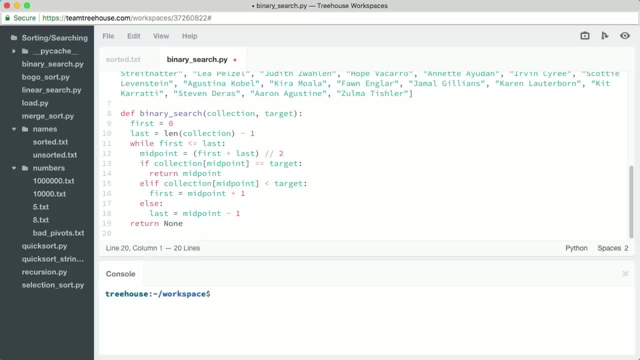 By unindenting here we mark the end of the loop. If the loop completes, it means the search range shrank to nothing without our finding a match, and that means there's no matching value in the list. So we return the special Python value none. 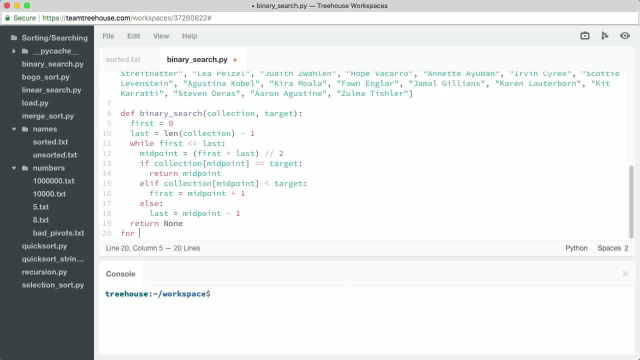 to indicate this. Lastly, just as we did in our linear search script, we need to search for each of the 100 names. We loop over each name in our hard-coded list and we call the binary search function with the sorted list of names. 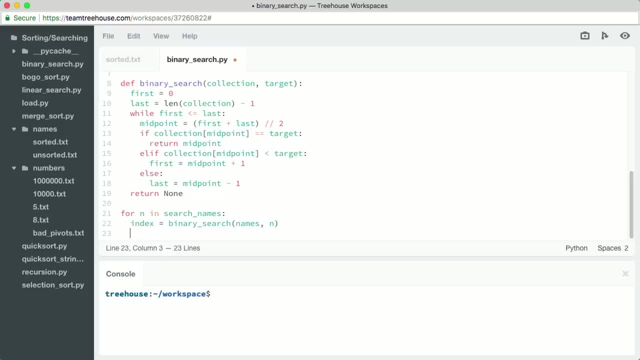 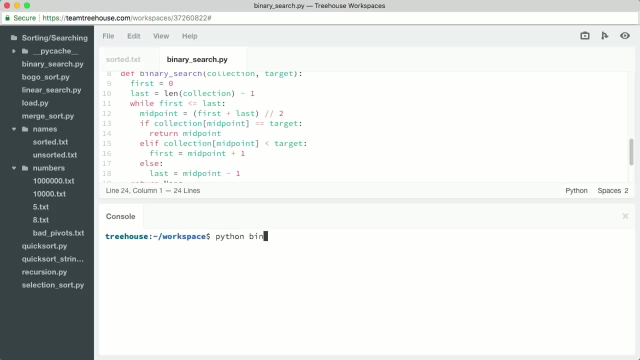 we're going to load from the file and the current name we're searching for. We store the returned list index in the index variable And finally we print that variable. Let's save this and go to our console and try running it. Python binarysearchpy. 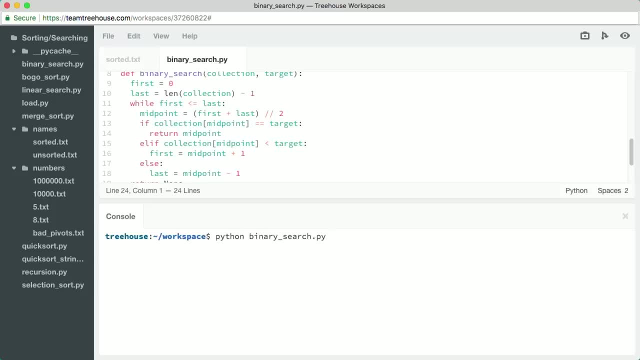 And it's important to give it the name of the sorted file. If it loads the unsorted file, the binary search won't work. So names, sortedtxt. Again it prints out the list of indexes for each name. I once again set it up. so the last two items: 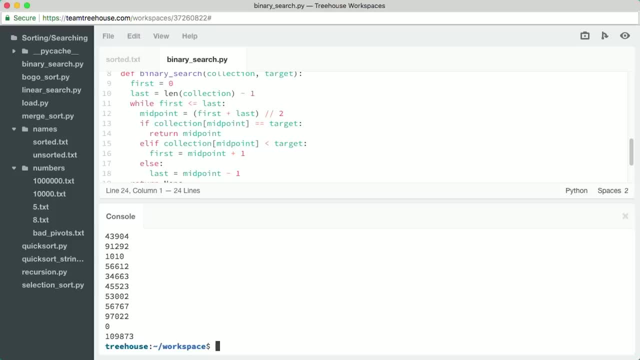 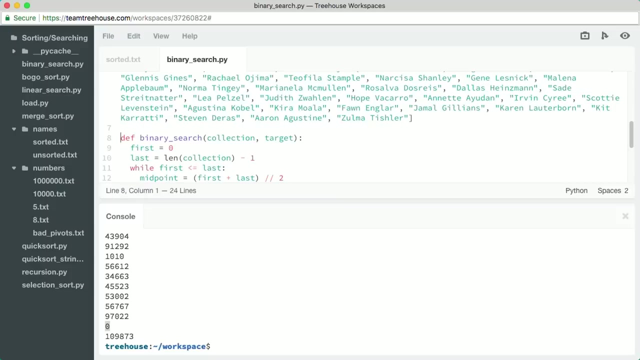 in the list of names we're gonna search for corresponded to the first and last name in the file. So it returned an index of zero for the second to last name And you can see that name. Here's the second to last name: Erin Augustine. 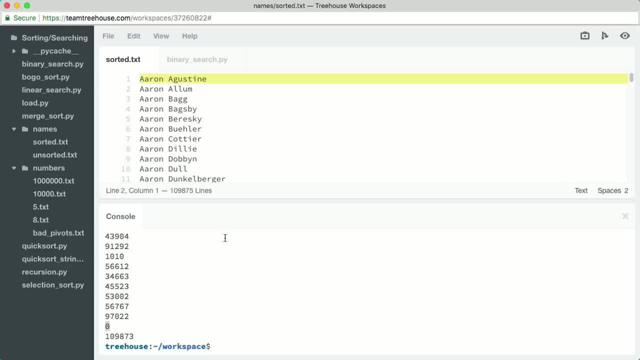 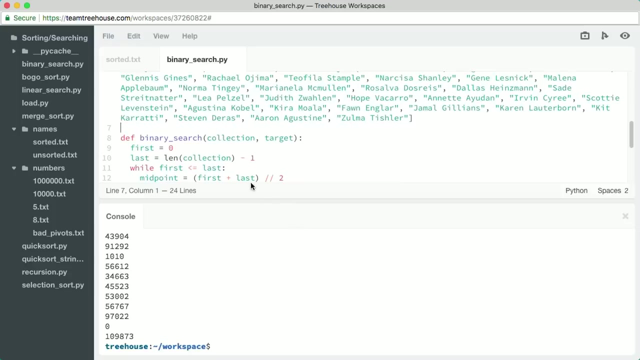 You can see that name here on line one of the file. And for the last name it returned an index of 109873.. And you can see that name here on line 109874.. Let's check the third to last name for good. 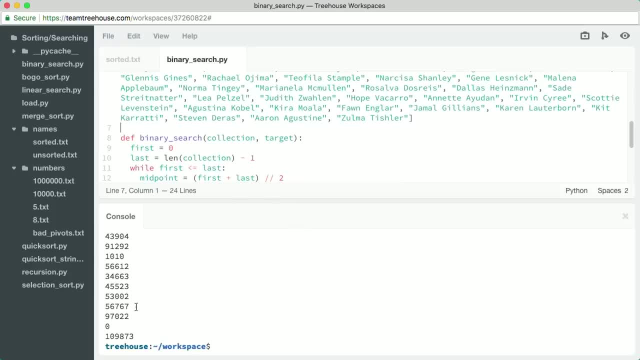 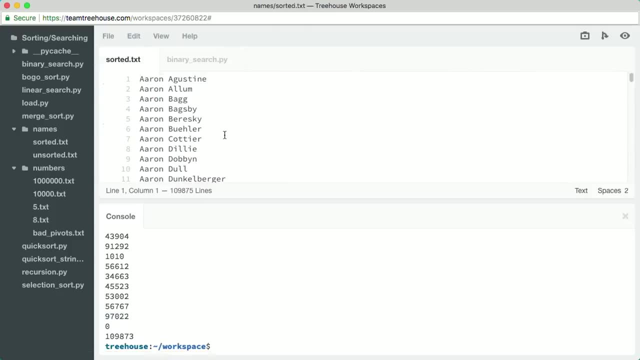 And for good measure, It looks like an index of 97022 was printed for that name: Steven Derus. Let's search for Steven Derus within the file, And here it is, on line 97023.. Remember that line numbers start on one instead of zero. 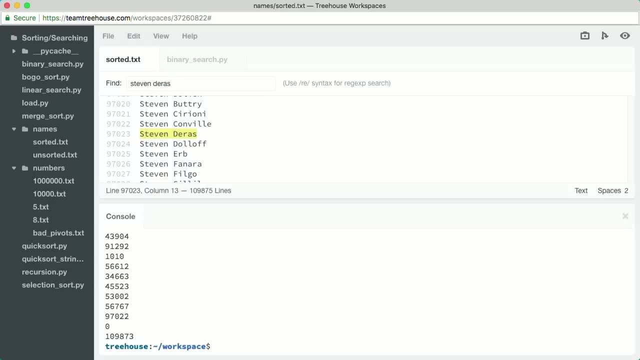 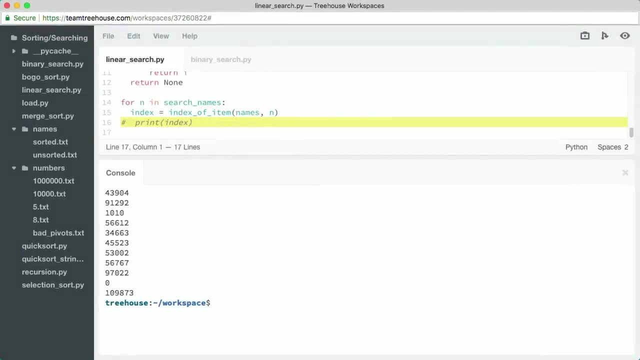 It looks like our binary search script is working correctly. Let's try our linear search and binary search scripts out with the time command and see how they compare. I've commented out the lines that print the indexes of matches in the two scripts. That way they'll still call their respective search functions. 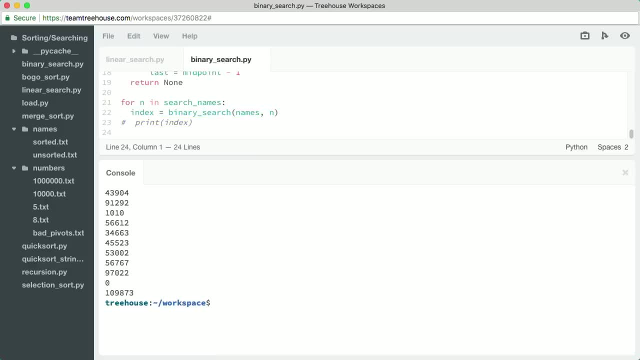 with the 100 names we're searching for, but they won't actually print the indexes out, So we won't have a bunch of output obscuring the results of the time command. First let's try the linear search script: Time Python. 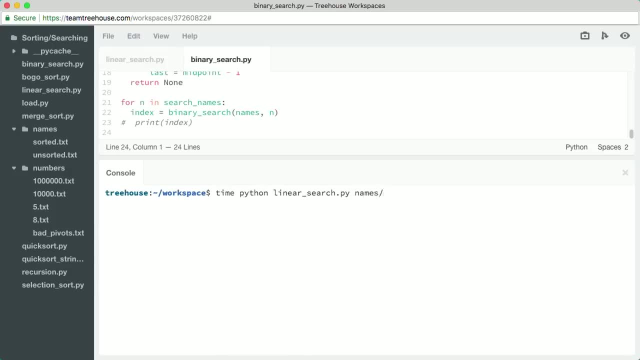 LinearSearchpy Names and we can just use the unsorted list of names for linear search. Remember we want to ignore the real result and add the user and sys results together. It looks like it took about 0.9 seconds for linear search to find the 100 names in a list of 100,000.. 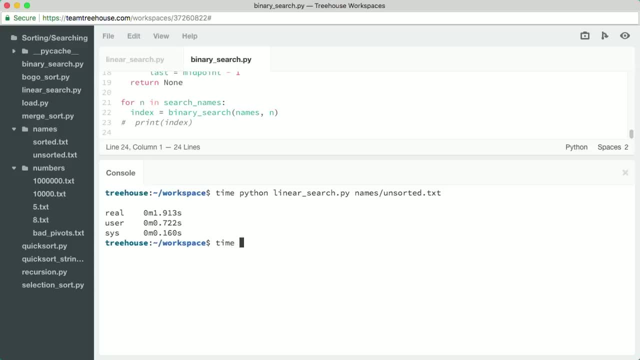 Now let's try timing the binary search script. Time Python BinarySearchpy Names, And for this one we need to use the sorted list of names. Looks like that took around a quarter second, so less than half as long.